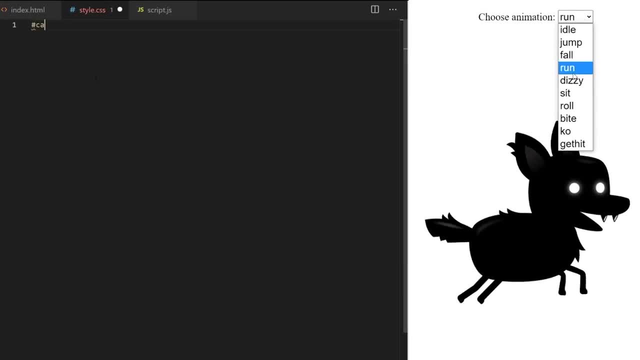 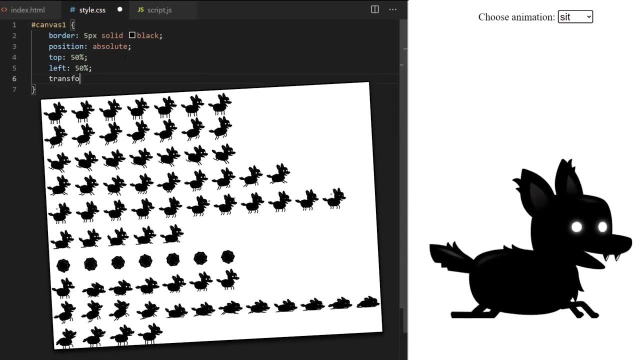 games In the first class. we will explore two different JavaScript techniques you can use to animate sprite sheets and we will build this project where you can choose different player animations from the dropdown. We are giving away a lot of free art assets. You can download them. 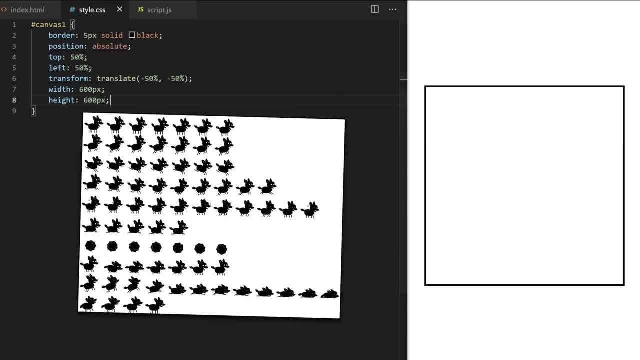 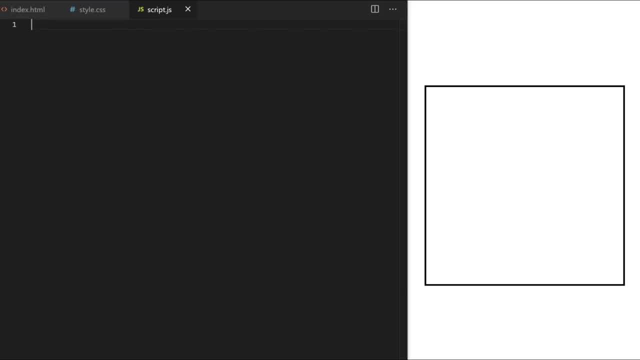 in the video description And you can use them to follow along with this course. For more beautiful game art assets, visit this website Now. let's do a quick JavaScript setup. I will show you how little code you need to animate something on canvas. I create a custom variable called canvas that will hold a reference to. 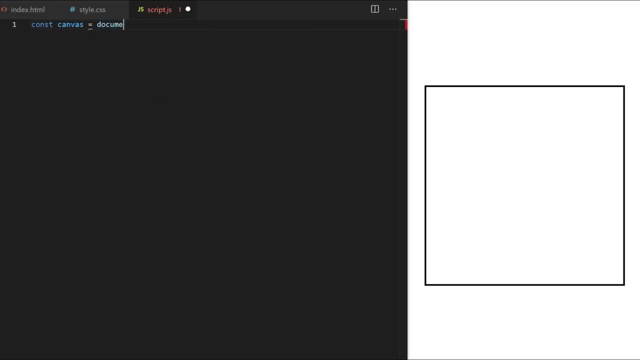 my actual HTML canvas element I created in indexhtml. I point JavaScript towards it using getElementById and I pass it id. I gave it canvas 1. Constant variable. I call for example CTX. shortcut for context is equal to this canvas variable from line 1.. Don't worry, I will show you how to do this in the next class. 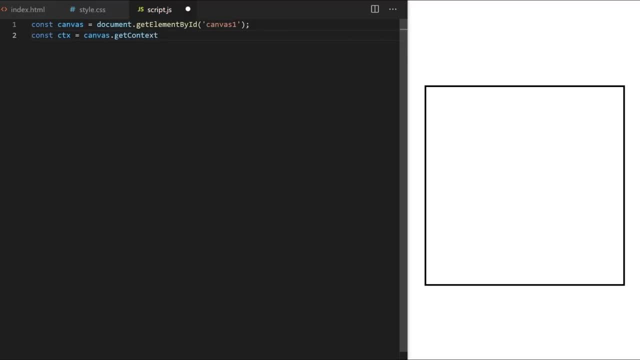 I will show you how to do this in the next class. Don't worry, I will show you how to do this in the next class. getContext and I pass it 2D. I could also pass it WebGL here, which would give us access. 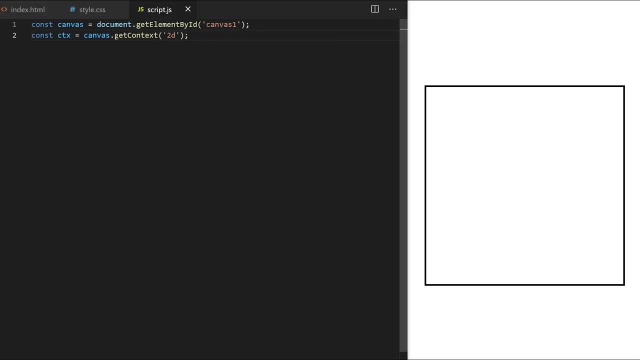 to a completely different set of drawing methods, but that's for another video. Now I have all canvas 2D drawing methods stored in my custom CTX variable and I can call them from here. For example, CTXFillRect will call a method to draw a rectangle on canvas. 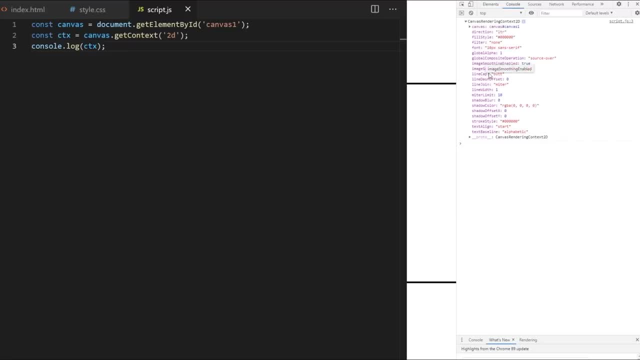 If I consolelog CTX, we can inspect this object. It has some properties which basically are global canvas settings, such as FillStyle, that says cut. I can also call it fillRect, which will call a method to draw a rectangle on canvas If 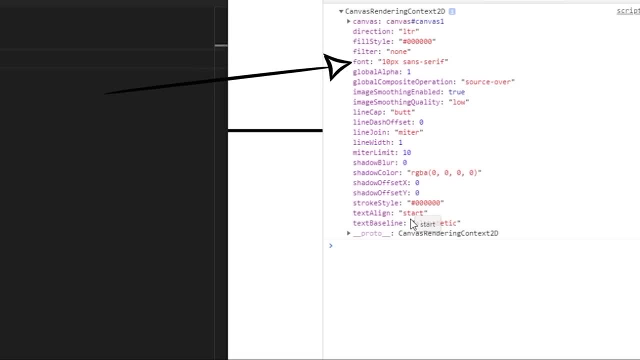 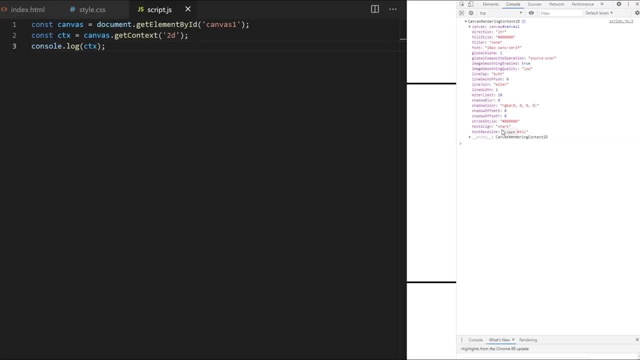 I consolelog CTX. we can also call it fillRect, For example. I can also call it fillRect, For example. I can also call it fillRect. This tutorial will be focused on sprite animation. We want to learn how to create animated characters. 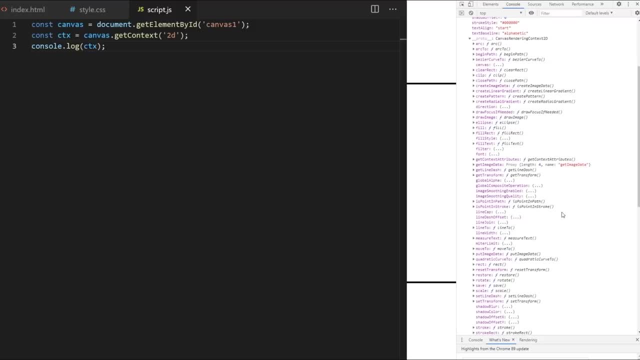 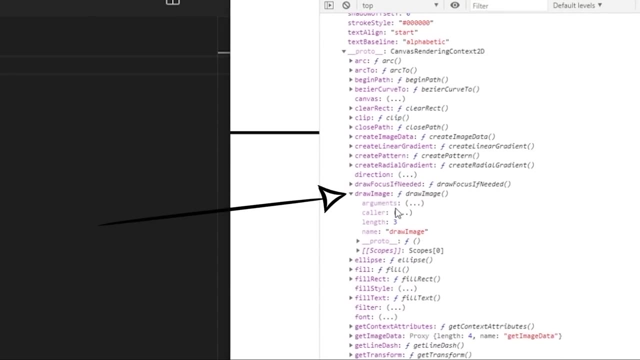 for games. So we are most interested in build-in canvas drawImage method, which sits right here. I will explain everything you need to know about drawImage method and its three versions in a minute. It's easy, don't worry about it. 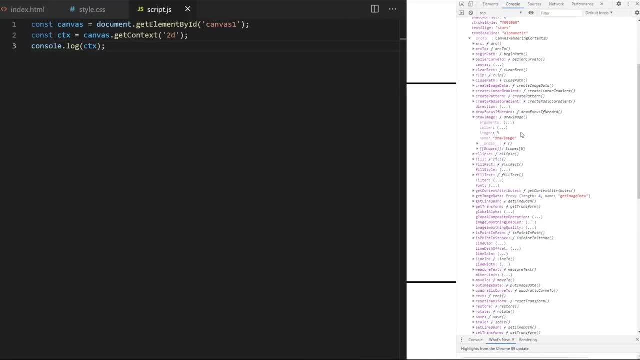 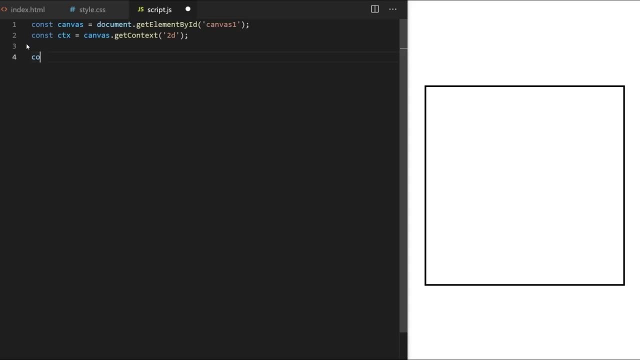 Before we do that, I will quickly finish canvas settings. Control over the bottom left-hand side of canvas and use the Profile button to select the richest display up. To make sure we have correct scaling, I need to set canvas width and canvas height. By default, canvas will be set to 300 times 150 pixels and our drawings 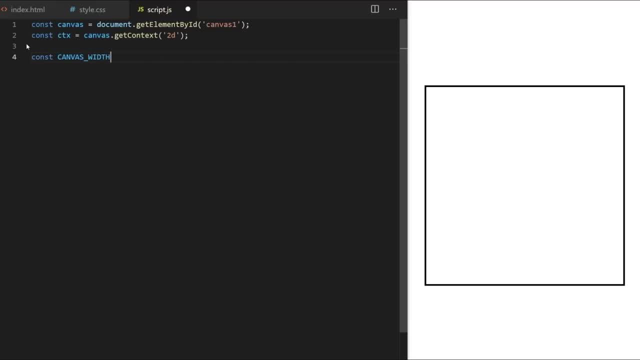 can come out distorted. That's why I will manually set it to 600 times 600, the same values I gave it in style CSS. I create a custom variable called canvas width. I will use capital letters here to make it clear this is a global variable. 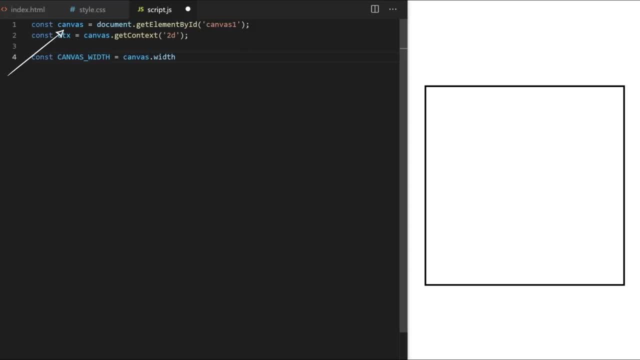 I set it equal to canvas from line 1 dot width and I set it all to 600.. Same width, I gave it in style CSS. I do the same for canvas height, also 600.. Now that we made sure scaling is correct, let's bring an image into the project In. 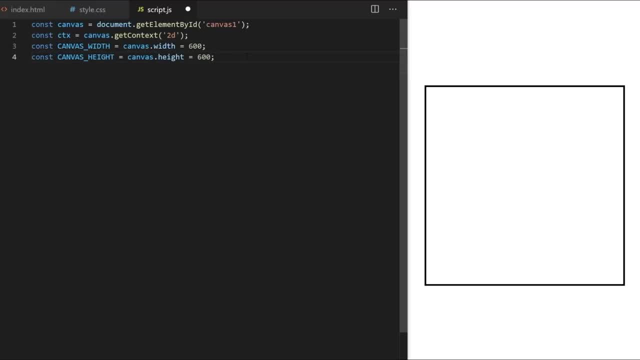 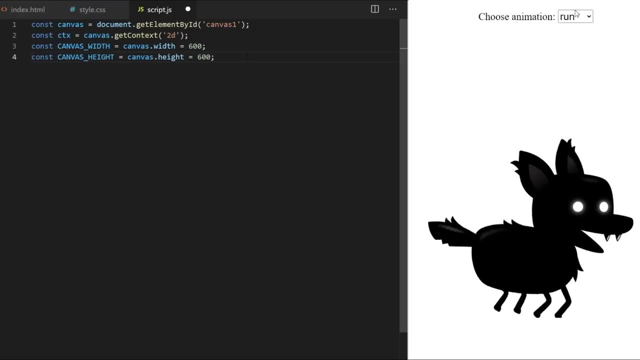 this tutorial I want to show you two different ways you can animate sprites: Very simple one for beginners, and then more advanced, more complex and flexible way where you can just run commands like run, jump, sit, and it will play the correct animation for us. When you know both, you can decide which one. 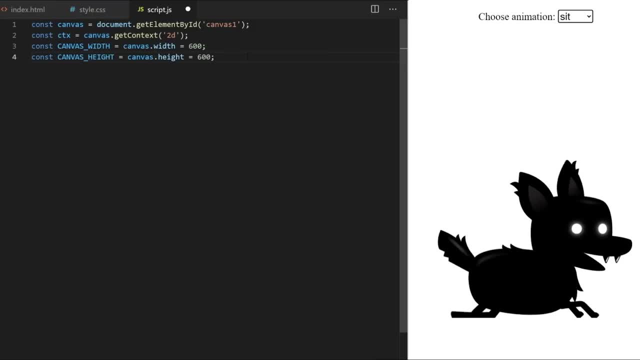 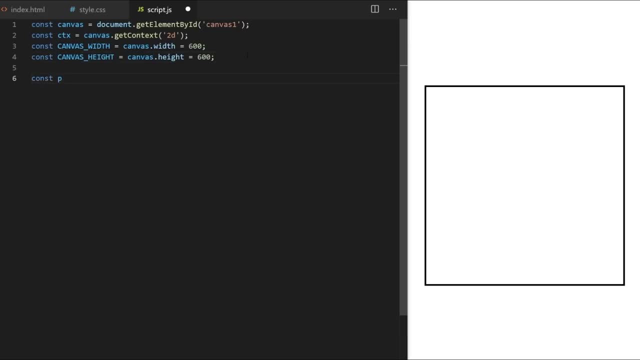 to use when you are building your games. I want everyone to get the same result. That's why I will be giving away this animated sprite sheet for free today. To bring image into JavaScript project, I can just declare a custom variable. I call, for example, player image and I set it equal to new image. like this: This is: 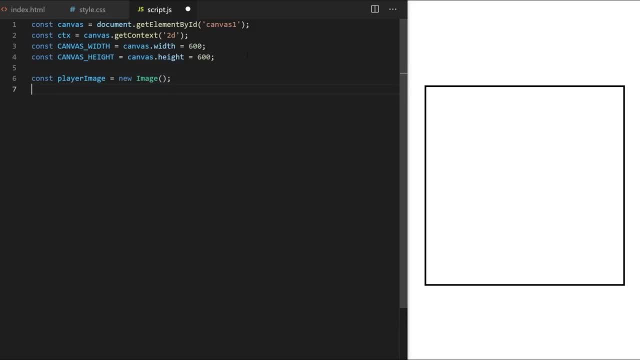 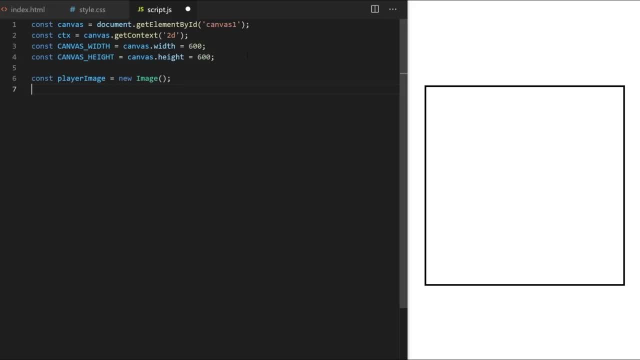 in index HTML markup. We can append it to our web page if you want, but today we will just use it to store that sprite sheet image for us so that we can animate it with a JavaScript. I need to give it source, so player image variable. 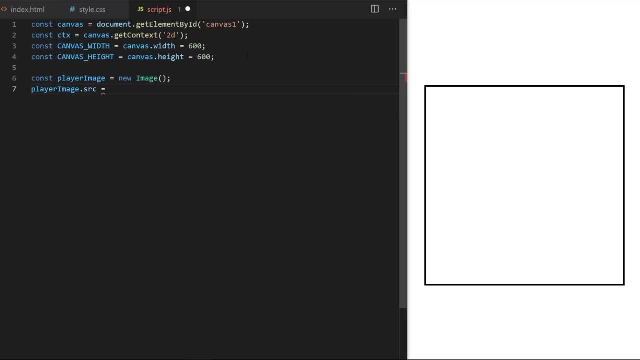 from line 6, dot SRC, and I set it to path to my sprite sheet. Your path might be different. it depends on how you organized your project files. Let's animate something on canvas. I create a custom function called, for example, draw frame. Actually, let's call. 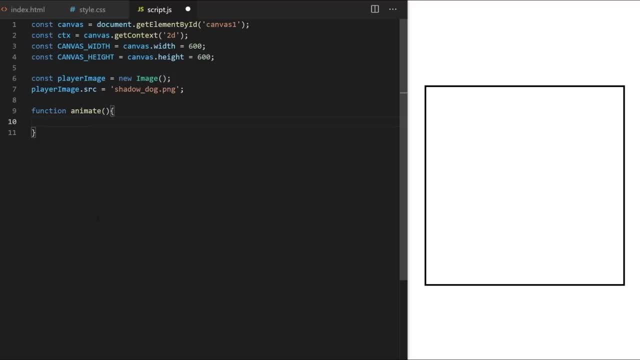 it animate, because this is our animation loop. Let's make sure that's clear Inside animation loop. first I want to clear old paint from canvas between every animation frame. so I take CTX variable from line 2, dot clear rectangle built-in method. It expects four arguments to specify. 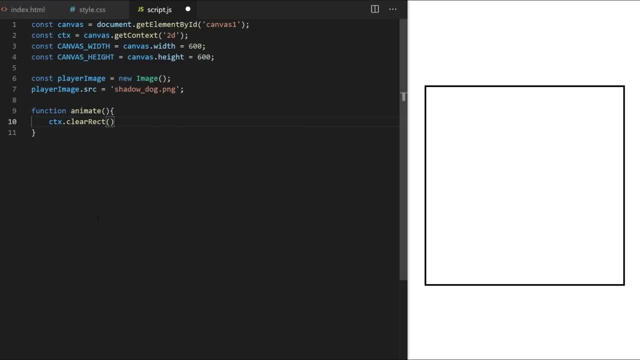 what area on canvas we want to clear. I want to clear the entire canvas. so from coordinates 0,0 to canvas width, canvas height. Now we can draw. I will just test if everything works by drawing a simple rectangle at position 50- 50 and I give it with an height of 100. 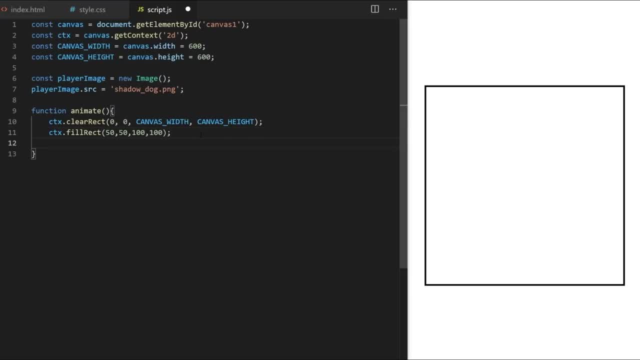 pixels. Now I can call a requestAnimationFrame built-in method which will simply run a function we pass to it. It will call that function once. If I pass it animate the name of its parent function from line 9, it will just run over and over. 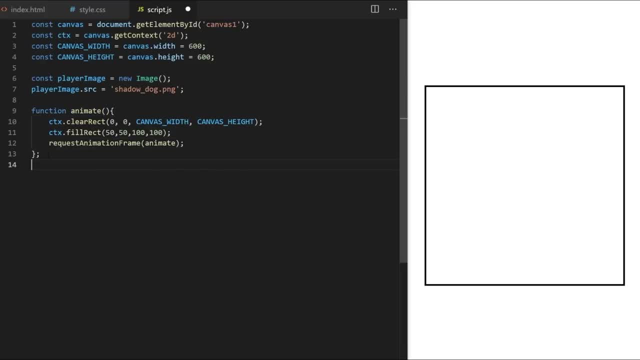 create an animation loop, so we declared animate. I also have to call it like this. and we have a black rectangle drawn on canvas. if we don't specify fill style color of shapes on canvas, always default to black. it looks like a static image, but it's actually animating the same rectangle over and over. I can simply: 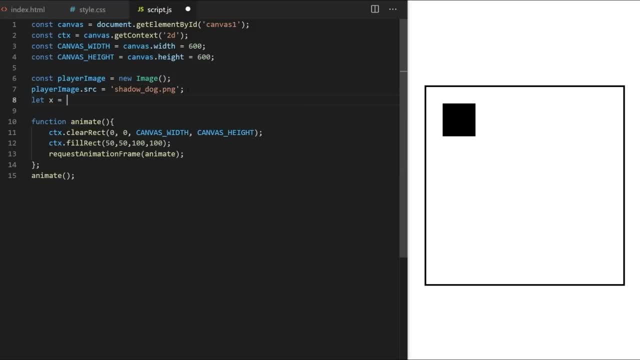 prove it by creating a global variable called X. I set it to zero and here, on line 12, I replace hard-coded value with this variable, and every time animation loop runs, I increase X by one. I told you you don't need much code to animate something on canvas. well done, you are a programmer now. see you later, okay. 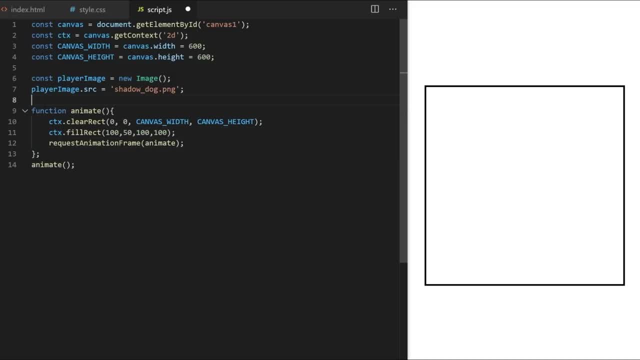 there's a bit more I can show you. let's put it back and let's use built-in draw image method to draw our sprite sheet on canvas. draw image method is a bit special. you can pass it three or five or nine arguments, depending on how much. 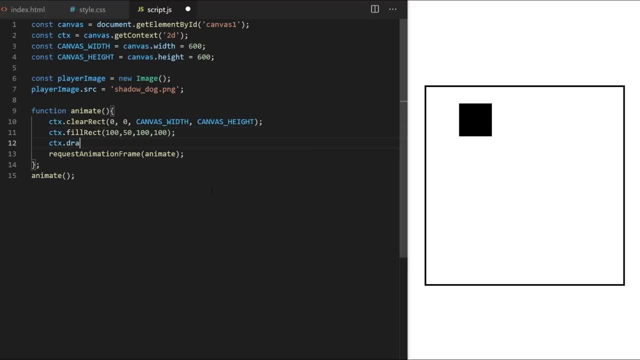 control do you want to have over the image you are drawing? the first argument is always the image you are drawing, you want to draw. so I pass it. player image variable from line 6. then I pass it X and Y coordinates where on canvas I want my image to be drawn. if I pass it. 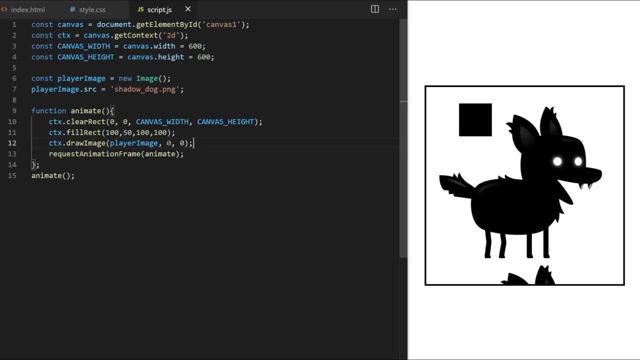 0 for X and 0 for Y. it will be drawn from the top left corner of canvas. coordinates 0- 0. it will also keep the image at the original width and height. the sprite sheet I'm using has 10 rows and 11 columns of animation frames. it's 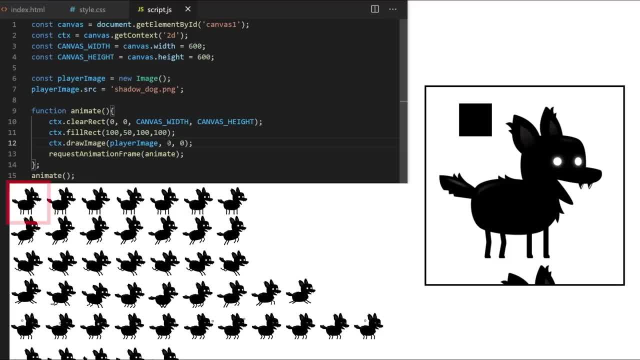 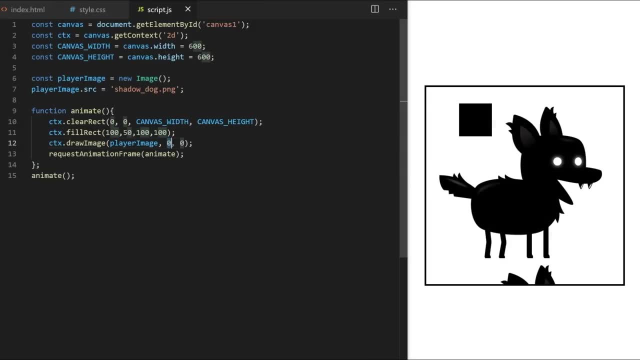 many times larger than my canvas. so now we can only see this small part, 600 times 600 pixels, in the top left corner of my sprite sheet. it's 600 times 600 because that's the size I set my canvas to. so this is the version of draw image with only three arguments. it works and you. 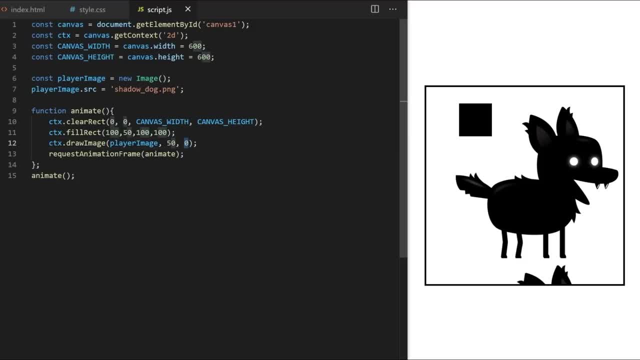 can change X and Y coordinates to move your image around, but you would need to resize your images using some other programs such as Microsoft Paint or Photoshop. but you don't have to do that because a draw image also accepts five arguments. that's its second version. 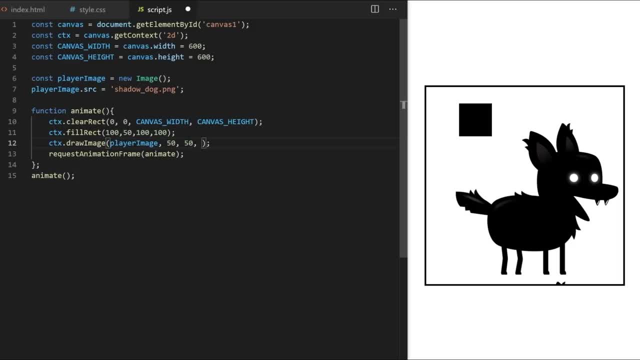 If you pass it 5 arguments, the 4th argument will be width and 5th argument will be height. so we are now able to scale the image up and down and we can also stretch it vertically or horizontally. If I pass it canvas width and canvas height, it will stretch the image to match my canvas. 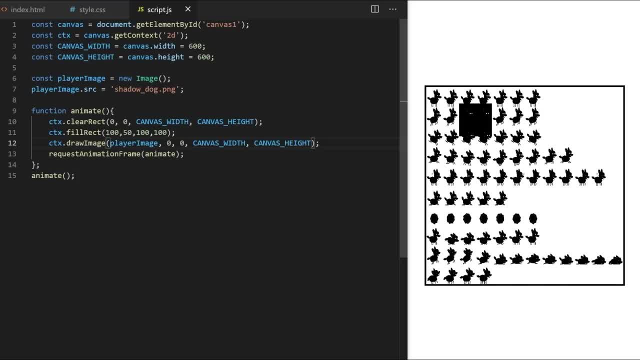 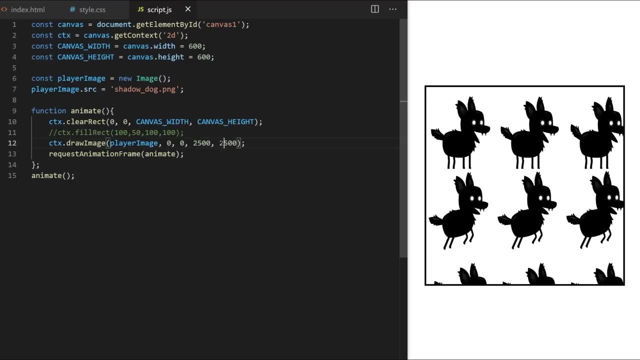 area 600x600 pixels And since the image is not the same ratio as my canvas, you can see the image is stretched just a little bit. Let's remove the black rectangle by commenting out line 11.. I can pass any values as width and height, and JavaScript will just stretch my image. 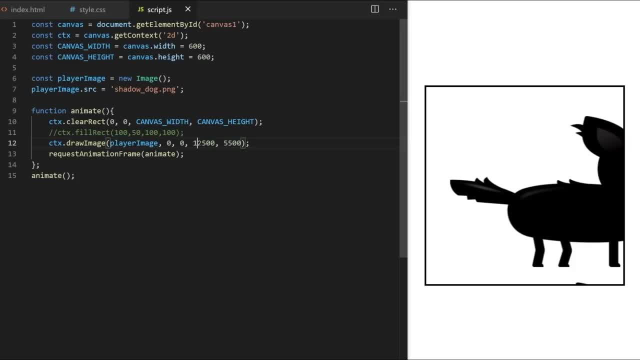 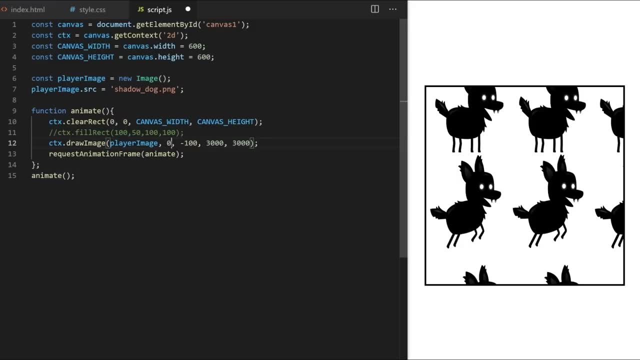 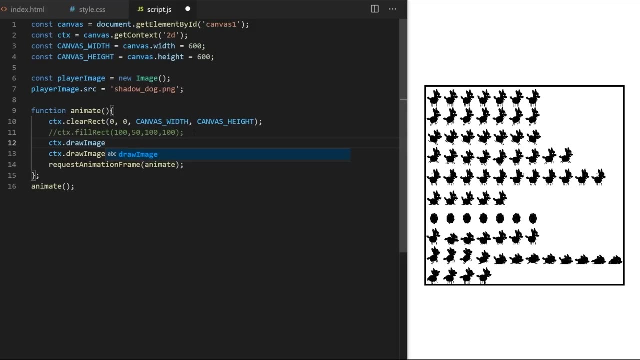 based on these values. You can also change x and y to move the entire image around. The final third version of drawImage method accepts 9 arguments. This gives us the most control over the image. The first argument again is the image you want to draw. 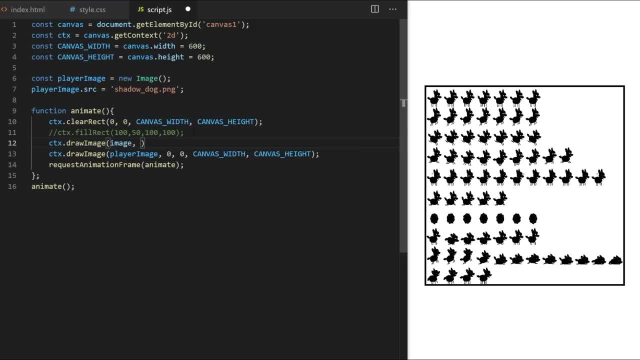 The next 4 arguments determine rectangle area we want to cut out from the source image: Source x, Source y, Source width and source height. And the last 4 arguments will tell JavaScript where on our destination canvas we want to draw just that cropped out part onto. 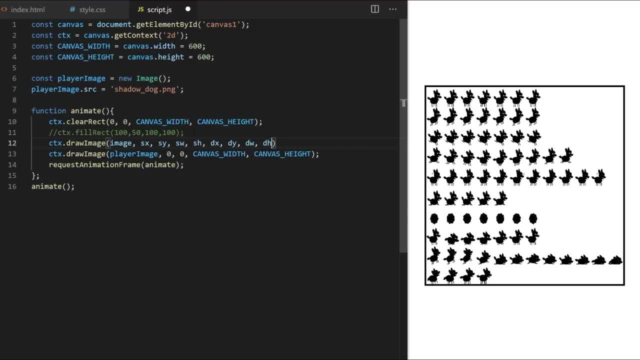 Destination x, Destination y, Destination width and destination height. These last 4 values basically work the same as these 4 values in the previous drawImage call I showed you. The only difference is they are not used to position and stretch the entire image, but just the area we cut out using these arguments. 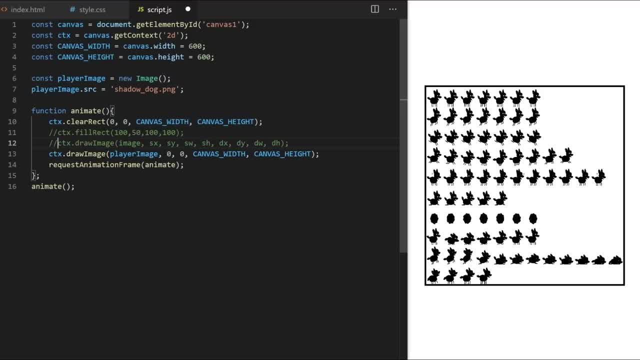 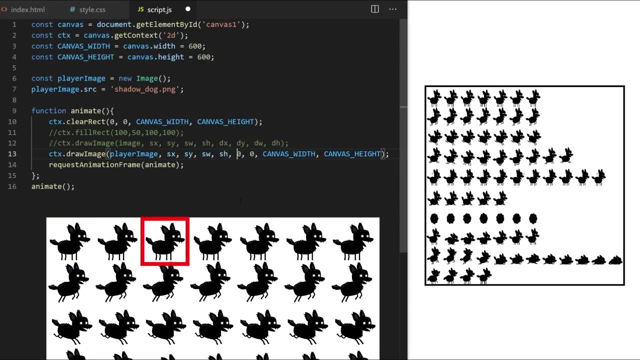 I comment out line 12, but I will leave it here for reference. And on line 13, I will add source x, source y, source width and source height arguments and I will use them to cut out only one dog at a time, One frame from my large sprite sheet. 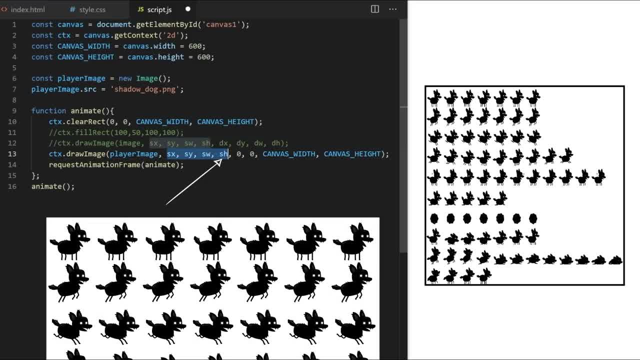 So these 4 values determine area we cut out from the original sprite sheet And I will use them to cut out only one dog at a time. And these 4 values determine where on canvas we want to place that cut out piece of image onto. 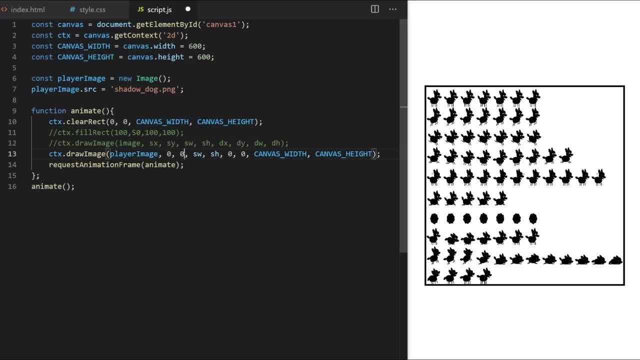 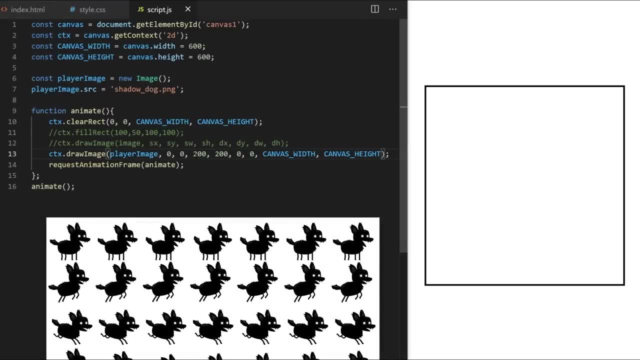 If I set source x to 0.. Source y to 0.. Source width to 200.. Source height to 200.. We are cutting out square 200 times 200 pixels from the top left corner. There is nothing in the area. 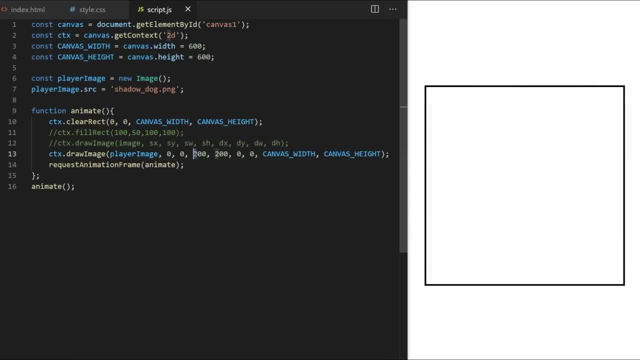 And I will use them to cut out only one dog at a time. Source width to 200.. Source height to 200.. Source width to 200.. And if I change it to square, 400 times 400 pixels, we can see part of our dog. 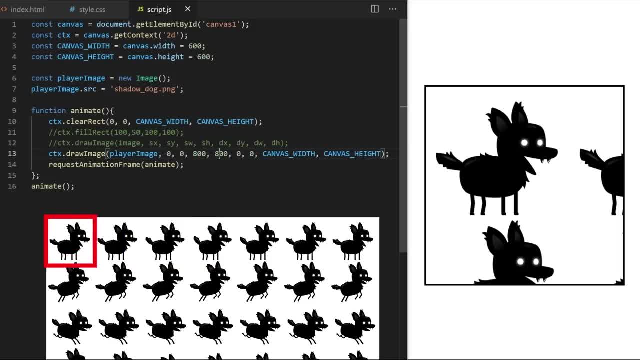 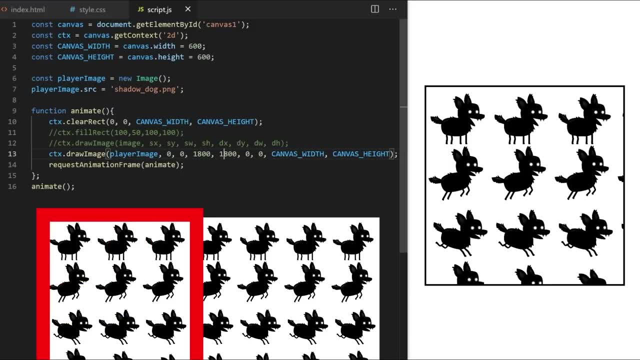 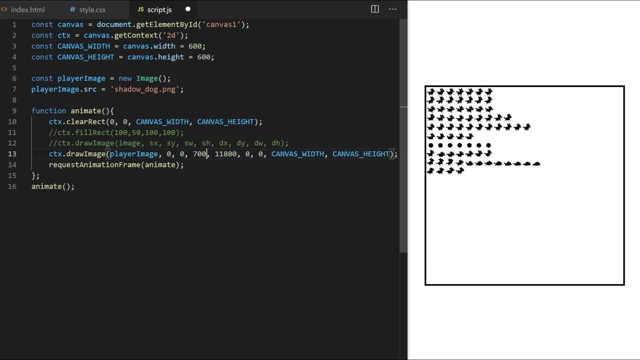 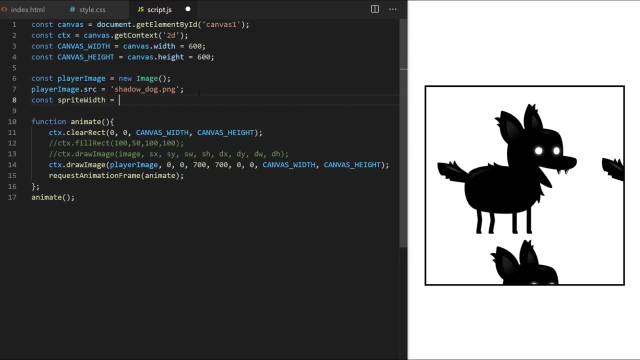 I can add any values here and cut out any chunk of the original sprite sheet I want. I can also scale it, Stretch it. I can do whatever I want. here I will create a global variable called sprite width. let's have a look at our sprite sheet. if i take width of the entire file and divide it by number, 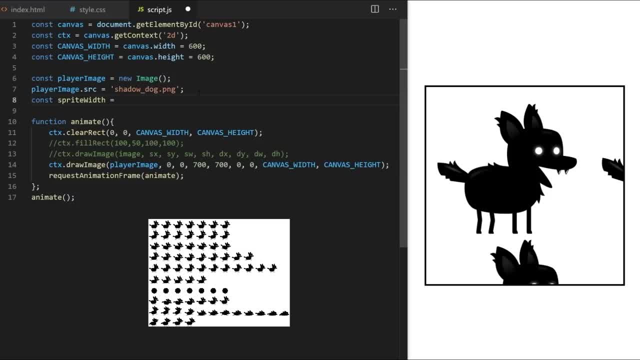 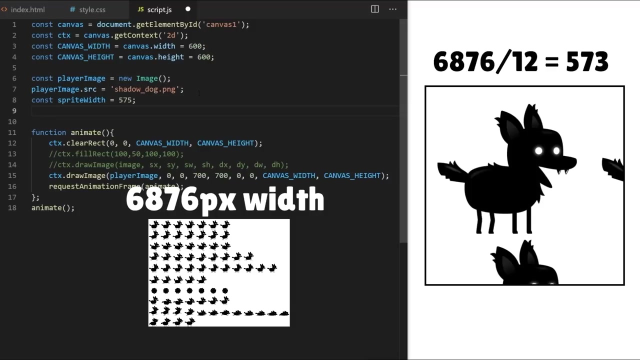 of columns i get width of one frame. my sprite sheet is 6876 pixels wide and it has 12 columns. 6876 divided by 12 is 573. i will use 575 for now because i made the last frame a bit smaller when assembling my sprite sheet in photoshop and there's some margin that's snuck in sometimes. 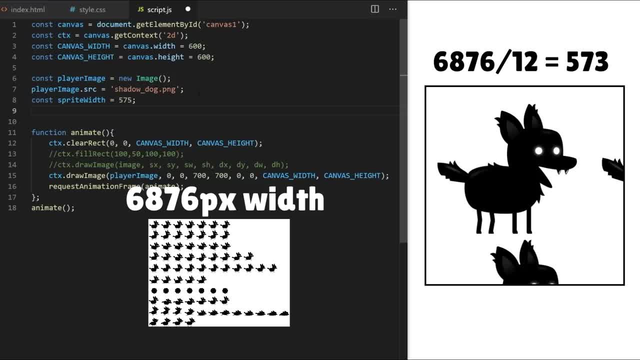 when you see that your animation is moving sideways when it shouldn't, try to fix it by adjusting width and height by small pixel amounts and watch what happens. i will show you a bit later what i mean. it's simple. you can just ignore it for now. sprite height or height of a single frame. 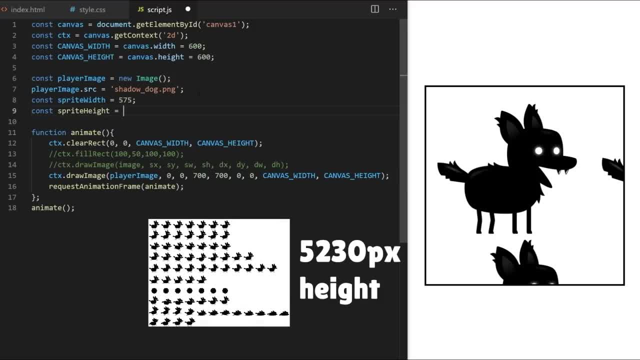 will be height of my entire sprite sheet, which is 5230 divided by the number of rows. we have 10 animations, 10 rows, so 5200, and 30 divided by 10 is 523. on line 15 i can replace source width and source height with sprite width. 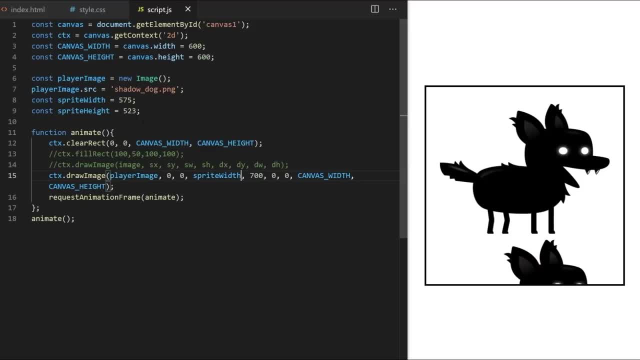 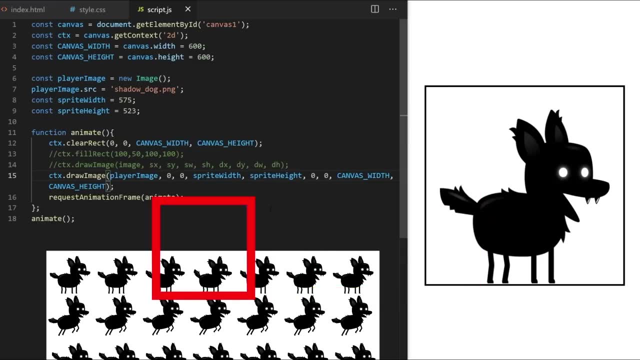 and sprite height variables i just calculated and now we are cropping out exactly one frame from our sprite sheet and in destination width and destination height, instead of stretching it to cover the entire canvas. i can also use sprite width and sprite height variables here and we are drawing the frame at its original size. if you are still not clear what each of these, 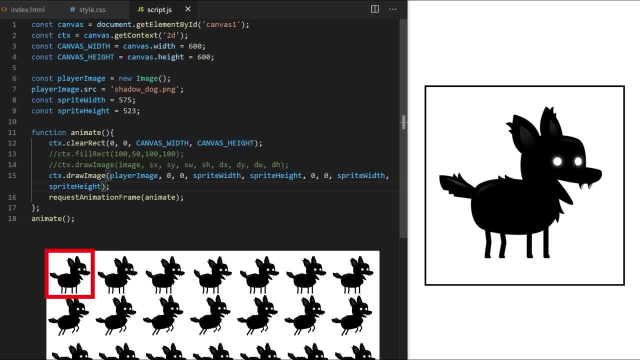 individual arguments passed. to draw image method. does feel free to play with it, change the values and see what happens. it's quite straightforward once you get used to it. here i'm giving it an image. i want to draw these four values. specify a rectangle area to crop out from the original. 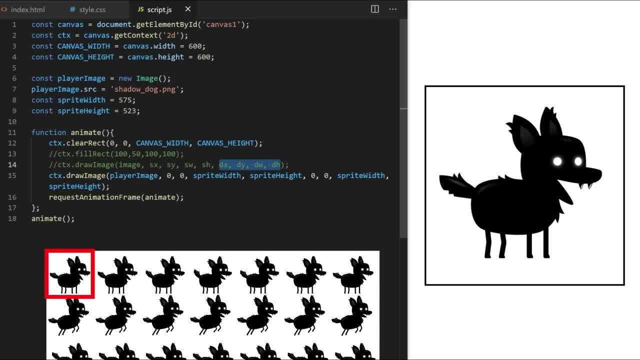 large sprite sheet. and here i am telling it where i want that cropped out piece of my sprite sheet to be displayed on canvas. if i set source x coordinate to one times sprite width, i am jumping one frame. as this number increases i am moving to the right, jumping by the amount of sprite width. 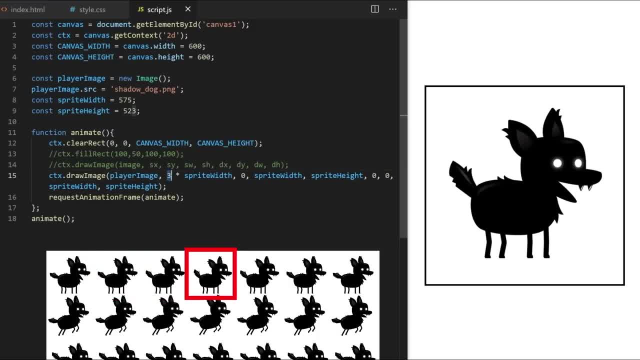 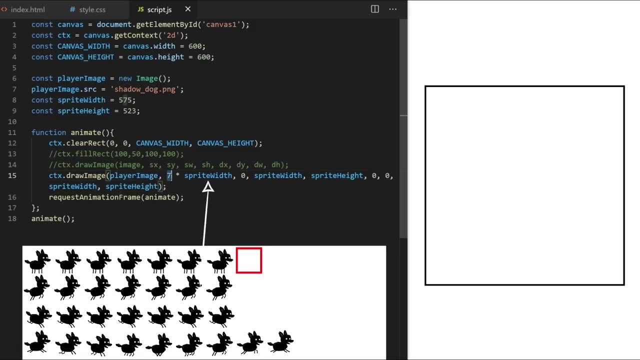 this way i can display my animation row frame by frame. when this number gets too high, there will be no frame there eventually. so source x argument allows us to cycle through sprite sheet horizontally. if i want to swap between different animations, the way our sprite sheet is structured, i have to travel through it. 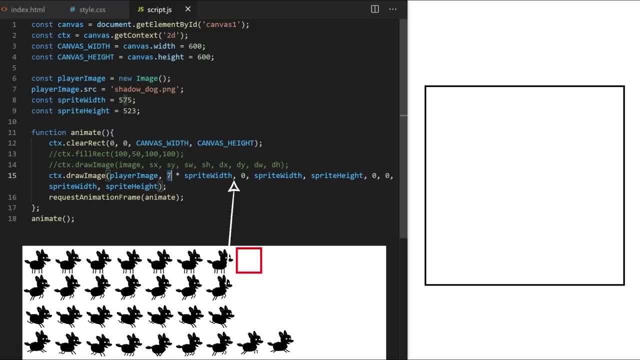 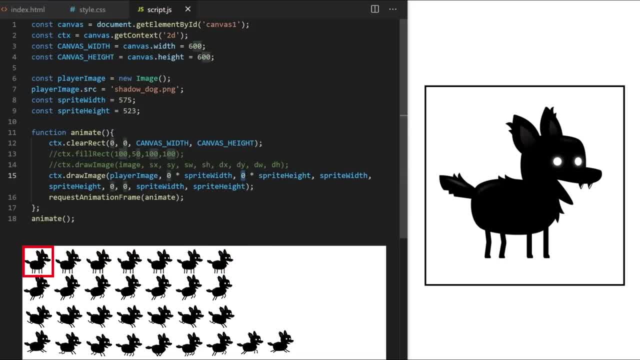 row. in this case we have idle animation there. one times sprite height is row two jump animation. then there is fall animation running and so on. traveling through this sprite sheet vertically along the y-axis switches between different animations and we do it by changing source y argument. traveling horizontally cycles between individual frames of these. 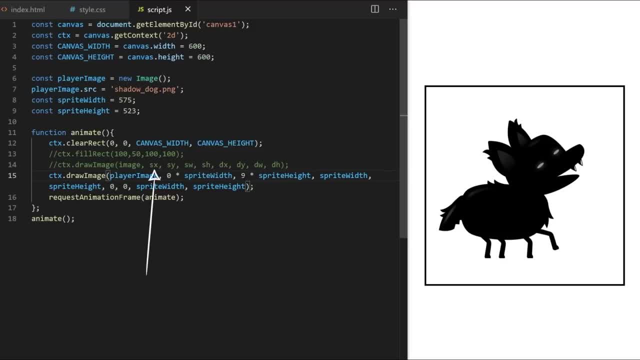 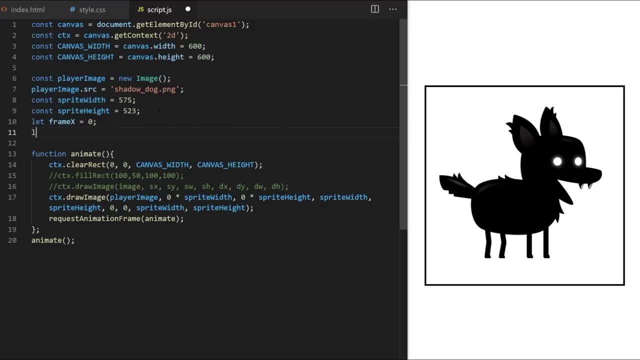 animations and can be done by changing value. we pass as source x argument. we pass as source x argument instead of manually changing numbers like this. let's output it to variables. i create variables called frame x and frame y and i set them to zero initially. then i just replace. 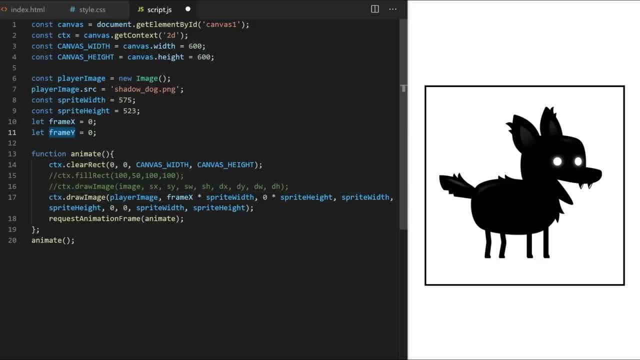 hard-coded zeros inside my draw image method with frame x and frame y, and now i can swap between animation frames by assigning different values to these variables. frame x cycles through frames of each animation. frame x cycles through frames of each animation. frame x cycles through frames of each animation. 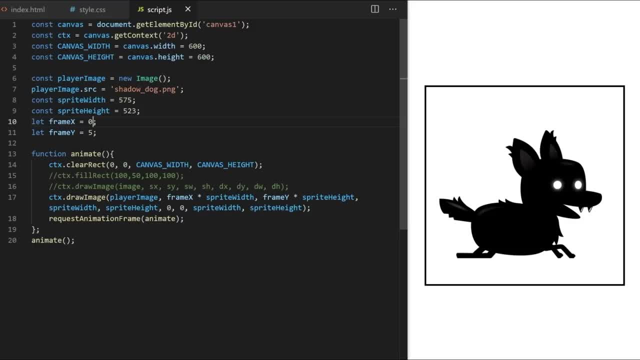 horizontally. frame y swaps between different animations. it travels through my sprite sheet vertically. now let's cover a very simple way you can animate your sprites and then i will show you proper, advanced, scalable technique that is suitable for both small and larger game projects. the simple way is this: we know that frame x- variable- cycles through our sprite sheet. 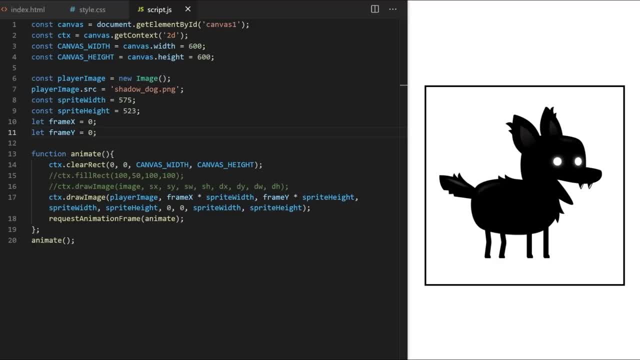 horizontally first row in our sprite sheet. is idle animation. it has 7 frames inside animation loop on line 18. i can make this frame height shortly corresponding to the actualvable frame. x variables is idle animation. it has seven frames inside animation loop on line 18. i can 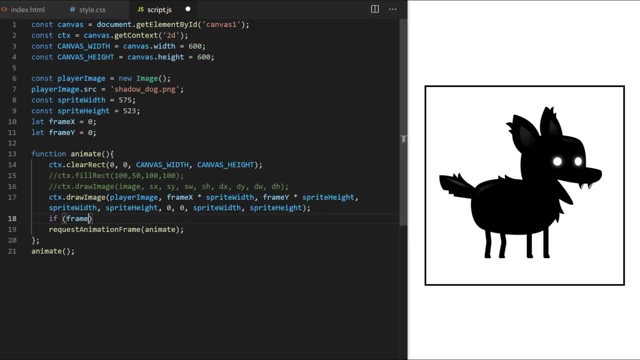 say, if frameX from line 10 is less than 7, increase frameX by 1.. FrameX++, Else meaning, when it's equal or larger than 7, reset it back to 0.. You can notice two things: Our animation is blinking and it's going very fast. 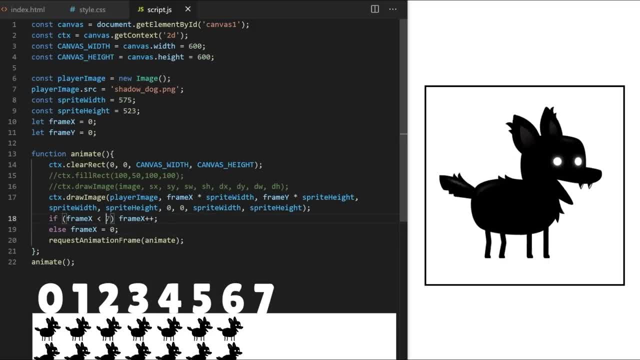 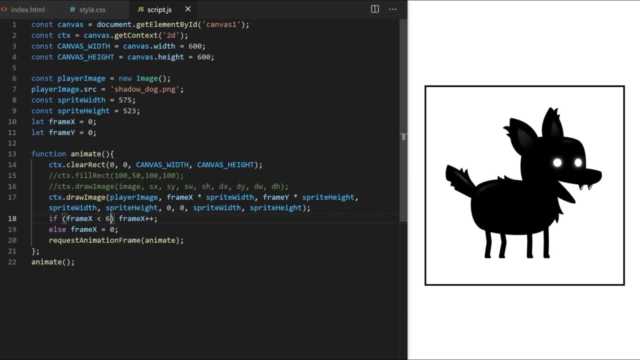 Let's deal with it. First frame is 0, so last frame is actually position 6.. If I change this to 6, the empty frame is removed and blinking is gone. On line 11, I can just change values of frameY and we are animating different rows in the 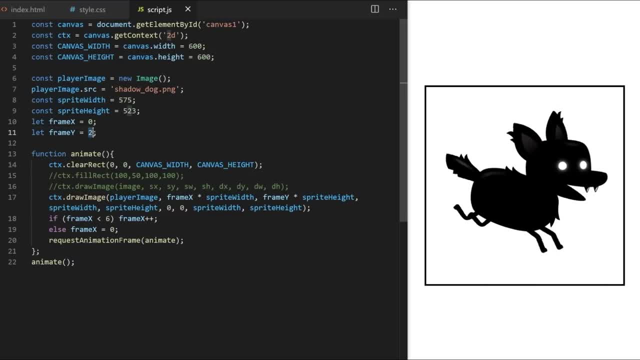 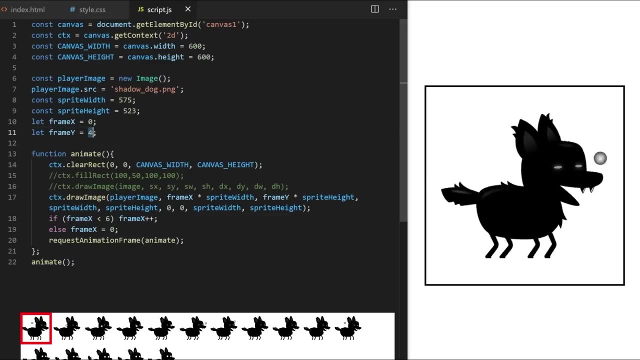 sprite sheet Problem comes when I get to frameY 4.. Which is row 5.. We are starting from 0.. This animation has 11 frames, but I am cycling only until frame 6. So we are not playing the entire animation. 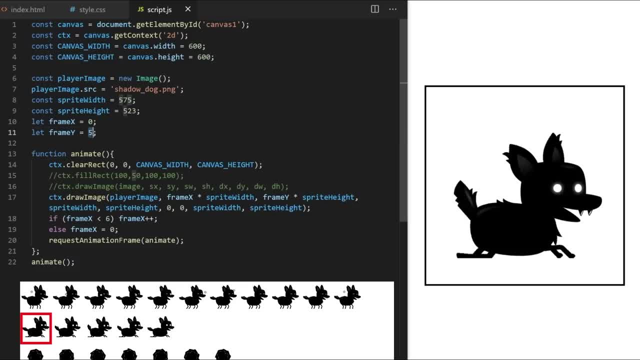 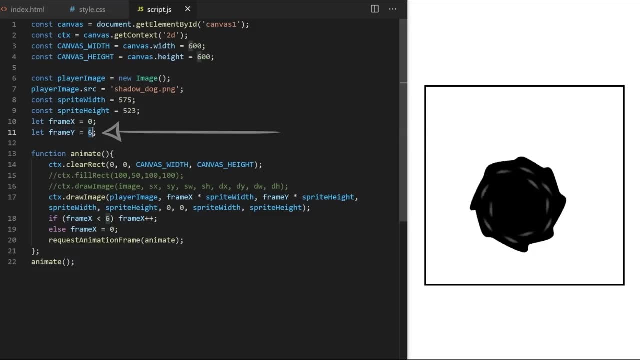 When I get to this row, we have a problem again. Sitting animation has 5 frames and we are cycling through more frames here, So now it's blinking because we are including some empty frames. To get this to work properly, Every time we want to swap between animations, we have to change frameY value on line 11,. 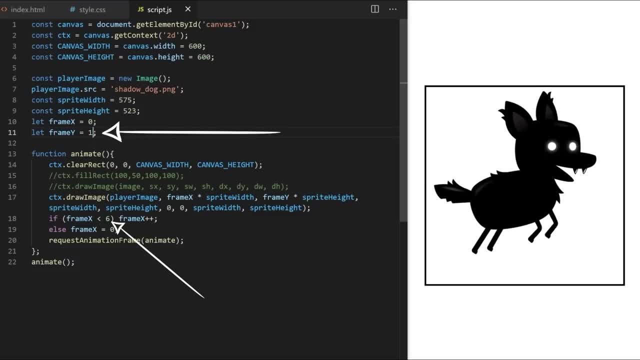 but also this hardcoded number 6 on line 18.. Ideally, it would have to be a variable that always changes to the correct value that reflects the number of frames for each animation row, depending which one we are animating right now. I would solve it by having variable called, for example, maxFrame. 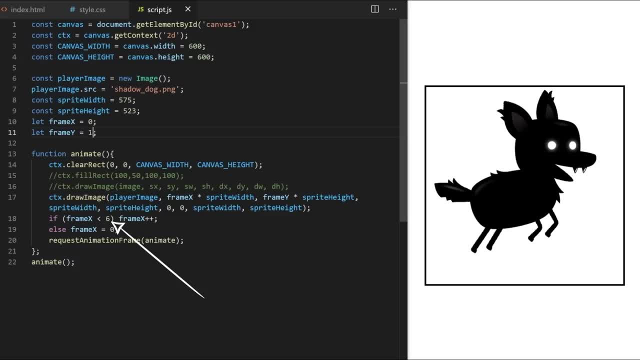 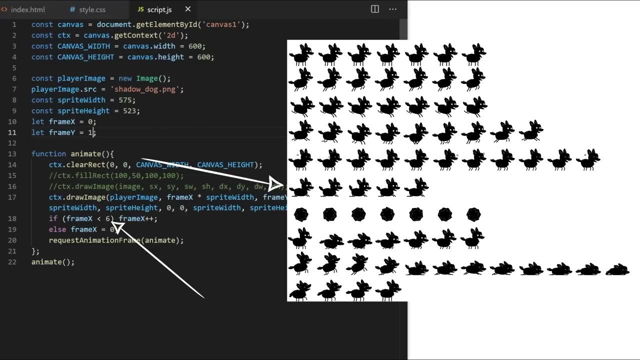 I would slot it here And every time I change frameY variable I would change value of that maxFrame variable from 6 to whatever value. I want To display all frames, So 10 for this row and 4 for this row, since we are animating from frame 0.. 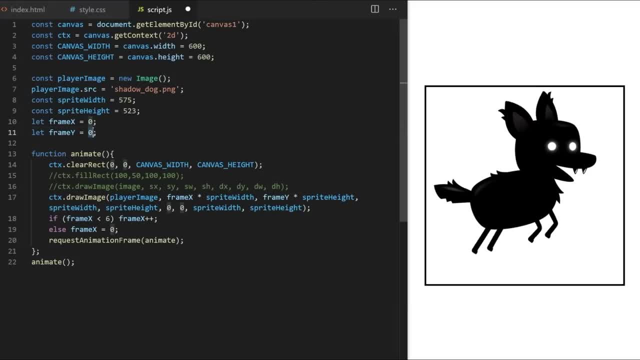 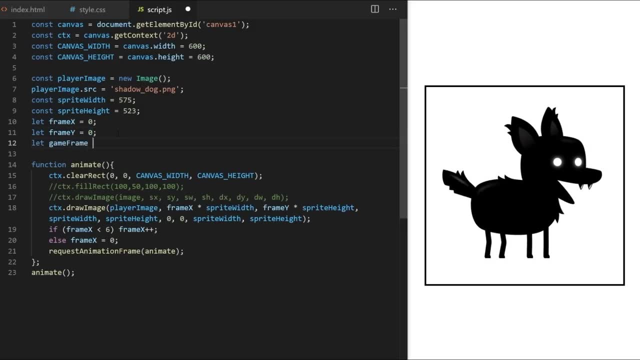 Animation is going very fast. To slow it down, we can use this simple trick. I will create a let variable called gameFrame and I set it to 0.. On line 22, inside animation loop, I take this gameFrame variable and for every loop we 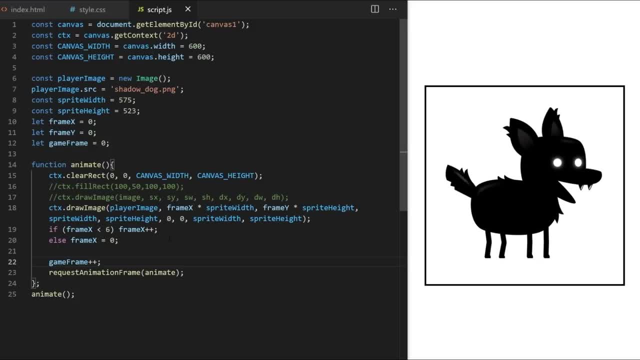 increase it by 1.. So now gameFrame is endlessly increasing as our animation loop runs over and over On line 19,. I create an if statement. Let me just write it and I will explain it when we see the whole thing. 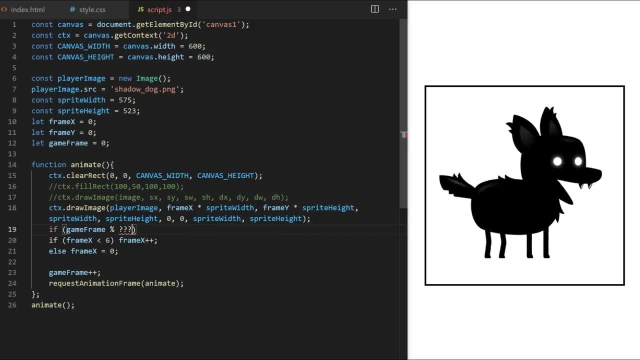 I say: if gameFrame modulus percentage symbol- something question marks for now- is equal to 0, only then increase frameX On line 13,. I create a custom constant variable called stackData. Let me just write it and I will explain it when we see the whole thing. 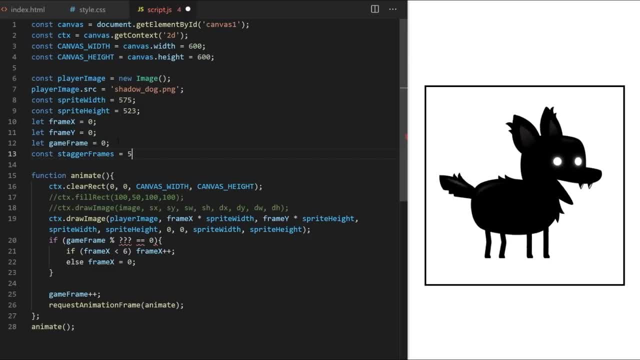 Whatever value I give it, it will slow down animation by that amount. Let's try 5.. On line 20, I say: if gameFrame modulus staggerFrame is 0, only then increase frameX Modulus operator. percentage symbol is also called remainder operator. 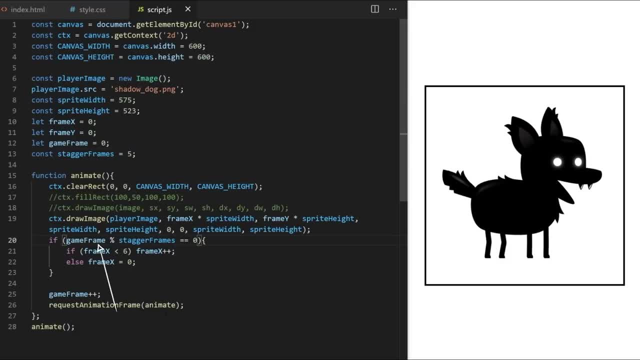 It returns remainder when we divide the first number by the second. Let's say gameFrame is 17. And staggerFrames is 5. 17, modulus 5 is 2. Because 17 divided by 5 is 3, that gives us 15.. 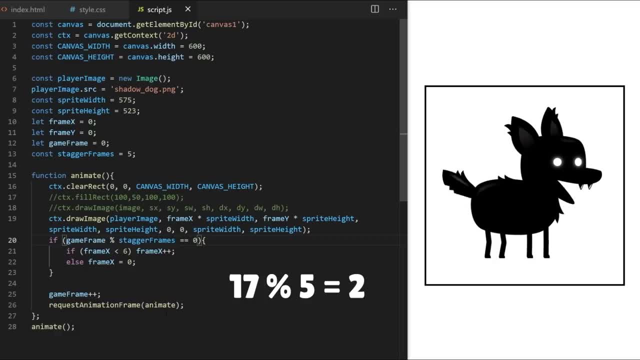 And remainder to 17 is 2.. Remainder operator simply divides the first operand by the second one and returns the remainder. Here I am checking if the remainder is 0.. GameFrame is ever increasing number and staggerFrames is always 5.. 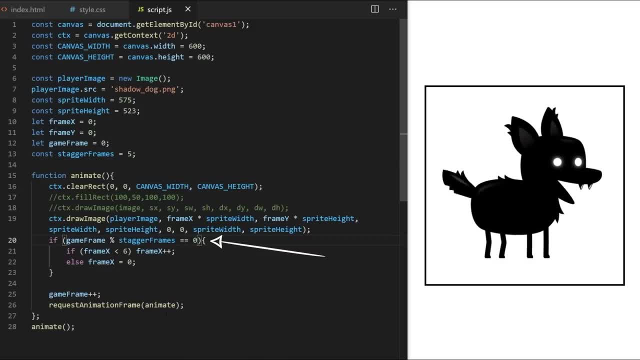 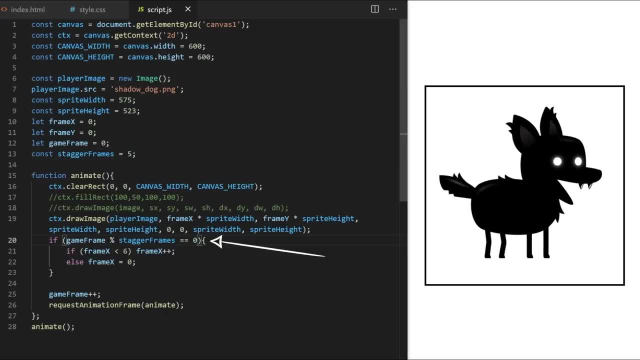 GameFrame is ever increasing number and staggerFrames is always 5.. GameFrame is ever increasing number and staggerFrames is always 5.. gameFrame is ever increasing number and victories are meant to count number in 5.. So gameFrame at the moment has 0. 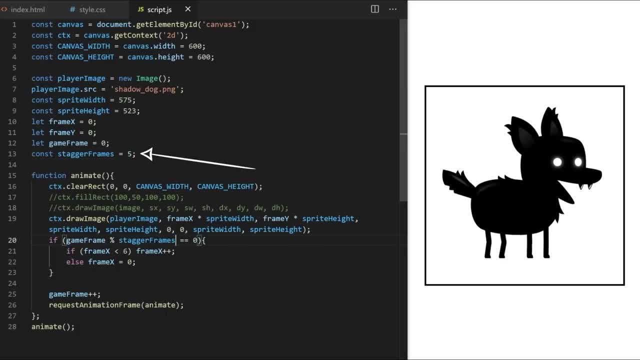 But, as anybody knows, staggers have only plus 1 piece and 2 pieces less, not As anybody knows. when a game Breatнять, tone here will become 0, in which caseaps stronger for the order of 5 frames. As anybody knows, game komplett will return. remainder 0 and A ≗ • 0 will be true. 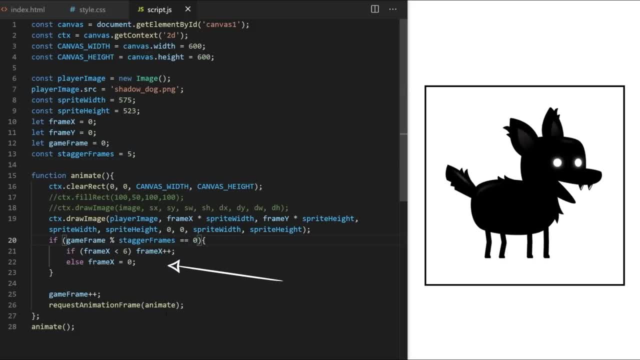 5 times. So because I set staggerFrame to 5, this code block on line 20 will run every 5 frames, slowing down our animation 5 times. new frame in our sprite sheet will only be served every time the main animation loop runs five times. i can also slow it just by two. 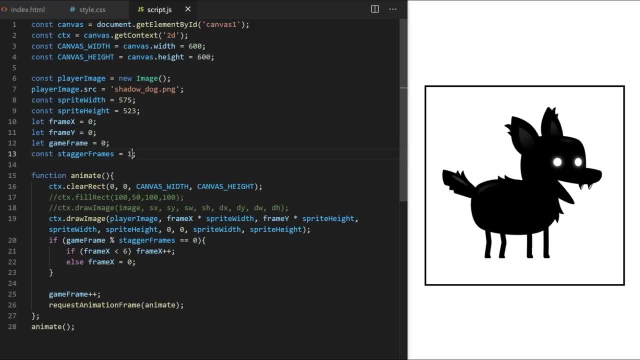 zero here will stop animating. the higher the number you use here as stagger frames, the slower the animation will be going. let's leave it at five for now. i think it looks good for most animations, as i said, when i change frame y to 4 if i want to display all frames in my 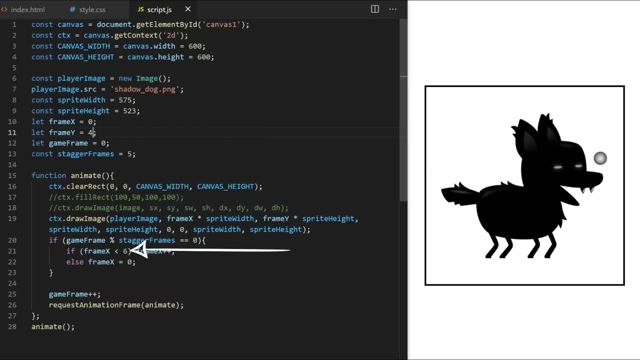 animation. i also have to change 6 here on line 21 to number 9 for shorter animation rows like this sitting animation. it has only five frames, so i have to change this number to four. so now we have a way to swap between animations, but we always have to change two values. 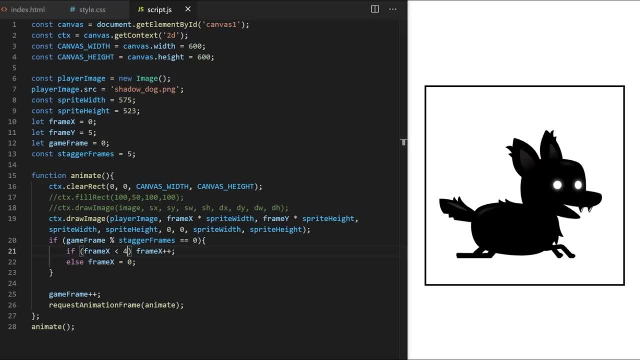 let's refactor this code and let me show you more advanced sprite animation method that allows us swapping between different animation states. by changing just one value, we are venturing into a bit more advanced territory. if you are new to javascript, don't worry if it takes you a bit longer. 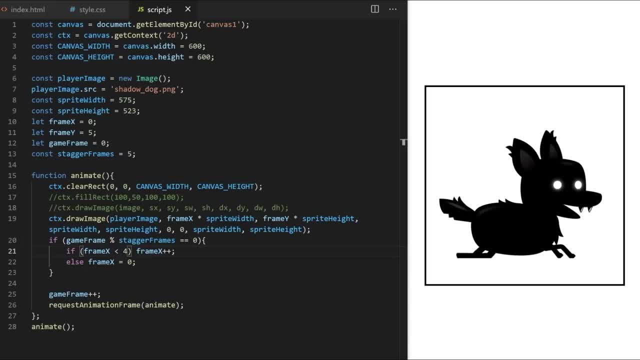 to understand what i'm about to show you. it becomes easier with practice. we all started somewhere. i delete code between lines 20 and 23. we used it to cycle between animation frames horizontally. in this more advanced method we will do it differently. i set frame y to 0. that's my top row. idle animation. i also delete lines. 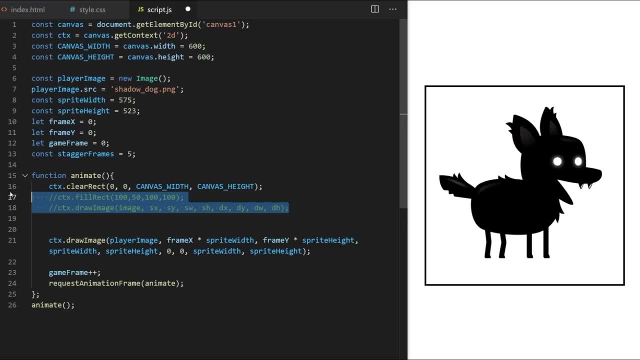 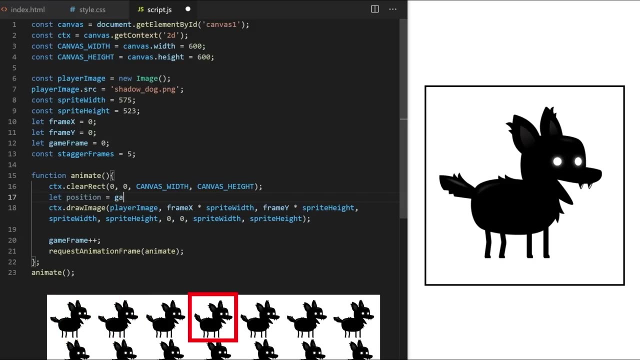 17 and 18. they are commented out. anyway, let's clean this up. inside animation loop on line 17, i create a let variable called for example position. its job will be to cycle through horizontal sprite sheets, but in a different way. we will need this later. i take a game frame variable from line 12.. this variable is increasing. 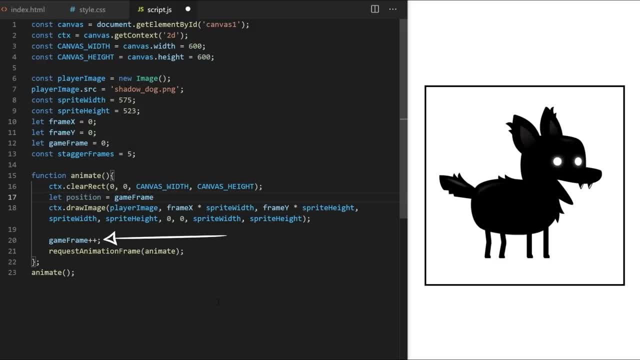 over and over on line 20 as animation loop runs. i divide it by stagger frames variable from line 13 and i wrap all of this in math dot floor to get rid of potential decimal points. i want this value to be only integers, whole numbers, without decimal points. then i take 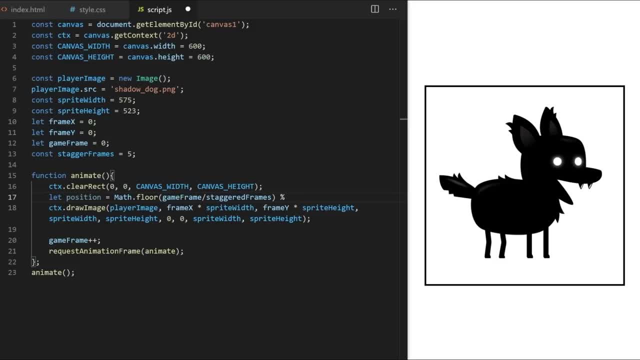 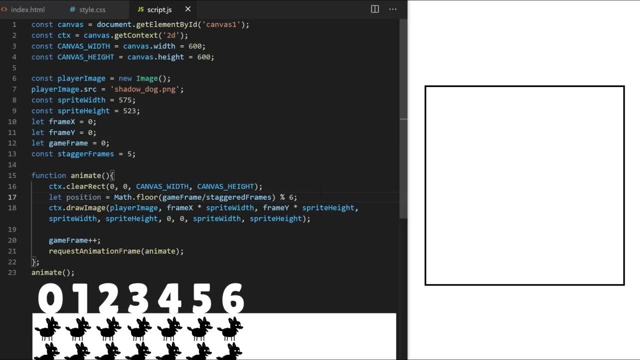 this entire value and i do remainder operator. and six. six is here because i'm doing idle animation which has six frames counting from zero. this line of code is not the easiest thing to wrap your head around. i said this would be slightly more advanced. don't worry if you struggle. 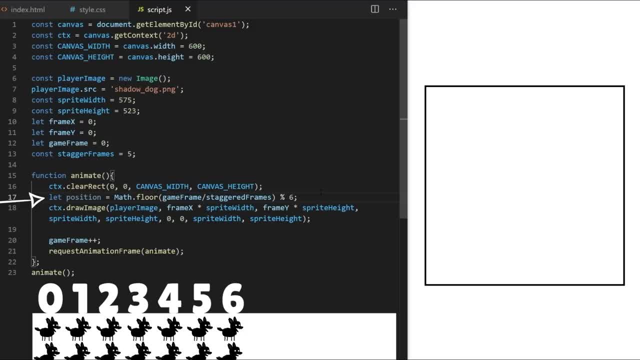 to read this. this is not beginner level javascript anymore. what's happening here? on line 17? game frame divided by stagger frames means we will have to increase game frame five times before we get to one, because, as game frame variable increases, one divided by five is 0.2. 2 divided by 5 is 0.4. 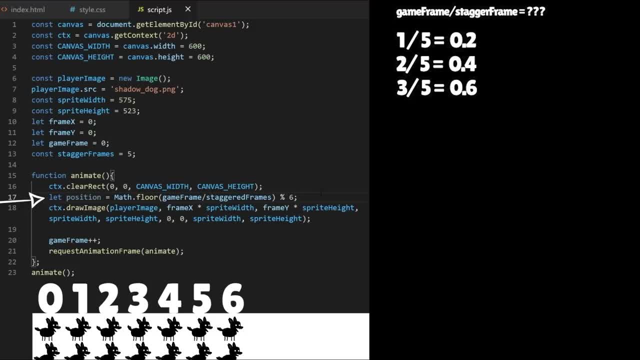 3 divided by 5 is 0.6. game frame 4 divided by staggerframes 5 is 0.8. and only when we get to game frame 5 divided by stagger frame 5, we get value of 1 here, so as game frame cycled from 1. 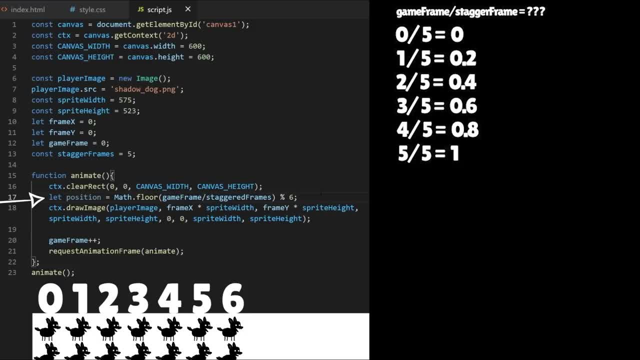 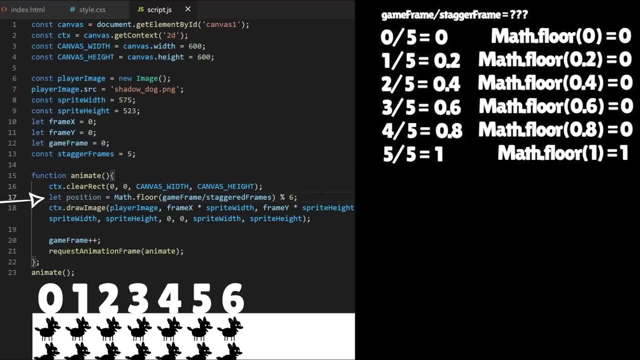 2, 3, 4, 5. by dividing game frame by stagger frames, we got 0, 0.2, 0.4, 0.6 and 0.8. all of these values were turned in order to increase game frame consommation in less than javascript 2.0 or max. 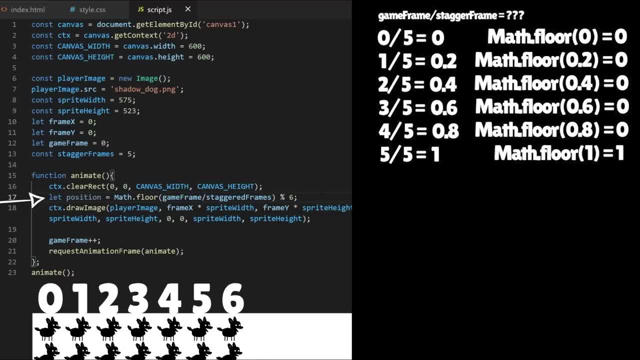 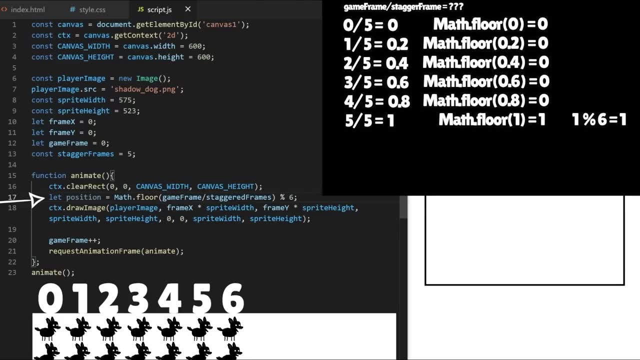 turned into zeros because it's wrapped in mathfloor. It took 5 animation loops, 5 increases of gameframe variable to get the number 1 here. When this is 1, 1 modulus 6 is 1 because 1 divided by 6 is 0 and remainder from 0 to. 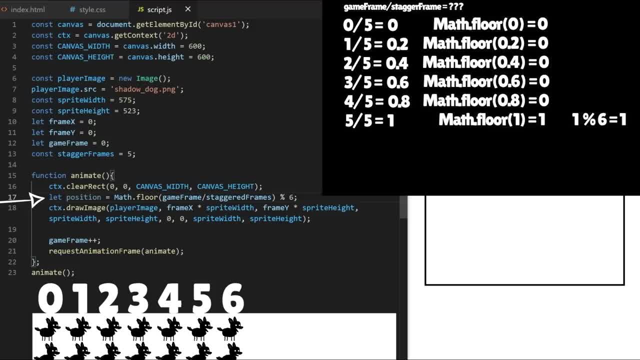 1 is 1.. Basically, this value increases by 1 every time gameframe variable increases by 5, slowing or staggering our animation 5 times, making it 5 times slower. We are using mathfloor, removing decimal points from these divisions. 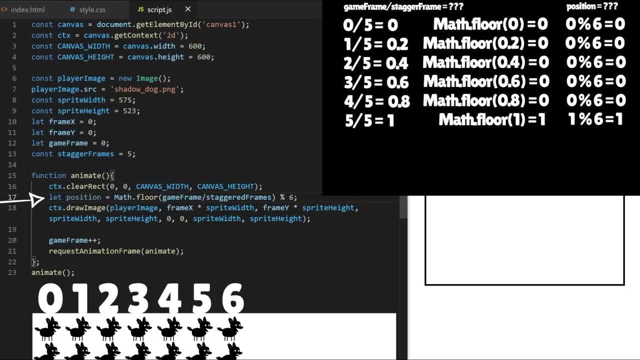 For the first 5 frames, we get 0 modulus 6, which is 0., Then this calculation increases to 1.. For the next 5 frames, 1 modulus 6 is 1.. Then 2 modulus 6 is 2, 3 modulus 6 is 3, and so on. 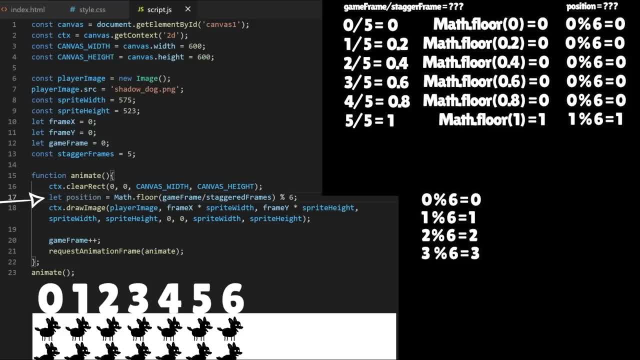 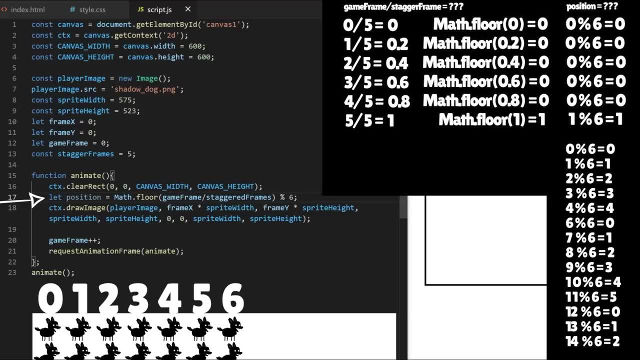 Position variable increases until it reaches 6.. 6 modulus 6 is 0,, 7 modulus 6 is 1,. 8 modulus 6 is remainder 2, and so on. This calculation makes sure position variable only cycles between 0 and this number. 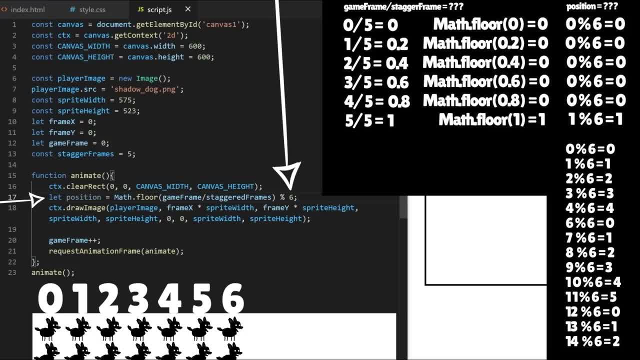 I appreciate that this calculation is quite complex. This is not course in advanced mathematics and logic, So for now, just take this little formula here and believe me when I say it works. Don't worry about understanding it completely. We are focusing on javascript today. 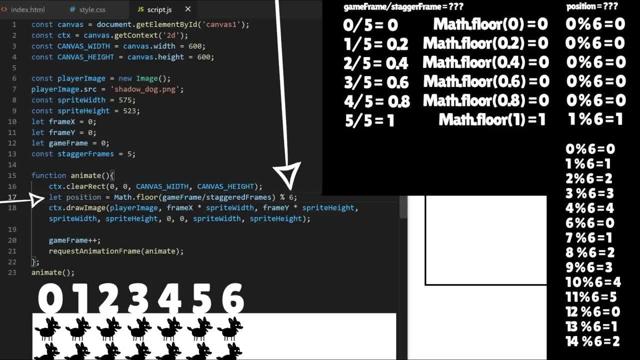 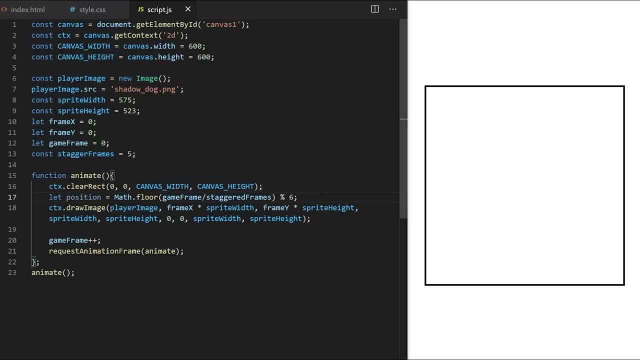 Being able to understand this calculation is very important. This calculation has nothing to do with your ability to be good with javascript. These are two unrelated skills. On line 18, I take frame x variable from line 10 and I set it equal to sprite width from. 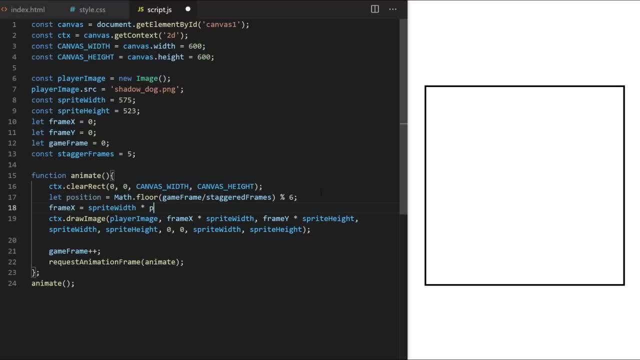 line 8. And I multiply it by this position variable we just calculated on line 17.. As I said, this position variable will cycle between 0 and number. we put here First row in my sprite sheet has 7 frames starting from 0.. 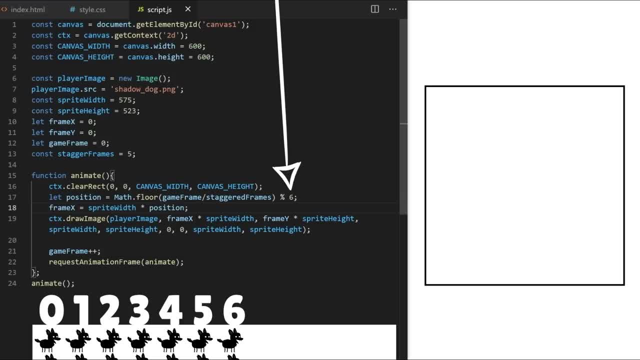 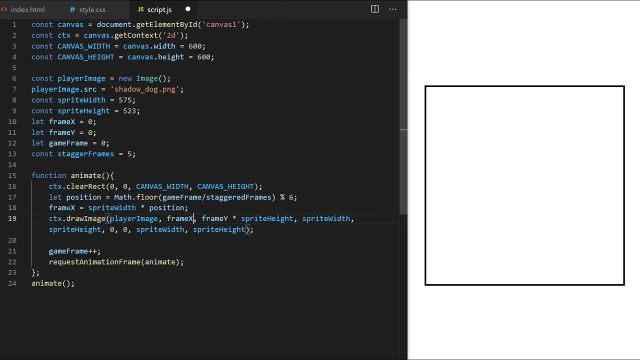 Frame x will be cycling through these values horizontally. On line 19 inside the draw image, I remove sprite width because width of our sprites is already accounted for inside my frame x variable on line 18.. I misspelled stagger frame x. This is a very common mistake. 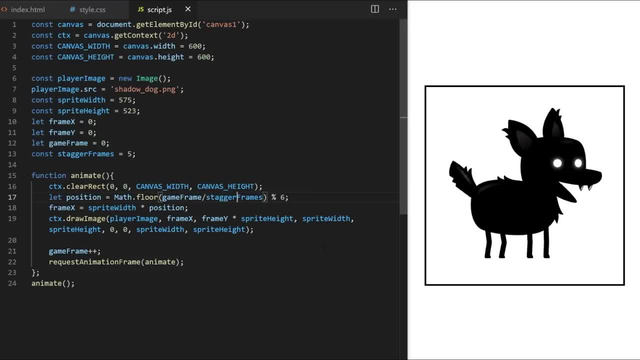 This is a very common mistake. When I fix this small typo, we can see this is working and we are animating row 1 in our sprite sheet. Don't feel that you need to fully understand this calculation on line 17 to be good at. 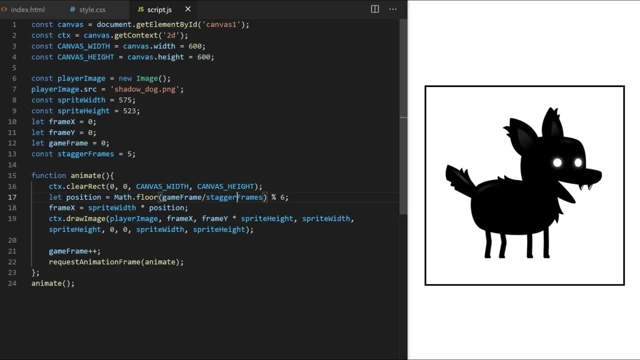 javascript. I did not come up with this formula. Tricks like this are usually figured out by someone much smarter than me. We can just use them and they will work for us. I could have achieved the same result using a bit more code and simple, more readable calculations. 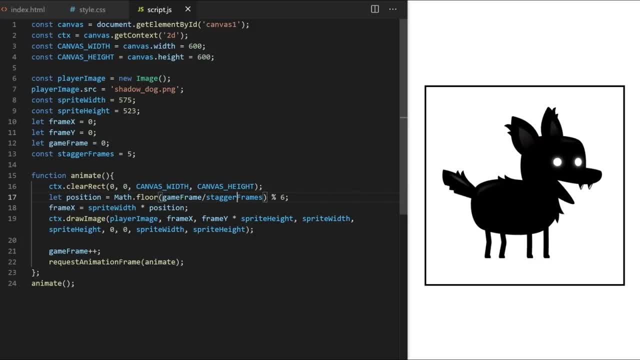 This is more complex and hard to read For beginners because it's such a short calculation. It's kind of a neat trick to use this, but it's not a necessity. I like it because it makes the code look clean and compact. I can still change value of stagger frames variable on line 15 and it will slow down. 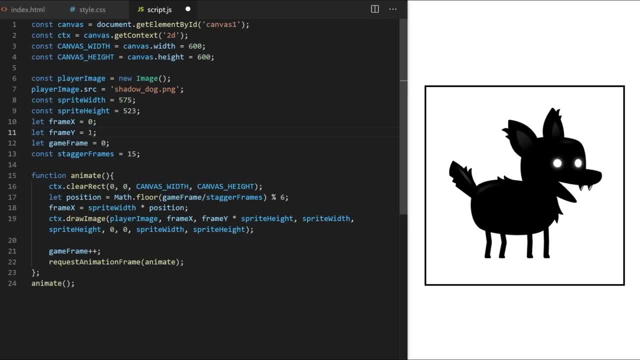 or speed up my animation. This is really nice code base to animate any sprite sheet, but it can be done even better To swap between animations. I still have to change frame y variable on line 11 and I have to make sure that this value on line 17 sets the correct amount of frames per row to 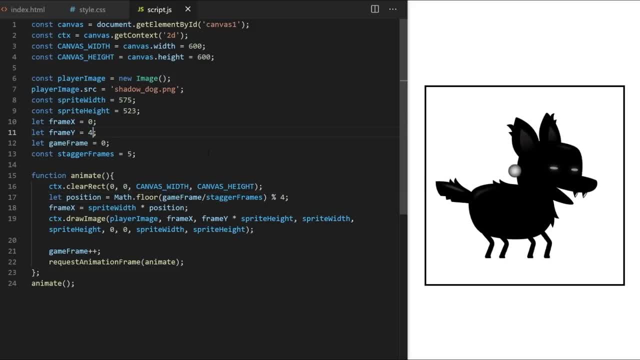 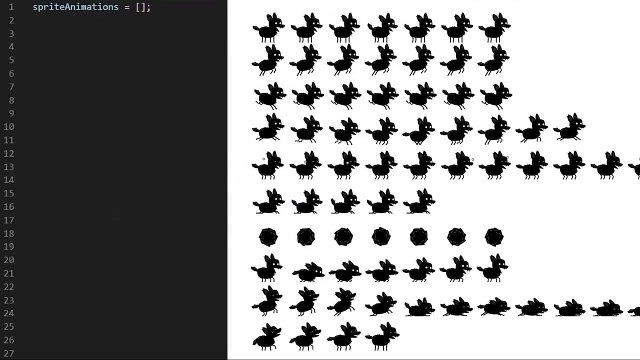 make sure we don't have any empty frames or that we are animating all available frames from that particular row, depending on what animation we are currently drawing. Ok, Let's try this. Ok, Ok, Ok, Ok, Ok, Ok, I can change gerne more, because I want to try it. 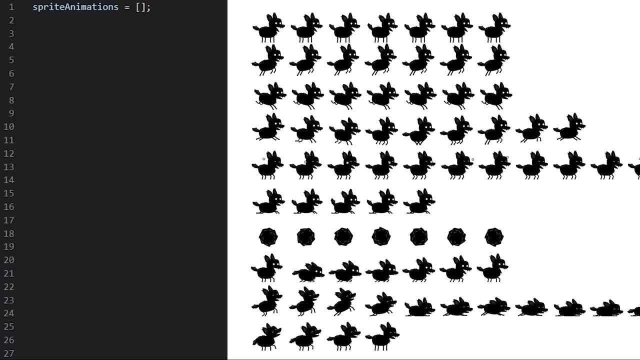 Lets jump right into it. What objects we can pick again. For example, there is a code structure like this: That document, which is called Some kind of data array- called, for example, sprite animations- That contains objects. Each objects name in this array is the same as the name of that particular animation. 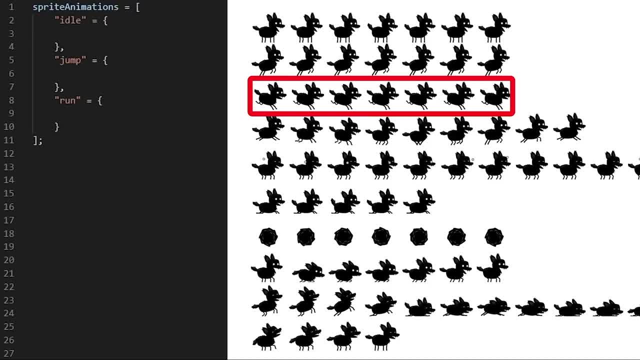 it holds data for, so, for example, idle, jump run and so on. Each of these objects can contain additional data. For example, for irregular sprites, I can be pixel values array. This location array will hold a set of JavaScript objects and each of these objects. 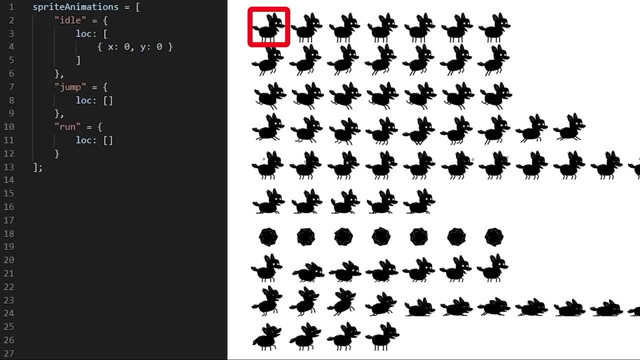 will have x and y property. Each of these objects represents one frame in that particular animation and its x and y properties will be coordinates. we need, if we want to use draw method, to cut out this particular frame from the sprite sheet. That way we can access any. 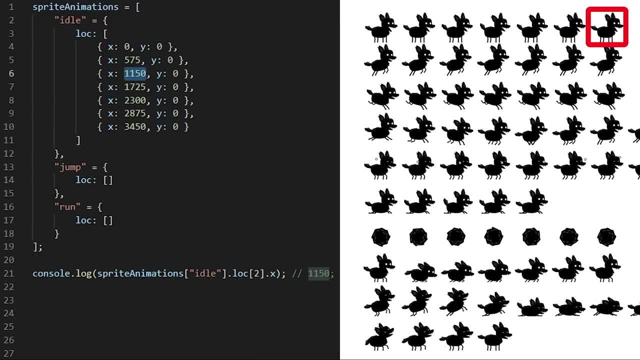 frame we want anytime by directly targeting positions in this array. I can just cycle through this location array with a for loop and it will always play the entire animation for me without the need to set up number of frames each animation has each time It will. 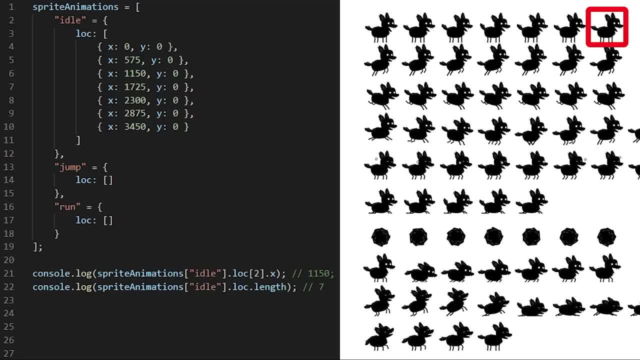 know how many frames that animation has. based on the number of objects in this location array, Each object will be one frame. So how do we create a data structure like this with JavaScript and how do we map it correctly to match our sprite sheet? Let me show you. 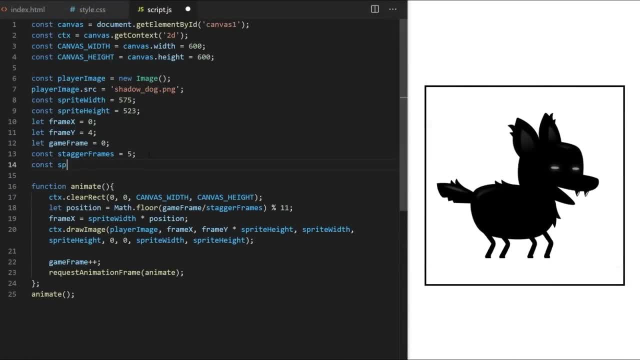 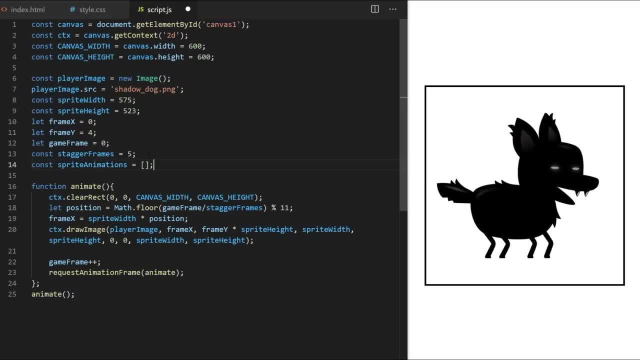 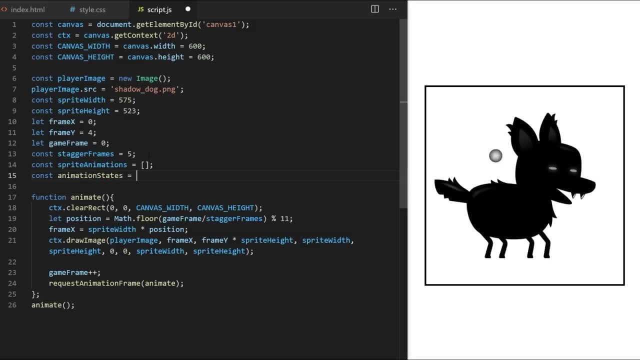 equal to an empty array. This will serve as the main container to hold all data for all my animations. I will create another variable I call animation states. This will also be an array and I will use it as a place where I can create kind of a simple map that will 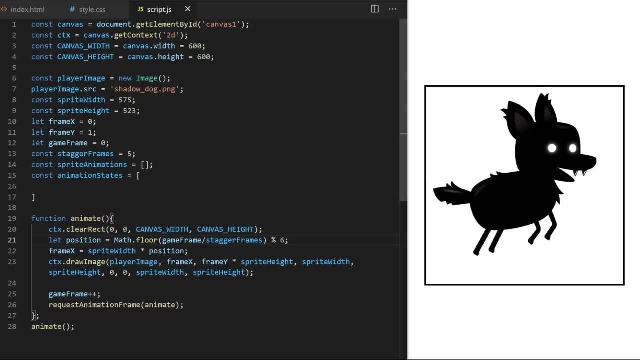 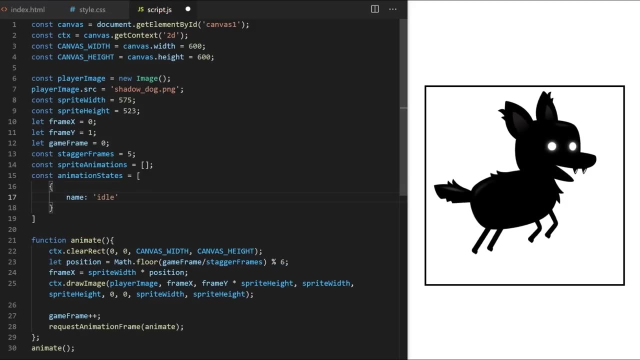 match my doc sprite sheet. I will go through my sprite sheet row by row, from top to bottom. for every animation row in my sprite sheet I will create an object like this with two properties. Name property will be whatever I want to call that animation row. So for the first row, let's call it idle And I will 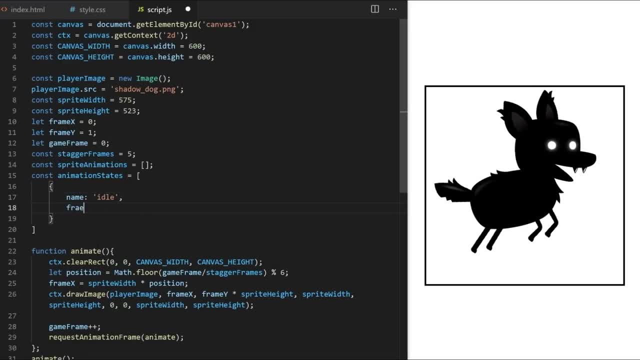 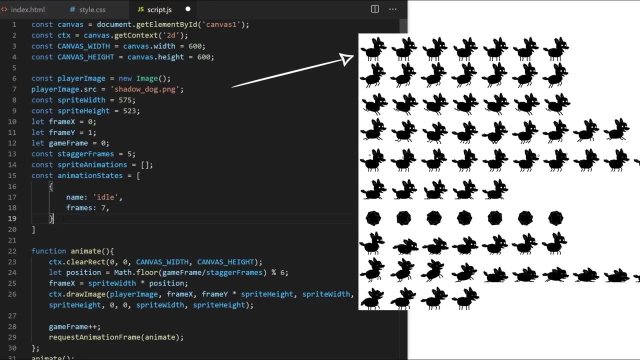 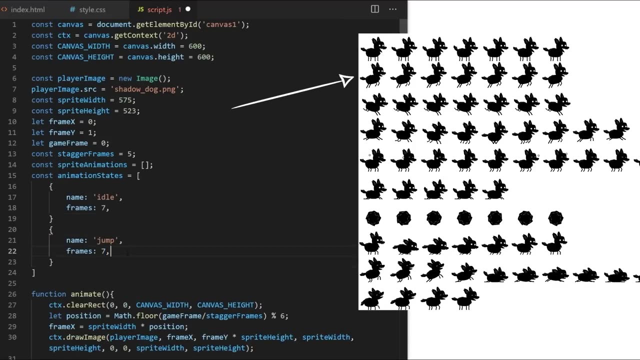 also need frames property. I check my sprite sheet and I see that idle animation is made out of seven frames. The second row I will call jump animation and it has seven frames. I will create an object like this for every row in my sprite sheet, going from top to bottom. but before I do that, 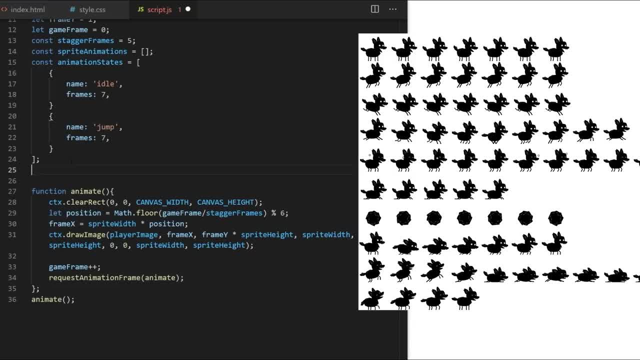 let's check if it works. on line 15 I have this animation states array which currently contains two objects, one for idle and one for jump animation. I could have also given it more properties, but this sprite sheet is not irregular, so name and frames properties is all I need to map coordinates for each animation. 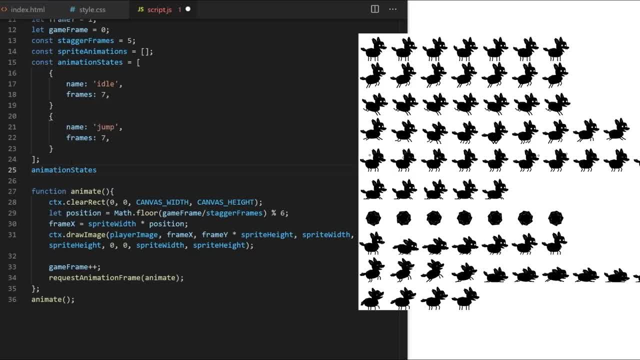 frame. I take animation states array and I call build in array for each method. for each method executes provided function once for each array element. I will do ES6 syntax here. this is so-called arrow function. it's a simplified syntax to write function expression in JavaScript. I can skip. 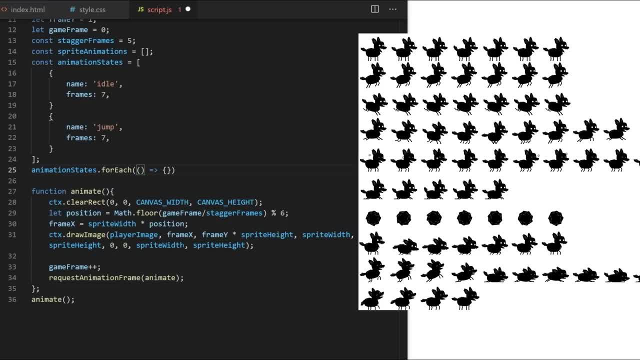 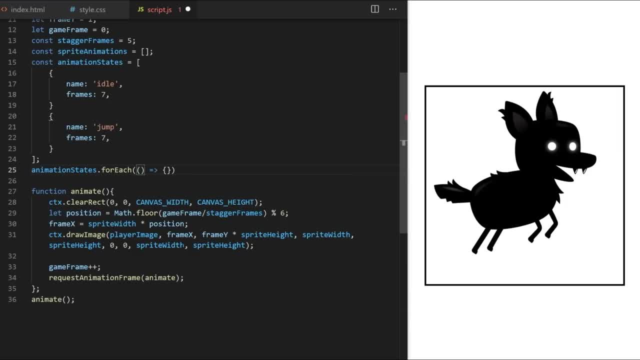 function keyword here, and I just create brackets where arguments I pass to this callback function go with for each. the first argument we pass to it is just a variable that will represent each element in the array as we are cycling through it. I will call it. state as for. 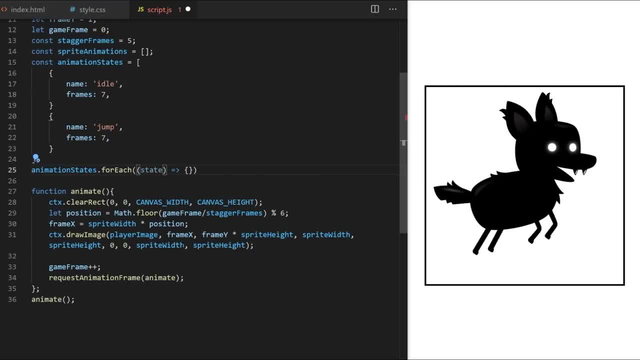 each method runs, state will first represent this object, then this object, and so on. if we add more, I'm simply saying inside this callback function I'm about to write, refer to these objects as state, so this name property can be accessed as state dot name, for example. I will also pass it. 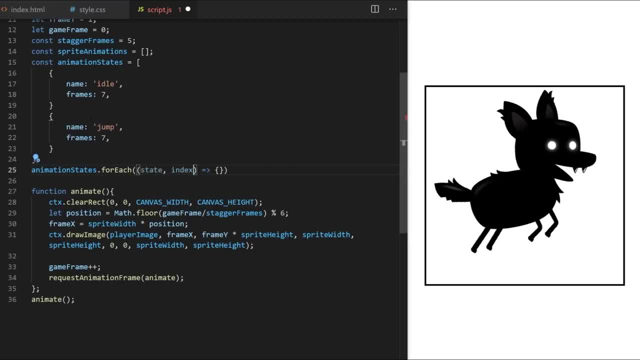 second argument I call index. index is another built-in feature of for each array method. it simply stores number of each element as we cycle through the array. so this first object will have index 0, this will have index 1, and so on. I expect you understand basic array manipulation with JavaScript and 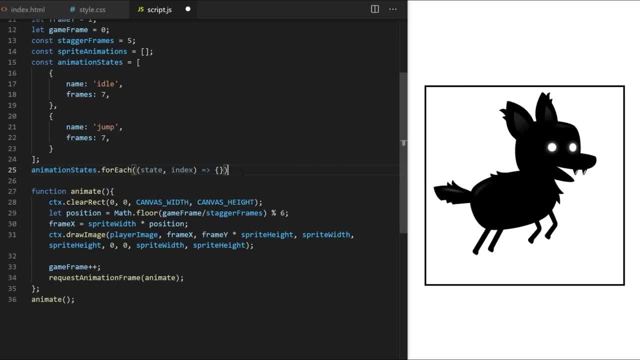 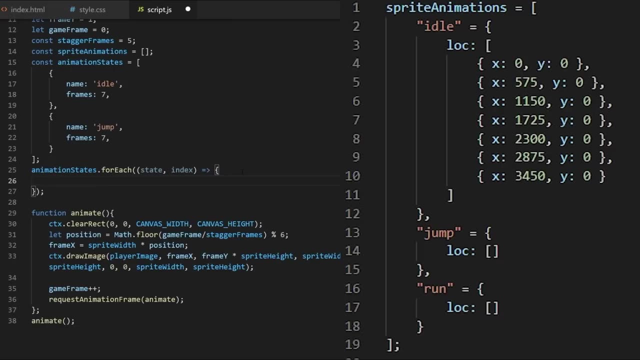 fundamental methods like for each, but I still wanted to explain in case we have some beginners here. so this callback function will run for each element in my animation states: array. now I want to run the array function. and I want to run the array function and I want to run theptp. 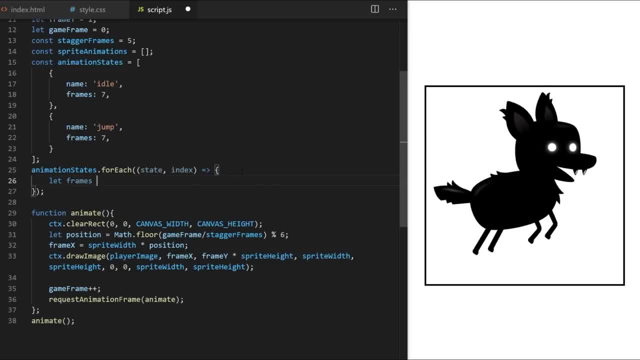 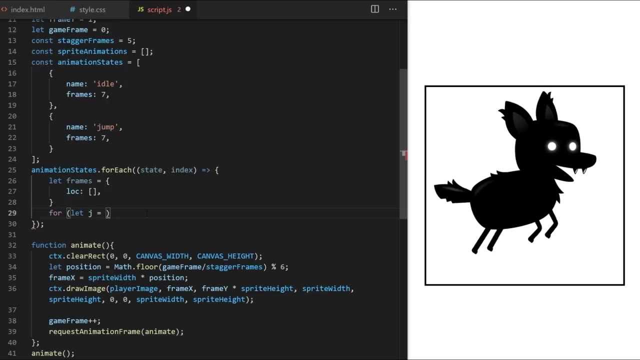 I createmay assignment arbitrary state in to run through animation states and create data structure like this that maps my sprite sheet and coordinates for each frame. I create led variable called frames and I said it equal to an object. inside I will have property called LLC location. 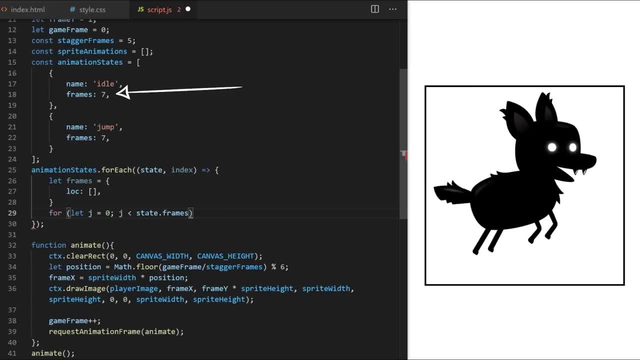 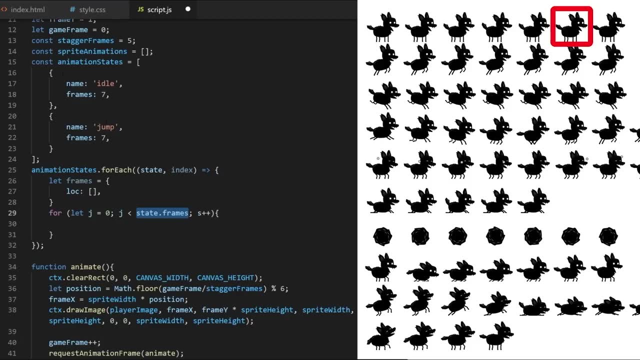 that will be an empty array for now on line 18.. Every time this for loop runs, I want to calculate x and y coordinates of that animation frame from my sprite sheet and I want to place them inside location array on line 27.. How do I? 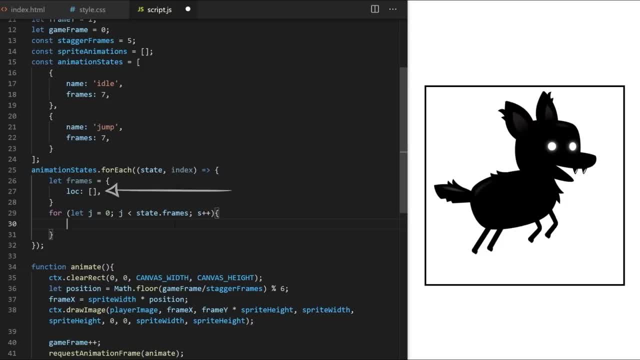 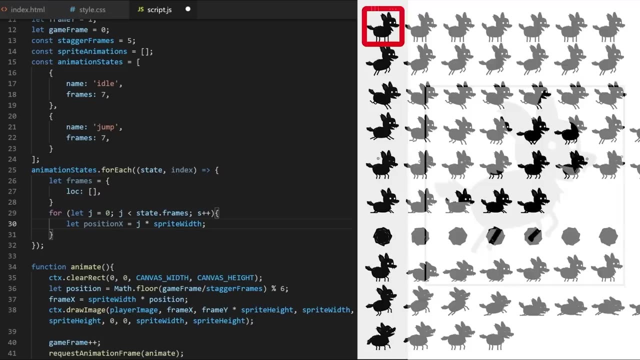 calculate that I create a temporary variable called position x and it will be equal to j variable from the for loop times sprite width that I set to 575 pixels earlier. As a for loop runs and j increases, position x will be calculated for each frame. I will also need position y, which will 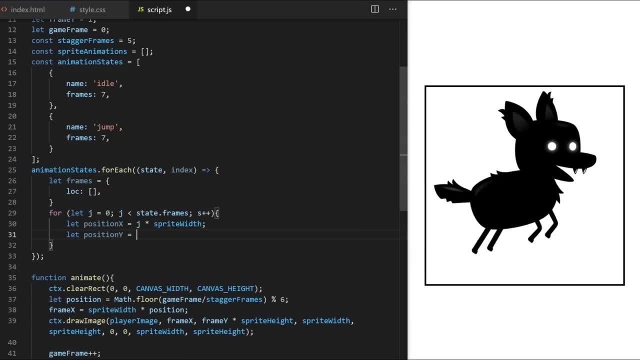 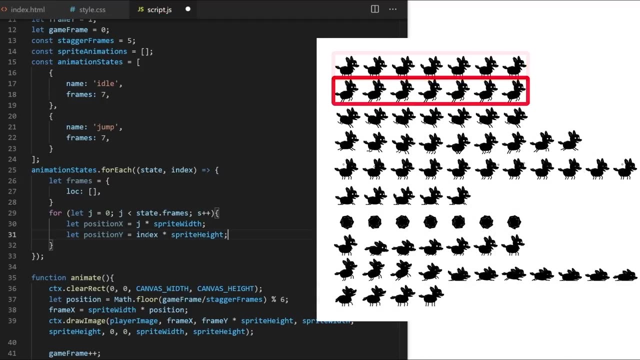 be index from line 25 times sprite height. We declared sprite height earlier and we set it equal to 523 pixels to match our sprite sheet. Position y will be the same for all seven frames of idle animation. When for each method moves to the second animation object, here index will increase. 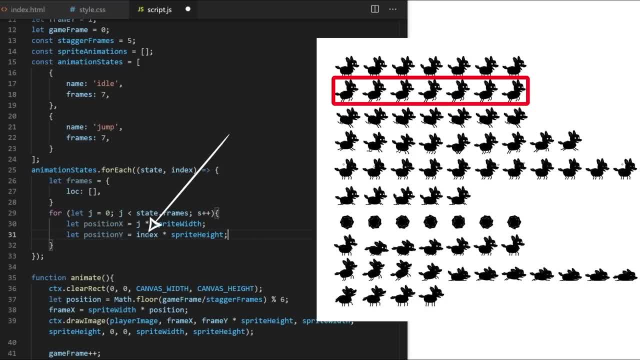 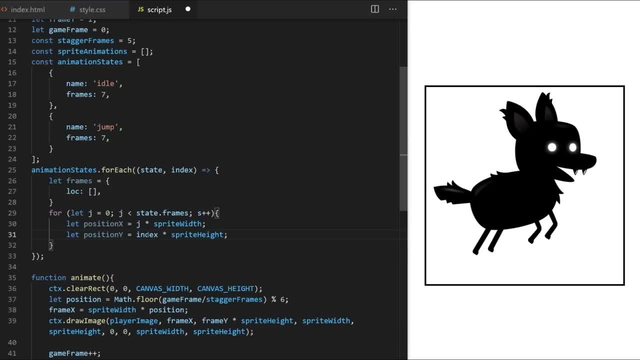 and for that animation row, different position y will be calculated. This might be quite a lot going on. if you are a beginner, This is more advanced than the first sprite animation method. Don't feel discouraged if you are struggling to follow. it takes time and practice. it wasn't easy for any of us at first. So this for loop calculates position x. 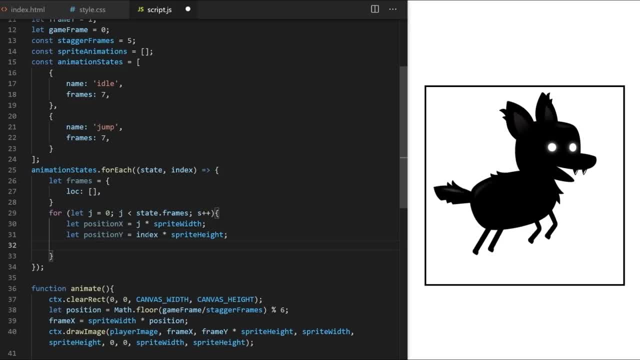 and position y for each frame as it cycles through my sprite sheet. Every time we calculate x and y, I take frames dot location array from line 27 and I use push method. I create a new for loop which will be x and y. from line 27 and I use push method, I create a new for loop and I set it equal to 575 pixels to match my sprite height. I create a new for loop and I set it equal to 575 pixels to match my sprite height. I create a new for loop and I use push method. I create. 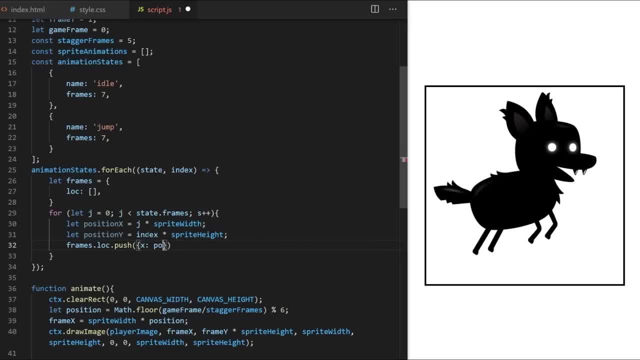 another small object here on a fly. it has x property set to position x from line 30 and y property set to position y from line 31.. i push these values into my location array on line 27.. so this for loop will run through all the frames in one row, in this case seven times, and once we 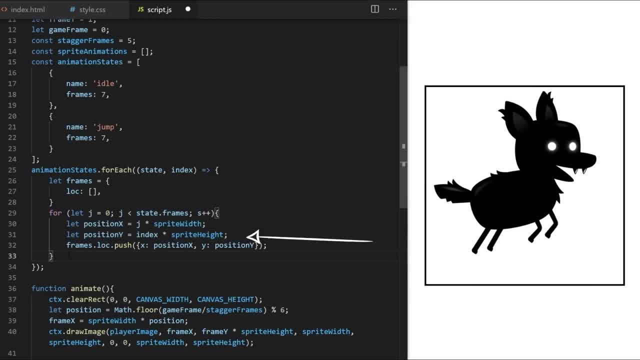 create seven objects with x and y coordinates and push them into location array. i take sprite animations array from line 14 and i create a new key in there. i will create something called key value pair. key is the name of the property, value is the value of that property. so i'm taking 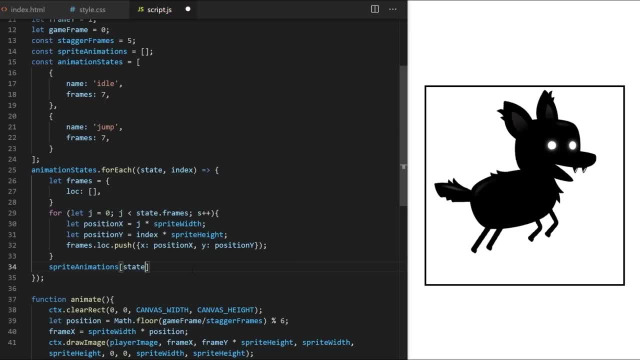 sprite animations array from line 14 and i'm passing it state dot name, which will first refer to idle, then to jump. as for each method runs through animation states array. i'm saying: create a new key, new property in sprite animations array, call it idle and its value will be frames from line 27: frames object contains locations array. 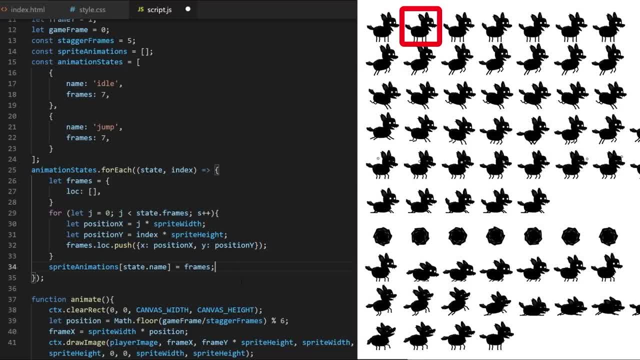 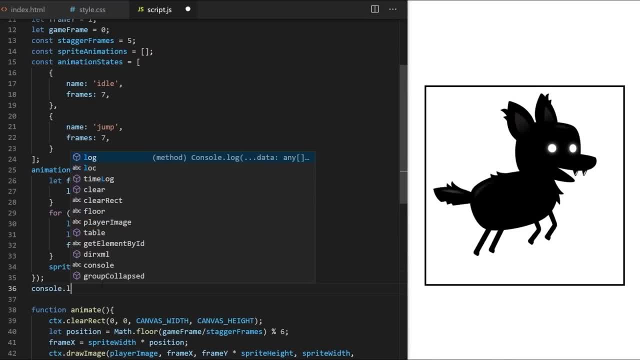 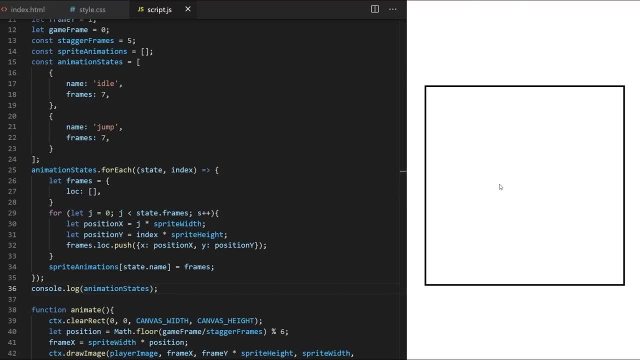 which i just filled with seven objects that contain x and y properties for each frame in this animation. that's it. we created the data structure that maps locations in my sprite sheet. i can console log it now. i can see i made a typo here on line 29. you probably noticed it already. 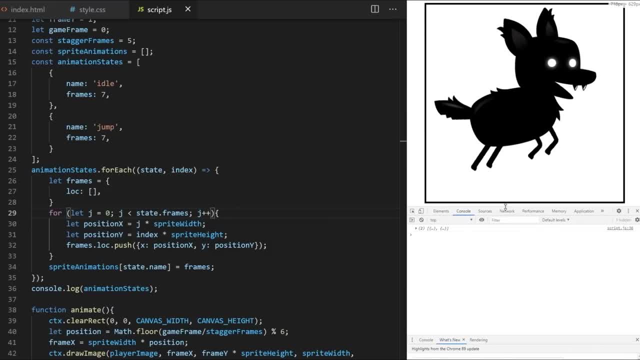 this should be j not s. so now i'm console login. animation states from line 15. that's fine, but what i actually want to see is sprite animations array from line 14, which we just created and filled with data. you can see that my sprite animations contains two properties. 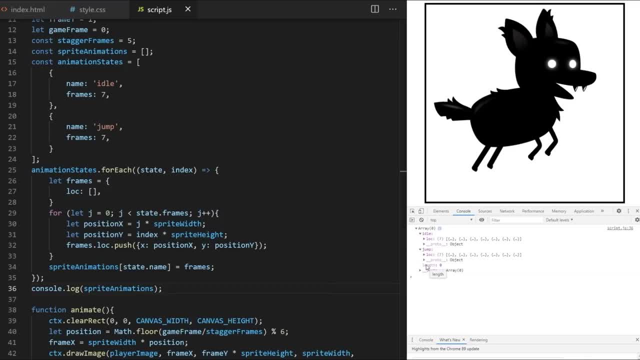 called idle and jump. if i look inside, each contains location array from line 27 and number of elements in that array corresponds to frames i declared for each animation. each of these values was calculated here on lines 30 and 31 you can see that all y coordinates for: 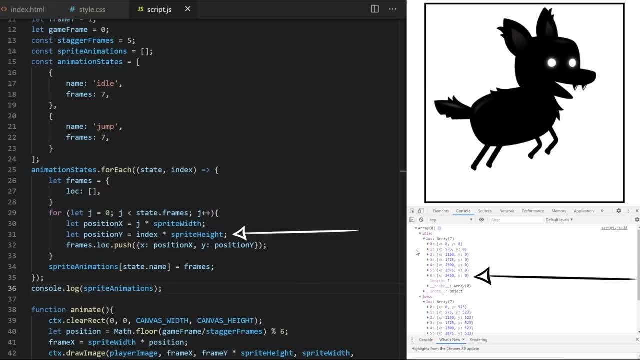 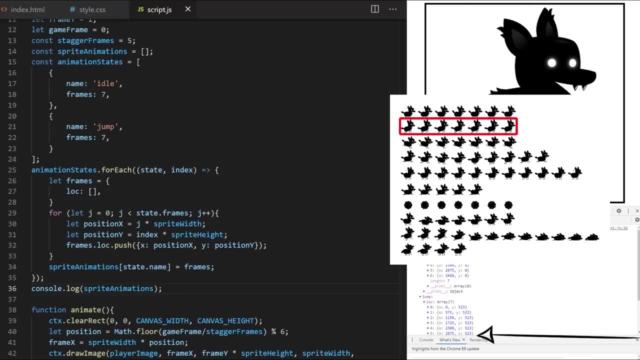 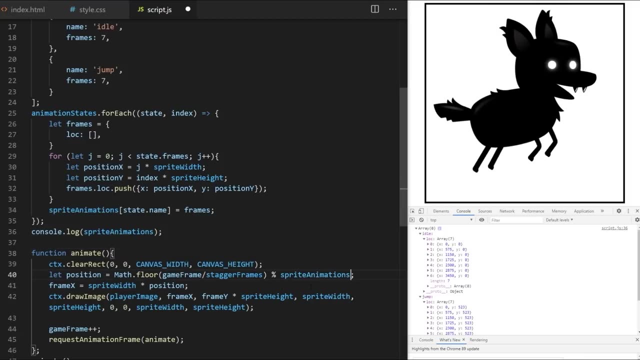 idle are zero and for jump animation vertical y coordinate is 523. as we moved on to the second row in our sprite sheet, now i can replace hardcoded number six here on line 40 with length of these locations arrays. i access this location array by targeting sprite animations. dot log- actually no, i. 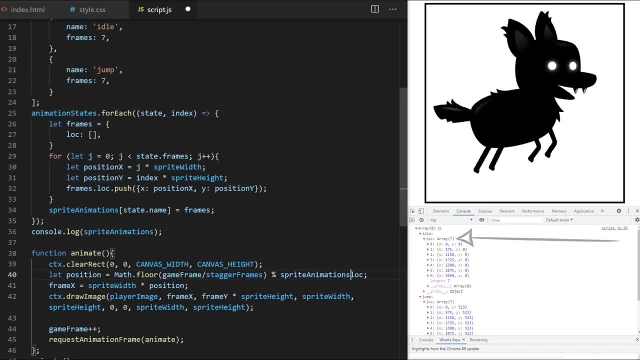 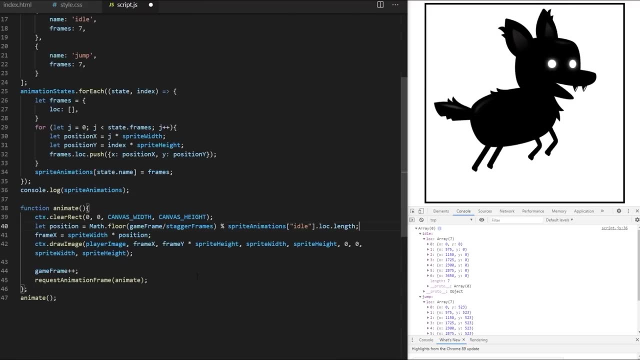 want to specify the location array for idle or jump. i need to specify. if i want location array for idle or jump- let's just hardcode idle here for a moment- and i want length of this array. remember, i am just replacing hardcoded number six that was here, so dot length and that's it. now it's dynamic. 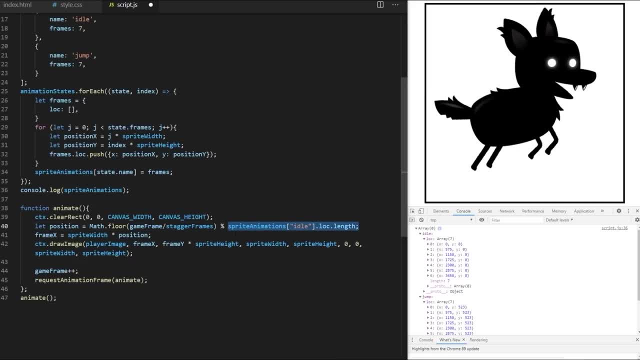 i can add animations with 4 or 15 frames per row, or however many i want, and it will still work with no blank or left out animation frames. here i am accessing sprite animations from line 35 to line 40, from line 14: idle location, dot length. 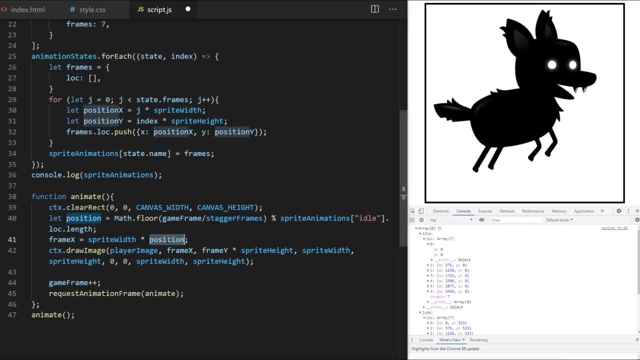 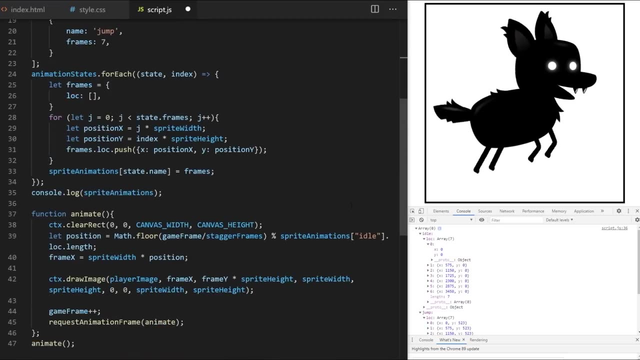 inside animation loop. we are still calculating frames using frame x and frame y variables from lines 10 and 11. we don't need these anymore because now we have the exact coordinates stored in locations array. i delete lines 10 and 11.. on line 40 i add let keyword in front of frame x. 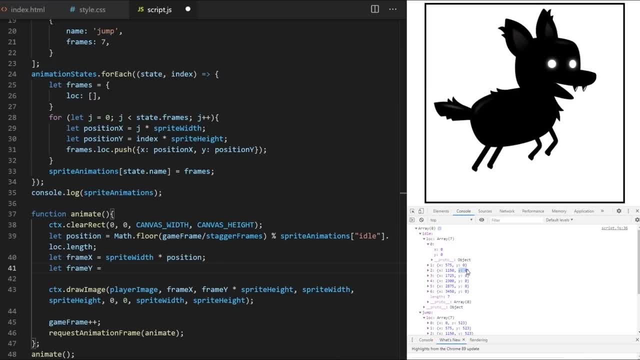 and i will declare frame y variable here. frame y is just the value we can see here, so i can access it by saying: sprite animations- idle, dot. location at index position from line 39, dot y. i could do the same thing for frame x or i can just leave it as is. both will work. let's replace idle with a jump. 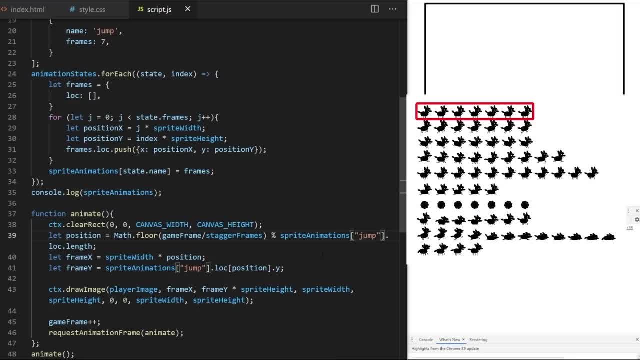 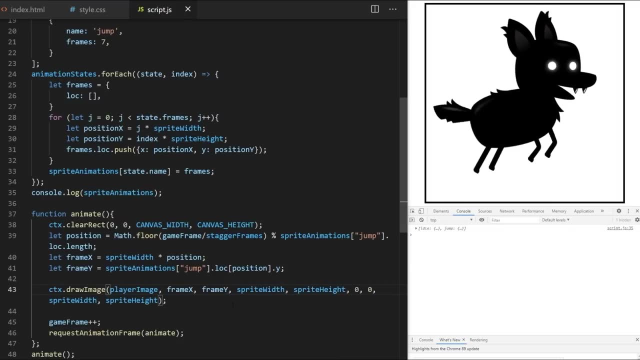 it breaks notice that row 1 with idle animation was working and row 2 doesn't, which suggests something is wrong with how we draw vertical position inside. draw image on line 43. i remove sprite width value from source y argument. we don't need it anymore, as frame y contains complete, already calculated. 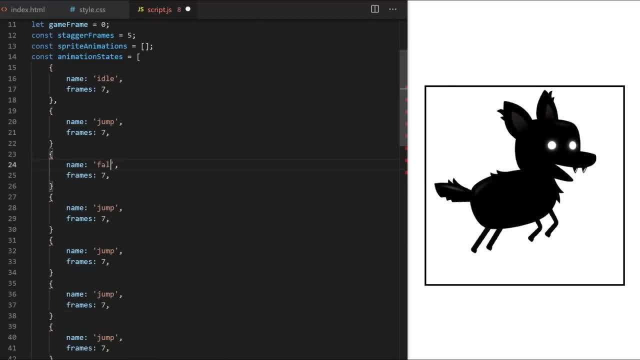 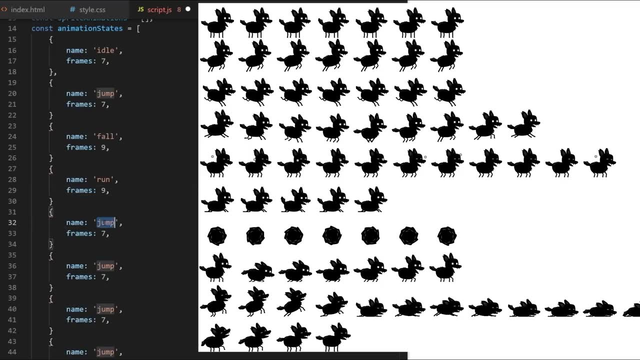 coordinate. now i can go back inside animation states array and i add data for all the remaining animations. it's important to understand that you can't skip rows here. you have to go back to your. you have to go row by row from top to bottom to match your sprite sheet, because vertical y. 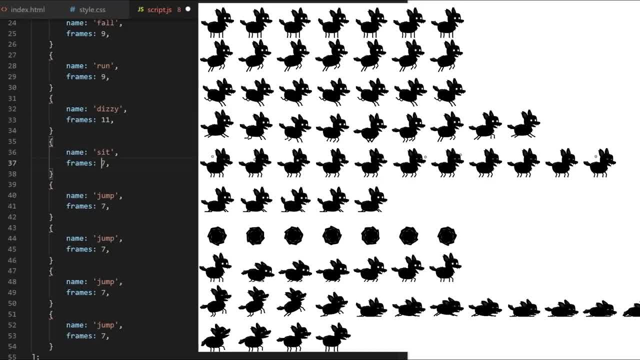 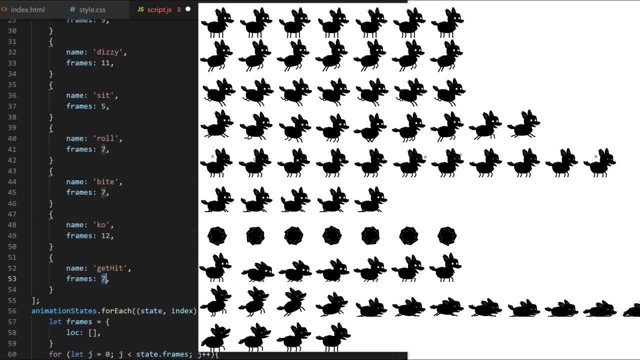 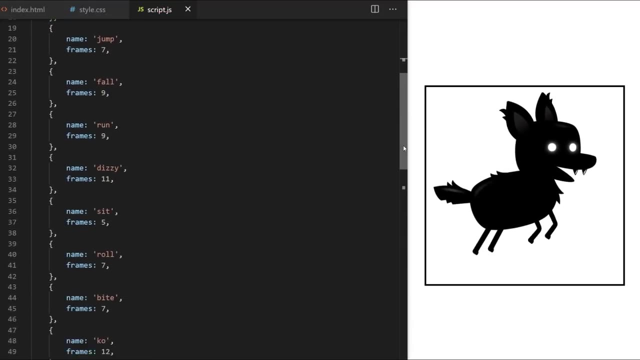 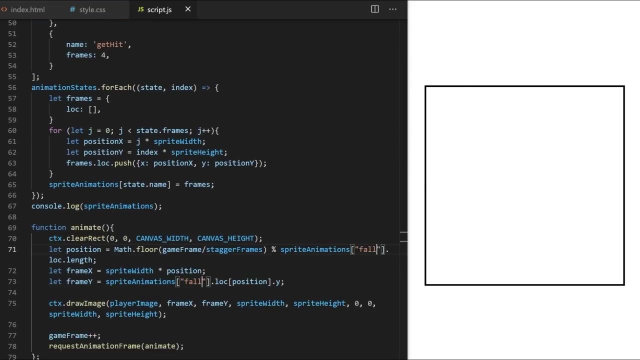 coordinate is tied to index in. for each method i add full animation with nine frames. run animation has nine frames, dizzy eleven frames, sit has only five frames, roll seven frames, and so on. i also need to make sure there is comma between every object. if i try fall, i get blink in. there must be an empty frame. fall animation is actually only seven frames. 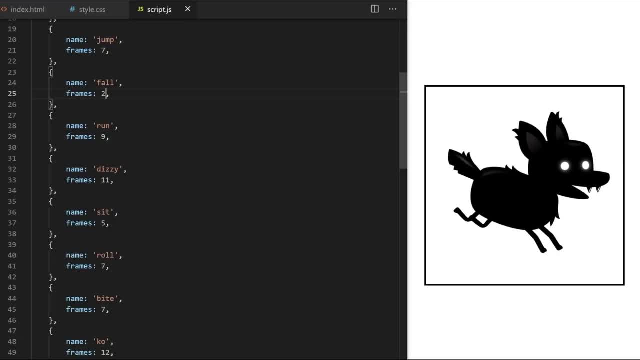 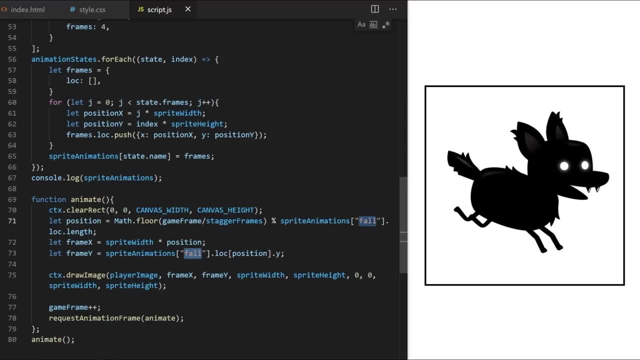 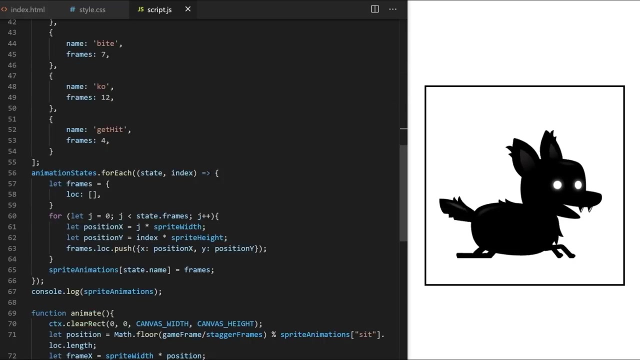 if i put less here, we play only part of animation. if i put more here, we get blinking because some frames are empty. run animation works, dizzy works, sit animation works as well. you can see: sit animation has five frames and dizzy animation has 11 frames, and i can swap between them easily without having to manually change number of frames. 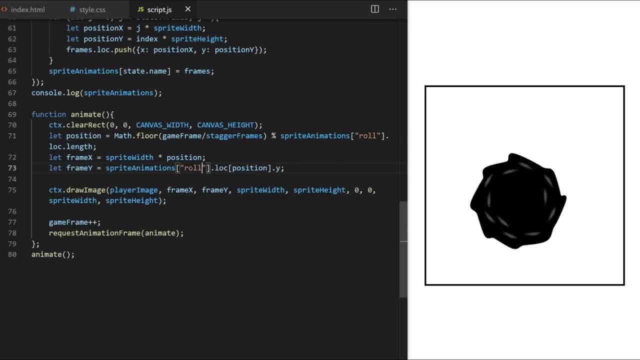 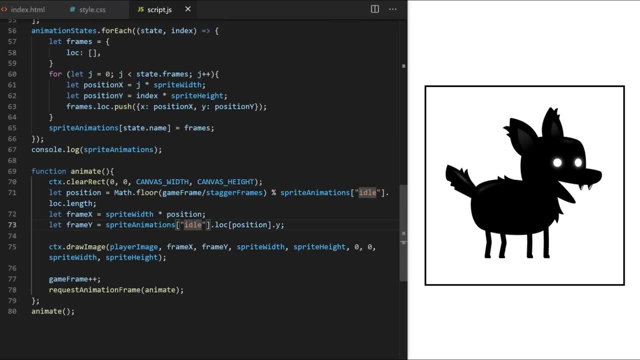 like we did before: roll animation works. byte animation works. let's go back to idle. put in hard-coded text here like. this is not ideal, of course. i go up to line 10 and i create a variable called player state. i select line 10 and i create a variable called player state. 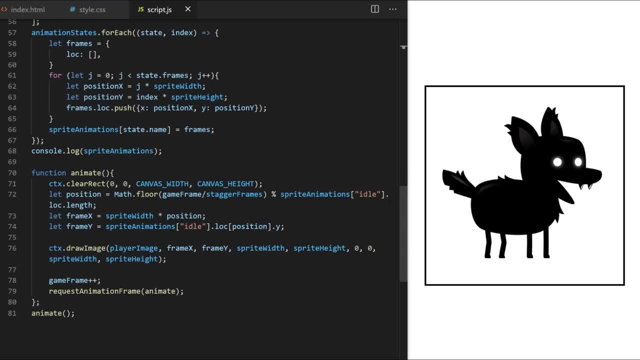 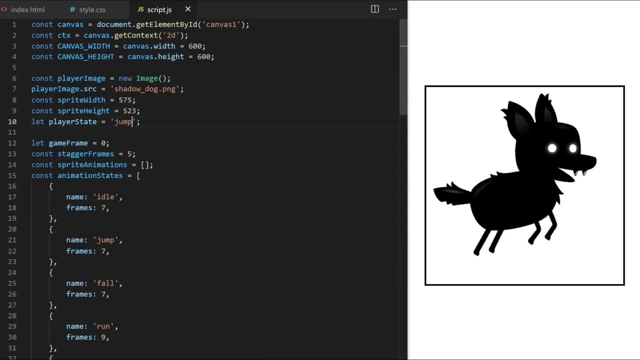 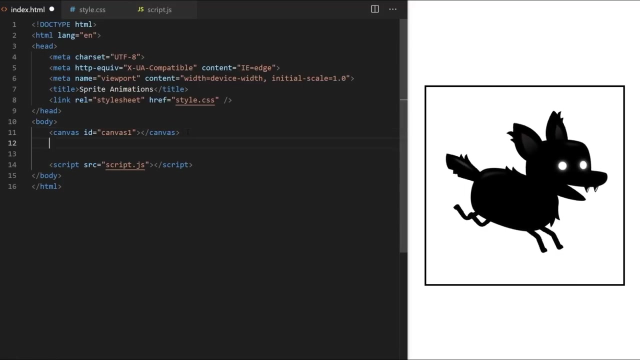 set it to run initially down. on line 71 and 73. i replace idle with this new player state variable. now i can swap between animations here on line 10.. sit works, jump works, fall works. in indexhtml i create a new div with a class of controls. inside there will be a select element. 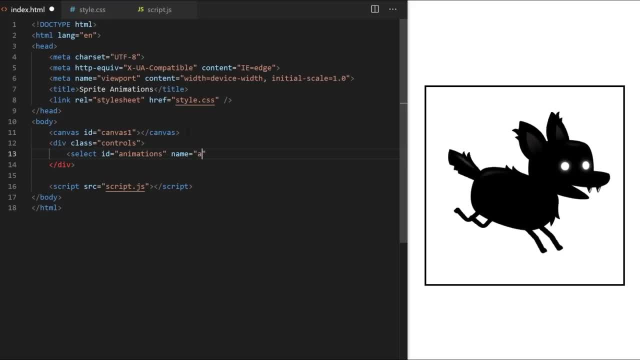 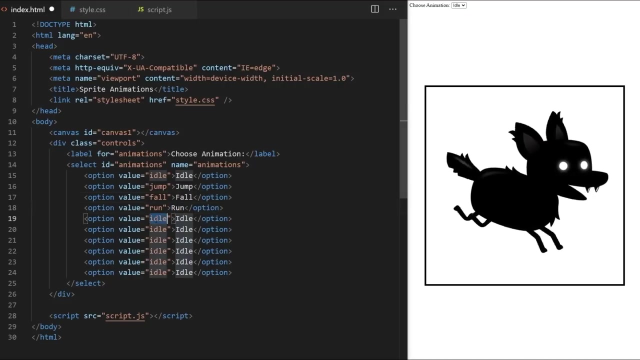 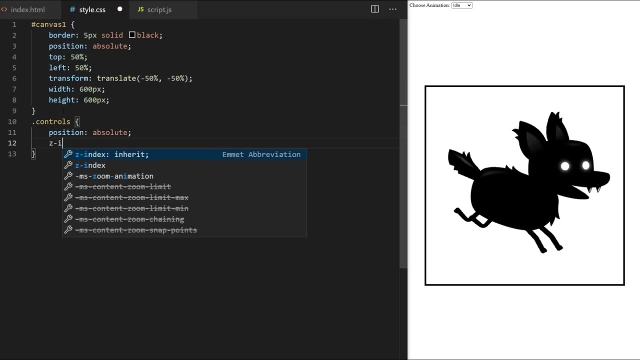 with an id of animations and name. animations label for animations will say: choose animation. i give it some options that match names we gave to animations in scriptjs file. in stylecss i target controls and i give it position: absolute z index: 10 top 50 pixels. 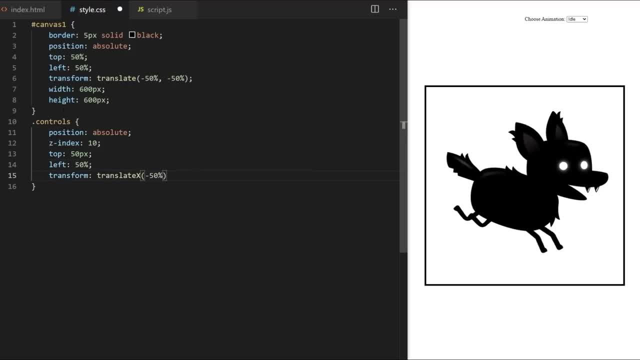 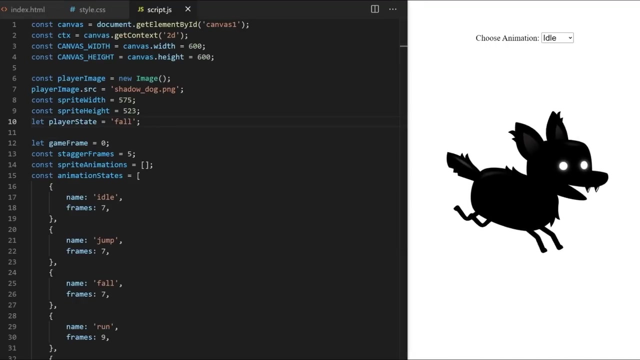 and transform: translate x minus 50 percent to center it horizontally. i take controls, select and option and i increase their font size to 25 pixels. i can also remove the border around my canvas. i want animations to change when i choose different value in this drop down in scriptjs. i take player state from line 10 and i put it up top on line 1.. 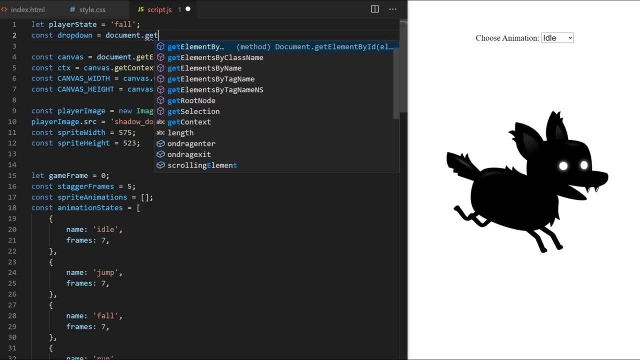 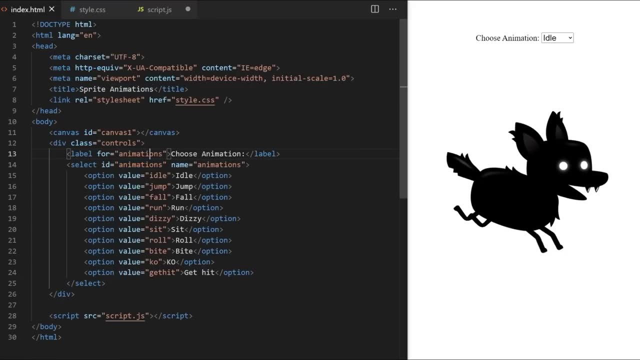 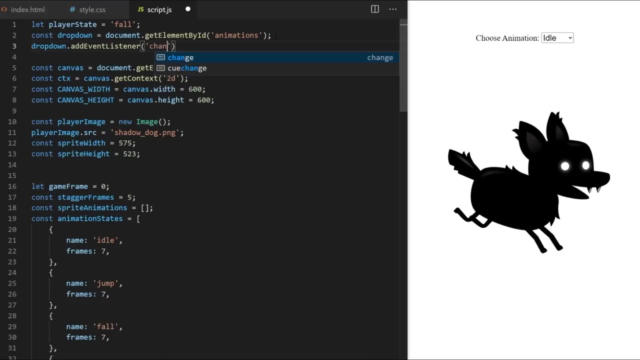 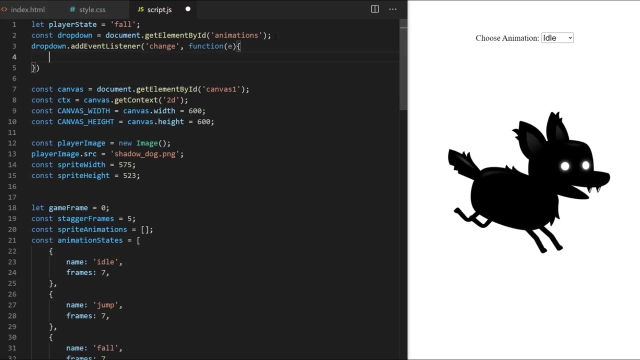 i create a constant variable called drop down and i point it towards this new select element with id of animations. i take drop down and call add event listener on it. i will listen for change event every time its value changes. we will take player state from line one and since we are inside, 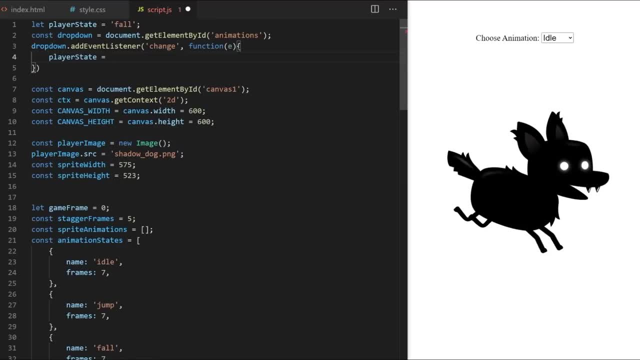 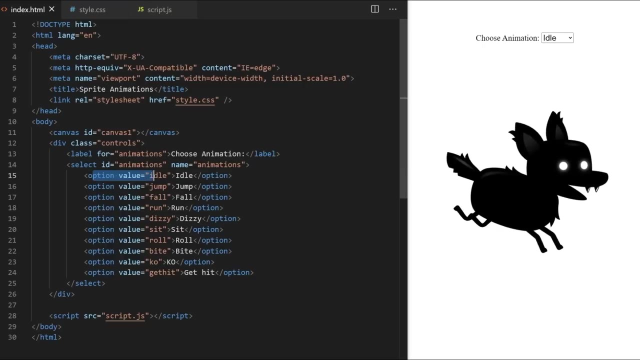 callback function on event listener. we have access to event object. i'm referring to it as e. event object has target property. target is simply referring to an element that was clicked and it has value property because i have added values myself whenever any of these option elements in my drop down is clicked. player. 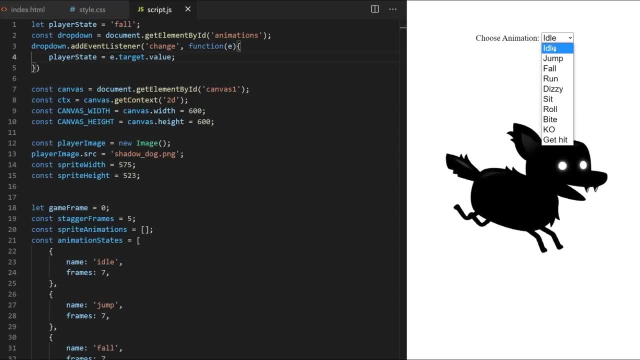 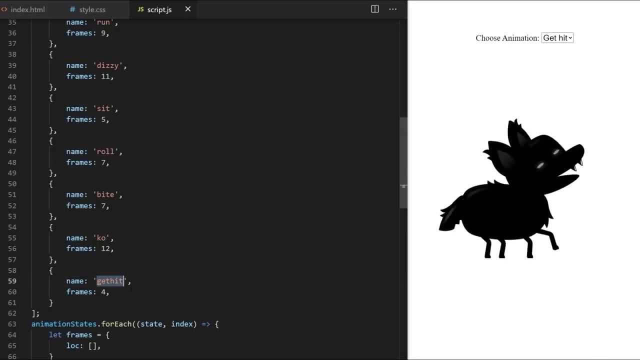 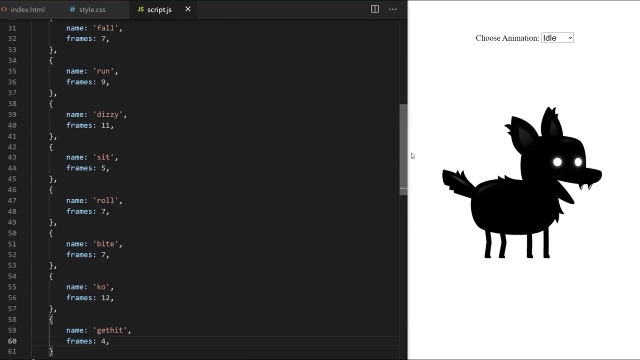 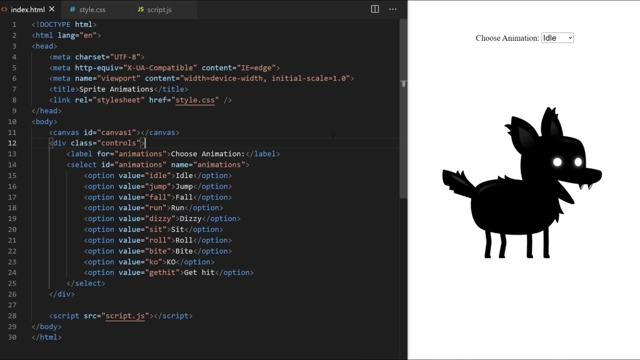 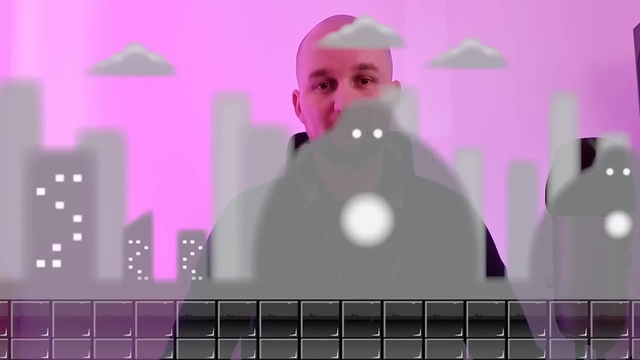 state variable will be set to its value attribute. now i can easily swap between different animations in my sprite sheet just by selecting different option in a drop down. so parallax scrolling is when background images move past the camera slower than the foreground, creating an illusion of depth in a 2d space. this is what my game looks without it. 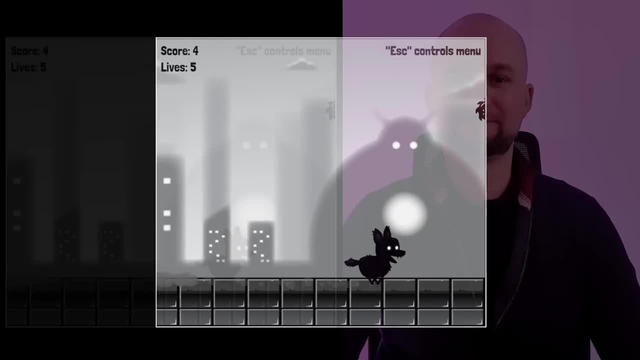 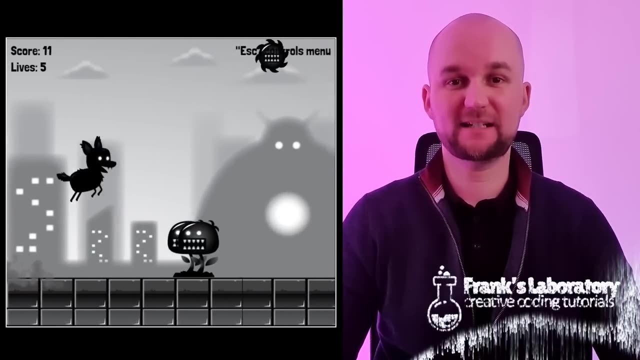 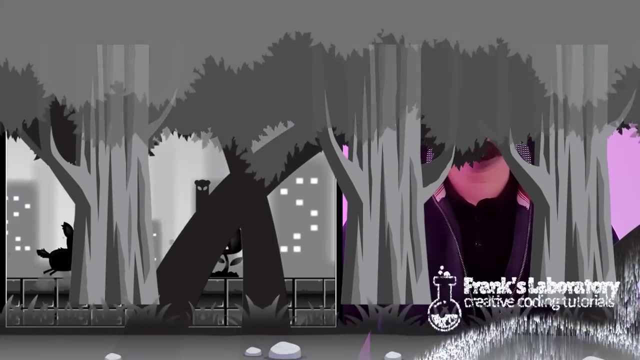 and this is what it looks with parallax. which one do you prefer? today we are learning about vanilla javascript game development for beginners, and by the end of this video, you will have deep understanding about endlessly scrolling backgrounds and how to add parallax effect to your games and websites when we have full control of. 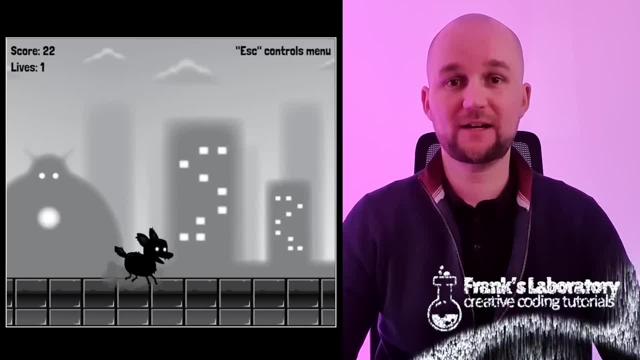 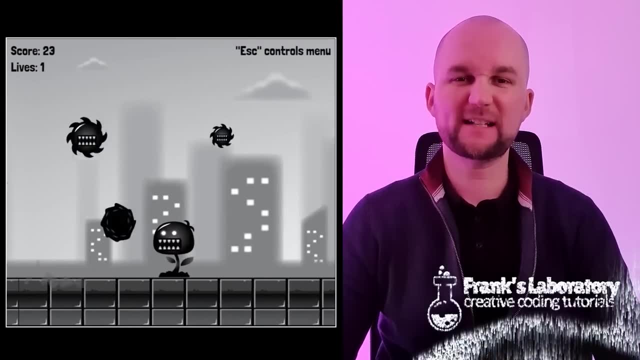 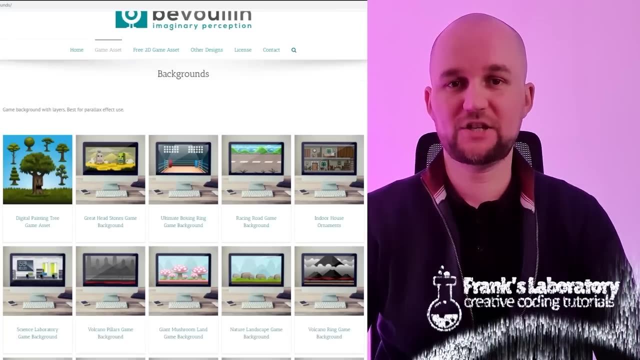 individual layers. we can match scroll speed to different actions our game character takes. for example, my dog character can sit down and the game stops moving, or it can do this rolling attack and the game speeds up. art assets for this episode were created by this amazing artist. check out their website for more. if 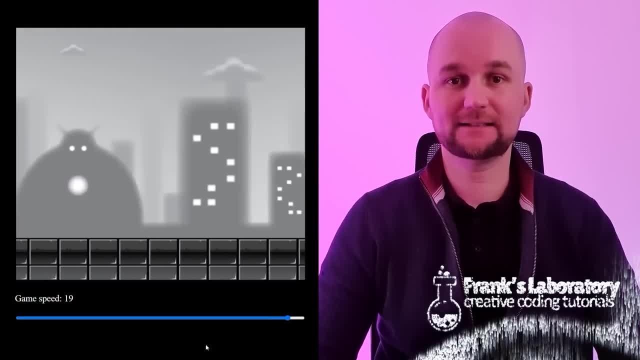 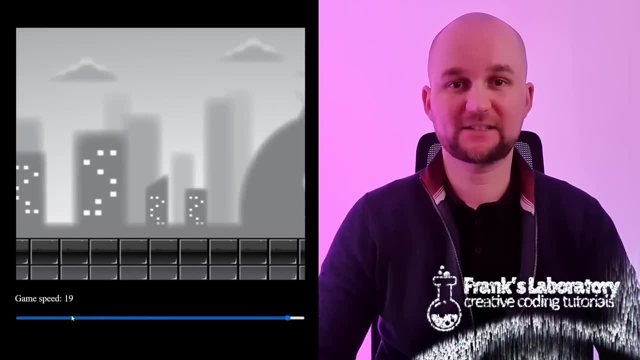 you want. what is the easiest way to create endlessly scrolling backgrounds? how to make different layers move at different speeds, to create parallax effect, how to make scroll speed dynamic so we can easily change it. we will learn all of that and more. let's bring our coding skills. 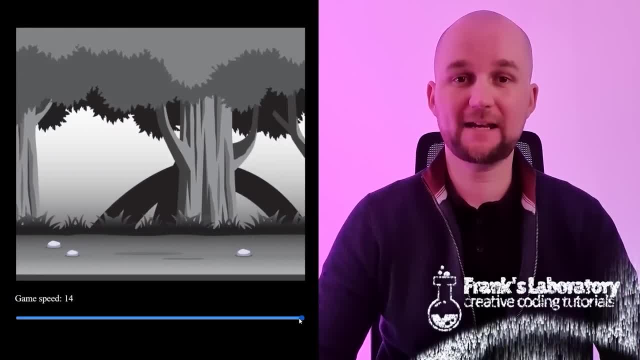 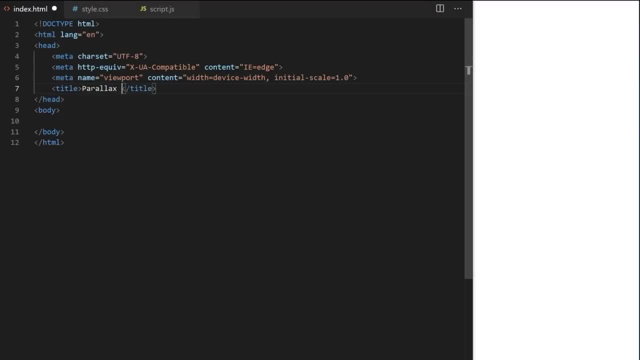 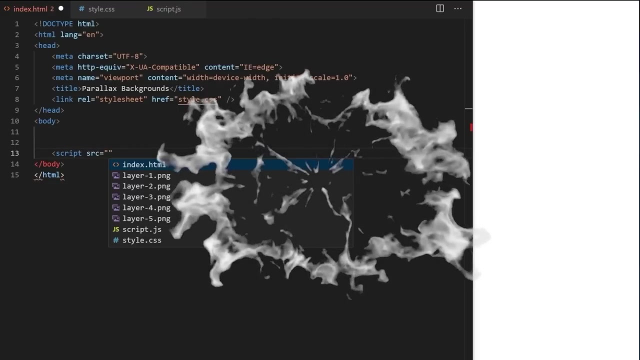 one step further today together and have some fun with plain vanilla javascript. this tutorial is for beginners. let's go click the like, please. i create a basic web page markup. in document head i use link tag to include my style css file. we will use it to position canvas. at the bottom of document body i place my script tag. 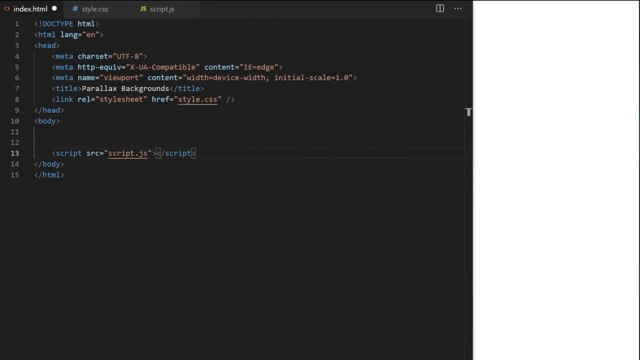 scriptjs file will contain all functionality and logic for our project. i also create html canvas element with an id of canvas1. it will be our main project area and we will draw on it with javascript in style css. i take body tag and i set its background to black. 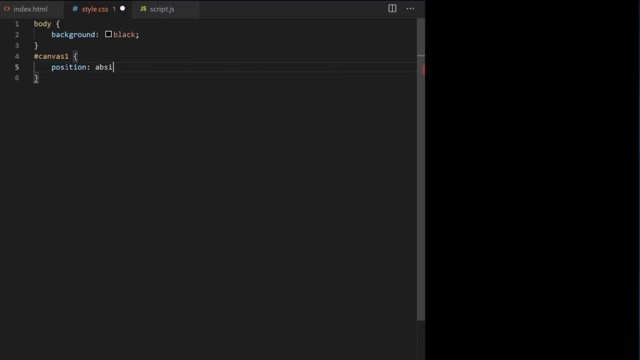 canvas will be set to position: absolute border: 3 pixels. solid white: width of 800 pixels. height: 700 pixels. i do transform, translate: minus 50 for x-axis and minus 50 for y-axis and then i offset top by 50 and left by 50 percent. this will center my canvas in the middle of the page. 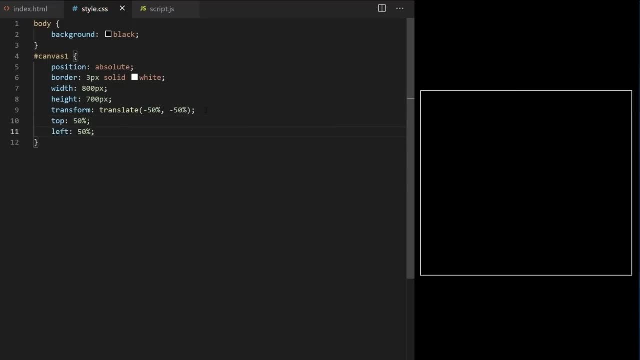 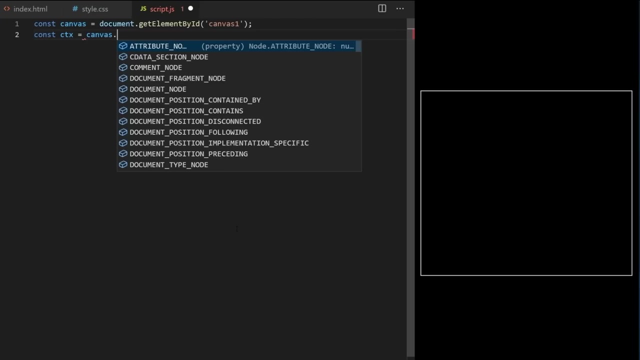 both vertically and horizontally. in scriptjs i create a custom variable called canvas and i point it towards my html canvas element by id: canvas1, ctx. shortcut for context will take this canvas variable from line 1 and it will call get context built-in method on it. get context can only. 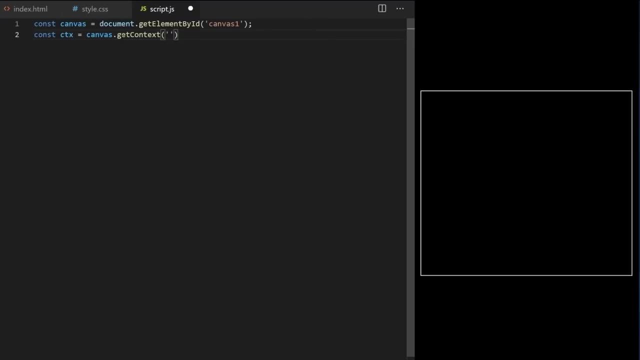 be called on a variable that holds a reference to canvas element and when I pass it argument that says 2d, it will create an instance of built-in canvas 2d api object that contains all properties and drawing methods we will need today. I need to make sure we have the correct. 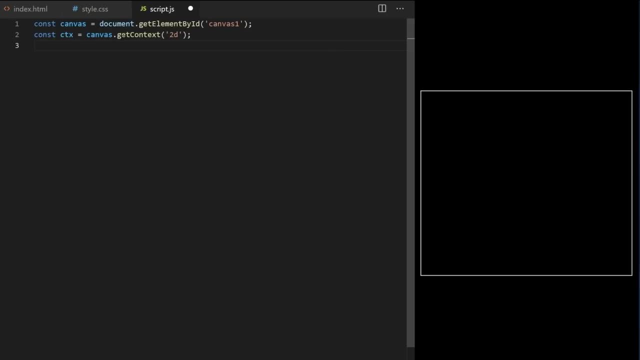 scaling because if you dot set canvas width and height it will default to 300 times 150 pixels. I create variable I call canvas underscore width, all capitals. to make it clear it's a global variable, I set it equal to canvas from line one dot width, which will access with attribute. 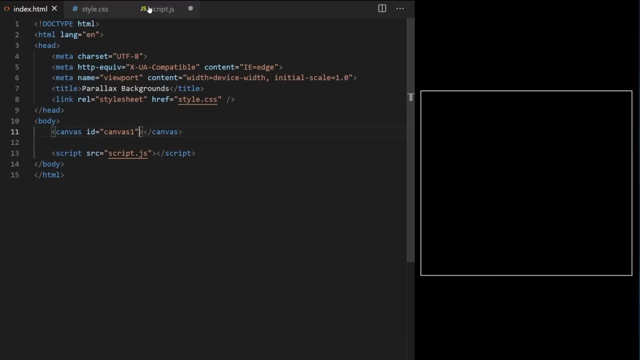 on html: canvas element we created in indexhtml and I set all to 800 pixels, The same value we give canvas width in stylecss. I do the same thing for height: canvas underscore height is equal to canvas dot height is equal to 700 pixels. This is how you set up most canvas projects. 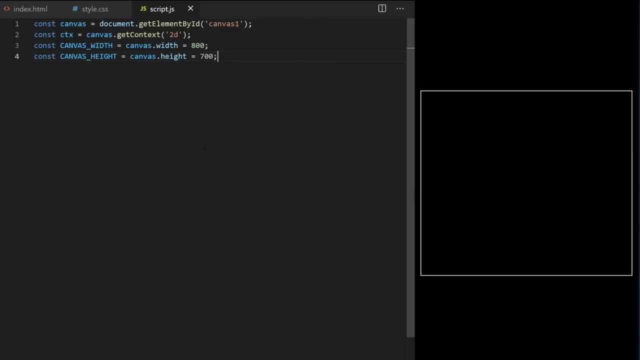 Now we need to make sure we have the correct scaling. We need to make sure we have the correct scaling. We have our drawing board ready and we can focus on built-in parallax effect. I want the scroll speed to be dynamic, tied to a variable, so that in our game we can speed up or 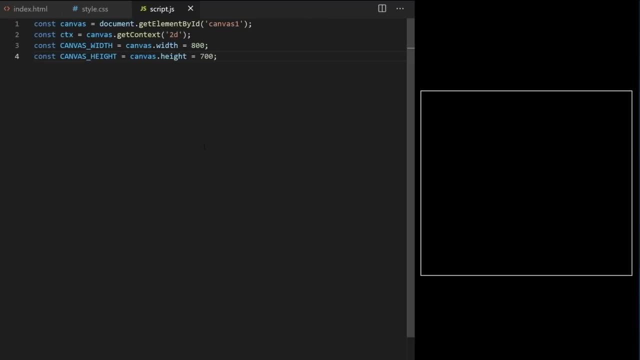 slow down using special moves with our character To control scrolling speed. I will declare a global variable called the game speed and I will initially set it to, for example, five. Notice: I didn't use const keyword here, I used let Let keyword in javascript is used to declare variables that. 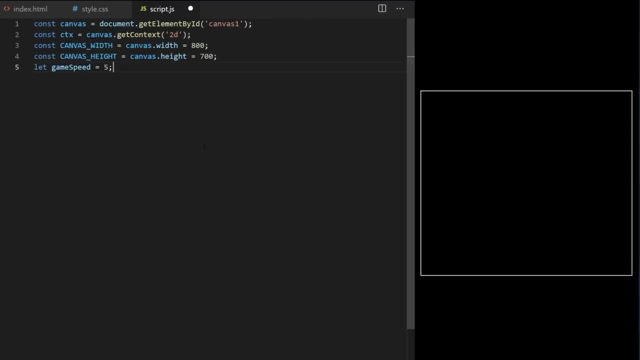 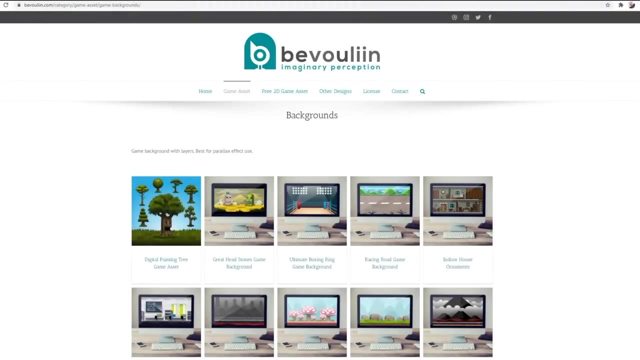 can be reassigned to different values later. I will not use const keyword here. I will use let. I will need this to be able to dynamically change scrolling speed. It's time to bring images to the project. Art for this episode was created by this artist. 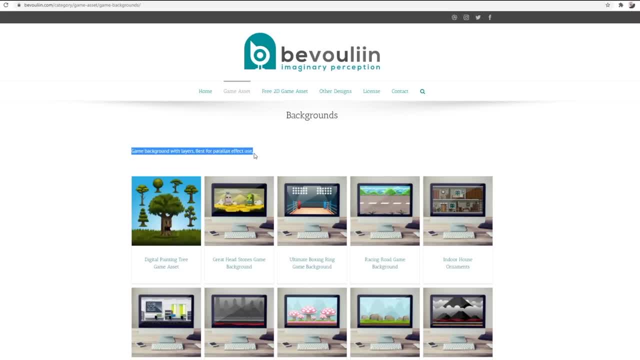 I really like his art style. You can download them in the video description. You can use these images for learning purposes. For commercial projects you will have to purchase a full license from his website. This effect will also work with any other image, but maybe you first. 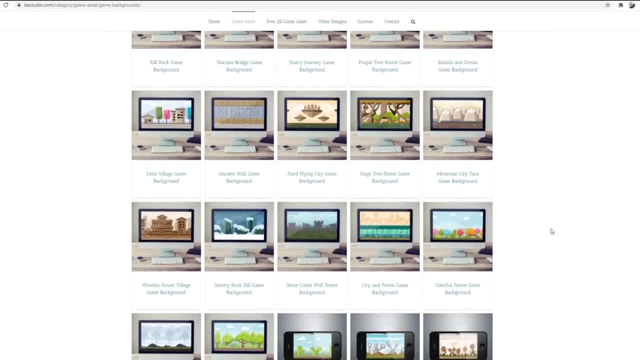 want to use the same files I'm using so that you get the same result and don't have to worry about calculating different values. I'm going to create a new image. I'm going to create a new image, I'm going to name the image, I'm going to set it to plus and I'm going to add the image to this. 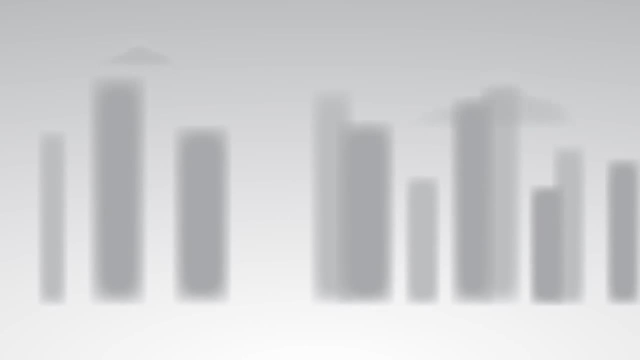 image. so I'm going to put it to full loading, I'll add the images and then I'm going to add a new image and then I'll add a new one. Once you fully understand the code from today's lesson, it will be easy to switch the images and adjust values so that the code base works with your own. 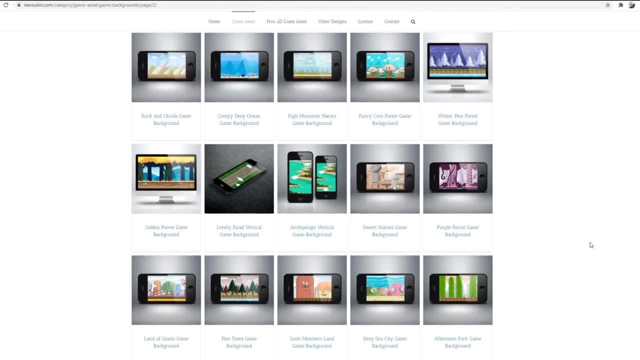 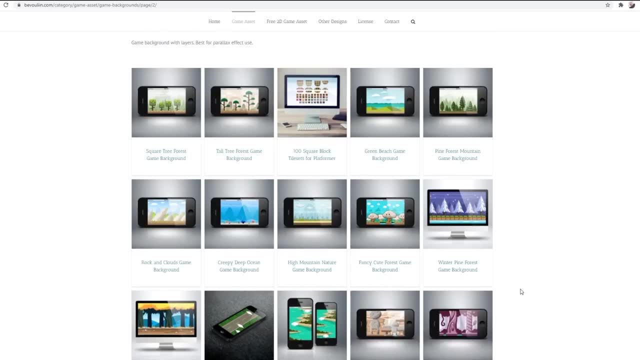 files. The images are very large. If you experience any lagging or frame drops, making images smaller will significantly improve performance. I kept them large on purpose so that we get nice clean visuals, but especially if you are creating a mobile game, these images can be much smaller. 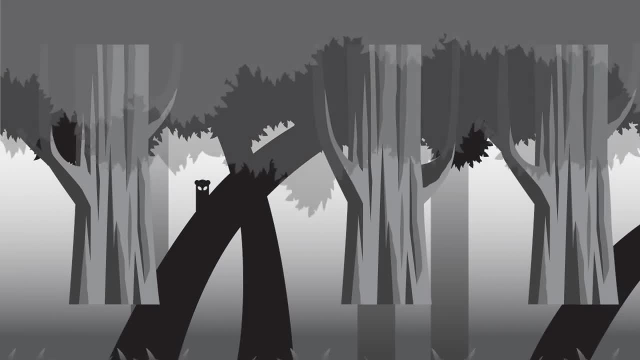 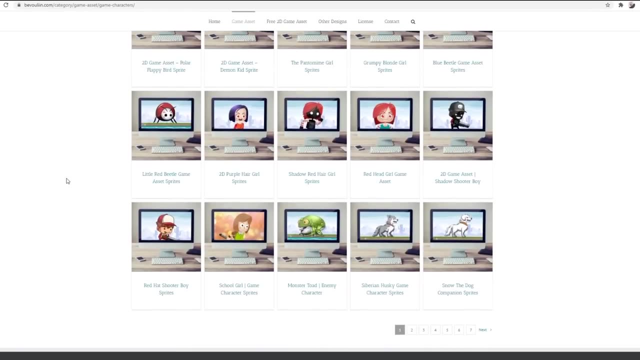 You can download the project files in the video description. Our background will have five layers. It is perfect to demonstrate seamless parallax scrolling for games. This is one of my favorite 2D game artists. If you want, you can go and check out his website. 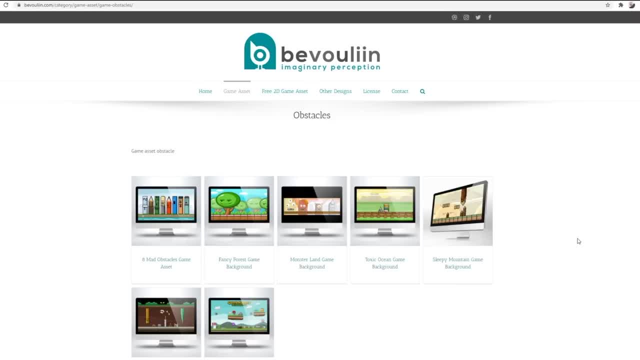 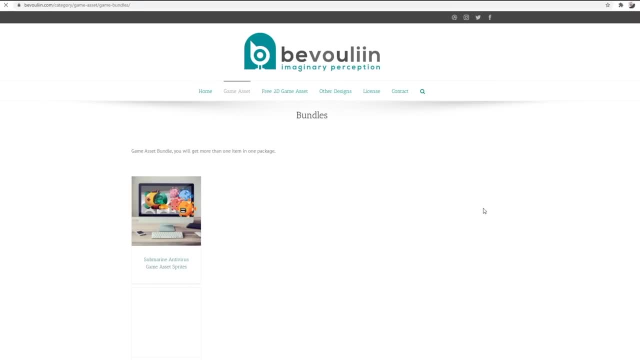 I will leave a link in the video description. He offers some free art assets you can play with and use in your games, but if you want something a bit more special, his prices are very affordable. There aren't many 2D game artists out there, so if you can help me out to support them and buy some, 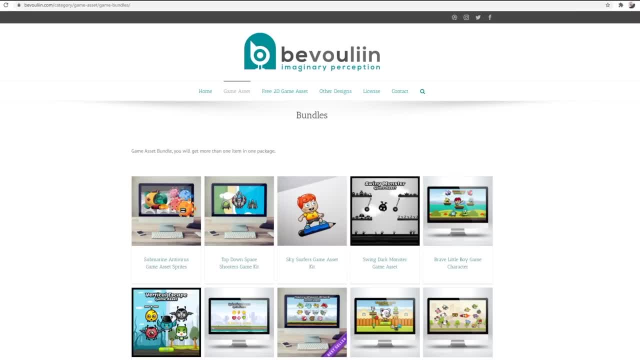 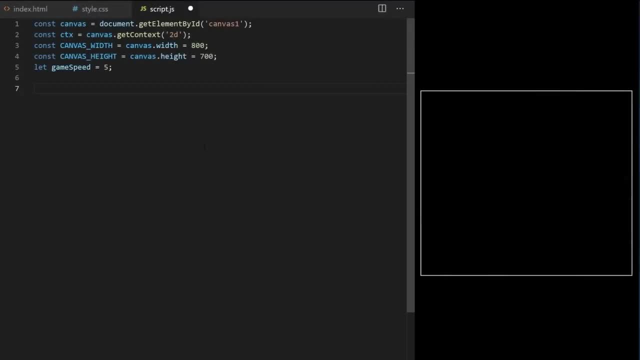 of their assets for your projects. it will help us to make our games unique and by purchasing from and supporting our artists, they can make more beautiful game assets for us. To bring image into our canvas project is very simple with javascript. I create a constant variable called background layer1 and I set it equal to new image. This is 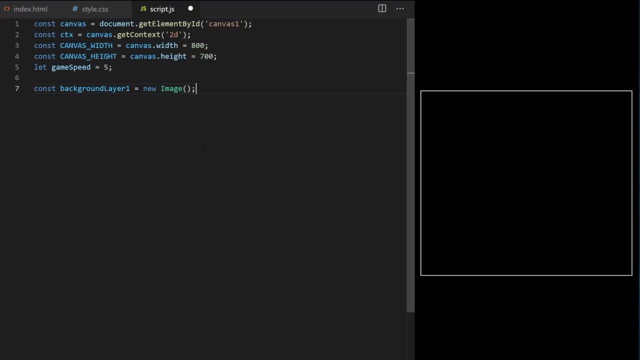 built in image class constructor. It simply creates an image element. We can use append child built in javascript method and it would look like this: This is the image class constructor. It simply creates an image element. We can use a pent child built in javascript method and it would. 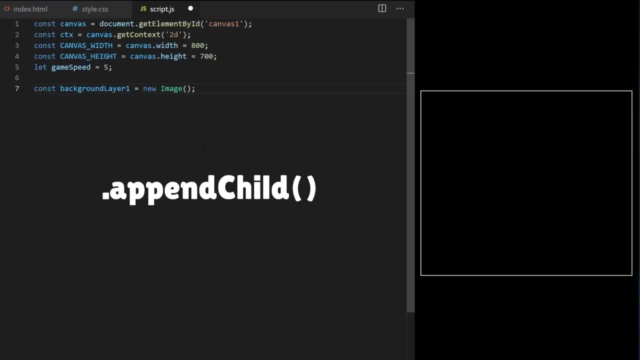 slot image tag- img tag- into our html file, same as if we wrote that tag in index html ourselves. We can also choose not to append it and it will stay hidden and it will just store the image for us. Image constructor has the same functionality as the document dot create element img. 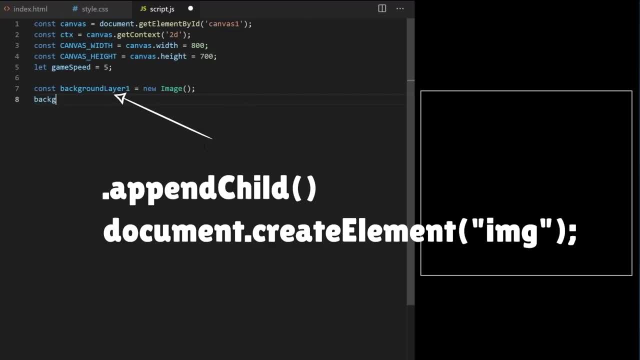 We are simply creating html image element and saving it in this variable. At first, that image element is blank, so I access its source property and I set it equal to layer-1 dot png. For you, the path might be different depending on how you structured your. 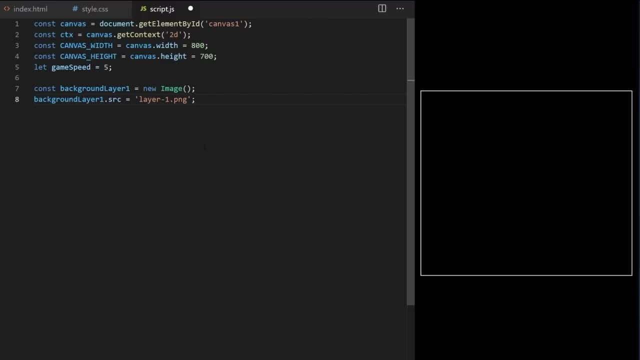 project files and folders. I left my image files in the same folder with my script file. for now We have five layers, five different images, so let's do the same thing for all of them. to bring them into the project. Let's create animation loop. I create a custom function called, for example, animate. It will 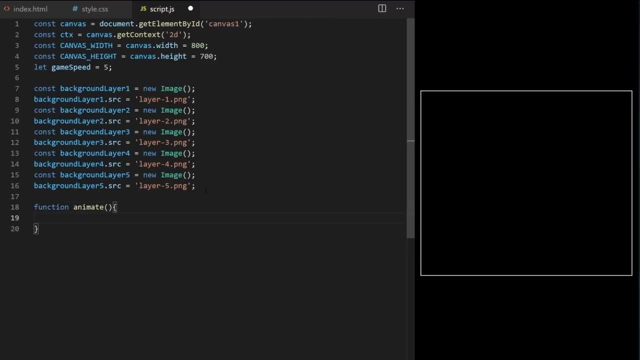 contain all the code. I create a custom function called, for example, animate. It will contain all the code code I need to draw my backgrounds. I will be calling it over and over to create animation. Let's start by calling ctxdrawImage built-in canvas method. This method will take image and 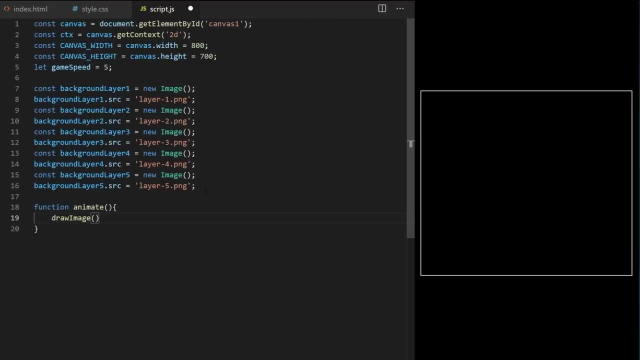 it will draw it on canvas. The first argument I pass it is the image I want to draw. so background layer 1 from line 7.. I want to draw it at coordinates 0, 0, so from the top left corner of canvas. 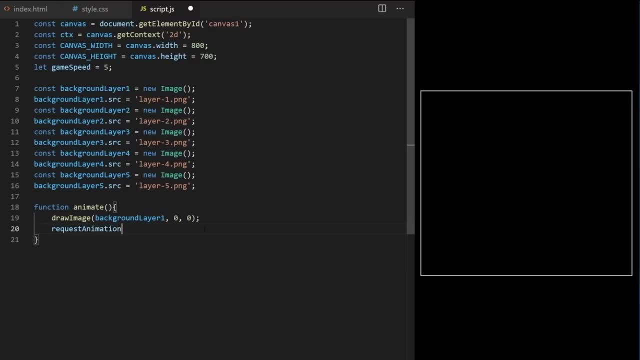 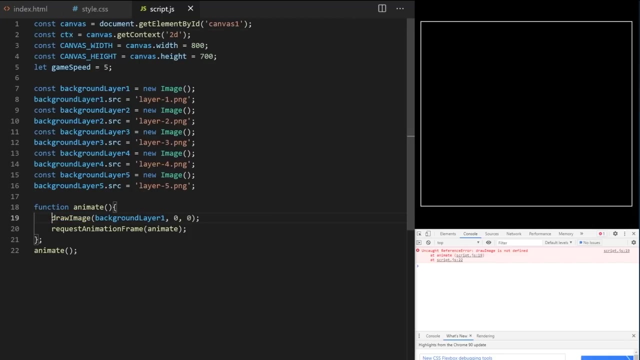 Then I call built-in requestAnimationFrame function and I pass it animate the name of its parent function from line 18.. This way, animate will run over and over creating my animation loop. On line 19 I need to call drawImage from my ctx variable from line 2.. Background layer 1 image. 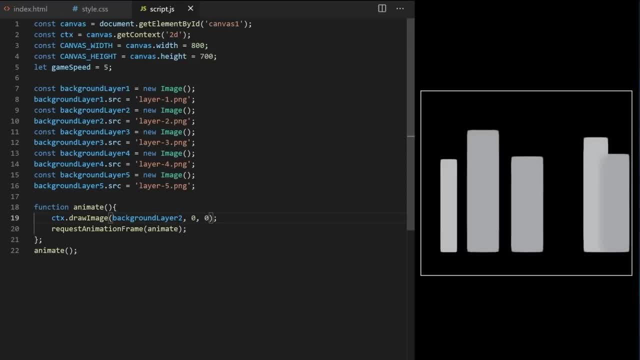 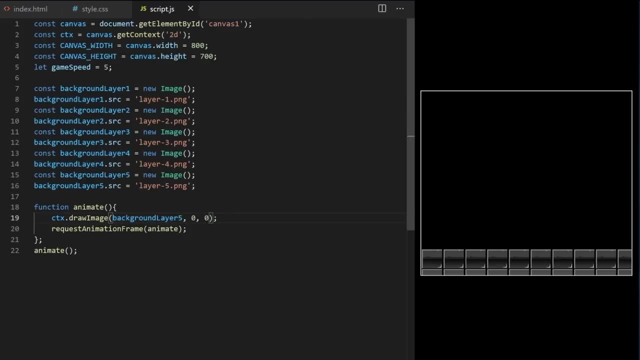 is not the best one to use as an example. Let's try layer 2,, layer 3, 4, 5.. Let's do this at first with layer 4 to see exactly what's going on, and then we can throw in. 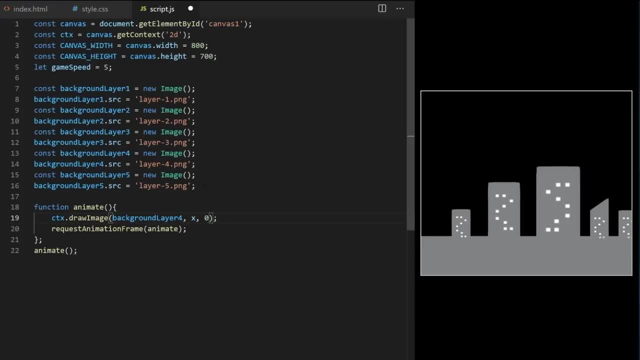 all the other layers It looks like a static image, but it's actually animating over and over. Let me show you. On line 18, I create a variable called x and I set it to 0.. On line 21, inside drawImage: 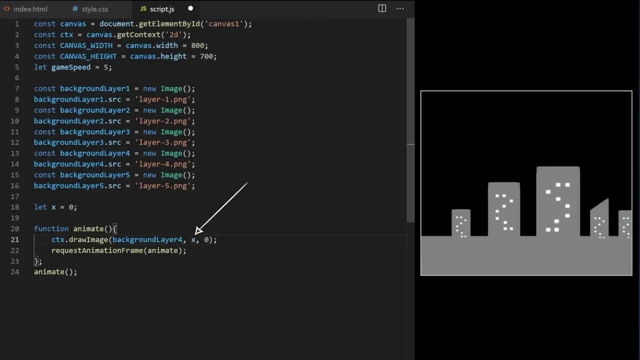 method. I replace hardcoded 0 with this x variable and every time animation loop runs, I decrease x by 1.. This will make our image move to the left In negative direction on horizontal x-axis. The reason the image is being smudged like this is: 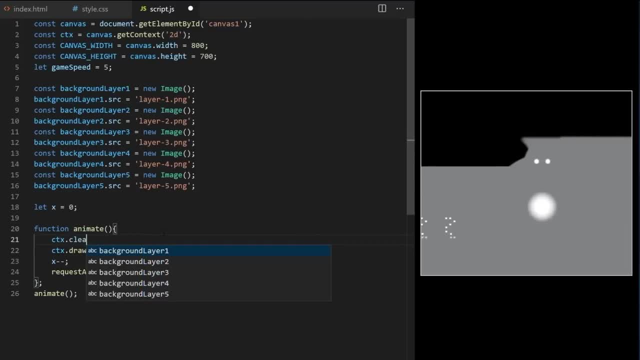 because we can see all previous frames. We can see old paint. If we want to see only the current animation frame, we need to delete old paint. I use built-in clearRectangle method. It expects four arguments to determine what part of canvas I want to delete. I want to clear the entire canvas. 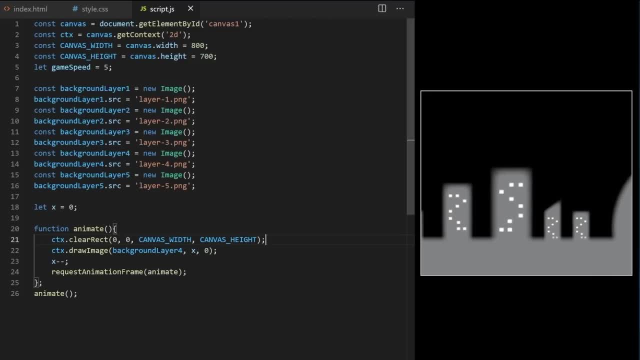 so from coordinates 0, 0 to canvas width, canvas height. Now old paint is being deleted and we can only see the current animation. frame Image is moving to the left by one pixel per frame. On line 5 we declared gameSpeed variable. so down here on line 23 I can say x minus equals gameSpeed. 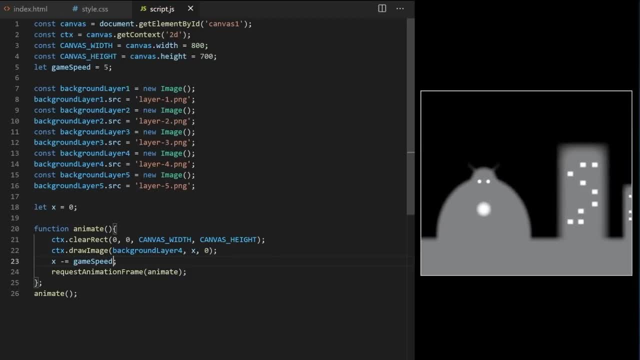 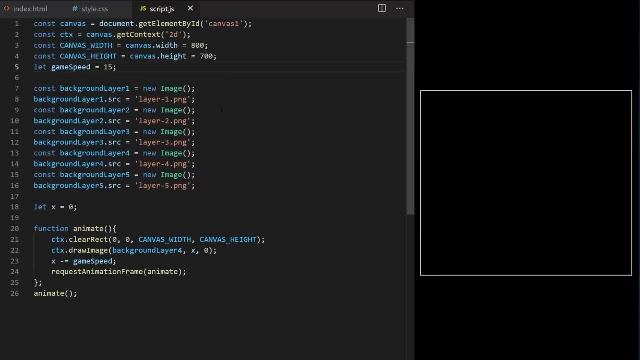 and now scrolling of our game is attached to this gameSpeed variable. If I do 15, it moves much faster. As you can see, the background just moves endlessly to the left and eventually it leaves canvas empty. These images were specifically crafted for endlessly scrolling. 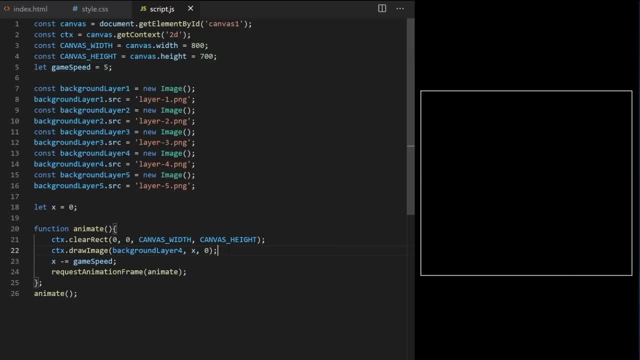 games and they are seamless. It means you can stack them next to each other and it will look like it's one repeating image. I need to somehow detect when my image has moved off screen and I need to reset it so it can scroll again. Let's try it. What if I say: if x is less than? 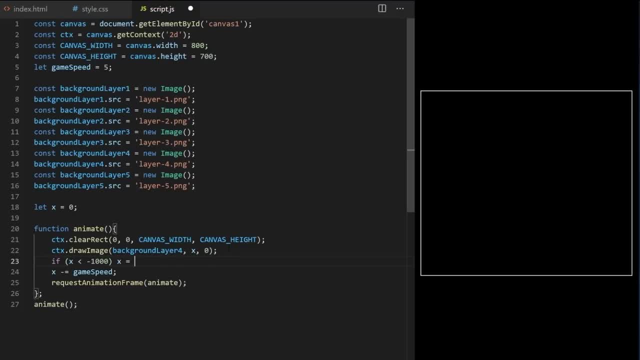 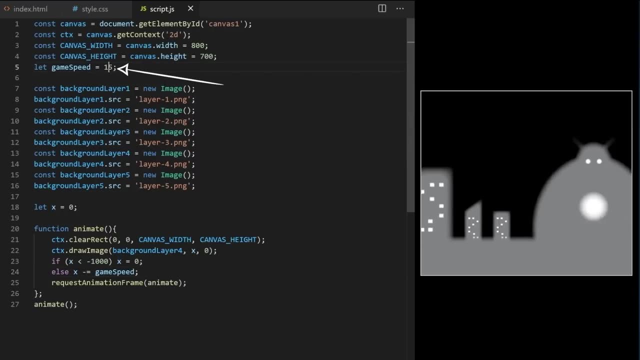 minus thousand pixels. set it back to zero, else diminishes gameSpeed minus. I increase gameSpeed to 15 here on line 5.. I increase gameSpeed to 15 here on line 5.. You can see the image is resetting, but we can clearly see the jump when the reset happens. Let's try 1600 on line 23.. 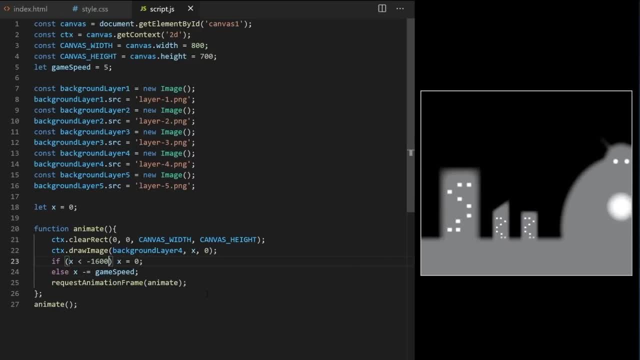 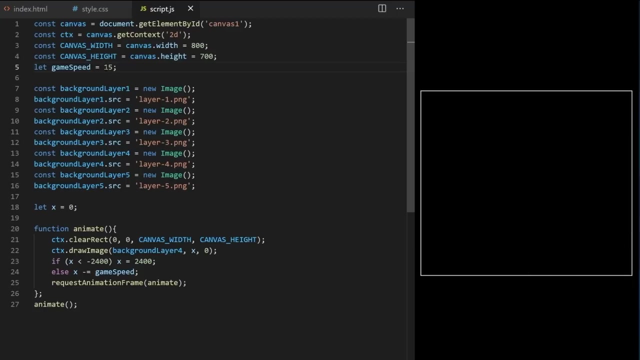 Still it jumps. I know that images we are using today are 2400 pixels wide, so what if I use 2400 pixels here And I also reset X to 2400.. Now we have this image that is 2400 pixels wide, scrolling endlessly over the. 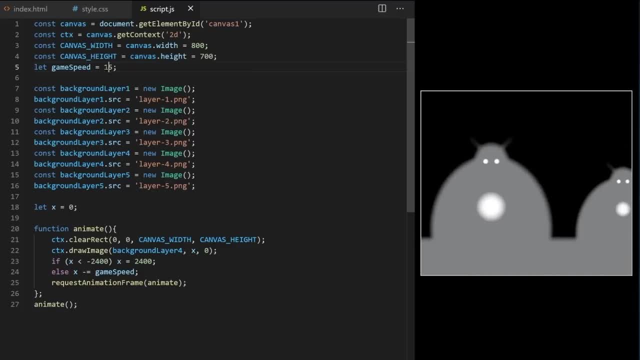 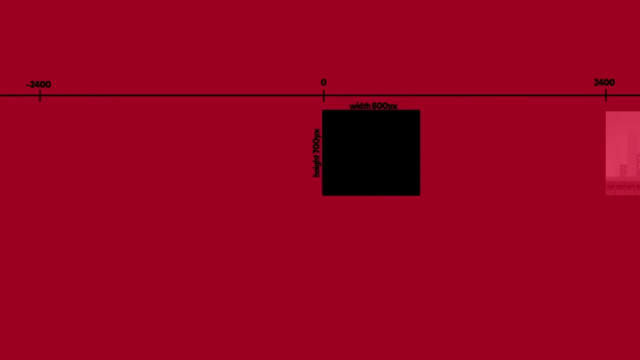 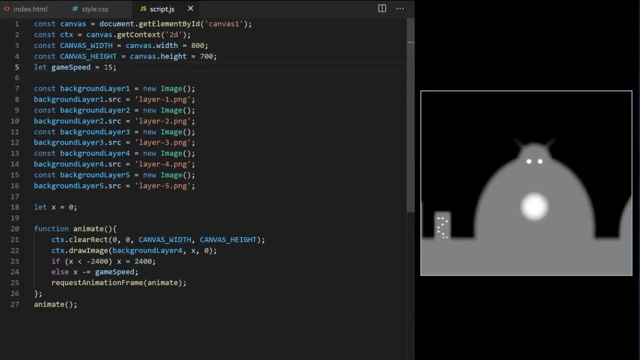 canvas And there is this black empty space that is also 2400 pixels wide. The trick people use is to simply draw the same image twice and always reset the one that has moved off screen so that it's available to scroll again and canvas is never empty. I will show you exactly what's going on using two 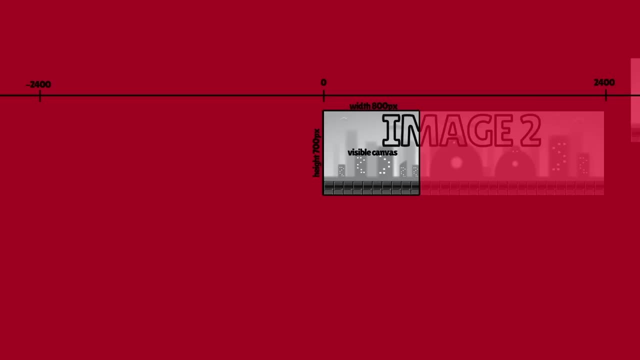 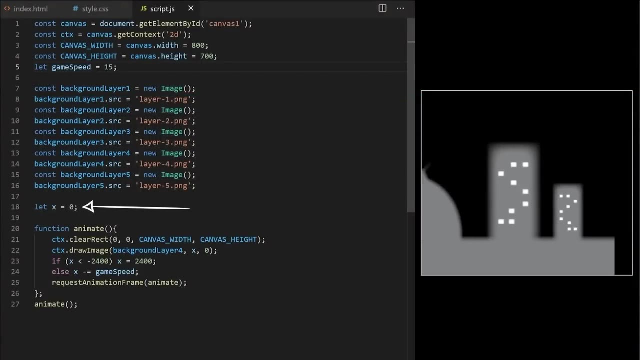 separate X variables, one for each image, and then we will optimize it once we fully understand what's going on. On line 18, I have X variable which will serve as a horizontal position for one of my background images. I will create a variable I call, for example, X2.. That's. 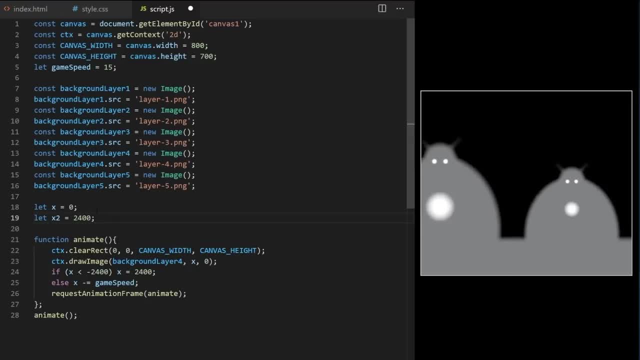 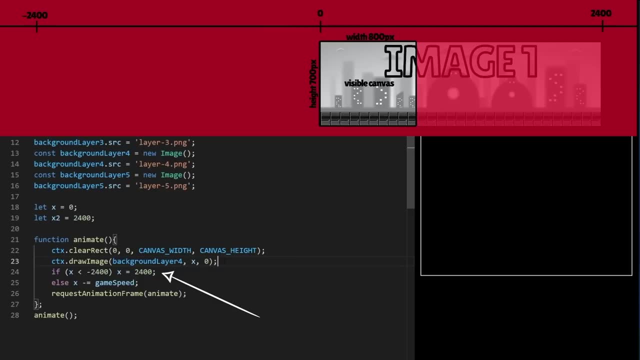 for the position of my second identical image. X will start at position zero and on lines 24 and 25, I have my reset checks to make sure it cycles around endlessly. X2 will start where the first image ends, Since my images are 2400. 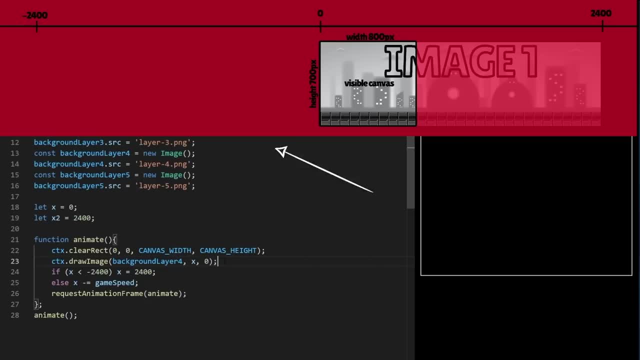 pixels wide. X2 will be 2400 and 2425.. 2400. Images we are using today are very large. You might experience frame drops and lagging. If you do, you can make them smaller, but maybe, if you can just follow along with me, 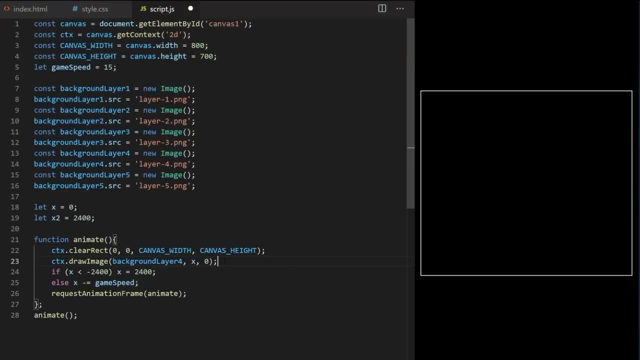 till the end and then refactor your code and image files for performance, just to make sure we are looking at the same numbers at first. It makes it easier for you to debug your code if it's the same as mine. Once you fully understand this technique, you can use. 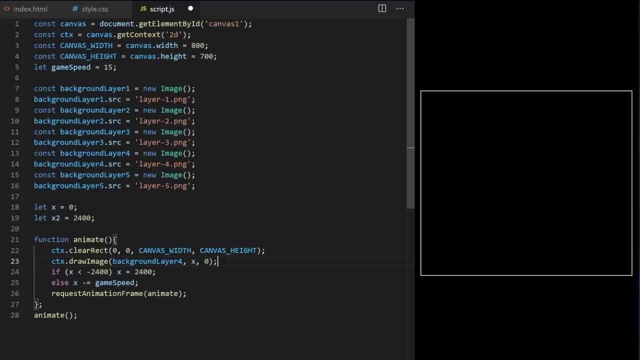 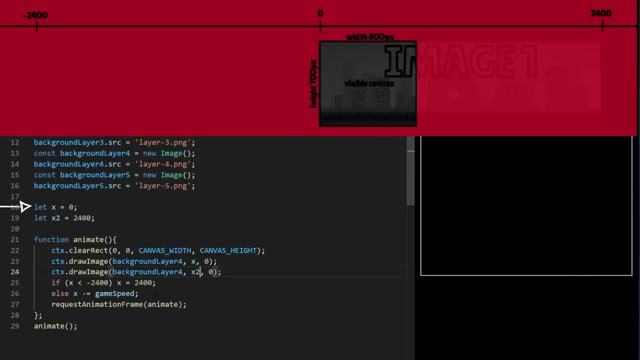 it for any image size and any scroll direction your game needs. On line 24, I just call drawImage, again for the same identical image, but instead of drawing it at position X from line 18,, we will draw it at position X2 from line 19,, like this: 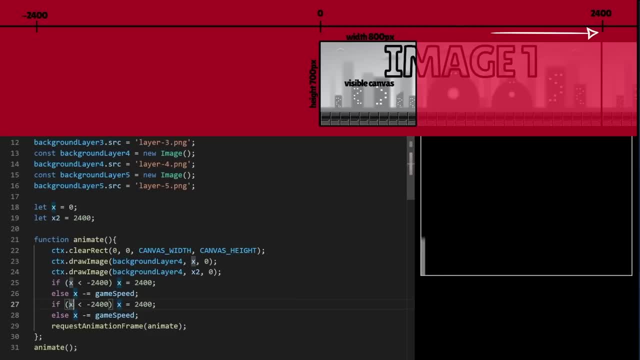 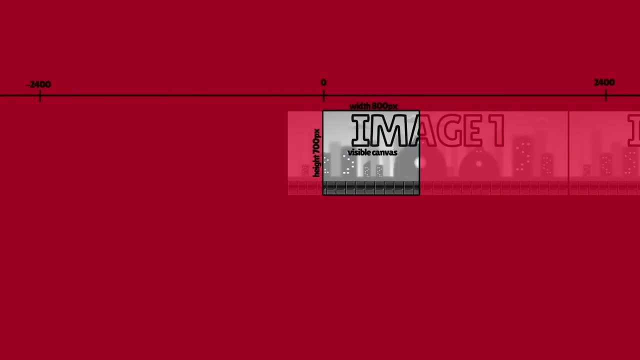 I also need to reset X2 the same way I am resetting X. This is so-called spaghetti code. We have some code repetition here and it doesn't look very clean yet. I'm just doing it for complete clarity, to show you what's going on. We will refactor it later. 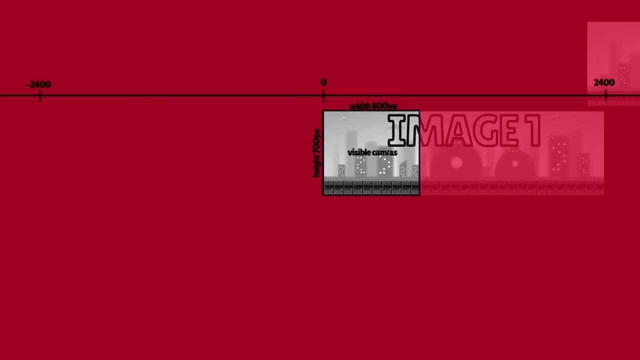 You will notice we have one problem when we do it this way, but don't worry, we will optimize it and fix everything. I want even beginners to understand. Now I can see some frame drops because my images are large, but I only see. 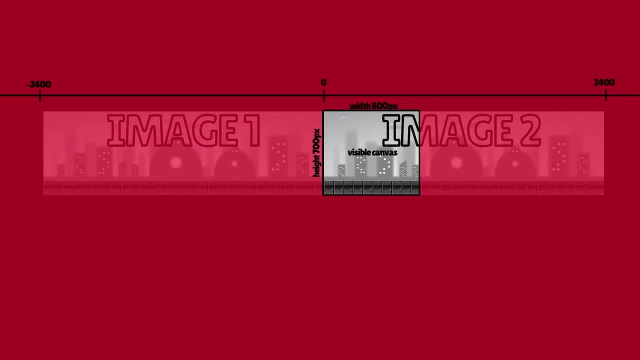 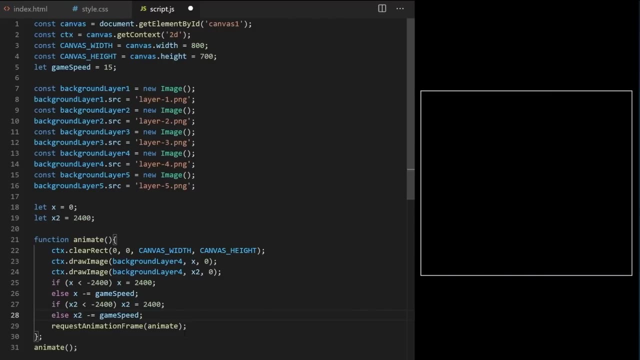 it on my screen recording software. it still runs smooth in my browser. Don't worry about the frame drops at this stage. it can be easily fixed by making our images smaller. Let's focus on the code first and make sure we understand it. You might notice there is a gap between. 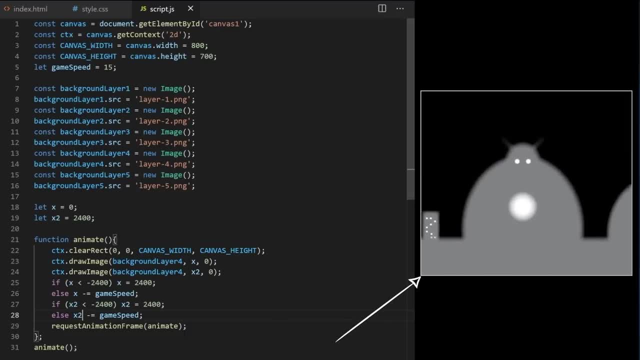 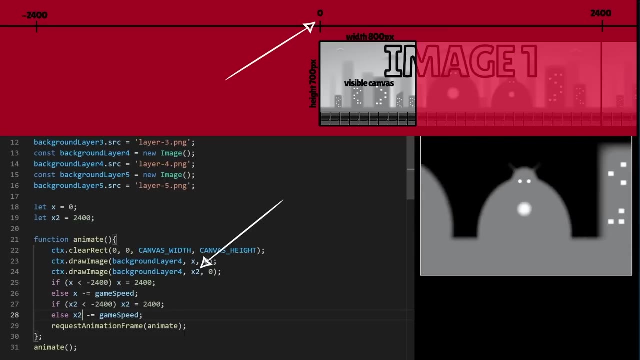 my images. What's happening now? I have image 1 drawn at position X from line 18 and I have image 2 drawn at position X2 from line 19.. The problem with this technique is that my images ignore each other. They reset based. 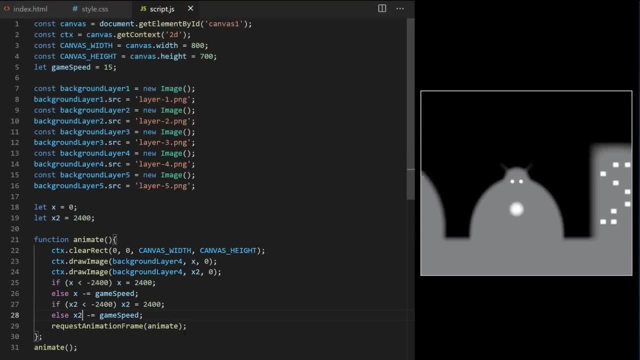 on two different variables, X and X2.. These variables are completely disconnected. so if width of my image is not divisible by gamespeed variable, it can actually happen that this gap will be invisible, or I will be able to spot it or at least not be discrediting. that We can avoid those mistakes and irregularly freely test. 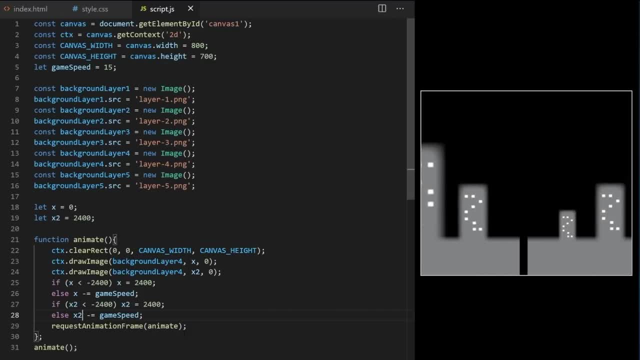 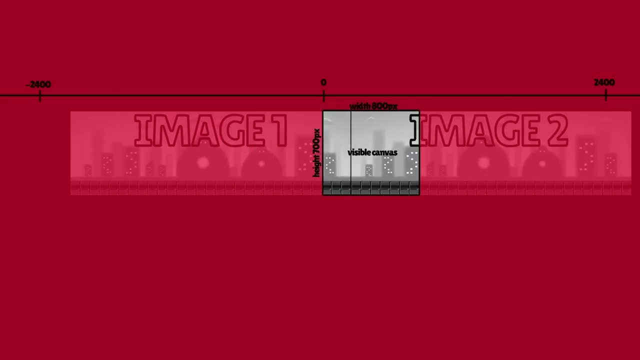 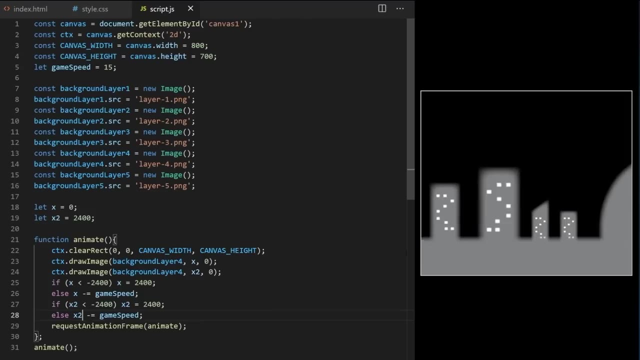 between images will grow larger or smaller over time, and we really don't want that. We want endlessly scrolling, seamless background. Let's deal with it step by step. So what's this gap between my images? Why is it there and how do I offset my images to get rid of it? Part of the gap is my game speed, because 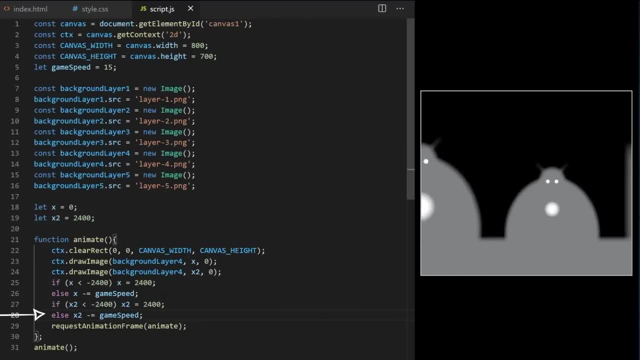 these if statements that reset X and X2 happen independently of each other. We have situations where X resets and X2 will move 15 pixels to the left for that frame- 15 pixels, because that's what my game speed variable is set to on line 5. 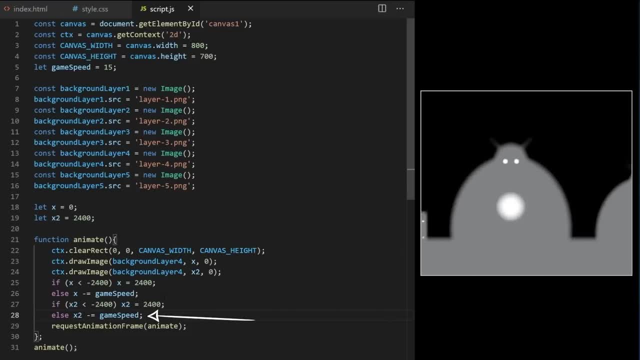 at the moment They never reset at the same time because one of them is always visible on canvas. So when X resets, image 1 resets on line 25, or when X2, image 2 resets on line 27, I need to offset the other one by the amount of game speed to 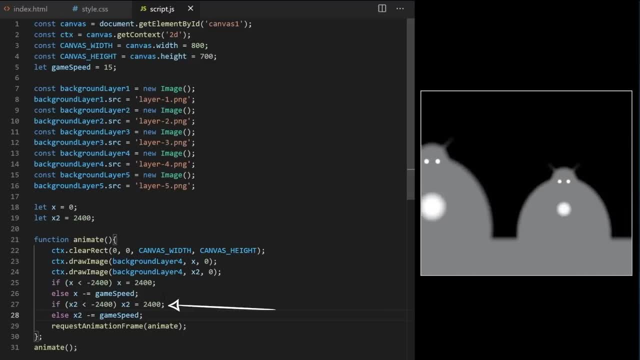 account for the fact that for that frame the other image kept moving while the other one was resetting. Gap is smaller now but there is still a gap. Game speed is 15 pixels per frame and my images reset when their X position is less than minus 2400.. So unless 2400. 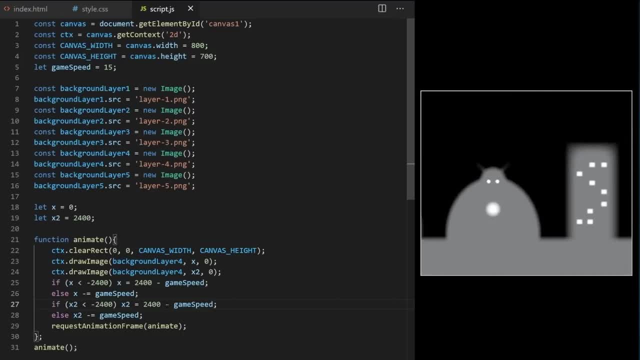 which is my image width, is divisible by the current speed, with no remainder. there will always be some leftover pixels creating a gap. This gap could even grow larger and larger as the scrolling and resetting continues. Some people deal with it by only allowing their game speed to be certain values, so 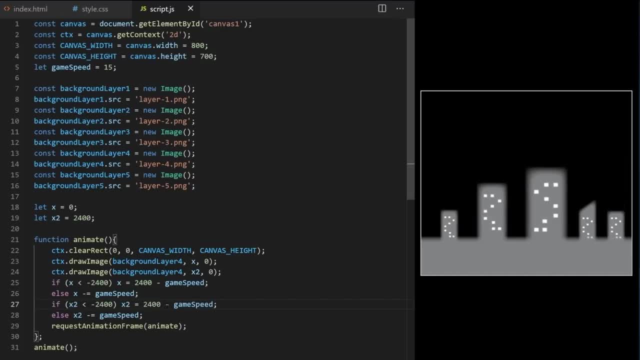 that image width is always divisible by game speed without any remainder. But we don't want this limitation. We want our game speed to be fully dynamic. Maybe you want your game to slowly go faster and faster as player progresses to more and more difficult levels, Or maybe you want to have special moves in your game and 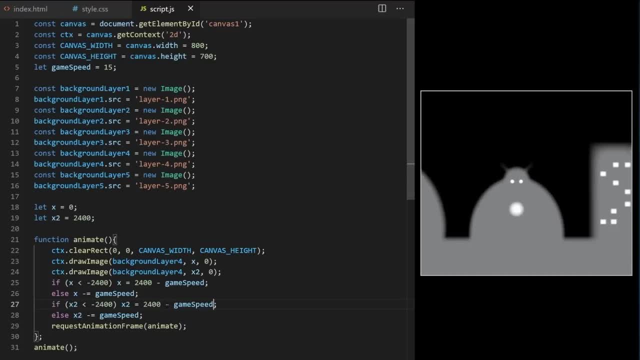 when player performs these moves, you want them to affect speed of scrolling, like I do here. So I'll show you how to do this with this roll attack, for example. To do this, we just need to make sure that our X and X2 reset statements. check position of the other image. 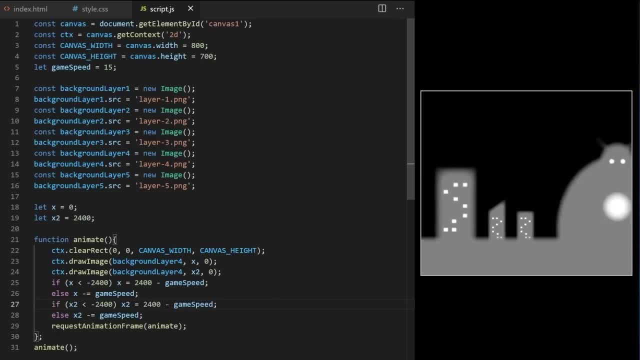 before they reset and they offset its new position based on the current position of the other image. That way, even when gap is somehow created, it auto corrects itself next time around during the next reset. I do it by accounting for the current X2 position. 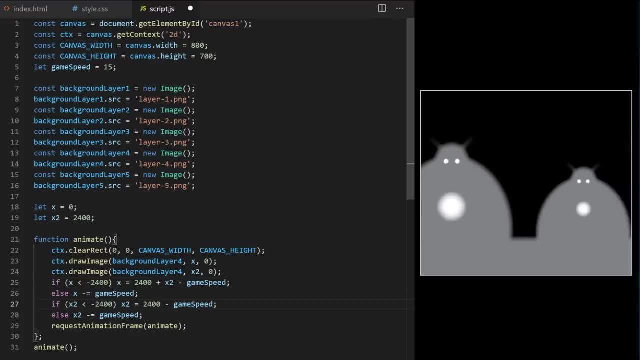 in my X reset check on line 25.. And I account for current X position in my X2 reset check on line 27.. Keep in mind that when these reset checks happen, X or X2 are small numbers somewhere around zero. at that point This might be a bit tricky to visualize and I know that some 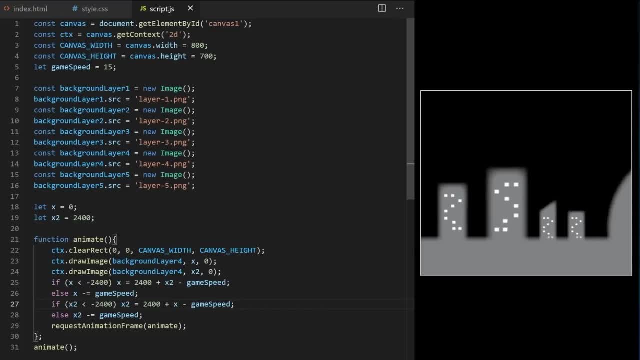 of you are already saying: Frank, what are you doing? There is much simpler way to reset endlessly scrolling backgrounds using just one variable. There is no need for this X2 variable. There is no need for all this offsetting by speed and position of the other image to synchronize them. It can be done with much less time. 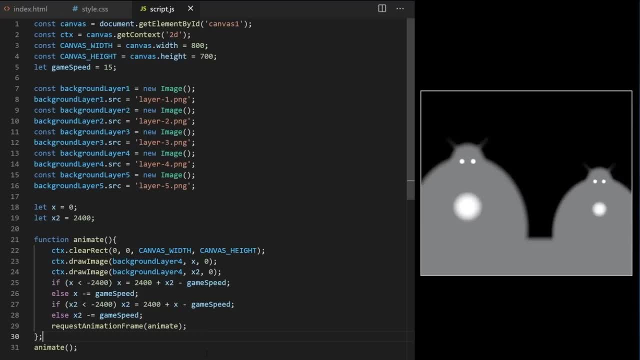 It can be done with much less code and it is so simple. And if you already realize that, well done. You are good. Let me know in the comments if you are one of those people. I went through all of this to show you my process and to actually show you how it works. I didn't. 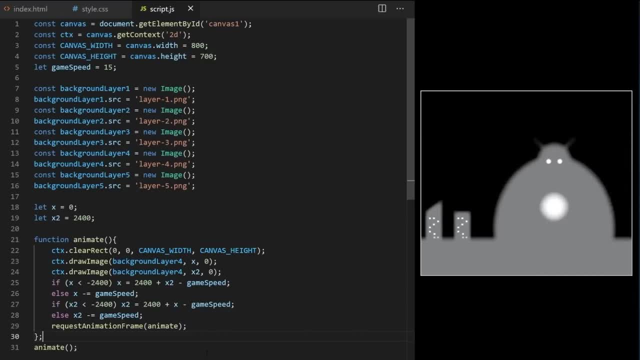 realize it can be done with one variable until I got to this stage when I was building the initial prototype. Also, I think everything we have done so far is really good for beginners to see what's going on and how this trick is achieved. We will clean this all up and optimize everything, But before we do that, let's animate all layers. 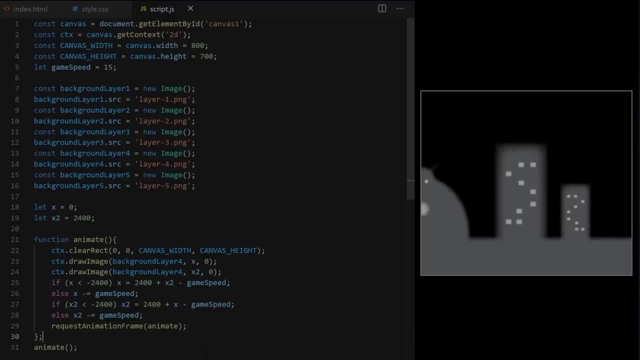 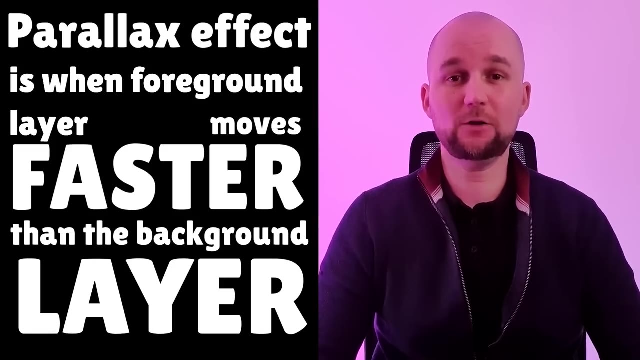 and make them move at different speeds. Parallax effect is when foreground layer moves faster than the background layer. It creates kind of a 3D effect, illusion of depth in a 2D space. It can be used in games, but it also looks really nice on websites. In our project we 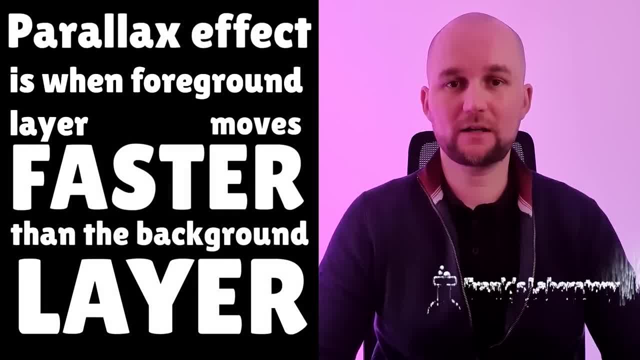 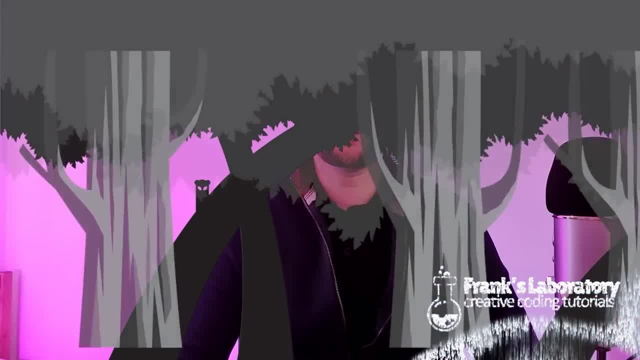 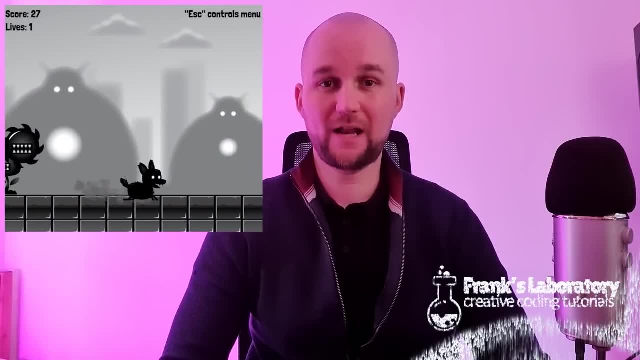 will have 5 layers, 5 images, and I want each one to move at a different speed. At the same time, I want all the layers to be tied to the same game speed variable So that when player moves, the speed of all 5 layers is affected proportionately. How do we do that? Let me, 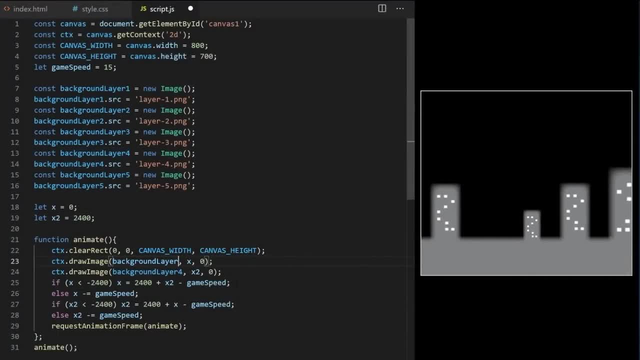 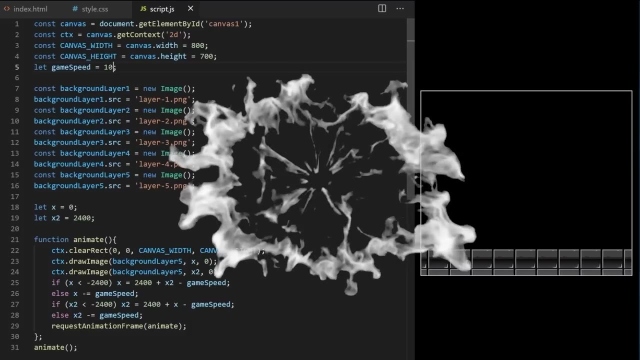 show you. First let's check if all 5 layers are animated correctly. Everything is working Perfect. So how do I animate all of these layers at the same time? I guess I could just copy, draw image on lines 23 and 24 and duplicate it for all. 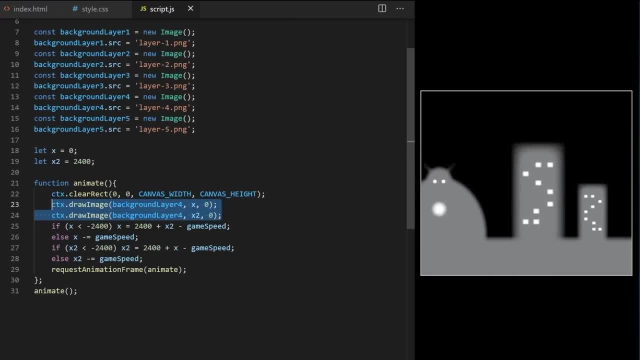 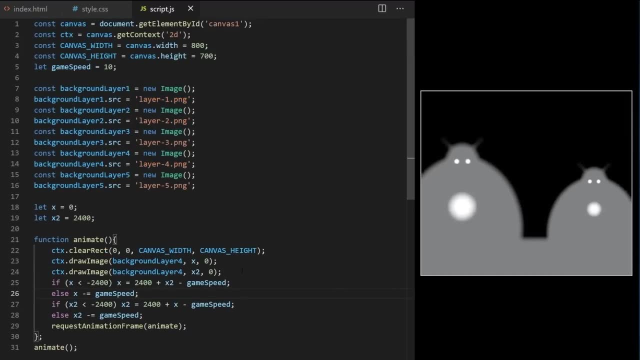 5 layers. Then I would have to create a separate reset checks for their X and X2 positions to make sure they scroll at different speeds. It's possible to do that, but there would be a lot of code repetition. Let's do it in a 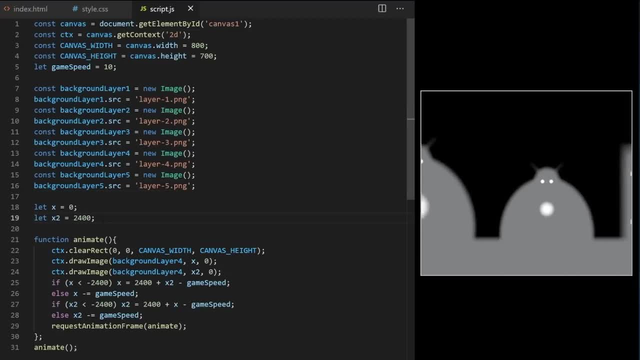 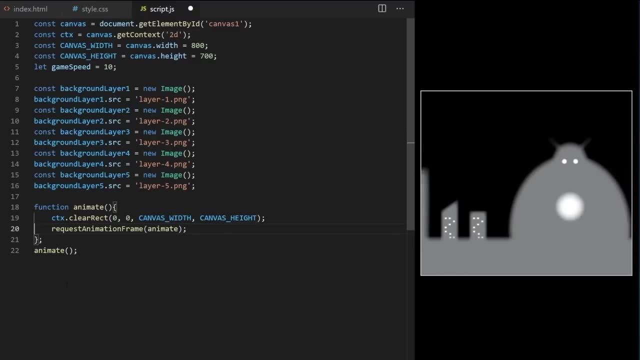 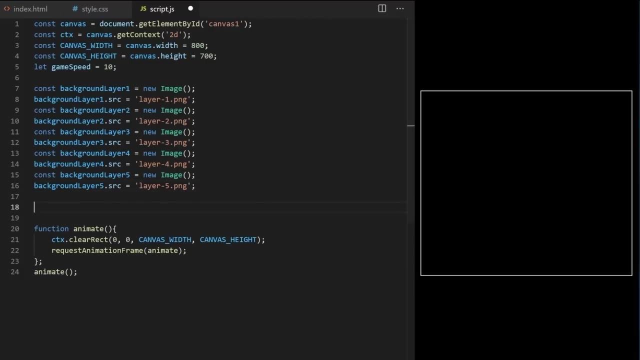 clean way. I delete X and X2 variable from lines 18 and 19.. I also delete all this code between lines 20 and 25.. I will use JavaScript classes to create a blueprint for a layer object. Then I create 5 instances of that layer class, one for each of my 5 layers. 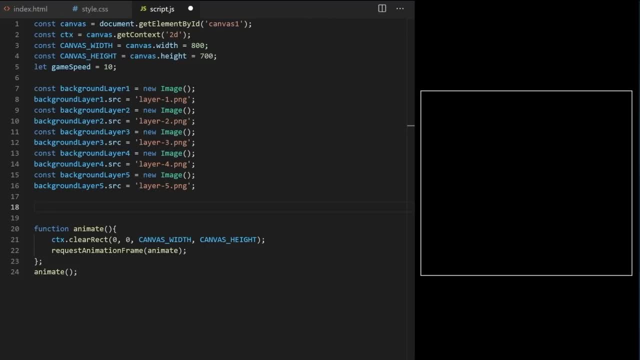 I will put all of them inside an array and I will be cycling through that array to update and draw them. It might sound complicated if you never used the JavaScript classes before, but don't worry, I will explain everything. It's actually quite simple. JavaScript classes are used when you want. 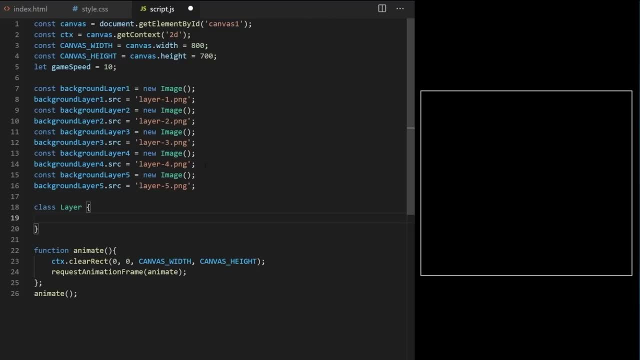 to create many similar objects. In our case, we will create five image layer objects. JavaScript class is a blueprint. I will define it and then, whenever I call it, it will create one instance of that object based on my custom blueprint. When I say it creates similar objects, I mean: 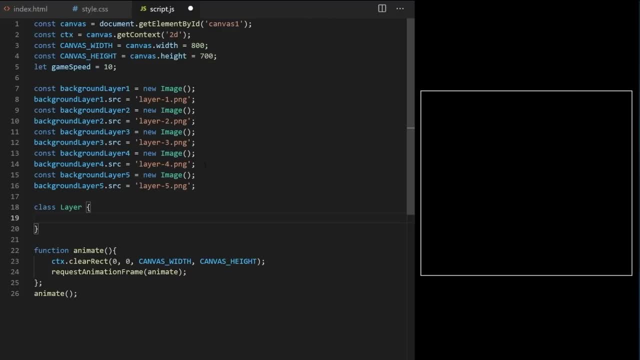 these layer objects will have shared properties and methods, but some of the properties will have different values. They will all have the same width of 2400 pixels. Each layer object will also have image and speed property, but each layer will have different image assigned to it and different. 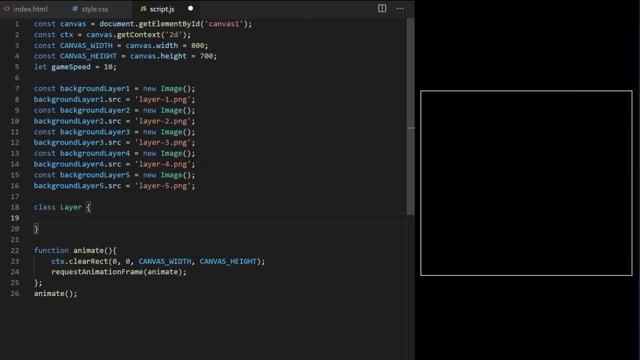 speed value. That's what it means when I say similar, Same properties, but maybe different values. Let me show you how simple it is, step by step. We define class by using class keyword followed by custom name of that class, starting with a capital letter. I will call my custom class layer, for example, Each JavaScript. 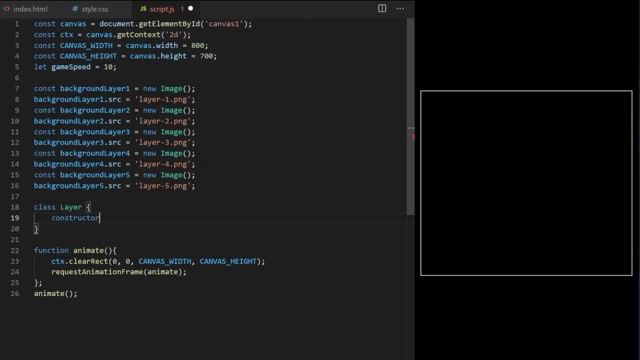 class has one mandatory method called constructor. In object-oriented programming when you say method, all it means is function attached to an object. Method is just a function. So this special mandatory constructor method has only one job. Whenever our class is called later, constructor will trigger itself. It will create one. 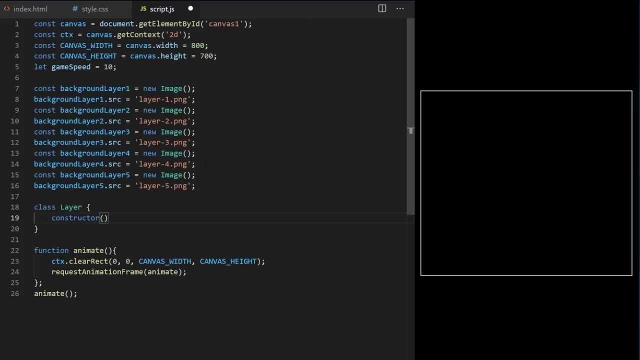 new blank object and it will assign values and properties to that new blank object based on blueprint inside the constructor. Constructor runs only once per object. every time javascript class is called using the new keyword I will show you in a minute- My constructor will expect two arguments: Image we want to assign to that layer and speed modifier. 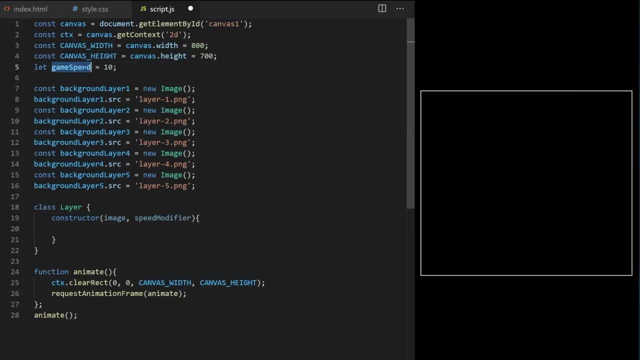 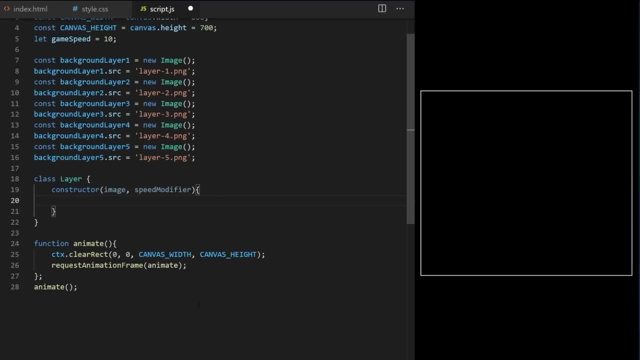 because I want each layer to scroll at slightly different speed. We will pass these arguments from the outside when we create a new object. We will pass these arguments from the outside when we create our 5 layer objects. I will show you in a minute. For now, let's finish our blueprint, The syntax. 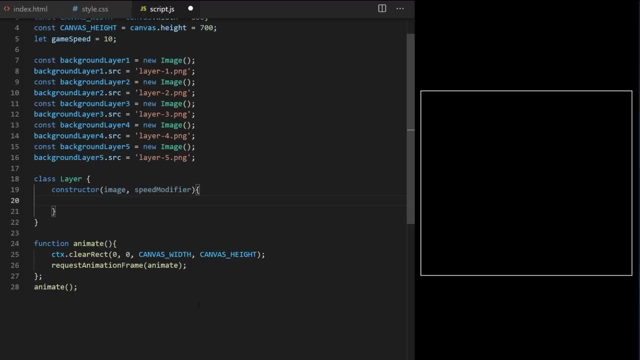 might be a bit strange for you if you are new to object-oriented programming. Each layer object will have horizontal x coordinate that starts at position 0. I say this dot x because my layer class will create many similar objects. so I'm saying here on line 20: set x property. on this: 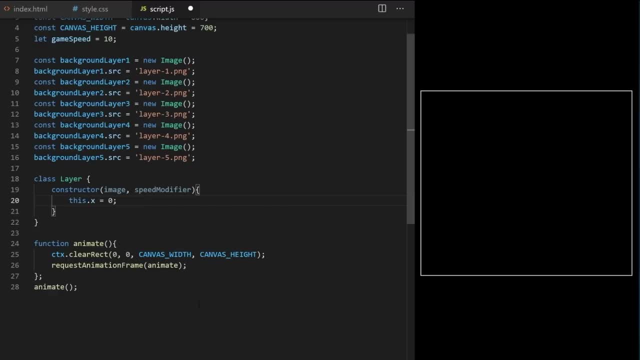 particular object you are creating right now to zero Because we are inside blueprint that will trigger every time we call our class to create an object. I will also have vertical y coordinate that will be set to zero. All our layers will have the same width of 2400 pixels. Height will. 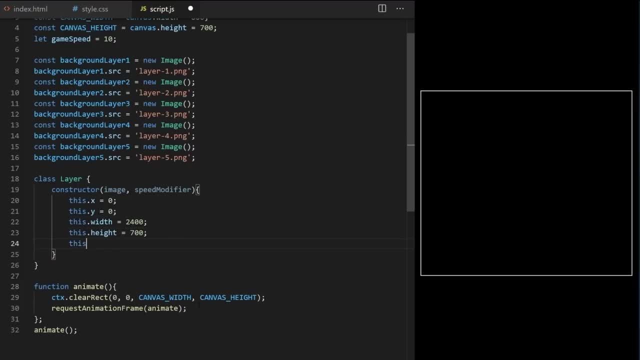 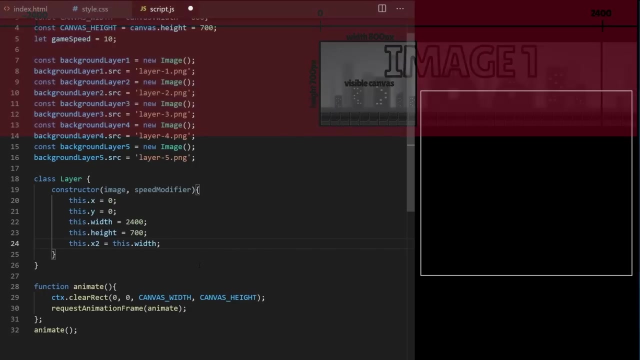 be 700 pixels for all my layers. X2 coordinate will be where we draw the second image. The second image needs to start where my first image ends, so at the horizontal position, 2400 pixels. I know I said we could do this without x2 property, using just one variable. Let me just recreate what 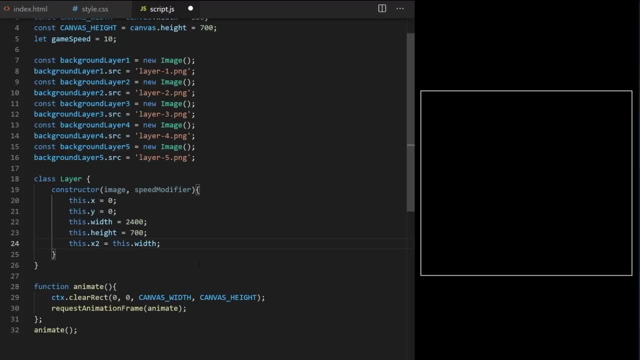 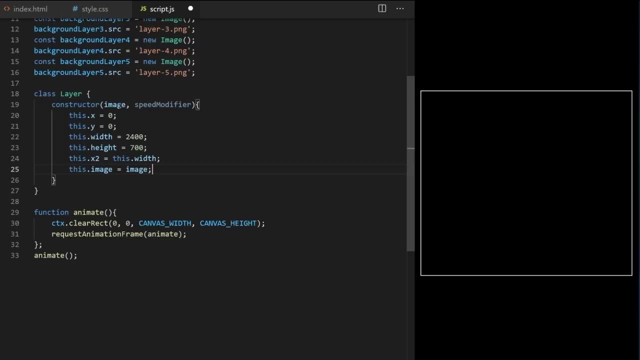 we had before as a class and then we optimize it together. I want to do this step by step for clarity. This dot image equals image. This declaration is a bit different. What I'm doing here, I'm telling my constructor create property called image on this new object you are creating. 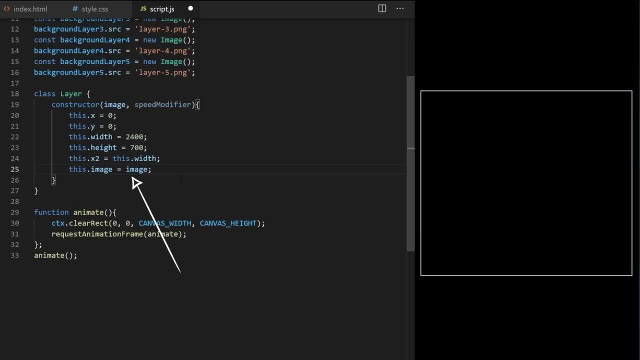 right now and set it to image we pass as argument on line 19.. I will show you how to pass arguments to constructors. I will show you how to pass arguments to constructors. I will show you how to pass arguments to constructors when the class is complete. I will do the same now with this dot. 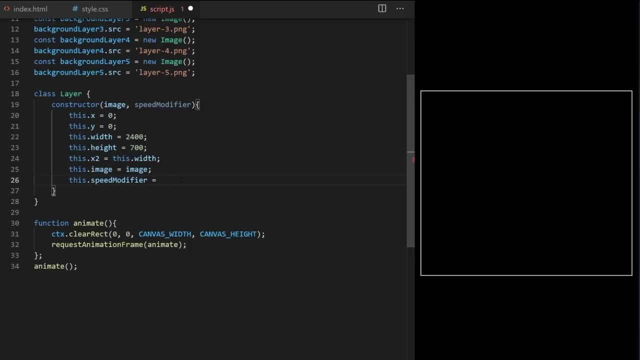 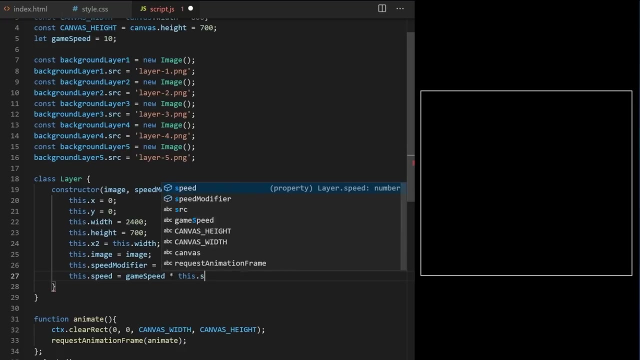 speed modifier. It equals the speed modifier passed on line 19 as an argument to my class constructor. This dot speed will be how fast is my image layer moving? I will calculate it by taking my global game speed variables and I multiply it times this dot speed modifier from line 26.. 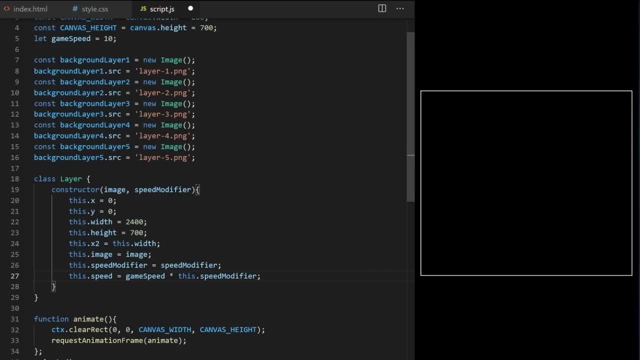 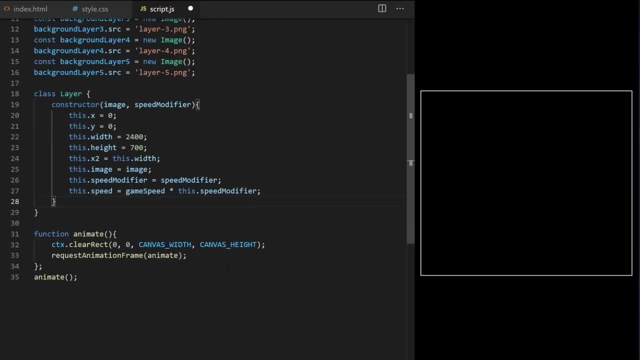 Doing this will allow me to pass different speed modifier value for each of my five layers and that way each layer will move at different speed, but it will still be tied to my global game speed. You will see in a minute My layer object will also have access to custom method I call for. 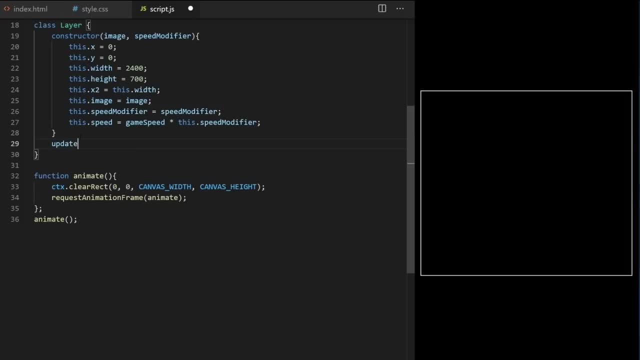 example, update. Its job will be to move layers horizontally by changing their this dot x and this dot x2 properties from lines 20 and 24, and it will reset them when the layers move off screen. This is the same way we did it before. We are doing the same thing we had before. 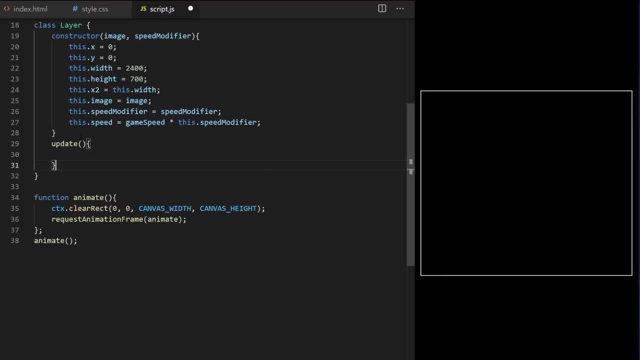 but this time we are wrapping it in a reusable class syntax so that we can do all of this at the same time for all five layers. We will also have a method I call, for example, draw. Its job will be to take information about this layer object and to draw it on canvas Every time update. method runs to change horizontal x. 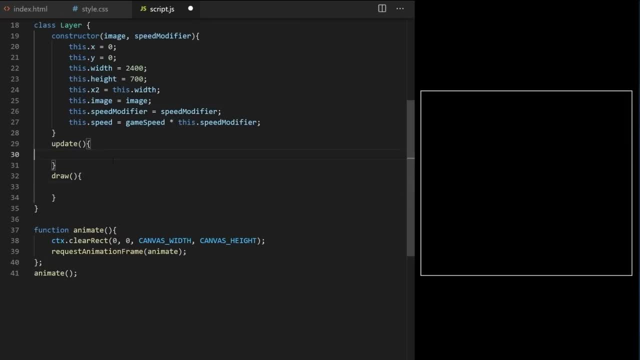 position draw will run again to redraw the image at the new position. To make sure my game speed is dynamic and always reacting to the current value of my global game speed variable from line 10, I need to recalculate this dot speed like this If you want your game to have a constant never. 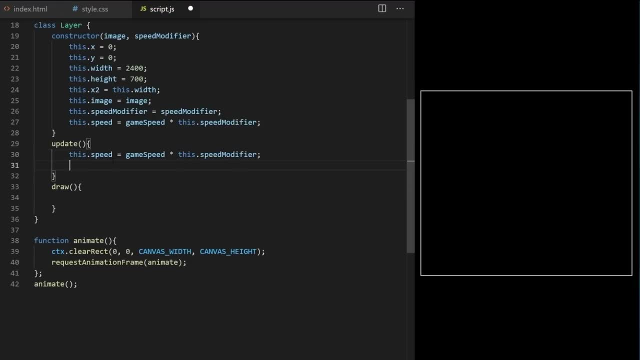 changing scrolling speed. you don't need to do this line of code Now. I just say: if this dot x from line 20 is less or equal to minus this dot width from line 22, so minus 2400 pixels, then set this dot x to this dot width plus offset it. 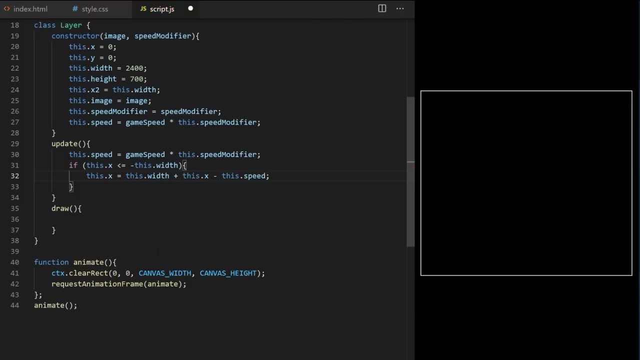 by the current position of my x2 minus thisspeed. I'm just recreating the same thing we did before. I explained why I'm offsetting it by x2 and speed. It is to make sure there is no gap between my images. I copy this entire code block and I do the same thing for thisx2 property from line 24.. 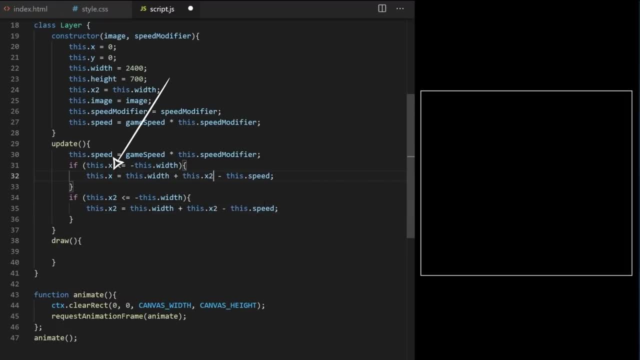 So thisx needs to be offset by the current value of x2 and thisx2 needs to be offset by the current value of thisx. If they are not resetting, I just want my x property to decrease by the amount of thisspeed. from line 27 to make my background layer move to the left, I will wrap. 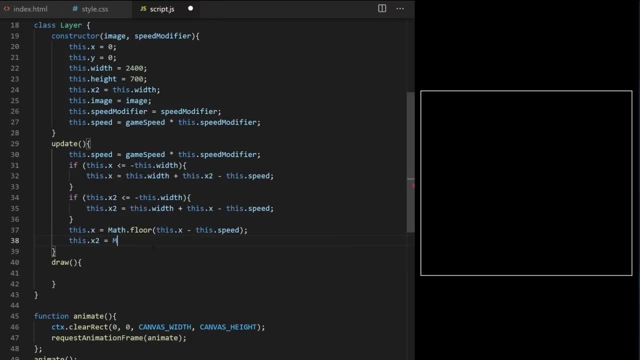 it in mathfloor to make sure we have no decimal points in there. Not sure if this is a good idea. let's see a bit later. I do the same thing for thisx2.. This can be optimized and simplified and we will do it in a minute. Now I can take these newly updated x and x2 coordinates. 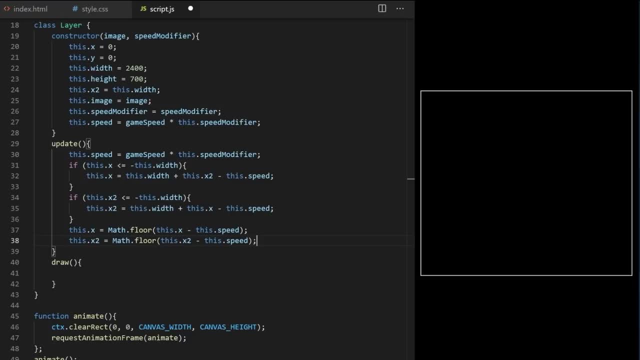 and I draw two identical images next to each other, like we did before. So drawImageBuildingCanvas method, I pass it, thisimage from line 25, thisx and thisy, thiswidth and thisheight, Then I draw the same image, but I will draw it at thisx2 horizontal coordinate, like we did before. And 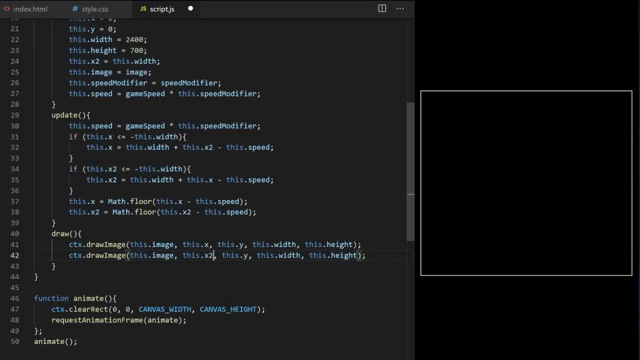 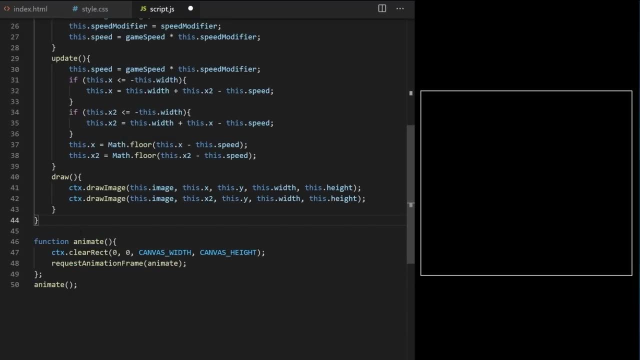 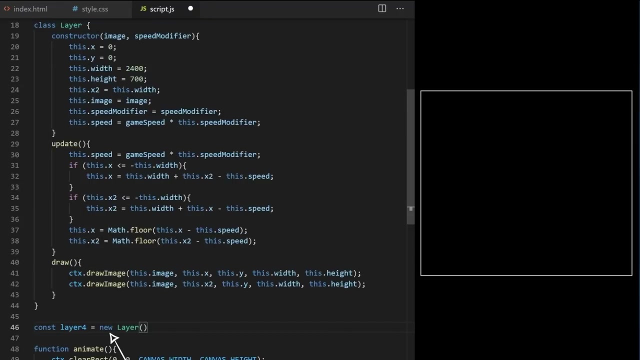 that's complete. We have a blueprint inside the constructor and my layer objects have access to custom update and draw methods. Now I can create a new constant variable. I call, for example, layer4, and I set it equal to new layer. like this: The new keyword is a special command in 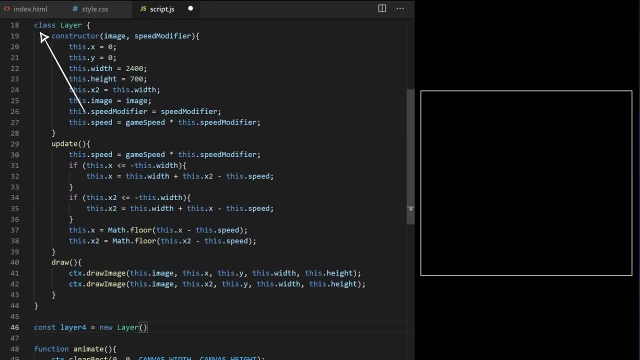 JavaScript. It will look for class with that name in our code and it will trigger its constructor On line 19,. I can see that my layer constructor expects two arguments: image and speed modifier. I need to pass them here when I'm creating an instance of my class. 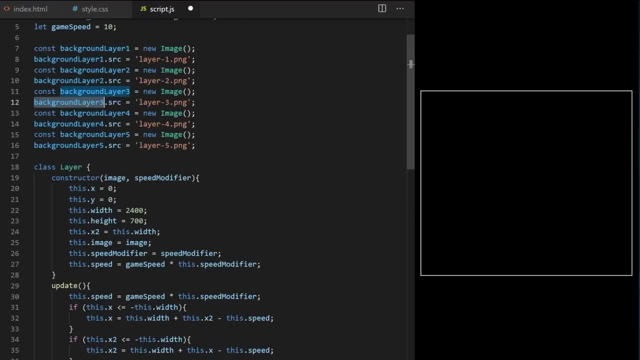 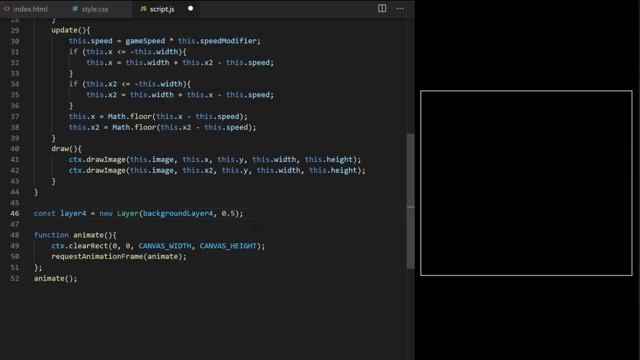 so I will pass it. background layer4 variable as image and speed modifier will be maybe 0.5. I want this layer to be moving at half of my game speed, So if my game speed is 10 pixels, this layer will be moving at 5 pixels per frame. Let's test it. So here, on line 46, I call my layer class. 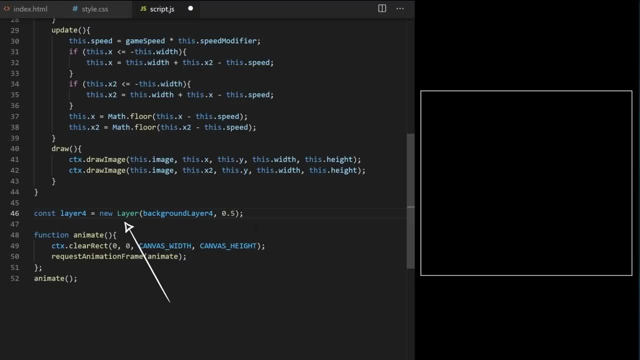 and assign it properties and values I defined in my blueprint between lines 20 and 27.. Then it saved that new layer object inside this layer4 variable. So this is how you create an instance of your custom JavaScript class. As we know, my layer class has access to update method from line. 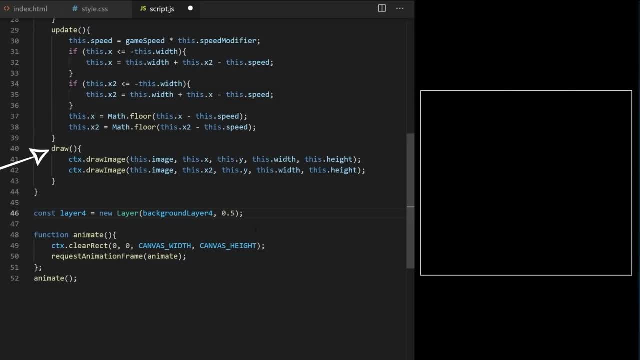 29 and to draw method from line 40.. I can just go inside my animation loop. I can take layer4 variable from line 46, and I can call update method from line 49.. I can also create a new layer object inside this layer4 variable and I can update and draw on it like this. 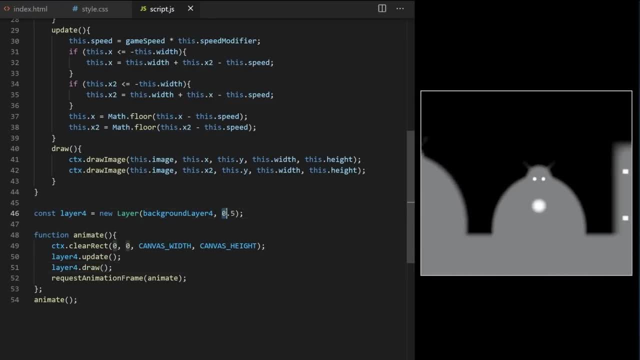 And here we go. We refactored our image layers into JavaScript class and now it's very easy to work with it. I can pass it different speed modifier on line 46 to make it move at a different speed. That speed is still relative to my global game speed variable from line 5, because I keep 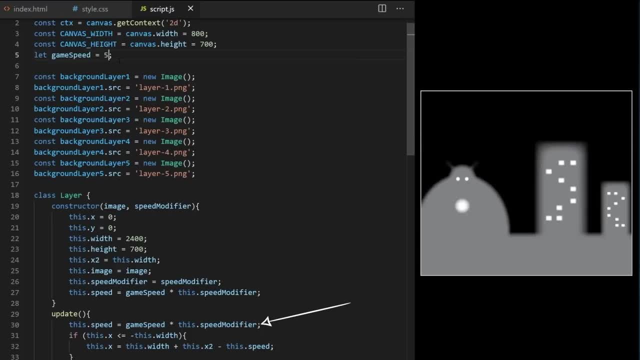 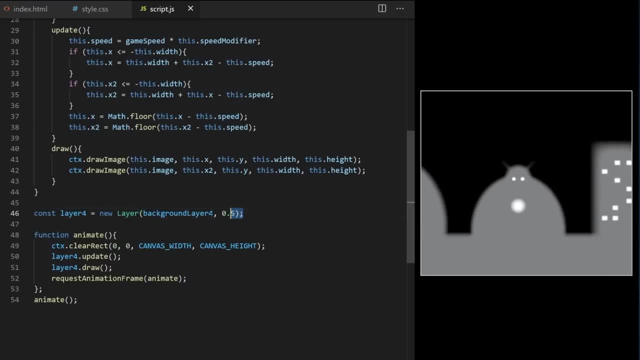 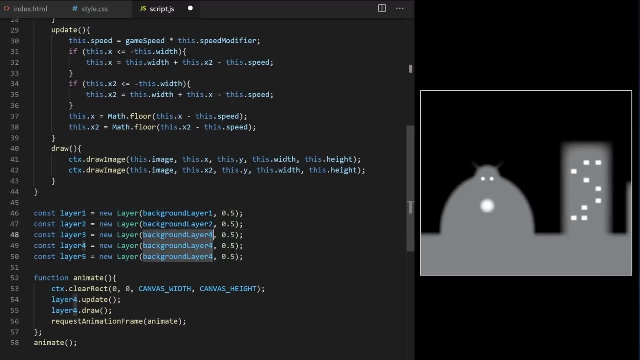 track of that. on line 30, inside update method, I create variables for all my five layers. I will pass different images to each one. I could just call their update and draw methods by duplicating lines 54 and 55 like this. Now I'm. 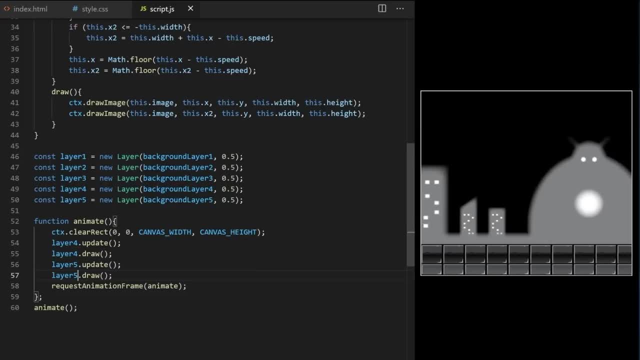 drawing layer 4 and layer 5, but there would be a lot of code repetition if I did it for all five layers. If I change speed modifier value, I pass the layer class constructions. Then I can pass the class constructor on line 50. You can see their relative speed changes and we have parallax. 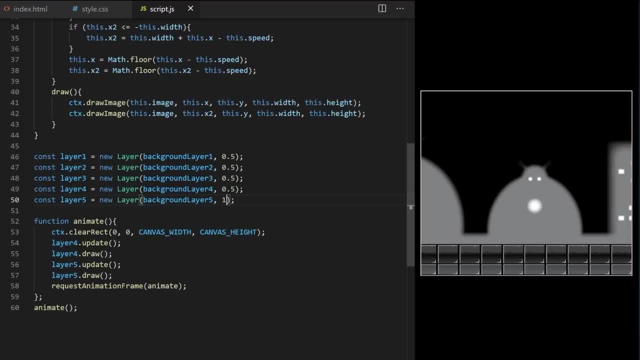 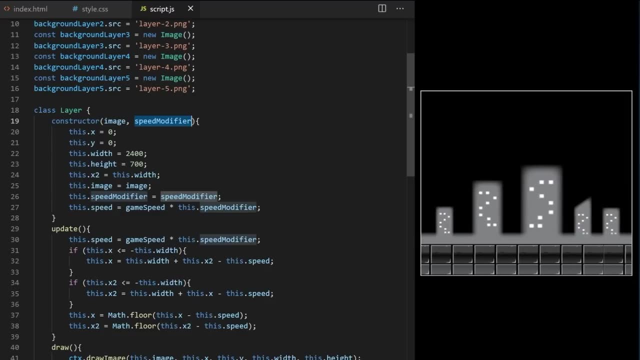 effect Awesome. It is because that speed modifier takes game speed and adjusts it by multiplying game speed from line- 5 times this modifier value. At first it happens on line 27 when the new object is created. Then it happens on line 30 whenever update method runs, to make sure we can change. 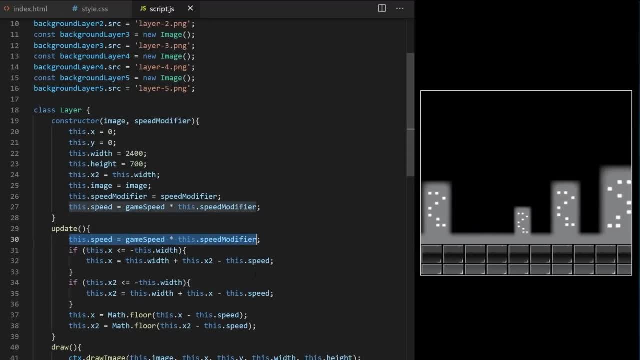 global game speed dynamically, which we will do in a minute. Then we are just using thisspeed property to recreate the game speed variable from line 5.. And here we go. We can see that the game speed variable from line 5 to line 5 is the same as. 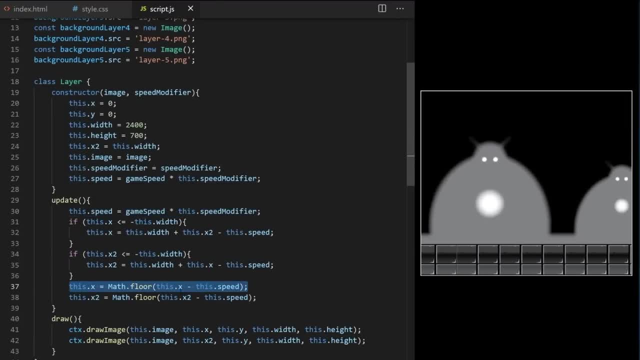 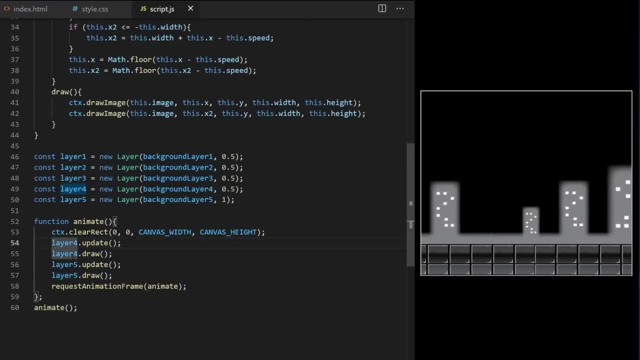 the game speed variable from line 6.. We can calculate horizontal exposition of our background images here on lines 37 and 38.. And this is how you make your layers scroll at different speeds but still tie them together by using global game speed variable Inside my animation loop. 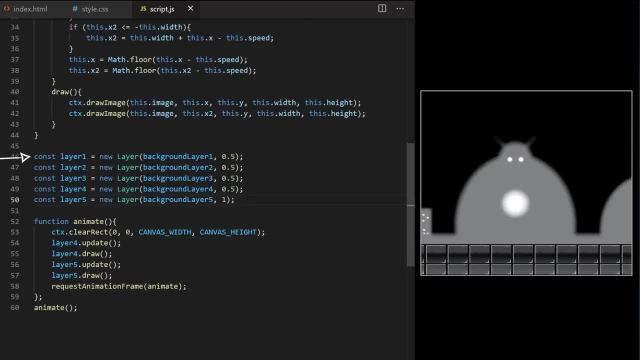 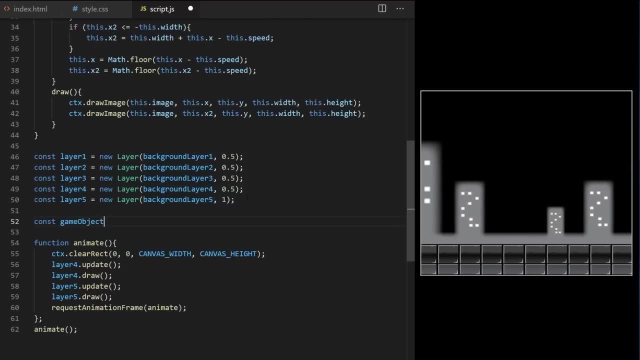 I can just call update and draw for all five layer objects, but I don't want any code repetition. I create a new variable. I call for example game objects and I set it equal to an array. I put layer 1 variable from line 46,. 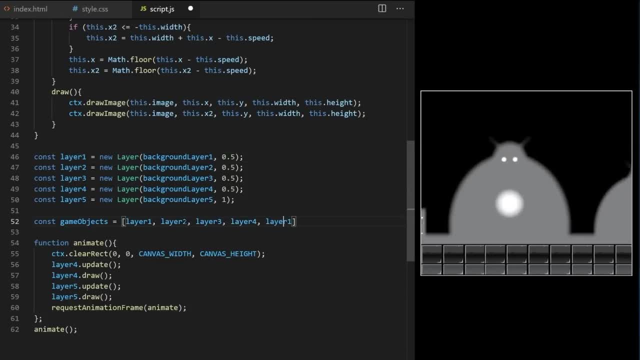 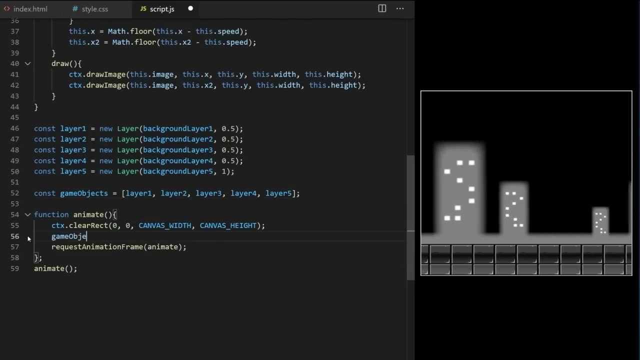 in there layer 2,, 3,, 4, 5.. Now I have all five layers inside a single array. So on line 56, I take this game objects array and I call built in for each array method. For each method will simply run through all elements. 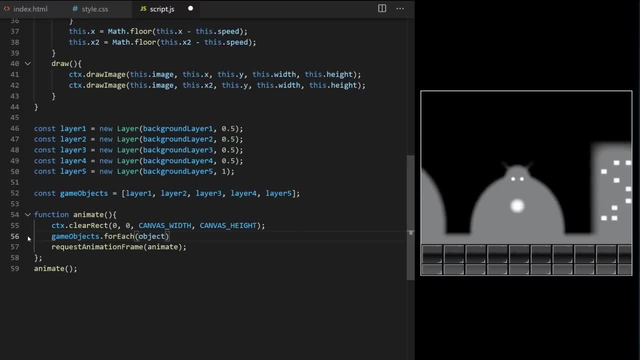 in the array and it will apply whatever callback function I give it to each of these elements, each of the layers. First, I need to declare how I want to refer to individual objects in game objects array within my. for each callback function, For each object, I need to declare how I want to. 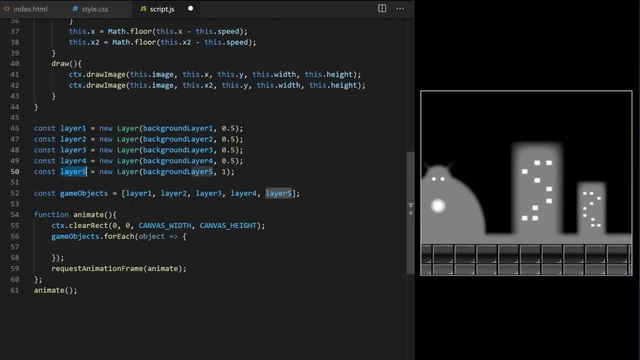 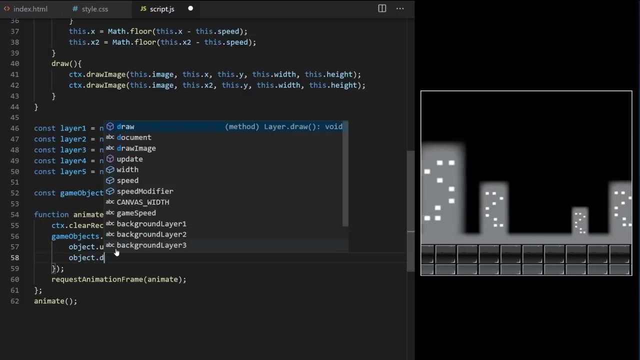 for each callback I will refer to them as object. for example, I'm doing ES6 arrow function syntax here, where you can omit function keyword. So for each layer object in my game objects array I will call their associated update and draw methods like this. Here we go, we are drawing all five layers. 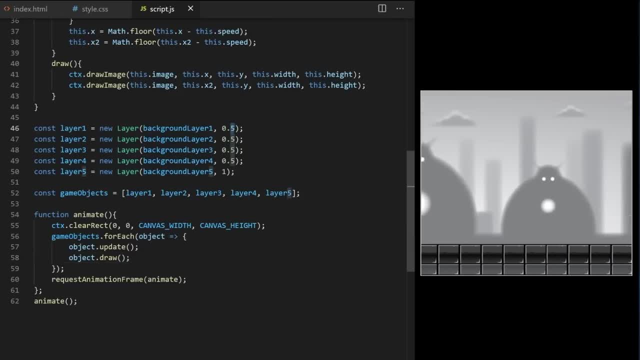 now awesome. Let's pass each layer a different speed modifier to create proper parallax effect: 0.2, 0.4,, 0.6, 0.8 and 1.. Now each layer moves at a different speed, but they are all still relative. 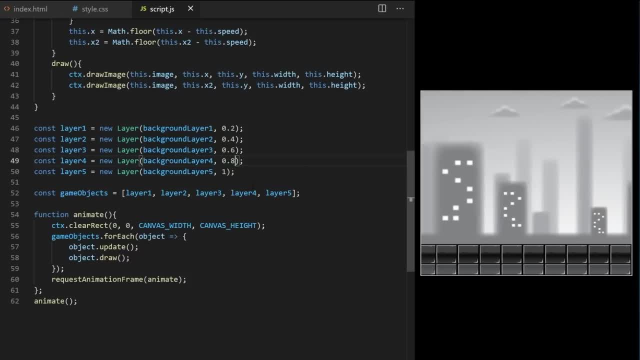 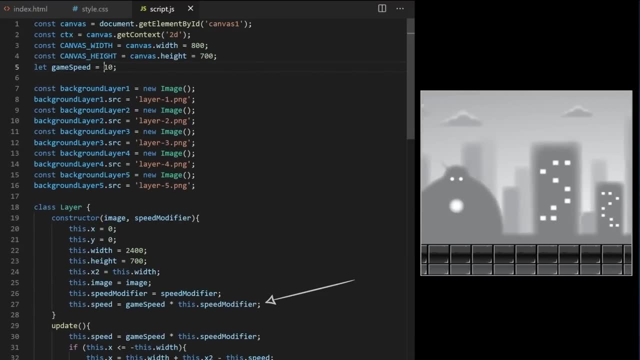 to our global game speed variable from line 5.. If I change global game speed variable, it will affect all five image layers proportionately, because their speed is calculated by multiplying game speed times speed modifier. If you get any frame drops at this point, it is because we are using 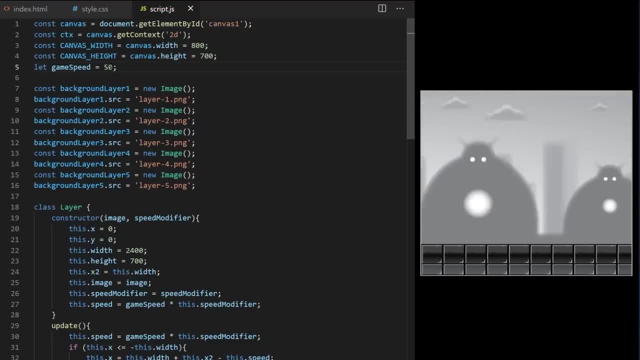 five images that are 2400 times 700 pixels. You can also change the speed of each layer. by changing the speed of each layer, You will get much better performance if you make the images smaller in Photoshop or some other graphics editor. As you can see, I can change my game speed to. 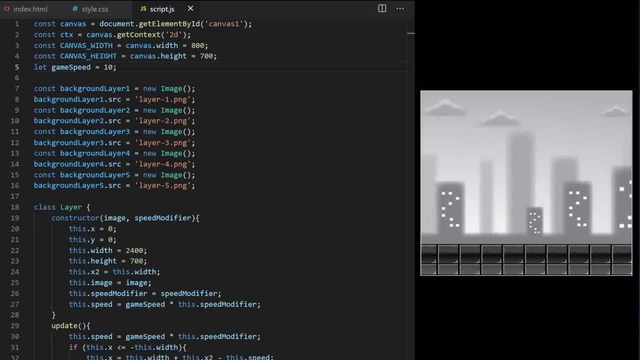 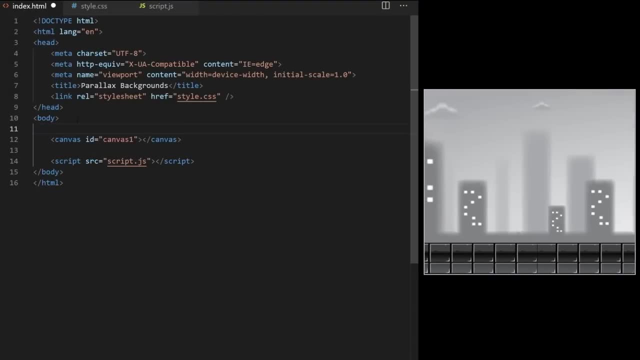 any value and parallax background will still scroll. based on that, I want to allow my users to easily change scroll speed. In indexhtml I create a div with an id of container. Inside I will have paragraph tag that will say game speed. colon and span element with an id of show game speed. This will show real time value of game speed. 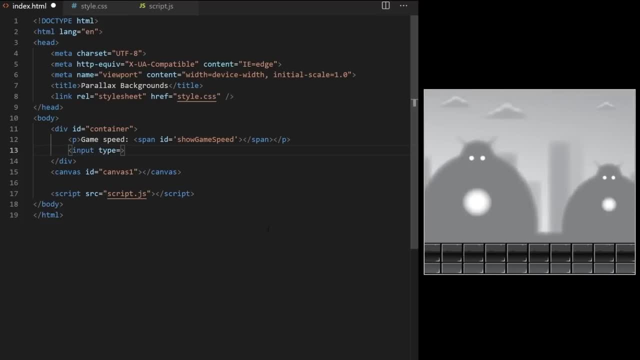 variable. I create html input element with type properties set to range. Min value will be 0,. max value will be 20,. start in value will be 5,. class will be slider, for example, and id slider as well. I put html canvas element inside the container. 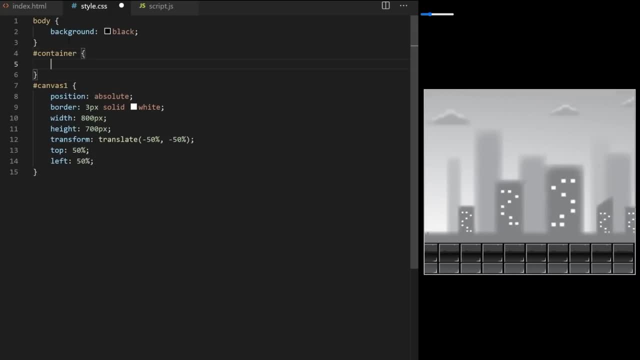 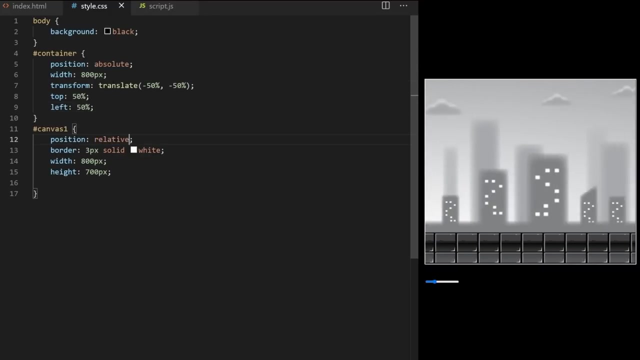 In style css. I take container. I give it position absolute Width, 800 pixels. I center it in the middle of the page using transform translate. I set canvas to position relative so that it aligns with container. I put border on the container so we see where it is Input with. 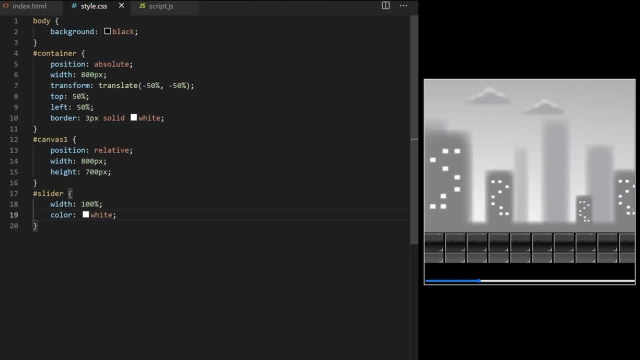 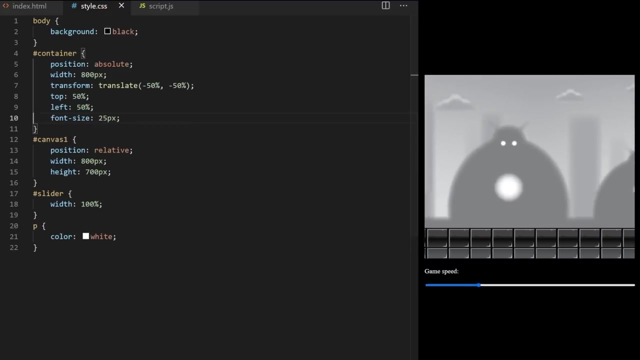 an id of slider will have width of 100%, Text color white. Ok, that doesn't work. I take paragraph tag and I move text color there. On container I set font size to 25 pixels And I remove border. In scriptjs I create a new constant variable. I call, for example, slider and I point javascript. 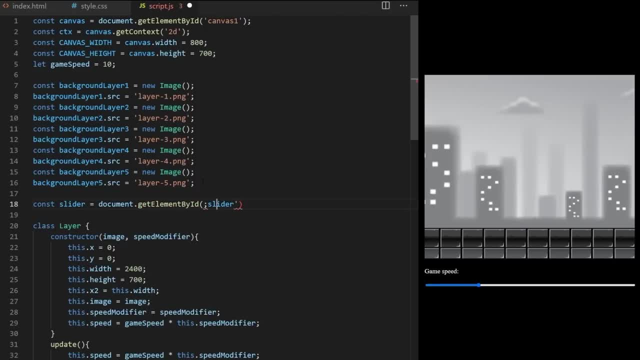 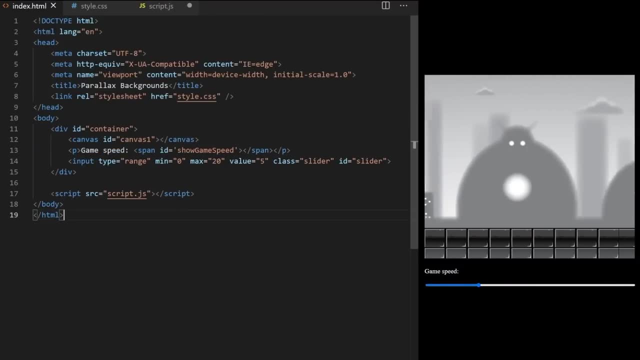 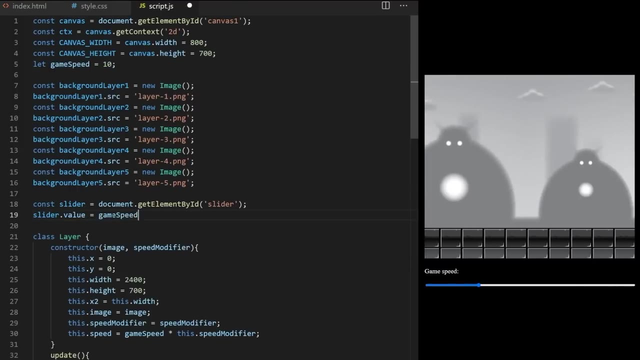 towards my new slider element with get element by id. On the first page load I will set slider value property, which is here. Then I take hold of this span element with id of show game speed and I save it in a variable i call show game speed as well. On the first page load I set its inner html equal to the current value of 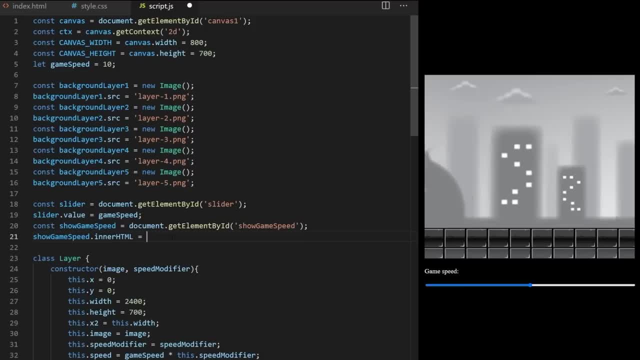 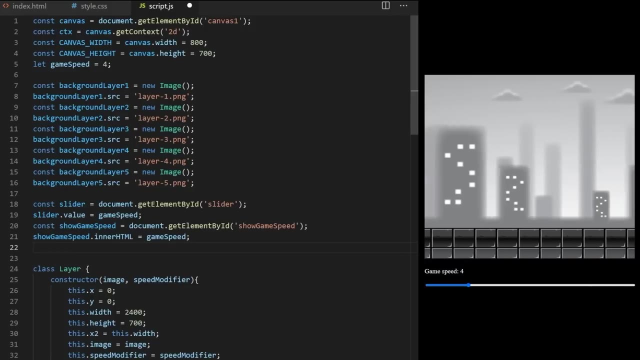 game speed variable from line five. If I change value of game speed and reload page, you can see it here works. Now I want to change scrolling speed of my layers when I click this slider. To do that I need to connect it to game speed variable from line 5.. On. 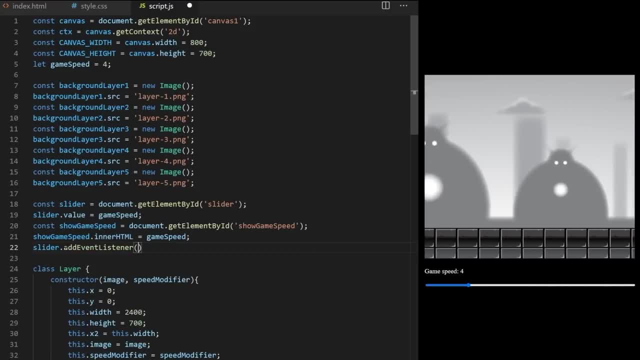 line 22. I take slider from line 18 and I call add event listener. We will listen for change event and in callback function whenever change event occurs on the slider, which means whenever user clicks on it to change its value, I will run some code. Callback function on event: listener has access to its built-in. 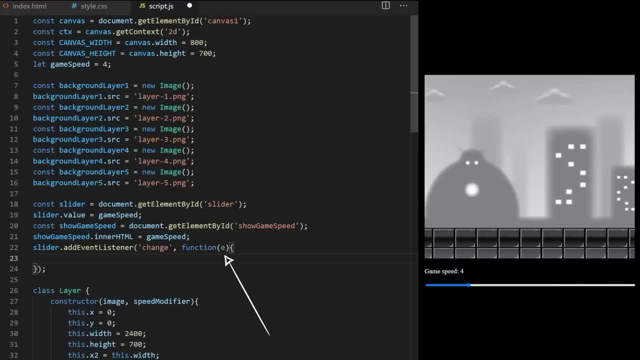 event object. I will refer to it as E here. I can refer to it however I want JavaScript knows that the first argument passed to callback function on event listener refers to this built-in event object. If I consolelog this E, you can see: 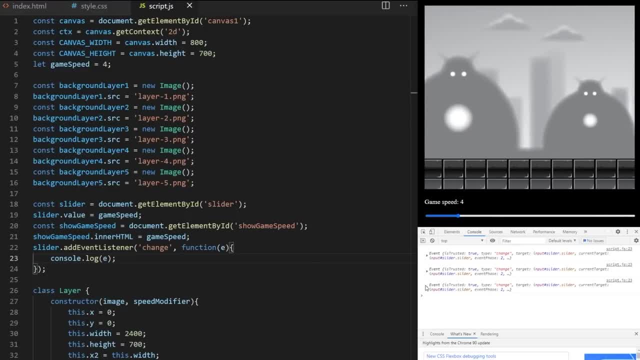 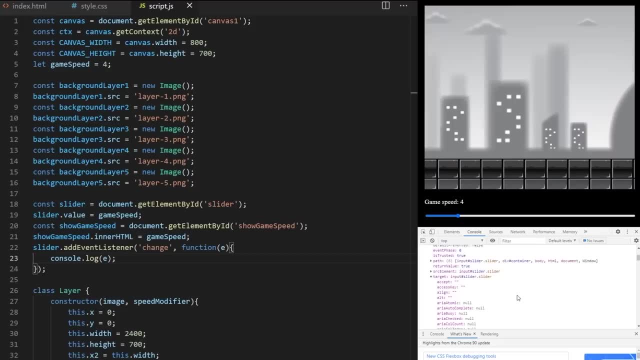 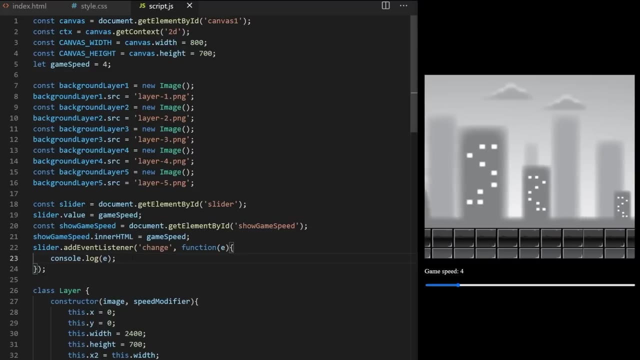 it gets consolelogged every time change event occurs on slider and it contains a lot of useful information about that event. Right now I'm interested in its target property, which references target of this change event, which is HTML input element with an ID of slider. When it gives me that I can access its 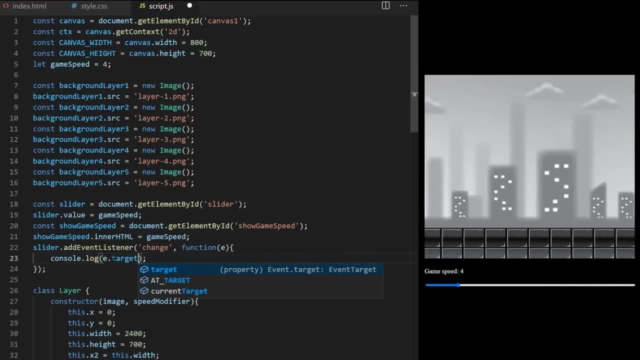 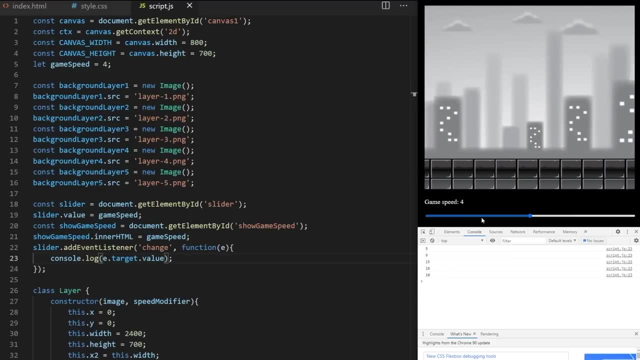 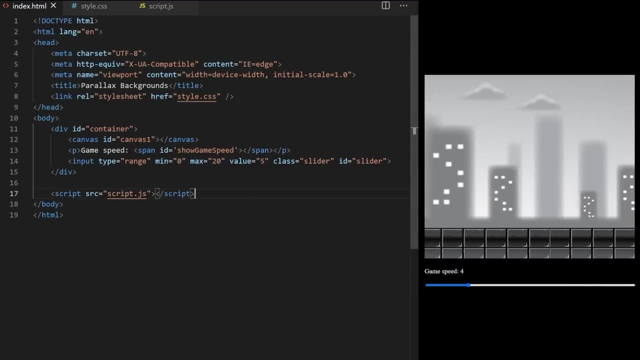 current value attribute, which is exactly what I need. If I consolelog E dot target dot value, it will give me the current value of this slider input element. I set minimum value to 0 and maximum to 20 here. All I have to do now is take game speed variable from line 5. 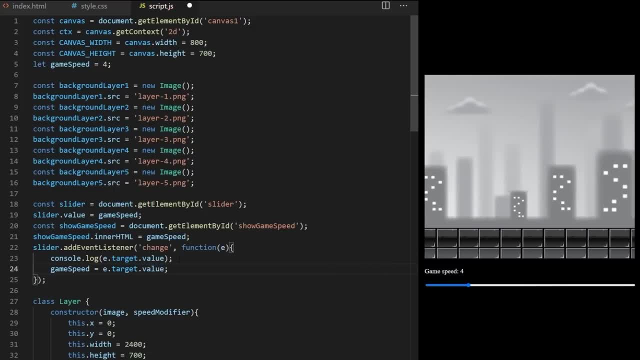 and I set it equal to E dot target dot value like this, And I will also update inner HTML in show game speed span so that it displays the correct current speed for us. Now I can change scroll speed of my layers by clicking on slider. 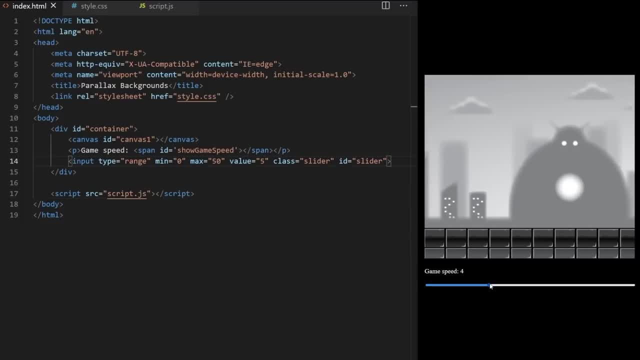 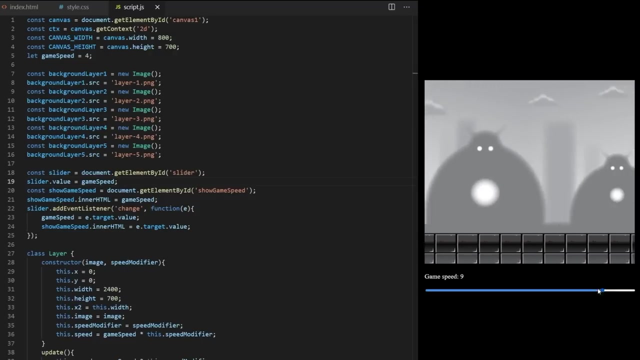 If I change it to max 50 we can get it to scroll really fast. I hope your computer can handle that. These images are too large. Let's set max value back to 20.. You probably already realized earlier that we don't need to have this dot x2 property. 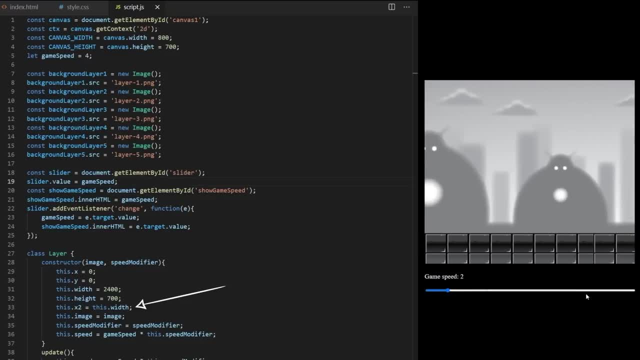 here on line 33, and we can calculate position of both images using just this dot x. That way we don't need to have two separate reset checks here, and since everything is coming from just one variable, we don't need to do all this complicated offsetting we did earlier. 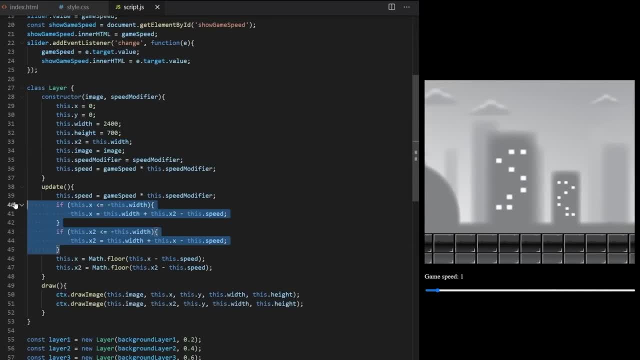 because we don't need to make sure x and x2 are synchronized. If you want little challenge, pause the video right now and try to refactor update method yourself by deleting all references to this dot x2 and using only this dot x to calculate positions of both images. If you don't know how to do it, don't worry. 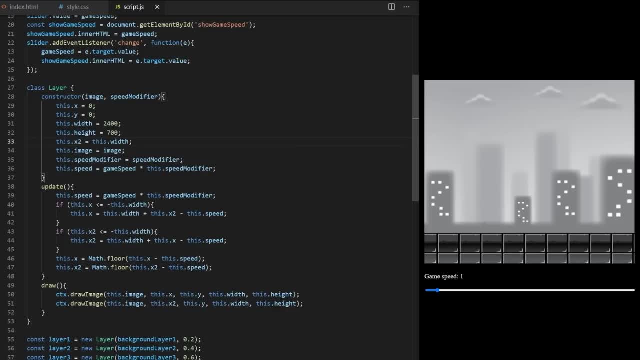 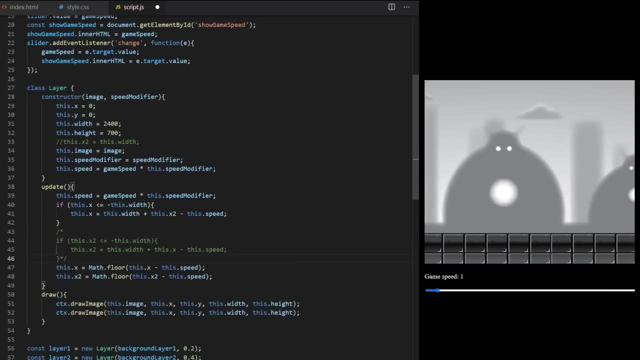 I also didn't realize it at first until I started working on this tutorial. I comment out line 33.. On line 51, inside draw image method, I replace this dot x2 with this dot x from line 29.. I comment out this if statement. 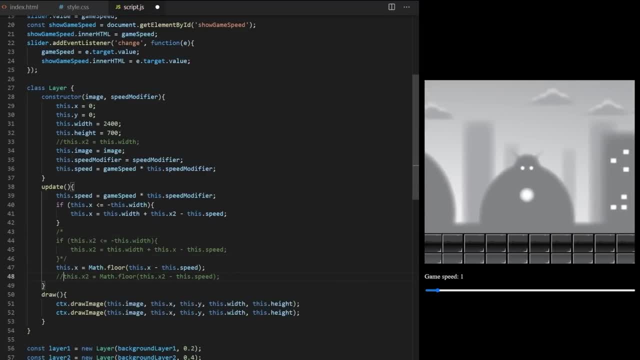 and also this line 48. I remove reference to this dot x2.. Since I'm using this dot x for both images on line 51 and 52, you can see our parallax has gap again. This time a big gap, haha. Lucky for us, it's. 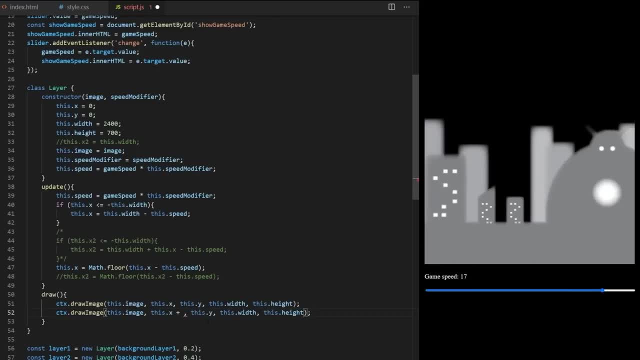 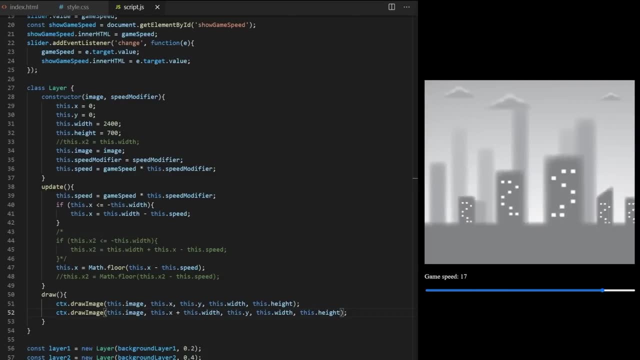 very simple fix. On line 52. I set horizontal x coordinate to this dot x from line 29 plus this dot width from line 31.. That doesn't quite fix it yet, as you can see. I also have to look at my if statement on. 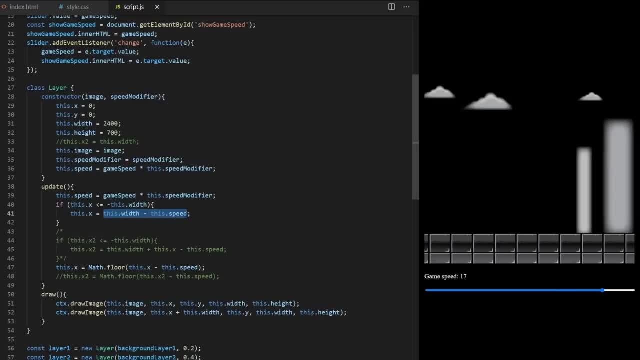 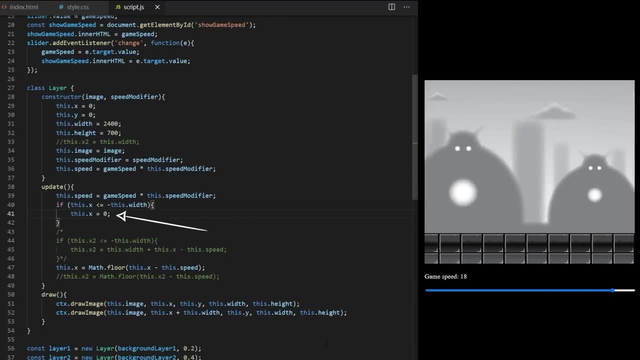 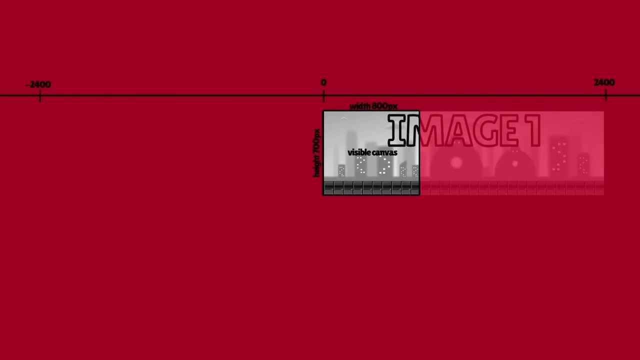 line 40.. If this dot x is less or equal to minus this dot width, minus 2400 pixels, set this dot x back to zero. If you don't understand what is happening right now, look at this. I have one image drawn at position X which starts at zero, and the second image is drawn at 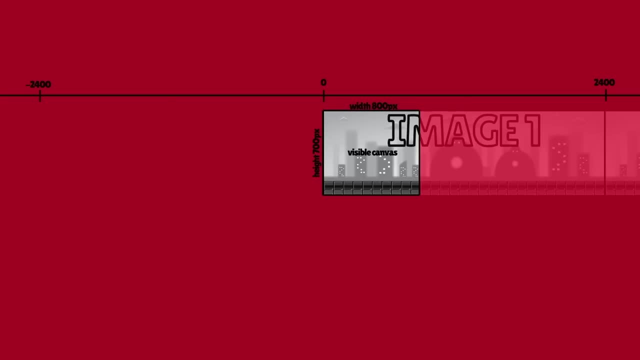 position X plus width. These images sit next to each other and scroll to the left together. like this: When the first image is drawn at position X plus width, the second image is drawn at position X plus width. Once the first image moves past the left edge of the canvas, the second image is there to 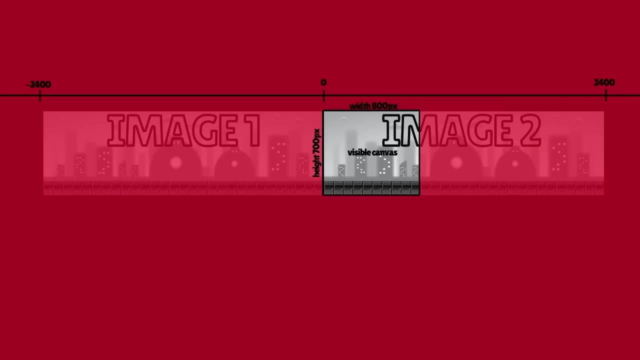 fill the gap and make it look seamless When the right edge of the first image hits the left edge of the canvas at the same time. this dot x is minus 2400 pixels because my image is 2400 pixels wide. we will trigger reset. It will just jump back here and start scrolling. 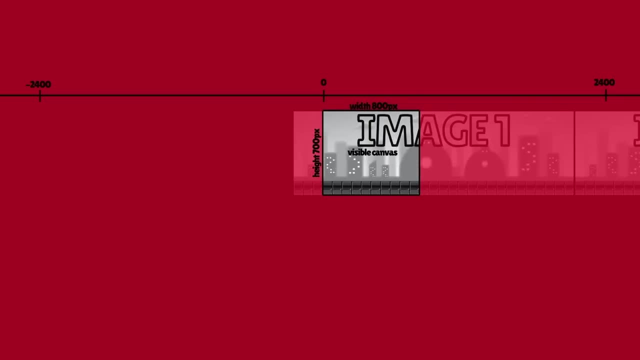 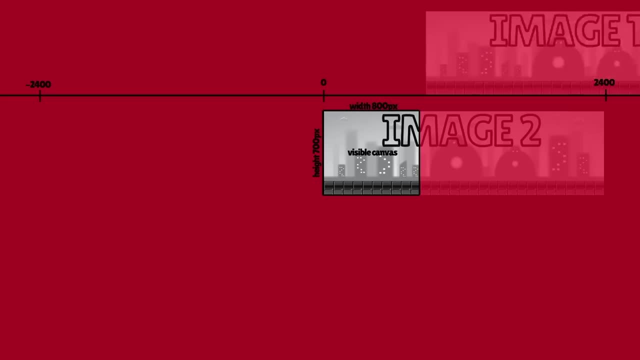 by their scroll speed and by the current horizontal position of the other image to make sure they stayed aligned. This is just a visual representation of what was happening. Of course, the transition itself, where the image resets after leaving the screen, was happening instantly. More like this. 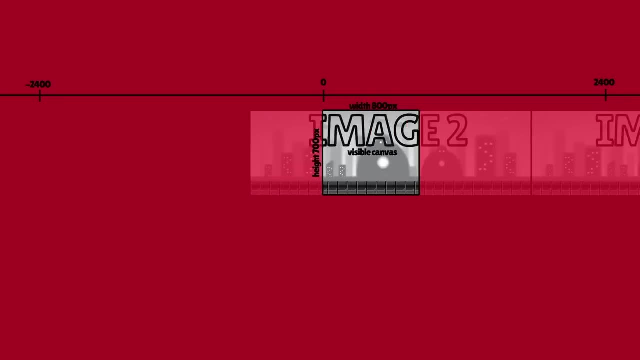 This image has been changed by the power of thisx2 example. This second improved technique uses just one variable to move images horizontally. This image is at position thisx and the position of the second image is calculated from that by adding thisx plus thiswidth. The second image is always 2400 pixels to the right of the first image. 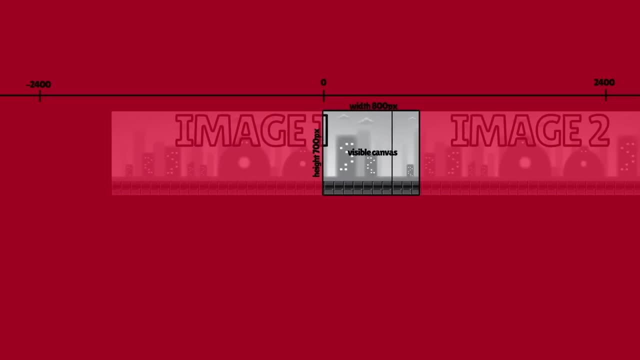 This way they will always be synchronized. since the position of both images is combined at a certain distance, Rather than slight Edgar-even pressure, we can switch the from the same variable. As you can see, the movement is different. now We never actually fully see the second image anymore. We just see this small part that 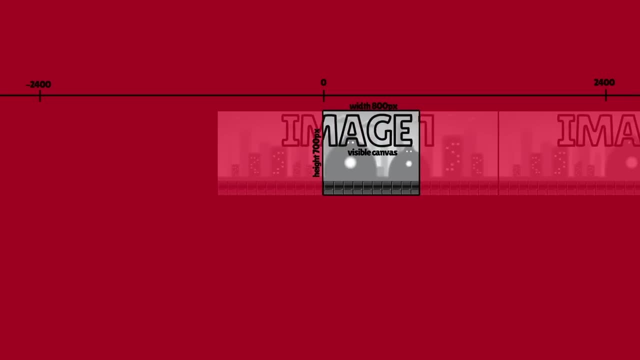 pops in place so that it looks like it's one long seamless image. Again, the transition, the reset, where the images move to the right to start from their original position, happens very fast. It happens instantly, so we jump from this to this and that makes it look like it's just one seamless movement. 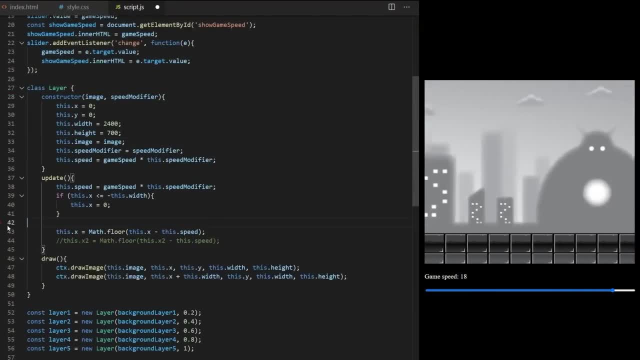 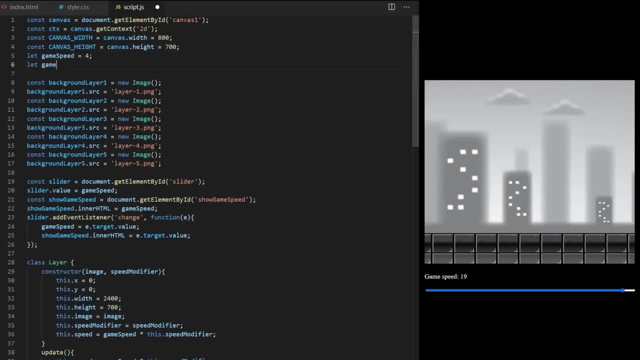 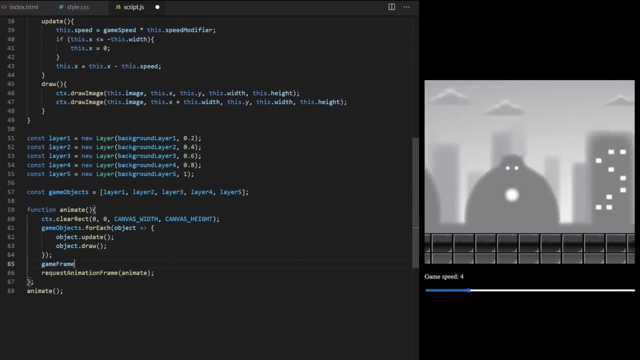 We can also calculate position X differently. I can create a game frame variable and I set it to zero. Then in my animation loop here on line 65, I increase game frame by one for every animation frame. This way we have a number that is endlessly increasing. Now I can replace this if 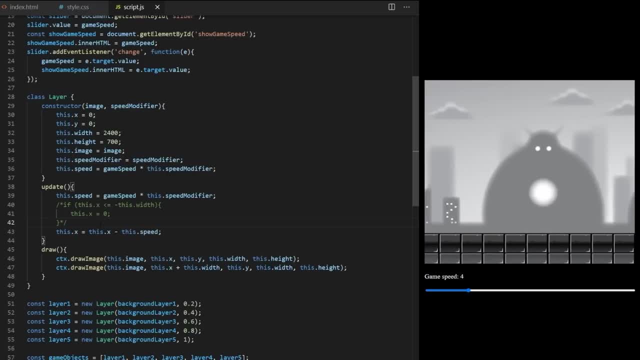 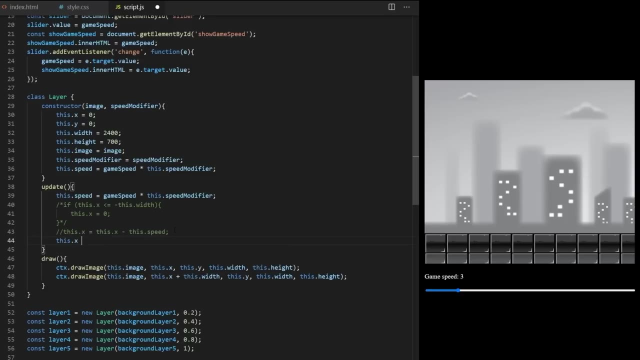 statement on line 40 with a different calculation. When I remove this if statement completely, the background's not longer reset when they leave the screen. I also comment out line 43 and I can replace all of this with just one line of code. I say thisx from line 30 is equal to game frame variable we just created and 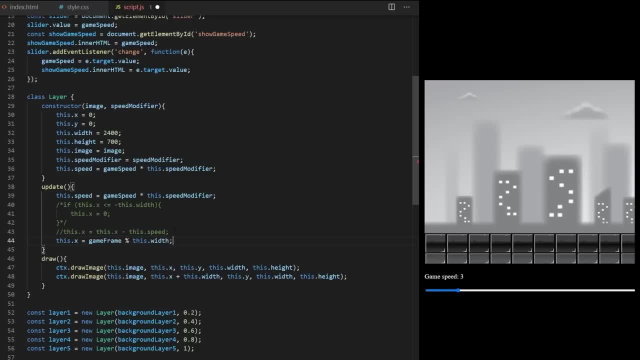 I use remainder operator and thiswidth from line 32.. Thiswidth is currently 2400 pixels and game frame is endlessly increasing number. This calculation will make sure thisx cycles endlessly between zero and the value of thiswidth between zero and 2400 pixels, which will 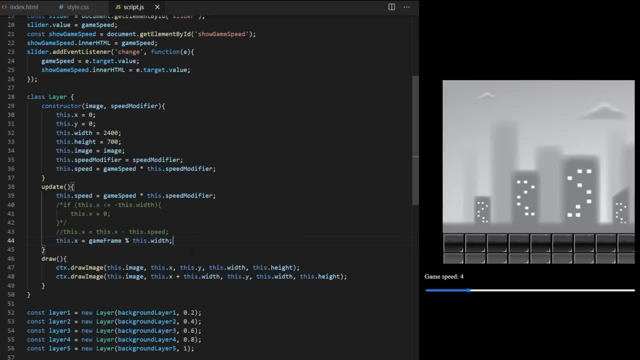 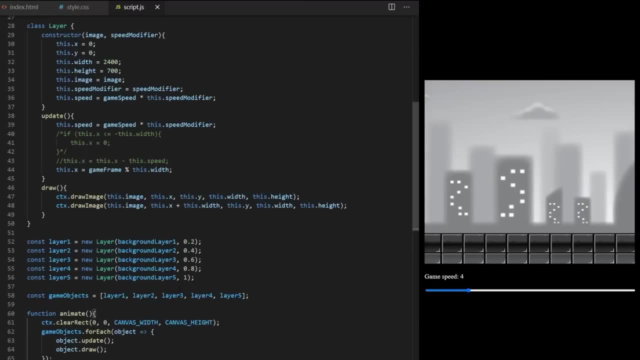 have the same effect as we had before. Oh, it will go to the right. I need to do game frame minus minus on line 66. That's better, But now all our layers are moving at the same speed. I need to factor in thisspeed from line 36 in this. 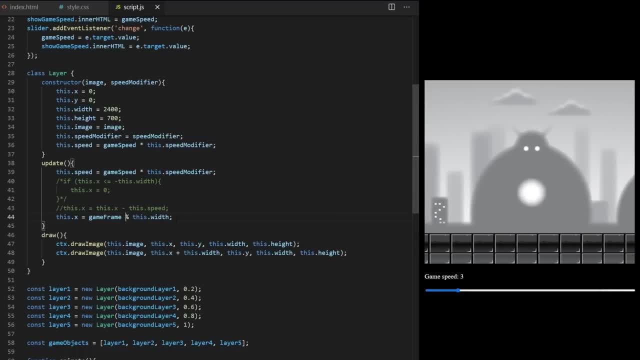 calculation on line 44.. Thisx equals to game frame times. thisspeed, modulus, thiswidth. Now we have the same parallax effect. This one line of JavaScript replaced all the code between lines 40 and 43. I don't think it's very clear and easy to see what's happening on line 44 just by looking at it. 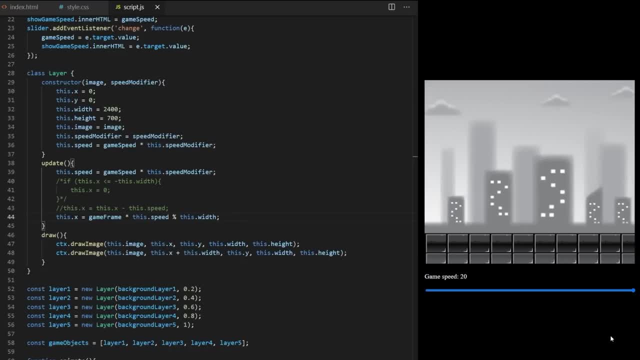 I really have to use my brain and remind myself how modulus operator works to understand why it's cycling between zero and thiswidth. I did a complete breakdown of this technique in my sprite animation video. I will link it in the video description. I'm not going to explain. 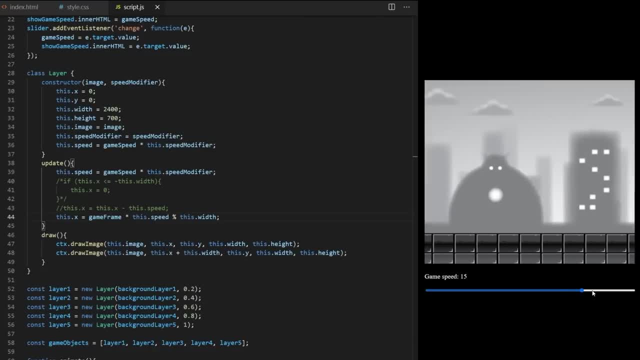 this calculation all over again. I don't think we need to understand this line, Because it has one disadvantage when compared to the code I had previously on lines 40 to 43.. Look, when I change scrolling speed, the position of background jumps somewhere else. because we 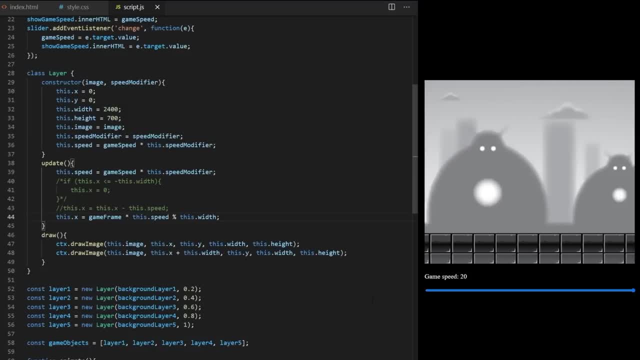 aren't gradually increasing thisx like we did before. We are recalculating that value completely every time game speed changes. Clicking this input slider changes game speed global variable. Changing game speed affects thisspeed because of line 39, and thisspeed changes value of thisx. 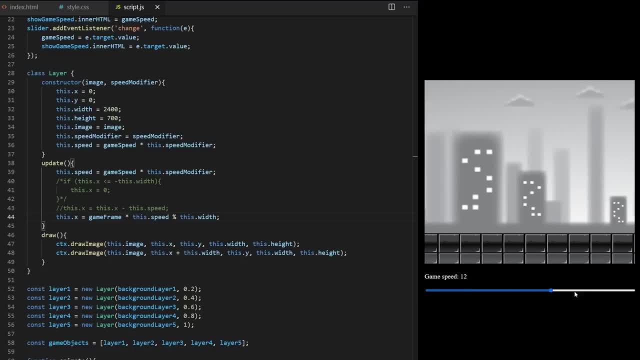 on line 44.. If you know how to use this technique to make it seamless, without jumps in horizontal position when I change game speed, let me know please. I'm sure there is some smart way to do it. I played with it for a while and I couldn't work it out. Do you see how the background jumps? 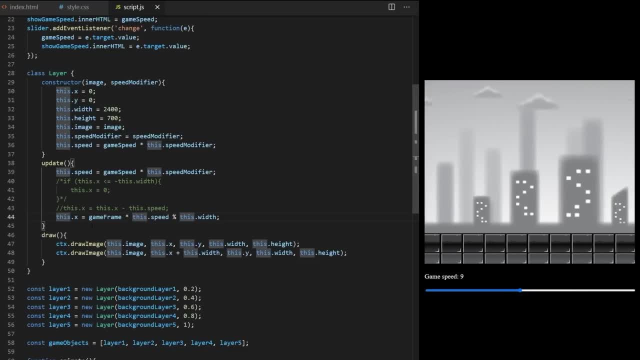 every time I change game speed. Let's comment out these lines so that we can compare it. When using the original technique, horizontal position transitions smoothly without jumps, and that is exactly what I want. I need to be able to change my scrolling speed dynamically, because I 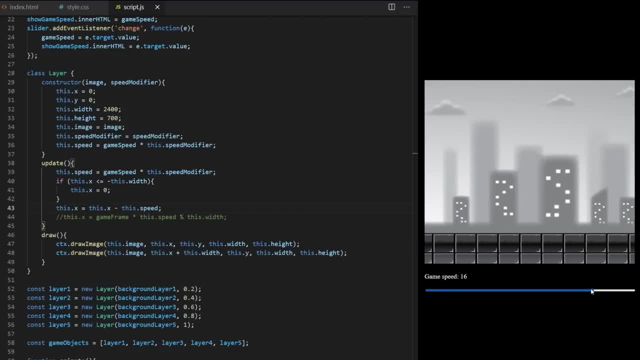 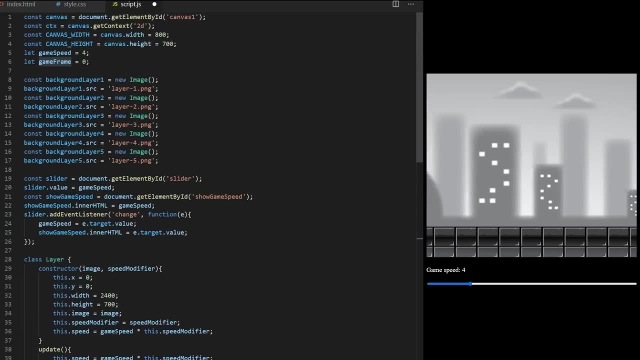 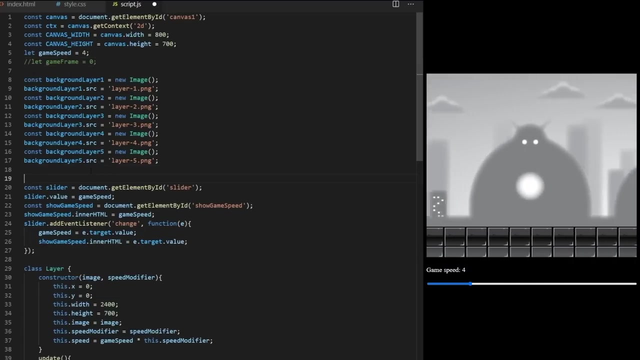 scroll speed of my game to change when a character performs special moves like roll or sit. Let's comment out line 66, since we decided not to use this technique, and I also comment out line 6.. Our images are large. It works well because I'm running my code locally, If this code base was. 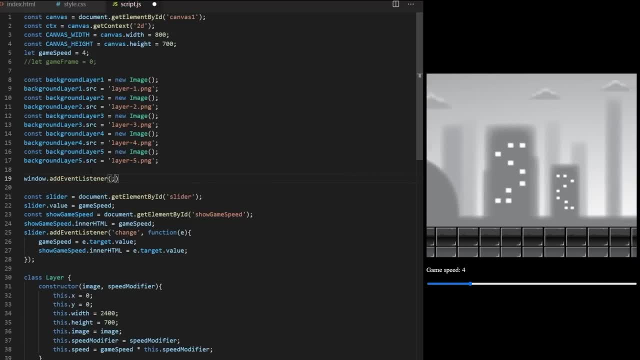 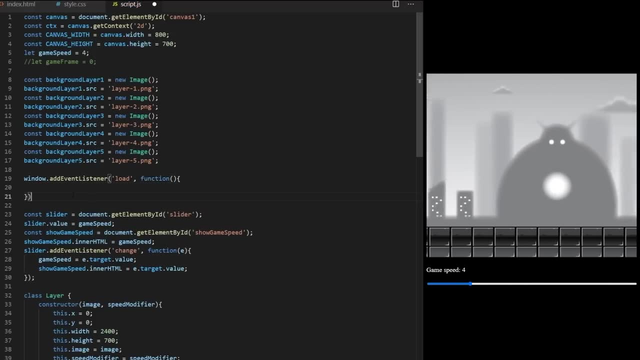 hosted somewhere online. we need to make sure all images and html elements on my page are fully loaded before we start the game. On line 19, I take browser window object and I call add event listener on it. I listen for load event In callback function when the page is fully loaded. 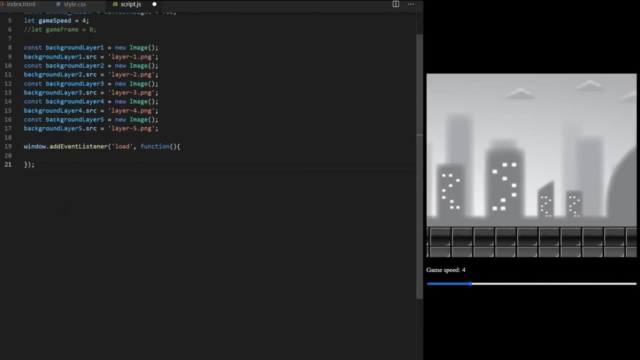 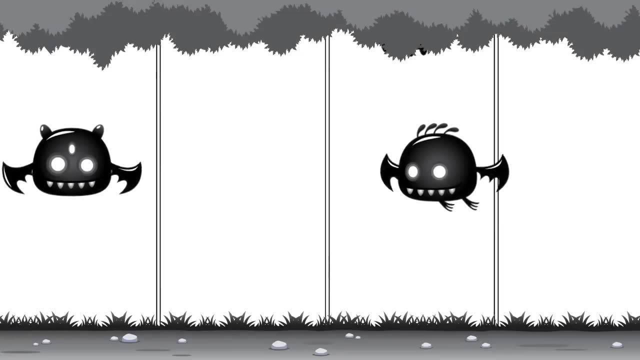 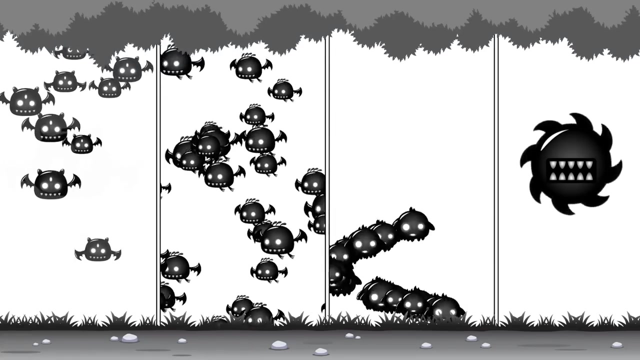 only then I will run all this code That depends on images, canvas and slider element to be properly loaded and available. In this video we will build four small projects completely from scratch. We will learn how to generate groups of animated, computer-controlled characters for our games. 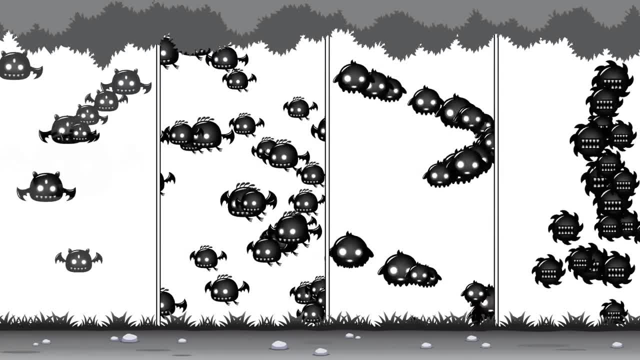 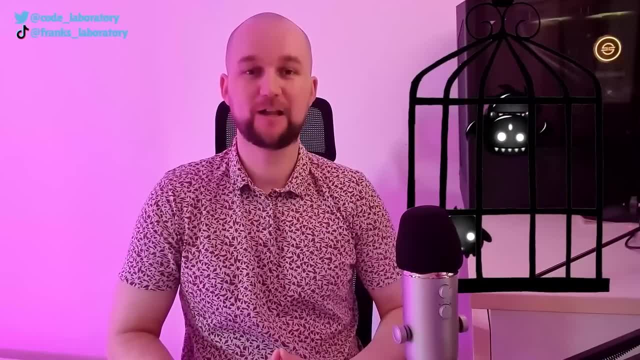 and we will explore four different movement animation patterns. I went to the forest and I caught some dangerous magical creatures for you Today, we will study them and learn how they move. Some of them have wings, some of them spin around and some just float in the air. 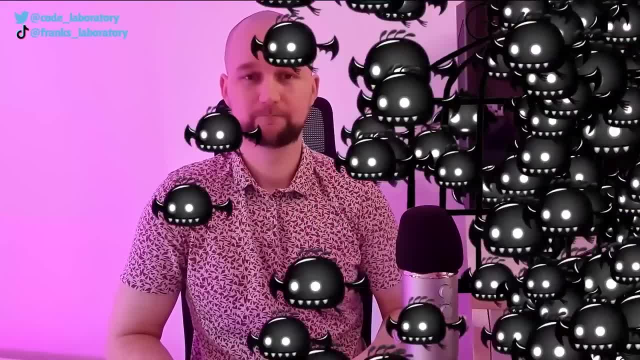 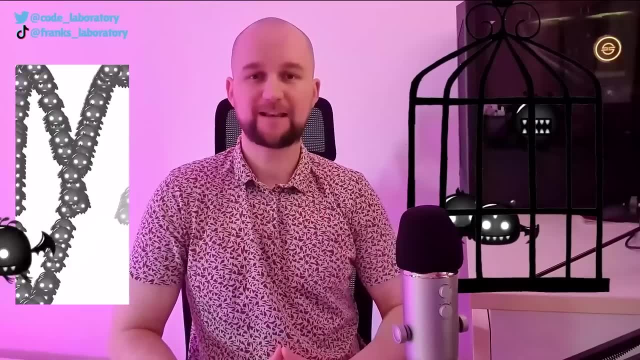 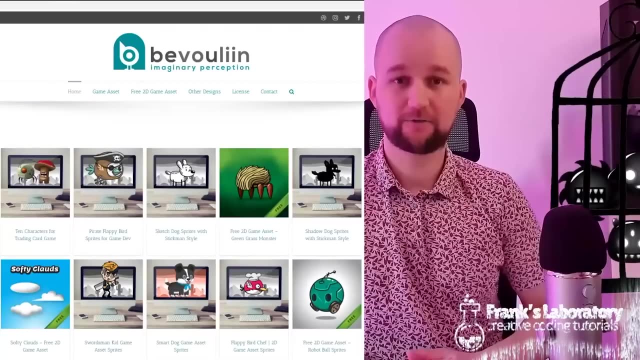 It will be interesting to explore their movement patterns. This is creative coding tutorial for beginners. Let's learn fundamental vanilla javascript principles and techniques by building fun projects together. Hope you get a lot of value today. Art for this episode was made by this amazing artist. 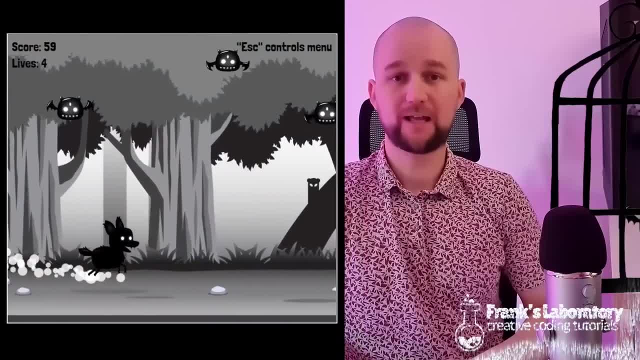 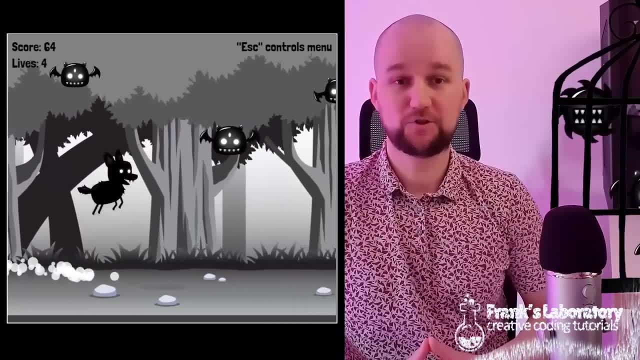 Go check out his website if you want to see more. We will cover four different movement animation techniques and by the end of this video you will have four complete projects and you will be able to introduce a variety of different enemies and movement patterns to your personal javascript games. 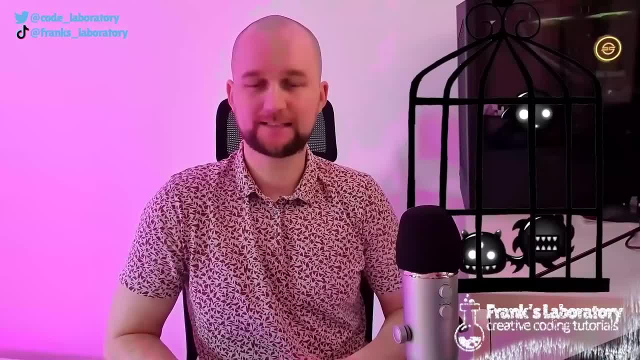 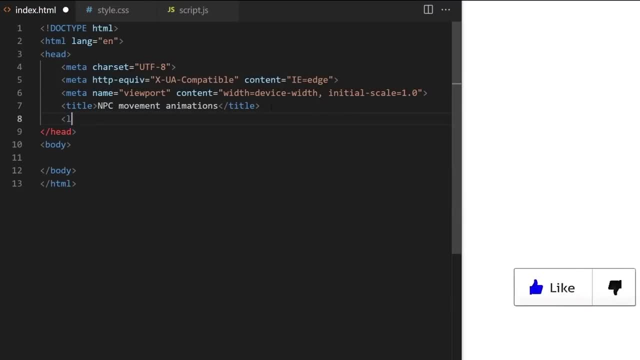 Sometimes we tend to make our games too easy and predictable. Let's give our players some challenge by including different enemy types. I create a simple web page markup, I give it some title, I link stylescss File in document head. We will draw everything on canvas, so I create it here and I give it id. 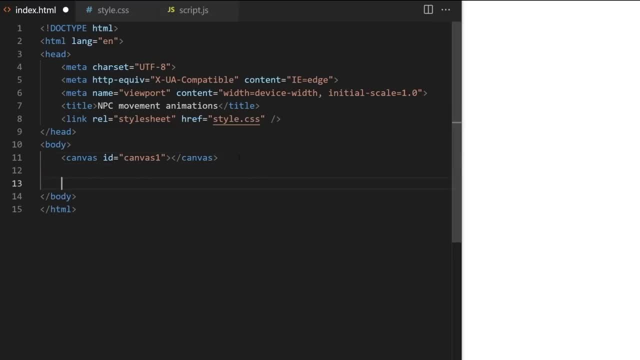 canvas1 so that we can target it with css and javascript later. I also link my scriptjs file which will contain all animation logic In stylecss. I take my canvas element I just created and I want to give it some border size and I want to center it in the middle of the page. So border. 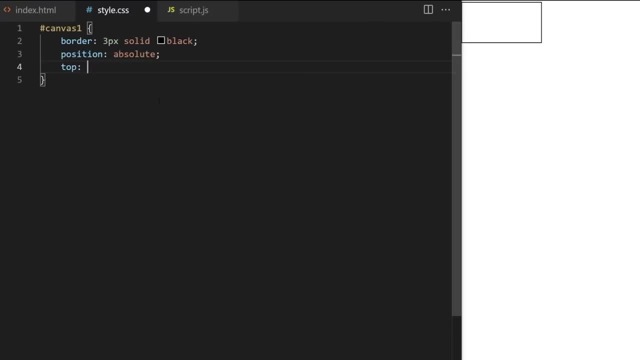 three pixels. solid black position: absolute top: fifty percent left. fifty percent. transform translate: minus fifty percent. minus fifty percent. now it's in the middle. Let's make it vertical. so height: thousand pixels. width will be, for example, 500 pixels. Everything else will be drawn with code in scriptjs. 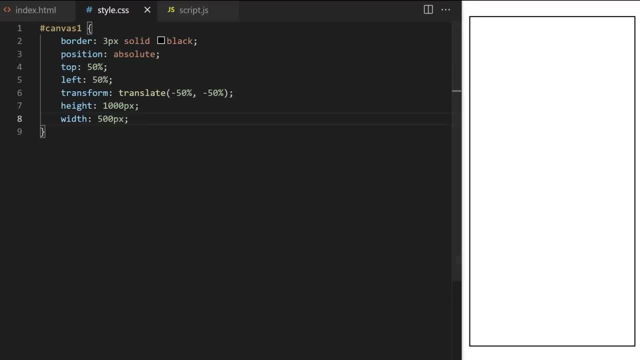 file. This is a beginner tutorial, so don't worry, I will take you through it step by step. As with every canvas project, I need to point javascript towards my canvas element. we just create it in index html. I do it by using getelementbyid and I pass it id. I gave my canvas. 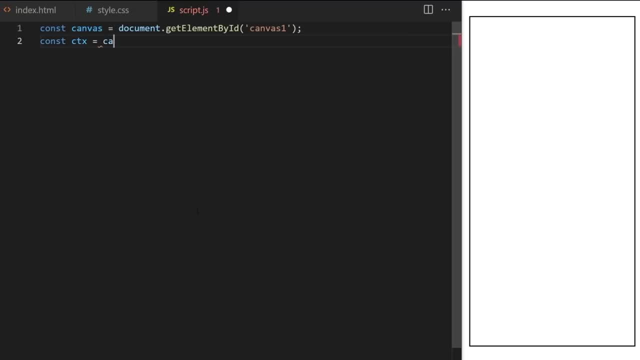 element canvas1, like this CTX shortcut for context is equal to canvas dot getcontext and I pass it 2D. We will use a built-in set of 2D drawin methods today. Now I can call all these: 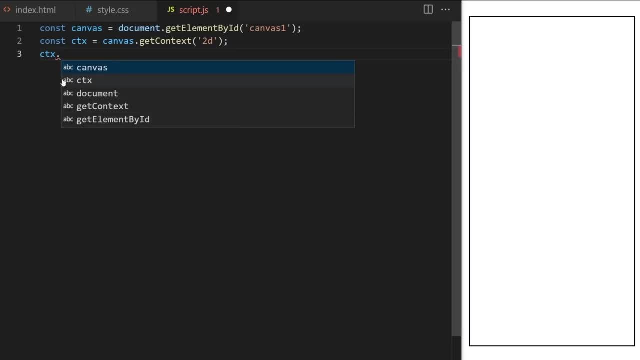 built-in methods from my CTX variable. If I type CTX dot like this, you can see that in VS code editor my autocomplete feature doesn't suggest any built-in canvas methods. If I want them to be suggested, I can go up to line 1 and type add type: HTML canvas element like this: 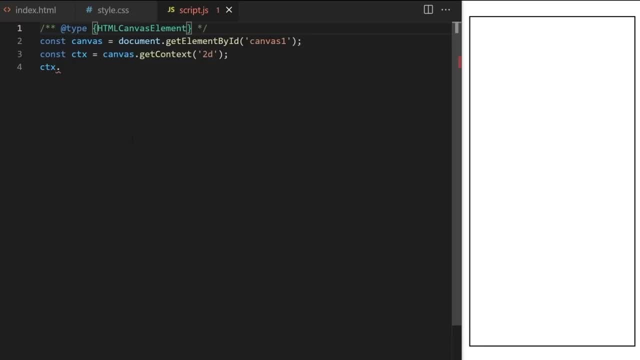 This way I tell VS Code this is a canvas project and it will suggest built-in HTML canvas methods for me. You can see arc method here to draw a circle, clear rectangle to delete paint from canvas, and so on. We will use some of these in a minute when we start drawing and 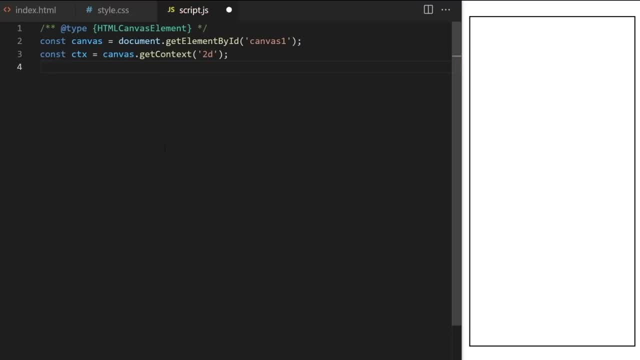 animating. But first let's quickly finish canvas setup. We need to set canvas width and height to make sure we get correct scaling of our drawings. So I create a custom global variable called canvas underscore width. I set it equal to canvas from line 2, dot width and I set it all equal to 500.. 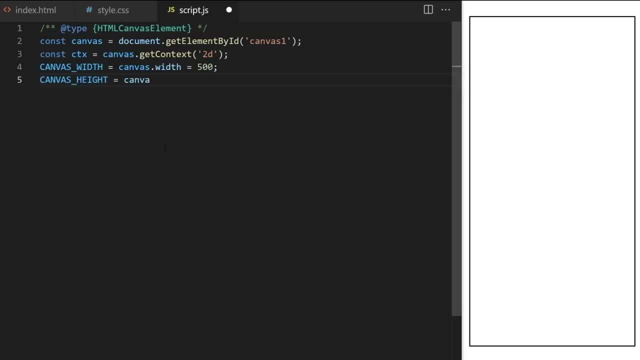 Canvas underscore height is canvas dot height is equal to 1000.. These values need to be the same. I gave it in stylecss. I want to make sure that canvas is equal to canvas height. I want to make sure that canvas is equal to canvas height. I want to make sure that canvas is equal to canvas height. I want to. 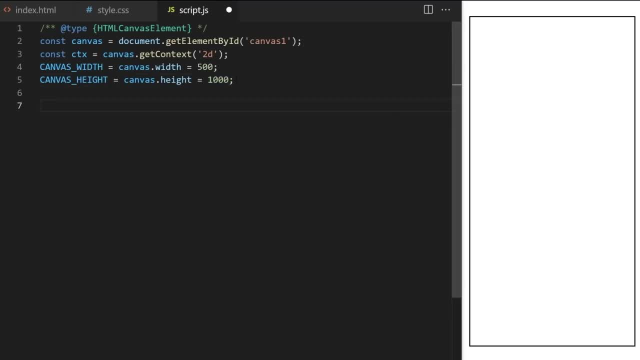 create a factory function that will produce many similar objects. for me, Each of these objects will be one animated enemy. Before we create many enemies, let's just build one and make it absolutely clear for beginners what's going on. When we have that, it's easy to scale it up. I will create a. 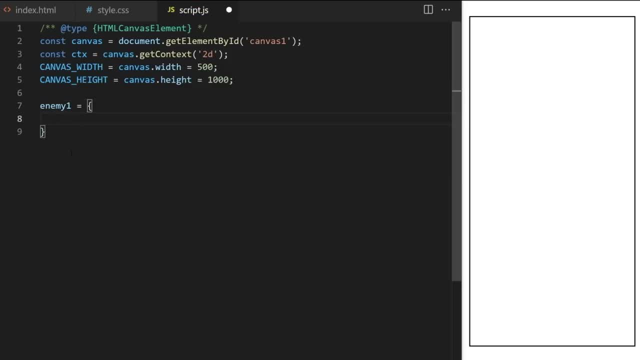 temporary enemy, one variable, and I set it equal to javascript object. I give it x and y properties and I set them to zero. These will represent horizontal and vertical coordinate on canvas where we draw that enemy. I will also give it width of 200 pixels and height of 200 pixels, like this: 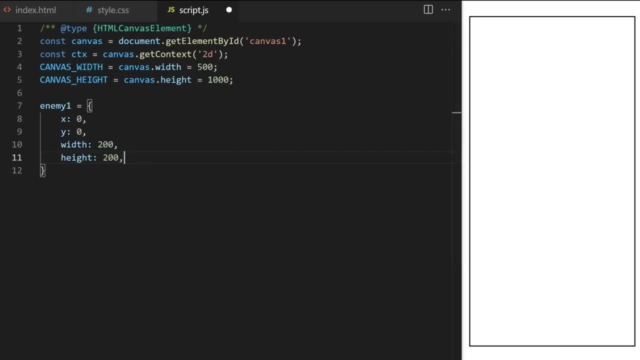 So now I have this simple javascript object that is storing position and size of one enemy. Let's animate it. To create animation loop, I like to write a custom function. I call, for example, animate Inside. I call built-in fill rectangle method. This method expects x, y, width and height. 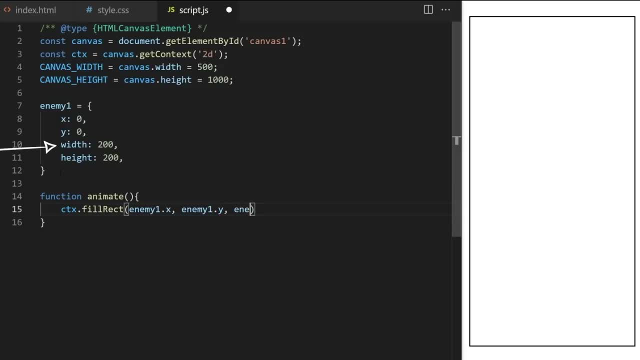 of the rectangle we want to draw, so I will give it x, y, width and height of this enemy object. When I call animate like this, we are drawing a black rectangle representing the enemy object. I can change its values and when I refresh the page it will be reflected on canvas. 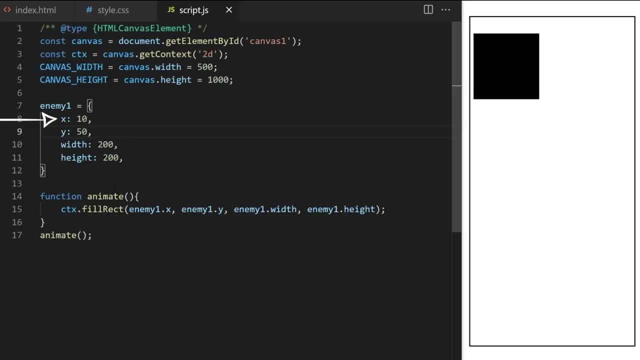 We are not animating yet. What if I want the horizontal x position to be slowly increasing to make the enemy travel to the right? I can say, for each run of animation loop, increase enemy 1.x property from line 8 by one To create animation loop. I call built-in request. 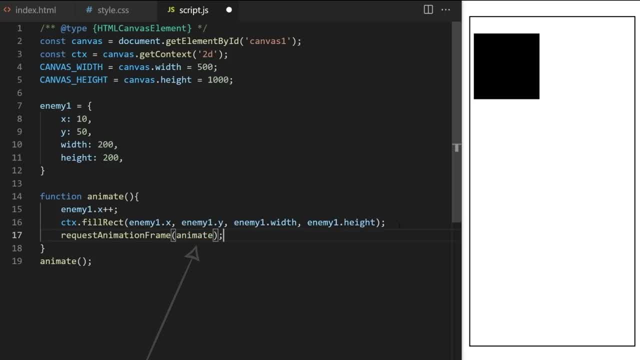 animation framer method. I pass it animate Now. animate will run all its code and then it will call itself again. This will create an endless animation loop. I also need to delete old paint, previous frames from canvas. I do it by using built-in clear. 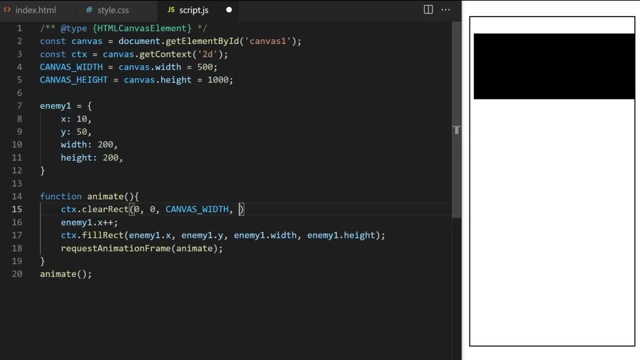 rectangle method and I clear canvas from coordinates 0, 0 to canvas with canvas height. Now we see only the current animation frame. I can also increase vertical y position by 1 for every frame, so we get movement towards bottom right like this. 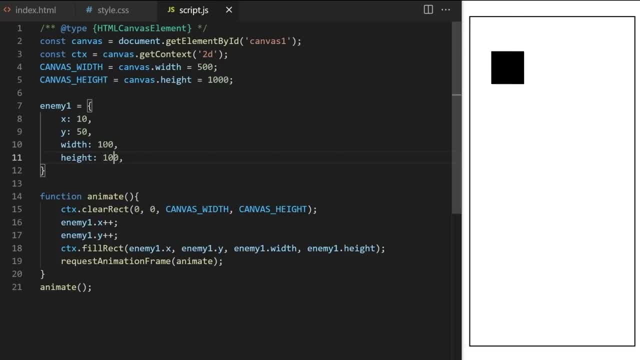 I can change width and height of my enemy easily. You get the idea. I think Let's comment out this temporary enemy object and make it into a javascript class so that we can generate a large number of enemies at once. Javascript class is kind of a template to create many similar object. 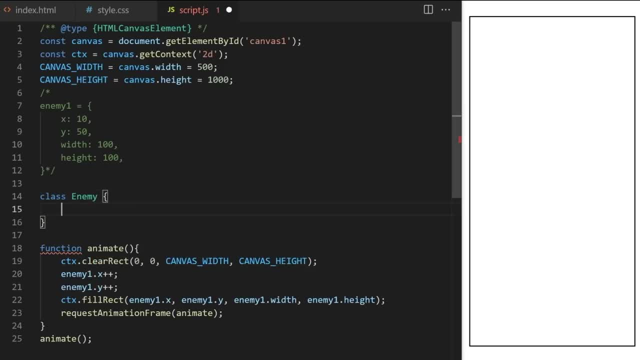 It's a factory and every time we ask it, it will produce one new object for us Based on a blue line. it will generate a new object for us Based on a blue line. it will generate a new object for us Based on a blue line. it will generate a new object for us. 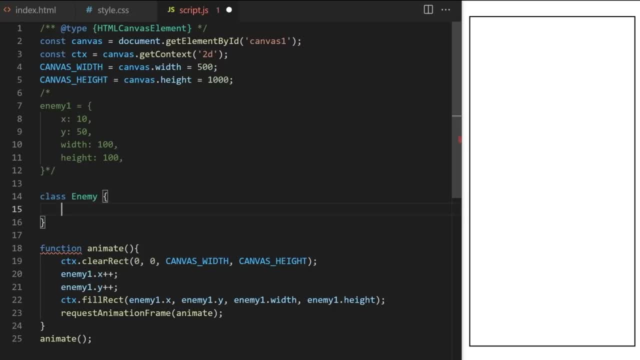 This is the blueprint we give it. Classes are a new syntax for older javascript prototypes. Under the hood, it's the same thing. It's just so-called syntactical sugar: Simpler, nicer way to do the same thing. Classes are very easy and intuitive. Let me show you. 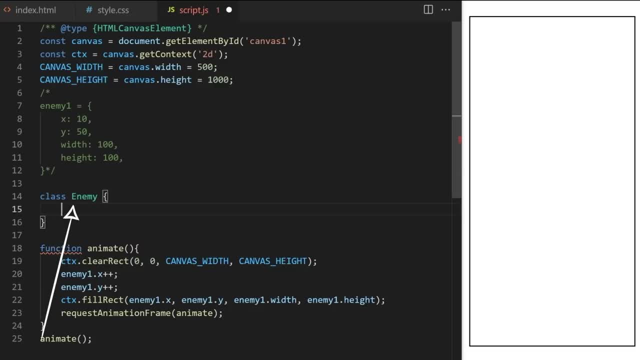 We use class keyword and then rename our class, starting with a capital letter. My class will be called enemy. Constructor is a mandatory method every class must have. It will contain a blueprint based on which every enemy object will be created. So here in constructor, I'm going to name my class: enemy. 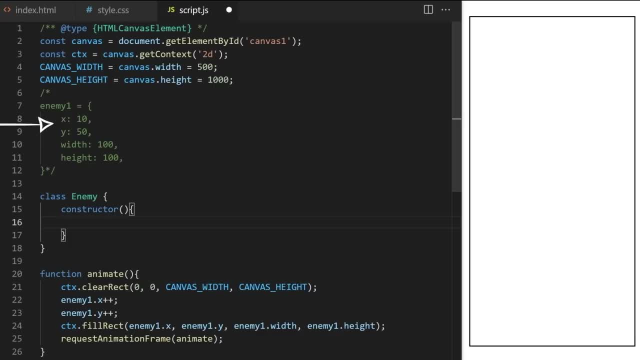 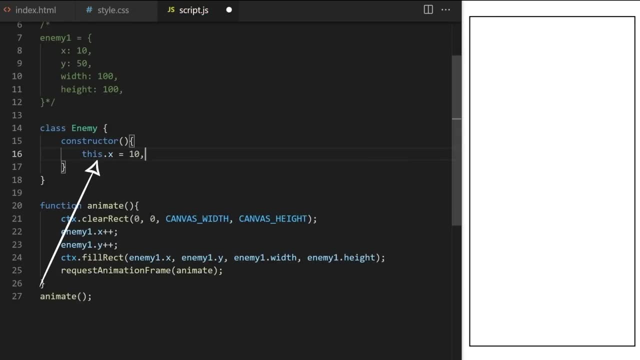 I just give it x, y, width and height, Same as we had in this simple enemy object on line 7.. The syntax might be a bit strange at first. Here I'm telling my constructor on this new enemy object you are creating right now. 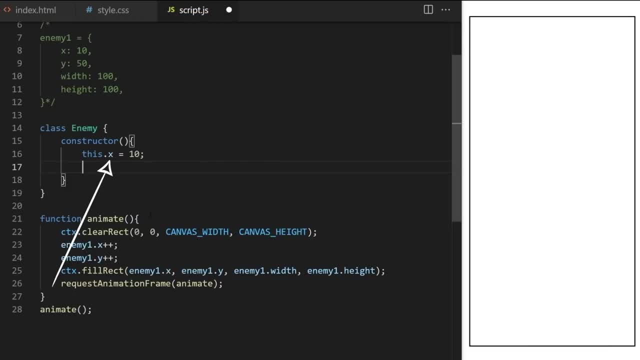 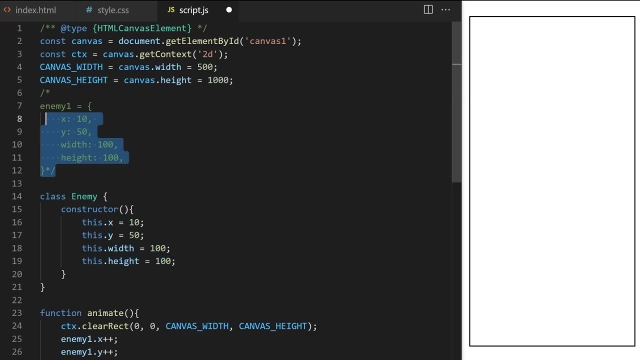 give it property called x and set it equal to 10 pixels. Starting vertical y coordinate will be 50 pixels, Width will be 100 pixels and height 100 as well. So this is how you recreate single javascript object. Now we can call our enemy class as many times as we want, and each time it will generate one new enemy for us. 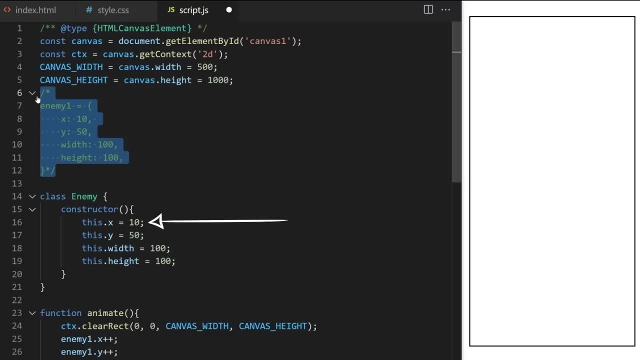 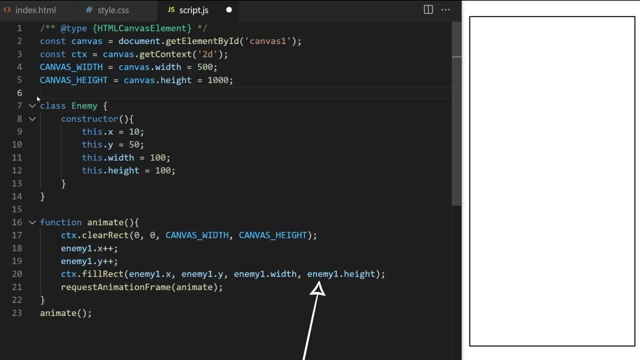 Based on a blueprint inside constructor method between lines 16 to 19.. I can delete the old code And now these variables are undefined because enemy1 doesn't exist. So I create a new constant variable called enemy1 again And I set it equal to an instance of my new enemy class. 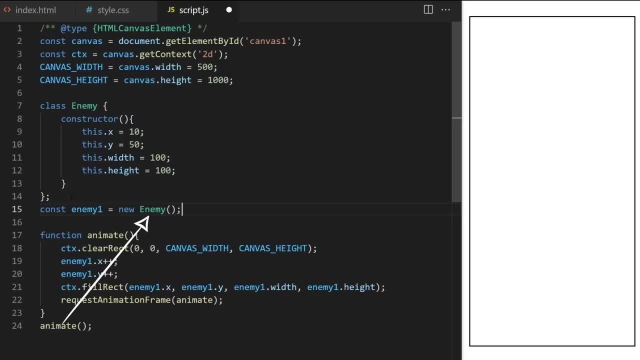 To do that, I use the new keyword followed by a class name. The new keyword will simply look at that class name in my code. It will enter its constructor, It will create one new blank javascript object and it will assign it values and properties based on a blueprint inside the constructor. 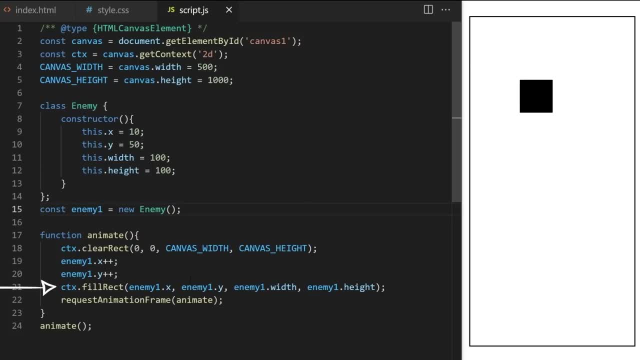 Now my fill rectangle method on line 21 can use these values again to display a rectangle. What if I want another enemy? I can create another variable called enemy2 and I set it to new enemy again Inside animation loop. I take enemy2 and I increase its x and y coordinates as well. 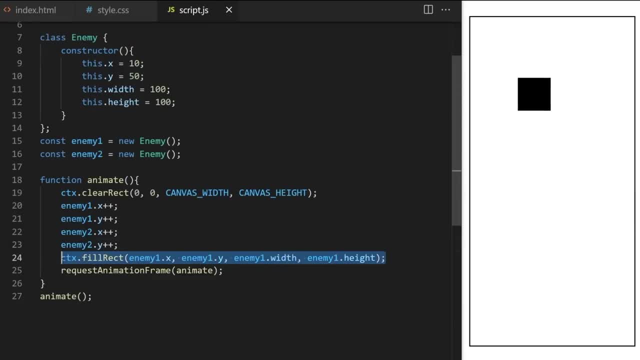 And on line 25 I need to draw another rectangle representing that enemy. like this: They are moving at the same speed in the same direction, so we can't see the second one. Let's adjust its speed, for example. Now we can see that there are two of them. 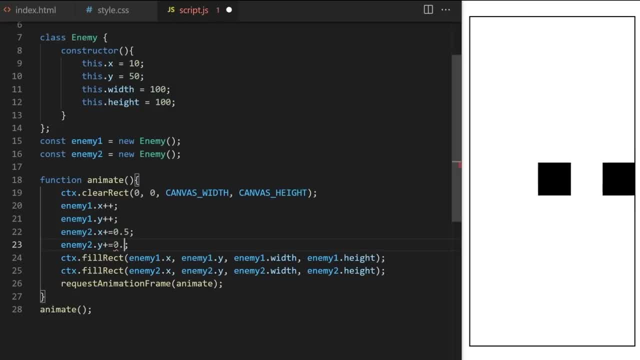 We can control them separately, like this, but this wouldn't be very efficient if we had, let's say, 50 or even 500 enemies. So how do we make this? How do we make this code better and remove repetition? First, let's output this code between lines 21 and 24, that handles movement along x and y axis. 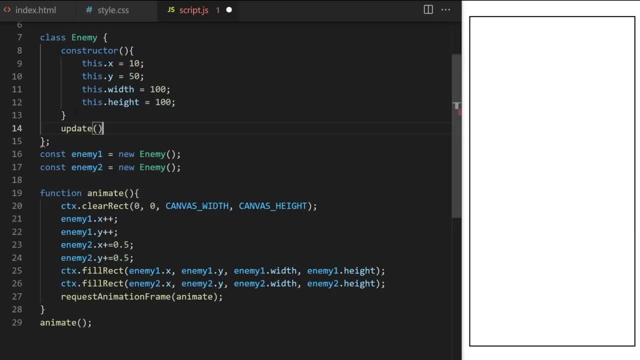 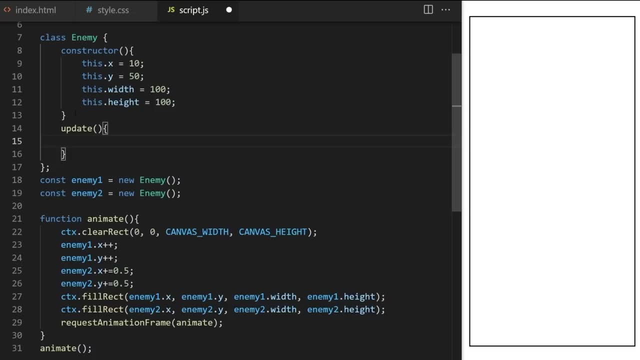 into a shared class method. That way, we can write this code only once and it will be available to all objects created by enemy class. I will call that custom function, for example, update, and, as I said, its job will be to update coordinates of my objects. 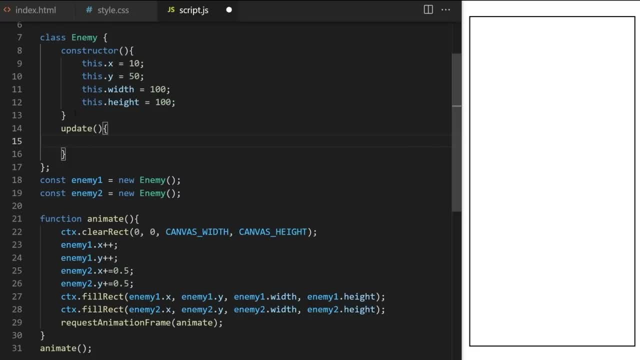 It will handle position calculation and movement. So inside I say, for example: update For every frame, increase x by 1 and also increase y by 1.. Let's delete all this code and to run update method I just created, all I have to do is call enemy1.update, like this: 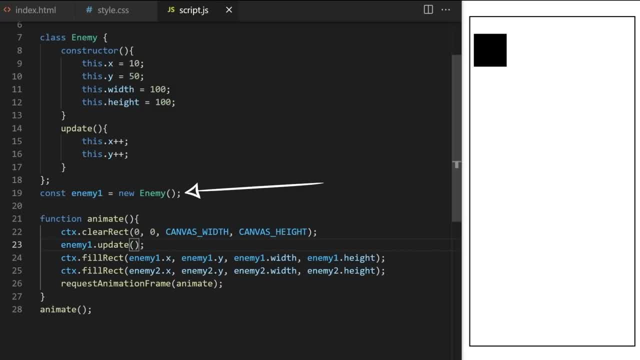 Since enemy1 object was created here on line 19 as an instance of my enemy class from line 7, it automatically has access to this new update class method from line 14.. I also need to remove line 25.. So now we put all movement calculation functionality into this update method. 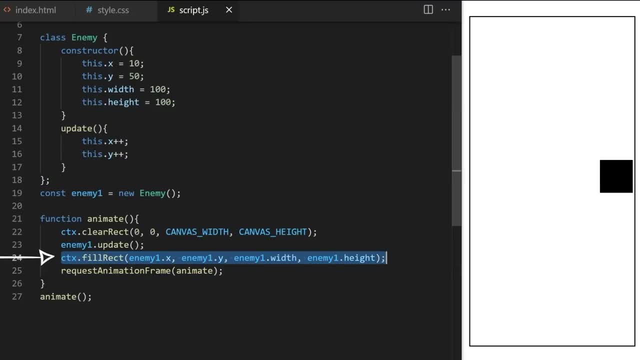 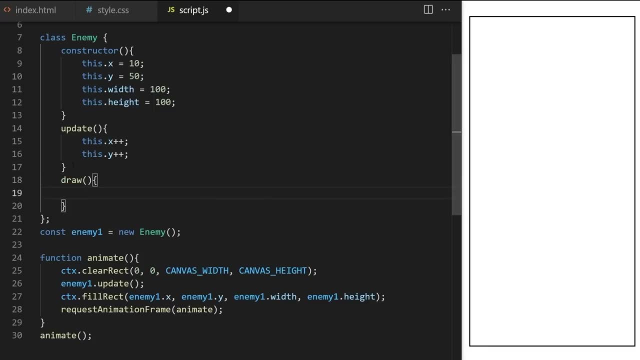 I also want to put this drawing code into its separate method, so that we can draw all enemies at the same time. We can also give them animated sprites and so on. I will show you in a minute. On line 18, I create a custom draw method. 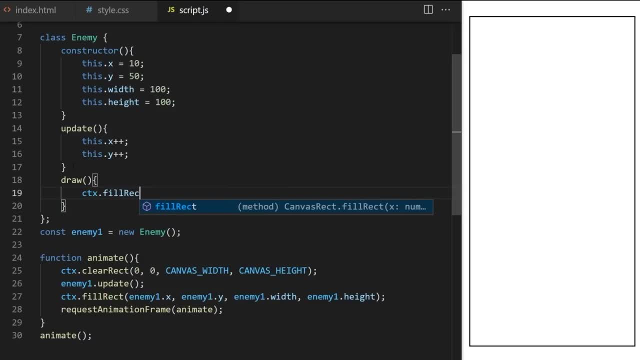 Inside I call ctx fill rectangle, the same way we did here on line 27, but instead of hard coding enemy1 object, here like this, I will use this keyword. That way this method will be reusable and can animate not only enemy1 but also enemy2, enemy10, enemy100., 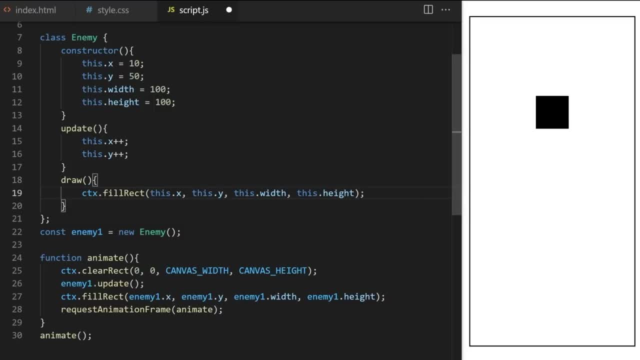 It can animate all the enemies created by this class at once. On line 27, I can replace these hardcoded values with enemy1.draw. It will look the same, but now it's reusable and scalable. Inside constructor. between lines 9 and 12, all enemies start at the same x and y coordinates. 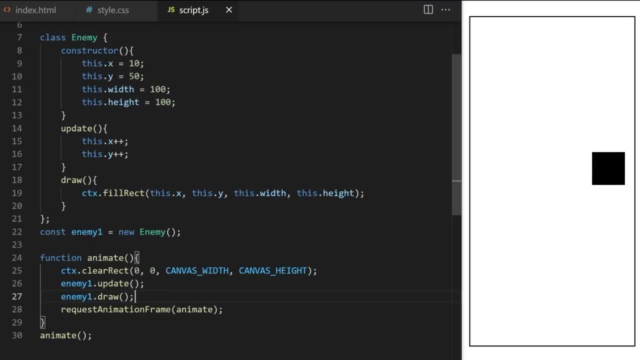 So if I create 50 enemies, they would all stuck on top of each other and wouldn't be visible. Let's randomize that. Every time I create a new enemy, its horizontal x coordinate will be a random number between 0 and canvas width. 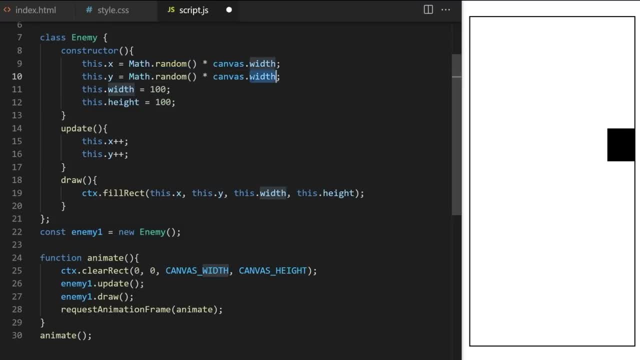 And vertical y coordinate will be a random number between 0 and canvas height. Now every time I refresh page, my enemy appears at a different position. I could also randomize width and height if I wanted to, to make each enemy random size. I think you get the idea. 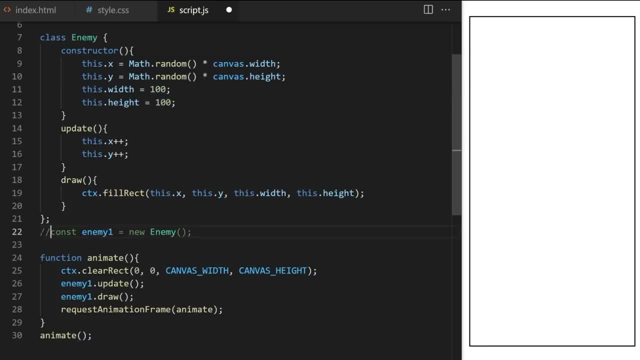 So how do I create many enemies instead of just one? I comment out line 22 and I create a for loop. This for loop will run, for example, 100 times. Actually, let's go up to line 6 and create a constant variable called the number of enemies. 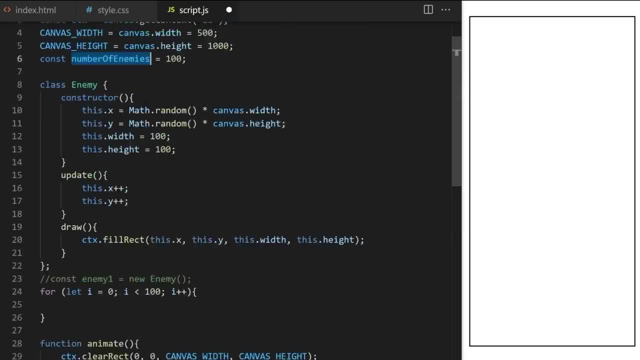 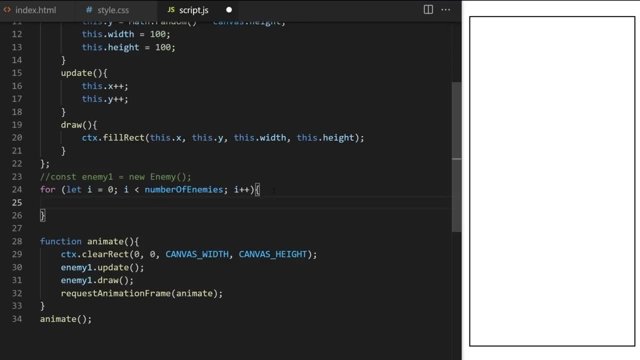 and set it to 100.. And I replace hardcoded 100 on line 24 with this new variable. That's better. We shouldn't be hardcoding values if we can avoid it avoided. I want this for loop to run 100 times and create 100 enemies for me using my custom. 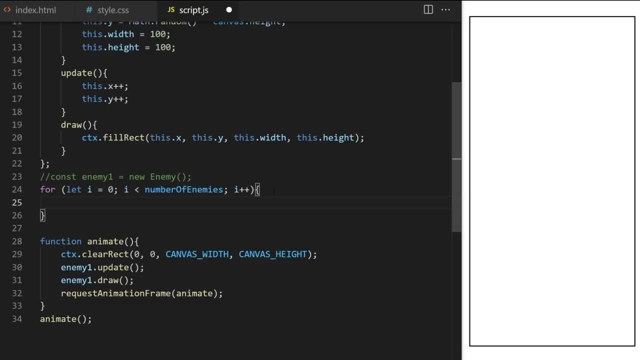 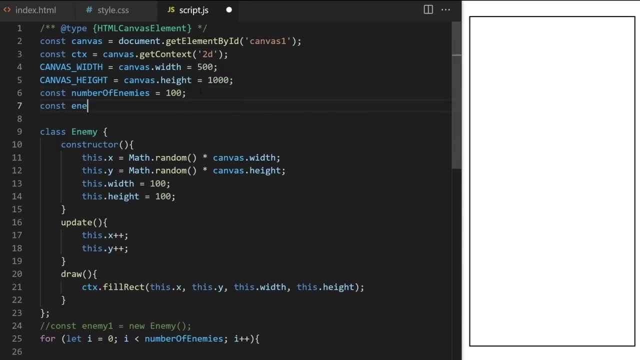 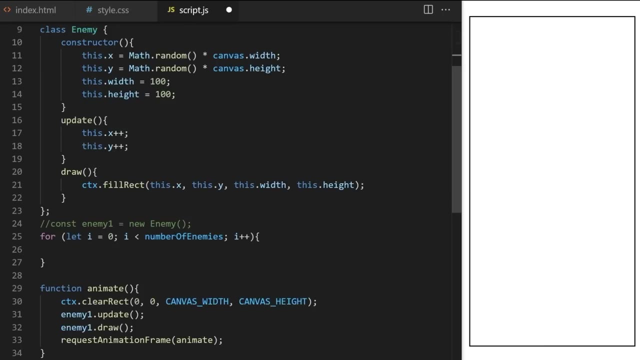 enemy class. But how do I store all these enemy objects and their properties, such as their x and y values? I can, for example, go up here to line 7 and create a custom variable called enemies array and I set it equal to an empty array. Down here on line 26. I take that enemies array and I call: 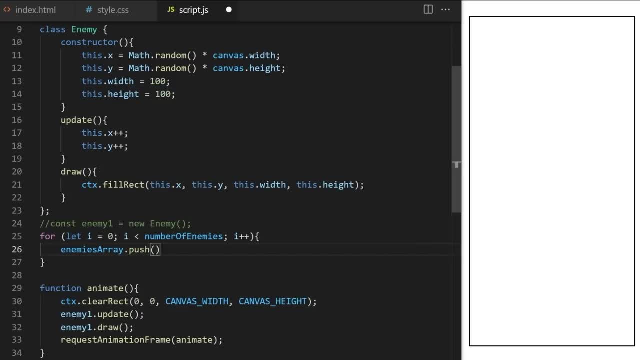 built-in array push method. Push method will just take whatever we pass to it and it will push it to the end of the array. I pass it new enemy Every time this for loop runs and it will run 100 times. it will create one new enemy using my enemy class constructor and it will push that new enemy into. 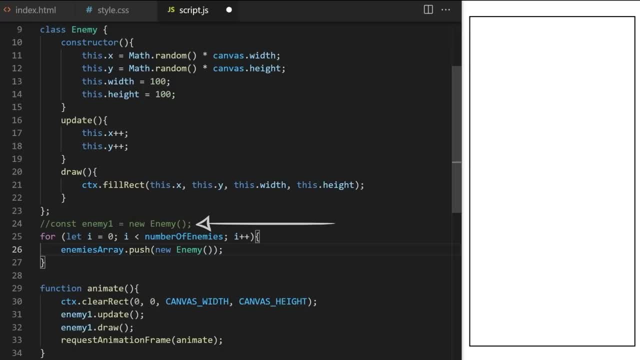 enemies array. It's the same as we did with enemy 1 on line 24, but here we are doing it 100 times. Let's do it again. Delete line 24.. I also have to comment out lines 31 and 32 because enemy 1 variable doesn't exist. 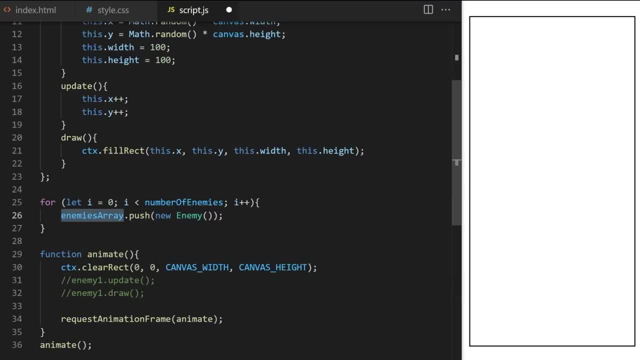 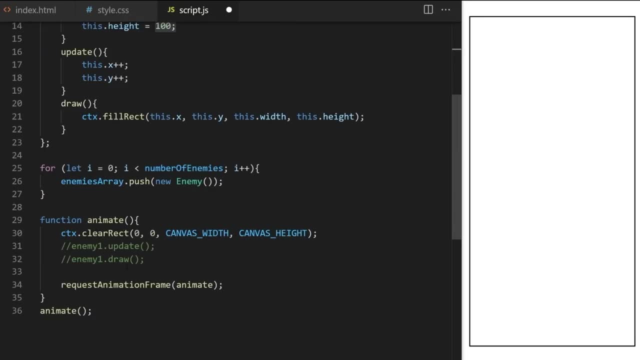 anymore. How do I access all these 100 objects I just pushed into my enemies array and how do I trigger their update and draw methods one by one so that they can be animated on canvas? First, let's consolelog enemies array to make sure that for loop on line 25 did its job, and 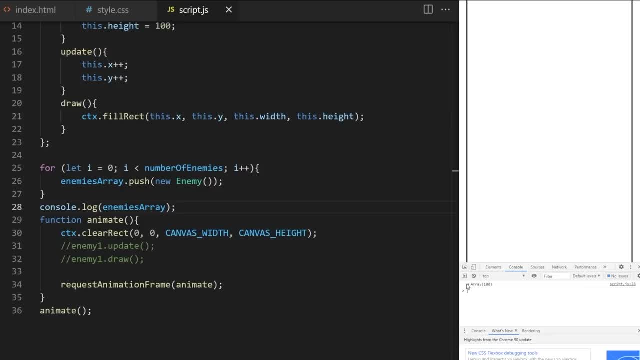 filled it with 100 objects. In console I can see we have 100 enemies and each one has randomized x and y coordinate- perfect. So, as I said, the goal now is to cycle through all 100 enemy objects inside enemies array and to trigger their update and draw methods. 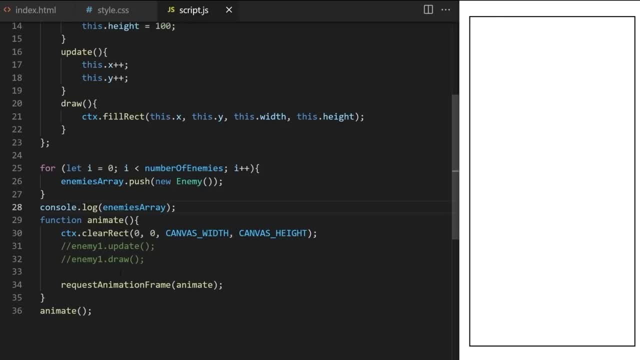 This will need to happen for every animation frame, over and over, because we need update method to constantly recalculate enemy position and the draw method to draw them at that new position. On line 33 inside animation loop, I take enemies array that contains my 100 objects and I call built-in array for each method. For each simply calls provided. 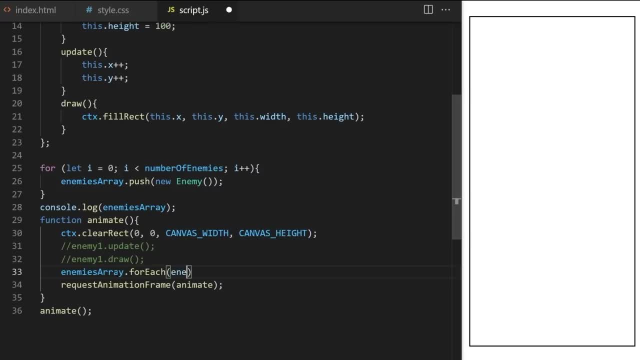 callback function for each element in the array. I will use new es6 syntax with arrow function here Inside my. for each callback refer to each individual object as enemy as you cycle through enemies array and for each of these objects call their associated draw method and also their update. 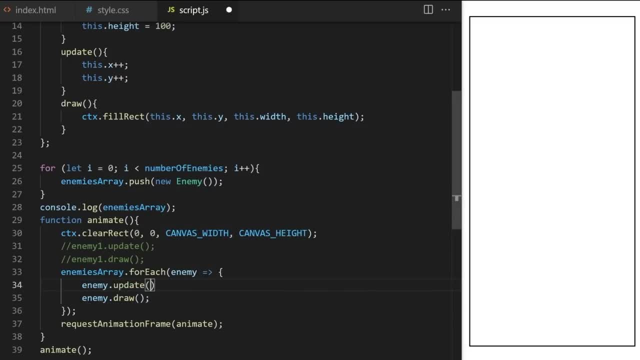 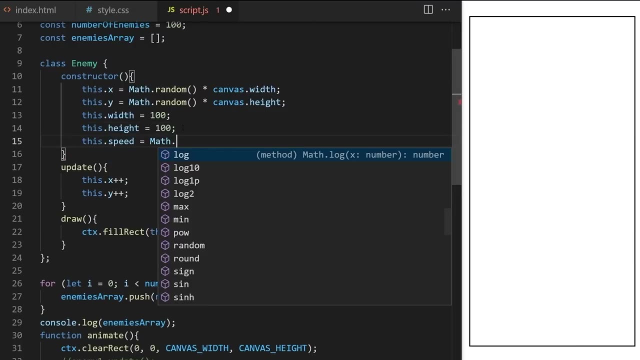 method like this, Perfect. you can see that each rectangle appears at randomized x position and they all move in the same direction because of lines 17 and 18.. What if my enemy had randomized speed? I create a new property called thisspeed and I set it equal to a random number between minus 2 and plus 2. 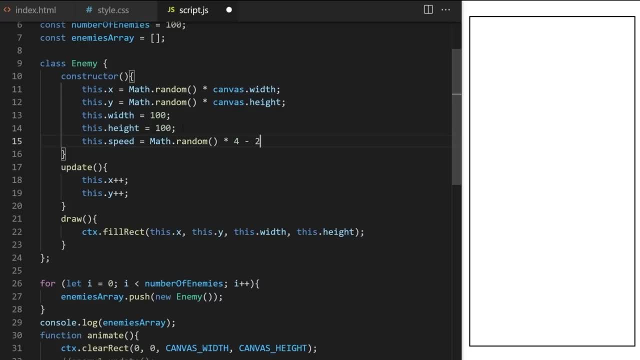 because I want some of them to go to the left and some of them to go to the right. If you find it hard to read this line of code as a random number between minus 2 and plus 2, think of it this way. This part of code generates a random number in this range, so between 0 and 4. 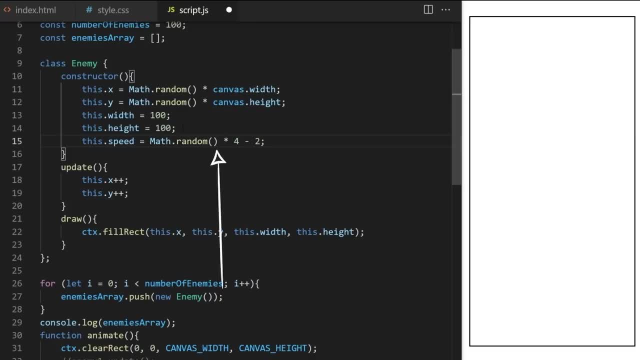 and this number sets the start of that range. so we are generating a random number between 0 and 4, but we are pushing that range to start from minus 2. so result we get is a random number between minus 2 and plus 2.. I remember I always found mathrandom very unintuitive until I found a better way to. 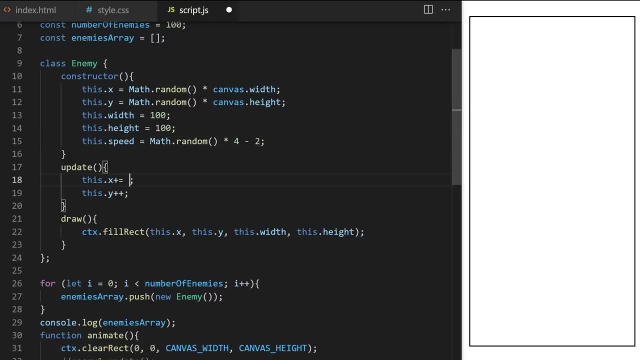 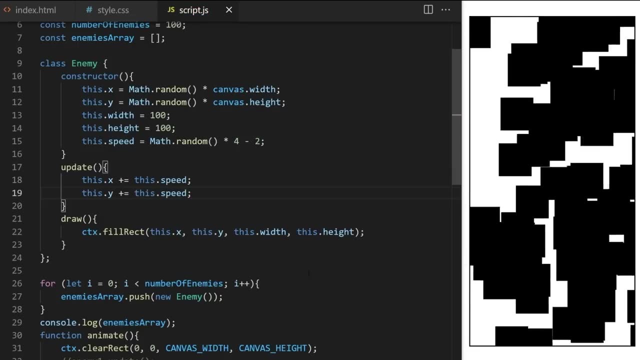 think of it. Anyway, now I have thisspeed property and I can use it to create a random number between minus 2 and plus 2.. I can replace it here, on line 18 for horizontal position and also on line 19 for vertical position. Now you can see we have rectangles moving in many different directions. 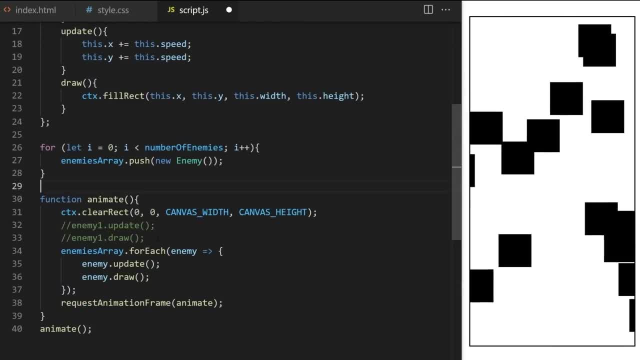 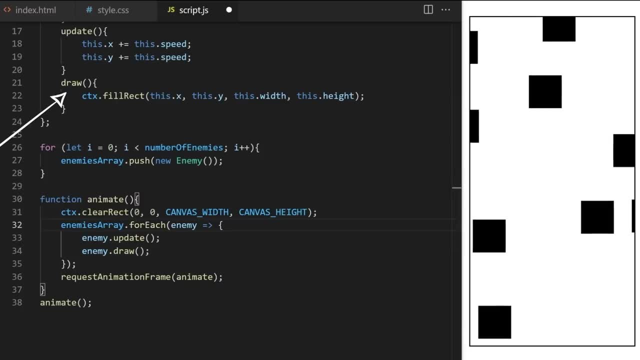 I delete code on line 29 and also on lines 32 and 33.. On line 21, inside draw method: our enemies don't have to be represented by a black rectangle. We can write any drawing code here and it will be called and replicated for all enemies at once. 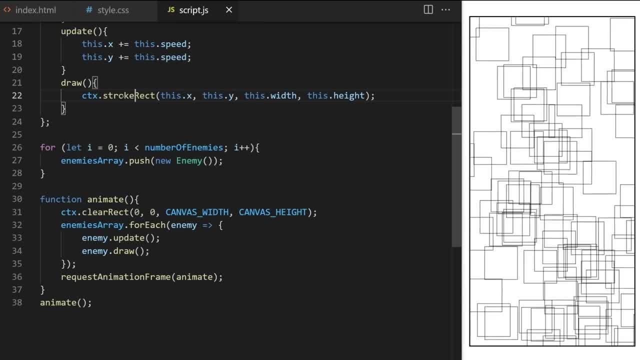 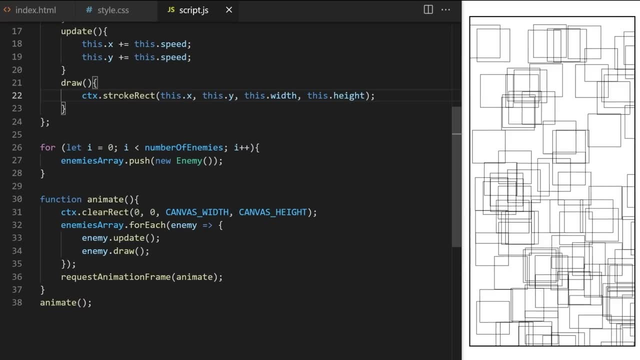 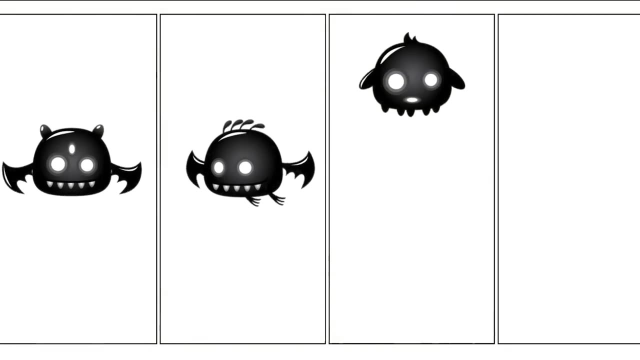 I can, for example, try stroke rectangle instead. We can also draw circles, stars. You can put selfies from your holidays to represent each enemy object. here We have complete flexibility. What I want to do here is to create animated creatures, because we want these to be enemies for our javascript games. 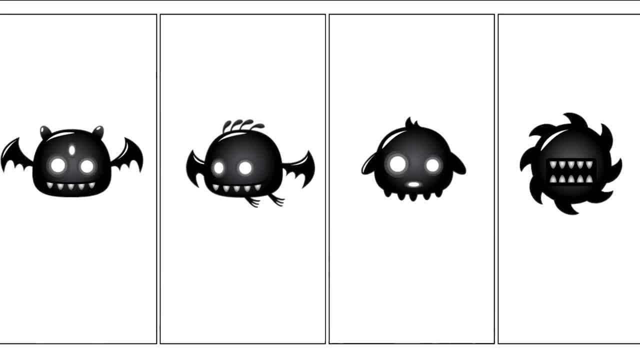 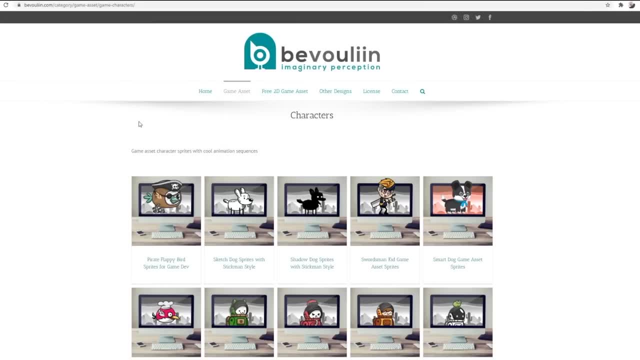 With this video, we are giving away four different animated enemies drawn by this amazing artist. Go check out his website for more content. He is very talented. He allowed me to share these sprites with you for educational purposes for free. I hope you enjoyed this video. If you did, don't forget to like, share and subscribe to my channel. Thank you very much. See you in the next video. Bye. 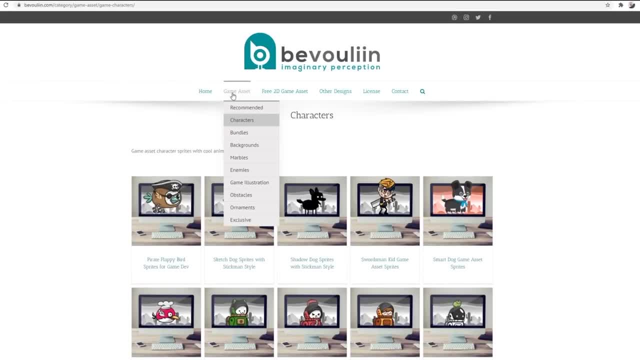 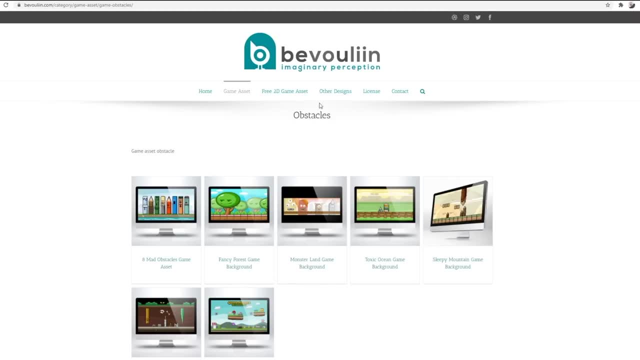 you can download them in the video description and you can also find link to his website there. if you want to use these sprites for commercial purposes, you would have to go to his website and buy a full license. they are free only for purposes of this educational video. show him some support if 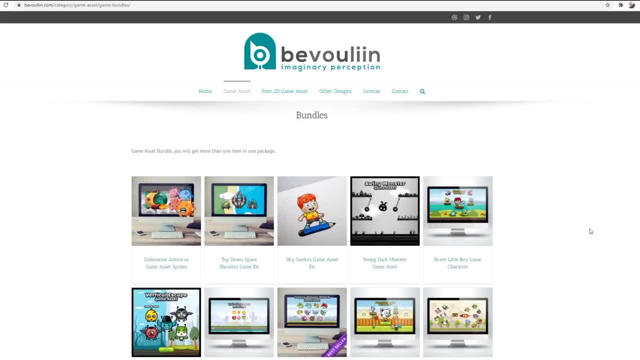 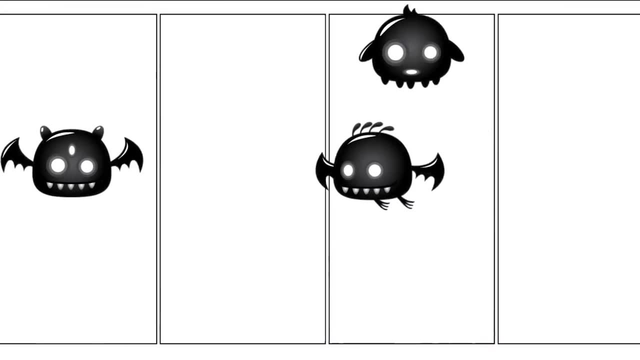 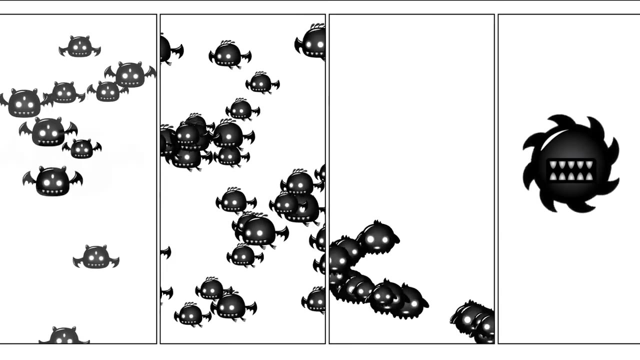 you can. we don't have many good 2d artists like this. if we support them, they will be able to create more beautiful game art assets for us. today we will create four different projects. each one will have different enemy with a different movement pattern, and on each one we will demonstrate different beginner friendly movement animation. 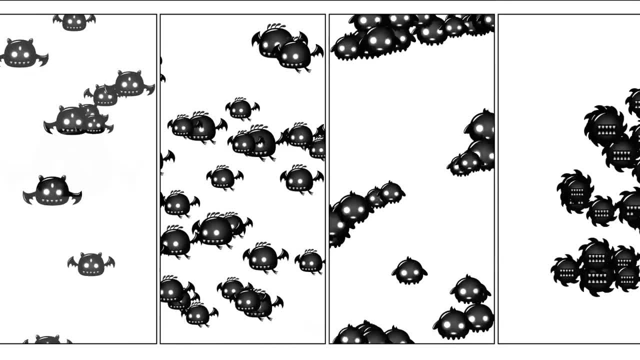 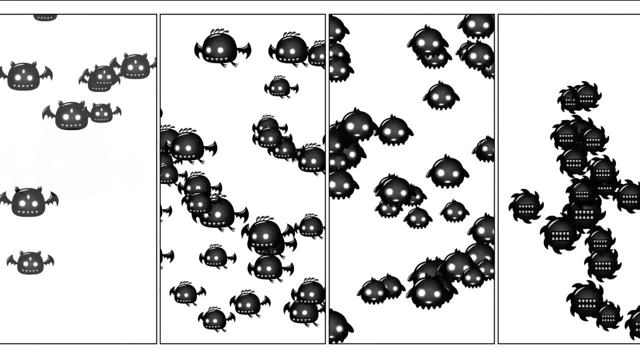 technique. i want you to always have a nice complete project at the end of my videos so that you have something to show to your friends or on your coding portfolio. it feels good to complete something, don't you think you can use these as animated backgrounds or a screensaver? 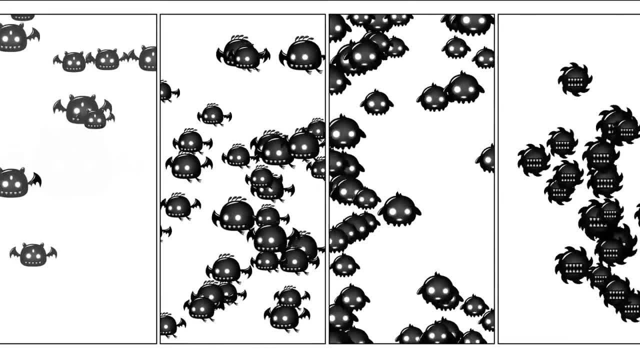 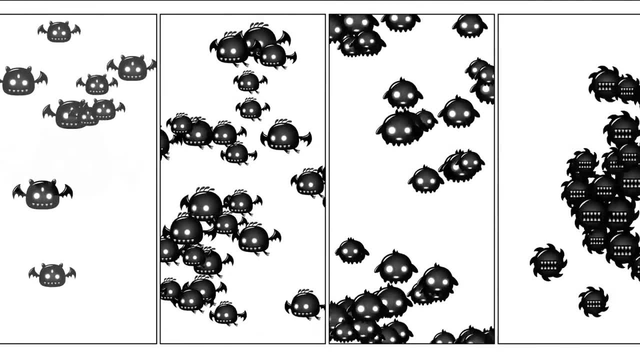 or you can take this code and slot it into your personal games. it will be compatible with my previous games if you follow these tutorials. let's start with a very simple one. the first project will have bots flying in random jumpy patterns- perfect for halloween game or even a website, for example. 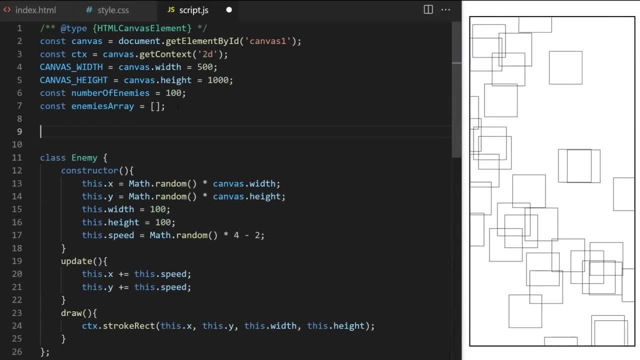 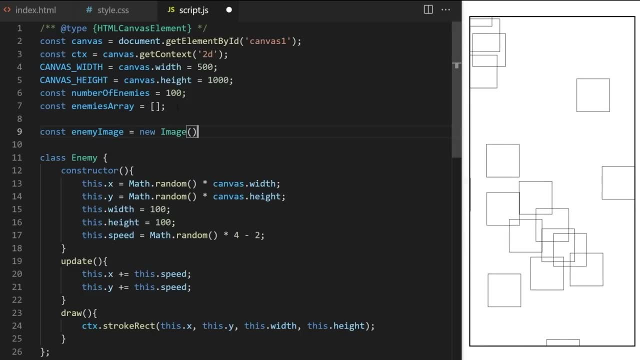 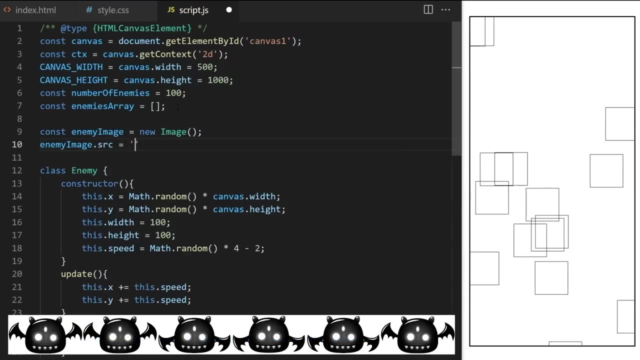 i'll leave the creative applications of this on you. first i need to bring new image into my javascript project. to do it, i create a custom variable called enemy image and i set it equal to new image. enemy image dot src is equal to enemy one dot png if you are using the same. 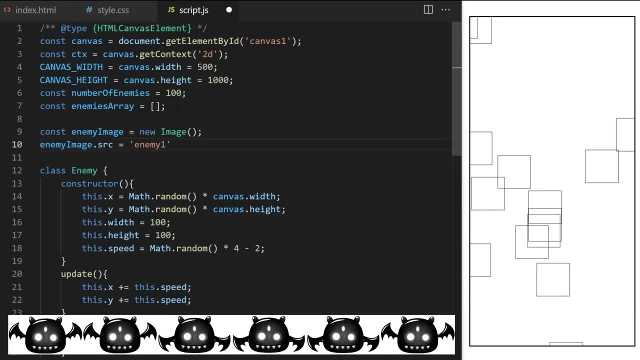 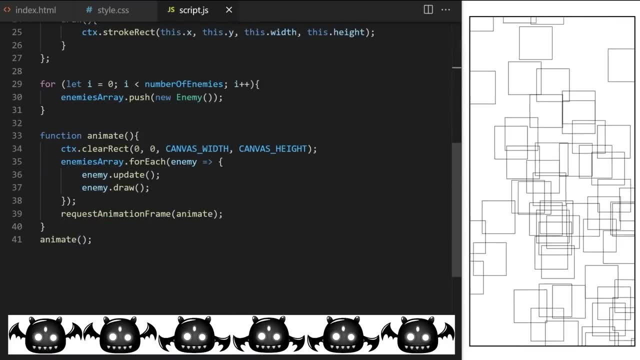 spreadsheet i'm using. it might be a good idea to use the same files at first and follow along and you understand the code. it's easy to adjust it and to use your own custom images online. 26 inside the draw method i call built-in draw image canvas method. we will use it to animate our bad sprite. 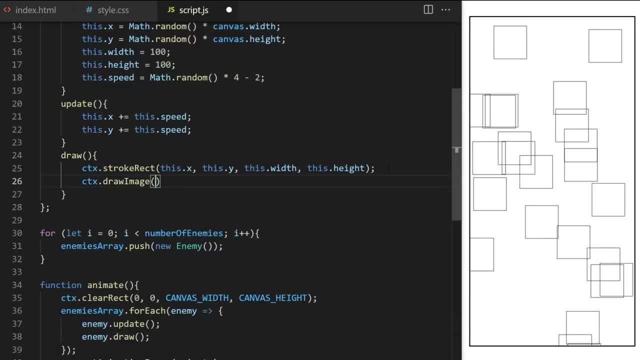 sheet. i will explain sprite animation quickly as i code. but if you need more detailed explanation, i made a special video where i focus on it in depth. i will link it in the video description. ctx, dot- draw image and i pass it. image i want to draw and i pass it. x and y coordinates. 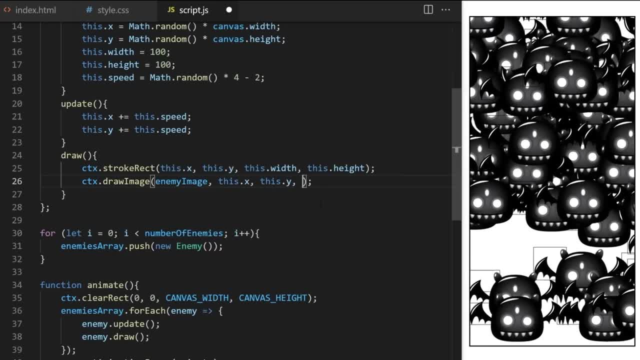 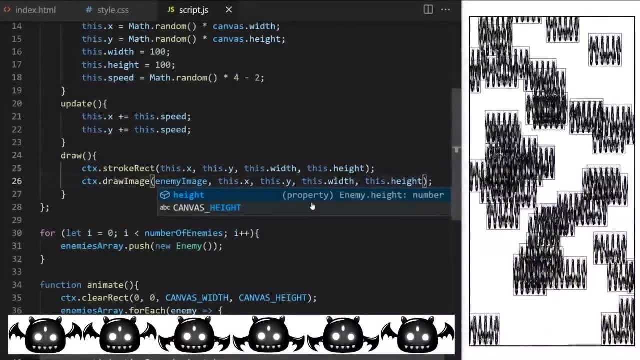 and this is what we get. we can also pass it optional width and height arguments, which will scale the entire image into that specified size. you can see it pushes the entire sprite sheet with all six frames inside the rectangle. we don't really want that. we only want to crop out one. 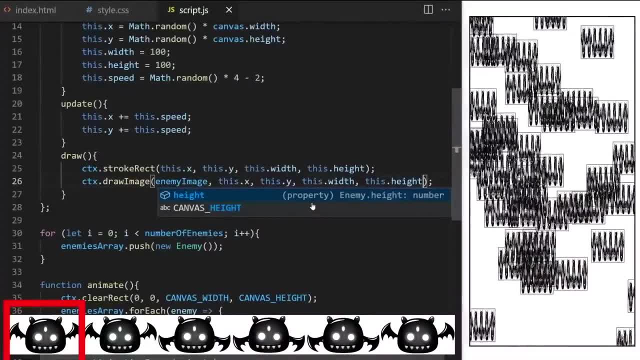 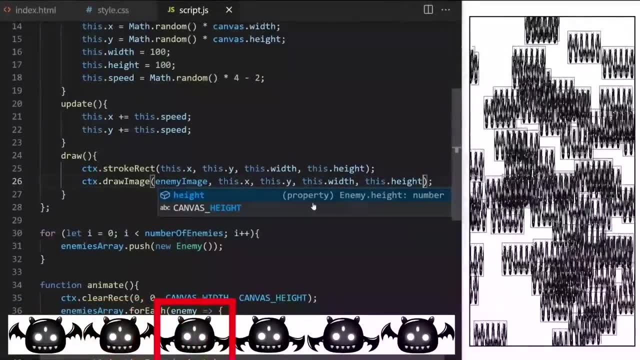 frame at a time and we want to be jumping by the amount of sprite width to the right to display the next sprite frame. we want to go frame by frame from left to right until we reach the last frame. we want to jump back to the first one and start again. we can do this with the draw image method. 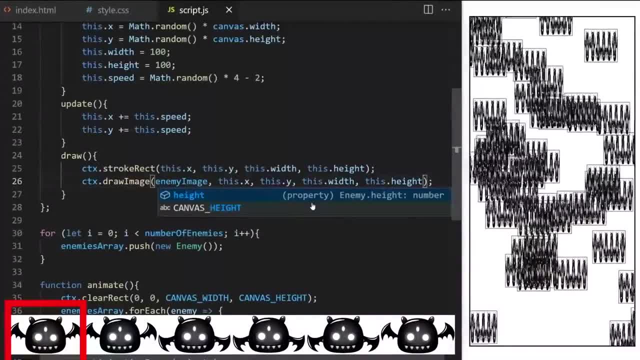 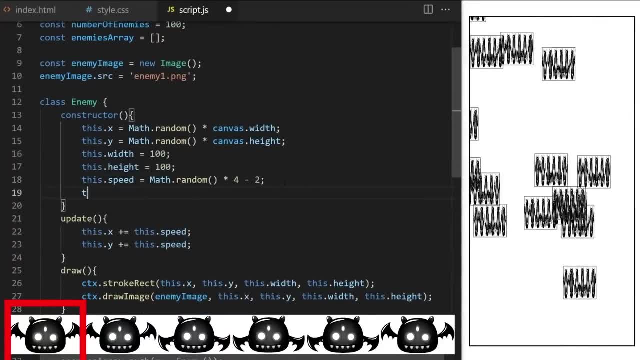 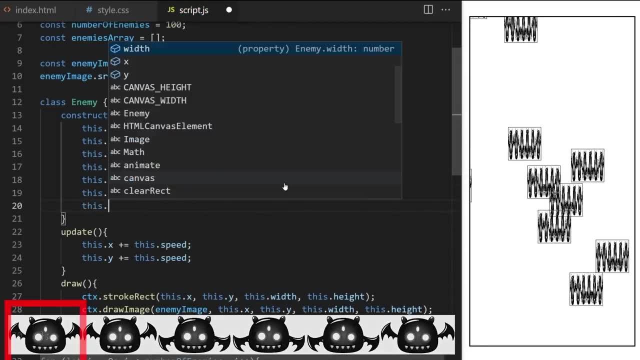 because it offers additional four optional arguments we can pass to it. let's go up inside animiconstructor to create property called sprite width. i check my sprite sheet, divide its width by the number of frames and i can see that width of a single frame is 293 pixels. sprite height of this. 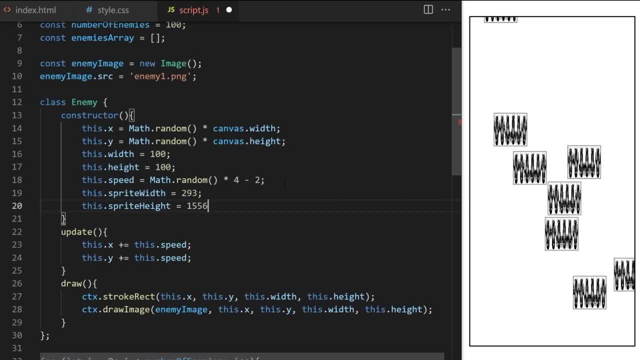 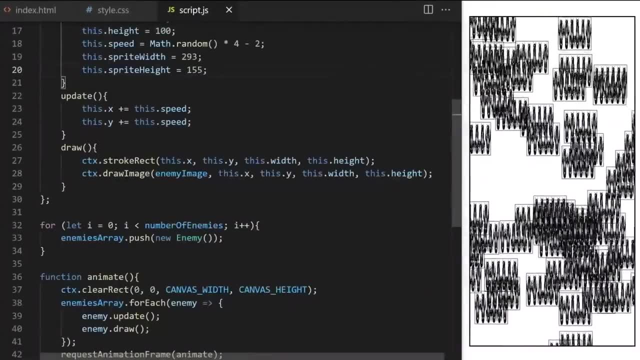 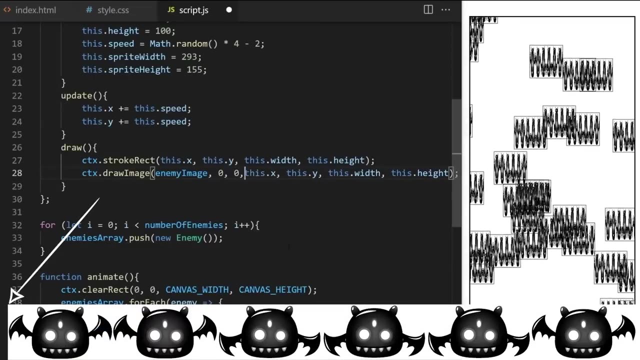 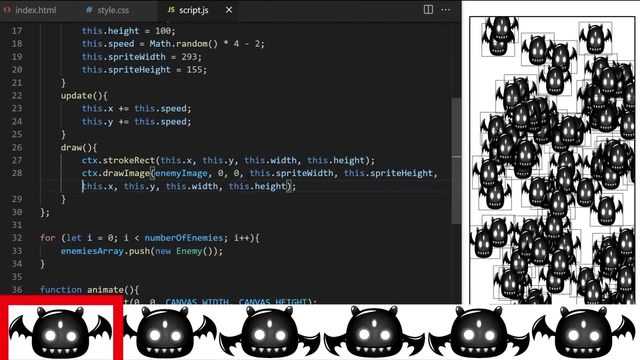 particular sprite sheet is 155 pixels. now let's add additional four arguments to draw image method. what area we want to crop out from this sprite sheet? to display only one frame, Let's start by displaying just frame 1.. So I want to crop out area from coordinates 0,0 to coordinates sprite width, sprite height. 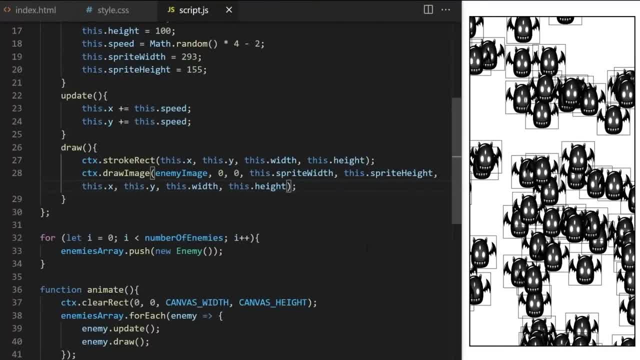 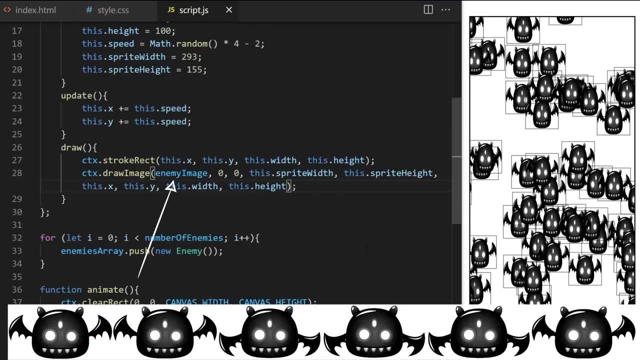 Now we are drawing just frame 1.. So in this version of drawImage method we are passing it 9 arguments in total. The first is the image we want to draw, The next 4 represent the area we want to crop out from the source sprite sheet, and these 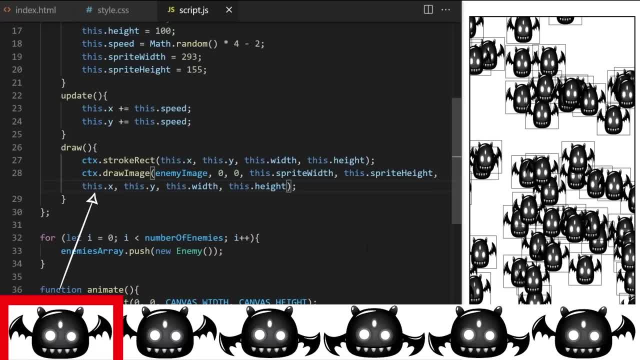 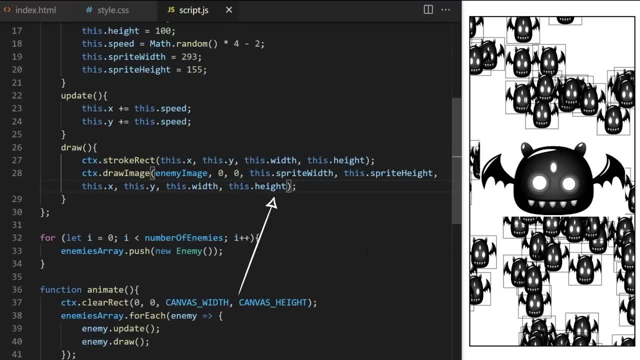 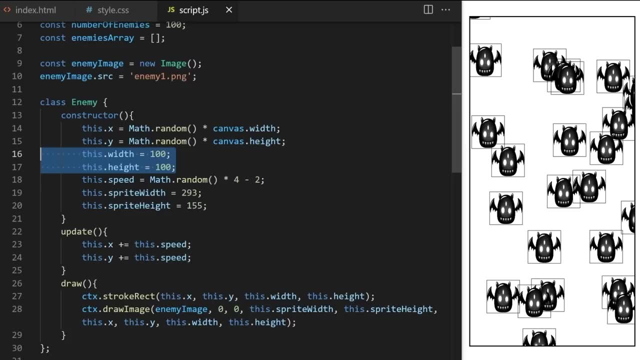 last 4 arguments determine where on canvas we want to place that cropped out frame onto. You can see my butts are slightly distorted because I am stretching them to fit this dot width and this dot height here, which are unrelated to the actual dimensions of my butt. 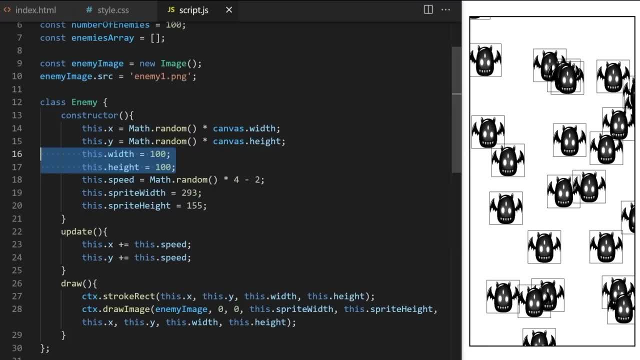 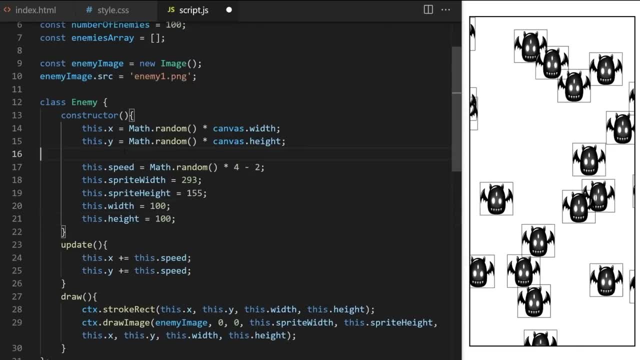 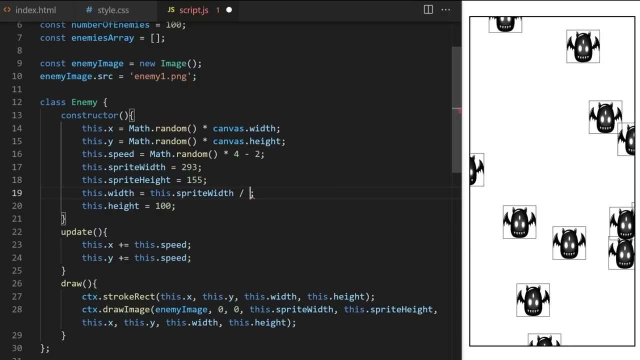 enemy character. Ideally I want to preserve the aspect ratio. so I make width and height relative to the sprite size. I take width and height and I move them to go after sprite width and sprite height so that they can see these values. Now I can make width 1 third of sprite width and height 1 third of sprite height. 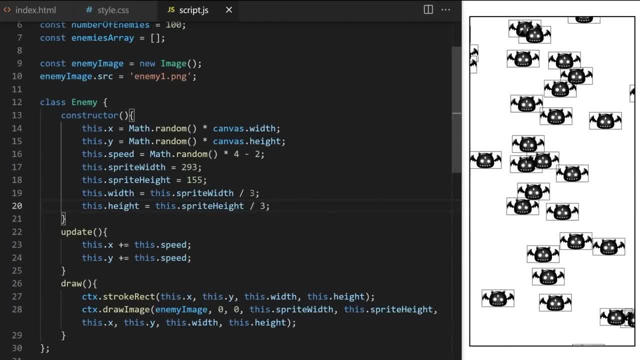 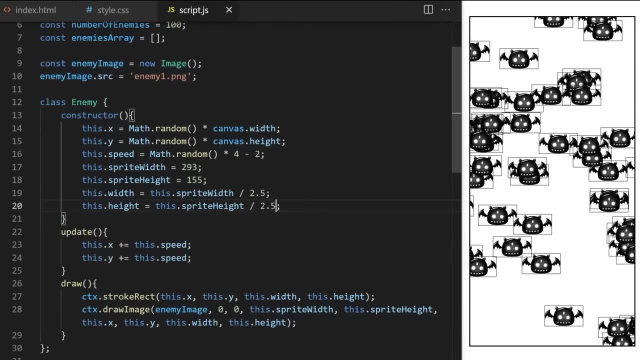 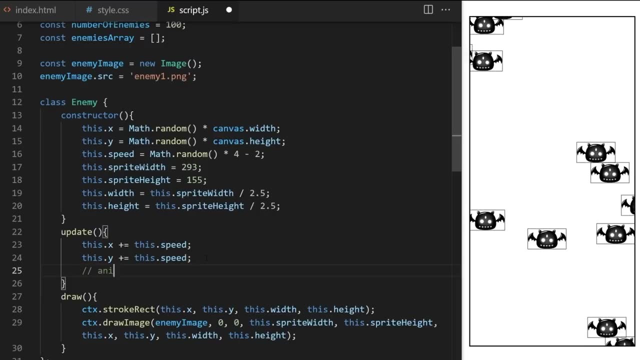 Now our butts are the correct ratio. maybe I want to make them a bit larger. Let's try 2.5.. That's better. Right now we are displaying only frame 1 because of these hardcoded 0,0 coordinates. Let's cycle through all frames and animate our characters. 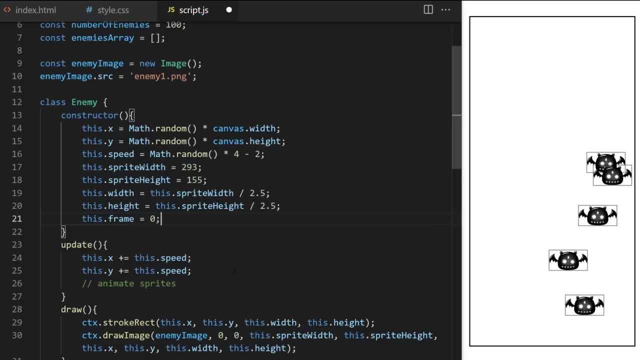 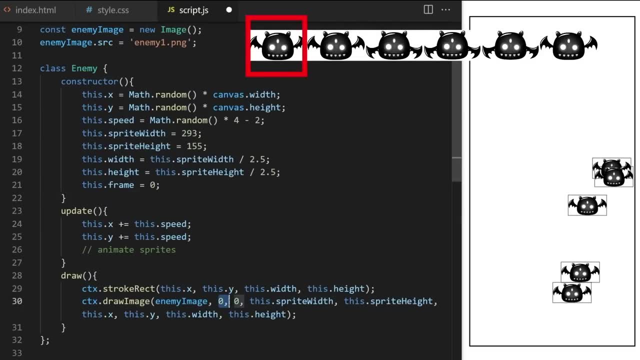 On enemy class. I need a new property called thisframe and I set it to 0.. On line 30, instead of hardcoding horizontal coordinate 0, which will give us this frame, I will take thisframe variable and I multiply it. times thisspriteWidth. 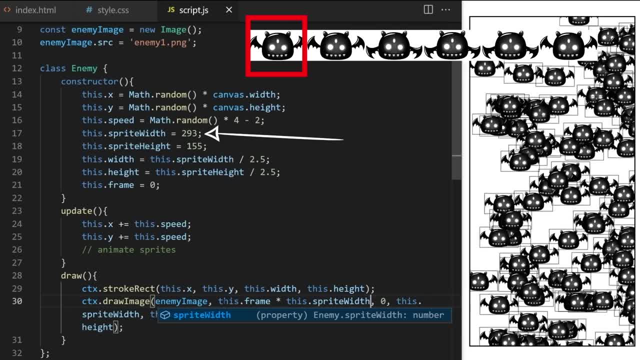 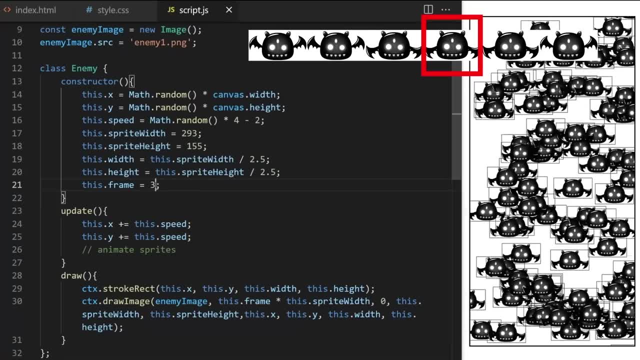 That way, when frame is 0, we display this frame. when it's 1, we display this frame. 2,, 3 and so on. So now all I have to do is that frame cycles between this and this frame, between 0 and. 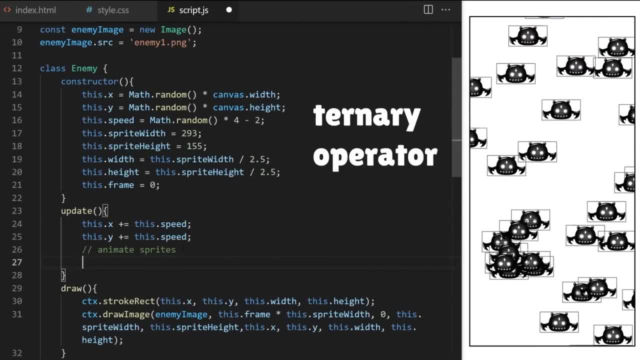 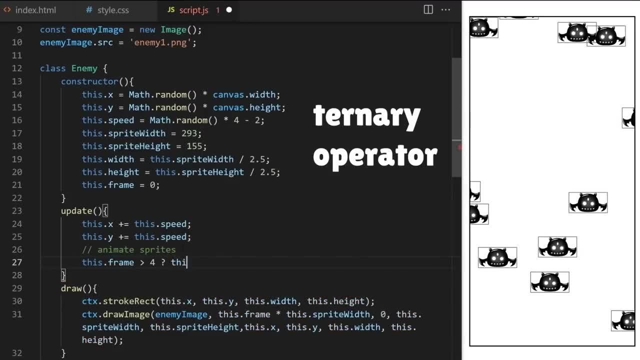 5.. I will use ES6 ternary operator, which is a simple one line if-else statement. basically, I say, if thisframe is more than 4, question mark, set thisframe back to 0.. Else colon: Increase frame by 1.. 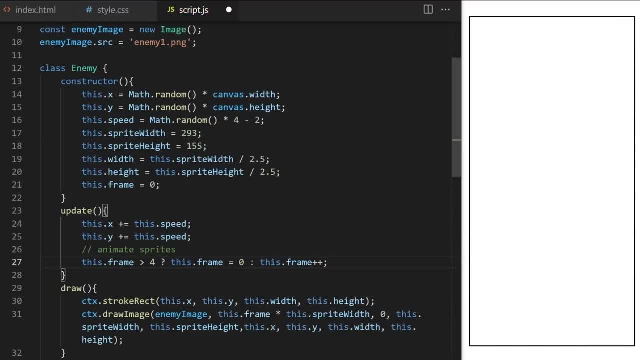 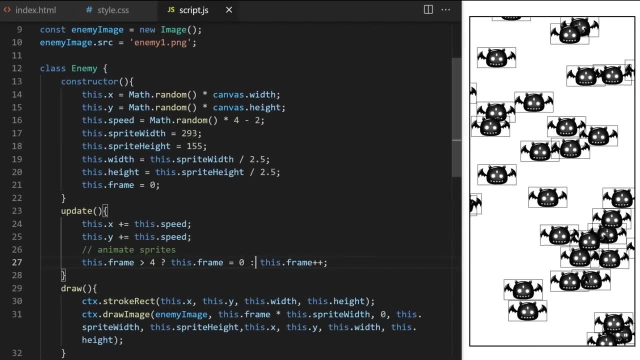 Thisframe plus plus. This should be colon. Our bots are flapping their wings and animating, but they flap very fast and all of them flap at the same time. Let's fix that There is a proper way to time animation frames using request animation frame and delta time. 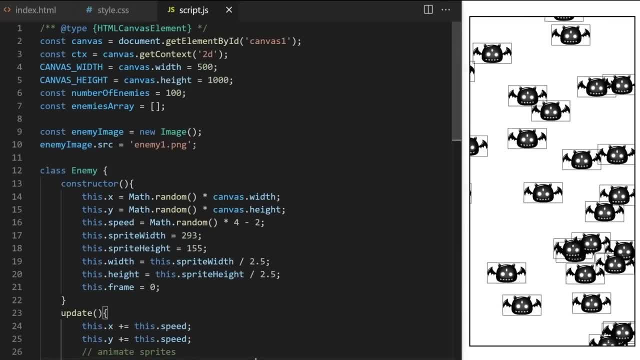 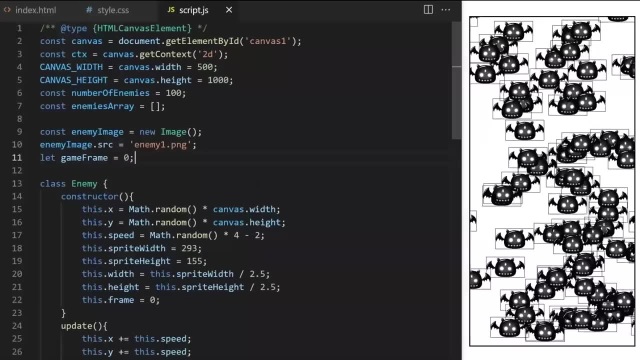 and I will show you how to do that in some other video Today. let's slow down our animation the simplest way possible. On line 11, I create a variable called gameFrame and I set it equal to 0.. Inside animation loop: on line 46, I increase gameFrame by 1 for every loop. 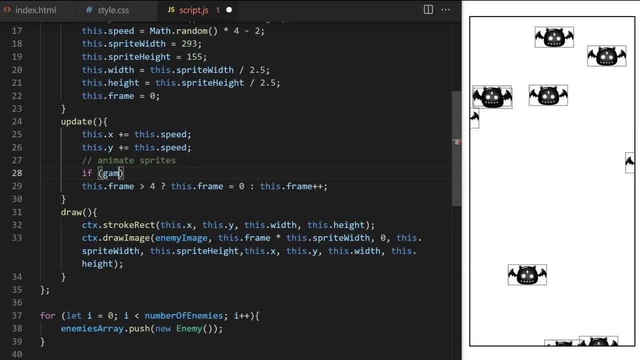 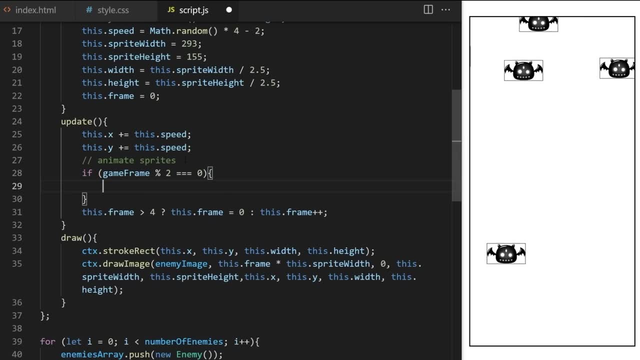 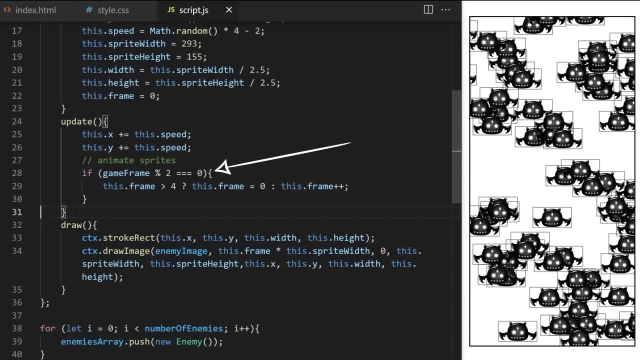 And up on line 28 inside update method, I say: if this ever increasing gameFrame variable is divisible by, let's say, 2, with a remainder of 0, only then serve new animation frame. This line simply means run this code only every 2 loops of main animation loop. 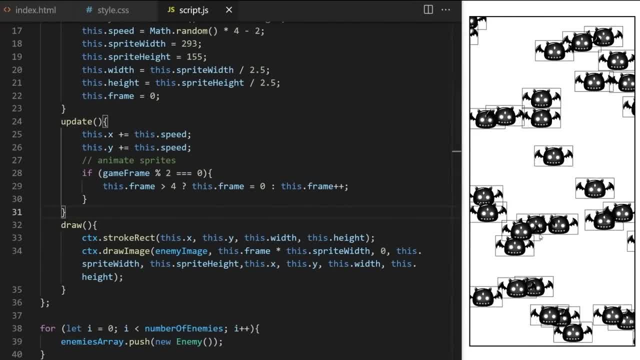 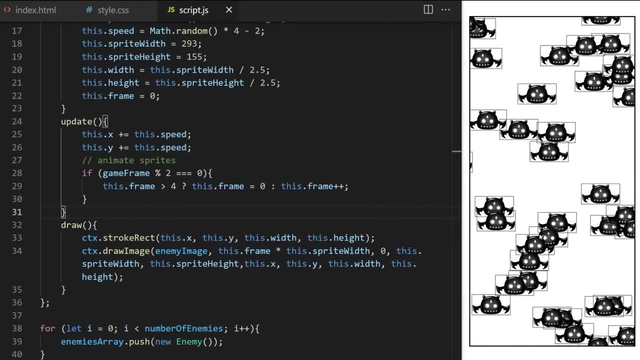 If you are getting a little unsure, I made a special sprite animation video where I go in depth and slowly over all of this. For now let's just move on and focus on movement patterns. Now bots animate slower, but they all still move their wings at the same time in the 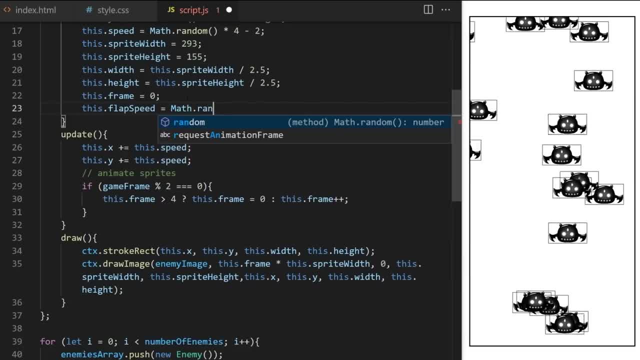 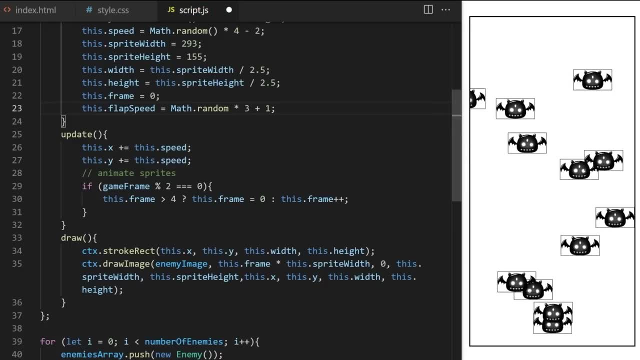 same rhythm. I want to randomize their animation frequency. I create a custom property called, for example, flapSpeed, and I set it equal to a random number between 1 and 4.. I replace hardcoded 2 on line 29 with this randomize flapSpeed value. 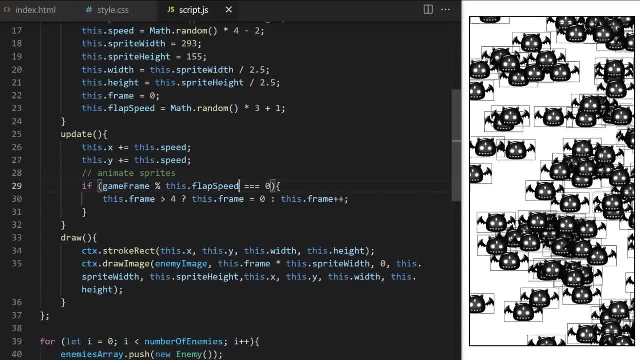 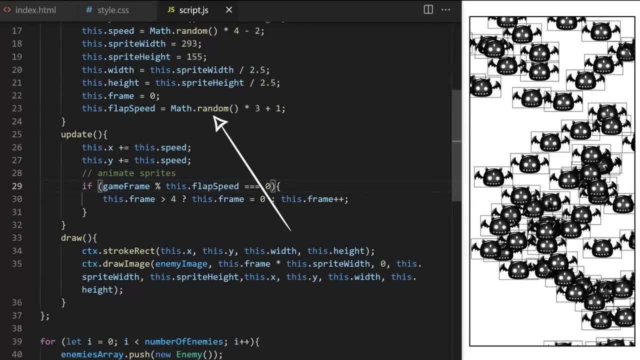 This will make some of them animate very quickly, Some of them slower. Some will animate every 1 or 2 or 3 or 4 frames. It will be randomized. The reason it doesn't work is because mathrandom returns numbers with decimal points, so gameFrame. 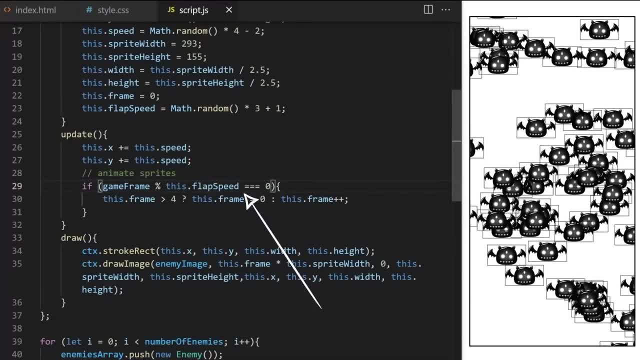 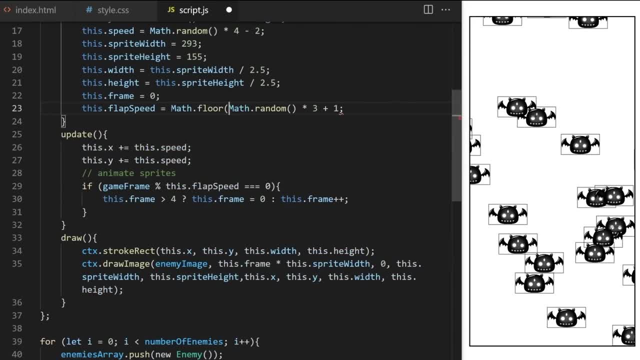 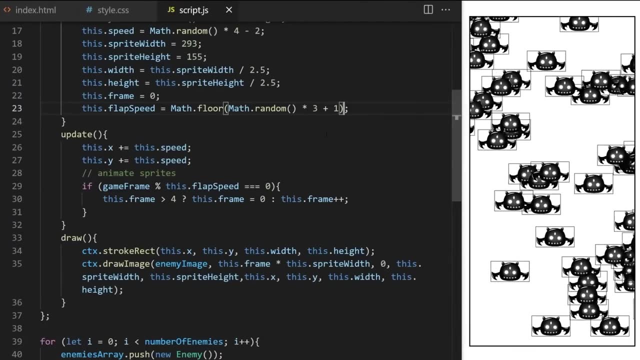 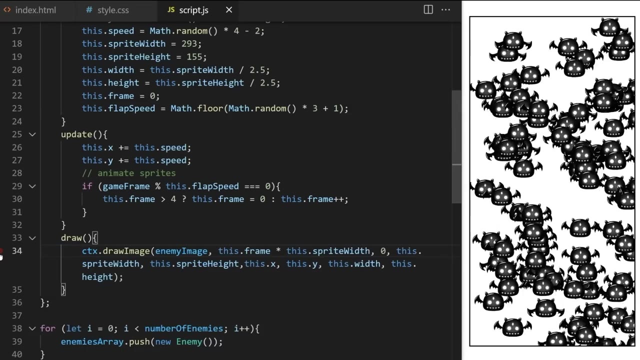 is never divisible by that very specific number, with a remainder of 0, and frames never increase. To fix that, I just need to wrap it in mathfloor. Now some bots flap their wings slower and some do it very fast. I will remove the stroke rectangle. 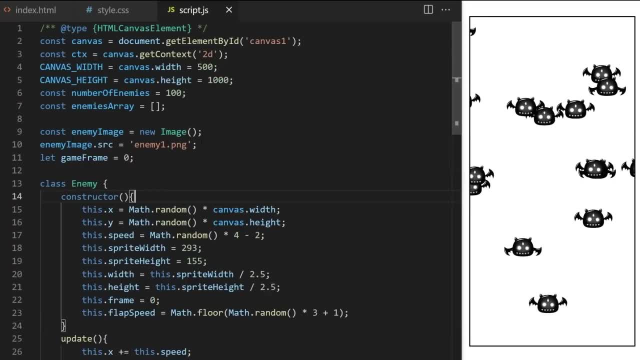 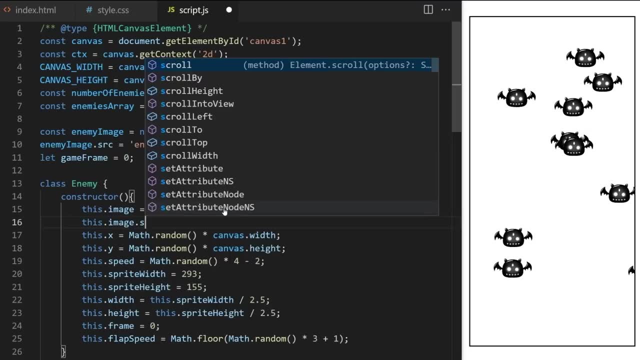 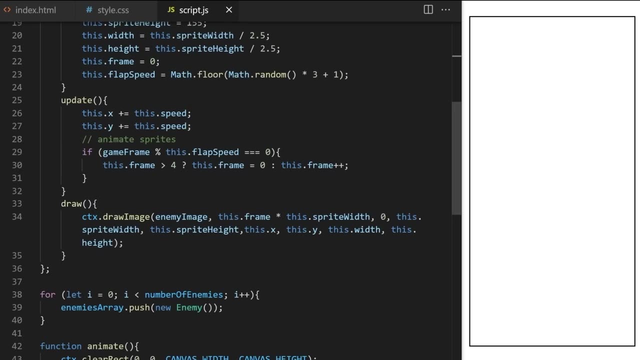 I can also take enemy image variable from line 9 and actually make it a property on javascript class like this: Thisimage equals new image. Thisimage src source is enemy1.png. I delete that And inside drawImage on line 34 I refer to thisimage instead. 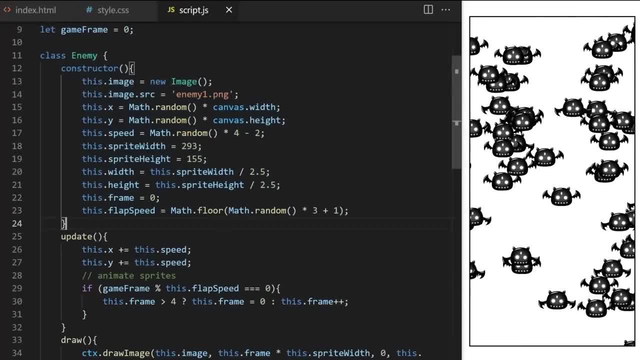 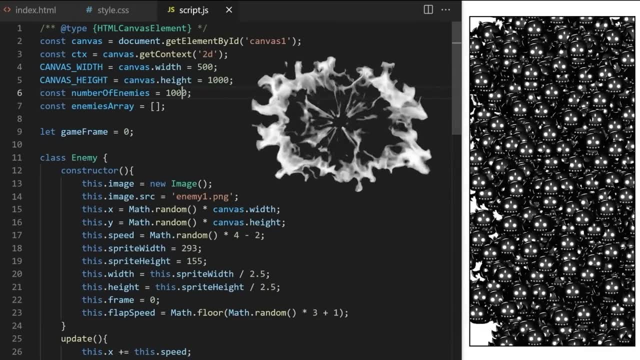 I delete that And inside drawImage on line 34. I refer to thisimage instead. By changing value of number of enemies on line 6, we get different number of bots in our project. By changing value of number of enemies on line 6, we get different number of bots in. 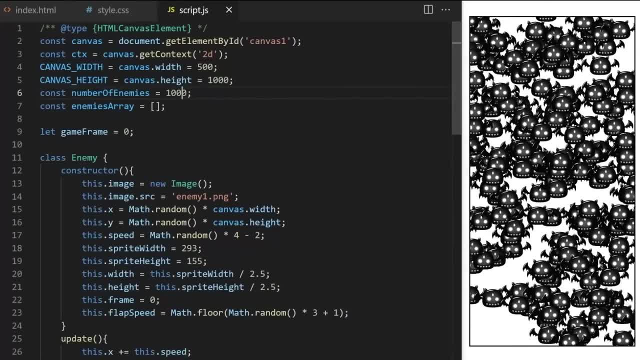 our project. By changing value of number of enemies on line 6, we get different number of bots in our project. Currently, our bots just fly away from canvas and never come back. We don't really want that. Let's create the first simplest movement pattern, which will simply be just randomized. 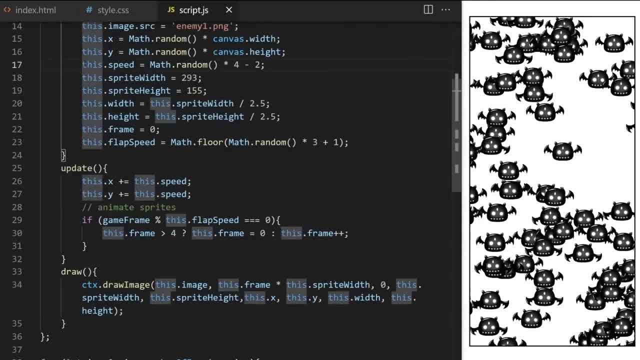 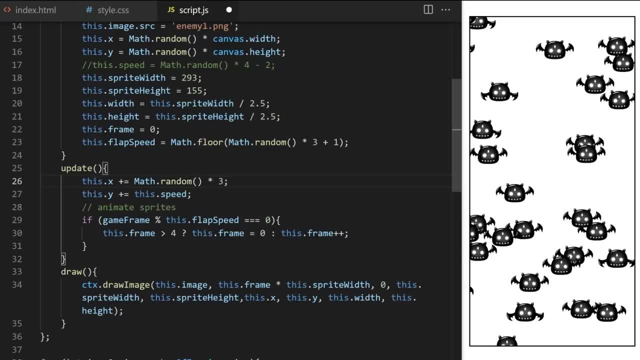 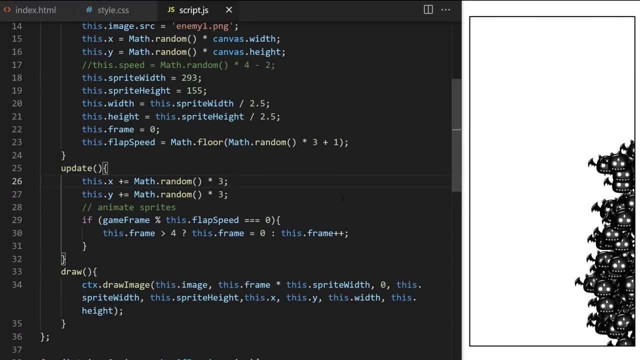 jumpy, chaotic movement. I comment out thisspeed on line 17 and on line 26 I replace it with mathrandom times 3.. I do the same with thisy on line 27.. Since we are adding positive numbers to x and y, all bots are going to leave canvas like. 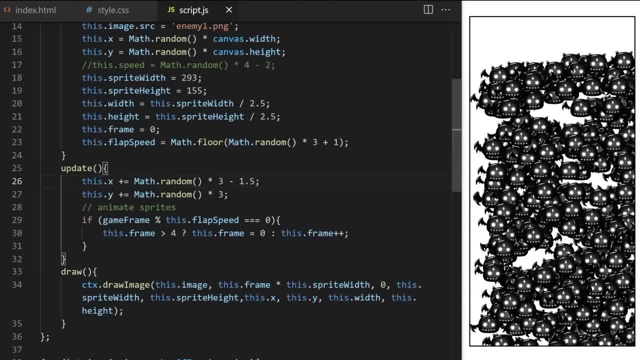 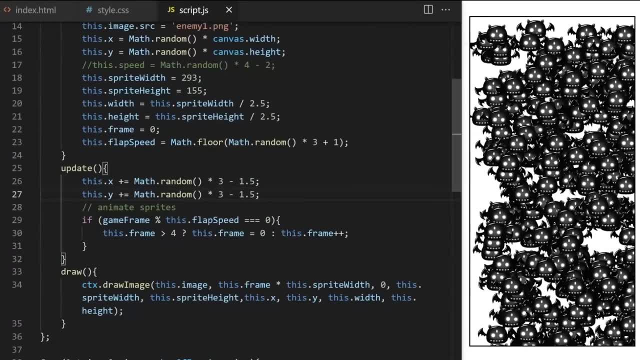 this: How about we tried a random number between minus 1.5 and plus 1.5.. Now they kinda stay in place and just wiggle around. We can increase their wiggle by giving this random number a larger range, for example. 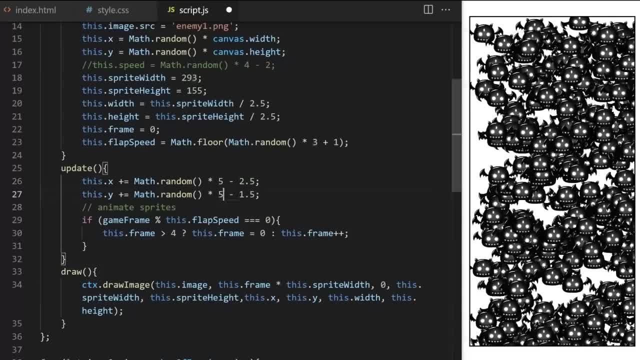 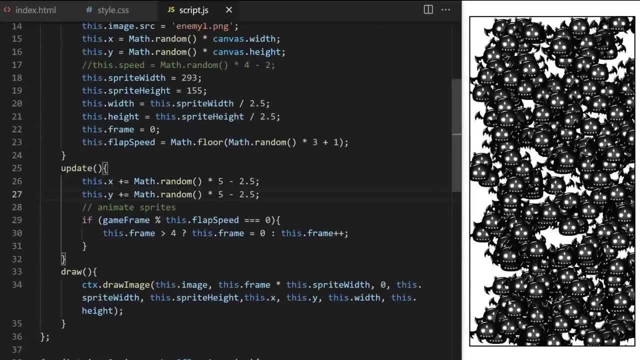 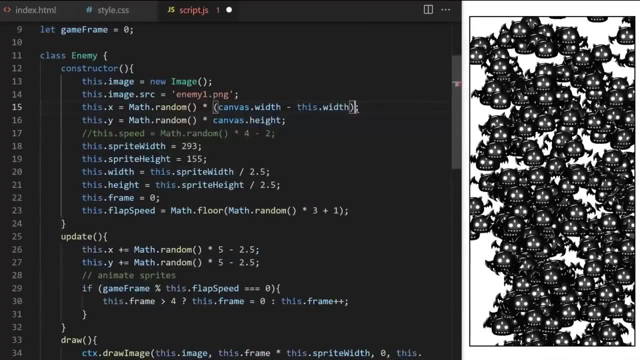 between plus 2.5 and minus 2.5.. I can see that my initial enemy x and y coordinates are not 100% within canvas. Let's adjust line 15 like this, And since I'm using this dot width here, I need to move it after this dot width has been. 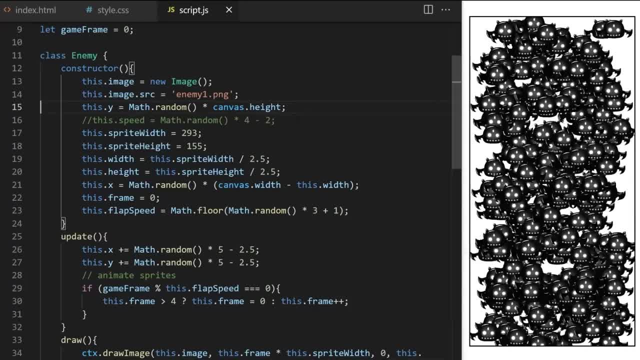 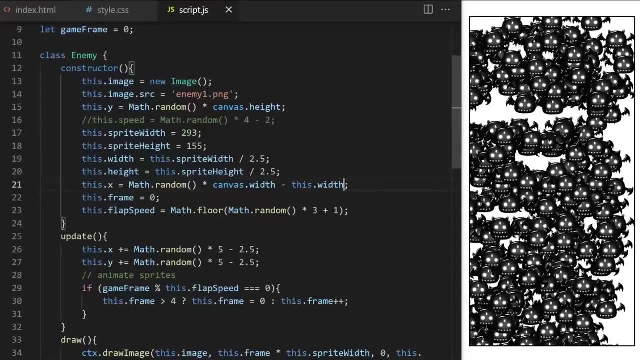 declared. Now, they initially spawn within canvas horizontally. These brackets are important. look what happens when I remove them. They just start from minus this dot width. They just start from minus this dot width, which is wrong. These brackets need to be here. 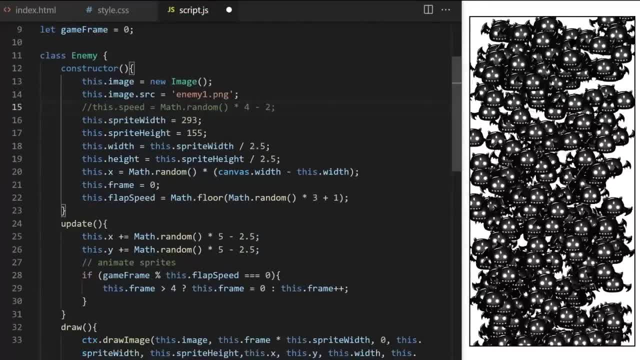 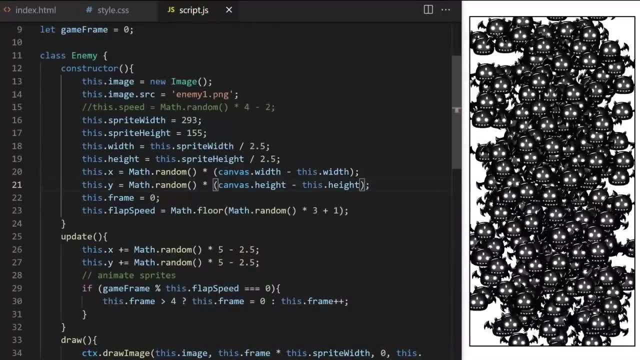 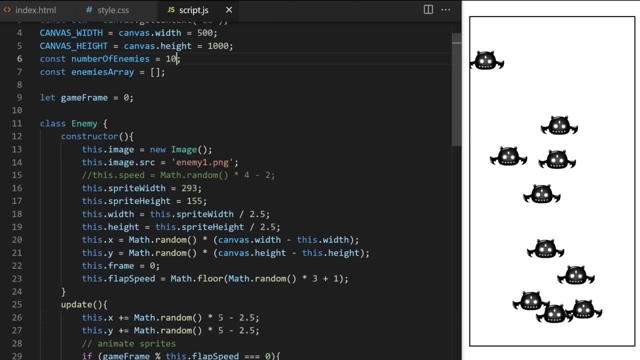 Let's do the same thing vertically. for this dot y, I reduce the number of enemies to 100.. Or 10. Let's make the range much larger on line 26.. Between minus 7.5 and plus 7.5.. 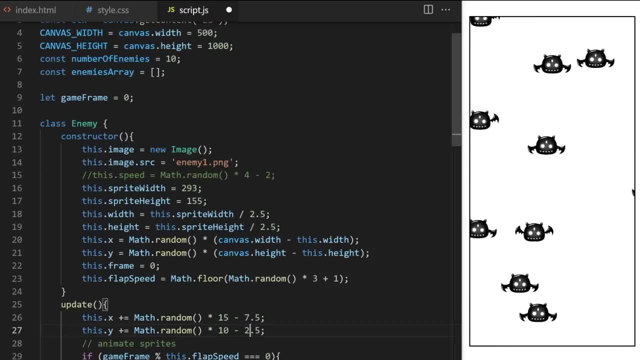 I can just play with these values And get the random sequence And get the random simple jumpy movement. This is the simplest way you can animate enemy characters or NPCs for your javascript games. We will do three more. add in little bit more complexity each time. 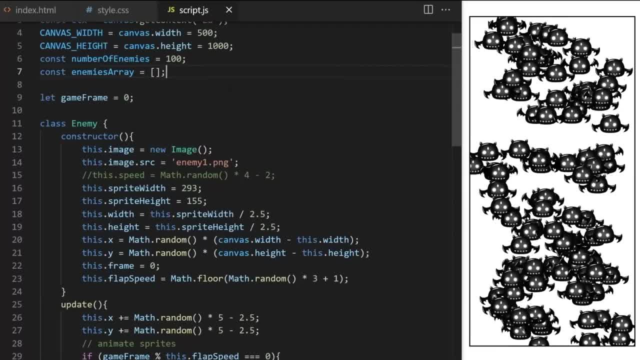 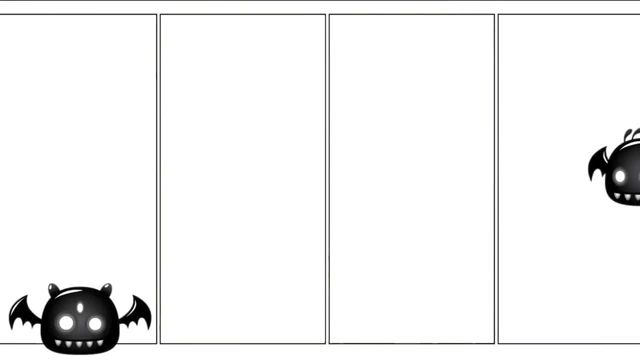 Let's see what comes out of that. I will be expanding, deleting and adjusting the same codebase. so, if you want, maybe it's a good idea to create a copy of this project at this stage so you have this movement pattern saved in case you want to use it for your games later. 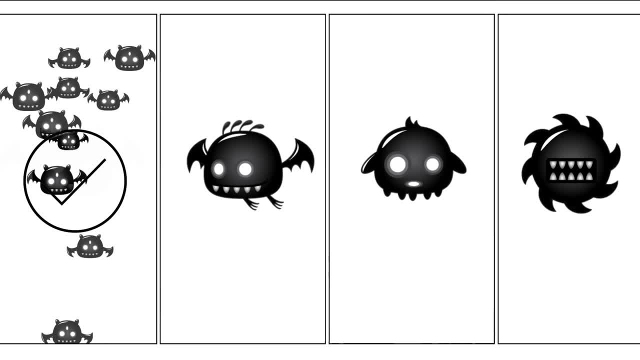 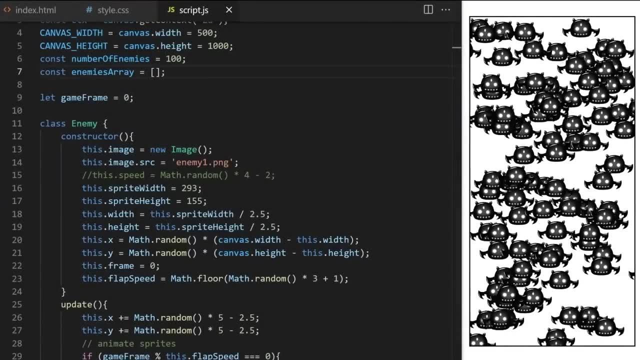 I will be using different enemy sprite sheet and different movement pattern for the next time. I hope you're having fun. For the second movement pattern, we will do something a bit different. First, let's switch to a different sprite sheet here on line 14.. 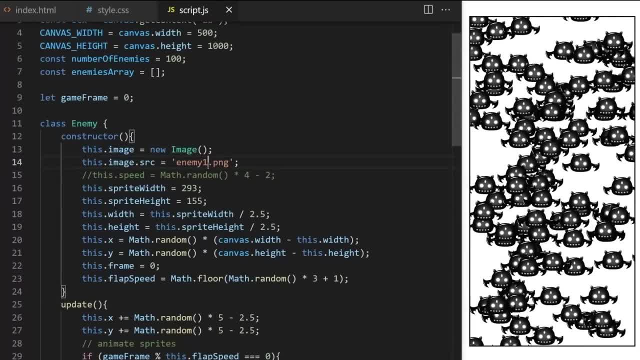 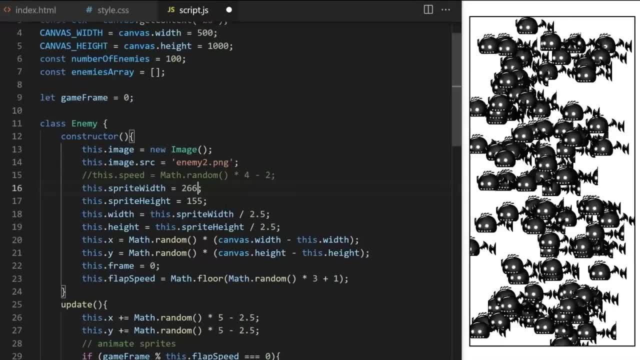 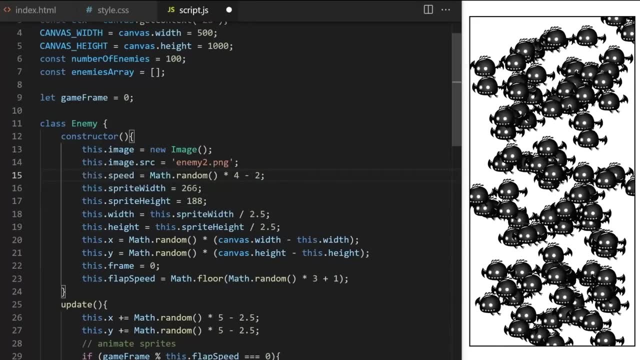 I will use image I called enemy2.png. It's different size so I have to change sprite width and sprite height. Sprite width is 266 pixels and sprite height is 188 pixels. I uncomment this dot speed on line 15 and I give each movement pattern a different size. 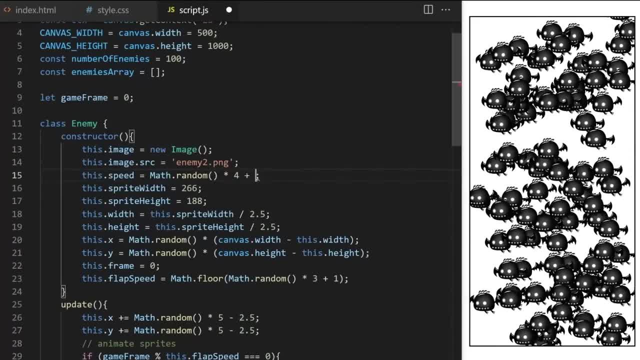 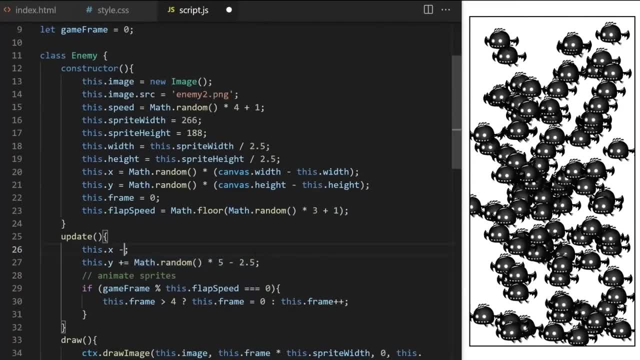 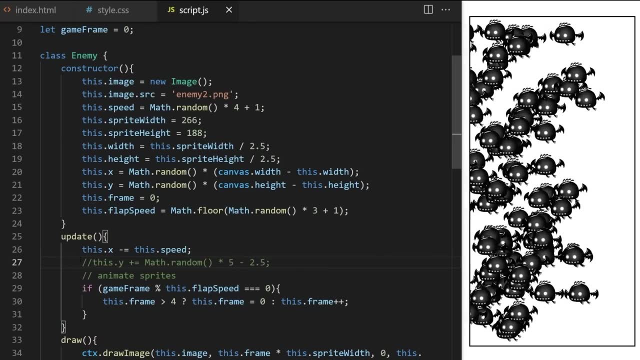 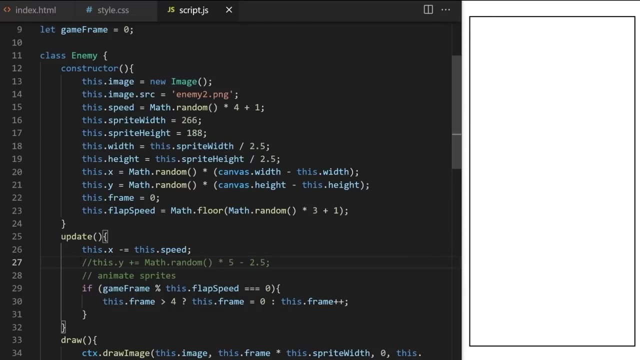 On line 16, I set this dot x to be equal to minus this dot speed. If I comment out y, we can see that bats just fly to the left in a straight horizontal line and they never come back. Let's first do a reset check. if this dot x from line 20 plus this dot width from line 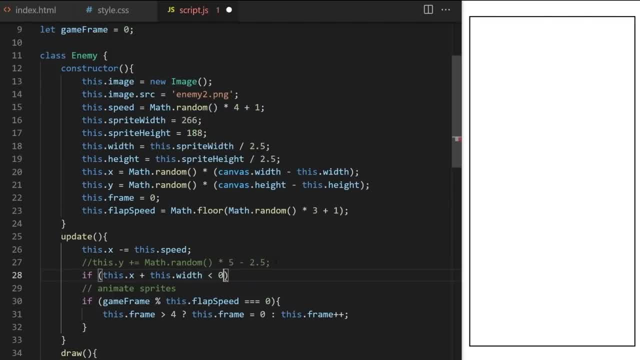 18 is less than zero, meaning when the character moved behind the left edge of canvas and is completely hidden. that's why I included this dot width here. When that happens, I want its horizontal x position to be reset back to canvas width. 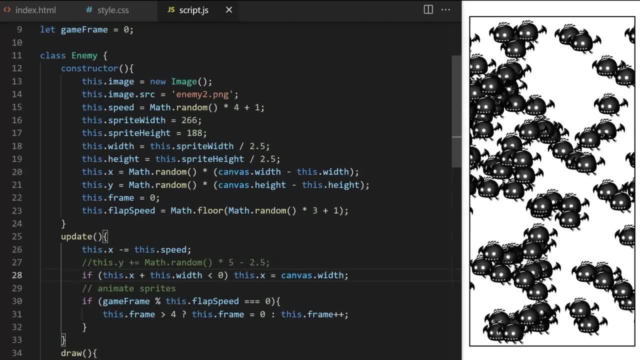 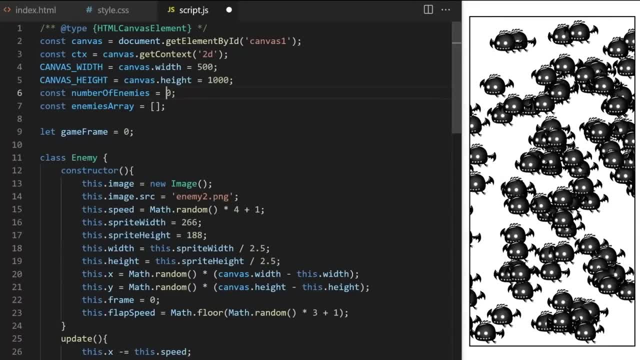 moving it behind the right edge of canvas so that it can do another flyover. Now we have endless right to left movement- Awesome. We already have something interesting here. but what if I want them to sway up and down as they flap their wings, making it a bit more dynamic? 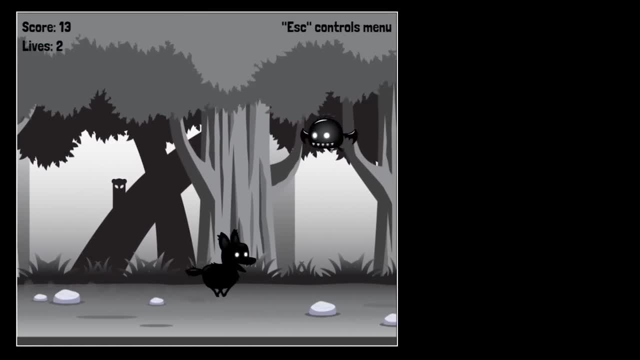 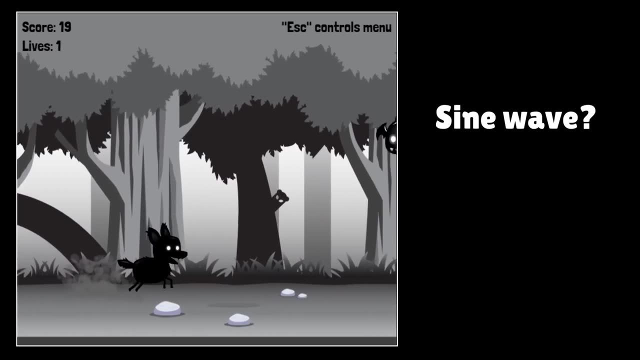 And if these were enemies in my JavaScript game, maybe it would make it a bit more difficult for a player to avoid them. How do I create wavy movement? Do you know what sine wave is? Let's do a little bit of very simple, beginner-friendly trigonometry. 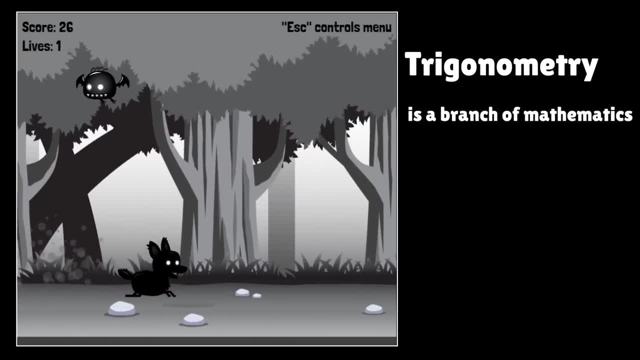 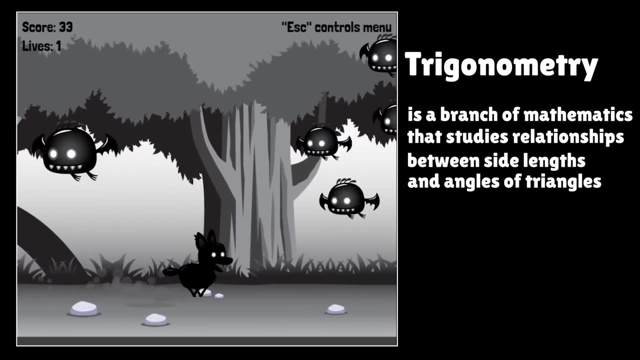 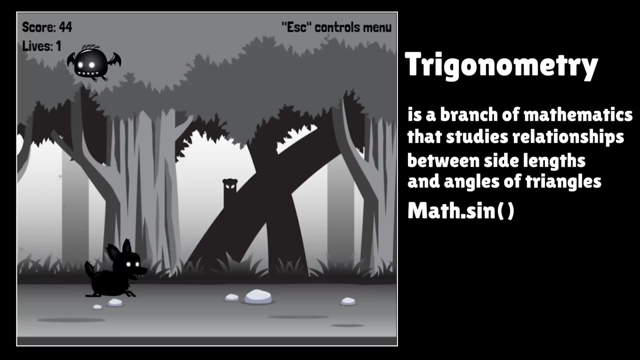 Trigonometry is a branch of mathematics that studies relationships between side lengths and angles of triangles. We use it to create wavy and circular movement in our JavaScript animations thanks to built-in JavaScript math methods. Today, we will have a look at mathsine and mathcosine built-in JavaScript methods. 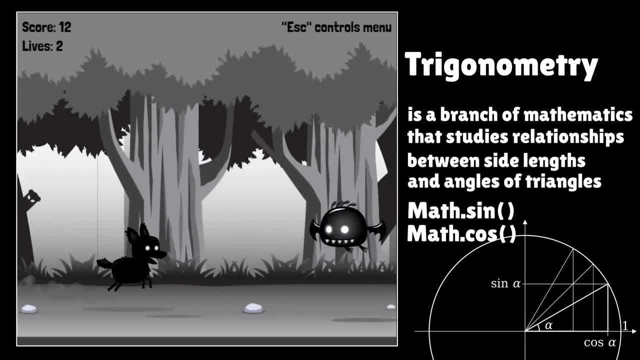 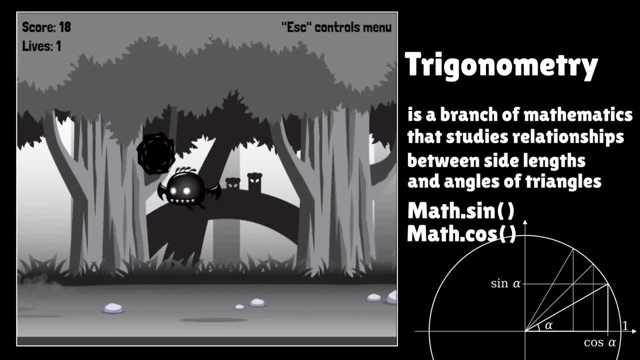 Sine is a trigonometric function of an angle defined in a context of a right triangle. All we need to know for now is that mathsine returns the sine of a number we pass to it. That number represents angle value in radians and it returns numeric value between minus. 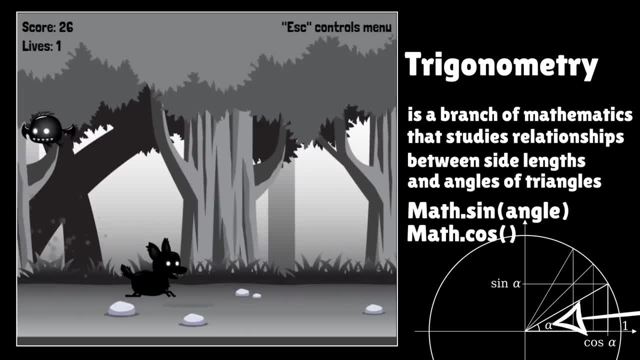 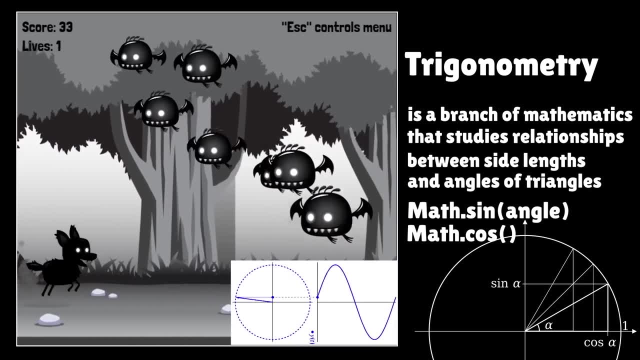 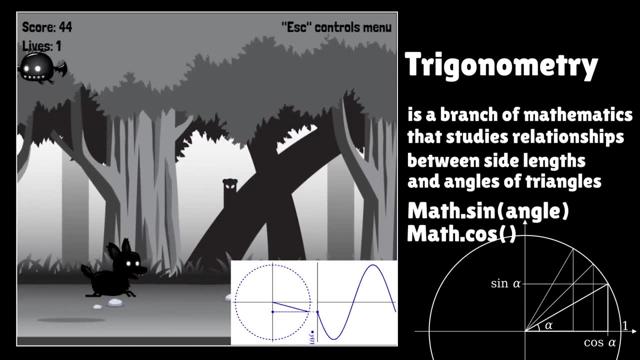 one and plus one. So this input angle value it takes if I put it inside animation loop and slowly move it by very small amounts. when I pass this angle value to mathsine, it will return a series of values that endlessly cycles between minus one and plus one, making it easy for us to. 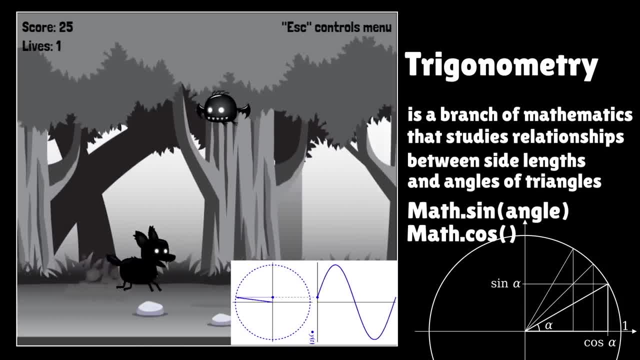 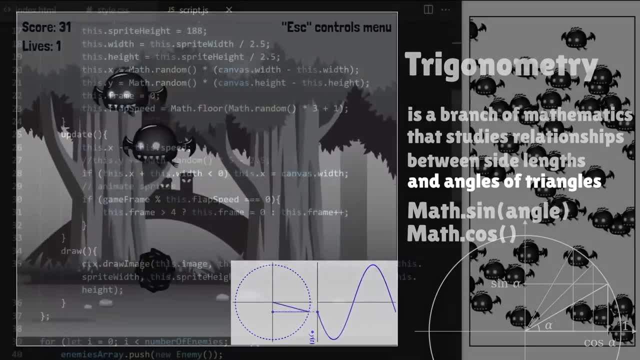 convert these values into wavy movement, so-called sine wave. What I just said might be a bit complicated for beginners and it might not make much sense. yet Let me show you. I will need thisangle property on my enemy class constructor and I initially set it to. 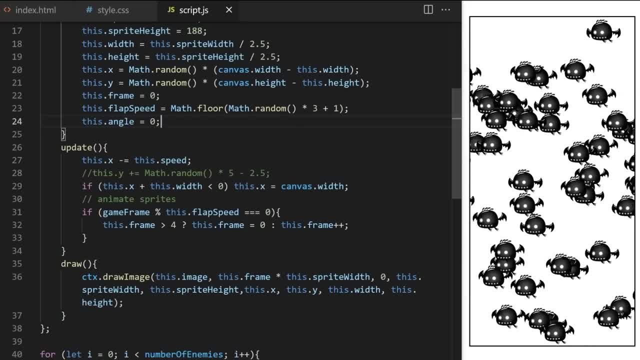 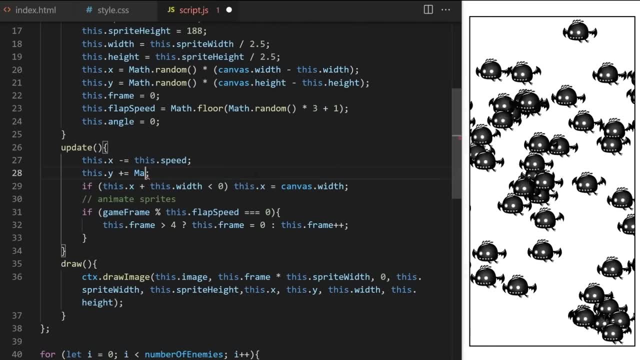 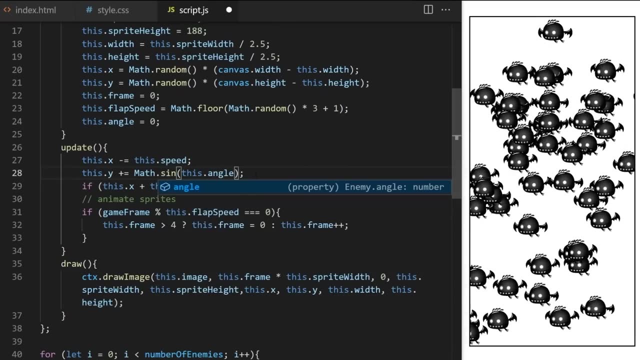 zero. This is the number that will be increasing and after being passed to mathsine it will give us that series of values between minus one and plus one, as I just mentioned. Let's do it so you can see. On line 28 I set position y plus equals mathsine and I pass it thisangle. 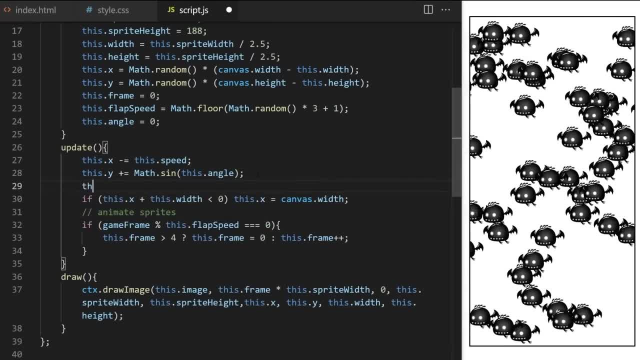 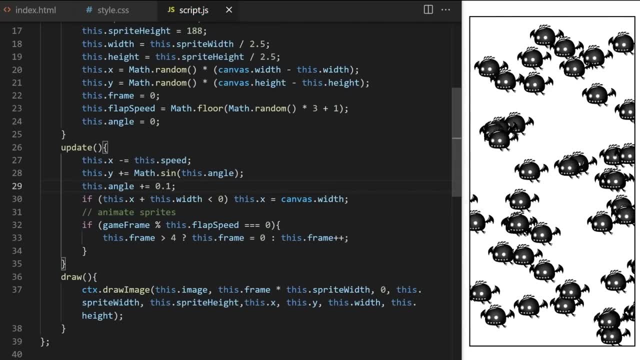 Then I increase thisangle by 0.1 for every animation frame As the angle slowly increases. do you see the waves? I can change the value here, on line 29, to change it to zero. I can change shape of my sine wave. 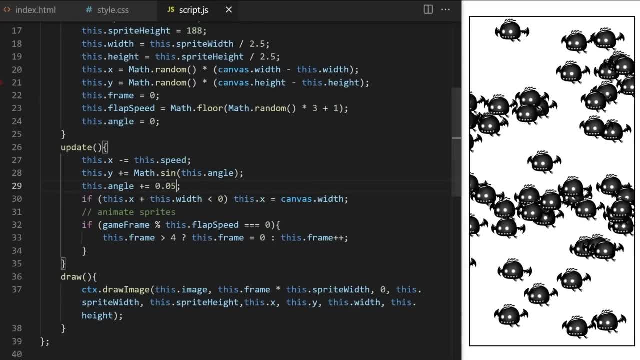 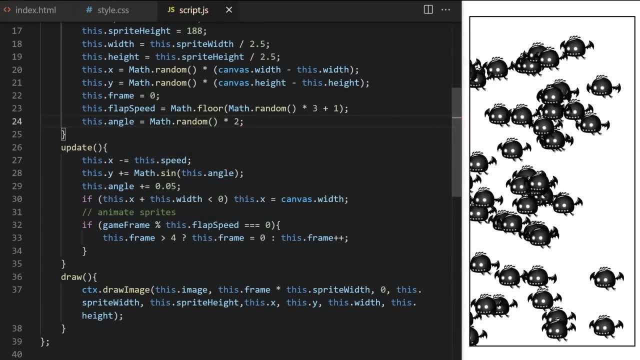 Angle doesn't have to start from zero. it can be a bit randomized. Let's try with mathrandom times 2. It will not be very visible. It will become clearer what it does a bit later. I will point it out. Quickly said, starting value of thisangle determines what position along the sine wave. 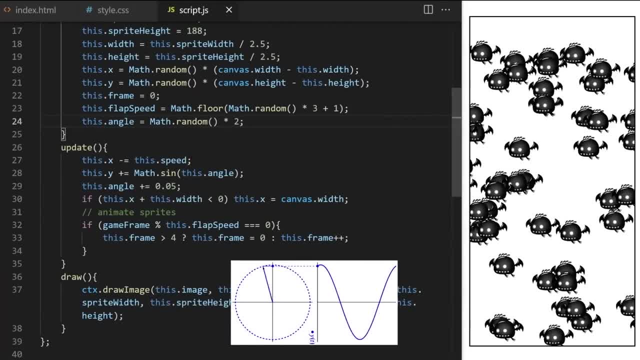 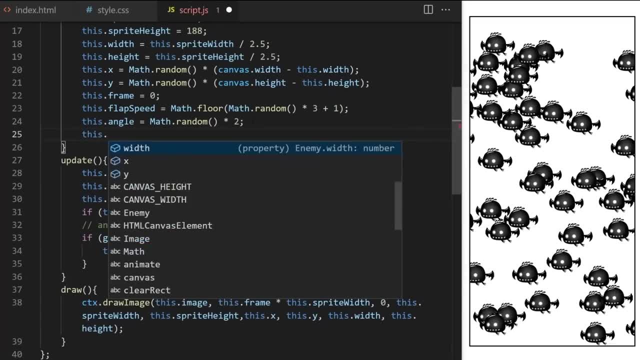 this particular character appears at first, before it starts moving. It's more obvious if we map movement to a circle, and we will do that in a minute. I can also randomize the speed at which angle value increases on line 30. I do that by creating a new property called, for example, angleSpeed. 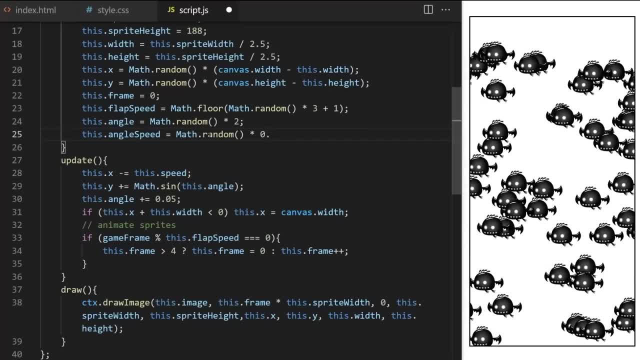 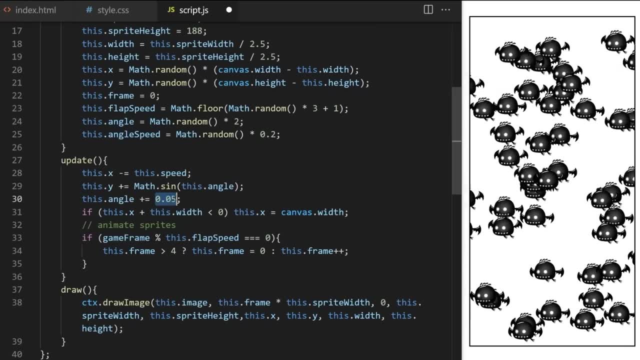 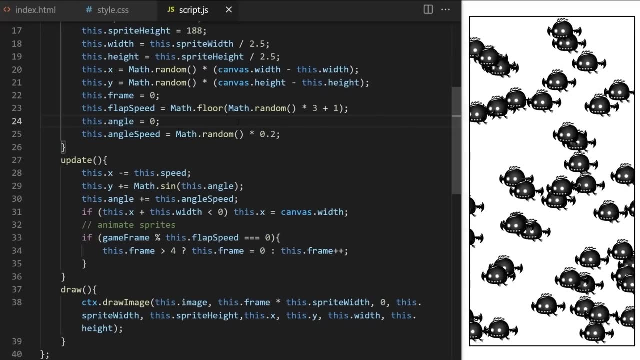 and I set it to a random number between 0 and 0.2.. Then I take this variable and I replace this hardcoded 0.05 with it. Now each enemy has its own angle value that is being increased by a slightly different amount for each frame. 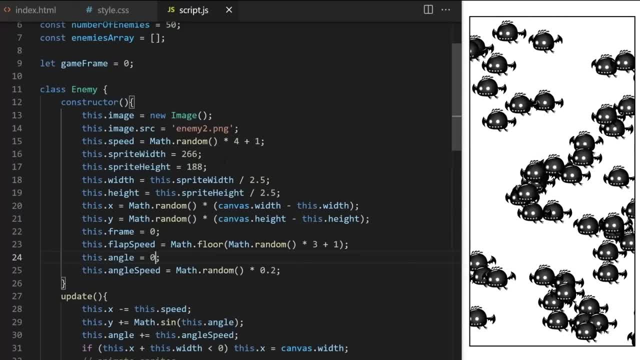 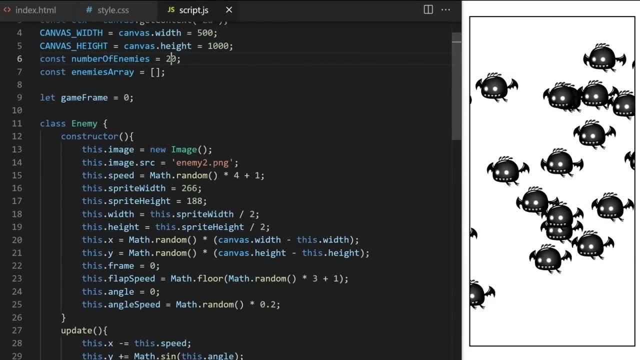 This will randomize the wave shape for each enemy. Let's set thisangle to 0 for now. I reduce the number of enemies on line 6.. As I said, mathsine returns values that cycle periodically between minus 1 and plus 1.. 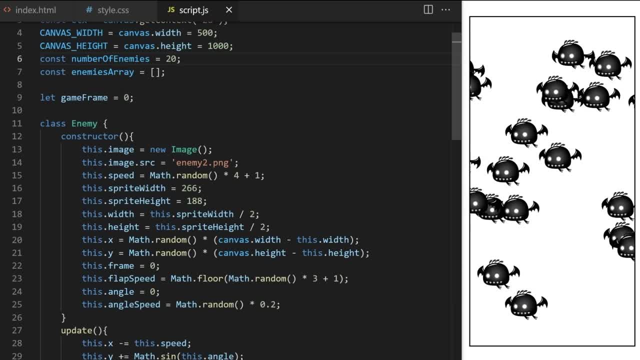 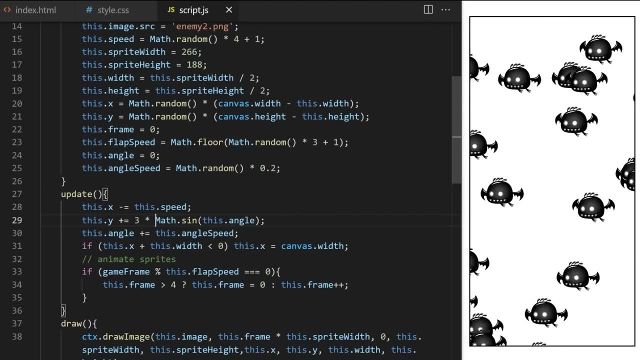 What if I want to make the curve more prominent? I can simply just multiply it times 3 here on line 29,. and now we are getting values that cycle between minus 3 and plus 3.. Do you see how the sine wave of enemy movement is more prominent? 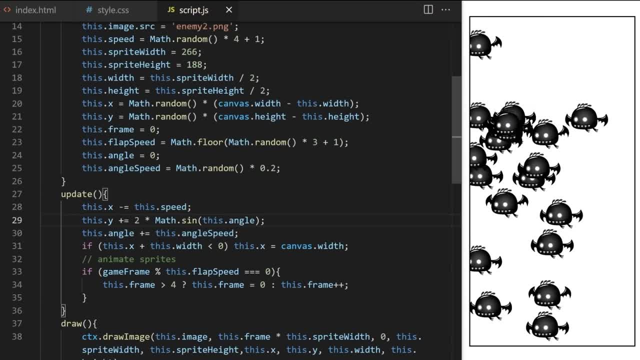 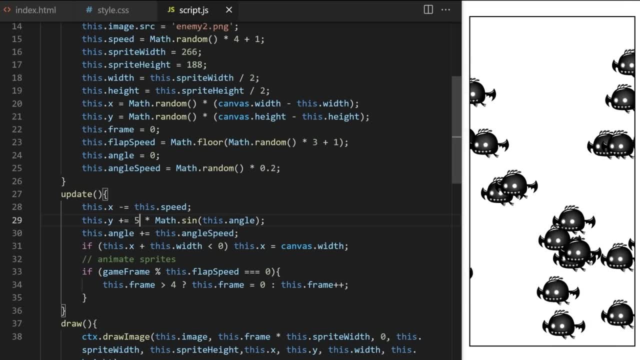 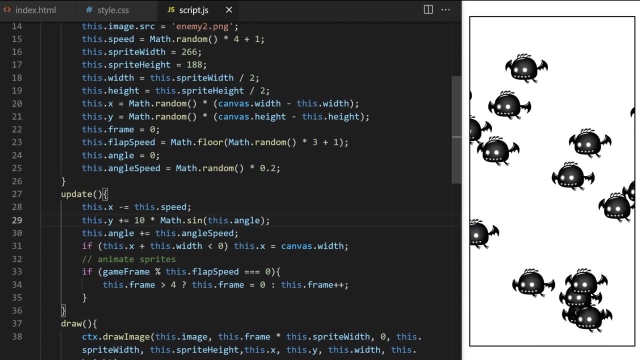 Look what happens when I put the different numbers here. I hope it's becoming more clear what I'm doing. If I put times 10, we get a very prominent curve. If these are enemies in your game, good luck to all players trying to avoid them. 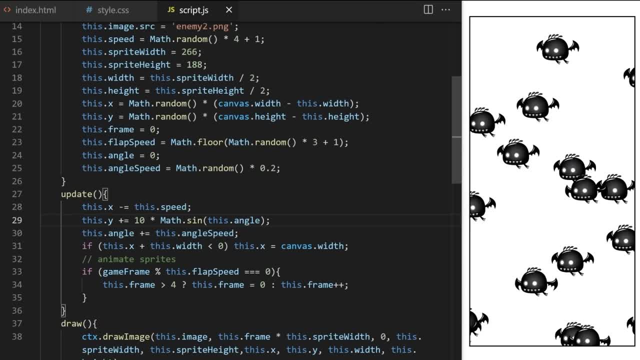 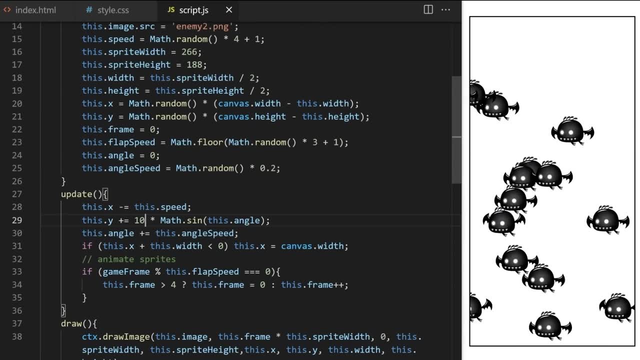 Especially for certain sprite sheets, this movement might be very suitable. Maybe you have some strange aliens in your space game and you want to move them in this weird wavy pattern. Instead of hardcoding number 10 here, I can again put this value in a variable that will be randomized for each enemy. 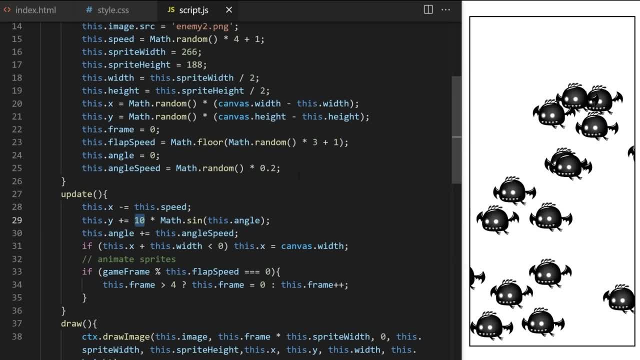 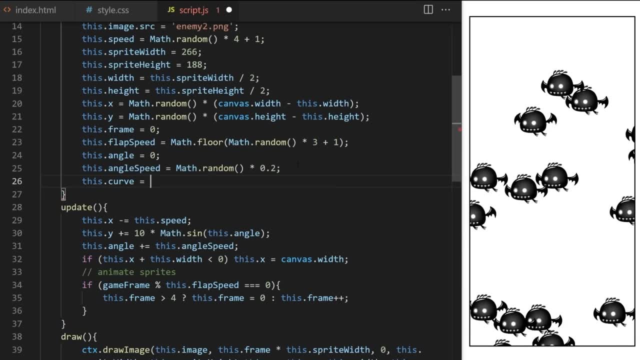 That way we get even more variation in movement between enemies. I will call it thiscurve, for example. Sorry about my variable names. Sometimes it's hard for me to come up with suitable names for all these custom properties. I hope it's becoming at least a little bit clearer what each of these properties does so far. 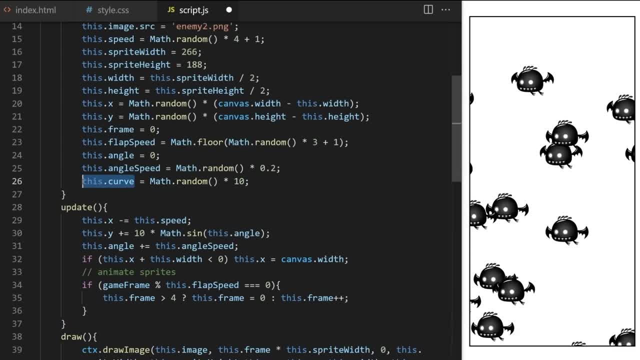 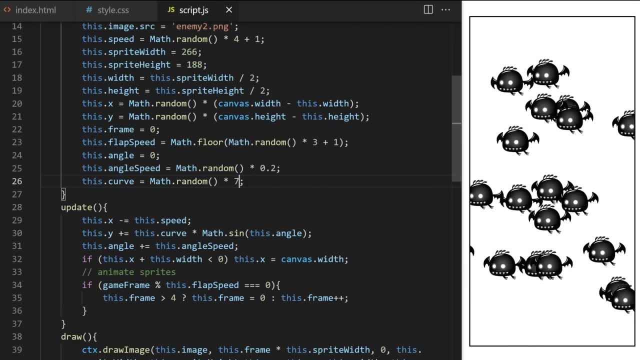 I want curve property to be a random number between 0 and 10. And I replace this hardcoded 10 with it Here on line 30.. Maybe 10 is too much. Let's do times 7 here on line 26.. 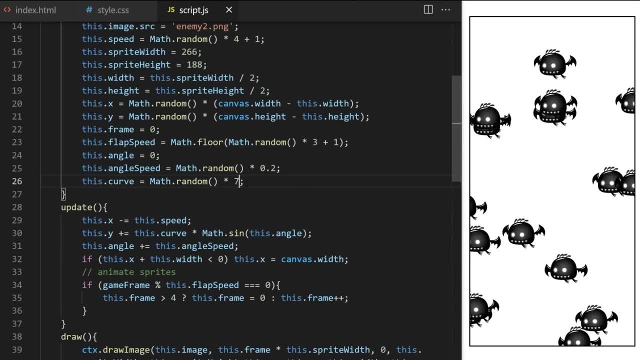 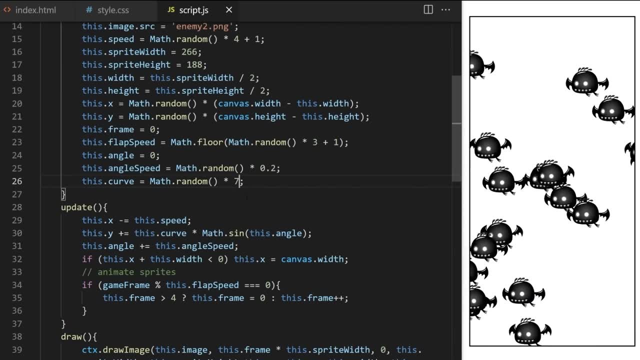 Do you see what we just did? Some of them move in very prominent waves. Some have barely any vertical movement. This would make our game more unpredictable. I can add as many enemies as I want. Let's put 200 here on line 6.. 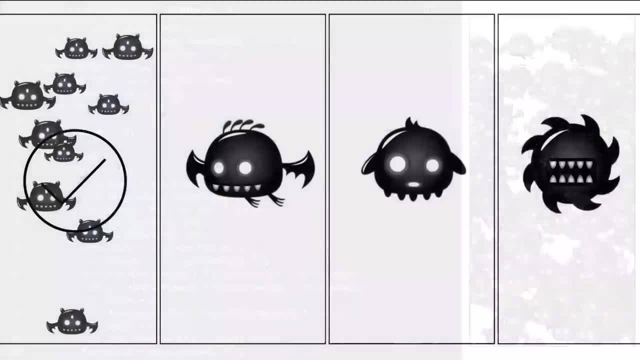 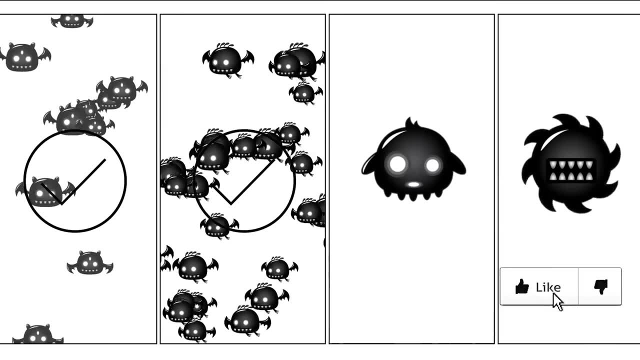 Haha, butt infestation. This will be a hard mode in my game. So we did endless horizontal movement with vertical sine wave element to it. What if we bring it a step further and also add some trigonometry for horizontal X coordinate? 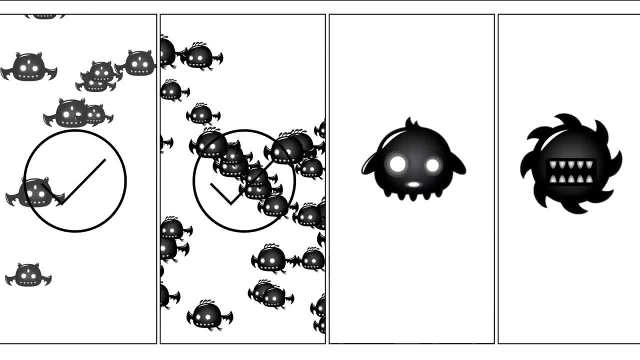 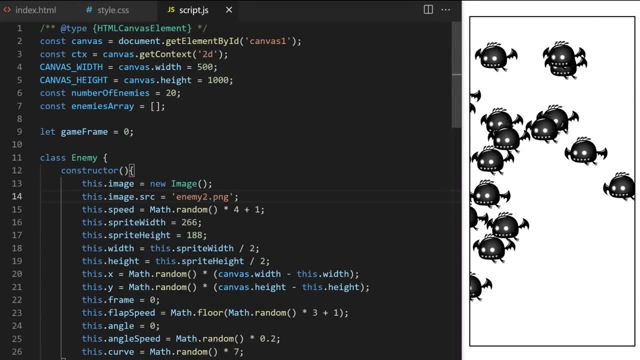 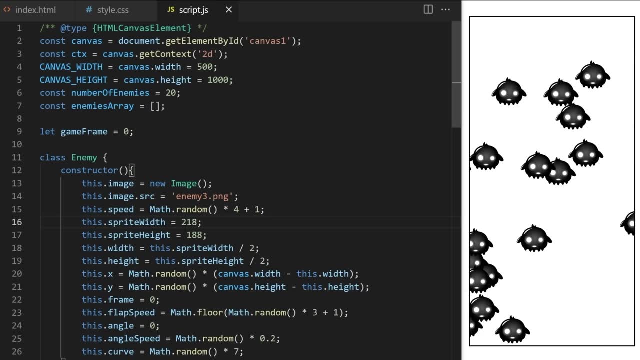 We can make the enemies move in all kinds of different shapes and patterns. that way, Let me show you. As usual, I will first swap to a different image. On line 14, I set image src to enemy3.png. I check my sprite sheet and I see that width of a single frame is 218 pixels and height is 177 pixels. 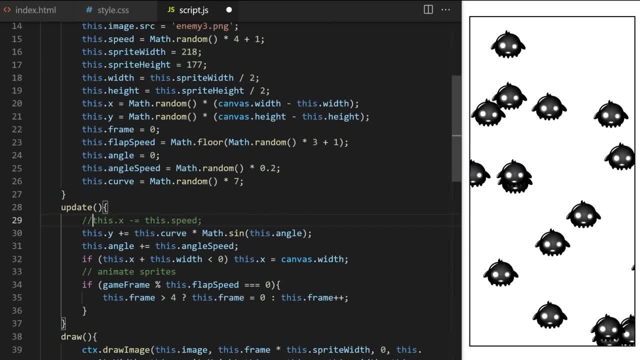 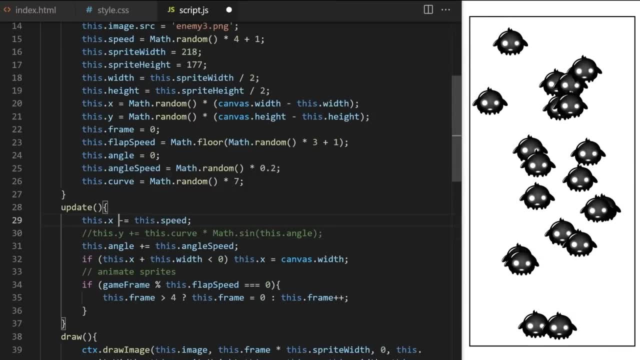 Let's comment out lines 29 and 30.. Which will stop our character from moving around. On line 29, I want horizontal movement to be cycling within a certain range. I call mathsign and I pass it thisangle from line 24.. 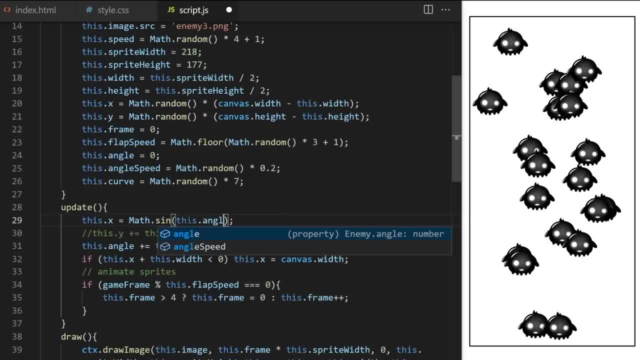 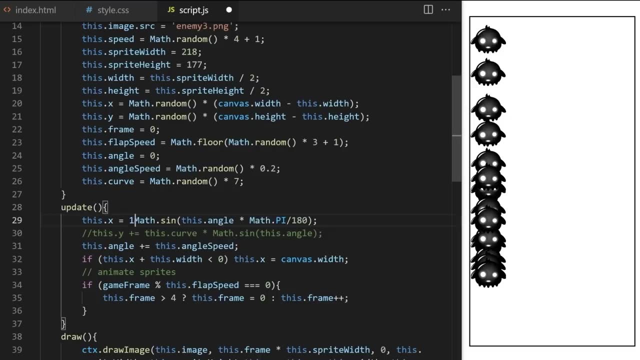 Thisangle value is increasing over and over on line 31, as update method is called from inside animation loop. I will also multiply it times mathpy divided by 180.. Let's just experiment here a bit. If I multiply this whole thing by 10, nothing happens. 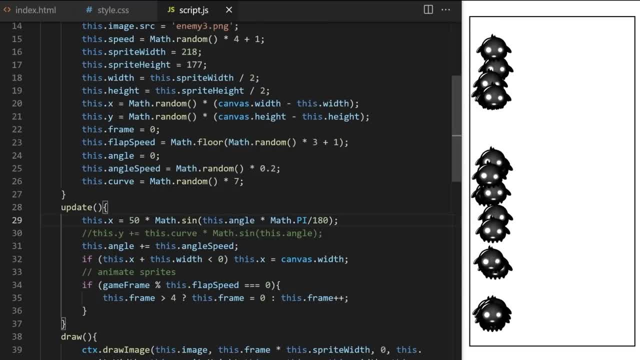 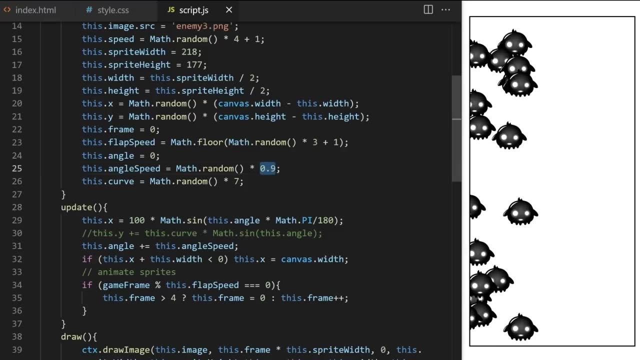 50? We see some movement. 100? Yes, they are moving. now This angle speed on line 25 affects how fast angle value on line 31 is increasing. If I set it to 0.9, they will move faster. 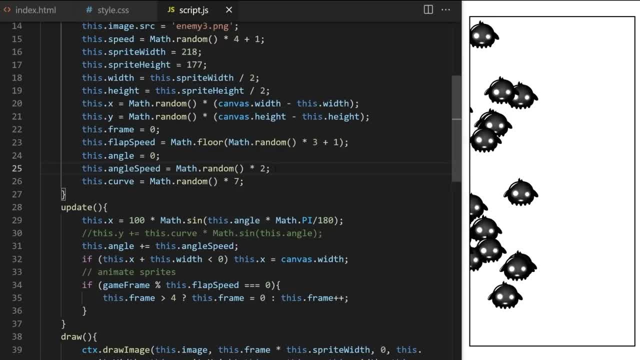 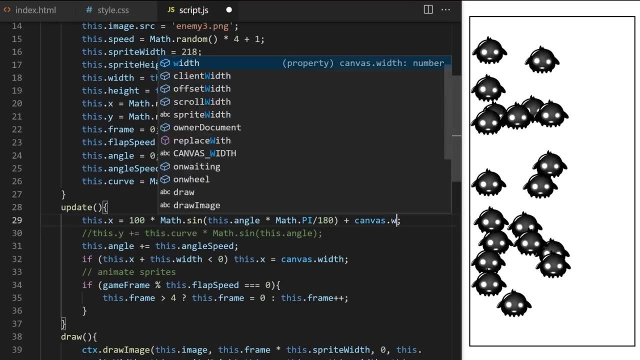 Times. 2 might be a good speed, for now They kinda disappear behind canvas edge. I can move them by adding some value to thisexposition Like this: Plus 10 will move everything slightly to the right. Plus 100? How about plus canvas width divided by 2?? 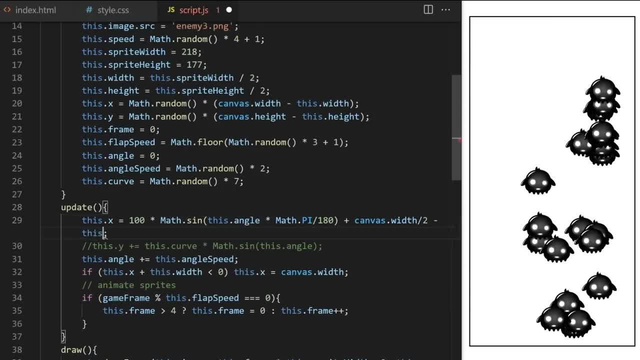 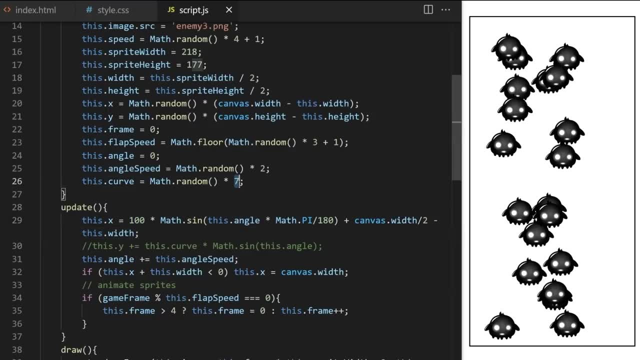 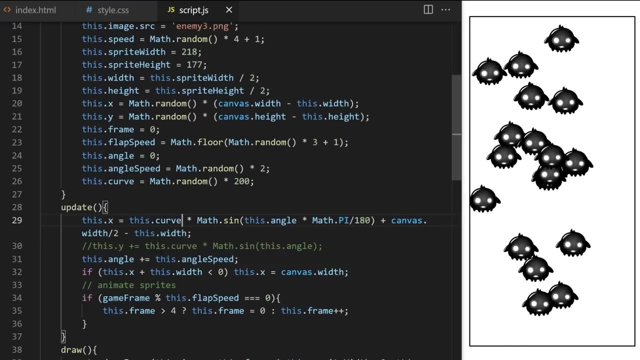 I want to center them horizontally. Now they are too much to the right. I need to offset them by the amount of their width. I change this dot curve on line 26 to be a random number between 0 and 200.. And I replace hardcoded 100 on line 29 with this dot curve property. 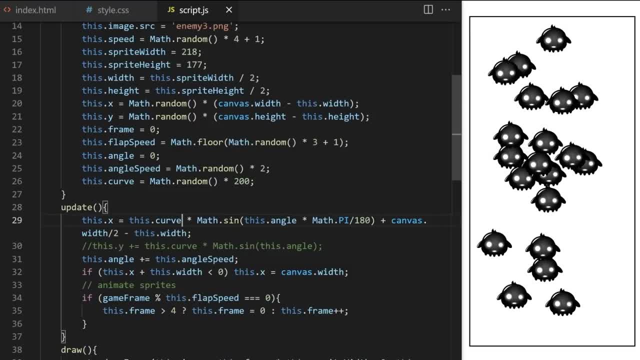 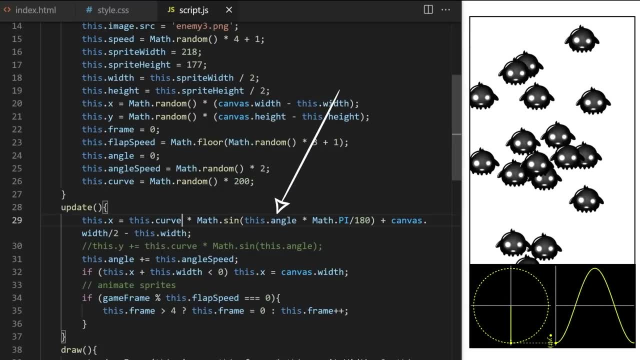 Now, some of them move in a large range, Some only in a small area. As we said before mathsign, when we feed it an angle, it will return a value between plus 1 and minus 1.. Since this angle is ever increasing, on line 31, we are getting a continuous series of 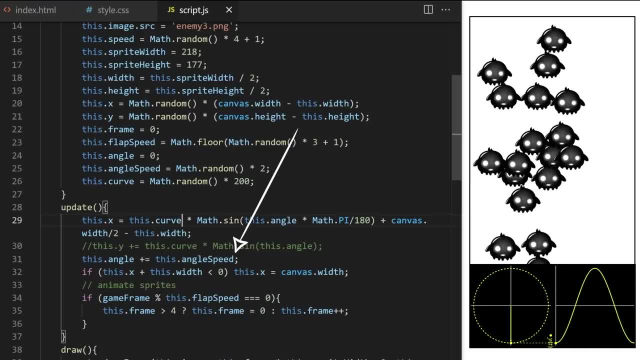 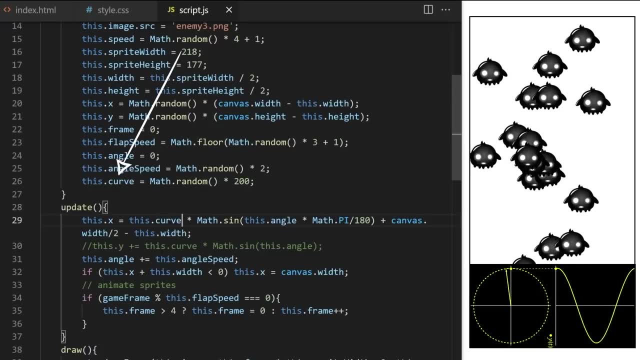 values that endlessly bounce between minus 1 and plus 1.. By multiplying all of this by this dot curve- here for characters that have this dot curve, 200, for example- they are endlessly cycling between minus 200 and plus 200.. Put it in brackets. 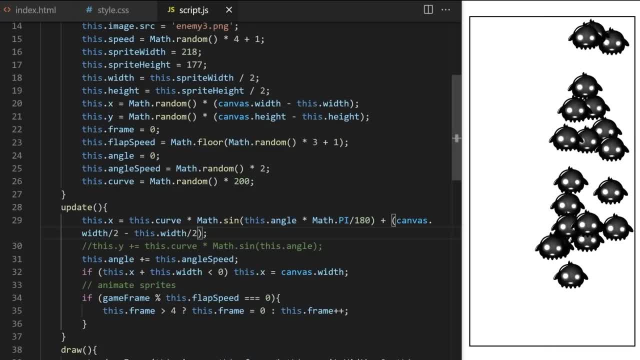 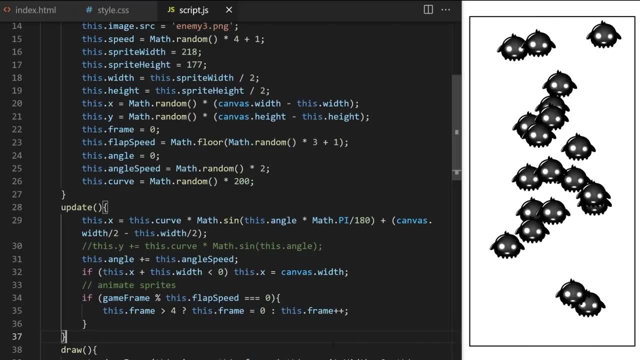 Actually this has to be this dot width divided by 2.. Yeah, now they are centered horizontally On line 29,. we are animating horizontal X position. Let's also do this with this dot Y on line 30 and see what happens. 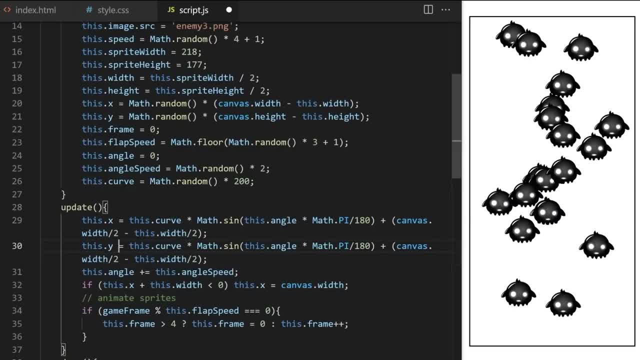 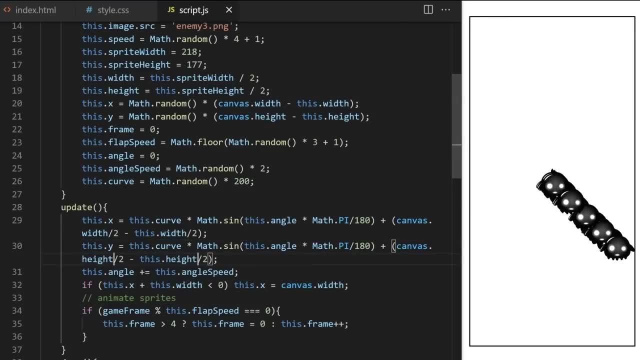 If I copy the same formula and replace width with height, because we are dealing with vertical movement, we get this pattern. This is where cosine comes in. I am not going to explain trigonometry in detail in this video, but the main idea is. 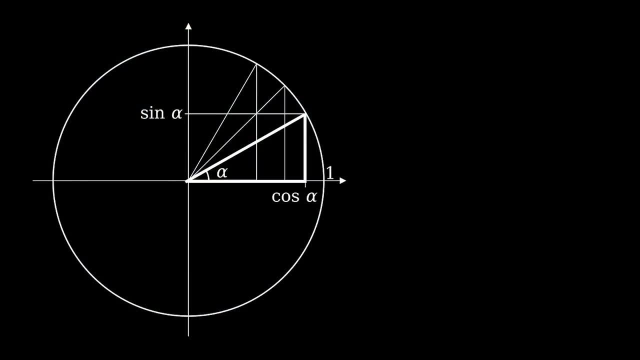 you have a circle and radius of that circle can represent hypotenuse, the longest side of a right angle triangle. If we connect lines like this to complete the triangle, sine value represents relationship between opposite side of the triangle and hypotenuse. cosine is the relationship between the adjacent side of that triangle and hypotenuse. 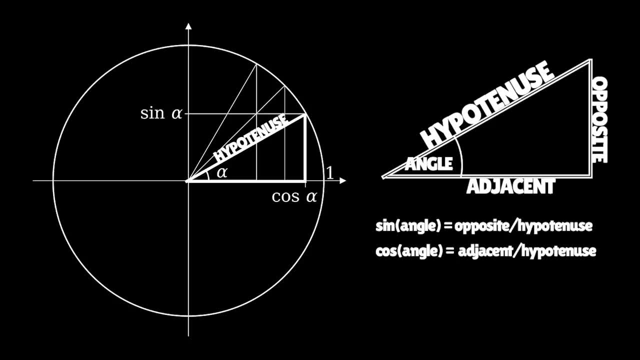 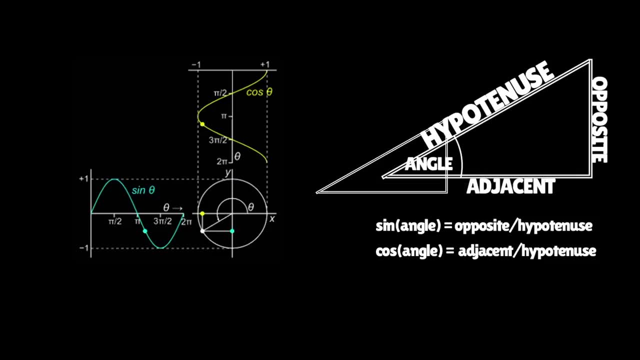 Hypotenuse size never changes, but sine and cosine cycle periodically as the size of opposite and adjacent side of this imaginary triangle changes. As a result, sine and cosine complement each other to map a circular path, And that's what we are taking advantage of here. 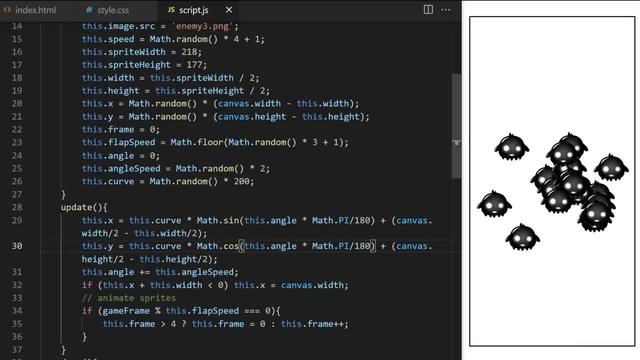 Mathsine is creating periodical horizontal movement for me on line 29, and on line 30, mathcosine is doing that for vertical values. Together they complement each other in a way that results in a circular movement. You can play with these values: swap sine and cosine, make both of them sine or cosine. 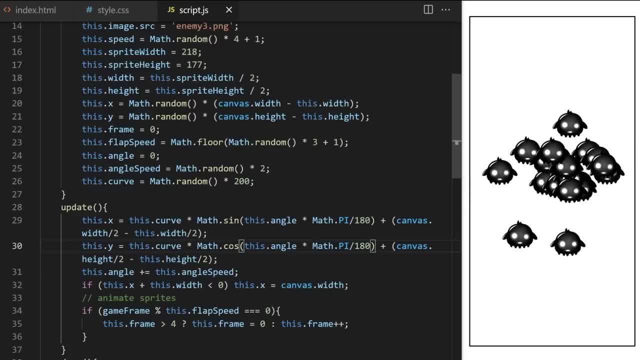 it should illustrate it better what's going on, if you see how these changes affect our animation. If I want to have some space in the middle, we know that this dot curve determines radius of the circle my characters are moving in. That value is randomized for each one. 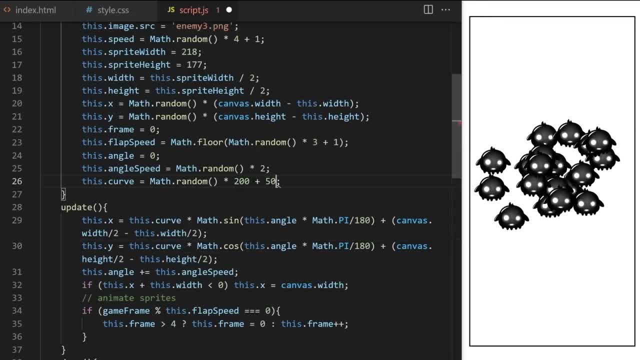 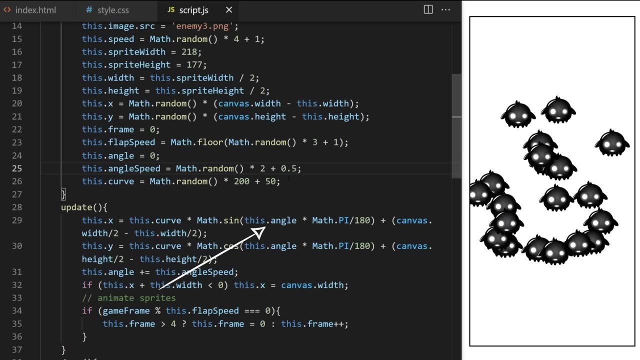 I can give it a minimum value. for example, let's do a random number between 50 and 250.. I can also change angle speed on line 25.. This will affect how fast angle is increasing on line 31.. And because that angle is being passed over and over to mathsine and mathcosine. 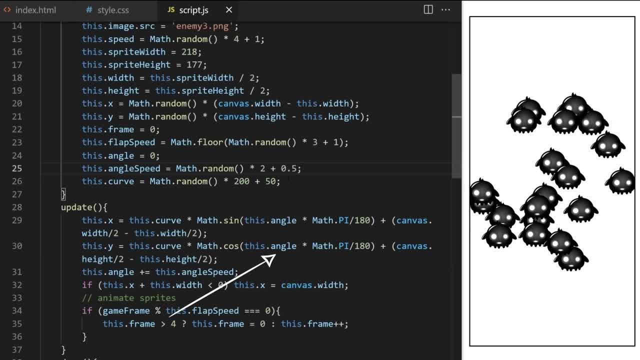 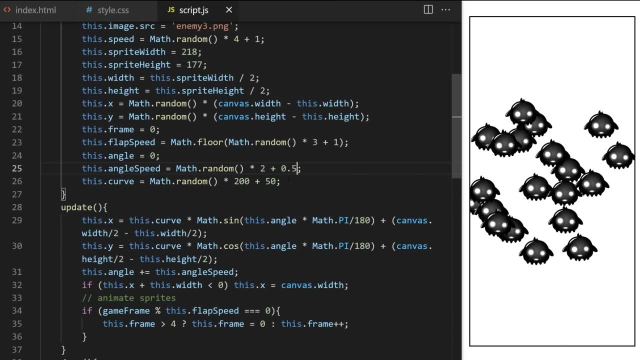 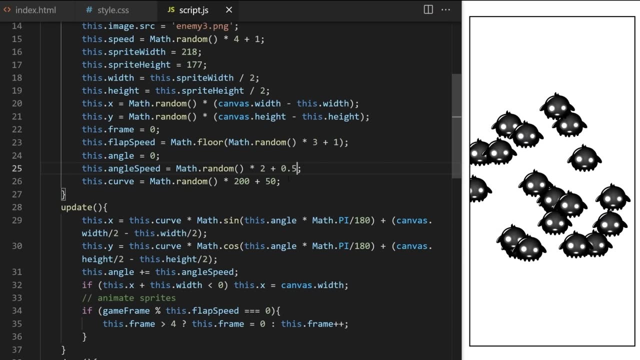 it will increase that speed at which our characters move along the circular path. See, here we already have some interesting movement pattern for our enemies. I could use this in some parts of my game Right now. sine and cosine are even. What I mean is they cycle between the same set of values over and over. 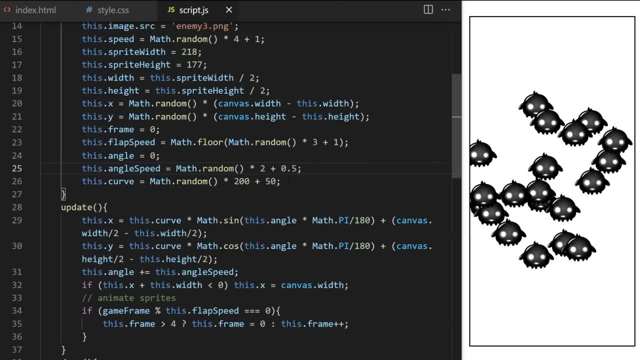 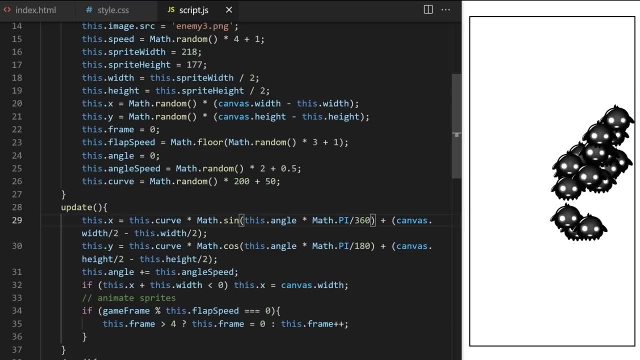 which results in even circular movement. What if I make the horizontal position to cycle at half the speed compared to vertical position By saying mathpi divided by 360? here Now, vertical position does two cycles, while horizontal position does only one, Because of the difference between 360 and 180.. 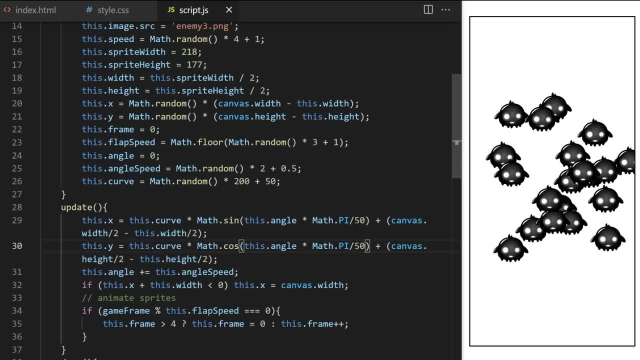 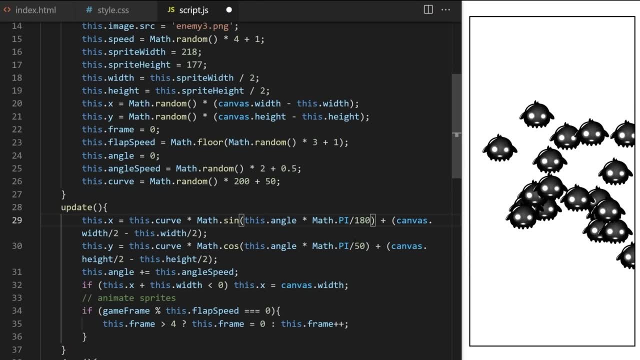 These two values here. This will give us a different movement pattern. If I give both of them the same number, it will be a circle. Smaller numbers will result in a faster movement. The result in movement is always a relationship between these two values. 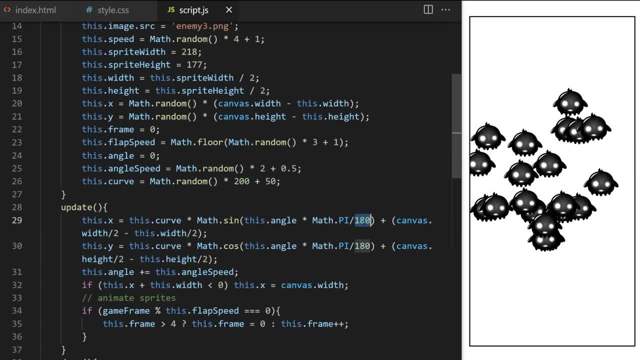 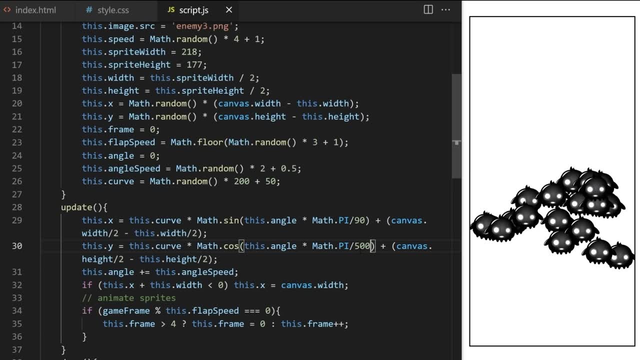 These values don't have to be directly divisible by one another, but it might help to visualize it better. For example, here horizontal position will go over five cycles, while vertical position will do one cycle. It's because of the relationship between 90 and 500. 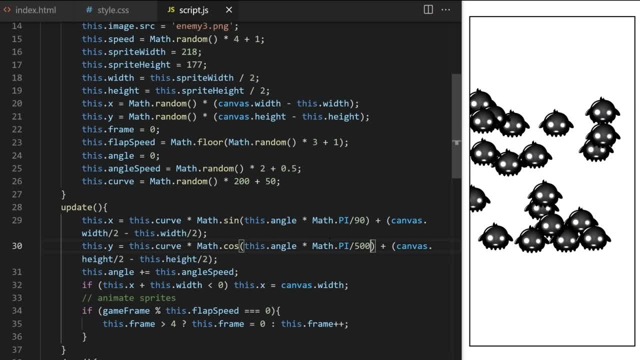 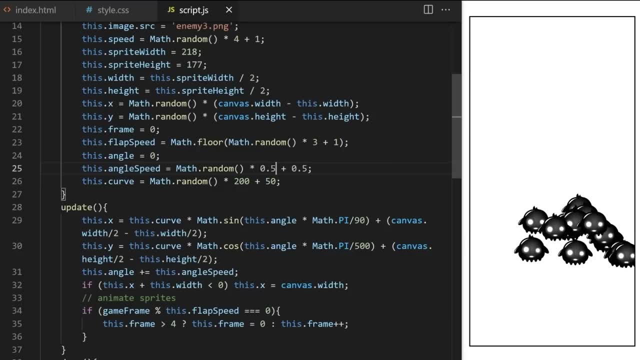 It gives us interesting movement. I can change their speed also by adjusting thisangleSpeed on line 25.. So this technique can be customized to achieve movement pattern you are looking for. Maybe your game starts easy, but later it becomes more difficult, so you need faster enemies. 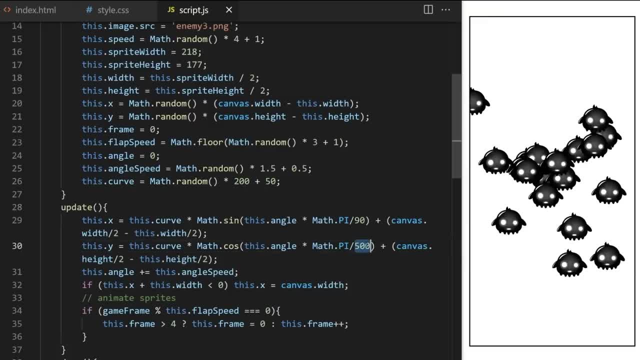 If I put 360 here, 360 is divisible by 90.. If you watch the animation, we will get four horizontal cycles before we get one vertical cycle, Because 360 divided by 90 is 4.. Don't feel like you have to fully understand sine and cosine at this stage to take advantage of this technique. 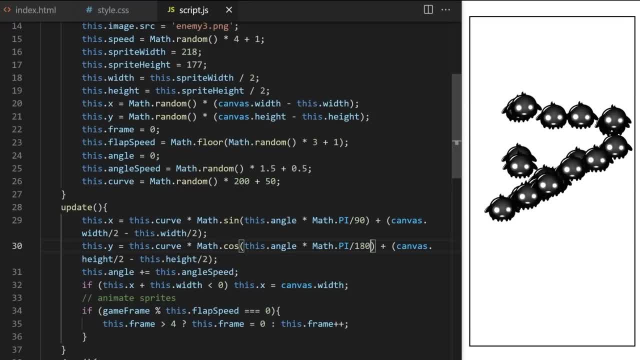 I will make a special video where we deep dive into this functionality. For now, this is all we need to know to be able to use this for our games. If I want the shape to be number 8, I can just make vertical value double of horizontal value here. 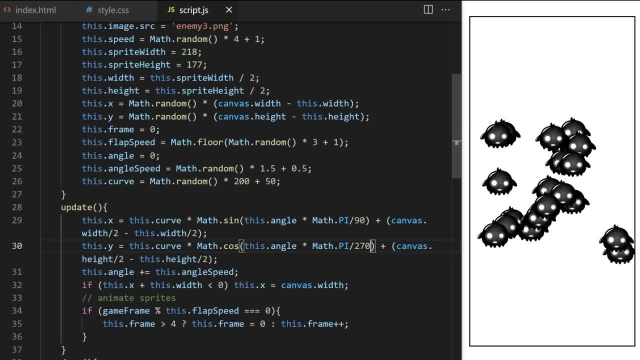 I can play with different numbers and see what happens. I can also have cosine for both. like this, It will cause them to backtrack, to go back and forth following the same path, rather than moving in circles. Swapping sine and cosine will make our characters follow circular path in the opposite direction. 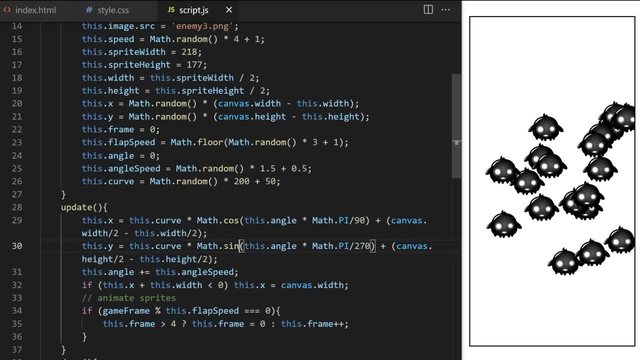 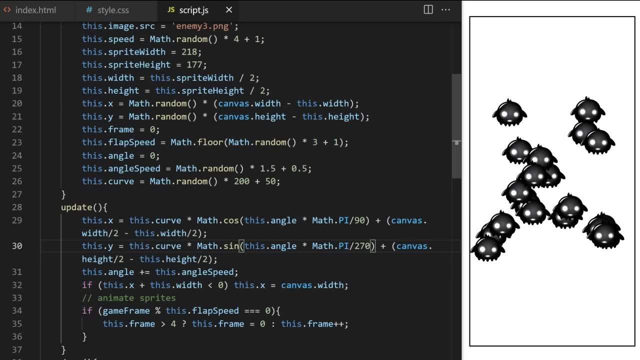 I don't like how they fill the entire width but they don't fill the height of my canvas. How do I make them use all available space? We are using this dot curve, which is a random number between 50 and 250.. 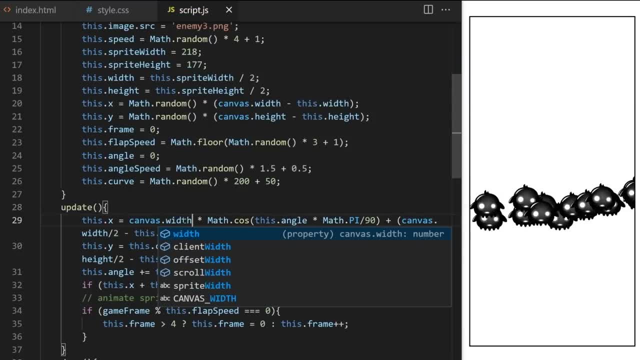 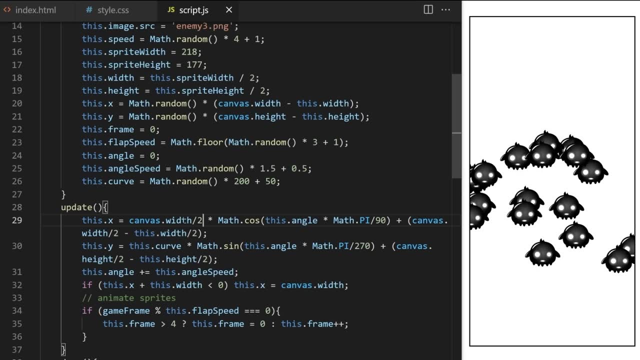 And it makes them move within that range. What if I replace it with canvas width on line 29?? Okay, that's too much, because this value is radius of their movement: half circle. If I want them to cover width of canvas, I need to give them canvas width divided by 2.. 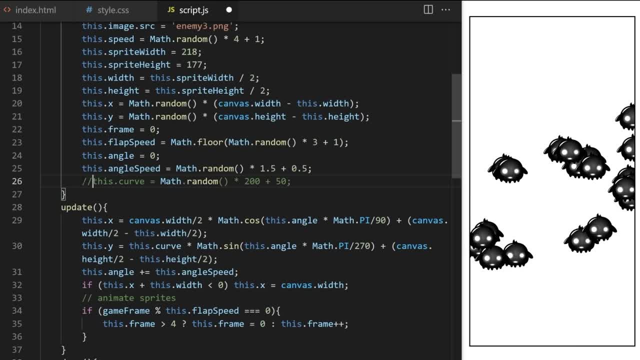 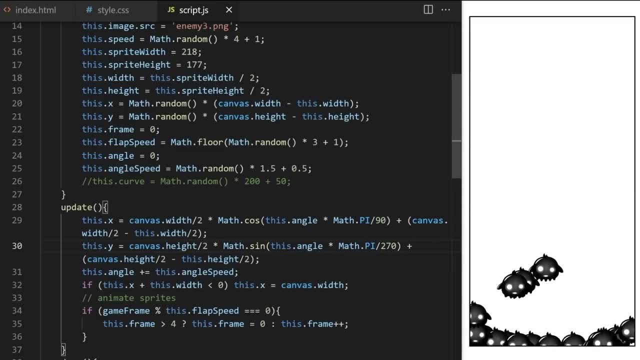 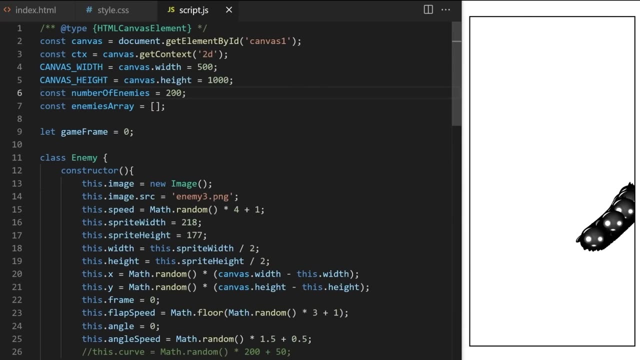 Much better. Let's do the same for vertical position on line 30.. Canvas height divided by 2.. Awesome, now our movement path is even more obvious. I will increase number of enemies on line 6, just so that we fill the path with more objects and see it better. 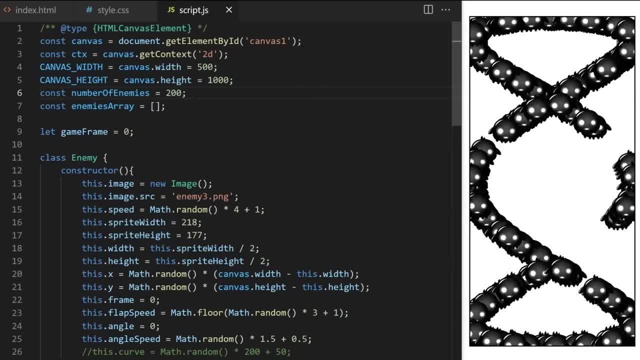 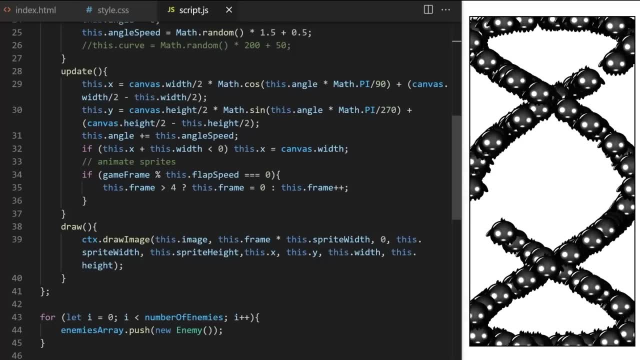 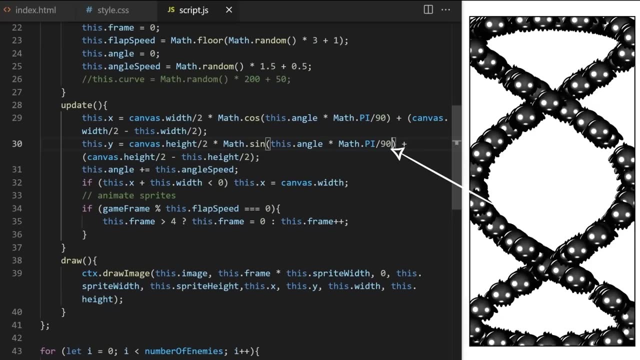 Now you can clearly see that our enemies are running along a set path. Shape of this particular path is determined by relationship between 90 and 270. here Three horizontal cycles fit into one, Because 270 divided by 90 is 3.. If I make the values the same, we get circular path again. 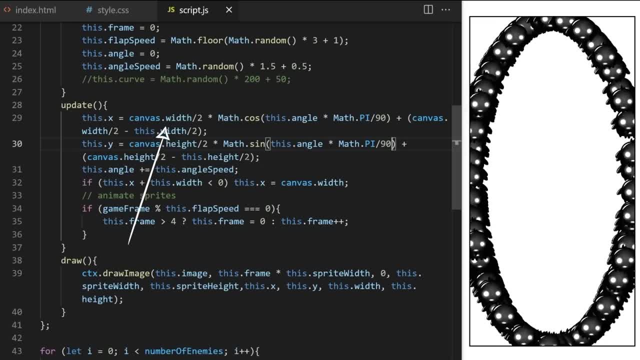 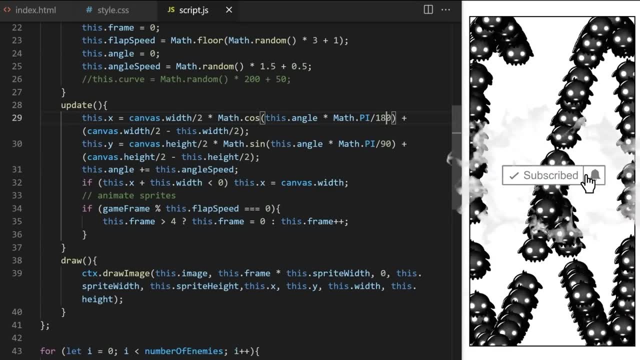 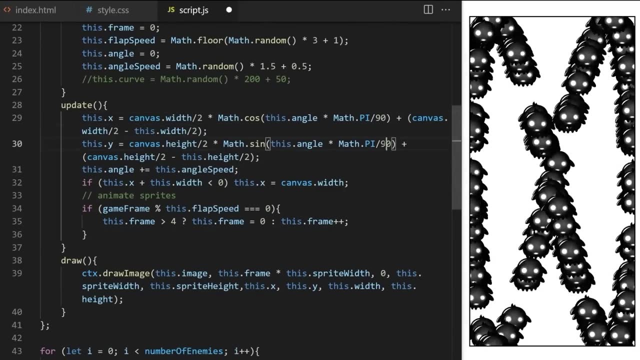 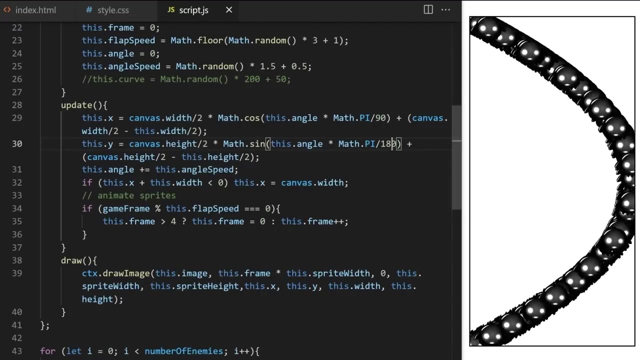 It's an ellipse because I'm stretching the movement here and here. 180 in X and 90 in Y will mean two vertical cycles happen before we get one horizontal cycle. What happens if I swap 180 and 90?? Interesting To get 8 shape, I would have to swap sine and cosine here. 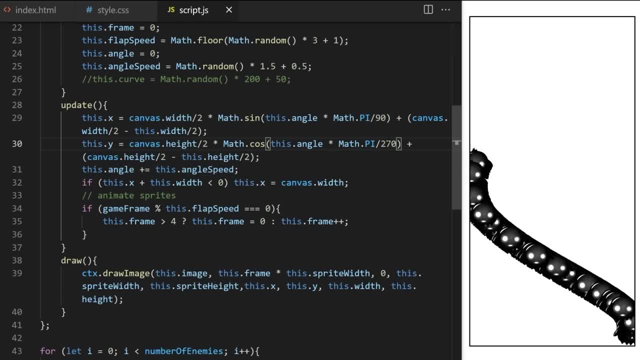 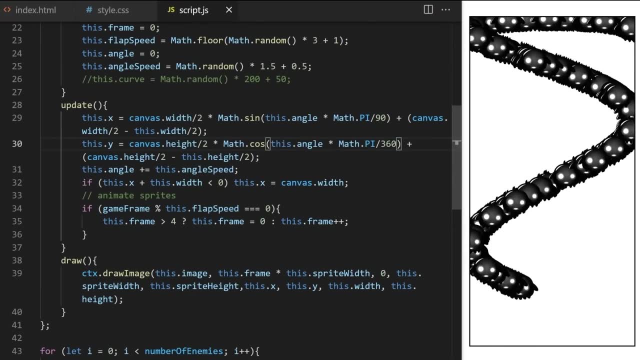 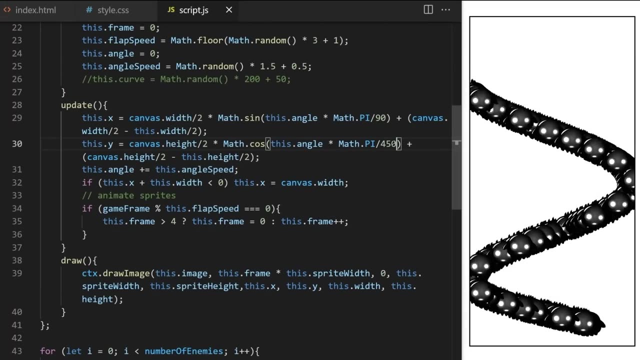 Are you starting to understand how these values affect the shape of path our animated characters take? You can play with this for a while. experiment with different values and see what happens on canvas. Trial and error can sometimes be the best way to come up with unique, interesting results. 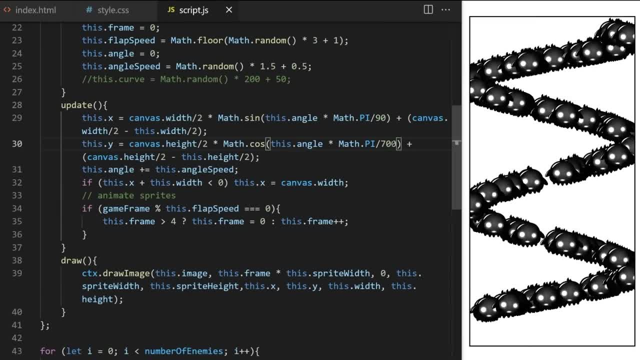 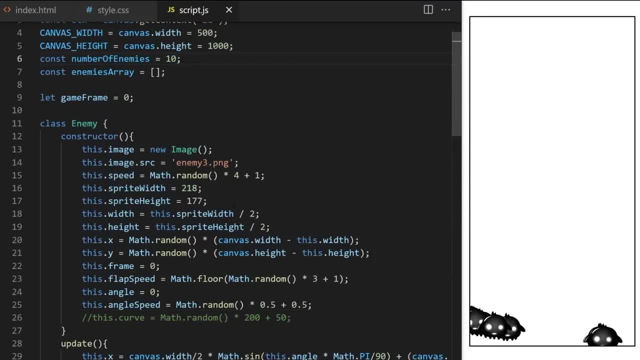 Trigonometry is a big topic and we will come back to it in some other course. I'm sure some of you get other ideas for this technique. It doesn't have to be used for patrolling enemies in games, as we are doing here. 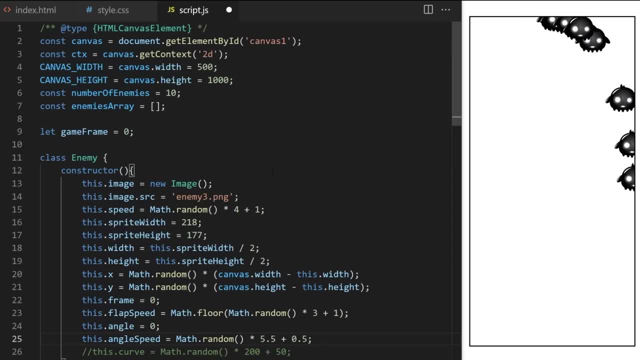 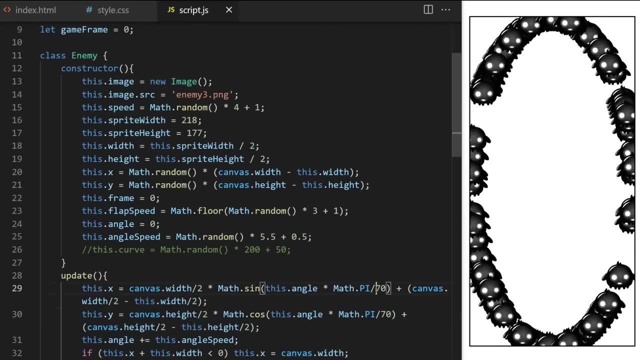 You can, for example, use it to create automatically moving particle effects and animations for website and many other things. Creative coding gives us a lot of opportunities to come up with unique, beautiful stuff, And that's why we are building these projects together. 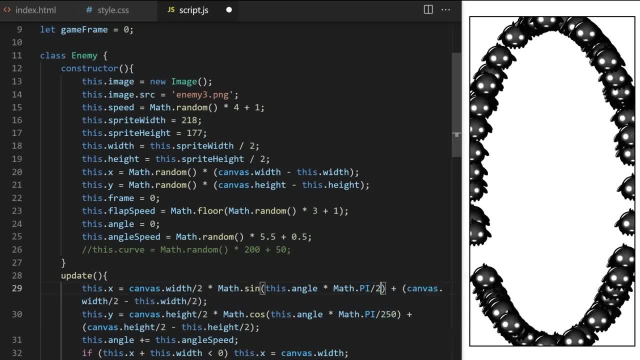 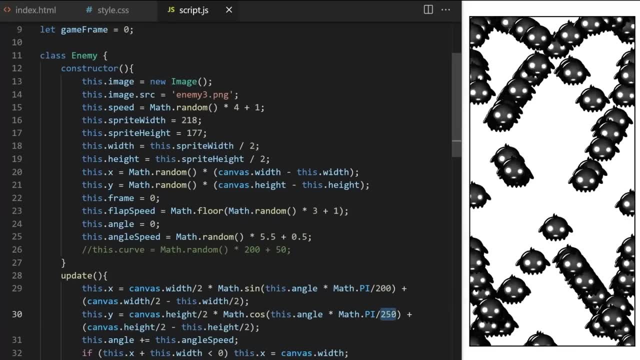 To improve our vanilla JavaScript skills and, at the same time, to explore what's possible. Maybe it will spark new ideas in some of you. I know that there are many creative people watching my videos. I'm just here to give you the tools. Where you take it and how you decide to use it is up to you. 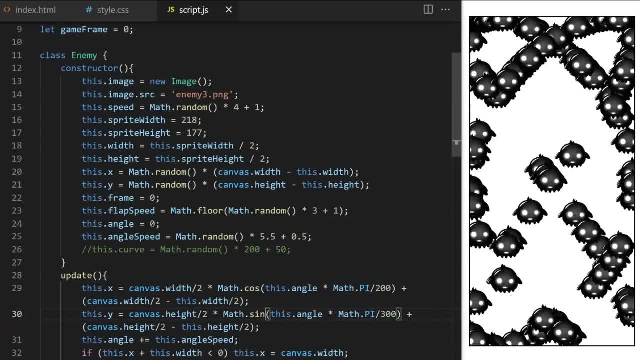 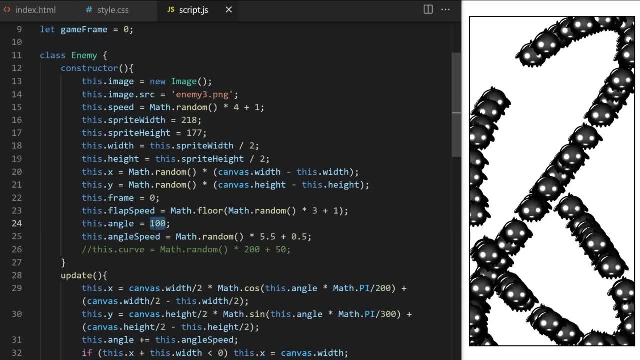 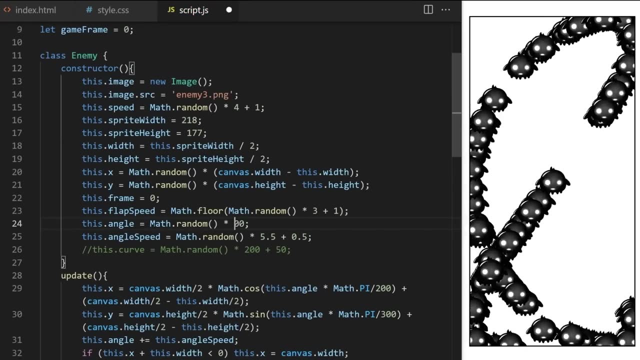 We can play with these values and create different paths. This angle property on line 24 determines where along our path our animated characters appear at first. I can spread their starting position along the path By using mathrandom. I could have also used something a bit more unusual, like oscillators or pearly noise here. 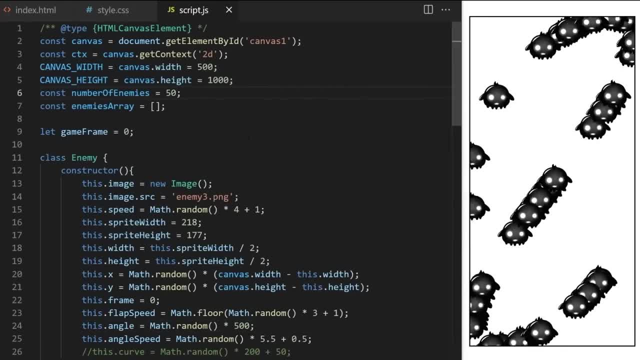 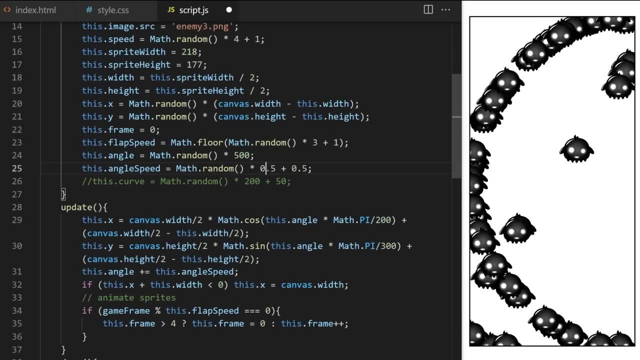 But I want to keep this video beginner friendly. We can do more advanced path following and random movement algorithms later. Another simple technique uses a completely different trick And it results in what I think is the best movement pattern If you want your enemies to appear like they have mind of their own. 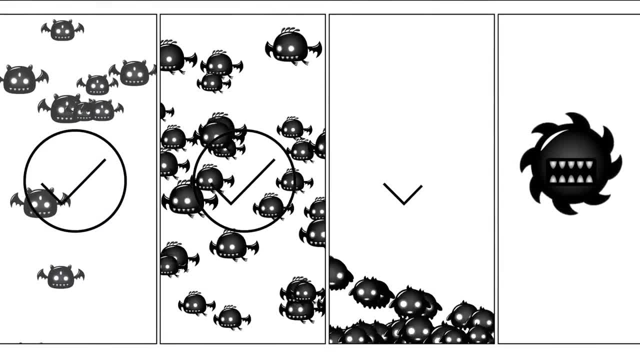 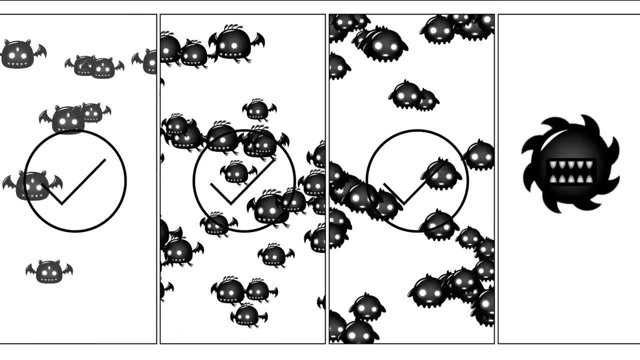 At least when we stay in the world of simple beginner algorithms. There are many advanced AI techniques you could use, But this is JavaScript for beginners. You might want to make a copy of this codebase Because, to achieve the next effect, I will break this one a little bit. 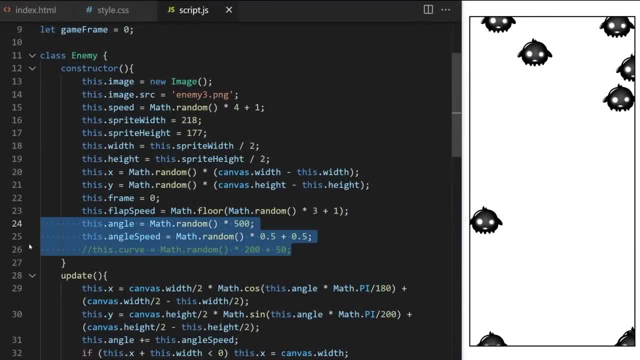 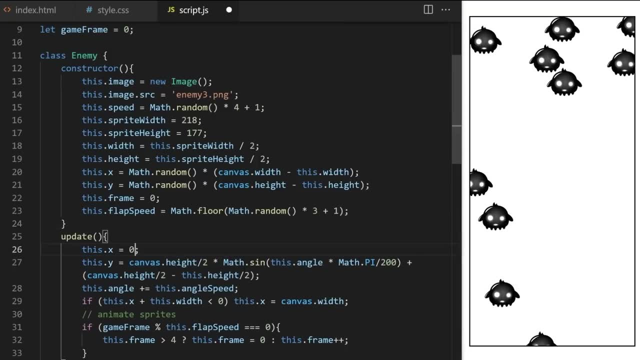 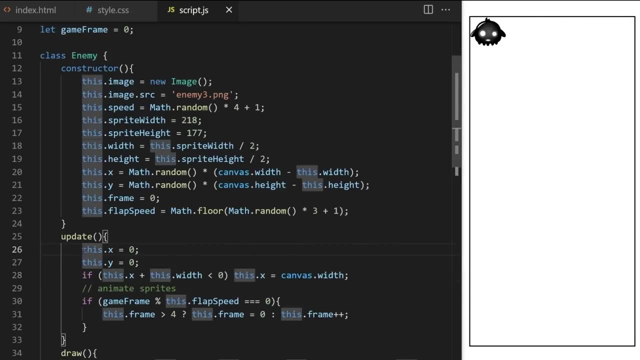 Let's delete lines 24, 25 and 26.. I will also set thisx and thisy to 0 inside my update method And I delete line 28.. I comment out lines 26 and 27.. And now initial x coordinate is randomized on line 20.. 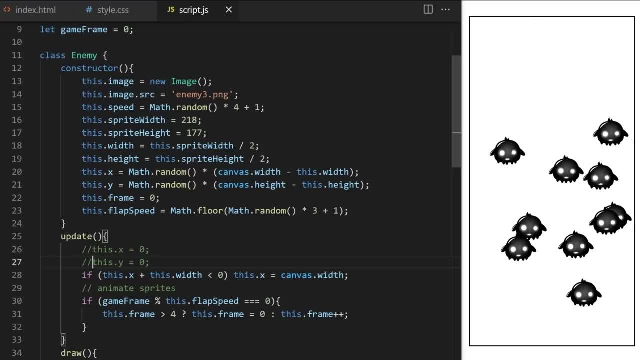 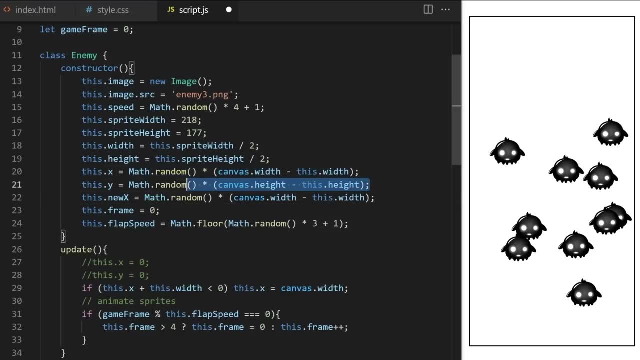 And vertical coordinate is randomized here on line 21.. I will create a new property. I call, for example, new x And I set it to random number between 0 and canvas width. I do the same for vertical y coordinate with thisnewy property. 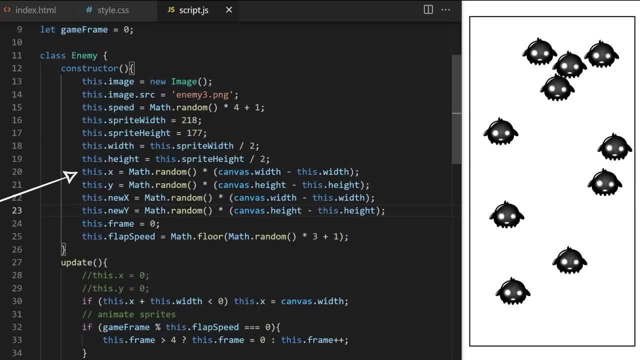 So I have initial horizontal position on line 20.. And I have new horizontal position on line 22.. On line 9 I have game frame variable That is endlessly increasing. inside my animation loop I will say every time game frame is divisible by 30.. 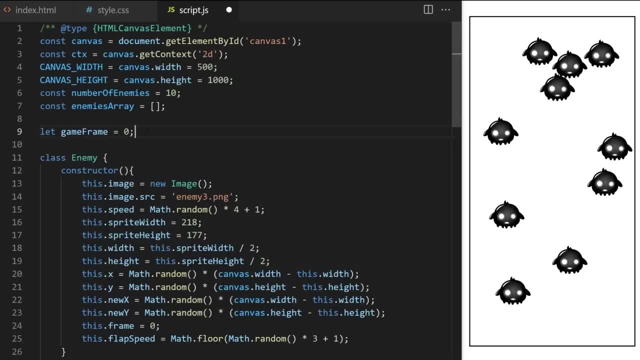 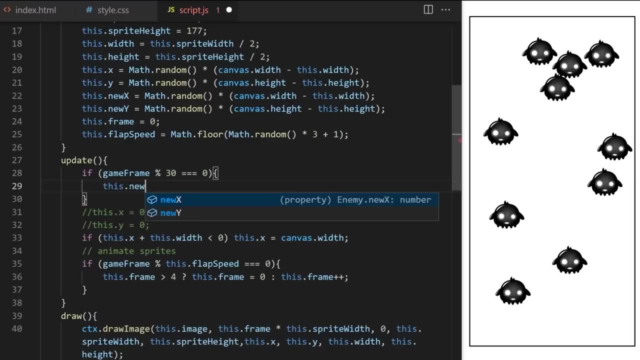 With a remainder of 0. Which basically means every 30 frames of my main animation loop. I want to reset thisnewx and thisnewy to different random position. Basically, I just need to copy lines 22 and 23 here. Now I will calculate variable. 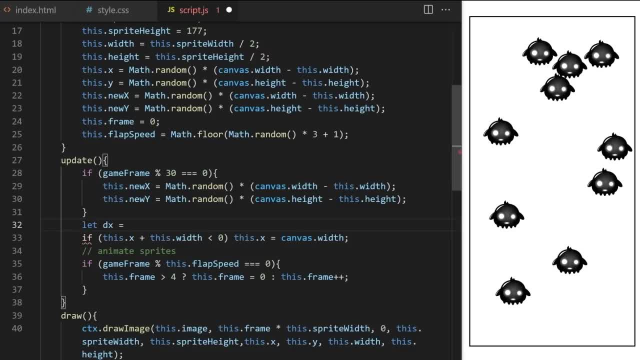 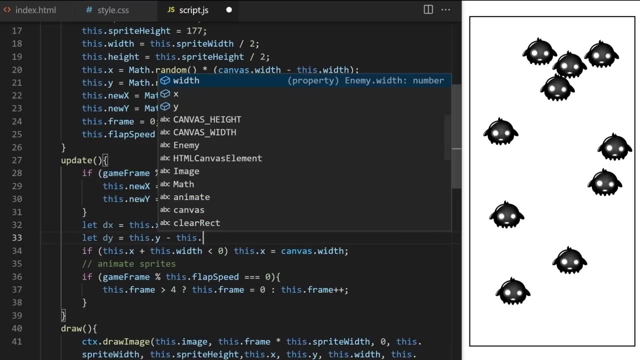 I call for example dx Distance on horizontal x axis. It simply is the difference between thisx from line 20 and thisnewx from line 22.. dy distance on vertical y axis is thisy from line 21 minus thisnewy from line 23.. 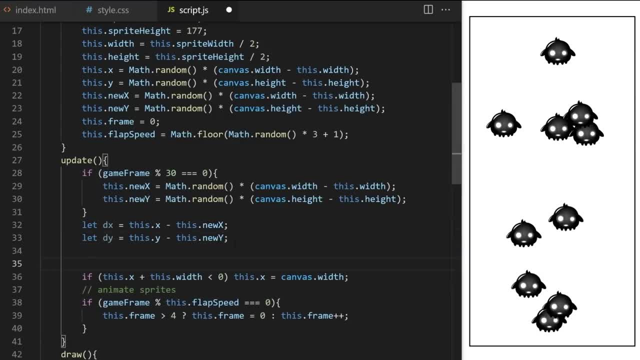 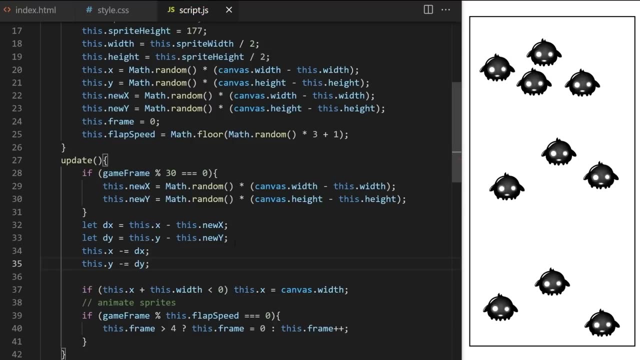 Now that we have distance between current position and the new position, I can make characters move towards that new position by saying: thisx minus equals dx from line 32.. And thisy minus equals dy from line 33.. It's resetting too fast. 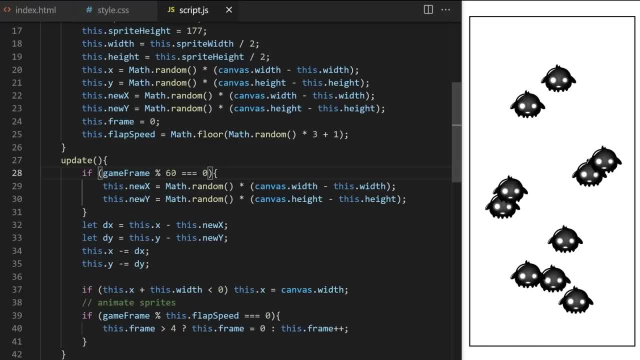 Let's change 30 to 60 here on line 28.. Now we get instant position change every 60 frames. I can make them travel towards that position by saying dx divided by 20.. I can also do that for vertical position by saying dy divided by 20 here. 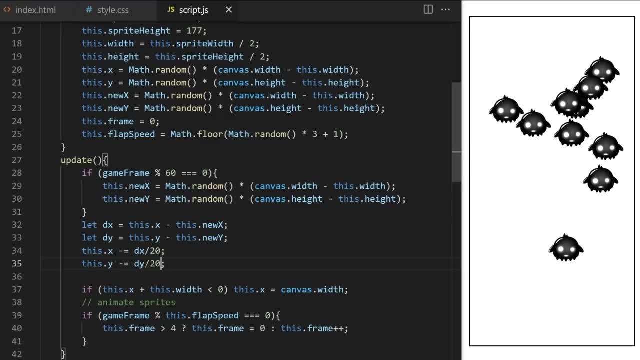 Now current position is always moving towards the new position by 20th of their distance for every animation frame. I can increase these numbers to make them move slower. I can also increase the interval on line 28.. I like this, but you can see that positions reset every 100 frames for all enemies at the same time. 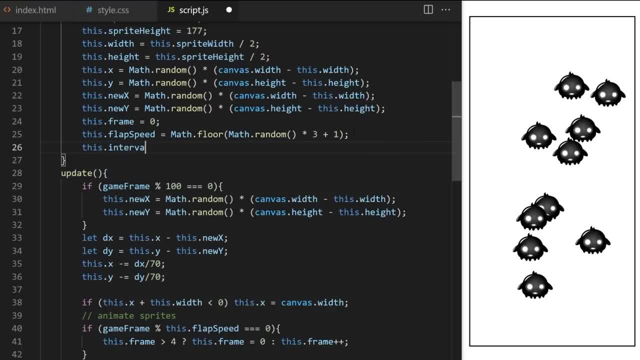 That looks a bit weird. I want each character to reset at its own randomized interval. I create a property, I call, for example, thisinterval, and it will be a random number between 50 and 250.. Then I replace hardcoded 100 with thisinterval on line 29.. 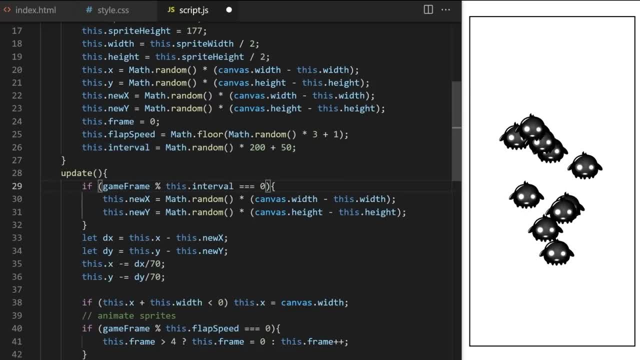 Then I replace hardcoded 100 with thisinterval on line 29.. It won't work yet, because thisinterval is a random number with decimal points, so gameframe will never be divisible by that very specific number with a remainder of 0. So new positions will never be calculated. 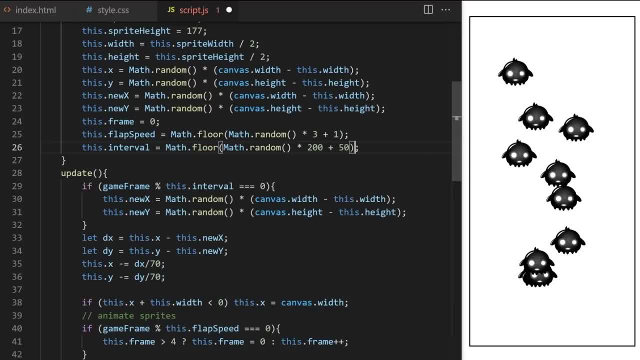 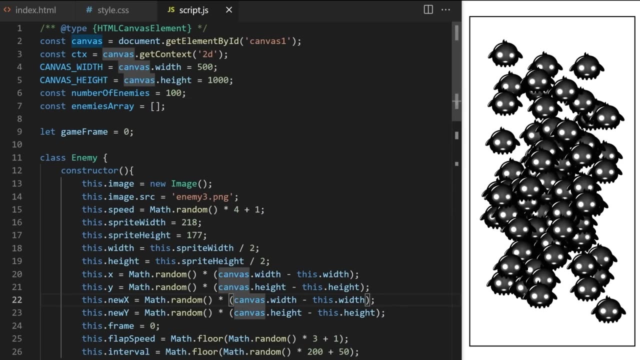 To fix that, I need to wrap this in mathfloor, which will round it down and make sure we get only integers, whole numbers, without decimal points. Awesome, Now you can see that each enemy is moving at their own rhythm. I can add more enemies on line 6.. 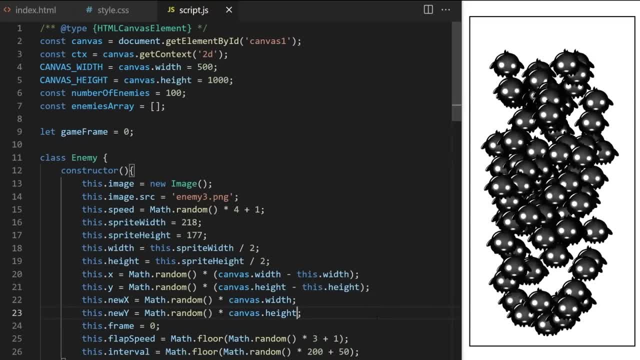 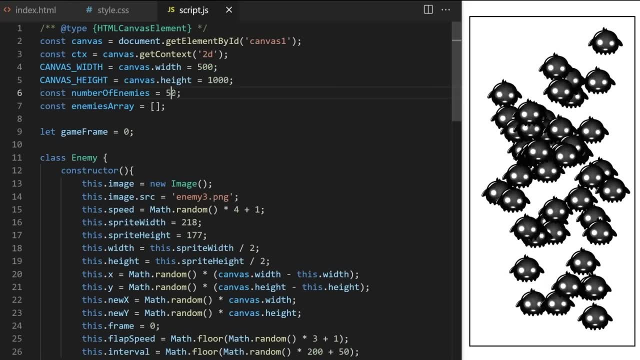 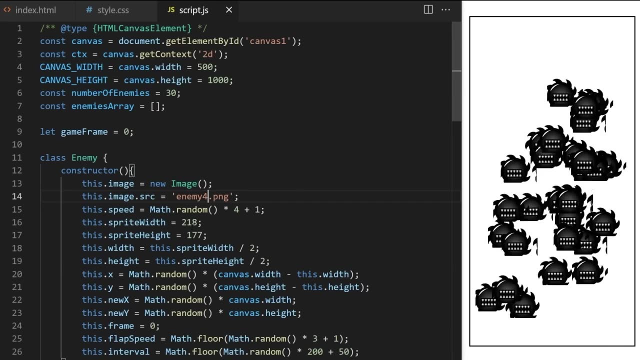 It kinda looks like a swarm of mosquitos. I also need to swap enemy sprite sheet. to keep up with tradition, I will use enemy 4png here. I look at my sprite sheet and width and height is 213 pixels this time. 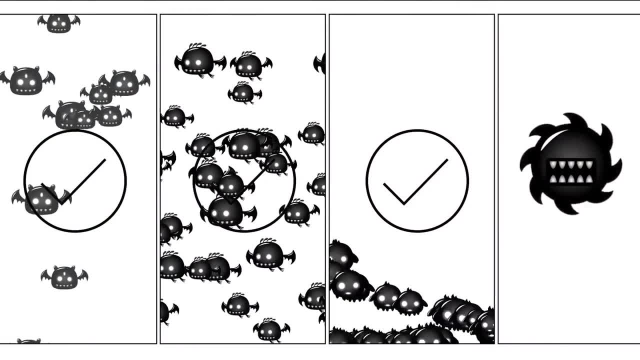 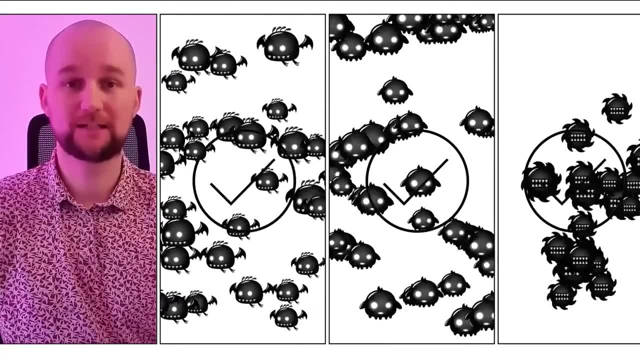 There are many other calculations and algorithms that you can use to make enemies move in a certain way. Let's make that today's challenge. Can you alter some of the code we wrote today and create your own movement pattern? You can also make enemies follow the mouse or maybe try to avoid it. 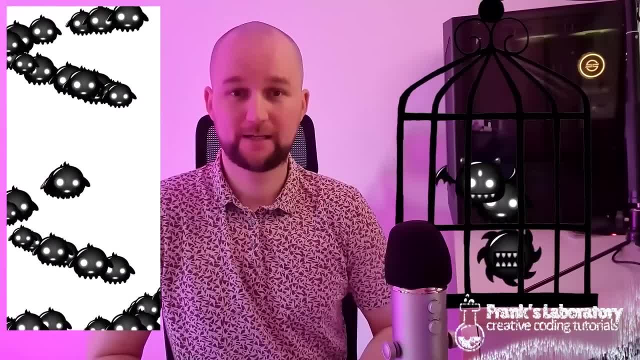 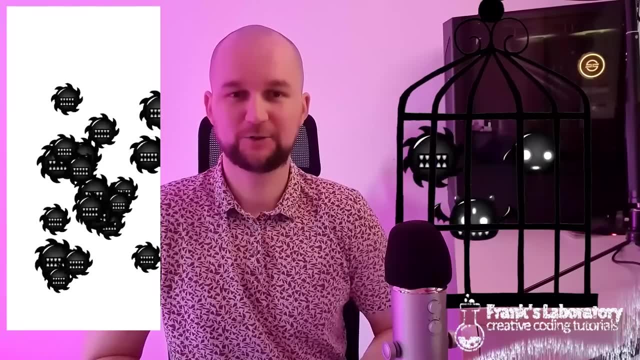 There are many ways to make this interactive. Let me know in the comments if you watched all the way here, If you did, well done. Today we added an important set of techniques to our vanilla JavaScript game development toolkit. I'll see you soon. 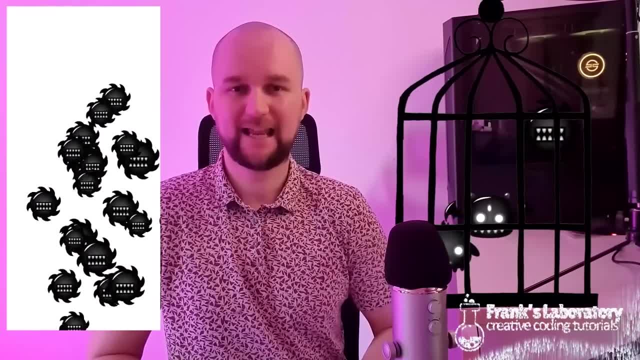 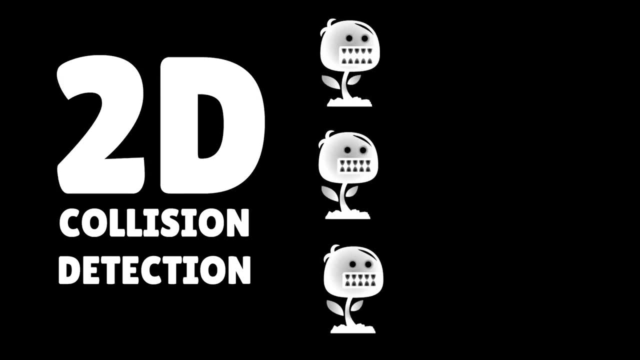 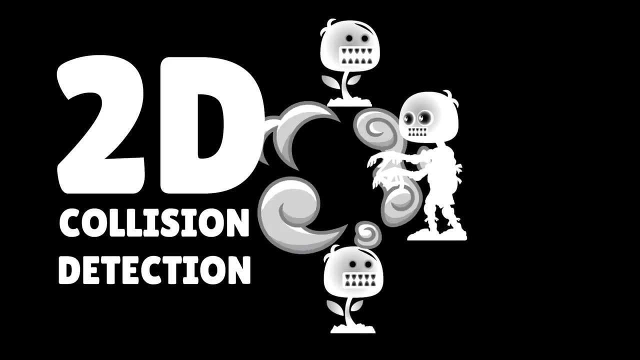 If you want more game development, check out my playlists- Links in the video description. Collision detection is important if you want to build the JavaScript games and you need to detect when two elements collide Or when you are building particle systems where objects interact with each other. 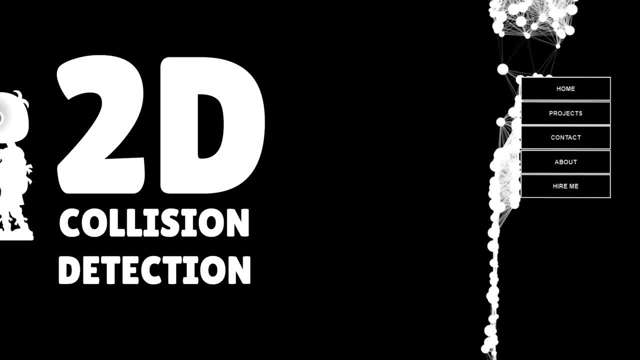 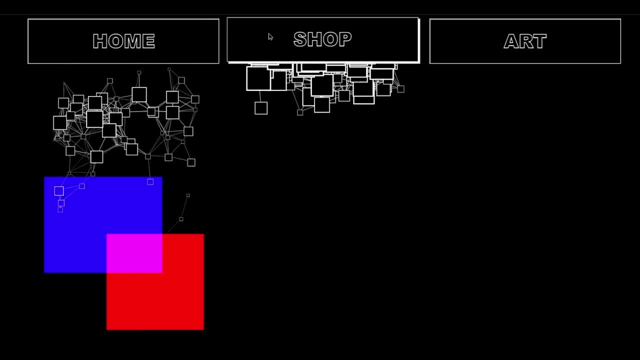 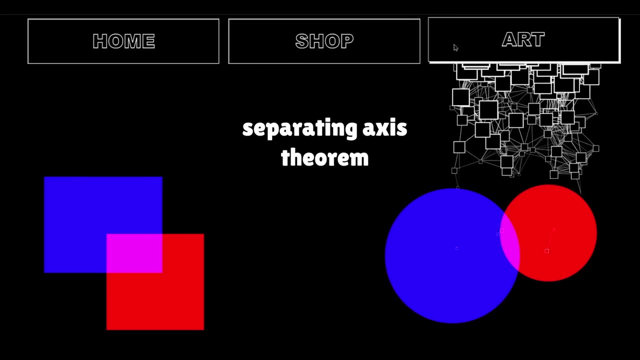 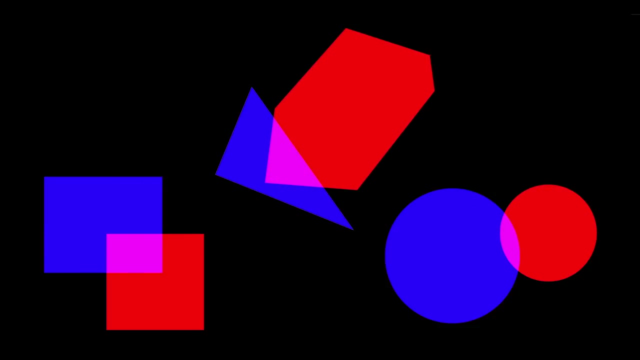 Or maybe you want your canvas animations to interact with regular website elements. For most projects, all we need is simple collision detection between two rectangles or between two circles. For more complex shapes, we also use collision detection technique called separating axis theorem. It can be used to detect collision between convex polygons or rectangles that are rotated and aren't axis aligned. 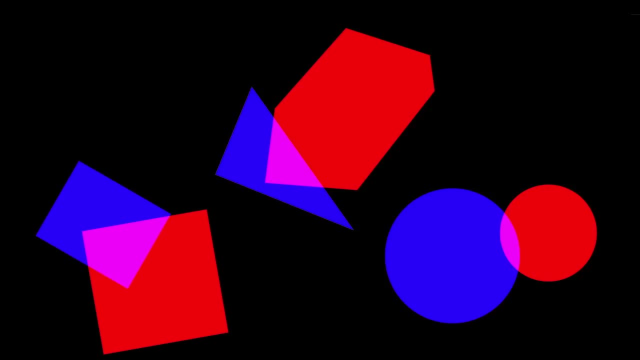 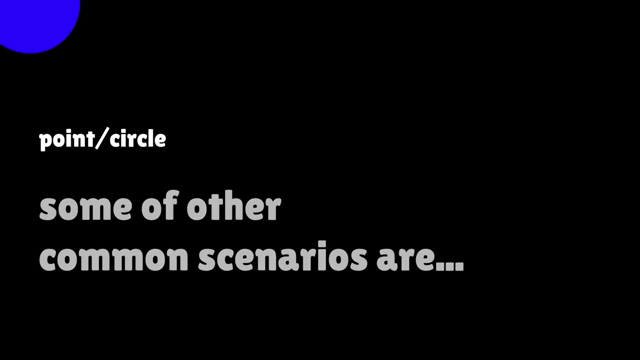 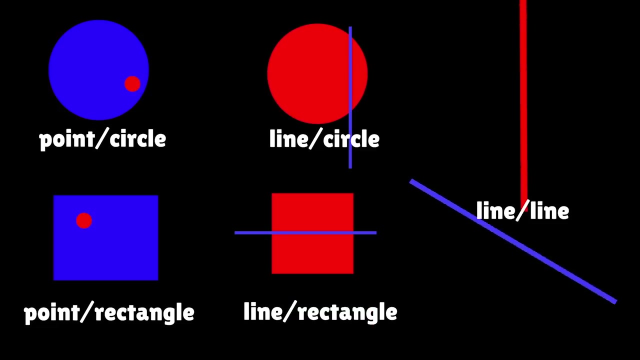 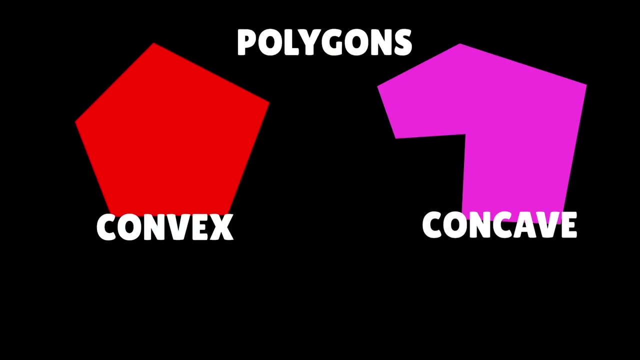 You might also have more specific needs for your games or creative coding projects. Some of other common scenarios are collision detection between point and circle, point and square between line and circle, line and square between two lines, and so on. It becomes more complex when you need to detect collisions where shapes such as convex and concave polygons are involved. 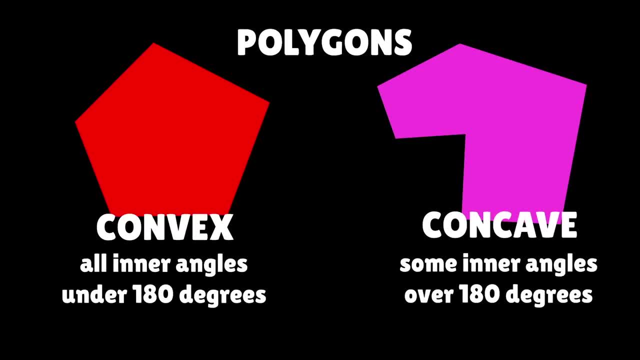 There are some clever tricks people came up with to handle these more advanced scenarios, such as detecting collision by color or projecting lines from a point and checking if the number of intersections between that line and polygon is odd or even number. With more complex shapes, it's a good practice to wrap them in simple rectangles. 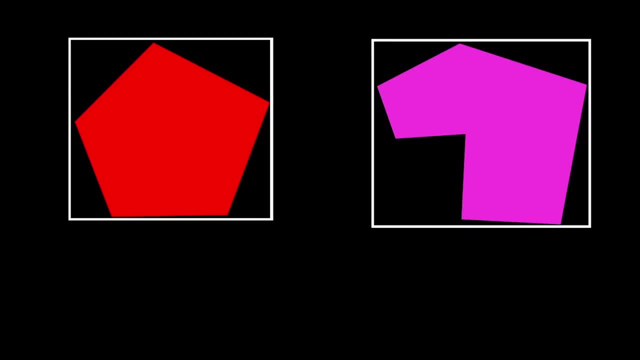 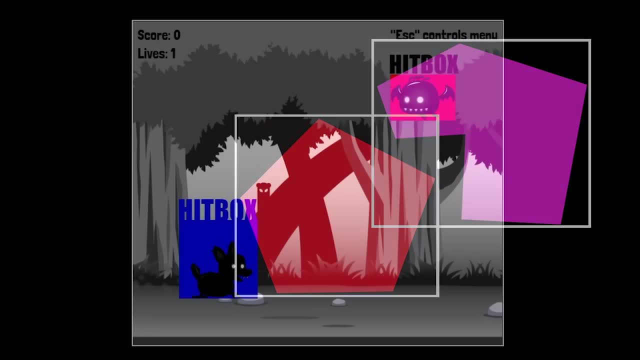 and only run advanced collision checks if these rectangles collide and we know that the shapes are close enough and collision is possible For many games, all you need is to create a generic shape around our objects, so-called hitbox, Even though the collision is not pixel perfect. 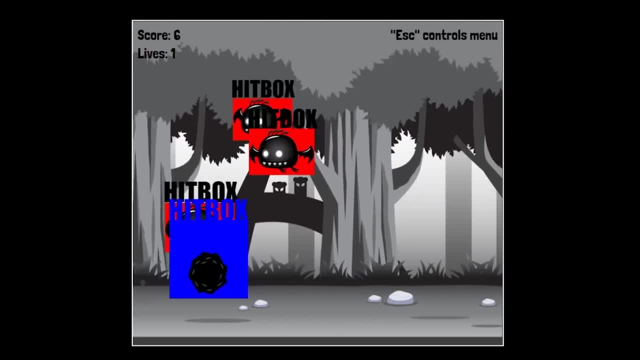 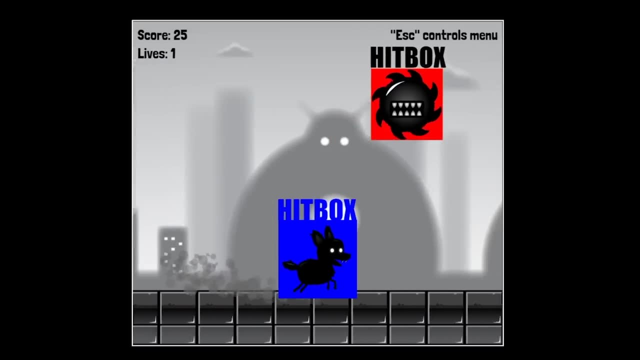 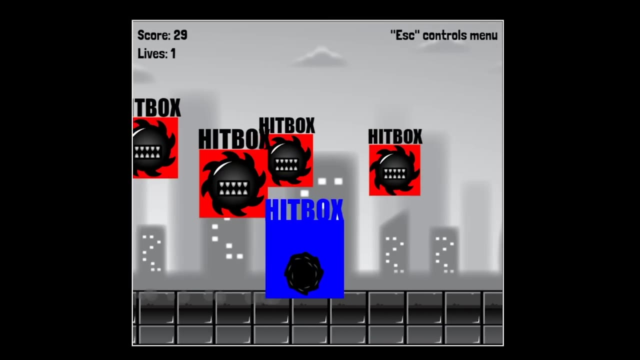 we can adjust these hitboxes to roughly match collision areas of objects with different shapes. Main advantage is that the code is very simple and performant, Because it doesn't require complex calculations to determine whether two objects collide or not. These hitboxes can have shape of rectangle, circle or polygon. 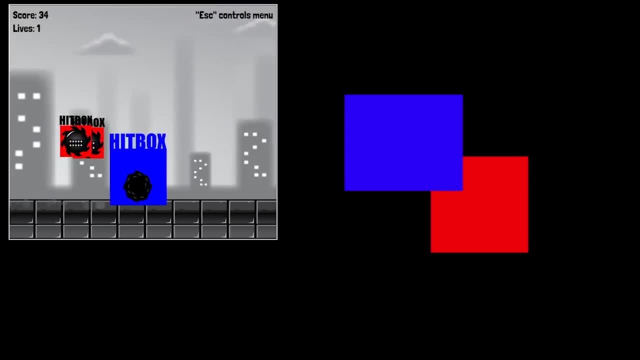 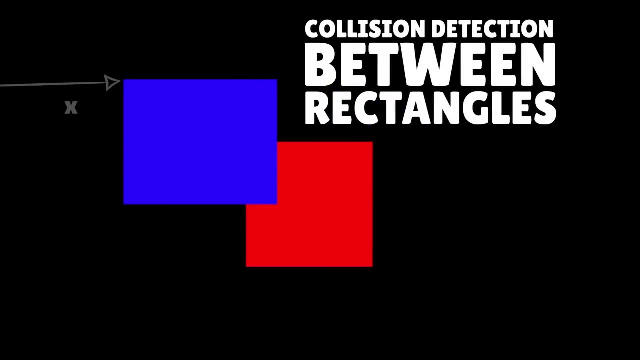 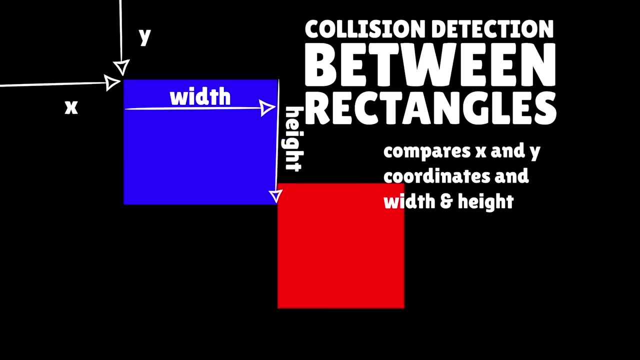 The simplest collision detection algorithm is between two rectangles that are axis aligned. It means that they are not rotated. It simply compares x and y coordinates and width and height of these two rectangles. If they overlap, we get collision. If there is a gap between them, we know there is no collision. 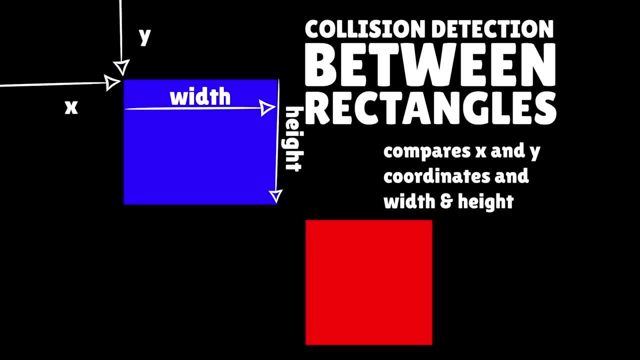 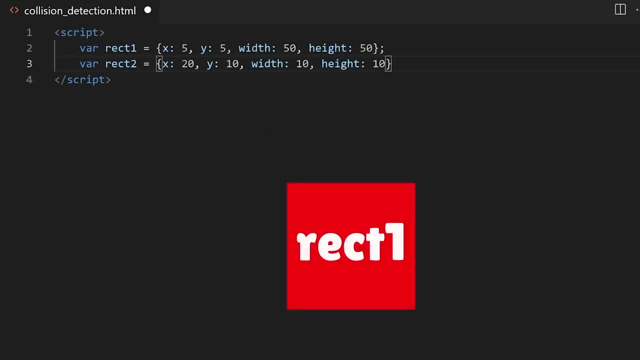 Let me show you two different simple algorithms you can use to detect collision between two rectangles, two hitboxes in our games. Let's say we have rectangle 1 and rectangle 2. Both of these objects have x and y coordinates and some width and height. 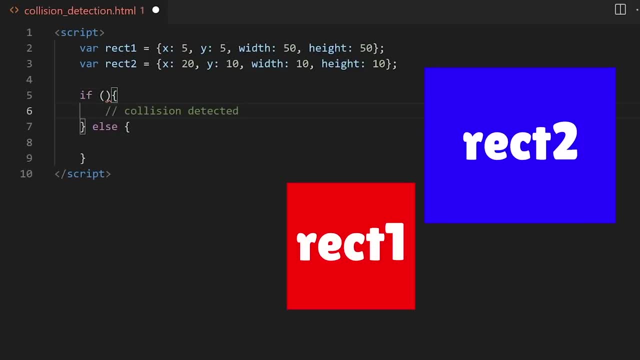 The first way I can check if they collide is this: I create a simple if statement and I check if horizontal position x of rectangle 1 is less than horizontal position x of rectangle 2 plus width of rectangle 2.. Basically, if this point is less than this point, 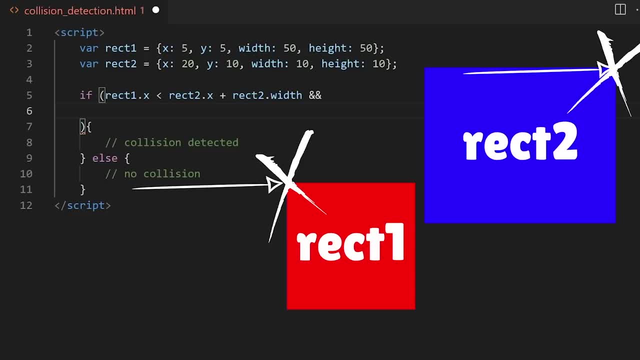 Less means if it's to the left on horizontal x-axis. At the same time, we want to check if x of rectangle 1 plus width of rectangle 1 is more than x of rectangle 2.. That means if this point is to the right from this point. 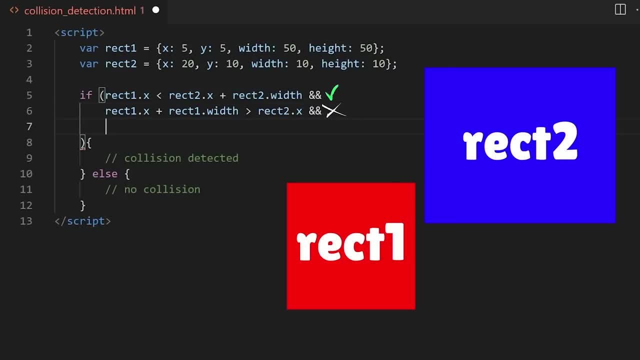 We also do this vertically. so we check if vertical y coordinate of rectangle 1 is less than vertical y of rectangle 2, plus height of rectangle 2.. If this point is above this point And lastly, we check if vertical coordinate of rectangle 1 plus height of rectangle 1. 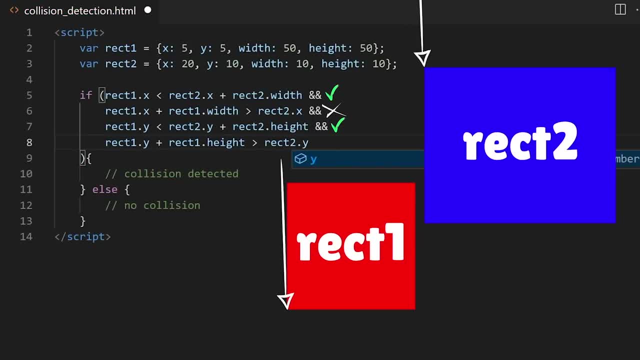 is more than horizontal y position of rectangle 2.. If this point is below this point, If all of these four conditions are true, we enter this code block in our if statement and collision is triggered. Else we know there is no collision. 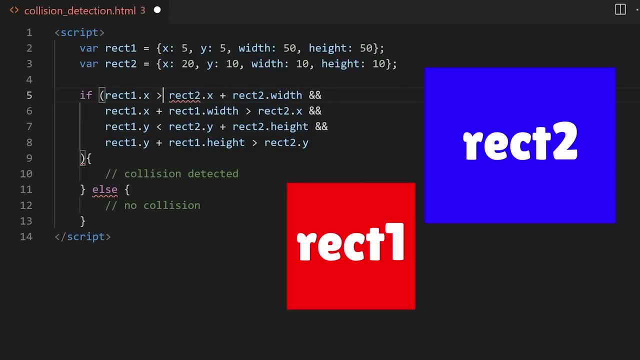 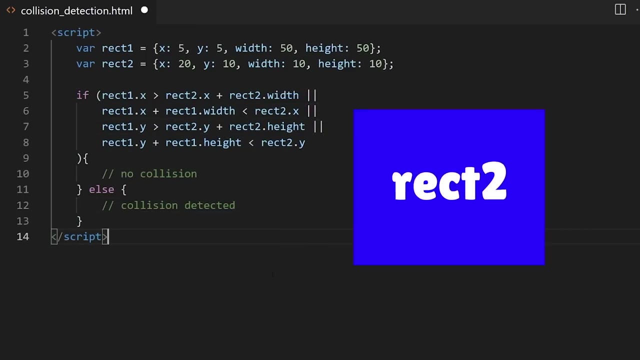 We can also flip the logic completely. This second algorithm does the same checks, but it's a bit more efficient. If I change the logic a little bit and use OR operator, it returns true if at least one of its operands are true. Let's go through the logic here. 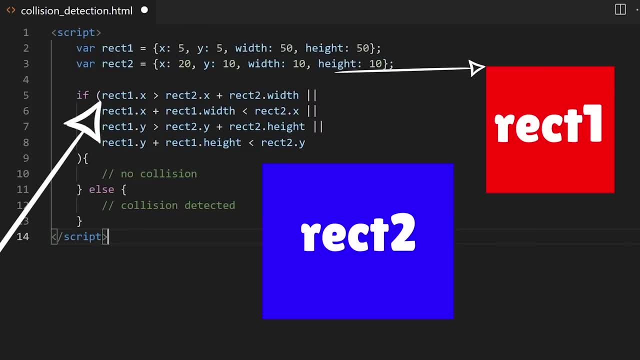 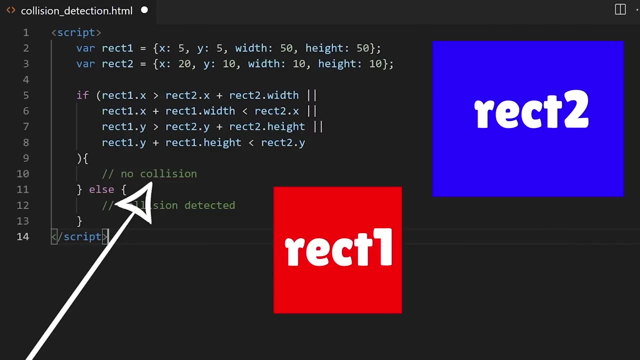 If x of rectangle 1 is more than x of rectangle 2 plus width of rectangle 2, we know they cannot possibly collide. So this will return true and we know straight away there is no collision. Also, if x of rectangle 1 plus width of rectangle 1, 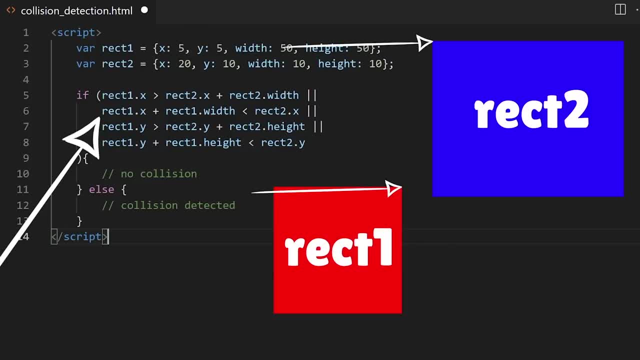 is less than x of rectangle 2, again, we know these rectangles can't possibly collide. Just one check and we know there is no collision If y of rectangle 1 is more than y of rectangle 2, plus height of rectangle 2,. 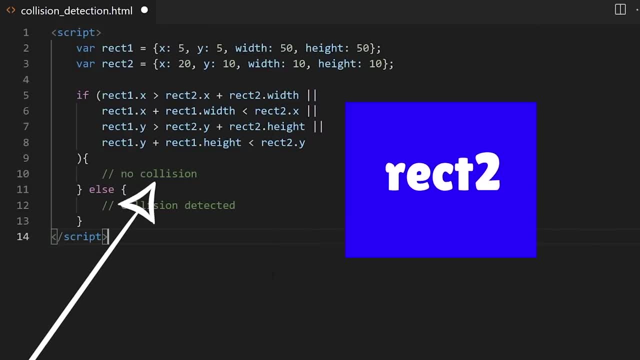 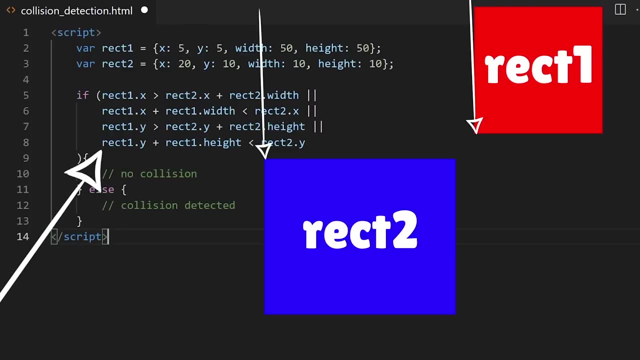 there is no way for collision to happen If y of rectangle 1 plus its height is less than y of rectangle 2, we also know they don't collide. So if at least one of these four checks is true, we know there is no collision. 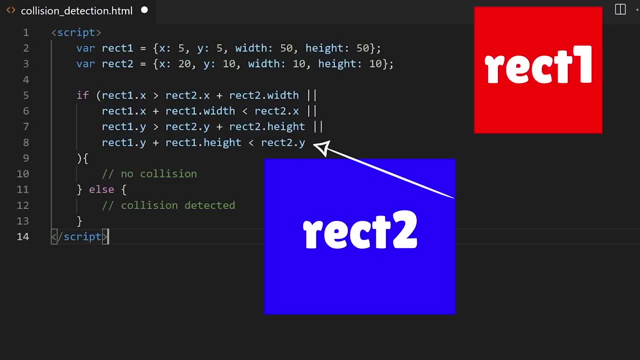 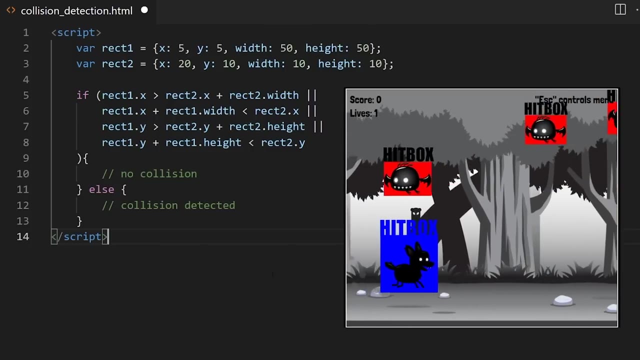 If all four return false, we know that the rectangles must collide, else statement is entered and collision is detected. I hope this was visual enough and you got some clarity on how these checks work. If you have any questions, let me know If you want to see how to implement. 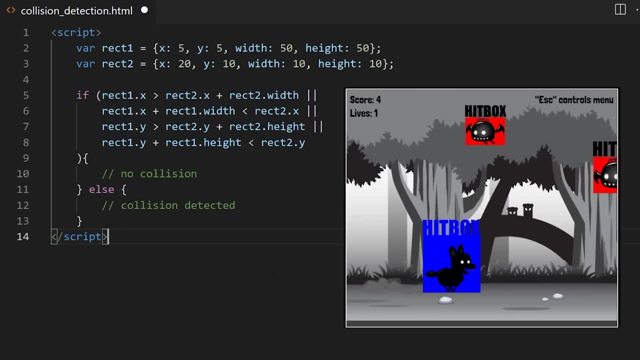 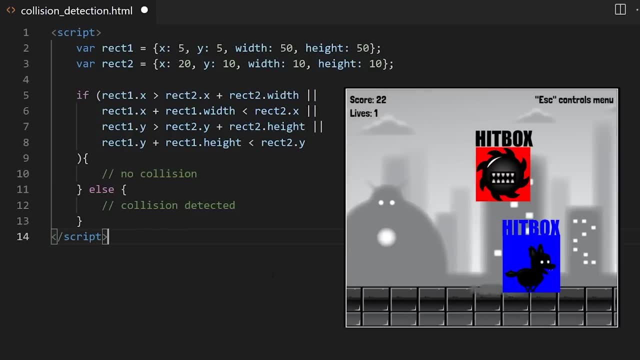 these particular algorithms in an actual project and where exactly to place them in your codebase. I use them in many of my games, such as in Tower Defense, Frogger, Flappy Bird and many more. I will link some in the video description. 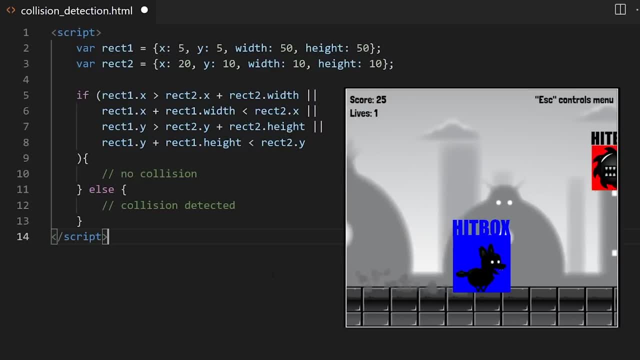 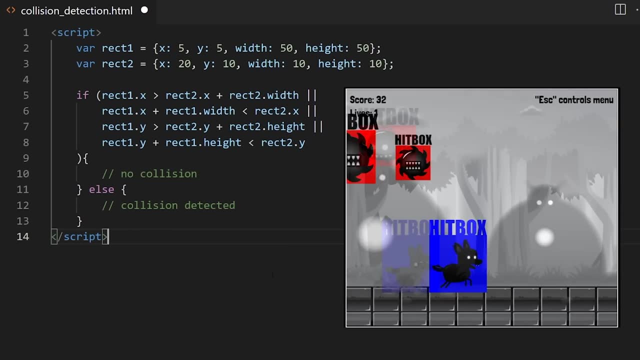 If you want to learn more with me, check out some videos on my Vanilla JavaScript game development playlist. I also do web animations, generative art for beginners and more. Everything with Vanilla JavaScript, using no frameworks and no libraries. Hope you have fun and show me some of your creative coding projects, please. 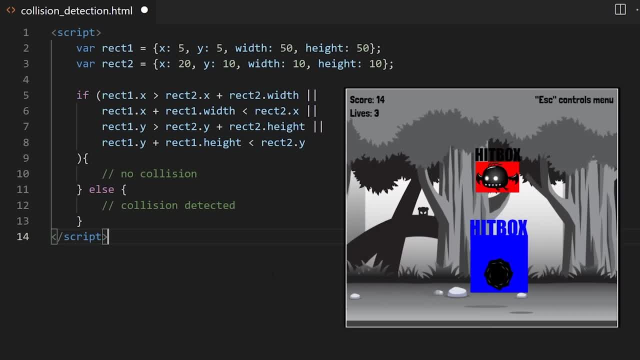 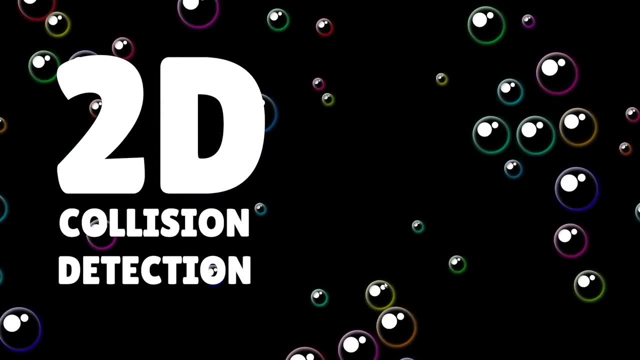 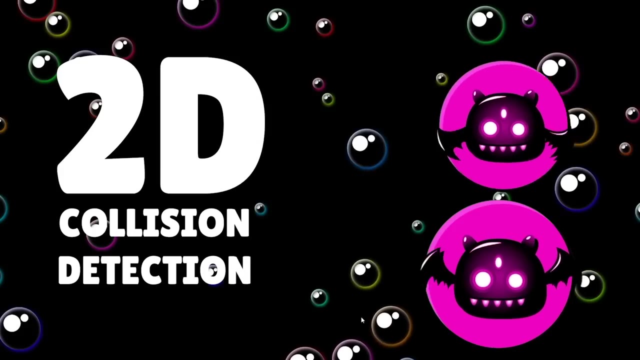 You can message me on Twitter if you want. Let's be friends. Collision detection is important if you want to build particle systems where elements interact with each other, Or when you are building JavaScript games and you want to detect when two objects collide, Or maybe when you want your canvas animations. 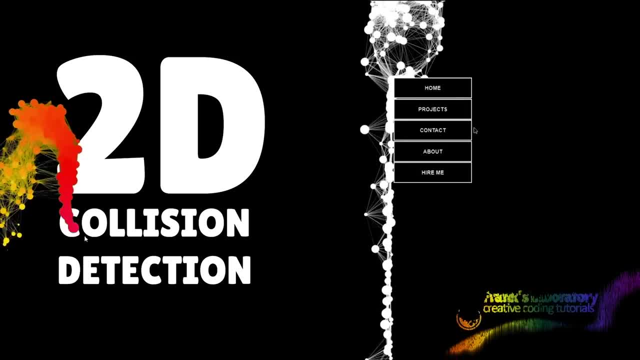 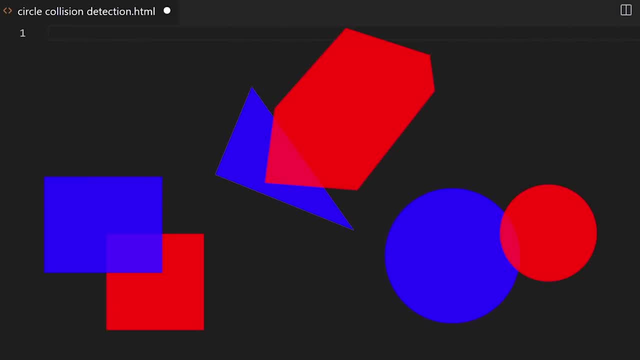 to interact with regular website elements. Three of the most common techniques we use for games and creative coding are collision detection between circles, rectangles and polygons. There are also other potential scenarios, and some clever people came up with interesting ways how to detect them with code. 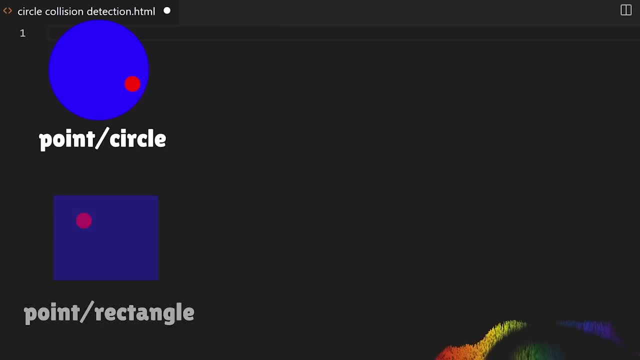 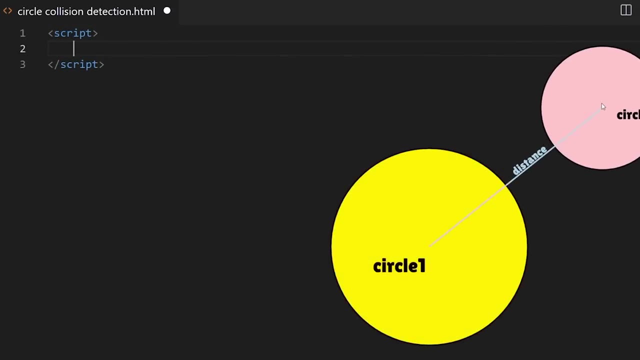 Some are easier than others. One of the most useful ones is collision detection between two circles. You can detect if two circles collide with JavaScript very easily. The algorithm just takes two center points of our circles and checks if the distance between them is less than the radii. 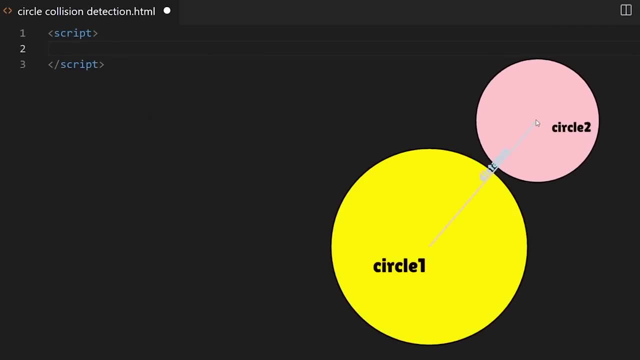 of these two circles added together. What does that look like in code? Let me quickly show you. Let's say we have two JavaScript objects, circle1 and circle2.. They have some coordinates, so position on horizontal x-axis and position on vertical y-axis. 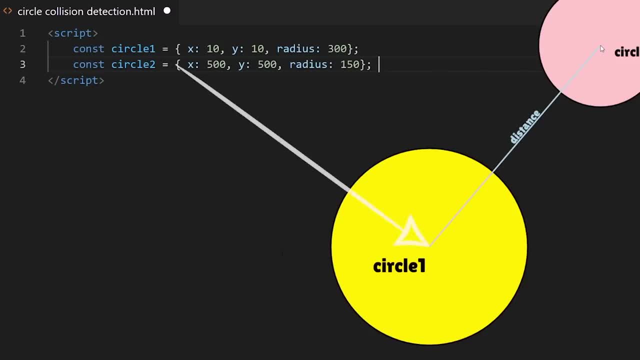 and some radius. I connect their center points with a line. This line represents distance between center points of these two circles. I connect position of circle2 to my current mouse position so we can move it around If the distance between these two center points. 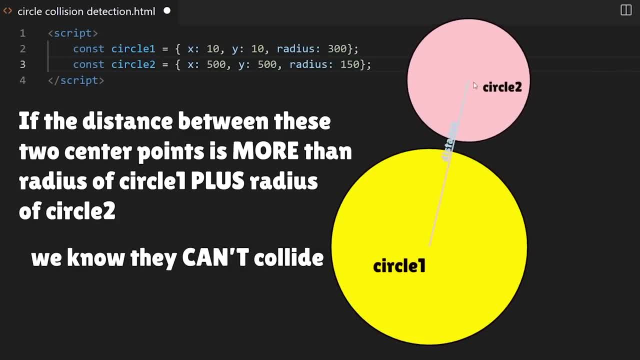 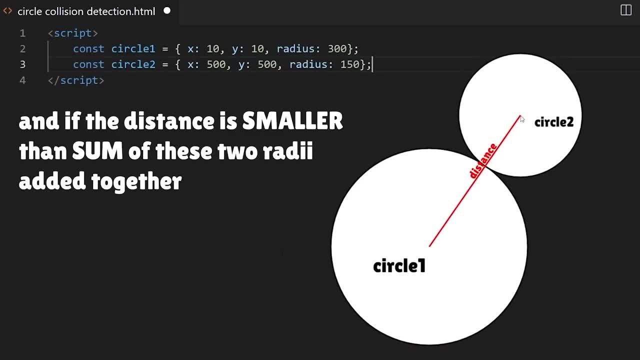 is more than radius of circle1, we know they can't collide. If the distance is the same, we know they touch. And if the distance is smaller than sum of these two radii added together, we know the circles overlap To be able to measure distance. 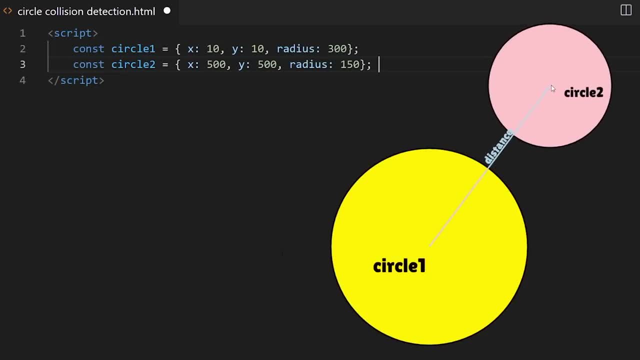 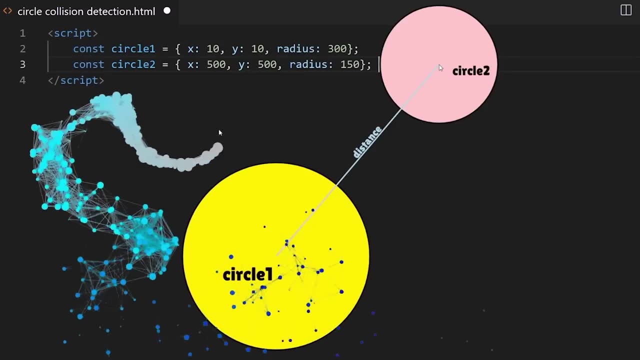 between two points with JavaScript, in this case center point of circle1 and center point of circle2. we will use simple and very powerful algorithm. Once you learn this and get comfortable with it, you will unlock next level in your coding and animation projects To measure the distance between these two points. 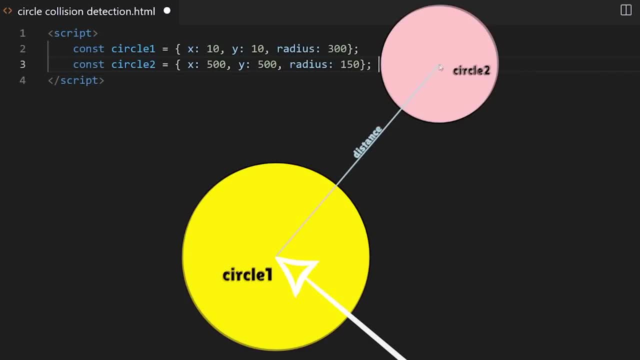 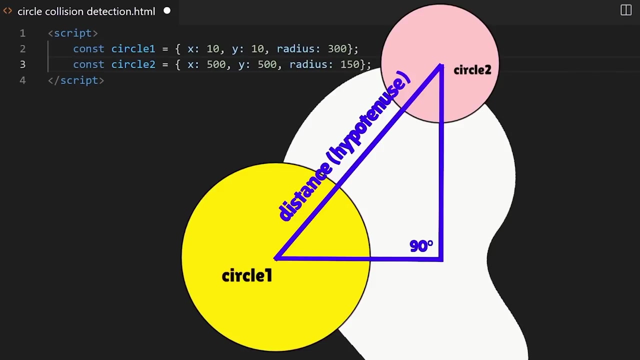 we need to know length of this line. We calculate it by imagining there is a right angle triangle in between, like this: In this triangle our distance is actually hypotenuse- the longest side of a right triangle opposite to the right angle. This is the right angle: 90 degrees. 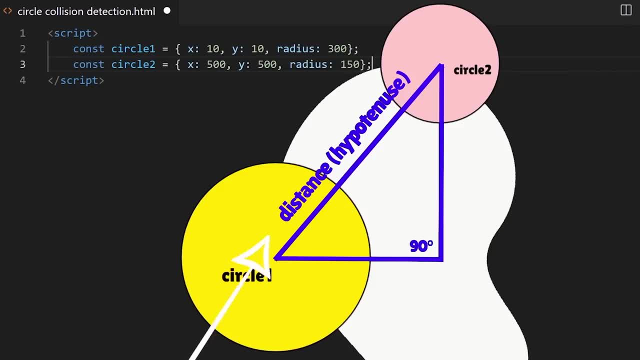 We know x and y position of center point of circle1, and we also know x and y position of center point of circle2.. With that we can calculate length of both arms of the right triangle. This side is simply just the difference between horizontal x position. 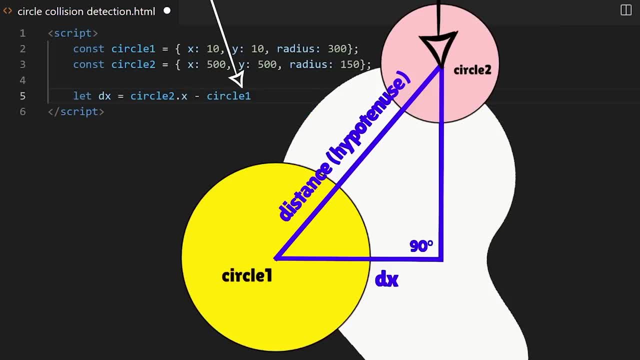 of center point of circle2 minus horizontal x position of center point of circle1.. We can do the same thing to calculate this side: Vertical position of this center point minus vertical position of this center point. Now we have this imaginary right triangle between our two points. 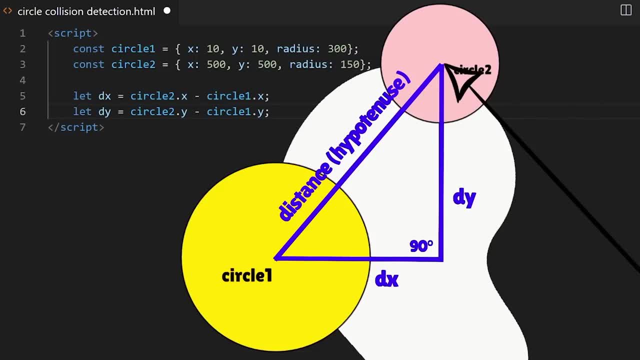 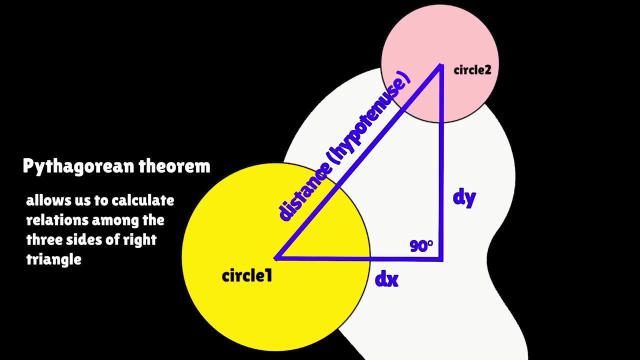 We know this side and we know this is right angle: 90 degrees. Now we want to know how long is this side hypotenuse of our triangle opposite to the right angle? We can achieve that easily with Pythagorean theorem. It allows us to calculate relations. 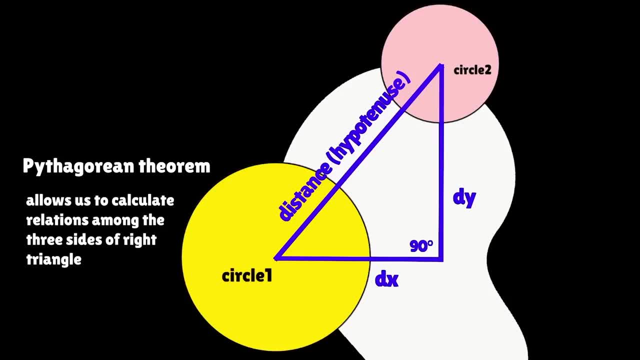 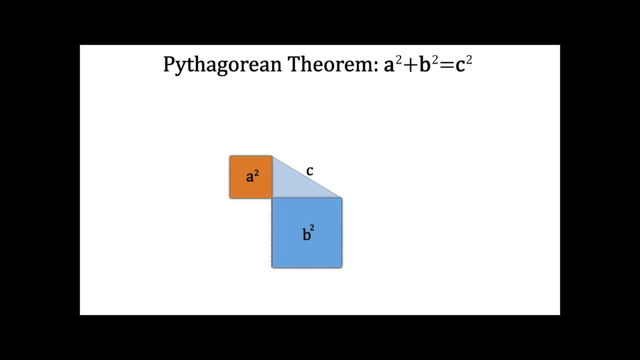 among the three sides of a right triangle. Imagine we draw squares on top of each line like this: Pythagorean theorem tells us that the sum of the areas of the two squares around the right angle equals to the area of the square on the hypotenuse. 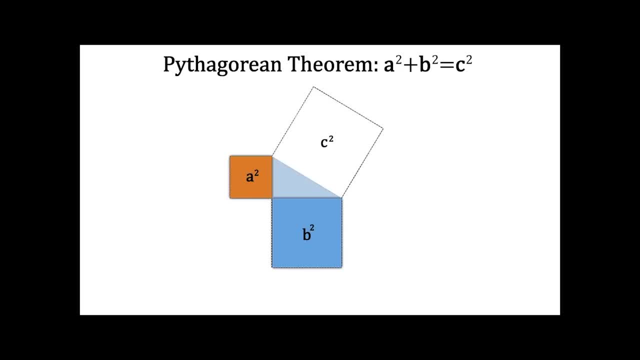 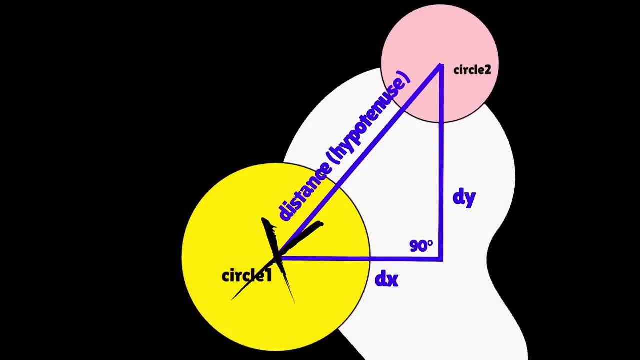 c squared is equal to a squared plus b squared. That means c is square root of a squared plus b squared. If you want to know why this is true, check out Radu's video. I will link it in the video description. So distance between center point of circle1. 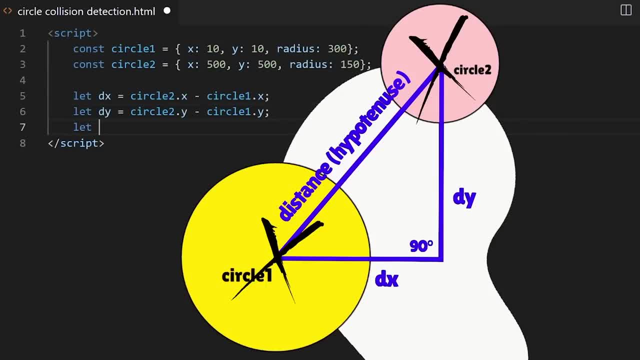 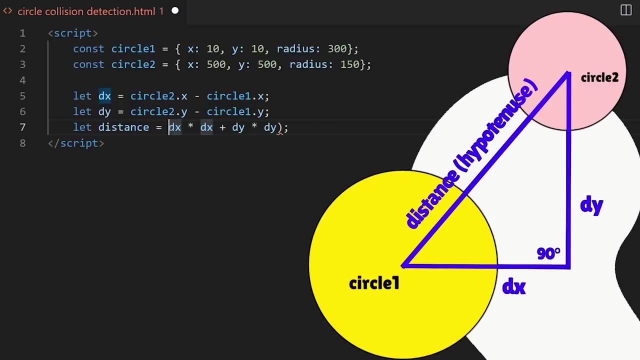 and center point of circle2: dx times dx, which is side a squared, plus dy times dy, side b squared. This would give us squared value and I want square root, so I wrap it in mathsquare root like this: Now we calculated hypotenuse of the right angle triangle. 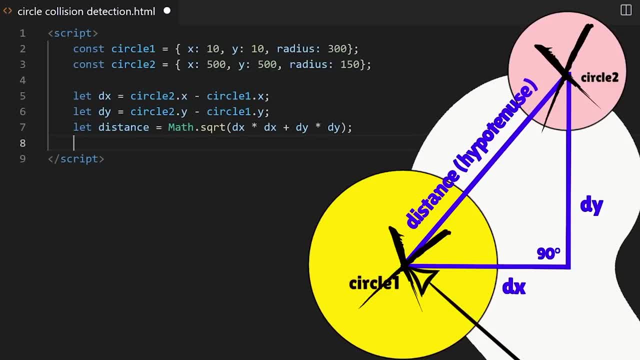 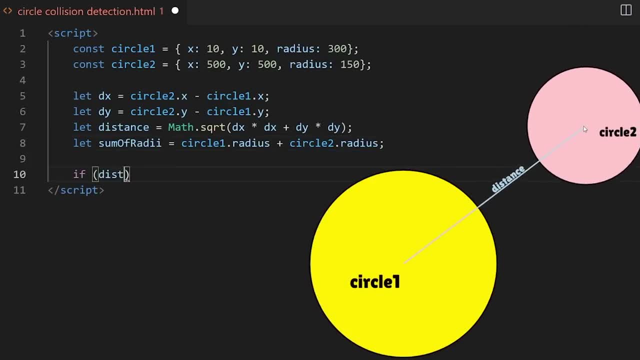 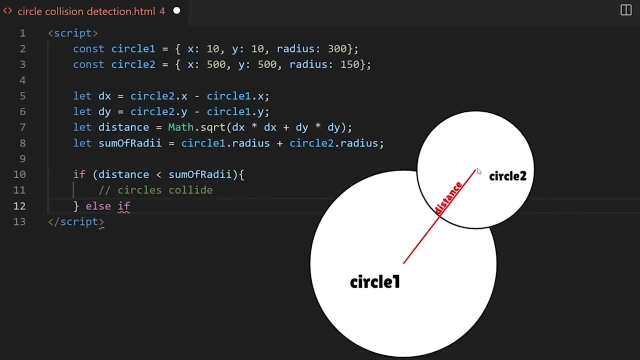 which is the distance between center points of circle1 and circle2, and we have a collision If the distance is less than radius of circle1 plus radius of circle2. we have collision If the distance is exactly the same number as the sum of radius of circle1. 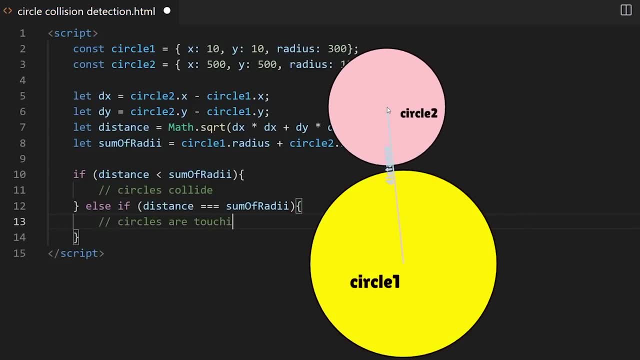 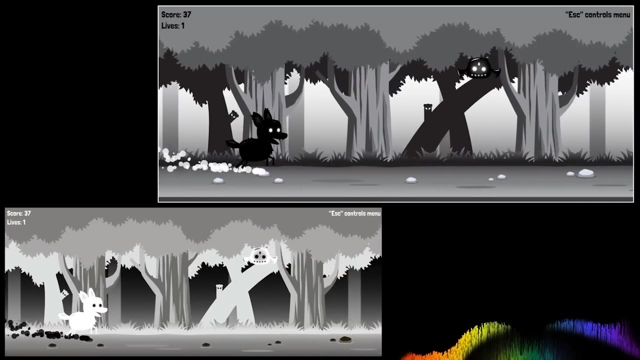 plus radius of circle2. we know they touch If the distance is more. we know there is some space between the circles and they don't collide. Visual and audio feedback that reacts to player actions and in-game events is really important if you want your javascript games to feel good. 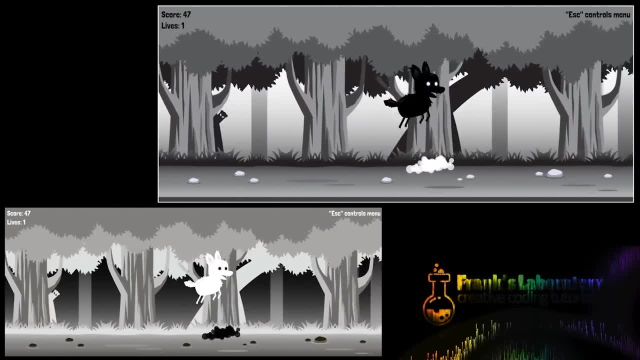 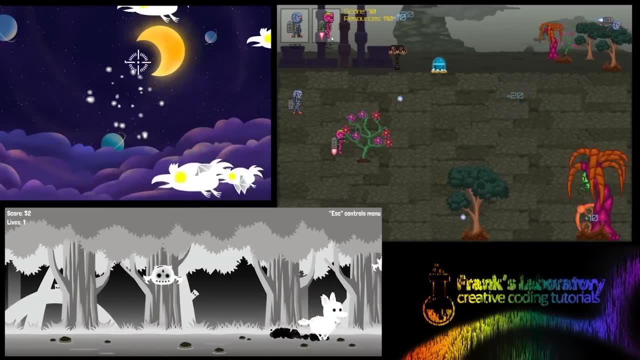 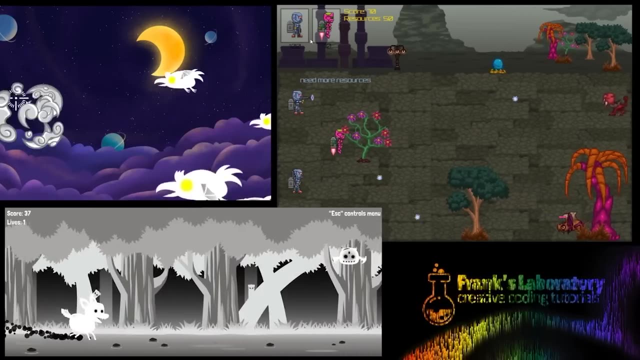 You can, for example, attach sound and explosion animation whenever collision happens in your game. You can also use this technique to make score points float from defeated enemies or from collected items. Today we will build an easy, fun project together that combines javascript, audio and sprite animation. 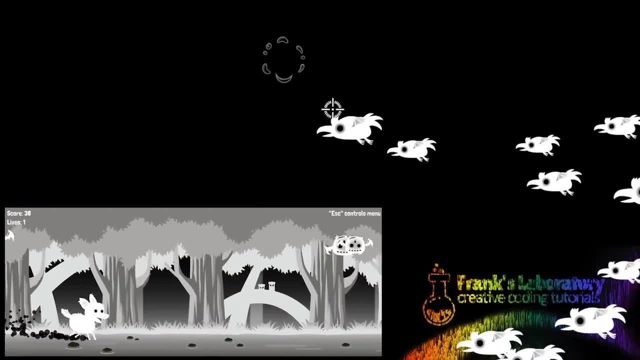 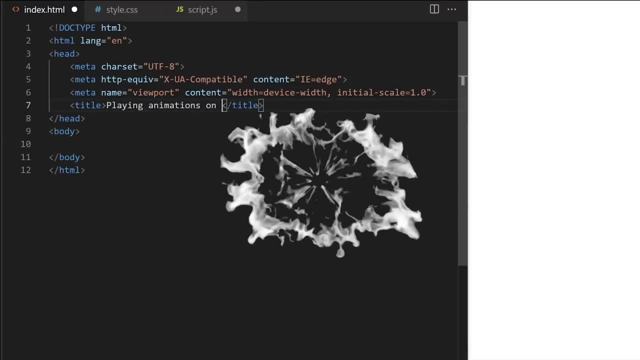 To create triggered event based animations. we will build a game that will look something like this. to really put all these principles in action, I create a regular web page markup In document head. I link my CSS style sheet. I create HTML5 canvas element with an ID of canvas1. 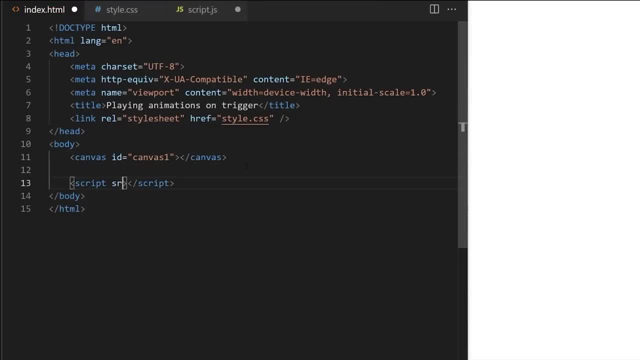 we will draw on it with code. I also link my javascript file down here at the bottom just before the closing body tag. All I need to do in style CSS is to position my canvas element. so I target it with ID. I give it border: 3px, solid black. 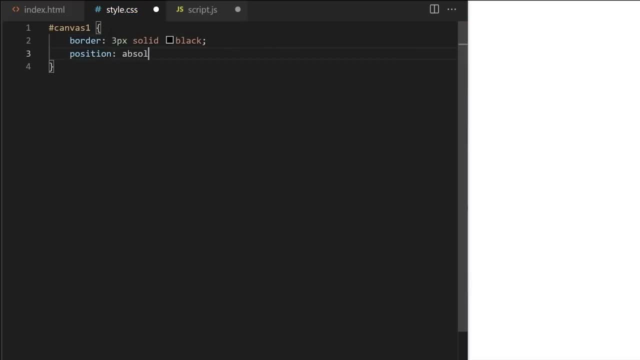 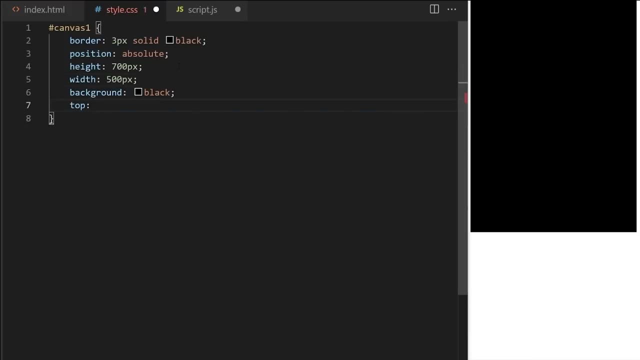 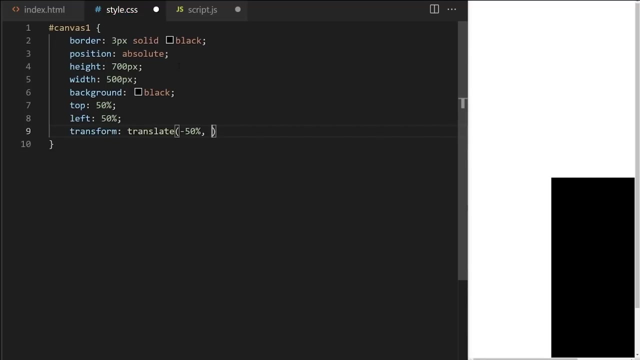 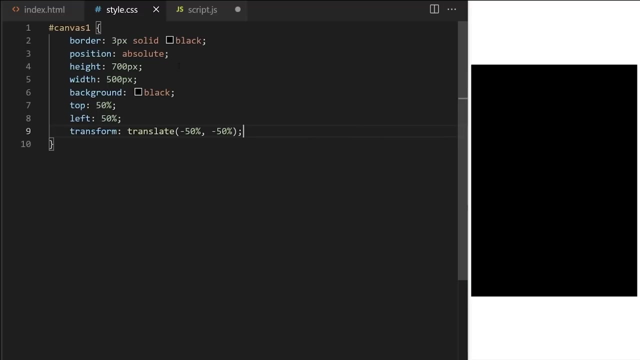 position: absolute height: 700px. width, 500px, background: black. let's center it so: top 50%, left 50% and transform translate: minus 50% minus 50%. this trick will only center elements that have position set to absolute with plain vanilla javascript. 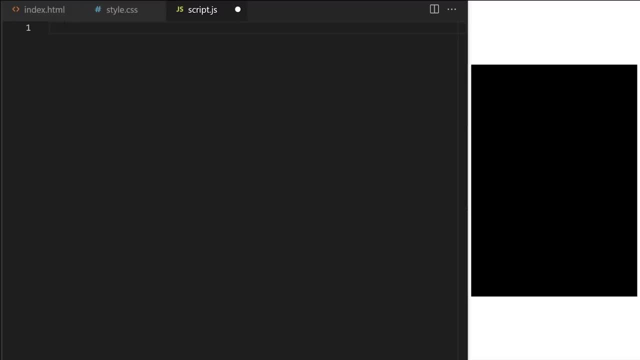 here in scriptjs file I need to point javascript towards my canvas element. so custom variable called for example, canvas, is equal to documentgetElementById. canvas1 CTX shortcut for context is equal to canvasgetContext2D. this will instantiate object that holds all 2D drawing methods. 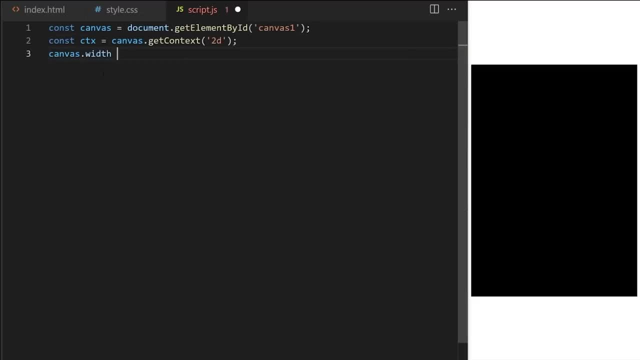 we will need today. canvas width is 500. canvas height is 700. let's test if we set it up correctly by drawing a quick, simple shape. it's good to test. your code as you go makes it easier to debug. I set global canvas fill style to white. 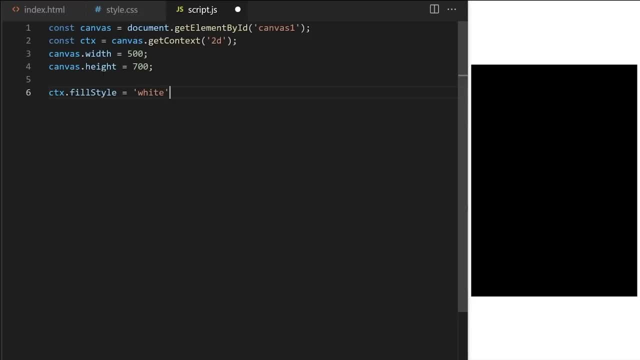 this will apply to fill of all shapes now, unless I redeclare it again and give it a different color. I call built in fill rectangle method. I pass it. coordinates 50, 50, width, 100px and height 150px. perfect, we set it up correctly. 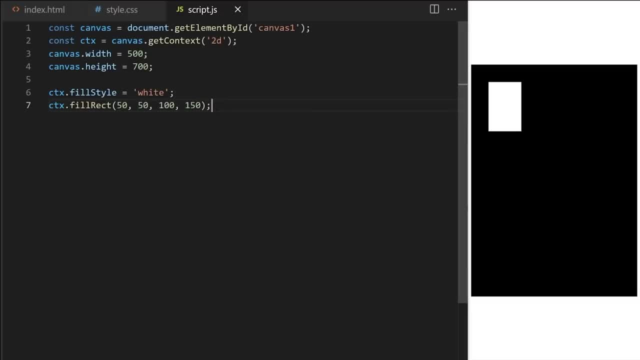 and we are drawing on canvas now for fun. I delete the rectangle and I create a variable called, for example, explosions. I set it equal to an empty array. its job will be to hold all active explosion objects I create. I create them using javascript class. I call it, for example, explosion. 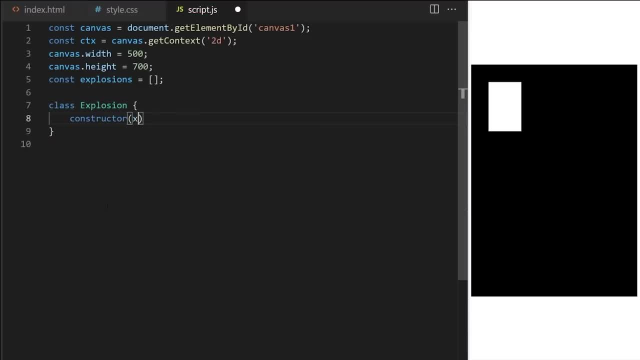 with a capital E constructor will expect x and y coordinates coming from the outside. this is important because we want the animation to be triggered at a specific location where the event happens. I want it to animate at coordinates where two elements collided or at coordinates of mouse click. 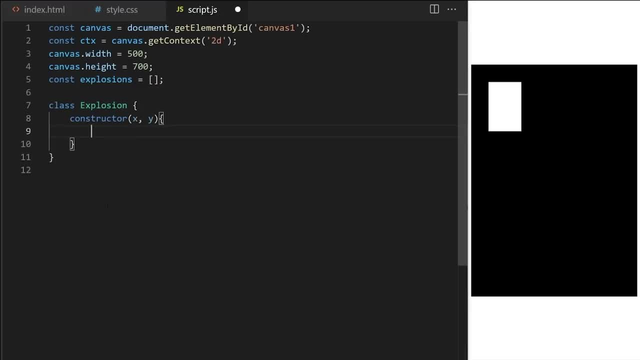 I will pass these x and y coordinates to the constructor whenever I want to trigger new animation and create new object using this class. it's very simple. I will show you in a minute so on, this new explosion object, give it thisx property and assign it to x. that was passed. 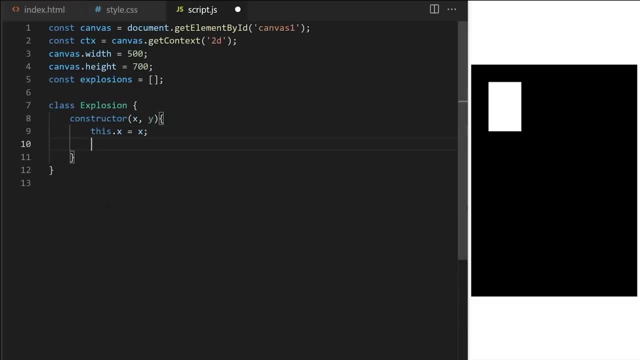 as an argument on line 8 from the outside. do the same for thisy vertical y coordinate. this will be the width of a single frame in my sprite sheet. I calculated by taking width of my sprite sheet and I divided by the number of frames. in this case, my sprite sheet is 1000 pixels wide. 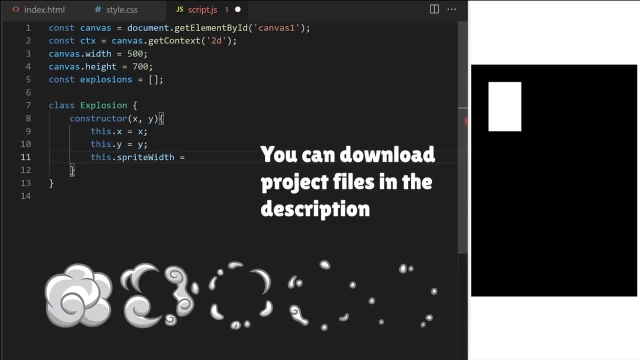 and has 5 frames. 1000 divided by 5 is 200. height of my sprite is 179 pixels. sometimes you get sprite sheets that are too large or too small, so you might want to scale it while still keeping the aspect ratio relationship between width and height. 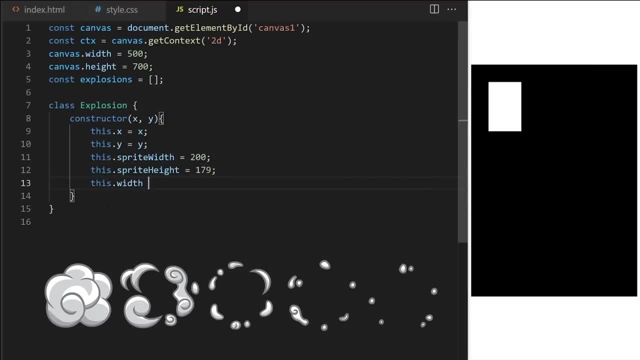 so it's not stretched or squished. I declare thiswidth property and I set it equal to thisspriteWidth from line 11 divided by 2. thisheight will be thisspriteHeight divided by 2. it's important to divide or multiply them by the same number to keep the same aspect ratio. 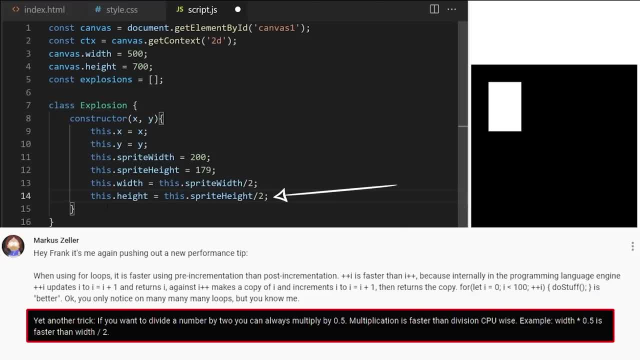 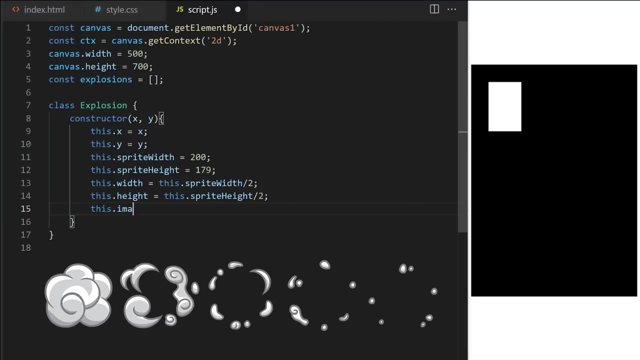 by the way, for optimization it's always better to multiply than to divide. division operation in javascript is more performance expensive, so instead of dividing them by 2, I will bring my sprite sheet into the project. you could declare it as a global variable, but I think it's a bit cleaner. 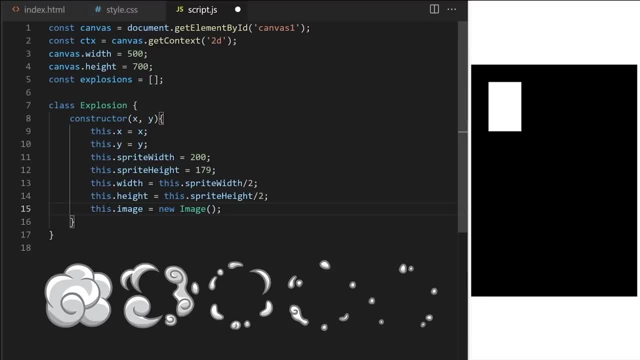 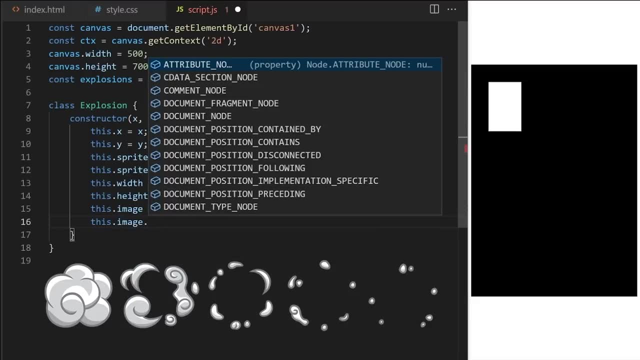 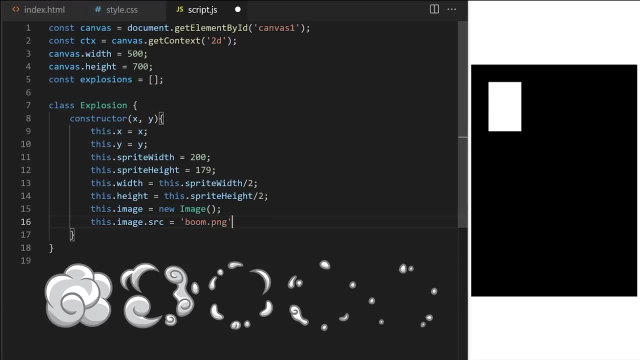 to put it as a property on class like this: thisimage equals new image. this is just image class constructor and it will create new blank html image element. thisimage src will give it source attribute and I set it to boompng if you want to use the same file. 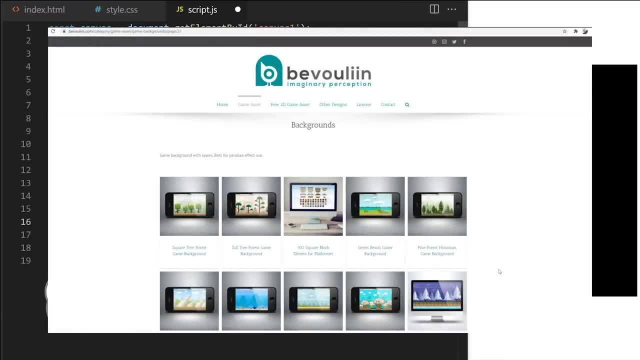 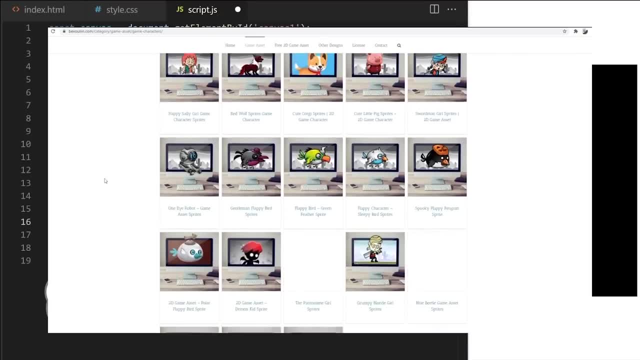 you can download it in the video description. this image was kindly provided by one of my favorite game artists. I will link his website in the video description. he has a lot of cool game art there. if you are interested to animate this sprite sheet, I will crop out one frame. 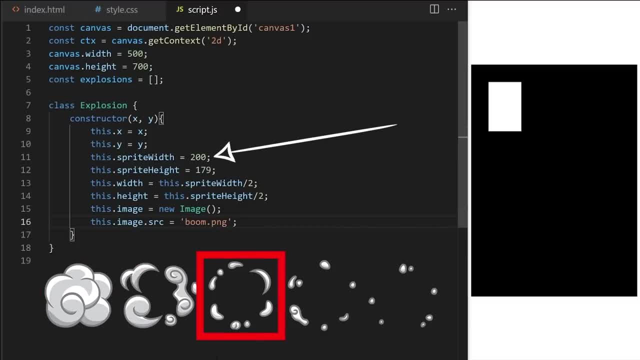 and I will be jumping to the right by the amount of sprite width, frame by frame. to do that, I will need thisframe variable. I will set it to 0 at first. we will also need to add some behavior to this class. we do it by creating class methods. 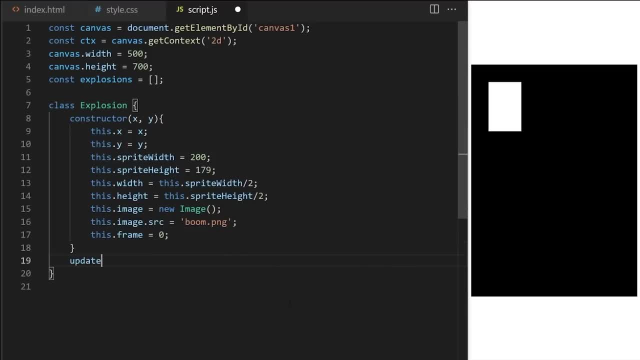 I will need one to update and one to draw my explosions. we will only have one job for now: to increase thisframe from line 17 by one for every animation loop. thisframe plus plus draw method will take values from the constructor and it will draw current frame of animation. 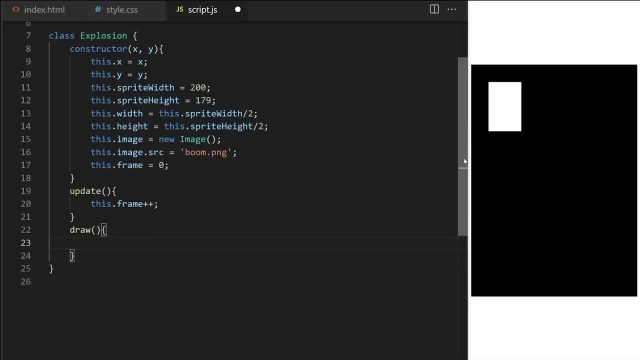 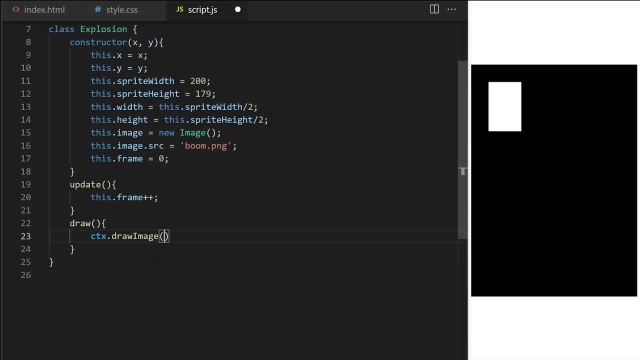 on canvas. we will use built in html canvas draw image method that takes image we passed to it and it draws it. draw image method has 3 versions with 3 or 5 or 9 arguments, depending on how much control you want over the image you are drawing. 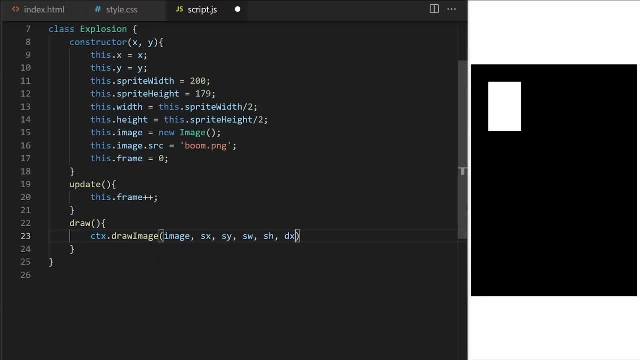 since we are animating a sprite sheet, we will only use the longest version with 9 arguments. the arguments we need to pass to it is image: we want to draw source x, source y, source width and source height of area you want to crop out. 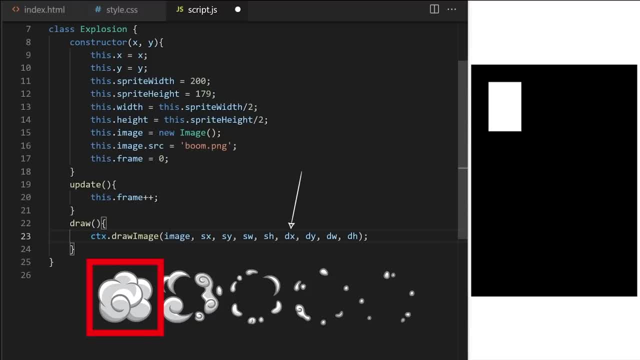 from the source sprite sheet and destination x, destination y, destination width and destination height. these last 4 arguments will determine where on destination canvas you want to place that cropped out image onto. it might sound complicated if you used it couple of times when you learn how to use draw image method. 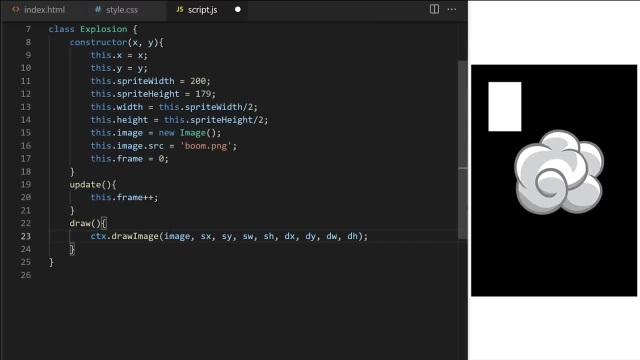 and you get really comfortable with it, you will have complete control over sprite sheets you want to animate. it's really good and so useful. so now i will replace these placeholder values with actual variables we prepared inside constructor. image we want to draw is thisimage from line 15. 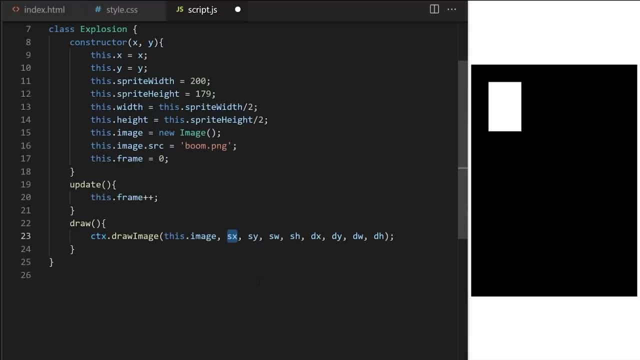 source x is the only one from these 9 arguments that might be a bit more complicated for beginners to calculate current horizontal position. so i will multiply sprite width from line 11 and i multiply it times thisframe from line 17. as the program runs, thisframe increases inside update method. 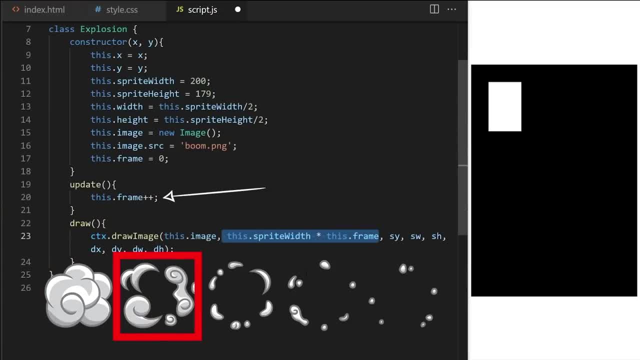 on line 20 we will get frame 0,, 1,, 2,, 3, 4 because we are multiplying sprite width times, frame source y is horizontal y coordinate we want to crop out from the source, since this sprite sheet has only one row. 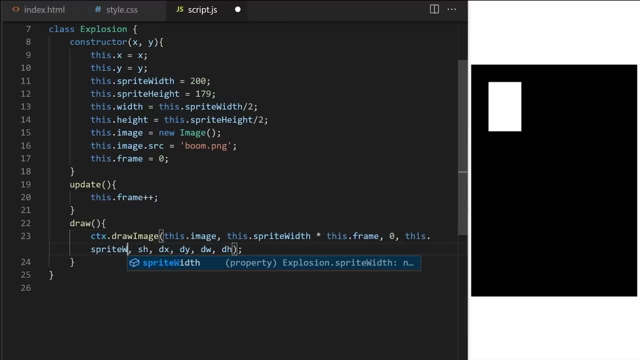 source y will always be 0, source width is thissprite width and source height is thissprite height from line 12. so now we told javascript what sprite sheet we want to draw and what area we want to crop out from it, to display just one frame. 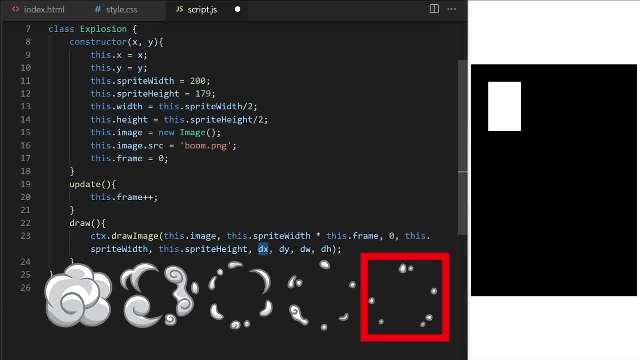 now i just simply tell it where on canvas i want to draw it. destination x is thisx from line 9. destination y is thisy from line 10. destination width and height is thiswidth and thisheight from lines 13 and 14. our class is complete. 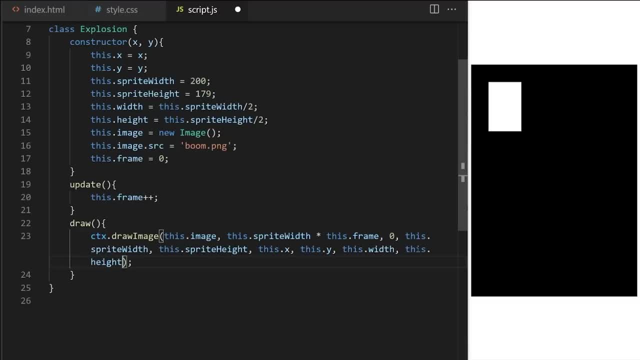 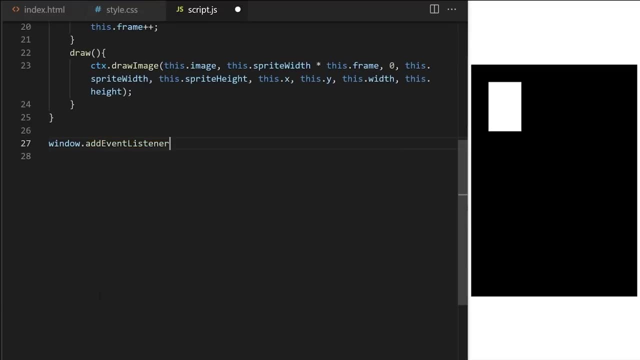 this is all we need to trigger this dust cloud animation and attach it to any event we want to. there are many events we can do here. let's try one. i call windowaddEventListener. built in javascript method, we will be listening for mouse click event and in callback function that will run. 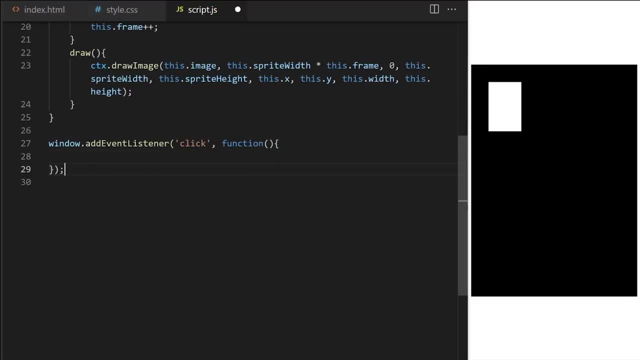 every time click event occurs, i will at first just draw a simple rectangle to make sure everything works. fill rectangle expects 4 arguments: x, y, width and height. i want this rectangle to be drawn at the current coordinates of my mouse click. to do that is easy. 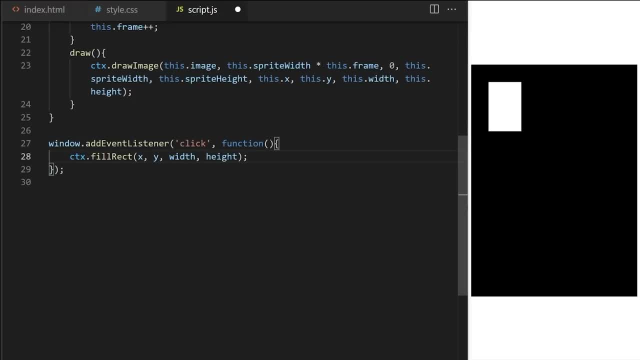 callback function on event listener has access to built in event objects. usually we name it e or event like this, but you can name it anything you want. javascript knows that this argument passed to callback function on event listener refers to event object. you can put abc here and it will still work. 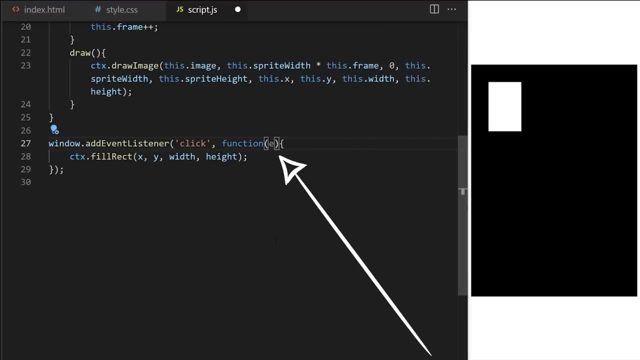 as long as you refer to it as abc later in the code as well. take event object with information about this, click event and save it in a custom variable. i call e. if i console log this e, i will get an error. let's comment out line 29. 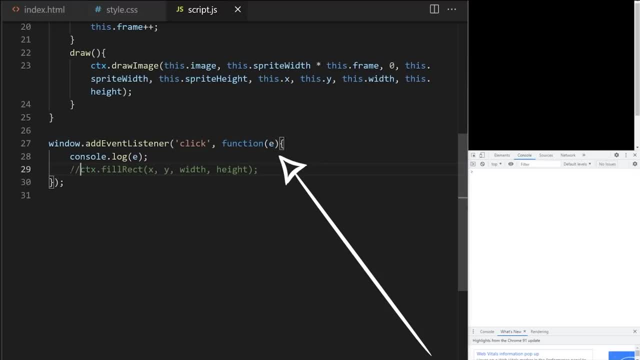 for a second now. whenever i click on canvas i get this console log that contains all information about current click event that just occurred. if i open it i can see we have all kinds of details here. all we want is where on canvas this event happened so we can draw our rectangle at these coordinates. 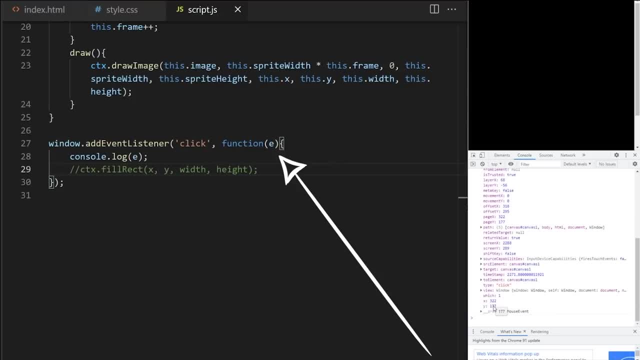 x and y coordinates are down here as properties called x and y. now that i know the name of properties i'm looking for, i can use these values inside fill rectangle method. i want to draw it at x coordinate of current mouse click. i know that value is stored on my event object. 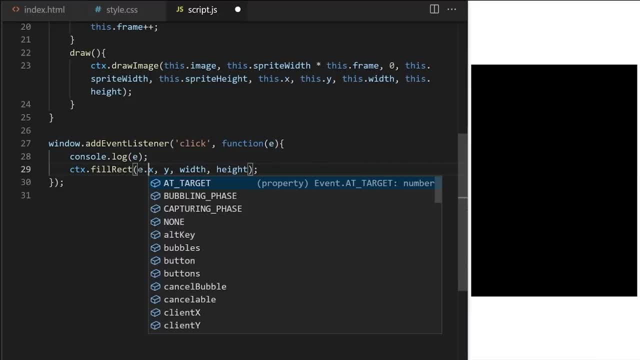 in a property called x, as we just saw. so i put ex here and ey. width and height can be anything i want. i want my rectangle to be, for example, 50x50 pixels. i can't see anything when i click. that is because i used black background. 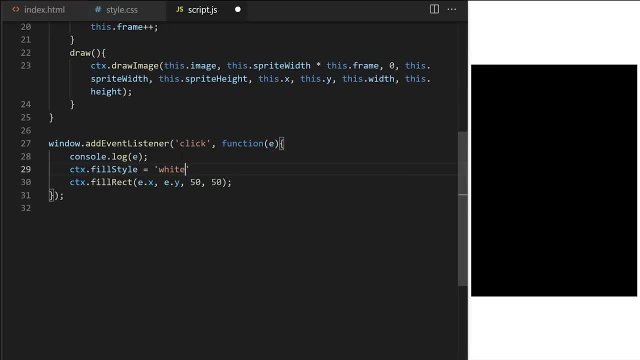 and default fill is also black. i set fill style to white color. when i click, you can see that we draw a white rectangle on canvas, but it's not being drawn under mouse. why is that? in this case, eventx gives me value that doesn't account for this top and left margin. 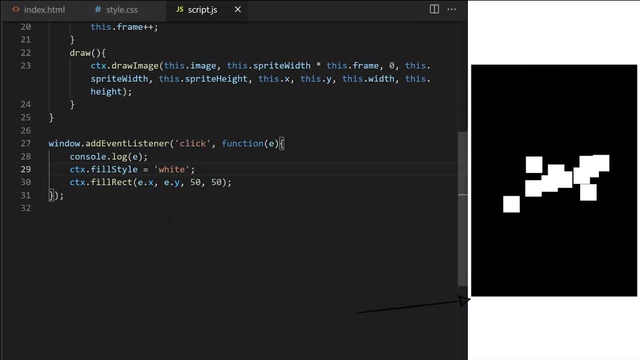 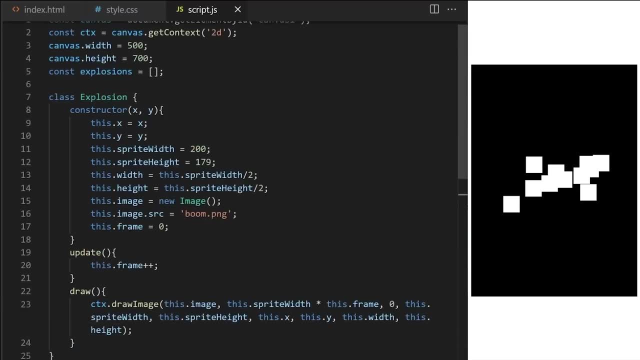 between start of my web page and start of canvas. what i need to do is offset my coordinates to account for it. good way to do that is to measure canvas position first. you can do this with one line of code. i create a custom variable called for example. 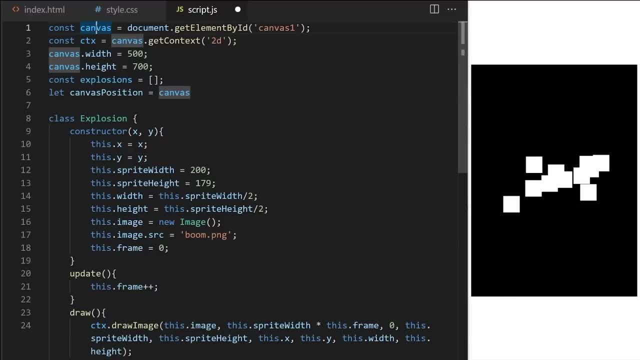 canvas position and i set it equal to canvas from line 1 and i call get bounding line rectangle built in method on it. get bounding line rectangle is a very useful built in javascript method. it returns an object providing information about the size of an element and its position relative to the viewport. 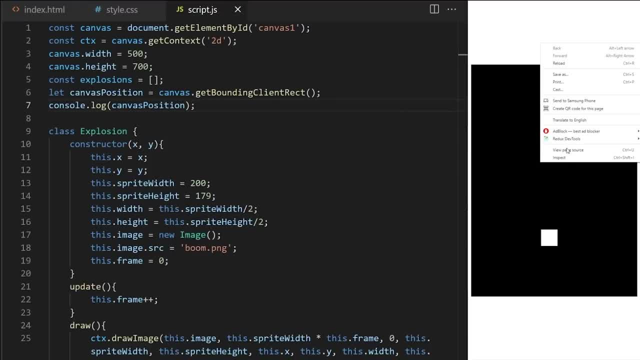 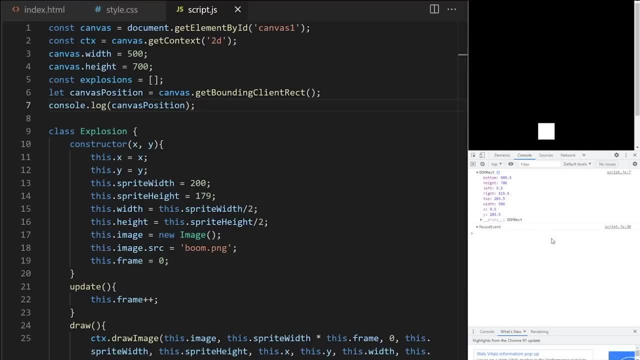 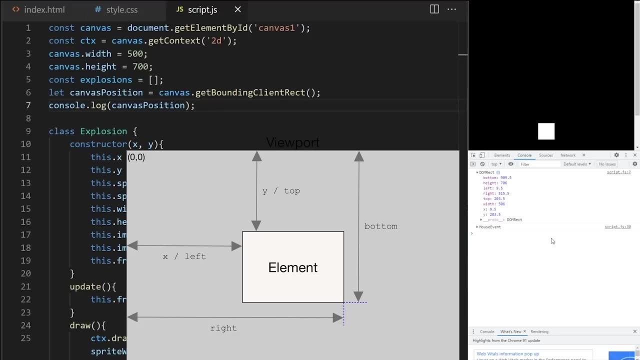 i can console log my canvas position variable now and you can see the object here. it contains bottom, left, right and top position on the graphics. here you can see exactly what these values represent. it also contains information about its width and height and its x and y position. 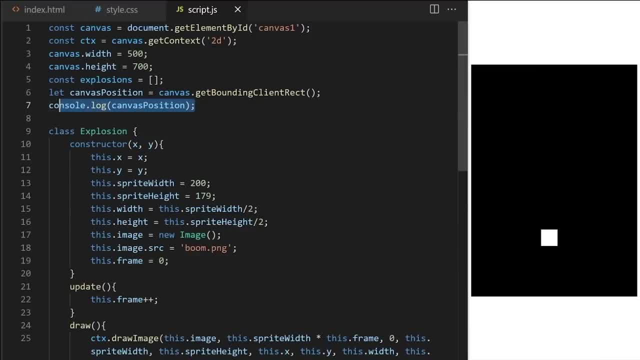 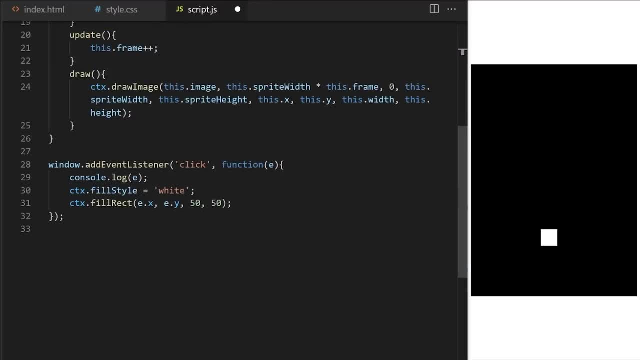 you can use this to measure any HTML element on your page. if you are offsetting something, it's really useful. i delete console log on line 7. i like to clean up after myself as i go, so if i want my white rectangle to be drawn under the current mouse position. 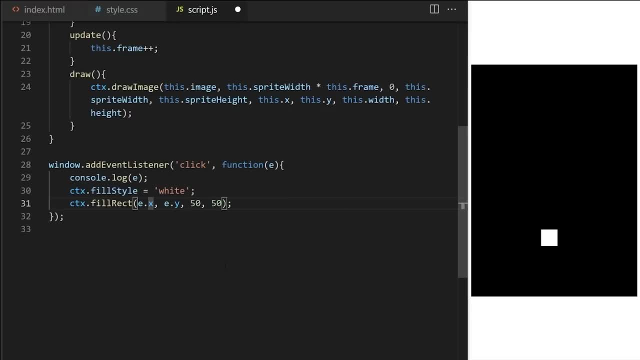 i need to offset ex and ey by top and left margin between viewport and canvas. horizontal x coordinate is ex minus canvas position, dot. left. now you can see that horizontal position is exactly under mouse. i also fix vertical position by saying ey minus canvas position top. 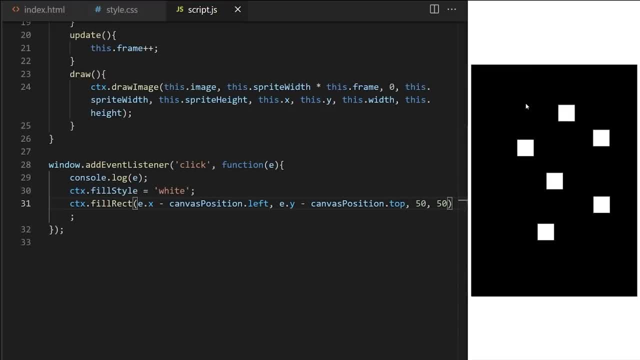 perfect. you can see that rectangle is being drawn towards the right bottom from my mouse cursor. this is how rectangles work on canvas: to be exactly in the middle of the rectangle, both vertically and horizontally. i need to do one more small tweak here. i offset my positions by half of width and height. 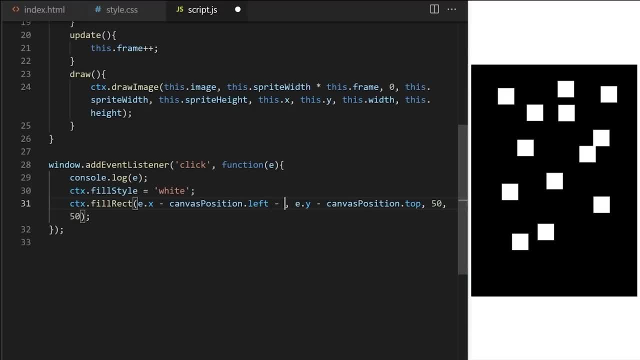 my width and height is 50, so i offset x and y by minus 25. now, when i click, mouse cursor is exactly in the middle of white rectangle when i place it on canvas. i know this might be very basic for some of you, but i want beginners to be able to follow along with us. 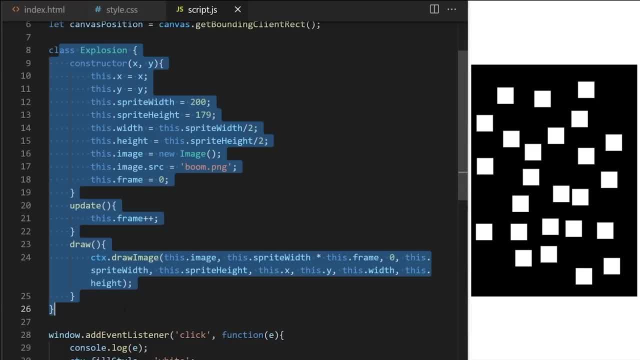 this course is for everyone. now that we understand how to draw a simple rectangle on click, let's take it to the next level and use our custom explosion class to create sprite animation every time we click somewhere on canvas. first thing i want to do is to take this calculation: 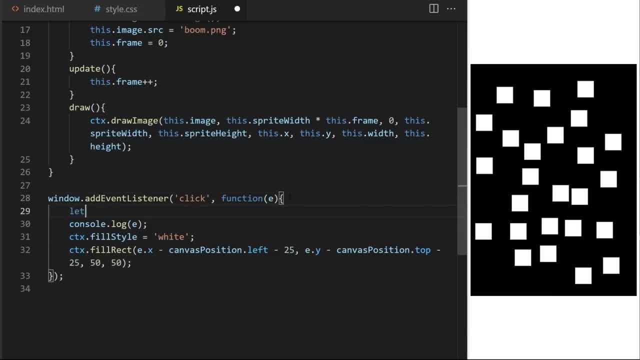 that offsets and centers my horizontal and vertical positions and i put them here in separate variables. this is just to keep my code clean and easy to read. i call them position x and position y and i just copy this formula in there. i can't really do minus 25 here. 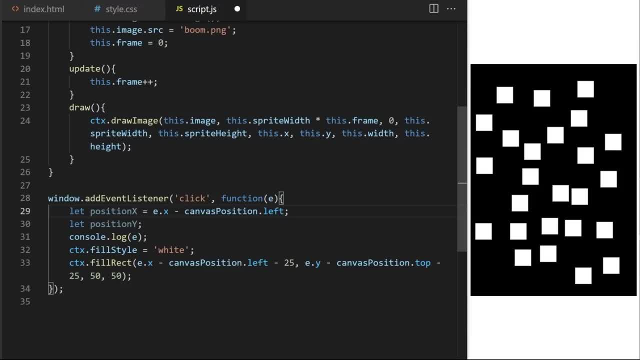 if i want to keep my code clean and keep my code base reusable, i need to offset it inside my explosion class. i will show you in a second. i do this. position y- vertical formula. i remove console log on line 31 and i also delete my white rectangle. 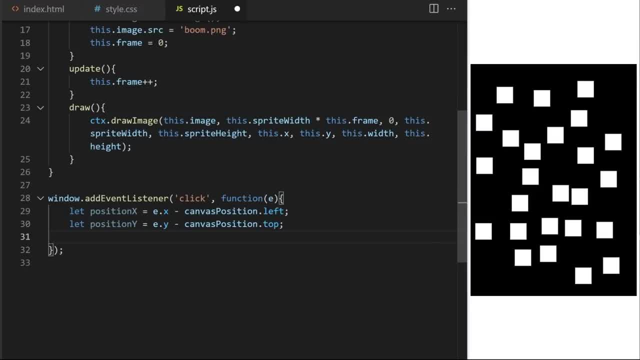 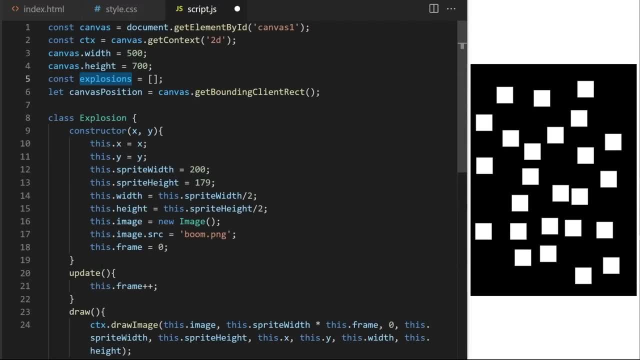 we will be drawing animated cartoon explosions. now on line 5 i have this array that will hold all my current active explosion objects. the goal is to use explosion class on line 8 and when we click we push new object into this array from line 5. 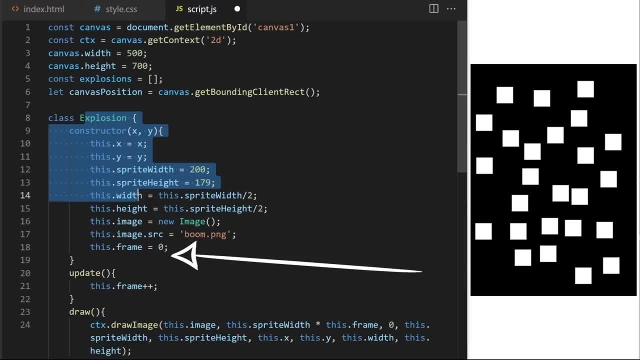 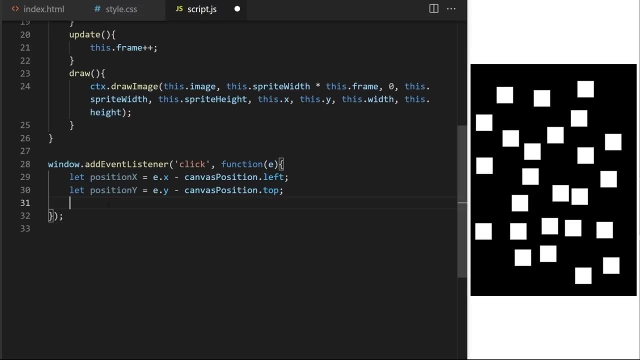 we cycle through all its frames using update method. on line 20, we draw each step to display the animation and then, when we reach the last frame, we remove the object from the array and we delete it. on line 31, inside click event: listener. i take this empty explosions array from line 5. 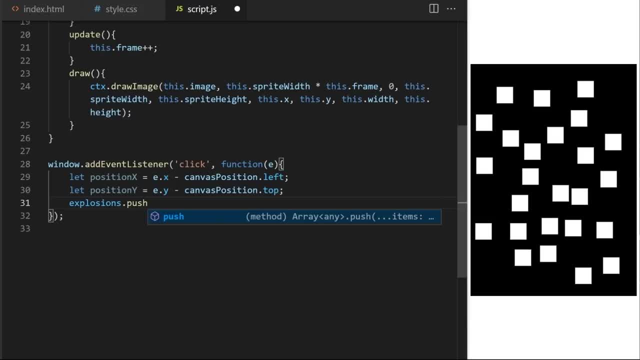 and i call push on it. push is a built in array method. it will take whatever we pass to it as an argument and it will push it at the end of the array. i pass it. new explosion. the new keyword will find my class on line 8. 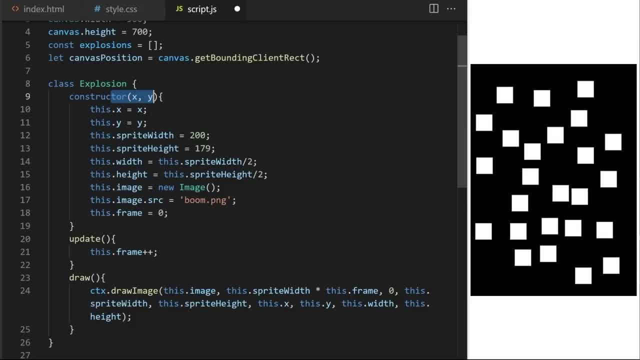 and it will run its constructor to create a new object based on this class's blueprint. on line 9 i can see my constructor expects two arguments for x and y coordinates. this is important because we need to know where on canvas we want to create this triggered animation. 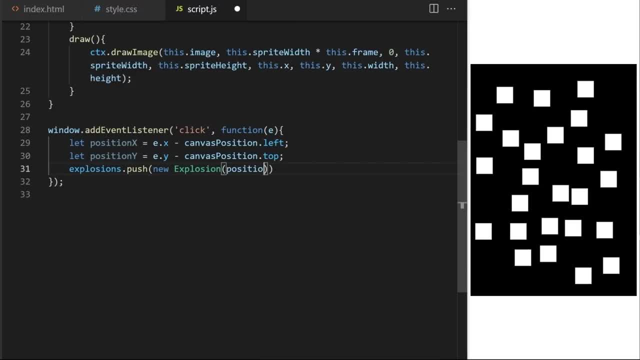 here on line 31. i just pass it. position x and position y variables we calculated on lines 29 and 30, so now i have a way to add new explosion object into my array on mouse click. i will need a function to cycle through all objects in the array. 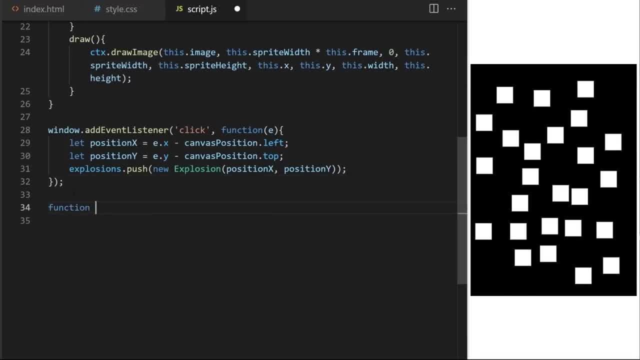 to update and draw them. let's create animation loop. i will write a custom function called animate. inside i create a for loop that will cycle through all elements in the array. sometimes, if we click really fast in sequence, we will have many objects animating at the same time. 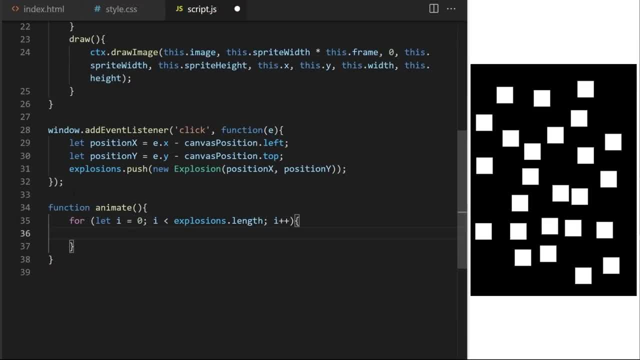 sometimes this array will be empty, it will have zero elements and this loop will be skipped. we will call its update method and also its draw method to create animation loop. i call built in request animation frame function and i pass it. animate the name of its parent function from line 34. 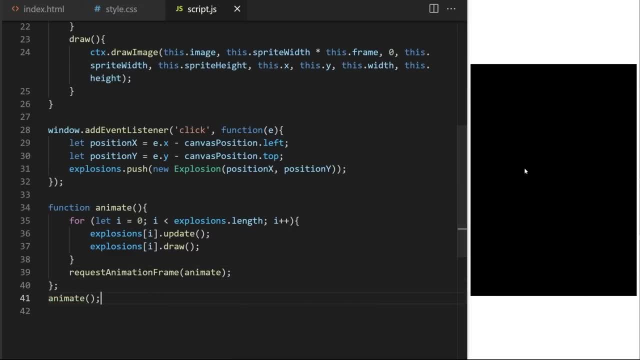 now i can call animate to kick off animation loop. awesome, this is working kinda. we can see old frames because we are not clear in canvas and i also need to center my animation around the cursor better to only see the current frame. i call built in clear rectangle. 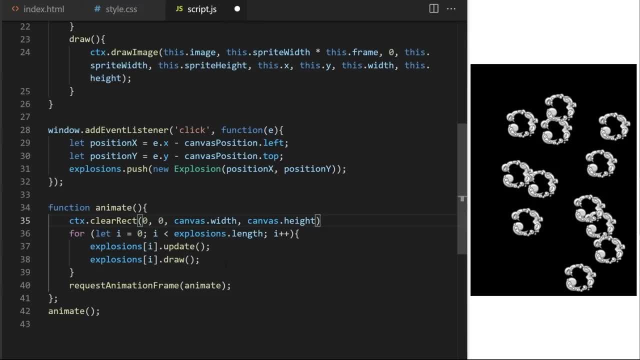 and i want to clear the entire canvas. if you look closely, you will notice we are skipping frame 0 because update method increases frame variable by 1. before we draw the first frame, i want each triggered animation to have its own timer. that way we can stagger the animation speed. 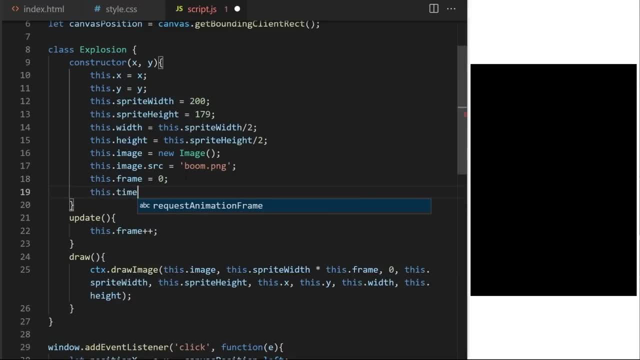 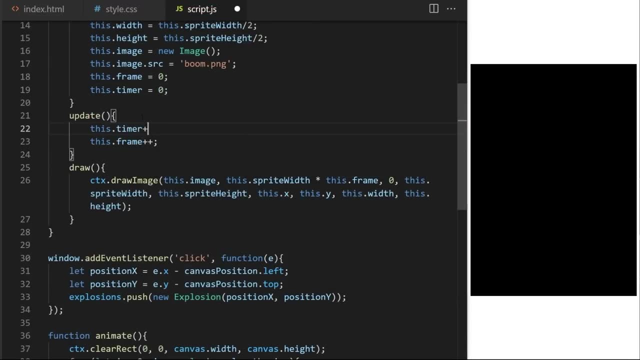 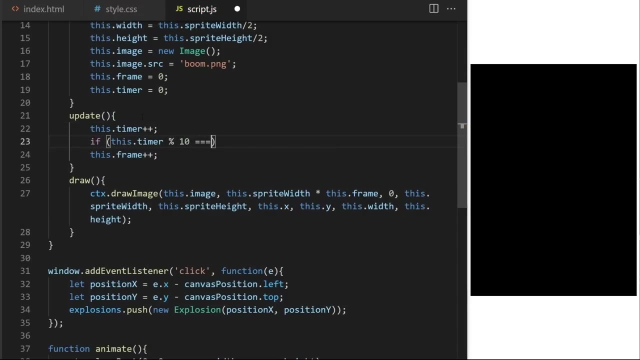 on line 19 i create thistimer property and i set it to 0. on line 22, inside animation loop, i set timer by 1 for each animation step. now i can say: if thistimer is divisible by 10 with a remainder of 0. 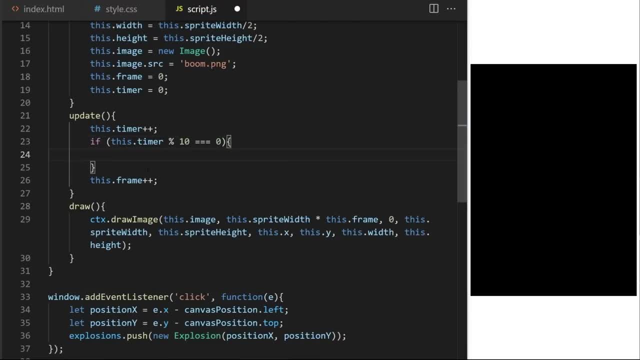 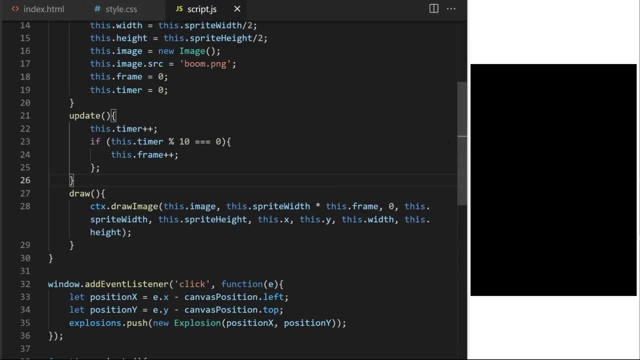 this simply means run this code every 10 frames only. when timer is divisible by 10, increase frame by 1. this will slow down the animation. timer has to increase 10 times before frame increases. once now we can see the initial first frame as well, and animation speed is 10 times slower. 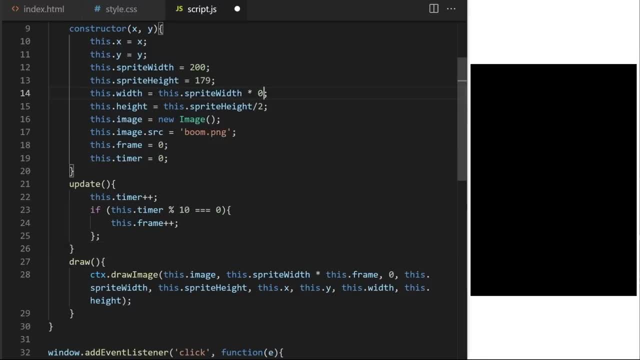 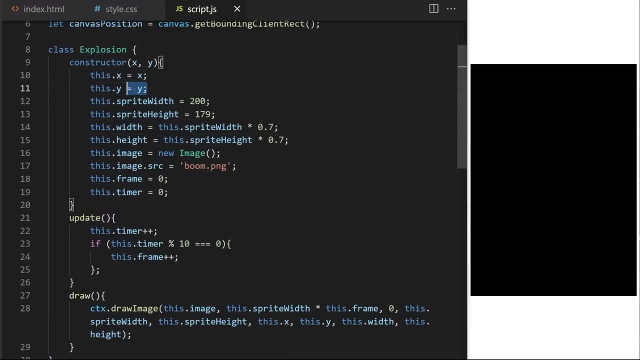 than before. let's make width and height slightly bigger. on lines 14 and 15 you can see that my animation is drawn too much down from mouse cursor, same as we did with white rectangle before. i want mouse cursor to be in the center of the animation. 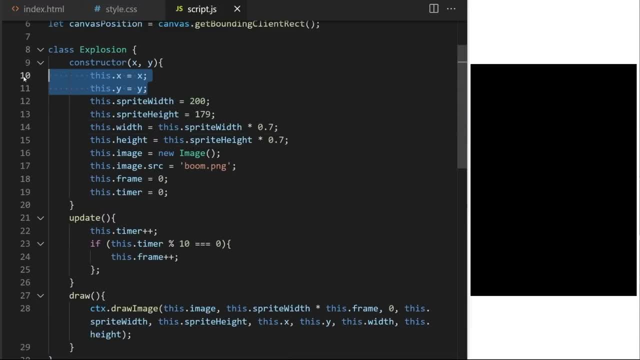 to do that, i can simply offset x and y by half of width and height. i can either do it here or i can also do it here inside draw image method. it would give us the same result. i can't offset x and y here, in my event, listener. 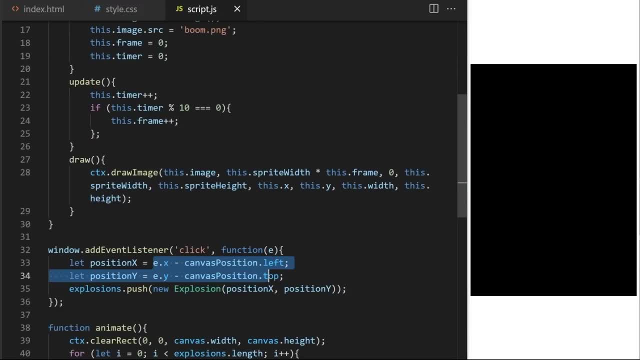 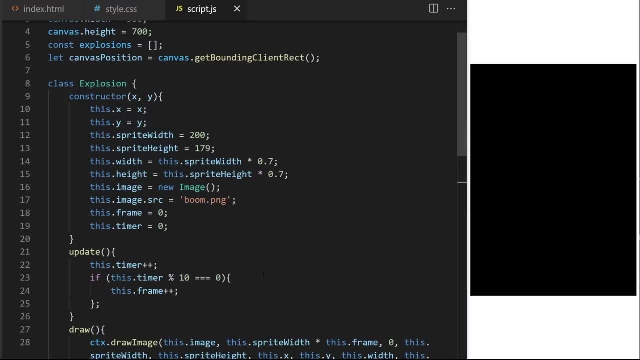 because at this point i don't know what width and height my animation is. i could hardcode some values here, but that would not be reusable. i think the cleanest way is to move thisx and thisy to go after width and height here so that they can see these properties. 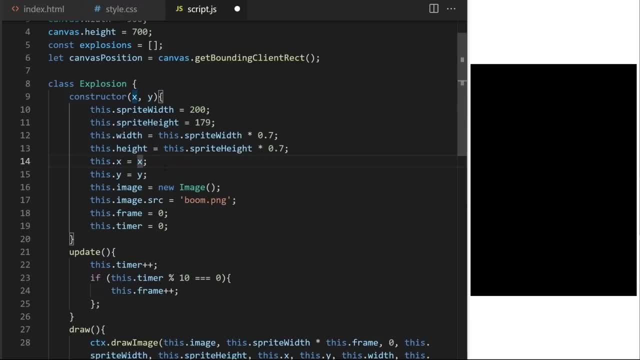 and i offset them here. thisx is equal to x, which was passed as an argument on line 9, minus thiswidth from line 12 divided by 2. this centered my animation around the cursor horizontally, and thisy is y minus thisheight divided by 2. 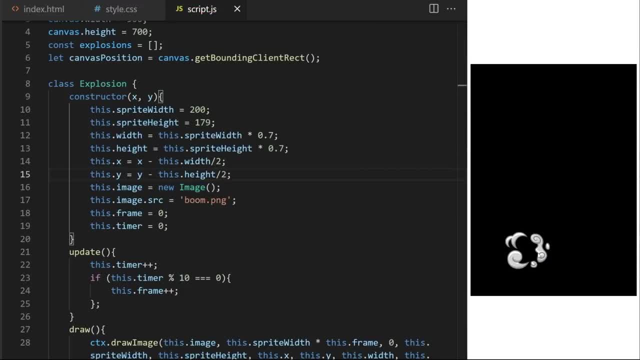 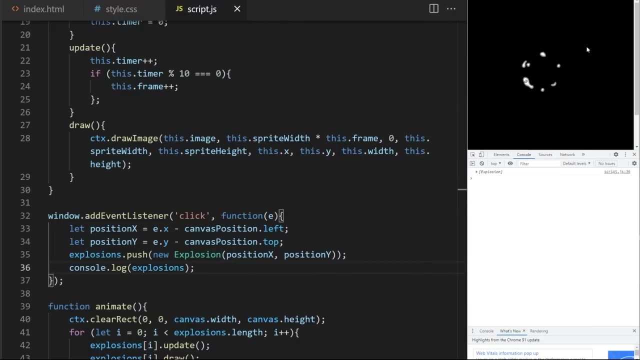 perfect. right now i am just adding more and more objects into my array. they stay there even after they stopped animating. you can see that if we consolelog explosions array from line 5, we are just adding more and more objects into the array every time we click. 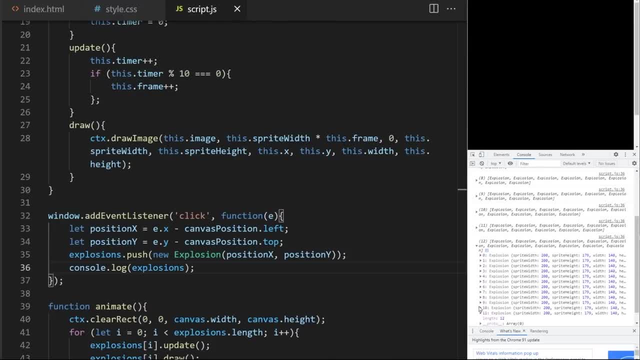 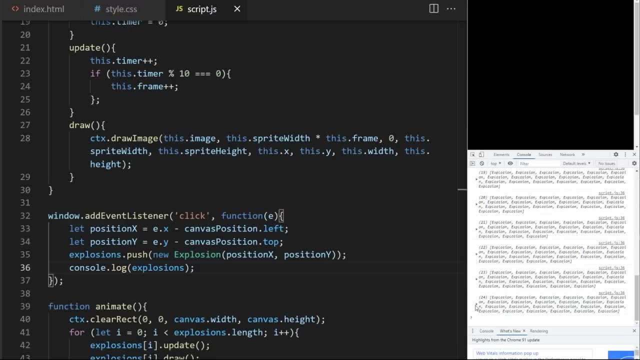 i need to find a way to remove the ones that have stopped animating. we could do object pooling here to avoid instantiating and deleting objects over and over, but i will show you how to do that in some more advanced tutorial. today let's just do the simplest solution. 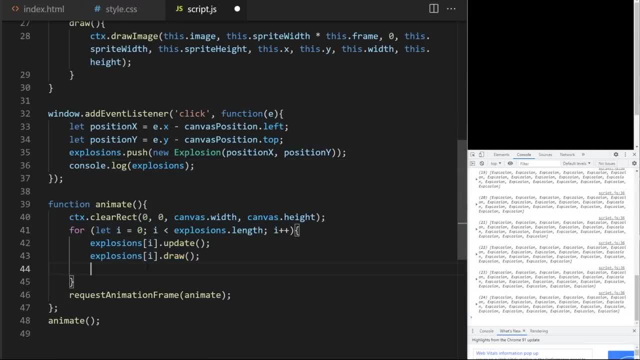 on line 45 inside the for loop that runs through all objects in my explosions array. after i draw and update them, i check if this particular object has frame property more than 5 frame property comes from line 18 and on line 24 we are increasing it. 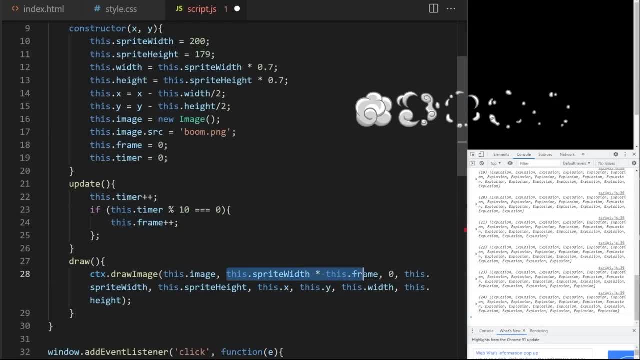 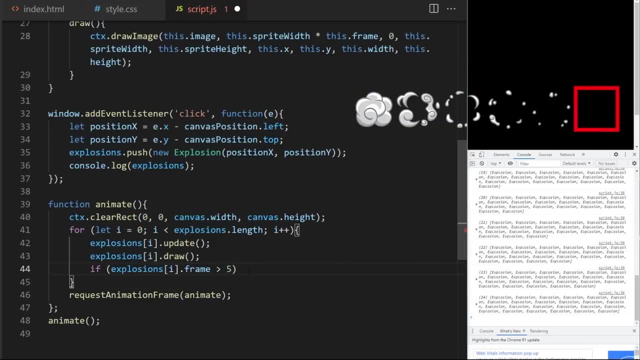 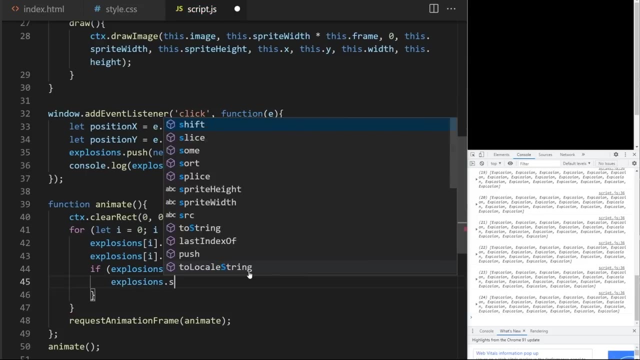 to draw our animation frame by frame. sprite sheet has 5 frames and we count from 0, so i know if frame property is more than 5. we played the entire animation on line 44. if this particular object has frame property more than 5, i will remove it using built in. 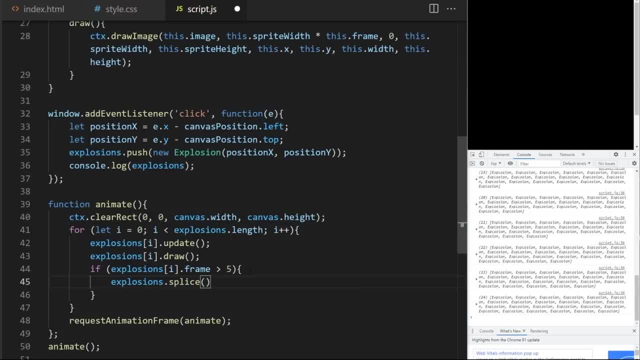 array splice method. splice method just wants index of object we want to remove, so i for index and i want to remove one object at this index, so i,1 to make sure the next object in the array is correctly updated and animated and removed its neighbor. we need to adjust index by minus 1. 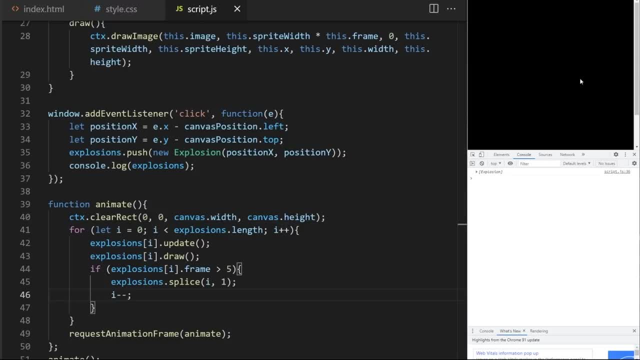 i minus minus because i am console logging my array. on line 36 in browser console, i can see that we are correctly adding and removing objects from the array. awesome, we have a solid infrastructure for triggered animation and we can connect this code to collision coordinates, for example, and run this animation. 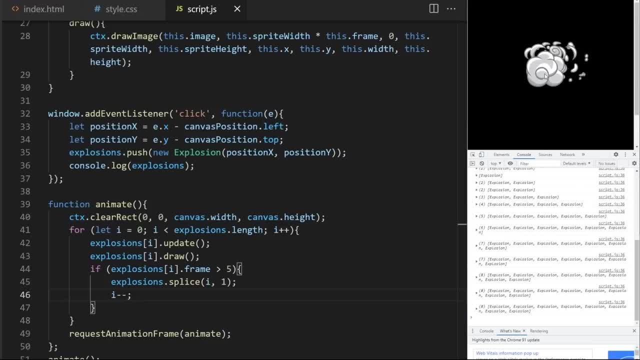 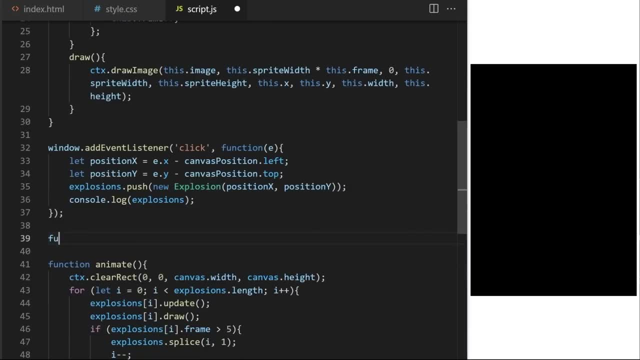 when two objects collide in our game. we can also connect it to different events and user input. it doesn't have to be a click event. in addition, i will put this code into a separate custom function. i call, for example, create animation. i cut all this code. 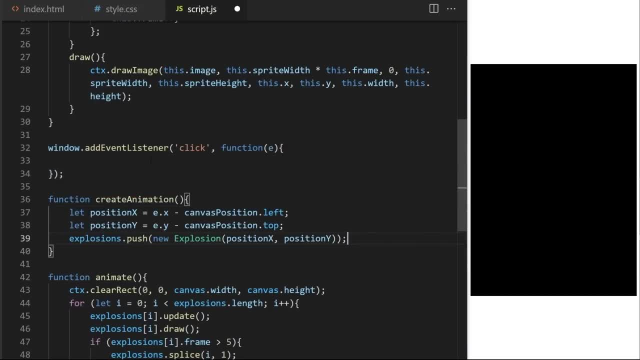 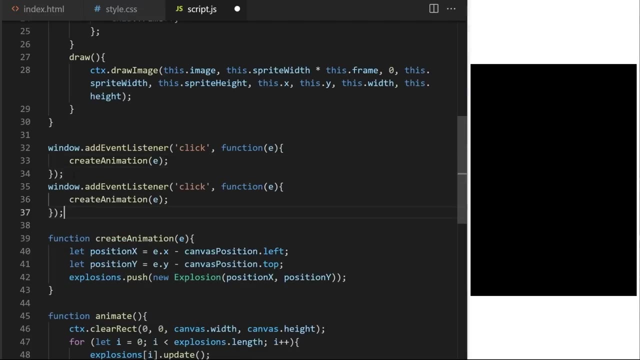 and i paste it here. i call create animation from inside my click event. we need to pass down reference to event object to calculate coordinates like this. look what happens if i connect it to mouse move event. it gives us pretty cool effect experiments. this looks like some deep sea creature. 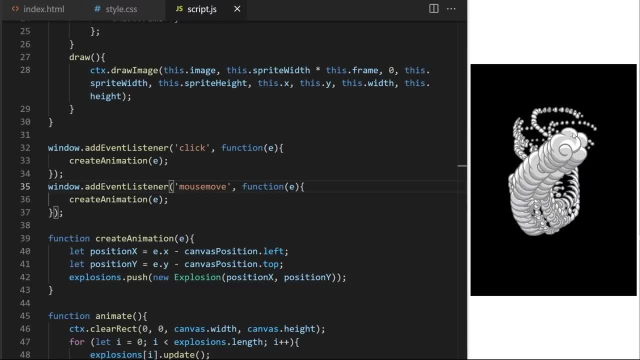 when i move it like this, you can see that the first frame of dust cloud animation is always rotated the same way. maybe i want to rotate it at different angle every time we create new explosion. to do that, i use built in save and restore html canvas methods. 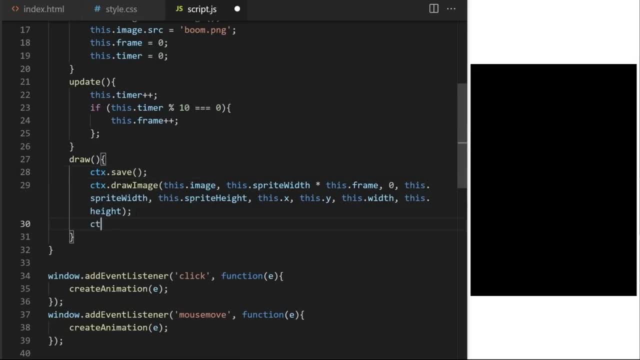 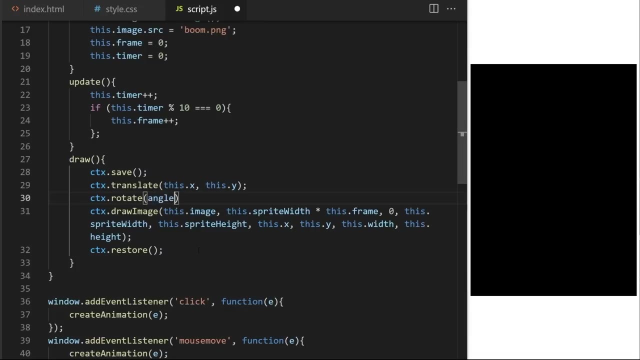 let me just write this and then i will explain what's happening. translate will set rotation center point. in this case, i want to rotate around its center. so this dot x and this dot y, i want each one to be rotated by different random angle value. i create a new property. 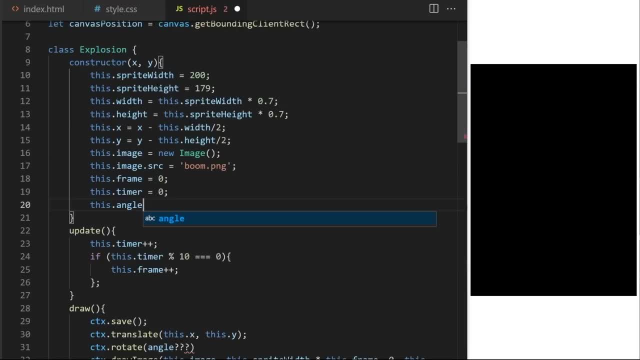 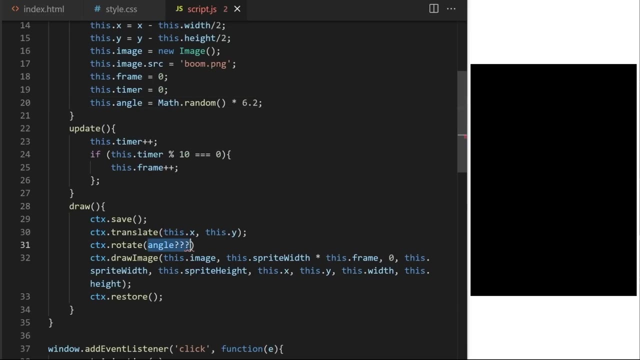 on line 20, called this dot angle. circle is 360 degrees. html canvas rotate method expects radiance, so 360 degrees is roughly 6.2 radiance. this dot angle will be a random number between 0 and 6.2. i pass this dot angle. 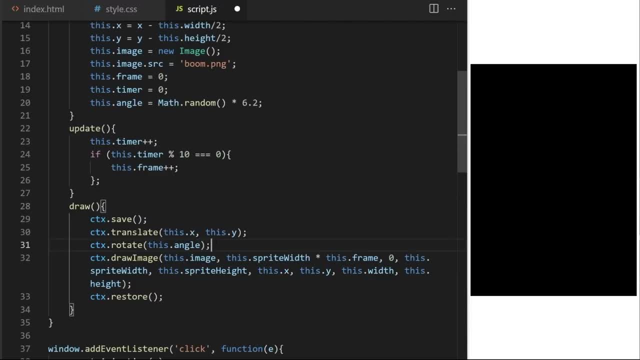 to canvas rotate method on line 31 like this: now it's rotating too much, it's because i translated drawing context to this dot x and this dot y on line 30. then i rotate it and then i go from that point further to another, this dot x and this dot y here. 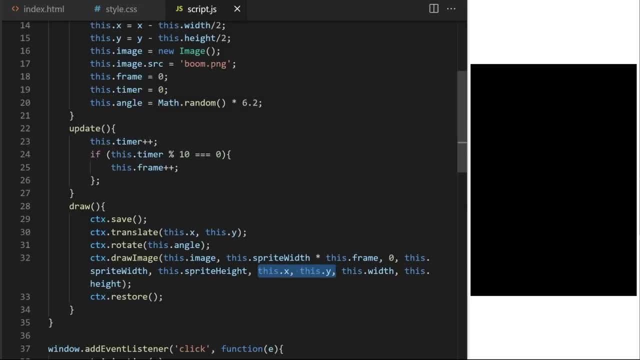 x and y coordinates for our animation are already captured here on line 30, so on line 32 i replace this dot x and this dot y to 0. think about it this way: i use translate, which would be 0.00 on canvas, to this dot x. 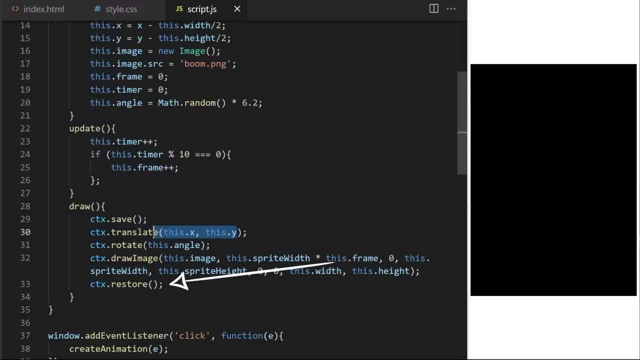 and this dot y. so between these save and restore calls, 00 is actually this dot x and this dot y. that's better. i also need to offset it by this dot width divided by 2 and this dot height divided by 2, here inside draw method. 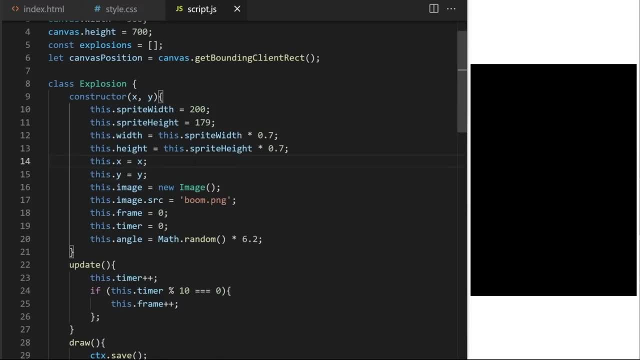 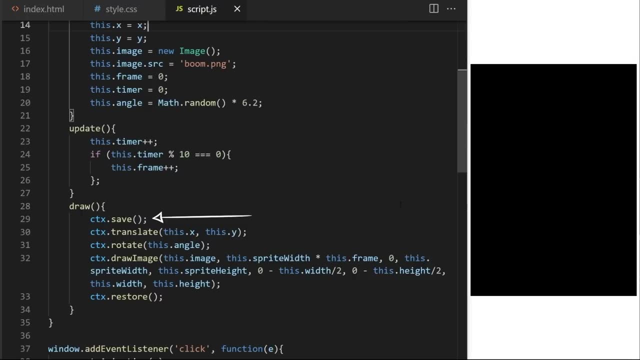 and remove it on lines 14 and 15. this is how you rotate anything on canvas. you save the current state of canvas to make sure the following changes affect only one draw call. i translate: rotation: center point on top of my current object. i want to rotate. 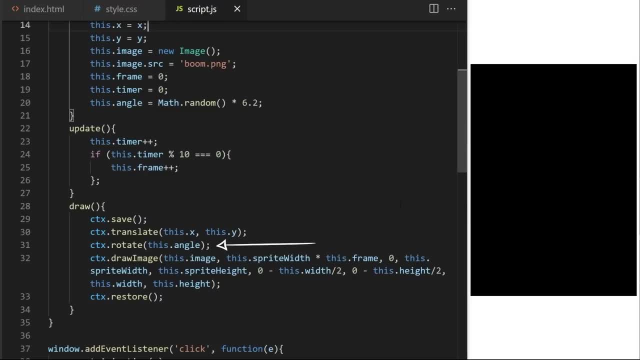 i rotate the entire canvas context by random angle value. we draw our image and we restore canvas context to the original save point. to make sure this translate and rotate only affects one draw call of one object. canvas rotation is one of the more difficult concepts for beginners to understand. 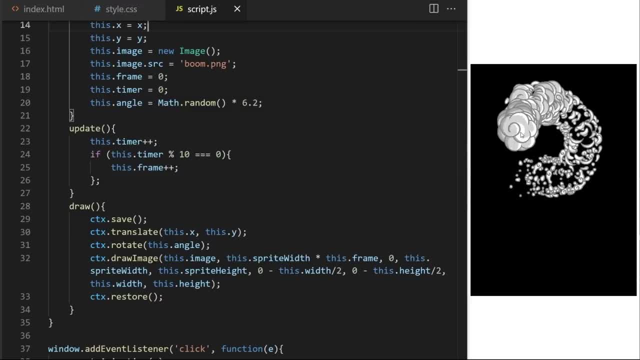 i spent the entire halloween episode explaining it, so don't worry if this was too fast for you. if you want more details on how to rotate things on canvas, i will link that episode in the video description. for now, let's just move on. you can see each dust cloud is now. 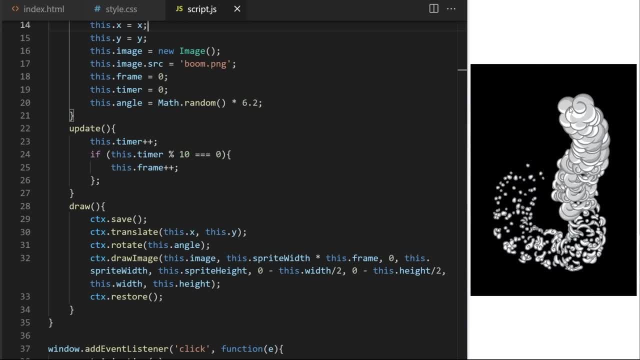 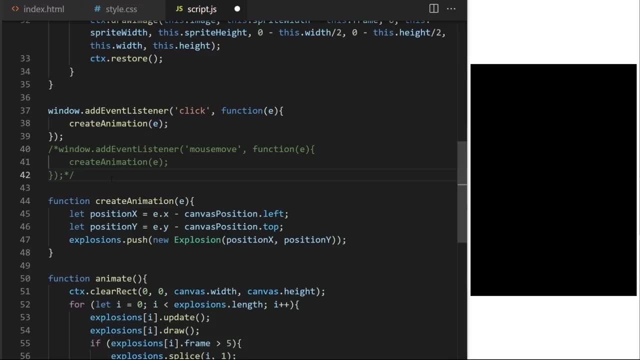 rotated randomly, so the trail itself looks more chaotic, as every dust trail should. let's comment out mouse move event. now we have this nice cartoon dust cloud animation whenever we click on canvas. it's missing something. let's give it some sound. it's really easy to attach sounds to. 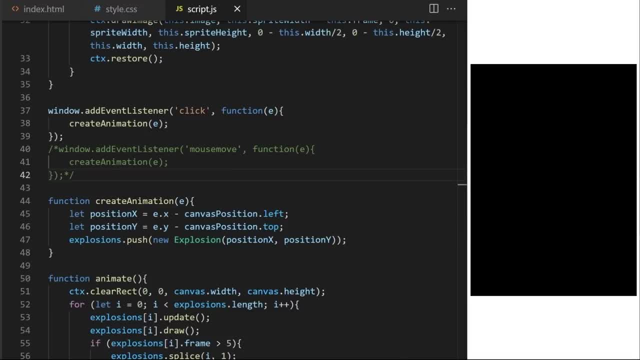 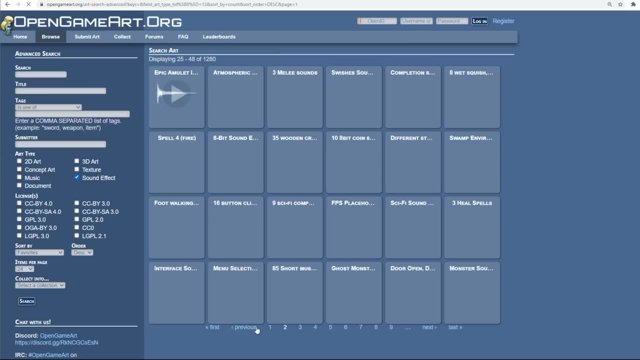 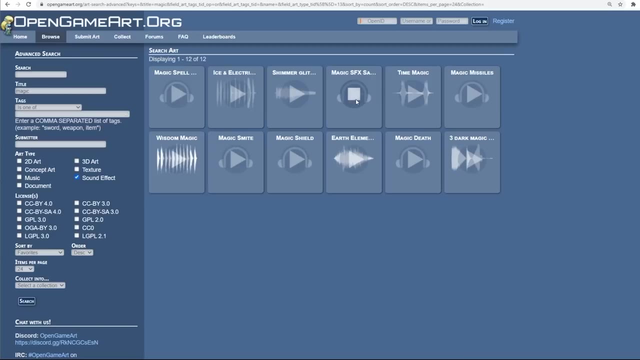 event animations in javascript. i go to opengameartorg and let's click browse. and sound effects. i remember there was one i really liked here on left. i will type magic in title search. oh yes, it's this one magic special effects pack. it contains four cool magic sounds. 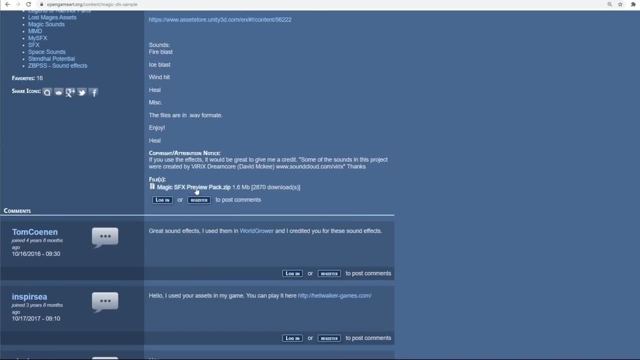 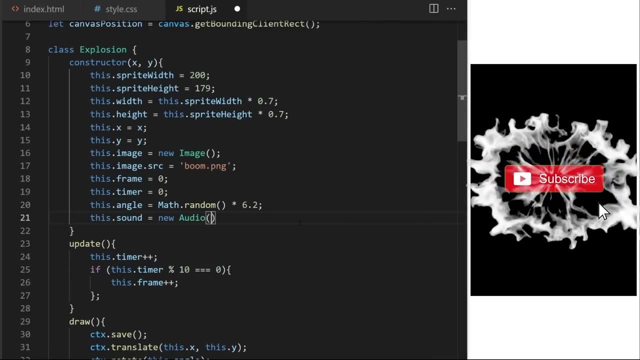 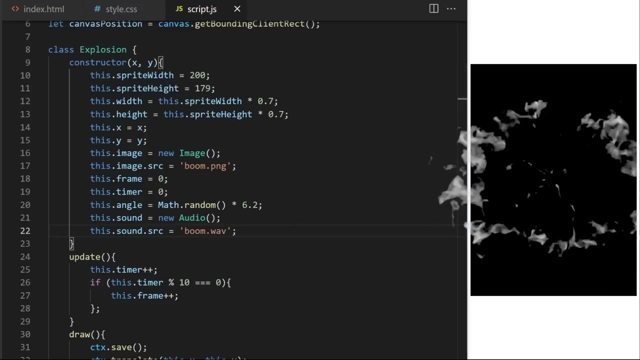 i download it and i take the one called ice blast. i rename it to boomwm wav. for you the path might be different if you chose different file or you placed it in a different folder. i only want to play this sound file once per animation, so in update method. 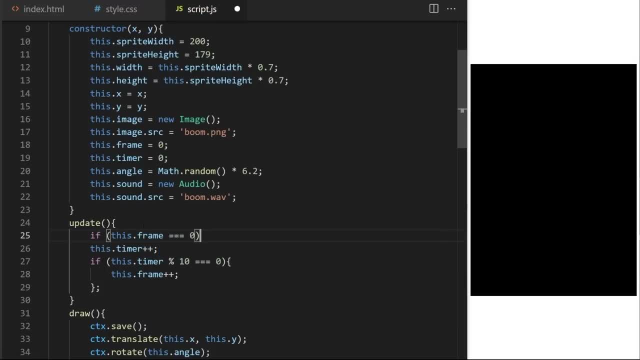 on line 25. i say: if this dot frame is equal to zero, take this dot sound from line 21 and call built in play method on it. like this: choosing the right sound and animation speed is very important to how your game feels in the end. if you do it well, your game will be. 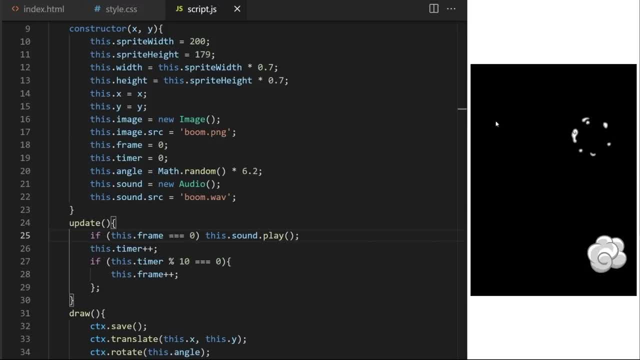 satisfying and your users will love to play it. don't forget to click the like if you learned something new today. for more vanilla javascript game development and animations, check out my playlist. i will link relevant videos in the description down below. thanks for coding with me today. hope you had fun. 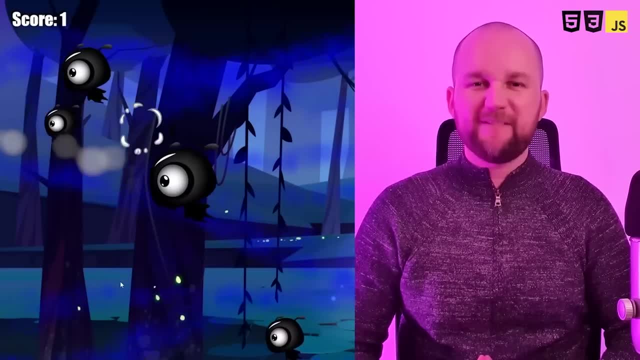 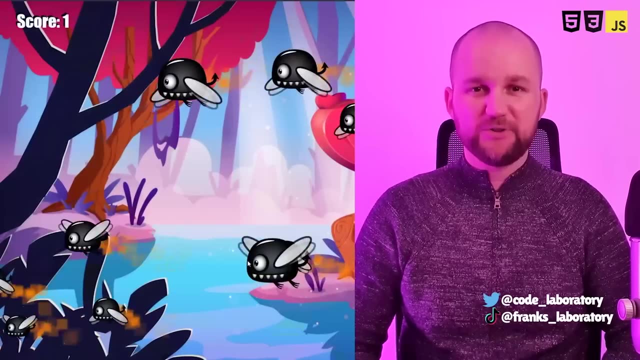 do you want to build awesome games and master front end web development at the same time? in this vanilla javascript and html5 canvas game tutorial, i want to show you 5 techniques i wish i used sooner today. we will build a game completely from scratch, step by step. 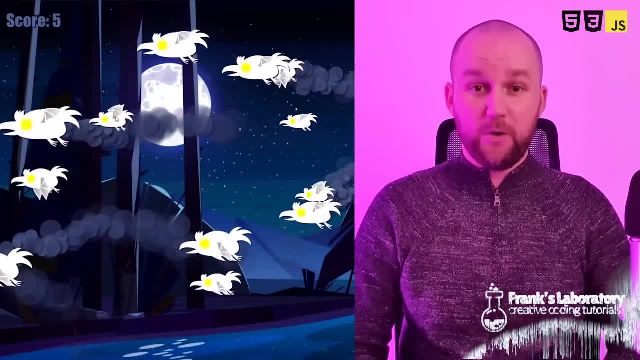 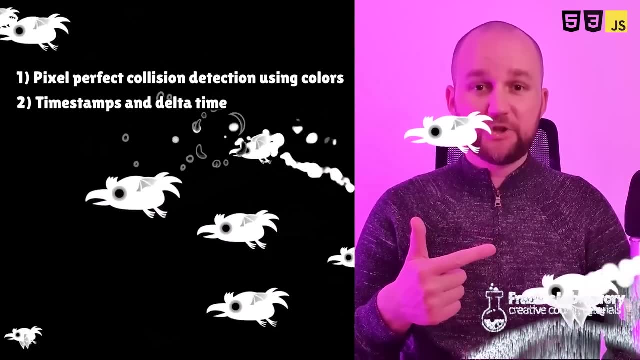 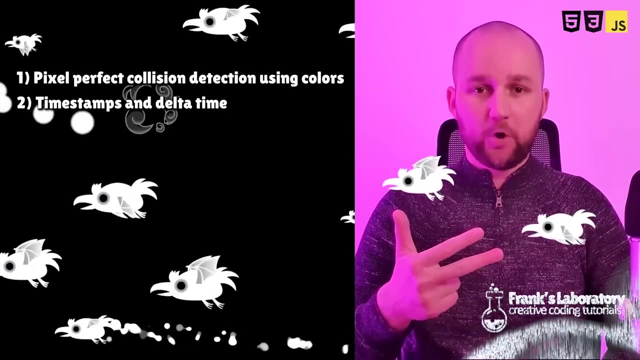 with no frameworks and no libraries. we will learn how to achieve pixel perfect collision detection using colors, how to use timestamps and delta time to make sure our game runs at the same speed on different machines. we will learn about arrays and i will show you how to remove old game objects from the game. 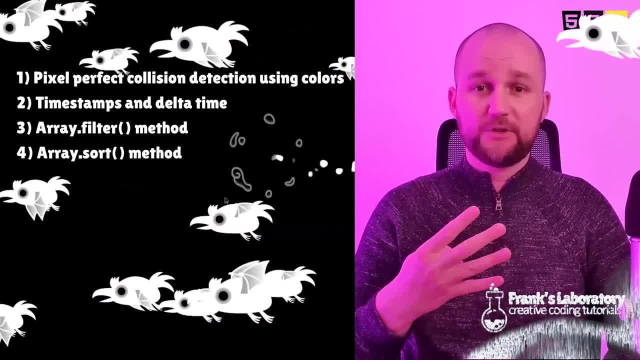 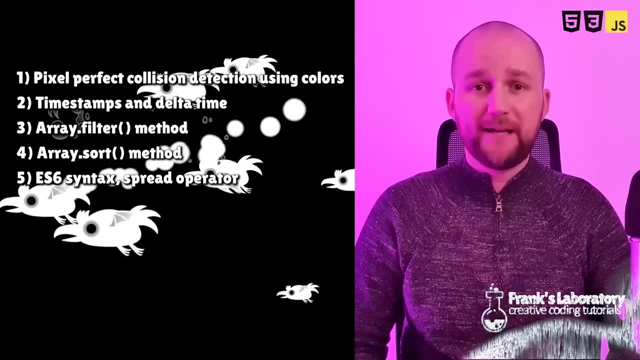 using array filter method and how to use array sort method to create a correct draw order in a 2d game. we will also talk about modern javascript syntax and we will learn how to make our animation code cleaner and less repetitive with spread operator. i will also share many small tips. 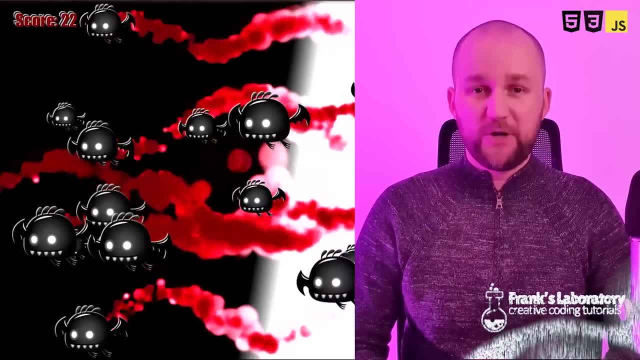 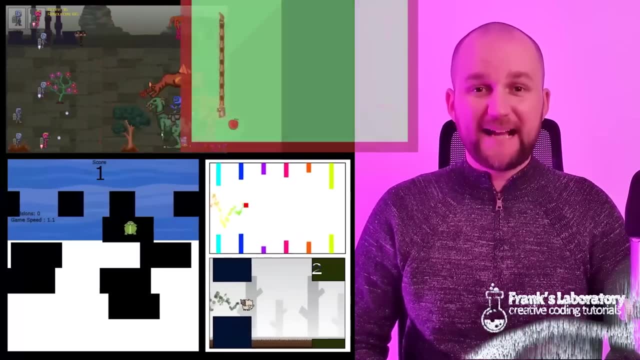 and tricks as we go along. students of today's course will get two premium spreadsheets completely for free, kindly provided by this amazing artist. check out his website for more. click the like, please, if you are excited and ready to learn. let's talk about javascript. have fun. 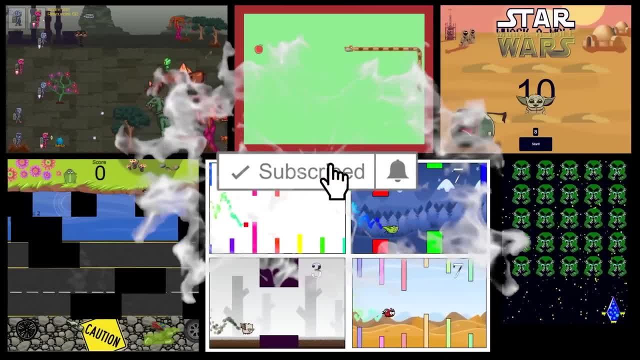 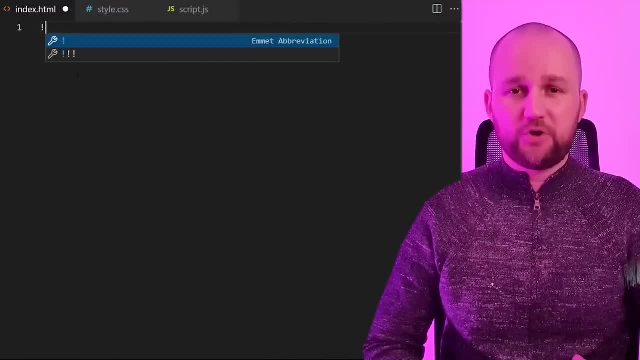 i want you to build projects you can show off to someone and be proud about. so, as usual, we will build a game and by the end of this tutorial you will have a complete project. i learned some of these techniques from my friend, radu. he has a. 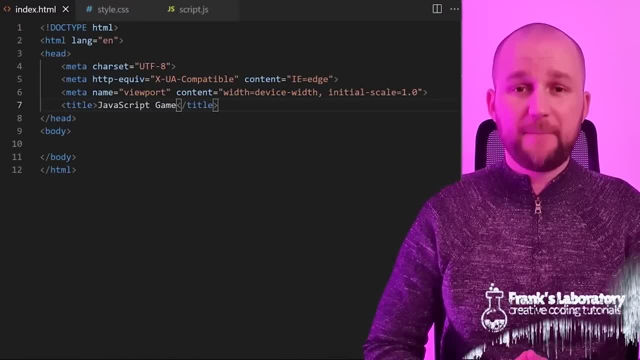 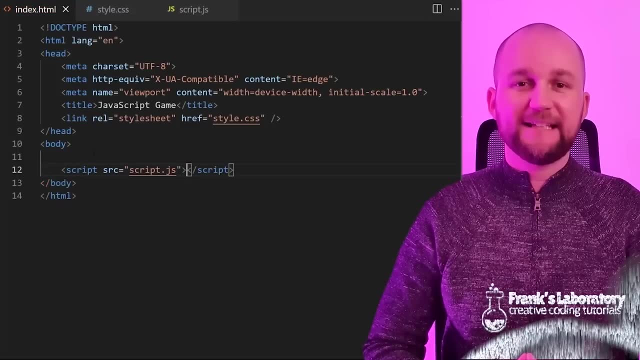 lot of other cool things to teach you. if you want, you can go and check out his courses. i will link some in the video description. some of you tell me that you only make games by animating divs, so i will show you how to do it in. 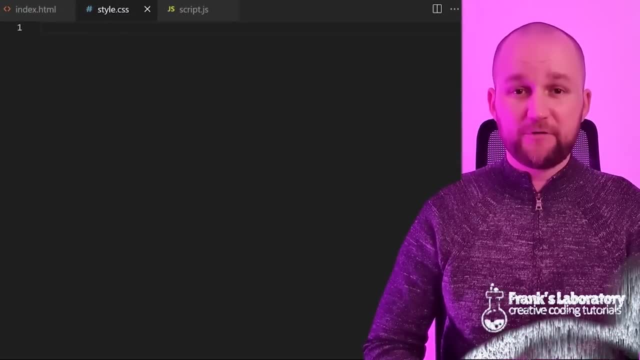 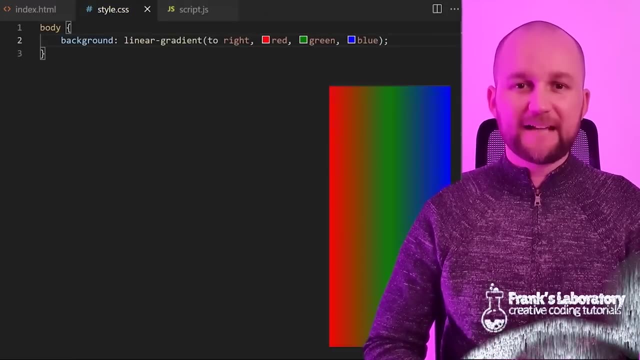 this video. i will show you how to do it in the video description. some of you tell me that you only make games by animating divs and other html elements. it's a great way to start and learn the basics. html canvas can handle many more moving objects at the same time, so if 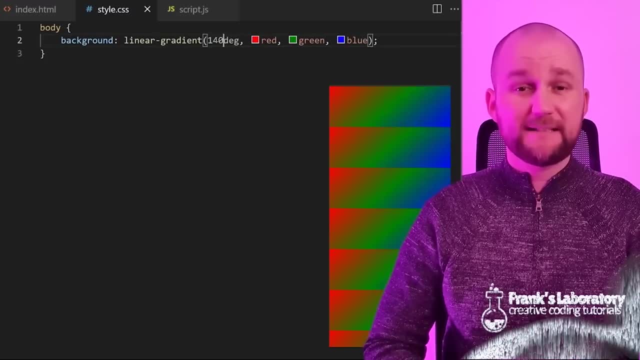 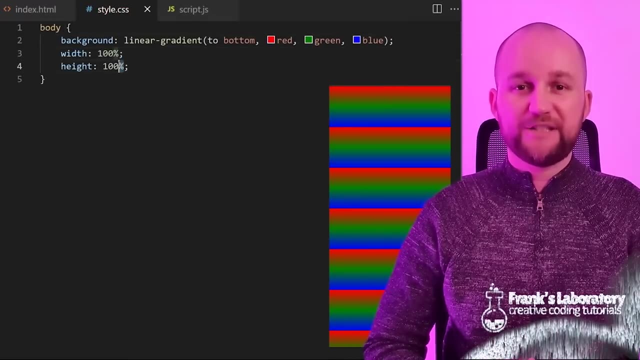 you want to try and build games that have a little bit more complexity. maybe this is the time for you to give canvas a chance. let me show you. it is easier than you think to build interactive animated projects with it. i will take you through it step by step and help you. 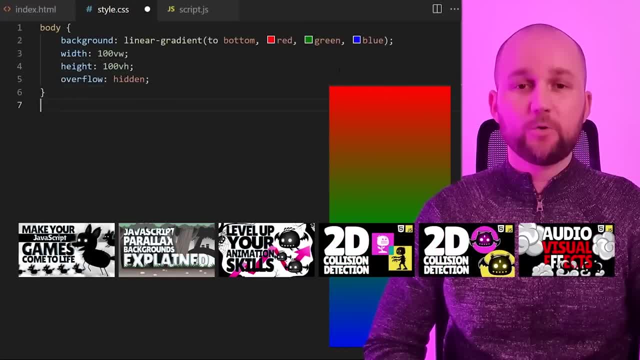 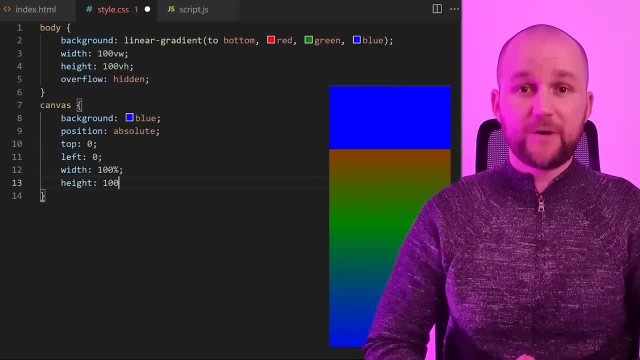 understand. i have a introductory game development series and a beginner playlist where i go slower over all the important techniques. if you find it interesting or you think i'm going a bit too fast, maybe try to watch that one first. over there we also create really cool projects, but i keep beginners in. 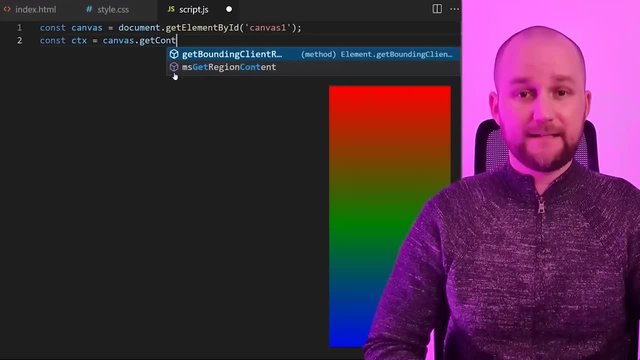 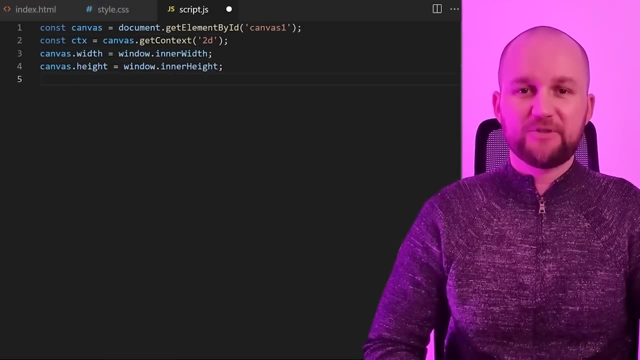 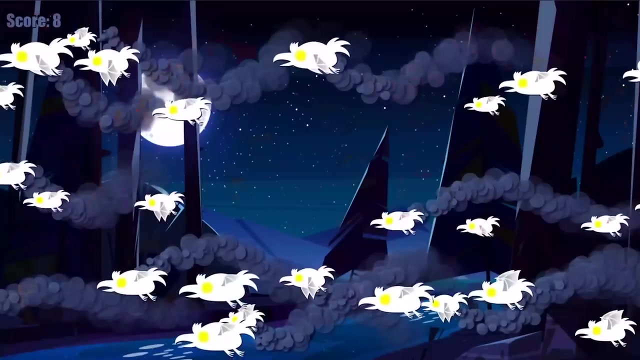 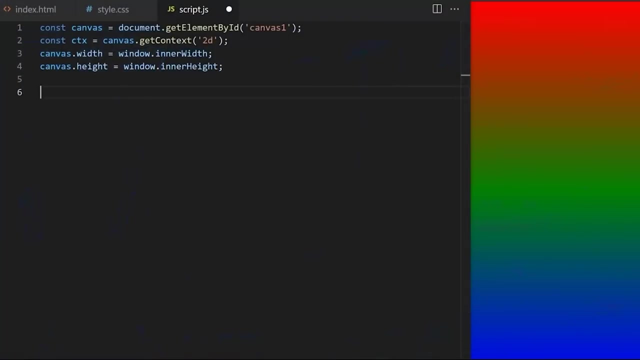 mind at all times. it might be an easier starting point for you, and then you will be ready to take on videos like this one and actually properly understand everything. i will leave some links in the video description. let's go, let's create some ravens. i will have an. 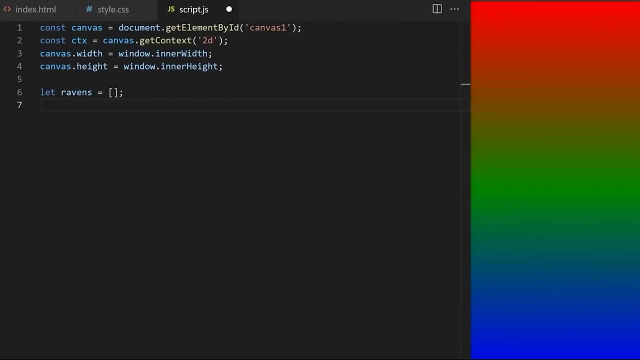 array that will hold all my raven objects. it needs to be a let variable, not const. i will explain why. in a minute i create a custom class called raven. it will be a blueprint based on which all my animated ravens will be created by javascript. constructor will create one. 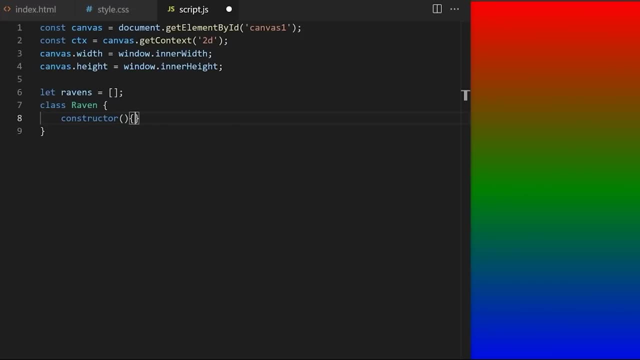 blank new object every time it is called and it will assign it properties and values as we define them here. it will have width, properties and values as we define them here, and its value will be, for example, 100 pixels. height will be 50 pixels. this dot. 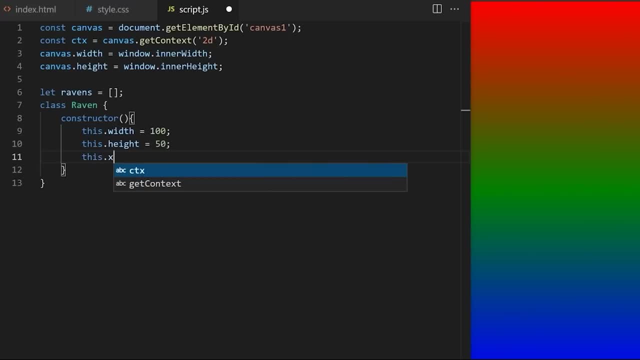 x. starting. horizontal x coordinate will be just behind the right edge of canvas so they can fly across to the left. so canvas width. vertical y coordinate will be a random number between 0 and canvas height, since rectangles on canvas are drawn from the top left corner going. 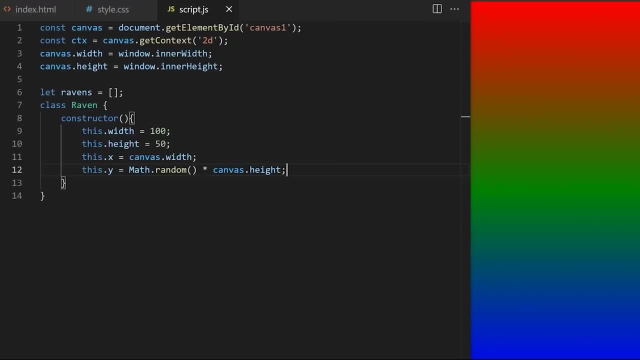 right and down. i don't want any ravens to be partially hidden below the bottom edge of screen. initial y position will be a random number between 0 and canvas height, minus the height of a raven between here and somewhere around here. it needs to be in brackets like this to: 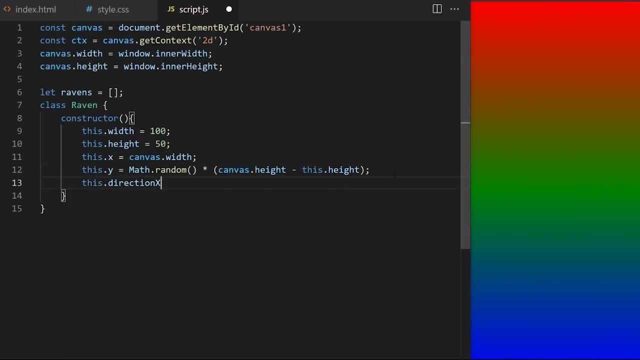 give us the correct range of values. direction x will be horizontal speed. basically it will be a random number between 3 and 8. i want ravens to bounce up and down as they fly, so the initial vertical speed i call direction y, for example, will be a random number between 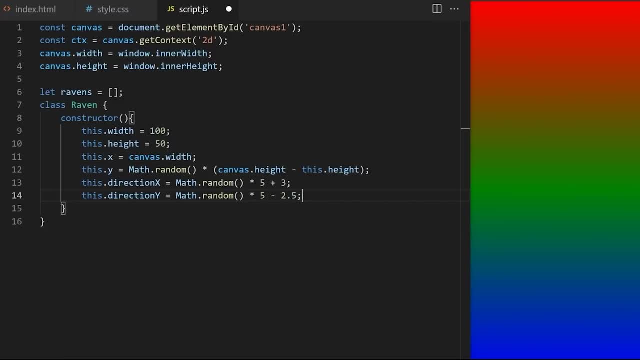 minus 2.5 and plus 2.5. minus values will move upwards. plus values will move the raven down along the vertical y-axis. update method will move the raven around and adjust any values that need to be adjusted before we draw the next frame. 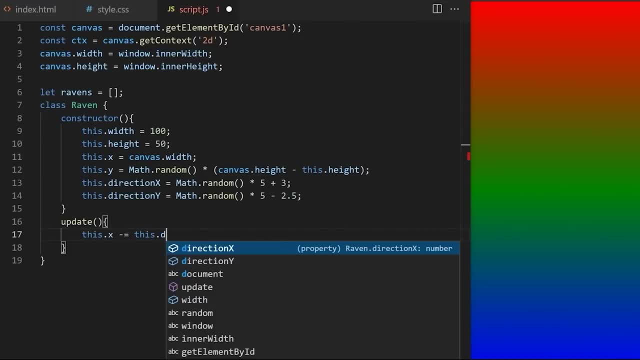 at first i will just simply move it to the left, so this dot x from line 11 minus equals this direction x from line 13. draw method will take these updated values and any drawing code we put here will represent single raven object visually. first let's start with a simple 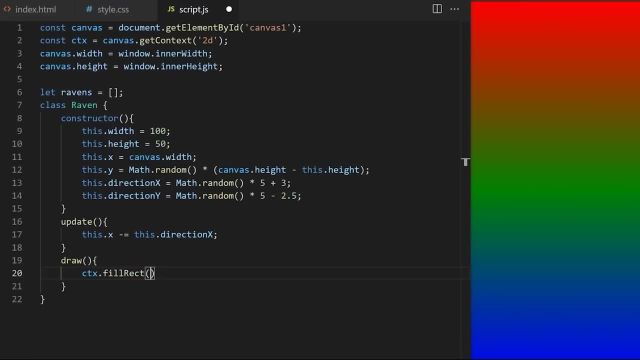 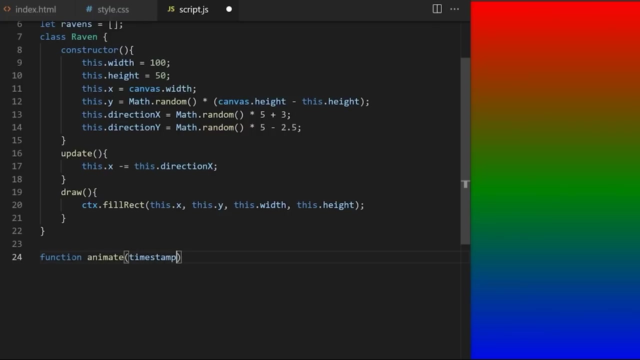 rectangle. i call built-in fill rectangle method and i pass it. x, y, width and height. raven class is complete. we have a way to create ravens. let's create animation loop. i create a custom function. i call, for example, animate. it will take argument. i call timestamp. this will be a. 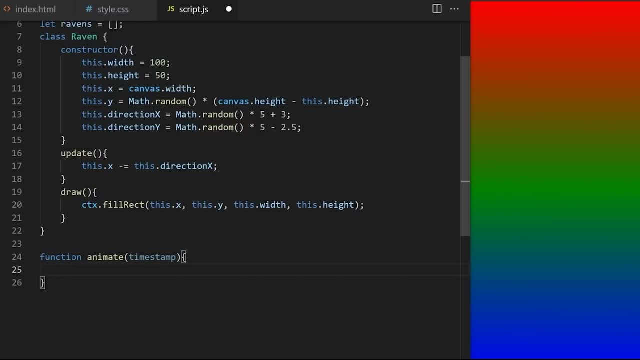 numeric value in milliseconds, so one second will be number 1000. i will show you exactly how it works. any code inside this animate function will run over and over updating and drawing our game frame by frame. the first thing we will do between every frame is clear, old. 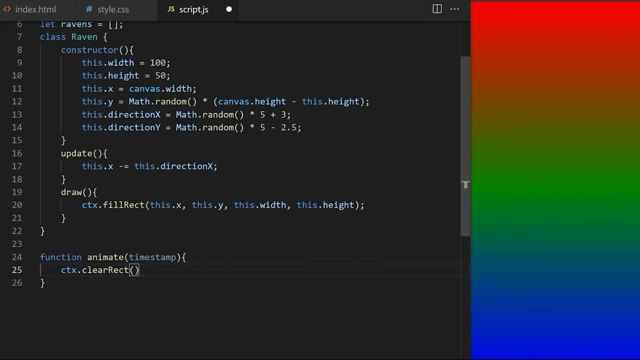 paint all the drawings from the previous frame, so clear rectangle and i want to clear the entire canvas from coordinates 0: 0 to coordinates canvas width, canvas height. we will run some code in between and then at the end we will use request animation frame method that will call: 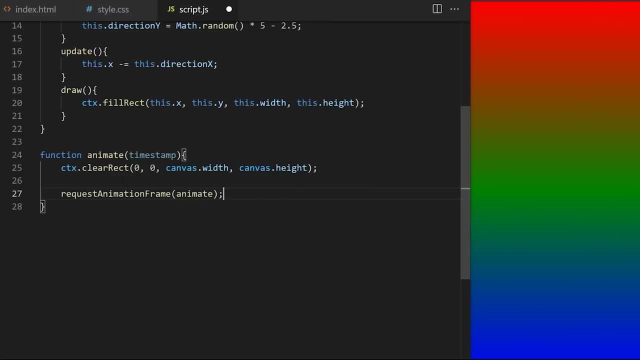 animate again, create an endless animation loop. i will console log test to make sure it works and i also need to call animate like this on the first page load to trigger the first loop in browser console. i can see the loop is running perfect. it gets to test your. 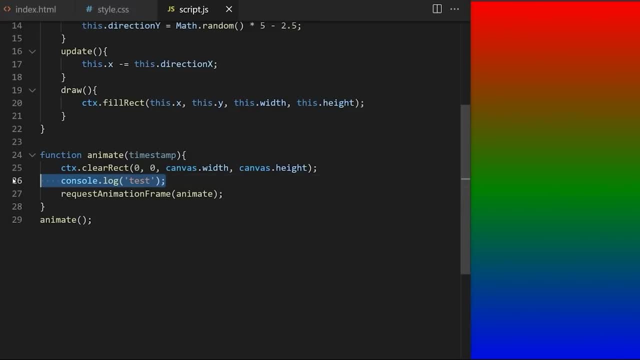 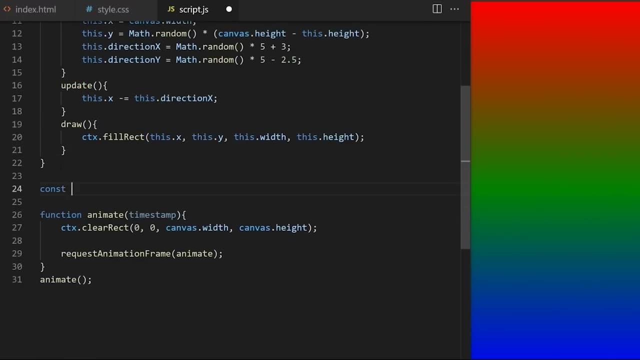 code as you go to make sure there are no typos. it's safer than to write the entire project and then try to look for bugs there. step-by-step approach will save you a lot of time. i can also test if my raven class is working. i will use. 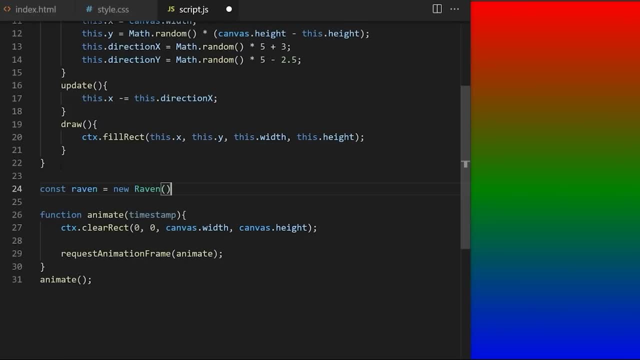 it to create many ravens, but i can also just create one. i create a variable called raven and i assign it to new raven like this: this will create one raven object for me, which will have access to update class method from line 16 and draw method from line 19. 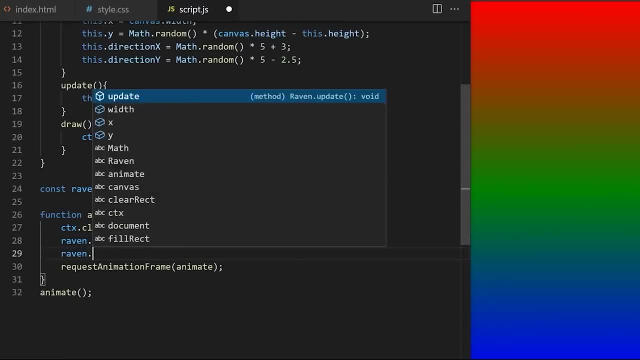 i call it from inside my animation loop and here's my raven. it just flies over once. if i refresh the page, it flies again. this works so far. we are doing great. instead of having one raven, i want to create a new raven periodically and i 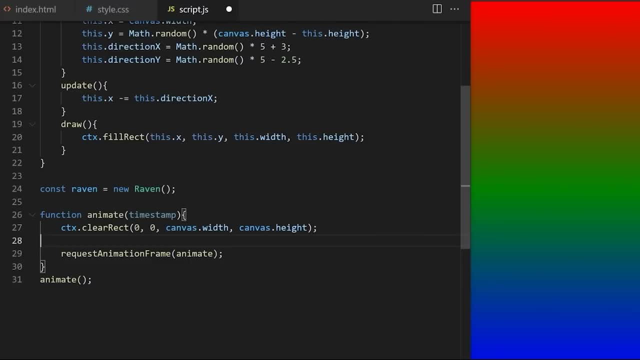 want to make sure that periodic event is triggered at the same interval on very slow old computers and on brand new gaming super pcs. to make sure the timings in my game are consistent and based on time in milliseconds rather than on the power of my computer and its. 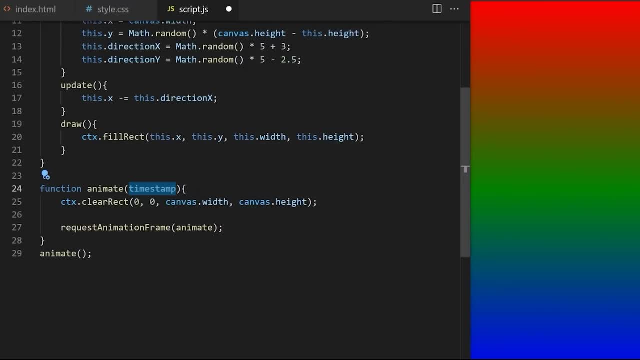 ability to serve frames at a certain speed. i will use timestamps, i will compare how many milliseconds elapsed since the last loop and only when we reach certain amount of time between frames, only then we will draw the next frame. it's actually very simple. you can do this very simple, but it might take. 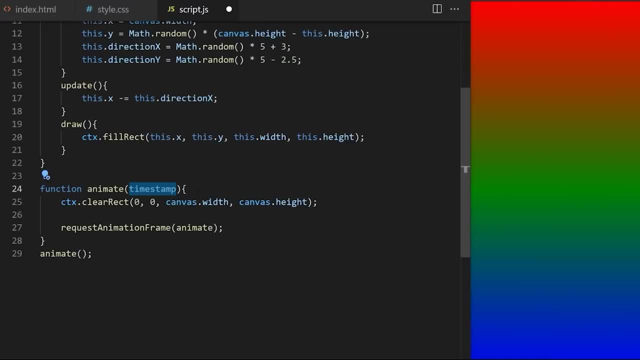 some time to get used to it. if you are a beginner, let's do it and see how it works. what is happening here? we are calling animate using request animation frame. animate becomes a callback function on request animation frame method and default javascript behavior for callback here is to pass it. 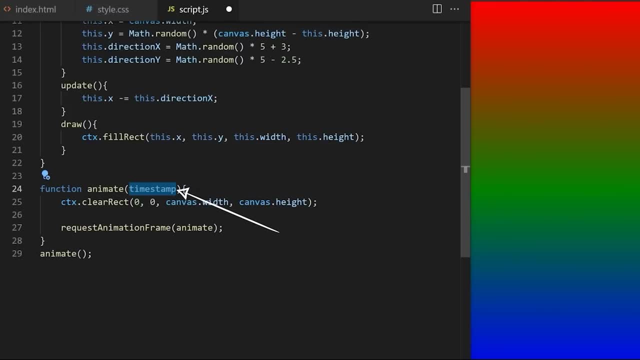 automatic timestamp as an argument. its value is in milliseconds, just so you know where this timestamp will be coming from. it's a default javascript behavior. when using request animation frame. it will pass its callback function, in our case animate automatic timestamp argument. we will see it better in a 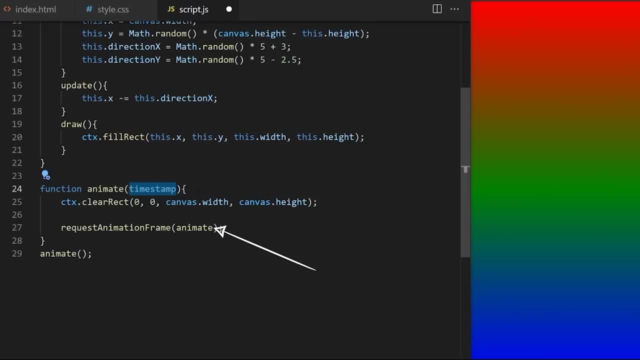 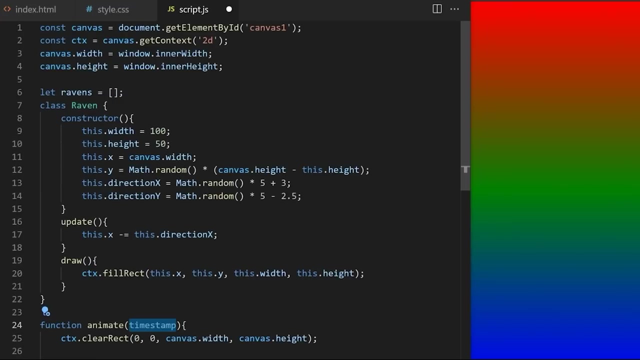 minute as the loop runs. request animation frame calls animate over and over passing it timestamps. my goal here is to take time from the current loop, save that value, run the loop again with a new timestamp value and compare them to see how many milliseconds it took in between frames. i will need some helper. 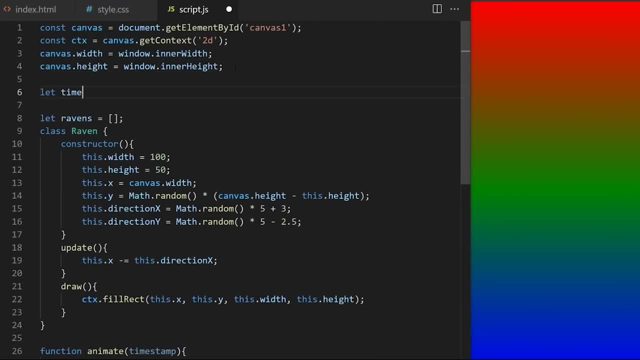 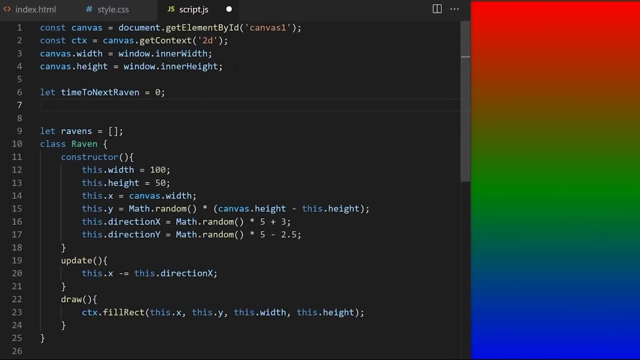 variables here. time to next raven will be a variable that will accumulate millisecond values between frames until it reaches my interval value and trigger next frame. initially it will start at zero. raven interval will be a value in milliseconds every time time to next raven accumulates enough to reach. 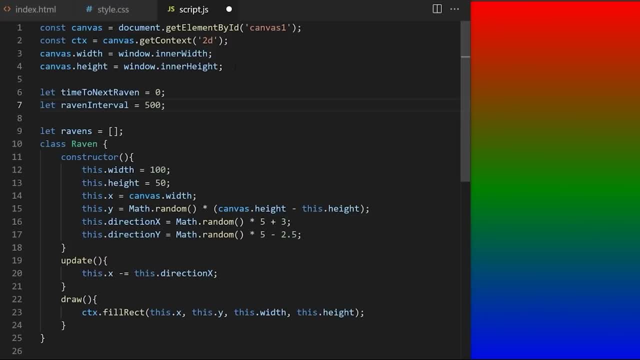 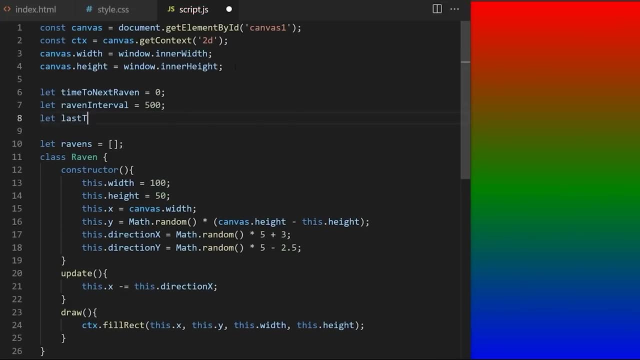 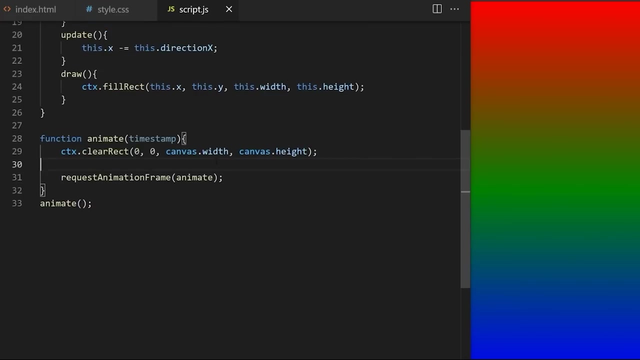 500 milliseconds. it will trigger next raven and it will reset back to zero to start counting again. i will also need variable that will hold value of timestamp from the previous loop. the initial value will be zero. inside my animation loop i will calculate delta time. this will be a 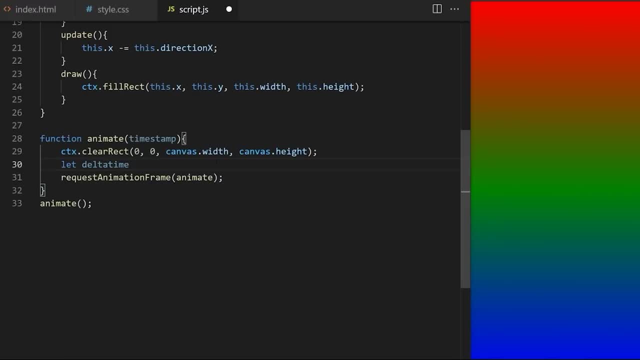 value in milliseconds between timestamp from this loop and saved timestamp value from the previous loop. after i used last time value to calculate delta time, i will assign last time variable from line 8 to the new timestamp passed here in this loop so that we have that value ready to compare. 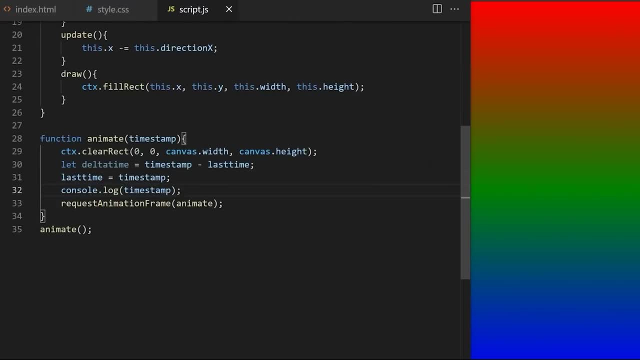 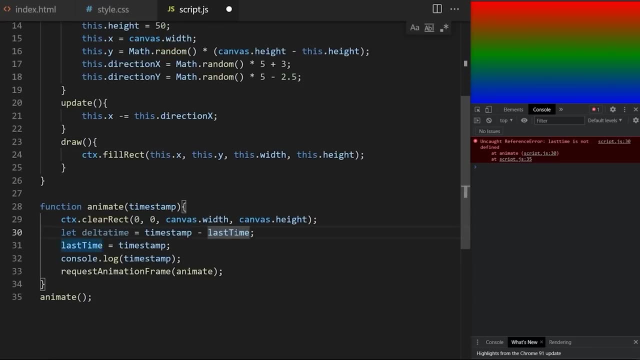 in the next loop let's consolelog timestamp. i can see i misspelled last time here. capitalization of letters is very important in javascript. you can see in console. i'm getting timestamps in milliseconds. since the loop started, the very first value is a second, so it. 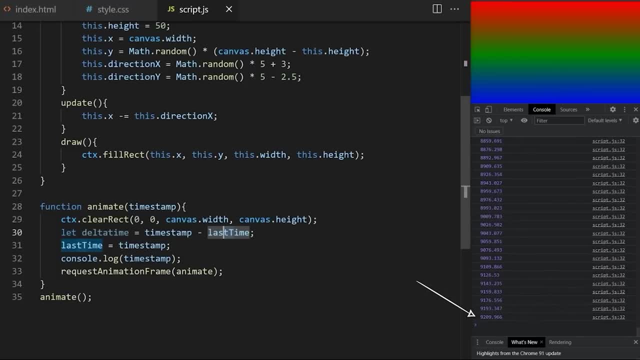 goes like this: seven, eight seconds and so on. so this is the automatically passed timestamp value here. it's generated by default by javascript, because we made animate into a callback function on request animation frame method here on line 33. there is a way to do this without. 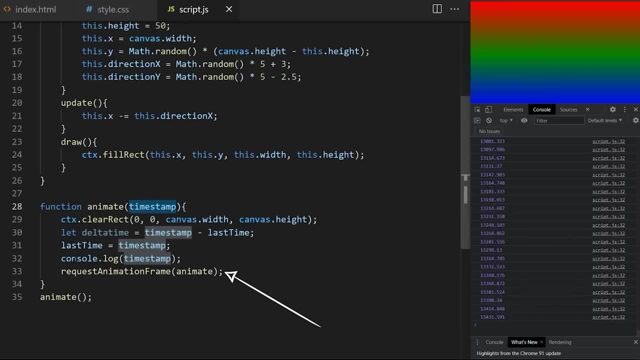 calculating delta time at all. but i haven't tested that and i'm not sure what is the browser support for that technique. so let's go with this tested, safer solution. today i will remove consolelog, leaving too many consolelogs in your projects, especially the ones running. so 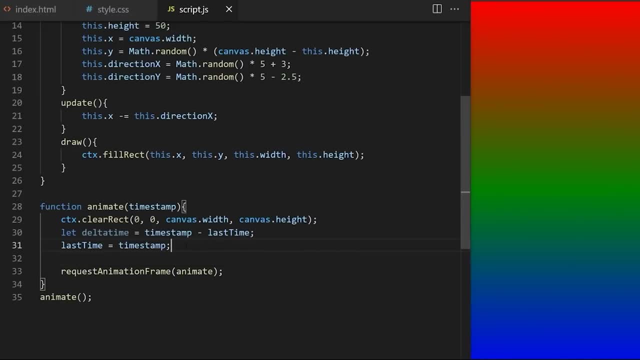 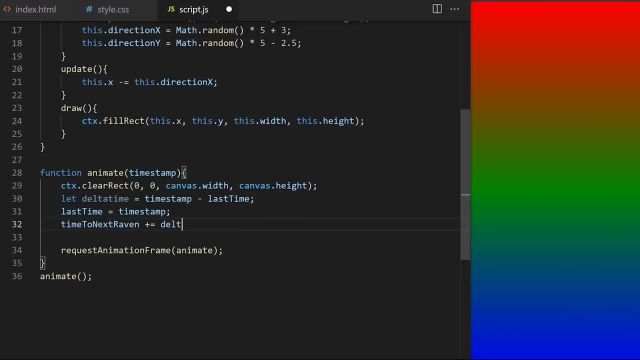 often like this can affect your performance, so keep that in mind. on line six, i have time to next raven variable here in my animation loop. i will increase its value by delta time for every animation frame. i will consolelog delta time. now again, i need to be careful about. 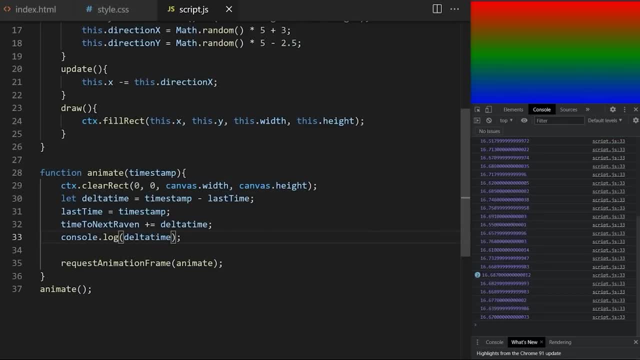 spelling my variables correctly here, i can see that on my computer time between frames is around 16 milliseconds. my computer is powerful and it is able to serve a new frame every 16 milliseconds. on your computer the number might be different. i would actually be very interested to know if it's the 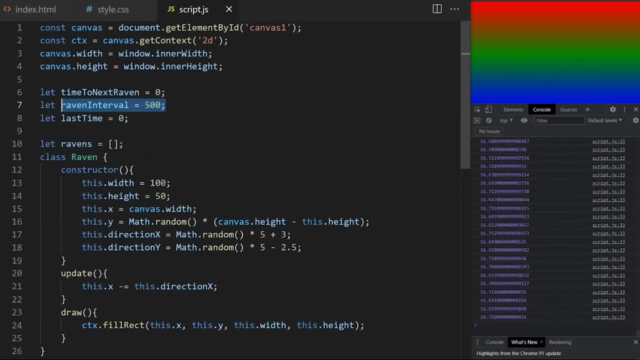 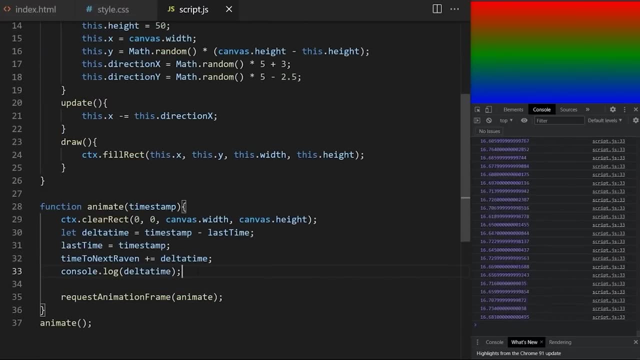 same number or a different one for most of you. if you are following and coding with me, can you leave a quick comment with that number please? you can just type 16 if it's the same number or whatever different number you are getting right now. so time to next raven starts at a zero. 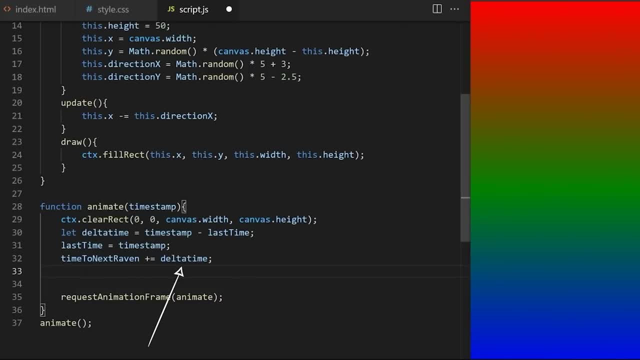 and is increasing by this value of around 16 milliseconds per each frame. on line 7, i created a variable called raven interval and i set it to 500 milliseconds. in my animation loop i will say when time to next raven reaches this raven. 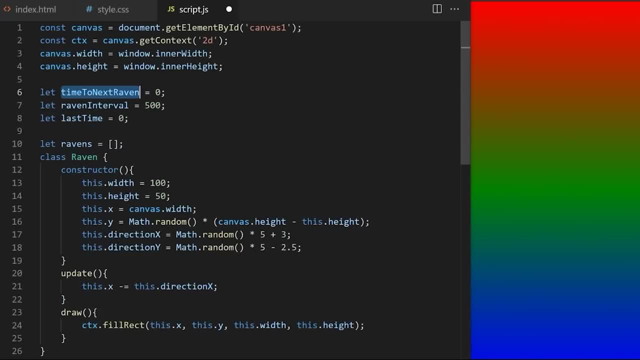 interval when this number that starts at zero and increases by the amount of milliseconds that happened between frames reaches 500. at that point we will take raven's array from line 10 and use built-in array push method. i will pass it new raven which will: 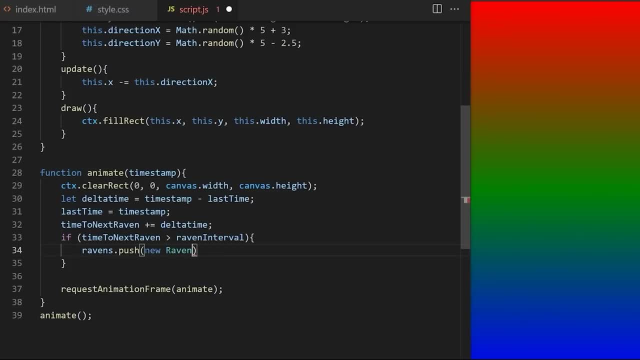 trigger my raven class constructor, create one new raven object and it will push it inside raven's array. when that happens, i set time to next raven back to zero so it can start counting again from the beginning. i know i just said raven a lot time to. 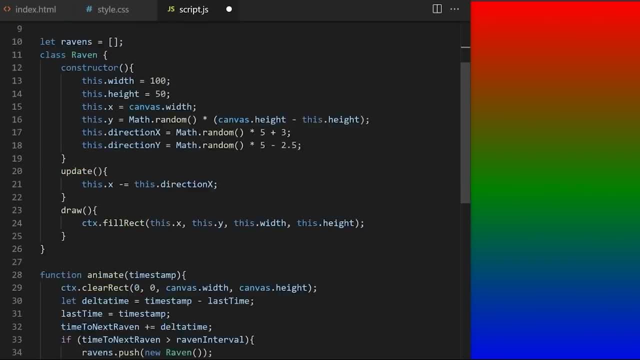 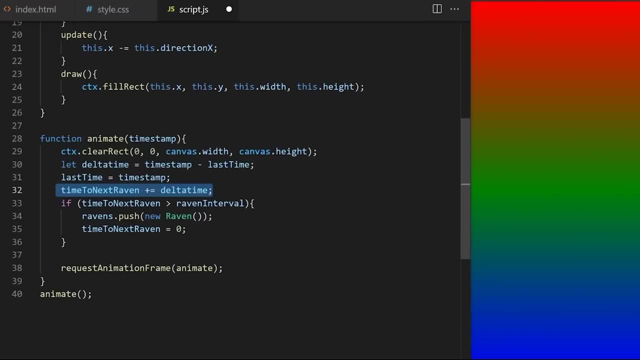 next raven starts at zero, it increases by the amount of delta time, by the amount of milliseconds between each frame, which will be dependent on performance of your computer. however, since slower computers will take longer to serve the next frame, their delta time will be a higher number. 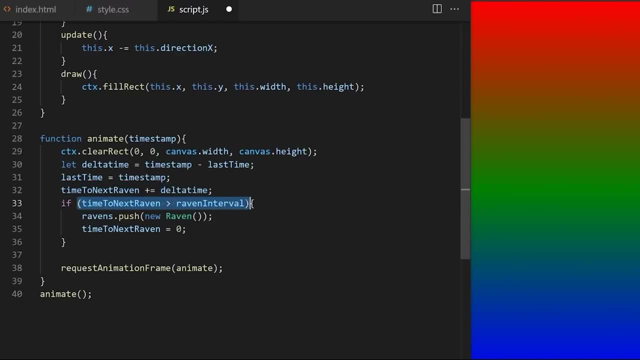 and it will move towards our target raven interval in bigger steps. as a result, this code will be triggered at the exactly same time on slow and fast computers. this is one way how you can properly trigger periodic events in your projects using timestamps. this might be a bit too much to wrap. 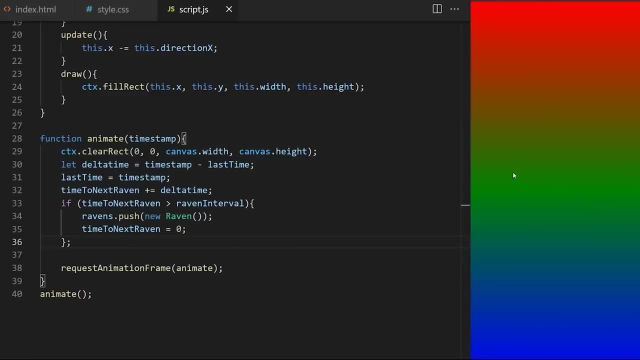 your head around if you are a beginner. it's one of the reasons i don't always use timestamps in my animation tutorials, because i can't really explain all of this in every single video, but try to learn it if you can. if you still don't get it, don't worry, i. 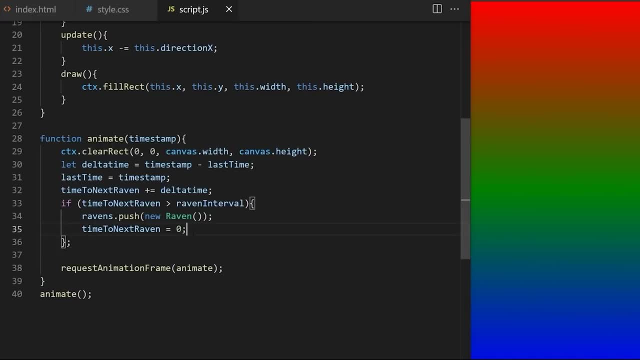 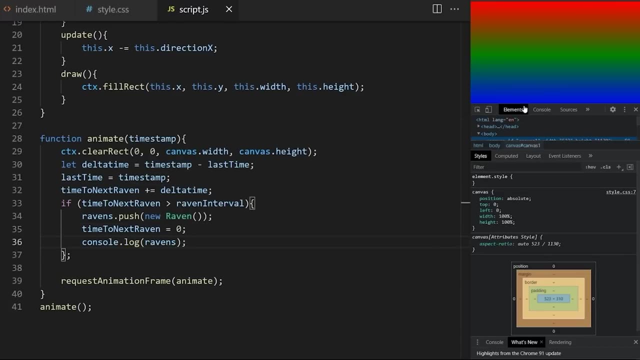 will explain it in future projects again, so eventually it will start making more sense. repetition and practice is the best way to learn, at least for me it is. i console ravens and i see nothing is happening, even though my animation loop is running. it seems that this if statement never 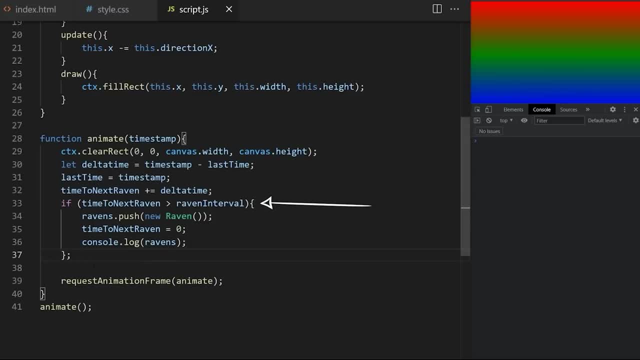 evaluates the true, so the code inside is never triggered. console is great for debugging. i console time to next raven first. oh, i can see it's vibrating. the value is none, not a number. here's our problem. why is it this value? it must be because we are adding delta time to. 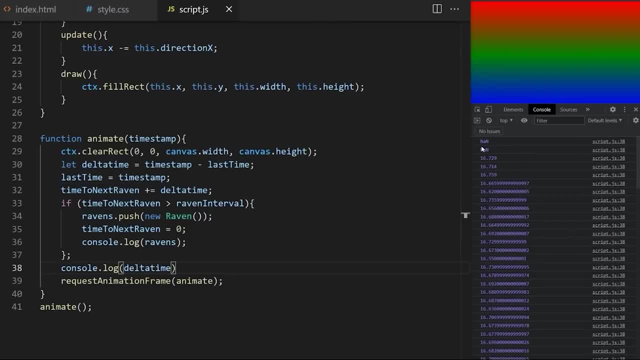 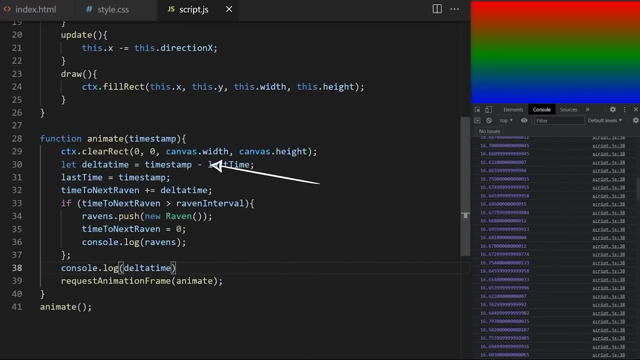 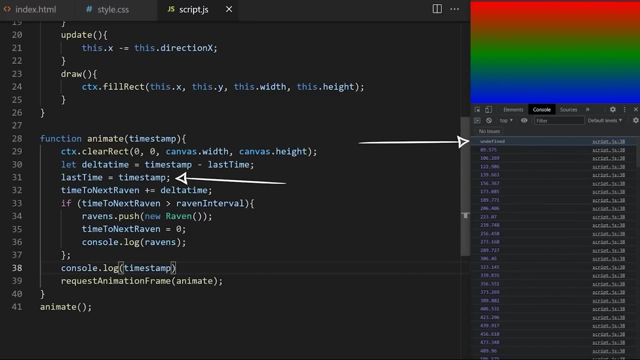 it here. i console delta time and i can see that the first initial value is also not a number. delta time is calculated here on line 30. so now i console lock timestamp and this is the root of our problem. that cascaded all the way through my variables. 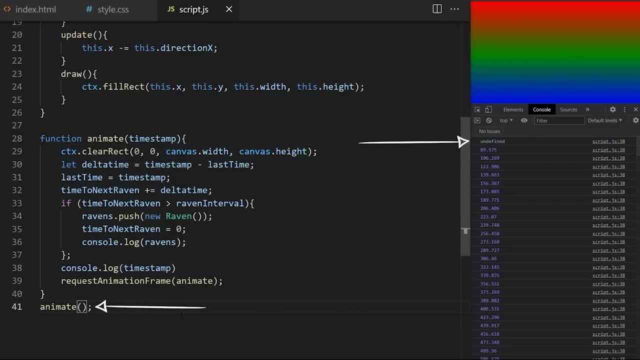 that use each other to calculate their values. when the animate loop starts, the very first timestamp is undefined because timestamp only gets created on the second loop, here on line 39, when we call request animation frame. to fix that is easy, i just need to give timestamp a starting value on the first. 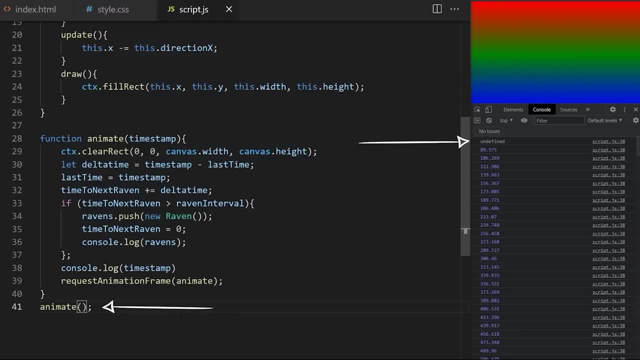 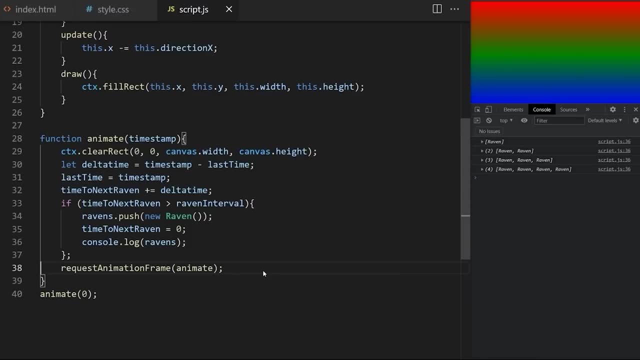 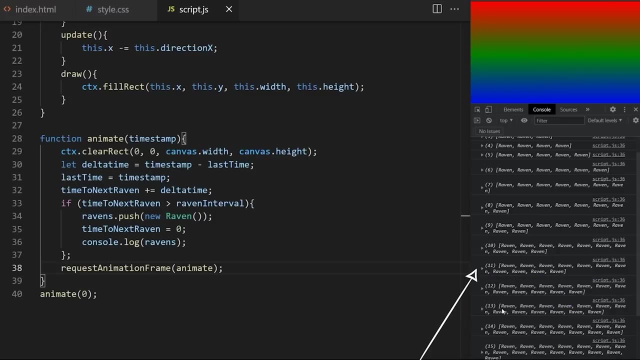 call of animate. that starts my animation loop here. i will pass it timestamp of zero as an argument. awesome, that fixed it. and since i'm console login ravens array on line 36 i can see it adds new raven object to the array every 500 milliseconds. 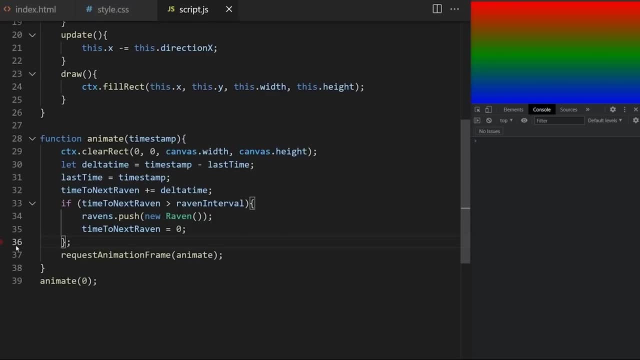 i remove the console log. we have data for ravens inside the array. we just need to cycle through that array, through every single raven object, and call their update and draw methods so that we can actually see movement on canvas. i declared my ravens array here on line. 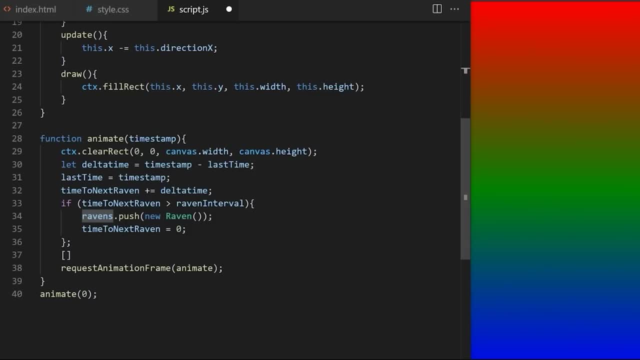 10 inside animation loop. i will use this syntax, which might be a bit unusual for you. here i'm creating so-called array literal by just dropping square brackets. like that, i'm creating a quick new array on the fly and these three dots are so-called spread operator. 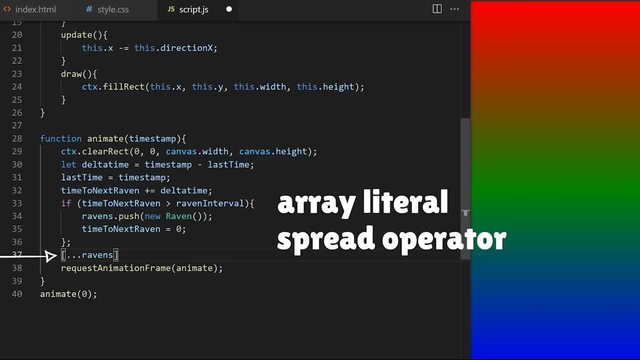 now i'm spreading my ravens array inside this new quick array i just created. spread operator allows us to spread iterable such as this ravens array to be expanded into another array. let's finish writing this line of code and i will explain why i'm doing that. since we are dealing 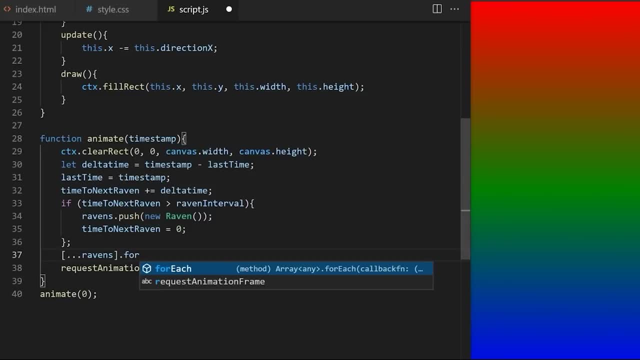 with an array, i can call built-in array. for each method i need to assign it a variable name for each object in this array so we can use it as we iterate, as we cycle through it. i will call that variable, for example, object. so this object variable now represents each. 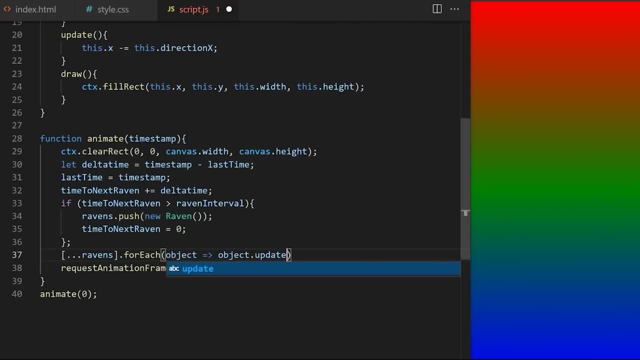 individual raven object in ravens array. and i can say, for each raven object in ravens array, call their associated update method. we wrote on line 20, so this line of code will cycle through the entire ravens array and it will trigger update method on all of them. 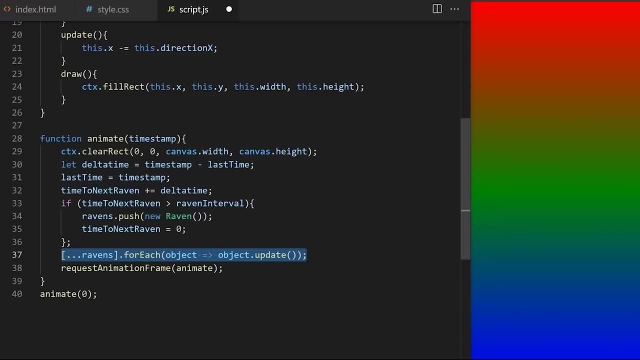 since we are inside animation loop, this will happen over and over for each animation frame. i will do exactly the same thing for draw method from line 23, and we are updating and drawing our ravens- awesome. now you might ask: why am i using this fancy syntax here? 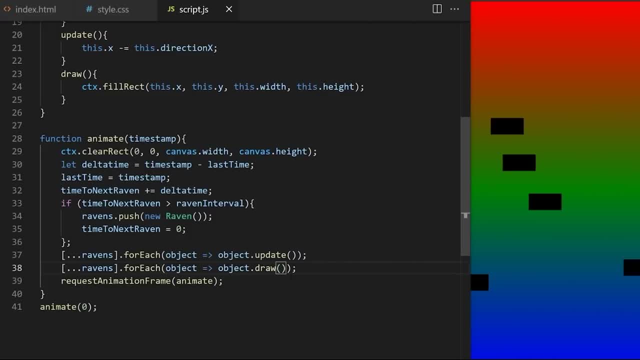 where i created a new array and i used spread operator to expand my ravens into that new array just so that i can call update and draw on them. i could have just called it on ravens array directly without expanding it like this. the reason i did that is because when i 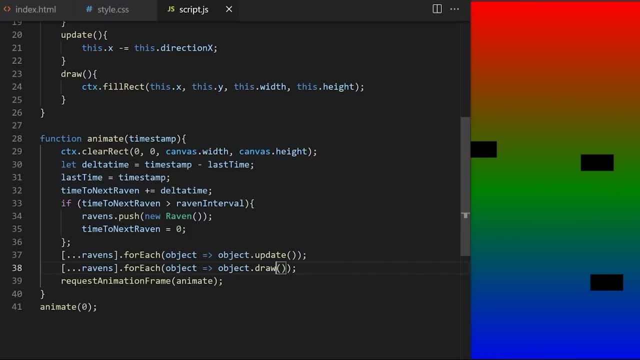 create particle class in a minute. i can just spread my particles into the same array along with the ravens. as long as my particle class will have update and draw methods to call, the code will work and i can call all my classes by just expanding more and more arrays. 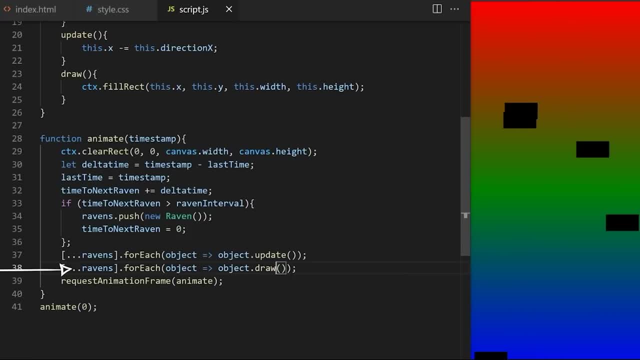 in here. i can, for example, also have an array of enemies, obstacles, power ups and other elements in my game. i can spread all of them into a single array and call their update and draw methods all at once. i will show you exactly what that looks like in a minute. i think it makes the 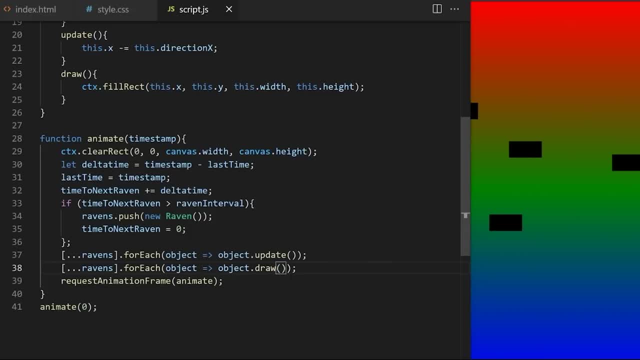 code look clean and easy to read. what do you think? on line 34, i'm periodically adding new object into ravens array. right now it's an endlessly growing array of objects, and on lines 37 and 38, i'm iterating over all of them, even the ones that have moved off screen. 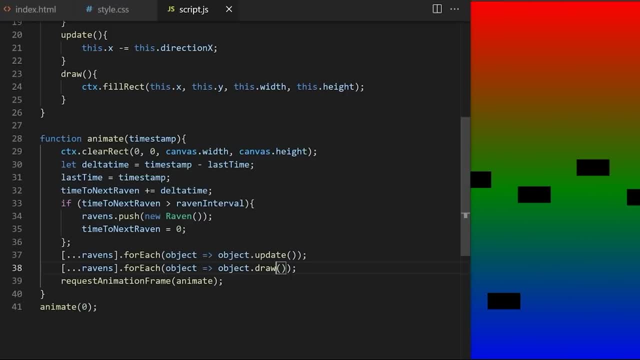 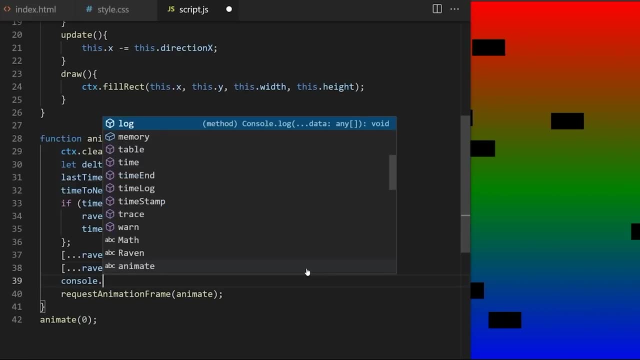 and are not visible anymore. eventually this would build up and cause performance issues, so i need a way to remove the ones that have moved past the left edge of game area. sometimes i use array splice method to do that. i used splice in many other tutorials before, but there might be a. 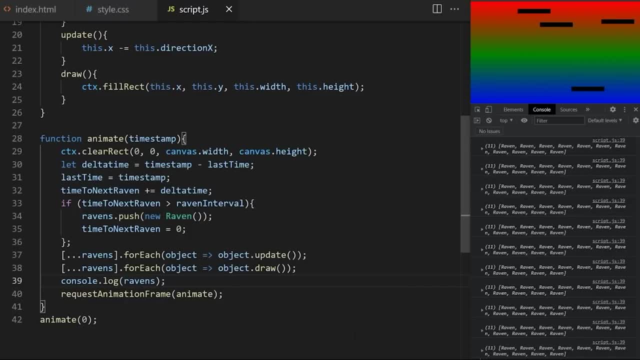 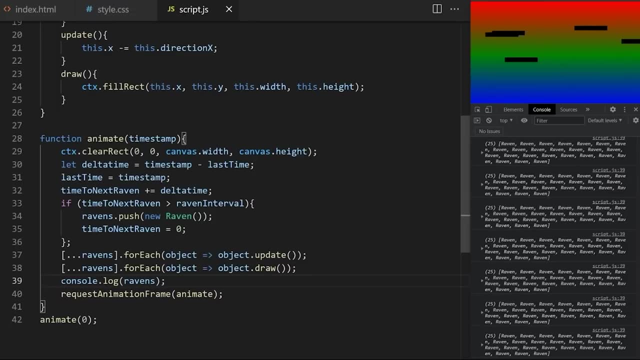 better way to do it, using splice. while cycling through the array removes objects from somewhere in the middle of the array so that they are not visible to the middle of the array. so then we have to write code to adjust the index to make sure neighbors of that object. 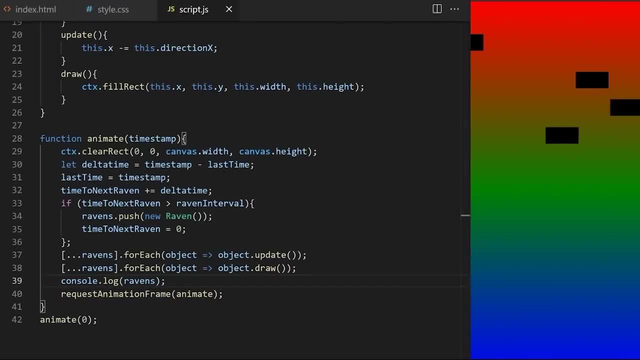 don't get skipped. easier way to discard objects we don't need might be using built-in array filter method. we will just run through the array call, update and draw for each raven, and then we will filter out ravens that have moved past the left edge of screen. 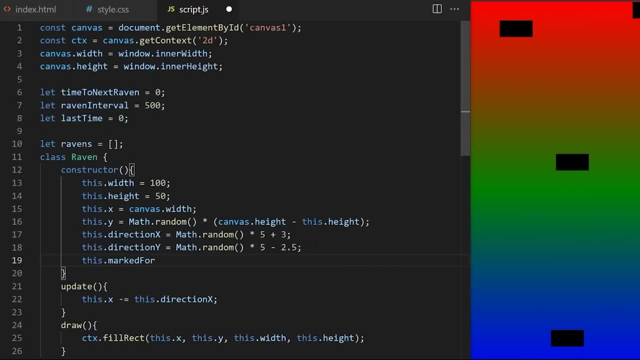 what does that look like in javascript? let me show you. i create a new class property called marked for deletion, and initially i set it to false. in update method i say: if horizontal x coordinate of this particular raven object is less than zero minus this dot width, meaning it has: 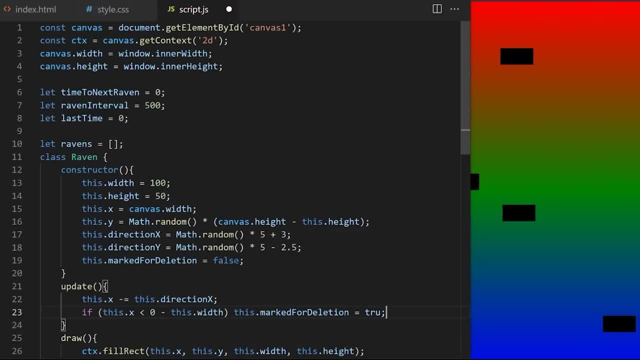 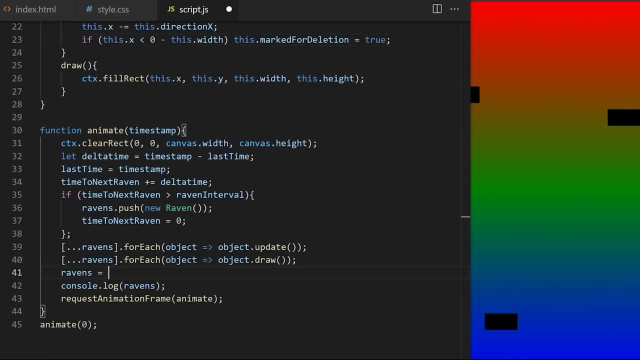 moved all the way behind the left edge. i set its marked for deletion property to true. inside animation loop: i take the variable that holds my ravens array from line 10 and i reassign it to a new array. that's why the initial declaration of ravens 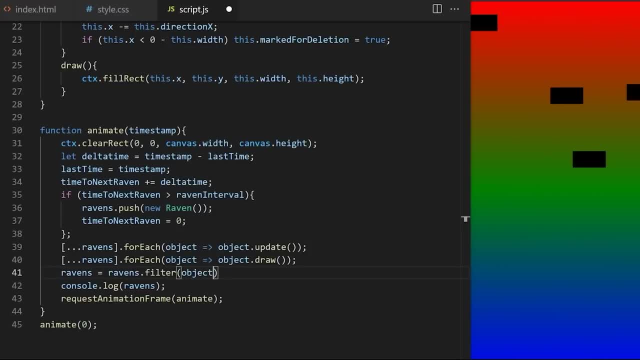 array needs to be a let variable, not const, because const variable cannot be reassigned and variable cannot be reassigned. it will be the same array, but objects that have marked for deletion property set to true will be filtered out. filter method creates a new array with all elements. 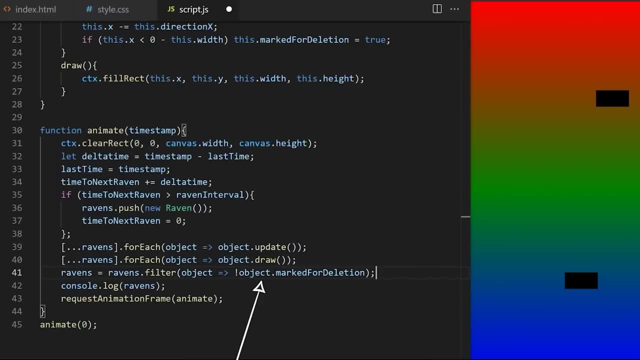 that passed the test implemented by provided function. so here i'm saying: take ravens variable from line 10 and replace it with the same array. but i want that array to be filled only with objects for which this condition is true. here we have a little bit of double negative. 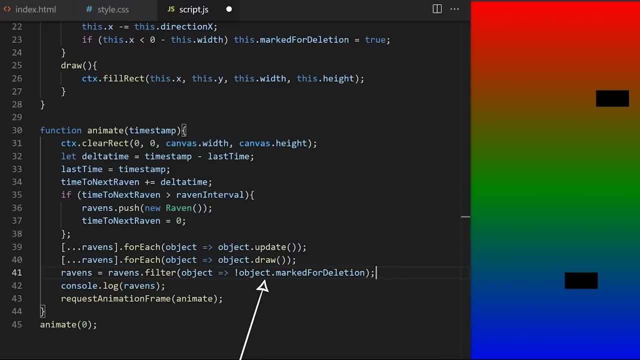 sorry, the test in my callback function wants marked for deletion value to be false. if marked for deletion is false, then this condition evaluates as true and this particular raven object will not be deleted again. and said very simply: take ravens array from line 10, delete everything in there and replace. 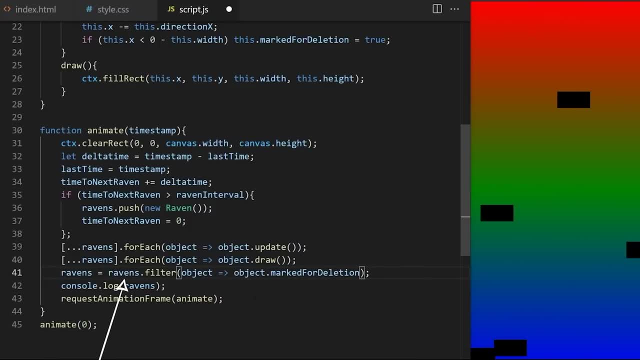 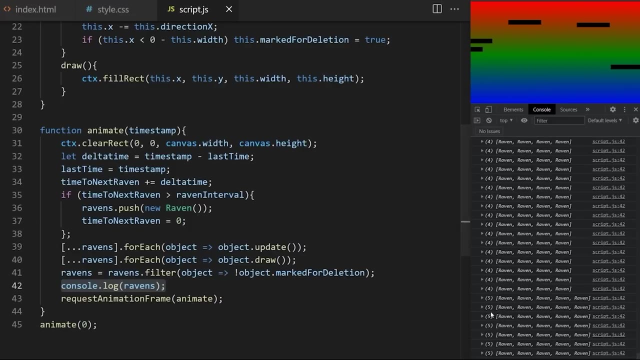 it with contents of the same ravens array, but only with those objects that have marked for deletion property set to false. exclamation mark here means false. since we are console log in ravens array on line 42, i can check in browser console and i can see that number of objects in 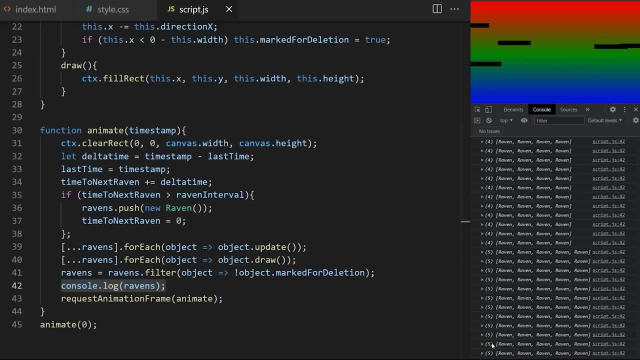 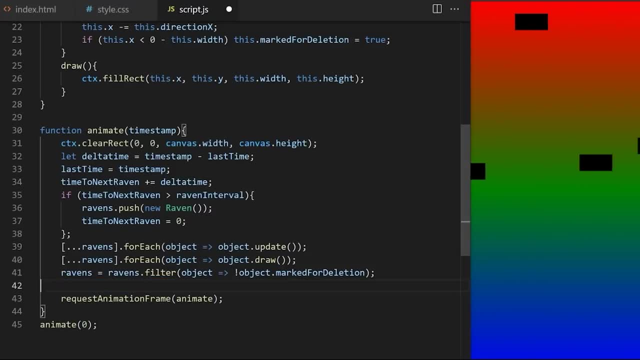 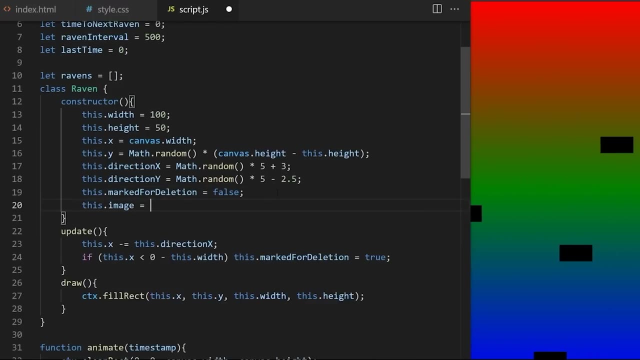 the array is between three and six. it only contains ravens that are active and visible on screen. perfect, i remove the console log. these ravens look a bit boring, just black rectangles. let's use animated sprite sheets instead. on my class, i create a new property called 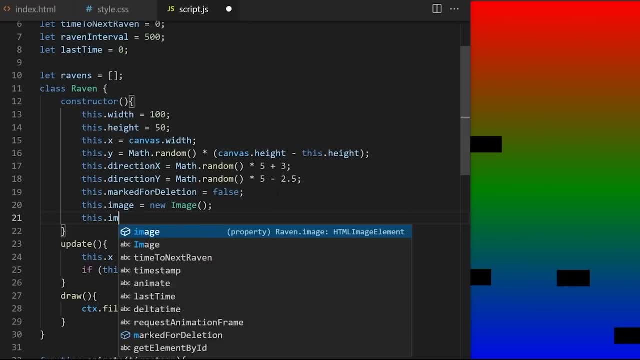 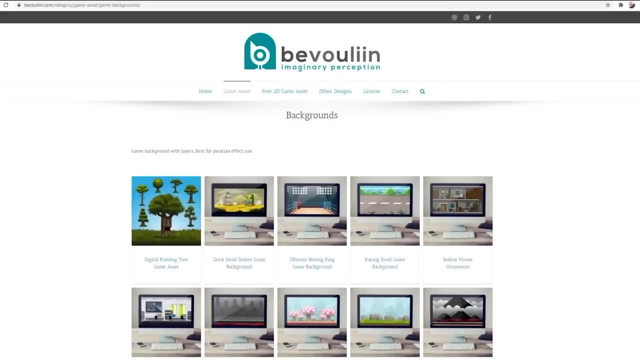 thisimage and i set it equal to new image. i set source on that new property and i set source on that new image as raven. png. art for this episode was made by this amazing artist. link to his website is in the video description. he also allowed me to share this. 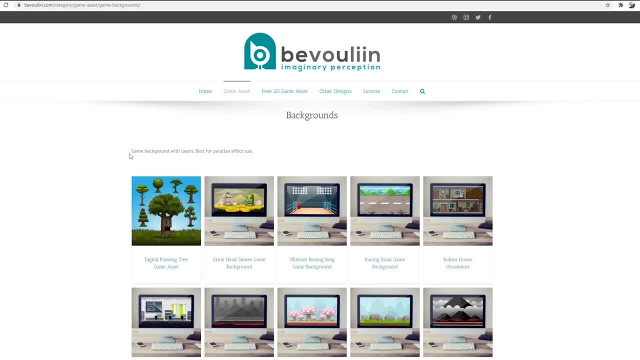 particular sprite sheet completely for free with my students, so you can download it along with all other project files in the description for more game art. check out his website and support him if you can. there aren't many good 2d artists like this and he's one of my favorites. 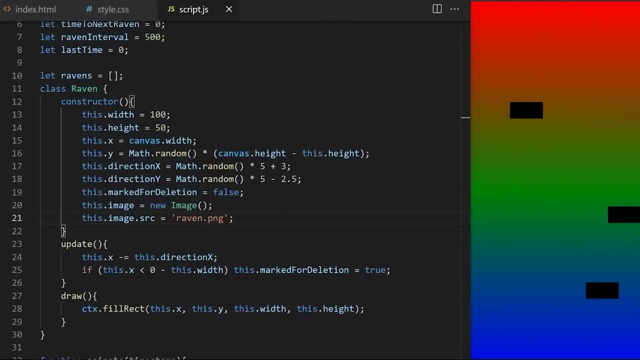 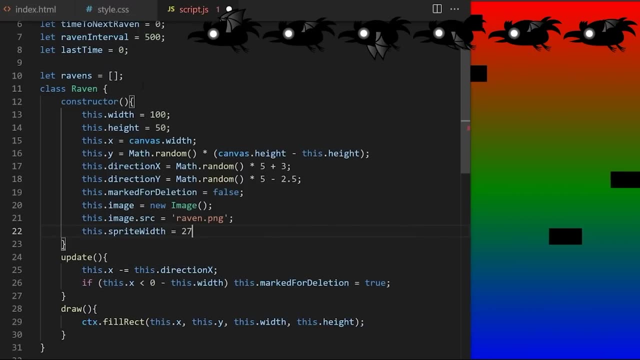 i try to buy his game art assets whenever i can. i will need a couple of helper properties here. thissprite width is width of a single frame in my ravens sprite sheet, in this case 271 pixels. if you are using a different sprite sheet, take its width and divide it by. 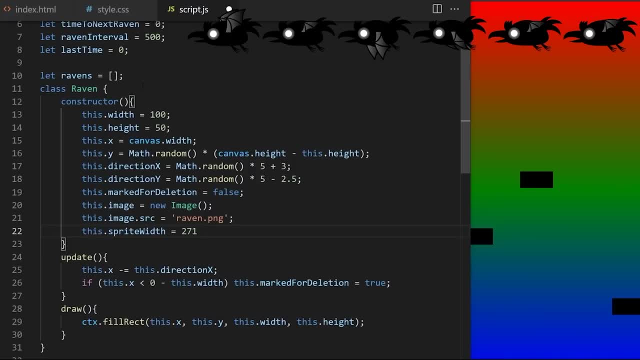 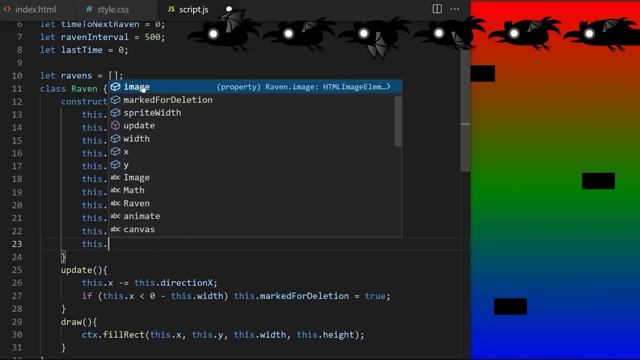 the number of horizontal frames. maybe it would be easier if you follow along with me using the same sprite sheet and then, when you understand the code and it's working for you, you can replace it. sprite height is 194 pixels and the height is 192 pixels. 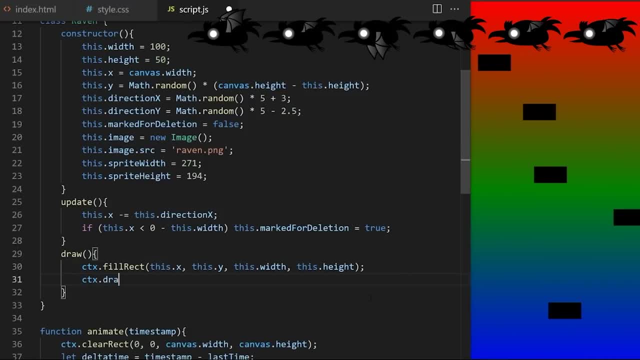 on line 31, inside draw method. i call built-in draw image method. it expects between three and nine arguments depending on how much control you want over the image you are drawing. minimum is three arguments: image you want to draw. so this dot image from line 20. 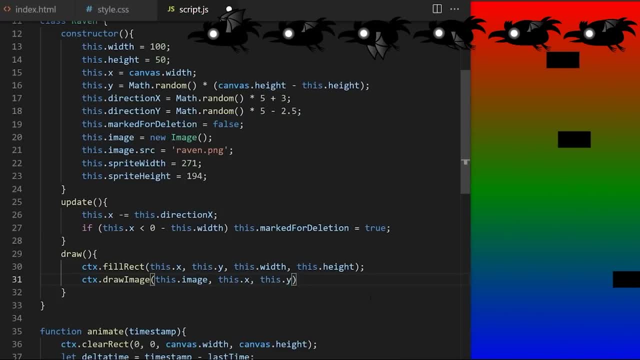 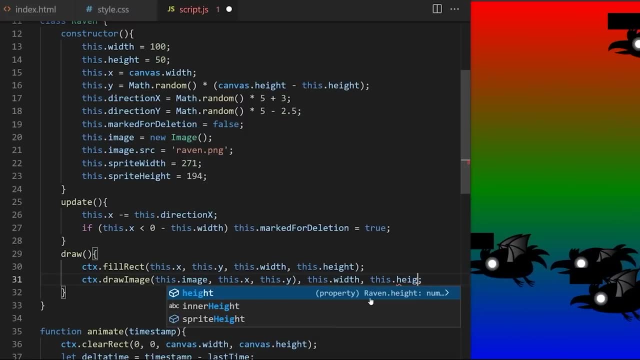 and x and y coordinates where to draw it now it's just simply taking the entire sprite sheet and drawing the whole thing at its original size. we can also give it optional width and height arguments which will scale it. i need to make sure my brackets and commas are correct here. 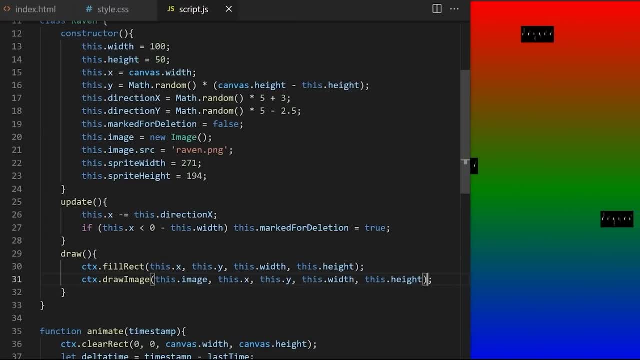 so now it's scaling the entire sprite sheet to fit inside 100 times 50 pixels. let's do stroke rectangle here so we can see it better. we can also give it a total of nine arguments. these additional four arguments will allow us to only crop portion of the. 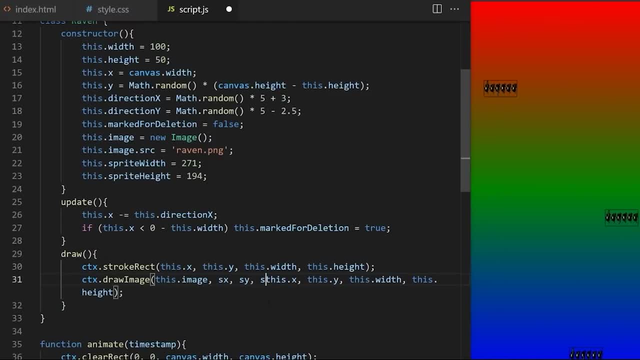 image: source: x, source y, source width and source height. so the longest version of draw image method takes nine arguments: image we want to draw x, y, width and height of area to crop out from the source. image x, y width and height of where to place that cropped out image on destination. 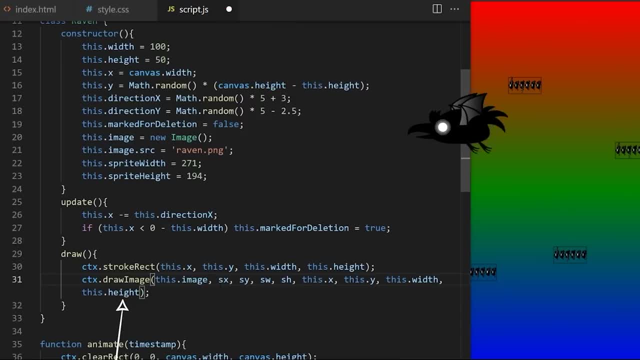 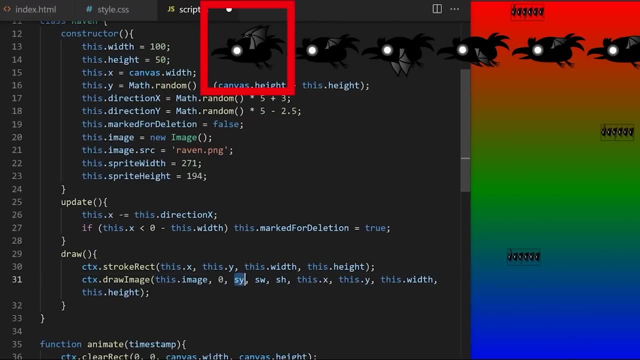 canvas. let's just crop out the first frame now. source x and source y is coordinates 0: 0. source width is sprite width and source height is sprite height. you can see our ravens are a bit stretched. it's because these initial width and height values are completely 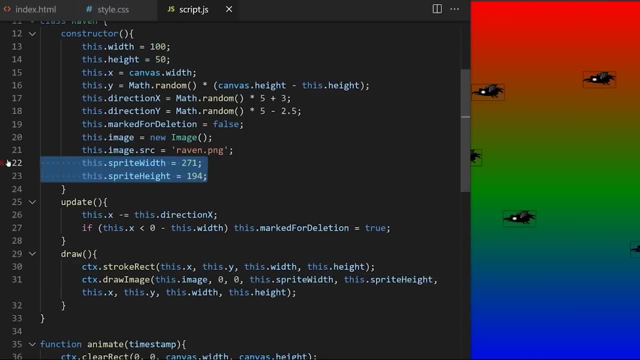 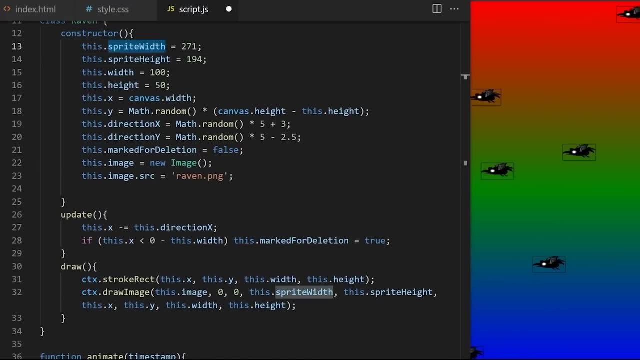 disconnected from the actual dimensions and aspect ratio of our sprite sheet. i move sprite width and sprite height up here so that we can use them to calculate values that come after. width could be, for example, sprite width divided by 2 and height could be height divided by 2. 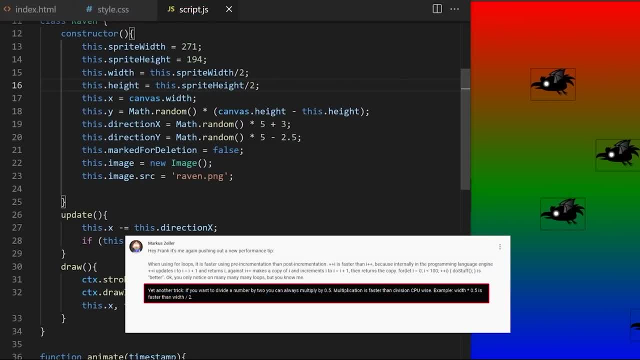 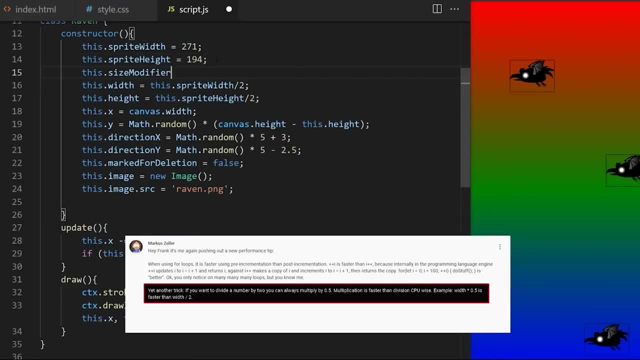 this works, but now all our ravens are the same size and, as my friend marcus says, multiplication is faster than division. so let's create a new property called size modifier, and it will be a random number between 0.4 and 1. now, instead of dividing it by 2, i will 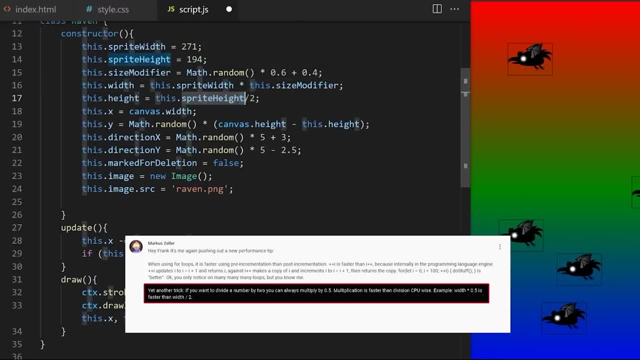 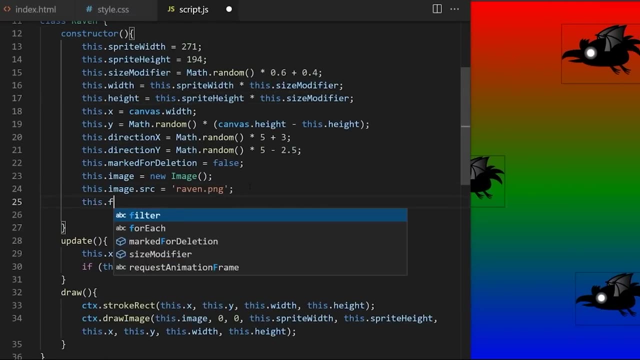 multiply width and height by this random size modifier value, which will make the ravens be different sizes while still preserving the aspect ratio. so no stretching. this dot frame is a number of frames in our sprite sheet counting from 0, so the initial value will be 0. 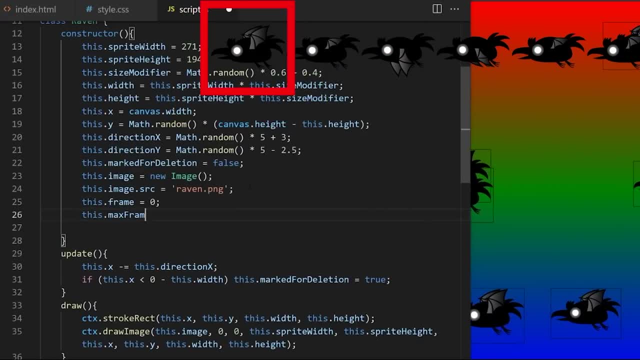 this frame. this dot max frame could be 4 or 5 depending on how you reset it back to frame 0. let's go with 4. maybe i will adjust my frame reset check to this value in a minute if this dot frame from line 25 is more. 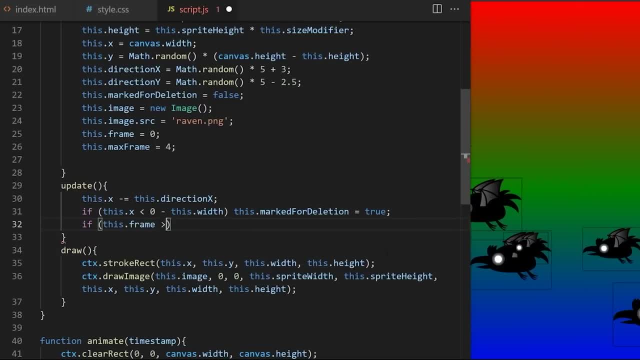 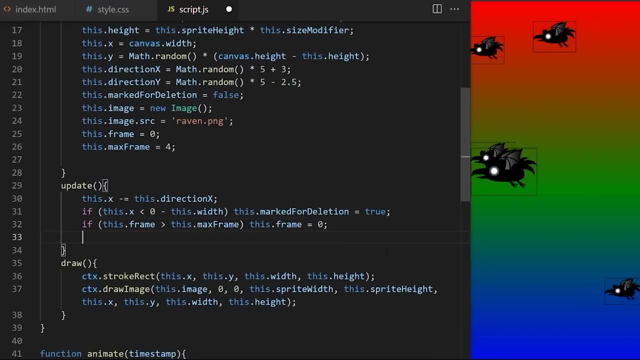 than this dot max frame. from line 26: set this dot frame to 0. now let's set this dot frame to 0, else increase frame by 1 to actually reflect this value on canvas. i replace source x argument on line 37 with this dot frame times this dot. 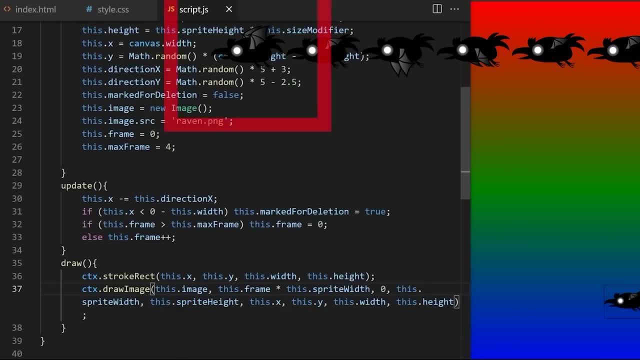 sprite width. so it will go 0, 1, 2, 3, 4, 5 and back to 0 as frame variable cycles. on line 32 all the ravens are flapping wings very fast and at the same interval. how do we speed up or slow down sprite animation: the? 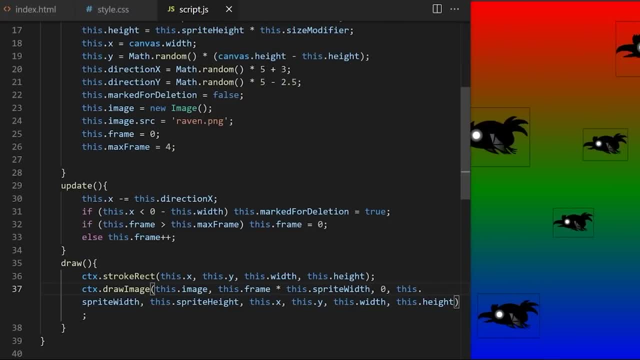 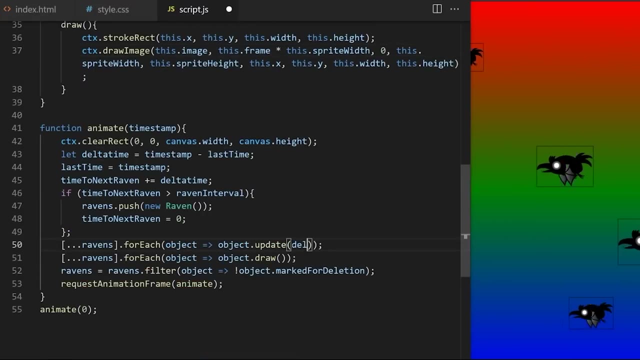 speed at which the next frame is served and how do we make sure it's consistent across all machines, on old, slow computers and new, powerful ones as well? we can do that by using delta time. we calculated delta time on line 43 inside animation loop. delta time is the. 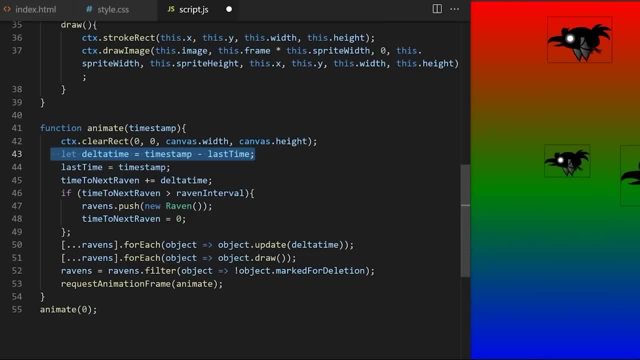 difference in milliseconds between last frame and current frame, and this value will differ based on power of your computer. some computers can serve frame much faster than others. since i already calculated this speed at which my machine can serve frames in my game, i will just pass a delta time as an. 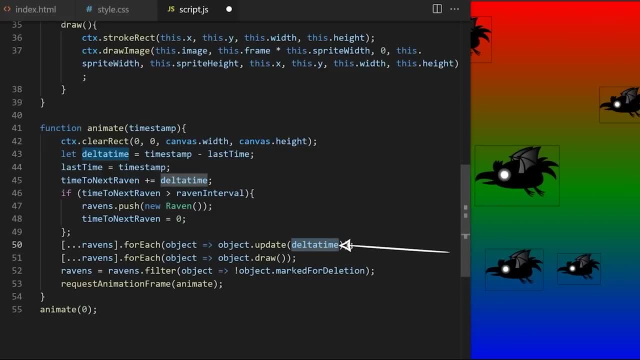 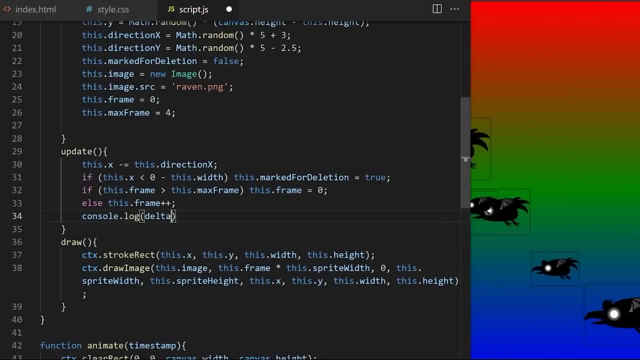 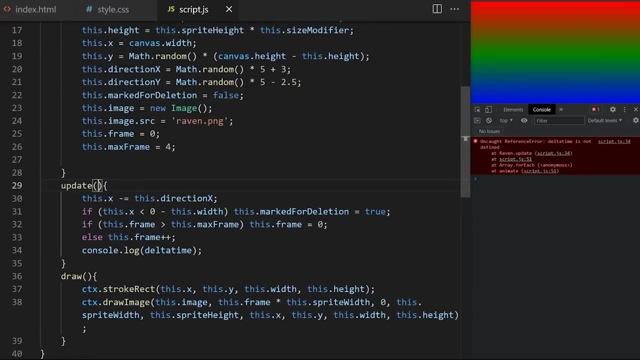 argument to my update method here on line 50. that way it will be available up here. let's test it. i console delta time. it won't be available until i passed delta time as an argument here as well. now the values are coming through, i will need a couple of helper properties: time. 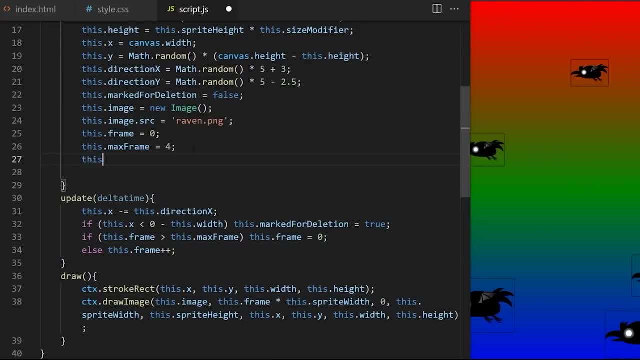 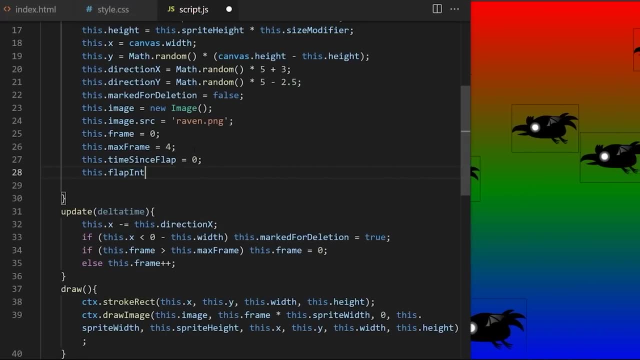 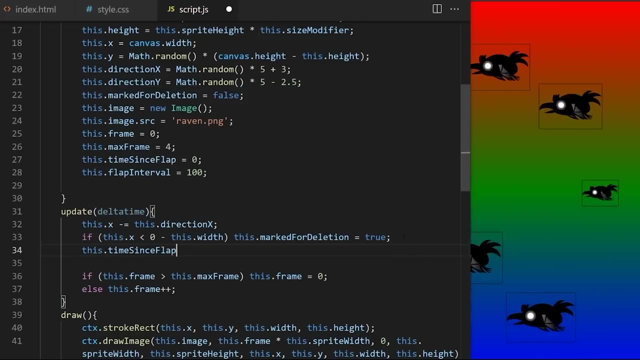 since flap will be zero at first, it will be growing by the amount of delta time until it reaches value in flap interval. then it will trigger next frame of sprite sheet and reset back to zero this dot time, since flap plus equals a delta time. remember that delta time is. 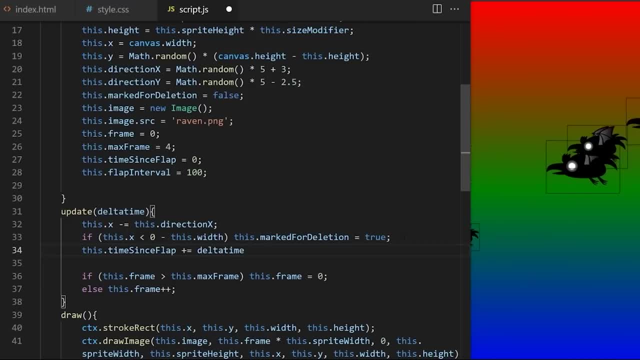 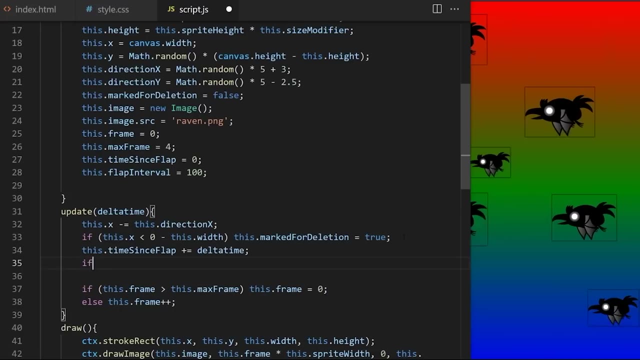 the amount of milliseconds between frames. so faster computers will have smaller numbers here. slower computers will have high delta time values. as a result it will reach the target value. at the same time, on slow and fast computers unifying animation speed across different devices, i say if this dot time since flap from. 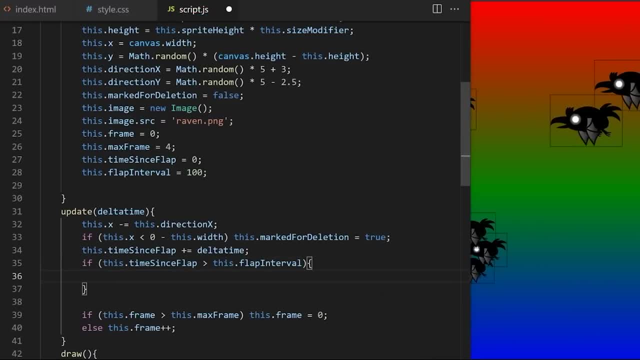 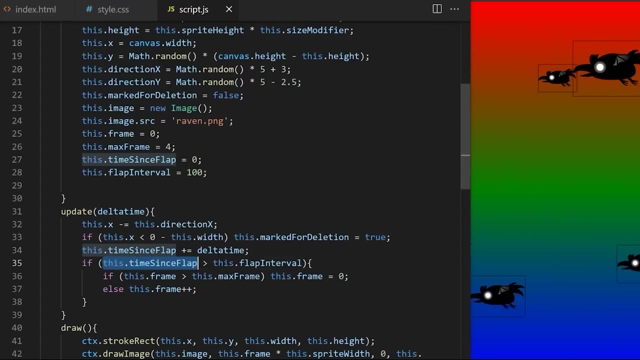 line 27 is more than flap interval from line 28. only then run this code that handles cycling through frames. for this to work, every time this condition is met and if statement is entered, i also have to reset time since flap back to zero so it can start counting again when to serve. 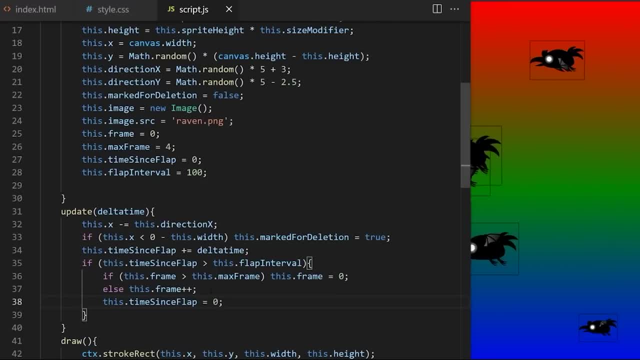 the next frame. now i can change the value of flap interval and you can see it changes the speed at which we cycle through frames in our sprite sheet. 500 milliseconds per frame is very slow. 5 milliseconds per frame is fast, faster than my computer can handle, since we know my computer can. 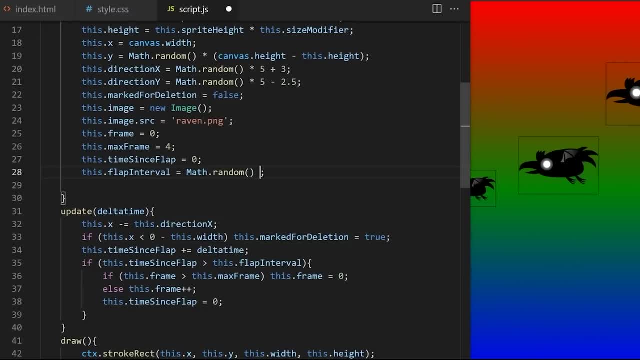 handle to serve next frame every 16 minutes seconds as maximum. i can also randomized flap interval so that each raven animates at a slightly different rhythm. random number between 100 and 200 feels too slow. how about a random number between 50 and 100? 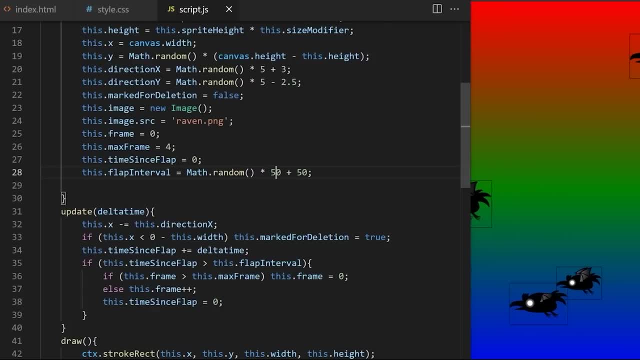 that feels better. quick recap: we are calculating delta time difference in milliseconds between last frame and current frame. the value of delta time will be different on slow and fast computers to make sure we have consistent time in across different machines. we have time since flap variable that increases by the value of. 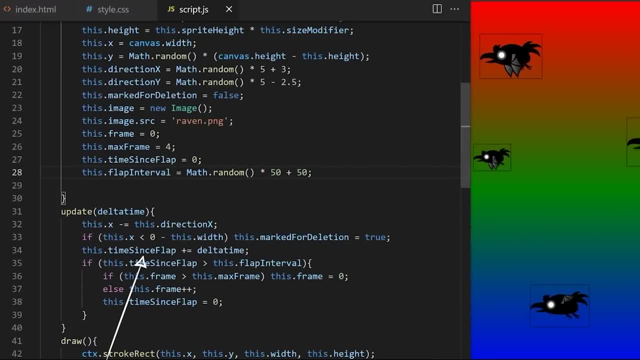 delta time per each frame until it reaches target value in flap interval. then it serves the next frame, resets back to zero and starts counting again, preparing to serve the next frame. ravens are flying in straight lines from right to left. i also created a direction y property on line 21. it's a random. 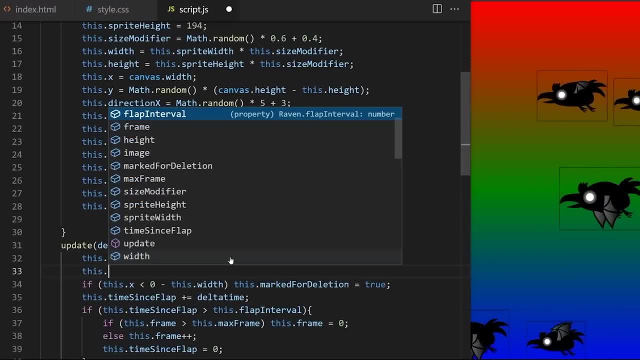 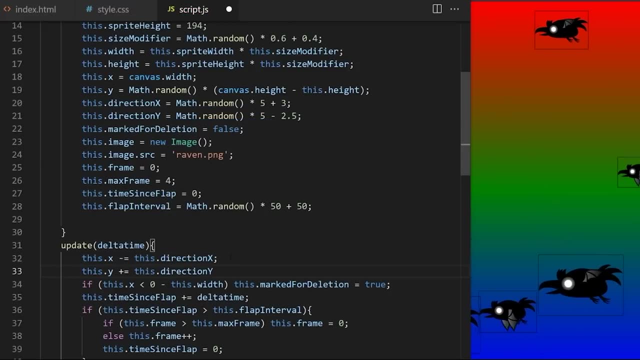 number between minus 2.5 and plus 2.5. so some ravens will move up and some will move down in negative or positive direction along vertical y-axis. based on this value inside update method, i say this: dot y plus equals this dot direction y. now you can see some. 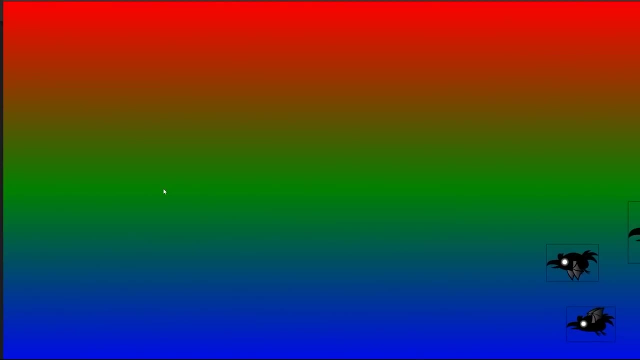 vertical movement, it's now a little bit harder to target them, making our game more difficult for players. one thing i don't like now is how they disappear behind the top and bottom edge. i want them to move all the way across the screen and when they touch bottom or 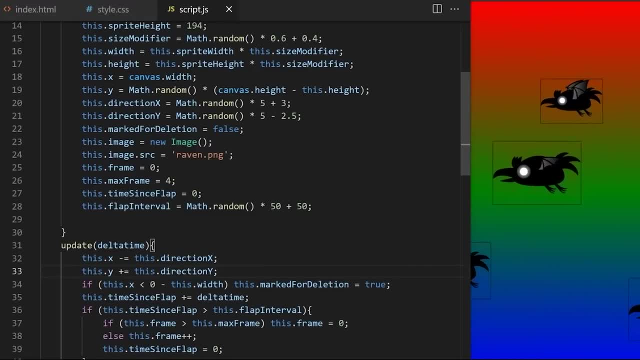 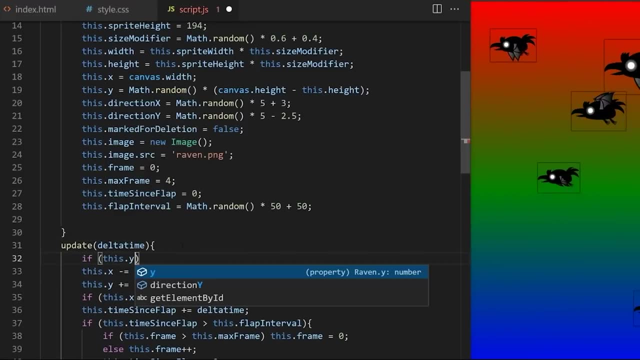 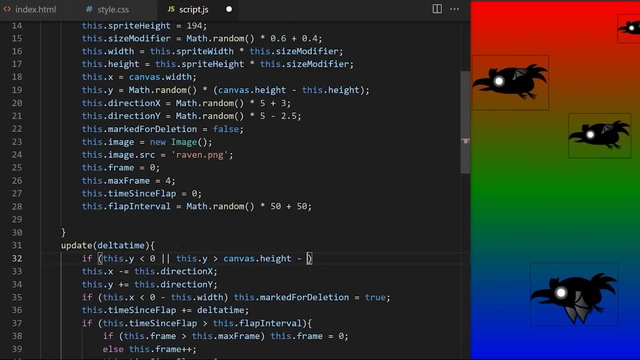 top edge of game area. i want them to kind of bounce and reverse their vertical movement to the opposite direction. i do that with an if statement. i say if this dot y is less than zero, or if this dot y is more than canvas height minus this dot height. 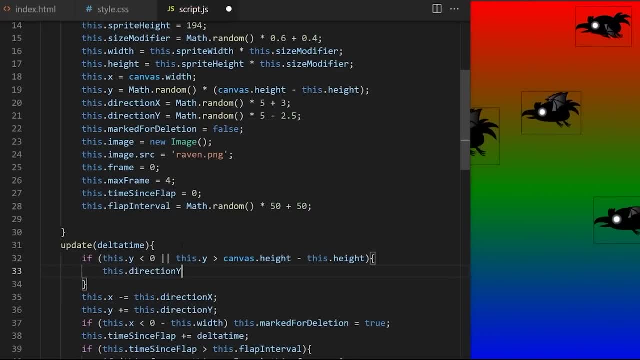 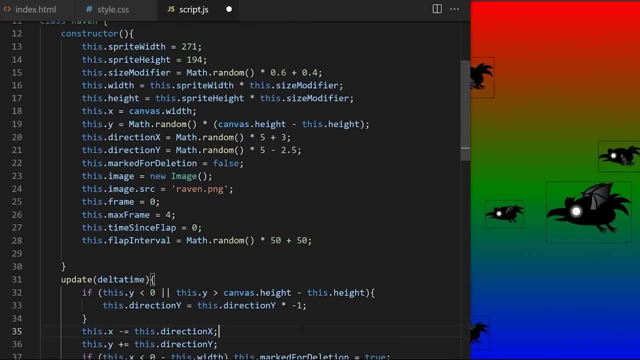 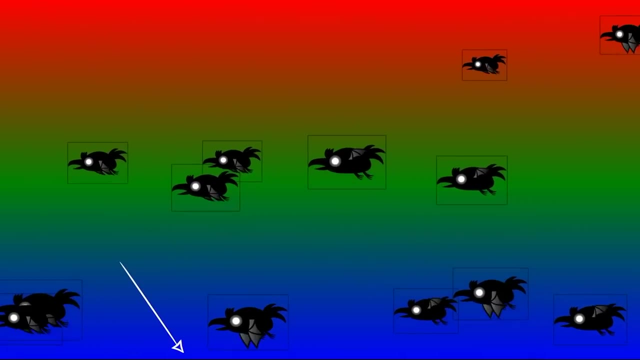 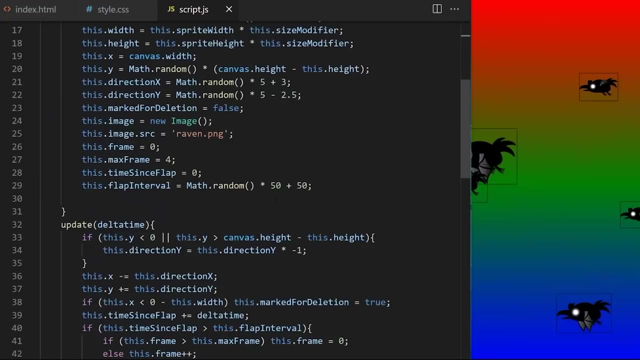 set their direction property for this from line 21 to its opposite value. this the direction y times minus one. now they just bounce when they reach edges of the game area. let's draw score. i create a lead variable called score and i assign it to zero initially. i create a custom. 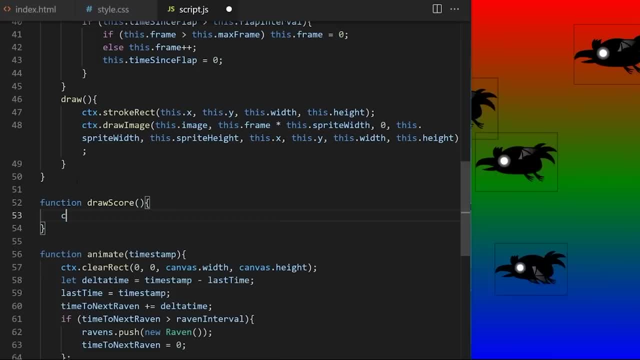 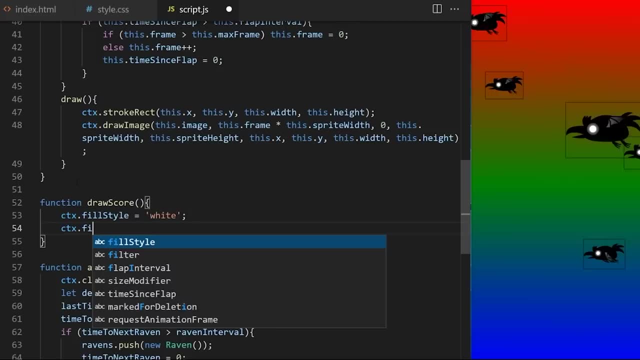 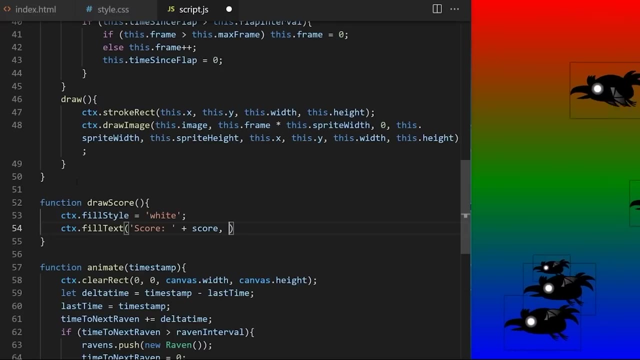 function called draw score. inside i set fill style to white. i want white number, i want white numbers. i call built-in fill text method. inside i will hard code string, score, colon, space plus score variable. we just declared, and i wanted a drone on canvas at coordinates 50, 75, for example. 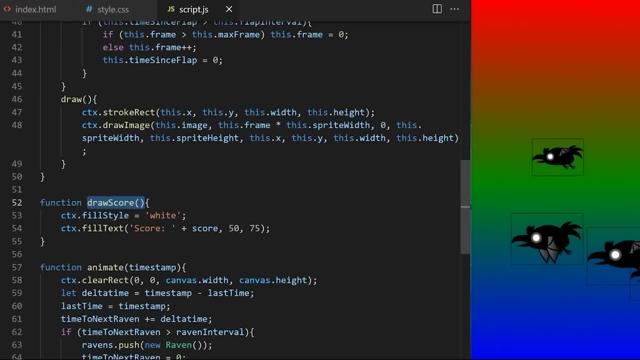 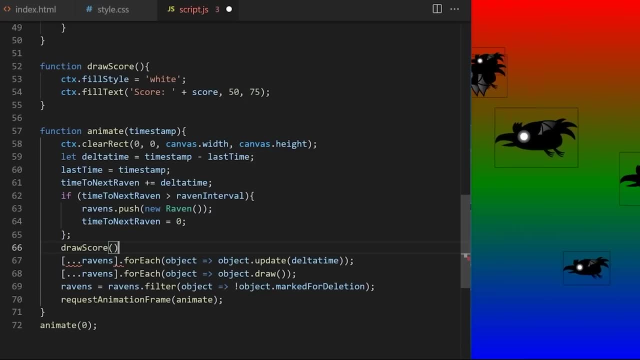 now i just call draw score from inside my animation loop. keep in mind, since we are drawing everything on the same canvas sequence in which you call this layer, this will affect how our game is layered. i want score to be behind ravens, so first i draw score, then i draw. 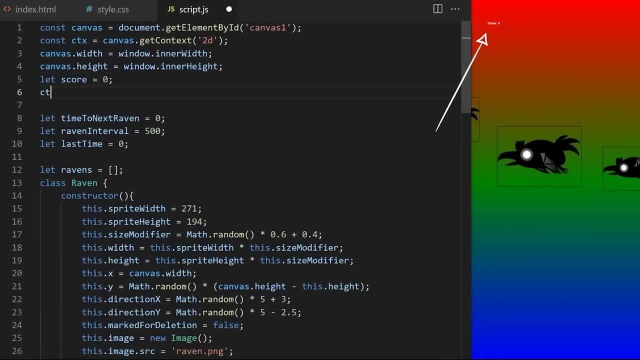 ravens. it's very small, so let's set a global canvas font to 50 pixels. impact: now it's easier to read. i will play with it a bit. i can use canvas shadows here, but i can also just draw the same text again at slightly different coordinates. 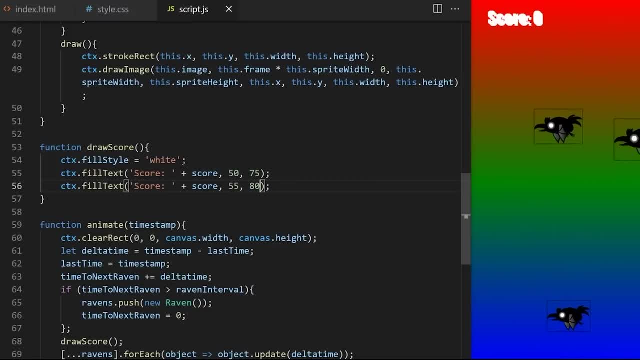 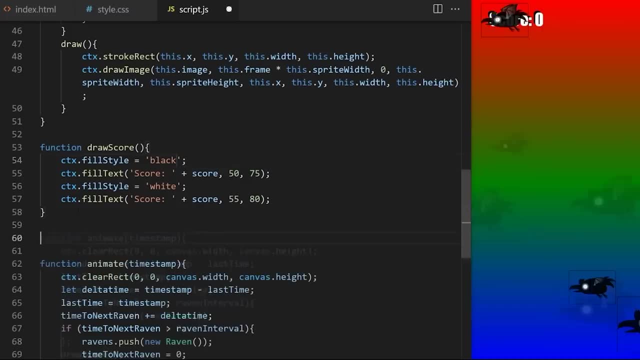 for example, 55 and 80. the first layer will be black. the second layer will be white. in the game we will have to click ravens before they disappear. behind the left edge of screen i create an event listener for click event callback function on. event listener has the: 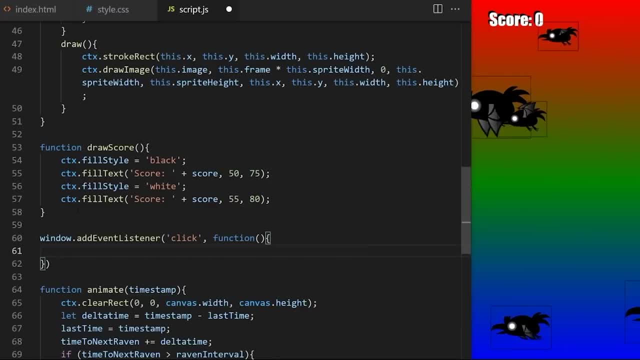 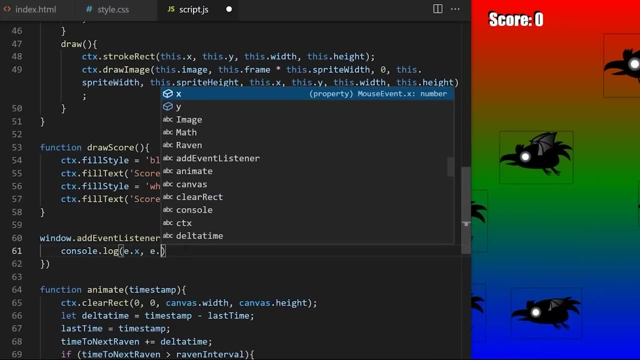 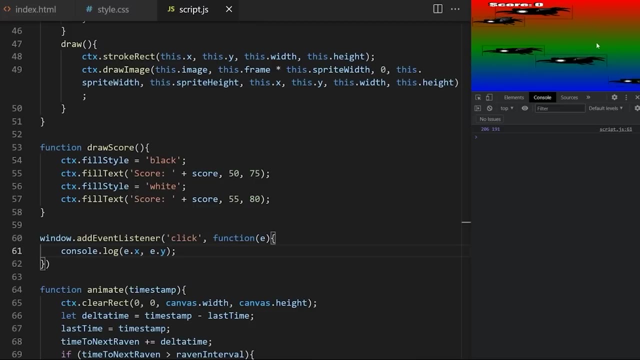 default access to this event object. i assign it variable name, for example e. it contains information about the click event that happened, for example its x and y coordinates in relation to viewport. if i consoleexe and ey, i get coordinates of my click whenever i click somewhere in the game area. i. 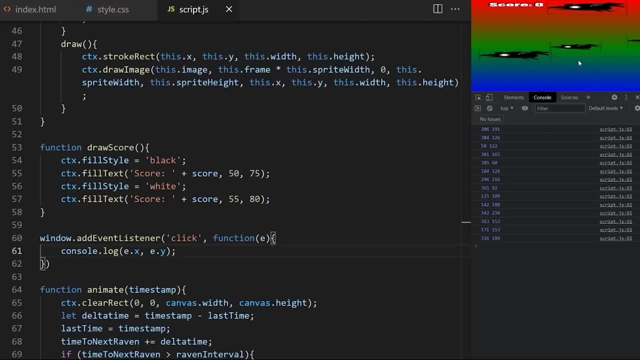 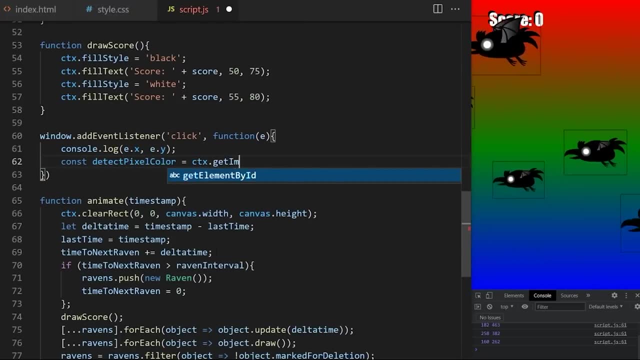 promised we would do collision detection by color today. to do that, we first need to know what color is the pixel we are clicking on. i create a custom variable. i call, for example, detect pixel color. it will be equal to built in get image data method. get image data simply scans area. 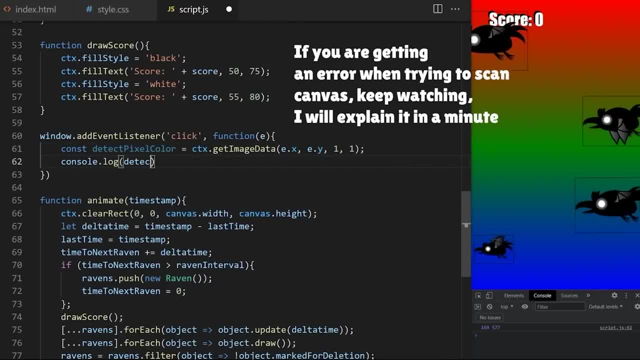 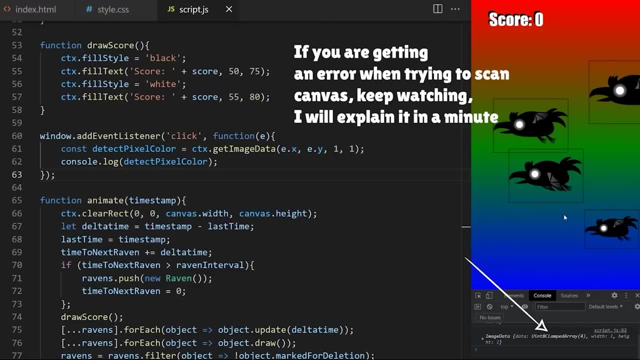 of canvas and returns an array like object called uint8 clamped array. it's a simple data structure full of unassigned 8-bit integers. it's clamped, which means it can contain only integers, whole numbers, between a certain value range, specifically between 0 and. 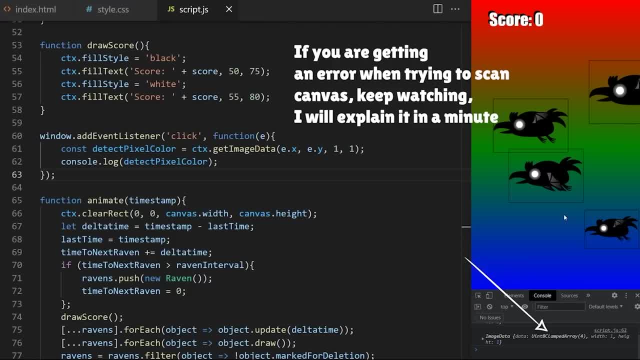 255. let's scan canvas and inspect what it gives us get image. data needs four arguments: x, y, width and height of area we want to scan. i want to scan just one pixel we click on with mouse, so coordinates of this click event will be scanned: e dot x, e dot y and width and 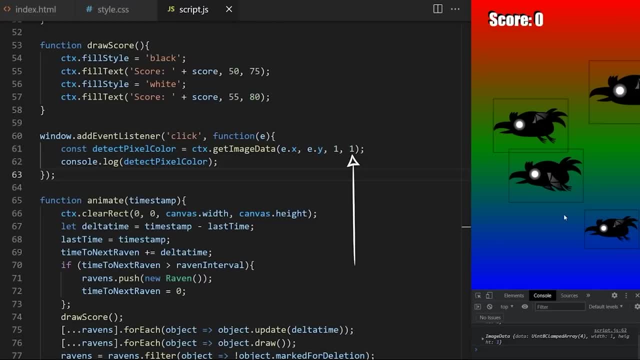 height of scanned area will be just one pixel. we want pixel perfect precision here. okay, let's just console lock this variable to see in what format get image data gives us the pixel color, to make sure we understand how it works. if you are getting error at this point, keep. 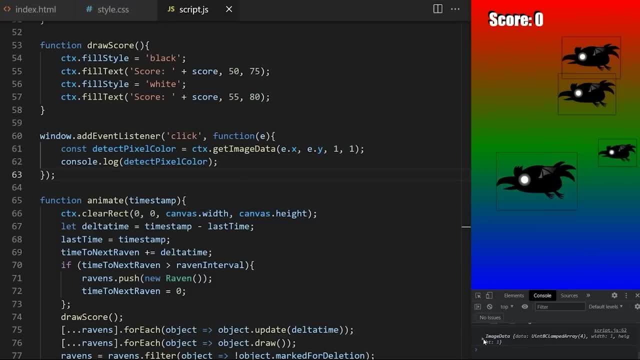 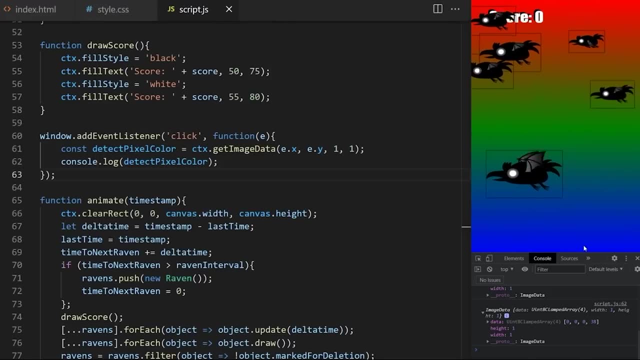 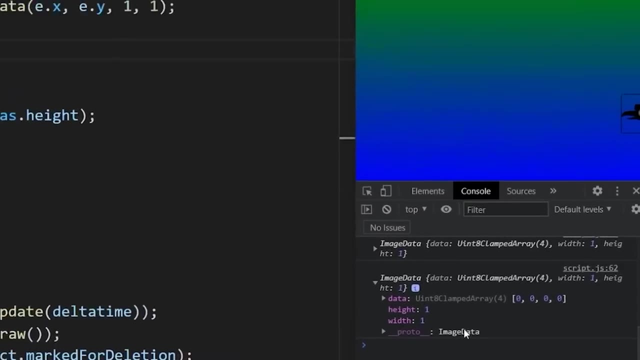 watching. i will explain it and i will show you how to deal with it. now, whenever i click somewhere on canvas, get image data scans, area of one pixel directly under the mouse, click and it gives us this image data object. this auto-generated image data object contains three main properties: data. 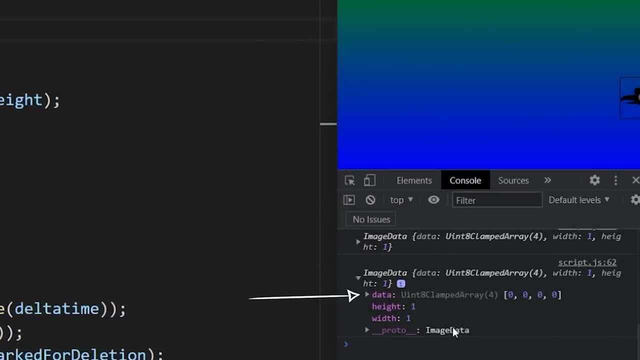 property, which is an array. currently it has four numbers inside and with an height of scanned area, in our case, one pixel. the way color data is structured here is that each four elements in this data array represent one pixel. specifically, it's red, green, blue and alpha value. if you use CSS, you know that. 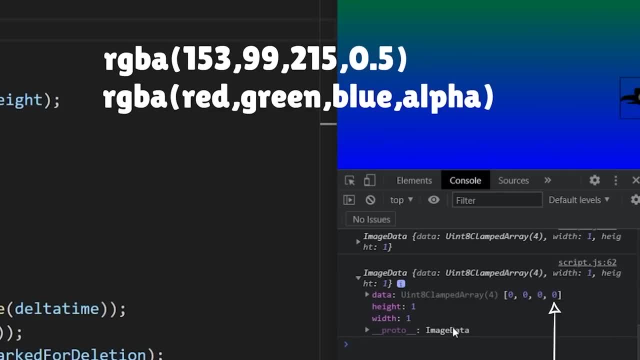 any color can be created by combining a certain amount of red, green and blue. the only difference between CSS rgba declaration and this is that in CSS, opacity is a value between 0 and 1. here, opacity alpha is also a number between 0 and 255. 0 is transparent, 255 is fully. 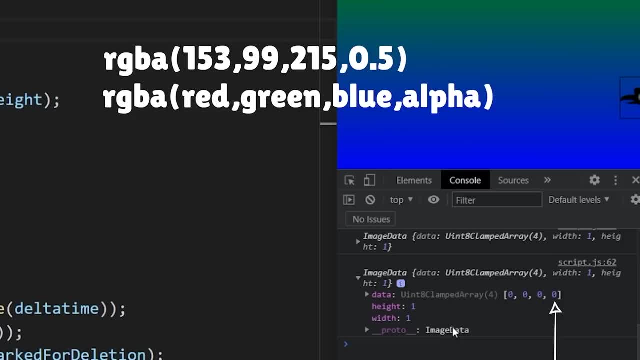 visible here, for example. you can see I clicked and it gave us 0, 0, 0 for red, green and blue and 0 and blue for red and 0 for alpha. it means we click somewhere in the empty area. keep in mind that canvas is just the Ravens and 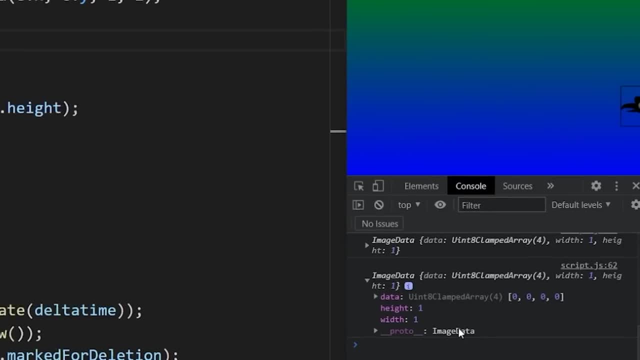 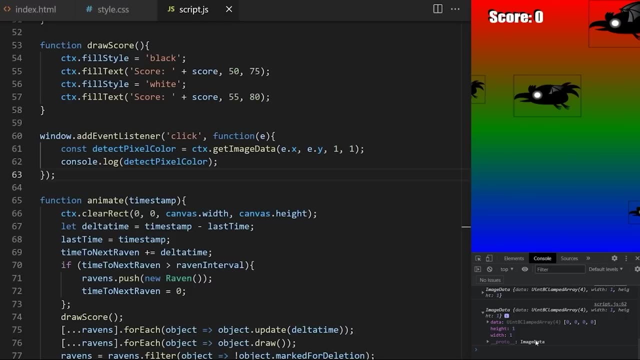 score. the rest is transparent. rainbow colors you see are on the background and are applied to body element. with CSS. we are calling get image data on CTX variable, so it is just scanning that particular canvas element. it doesn't see anything else. some of you might be get. 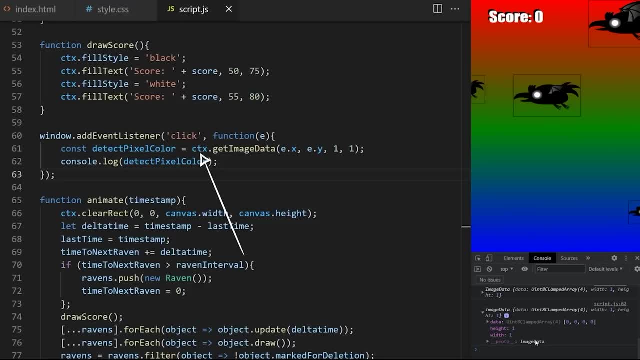 an error when you click on canvas and try to run get image data on it. we are drawing sprite sheets, our Raven images, on canvas. in some browsers you won't be able to call get image data on the same canvas where you draw images. it will give you an error that says something. 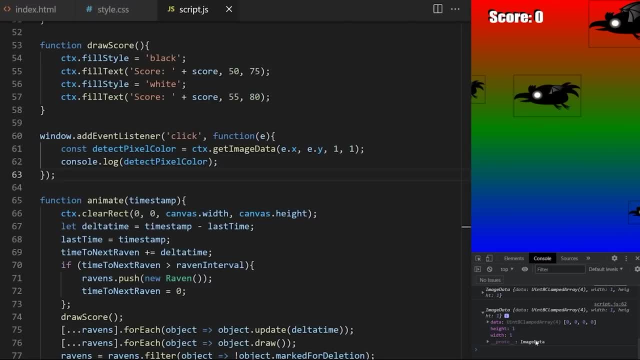 like canvas, was tainted by cross-origin data. if you are running your code locally, most likely you see that error. I'm using local server, so I'm not getting that error right now. it's a security measure related to cross-origin resource sharing. apparently there could be viruses hidden in some images and by 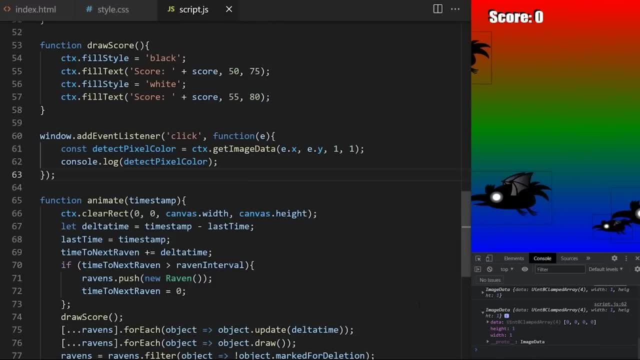 scanning that image with get image data, you could expose yourself to that virus. there are many ways to get around this problem and scan canvas without exposing yourself to any potential risks. in our case, it's simple. let me show you, but first I will assign a differently colored hitbox to each Raven. so I want 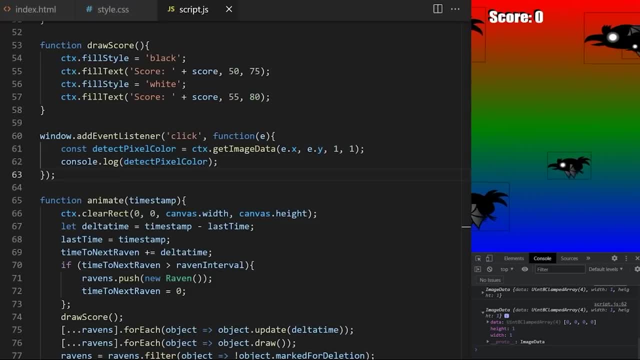 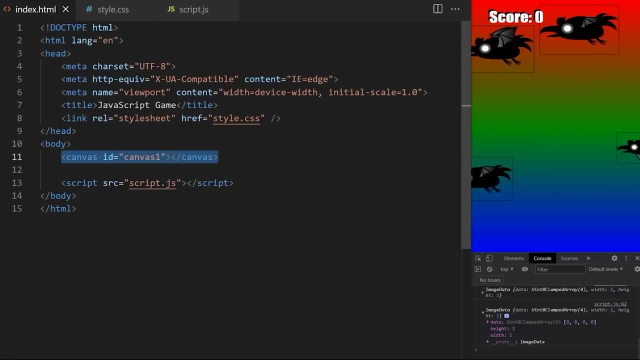 one canvas that has only these hitboxes and no Ravens, because when I click it I want to get color of that particular hitbox, not of the black Raven. if I create a secondary canvas and I use it just to draw these hitboxes and draw a new canvas and no images, it won't give. 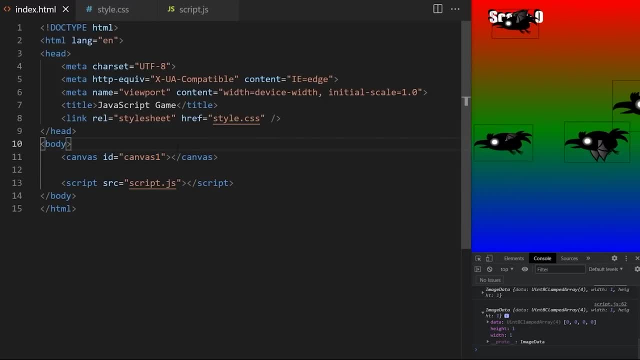 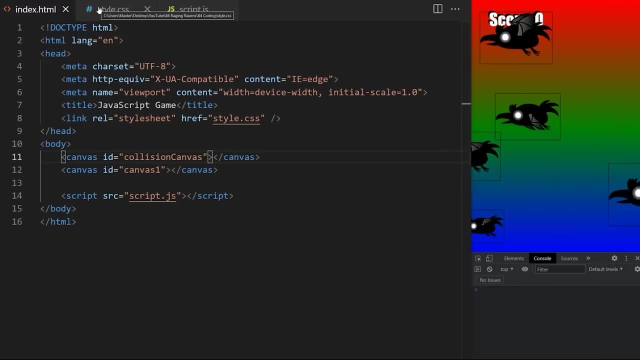 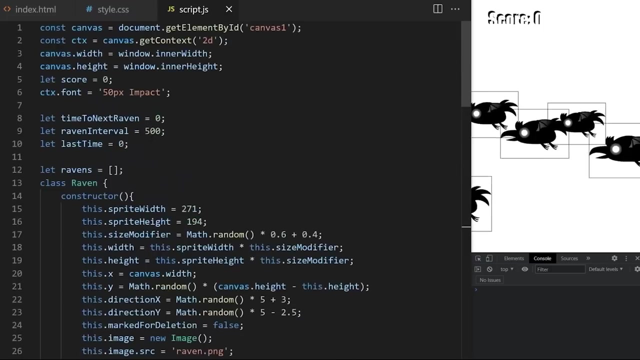 me: tainted canvas error. I will explain more as we write it in index HTML. I create an additional canvas with an ID of collision canvas, install CSS. I comment out rainbow background for a moment so that it's very clear what we are doing, the same as I set up the first. 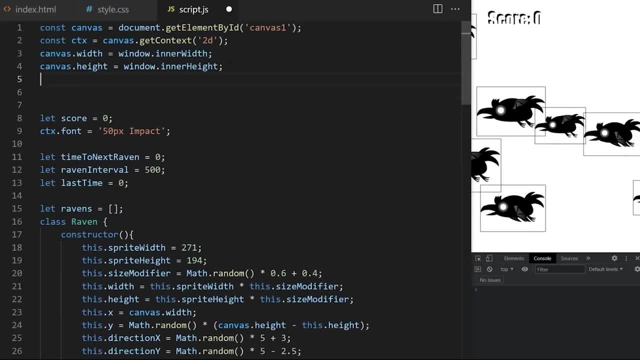 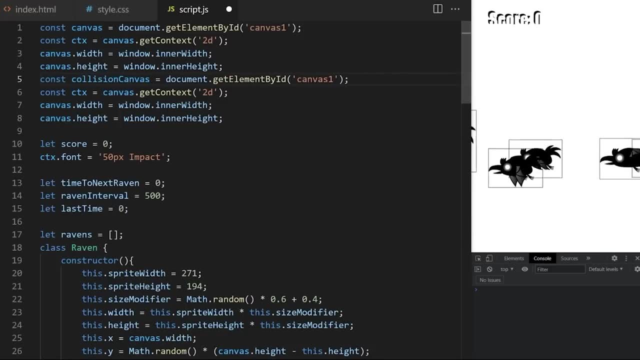 canvas. I will also set up this new collision canvas. be careful here. I always make mistakes and typos when assigning multiple canvases like this. for some reason- I don't know why- constant variable called collision canvas is document get element by ID: collision canvas. collision CTX, which is 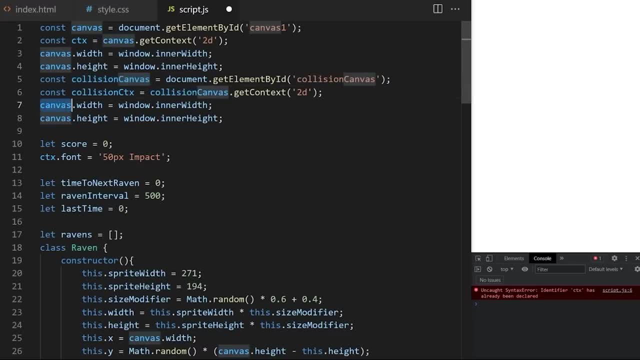 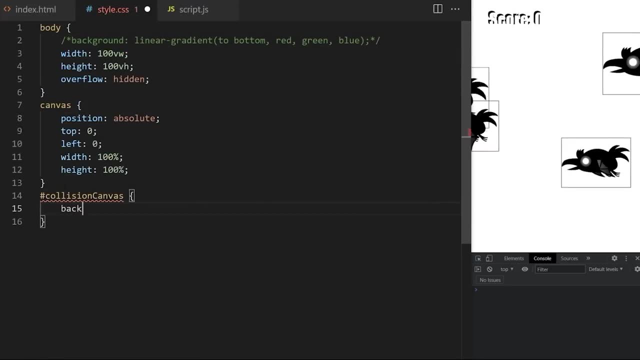 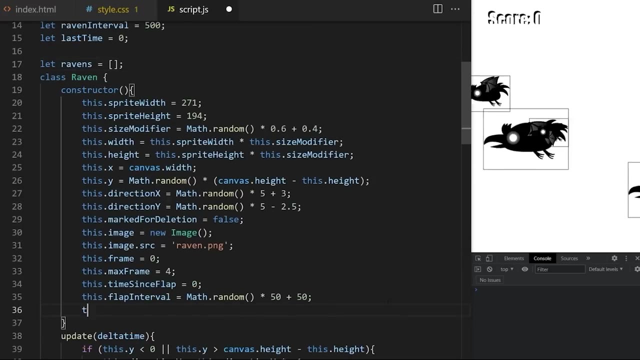 context is collision canvas dot. get context 2d. I also set collision canvas width and height. just to check, I give it red background. yes, it's covering the entire browser window. perfect. on my Raven class, I create a property called random colors at the point where each Raven is. 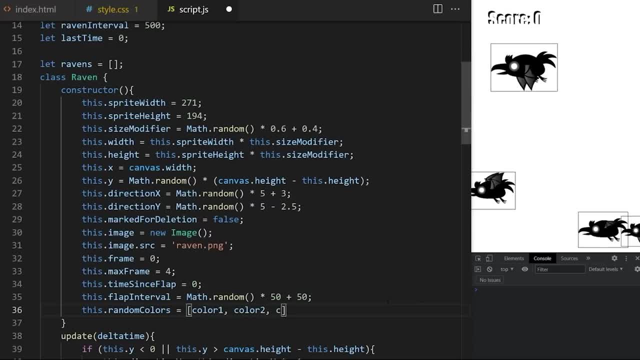 created. I want to roll the dice and randomly give it red, green and blue color value. we know that color values can be in a range between 0 and 255, so red will be math at random times. 255. like this, it will give us decimal points. 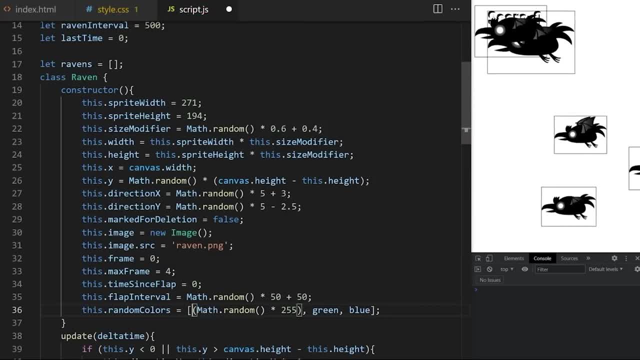 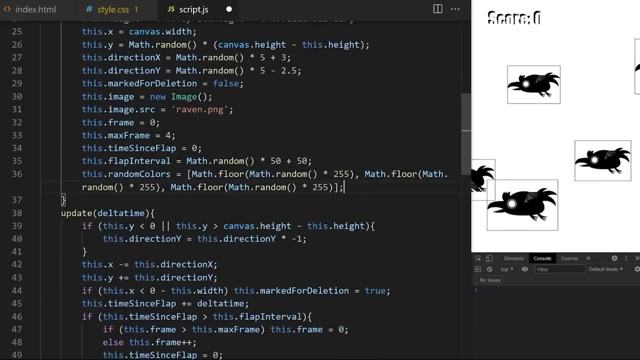 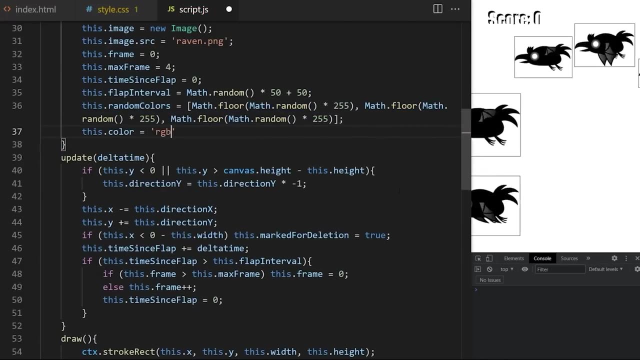 I need only integers here, so I wrap it in math dot floor. I do the same thing for green and blue. now we have three random values in this array assigned to each Raven object. I create one additional property called this dot color, and here I concatenate RGB, a color declaration. 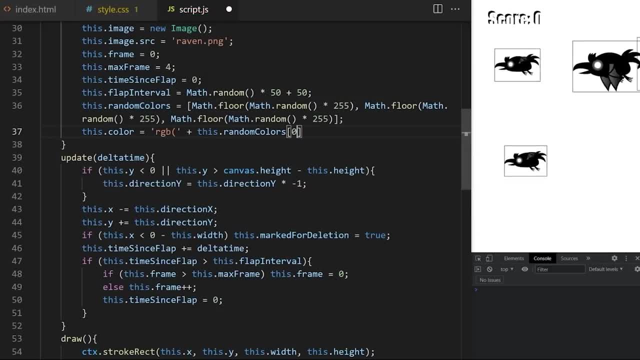 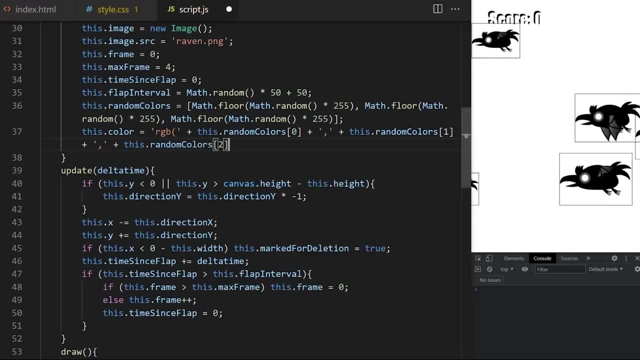 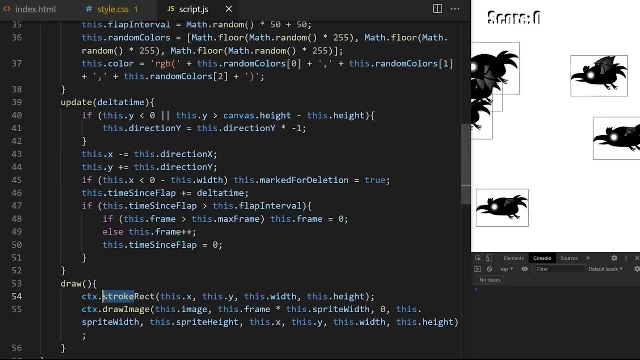 using these values: red is random colors, index 0, green is index 1 and blue is index 2, plus closing bracket like this: to use this color: I declare fill rectangle on line 54 and I set fill style to this dot color from line 37. 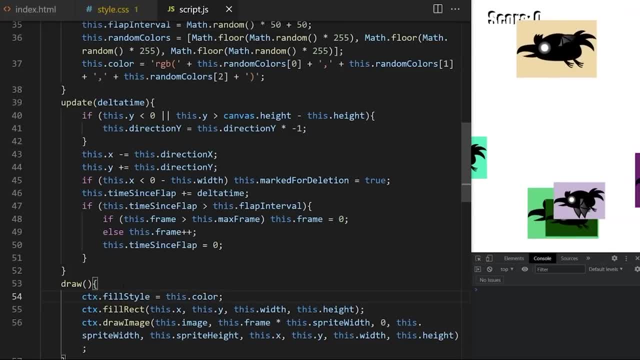 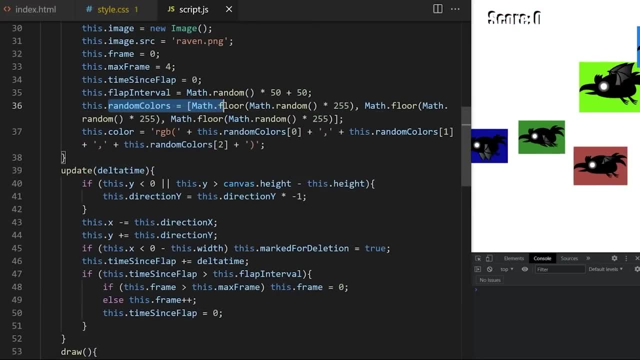 now, each Raven has a random red, green and blue color assigned when it's created by our class constructor and we use these three values to create RGB color for its hitbox. hitbox means collision detection area and in our case it's the colored rectangle around each. 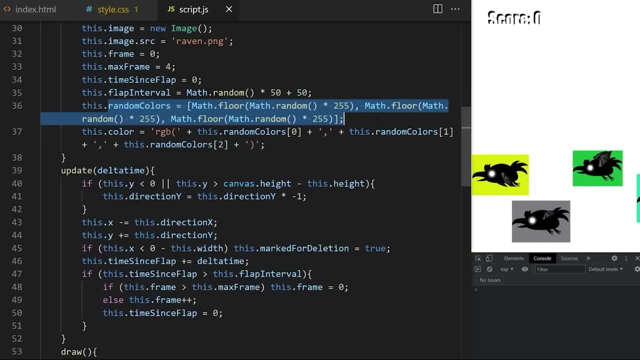 Raven. we can also do much more complex shapes and still get pixel-perfect collision detection. but for purposes of this tutorial, rectangles are fine. I don't want to complicate things too much. this tutorial is to help you understand the technique. so now each Raven has an. 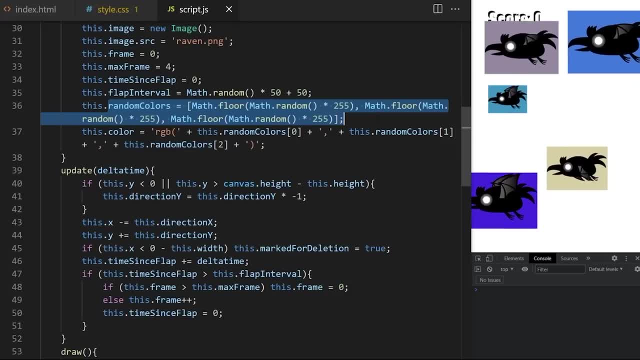 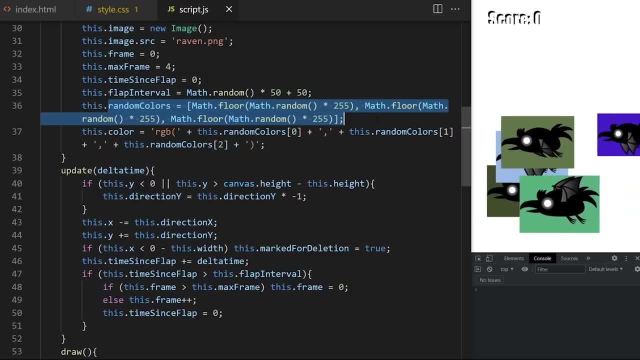 array of three random values between 0 and 255 and these values are used to draw its hitbox. we will use these values kinda as a unique password for each Raven. we click on canvas, get RGB value of that pixel. we clicked on using get image data method and we compare them. 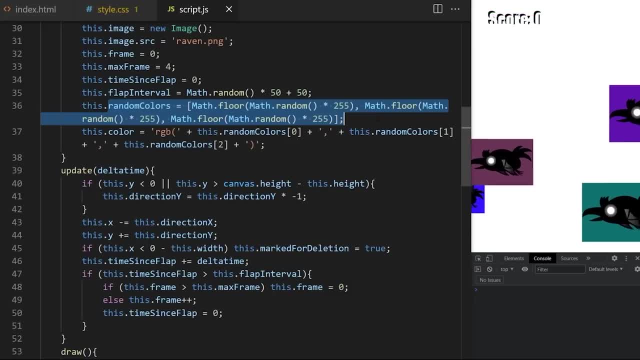 with this random colors property. if they all match, we know we click on this particular Raven. this technique has one downside: there is a very small chance that there will be two identical colors generated next to each other, but since we do random number between 0 and 255. 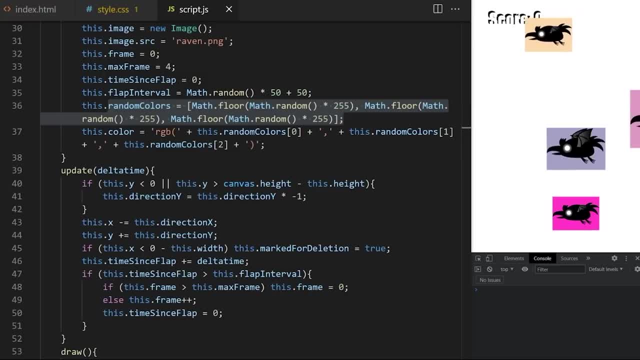 three times and we only have between 3 and 7 active Ravens on the screen at any given time. the chances of that happening are astronomically low. if we have any math experts who can run the numbers, let me know in the comments. it will be one. 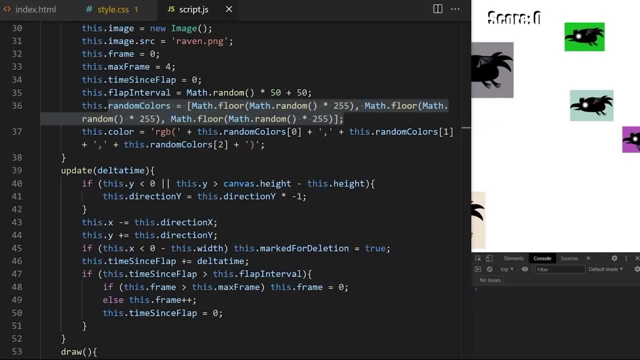 in millions, possibly billions. now I told you what I want to do. what does that look like in JavaScript? before we write collision code, there is one small thing: layers. I want big Ravens to be up in front and small Ravens to be behind, to create a sense of depth and correct the 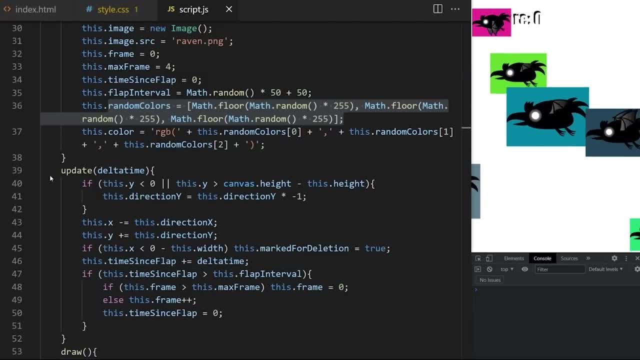 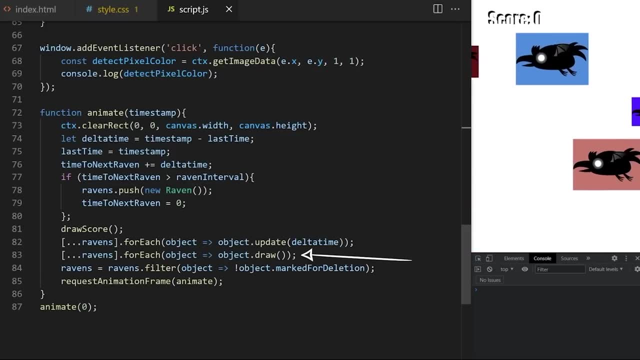 draw order in a 2d space. right now, sometimes you see smaller Ravens up front because they are drawn here on line 83, based on the order at which they were pushed into the array on line 78. I don't have to sort them for every animation. 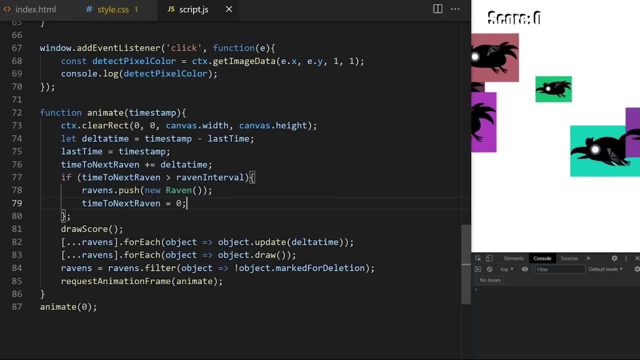 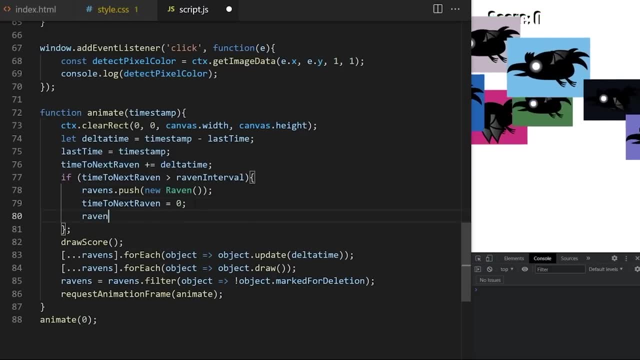 frame only every time I push new Raven to the array. I want to sort out all objects in the array by size. I use built-in array sort method. sort method will simply reorganize order of elements in the array, their indexes, based on provided check in a callback function. it will run. 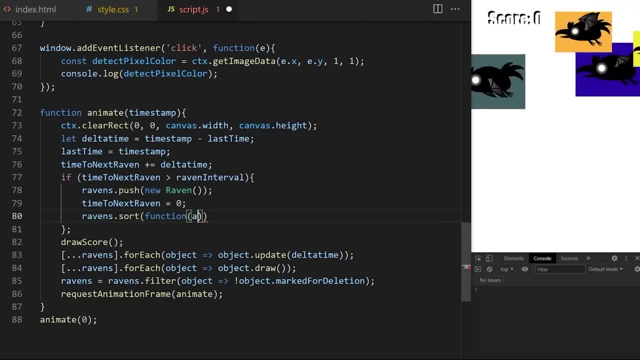 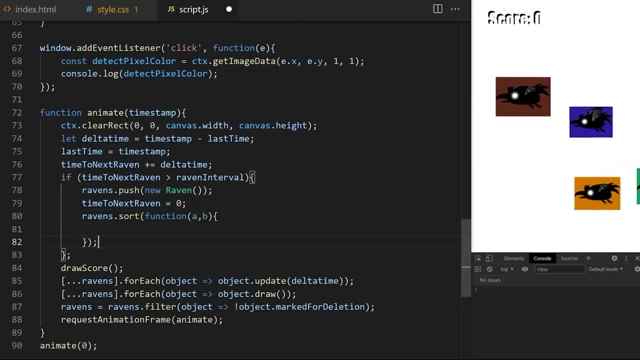 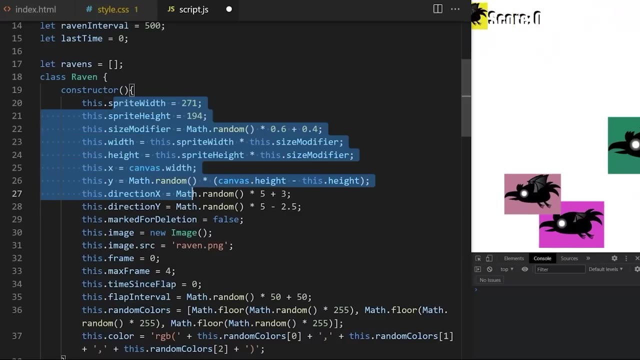 through the array and compare every element against every other element and sort them in ascending or descending order. ascending order is default. it will run over my Ravens array and use these A and B variables for each object. I can choose many different properties to sort them by. today I will choose width. 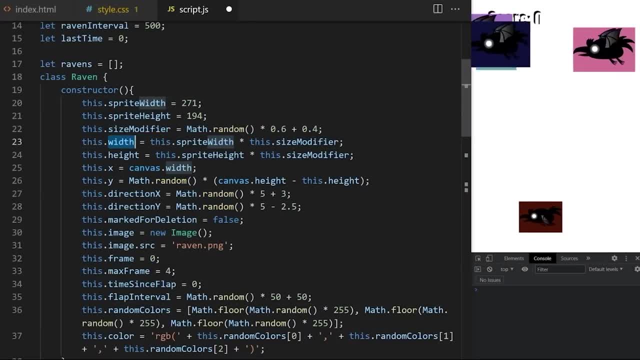 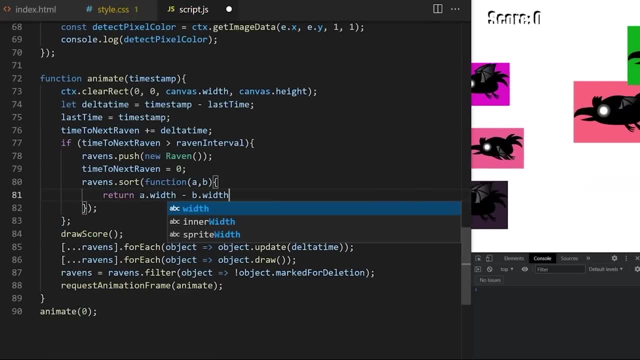 because I know Ravens in the back will have smaller width than the ones up front. I'm just going to return it like this simple syntax, and I'm comparing width of every element in the array against the width of every other element in the same array. A minus B will sort my 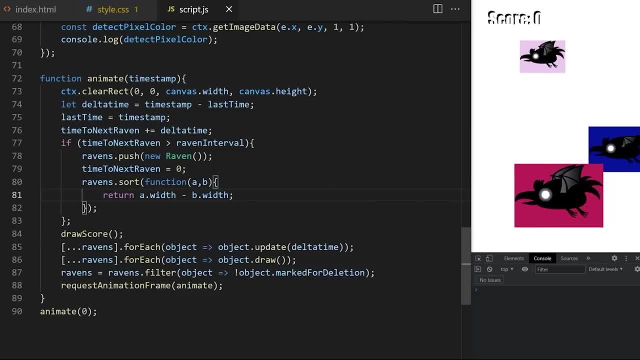 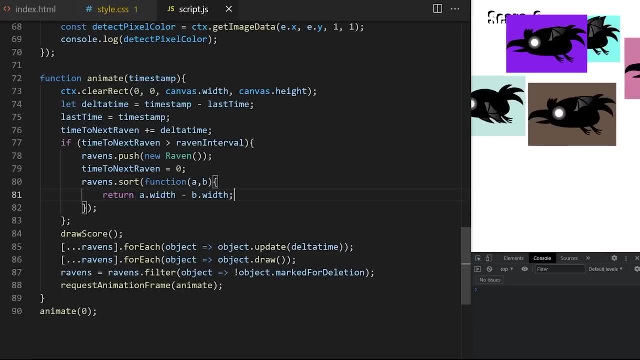 array in ascending order based on width, which is exactly what I want. I want small ones to be drawn first and larger ones to be drawn on top. you can read more about built-in JavaScript sort method online. we can see that it works. large Ravens are up front and smaller. 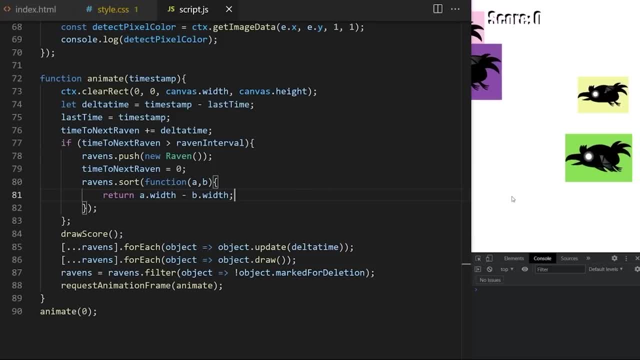 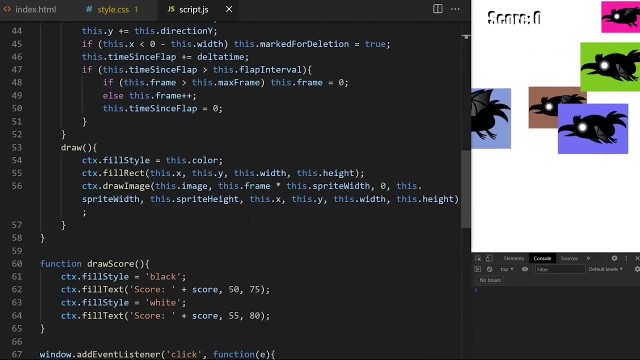 ones are behind perfect. as I said, I want to avoid tainted canvas error so I need to make sure I have a separate canvas I can scan color from that doesn't have any images are drawn on it. I take collision context variable I declared on line 6 and I draw my colored rectangles. 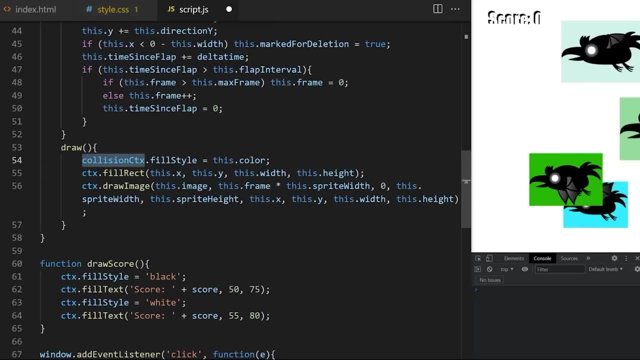 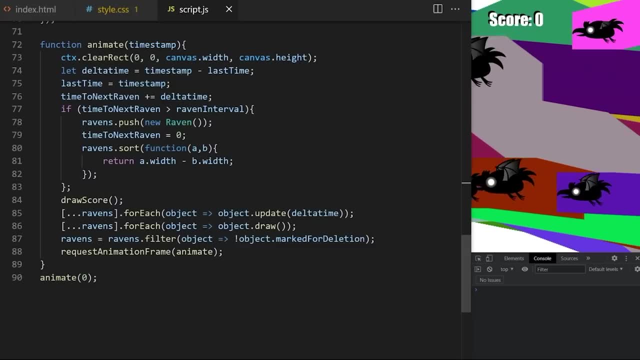 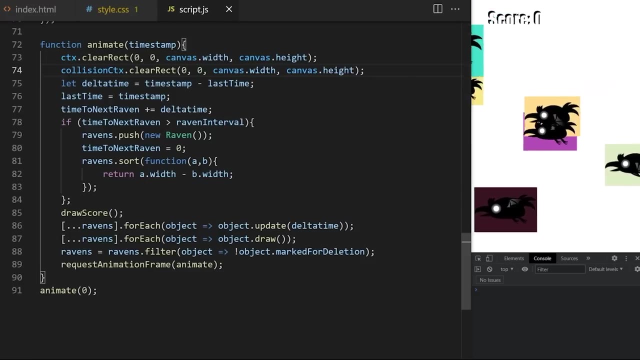 on that canvas instead by adjusting code here on lines 54 and 55. nice, that worked. I can see we are not clearing the old paint on that canvas. so online 74 I call clear rectangle on collision context as well. now we have two canvas elements. one has colored. 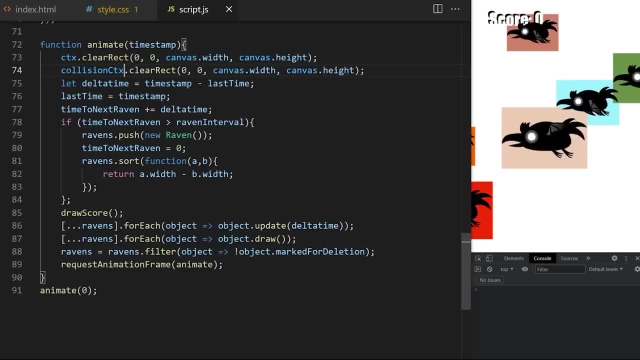 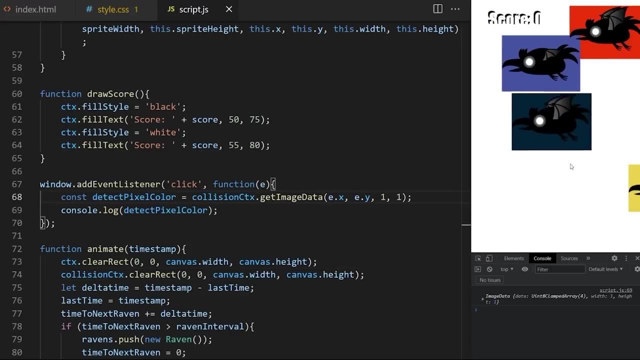 collision rectangle and the other has Ravens and score drawn on it online 68. inside click event listener. instead of scan in my main game canvas for pixel data, I will scan just collision canvas instead. now when I click on collision, now when I click, it will ignore the. 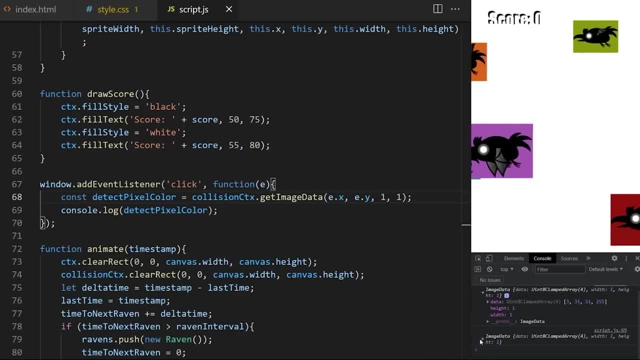 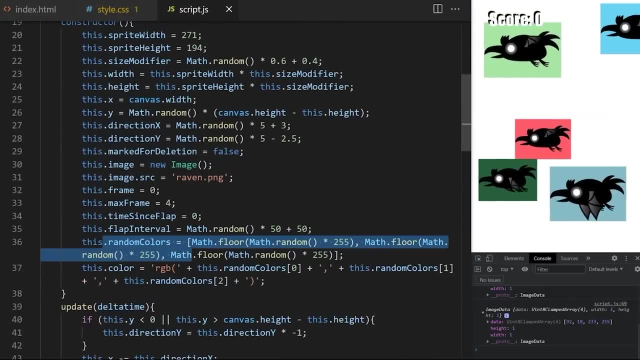 black Ravens and image data object will give me red, green, blue and alpha value of rectangle I clicked on. I will compare it with red, green, blue value inside random colors property on each Raven to know which one was clicked on and then I will set its marked for deletion. 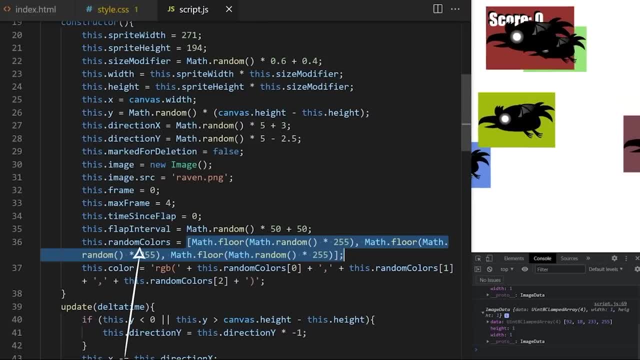 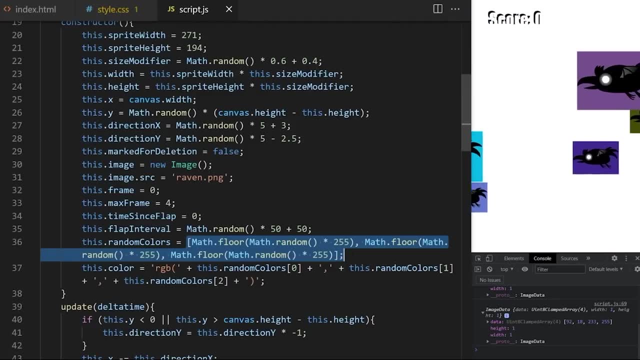 property to true. there are many techniques you can use to compare two array like objects against each other. let's just keep it simple. when I click on one of these rectangles I can see the values are inside this image. data object on a property called data. data is an. 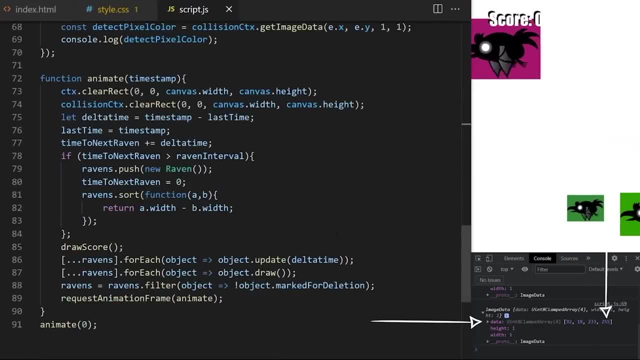 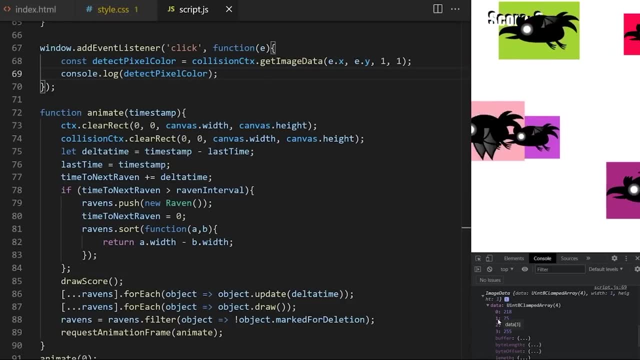 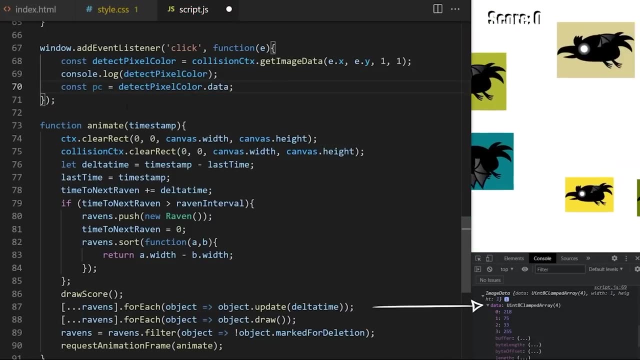 array with red, green, blue and alpha value of pixel. we clicked on, I create a variable to get hold of this array. detect pixel color dot data, which refers to this UI NT 8 clamped array with four elements. there is also a way to check for collision detection between: 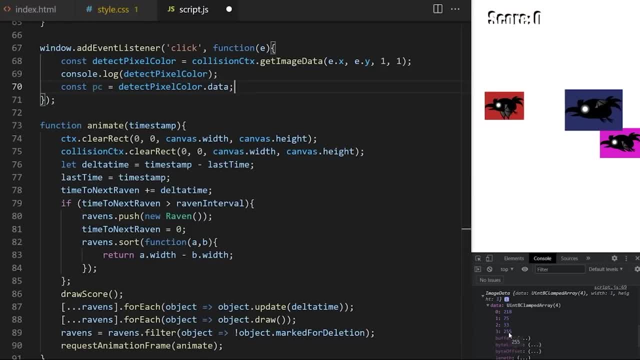 two objects based on a particular capacity, alpha value like this, but today we will do collision between point and shape, between mouse and Ravens. I will ignore alpha value from now on and I will just focus on these three values: red, green, blue. so this PC pixel color variable holds this data array with four. 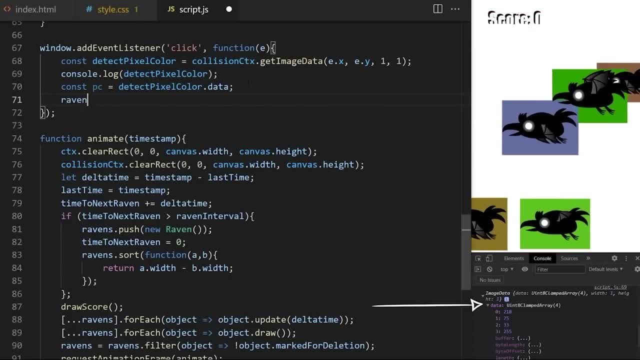 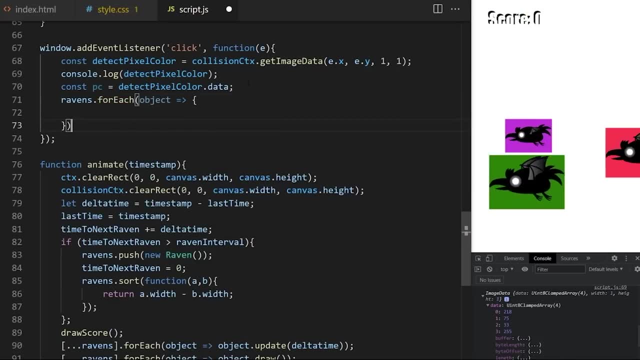 elements. I take my Ravens array and I call for each on it. for each Raven object in the array I will check if it's random colors. property from line 36. if the first element in the array, index 0, is the same value as pixel, we clicked on. 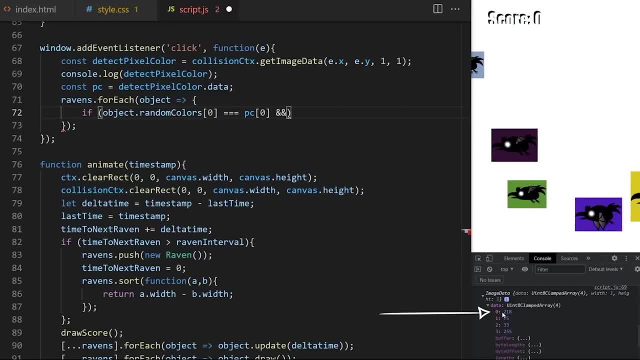 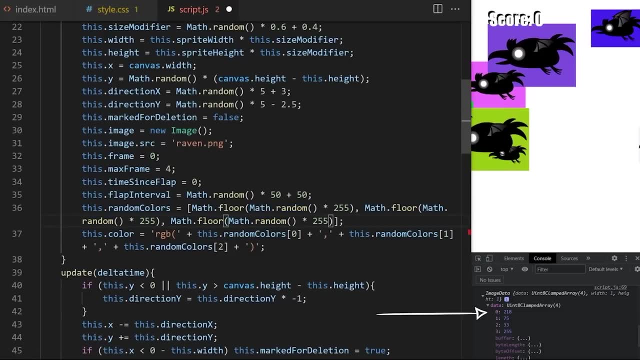 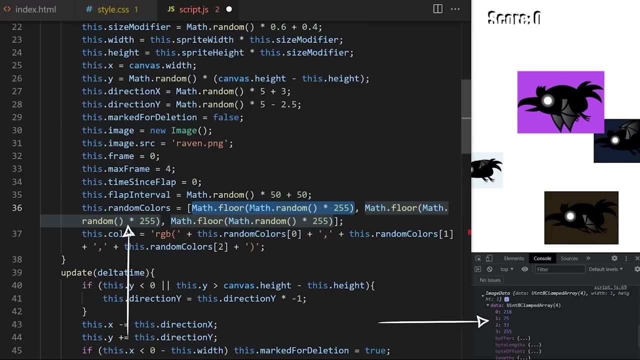 at the same time we also needed the second and the third element to match. if random colors array on my Raven matches exactly red, green and blue values on pixel we clicked on, we know we have a collision: index 0 is red, index 1 is green, index 2 is blue. we are comparing. 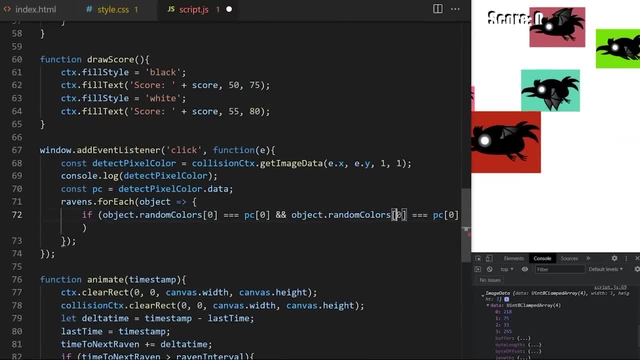 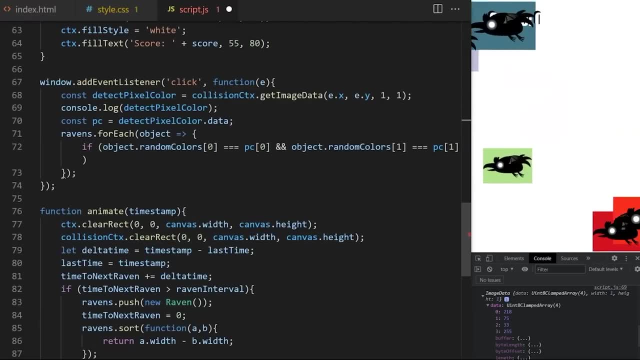 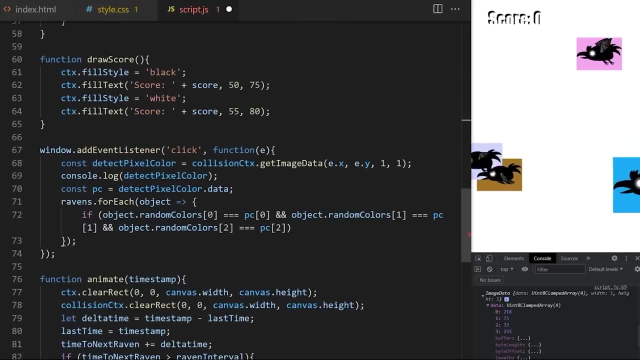 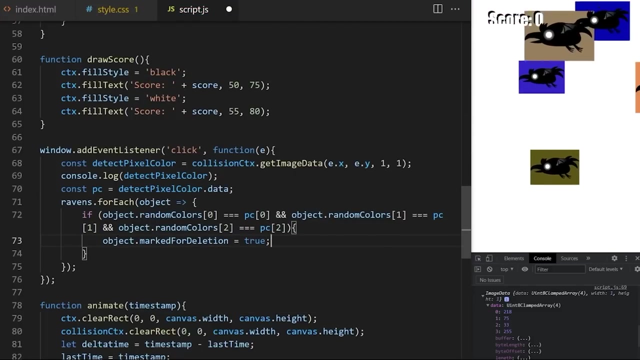 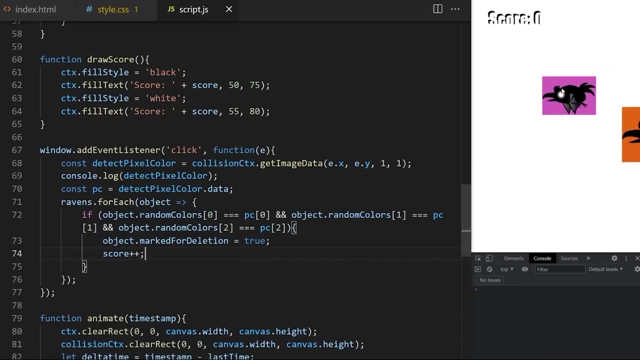 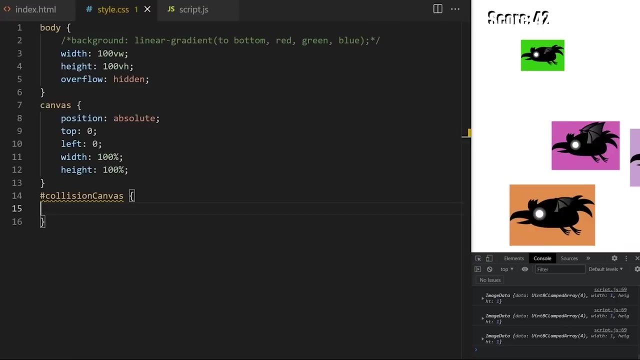 the two if they match, we have collision. so I will take that Raven object and set its marked for deletion property to true and I will increase score variable by one. awesome, it works. I can click on Ravens and they disappear and increase my score. I can set opacity on collision canvas to. 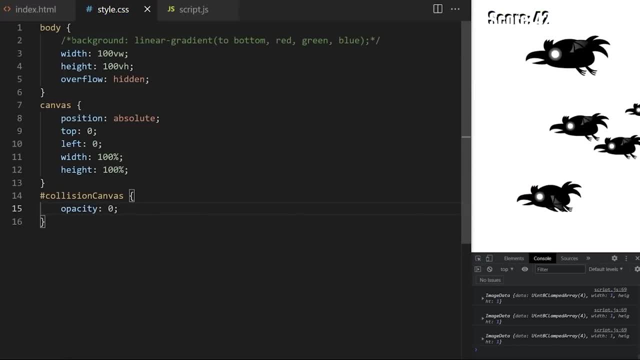 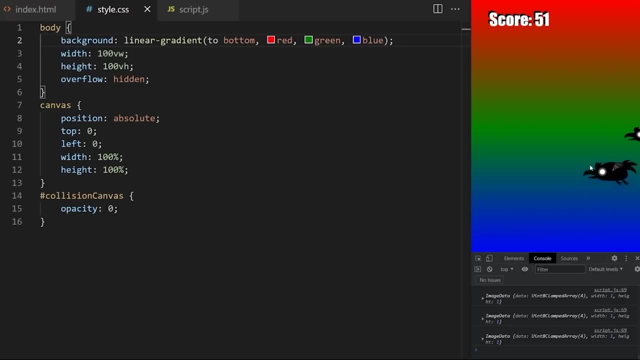 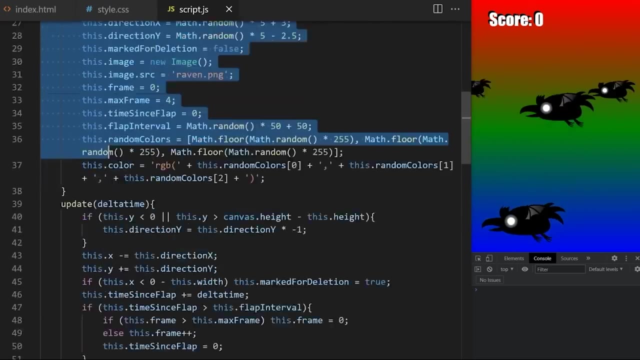 0 and I can enable rainbow background on body element collision detection still works correctly. well done. if you followed this far, you are doing great. what should we do next? how about we add explosion animation and sound effect whenever we click on a Raven? I will just repeat the same. 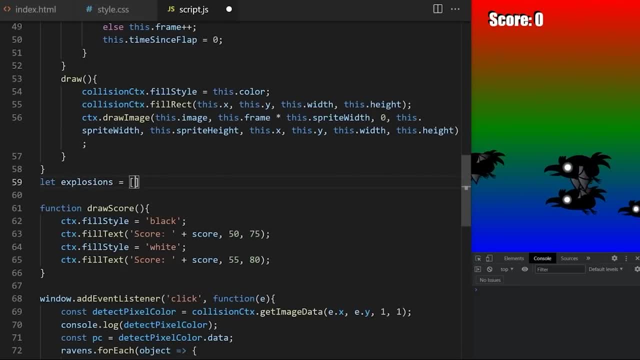 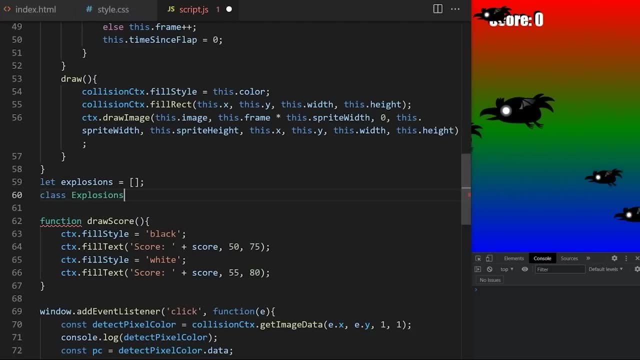 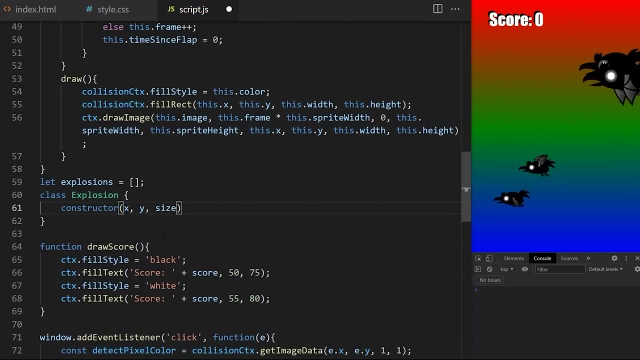 pattern we did for Raven class, I create an array called explosions. it will hold all active animated explosion objects. I will create a class to create a blueprint for these objects. its constructor will expect three arguments: X, Y and size, because position and size will come from the outside and will 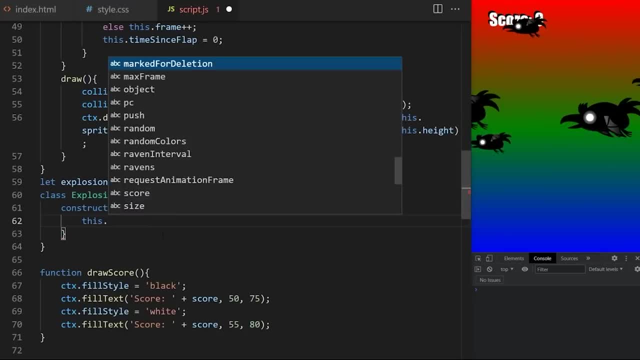 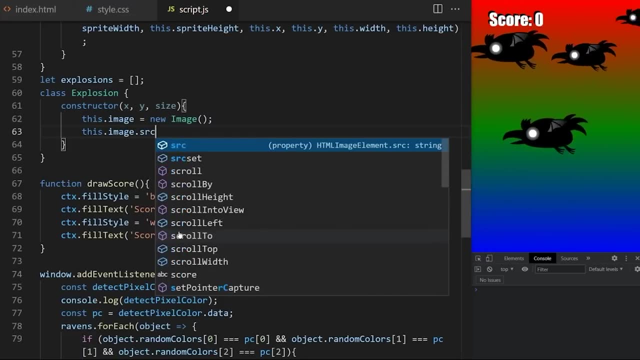 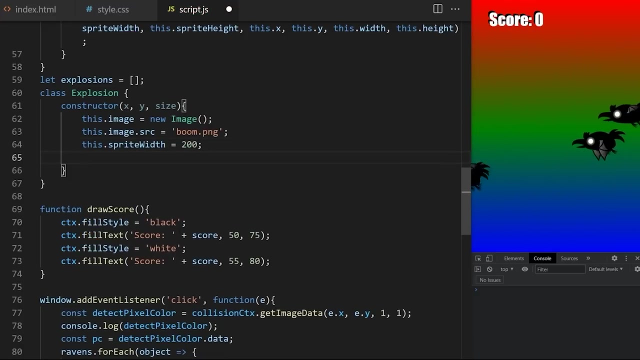 depend on the Raven. we clicked on this one. this dot image will be new image. this dot image SRC will be boom PNG. you can download the sprite sheet for free in the video description. sprite width will be 200 pixels. sprite height: 179 pixels. this dot size. 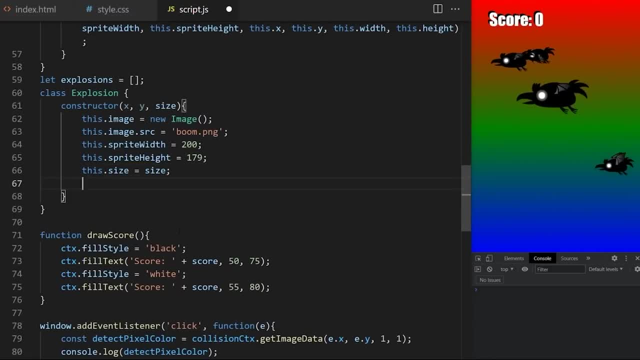 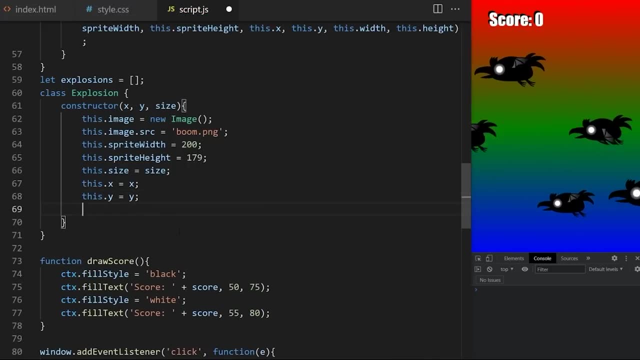 will be size. we passed as an argument on line 61. same for this dot X and this dot Y. these values come from the outside. this dot frame active frame will start from 0. this dot sound will be new audio like this: this dot sound SRC source and here as a: 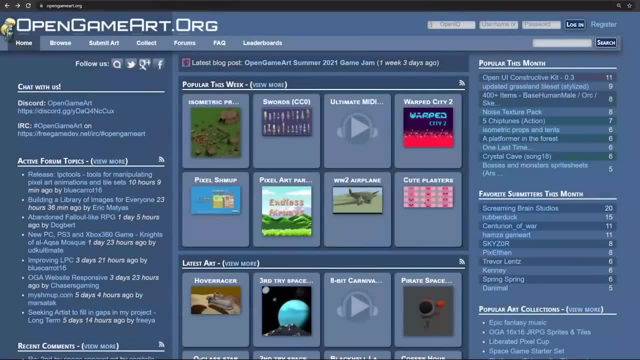 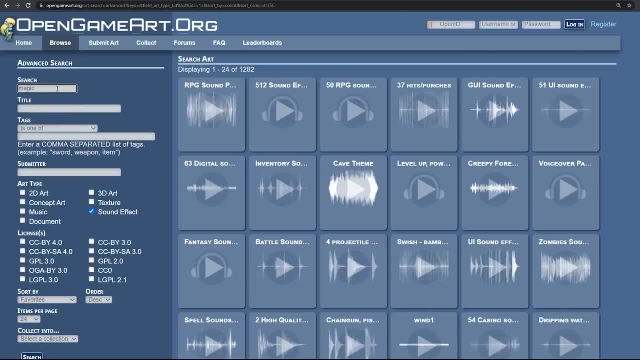 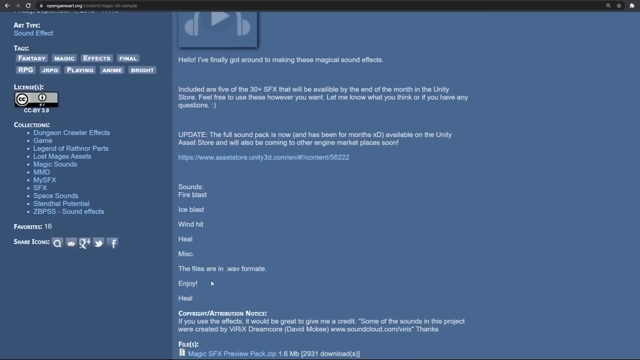 source. you can add any sound you like. for example, I will go to open game art org website, I click browse sound effects and I will search for magic SFX special effects. I will choose this pack of four sounds, I download it and I will use the one. 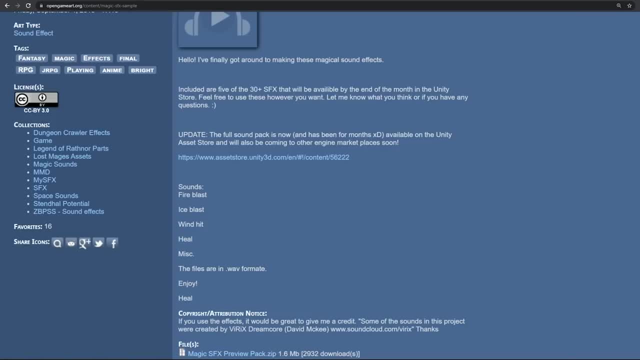 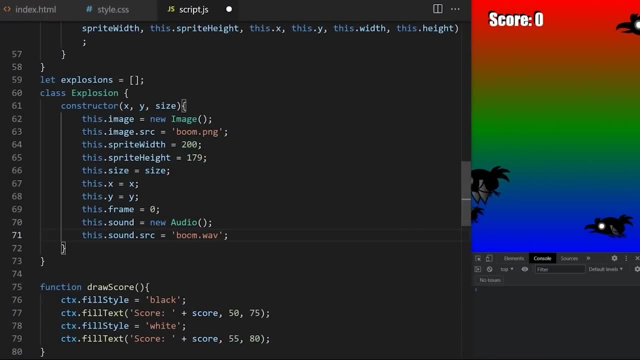 called ice blast. I will rename that file as a boom dot wav and I will add it to my project folder. you can choose a different sound if you want. you can also have multiple sounds and play a random one here. it's up to you in update method. 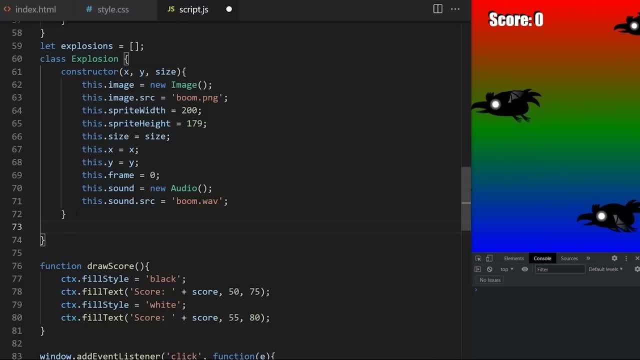 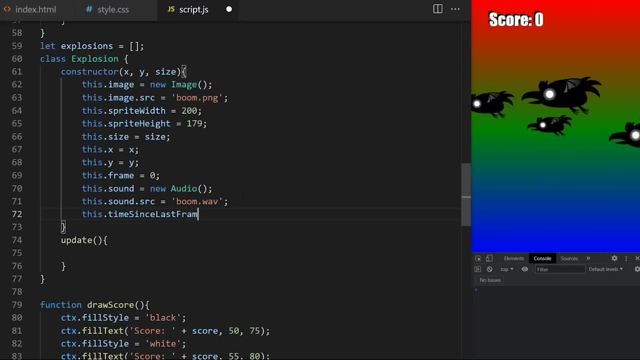 same as we did before. I will use Delta time to time my animation. we will have one variable to accumulate Delta time values, called for example time since last frame. it will start at 0. then we need a second variable to define limit when the next frame triggers. I call it for. 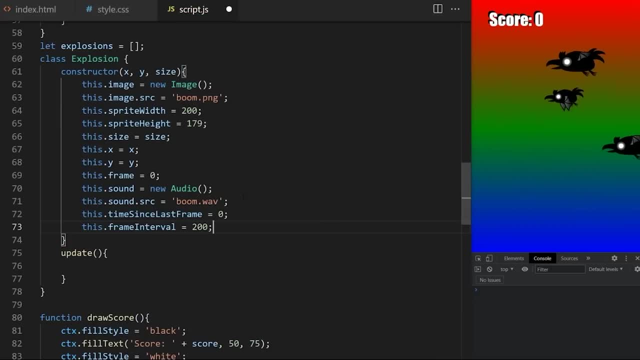 example, frame interval and I set it to 200 milliseconds. I pass Delta time as argument to update method. it will be coming directly from animation loop. I will show you in a minute this dot time since last frame will be slowly increasing by the amount of Delta time. 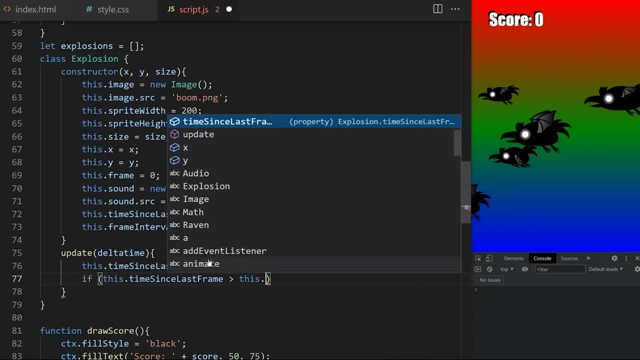 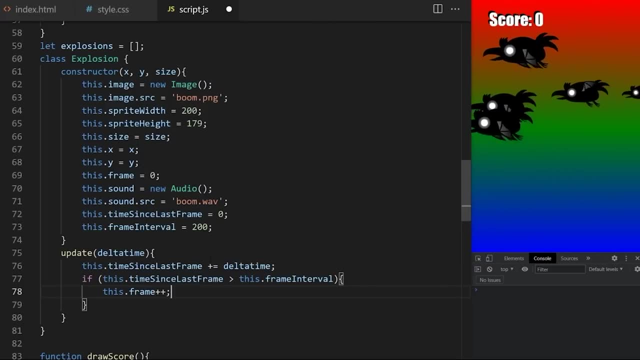 if time since last frame is increasing more than frame interval- 200 milliseconds, I increase this dot frame from line 69 by 1. I also want to play the sound when we are on frame 0, when the explosion first appears. there are better ways to do that, but for today I. 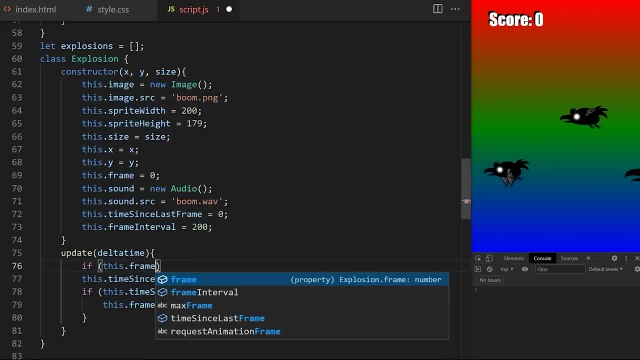 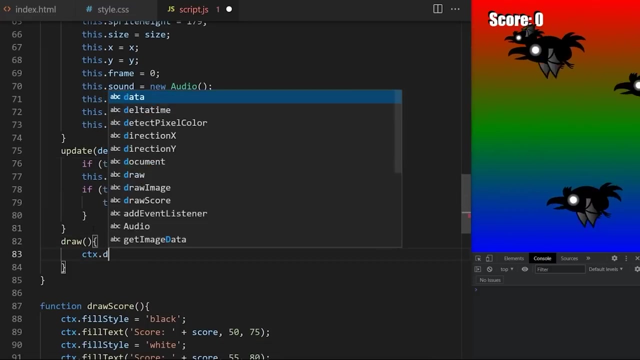 will simply check if active frame of this explosion is 0 and I take the sound from line 70 and I call built-in play method on it. explosions will also need draw method, which will draw the actual sprite sheet animation. we will pass a draw image, 9 arguments, same as we did. 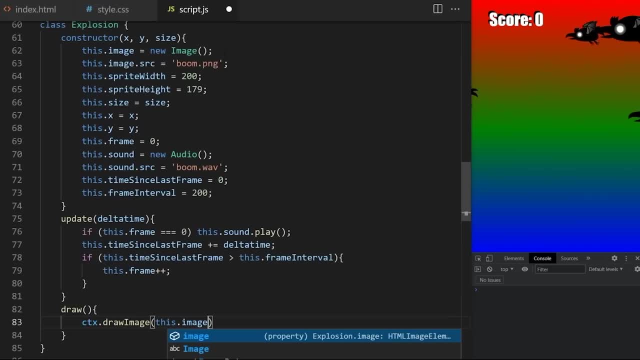 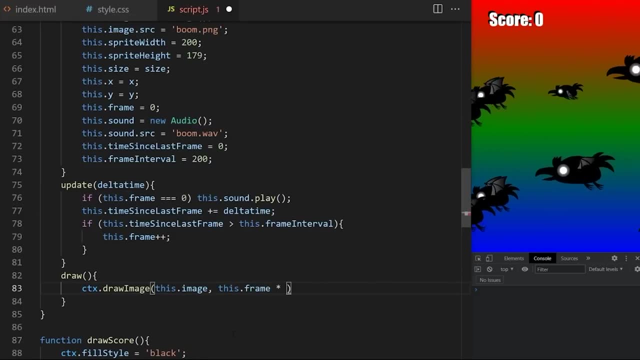 with Ravens image. we want to draw this dot image from line 62 for values for area to crop out single frame. so source X is this dot frame times this dot sprite width. source Y will be 0 because we only have one row of sprites. source width will be sprite width from line 64. 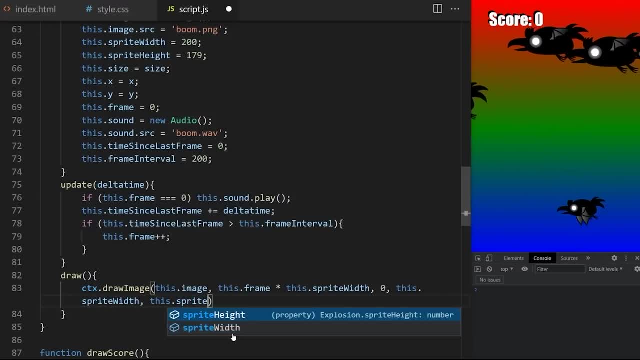 and the source height will be sprite height from line 65. so now we told the JavaScript what area we want to crop out. now we need to give it X, Y, width and height where to place it on destination canvas. so this dot X, this dot Y and this dot size for width and 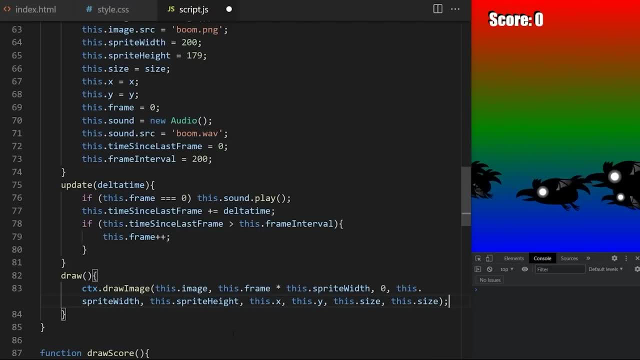 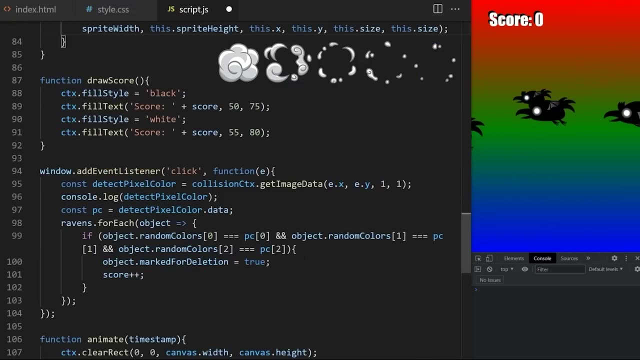 this dot size for height, as this dot frame variable increases here on line 79 because of this source X property. here we will show frame 0, 1, 2, 3 and 4. now we're done. where do we trigger this code to create and animate new explosion? the best place. 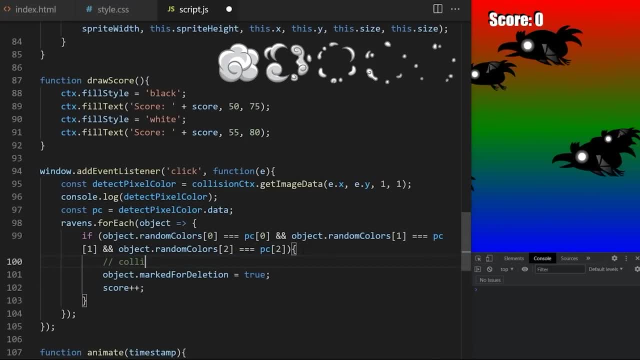 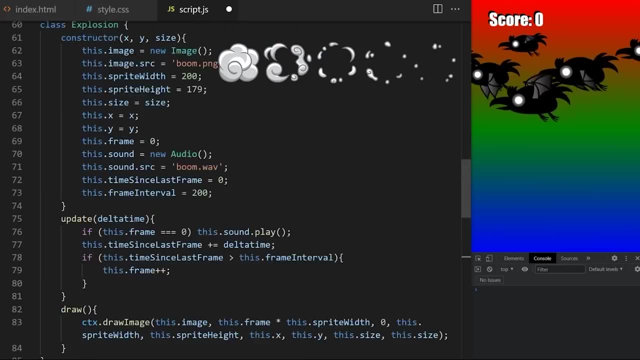 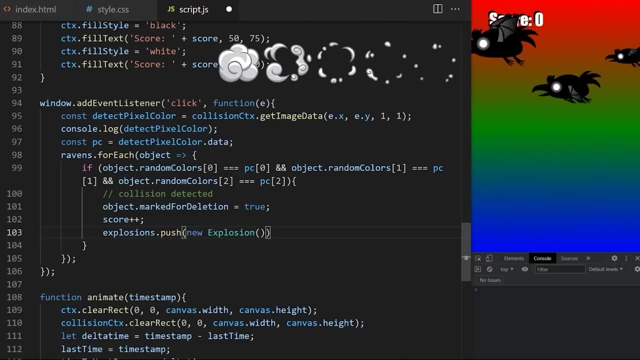 would be here. I think this if statement detects collision by color. so when collision is detected I take explosions array from line 59 and I push new explosion in there. this will trigger explosion class constructor. on line 61 I can see it expects value for X and Y coordinates and size, because 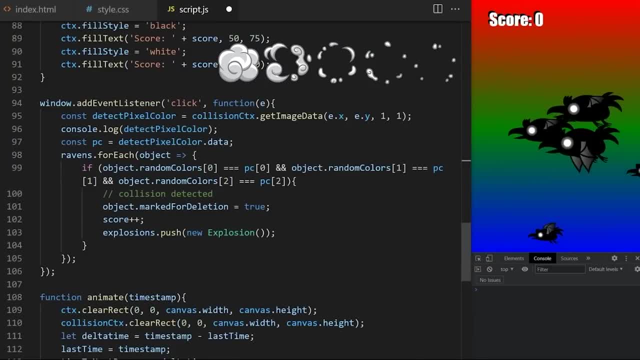 I want explosion to depend on the size of the Raven we clicked. so here we are cycling through Ravens array, referring to individual Ravens as object. I want to pass X, Y and width of that Raven as X, Y and size arguments here. okay, that should work. I can test it by. 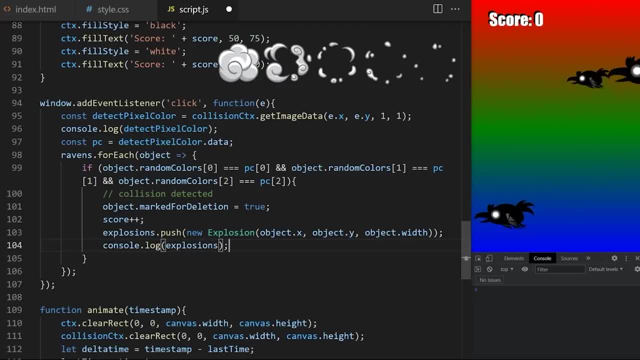 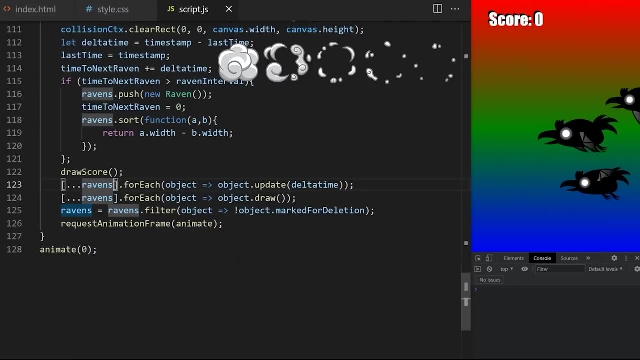 console again: explosions array. from line 59 I can see as I click and hit Ravens, explosions are being added. perfect, I made sure my explosion class has update and draw method same as my Raven class. that's why here on line 123, I can simply just use spread operator and 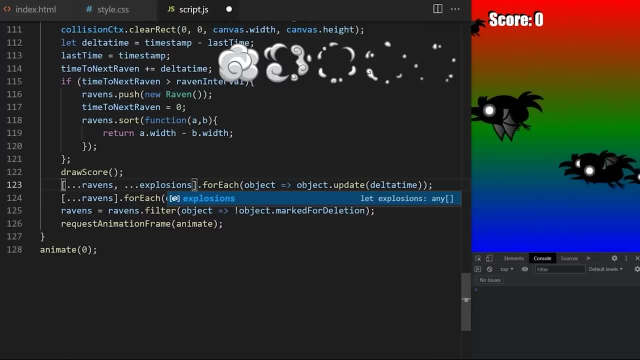 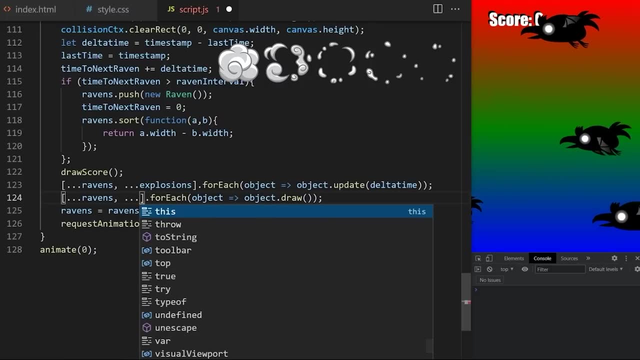 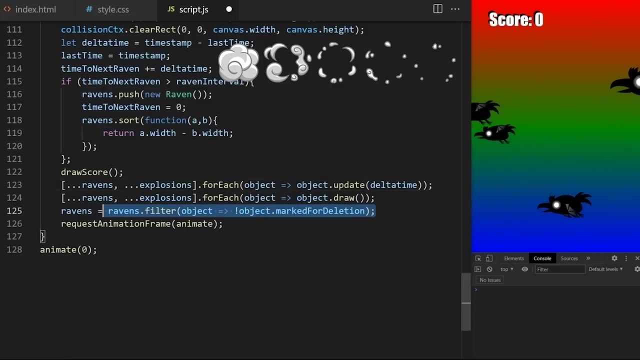 expand the entire explosions array into this array I'm creating on a fly so that I can call update on all Ravens and all explosions at the same time. like this, I do the same thing for draw method online 124. I like this syntax. it looks clean down here. I will also remove all. 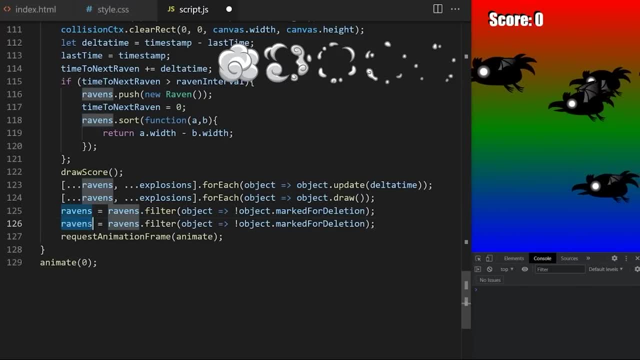 explosion objects from the array using built-in array filter method. I need to create a property called marked for deletion on my explosion class for this to work. as you can see, I'm repeating the same pattern we used for Ravens. I hope that using the same structure like this: 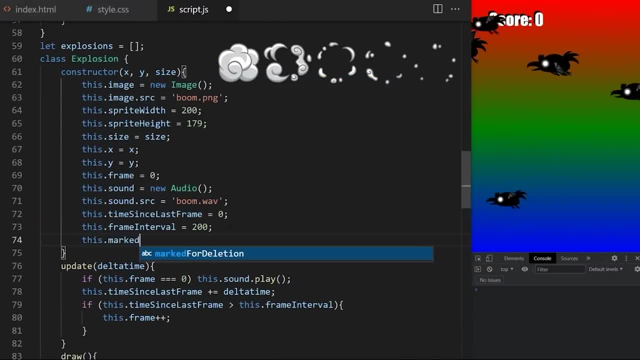 helps you to understand and navigate in the code a bit better. initially I set it to false in update method. I write an if statement. if this dot frame is the same as the frame from line 69 is more than 5, which means after all the frames of sprite. 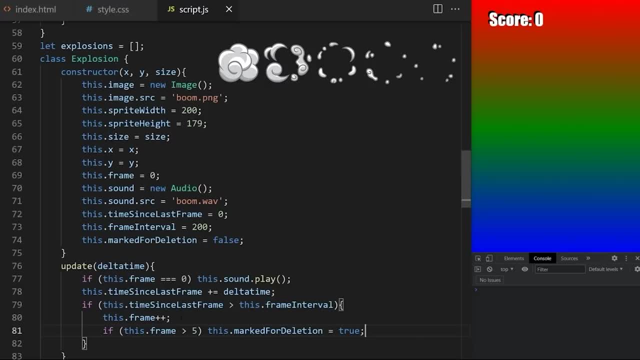 sheet have been displayed one by one and explosion animation is complete. I set marked for deletion from line 74 to true. when I click on Ravens sound place and explosion sprites are animated. we are making great progress. we just need to polish some details here. if I change. 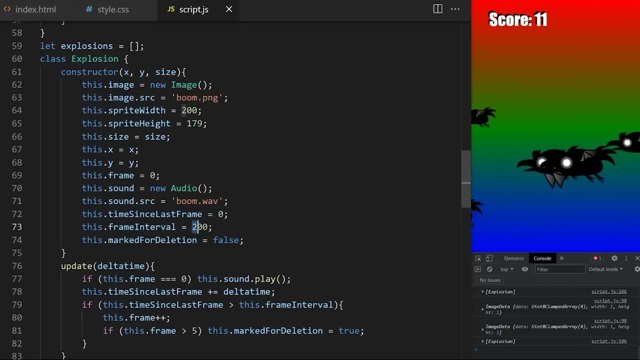 frame interval on line 73 to 500. you can see it only affects the first frame. the rest of animation is playing really fast. hmm, oh, it is because I need to reset time since last frame back to zero every time, so it can count towards the next. 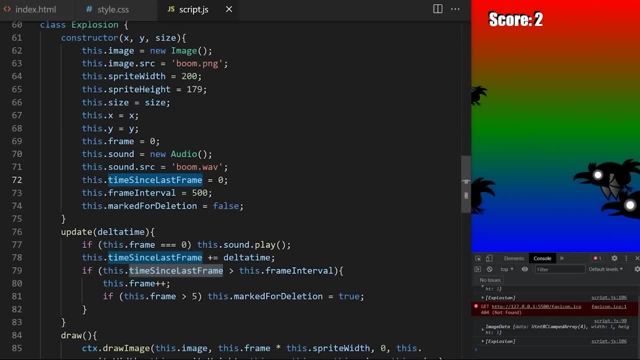 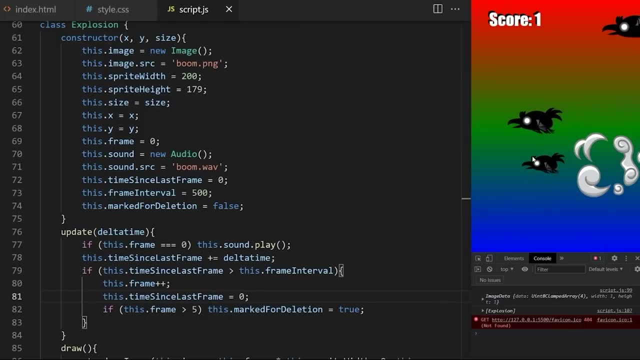 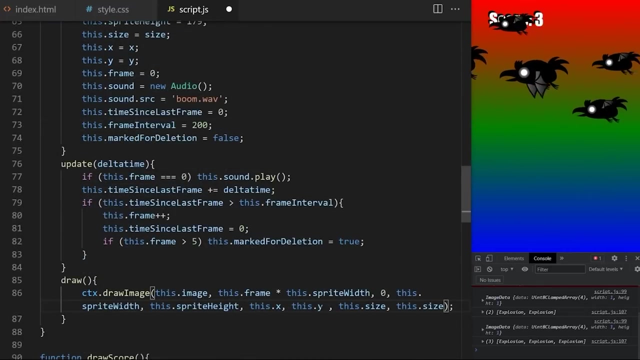 frame interval over and over to serve next frames. 500 milliseconds is too slow, let's try 200. I want to align explosion animation better over the Raven sprites. let's move it a bit upwards by adjusting destination Y argument in draw image method. I will make it. 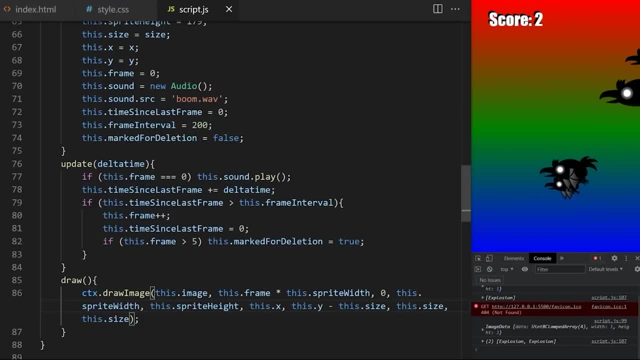 relative to size: this dot Y minus this dot size, this dot size divided by 4. yeah, I think this is aligned well. now let's create game over condition. on line 11, I create a global variable called game over and I set it to false initially in. 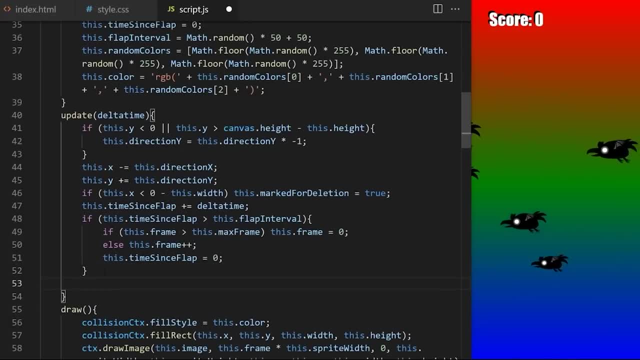 sight update method on Raven class. I create an if statement. if any Raven manages to get all the way across the screen and behind the left edge of game area, game will end. if this dot X is less than 0 minus this dot with set game over from line 11 to true and inside. 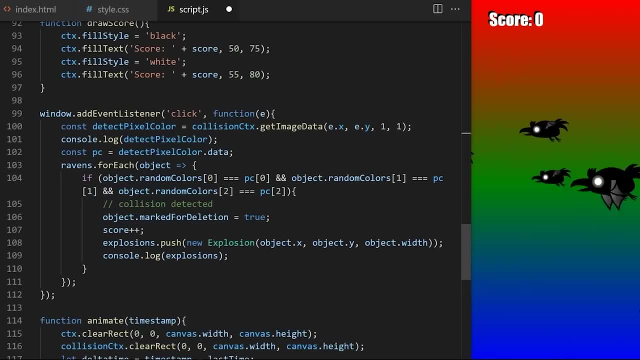 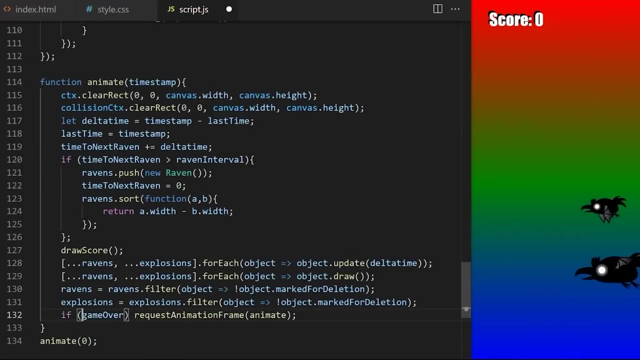 animation loop on line 132. I only want to run request animation frame and serve the next frame of our game. as long as game over is not true- exclamation mark here- when Raven gets all the way across screen, game over will be set to true and game will stop. like this: I also want to. 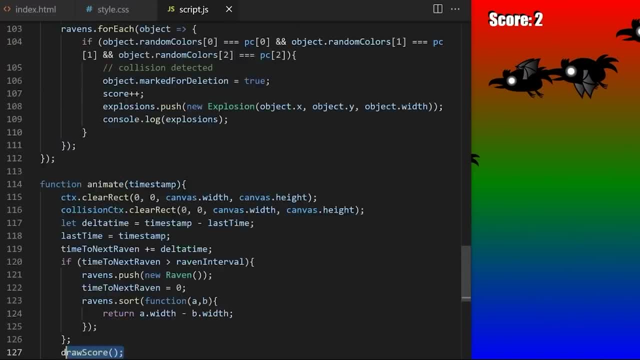 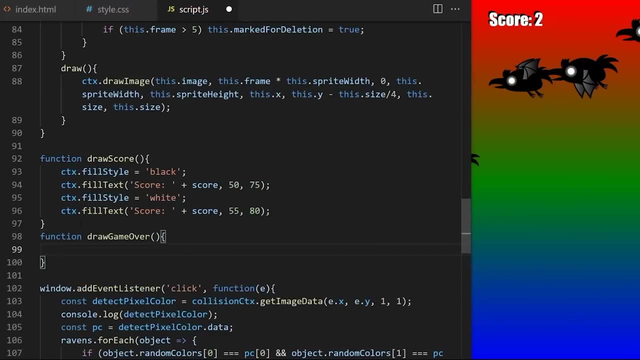 display game over message. same as we did a draw score, I will create a function called the draw game over. first I will be black. fill text will be, for example: game over. your score is. your score is plus I concatenate score variable. I want it in the middle of the screen, so 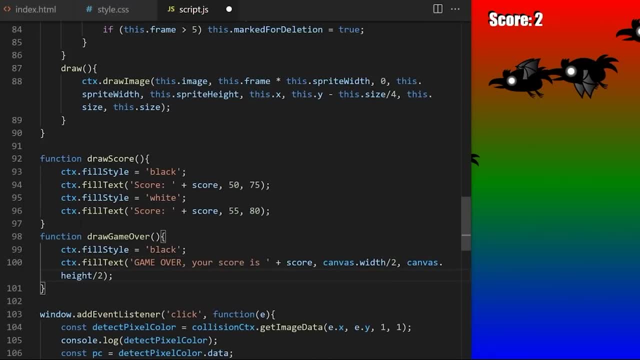 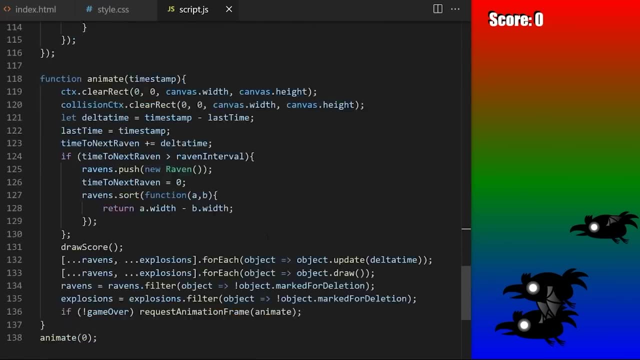 X coordinate will be canvas width divided by 2 and Y coordinate will be canvas height divided by 2. now I need to call my draw game over function here in animate. if game over is false, keep serving the next frame. else, call draw game over. method to display message. and. 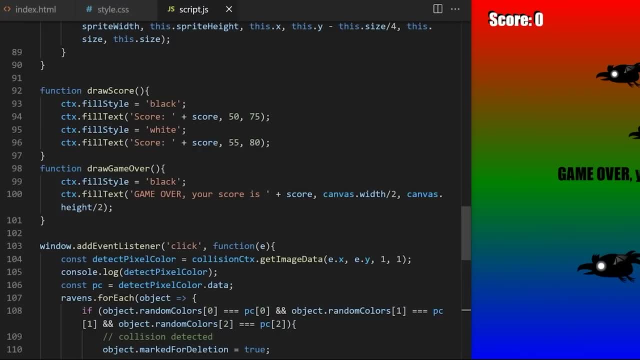 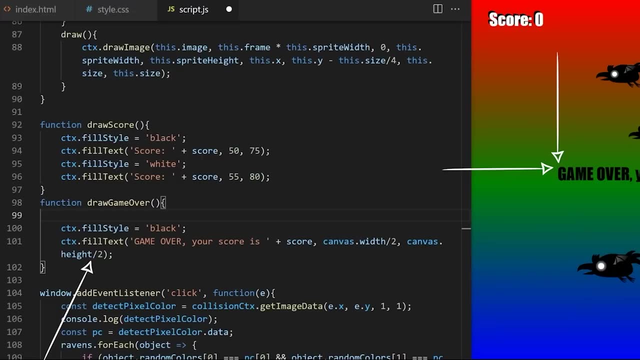 final score. it's not centered. it's because these coordinates online have a hundred and one mark, top, left, corner, and the text goes towards right and bottom from that point, same as when you are drawing rectangle or image on canvas with text. it's easy to Center by setting. 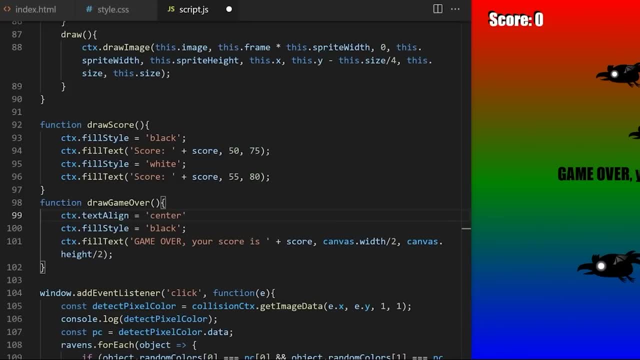 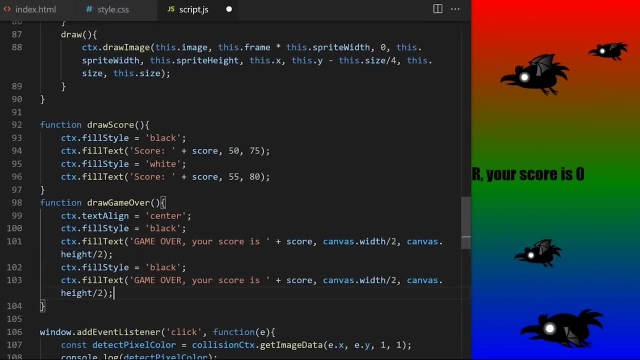 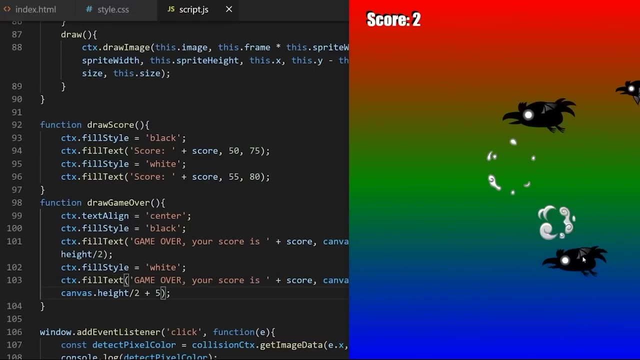 text. align property to Center like this. yes, that worked, same as I did with score. I want to give it shadow. I will use this trick where I draw the same text twice with different fill color and I offset it by five pixels. nice, let's change direction of. 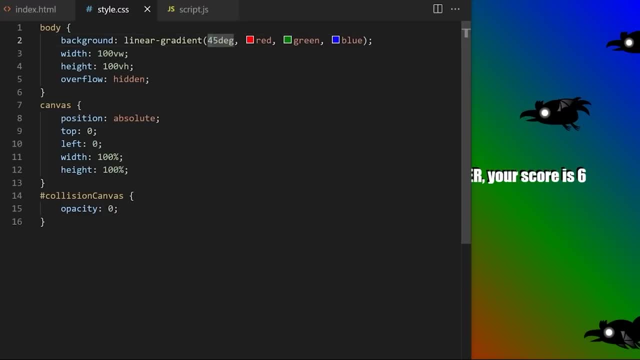 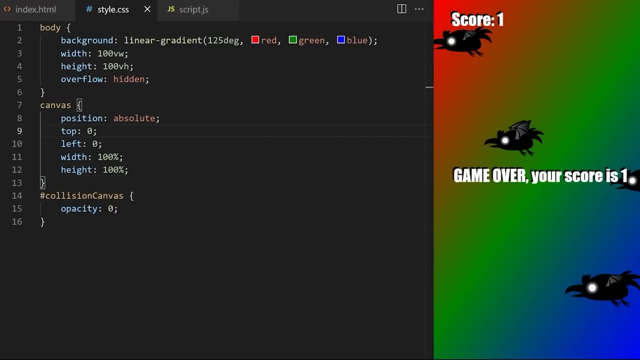 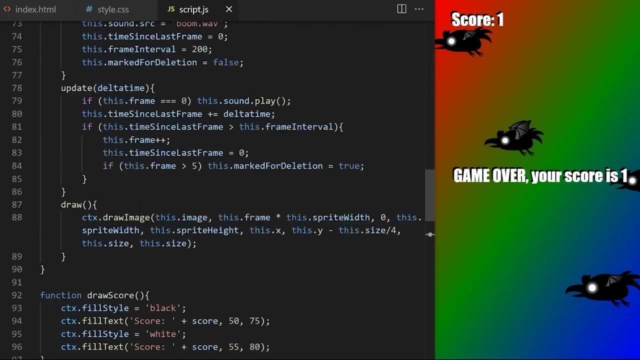 background gradient: maybe 45 degrees, 125 degrees. let's do a little bit of experimenting now, and also to solidify what we learned today. I will use the same code pattern we used for Ravens and explosions to add particle effects to our game. I will go a bit faster now. this: 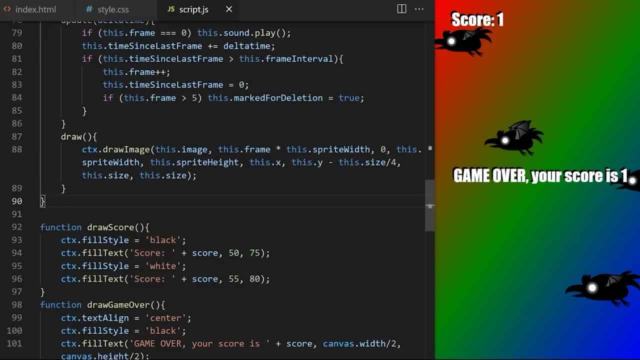 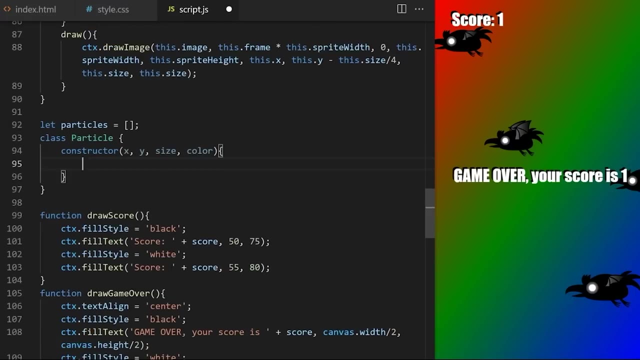 part is just for fun. feel free to run your own coding experiments. I create an array that will hold all my particle objects. I create particle class. constructor will expect X, Y, size and color. this will be coming from outside the class and will depend on what Raven is leaving. this. 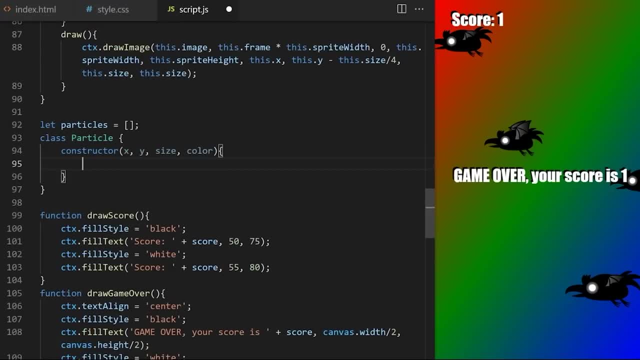 trail and creating these particles. it will be shooting from their tails, as usual. we will create properties for this dot X and this dot Y, this dot radius: since particles will be drawn as circles, it will be a random number tied to size of a Raven. let's try this formula and 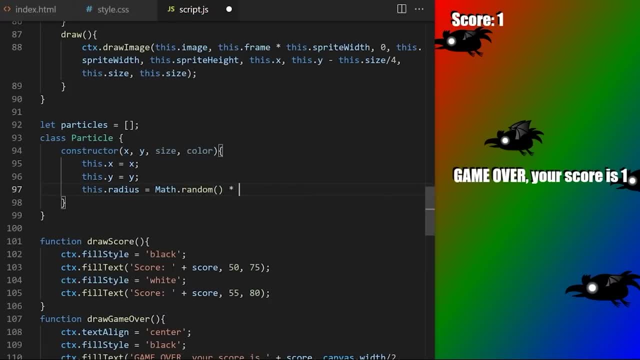 see what it looks like. particles will be growing in size, so we need max radius to know when to remove them and also at which point they reach maximum opacity. it will be random number, between 35 and 55, for example. marked for deletion, as usual, will be false at first. horizontal speed. 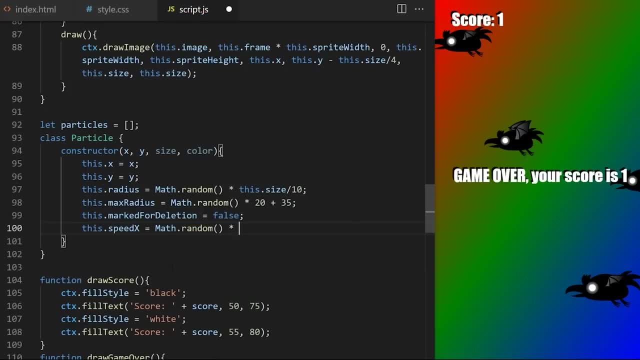 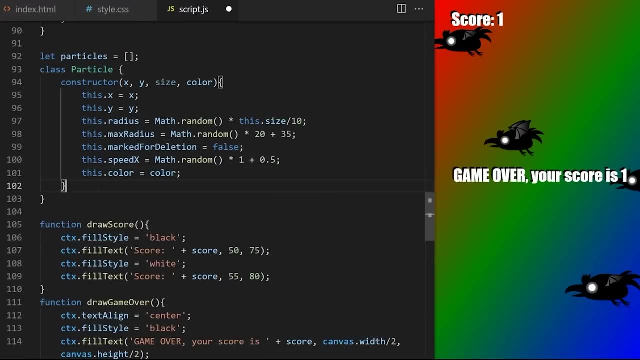 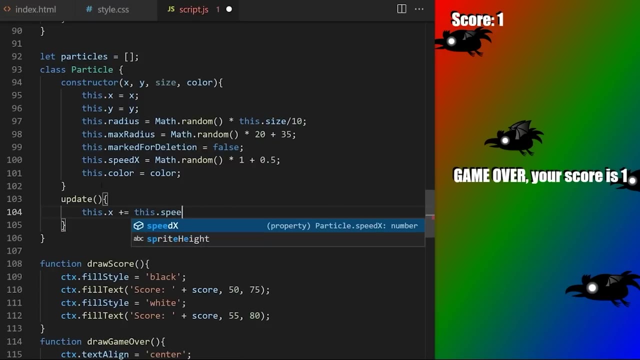 X will be a random number between 0.5 and 1.5 because I want the particles to slowly drift to the right. this dot color will be passed from the outside. update method will move particles to the right horizontally. it will increase radius by 0.2 per. 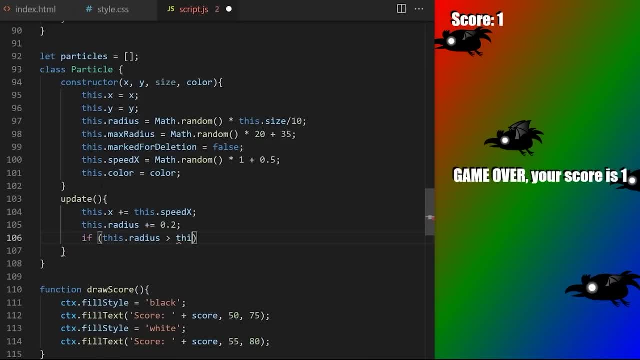 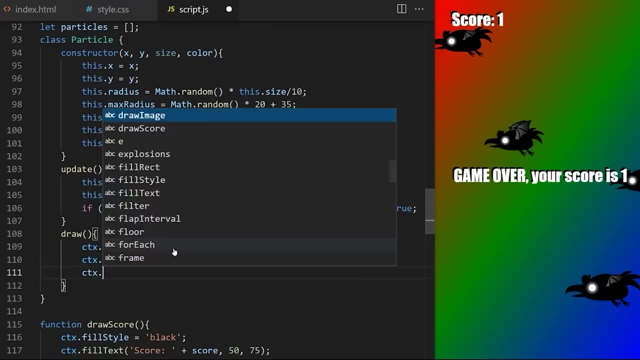 frame and it will check if this dot radius is more than max radius. if it is, it will set marked for deletion. to true draw method will just draw a simple circle. begin path to start. the drawing fill style will be this dot color from line 101. arc method to draw a circle I: 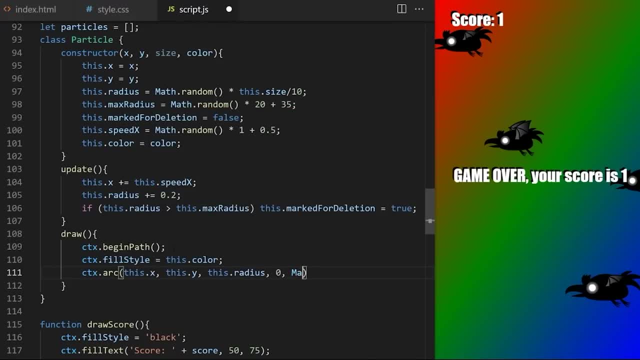 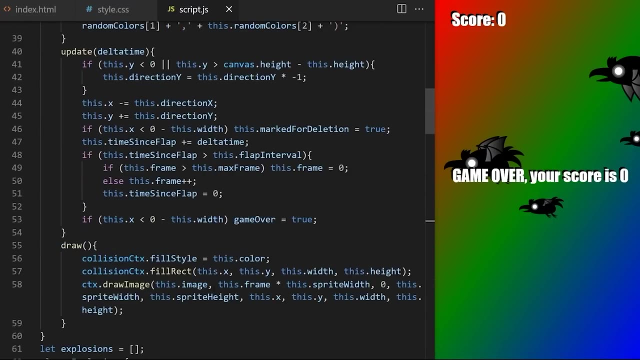 pass it X, Y radius, start angle and end angle like this and we fill circular path with color. we have a class that will serve as a blueprint to create particles. I want them to follow Ravens as they fly, to create trails behind them. to do that, I go up inside update method. 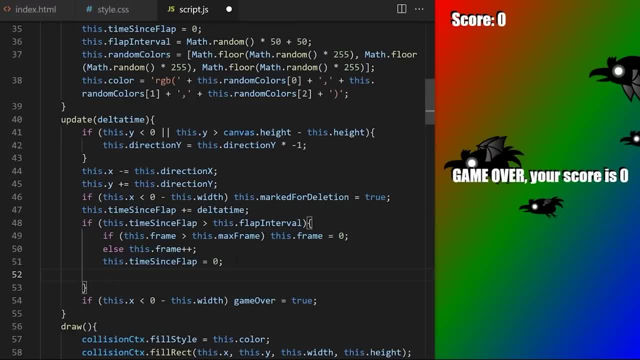 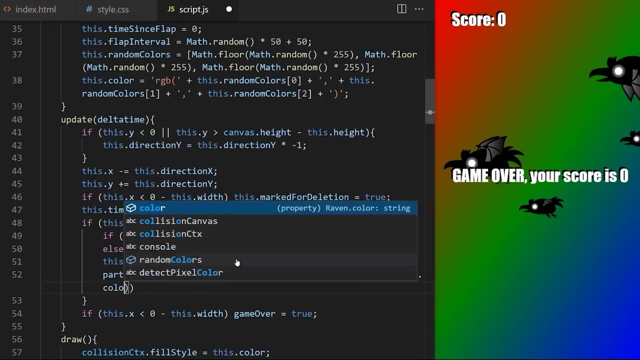 on Raven class. every time we serve next sprite sheet frame at the same interval we are going to take particles array we just created and we will push new particle inside my particle class constructor. constructor expects four values to come from the outside: X, Y, size and color. so I 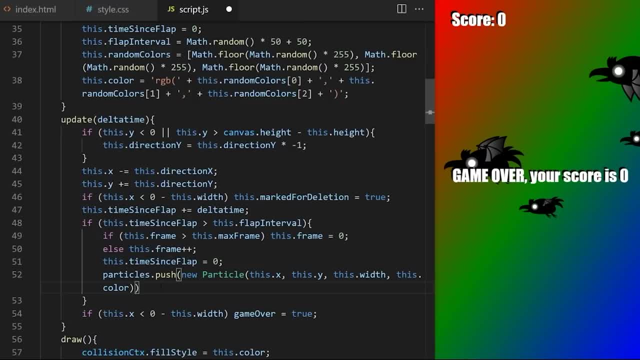 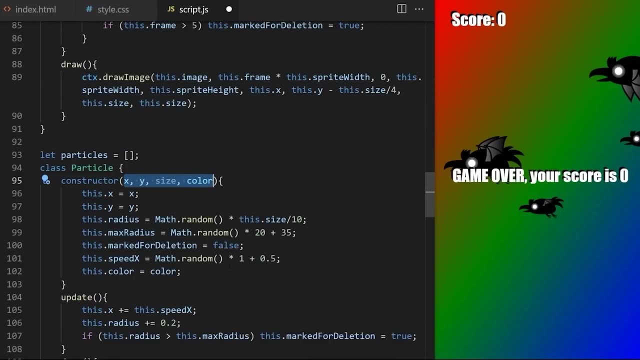 pass it X and Y of this Raven, width of the Raven as a size argument. and this dot color we use for collision detection rectangles will also be color of particle trail for that particular Raven. you can see here on line 95: constructor wants these four properties to come from. 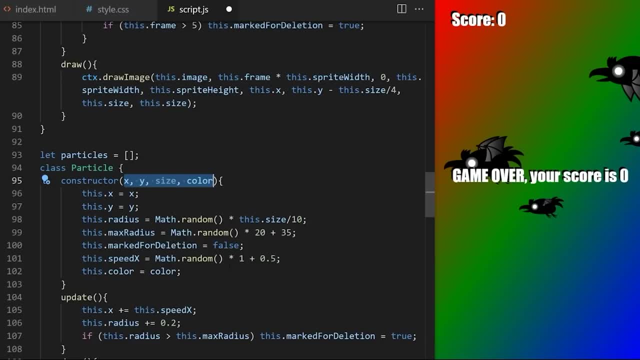 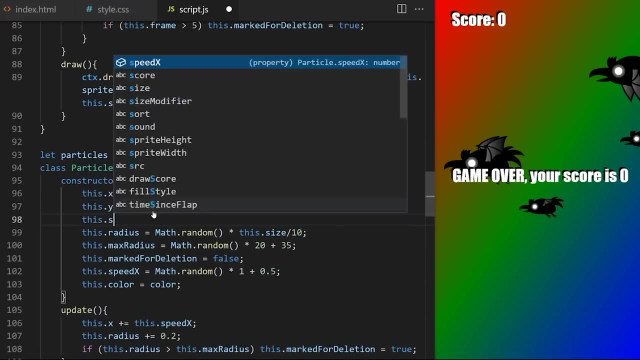 the outside so that it knows where on canvas to draw the particles, how large and what color I can see. I forgot to declare this dot size here. like this, it will come from here and it will be used here to make radius of particle circles relative to the size of Raven. smaller ones should. 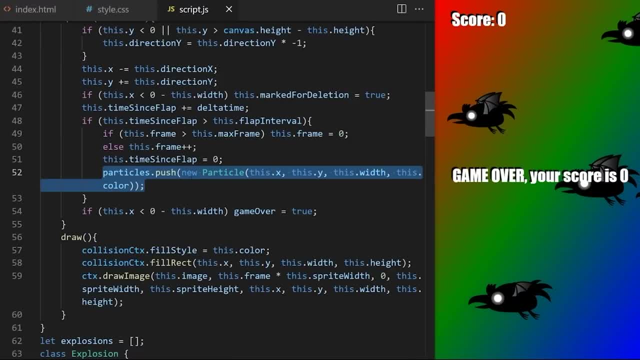 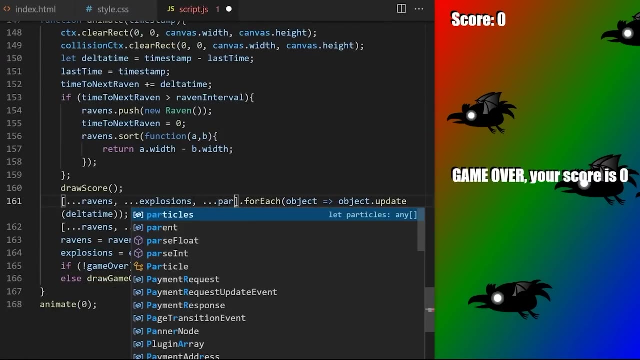 have smaller trails. so we have particle class here. on line 52 we are creating new particle object and pushing it into particles array inside animate. I use spread operator again to expand contents of particles array here so that their update method gets cold, and I also expand it here for draw. 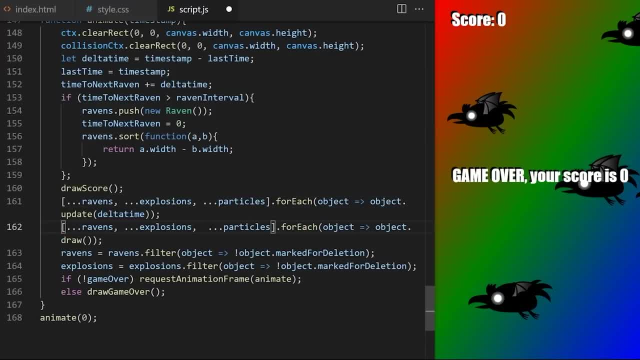 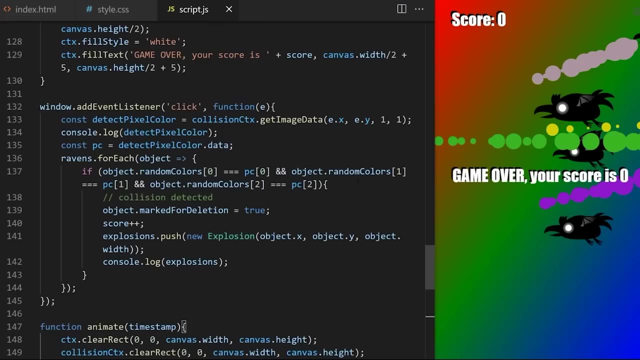 method. I also need to make sure old particles with marked for deletion properties set to true get filtered out from particles array. nice, we are drawing particle trails. you can see they come from the top left corner of Raven hitbox. I will adjust that position a bit here inside. 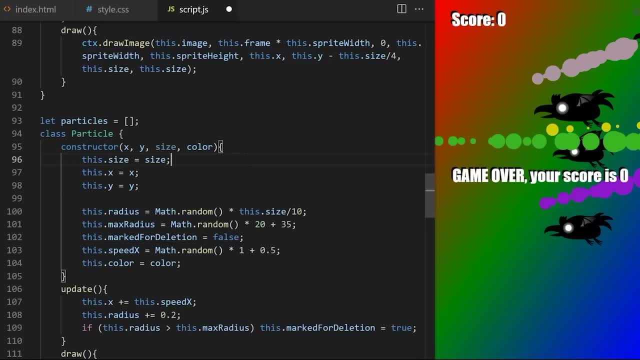 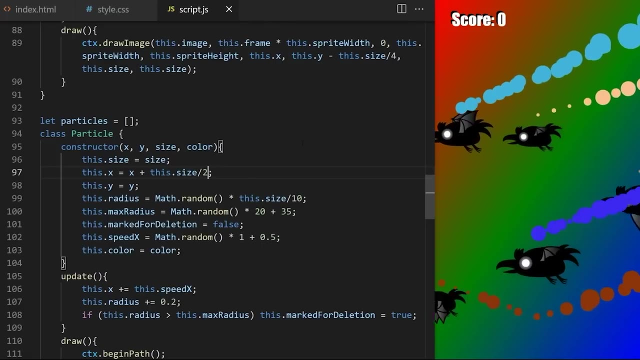 particle class constructor. first I need to move this dot size up so that its value is available for all properties coming after it. this dot X will be X. past as argument on line 95, plus this dot size from line 96, divided by 2, to Center it horizontally. yes, this dot Y. 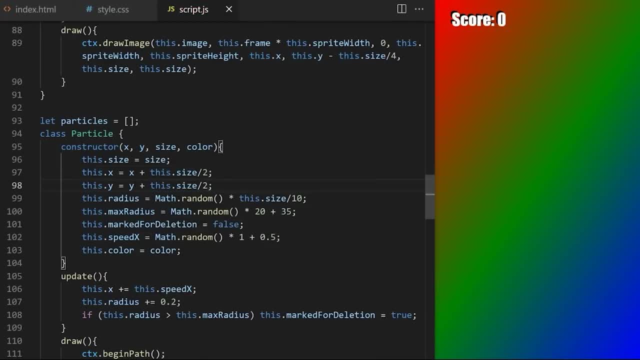 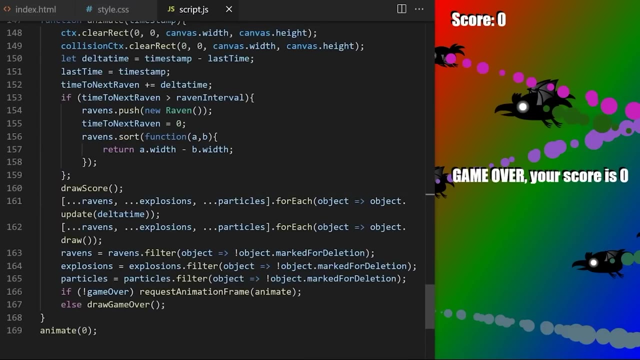 will be Y, plus this dot size divided by 2. no, that's too low. this dot size divided by 3, much better. I want particles to be drawn behind Ravens. we are drawing everything on a single canvas element, so how things are layered depends on the order at which JavaScript cycles through. 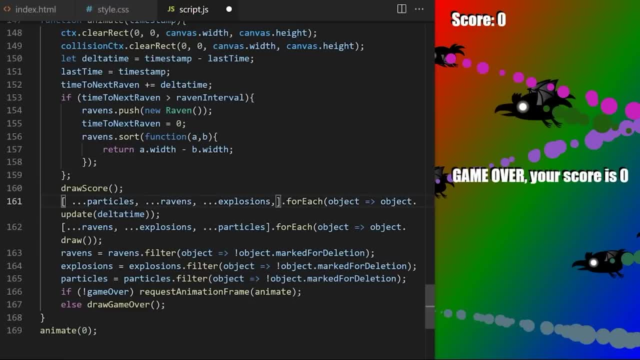 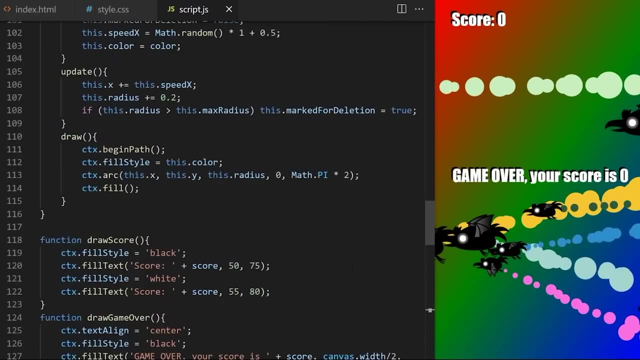 these objects and calls their draw methods for every frame. I will change the order here to draw particles first, and then Ravens and explosions will be drawn over them like this. awesome, we have a work in code. let's clean it up in update method. on particle class: I want radius to grow faster- 0.5. 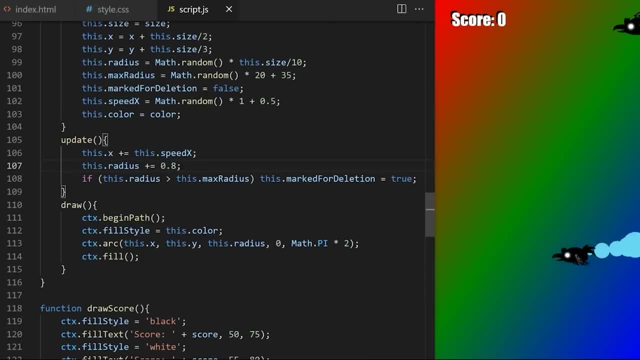 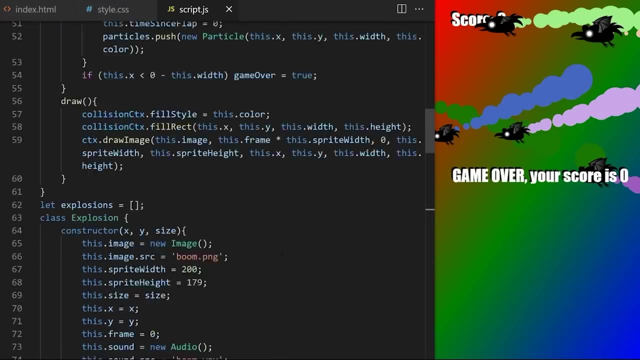 0.8, 0.5 is fine. drawing trail on every single Raven can be performance expensive. I want a property that will allow me to randomize it and allow me to set what percentage of Ravens will have particle trails on my Raven class. I create a property called this: dot has. 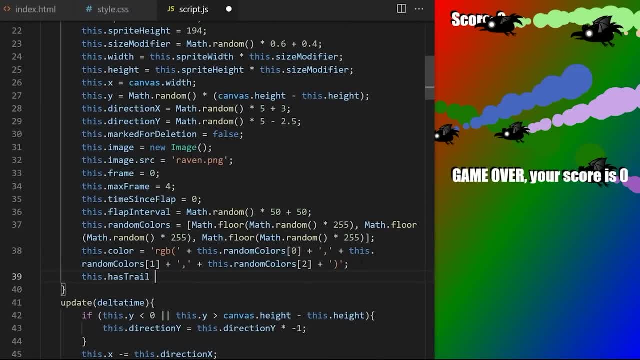 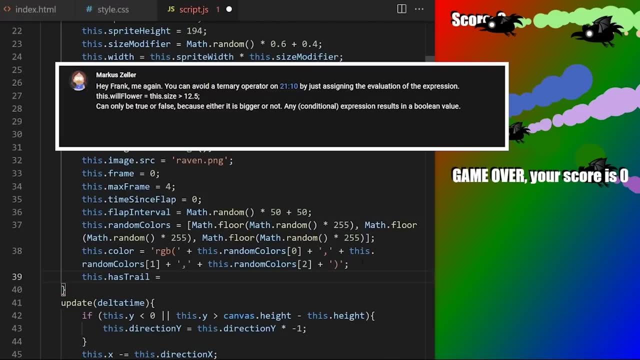 a trail. I want this property to be true for certain amount of Ravens and false for the rest. as Marcus pointed out in my generative arts tutorial, any conditional expression results in a boolean value. so instead of doing if else statement here, I can simply just roll dice with math at random, math at. 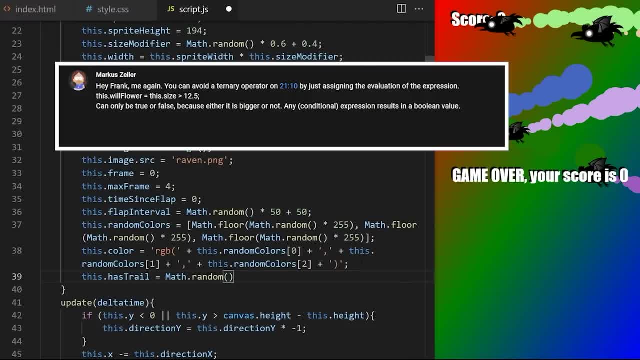 random called like this will return a random value between 0 and 1. so I call it and I check if that random value is more than 0.5, and that's it. it should be true. roughly for 50% of Ravens this conditional expression results in a. 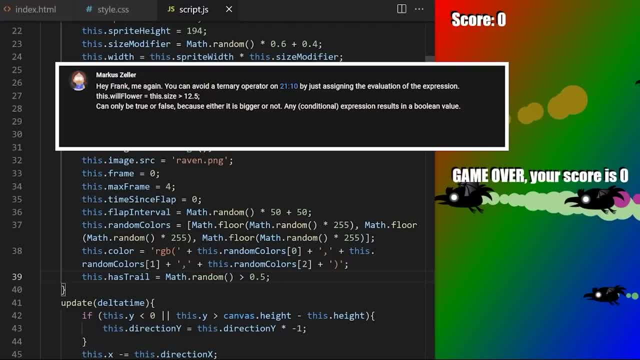 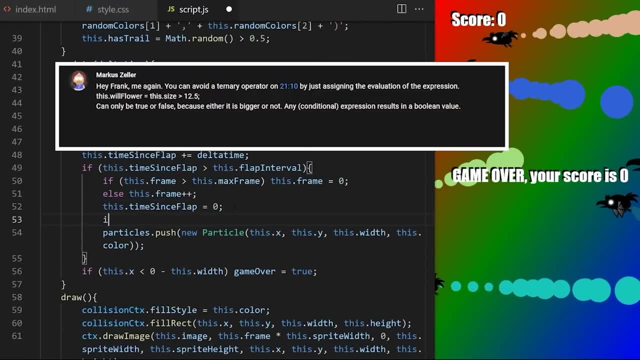 boolean value true or false, depending on if math at random rolls a random number that's higher or lower than the random value, then 0.5. I really like this syntax, very simple and clean. inside update method on Raven class. I will only create new particles if this dot has trail is. 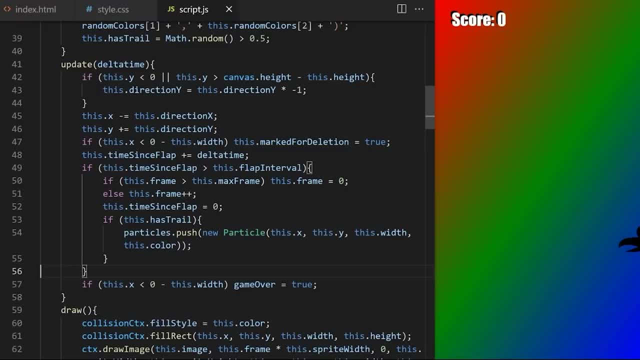 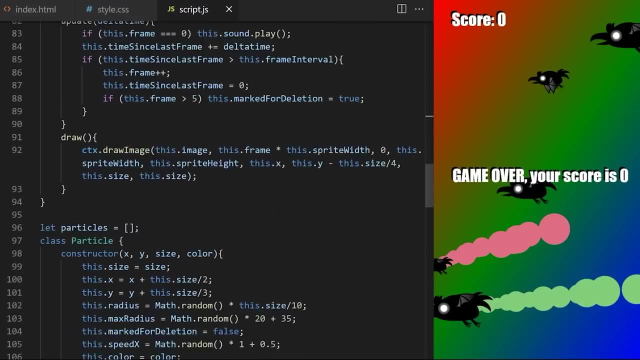 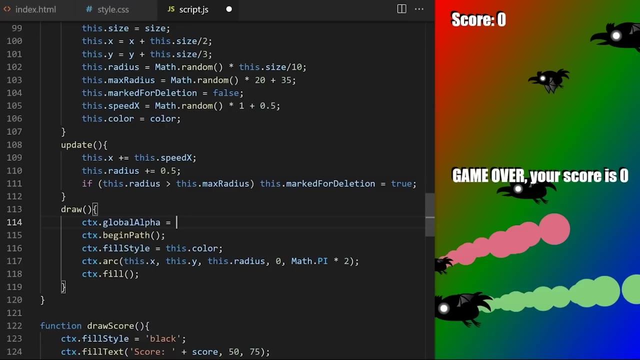 true like this. now, only half of my Ravens will have trails. I also want particles to animate from fully visible to transparent. inside draw method. on particle class: I set global alpha property on my canvas to be one which is maximum, fully visible minus the current size of the particle. 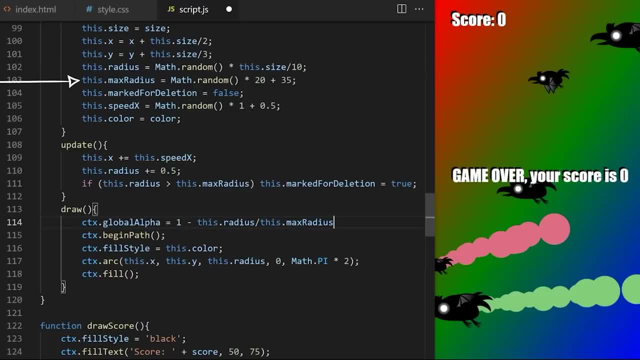 divided by max size. as the particles, radius grows, eventually radius will be the same size as max radius. so let's say max radius is 30 pixels. at that point where the current radius is the same size as max radius, we will have 30 divided by 30 here, which is 1 and 1. 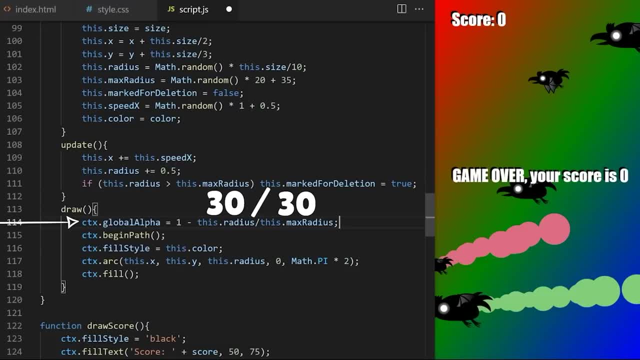 minus 1 is 0. particle is slowly growing more and more transparent and at the point when it reaches maximum radius, it will be at 0 global alpha. this formula might be a bit difficult to completely understand if it's the first time you see it, but it's very useful. we will talk. 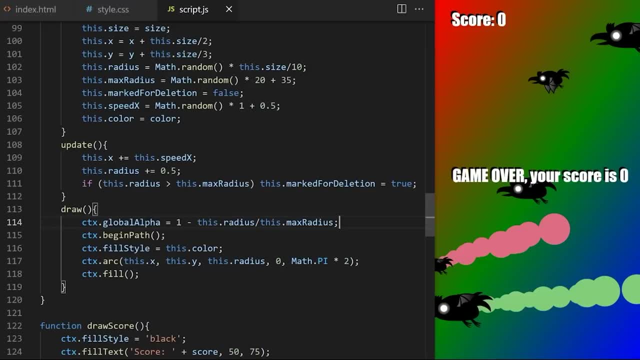 about it again in some other video. as you can see, global alpha is spilling over and affecting my Ravens as well. that's an easy fix if you want to change some global canvas properties, such as fill, style, global alpha, rotate, translate and so on, and you want those properties. 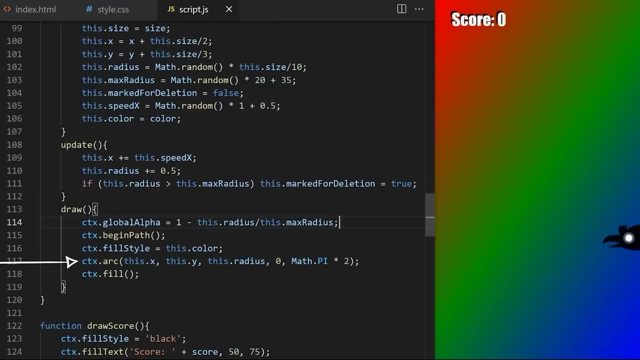 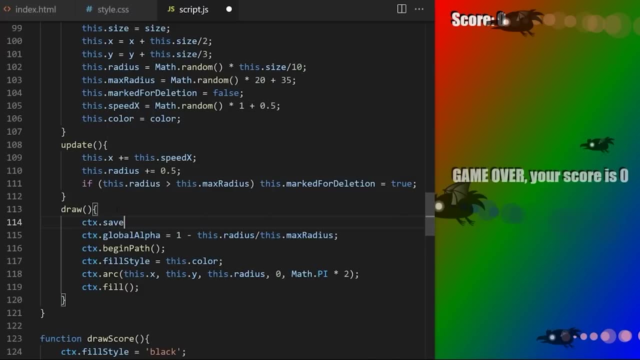 to affect only a single element you draw and not the others. you can just wrap that drawing code between built-in save and restore methods. save will create a snapshot of current canvas global settings and then we change global alpha here which will affect just this one particular particle, and then I 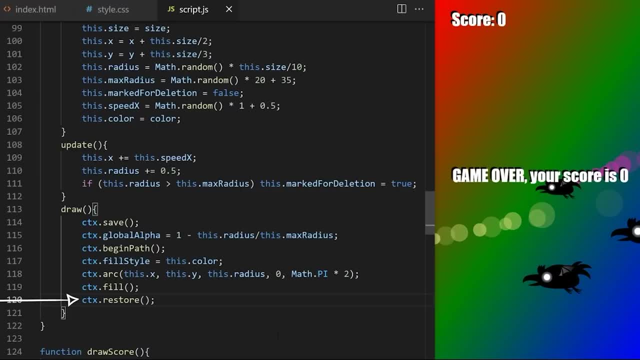 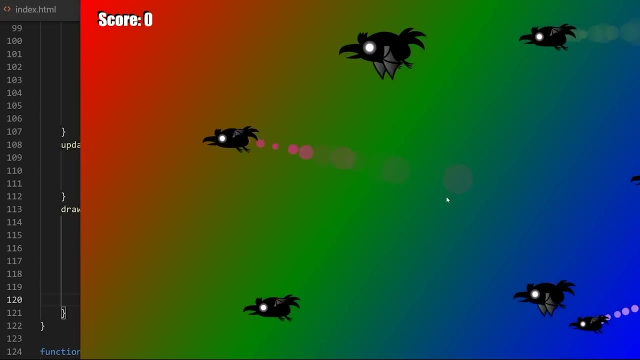 call restore to revert canvas settings back to what they were at this point. save and restore are especially useful for rotating elements on canvas, but you can also use them for other things, like data space. my particles are blinking before they disappear. it is because javascript first runs over the entire array before it. 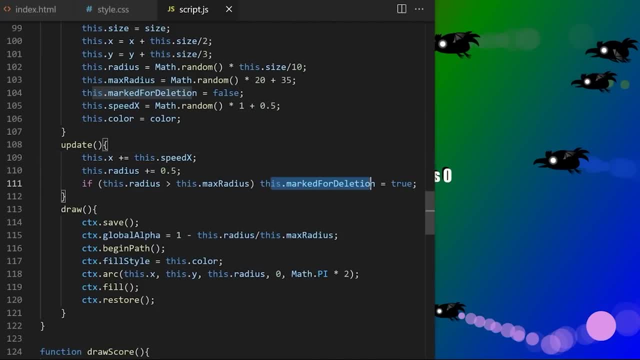 filters the particles that are too large out and my global alpha formula works only in a specific range between 0 and max radius. some particles get outside that range and are drawn fully opaque for a second before they get filtered out. to fix it is simple: I just trigger mark. 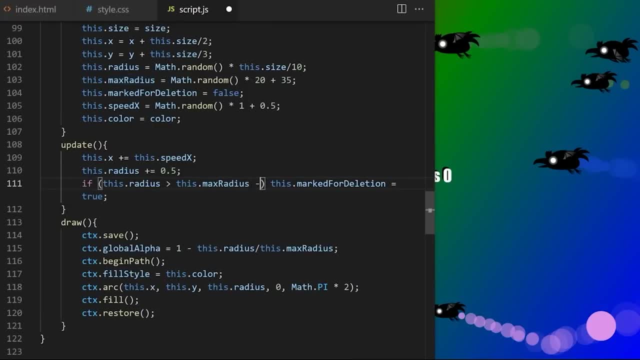 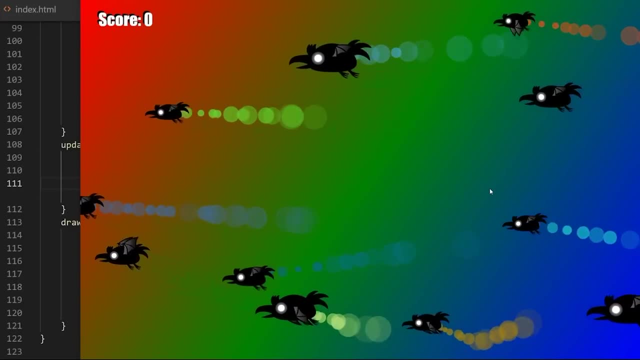 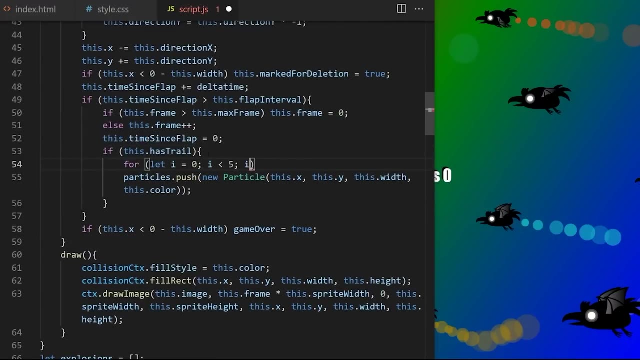 for deletion a little bit sooner, for example by saying max radius minus 5 in my check on line hundred and eleven. let's make the trail nicer. I will add five particles every time instead of adding just one. on line 54, I create a for loop like this and I put this code: 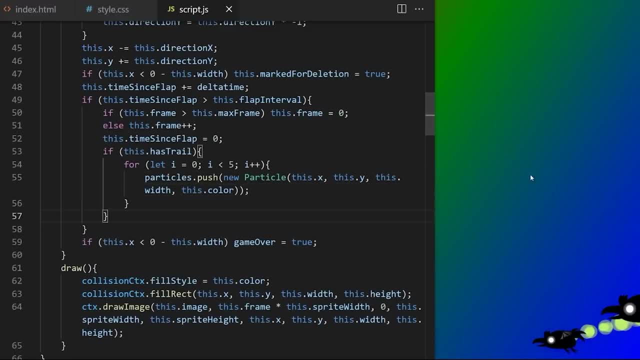 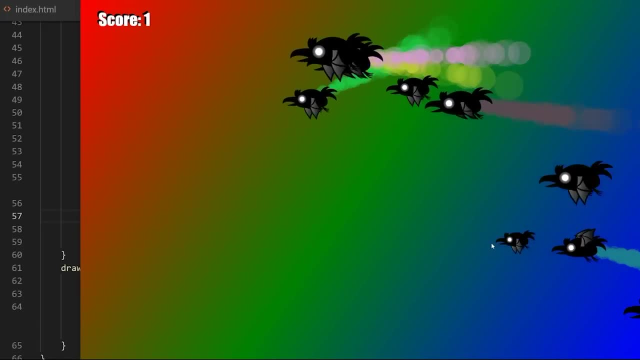 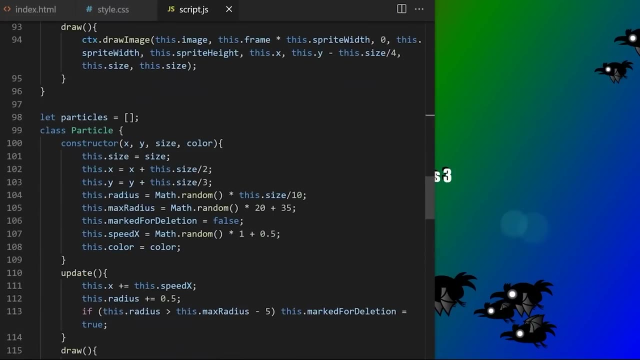 inside. if I make radius grow slower, trail will be longer because it will take particles more time to reach max radius. if I make radius, be a bit careful here not to have too many active particles on screen at once because at some point it will start affecting performance and frame. 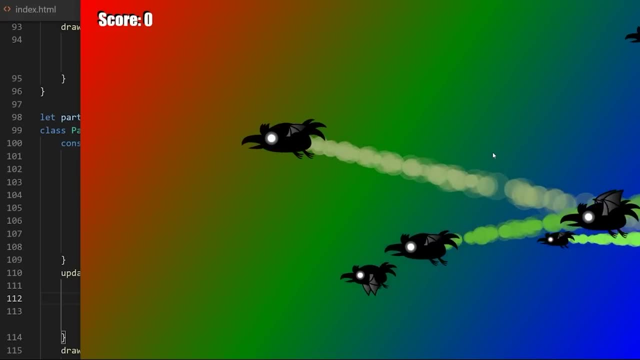 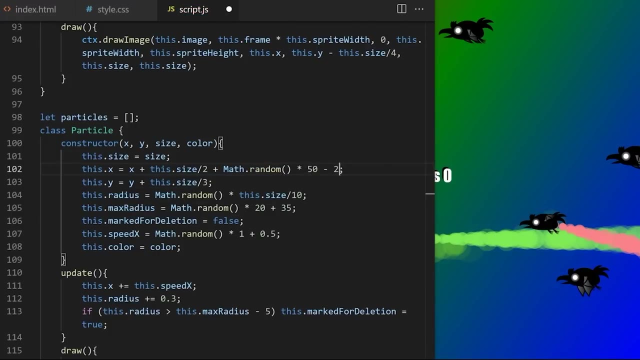 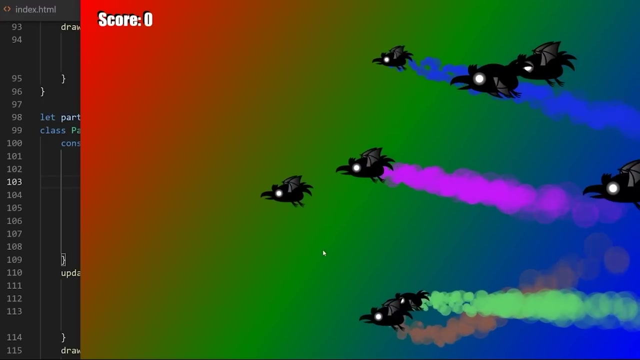 rate. I can also randomize the initial x and y coordinates a little. for example, I can add random number between minus 25 and plus 25. I think it looks a bit more interesting like this. I can also add more enemy types. for example, I can add: 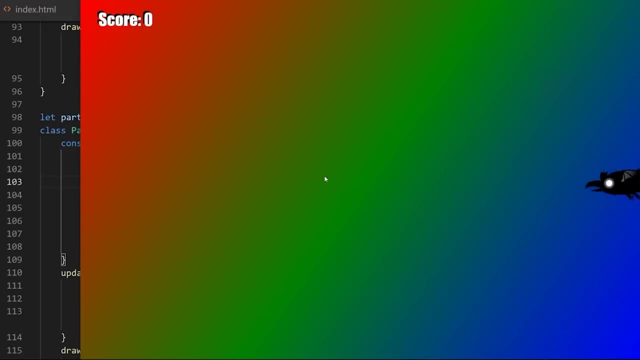 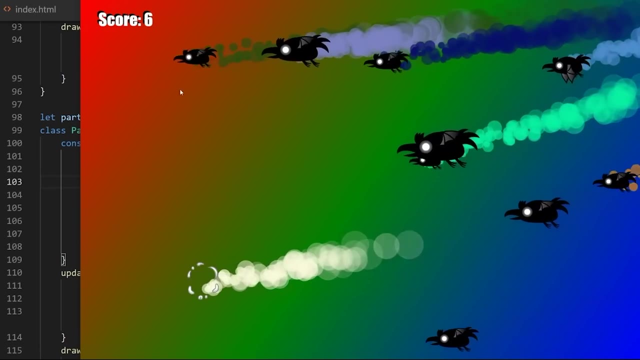 fast flying bats that will be worth extra score points. maybe I want Ravens with trails to be worth more score but also have more lives. there are many things we can do here. if you are still feeling creative, check out some of my playlists. I have creative coding for beginners. 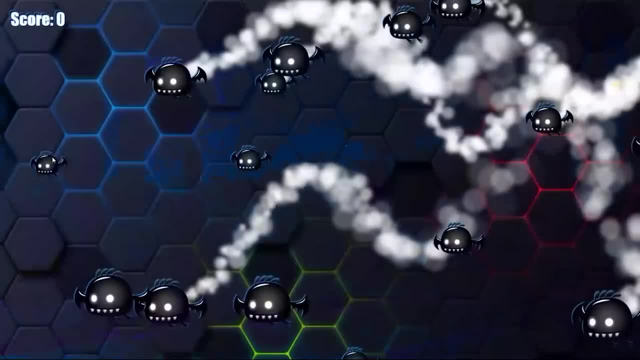 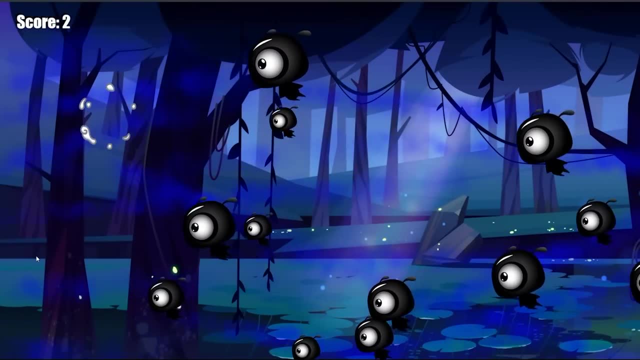 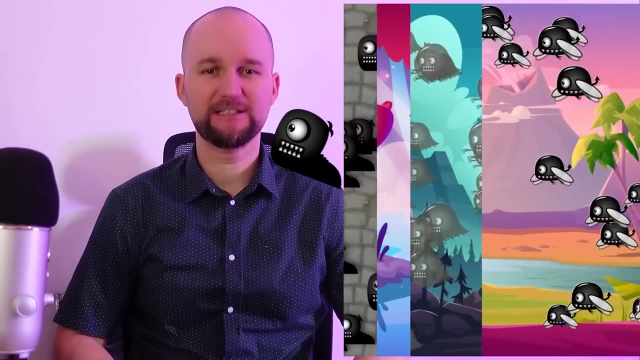 game development playlist and advanced animation effects, everything which is HTML, CSS and plain vanilla JavaScript. no frameworks and no libraries. check out some recommended courses in the video description. I'll see you there. if you want to build games with the JavaScript, all you need is a small set of tools. 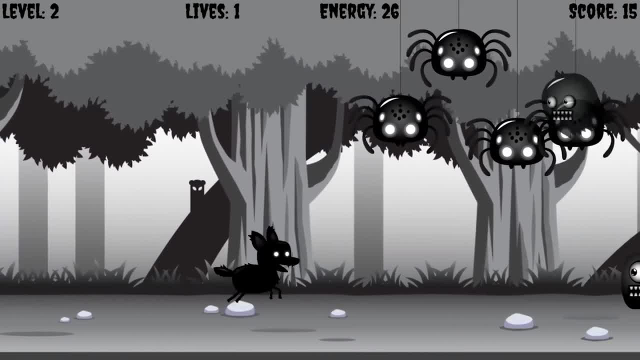 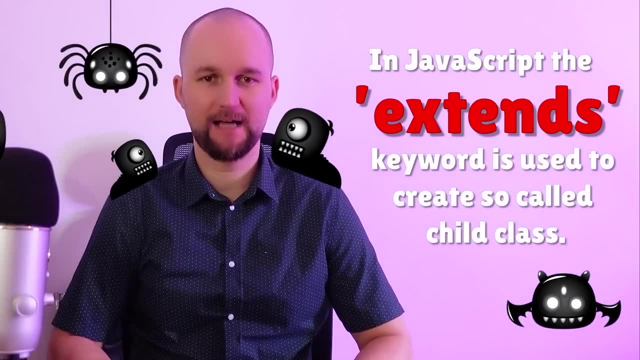 and techniques. let's add a couple more of them to our toolkit today and make sure we really understand them. in JavaScript, the extends keyword is used to create so-called child class. that way I can have my main parent class, where I define properties and values share between all my enemy types, and then I 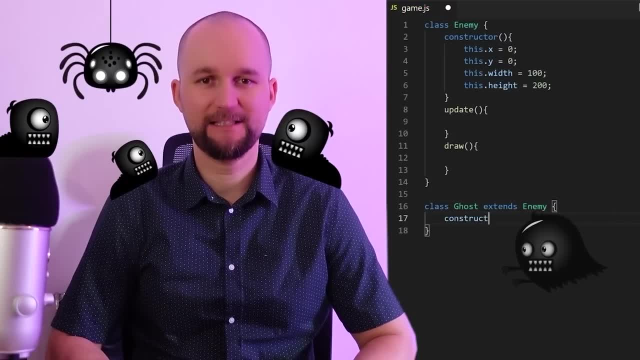 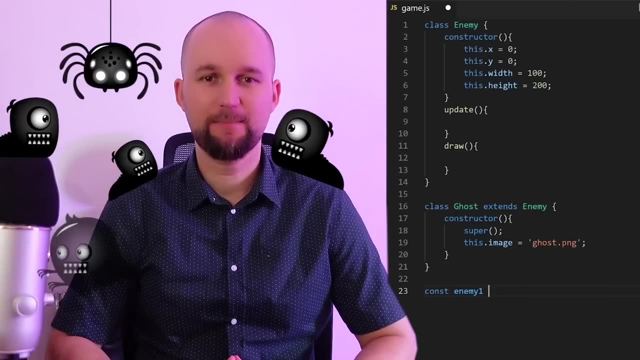 can have child subclasses that define specifics such as different visuals, different movement patterns and so on for each enemy type. then when I instantiate my ghost object I can add a new object and I call update on it. if JavaScript can't find update method on the ghost class, it will go look for it. 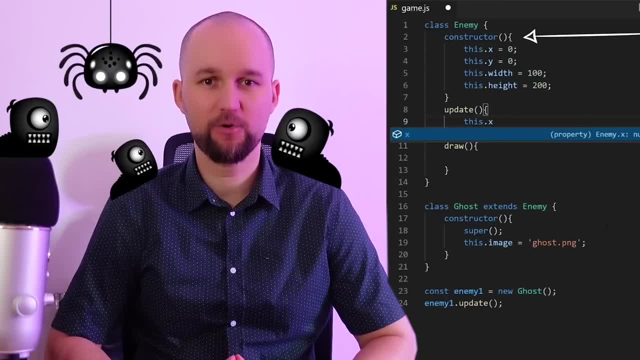 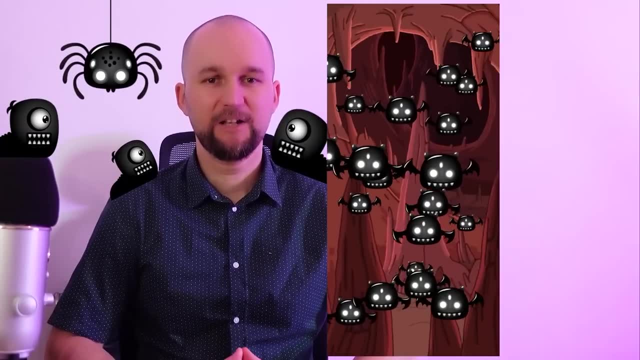 automatically on the parent enemy class and it will run the code from there. there is another special keyword called super. today, I will show you exactly when and how to use it. let's build a project step by step, completely from scratch, and in the process let's learn everything we. 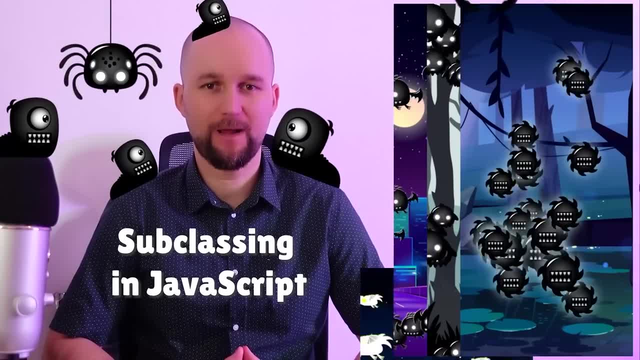 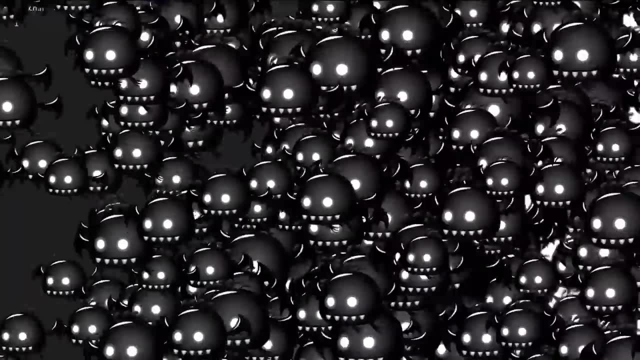 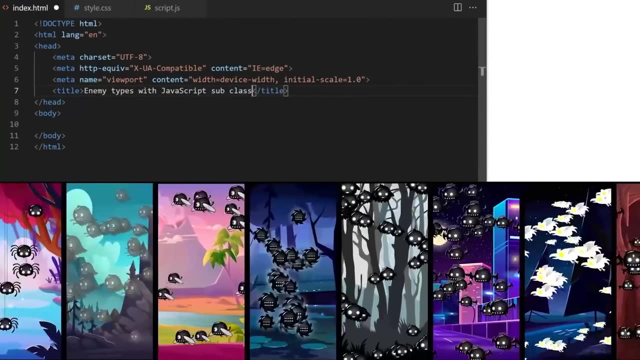 need to know about subclass in in JavaScript and how to use it to keep our code modular, clean and easy to read. this tutorial is for beginners. I will take you through the code in a way to make sure you understand everything. we will build a really fun animation. 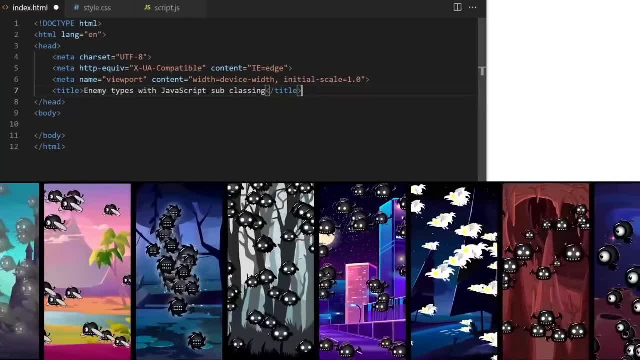 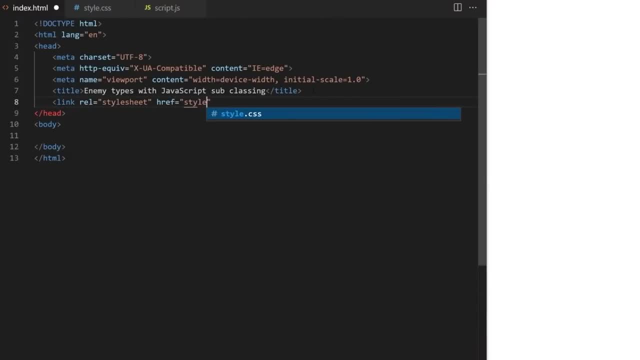 project and I will show you many game development techniques today. this video is independent and I will explain the code from scratch, but it's part of a larger series where I teach you tools and techniques you will need if you want to be a game developer or if you just 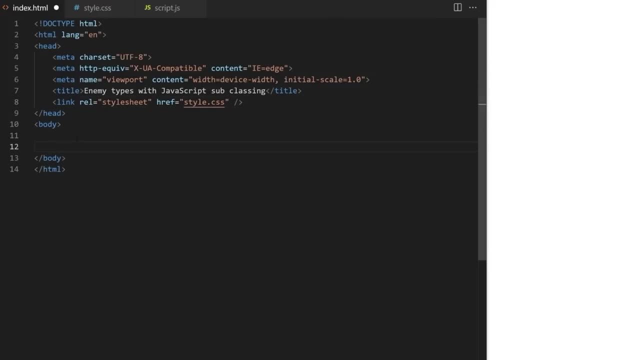 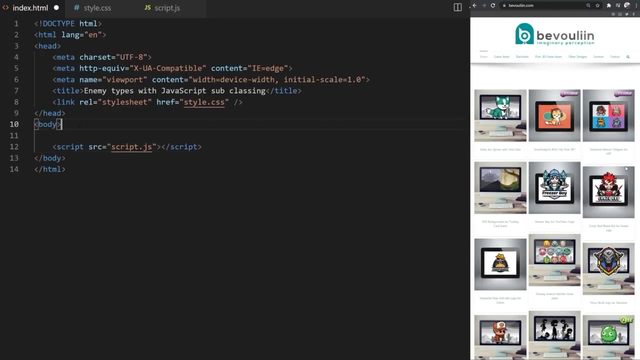 want to learn front-end web development and JavaScript on fun visual animation projects. if you code along with this, if you code along with me today, you will get three free premium sprite sheets so that you can get exactly the same result. check out this website for more beautiful game development art assets to. 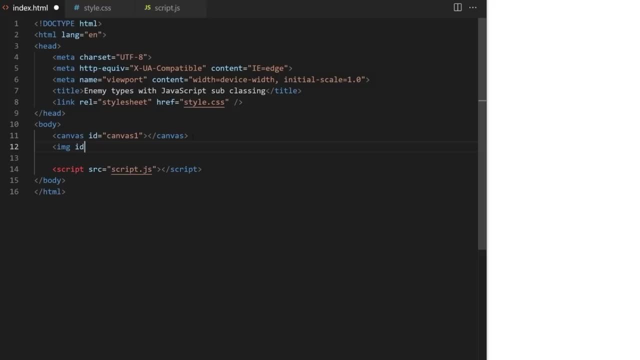 start my project. I create a basic web page boilerplate markup, I link style CSS file, JavaScript file and I created HTML 5 canvas element with an ID of canvas 1. I bring my three images into the project by creating three IMG tags with IDs: worm, ghost and spider. you can find these. 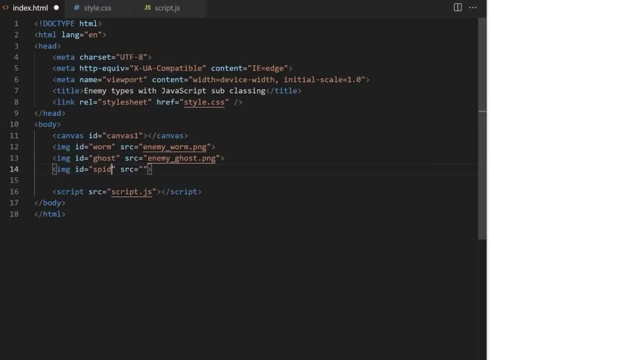 images to download in the video description. it might be a good idea to use the same images as me at first and then modify the code and use your own art assets. once you get everything working, it might save you a lot of time debugging if you follow exactly what I'm. 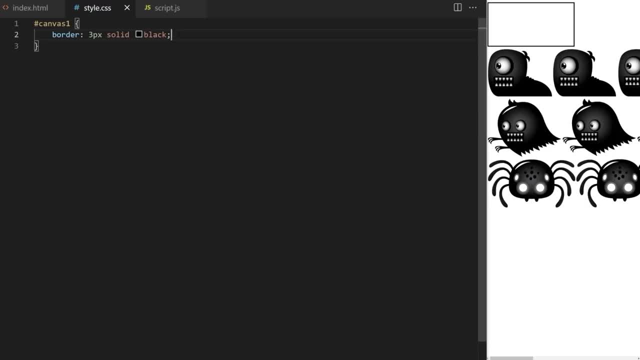 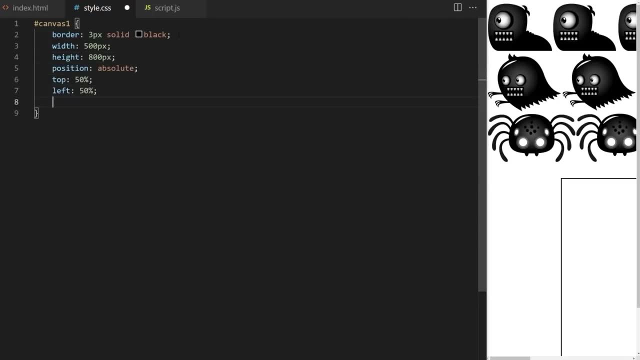 doing, especially if you are a beginner. I give my canvas a border width and height and I position it with CSS in the middle of the page. I will also hide the project images with images. we will draw them and animate them with JavaScript in a minute by including images as image tags. I can. 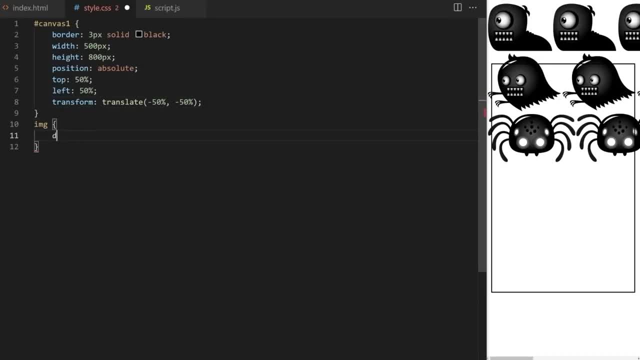 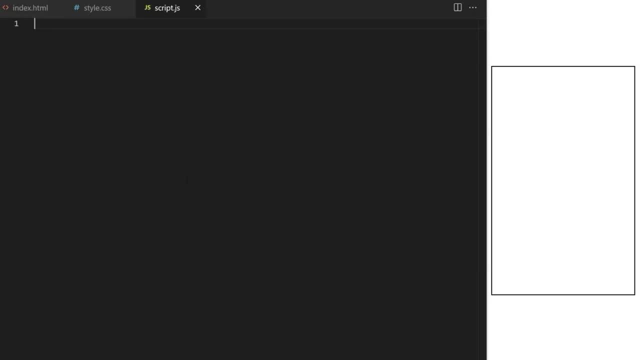 make sure they are fully loaded before my JavaScript code runs by using load event listener. it will prevent potential errors. I will show you exactly what I mean as we go along. I set up my canvas using these four lines of code, as usual. let's outline the entire project. 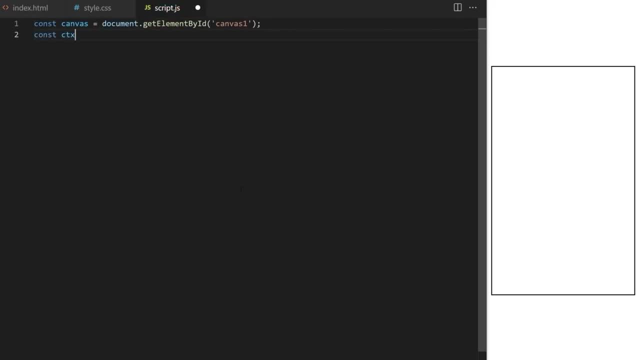 structure now so that you can see what functions and classes we need and how they are connected to each other. when we have the complete project structure, we will be expanding on individual parts to add more functionality. the most important thing today will be my game class. I will use it as the wrapper that 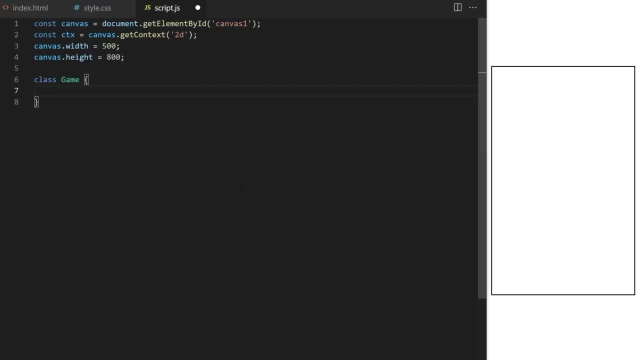 contains and controls all movement and animation, logic and basically everything else. it's a JavaScript class, so it will need a constructor which is a monitor method for all JavaScript classes. it will also have update and draw methods in game. class constructor. I create a property, I call this dot. 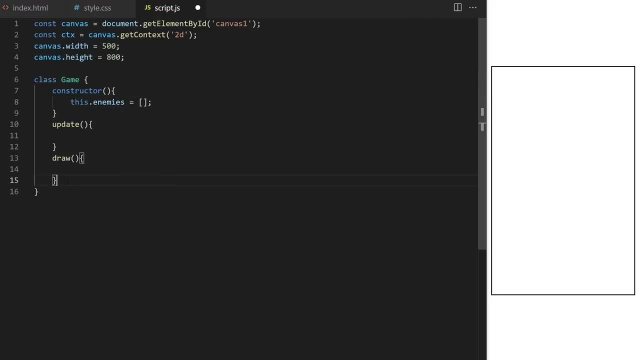 enemies. my game object will hold an array that contains all enemies like this. my game class will also have a private method called add new enemy. this method will be called every time I need to create and set up a new enemy for my game. if methods name starts with a hash. 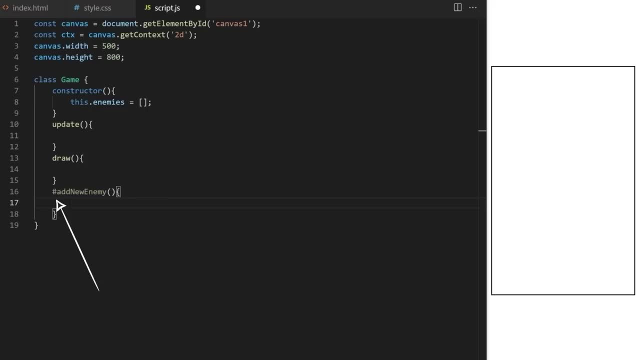 symbol like this, it will be a private class method. it means it can only be called from within my game class to manage some kind of internal functionality, in our case adding a new enemy into this dot enemies array from line 8. if you try to call this array, 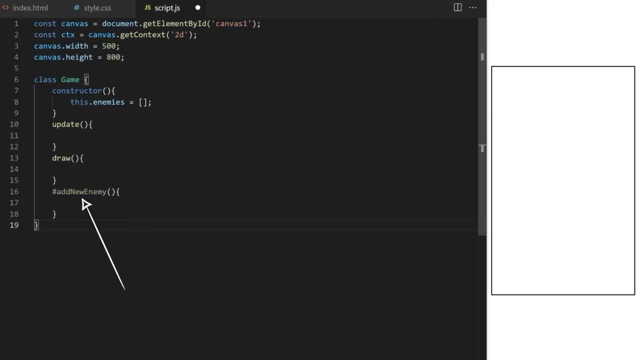 this private method from outside game class, you will get an error. notice that update and draw methods are public because I will need to call them from my animation loop from the outside a bit later. my add a new enemy private method will need a way to create new enemies. 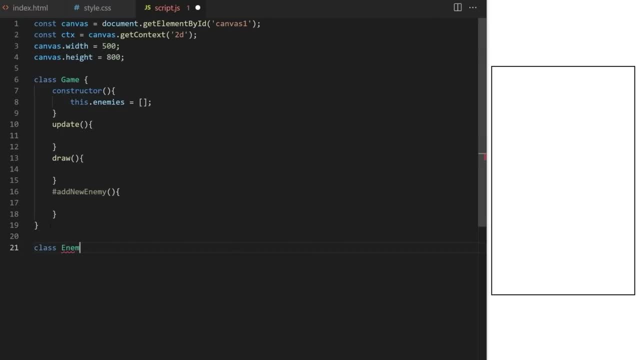 for the game. so we will write another class I call enemy and inside we declare a blueprint whenever I call this enemy class from inside. add new enemy method. it will create one new enemy object for me. I will show you how to make animated ghosts, worms and spiders. they will all. 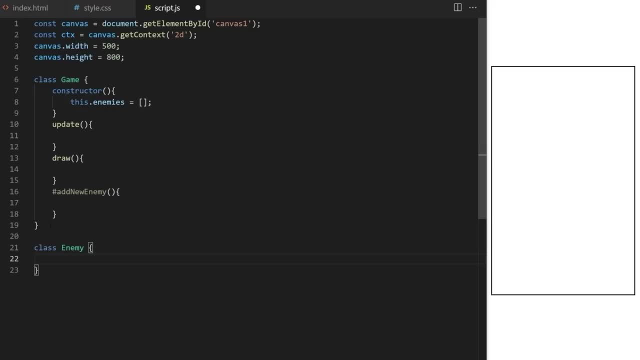 be created by this enemy class, but they will have different animations and different behaviors to make our game more interesting and maybe more difficult for the players. so again, as you know, every class needs a constructor to hold the blueprint and we will also have update and draw methods. 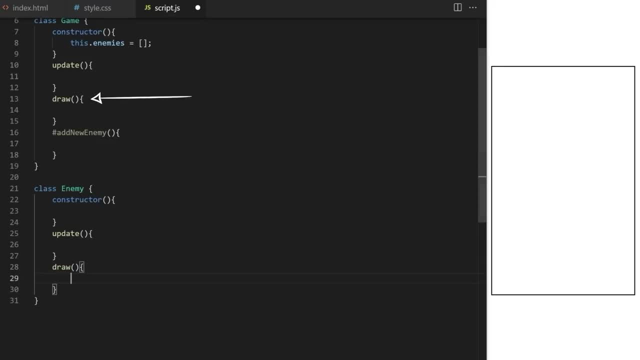 here. update and draw method on game object: here will be handling, updating and drawing my entire game, for example, all enemies, player, obstacles and backgrounds, menus and so on. update and draw method here on the enemy class, will be handling only each individual enemy, such as their position, movement pattern. 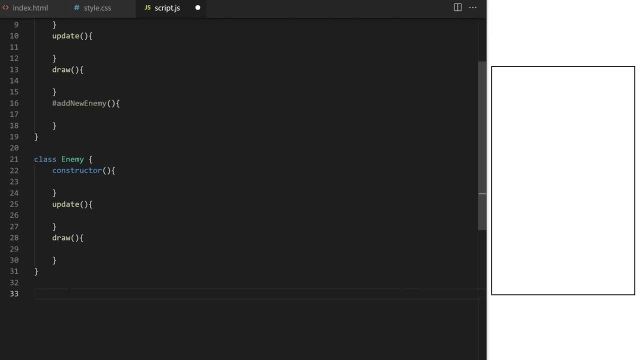 sprite, animation and so on and finally, to complete the skeleton of our project, we will need a custom animate function that will call what needs to be called and a loop around to move and animate things in our game. here in animation loop, I declare what happens in our game frame. 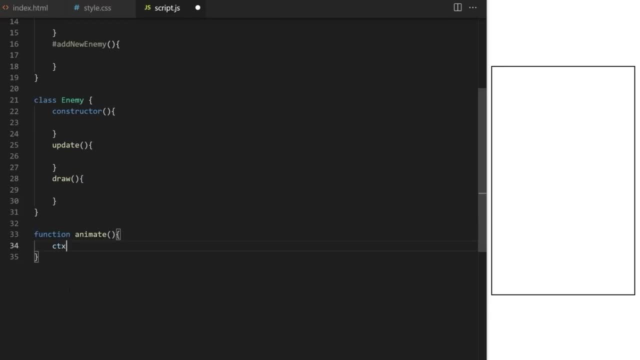 by frame. at first we will call built-in clear rectangle method and we will clear old paint from the entire canvas. so from coordinates 0: 0 to coordinates canvas width, canvas height. if you are a complete beginner, this is horizontal x-axis and this is vertical y-axis. so 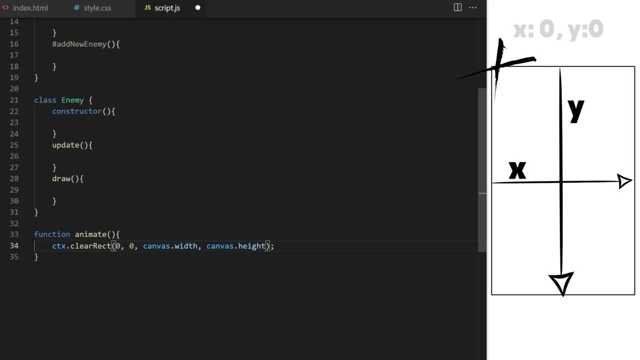 point 0: 0 is here and point X, 200, Y, 200, for example, is here. this is the basic thing you need to understand if you want to draw on canvas. so we cleared old paint from canvas to make sure we can only see the current animation frame. so 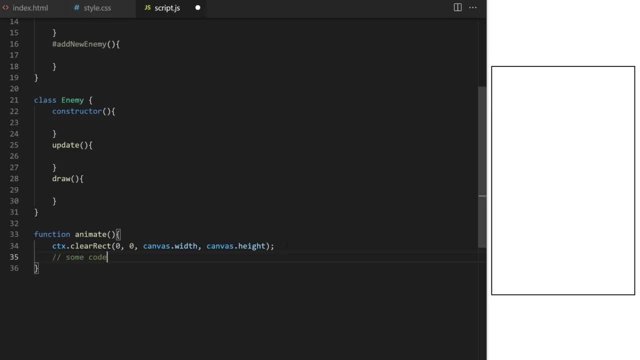 we will create a loop in our game. we write some code here depending on what we want to happen in our game, and we call request animation frame built in JavaScript method, which will simply take function we pass to it and it will call it once animate will run its code. 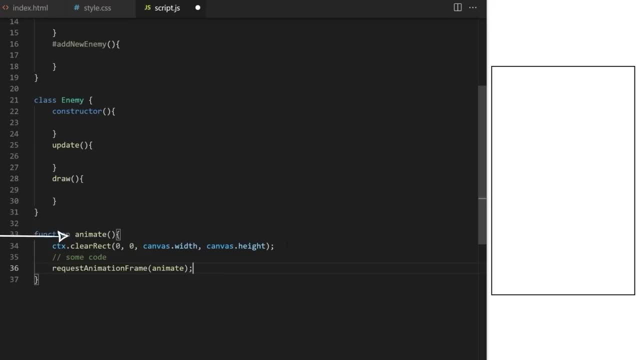 and call itself again. run its code and call itself again over and over. this is how you create animation loop. I don't want any of this code to run until I'm sure my web page, including canvas element and all project images, have been loaded. so I highlight all the code and I 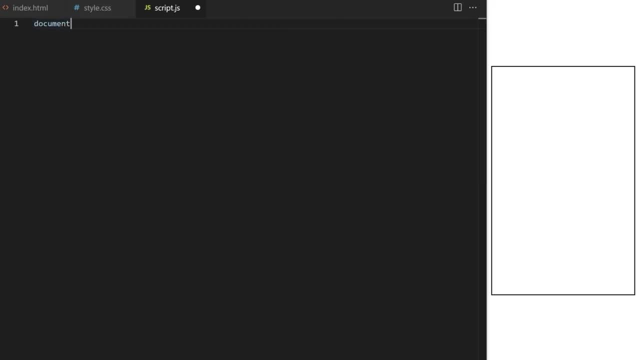 cut it for a second. I want to put it inside: load event listener: document dot at event listener and we will listen for Dom content loaded JavaScript event. I actually made a mistake here, because Dom content loaded event fires when the initial HTML document has been loaded and parsed. but 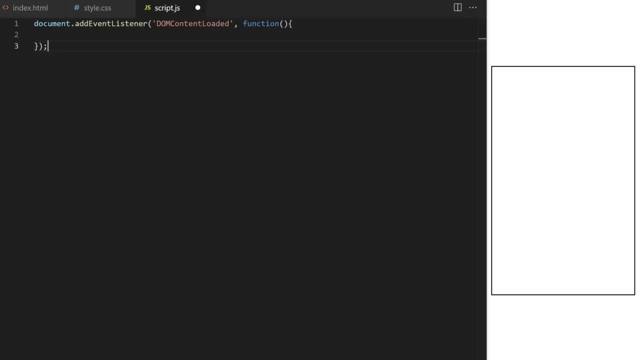 it doesn't wait for style sheets and images. the correct event listen for here is the load event, which only fires when the whole page has been loaded, including all dependent resources such as style sheets and images. so please replace Dom content loaded event with load event here. you will not notice any difference. 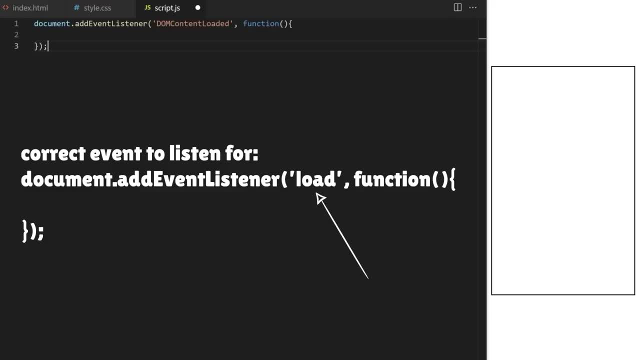 if you are working locally, because images will load instantly. but if you are loading images from an online server somewhere, load event is the one you need here. so I paste all the code back here inside my load event listener. we have kind of a setup main game class. 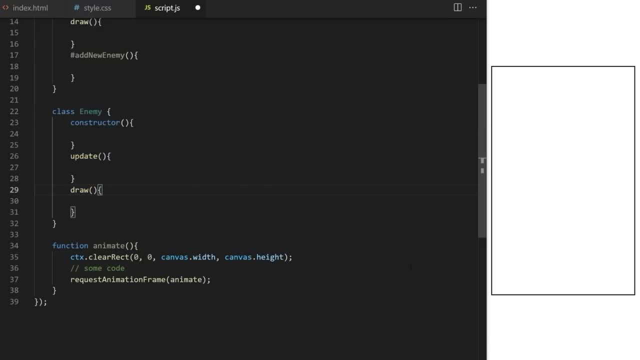 enemy class and animate function. and if you want to animate something, it's important that it runs at the same speed on slow old computers and on brand-new gaming super PCs. not every computer is able to serve frames at the same speed. also, some screens have different refresh rates and request animation. 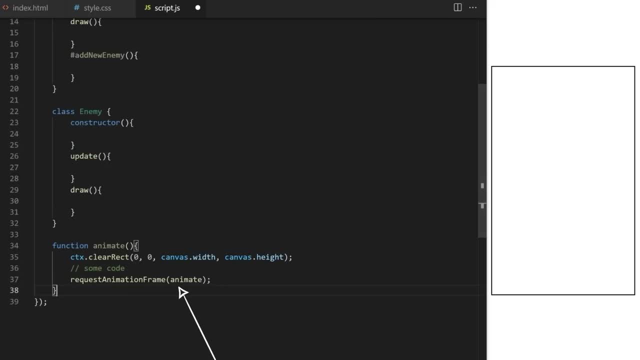 frame adjusts when it serves the next frame based on screen refresh rate. so what I want to do now is count how many milliseconds happened between frames, and only when we reach certain threshold we will serve the next frame. since we are passing animate as an argument to request animation frame here, request. 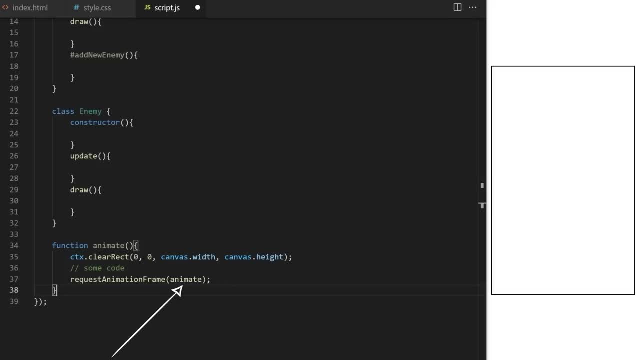 animation frame has another secret feature: it will pass an automatic timestamp argument to the function it calls, so our animate has access to timestamp argument, which was automatically generated by JavaScript, because I called animate using request animation frame. here I want to calculate the difference between previous and current animate call in milliseconds. 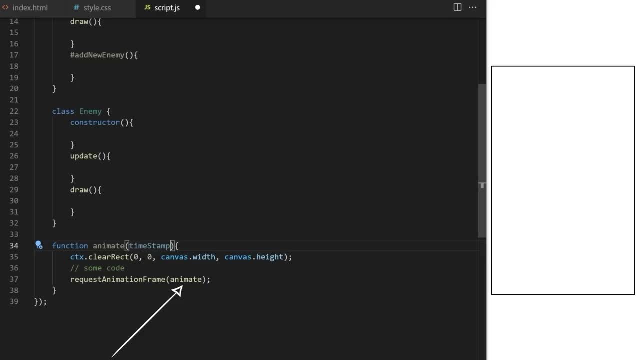 difference between frames in animation is also called Delta time. simply explained, as request animation frame runs over and over it is passing animate this automatic timestamp argument. I want to know what is the difference in milliseconds between previous timestamp and timestamp from the current loop, so-called Delta time. I will calculate it. 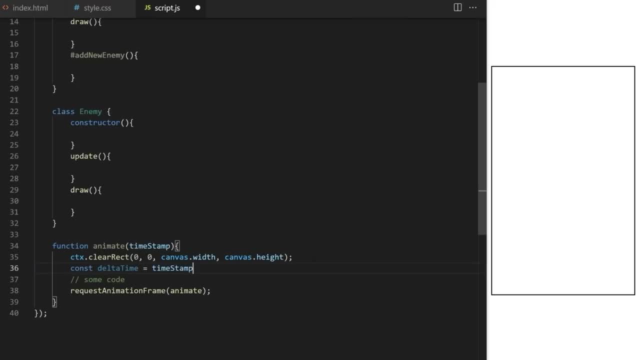 by saying a timestamp that was passed in this loop minus timestamp that was passed in the previous loop. I will call it for example: last time, after I use last time variable that was holding old timestamp from the previous loop to calculate Delta time, I can reassign last time to the new timestamp from this. 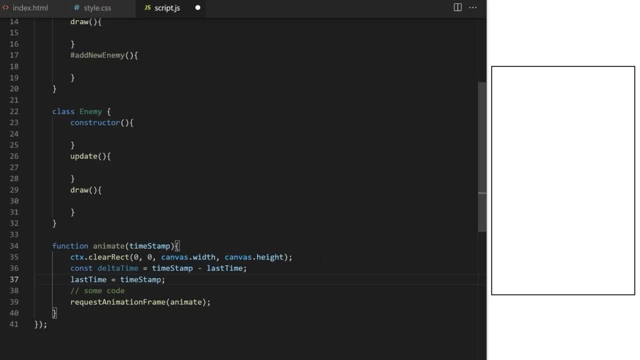 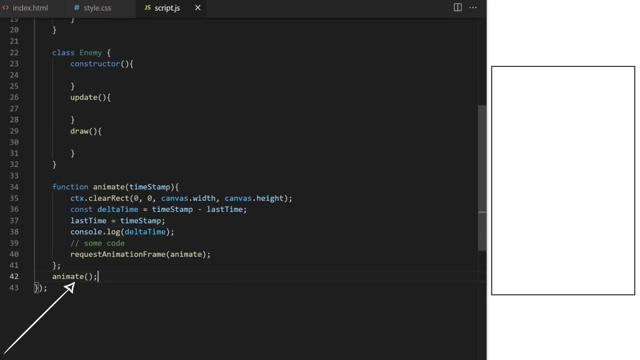 loop so that it can be used in the next loop again. let's console Delta time to see if it works here. I declare animate. I also need to call it to start the first animation loop. oh yeah, last time is not declared. I declare it right here and I. 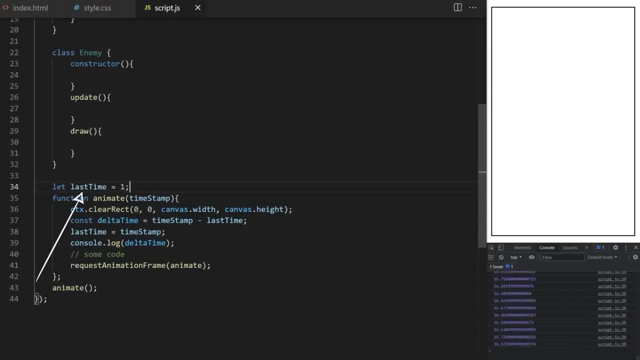 initially set it to one. this value of one will only be used for the first loop, because on the second loop it will get reassigned to the current timestamp in console. I can see my Delta time is around 16 milliseconds. this is very common refresh rate for most computer. 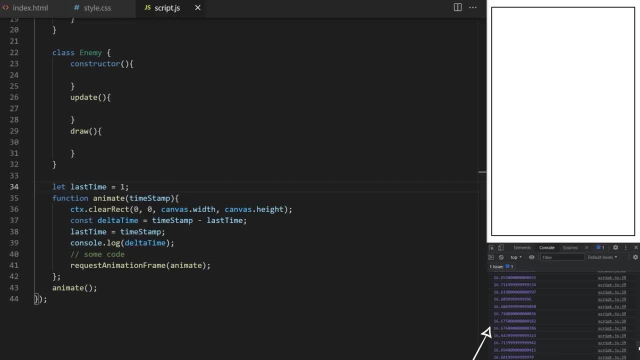 screens. but if you have high refresh screen you can get a lower number here, and if you have old computer you can get higher number here, especially when you create a bigger project where you animate many moving parts. at this point even very slow computer should handle 16 milliseconds Delta time time between 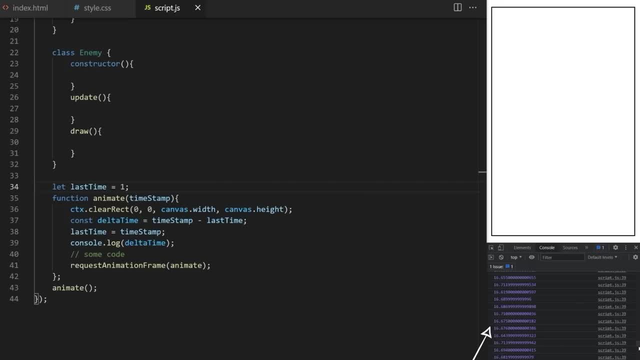 animation frames, since our game doesn't have any graphics yet. if I scroll in console all the way up to my first Delta time console logs, I can see the initial call was none, not a number. it's because animate only receives automatic timestamp argument here when it gets called by request animation. 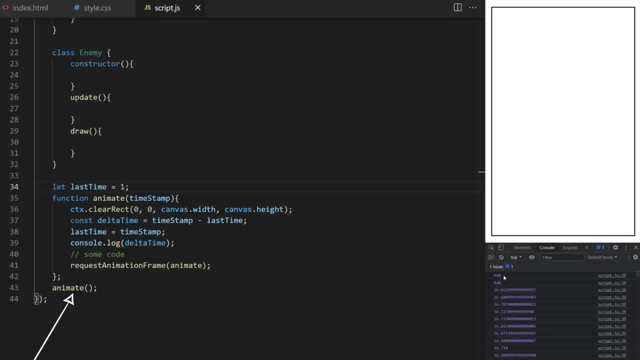 frame on the very first initial call. it doesn't have any timestamp argument, so I will pass it 0 just for that first loop. now we know how to calculate Delta time number of milliseconds between frames. faster computers will have lower number. slower, old computers might have higher. 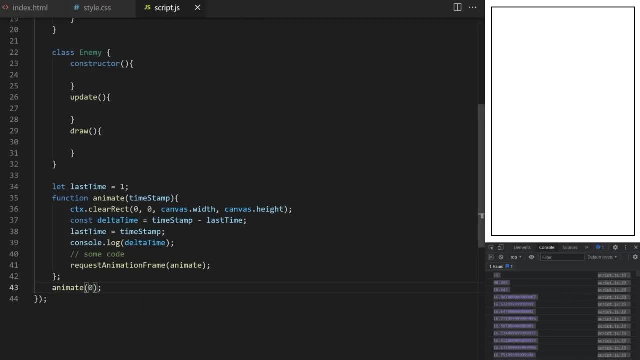 Delta time because it can take them more milliseconds to serve the next frame. since we have this Delta time value, we can adjust animation speed with it to make sure our game runs at the same speed on slow and fast computers. I will show you where and how to use it, as we 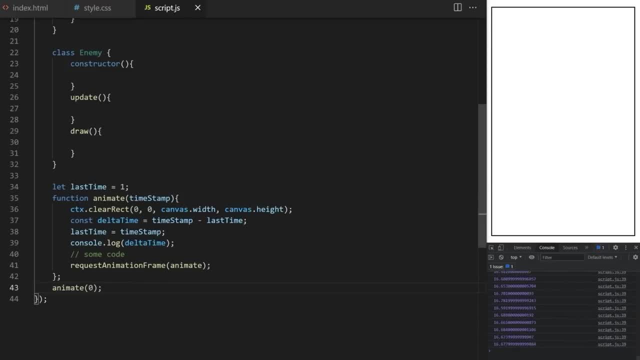 build our project and start animate and move game characters around on canvas. console log like this can cause performance issues, so don't forget to remove your console logs when you don't need them anymore. on 922 I have my enemy class. it has a mandatory constructor method which will be used as a blueprint. 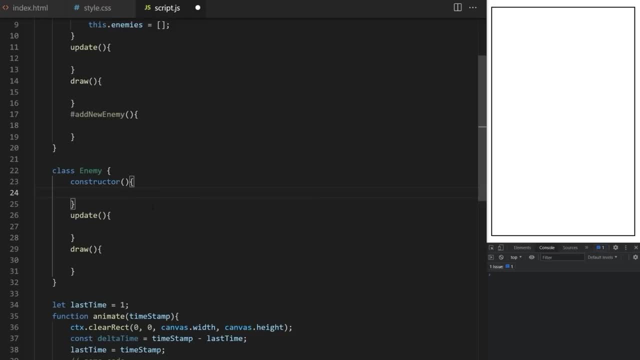 to create one new enemy object. whenever I call this class with a new keyword from somewhere in my project, let's write that blueprint and inside we declare properties and values of our enemies. each enemy will need X&Y starting coordinates so that JavaScript knows where we want to draw them on canvas. I 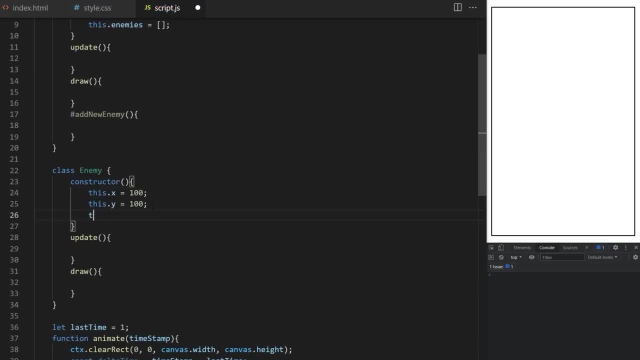 will first hard code coordinates: 100, hundred. we will change that in a minute. I will also give each enemy width of hundred pixels and height of hundred pixels. update method on enemy class will just move the enemy by one pixel to the left. draw method on my custom enemy: 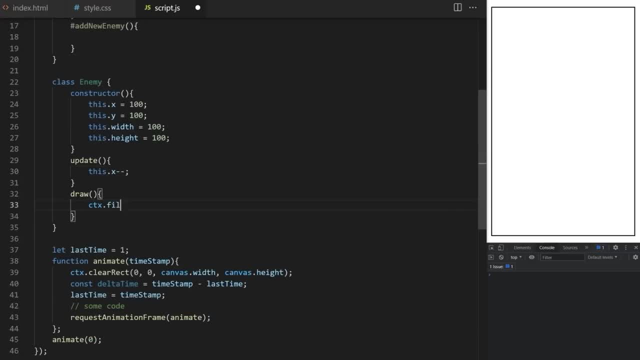 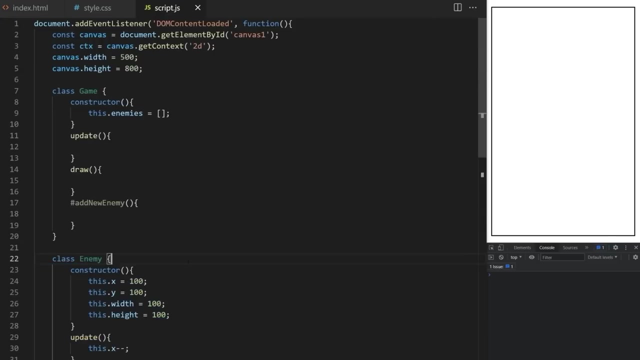 class will call built-in fill rectangle method and it will first draw a black rectangle representing my enemy. I pass it this dot X from line 24, this dot Y, this dot width and this dot height. great, we have enemy class. now we can call it to create enemy object and add it to our. 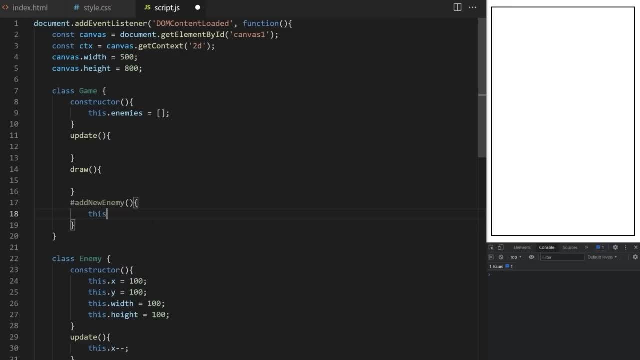 game inside. add new enemy: private method. I take this lot enemies from line 9 and I call built-in push method. push method can be called on arrays and it will take whatever we pass to it and it will push that at the end of the array. so I pass. 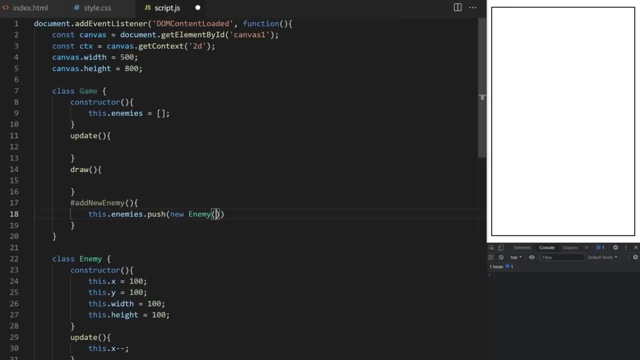 it new enemy. the new keyword is a special command in JavaScript. it will make JavaScript look for a class with the name enemy and when it finds it, it will take its constructor and use the blueprint inside to create one new blank JavaScript object and assign it values and properties based on instructions. 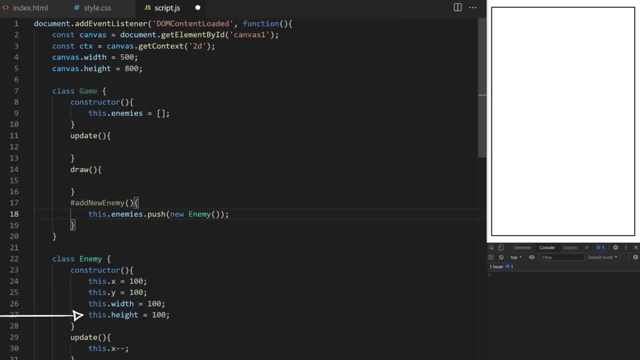 inside the blueprint that new enemy object will also automatically have access to update and draw method on enemy class. when you instantiate object with the JavaScript it will run its blueprint inside constructor. so I will do something which might look a bit strange to you. any code put inside the 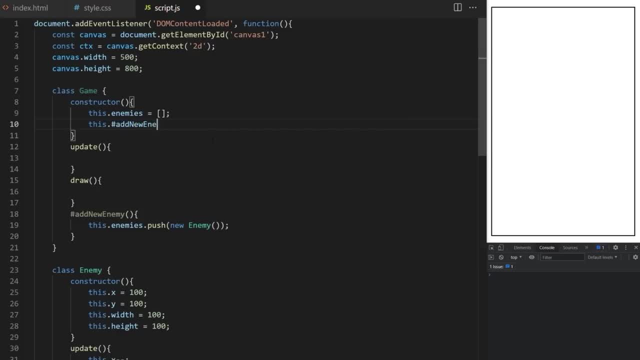 constructor will be executed in the same way I did when you create new instance of that object with the new keyword. so here, when I create new instance of my game object, I will create enemies array and I will call its private add new enemy method automatically, which will push new enemy. 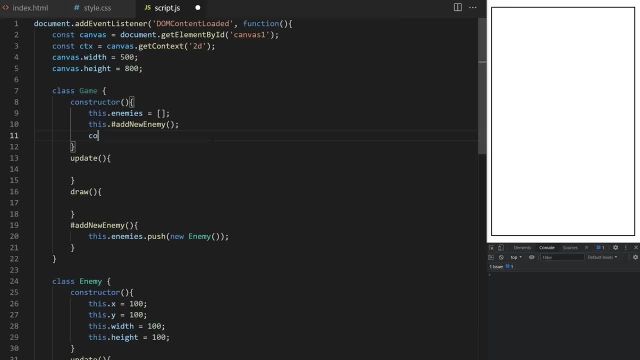 inside enemies array to check if that really happened. I will also console log this dot enemies. to execute all this code here, all I need to do is to instantiate my game class. so let's do it down here. on line 39, I create a new constant variable. I call, for example: 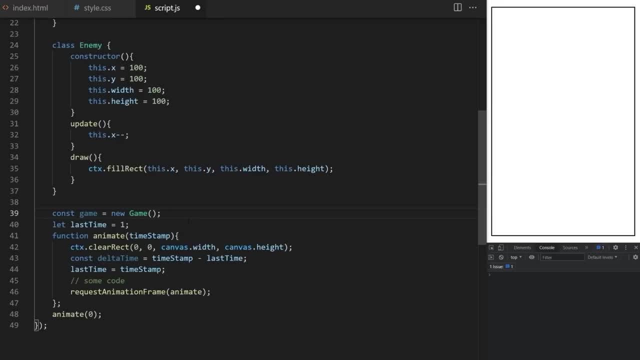 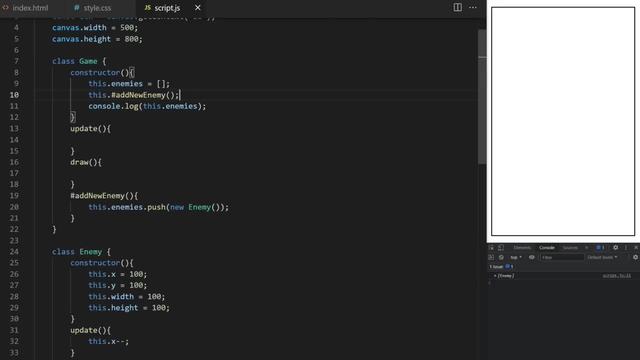 game and I set it equal to new game. like this, doing that created one new blank game object and a train code inside constructor here on line 8. so this console log from line 11 is showing that this dot enemies from line 9 contains one new enemy object. perfect, you can see. 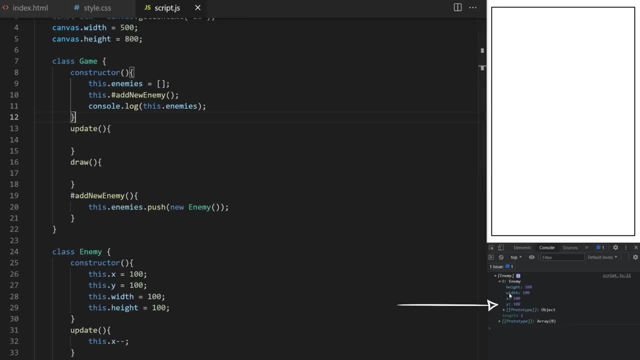 that enemy object has X&Y width and height as we declared here on line 25. now inside update method on game class, I will cycle through all enemy objects inside this dot enemies array and I will call their update method from line 31. I hope you know syntax of for each method. 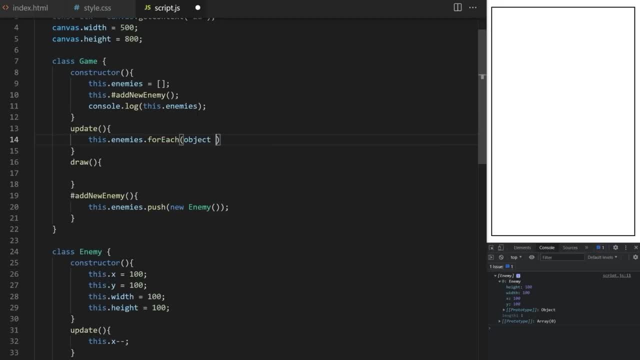 I'm simply saying here: take this dot enemies array from line 9 and for each object in this array run their associated update method. this is es6 syntax, so called arrow function. I will also take the same enemies array from line 9 and I will call draw method from. 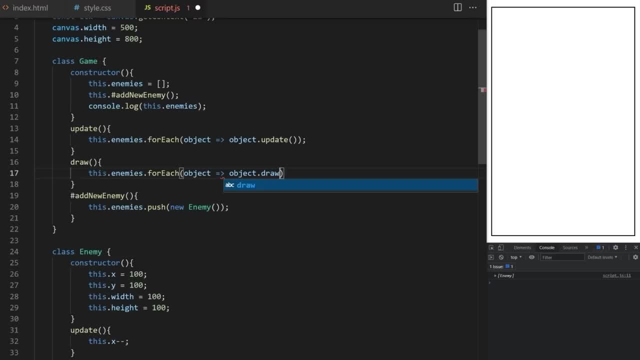 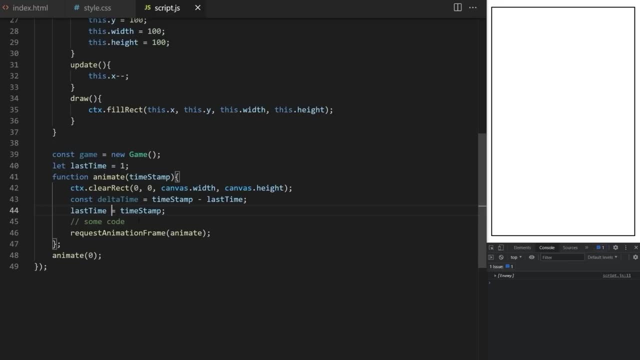 line 34 on all these enemy objects. currently there is only one inside, but there can be many more down here inside my animation loop. I take instance of my game class from line 39. I call update method, we just wrote- and I also call draw method. and here we. 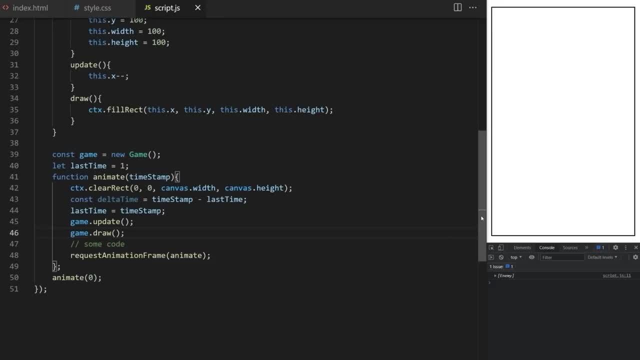 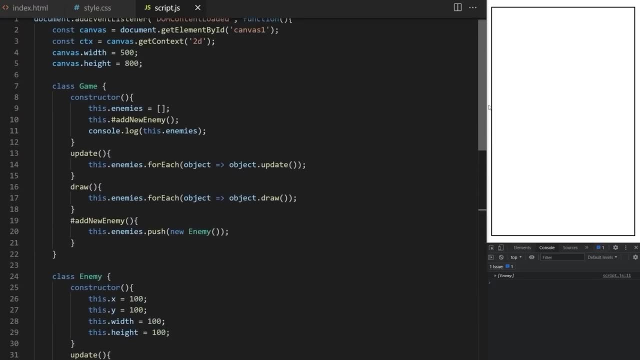 are animating one enemy in our game. hope you can see advantages of code structure like this. let's say I also have array of obstacles, background layers, power-ups, players and so on. I can call all of these from update and draw method on my game class to get everything moving. 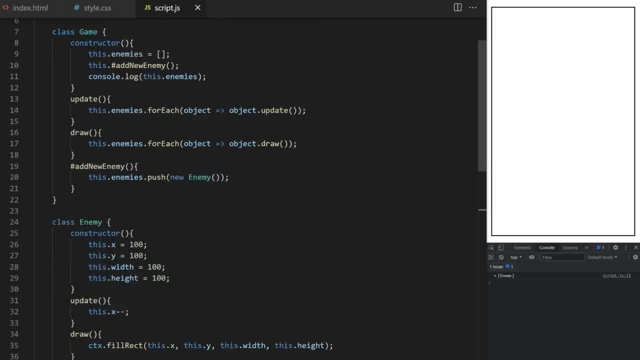 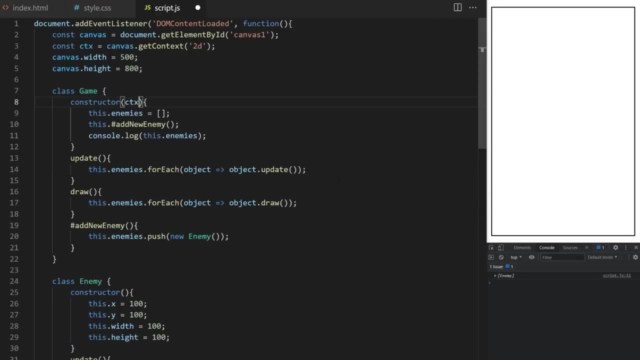 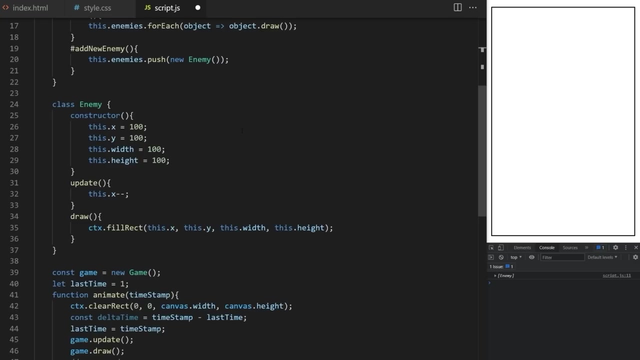 with very little code from a single wrapper function, keeping my code clean and organized this way. it's a good practice not to use global variables inside our classes, so I will take context width and height and I will put them inside my game class. these arguments will be passed here, on line 39. 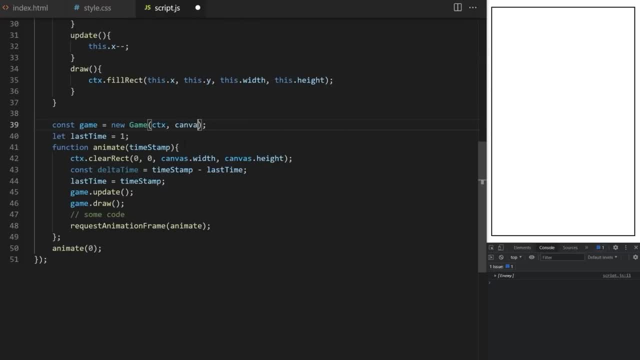 when I create an instance of game class. so I pass it CTX from line 3 to tell JavaScript which canvas I want to draw on. I will define width of my game by passing it canvas width from line 4 and canvas height from line 5. 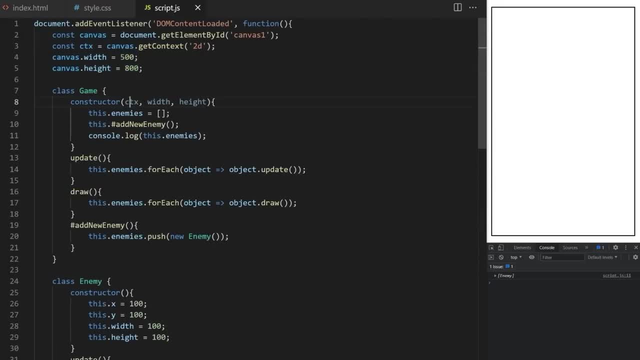 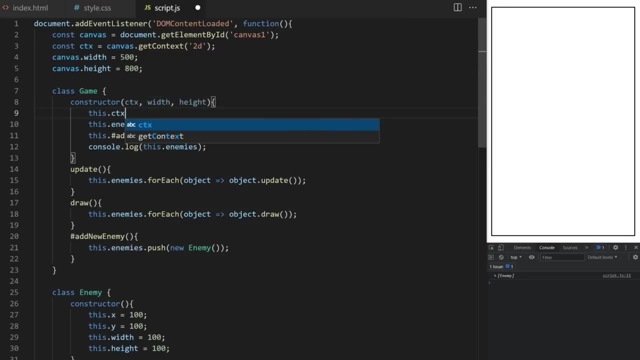 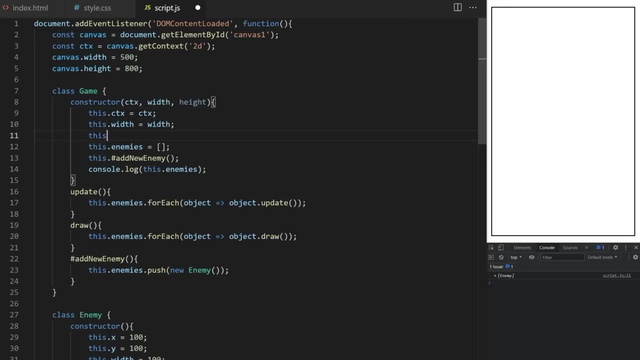 these three variables, just as my game class constructor expects here on line 8, then I take these arguments and convert them into class properties. this dot CTX is CTX passed on line 8, this dot width is width and this dot height is height. now I converted public variables into: 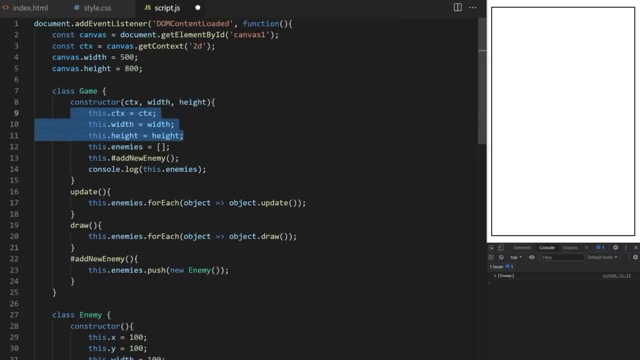 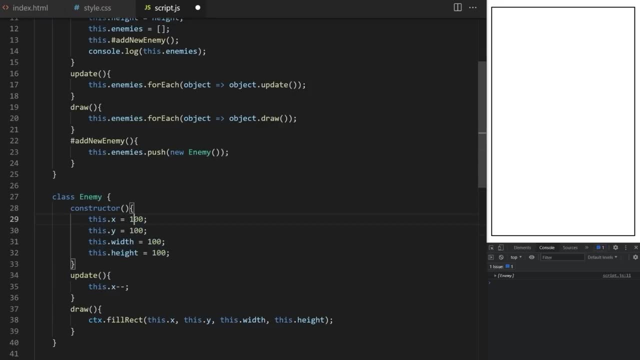 class properties and I can pass them around when I need them by passing game object. as an argument I will show you. let's say, I need width and height of my game inside the enemy class because I want my enemies to appear behind the edges of game area on line 23, when I 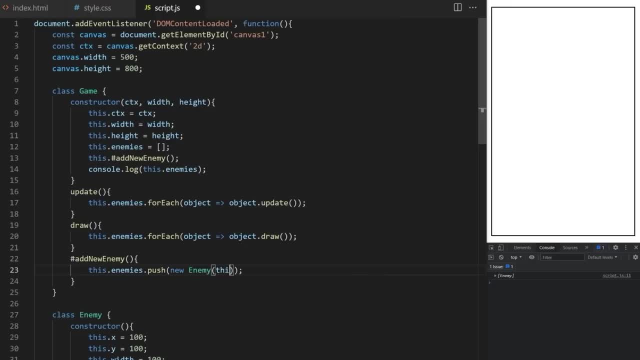 create new enemy object, I will pass it this keyword, which here refers to the game object we are currently inside. that game object will carry all references to its width, height and other properties with it. let me show you so I'm passing this keyword and inside my enemy. 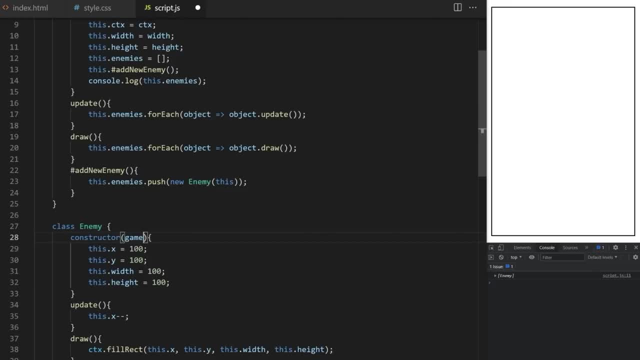 constructor, I will call it game here. I created this dot game property and I set it to game. that was passed as an argument. now I have access to game object from inside my enemy class. I can console log it and you can see all its properties, including width and height. so 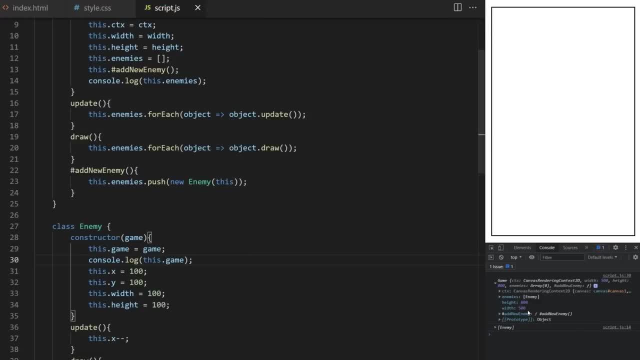 now I have access to width of my game from inside enemy class by saying this: dot game dot width. the initial starting X horizontal coordinate for enemies will be just behind the right edge of canvas. initial starting Y coordinate will be a random number between 0 and this dot game height. 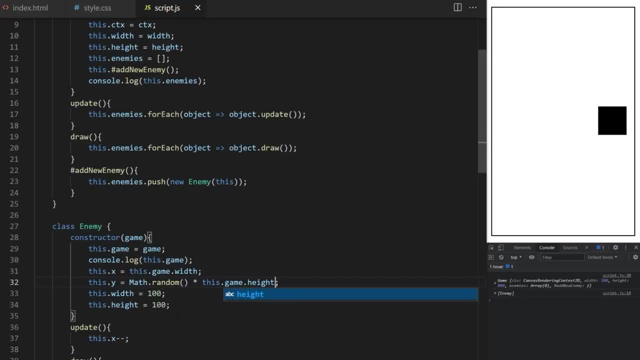 so in this case between 0 and 800 pixels, because height of my game is 800. now, whenever I reload page, new enemy is generated with random vertical coordinate. I achieved that by passing reference to my game class to enemy class constructor on line 23, which will take: 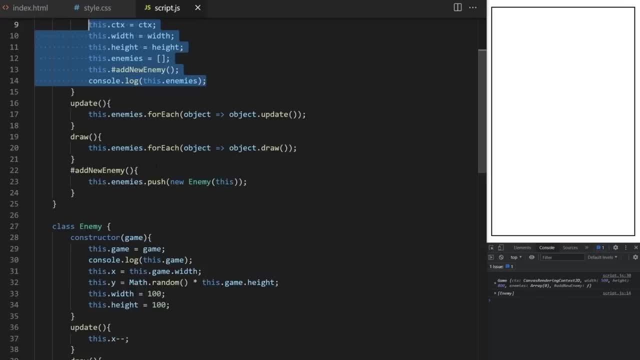 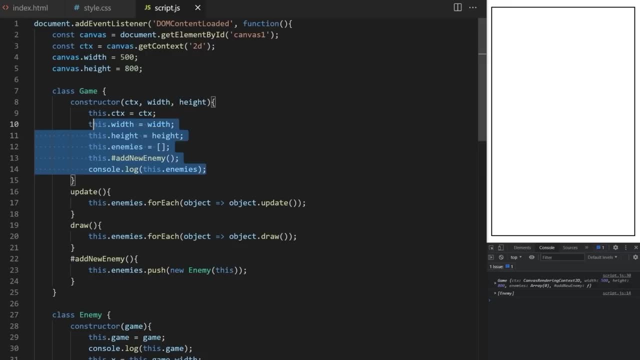 all these properties and values with it. I call it game and convert it into class property on my enemy class, making them available when I need to position a newly created enemies. this is one way how you can pass class variables around if you want to avoid using global. 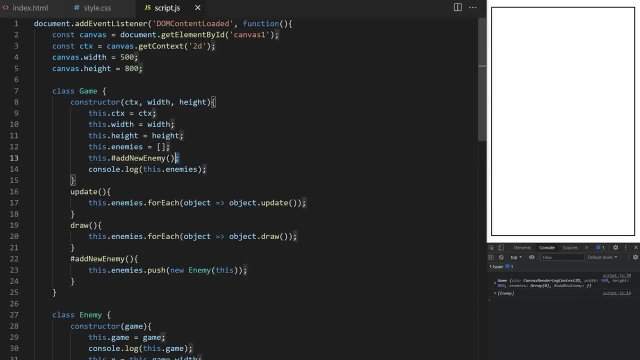 variables in your projects. I don't really want to add just one enemy when I create instance of game class. I want to create new enemies over and over in a certain interval. if I just call this dot add new enemy from inside update method, it will create new enemy for every. 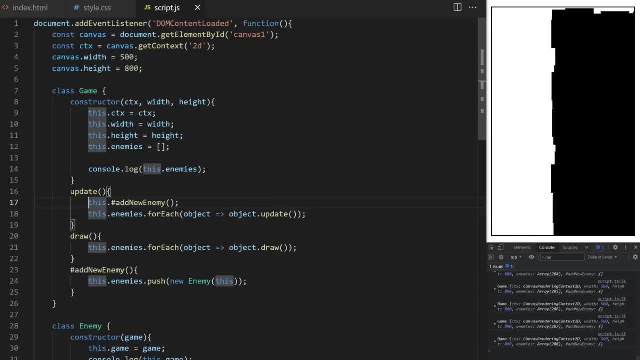 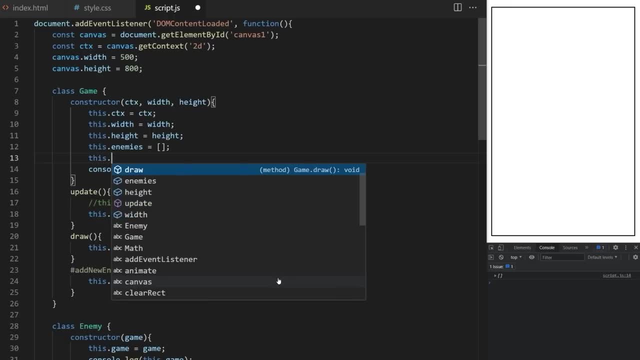 animation frame. that is too many and it would freeze my game very quickly. I commented out: game class is responsible for adding new enemies to the game, so I will give it two new properties. this dot enemy interval will define number of milliseconds between adding each new enemy into the game. let's try 400. 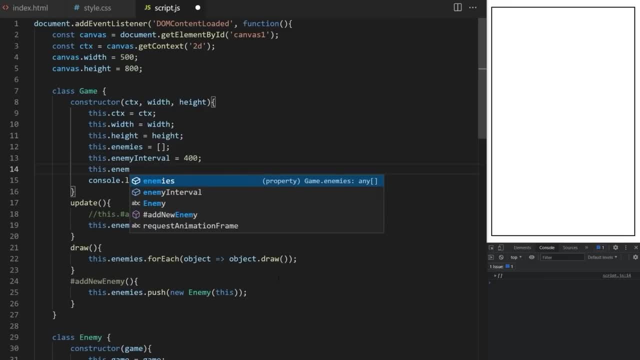 milliseconds. this dot enemy timer will count milliseconds from 0 to 400 over and over. in update method I can say: if this dot enemy timer is more than enemy interval call, add new enemy private class method. also at that point we want to reset enemy timer back to 0 so it can start. 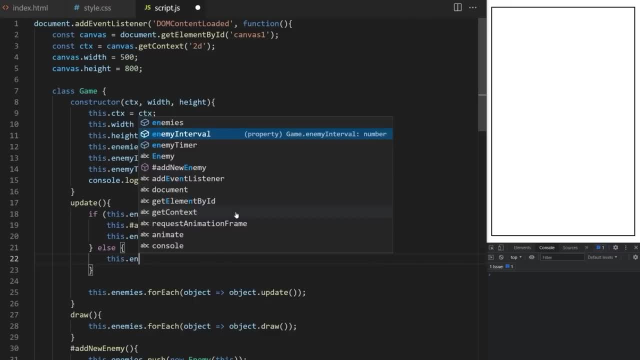 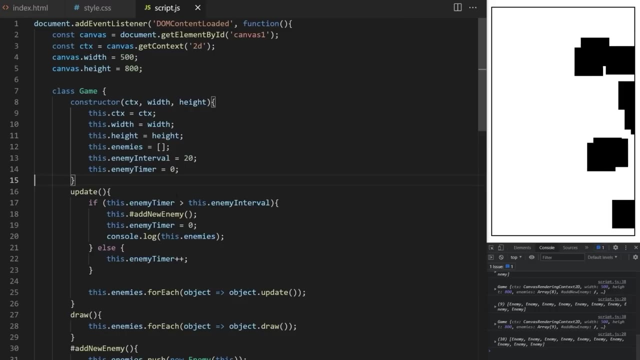 counting again. else meaning if enemy timer is less than 400 milliseconds, increase enemy timer by one every time we add a new enemy. I will console lock this dot enemies array from line 12, just so we can check if it's adding objects or not. I decrease enemy interval on line. 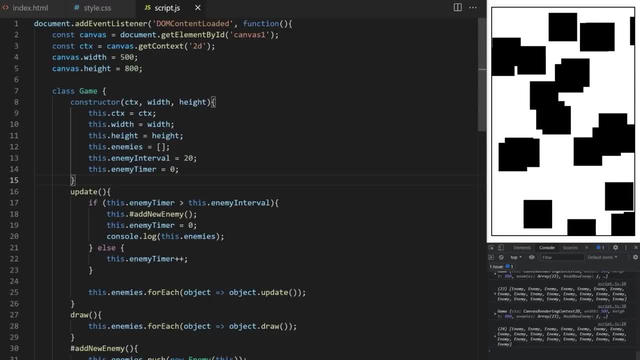 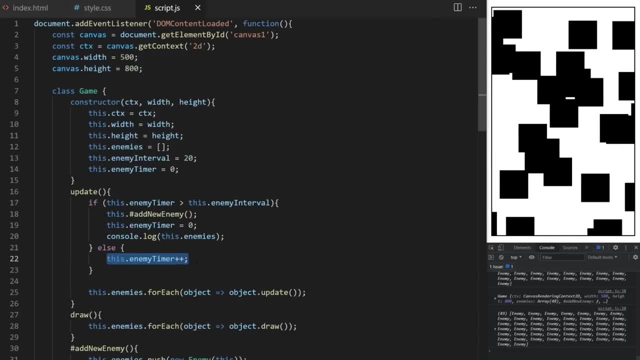 13: awesome, we are adding enemies. but you know how we said that each computer could run at a different speed. that could mean that enemies are being added faster or slower on some computers. I want my game to run at the same speed on every computer and that's why down here. 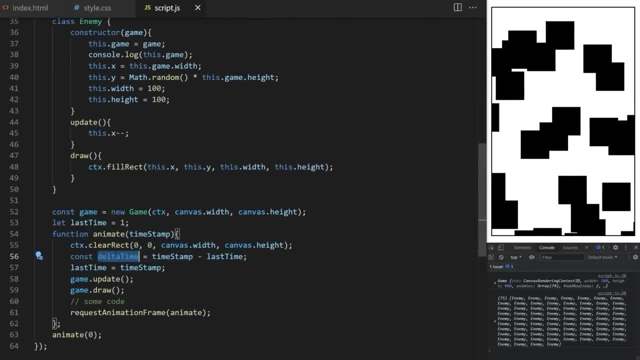 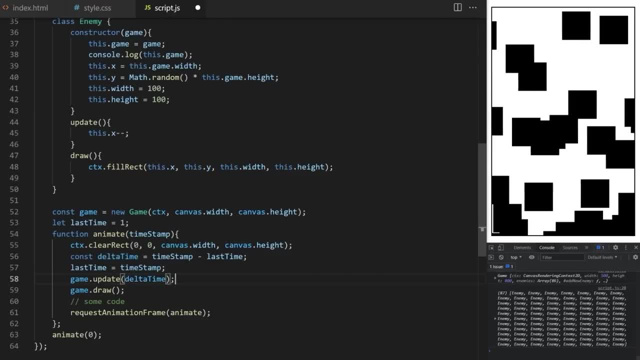 on line 56 in animation loop we calculated the Delta time time between frames in milliseconds. I will use it now. I pass Delta time to game dot update method on line 58. from my previous console log I know my Delta time is 60 milliseconds. my computer can serve new. 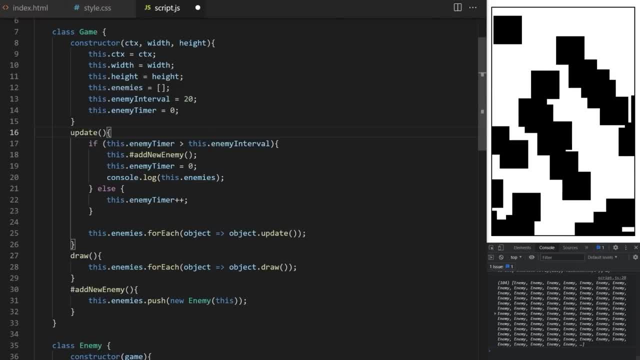 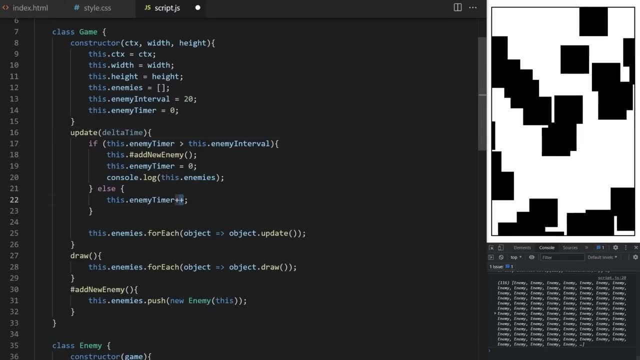 frame every 16 milliseconds. value of Delta time is dependent by the power of your computer, but also on your screen refresh rate, because request animation frame method adjusts to maximum screen refresh rate if the computer can handle it. now I have access to Delta time value here in my update method. so instead of 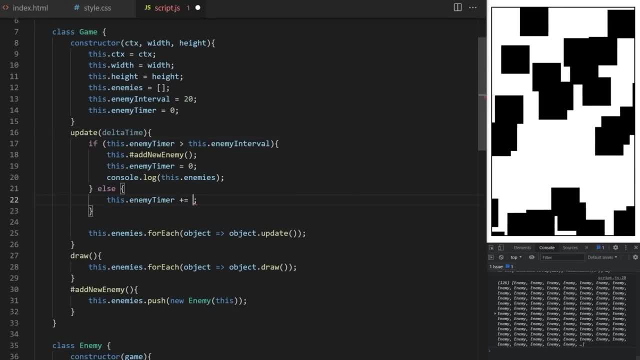 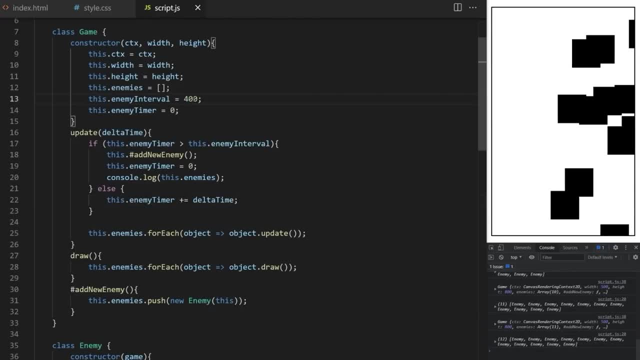 adding hard-coded value plus 1, I will add value of Delta time to my enemy timer. on line 13 I set enemy interval to 400 milliseconds or maybe 1000 milliseconds. here I am increasing enemy timer by 16 milliseconds per frame when we accumulate enough to reach 1000. 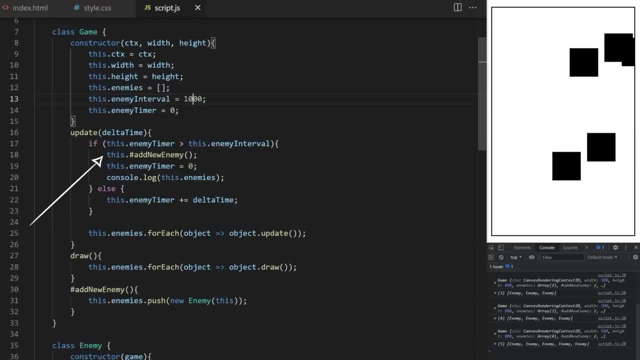 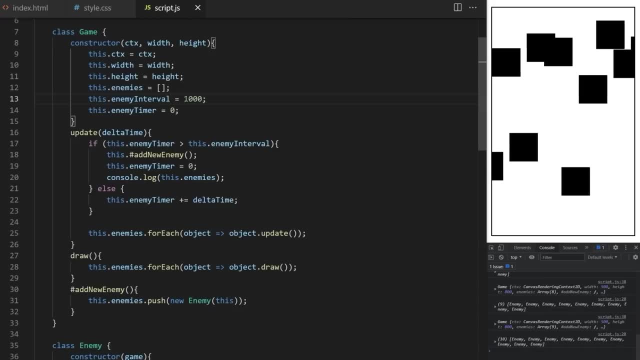 milliseconds, one second, we will add new enemy to the game. if somebody has a faster computer, their Delta time will have smaller value. on slow computers, Delta time will have higher value and will be getting near to the target 1000 less often but in larger steps. so in the 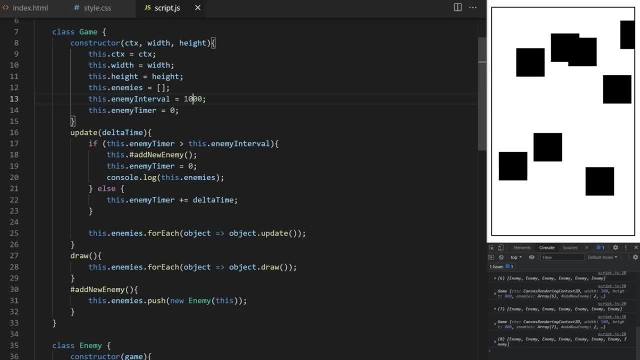 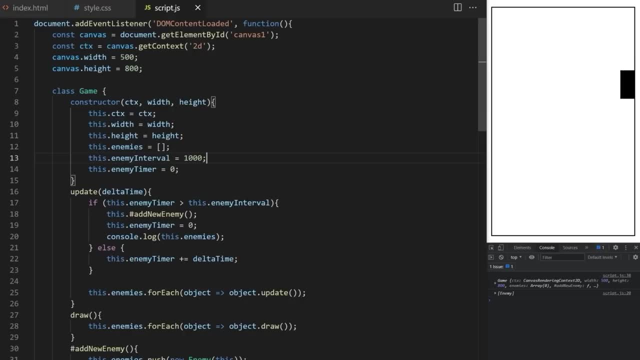 end. my code will run at the same or very similar speed on slow and fast computers, regardless of their power or monitor refresh rate, and this is how you use the Delta time to trigger periodic events in your games or animation projects. I also need to make sure I'm 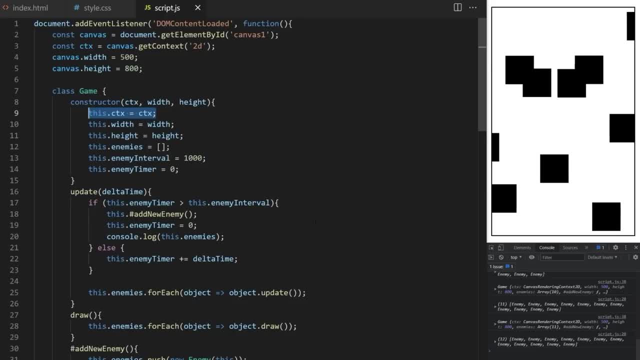 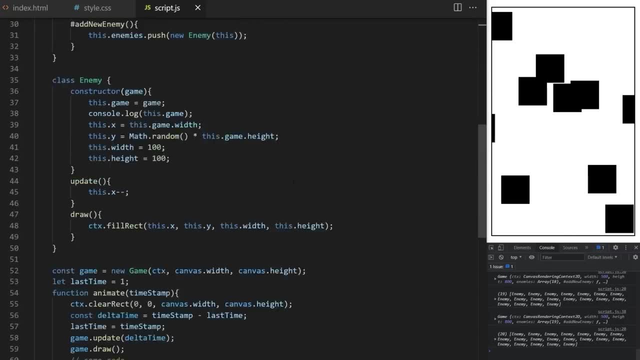 passing the reference to my canvas properly and not using global variable. let's follow the logic. we declare CTX here. on line 3, I passed the global variable to my game class when I instantiate it on line 52. on line 9, I take that argument and I will use the. 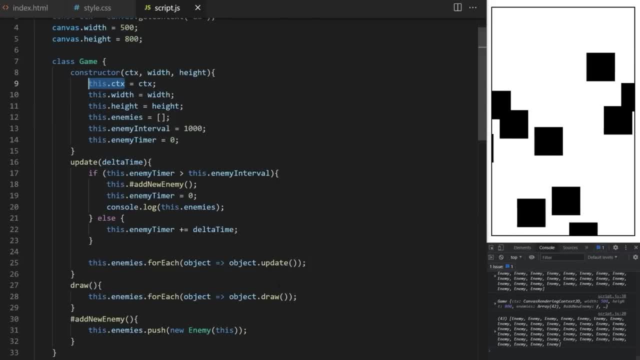 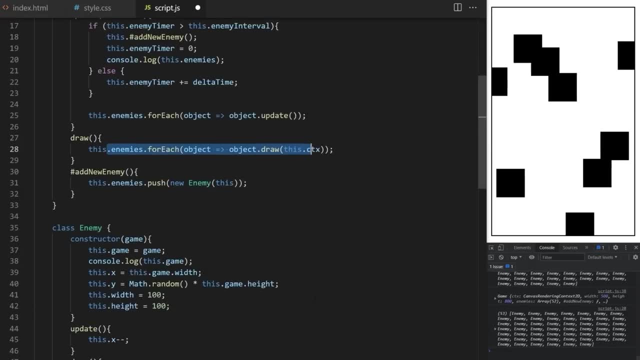 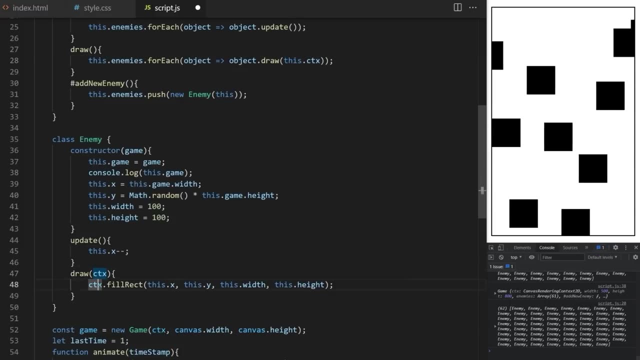 argument I converted to class property. then I pass CTX from line 9 to draw method on my enemies and on line 47 I need to make sure draw method on enemy class expects that argument and this way line 48 is using this dot CTX. that was. 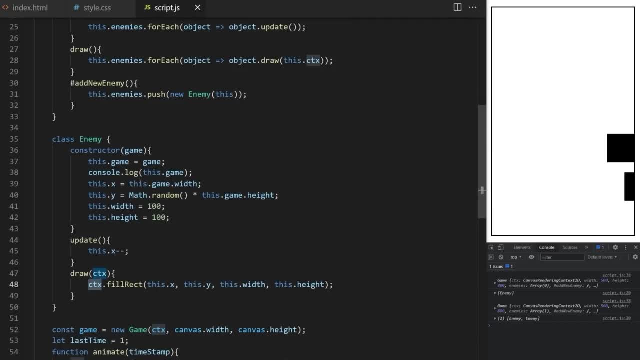 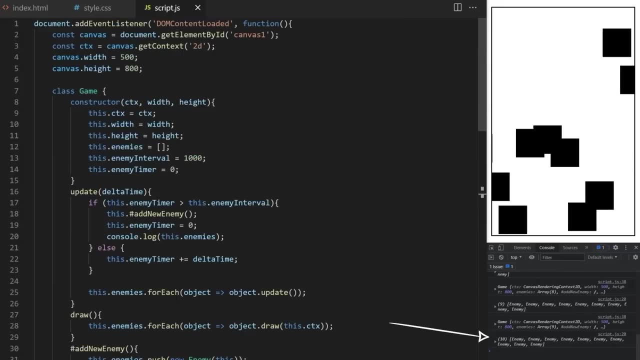 passed around from game object rather than using global CTX variable. I'm console again this dot enemies array on line 20 and I can see it keeps growing. I need a way to remove enemies that have left at the screen. we could potentially also use something called object. 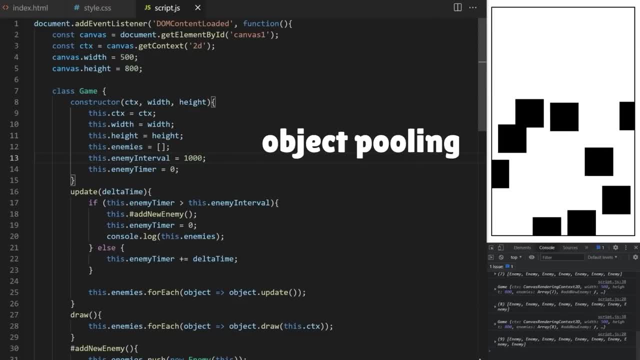 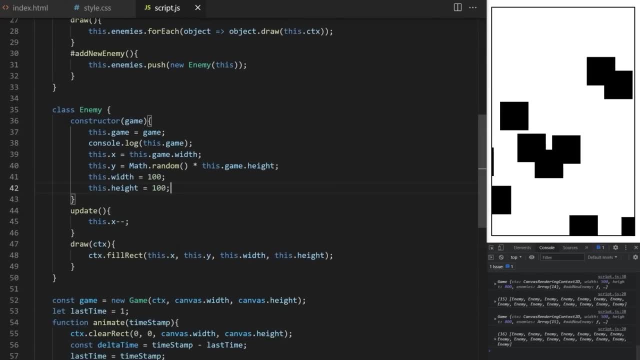 pooling here, but I will leave that for another episode. first I will need a flag on my enemy objects that will mark them as ready to be deleted, and then we will simply filter these objects out. I will call that property this dot marked for deletion, and I initially set it to. 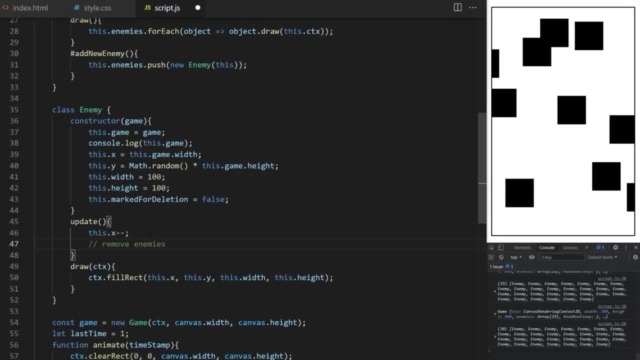 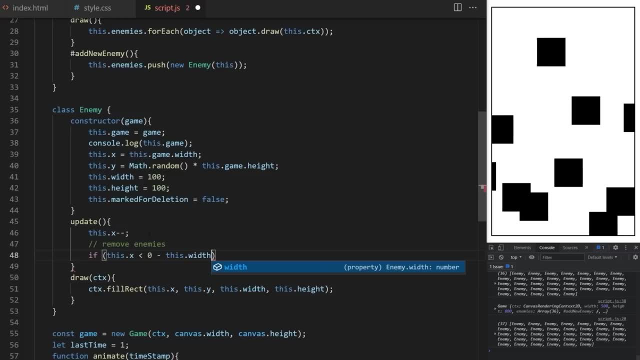 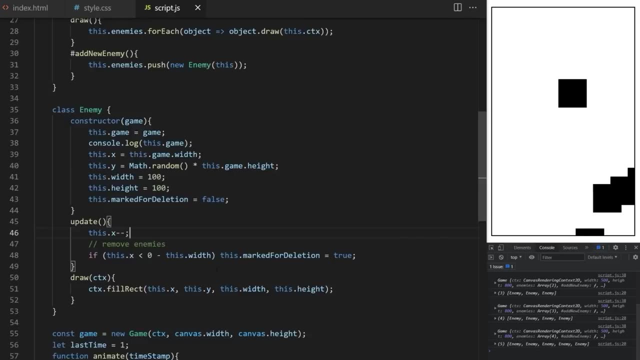 false, then inside update method. on enemy class, I will check if this dot X is less than zero minus this dot width, meaning the enemy has moved across the screen and behind the left edge of canvas. if it has, I will set its marked for deletion property to true. now I can go inside update method. 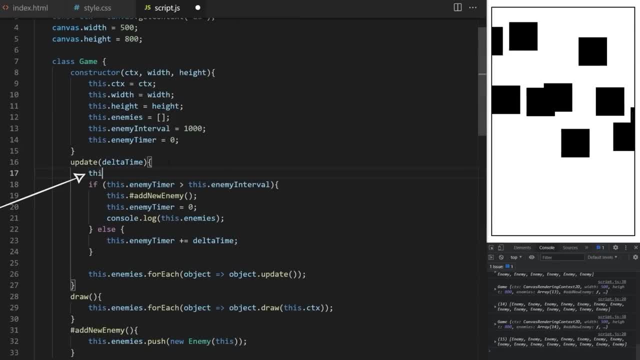 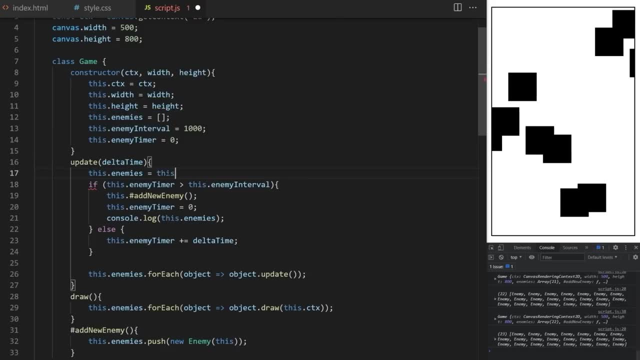 on game class, and here I will take this dot enemies array from line 12, which currently has around 20 objects and it keeps growing, and I will filter it. filter is a built-in JavaScript method that manipulates arrays. it simply creates a new array with all elements. 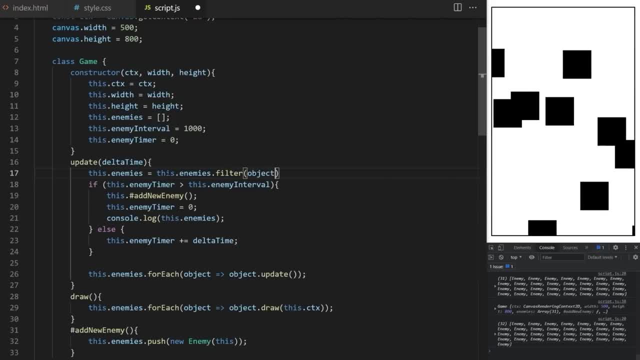 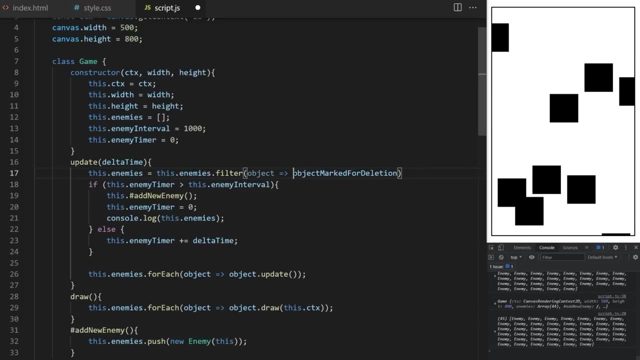 that pass the test implementation implemented by the provided function. so here on line 17, I'm saying: take this enemies from line 17 and reassign it to the same array, but only include elements that have this dot marked for deletion property set to false exclamation mark. 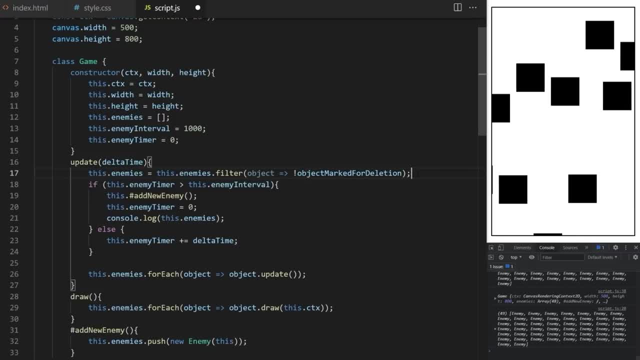 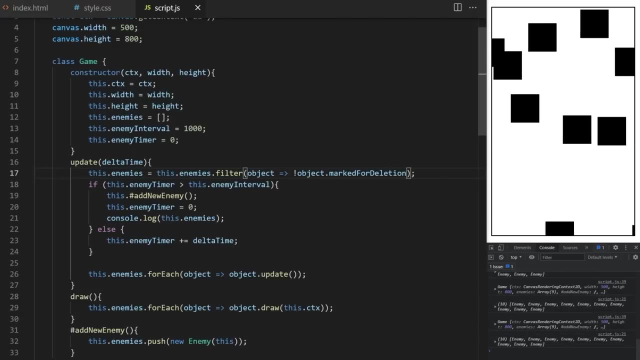 here means false. let's run the code and see if it works. yeah, we stop at 10 enemies and it's not growing anymore because we are removing old ones as we are adding new ones. might be one good performance idea here. you don't have to check and filter. 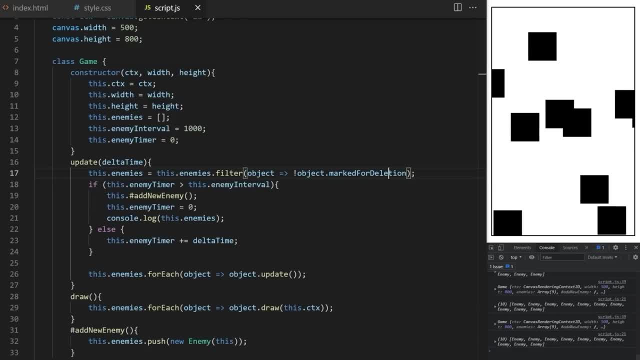 enemies for every frame of animation. we could, for example, do it in a certain interval. I could even take this line of code and put it inside this if statement. it would still filter old enemies, but it would run only periodically, whenever I add a new enemy to the game. 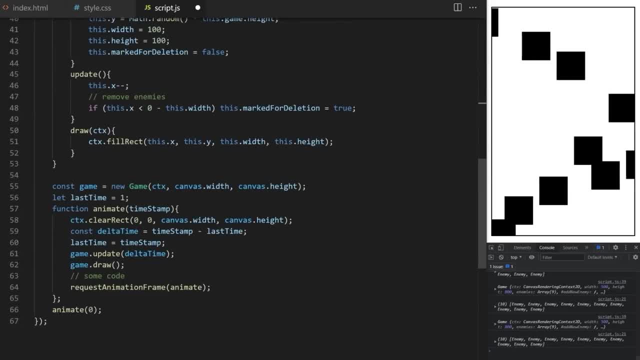 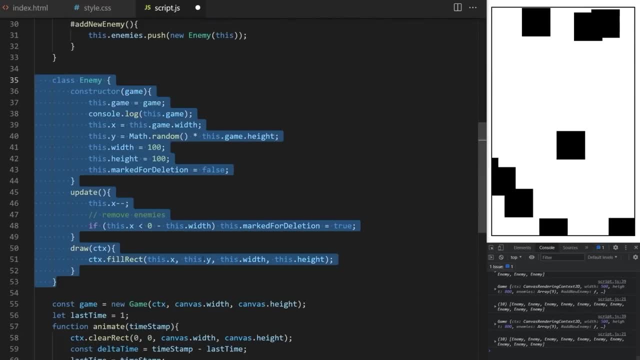 we are making nice progress. we have already implemented so many features here. between lines 35 and 53, I have my enemy class. it's a blueprint with properties and methods that determine what my enemies look like, how they move and how they behave. let's expand on it. 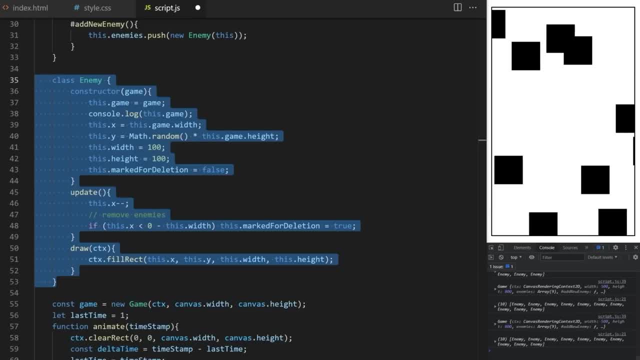 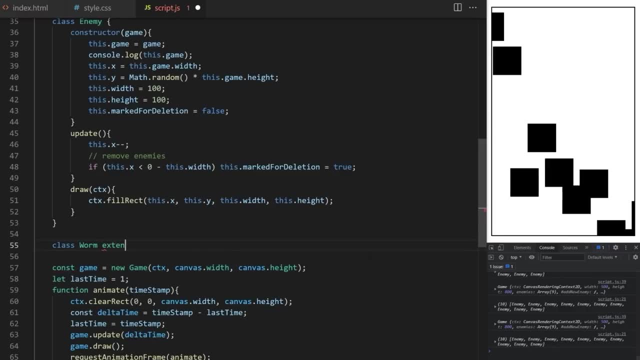 and make them more interesting. rather than simple black rectangles, I will create a so-called sub class or child class by saying class worm extends enemy. doing that will make enemies more interesting and more interesting. for example, if I call update or draw and JavaScript can't find that method on my 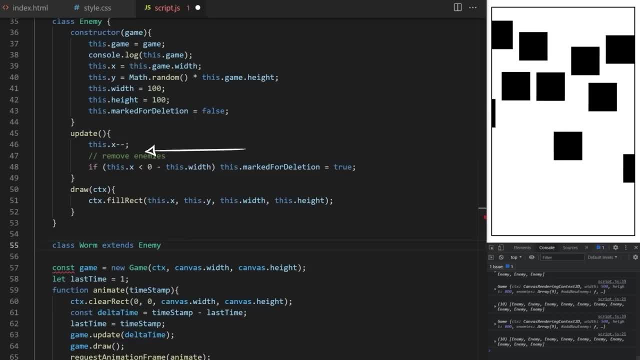 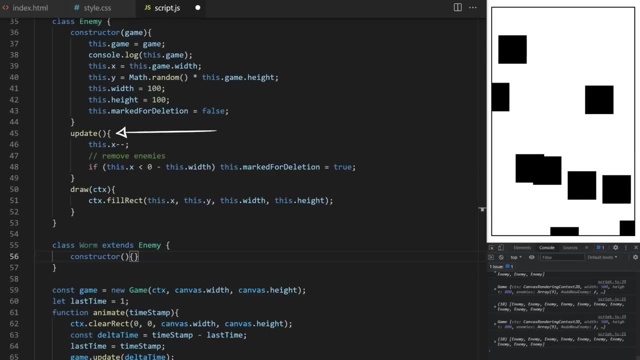 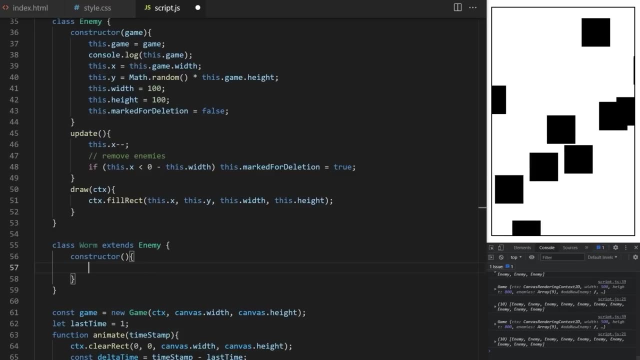 worm class, it will automatically go looking for it on the parent class. so it will look for that method. on enemy class, same goes for properties declared in constructor. if there is no constructor on my worm class, it will automatically use the constructor from enemy. when I do this I can have shared enemy class. that. 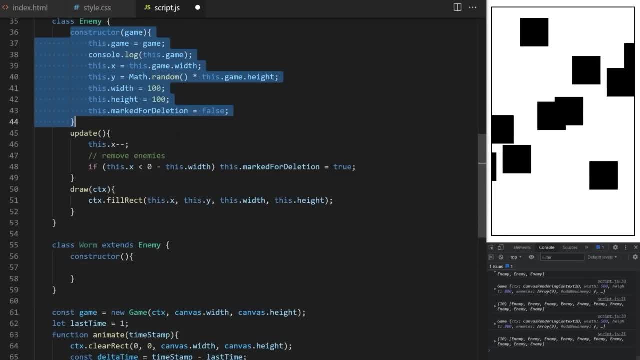 declares all logic properties, methods and features that all my enemies have in common, for example, their sprite, animation, logic collision checks with player, and so on- while at the same time, I can declare child classes where I can override, improve and change some of these properties and methods to create. 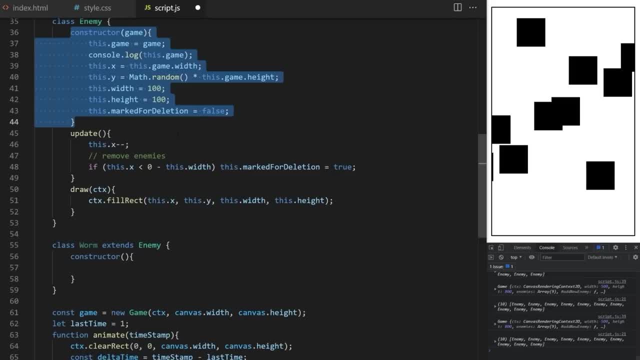 unique and very different behaviors for different enemy types, and that's exactly what we will do. now. let me show you how much visual and behavior variety we can create without repeating the code all enemies have in common. doing this will keep our code clean and modular, and you. 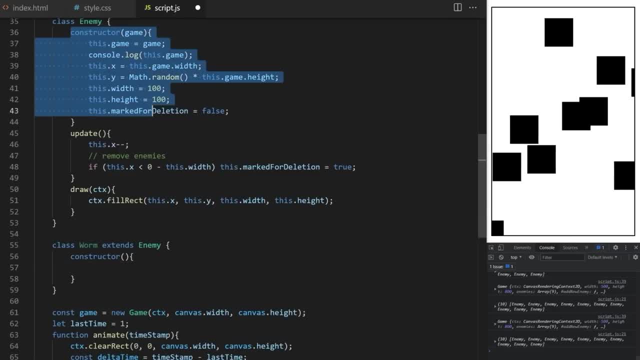 can go crazy with different enemy types while still keeping your logic organized and easy to read. on my worm class, I don't have to declare constructor at all and JavaScript will automatically use constructor from line 36 on enemy class. but in most cases you want each enemy to have different width. 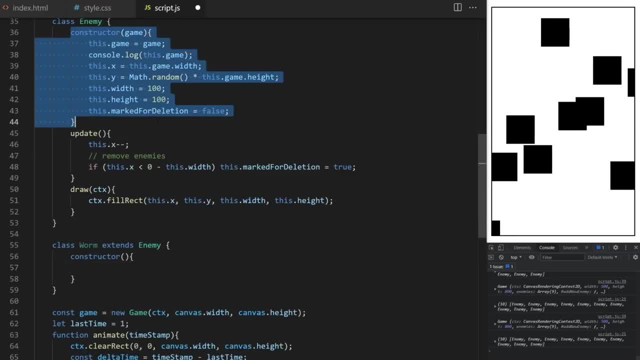 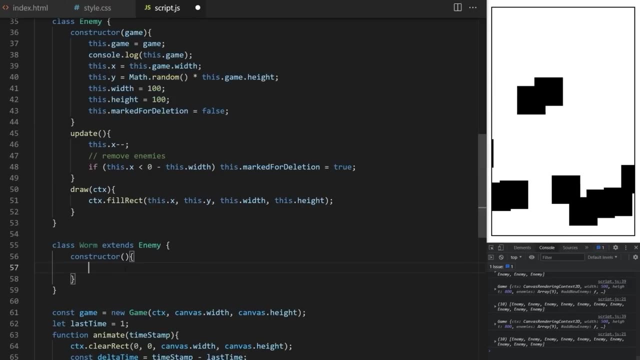 height, X&Y position and so on. so I kind of want to use both. I want to take all properties from enemy constructor and I want to add some additional properties on top of it. that will be specific only for my worm objects. I declare constructor and I know worms will have. 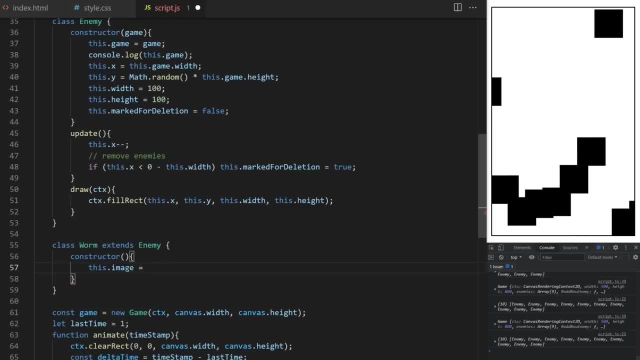 unique value for image property. so this dot image equals worm. this line of code is a weird syntax and I will explain what's going on and how come it works when I bring image to my project this way in a minute. let's first finish. constructor method on worm class same as. 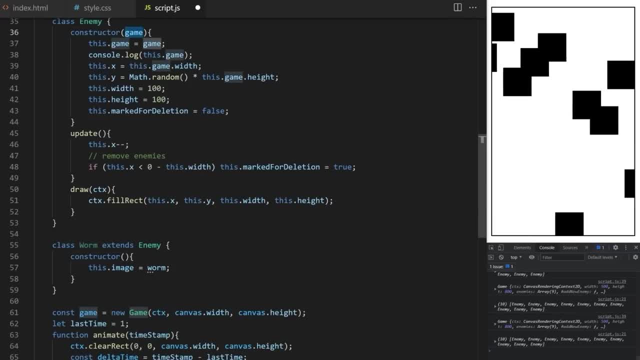 on line 36, worm class constructor will expect the game as an argument. now I want to say: take all the code between lines 37 and 38 and I will declare constructor on enemy class constructor and use it here. to do that we use special super keyword, the super. 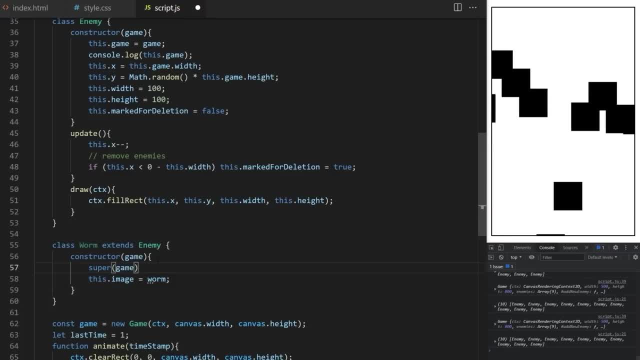 keyword is a special command in JavaScript and it's used to access and call function on an object's parent. so here I call super and I pass it game to literally run the constructor on its parent class. after that I can add more properties on my worm class constructor. 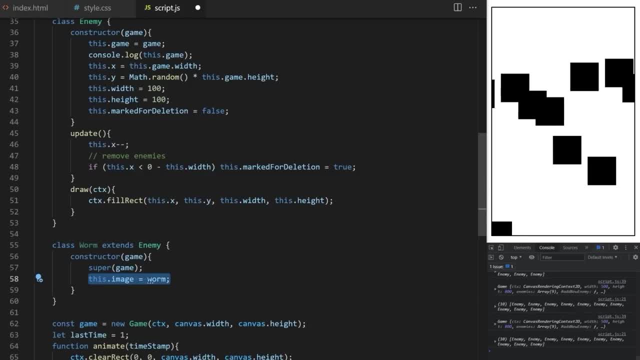 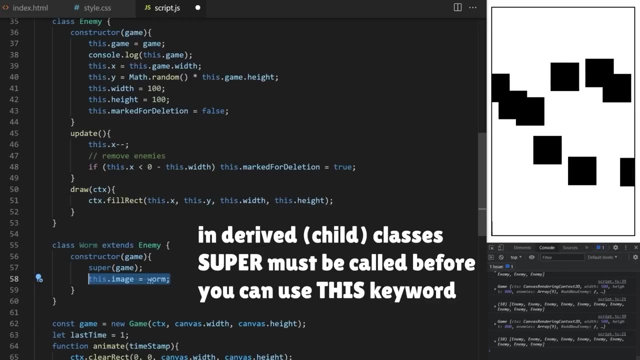 like this. important thing to note here is that you have to first call super and run parent constructor like this before you declare any additional properties using this keyword. otherwise you will get a reference error in derived classes like this. super must be called before you can use this keyword. so now my worm. 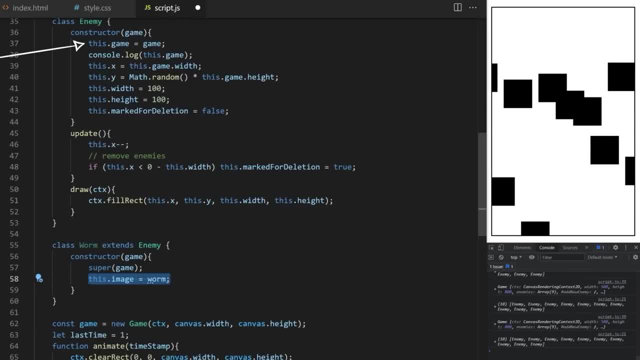 constructor contains all the code from between lines 37 and 43 and additional this dot image property set to worm. each enemy type will have different starting X&Y coordinates and different width and height, so I will actually take all these properties and put them on my worm. I. 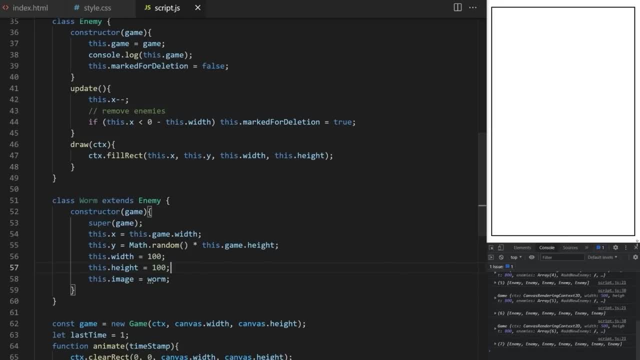 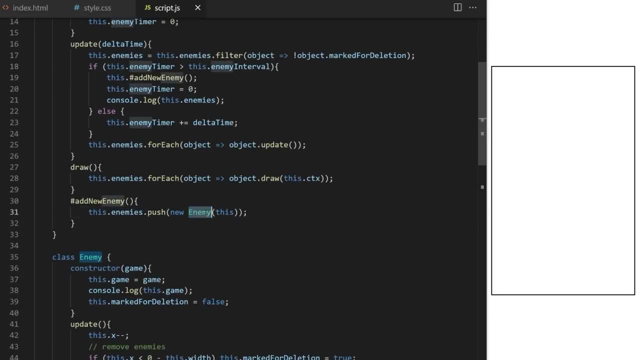 want enemy class constructor to have only properties and values that are shared for all my enemy types. up here on line 31 inside private add new enemy method. rather than instantiate in parent enemy class, I will instantiate child worm class again. I'm passing it, this as an argument and because we are inside. 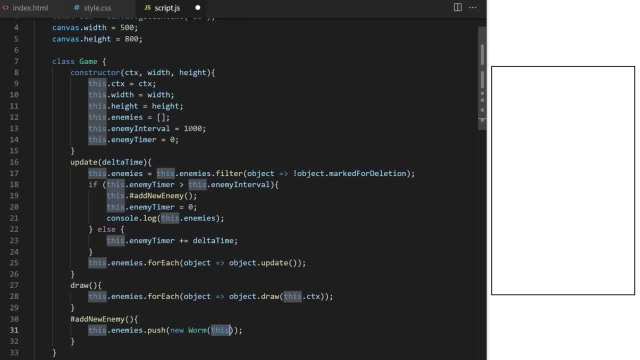 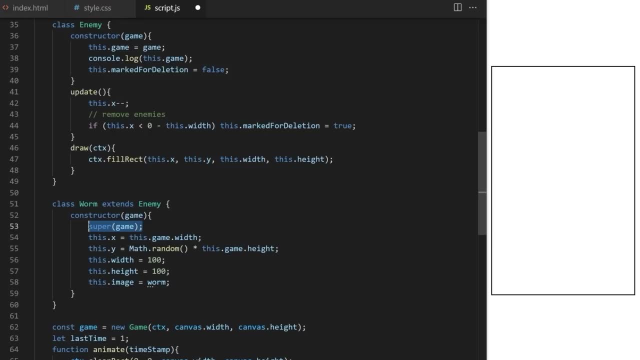 game class. this reference is the entire game object. so all these properties. we travel down to worm class and inside constructor. we are taking that game and passing it to super instantiating constructor of its parent enemy class, which is here. enemy class also has update and draw methods, and when I call update and draw, 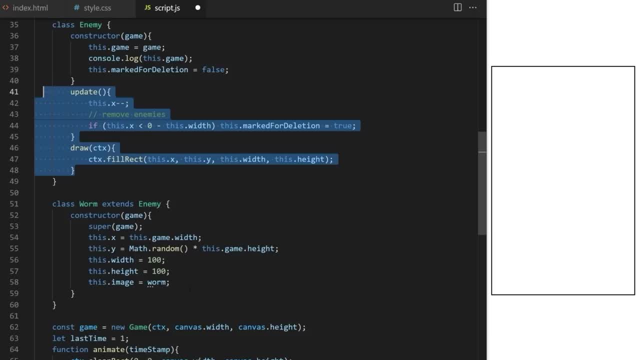 on my worm and JavaScript can't find it, it will automatically go looking for them on the parent enemy class. I hope it's becoming a little bit more clear how this works and how parent and child classes relate and work together. if I run the code, we have our worms come in. 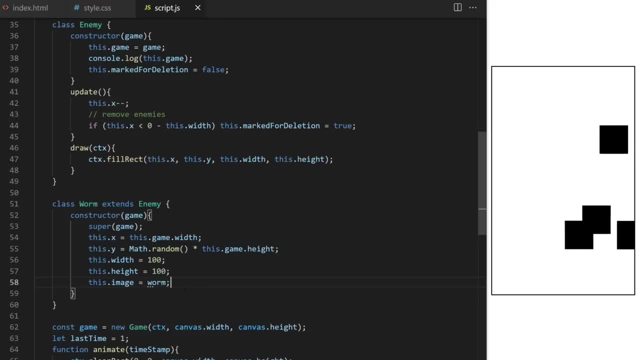 again, just to prove that draw methods- that is called from line 46 is taken: properties from worm class constructor. let's change this dot with online 56. as you can see, now my worms are 200 pixels wide. so what is this weird syntax? online 58? this is not how we usually bring. 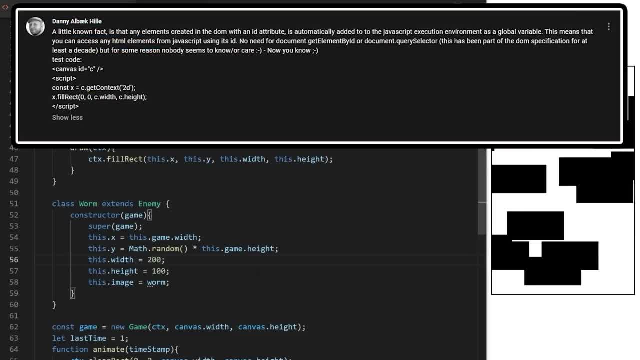 images into a project. usually I would use get element by ID to target my image element with an ID of worm that I created in index HTML. in the beginning I wasn't aware of this, so all the credit goes to Danny, who says a little-known fact is that any elements created in 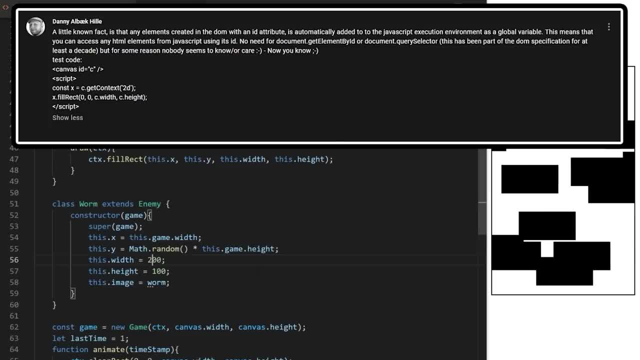 the dome with an ID attribute are automatically added to the JavaScript execution environment as a global variable. this means that you can access any HTML element with a JavaScript using its ID, no need for document dot, get element by ID or query selector. I'm just doing this as an experiment and you 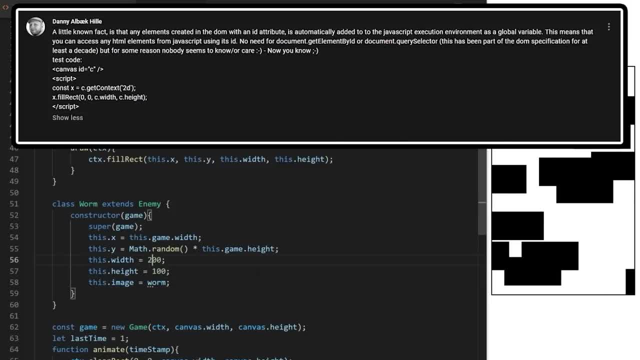 will see in a minute that it actually works. if you're having any issues, you can still bring the image into the project the usual way, and also you can also ideally pass it to the worm class constructor as an argument, so that we are not pulling global variables. 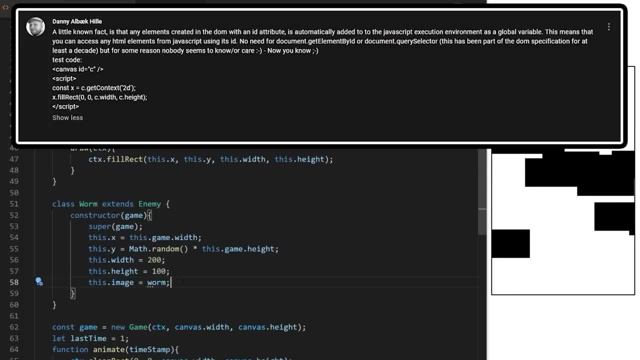 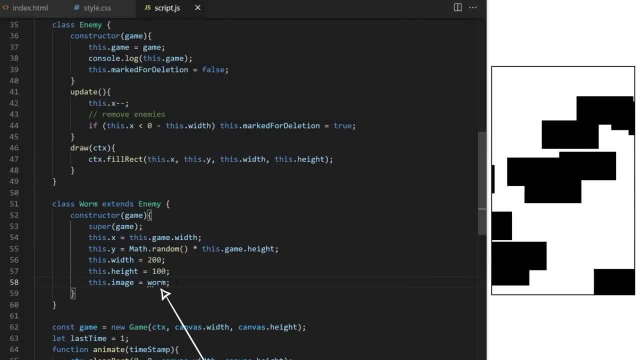 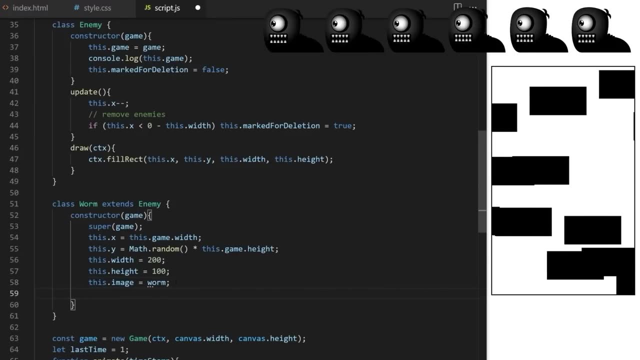 directly from the outside. I'm just experimenting here a bit. I really like tips like this. thanks, Danny. nowhere in my code have I declared this worm variable. the only place you can find this reference is ID online 12 inside index HTML. but this image will still work. you can test it by console login. 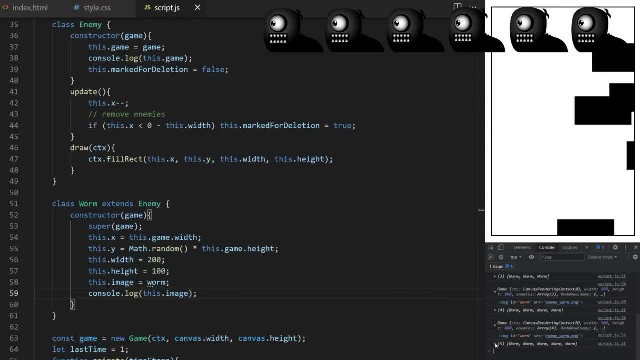 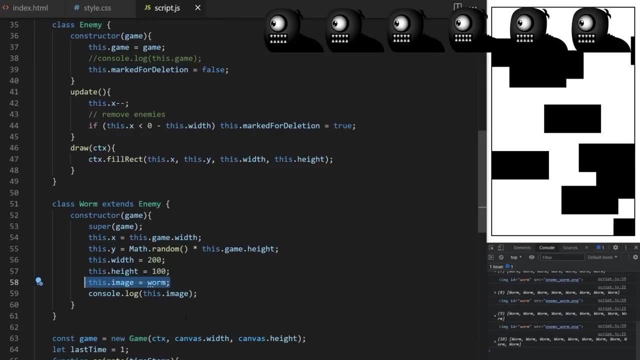 this dot image. I have too many console logs. let's comment outline 38. yes, you can see that the JavaScript is actually finding the image with an ID of worm automatically, without us having to use get element by ID like we usually do. so let's use that image and. 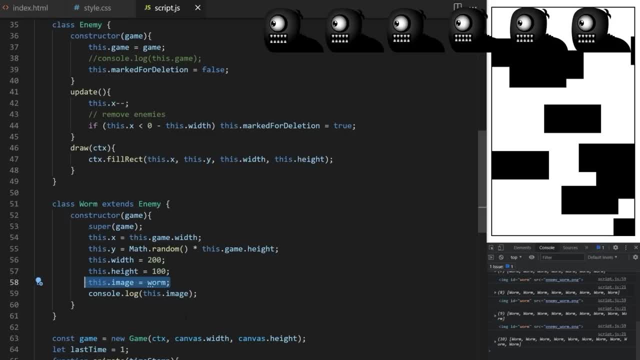 make our worms look a bit better than black rectangles. you can download these sprite sheets for free in the description and you can use them to follow along with this video for educational purposes. to use them in any commercial projects, you would have to buy a full license from the artists. 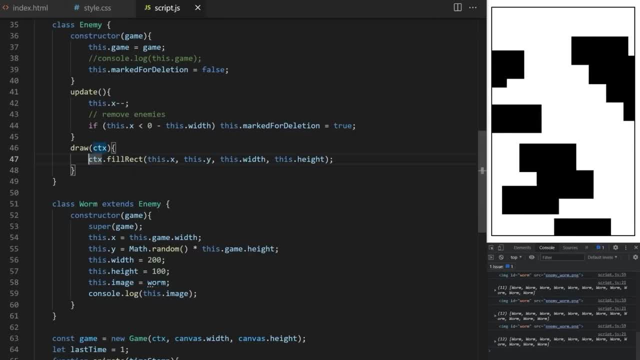 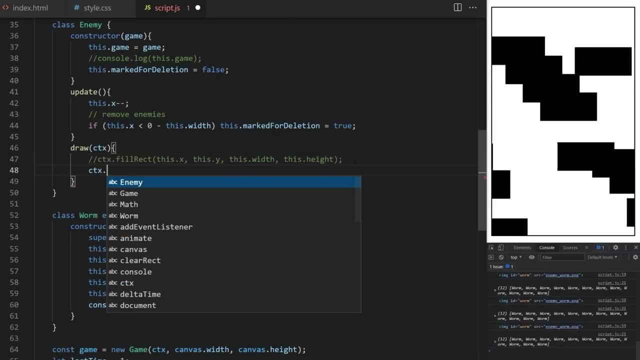 website. I will link his site as well. he has a lot of great game development art assets there. check it out. I feel like I explained built-in canvas draw image method hundred times on this channel. this method is so important. at first I will just use the version with five arguments. 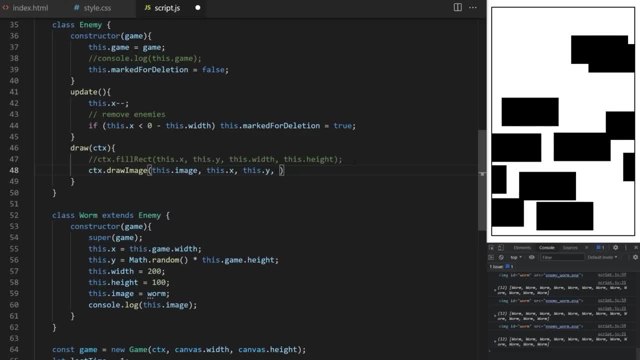 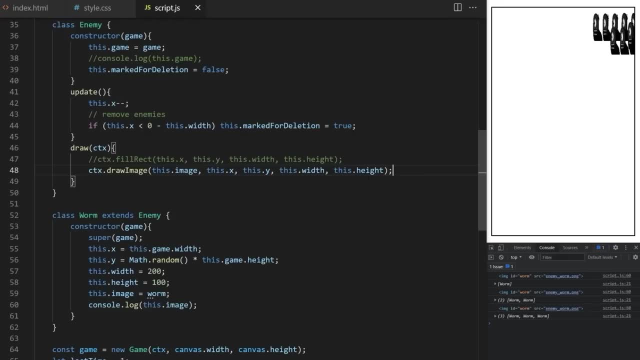 image we want to draw X, Y, width and height. where to draw it on canvas? this way, we will just squeeze the entire sprite sheet with all its six frames in to the predefined area of 200 times 100 pixels. notice that I'm calling draw method on my worm class it's using. 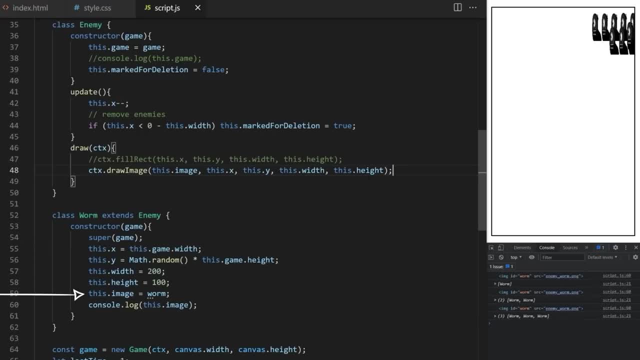 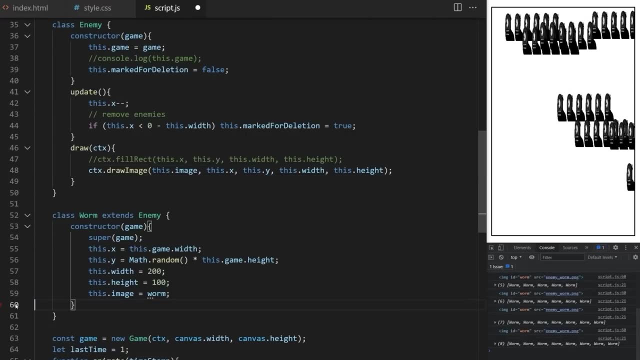 these properties. but since JavaScript can't find draw method on worm, it will look for it on parent enemy class and it will use that one. let's remove this console log and this fill rectangle as well. I can change width and height, but now I would actually like to draw just. 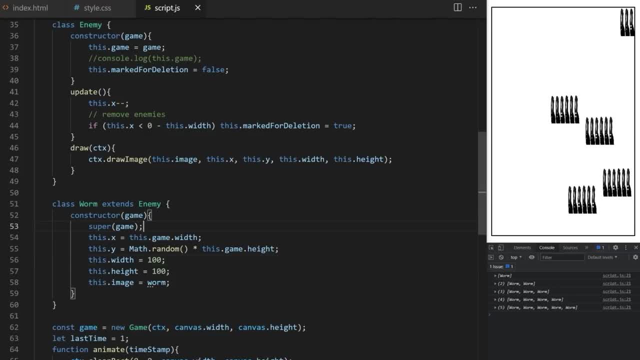 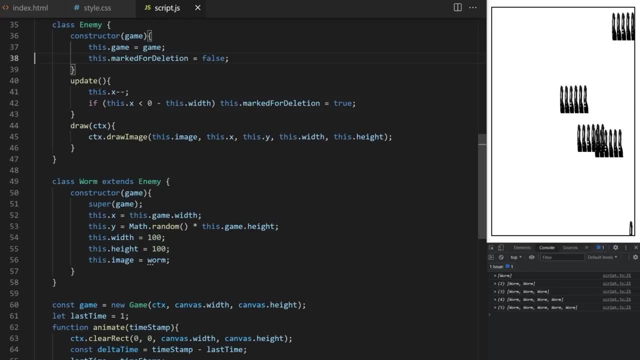 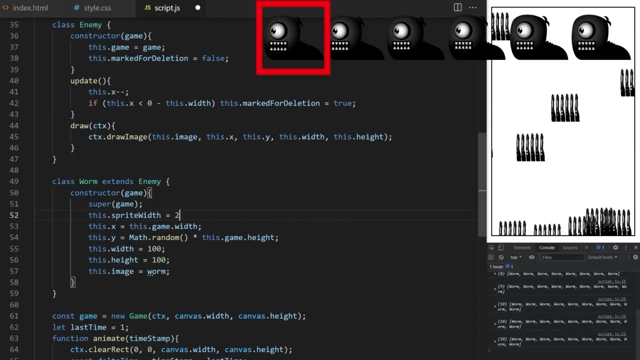 the first frame from the worm sprite sheet, I remove all these lines I commented out earlier. I create a new property on worm class called this dot sprite width and it will be a width of a single frame in my sprite sheet. if I take width of my sprite sheet and divided by 6, the number 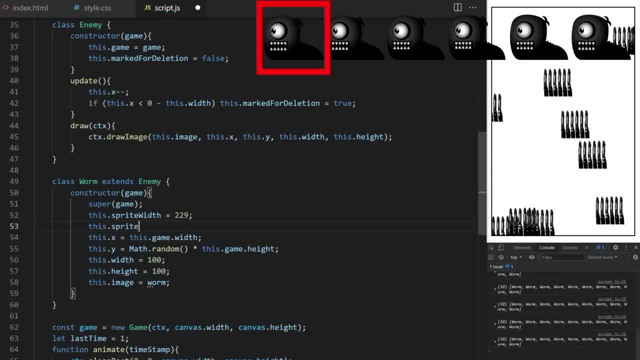 of frames I will get 229 pixels. height of a single frame is 171 pixels. I take width and height and move them up here. now I need to use draw method to cut out just single frame from that sprite sheet and place it on canvas. for that I will. 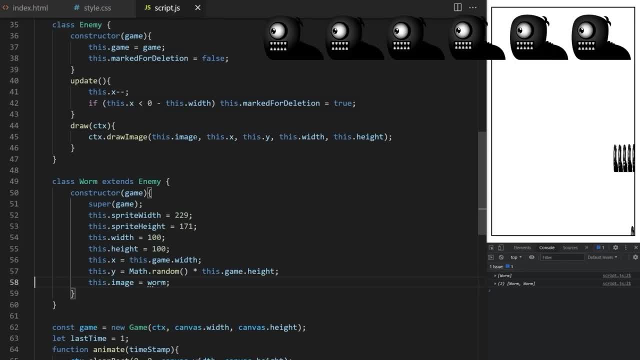 need to give it nine arguments, so additional four to tell JavaScript what area I want to crop out from the source image. I need to give it source X, source Y, source width and source height arguments. source X and source Y will be 0- 0, since I'm just cropping out the 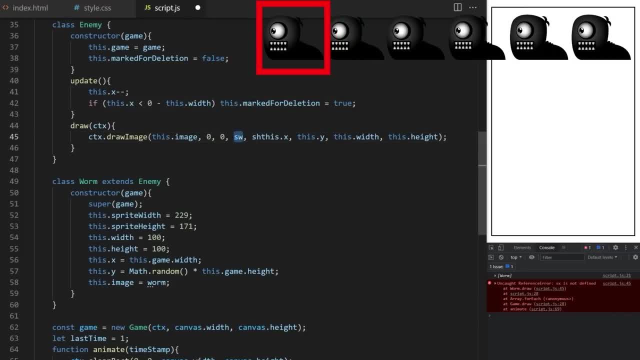 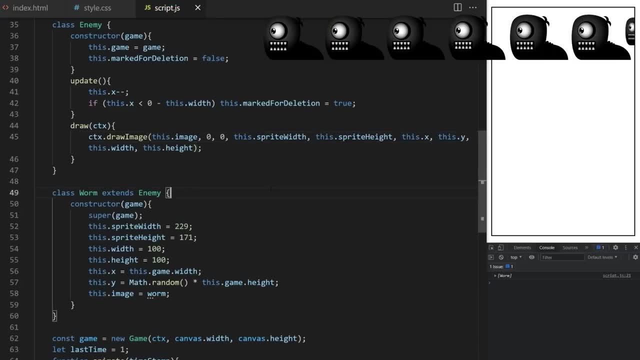 first frame, for now, source width and source height will be this dot sprite width from line 52 and this dot sprite height from line 53. so to create this dot sprite, I need to give it a single frame from an image. with draw image method, I need to give it nine arguments. 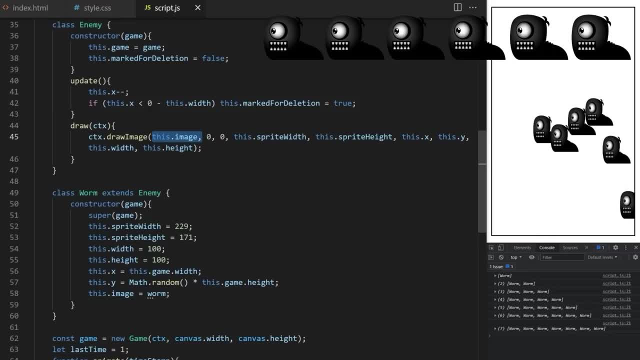 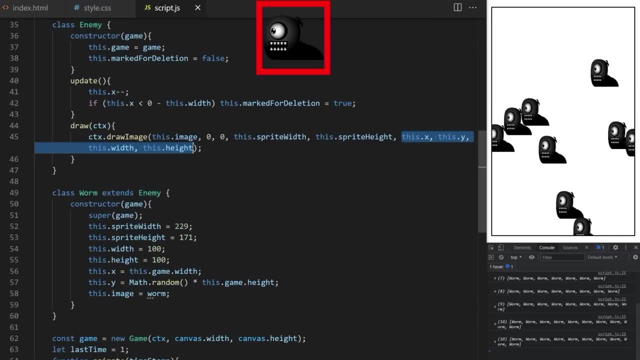 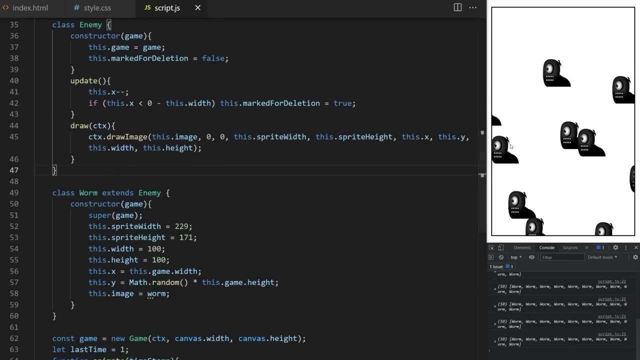 image I want to draw X, Y width and height of what area I want to crop out and X- Y width and height of where on canvas we want to place that cropped out piece of image onto. now we are drawing just one frame, perfect. you probably notice that it's a bit stretched, that's. 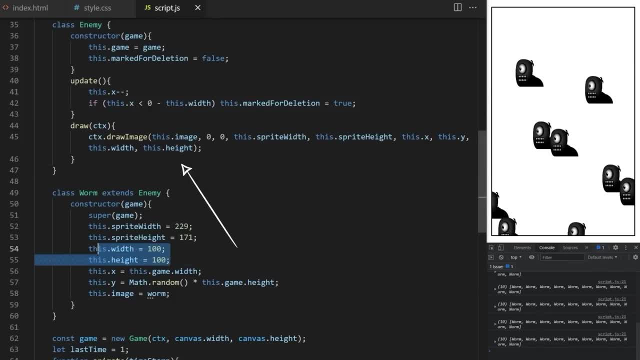 because this width and height, which is coming from here, has no relation to the actual size of a single frame, so the ratio is different. let's make width and height the same aspect ratio as our sprite sheet. I do that by making with half of sprite, width and height will be. 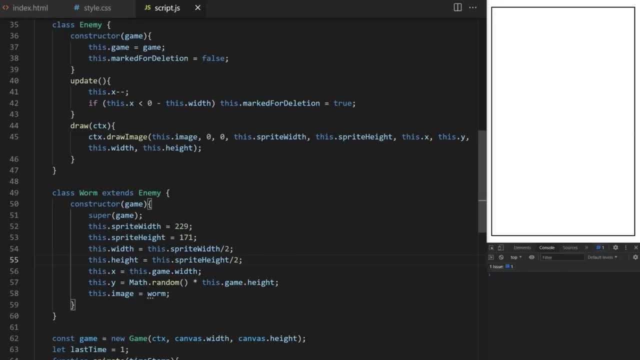 half of sprite height. I needed to do half because the original size would be too large. as long as I use the same modifier on both width and height- in this case I divide both of them by two- it will preserve the aspect ratio of the original sprite frame. all my worms are. 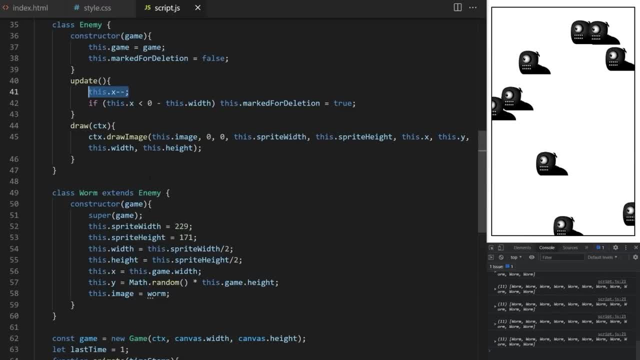 moving to the left by one pixel from the right side of the frame so I can change the aspect ratio by one pixel per frame. what if I want each worm to have different speed, for example, a random value between 0.1 and 0.2? 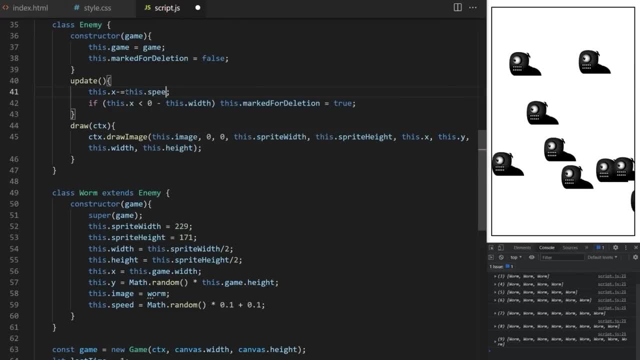 and up here inside update method on enemy class. I say this dot X minus equals this dot speed. that will be very, very slow. let's make it faster. you might have realized that I'm not using Delta time in this movement calculation, so let's use it to make sure the worms move. 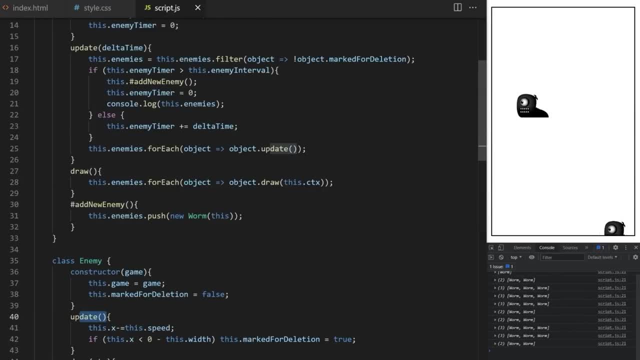 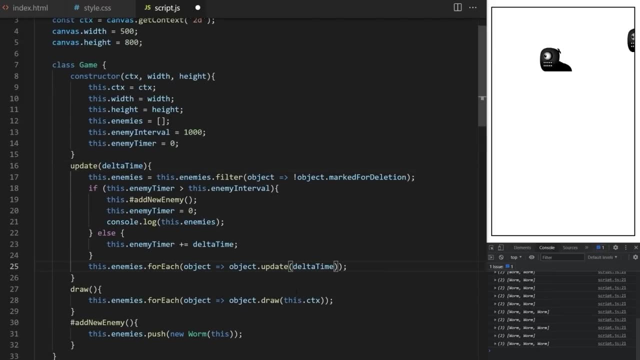 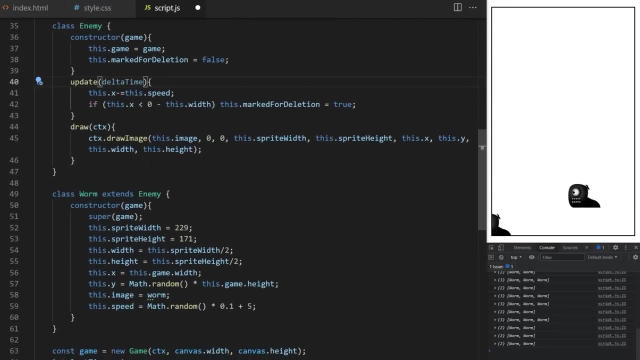 I'm calling this update method here on line 25, so I pass it. Delta time which we made available here before. now that I have access to Delta time in update method on enemy class, I will pass it here as an argument and to factor in time difference between animation frames. 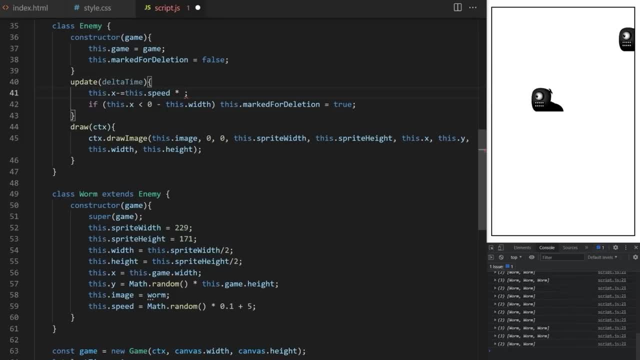 when moving something around we have to multiply it. that way, faster refresh rate with lower Delta time will move often, but by smaller steps. slower PCs will have higher Delta time. they will not draw frames so often but they will have higher Delta time so they will make larger steps to compensate for the 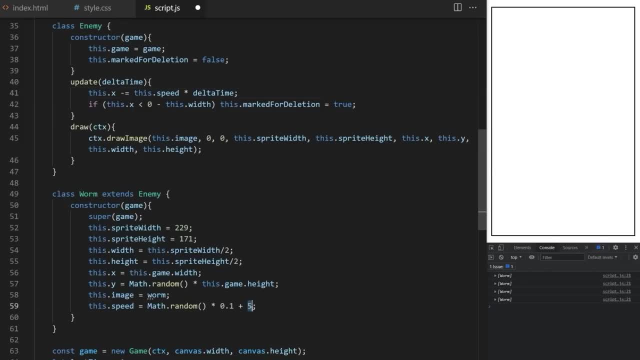 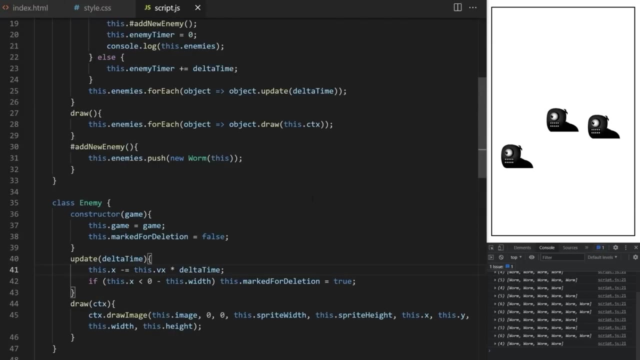 difference. now the base speed is too much, so I amend it. on line 59. I will actually rename it VX velocity on horizontal x-axis, because maybe some other enemies will have a vertical movement also. I need to rename it on line 41 if I go up on line 13 and reduce. 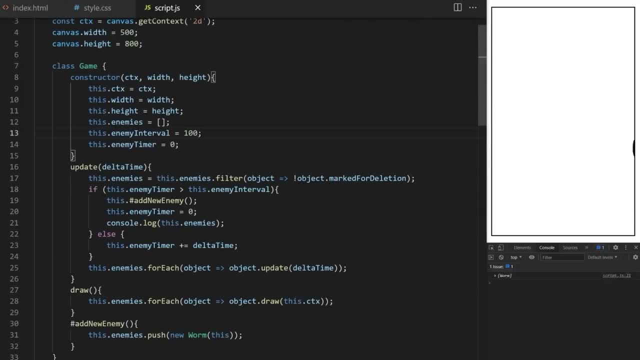 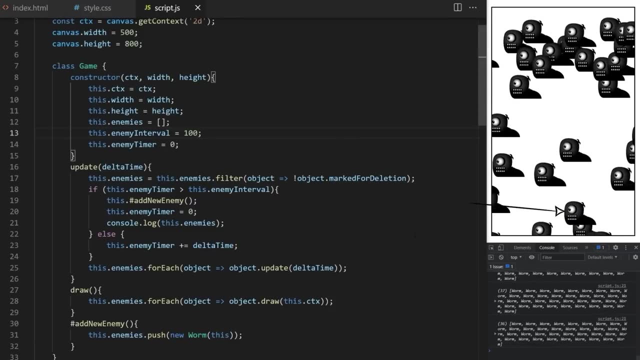 enemy interval to 100 milliseconds. then we will get a lot of worms and something will become apparent. they are layered randomly in order as they are added to the game. for example, this worm should be probably behind this one and this one behind this one, if we pretend. 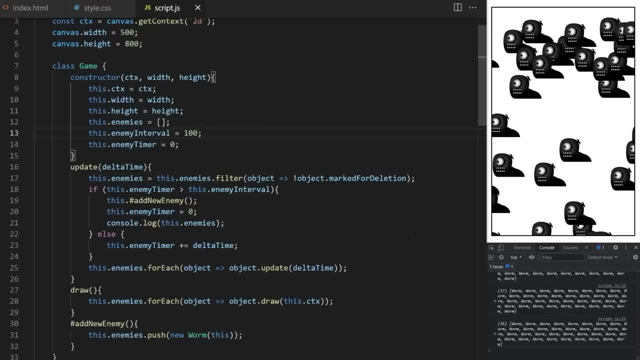 this is 3d game, space, and worms that are higher should be behind worms that are lower. it would look better. how do we achieve that? that index, or whether worm is in front or behind other worms, depends on order at which they are added to the array, on their index in that array. 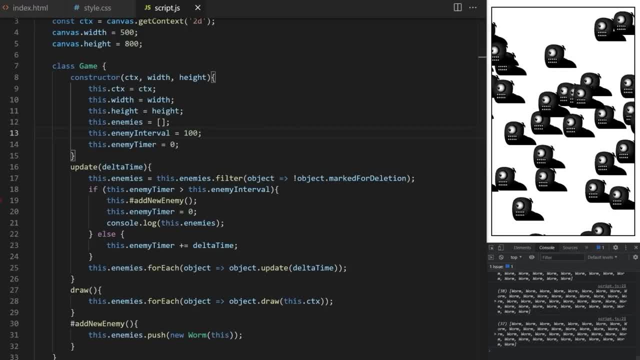 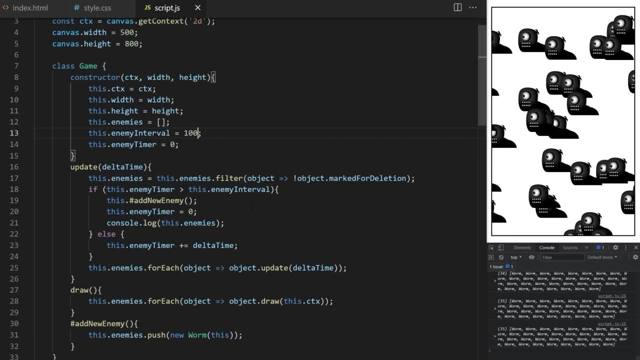 because as I push them into enemies array, one by one, we cycle through them from index 0 to the maximum index in that array and we draw worm with index 0, then worm with index 1 on top of it. if they are in the same area, then worm with. 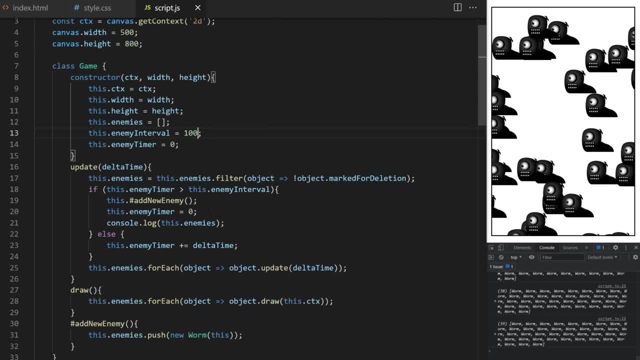 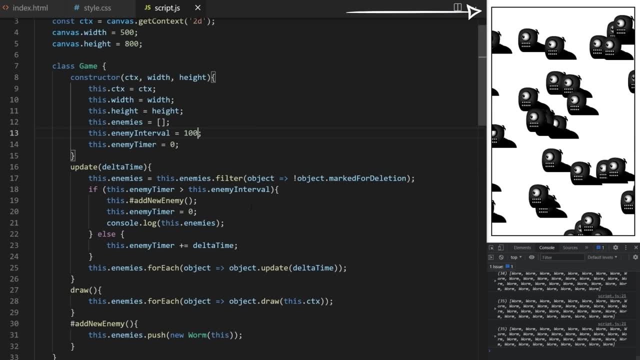 index 2 will be on top of them and so on. I want to reorganize my array so that index in the array is tied to their vertical position, so that we first draw worms in this area and then we draw the ones in this area on top of them and 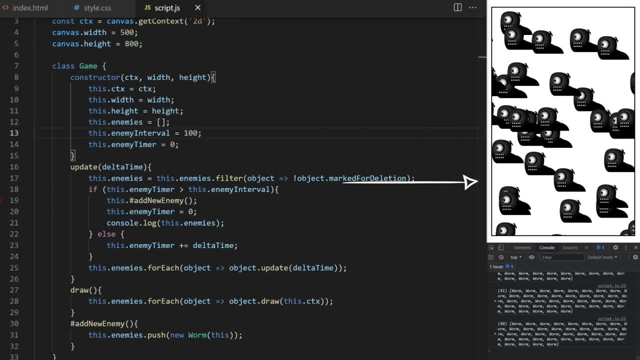 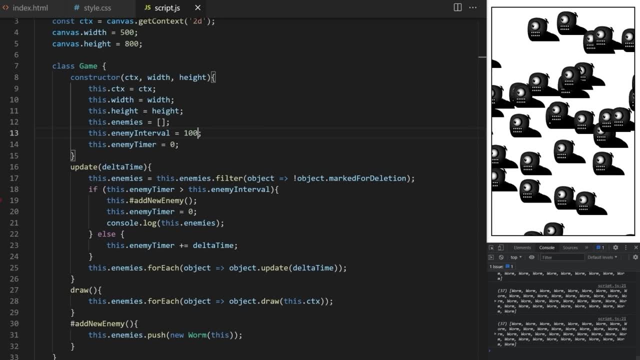 we go down on the page vertically in plus direction on vertical y-axis. that will cause worms to look like they are properly behind each other and not messy like this. look at this, this is a mess. this one is sliding over the other one's eye. so every time I push new worm into. 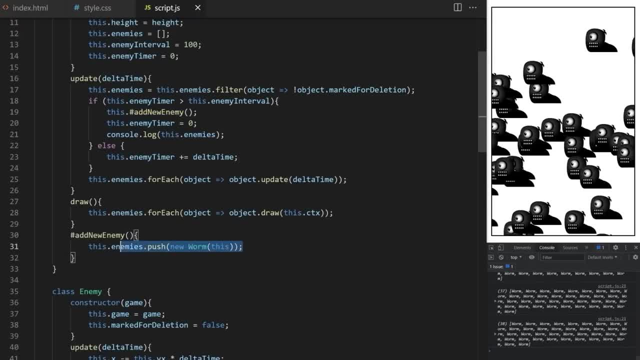 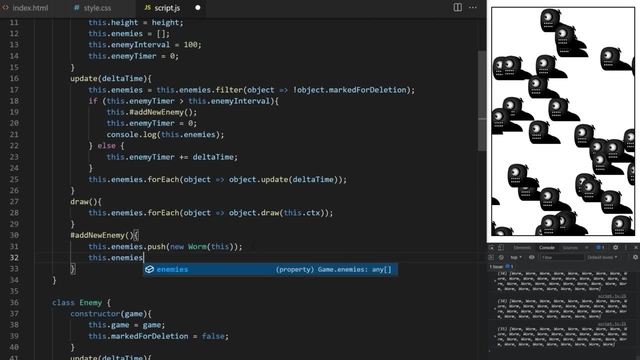 the array. I will just build JavaScript sort method. you can simply just call sort on the array and it will sort them in ascending order by default. if you want more control, you can give it a callback function. sort simply takes every element in the array and it performs a check comparing values. 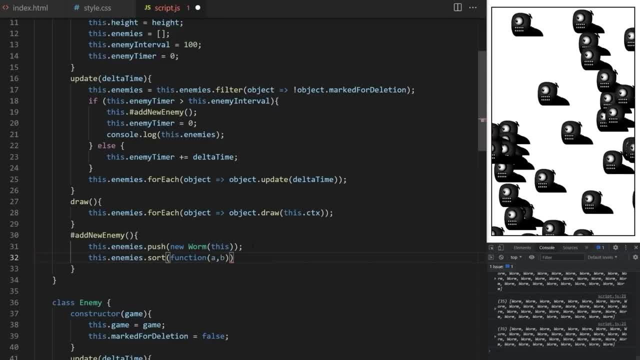 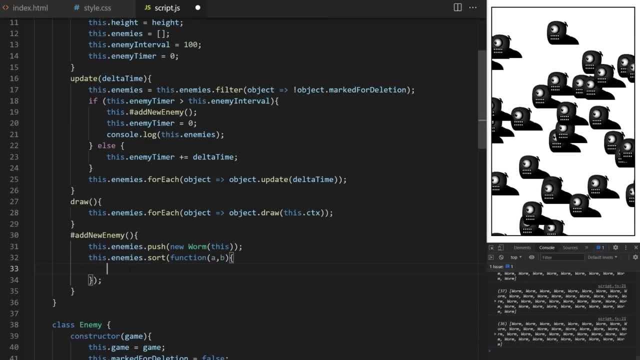 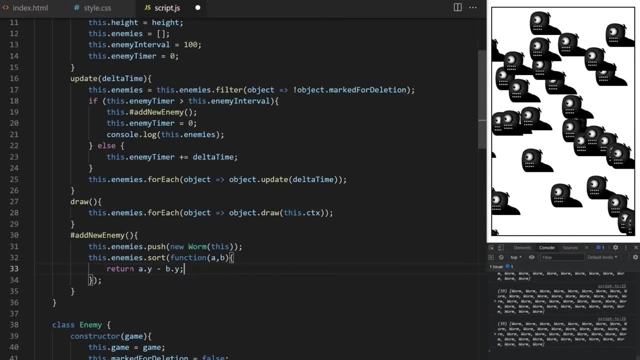 between these two elements, pushing them up and down in the array depending on the condition in the callback. I want worms with lower vertical y-coordinate to have lower index so that they are drawn first. so my condition will be a dot Y minus B dot Y. like this sort is a built. 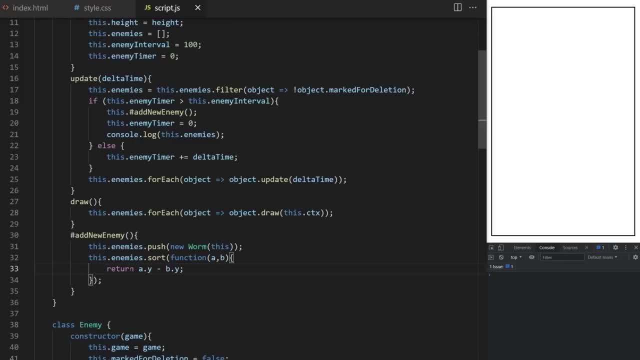 in JavaScript method. it abstracts away the actual algorithm that does the sorting work, so let's not spend more time on it now. all we need to do is to know for now is how to use it. when I run the code, you can see that worms that. 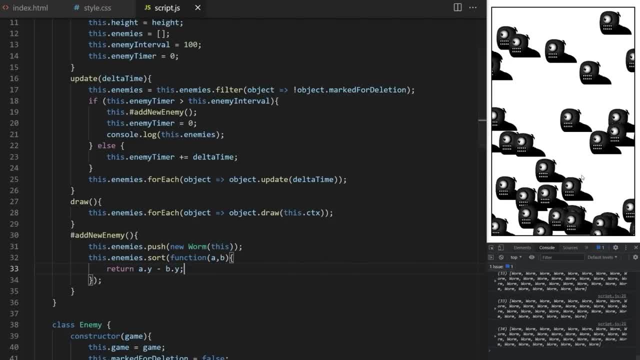 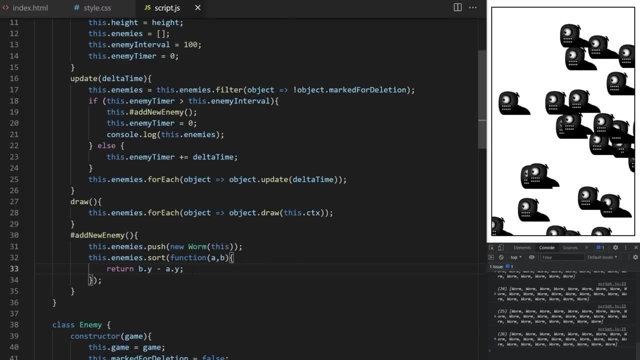 are higher are drawn behind the worms that are lower, making it look like they are moving in actual 3d or maybe in two-and-a-half the cartoon space. well, it doesn't look messy anymore. you can swap between ascending and descending order by swapping these values. in our case, we 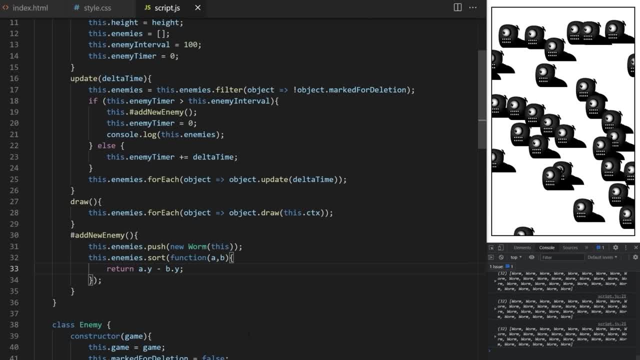 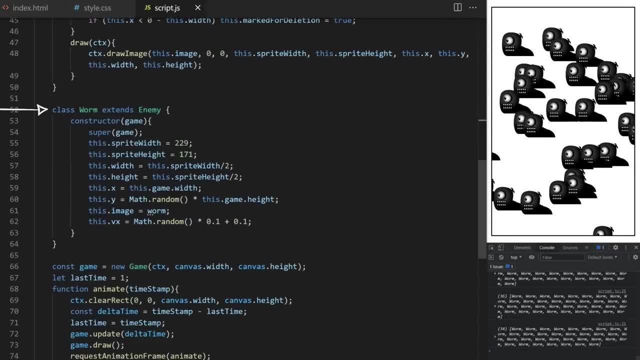 want a minus B. also notice: I'm not sorting the array for every animation frame, only when I add new enemy into the array. so this is our work in the class. it's a child of enemy and it doesn't have update and draw methods because, as we said, if JavaScript doesn't, 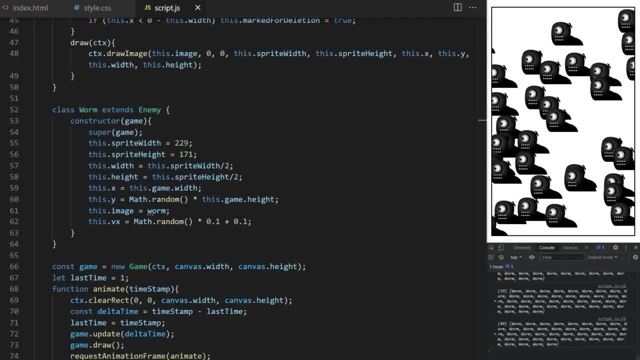 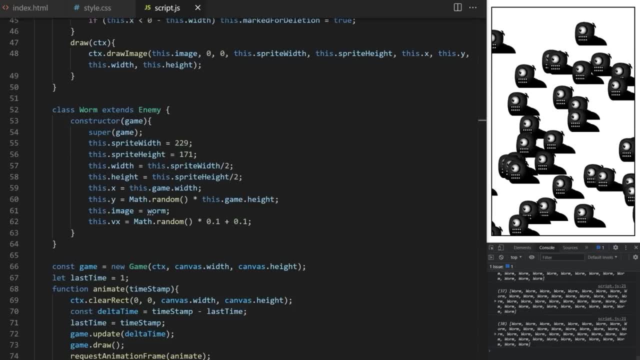 find them on the worm class, it will go looking for these methods on the parent class. but what if I want to use the base code from draw method on enemy class and I want to add some extra code to it to create some additional visuals? for example, as Boris suggested, ghosts need. 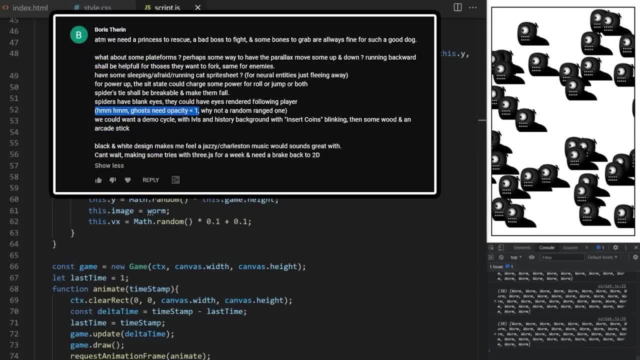 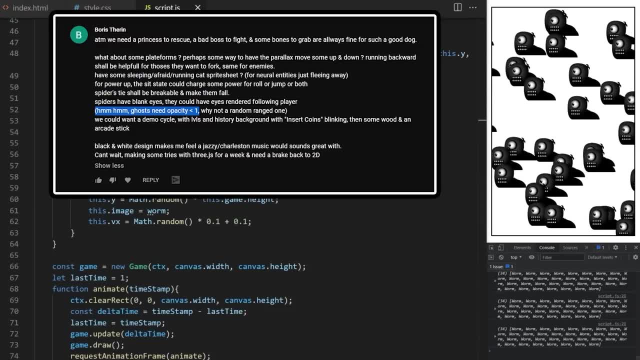 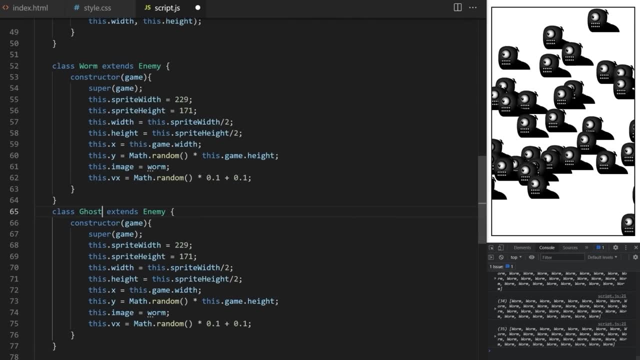 to be semi-transparent, but I don't want reduced opacity on worms, only on ghosts. so how do we do something like that? I'm sure you can come up with some clever if statement, but let's keep it clean and use child classes for that. I will copy my worm class and rename it. 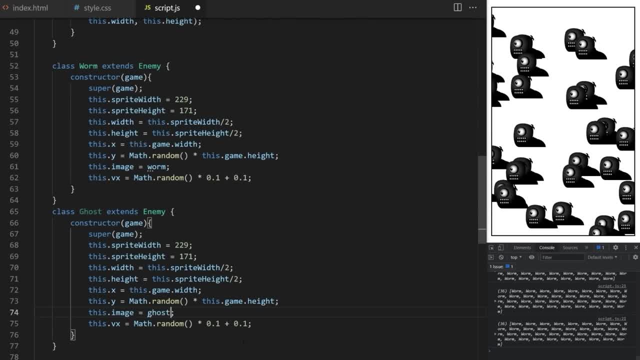 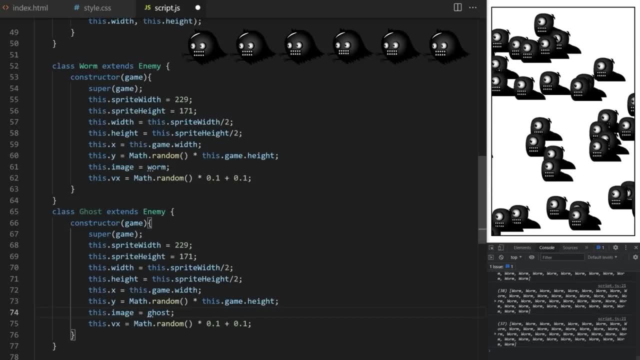 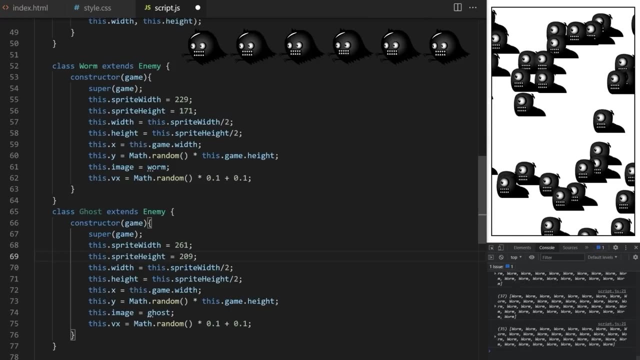 to ghost image on line 74 will be ghost reference in the ID here on line 13 in index HTML. I look at my sprite sheet width divided by number of frames. so sprite width of single frame is 261 pixels, height is 165 pixels and the 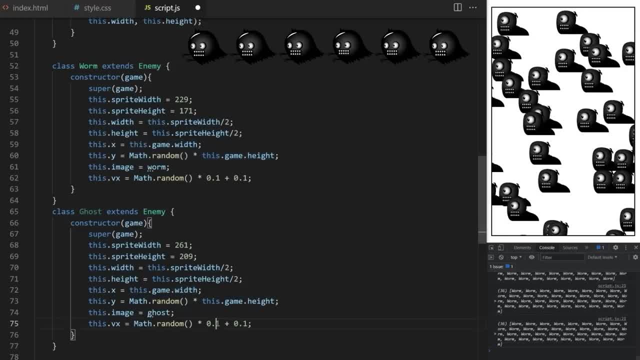 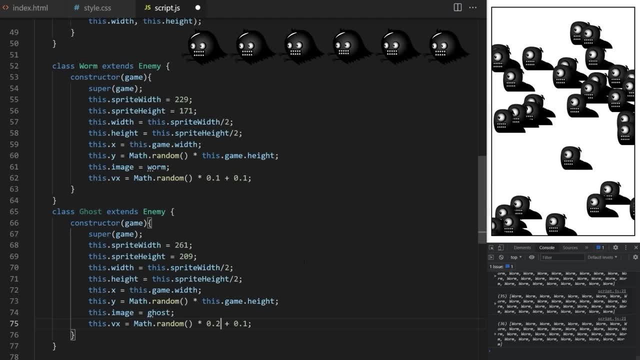 width: 209 pixels. in this case, horizontal speed modifier will be a little bit higher than worms. let's say a random number between 0.1 and 0.3. so that's the base ghost child class. how do I randomly push worms or ghosts into my game one? 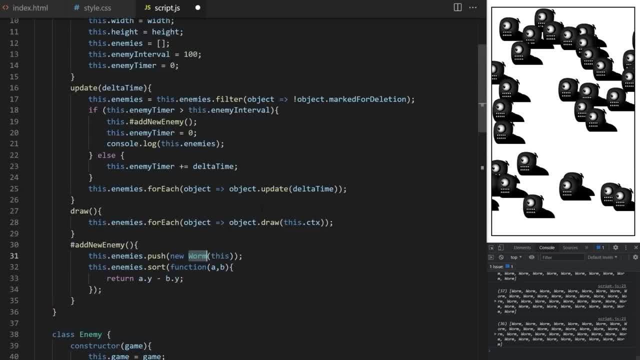 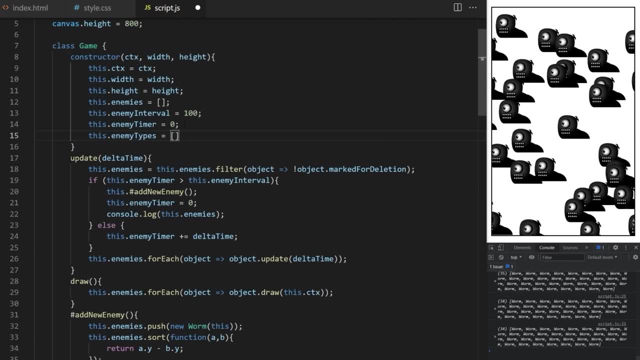 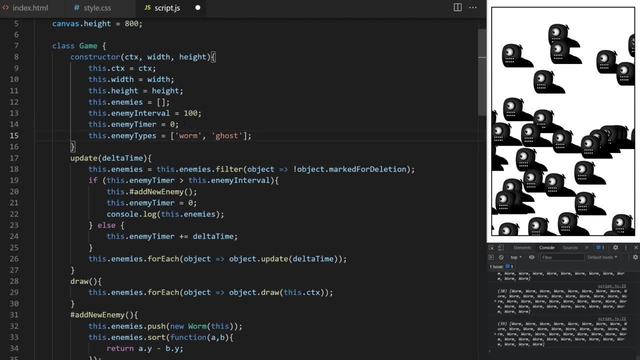 way to do that is to create a property on my main game object called this dot enemy types. it will be an array with two elements for now: worm and ghost. inside add new enemy private method. I will randomly pick one of the options in the array. I create a constant variable. 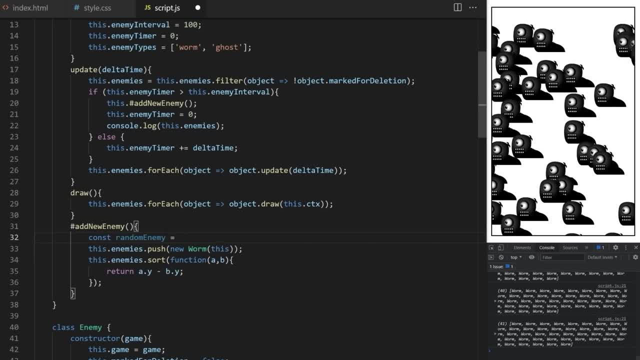 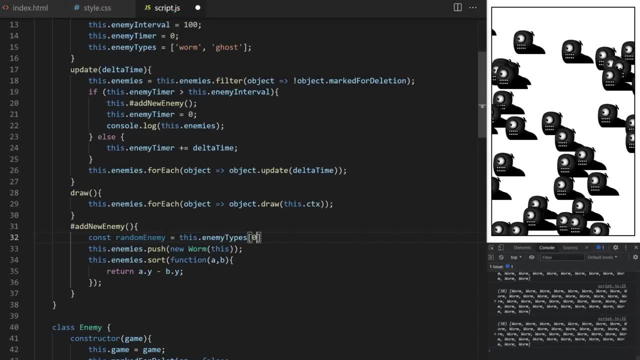 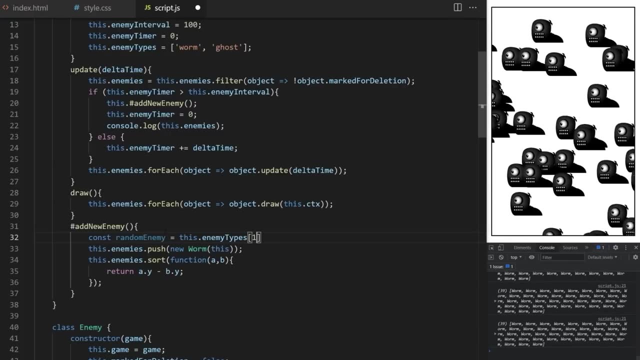 called random enemy and I set it equal to this dot enemy types and square brackets. so if index here is 0, we get worm and if index here is one, we get ghost. how do I randomize this index and let it choose one of these randomly every time we run? add new enemy method. I: 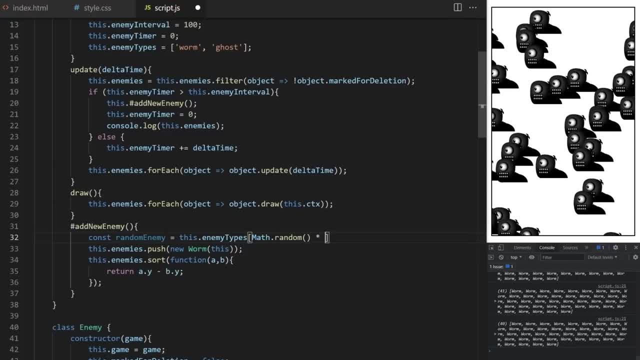 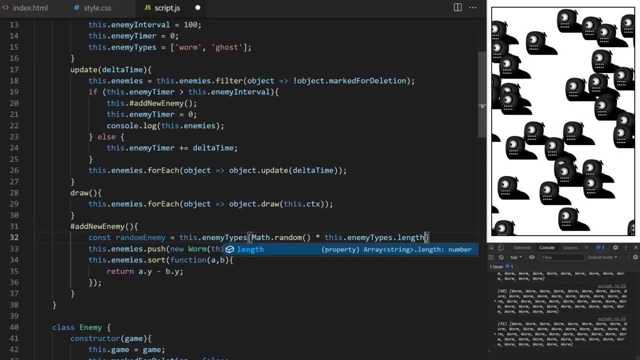 can just put math at random statement and it will be a random number, because it will be a random number between 0 and length of this dot enemy types array. that way I can keep adding more and more enemy types to the array and this code will still work. maybe my game will. 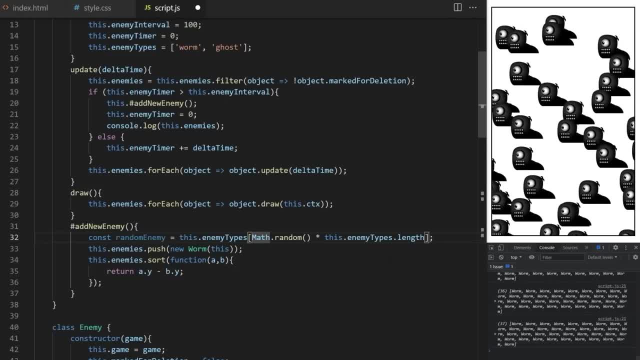 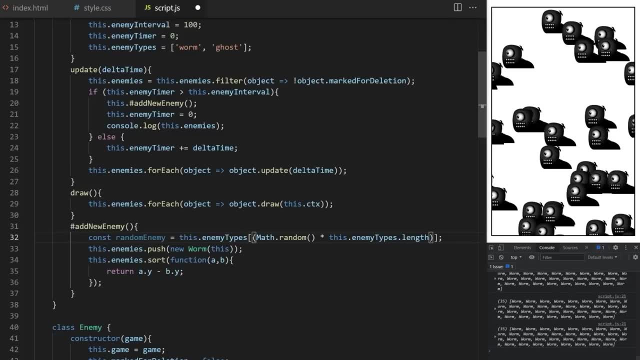 have 20 different enemy types, it doesn't matter, it will still work. the only problem is that math at random returns numbers with decimal points and there is no index 1.5 in this array. it's easy to fix. I will wrap it inside math at floor. 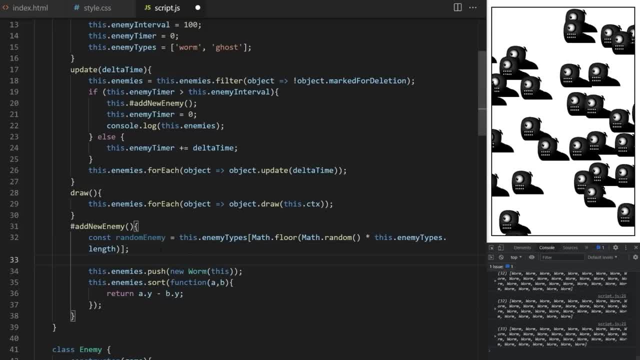 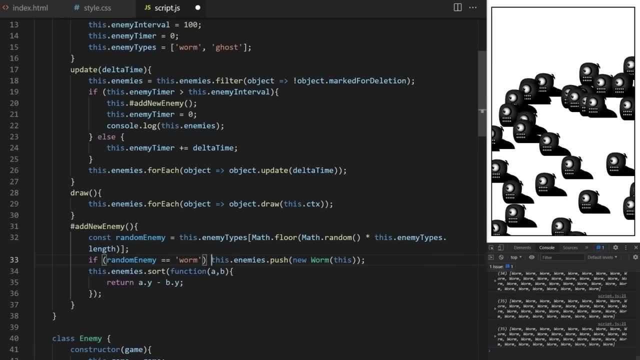 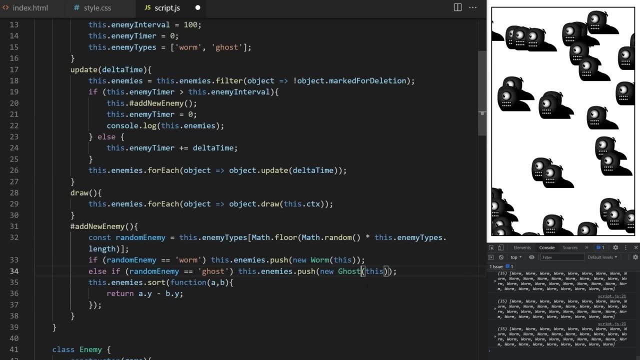 which will round it down to the closest integer. now I can check: if random enemy variable is worm, we will push new worm into this dot enemies array. else, if random enemy is ghost, we will push new ghost. perfect, so we have this dot enemy types array on the main game. 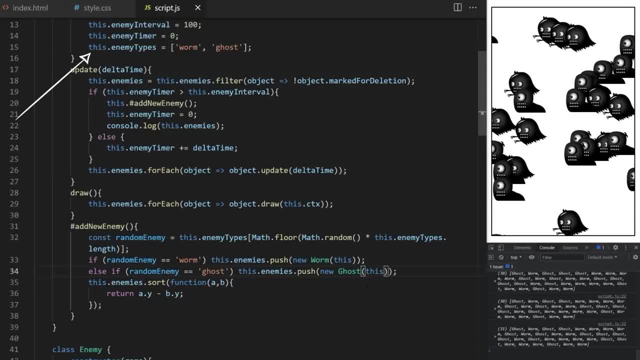 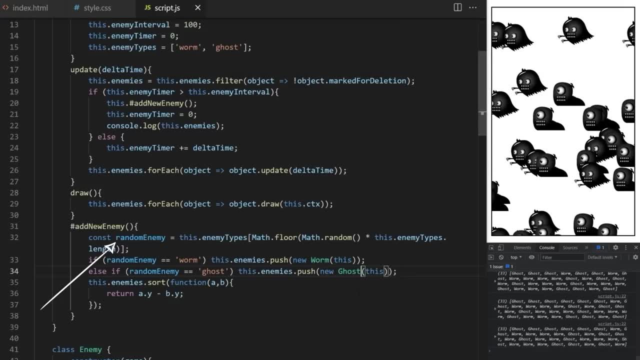 class. this can contain as many enemy types as you want inside. add new enemy. we randomly choose one of them every time we are about to create new enemy object and based on that random choice we create either worm or a ghost. so this is a ghost, so now both worm and ghost. 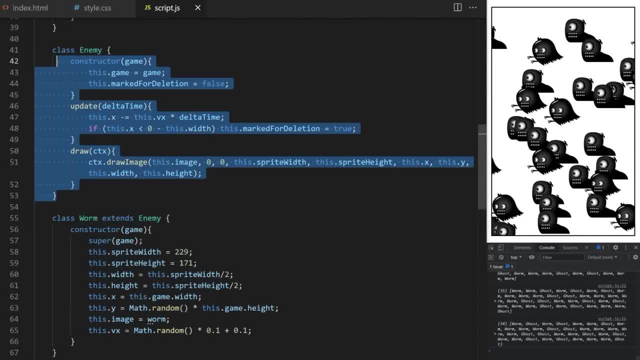 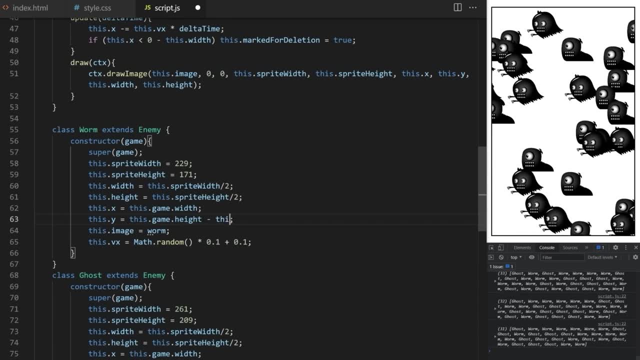 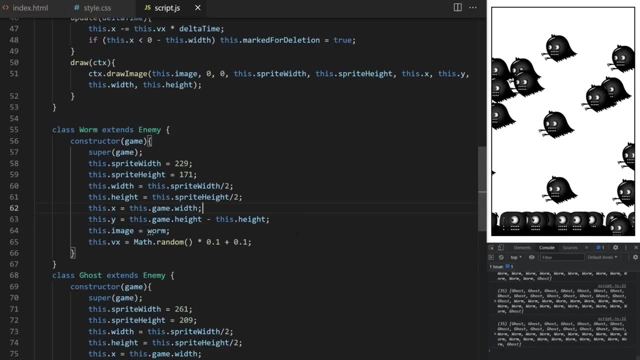 are child classes that extend my main enemy class. let's switch to kind of flat 2d view. I want worms to move only on the ground, so I change their vertical Y position to this dot game, dot height minus this dot height. worms are sliding on the floor, ghosts are flying in the 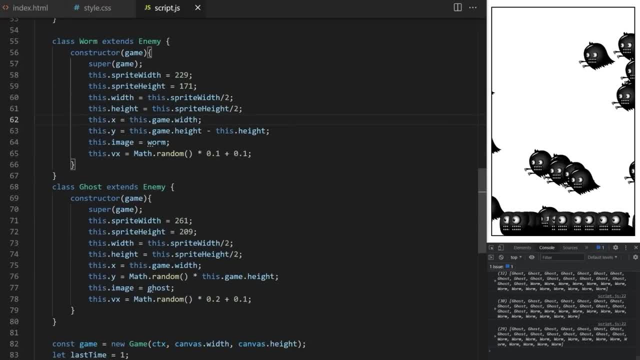 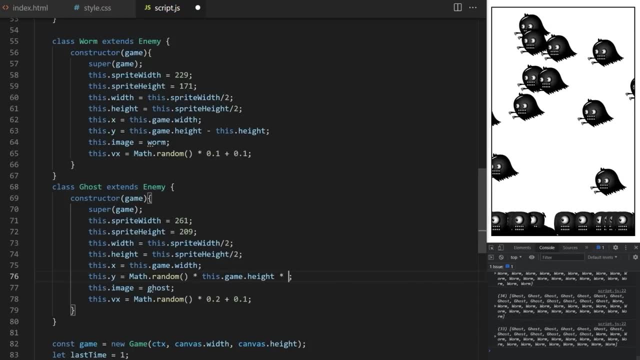 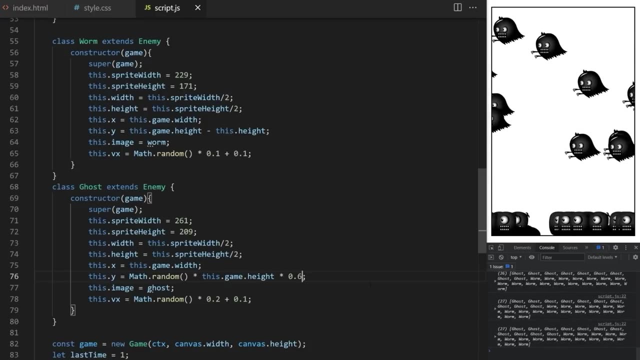 air. I want ghosts to take up only the top 80% of the game area, not to be so close to the ground. their vertical Y position will be a random number between 0 and game height times, 0.8 or maybe 0.6. yeah, since we switched to this. 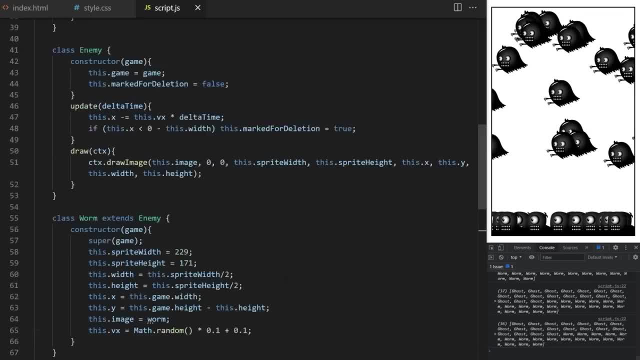 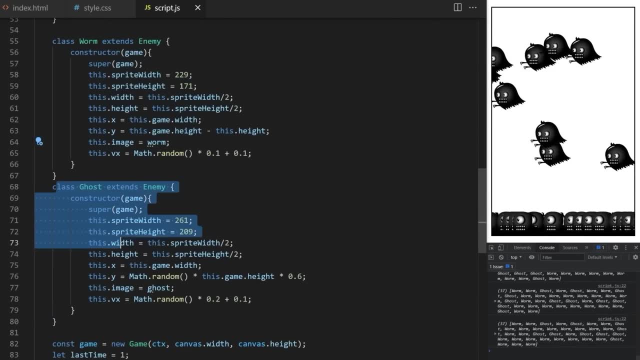 new view. I don't really need to be sorting my enemies by their vertical position anymore, so I comment out this code on line 35: with both worm and ghost we are only modifying properties on the constructor. they both inherited the same identical update and draw method from. 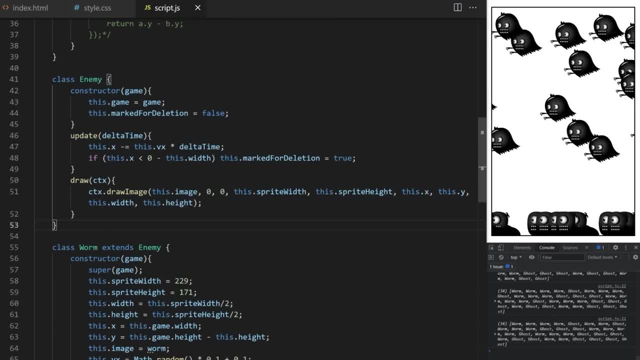 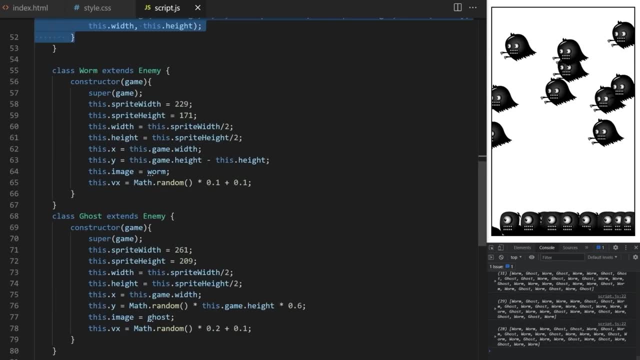 the main enemy class with no modifications at the moment. we only said we wanted to make the ghosts semi transparent. so let's do it. I declare draw method on ghost class. and now two things can happen. we can override the draw method with a completely different code here, because when we create a new 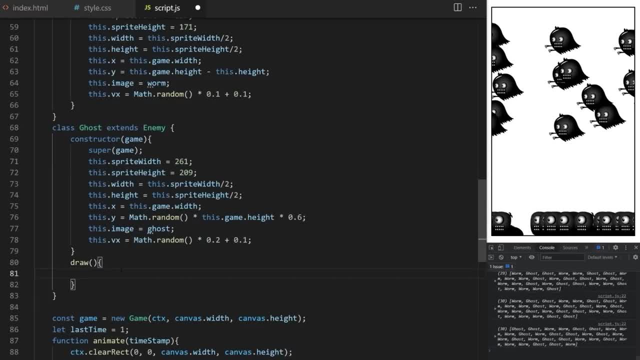 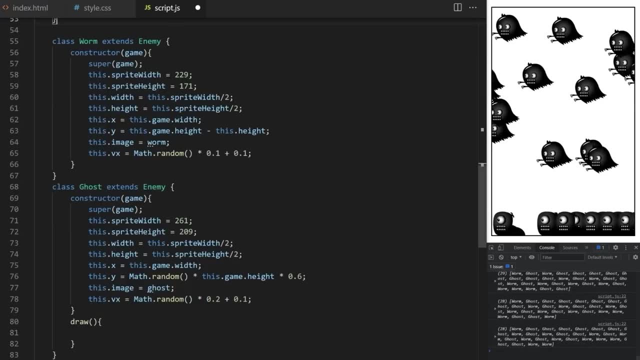 worm JavaScript will not find the draw method and we'll go looking for it on enemy parent class. but with ghost it will find the draw method right here and it will ignore the original draw method on enemy class. the second option is that I want the code from draw method on: 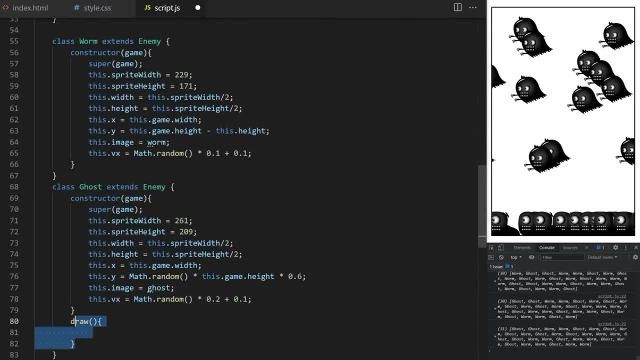 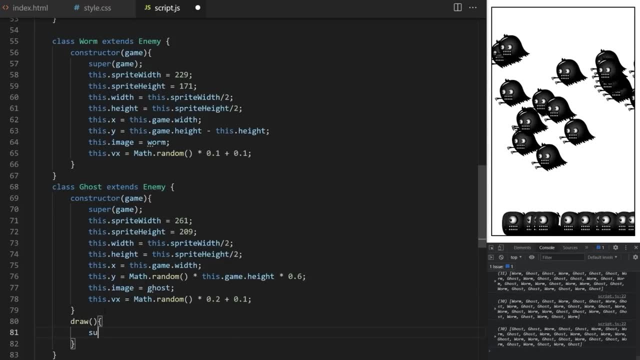 enemy class to run. plus, I want to write some additional code on top of it that will be unique only for ghosts. I can do that by calling super. the super keyword here simply represents parent class. so imagine I'm saying enemy dot draw because I want to call its draw method. 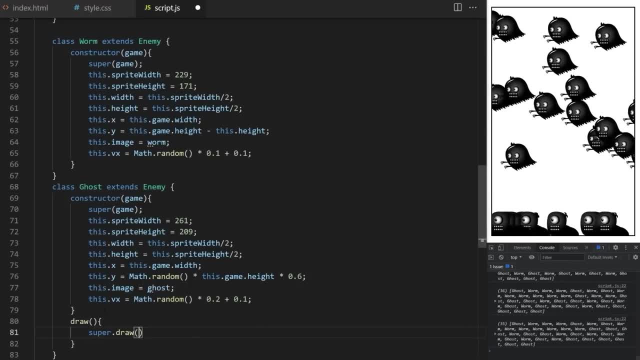 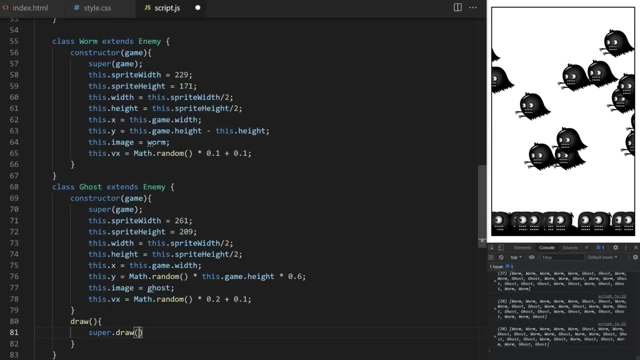 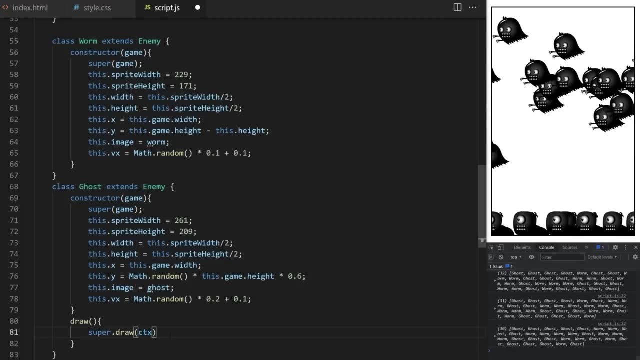 first, super dot draw means enemy dot draw. basically super represents the super class, the parent class. so here inside the draw method on ghost class. first I call draw method on enemy class and I know it expects CTX as an argument so that it knows what canvas we. 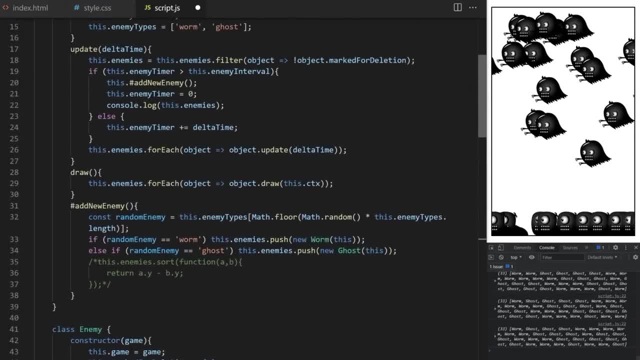 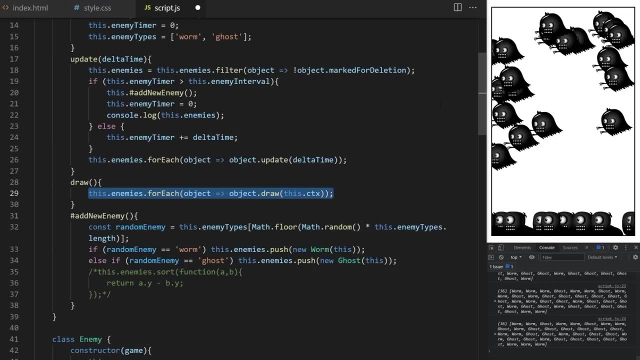 want to draw on. that CTX property is coming from here. on line 29, by the way, where I'm calling draw on all objects inside this dot enemies array, I'm calling draw on all ghosts and all worms at the same time. so first we call draw. 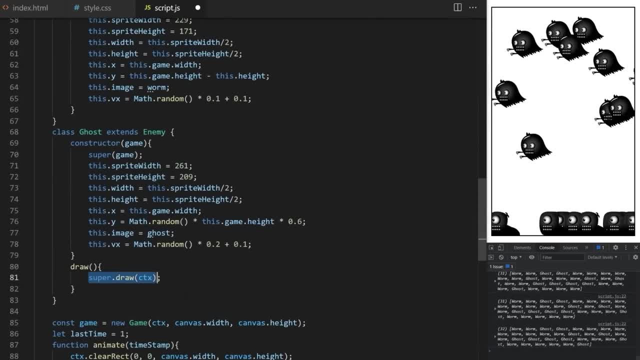 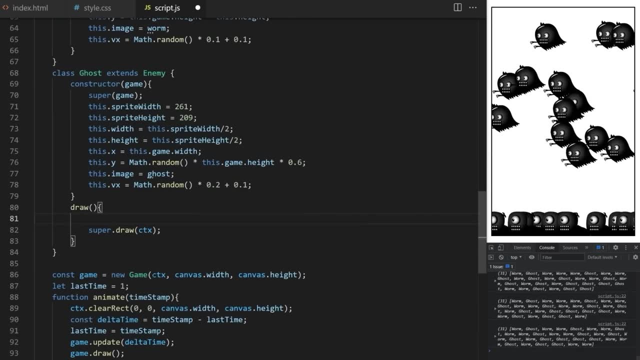 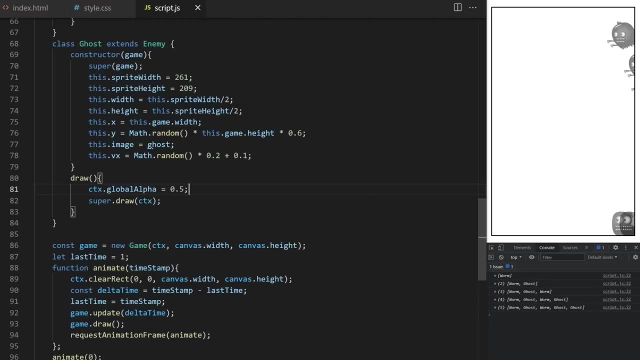 method on parent enemy class from line 50. we will run all the code in here, but we will also add some additional code that will be specific only for ghost objects. in this case I will set global alpha property to 0.5. this will set opacity to 50%. you can see that it. 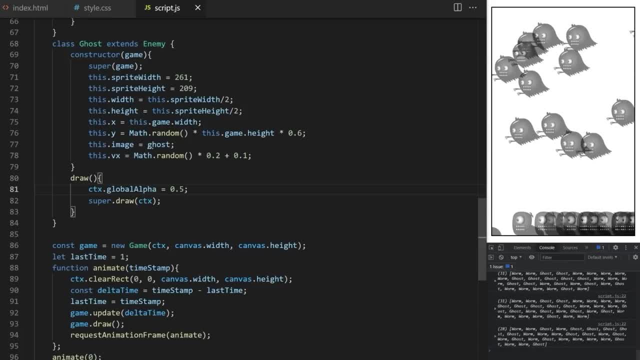 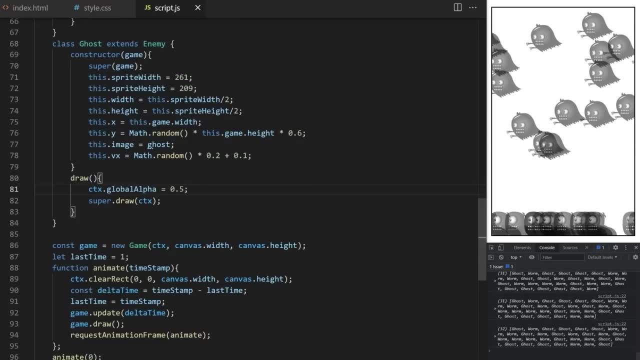 affects all ghosts and all worms as well. it's because global alpha canvas property works the same as fill style, for example. once you set it, you are setting it for the entire canvas. it will stay that value for everything drawn on the same canvas unless you redeclare it. 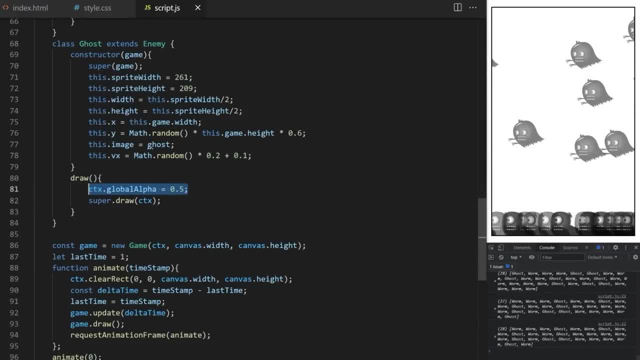 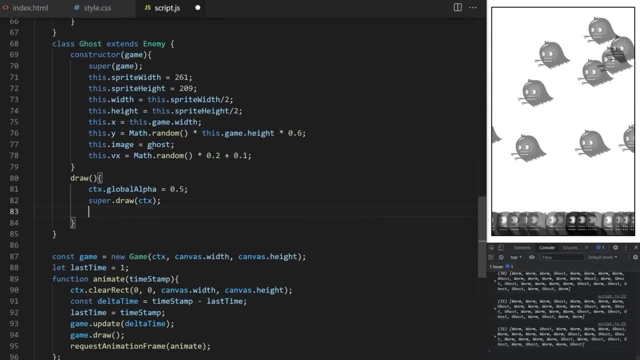 to something else. since I want to draw global alpha to only affect ghosts and nothing else on canvas, I set it to 0.5. I draw my ghost and I set it back to one. the alternative way to do this would be to call CTX save built-in method, which. 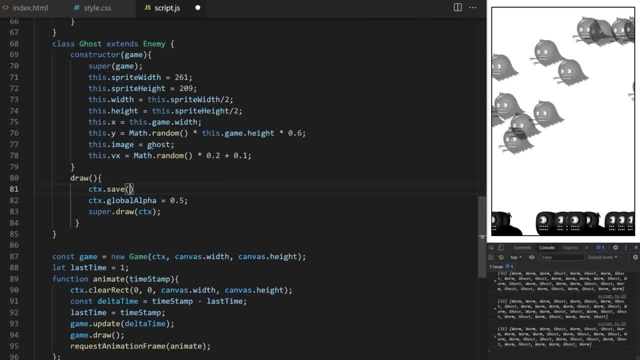 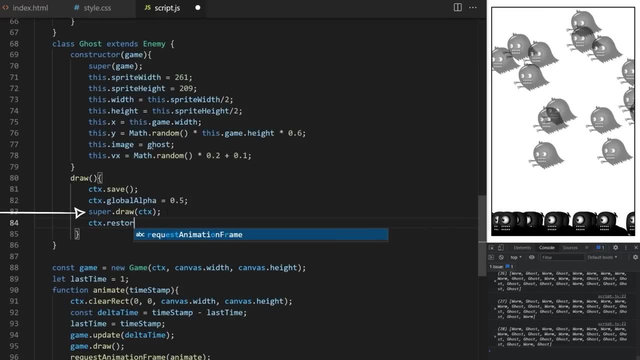 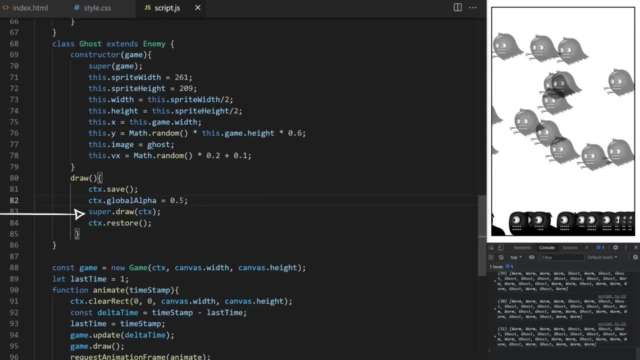 will take a snapshot of all canvas settings at that point. then we can change global alpha and anything else we need to change. we draw the ghost and we call CTX restore, which will automatically restore canvas properties, including global alpha, back to what they were at this point when we called. 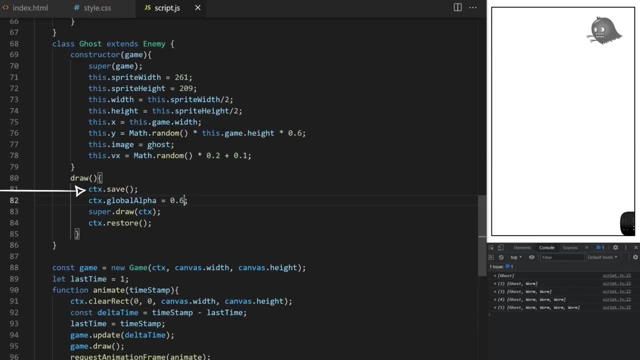 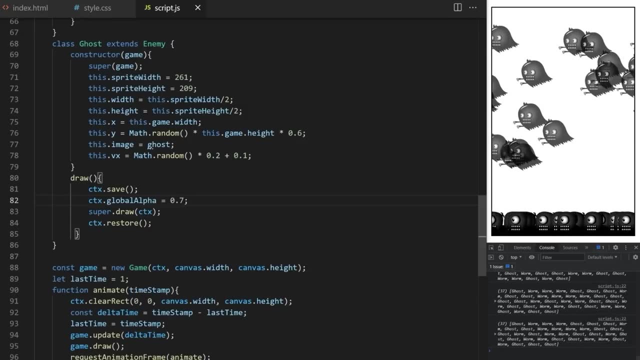 save for the first time. this technique is especially useful if I was changing multiple canvas properties at the same time, not just global alpha. so this is how you extend a method from parent class with a help of super keyword. now that we know how to do it, we can also. 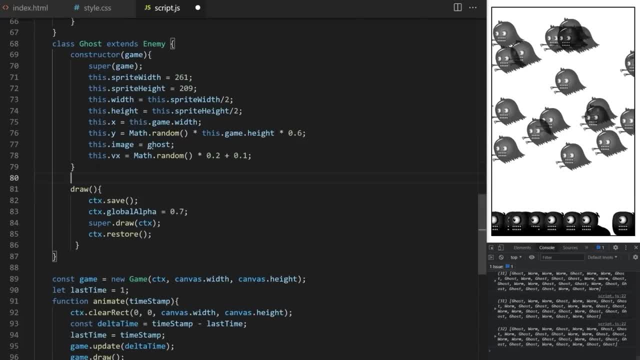 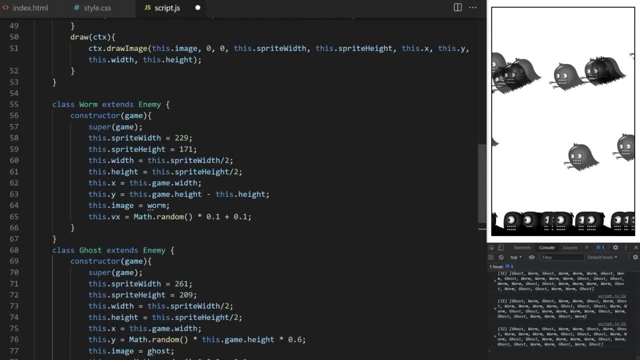 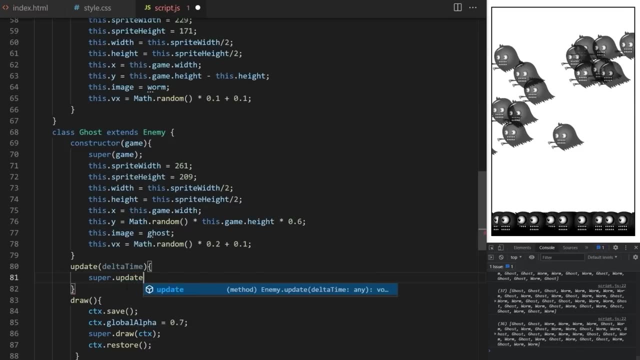 extend update method and make ghosts move in wavy patterns. let's try. I redeclare update method on ghost class and I pass it Delta time. I call super dot update and I pass a Delta time. this will run all the code in update method on enemy class from line. 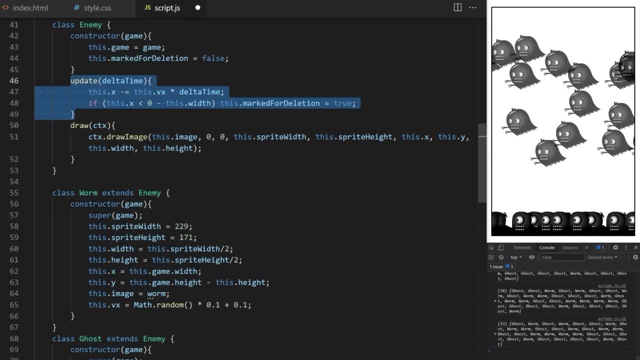 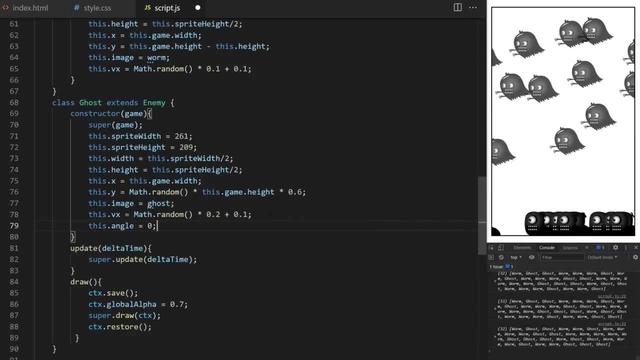 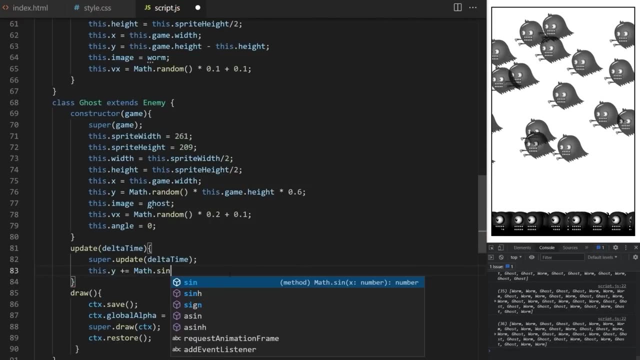 46. here I add a new property called this dot angle, and initially I set it to zero. then in update method I will say this: dot Y, vertical position of my ghosts plus equals mathsign- built-in JavaScript trigonometry function and I pass it- this dot angle, as an argument. 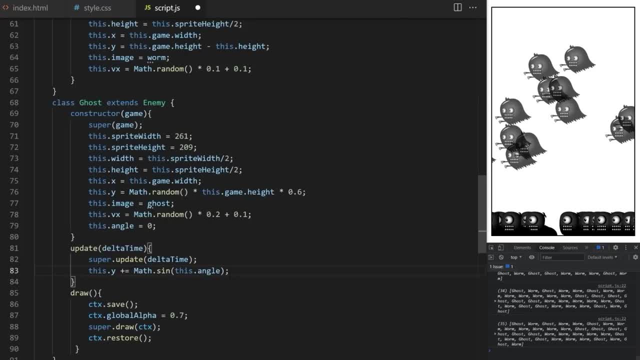 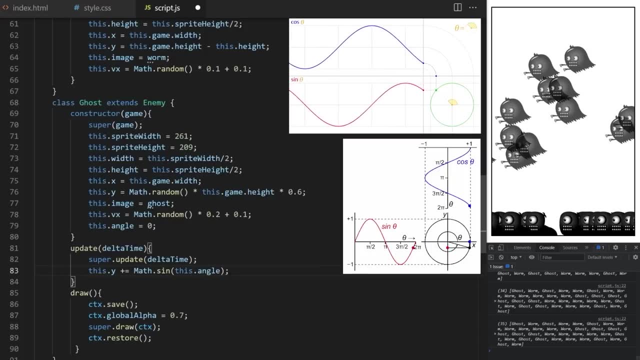 I covered this in my enemy movement patterns episode as part of this series before, so now just quickly. mathsign is a built-in JavaScript function that returns a sign of a number we pass to it. it expects angle value in radians and it will return a value between minus 1 and. 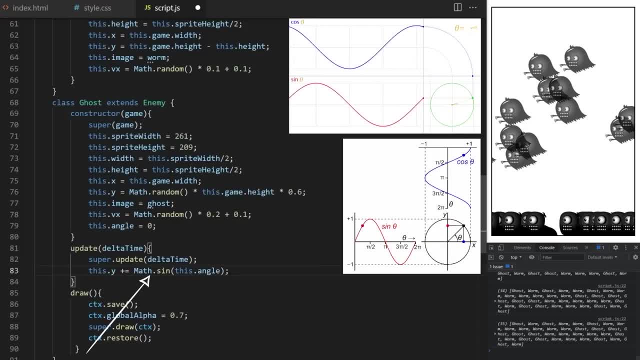 plus 1. if you keep calling it and passing it ever increase in angle value, as we are about to do here, it will endlessly cycle by small increments between minus 1 and plus 1, creating wavy movement pattern, so called sine wave. so every time update method runs, I will increase. 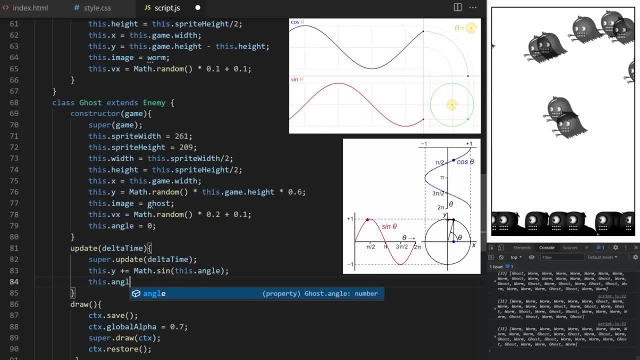 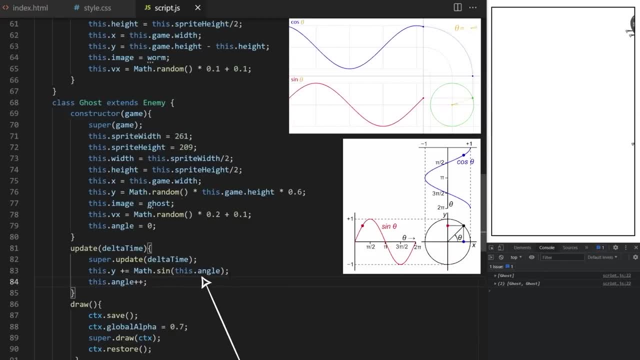 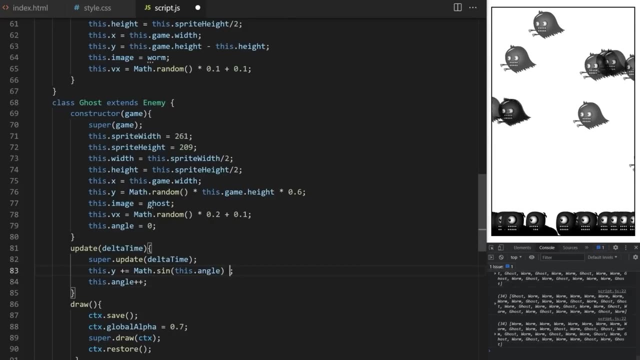 this dot angle from line 79 by 1. that angle value is being passed to mathsign function here at the same time. you can see, it makes the ghosts shake up and down. we can also multiply it times a certain radius value. this will make the curve larger. like this we need to be. 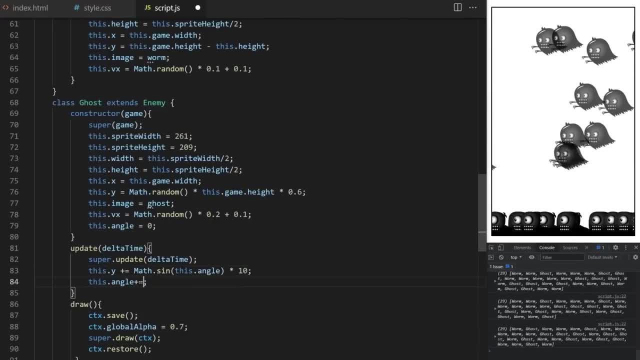 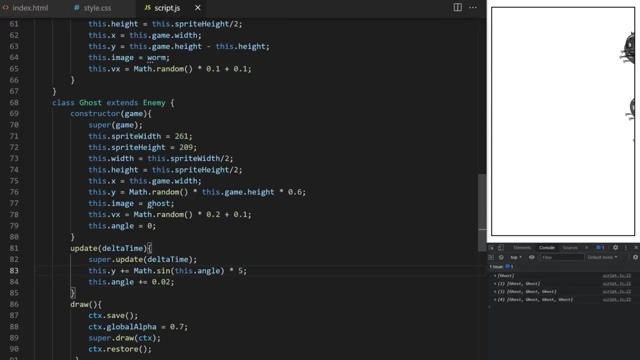 increasing angle much slower. let's see how it works. let's try 0.1 per frame, 0.05, 0.02. you can see how that affects the movement curve. I change radius value and angle value. let's randomize the wave size. for each ghost, I create a. 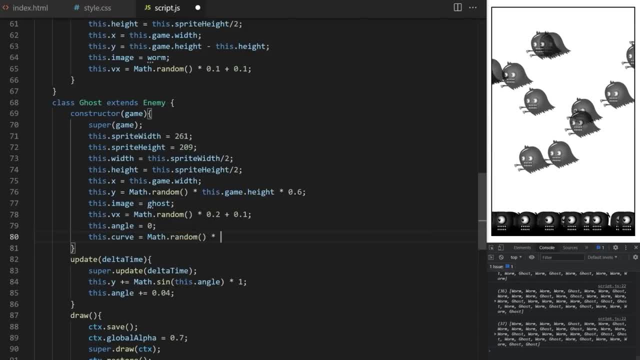 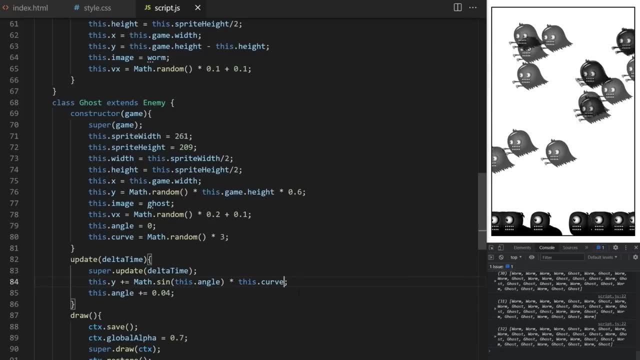 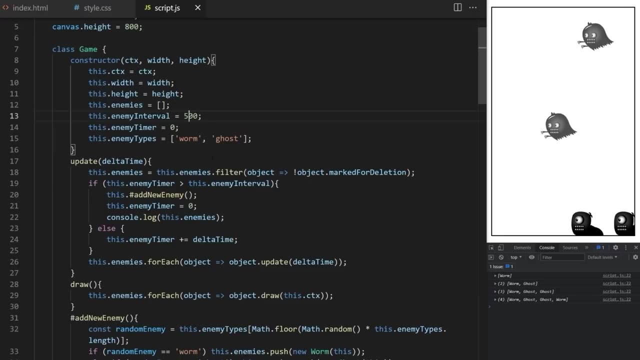 dot curve. it will be a random number between 0 and 3, and I use it here now. some ghosts move in smaller, some in larger waves. I reduce the number of enemies by increasing enemy interval on line 13. let's add a new enemy every 500 milliseconds for. 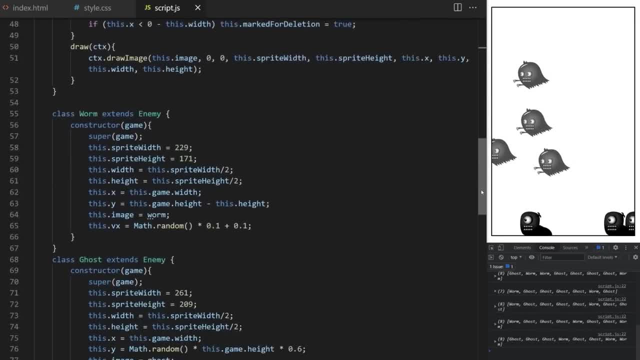 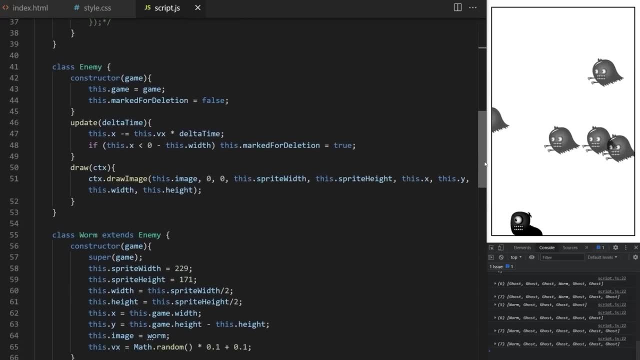 example. so with ghost class we are extending draw method to make it semi transparent and update method to give it wavy vertical movement. where we have a vertical movement, worm class is just using the base draw and update methods from its parent enemy class. let's create another child class and let me show you. 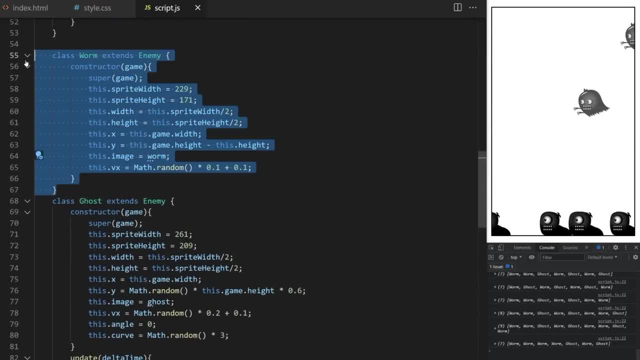 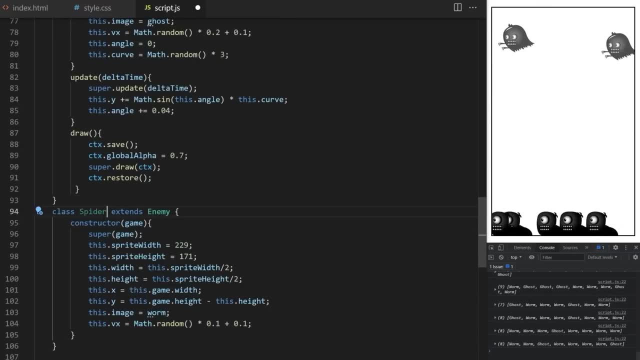 a completely different type of movement. for the third enemy type, I just copy worm class here so that I don't have to write all of that again. I will call it spider. I check my sprite sheet. sprite width. width of a single frame is 310 pixels. sprite height is 175. I want. 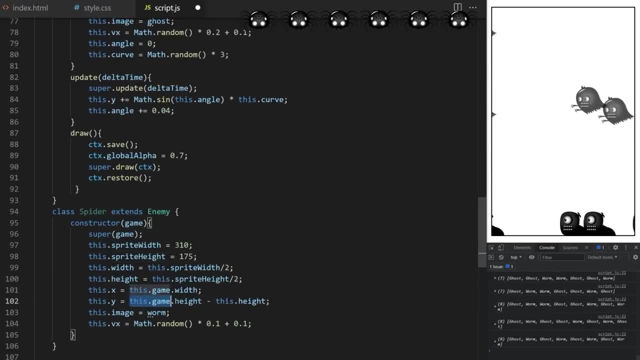 spiders to start from just behind the top edge of game area. so 0 minus this dot height, their horizontal speed will be 0. I only want them to move up and down. image will be spider. referencing this ID from line 14 in index HTML. I give them V Y, velocity, Y property and. 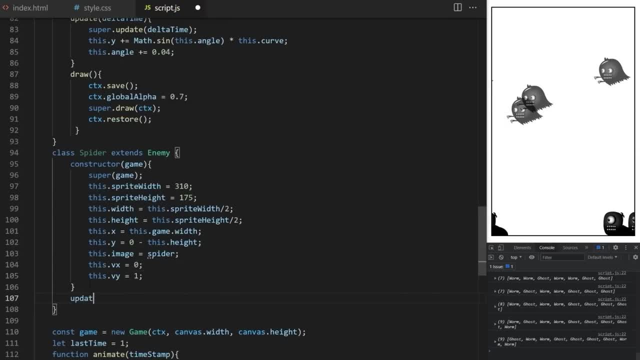 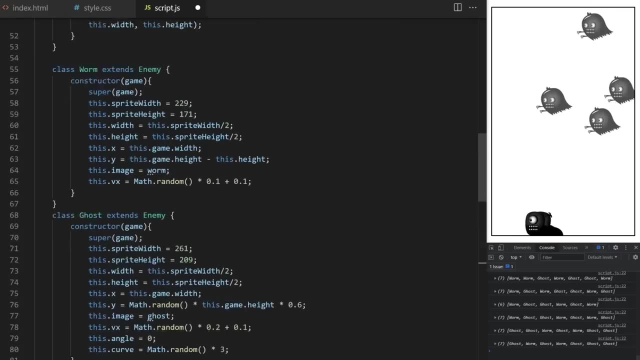 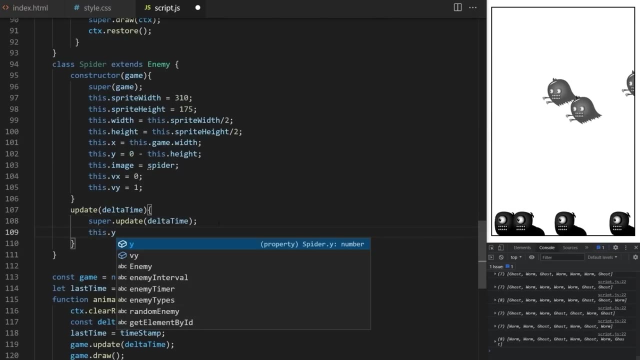 set it to 1. now I create update method. I pass it Delta time. first I call update method from parent enemy class from line 46, and then I add some additional code. at first let's just increase vertical speed by one. online 15. I add spider to my enemy types. 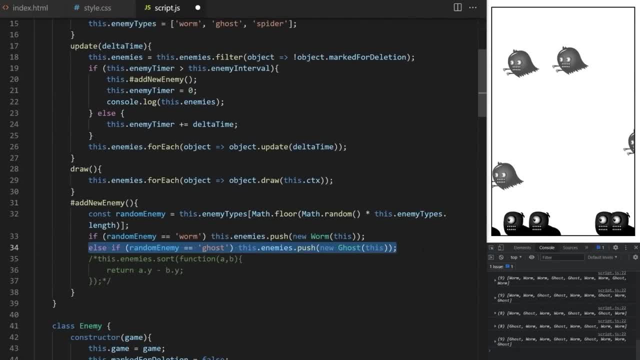 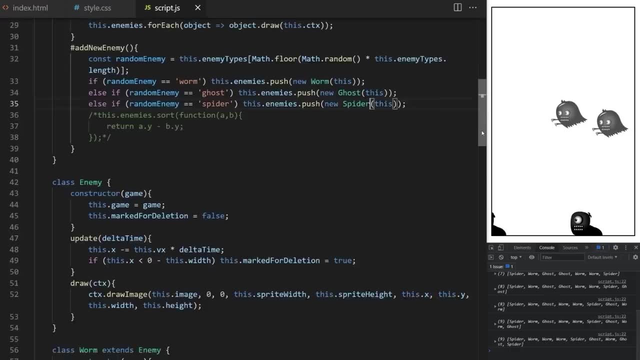 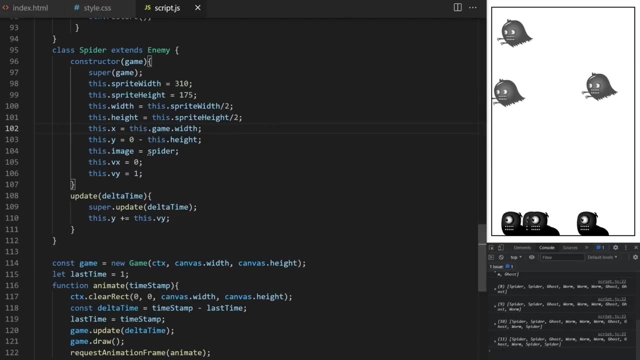 and here I say else: if random enemy is spider, push new spider object into enemy's array. my spiders are not showing and that's because, yes, they just move down and their horizontal coordinate is offset from the canvas so we can't see them. I said their horizontal coordinate to be a. 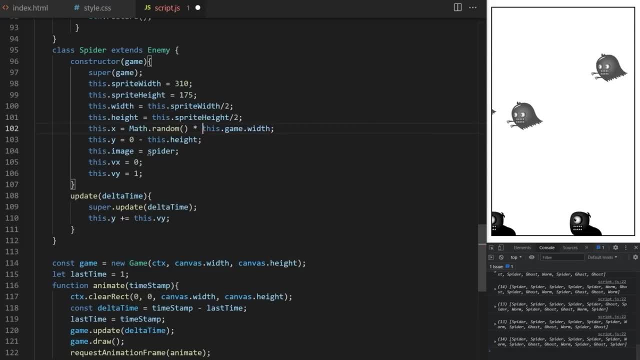 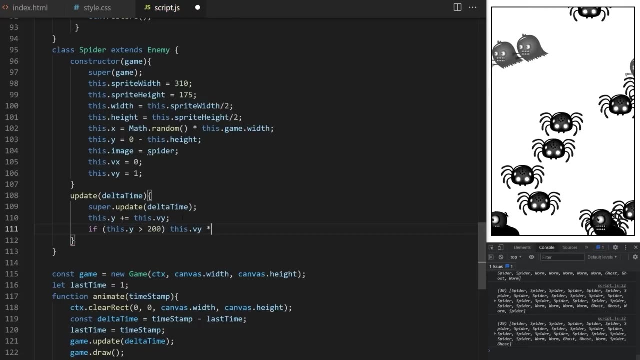 random number between 0 and game with nice. we have spiders here, let's make them move up and down. let's say, if this dot Y is more than 200 pixels from the top, revert this dot V Y to a negative number, since we are adding this dot V Y. 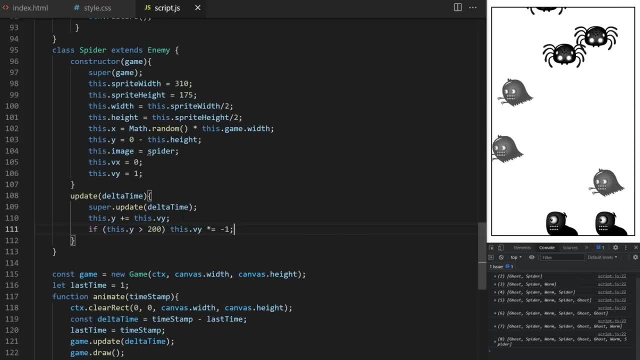 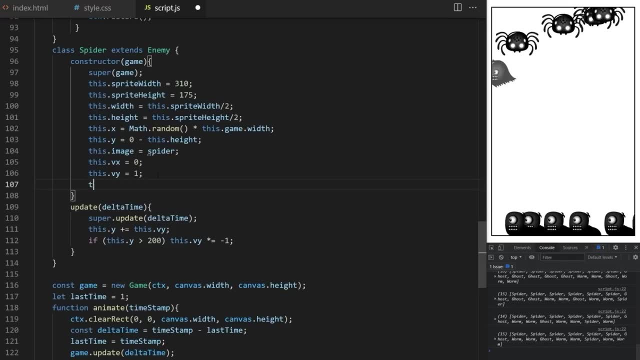 to vertical position here online 110. if it becomes a negative number it will make the spider go up. awesome, we have spiders going up and down. what about, instead of hardcoding 200 here? each spider will have a different maximum movement range. this dot max length is a. 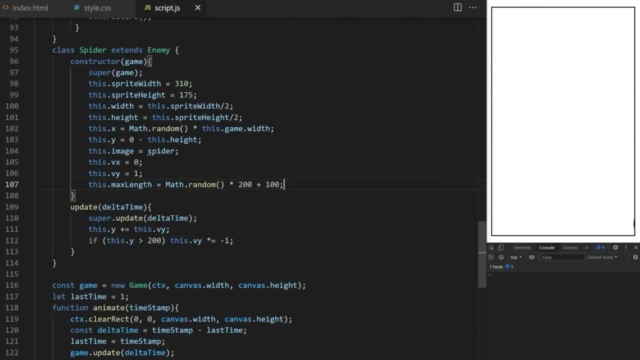 random number between 100 and 300, for example, actually between 0 and game height might be better. now I just replace hardcoded 200 with this dot max length. here I also want each spider to move up and down at different speed, so this dot V Y is a. 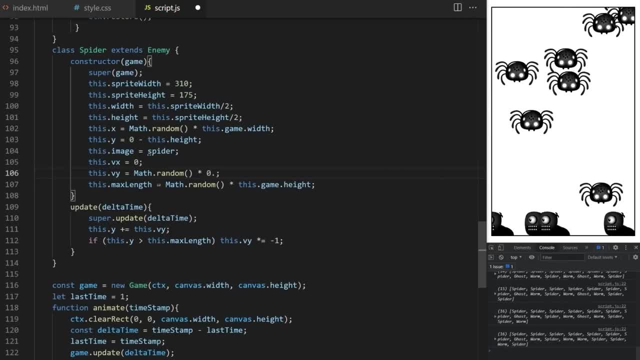 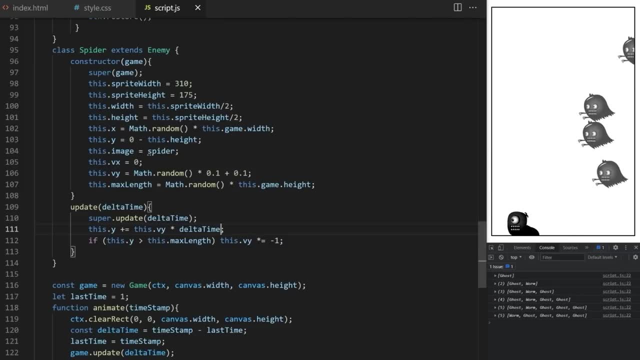 random number between 0.1 and 0.2. I should also multiply it times, Delta time, so we get consistency across different machines. I want the spiders to swing up and down from a spider web, so let's extend draw method as well and draw it. 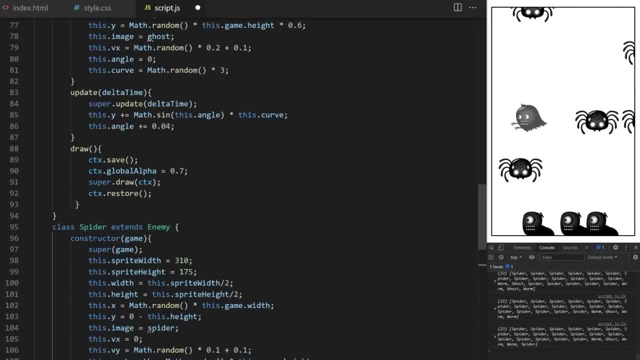 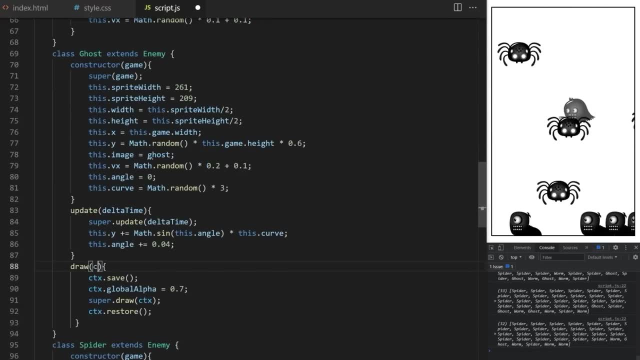 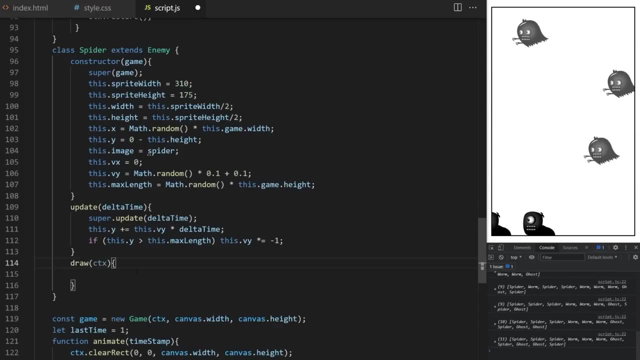 first I will call draw method from parent class from line 51. here on line 88 I need to pass CTX as an argument. I forgot to do that. we don't want to use global variables inside our classes, so online hundred and fourteen, I pass draw. 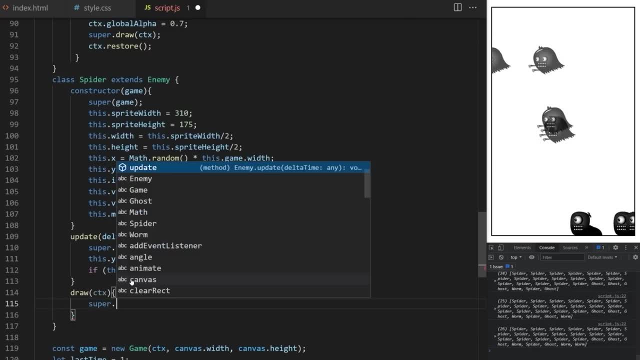 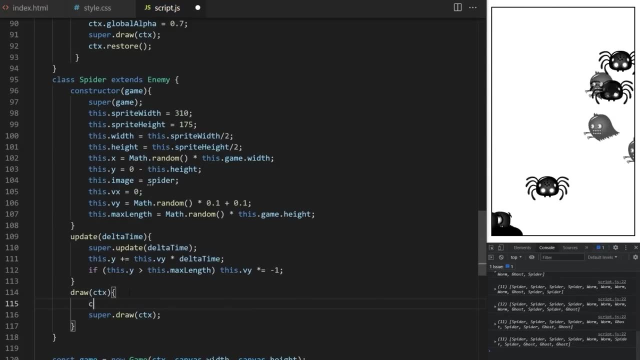 method CTX. I call draw from its super class, from enemy parent on line 51 to run all the code in there. and also I will draw a spider web here. so begin path to start a new shape built in canvas. move to method to set starting coordinates of the line. let's pass it. 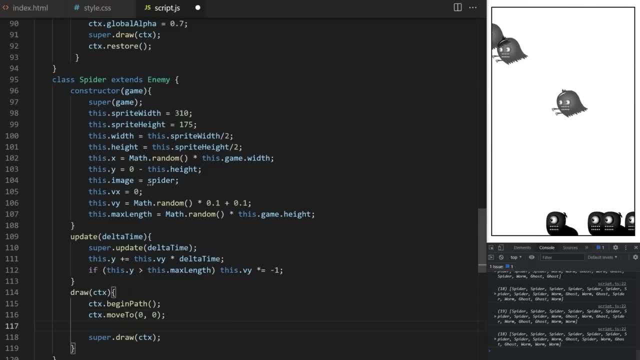 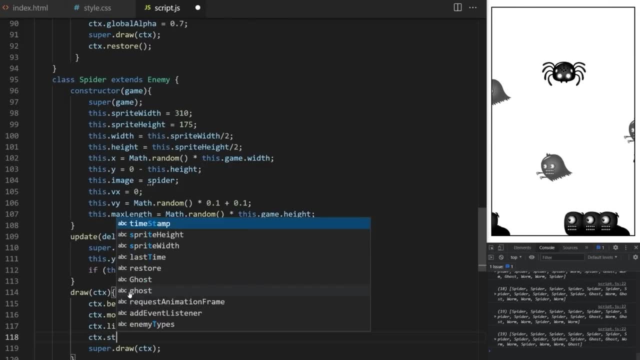 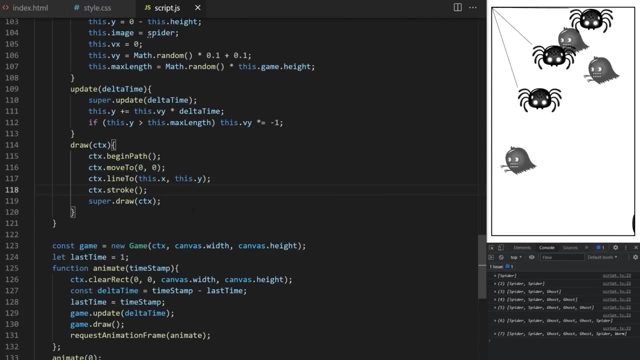 coordinates 0: 0. for now, line 2 will be the ending coordinates of my line. so this dot X, this dot Y, I want it to be where my spider is at the moment. I stroke the lines and here they are. we have spider webs coming from coordinates. 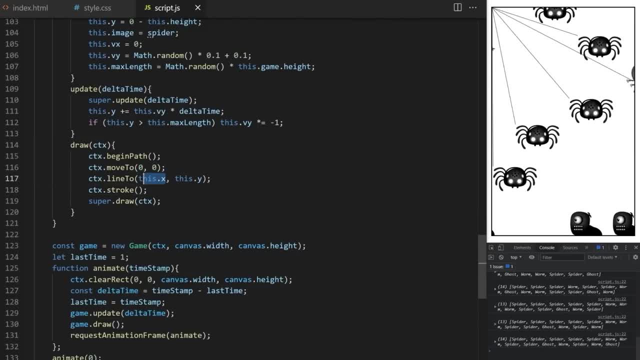 0, 0 to coordinates of my spiders. I change the starting coordinates to be exactly on top of the spider horizontally. so this dot X horizontal and 0 vertical. this dot X position is top left corner of my enemy rectangle. so if I want the web to come from the 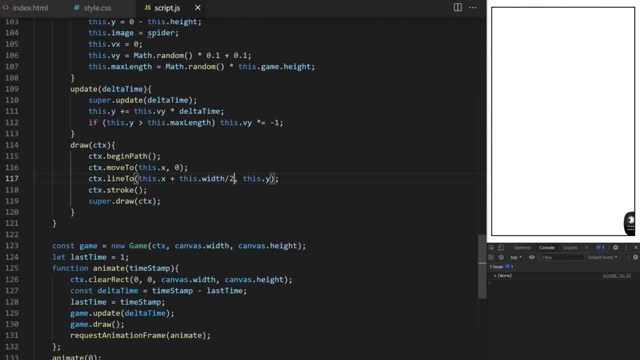 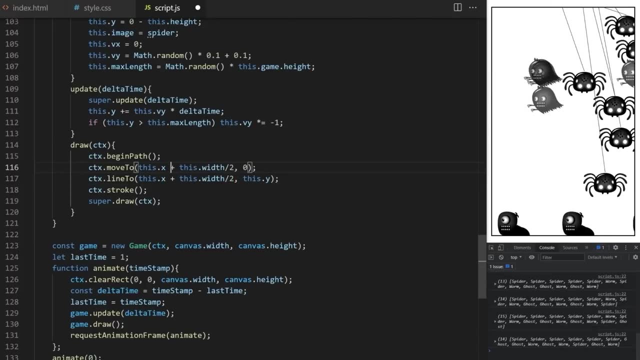 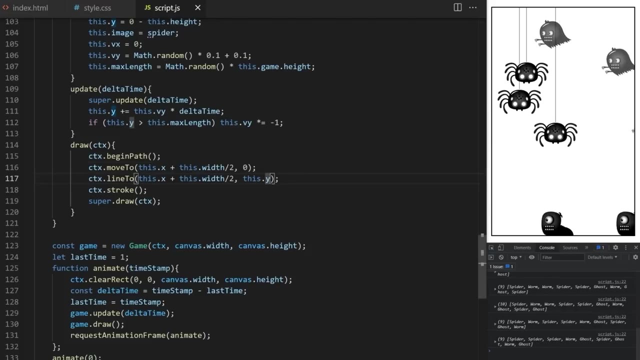 middle. I need to take this dot X position and add half of enemy width to it. I also do that for the starting coordinates. I can see there is a small vertical gap between spiders and the ends of their webs, so let's do this: dot Y plus 10. 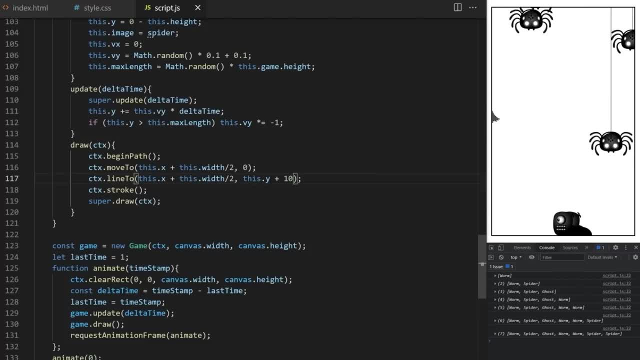 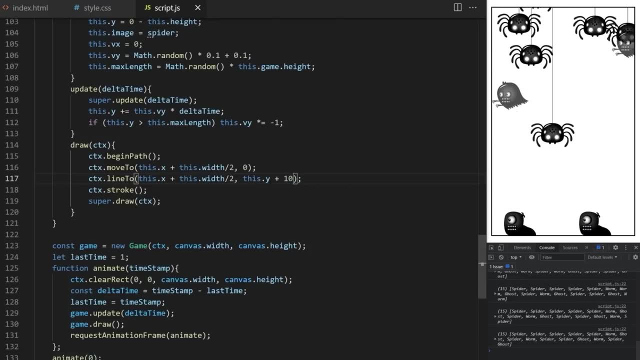 pixels to make the lines a bit longer. notice that I'm not actually animating the sprite sheets. we are just showing the first frame for each enemy type. the best thing about our code structure now is that I can just write sprite animation logic once and it will. 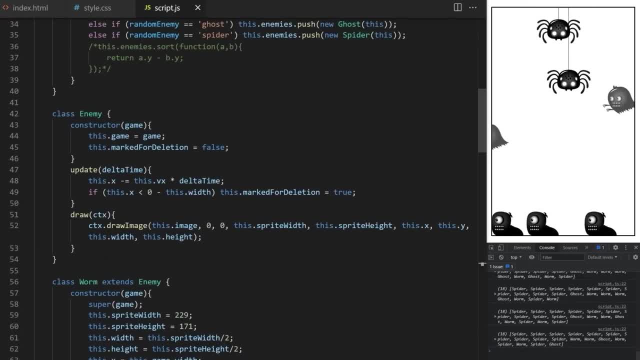 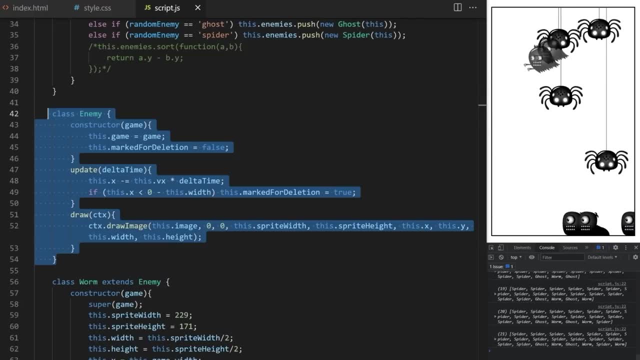 automatically be applied to all spiders, worms and ghosts. I go up to line 46 inside constructor on enemy class, where I declared properties and values that are shared between all enemy types in my game. we will need frame X property, which will cycle between 0 and 5 to specify which. 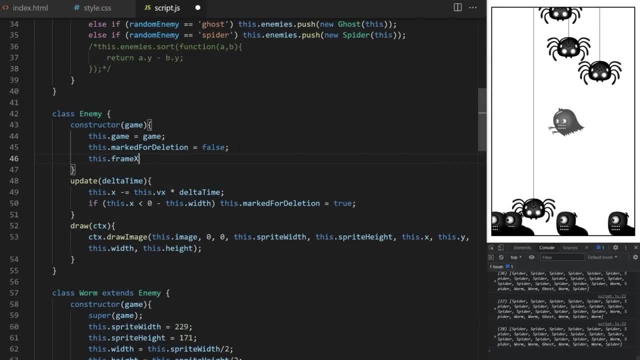 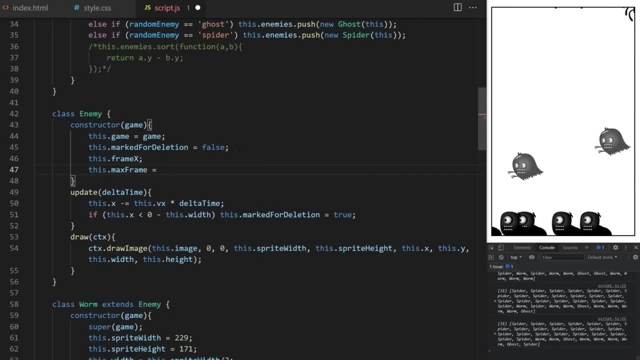 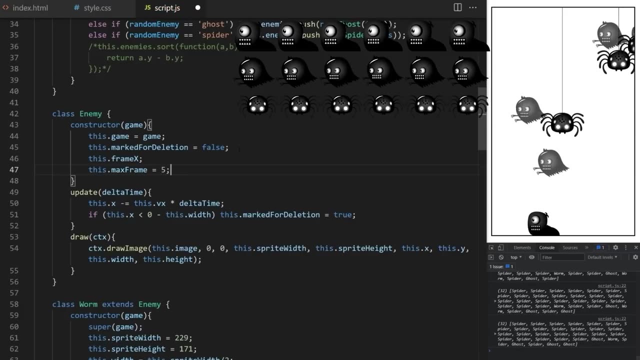 horizontal frame from the sprite sheet we want to show. I also declare this dot max frame, which could be specific to each enemy, but in this case all my enemy sprite sheets have six frames. we count from frame 0, so max frame is 5. I also need to account for Delta time when 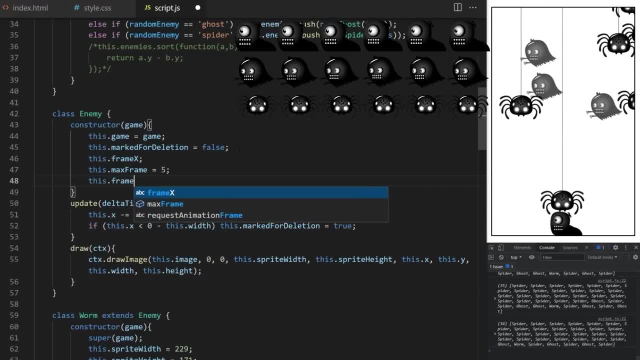 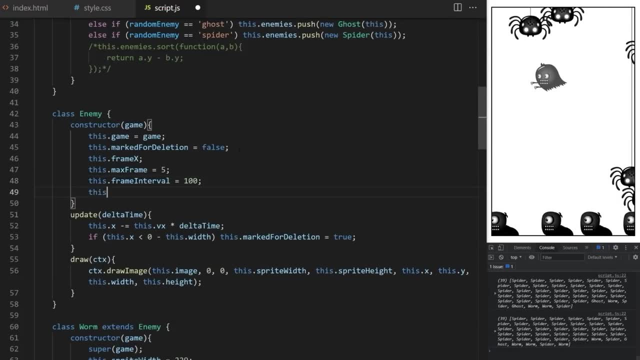 animating frames to make sure it runs at the same speed on slow and fast computers. we already done it once today. I will have five frames for each enemy frame interval variable, so let's say 100 milliseconds, and then I will have one accumulation variable that will be: 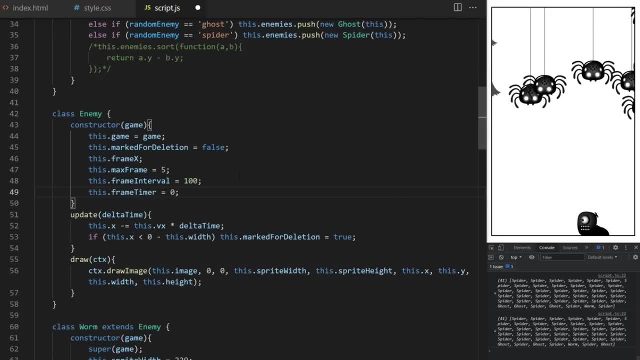 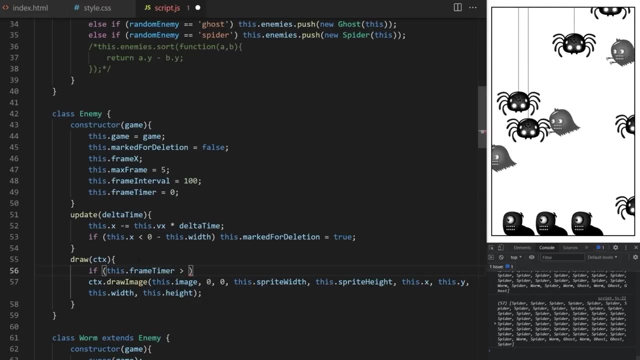 going from 0 accumulating Delta time until it reaches my frame interval value. I will call it, for example, this dot frame timer. I set it to 0 initially. I check if this dot frame timer from line 49 is more than frame interval from line 48. 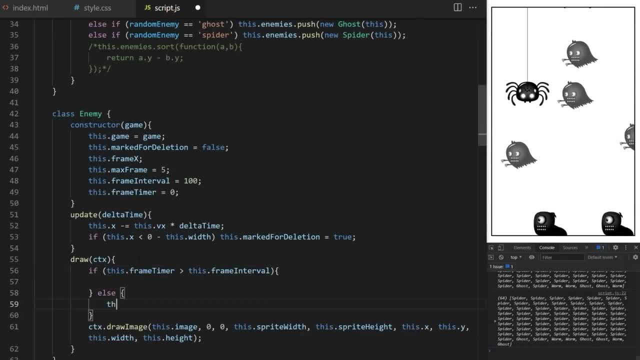 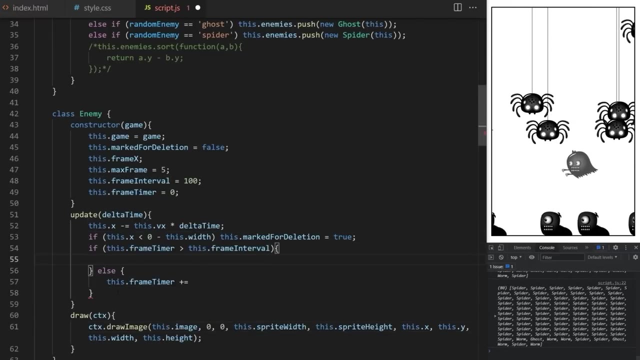 if it is, I do something else. I increase frame timer variable by Delta time. now I just realized we need access to Delta time here, so all this code actually needs to be inside update method here now I can say: frame timer plus equals Delta time. remember that Delta time is. 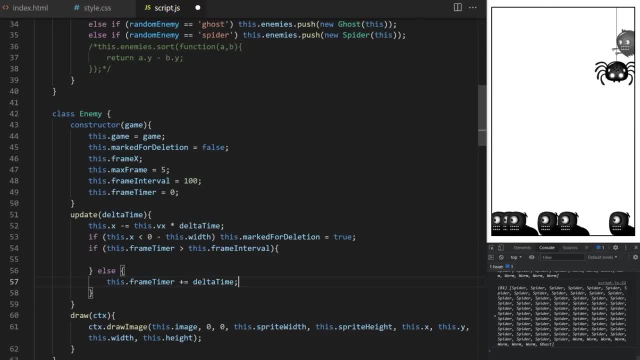 milliseconds between frames. so fast computers will serve frames of our game animation very fast but will have smaller Delta time. on the other hand, slow computers can't serve frames so often but their Delta time is less than their Delta time is larger. so as a result it evens out, and both fast and 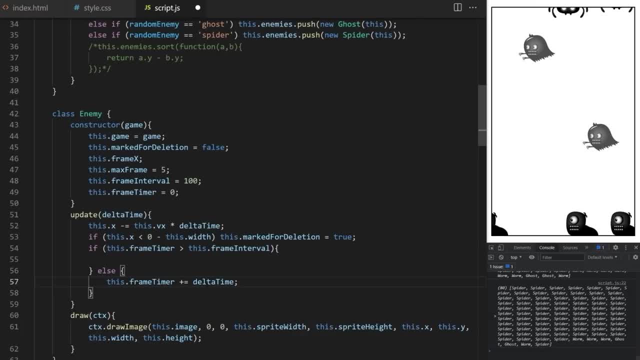 slow computers will reach frame interval of hundred milliseconds at the same time. this will ensure all the movement and animation in our games has the same timing, regardless of speed of the machine we run. the code on frame timer will start at 0. it will be increasing by Delta time and when it 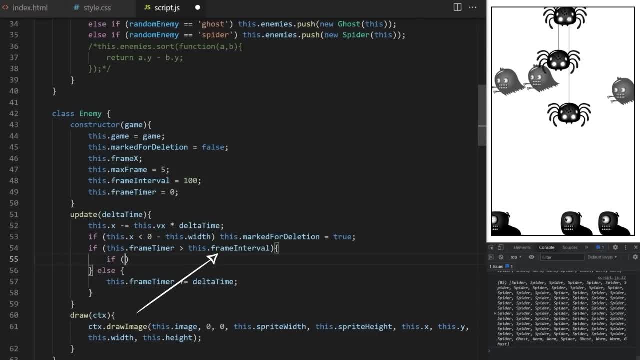 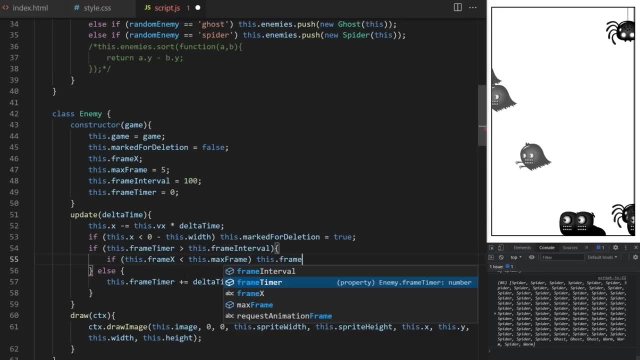 reaches frame interval, we can move to the next frame. in sprite sheet I have to check if current frame X from line 46 is less than max frame from line 47. if it is less, we increase frame X by 1, else we set frame X back to 0 at the same time I 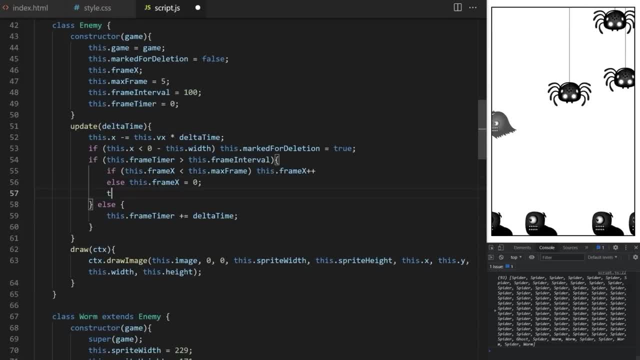 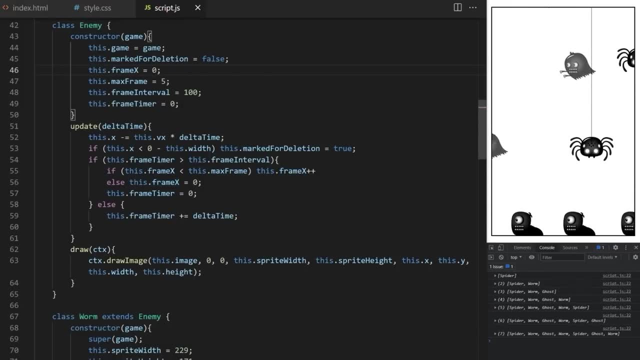 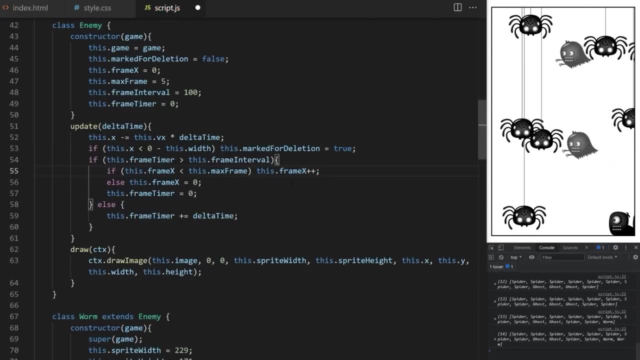 set frame timer back to 0 so it can start accumulating Delta time again. on line 46 I set frame X initially to 0. now I'm cycling between frame X 0 and frame X 5. to actually display that in game I have to replace hard-coded source X and. 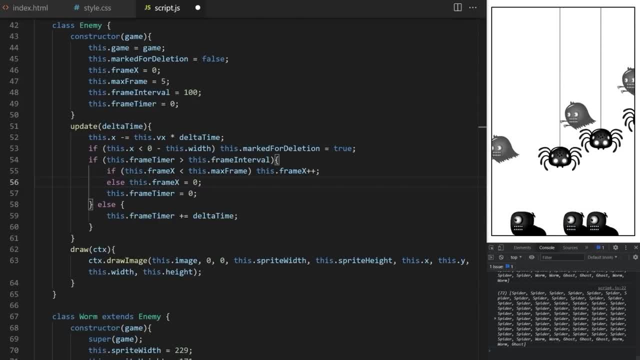 source Y properties in draw image method, which I set to 0- 0. I have to replace them with my new variables. source Y can actually stay hard-coded to 0 because our sprite sheet has only one row. there will be no vertical navigation within this sprite sheet. 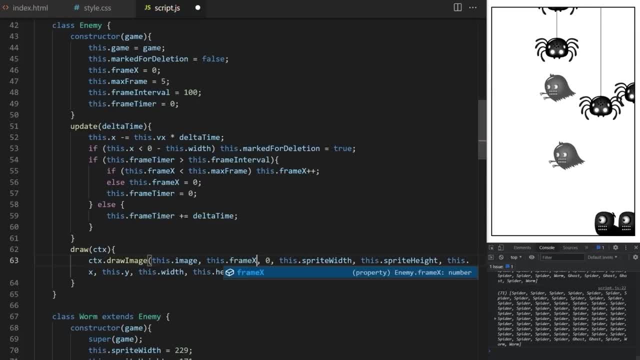 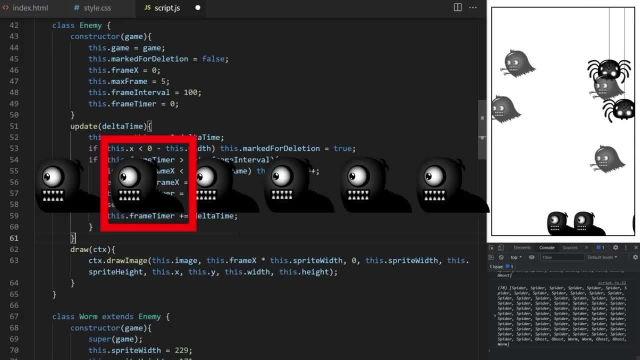 source X argument will be frame X from line 47 times sprite width from line 70. that way, when frame X is 1, we cut out this frame. frame X 2 is this frame, and so on. I have entire episode on this as part of this series, if you want more. 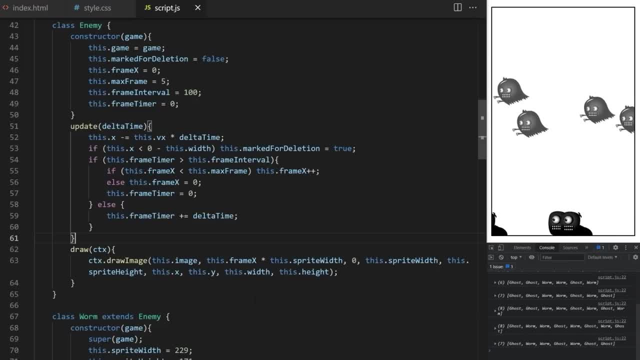 details about how to animate sprites properly, and in that episode I also show alternative techniques, how to do this. I can also add more functionality here in update method on enemy class and it will be shared across all my enemy types. it could be, for example, collagen checks with player, some JavaScript generated. 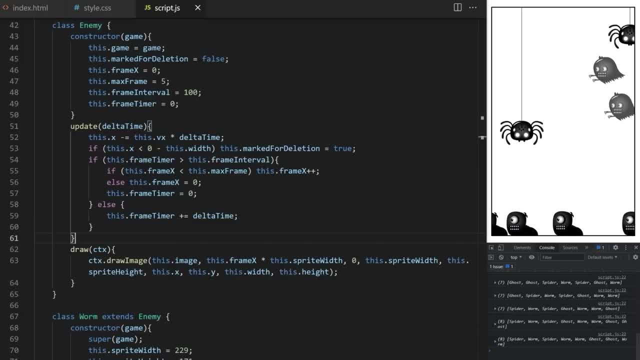 sounds. enemies can have particle effects and so on. being able to write code here in one place and share it for all my enemy subclasses will save a lot of code repetition that would happen otherwise. on line 53, I'm checking if enemies have moved behind the left edge. 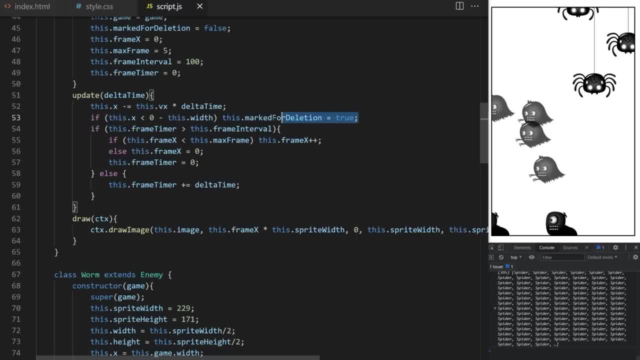 of screen and I'm marking them for deletion. this check works for both ghosts and worms as they move from right to left. the problem is that spiders never move past that point. they have no horizontal movement. so, as you can see in the console, if I let my game run, it will. 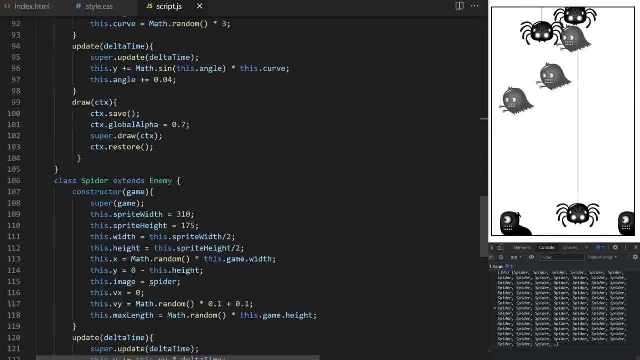 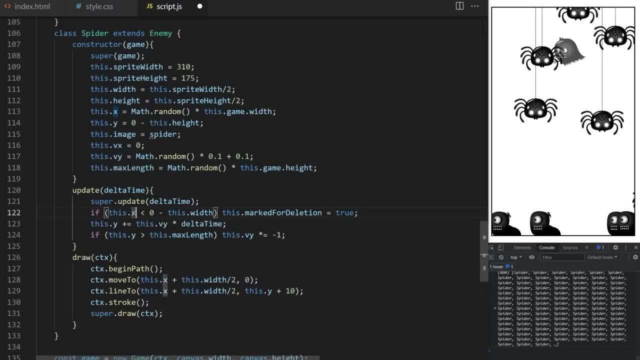 just keep accumulating more and more spiders. I need a different check here. to mark spiders as ready to be deleted, I go inside update method on spider class and I say: if this dot Y is less than the zero minus this dot height times two, then mark it as ready for deletion. 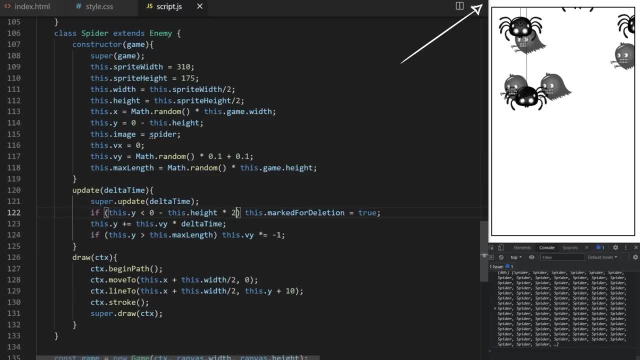 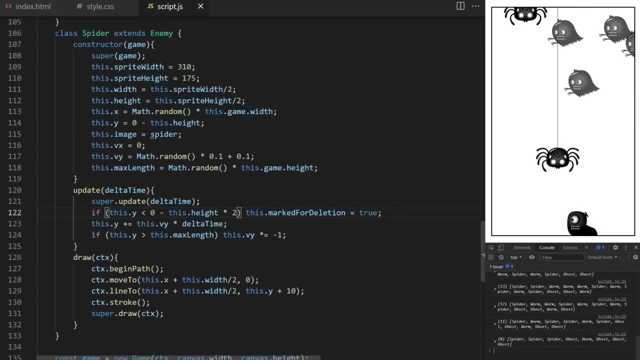 spiders start at zero minus this dot height, as declared here online hundred and fourteen. they will move down and then they will move back up. when they reach point zero minus this dot height times two, we delete them. I will be extending classes a lot in my games, so I 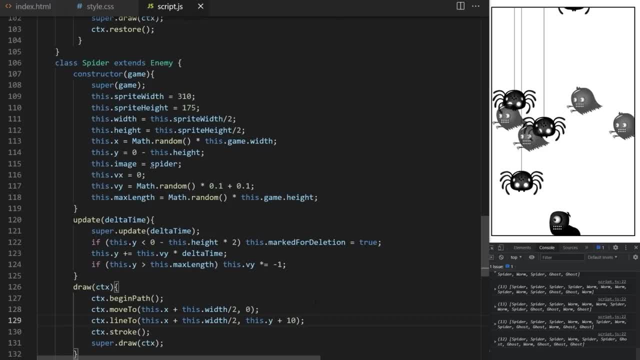 hope you learned something new today. creating child classes is not only useful for animations and game development, but it's a very important JavaScript technique with many different applications across all front and web development. I think sometimes it's better to learn these concepts on fun projects like this to learn more. 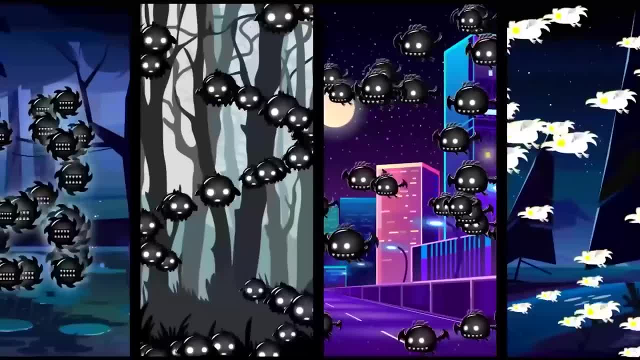 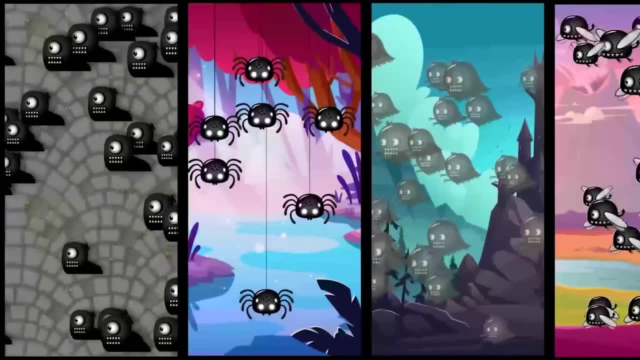 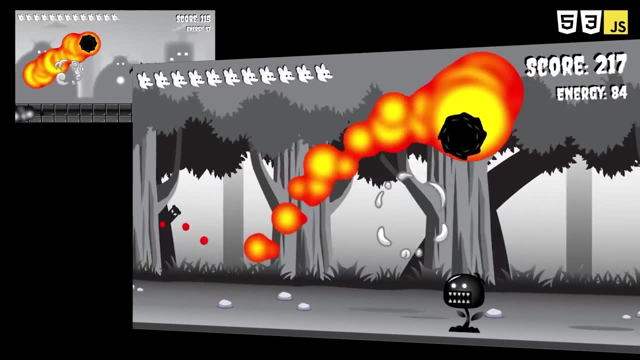 fundamental JavaScript techniques on creative coding projects. check out related videos in the video description. great job on completing today's course. say hi in the comments. hey, coders, so I heard you like making games- me too. I think projects like this are great, not only for aspiring game. 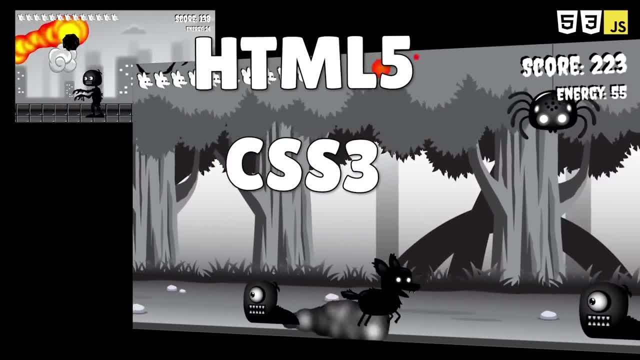 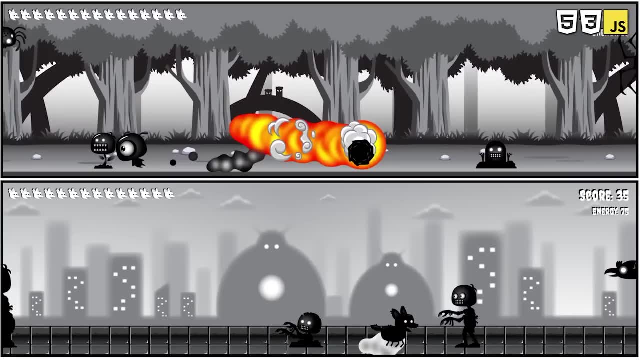 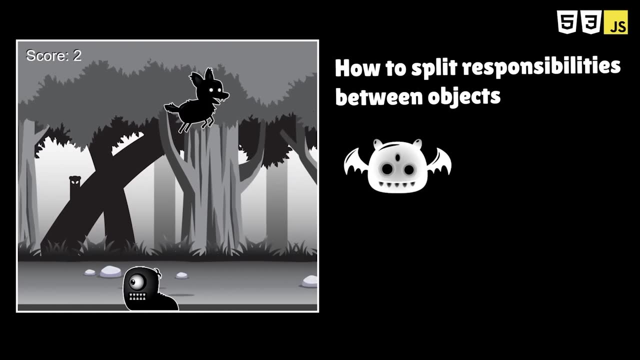 developers, but also to learn and improve HTML, CSS and JavaScript skills. in this class, we will build easy animated side-scroll game completely from scratch with plain vanilla JavaScript, no frameworks and no libraries. the main goal today is to learn about basic code structure, how to split responsibilities between objects. 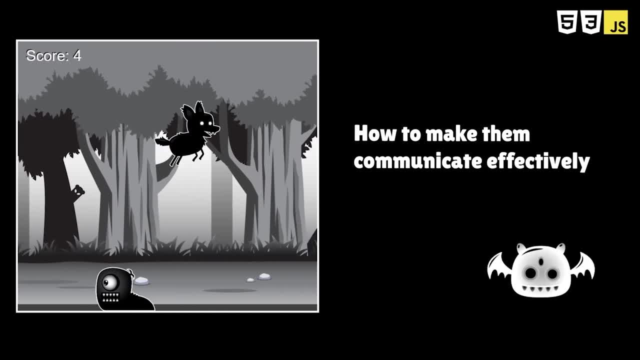 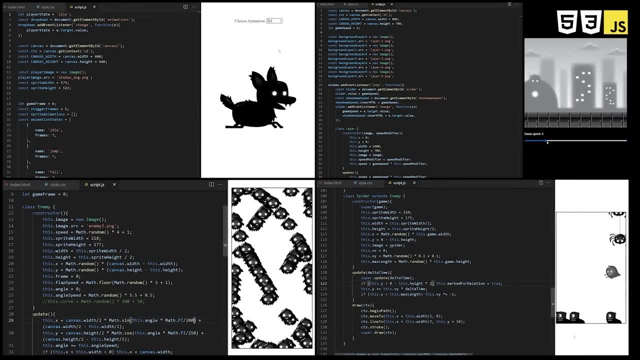 that make up our game, how to make them communicate with each other effectively and how to put all of that together in an easy-to-understand way. this class is a part of a longer series. in each episode we built a small standalone project for beginners to learn about. 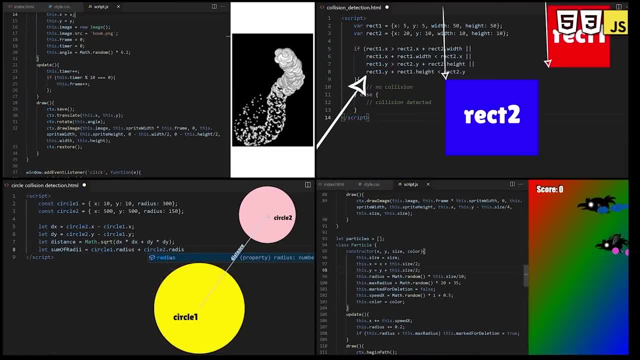 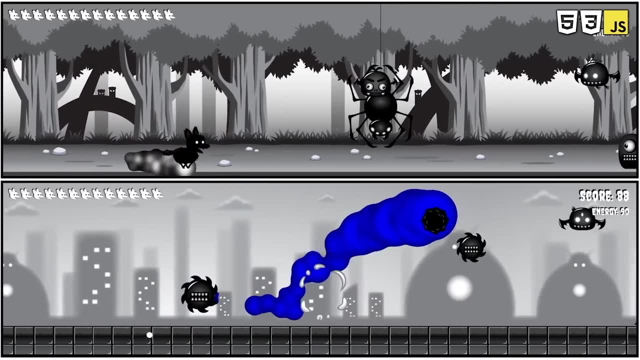 fundamental building blocks of game development with the JavaScript full series is linked in the description. in this part we will build a simple version of the game to learn the fundamentals. in the next part we will expand on each element using the things we learned across the series. let's see how it all. 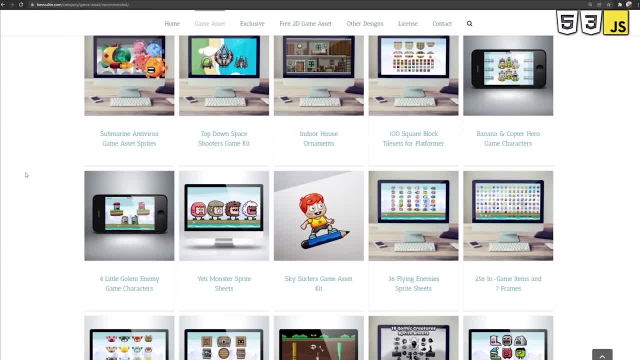 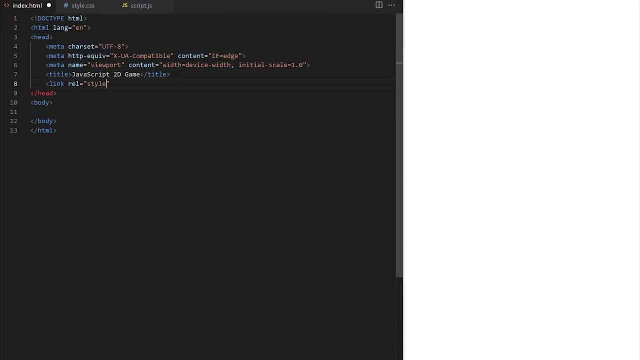 comes together, games should be exciting, full of secrets and special features. I hope this series helps you to bring your creative ideas to life. we will work with three files. in index HTML, I link my CSS style sheet and the JavaScript file I create HTML 5 canvas element with an ID. 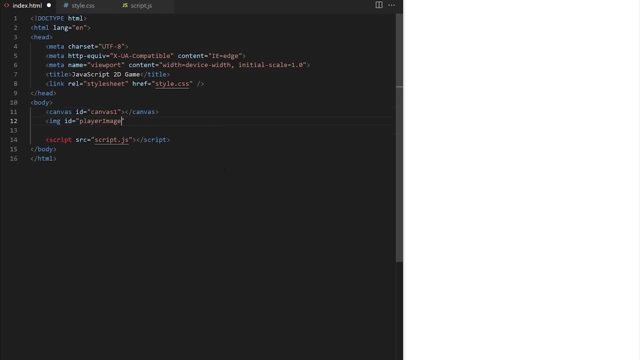 of canvas one and I put all my game assets here in this area so that we can use load event listener to wait for these assets to be fully loaded and available before we run the game. art assets were provided by this talented artist. you can find more on their. 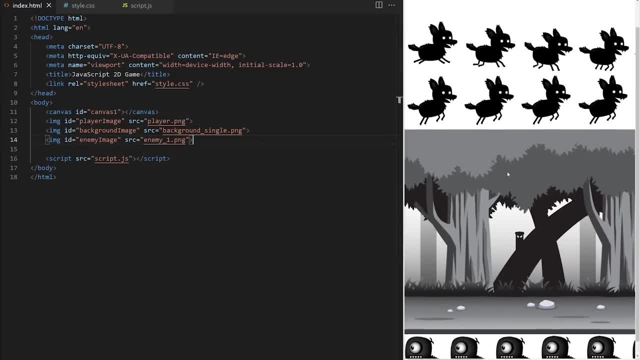 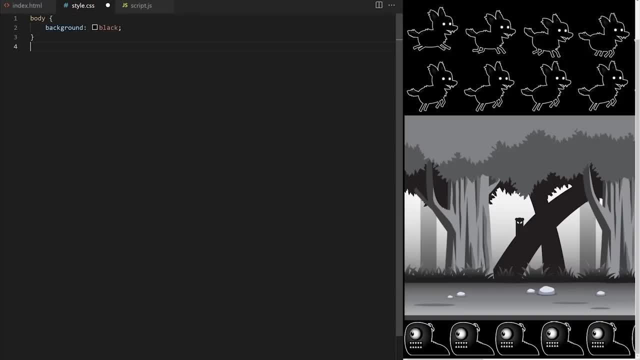 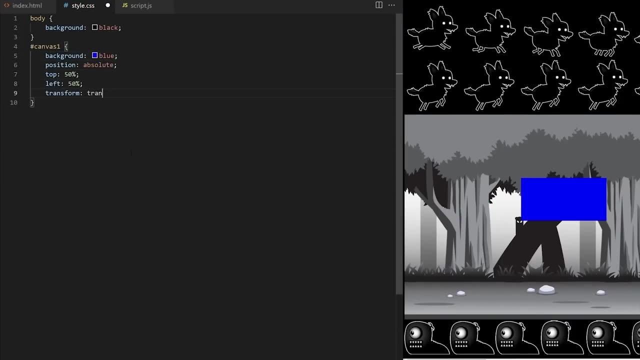 website. I will have player image, background image and enemy image. here you can download project files. in the video description install CSS. I give my body black background, I make canvas blue and I position it in the middle of my web page. I also want to hide my image elements. 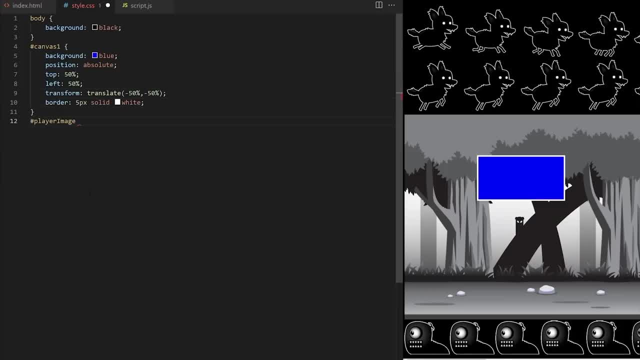 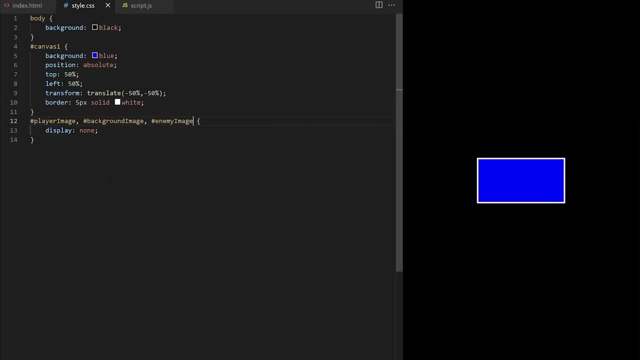 because we will draw them with JavaScript on canvas. so player image display. none same goes for background image and enemy image. I want the JavaScript to wait until all images are fully loaded, so I will wrap my game inside an event listener. we will listen for load event. load event waits for all. 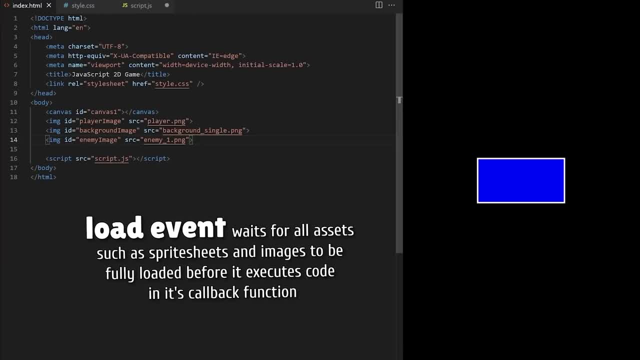 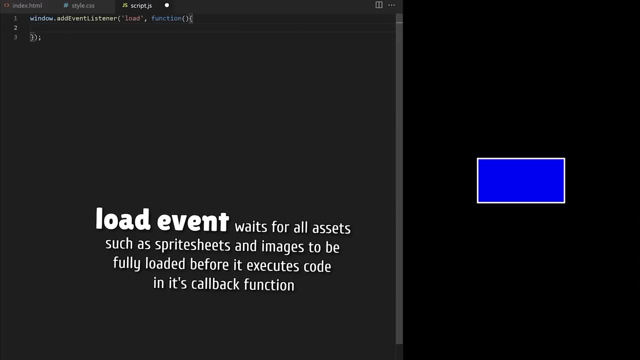 assets, such as sprite sheets and images, to be fully loaded before it executes code in its callback function. I will place the entire code of our game inside this anonymous callback function. in JavaScript, anonymous function usually means a function without a name. by placing all my code inside this anonymous 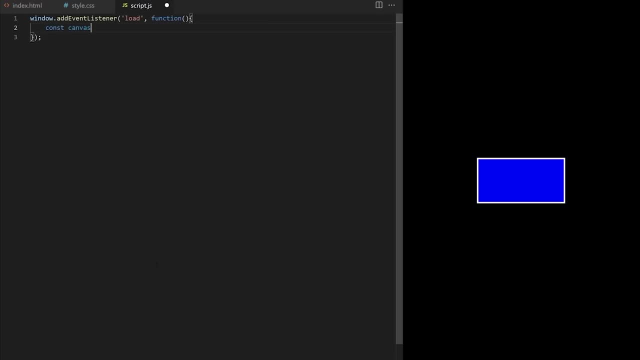 callback function. I separate scope of my game from a global scope to make sure my custom class and variable names don't clash with any other outside code. when all the assets are fully loaded, the code inside will be executed line by line. I assign variable to my canvas. 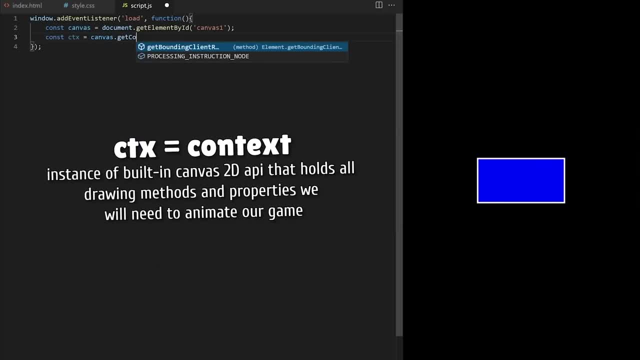 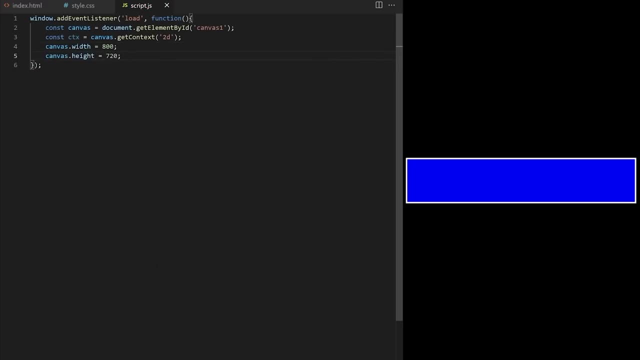 element. I create context instance of built-in canvas 2d API that holds all drawing methods and properties we will need to animate our game. I set canvas width to 800 pixels and canvas width to 720 pixels and canvas height to 720 pixels. I make canvas transparent in this. 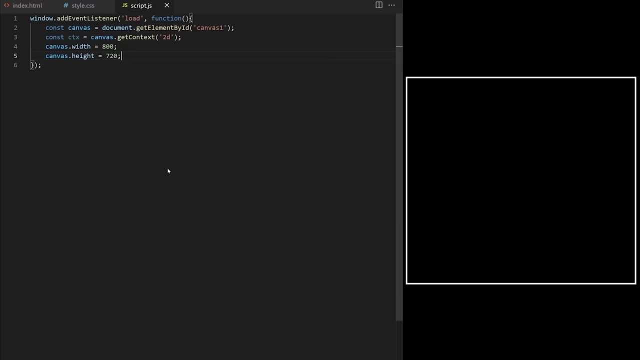 class. I want to make it very clear how we split responsibilities between objects and how these objects interact with each other to create a complete game. so let's just write all the building blocks we will need today. our game will need input handler class, which will apply event listeners to keyboard. 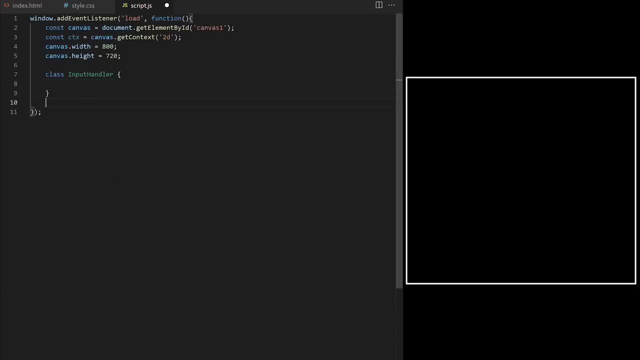 events and it will hold an array of all currently active keys. player class will react to these keys as they are being pressed, drawing and updating the player. I will have a simple, separate class that will handle endlessly scrolling backgrounds. we will also need a class that will generate enemies for us. we 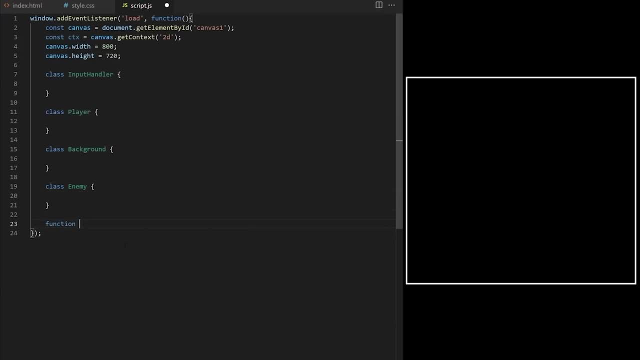 will have multiple active enemies in our game, so I will have a function called handle enemies that will be responsible for adding, animating and removing enemies from the game. I will have a utility function- I call, for example, display status text, which will handle things like displaying score or game. 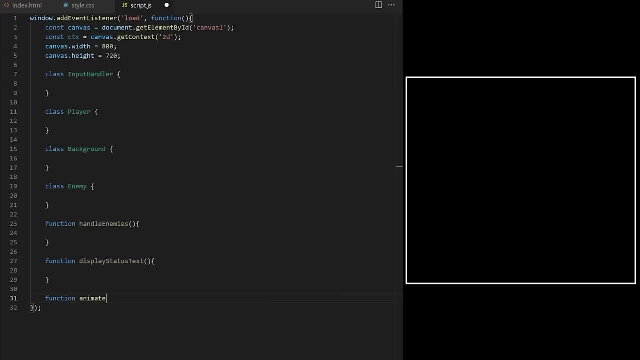 over message and, lastly, we will have main animation loop. this function will run 60 times per second, updating and drawing our game over and over. so that's it. here we can see all the building blocks we need to create a complete game. I could have wrapped everything in a. 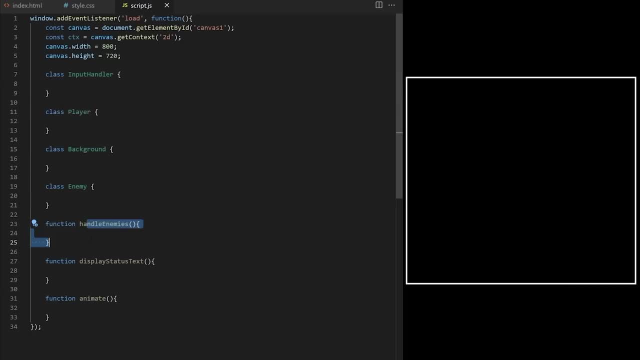 main game class, for example, but I'm trying to keep it clean and simple. today, input handler class will apply event listeners to the game and it will keep track of all keys that are currently pressed down inside constructor. I created this dot keys property and I set it equal to an empty array, the way I. 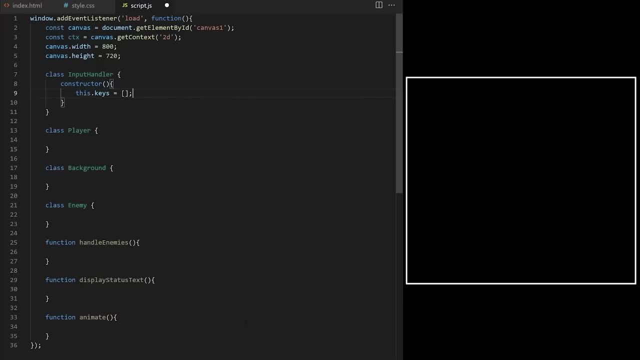 want to handle controls today will be a bit different from my previous courses. I want to have an array and I will be adding and removing keys from it as they are being pressed and released. that way I can keep track of multiple key presses. I will place event listener directly. 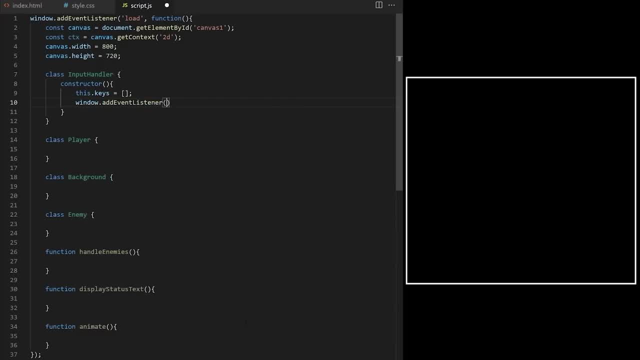 inside the constructor. when we create an instance of a class, all the components inside constructor is executed. because of that, just by simply creating an instance of input handler class later, all event listeners will be automatically applied. I will have event listener for key down event callback function on. event listener has access to. 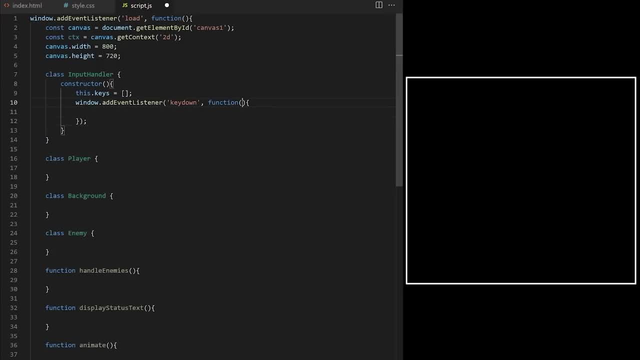 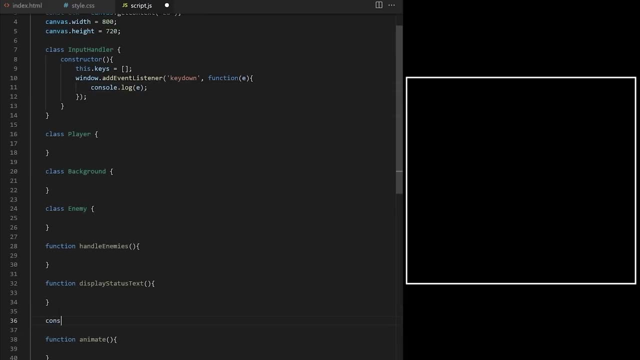 this built-in event object. I will assign it a variable name, for example e, and I console log it. now I create an instance of input handler class which will run all the code inside constructor. so at this point the event listener is applied. let's test it when I click my canvas and I press. 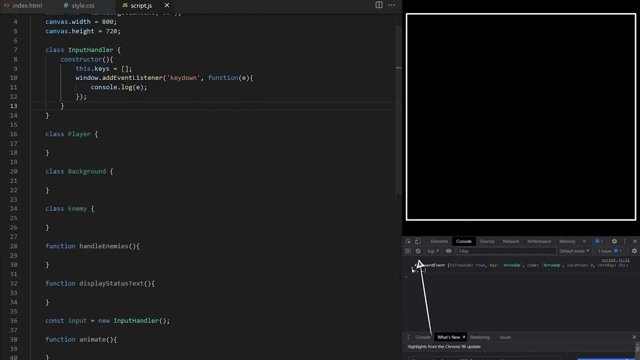 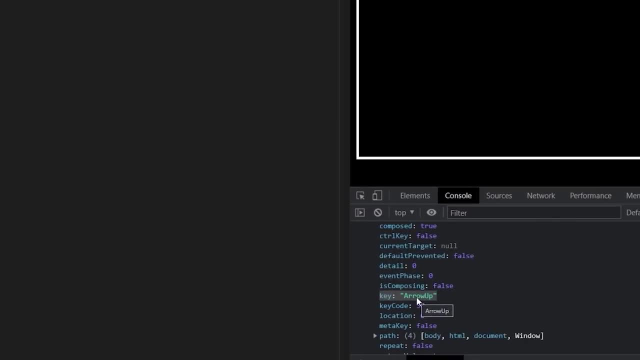 key on keyboard. I can see this event object here. it contains all different details about keyboard event that just occurred. what I care about today is this key property. it contains a string that represents name of key that was pressed so to get that value directly. I say e. 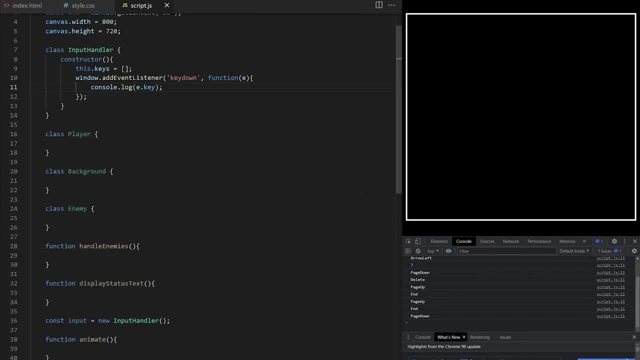 dot key. now I'm getting those values as console logs. I care only about arrow keys right now. so I say, if e dot key is arrow down, take this dot keys array from line 9 and push that value inside. I move this console log here and I will also. 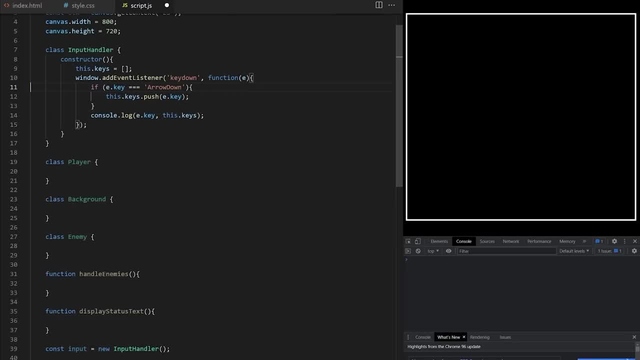 console log this dot keys, we will get an error. this dot keys is undefined. JavaScript cannot find it. it's because I'm instantiating input here and the event listener is called from window object. by the time that event listener is called, JavaScript forgot that this keyword refers to this input handler. 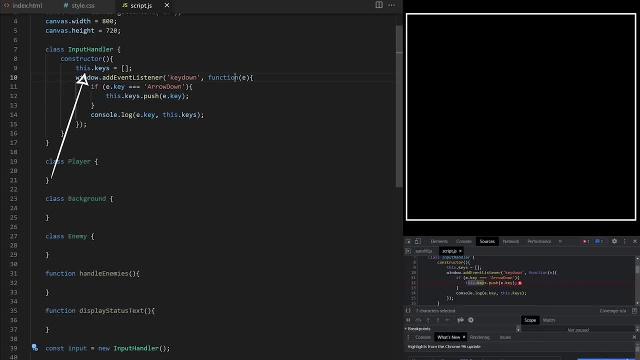 object and it's this dot keys property to make sure this keyword points to the correct object. I can use JavaScript bind method or I can use es6 arrow function. arrow functions don't bind their own this, but they inherited the one from their parent scope. this is: 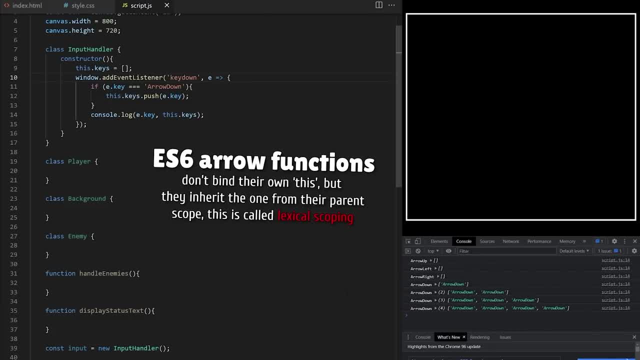 called lexical scoping. doing that will make sure JavaScript doesn't find this dot keys array in my control. so if I press this key, it will find this and will give me this dot key so I can then add it to my control and say that I'm going to call the key I want to do. 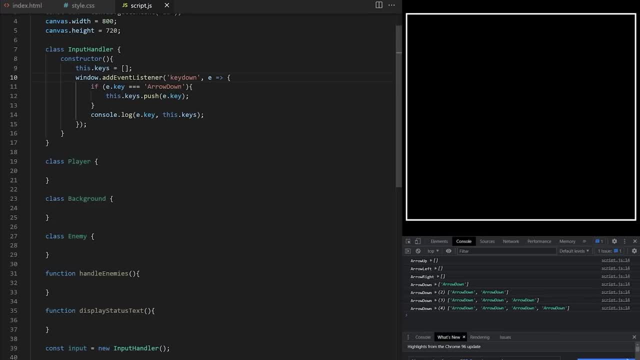 because I can't find out what that is actually is, but I can use it and I will just put it here in my control and possibly I'll just say that you can see that this dot key is information about a special location that I have here. so if I 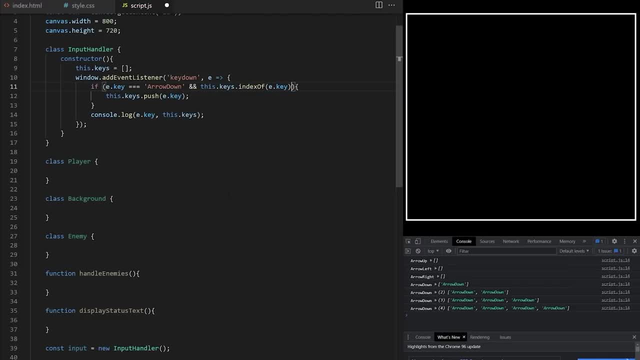 want this dot key to be my control location and I want to put the name of With arrays. if index of is equal to minus one, it means that element is not present in the array. So I'm saying if key that was pressed is arrow down and if that key is not yet inside this. 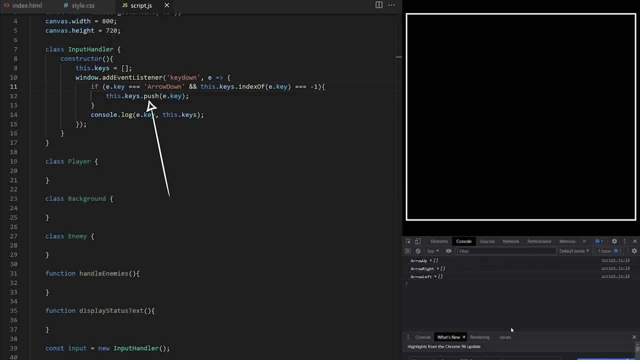 dot keys array only then push it into the array. Now you can see that when I press arrow down multiple times, it adds it to the array only once. Perfect, I copy this code block and I turn it into key up event. If key that was released is arrow down, I want to remove it from this dot keys array. 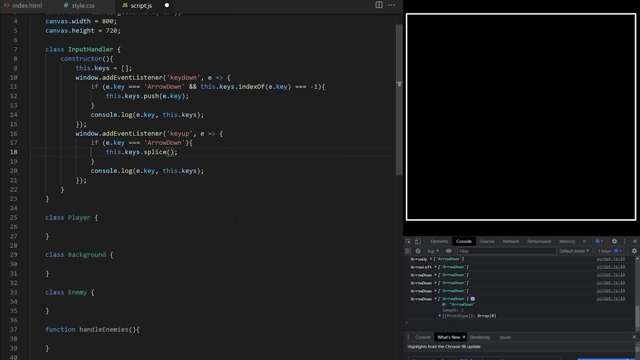 so I call splice. that takes two arguments: Index of element we want to remove and how many elements starting from that index we want to remove. So I find index of arrow down inside this dot keys array by using index of method again. And second argument to splice: I want to remove one element at this index. 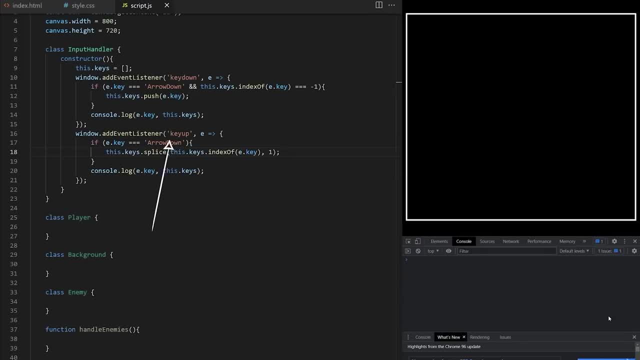 So here I'm saying: When we release this, If that key is arrow down, find index of that key inside this dot keys array and use splice to remove one element from that array. Now when I press down arrow key, it's added to the array. 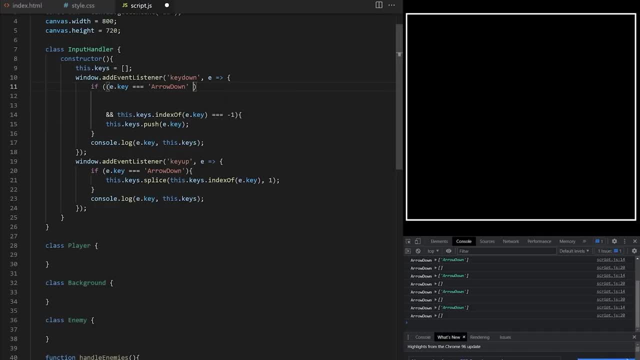 When I release it, it's removed from the array. Nice, Let's also listen for other keys using OR operator. I start with arrow up, Then we also need to listen for key down on arrow left And arrow right. I'm gonna break this down on individual lines for clarity, and I use tab key to make them. 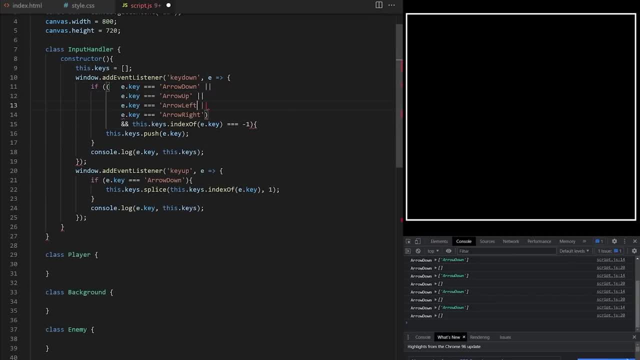 vertically aligned. Be careful here not to forget a bracket, otherwise the code will break. I will also listen for the same four keys inside key up event. So we have this dot keys array here In key down, if arrow down, up, left or right is pressed and that key is not yet present. 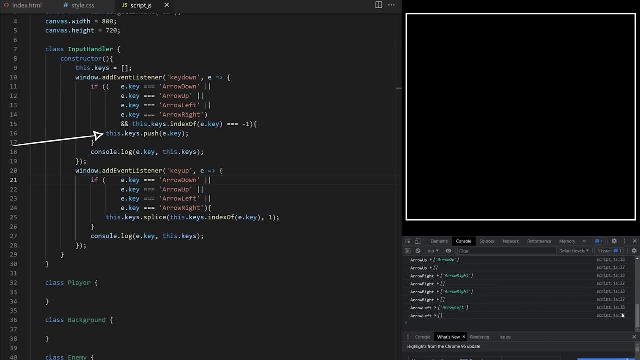 in this dot keys array. we push it into the array In key up. when any of these four arrows are released, we find index of that key inside this dot keys array and we use splice method to remove it. This dot keys array now holds information about which arrow keys are currently pressed. 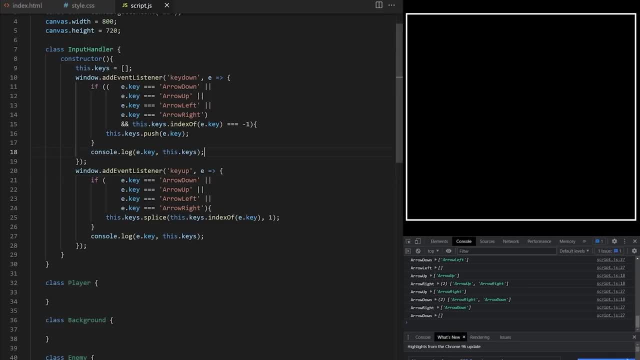 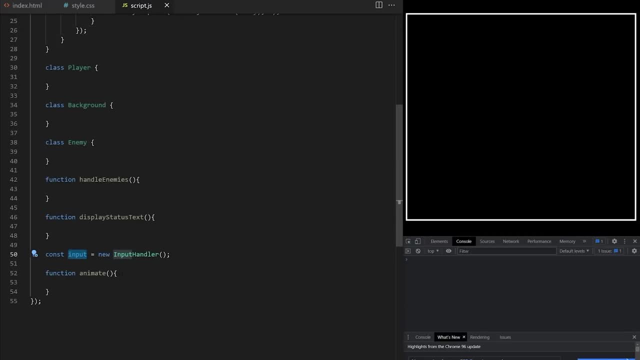 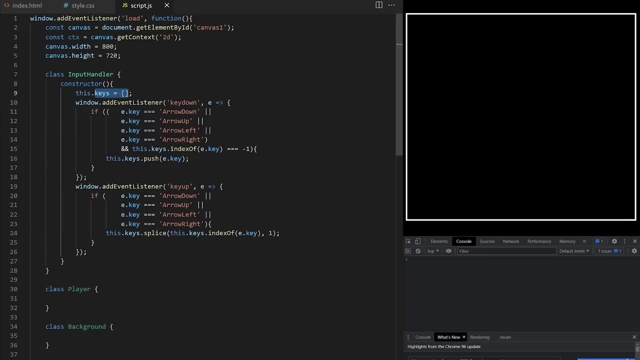 down. Sometimes it could be multiple ones at the same time I remove these console logs By instantiating input handler class here on line 50,. all the code inside constructor on line 8 will be executed, And that's it. We have this dot keys property as an empty array and we use key down and key up event. 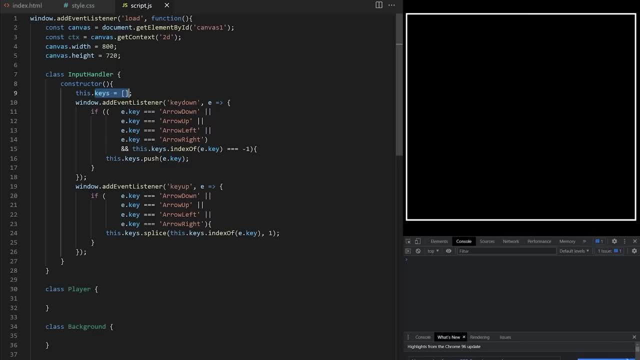 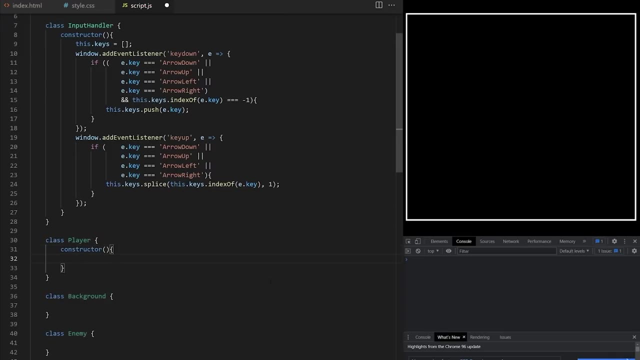 listeners to add and remove specific keyboard inputs from that array. And now we know how to handle keyboard inputs in a game. We will use them to move player around. in the next part, Player class will define properties of player object. It will draw it, animate it and update its position based on user input. 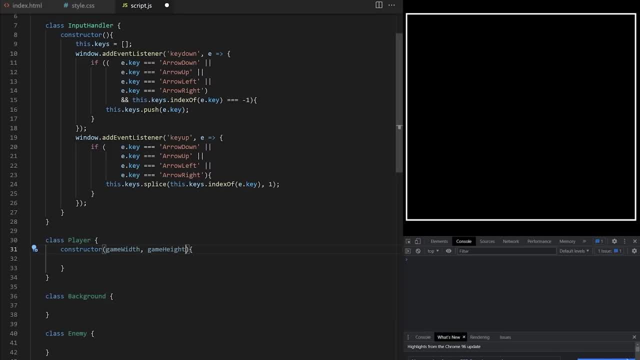 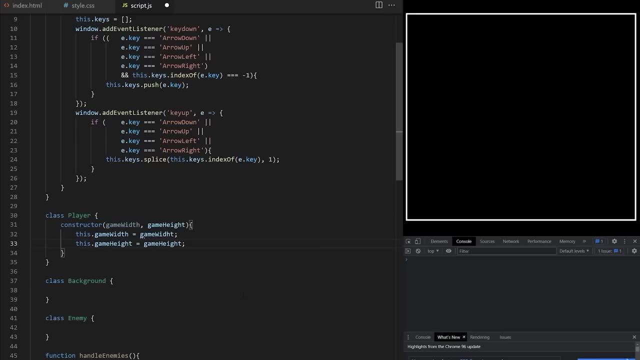 Player object needs to be aware of game boundaries. We don't want it to run off screen, so I pass it game width and game height as arguments and I convert them into class properties like this: I'm using spreadsheet of specific size. Here we have frames of width and height of 200 pixels. 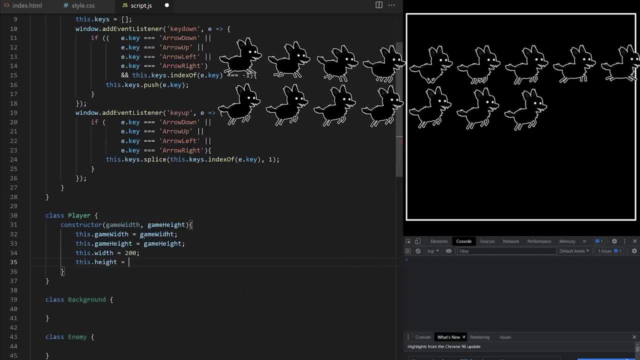 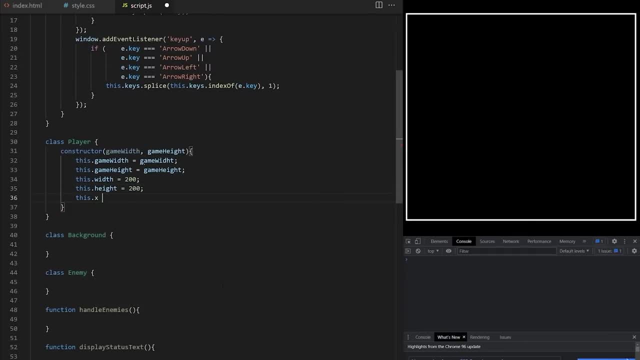 It's a good practice to size your spreadsheets to the actual size you will use in your game. I can also resize them with code, but it's cleaner to have art assets of the right size. This dot x will be zero And this dot y will be zero. 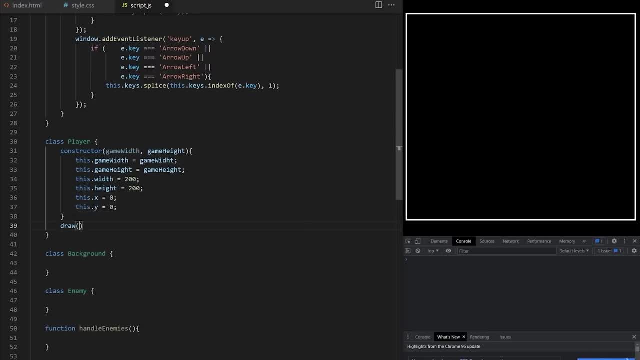 Player object will have public draw method. It will expect context as an argument to specify which canvas we want to draw on. in case we want multiple layers and multiple canvases in our game, I will start by calling built in fill rectangle method to draw a rectangle to represent our 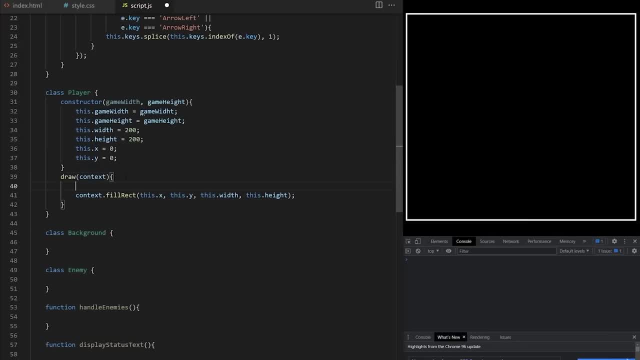 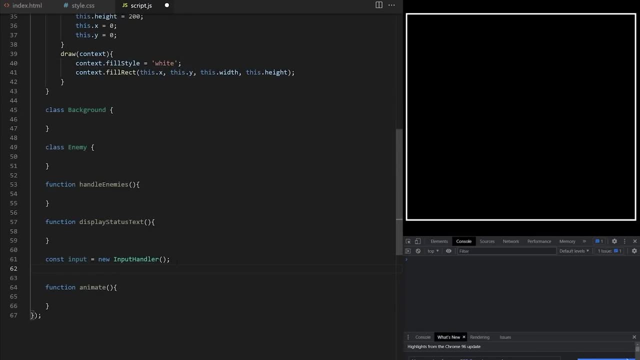 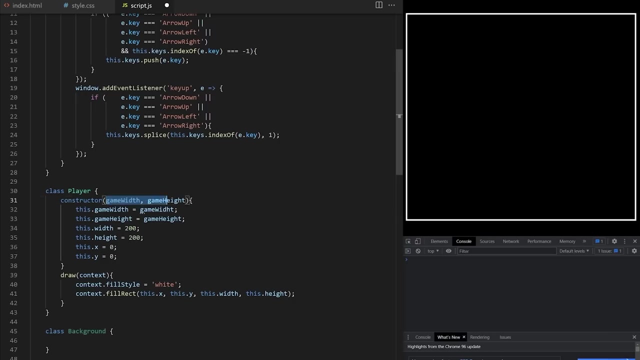 player. I pass it x, y, width and height. Since I have black background, I set fill style to white so that we can see the rectangle. On line 62 I create an instance of player class using the new keyword Here. on line 31 I can see player class. constructor expects game width and game height as arguments. 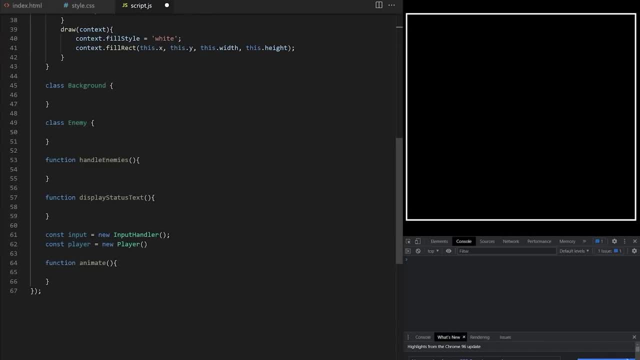 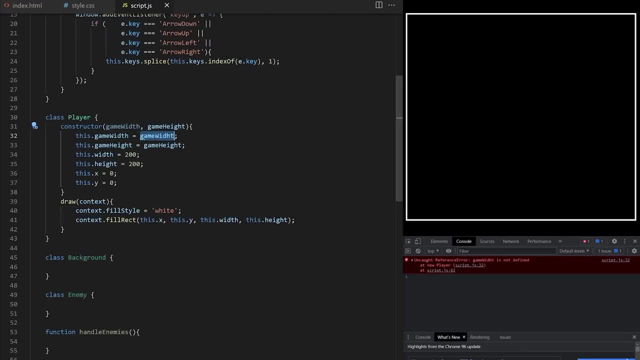 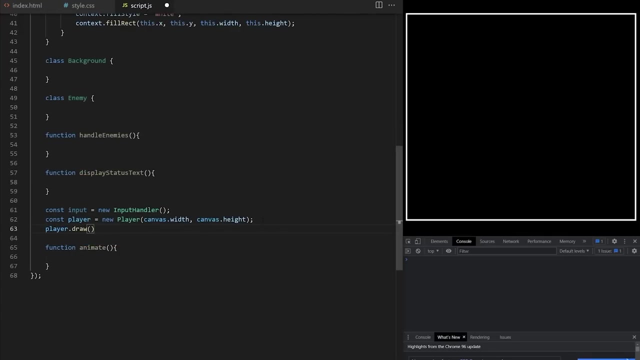 so I pass it: canvas width from line 4 and canvas height from line 5.. I get an error. Game width is not defined. It's because I made a typo here on line 32.. Now it works and I can display our player by calling its public draw method. we just wrote. 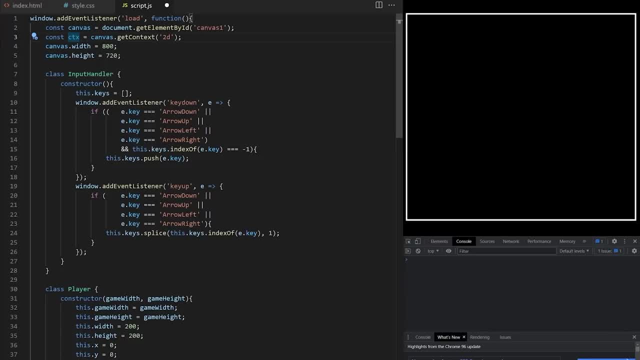 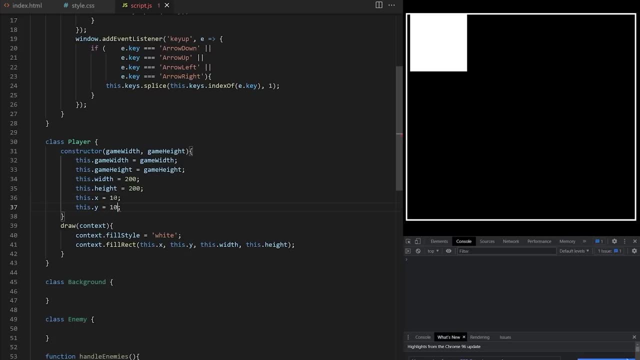 It expects context as an argument, so I pass it. ctx from line 3.. I can move player around by adjusting its x and y coordinates. Let's make it stand on the bottom of game area. so this dot game height minus this dot height. We will also need update method to move player around. 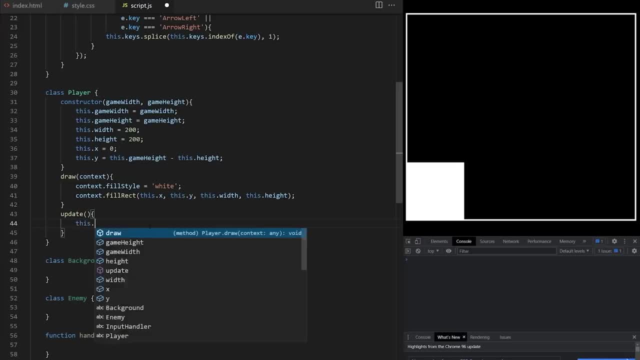 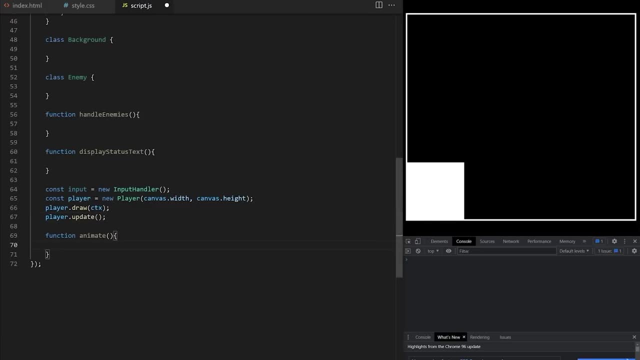 Let's start by increasing player's horizontal x coordinate by 1 for every call of update method. If I call update method just like this, There won't be any visible movement. I put it inside animation loop and I use request animation frame built in method to make it. 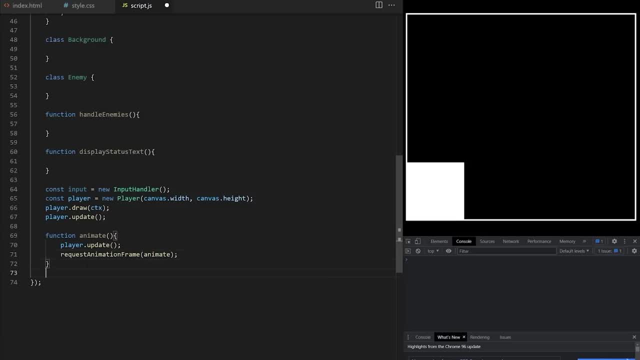 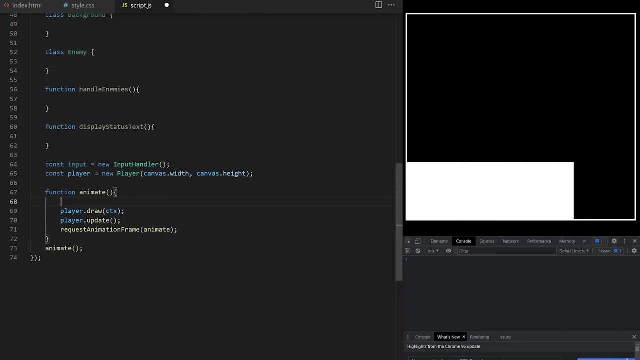 loop. I pass it animate the name of its parent function to create endless animation loop and I call animate like this to start it. I also need to put draw inside. I delete this. We can see trail behind player rectangle. I want to only see the current animation frame. 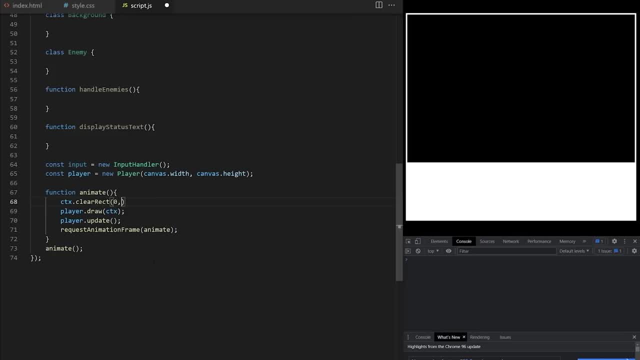 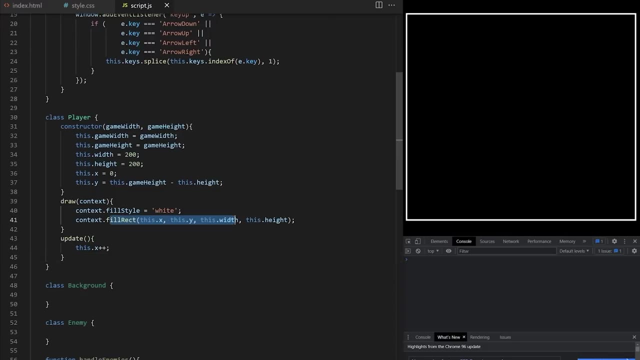 To delete old paint from canvas I use built in clear rectangle method. It will delete entire canvas between each animation loop. Perfect, Now we have player moving from left to right, as we defined in its update method. Instead of drawing a white rectangle, let's draw player image. 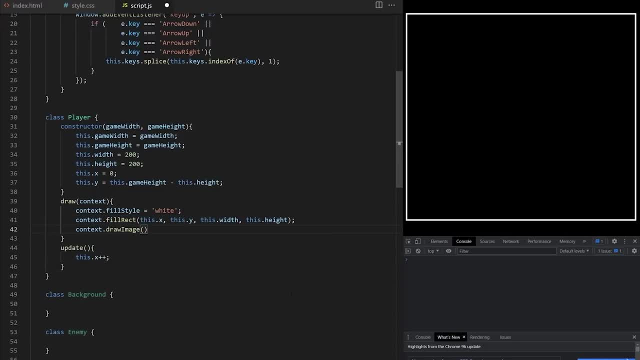 I call built in draw image method. I need to bring player sprite sheet into the project, so this dot image property is document dot get element by id and I give it id of player image. I pass this dot image from line 3.. I pass it x and y of 0,0. so top left corner of canvas. 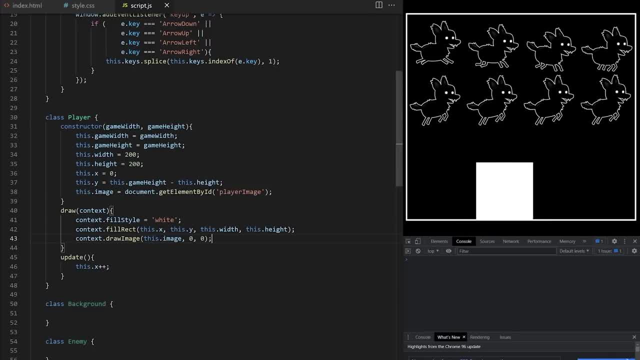 It will just draw the entire sprite sheet at these coordinates. I pass it this dot x and this dot y. instead You can see it just draws the entire large sprite sheet with all the frames. Draw image method can accept optional 4th and 5th arguments for width and height. 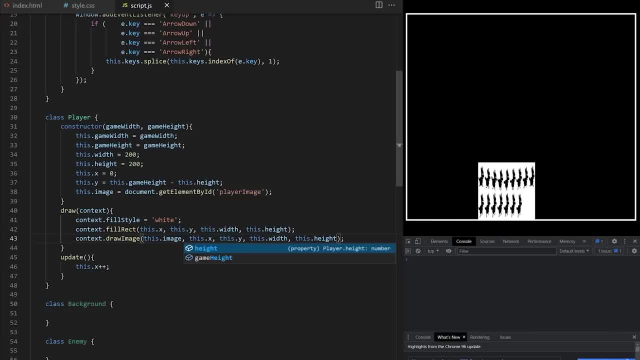 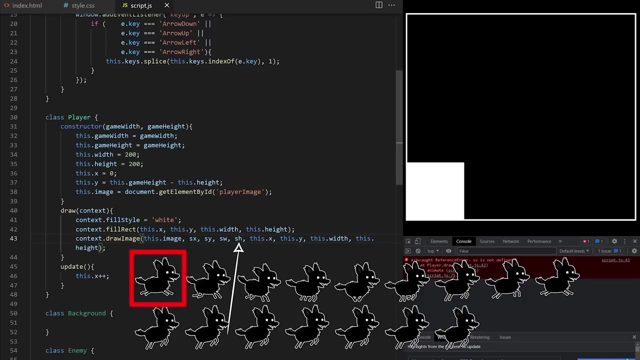 It will then stretch or shrink the image to fill all available area Like this. I actually just want to draw one frame, So I pass it another 4 optional arguments: Source x, source y, source width and source height. These define rectangle we want to crop out from the source sprite sheet. 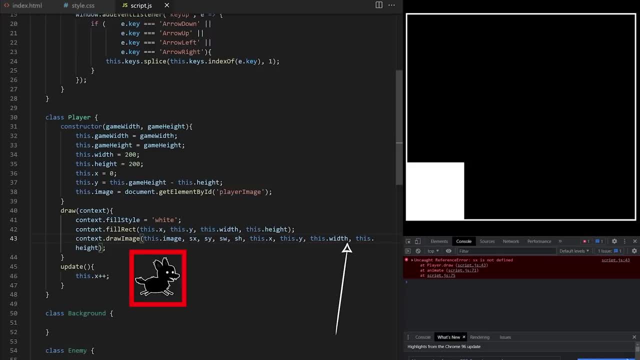 And destination x, destination y, destination width and destination height define where on destination canvas we want to place that cropped out rectangle onto. I pass it 0,0 as source x, source y and we are cropping to this dot width, this dot height. 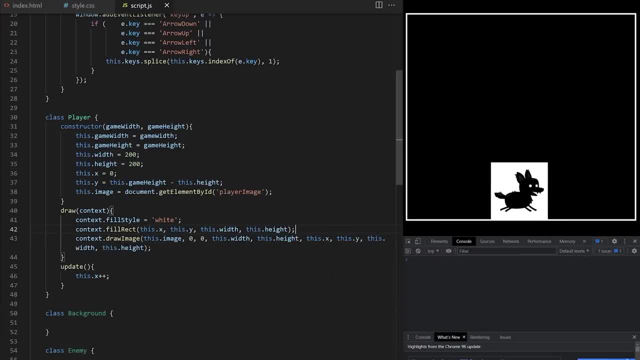 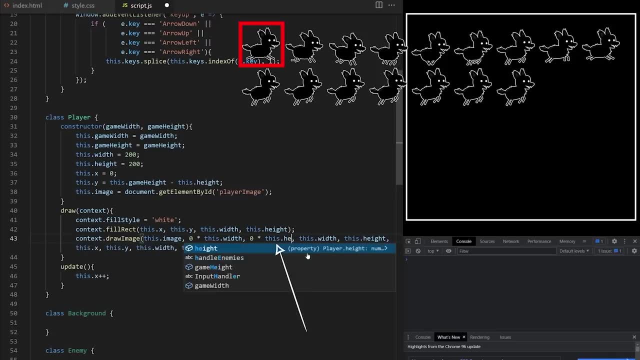 So this area. Now we can see top left frame in the sprite sheet. I can use source x and source y to jump around the sprite sheet. By changing value of source y, we can jump between different rows. By changing the value we pass as source x, we are navigating within the sprite sheet. 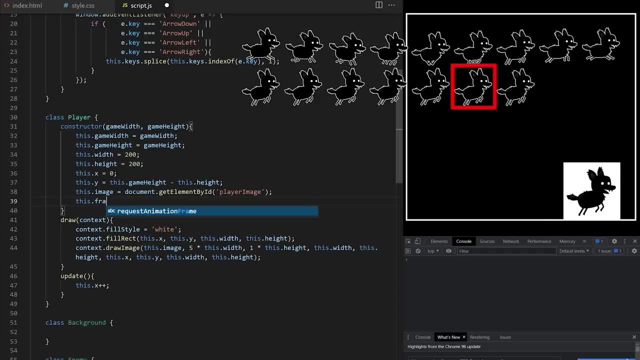 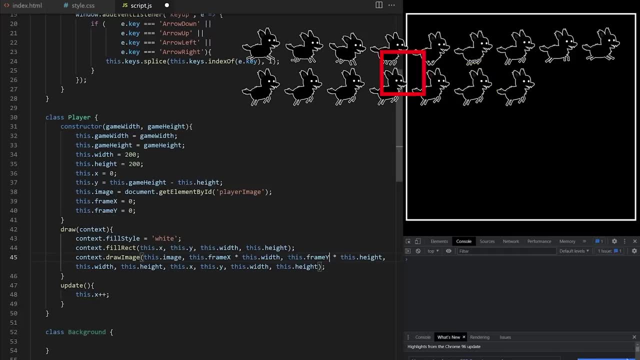 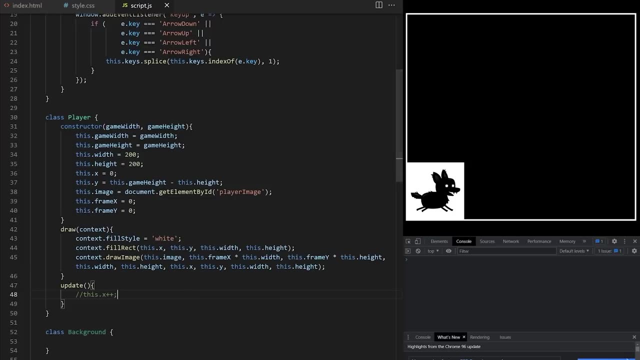 horizontally. Let's just turn these values into class properties, called, for example, frame x and frame y. I replace them here, And now we can navigate around sprite sheet. Now we can see that we can add this dot speed to this dot x at all times when it's 0 there. 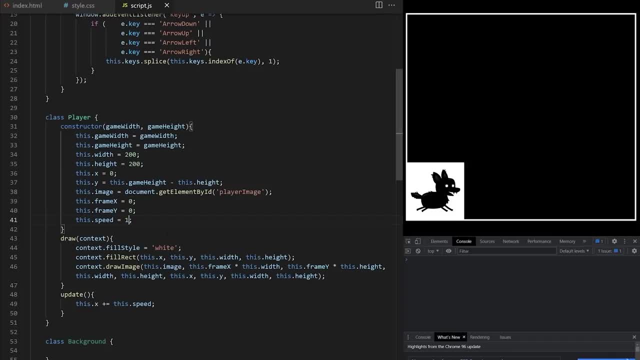 will be no movement. When this dot speed is a positive number, player will move to the right. When it's a negative number, player will move to the left on the negative direction on horizontal x axis. Now we can connect keyboard inputs to player movement. 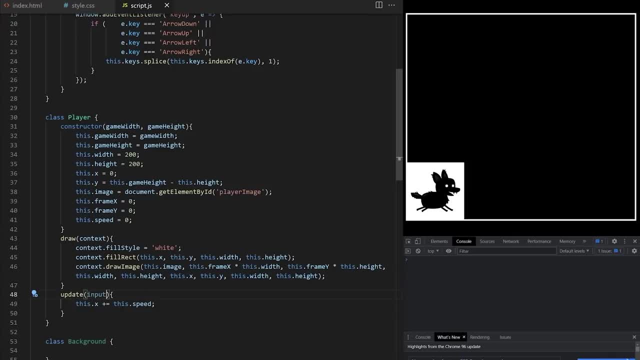 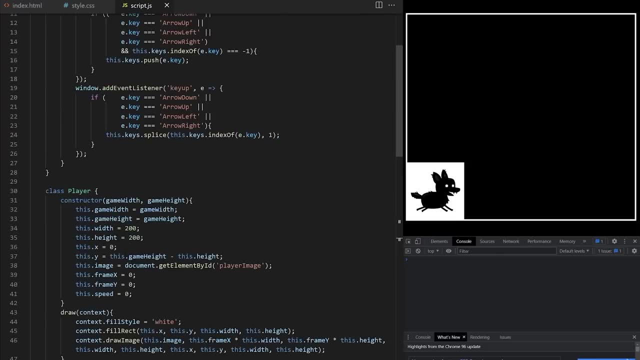 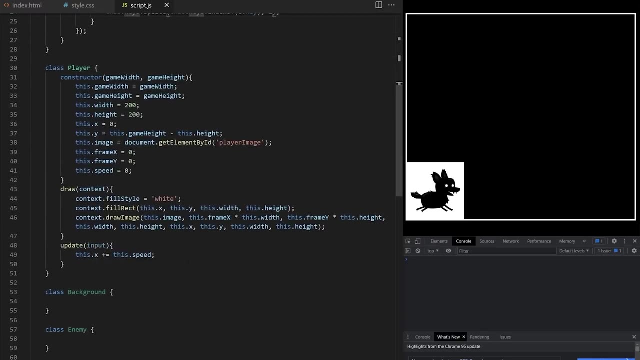 Update method will expect input as an argument. I take input from line 69 and I pass it to player update method here. We are interested in this dot keys property from line 9 which holds all currently active keys. We can access that property from input argument we are receiving here. 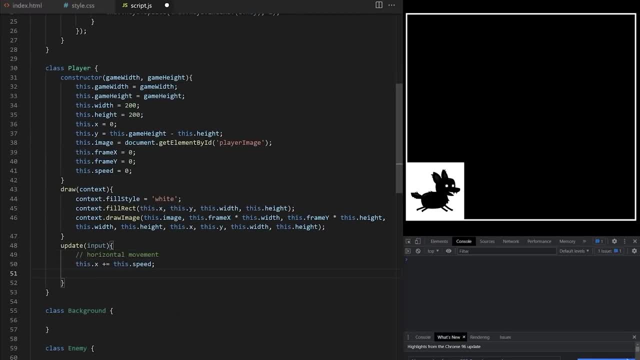 So this section will deal with horizontal movement If input dot keys contains arrow up. so if index of arrow up is more than minus one, we can run the following code: Actually, let's start with arrow right and set this dot speed from line 41 to 5.. 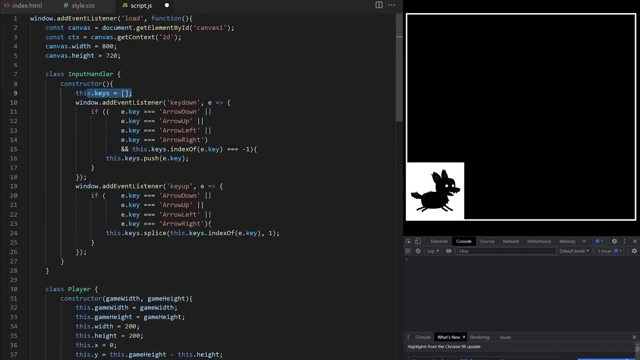 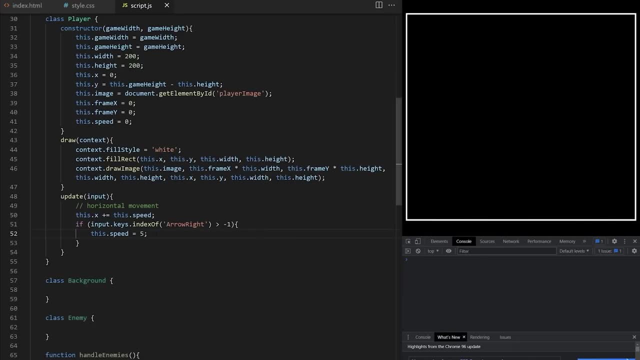 When arrow right is found in this array from line 9, set player speed to 5.. It will make player to move to the right, But there is nothing to set speed back to 0, so it never stops moving. I create an else statement here and inside I set player speed back to 0.. 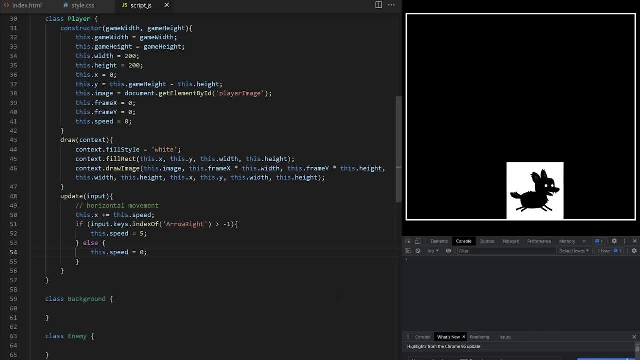 Now player moves to the right only when I hold down right arrow key. Nice, I do else. if statement here: Be careful about the brackets. It's easy to get it wrong and get an error here. Else, if arrow left is pressed, set player speed to minus 5.. 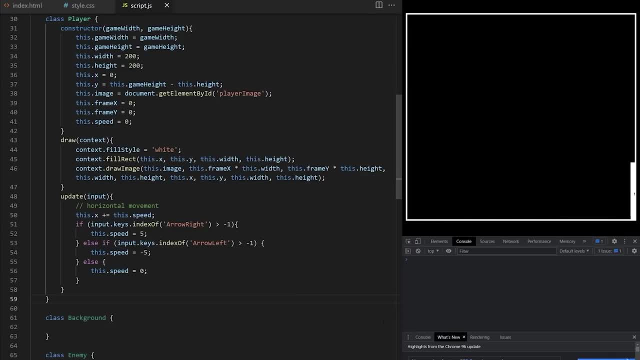 Now I can move player left and right. Player can easily move off screen if we hold the arrow for too long. Let's introduce some horizontal boundaries. If horizontal x coordinate is less than 0, set it back to 0.. Now we can't move past the left edge of game area. 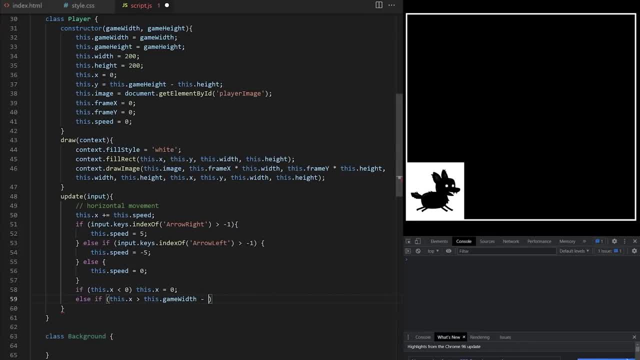 Else if Player's horizontal coordinate is more than game width minus player's width, meaning right edge of player rectangle is touching the right edge of canvas area. also, don't allow it to move past this point. Perfect Jumping is a bit more complicated but it's not that hard. 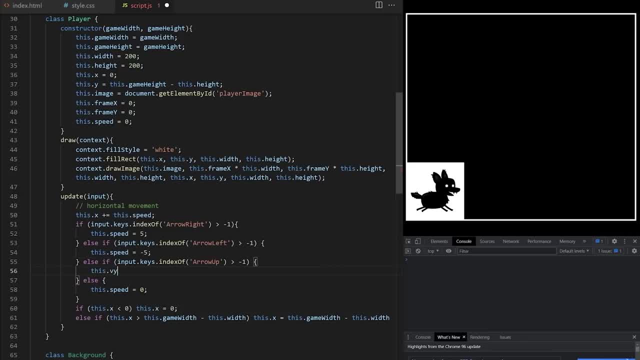 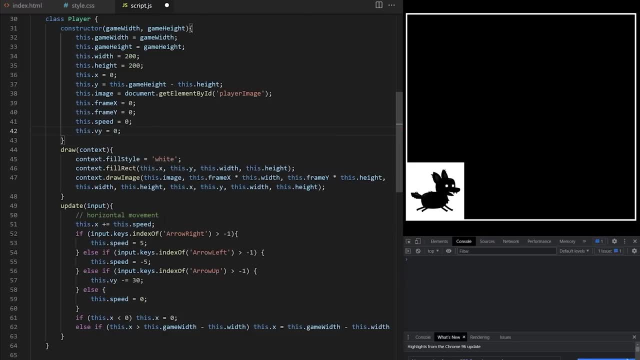 I say, if arrow up key was pressed, set velocityY property to minus 30.. I set velocityY property on player object and initially I set it to 0.. Let's just move this around. Let's just move this around. I have controls in one place- horizontal movement separate- and I create a section for. 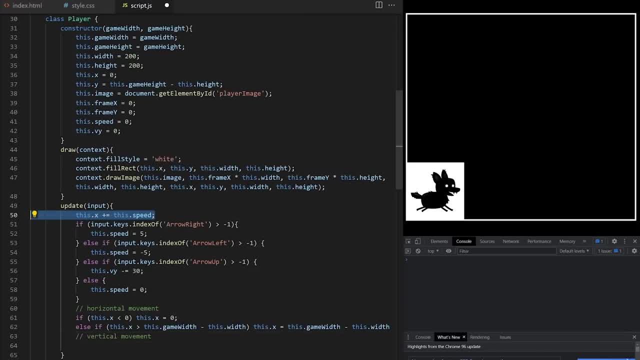 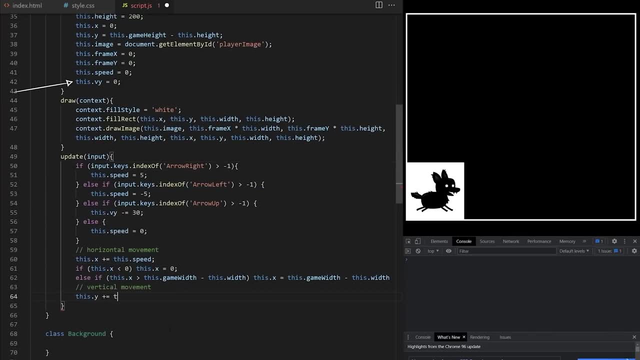 vertical movement. Actually, this line also belongs under horizontal movement. At all times. I will be adding velocityY property from line 42 to player's vertical coordinate from line 37. Initially velocityY is set to 0, so we will get no vertical movement. 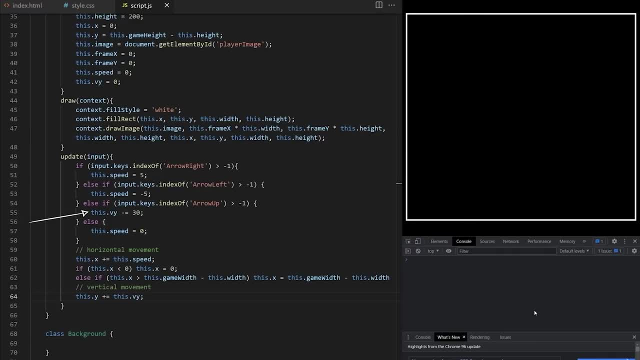 When I press up arrow key, velocityY is set to minus 30 and player just flies off screen. I need a force that will push in the opposite direction. I can call it gravity or maybe weight. I set it to 0 at first. 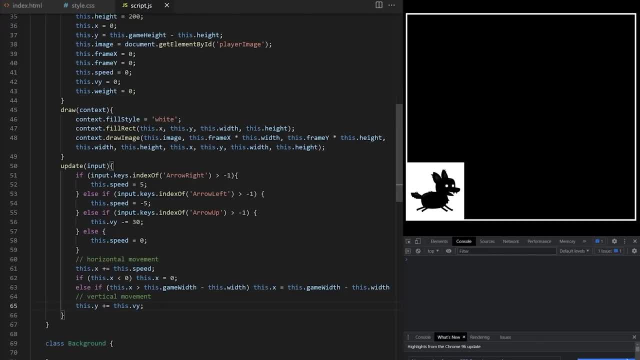 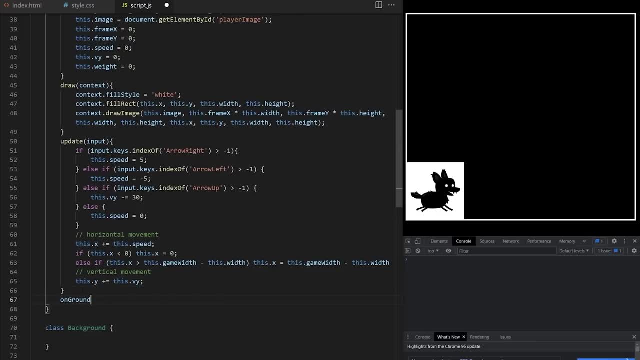 I need a check to see if player is in the air or standing on ground. I will need that check in multiple places, so I might as well make it into a utility method like this. I call it, for example, onGround, and it will return true or false based on how this statement. 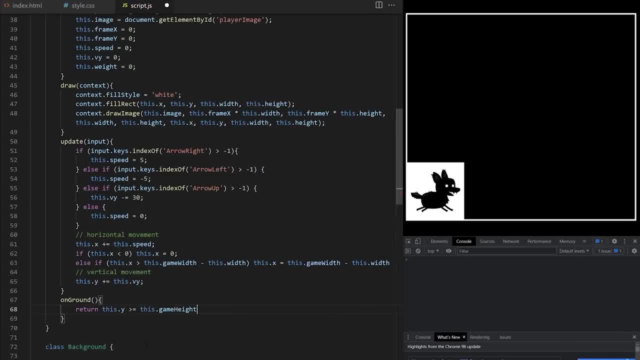 evaluates If thisy is more or equal to gameHeight minus playerHeight. We know player is standing on solid ground. Here in vertical movement section I say if onGround is false, meaning if player is currently in the air, take velocityY and start gradually increasing it by thisweight. from line 43.. 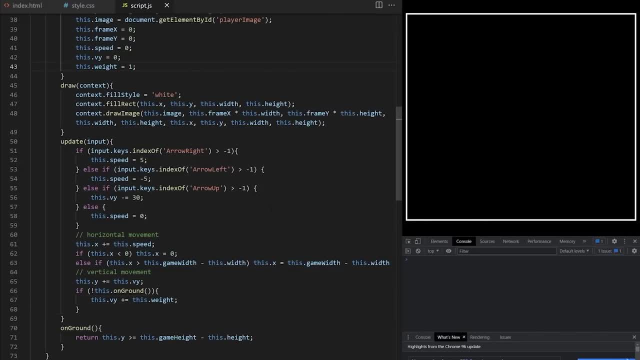 I set thisweight to 1.. We jump and eventually player falls back down. Size of the jump depends on how long you hold up arrow key. We don't want it to work like that. Let's fix it When we press up arrow key. 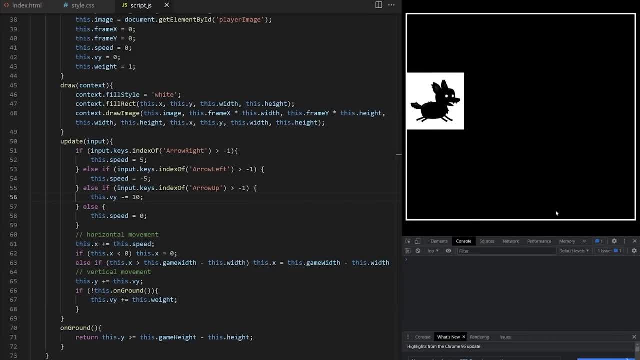 I set velocityY to minus 10 so we can see it better. I create an else statement here and inside we set velocityY back to 0. So if player is in the air, gradually add more and more weight to velocityY. Else, if player is back on ground, reset velocityY back to 0 to stop vertical movement. 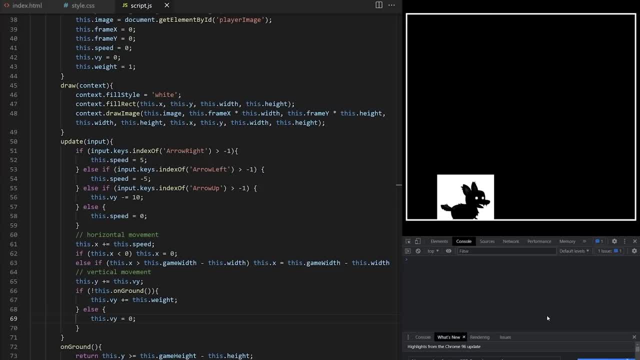 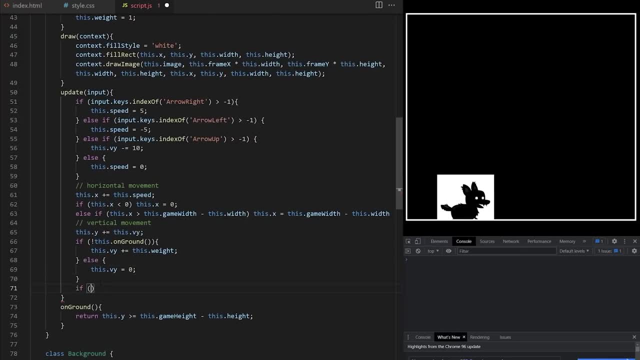 If I jump too high, player partially falls through the floor before velocityY is reset back to 0.. To prevent this from happening, let's introduce a vertical boundary On the ground level. If player's Y coordinate is more than game height minus player's height, I set it to. 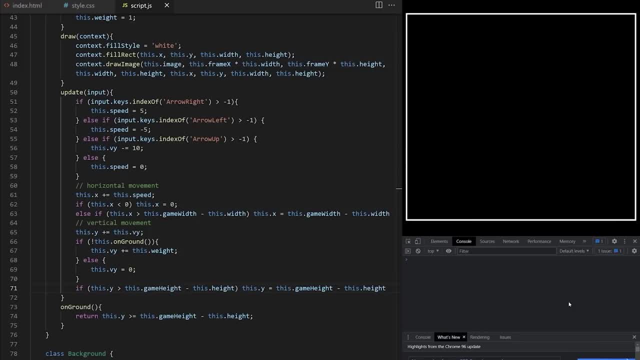 game height minus player's height. Player can never be below this point. That works. The height of jump is still dependent on how long I hold up arrow key, because each tick adds another minus 10 to velocityY. Also, if I press up arrow over and over, player will keep jumping higher and higher. 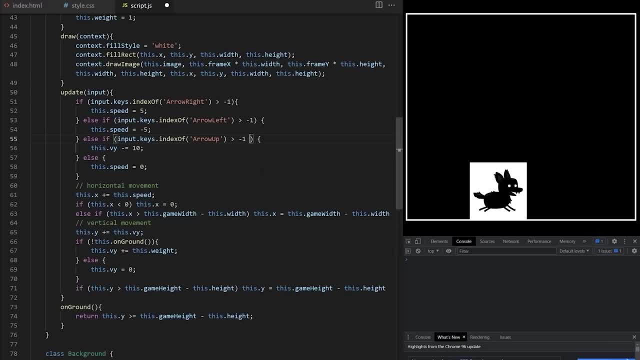 We only want player to be able to jump when it's standing, When it's standing on solid ground. Here on line 55, I say if up arrow is pressed and if player is on ground, only then decrease velocityY by minus 10.. 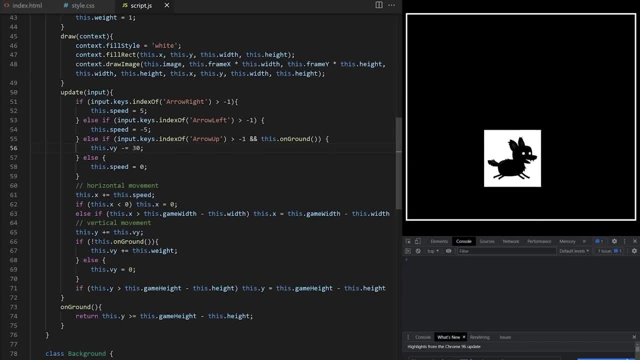 Now we can't double jump anymore. Let's do minus 30. for a bigger jump, Maybe minus 32.. So jumping works like this: VelocityY is 0.. When we press up arrow key, velocity is immediately set to minus 32.. 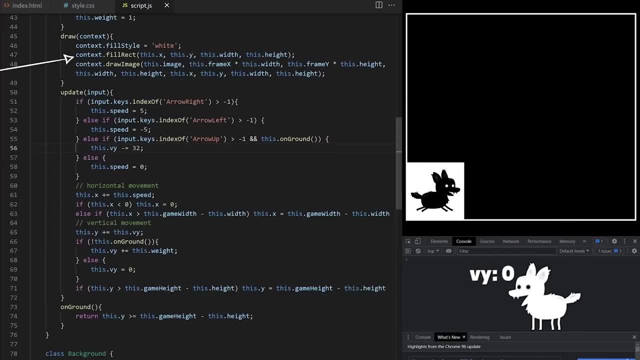 This statement on line 66 becomes true and weight of 1 is being added over and over to velocityY. That will make velocityY go from minus 32 to 0 and then back to positive numbers. so player will go up. it will gradually slow down, stop and it will start falling back. 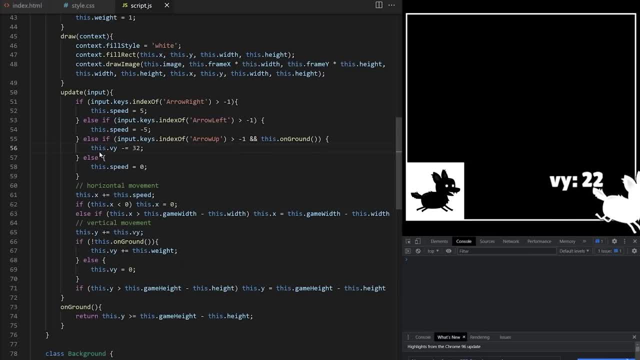 down again, as the value of velocityY goes from negative into positive numbers. When we hit the floor again, line 69 will set velocity back to 0 and jump is complete. When we jump, we want to animate a different row of sprite sheet. 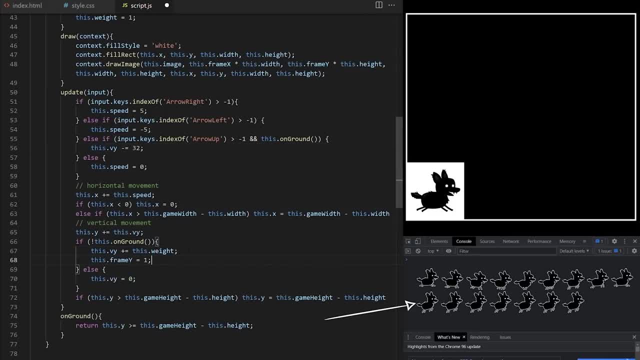 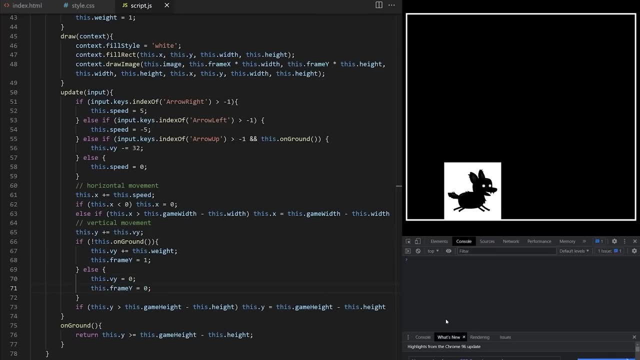 I want this jumping animation, so I set thisframeY to 1.. When we land back on ground, I set frameY to 0.. Endlessly scrolling backgrounds are very easy to implement. I made a special episode about different techniques I like to use and how to split it into individual. 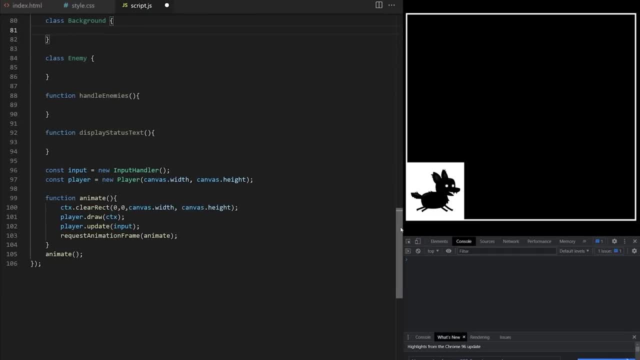 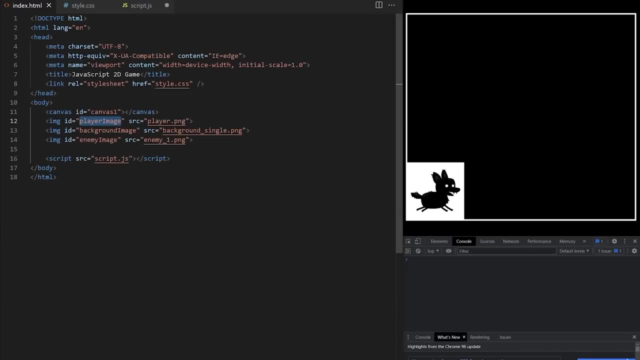 layers for parallax effect. Today we will just do a single endlessly scrolling layer. Let's go. Constructor will expect gameWidth and gameHeight and I convert these arguments into class properties. Thisimage will be my background image. I give it an id of backgroundImage spelled like this: 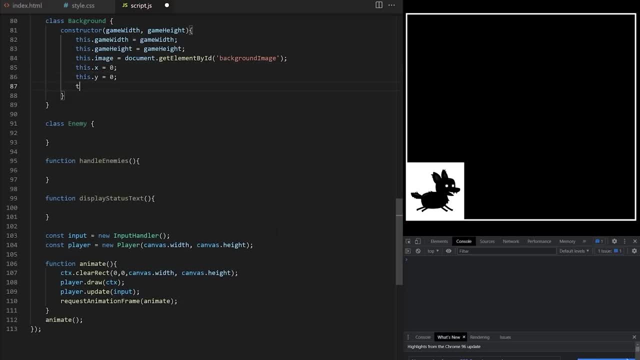 Thisx will be 0.. Thisy will be 0.. I check my image and I can see its width is 2400 pixels. Height is 720 pixels. Draw method will take context as an argument To specify which canvas we want to draw on. 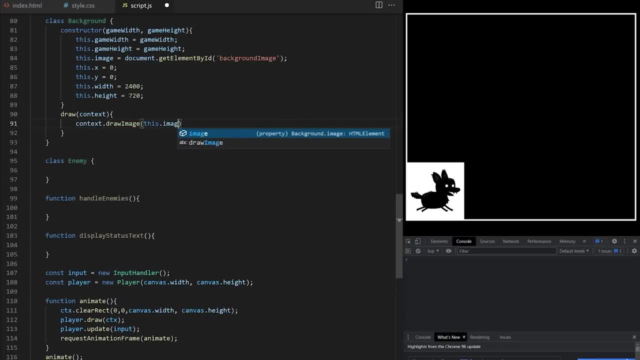 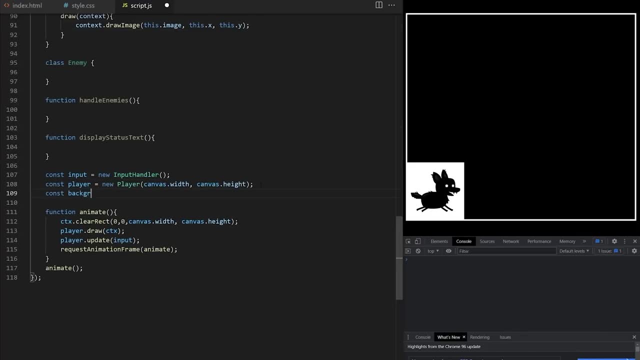 I call builtInDrawImage method and I want to draw thisimage from line 84.. I pass it x and y. On line 109, I instantiate my background class by calling the new keyword. I pass it gameDimensions, so canvasWidth and canvasHeight. 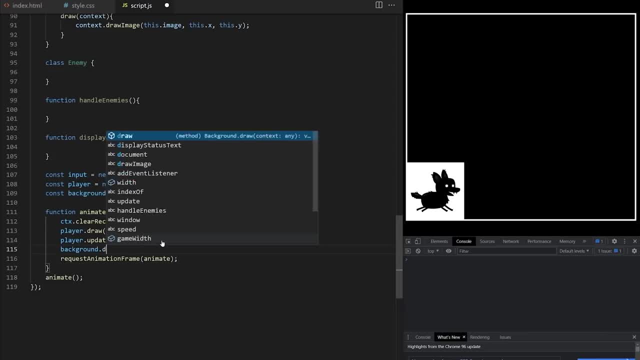 Inside animation loop. I call backgrounddraw. Draw method from line 90 and I pass it ctx as an argument. Draw method from line 90 and I pass it ctx as an argument. Draw method from line 90 and I pass it ctx as an argument. 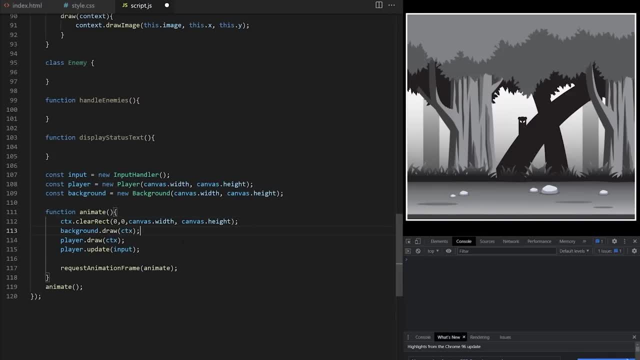 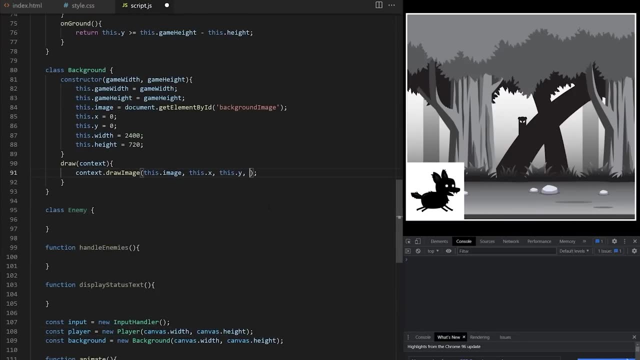 I have everything on a single canvas element, so I need to draw background first before I draw the player, so that the player is visible. Now I want to make the background animate to the left First. I pass it width and height here, even though I didn't have to do it since my art. 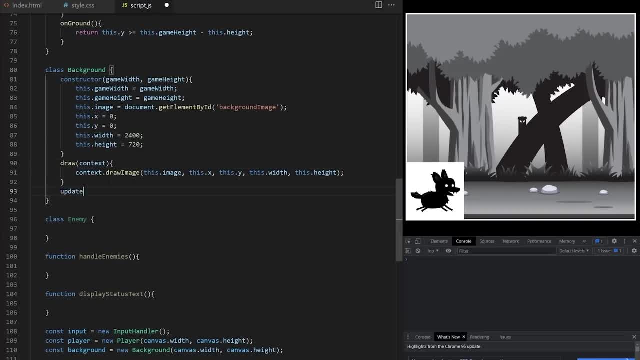 assets are already correct final sizes. There is no need for resizing them with code Custom update method. I create a property I call speed and I set it to 20.. Horizontal coordinate of the background will be minus equals 20 pixels. I create a property I call speed and I set it to 20.. 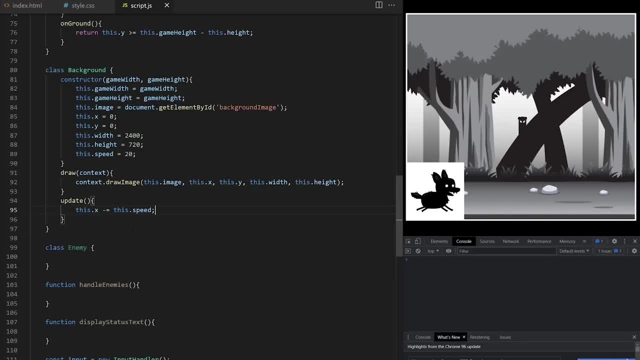 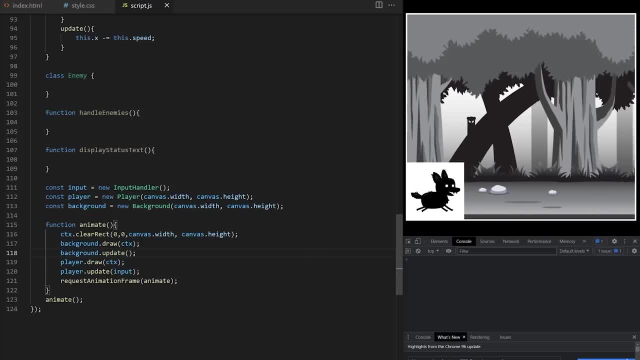 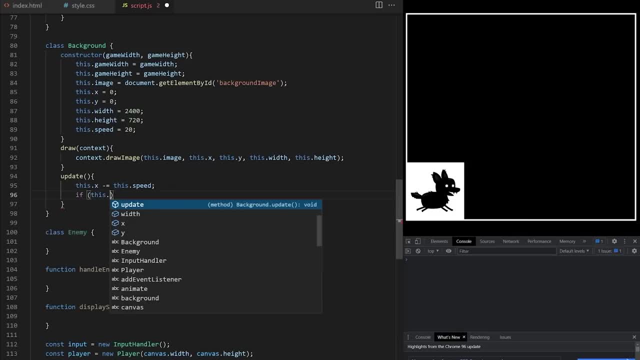 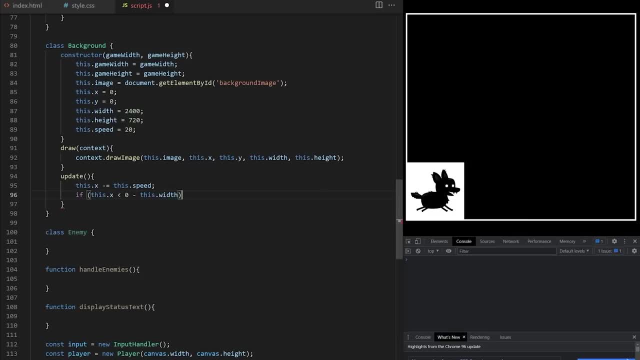 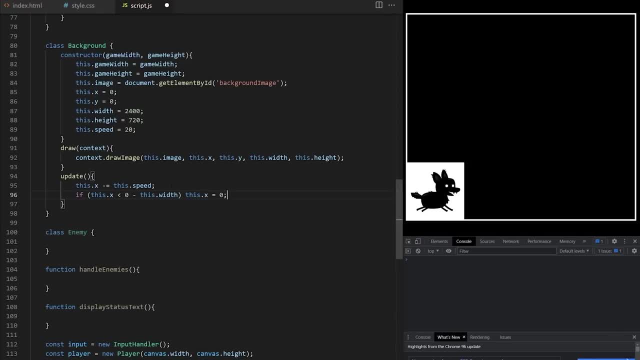 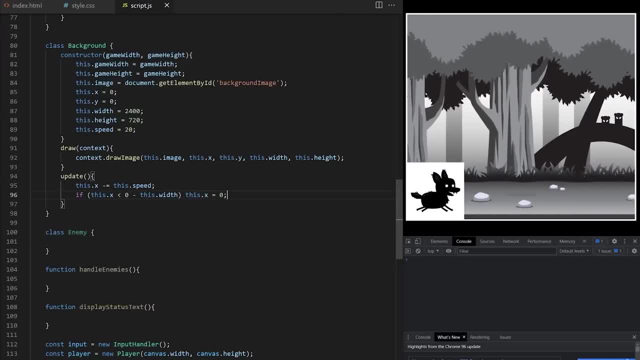 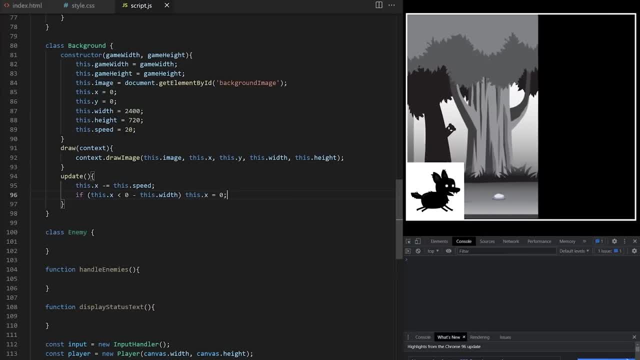 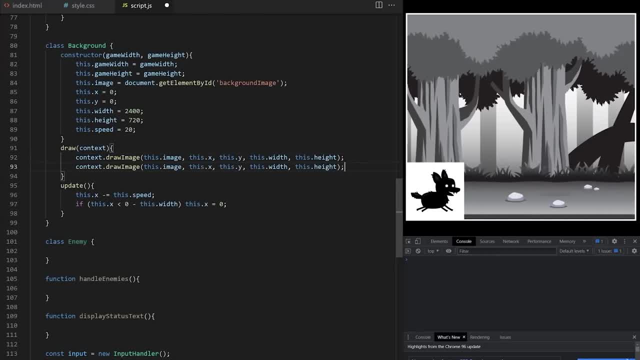 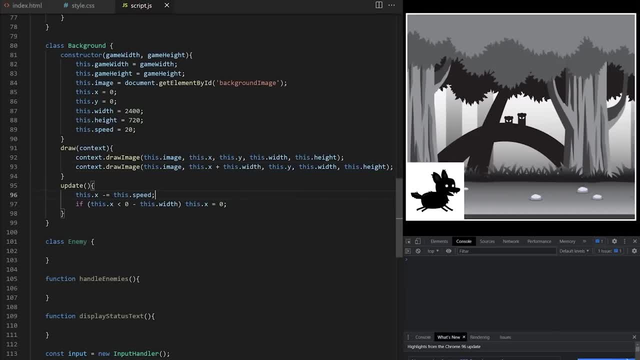 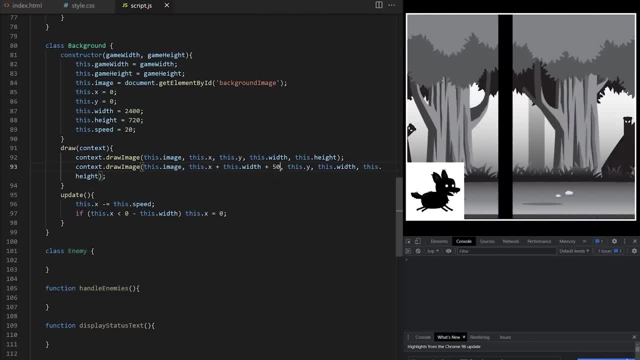 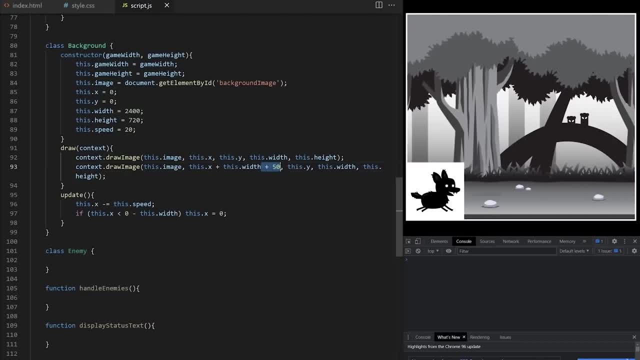 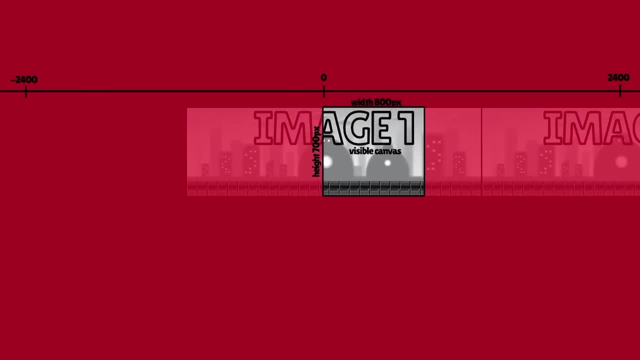 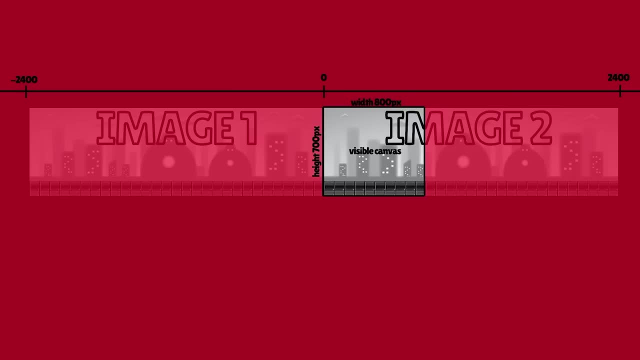 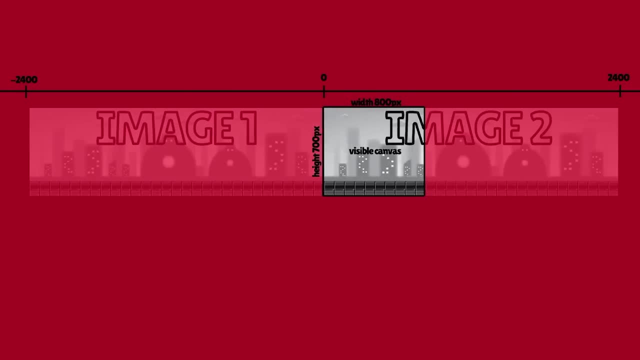 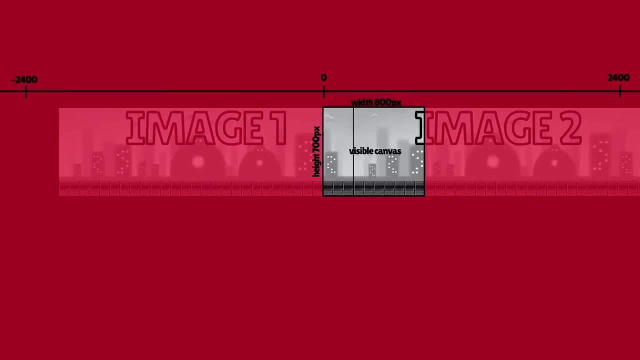 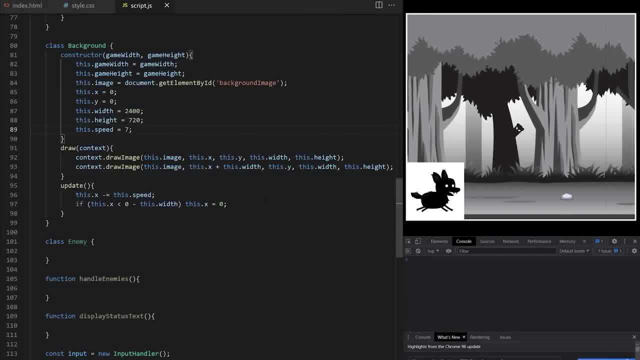 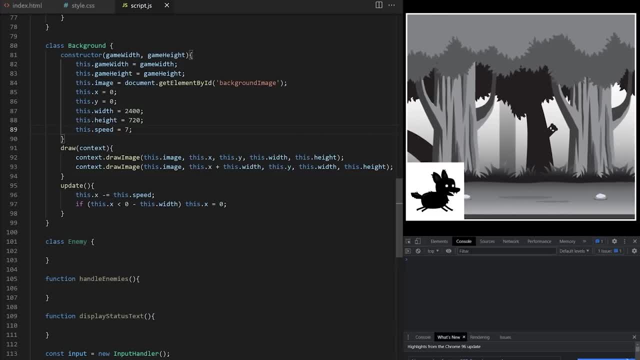 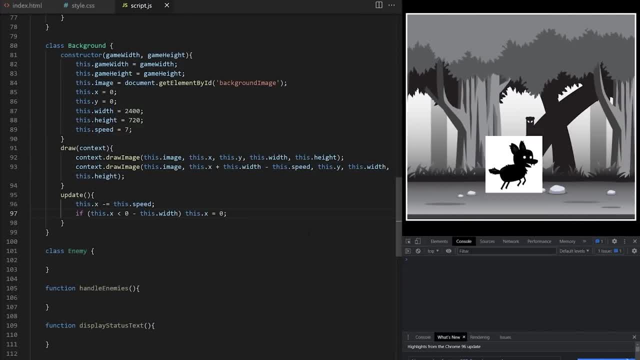 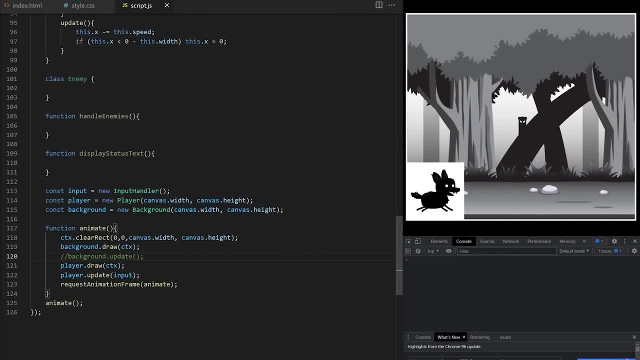 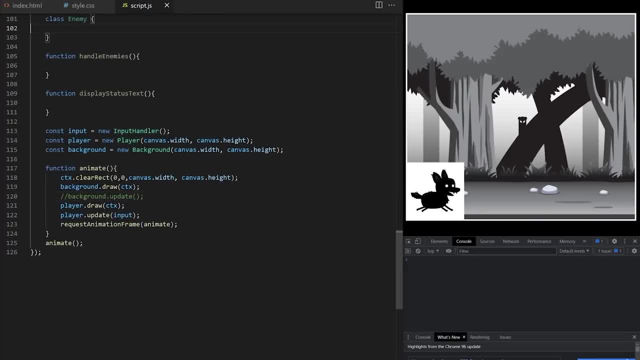 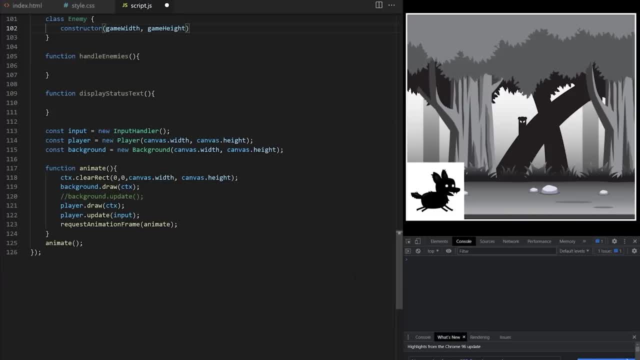 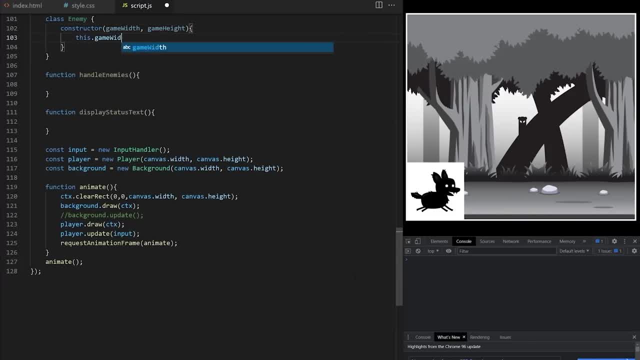 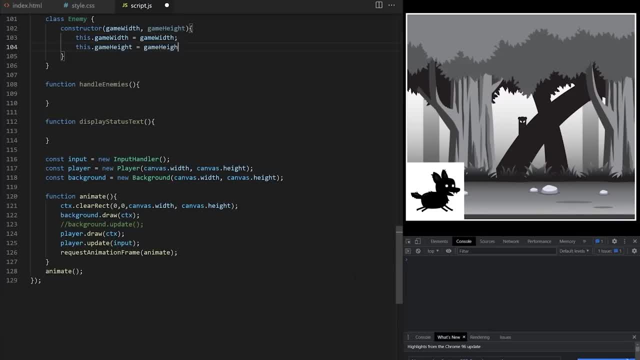 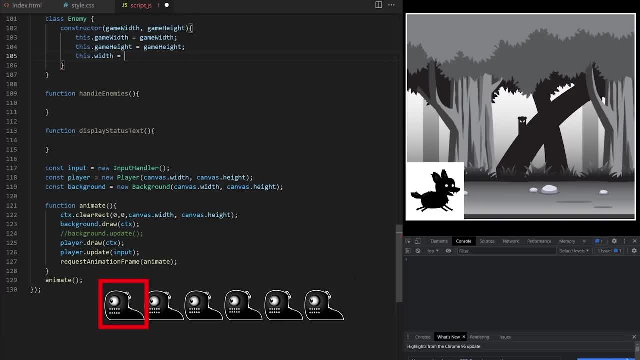 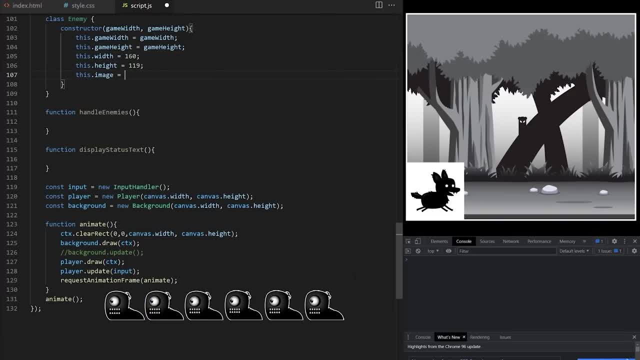 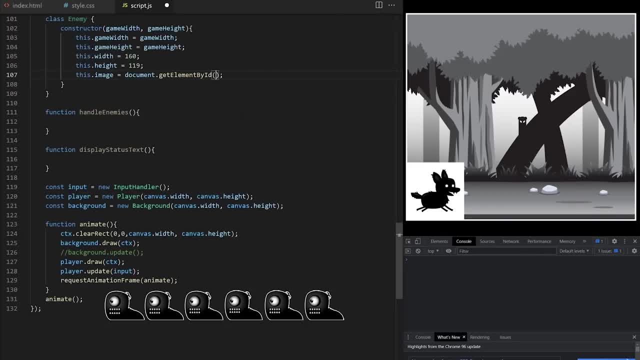 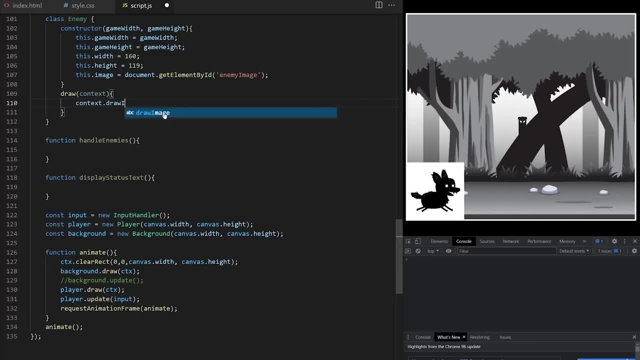 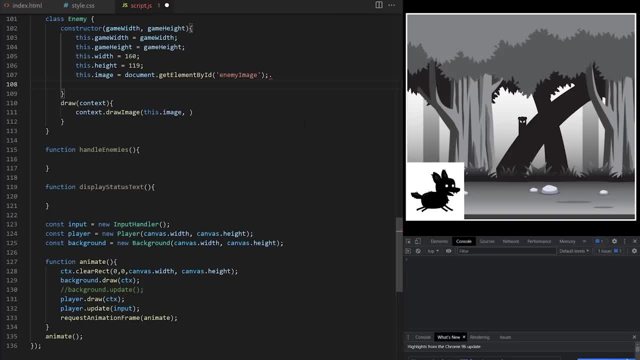 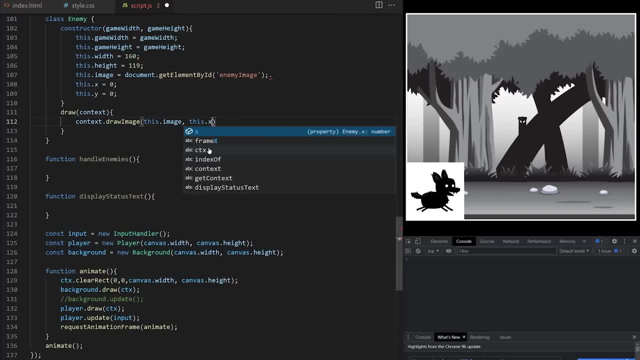 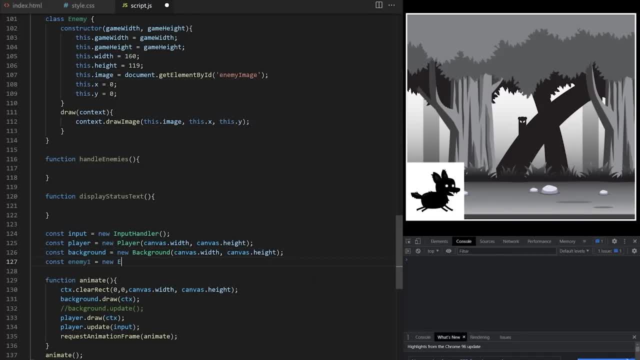 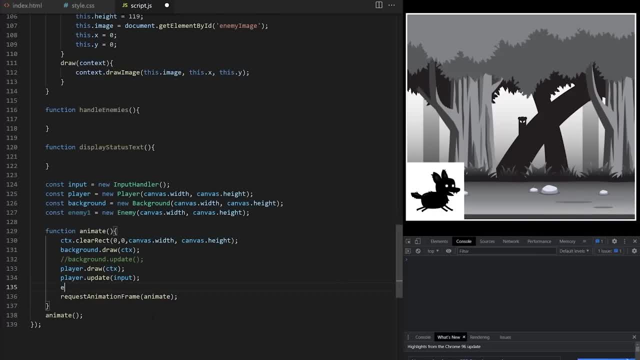 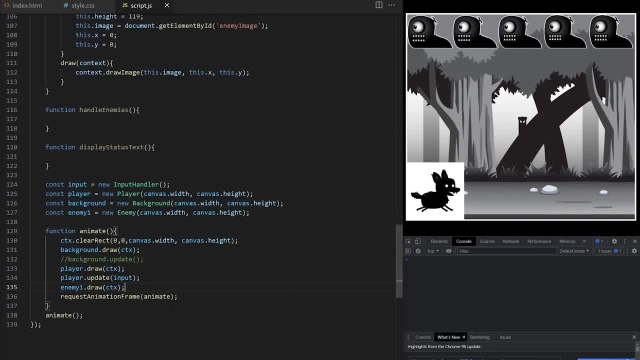 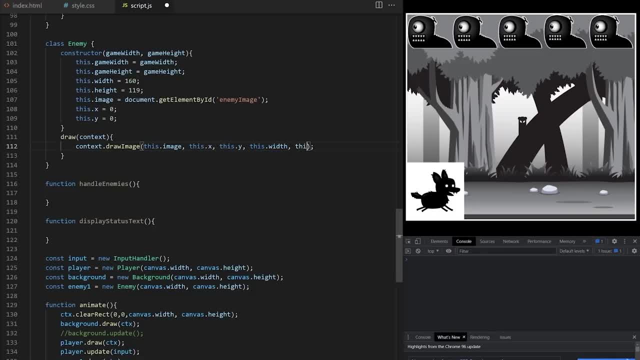 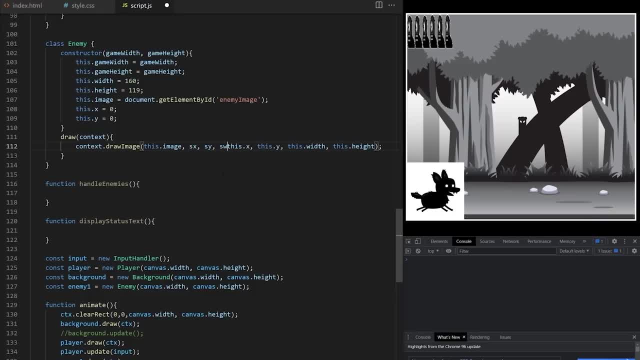 Horizontal coordinate of the background will be minus equals 20.. Horizontal coordinate of the background will be minus equals 20.. Horizontal coordinate of the background will be minus equals 20.. source width and source height, like we did with player, because we want to crop out single frame. 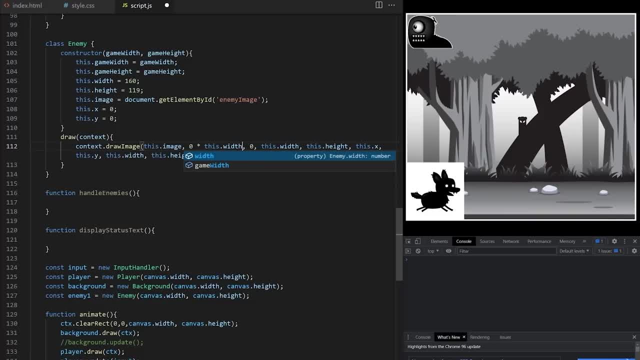 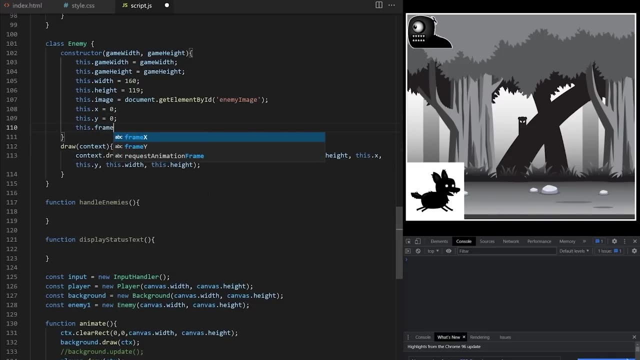 from the sprite sheet. Source x will be number zero times this dot width. Source y could be zero times this dot height, but since this sprite sheet has only one row, there will be no vertical navigation, so source y value can stay hardcoded to zero. I create frame x for horizontal navigation. 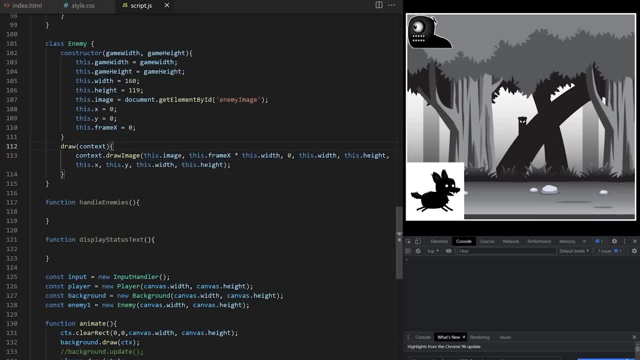 in sprite sheet and I replace it here. inside the draw image method, Vertical coordinate of the enemy will be game height minus height of the enemy and horizontal position is game width, so that it's hidden just behind the right edge of canvas. I create an update method and inside we 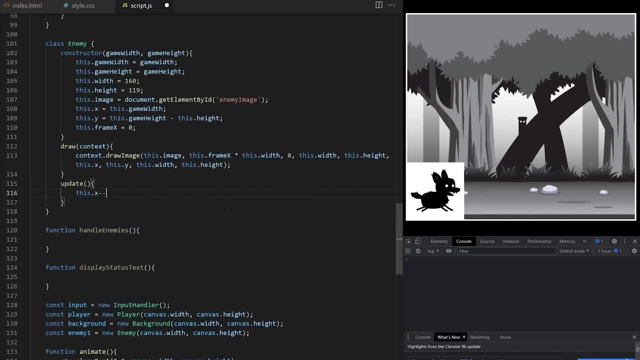 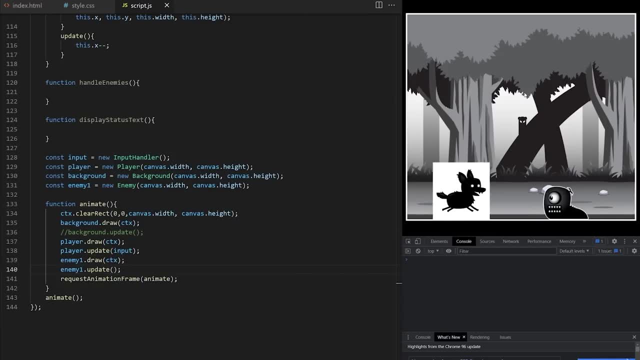 will just decrease x by one per frame to make enemy move to the left. I call enemy1 update from inside animation loop and we are animating one enemy created with our enemy class. I don't want to just have one enemy, I want to have multiple active enemies on the screen at the same time. 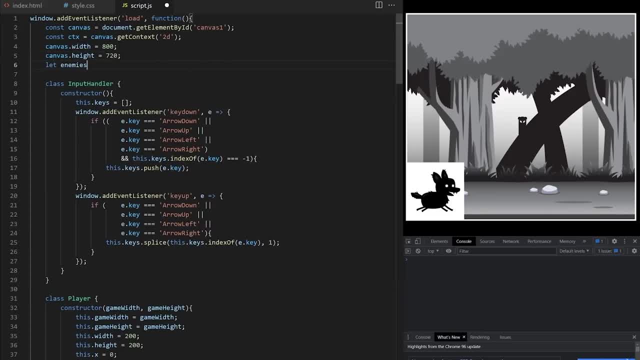 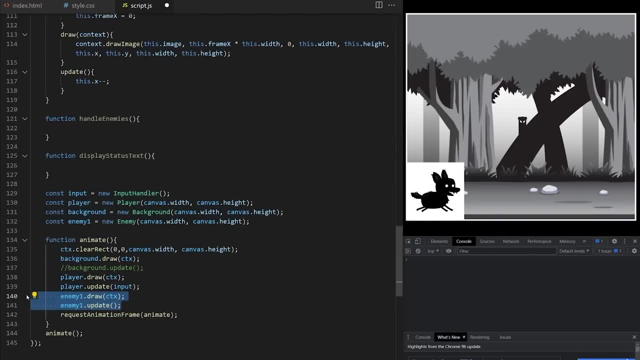 Upgrade the enemy to one enemy and create a new one. I create a new one and create a new one here on line 6.. I create a let variable, I call for example, enemies and I set it to an empty array. I delete these two lines of code from inside animation loop. We will draw and update our 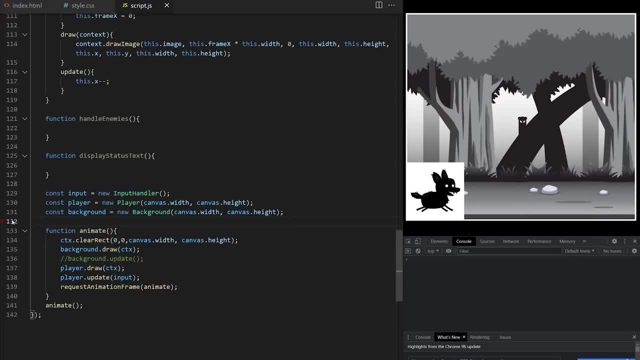 enemies from inside. handle enemies function on line 121. Handle enemies function will also be periodically adding new enemies to the game. so I take enemies array from line 6 and I call push on it. We will push instance of enemy class. so new enemy like this I know I have to pass it. 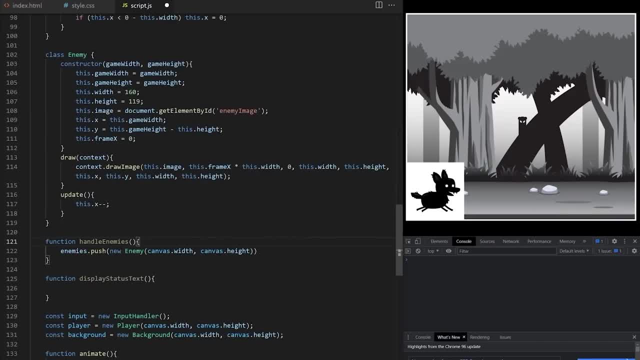 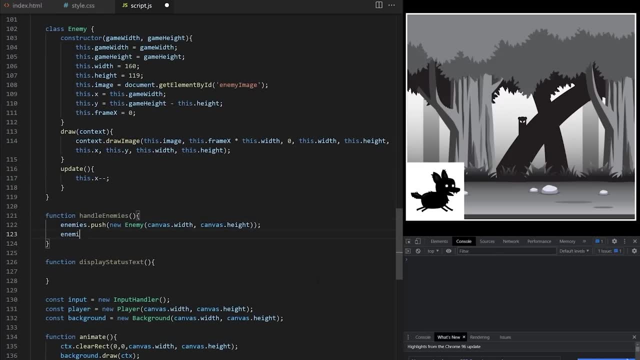 game width and game height. so I pass it canvas width and canvas height here. Then I want to call draw method and update method from line 116 for each enemy object in the array, so enemies for each, I call individual object in that array, for example enemy, and I use arrow function syntax. 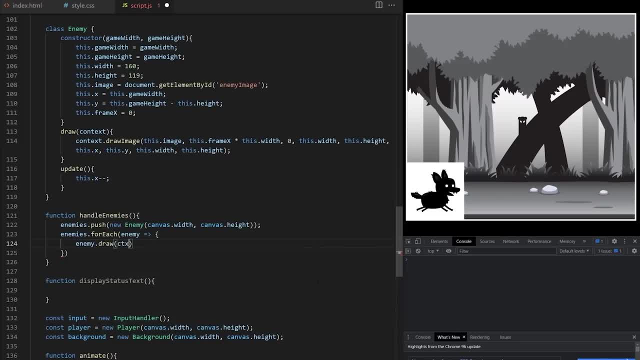 here. For each enemy object inside enemies array call their draw method. I passed C attorney �� and also called for their draw method and we will update its output configuration. So if we create a new one for example I will be calling handle enemy's functionnan the command from the 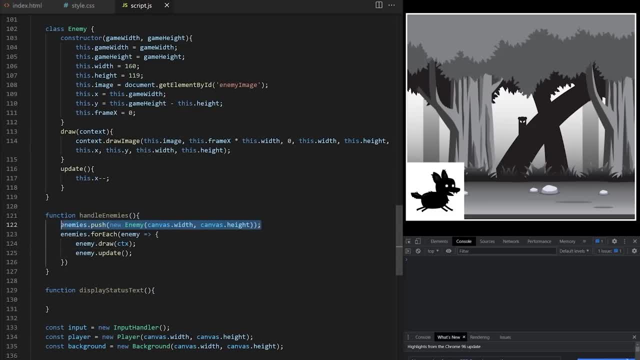 for every animation frame. so I can't just leave this line of code here like this. I don't want to push 60 enemies per second into our game. I take this line outside temporarily so it will just run once on the initial page load. So it will. 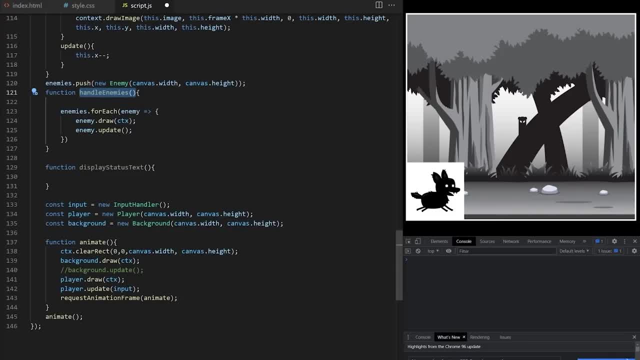 add just one enemy to the array at first. I call handle enemies from inside animation loop here on line 143.. Perfect, everything still works. Let's say I want to add new enemy into the array every two seconds. How do I do that? We can use. 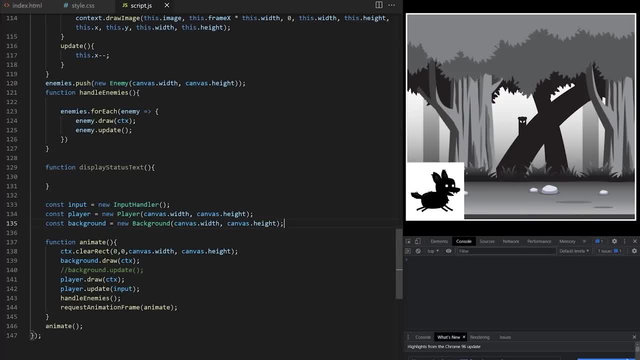 timestamps and delta time. I create a helper variable called last time, which will hold the value of timestamp from the previous animation frame. Inside animation loop I create a constant called delta time. Delta time is the difference in milliseconds between timestamp from this loop and timestamp. 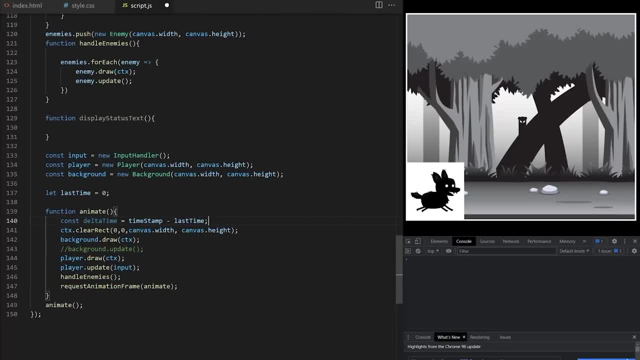 from the previous loop. The value of delta time tells us how many milliseconds our computer needs to serve one animation frame. Usually, if we are running at 60 frames per second, Delta Time is around 16 milliseconds. So Delta Time is timestamp from this loop, minus timestamp. 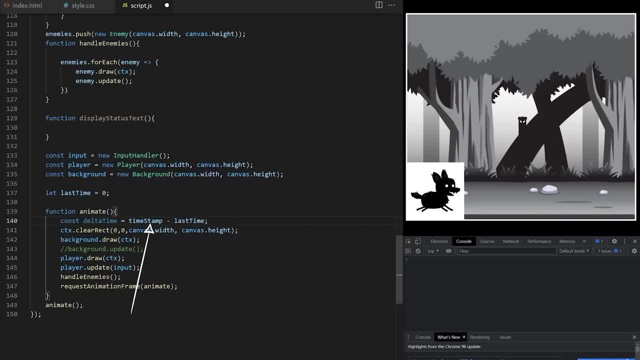 from the previous loop. This timestamp value is auto generated. here Request animation frame has a special feature: It automatically generates a timestamp and passes it as an argument to the function it calls. So because animate is being called over and over by Request animation frame, here it 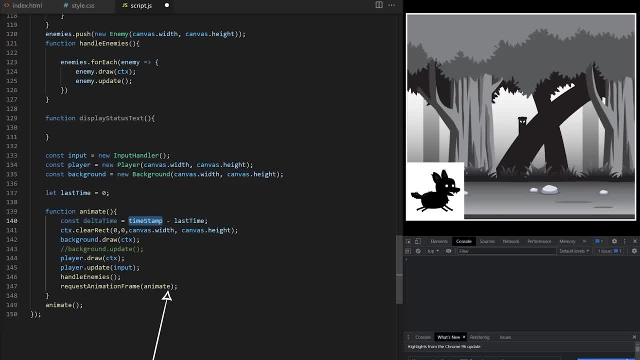 receives timestamp values as argument each time it's called. The first initial call of animate here on line 149 doesn't have auto-generated timestamp because it's not been called by request animation frame. so I have to pass it something here. I pass it 0.. When I 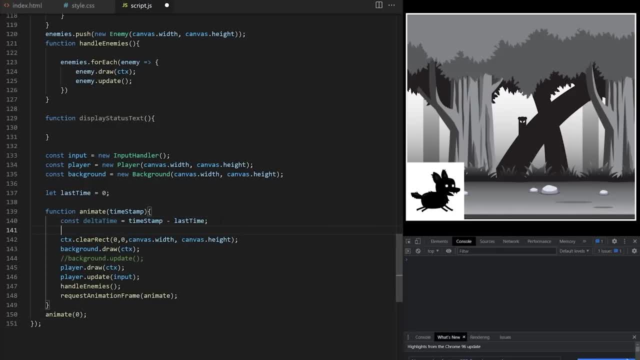 calculated delta time difference in milliseconds between timestamp from this loop and timestamp from the previous loop. I set last time to timestamp so that it can be used in the next loop as the value for timestamp from the previous loop. Our animation loop is created by request animation frame. It. 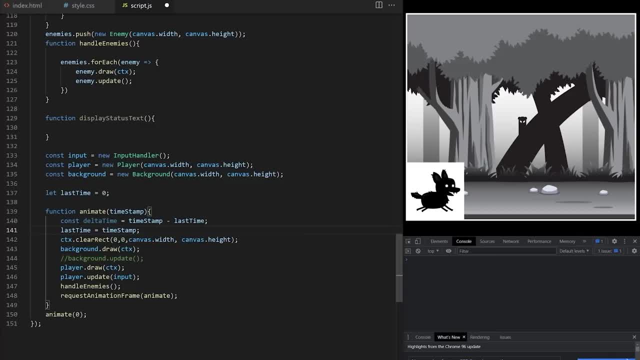 automatically adjusts the screen refresh rate. so most screens will run at 60 frames per second, which means if I consolelog delta time, I should get 1000 milliseconds divided by 60 frames per second. My delta time should be around 16.6 milliseconds. If you get a different number here, let me know. I wonder if we 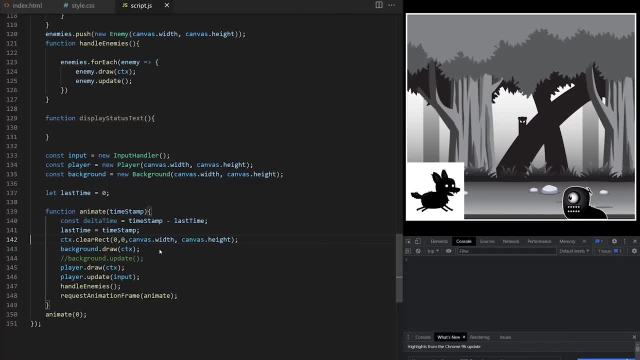 all get the same value. Now that we have delta time, we can use it to time different things around our code base. We will use it to trigger periodic events. I pass Delta time to handle enemies. I comment this out. I make sure the handle enemies expects Delta time. 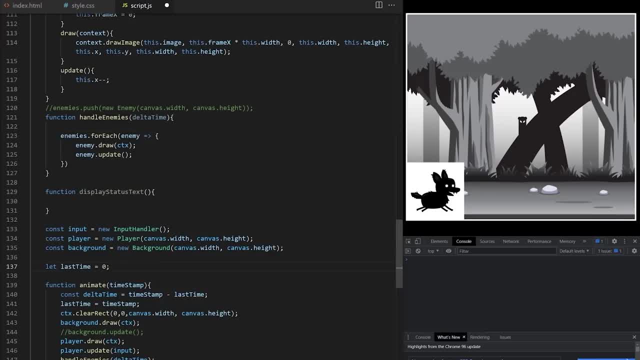 value to time something periodically with Delta time. I need two helper variables: Enemy timer, which will be counting milliseconds from 0 to a second, and every time it reaches that limit it will trigger something and reset itself back to zero. We will need enemy interval, which will be a value in milliseconds for that time. 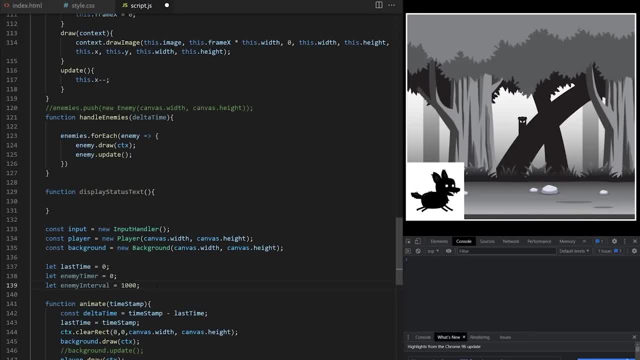 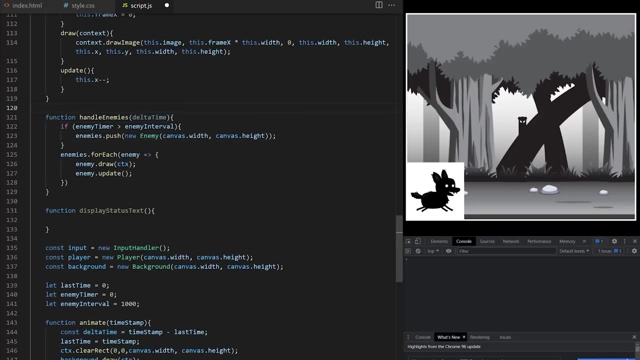 limit. I want to add new enemy in the game every thousand milliseconds, Every time timer reaches 1000.. In handle enemies I say: if enemy timer from line 140 is more than enemy interval from line 141, push new enemy into enemies array. Then reset enemy timer back to zero so we can count again, Else just. 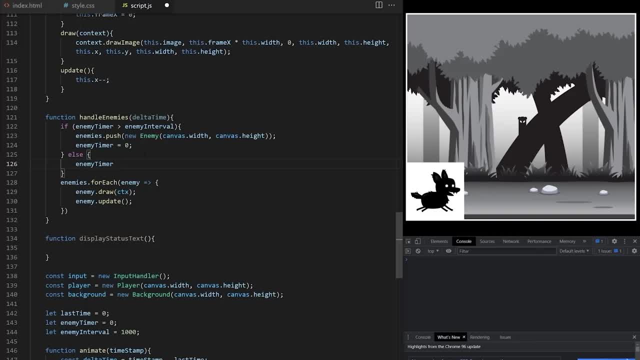 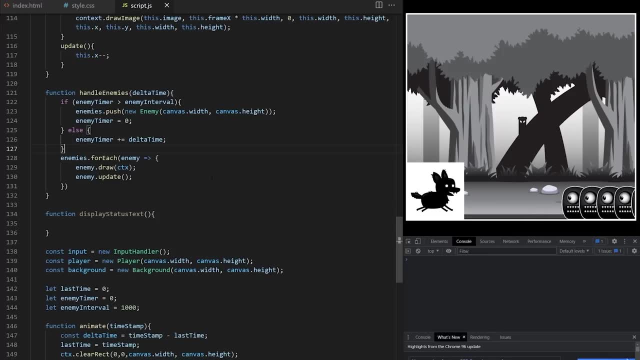 keep adding Delta time to our enemy timer until the limit defined in enemy interval is reached. Using Delta time like this will make sure our events are timed the same on slow and fast computers, because faster computer will have lower Delta time, so it will take more loops to accumulate enough in its 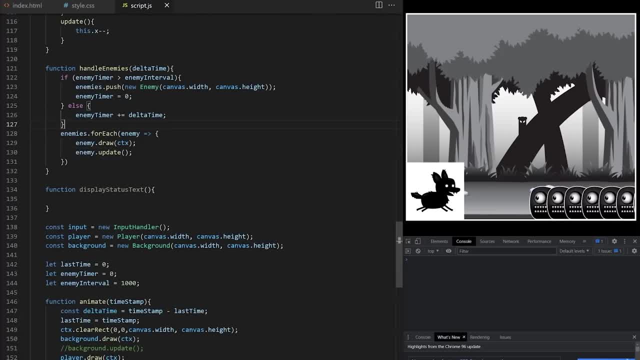 timer. That way fast and slow computer will reach the limit at the same time. I explain this in more detail. in a special class I can also set enemy interval to 2000 milliseconds, two seconds. I created this dot speed property on enemy class I. 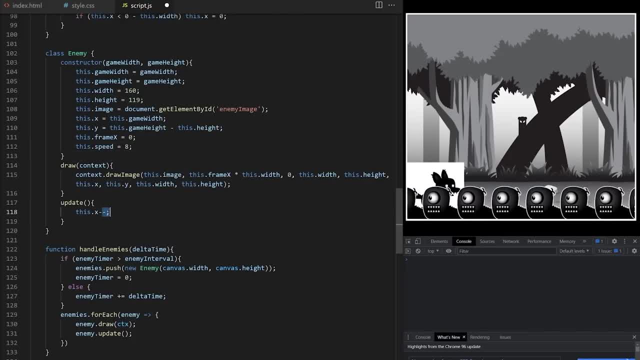 could give each enemy randomized speed. here using mathrandom, I will give all of them the same speed of 8, and here I say this dot X minus equals this dot speed. You can see enemies come in a set interval of 2 seconds, Very predictable. Maybe I want to randomize that interval. 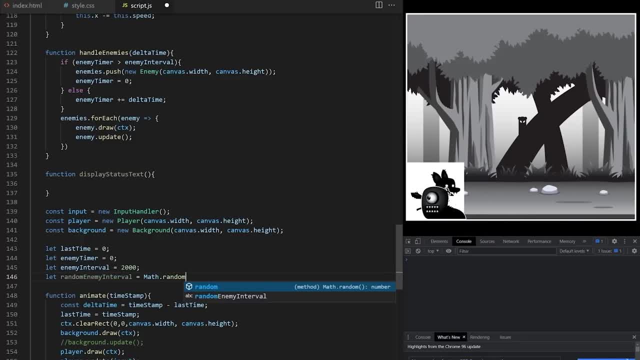 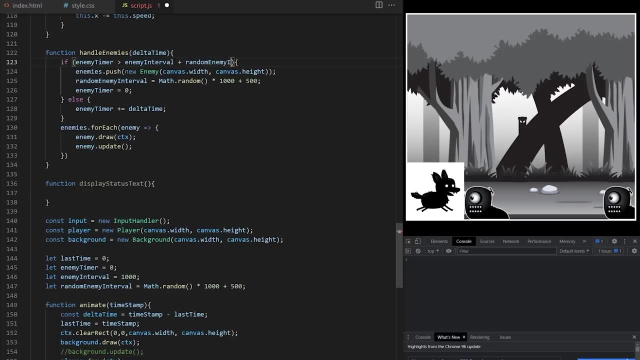 a little bit. I can, for example, create a variable called a random enemy interval and I set it to a random number between 500 and 1500 milliseconds. I change enemy interval to 1000.. Whenever enemy timer reaches enemy interval plus random enemy interval, I push new enemy and I set random enemy. 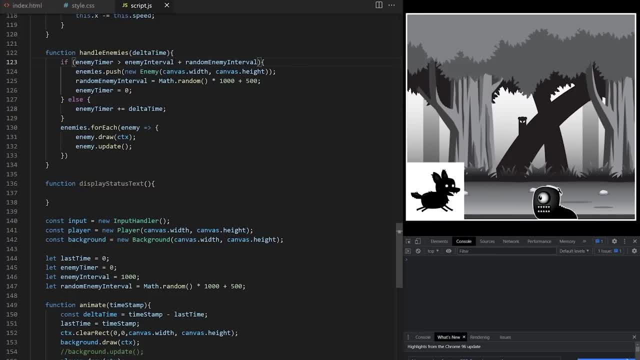 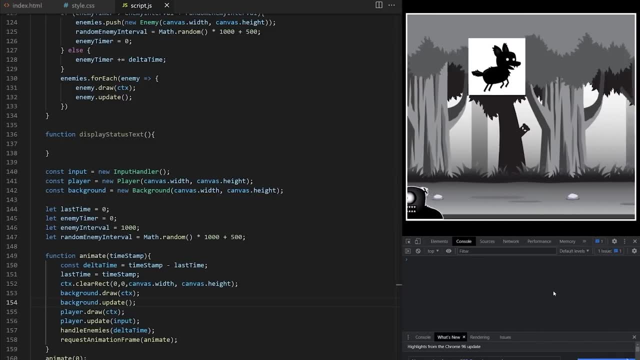 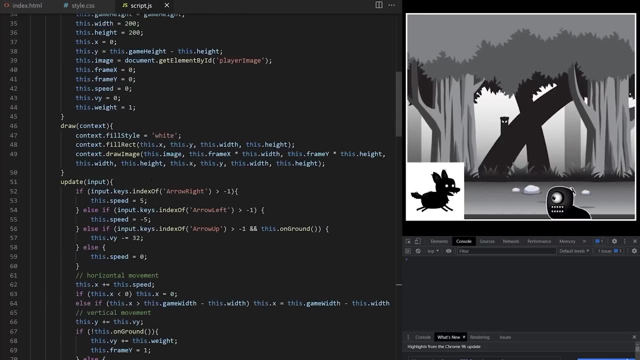 interval from line 147 to a different value. I could have also randomly set some enemies further along x-axis to get the same result. Now enemies are coming in more random, less predictable intervals. Inside the draw method on player class, I can remove the white rectangle behind. 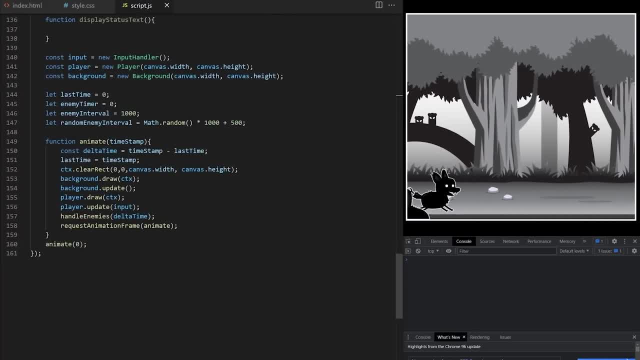 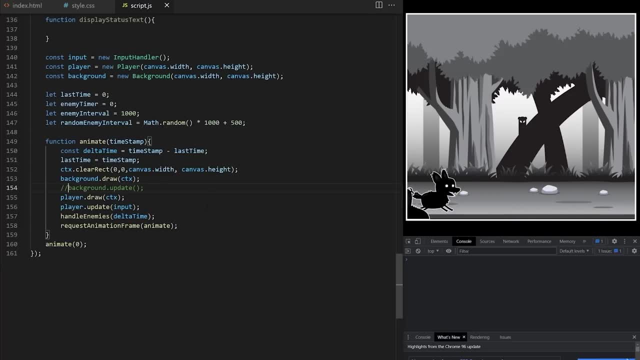 the player. I pause the background again by commenting out line 154.. We are displaying just the first frame in player and enemy sprite sheets. Let's actually animate those sprite frames. The sprite sheets we are using are optimized for speed between 15 to 20 frames per second. so I would like. 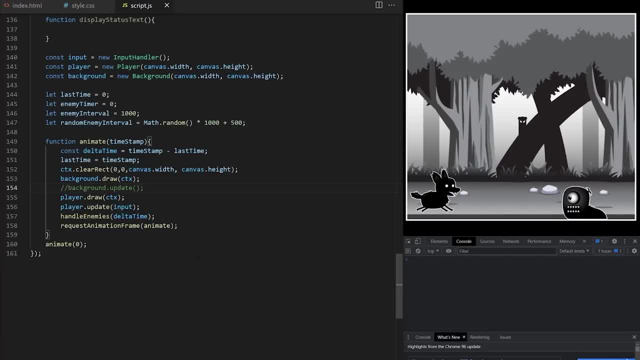 to be able to set FPS frames per second for sprite frame animation while still allowing the rest of our game- things like player position and background scrolling- to update 60 times per second? How do we do it With delta time? I am passing delta time to handle enemies here on line 157.. I pass it along to enemy. 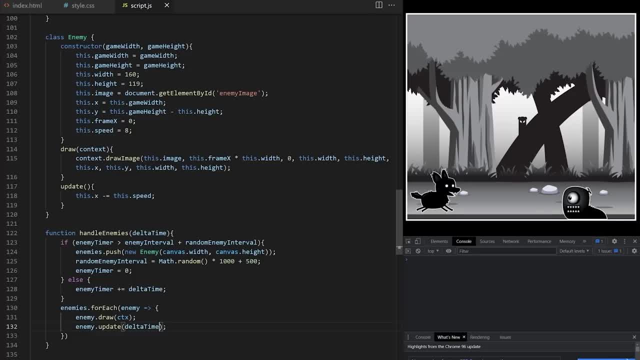 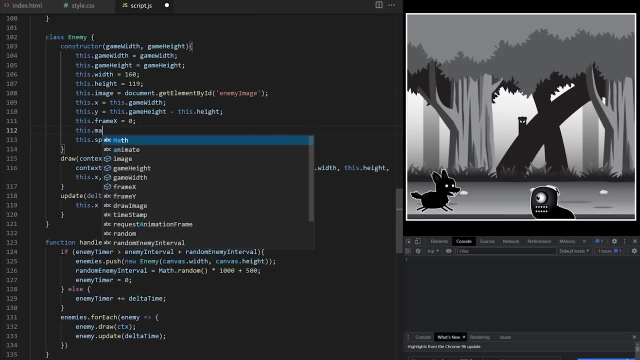 update method and I make sure update method on enemy class expects that value. Update method is being called from inside animate 60 times per second. Inside update method. here I will use delta time to keep track of how many milliseconds passed between individual calls and only when the right threshold is reached I will swap frames in the sprite. 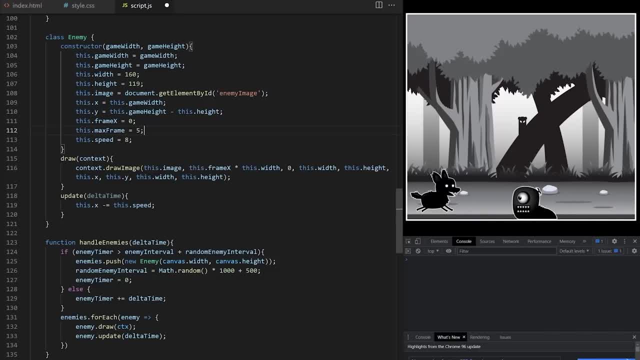 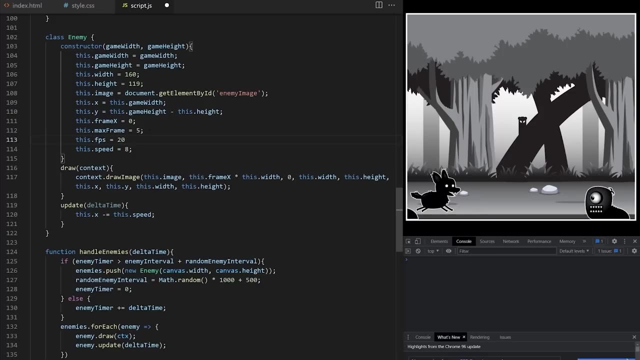 sheet. To animate sprite sheets horizontally, I will cycle between frame X of 0 and max frame which, in case of enemy sprite sheet, is 5.. To time frame rate with delta time, I will need three helper properties. Thisfps to set frames per second. Let's do 20.. Keep in. 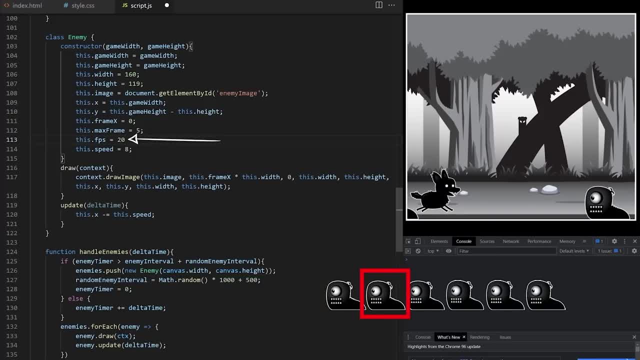 mind. this fps will affect horizontal navigation within enemy sprite sheet, How fast we swap between individual animation frames. Nothing else will be affected. I want the rest of the game to run at 60 frames per second second. i could use this technique to slow the entire game down to 20 frames per second, but 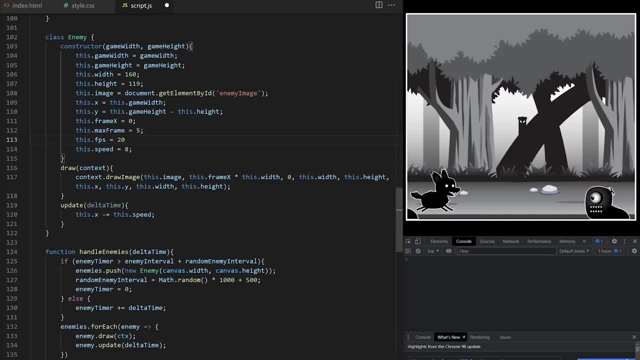 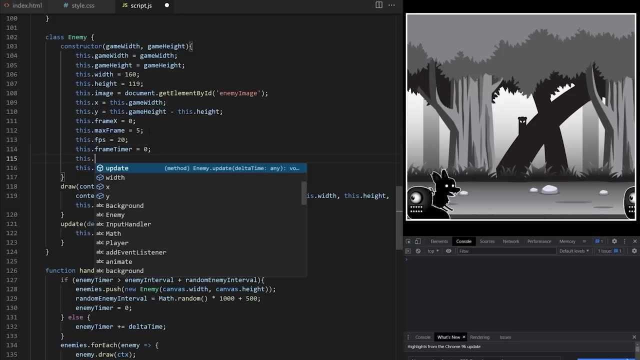 then player controls wouldn't feel very responsive, we would get delays in collision detection, displayed text and so on. i want to slow down only animation of enemy sprite sheet, nothing else. i will also need frame timer which will count from zero to frame interval over and over and 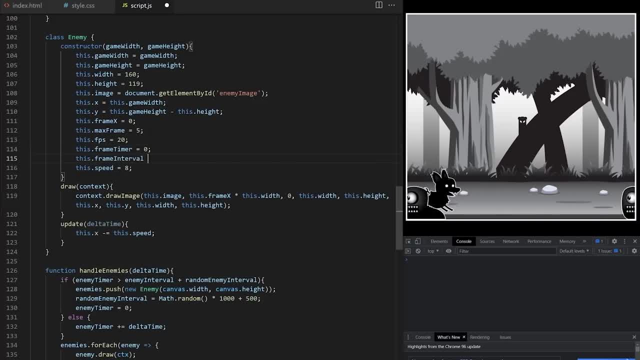 frame interval will define that value we are counting towards. it's a value of how many milliseconds each frame lasts, so thousand milliseconds divided by 20 frames per second in this case. first let's cycle between frames at full speed. so if this dot, frame x from line 111, 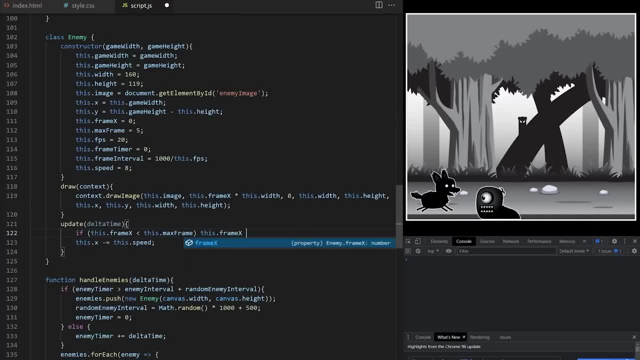 is more than max frame, set frame x back to zero, else increase frame x by one. i have to do more or equal here, so we don't get empty frame because of this source x attribute. we are passing to draw image method on line 19. cycling between 0 and 5 with frame x variable will animate sprite sheet horizontally. now you can. 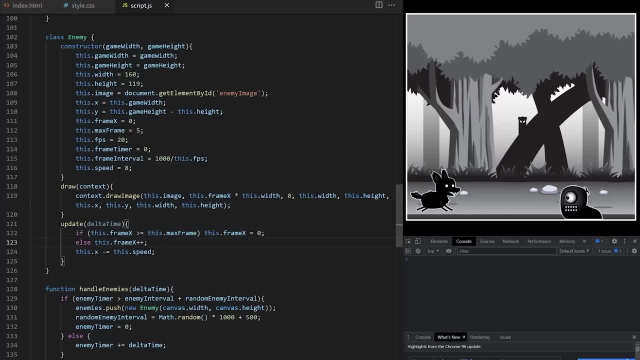 see enemy sprite sheet is animating, but it's very fast. these particular sprite sheets were designed for lower frame rate. we defined fps of 20 on line 113.. here i say: if this dot frame timer from line 114 is more than frame interval from line 115, only then run this code that manages frame x cycles at. 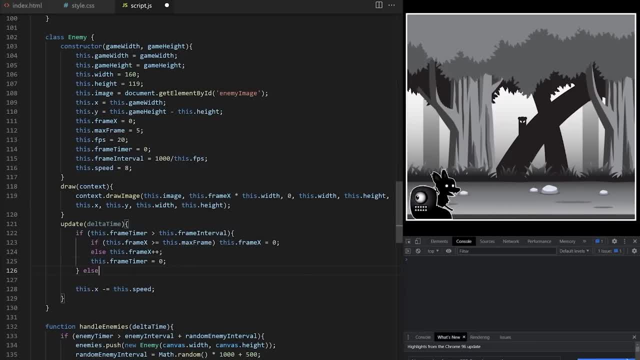 frame x and then set frame x to zero, and then set frame x to zero and then set frame x to zero so it can count again. else, just keep adding delta time to frame timer until the threshold of milliseconds defined in frame interval is reached. now you can see enemy sprite sheet is swapping. 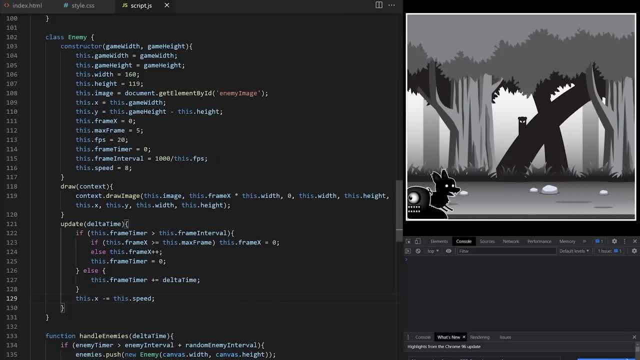 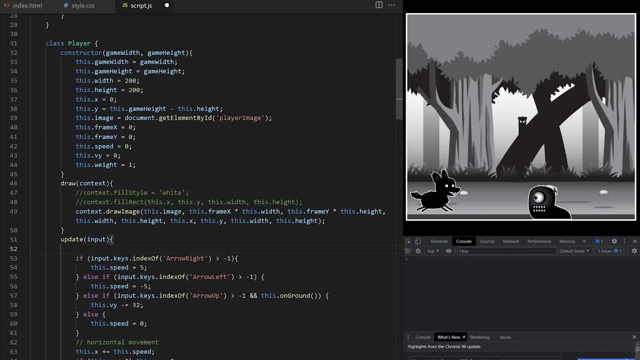 between frames slower at 20 frames per second, while enemy movement is still at original 60 frames per second. inside update method on player class. i will do exactly the same thing. first i say if frame x from line 40 is more than frame x, then the frame x will be the same as frame x from line 111. 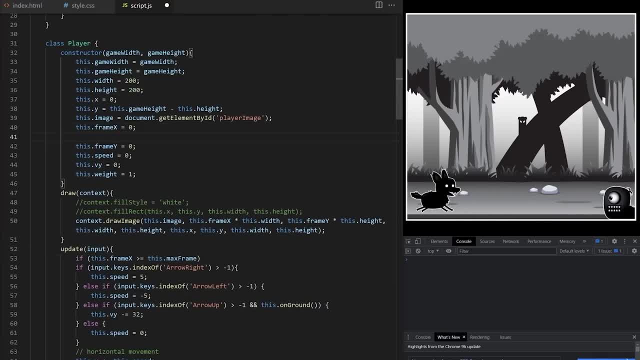 then max frame, which i need to define here. we will start with this row and there we have eight horizontal frames counting from zero. if frame x is more or equal to max frame, set frame x back to zero. else increase frame x by one. running animation on. player is animating. i go down here to enemy. 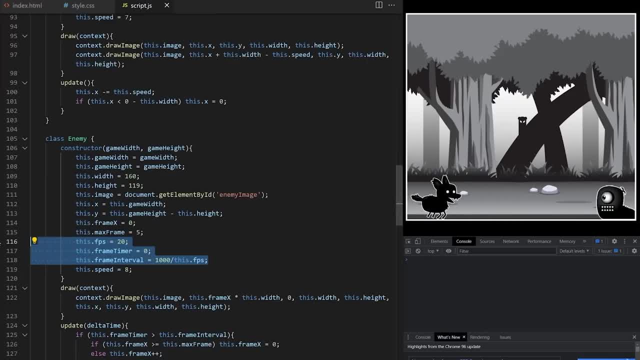 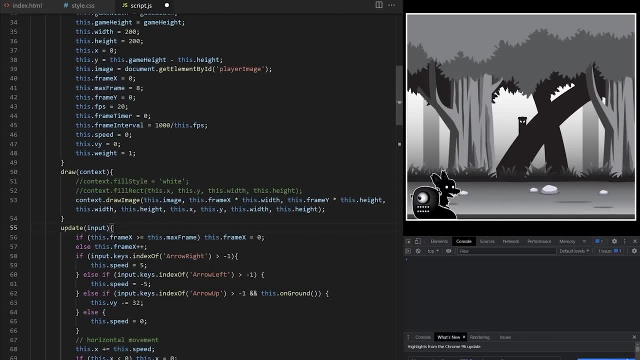 class and i copy fps, frame timer and frame interval properties and i paste them here on our player class inside update method. here we are dealing with sprite animation, here are controls. yes, so if frame timer from line 44 is more than frame interval, run all this sprite. 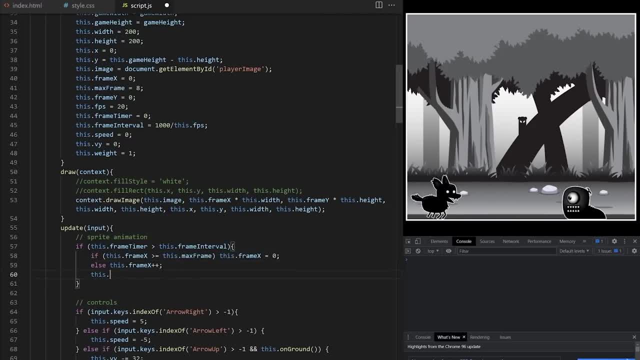 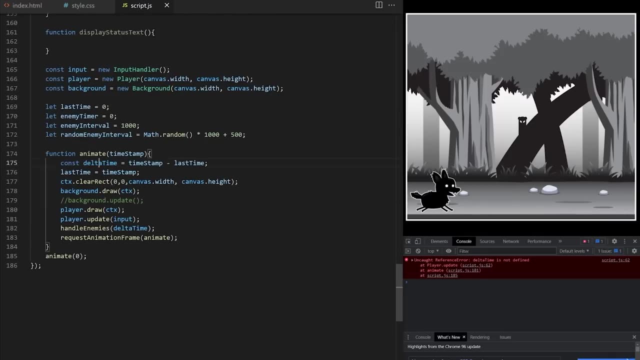 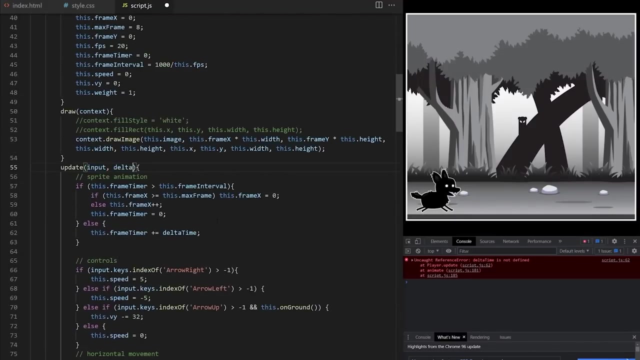 animation code and reset frame timer back to zero. else keep increasing frame timer by delta time. update method doesn't have access to delta time, so i make sure it takes it as an argument argument when we call it here on line 181.. Up here, I make sure update method expects that argument. 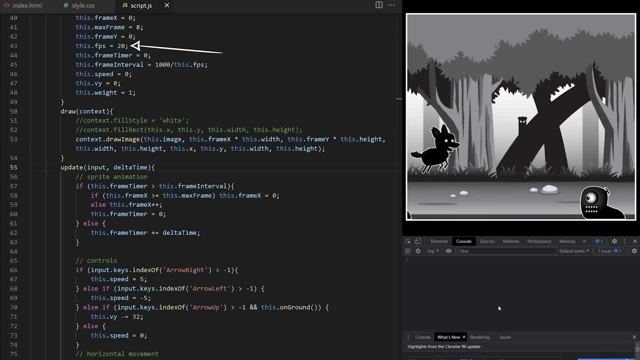 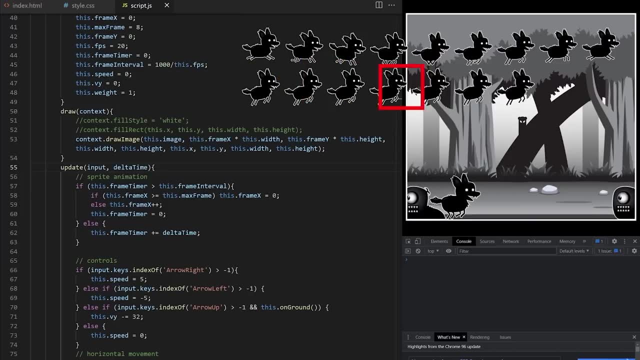 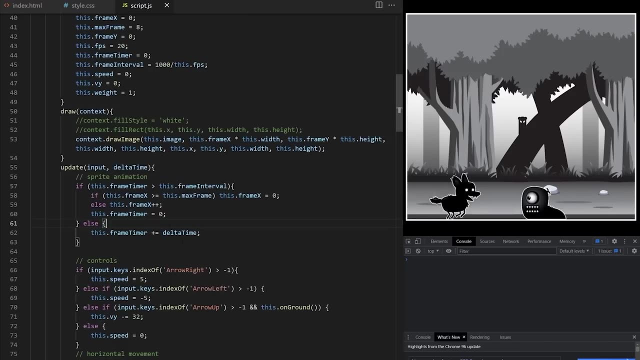 Now player sprite sheet is animating at 20 frames per second. When I jump we get blink in because max frame is set to 8 on line 41 and jump row doesn't have that many frames, so we are including empty frames. We have only two player states, basically jumping and running on ground. so dealing with 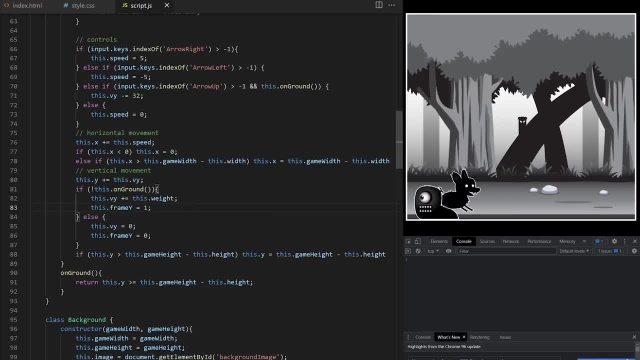 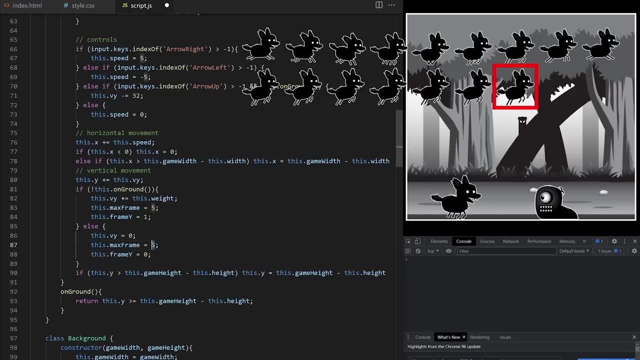 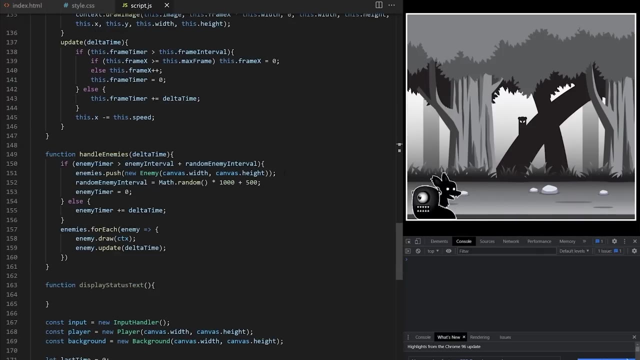 that is easy. Down here we deal with vertical movement When we are not on ground. we set max frame to 5 for jumping animation, else meaning we are on ground. set max frame to 8 for running animation. On line 151, we are adding new enemy to our game in a randomized interval. 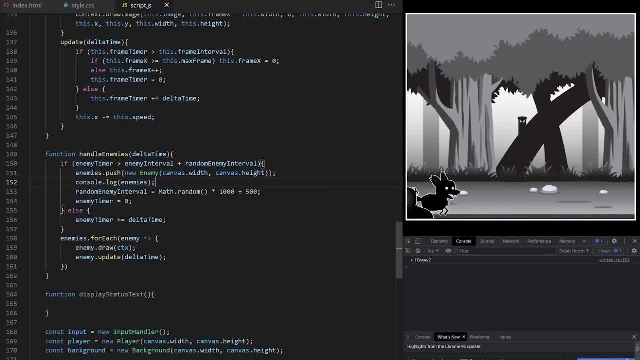 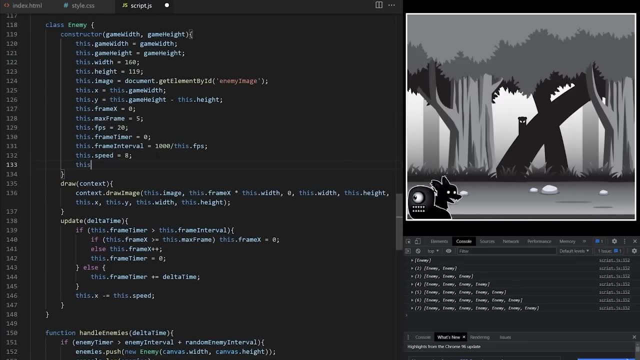 When I console log enemies array I can see it's endlessly growing and adding more and more enemies. I actually want to remove enemies that moved off screen from enemies array. On enemy class, I create a property I call marked for deletion and I initially set it. 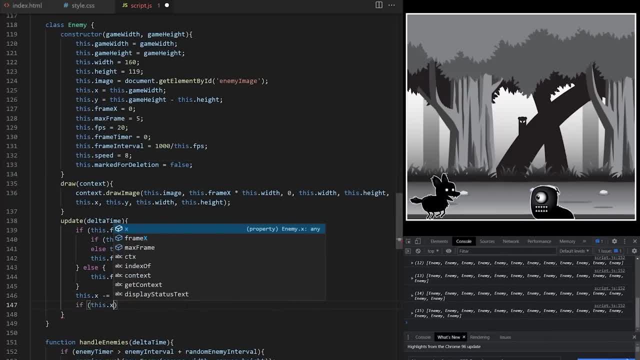 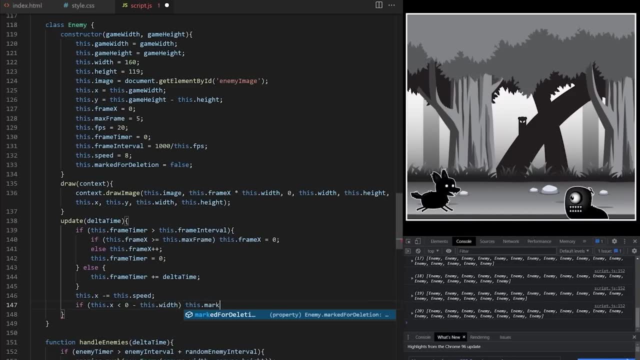 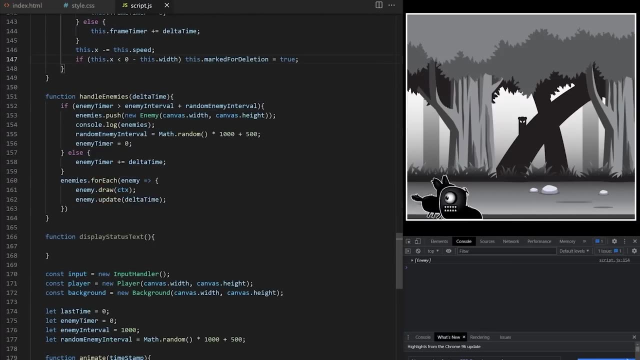 to false. In update method I say: if horizontal x coordinate on enemy is less than 0 minus enemy width, meaning if it has moved past the left edge of game area set marked for deletion. to true Inside handle enemies, I say: take enemies array which we defined earlier as a let variable. 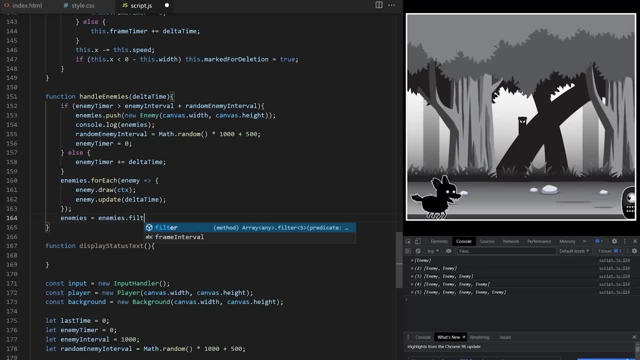 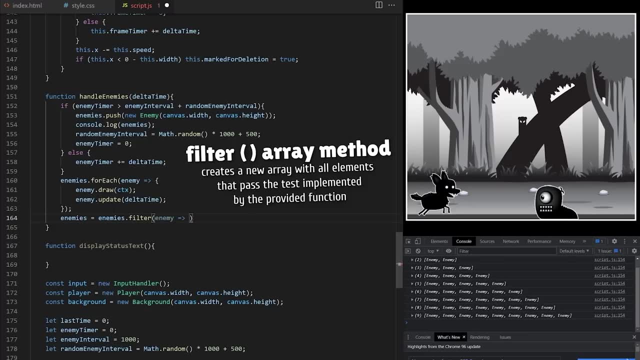 and reassign it to the same array, but filter that array first And only include elements that have marked for deletion property set to false. Filter is a built in array method which creates a new array with all elements that pass the test implemented by the provided function. 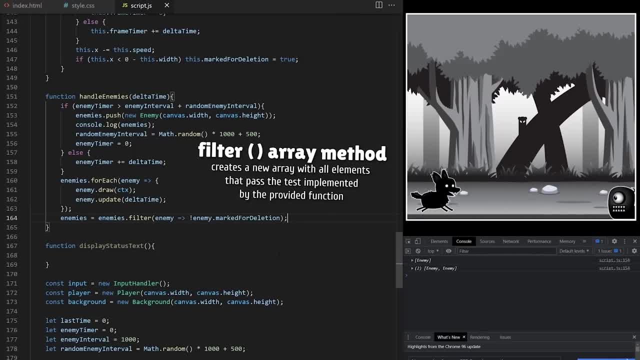 In our case, all our elements are tested and checked if their marked for deletion property is false. Now you can see in console. we have between 1 and 2 enemies in the array at any given time. All the enemies are being removed. I want to display score. 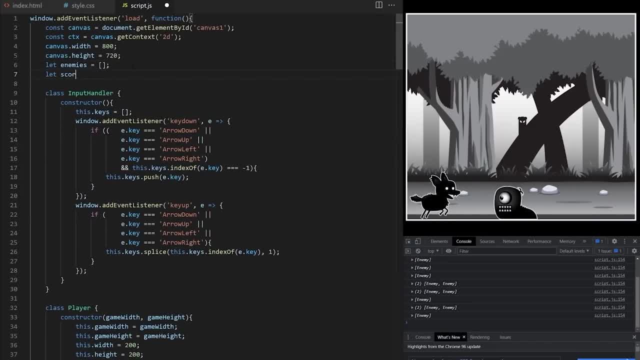 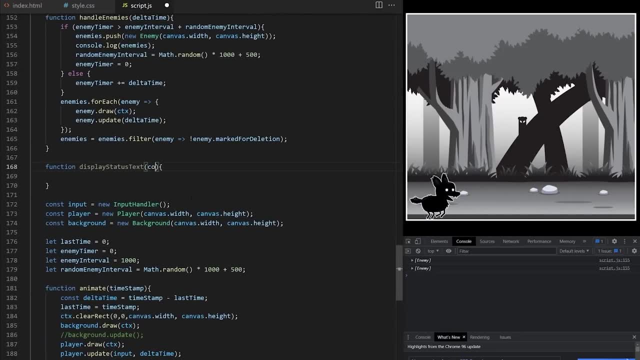 On line 7.. I define a let variable called score and I initially set it to 0.. On line 168 we have display status text function. I will use it to display current score. I pass it context as an argument to specify which canvas we want to draw on. 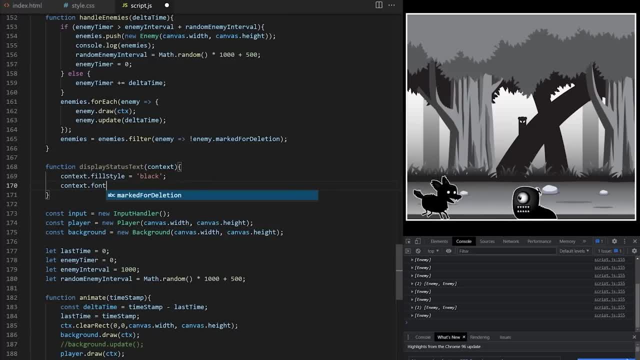 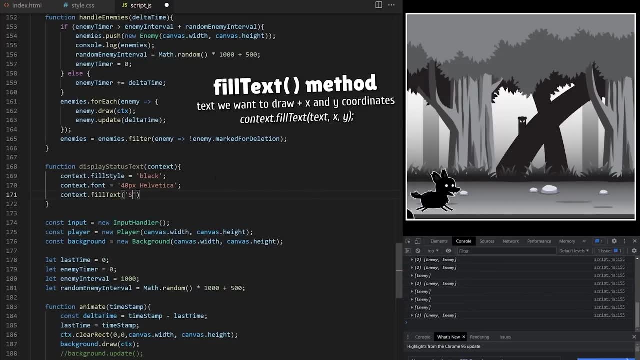 I set fill style to black color. I set canvas font to 40px. Helvetica Fill text built in canvas method will actually draw the text. It expects text we want to draw and x and y where to draw it. I want the text to say score colon space plus value of score variable from line 7.. 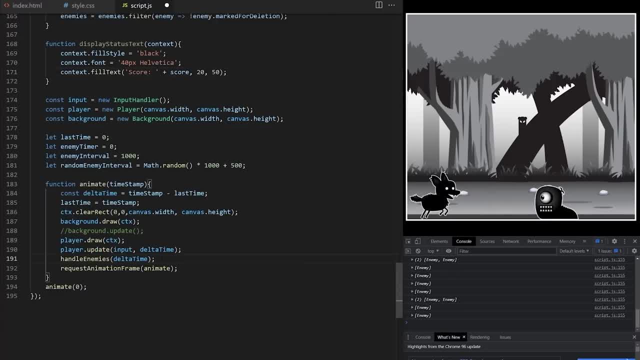 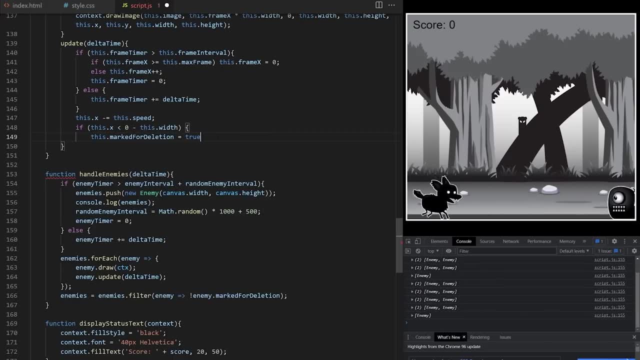 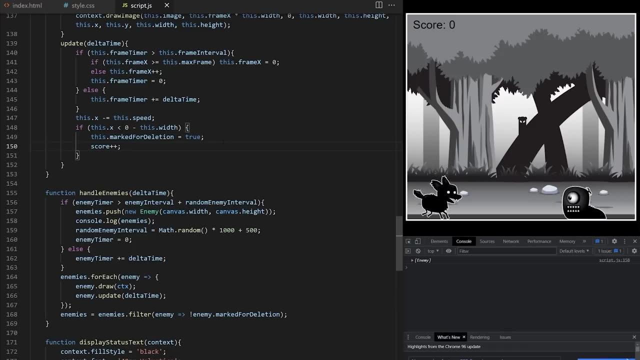 X, coordinate 20, y coordinate 50.. I call this new function from inside animation loop and I pass it. ctx: Inside update method on enemy class. I will count score every time enemy moves off screen, assuming player successfully avoided colliding with that enemy, And I increment score by 1.. 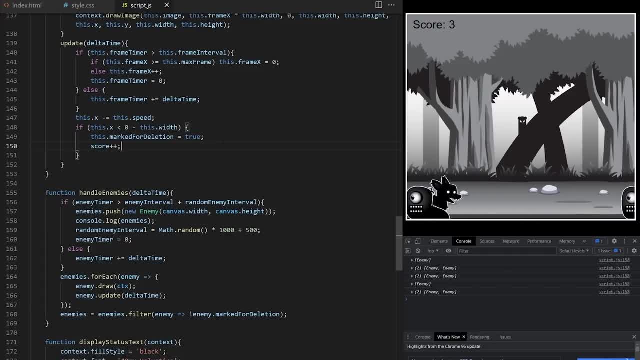 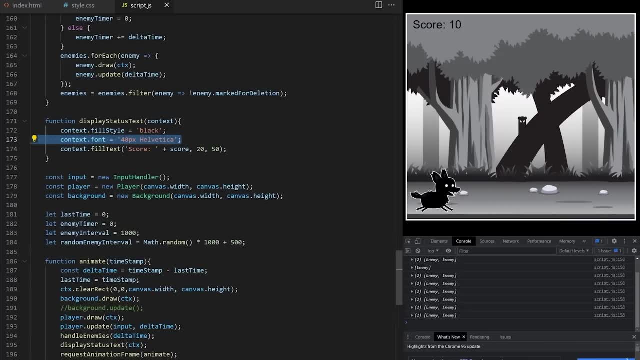 That works nice. I want to highlight the font. I can give it canvas shadow, but for some reason in firefox, built in canvas shadow property causes lag and frame rate drops. so I will do a trick here. I will draw the same message twice, One black, one white. 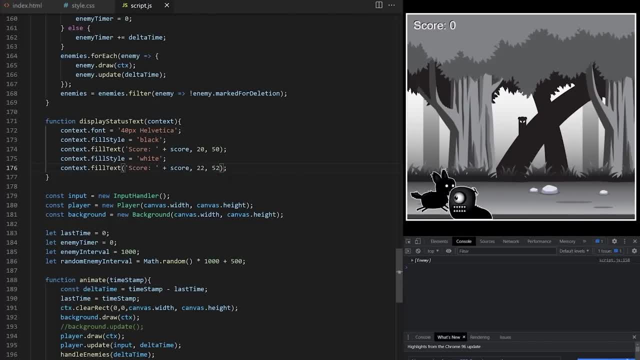 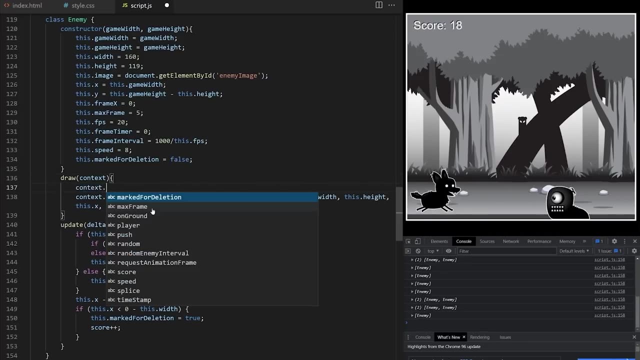 The top one will have 2 pixels offset, So I kinda created my own shadow manually. Let's check for collisions between player and enemies First. we need to decide on the right technique to use here. The easiest ones are collision between rectangles And collision between circles, where we give elements like player and enemy hitboxes shaped. 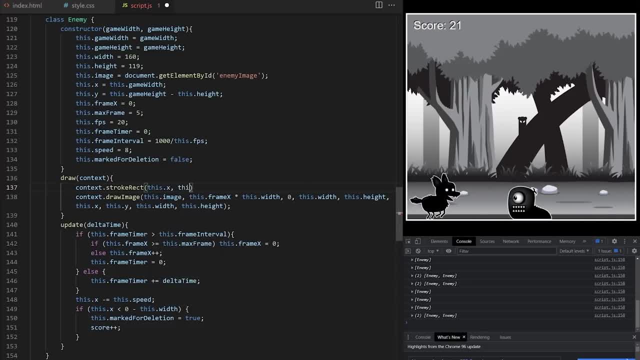 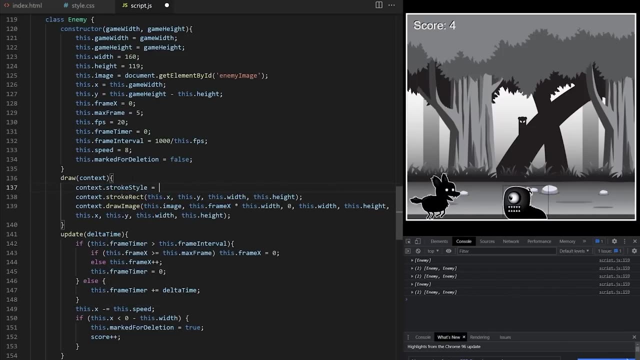 as rectangles or circles. We could also do more complex and more precise collision checks here, such as collision check between polygons, called separating axis theorem, or we can base collisions on color or opacity. I will stroke rectangle around our enemies so we can see basic collision hitbox. 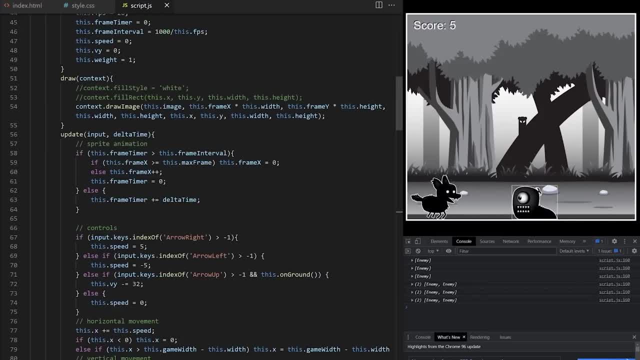 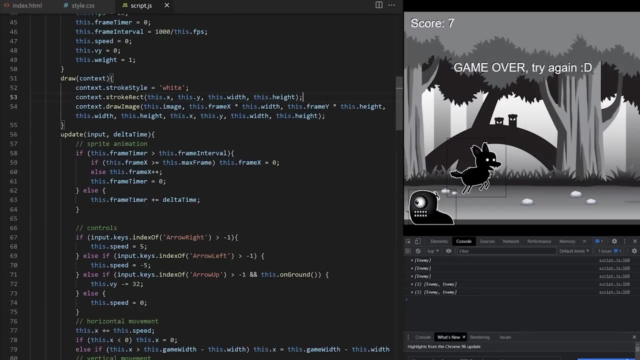 Let's make it white. I do the same for player. You can see the rectangles. now, If I use collision detection between rectangles and I keep those hitboxes at their base sizes whenever these two rectangles touch or intersect, we will get collision between player and enemy. 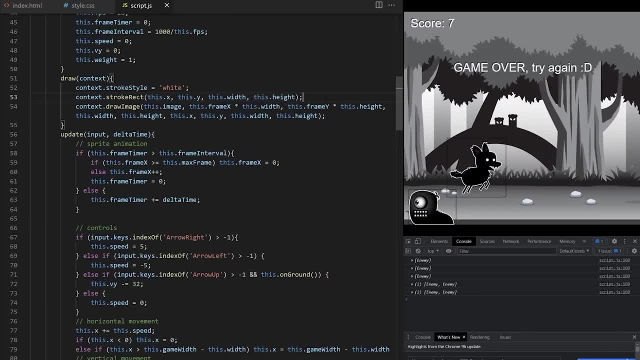 I tried to apply it before and I played with it and sometimes we get really unfortunate collisions, like on this screenshot where my player is landing from a jump. Dog and worm images are clearly far away from each other, but you can see that the corners intersect and we got game over. 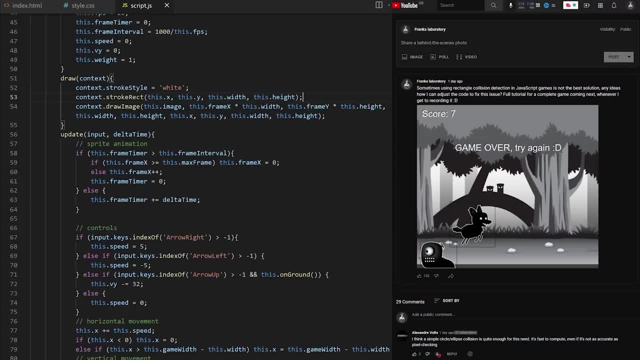 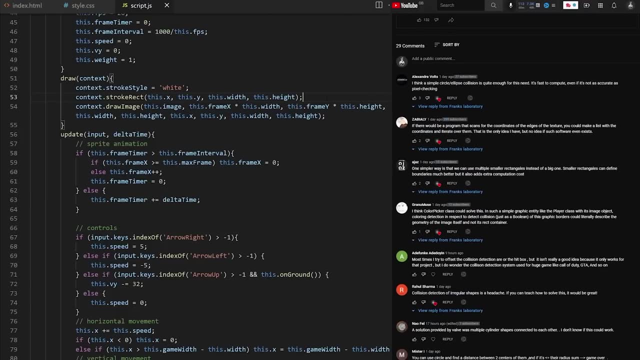 I asked you in my Q&A How would you approach this challenge. We spoke about different options we have here. Some of you suggested separating axis theorem for collision between polygons. Some of you think that we could use a set of smaller rectangles that match shapes of 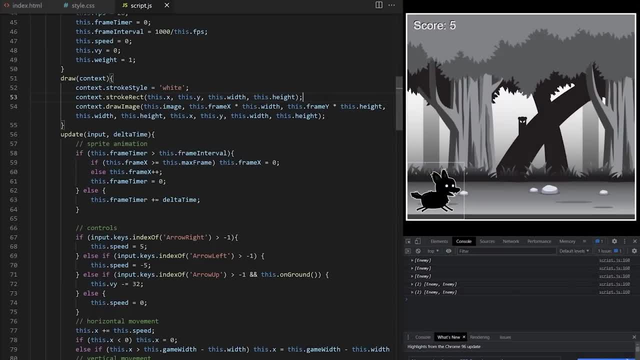 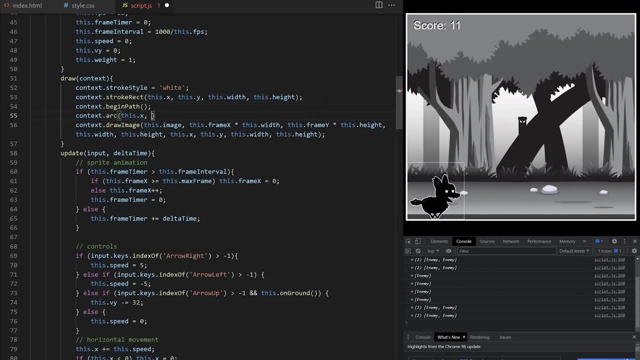 player and enemy sprites more closely than one larger shape. Some of you think that simple collision detection between circles would be enough. in this scenario, Let's try to draw circular hitboxes around our objects to see what it would look like. It's also easy to offset these circles by specific pixels. 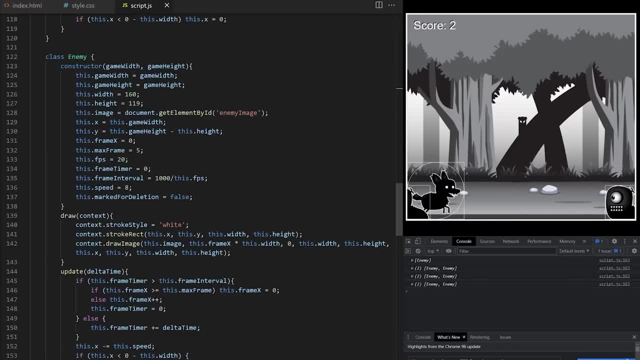 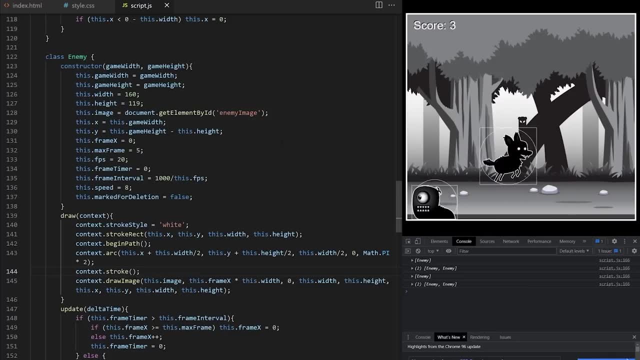 The first thing we need to do is to draw a circle around our objects. We can also make a specific pixel value horizontally or vertically in relation to player and enemy object. We can also make them smaller or larger if needed. I agree with you and I think that using circular collision detection for jump in game, like 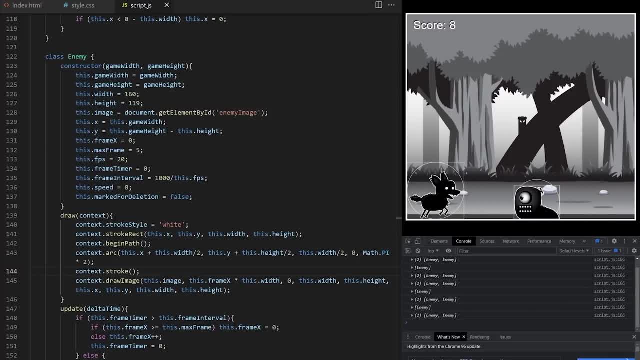 this will get rid of accidental collisions where two corners of rectangles collide. Now I need to decide where in our codebase we will run collision checks. I know I need to check position of player against position of all active enemies for each animation frame, So I might as well do it inside player. 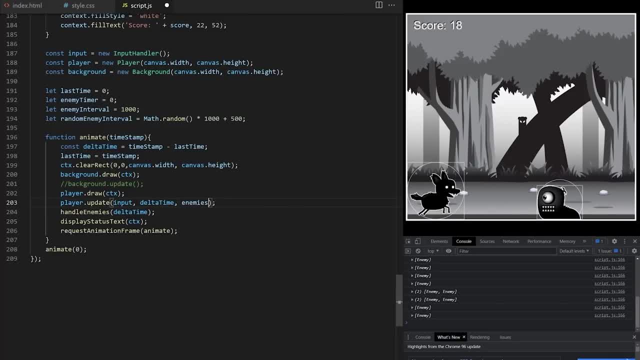 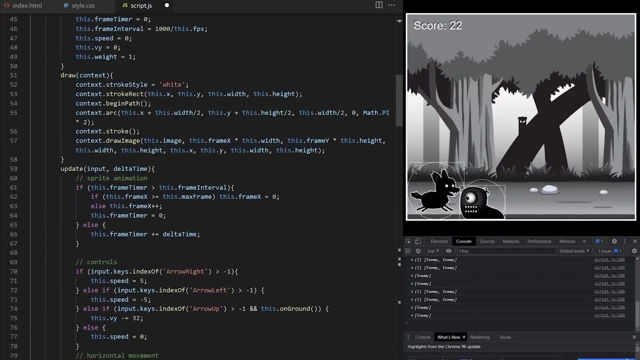 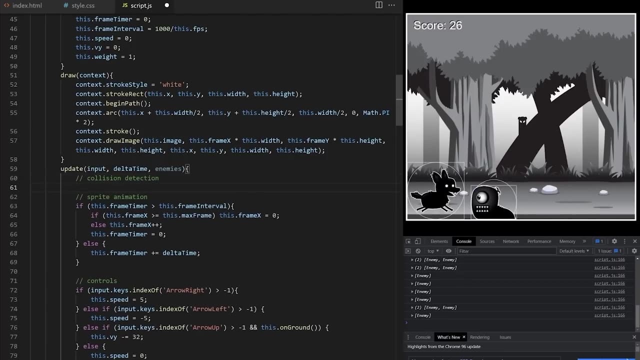 I pass it enemies array as an argument. It contains all currently active enemy objects On line 59 inside update method on player class. I make sure update method expects that argument. We will calculate collision detection here. We need to run it against every enemy object in enemies array. so enemies we passed as an. 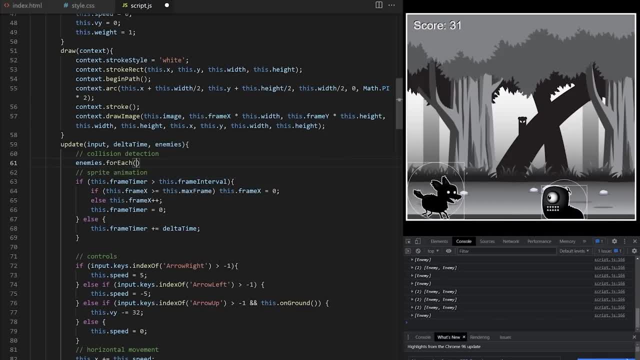 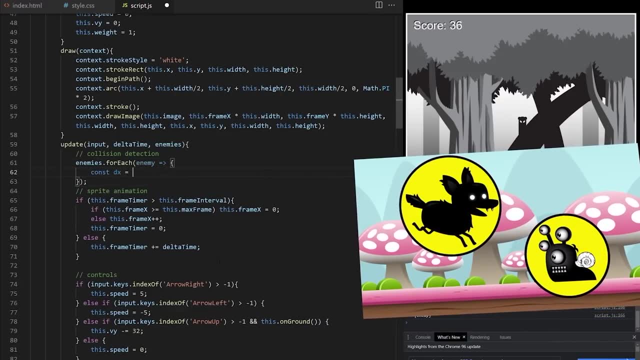 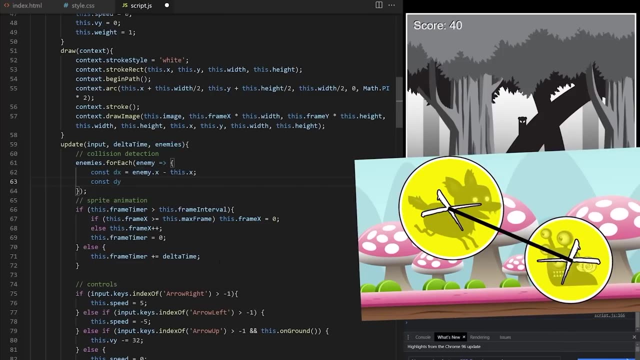 argument for each. and then I do collision detection calculation between player circle hitbox and enemy circle hitbox. To do that we need to calculate distance between center points of these two circles and we compare that distance with radius of circle 1 and radius of circle 2.. 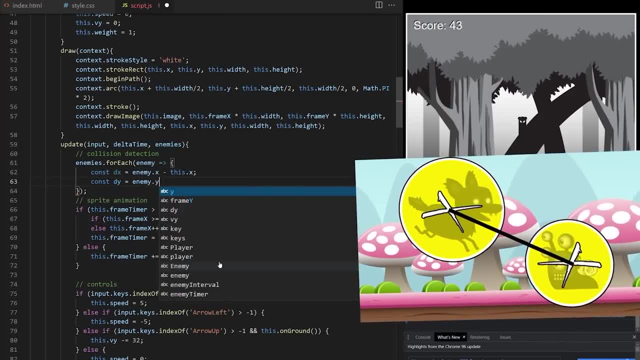 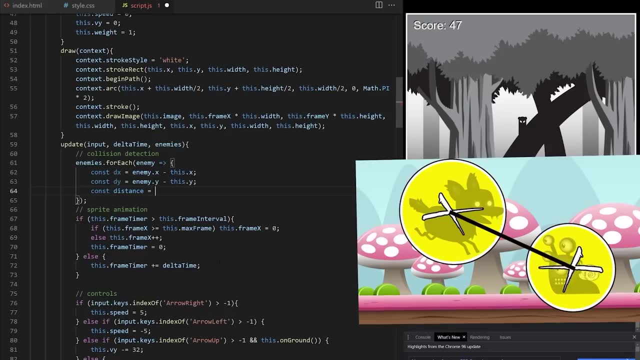 If the distance is less than these two radii added together, we know we have a collision. To get distance between two points, two center points, we use Pythagoras theorem formula. We have a center point of player circle and center point of enemy circle. 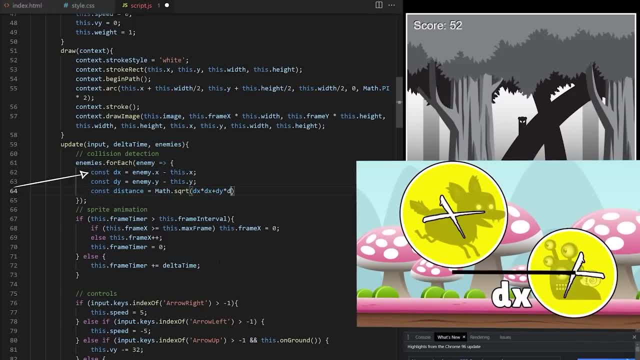 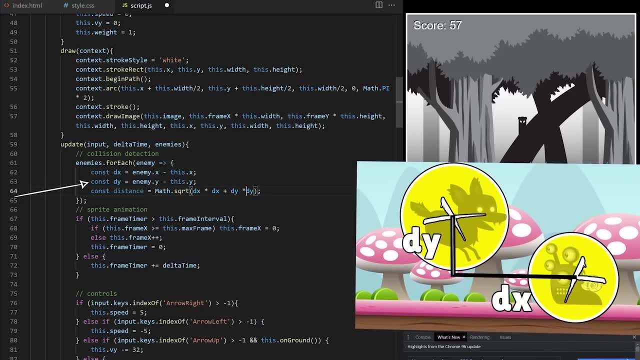 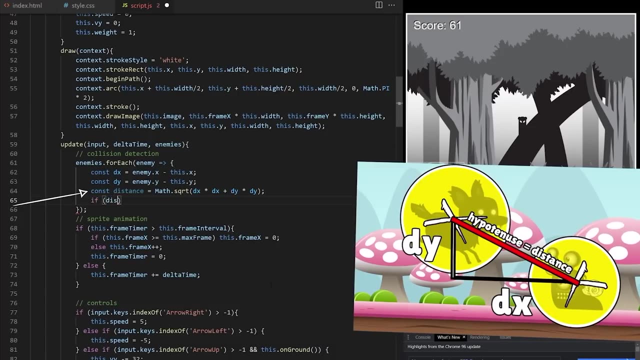 We calculate distance on horizontal x-axis dx. We calculate distance on vertical y-axis dy. It gives us imaginary right triangle and we know hypotenuse of this triangle is the distance between these two points. We calculate it as square root of dx squared plus dy squared. 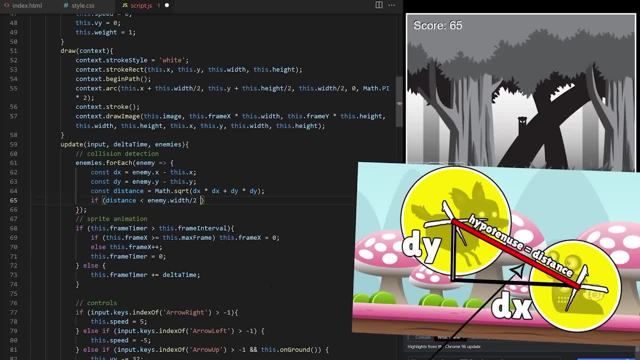 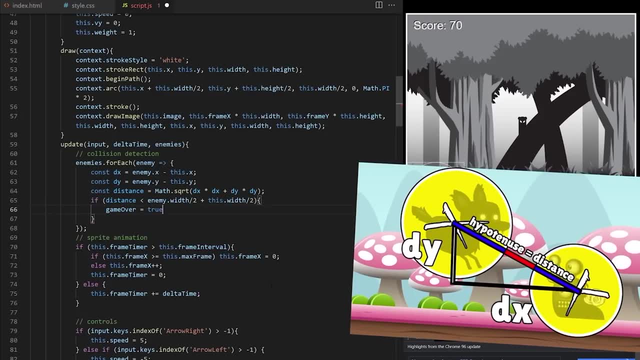 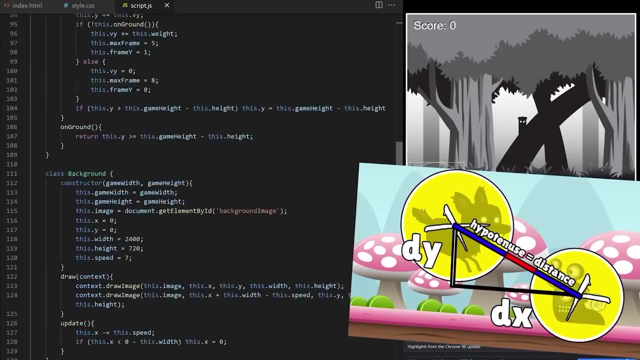 If distance between center point of player circle and center point of enemy circle is less than radius of enemy circle plus radius of player circle, we have collision and we set game over to true Up on line 8.. I create a let variable called game over and I set it to false at first. 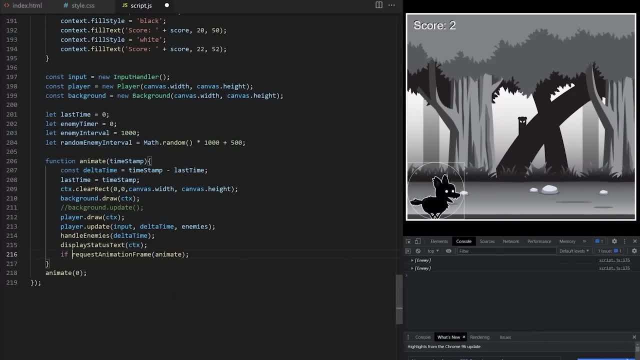 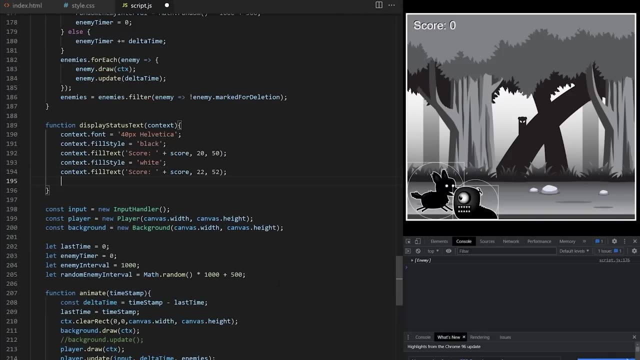 I want the game to pause when game over is true. so inside animation loop I say only run request animation frame and continue animating our game. if game over is false, You can see that when collision is detected game stops, Perfect. I also want to display game over message. so inside display status text function I say: 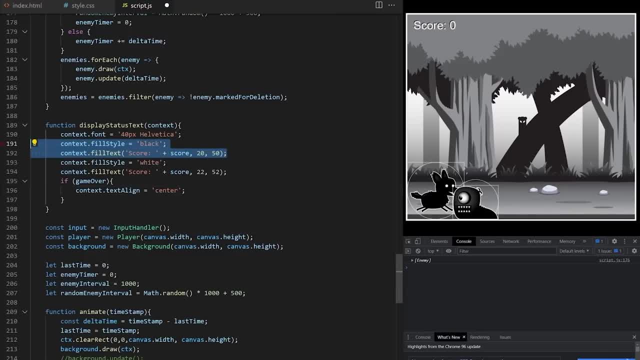 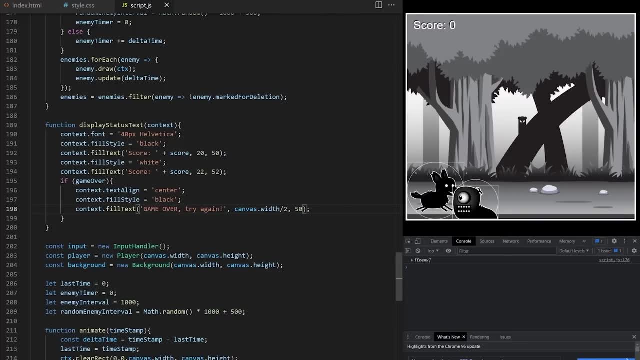 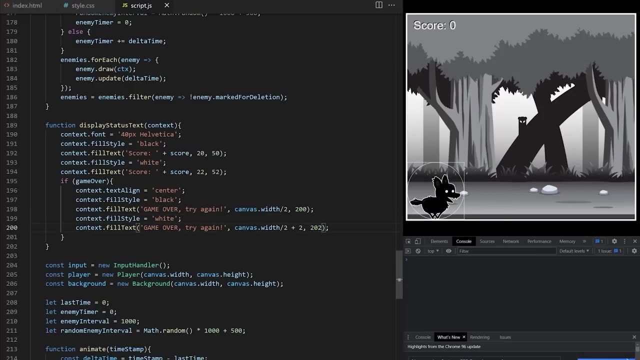 if game over is true. set text align to center. Fill style to black. Fill text Game over. try again. and coordinates canvas width divided by 2 and 50, 200.. Make a copy again. Set fill style to white and offset the second line by 2 pixels. 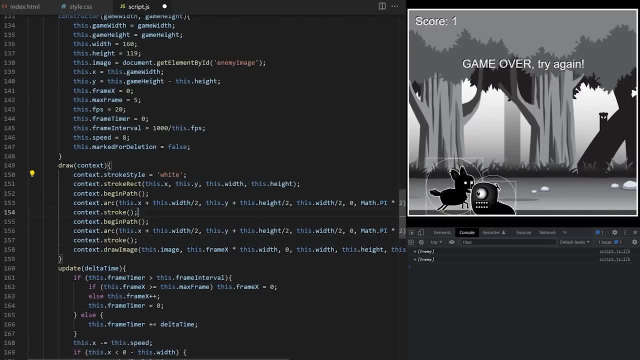 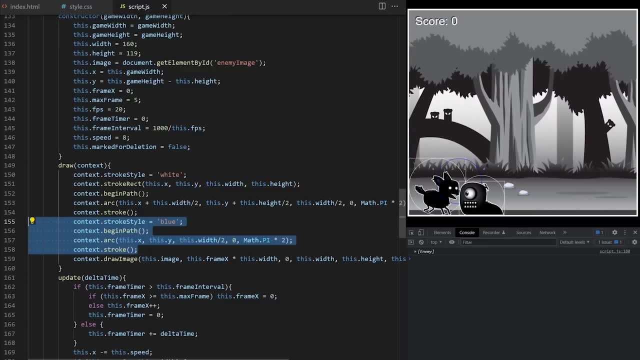 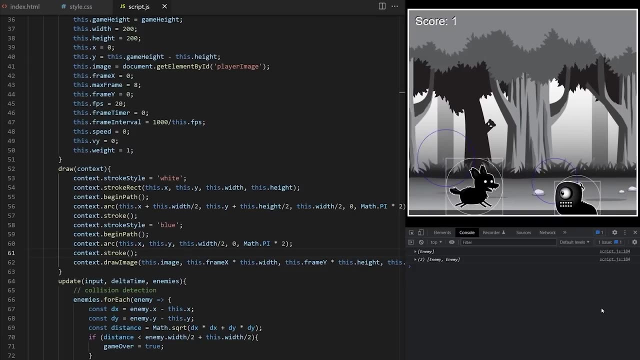 I need to fix our collision detection. We are using enemy x and enemy y coordinates as center points of collision circle, which means collision area on each enemy. is this blue circle And same with the player, Since player x and player y Is the top left corner of rectangle area from which player image is drawn? I can't set it. 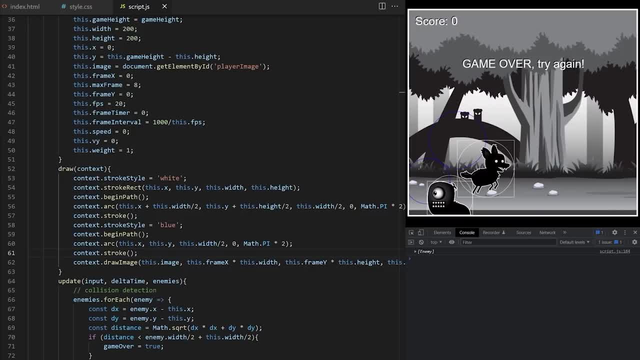 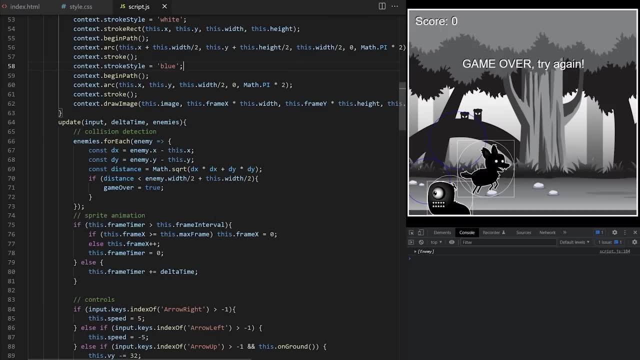 as center point of collision circle, Because I did do that. we are not checking for collisions between white circles, We are actually checking for collisions between the blue circles I just drew. The fix is simple: The x distance on the horizontal x axis between two center points needs to be offset by half. 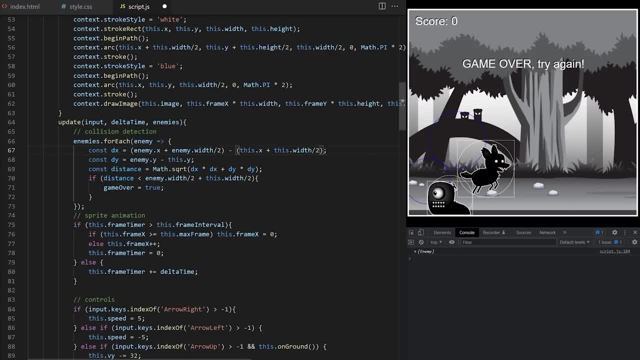 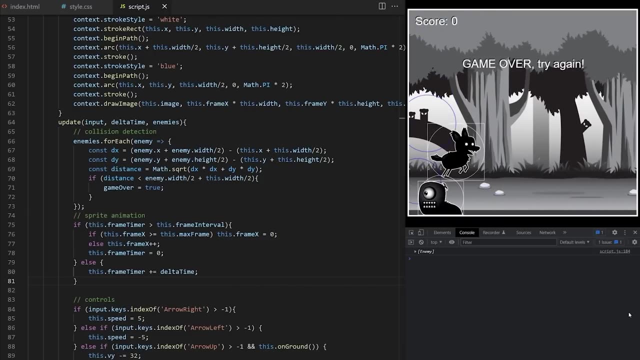 of enemy width and half of player width To move these center points from top left corner to the middle of rectangle area. Same goes for vertical dy check Brackets are very important here. Now, after this fix, collisions are correctly being detected between white circle areas. 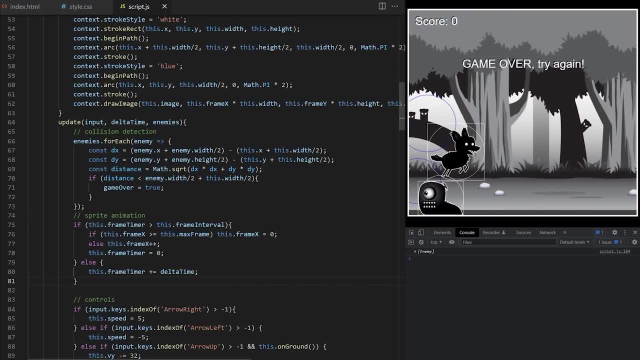 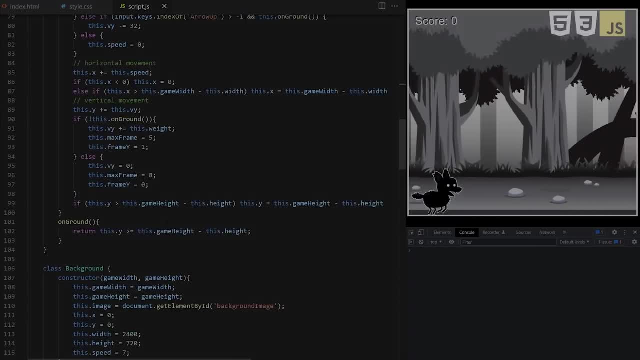 around player and enemies. I can offset these circles by a specific amount to move them around. I can make them smaller or larger. We will expand on this in the next episode. In this class we will learn how to use native javascript full screen functionality. 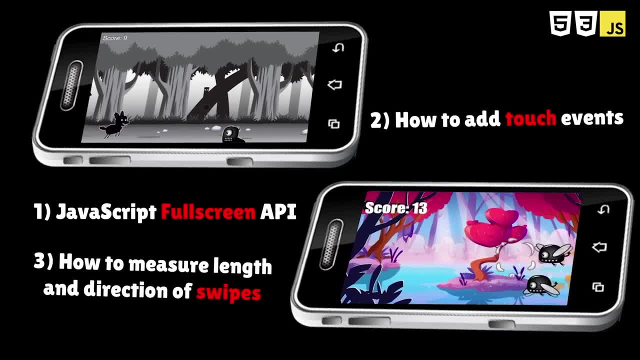 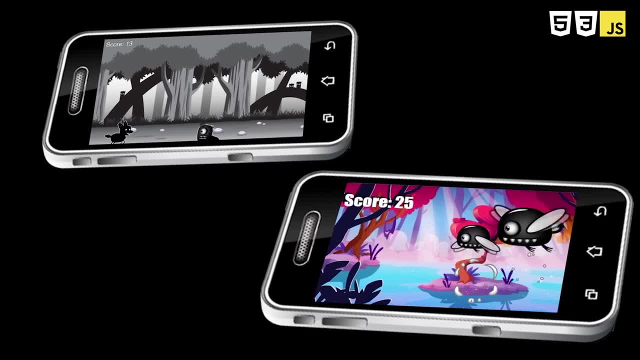 ability, how to add touch support to our games and how to measure length and direction of swipes so that we can attach specific events to them. Full series linked in the video description. Let's make a mobile game with HTML, CSS and JavaScript. 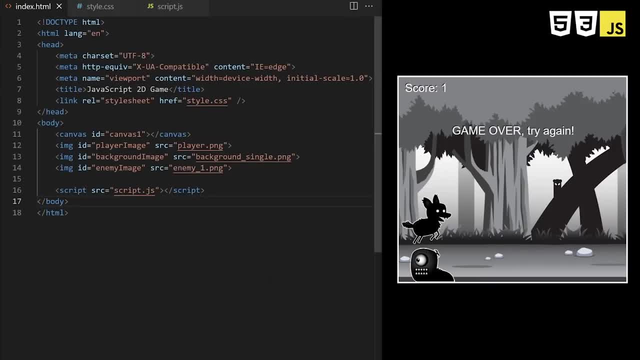 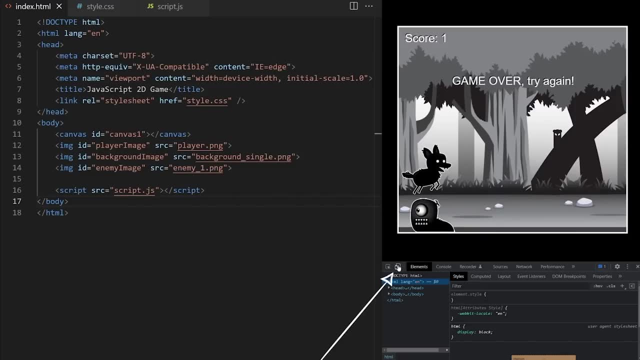 Let's go. This is the game we built in the previous lesson. I will be using Google Chrome browser as usual, and if I right click to inspect the page, we have this small mobile device icon here. This tool is great for designing responsive websites. 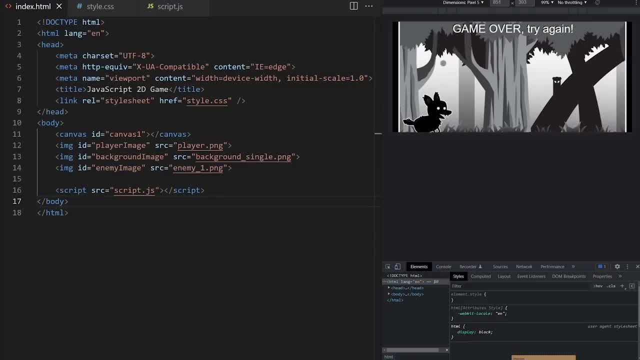 Keep in mind. this is just an estimate. There might be some differences when you run the same code on the actual device. This simulator is not 100% accurate. As you can see, Canvas doesn't even fit mobile screen on landscape Currently. this project is not mobile friendly at all. 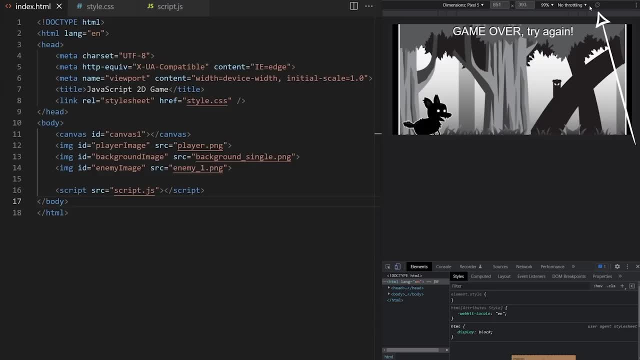 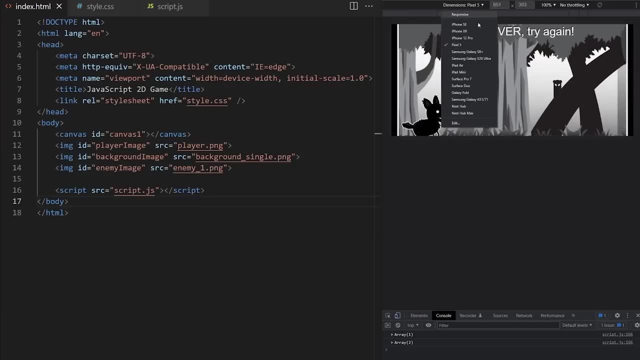 It's actually very easy to fix this. I can click this icon to toggle between landscape and portrait view. I can choose different devices from this drop down, So the first thing I want to do is to make sure we can see the entire canvas at all times. 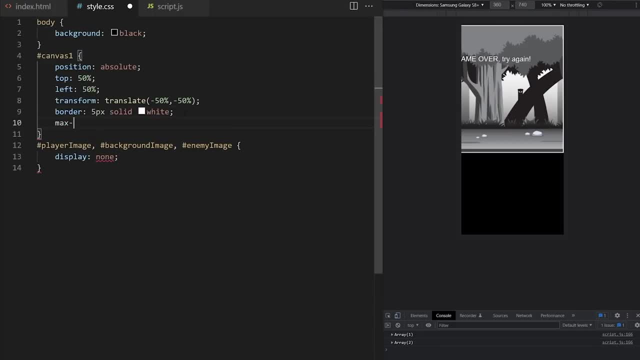 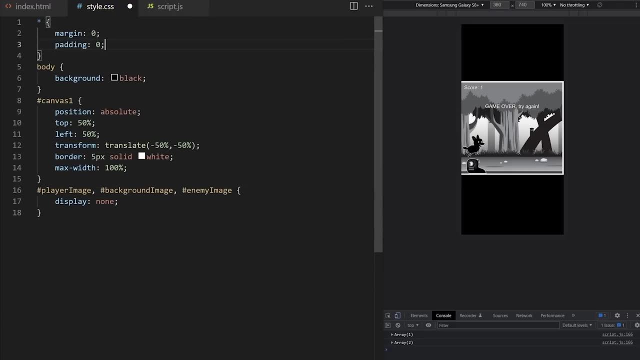 on mobile. I will do it with CSS. I give Canvas max width property of 100%. We are missing left border here. Let's reset all default margins and paddings and set box size into border box to make sure elements border is included in its total width. 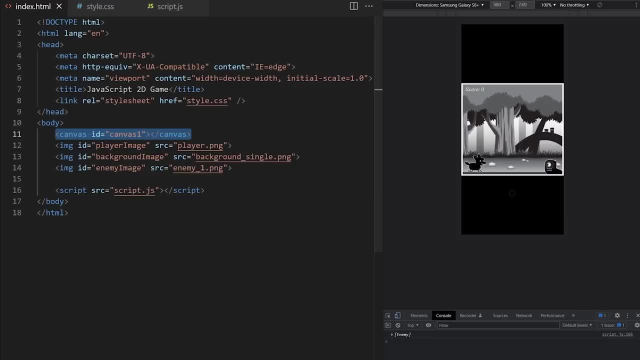 Modern CSS makes life so much easier. So now in portrait mode you can set canvas to any width and it will always scale up or down to make sure we can see all of it. I switch to landscape, No problem. How do we solve this? 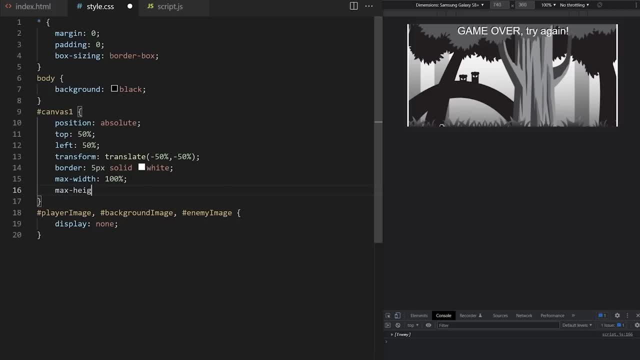 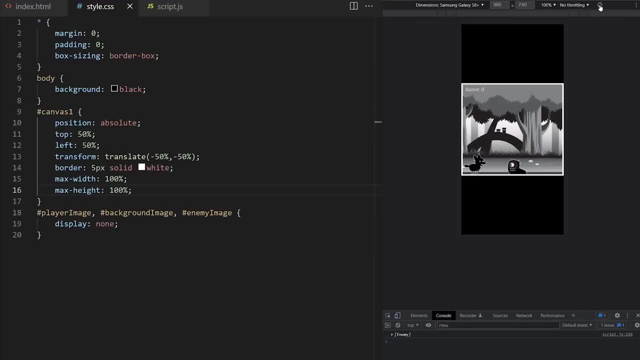 This is actually also very easy, barely an inconvenience. I give Canvas max height 100%. Now Canvas will scale until it hits edges of screen, vertically or horizontally, depending on aspect ratio. whichever boundary it hits first. Look what happens when I make Canvas wider. 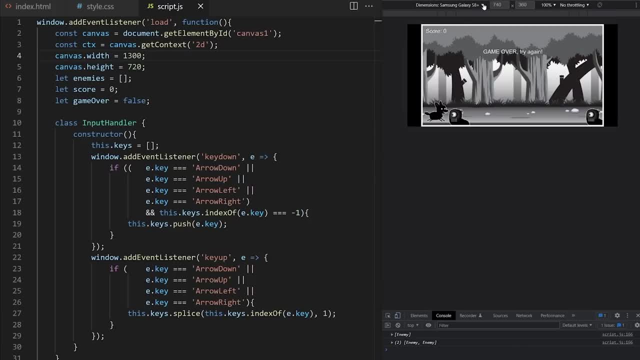 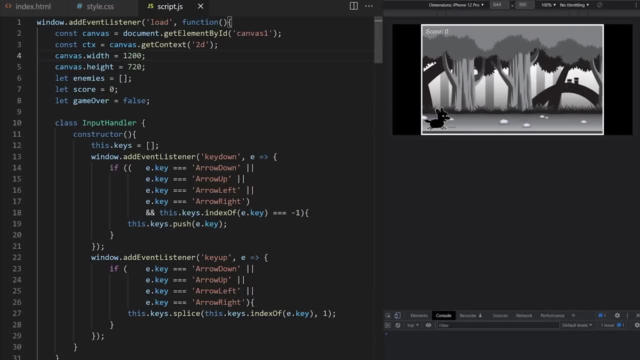 It still works. I can switch devices, toggle between landscape and portrait. We can see all of Canvas at all times, Perfect. There is also a way to make Canvas fit the entire screen with no black edges. But because of the scrolling background we are using here, I would have to calculate. 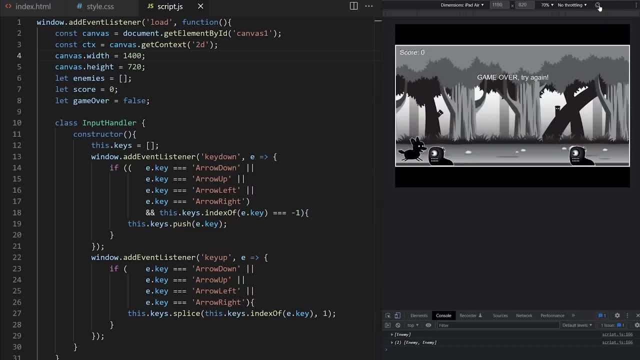 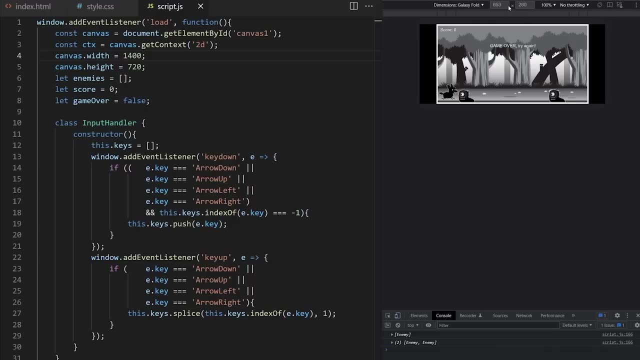 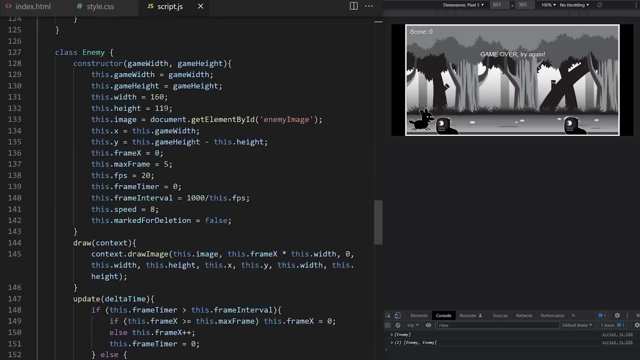 aspect ratio. I want to keep this class beginner friendly, with no algorithms, so I will get back to that in more advanced tutorial. Now you know a quick and easy way to make Canvas fit on mobile screen without stretching and distortion. The only way to restart game right now is to refresh browser window. 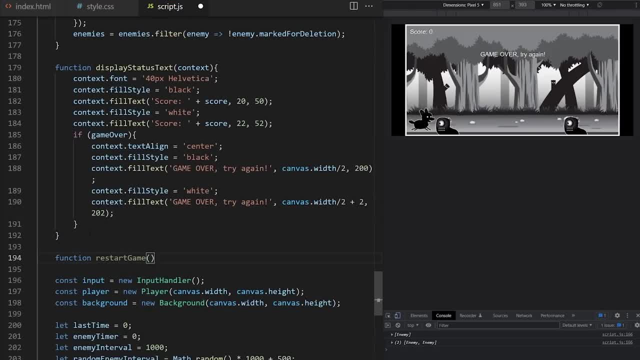 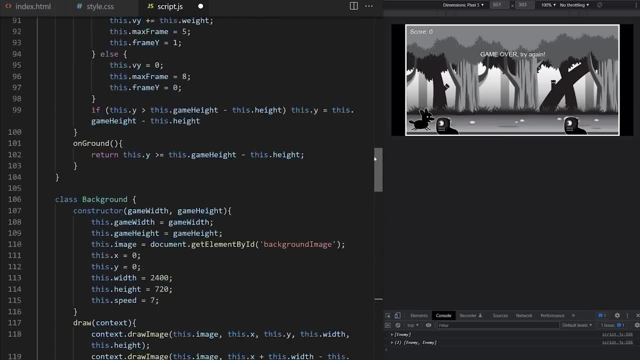 Let's write an actual restart game function so that we can connect it to buttons or key presses or touch events. We have to think What needs to happen when game restarts. Well, first we need to restart the player to its initial position. I will actually do it as a method on player class. 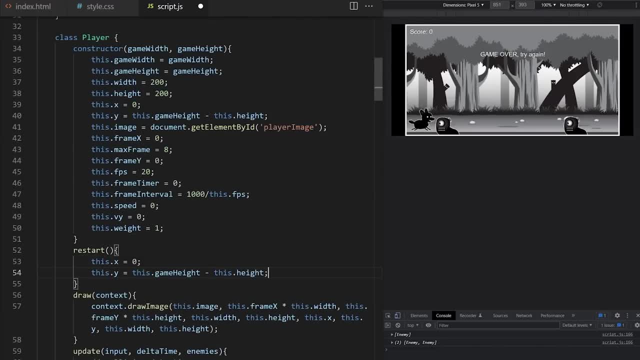 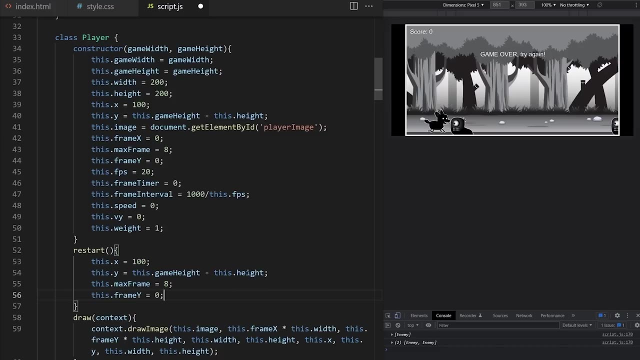 I will call it restart and inside we set X and Y to the original values. Let's move player 100 pixels to the right Here and here. That's better. After restart I want player in running animation, so max frame will be 8 and frame Y is 0.. 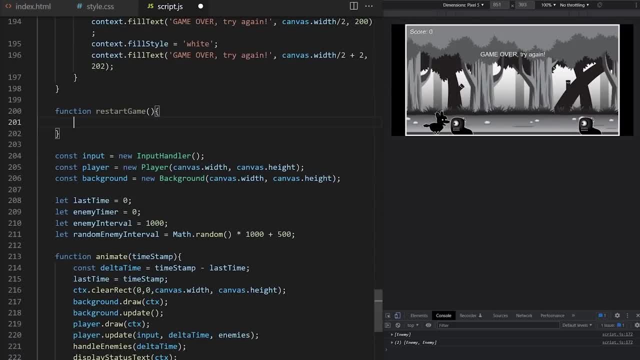 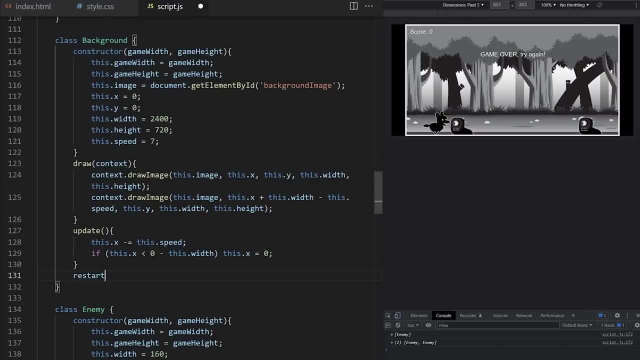 Down on line 200.. Inside our custom restart game function I take instance of player class from line 205 and I call restart method. we just wrote I don't really have to restart background, Or maybe I will just restart its exposition back to 0 so that we get some more visual. 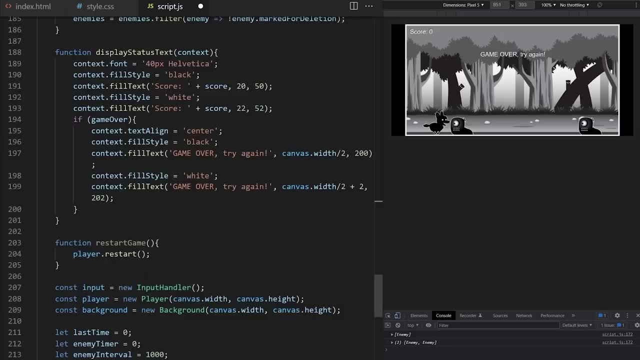 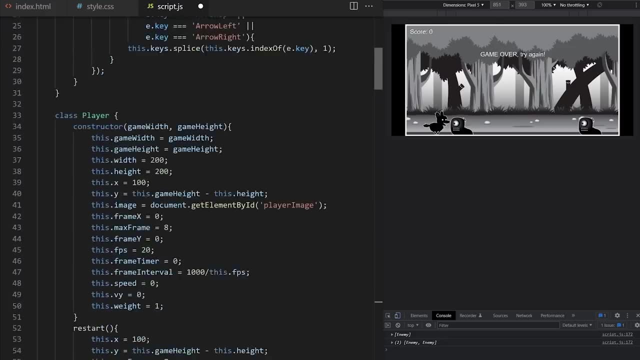 feedback that we are actually starting a new game Again. I take an instance of background class from line 210 and I call restart method. we just wrote The last thing I need to do when game restarts is to take enemies, array, score and game over. 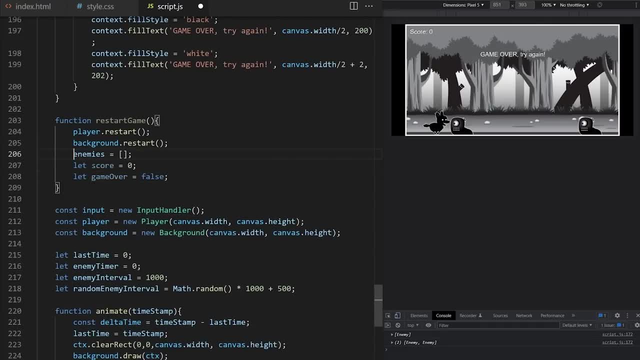 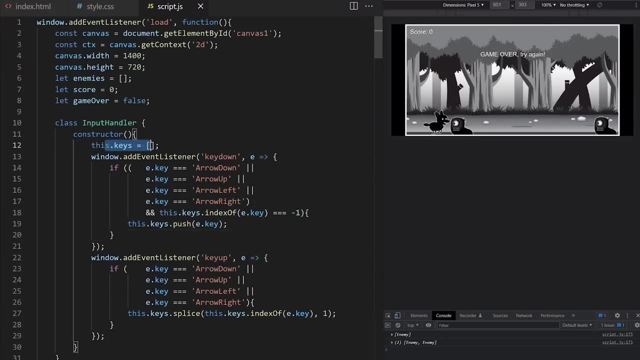 and set them back to their initial values. Notice, I am removing let keywords because I am not declaring new variables. I am just assigning new values to existing variables. Where do we call this restart game function from Here? inside event listener, inside key down event: we listen for arrows and we push them. 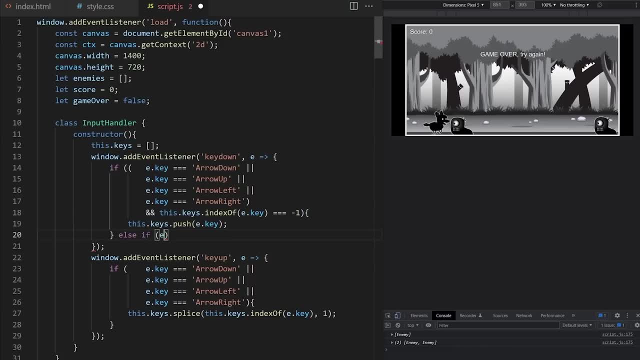 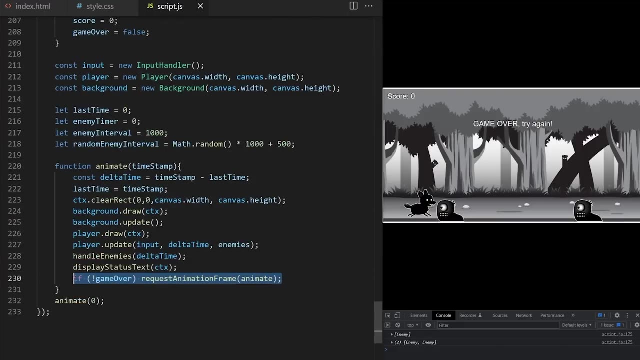 into this dot keys array, I will create an else statement. and if key that was pressed is enter and at the same time game over from line 8 is true, It is still not working and it is because when game over is true, I stop calling request. 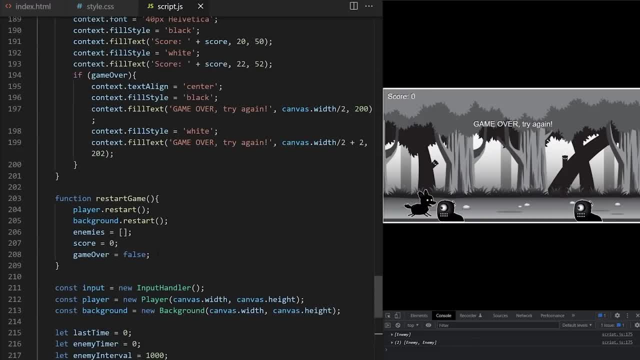 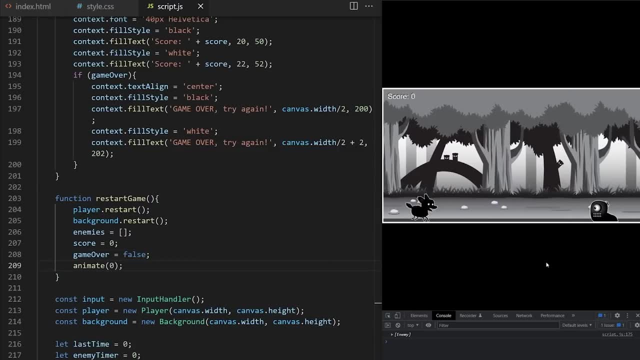 animation frame here. Since we are setting game over back to its initial false value, I can call animate again to start new animation loop. So we are playing. game is running. I get game over, I press enter and reset function resets our game. 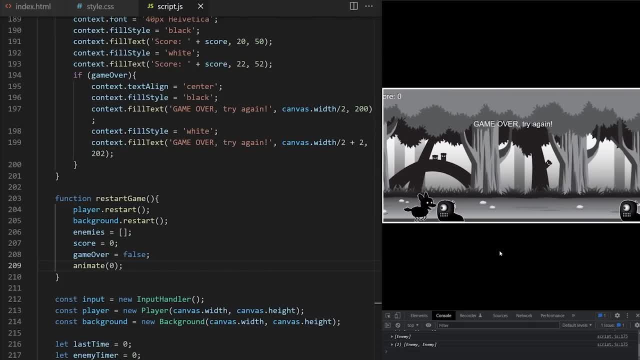 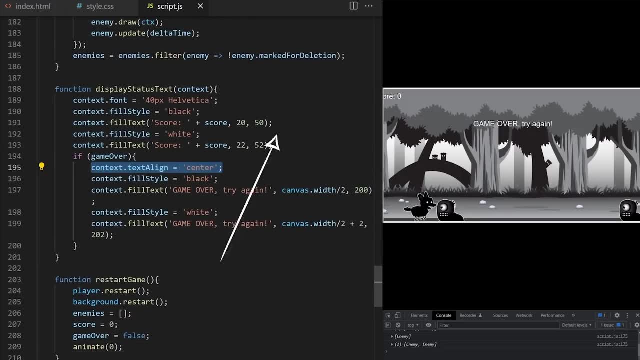 Awesome, we are doing great so far. I should tell the user to press enter, otherwise how would they know? You can see after game reset: score is off screen. it's because it's taking this text align center we used for game over message. 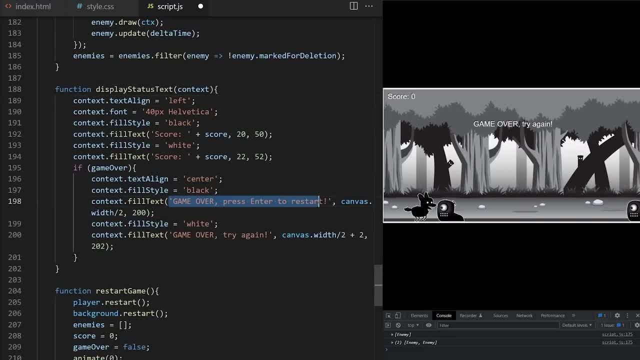 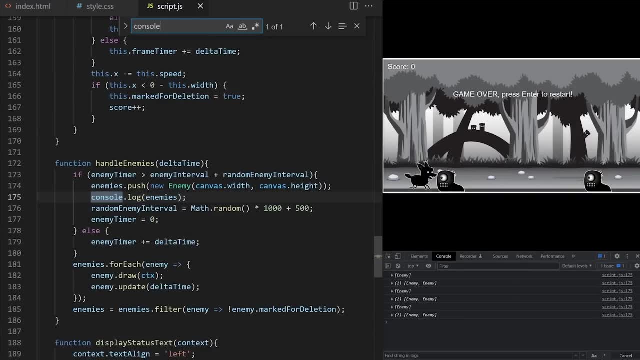 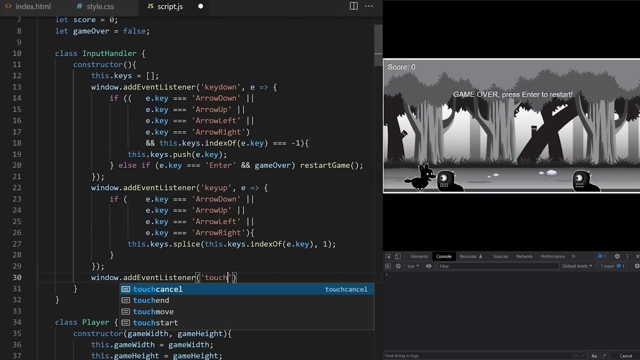 I need to set text align to left here And the message will be something like: game over, press enter to restart. This works, Ok. touch events. this will be fun. First, I remove this console log from line 175.. Up here inside input handler class, we will create new event listener for touch start. 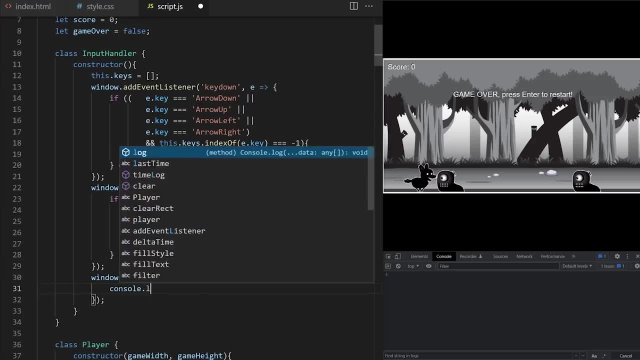 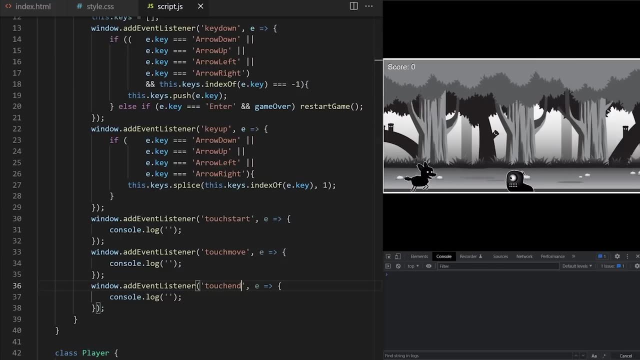 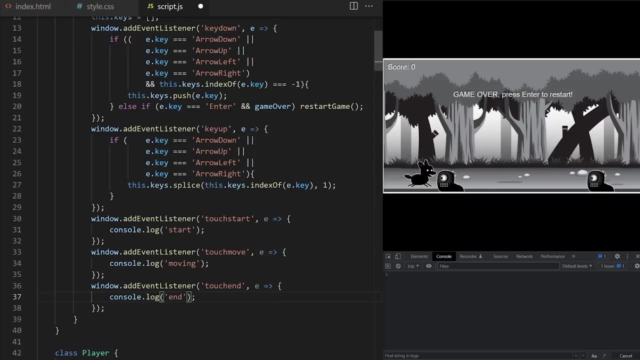 event. It will run. Now user touches browser window. When that happens I console log something. I will actually also need touch move and touch end events. I'm gonna console log start in touch start, move in in touch move and end in touch end. 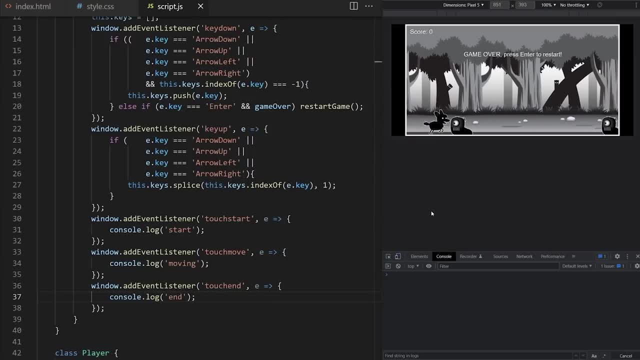 The way these work. touch start fires once as we start interacting with screen. then touch move fires over and over as long as we are moving finger over the screen and touch end just fires once when user releases the touch. This is important to remember as we have to consider these when we are structuring our 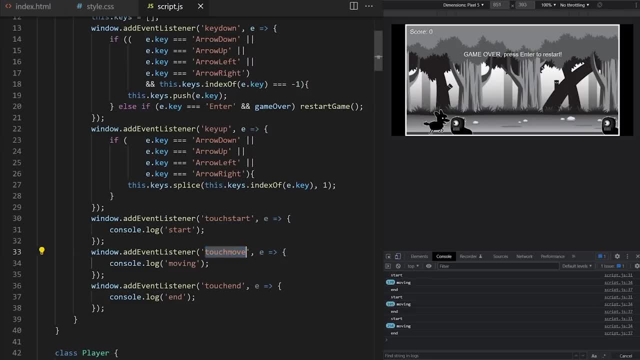 code. Code in touch start and touch end will run once and the code in touch move will run over and over as long as the event is firing. This is actually very useful and we can use touch start to set something up, touch move to make calculation such as direction and time of the event, and in touch end we do some. 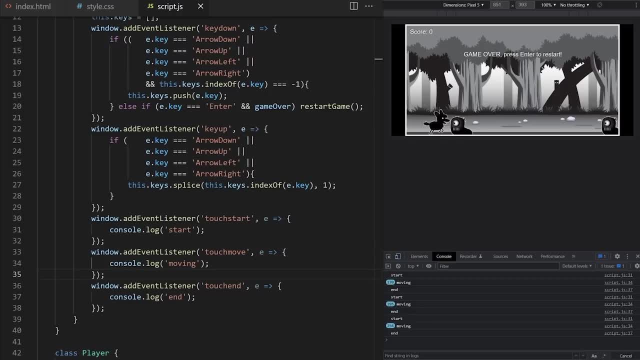 clean up and discard or reset values we don't need anymore. There is no swipe up and swipe down event, so let me show you how you can easily use these three touch events constantly. Let's have a look at autogenerated touch start event object by consolelogine. 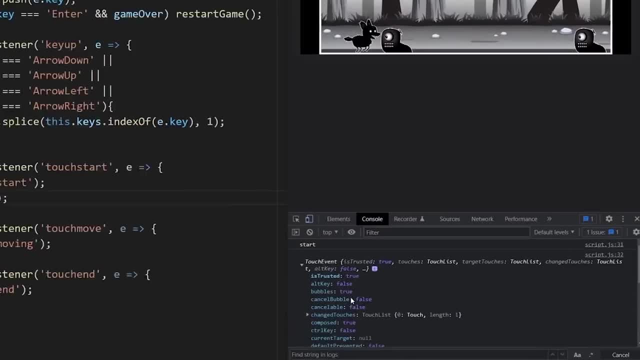 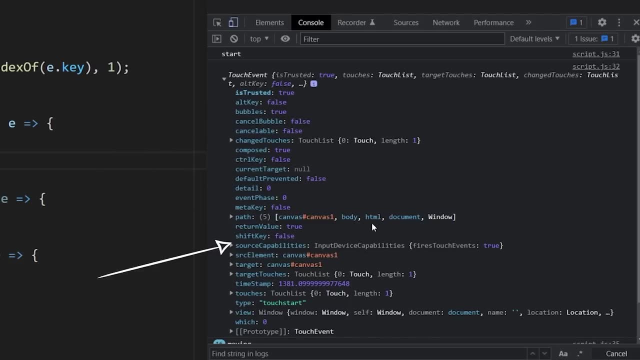 When I touch screen, this event fires and I can inspect it. There are many useful values here. for example, it keeps track whether alt and ctrl keys were pressed at the time of the event. We have timestamp of the touch here very useful. and the main thing we care about is 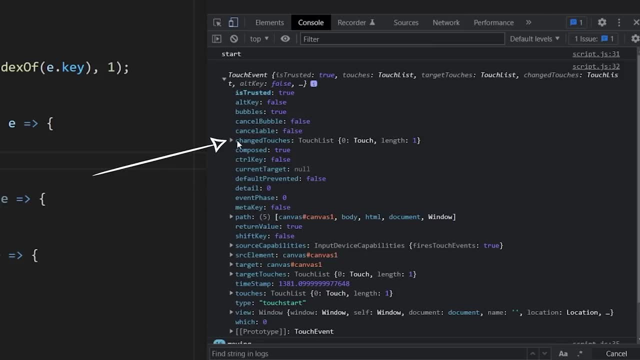 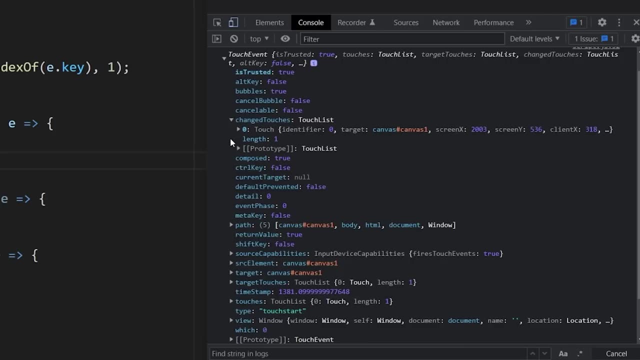 x and y coordinates of the touch. X and y coordinates of touch event are stored inside this read only changed touches property. It's actually very useful. It's a list that stores autogenerated touch objects that contributed to this touch event. With touch start event we get just one object, so we have to open index zero and here we 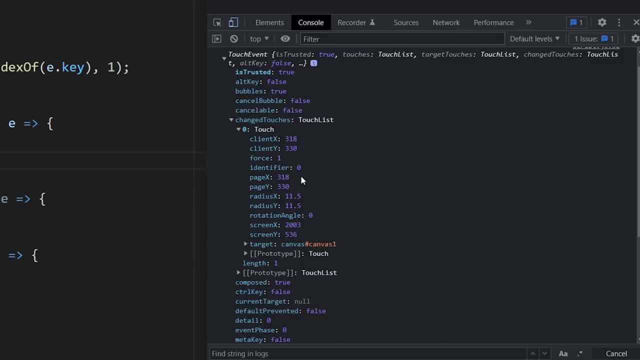 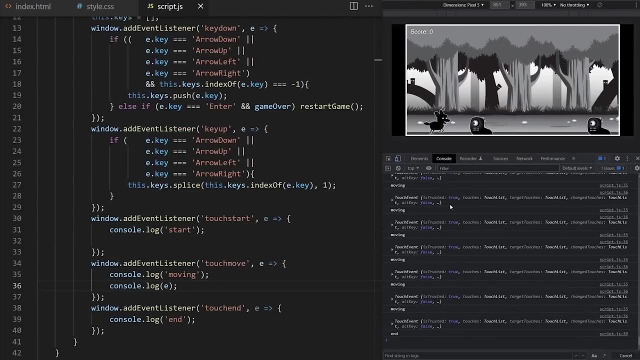 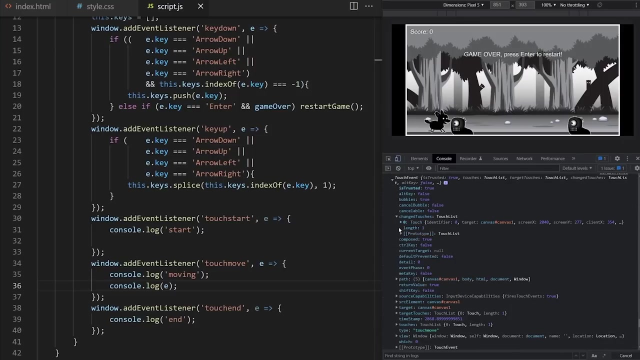 can see page x and page y properties. Perfect, we know where on screen this touch event started. If I consolelog touch move and I swipe across my screen you can see that event fires many times. Let's go to one of the ones at the start. if I check inside, changed touches list at: 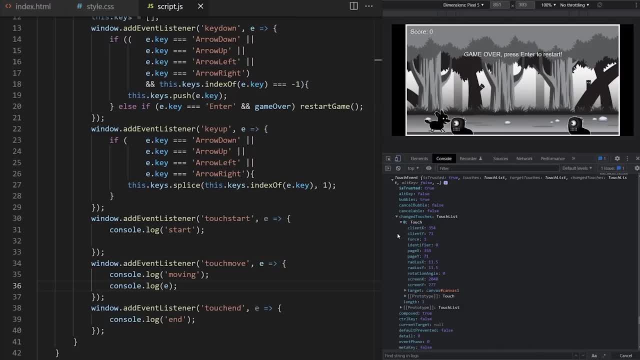 index zero. I can see page Y is 71.. As I was swiping, the event was firing, so let's go to the last time it fired. and here I see page Y is 104.. I know this particular swipe went vertically. 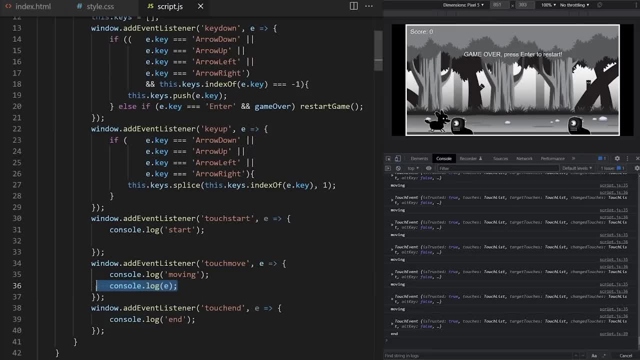 from coordinate 71 to coordinate 104.. We have all these values. we need to determine whether user swiped up or down. I put this console log into touch start event and I remove all other console logs To access vertical coordinate of touch event. 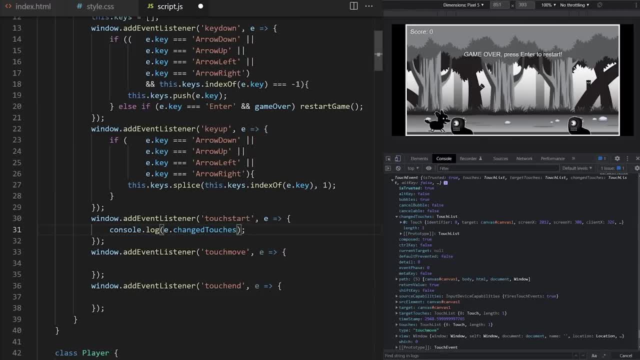 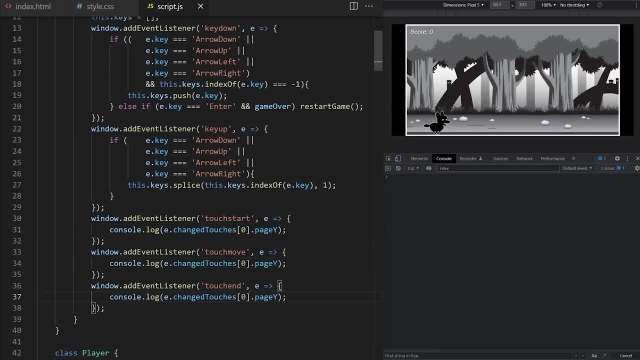 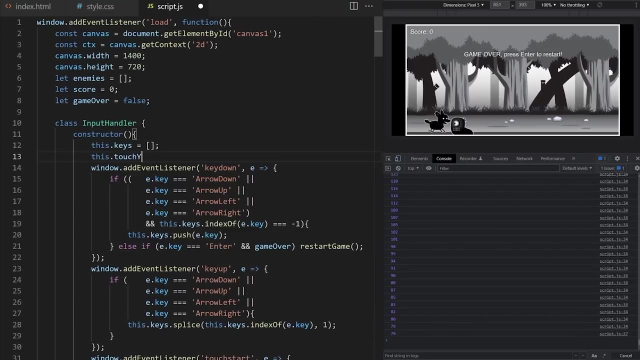 I say EchangedTouches index zero, because this is a list and I want this page Y property. Okay, let's put that inside: touch move and touch end. I create a new property on input handler class. I call it, for example, touch Y. 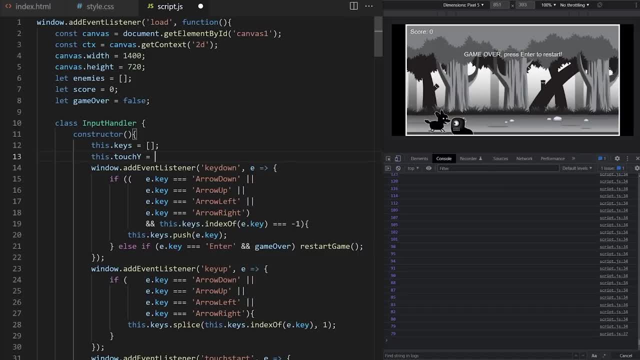 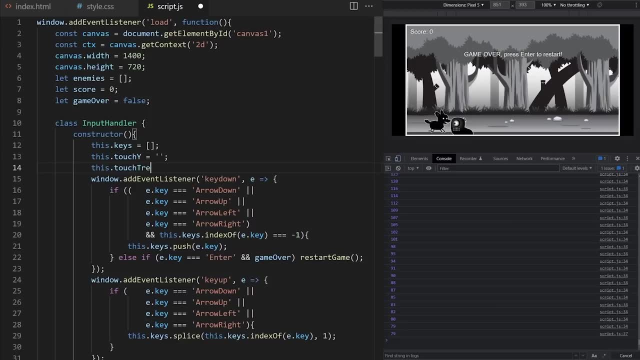 It will store the initial starting vertical coordinate. Maybe I also want the game to only react to longer swipes, to make sure user actually swipes and the game doesn't accidentally react to simple short taps. I will call this property touch threshold and I set it, for example, to 30.. 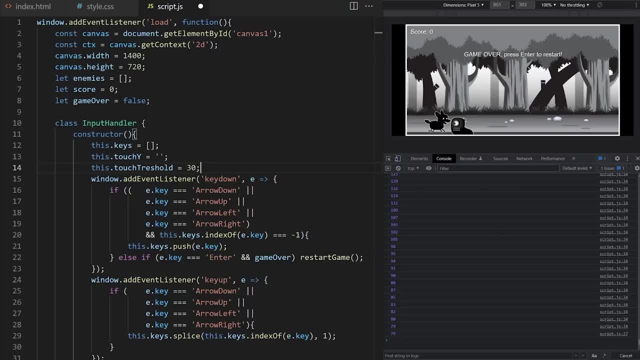 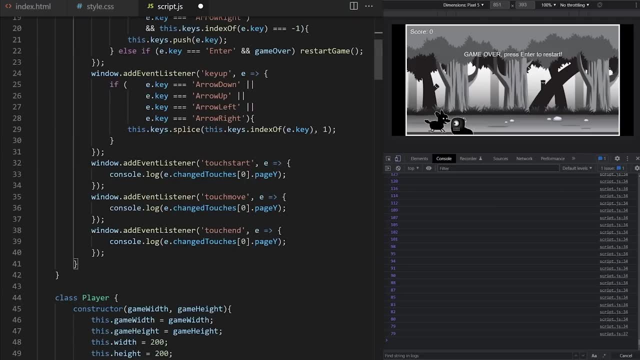 I wanted the starting touch point and the ending touch point to be at least 30 pixels apart to trigger the event. I could also make the player jump higher here based on how long the swipe is. This technique is easy and very powerful if you are designing mobile games. 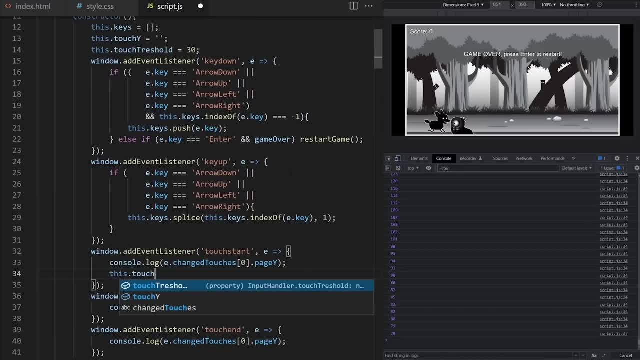 I hope you are realizing the potential here In touch start event. I just want to set starting coordinate. so thistouchY from line 13 is equal to page Y value from this event. Let's delete all these Inside touch move. I will compare current coordinate. 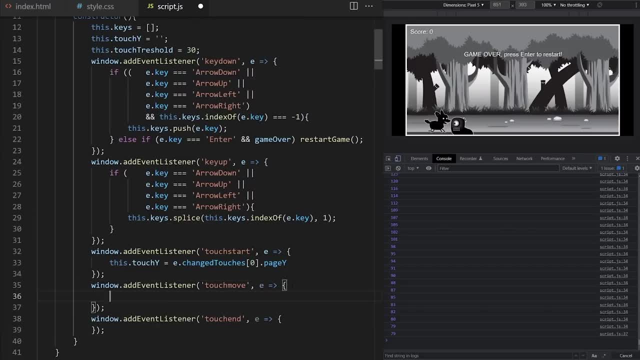 and starting coordinate to determine direction. So let's have a temporary helper variable, called for example swipe distance, and set it to page Y, value of this tick of touch move event minus the initial starting vertical coordinate, So minus thistouchY from line 13.. 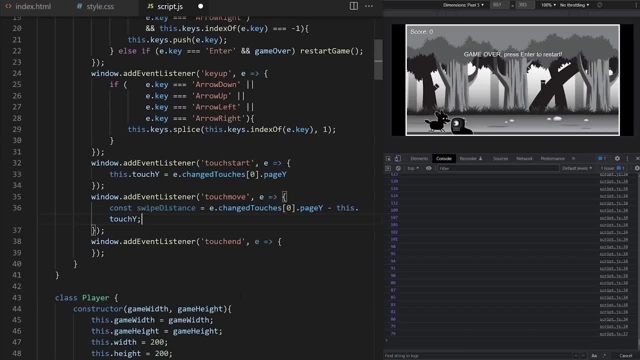 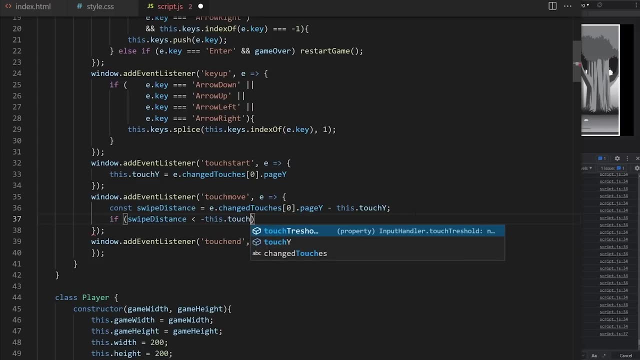 Keep in mind that touch move fires over and over again as long as user is swiping. I need more space here. If swipe distance is less than minus thistouch threshold from line 14, so minus 30, we are swiping up. 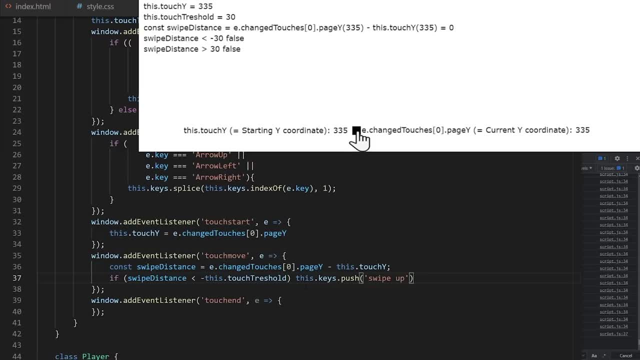 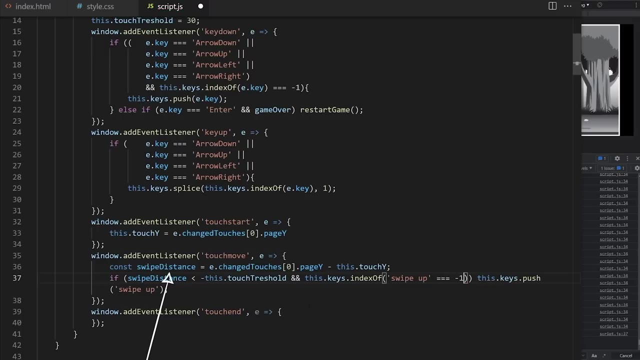 So thiskeys push swipe up. This might be a little bit difficult to visualize for some of us, so here's some animation, if it helps. At the same time, I want to check if swipe up is not yet in the keys array. So this is the distance between current vertical coordinate. 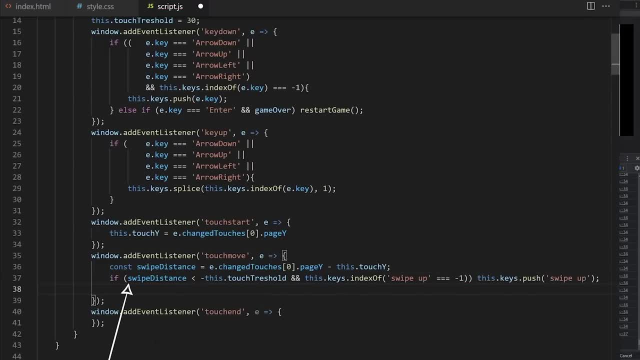 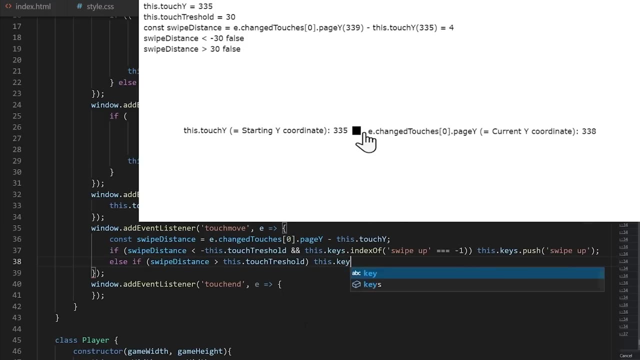 and starting Y coordinate. If this swipe distance is less than minus 30 and swipe up is not yet in keys array, push swipe up into keys array Else. if swipe distance is more than thistouch threshold- so plus 30, push swipe down into thiskeys array. 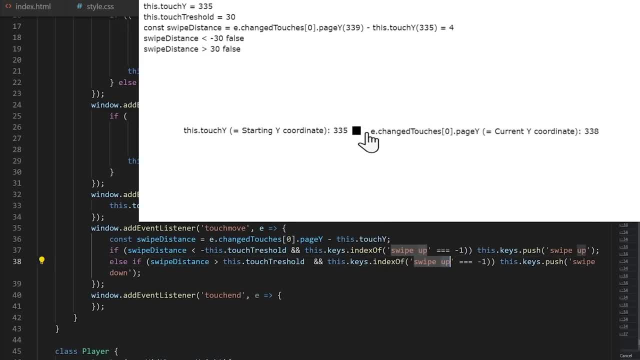 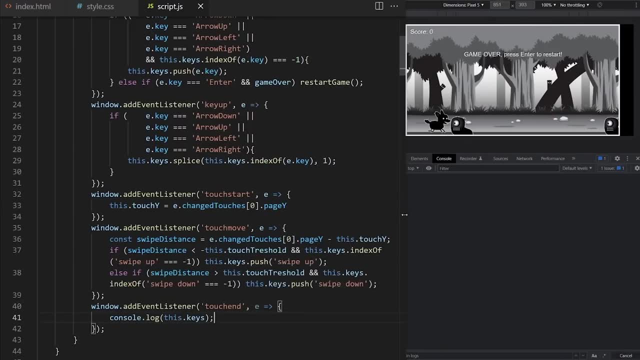 Also here. I need to check that swipe down is not yet in the array before I push it in there. I don't want duplicates of the same value In touch end. I just console log thiskeys. I can see we are getting many duplicates in the array. 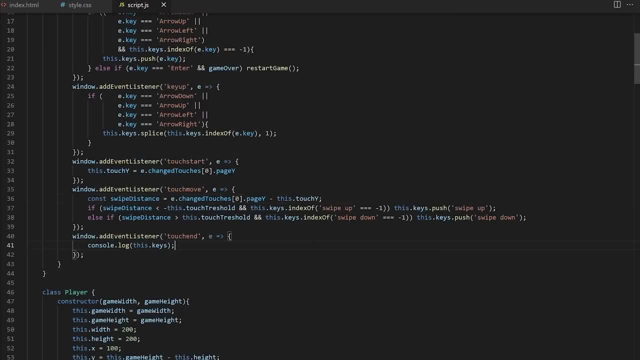 so something must be wrong here. I zoom out a bit so I can see the whole thing on a single line. These brackets need to be here. Brackets are important. It's easy to make a mistake and even a small thing can break the entire project. 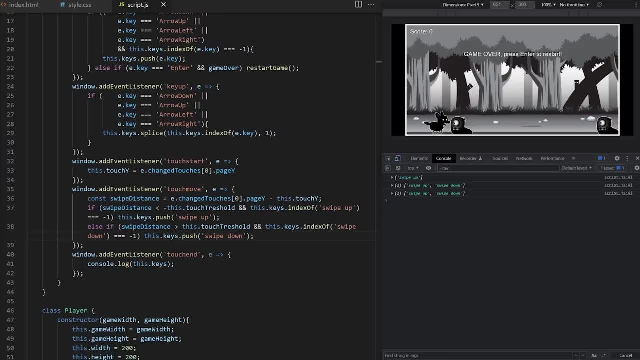 That's programmer's life: Attention to detail and debugging- Perfect. Now it gets added only once per value. As I said, I will use touch end event for cleanup. I will use splice method to find swipe up in keys array and remove it. 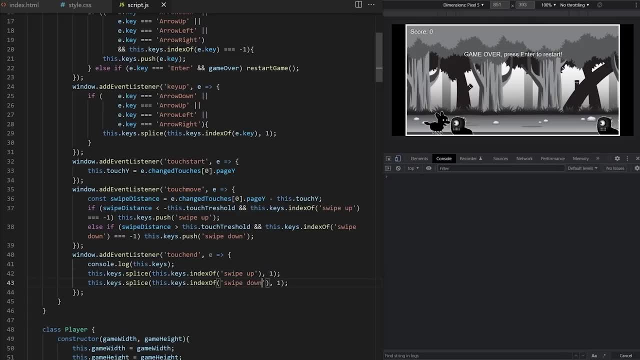 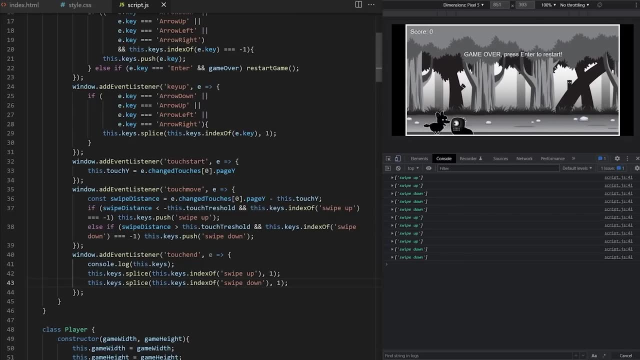 And I do thiskeysarray. I do the same thing for swipe down. So in touch start I save initial vertical coordinate of touch event. In touch move I compare starting vertical coordinate to the current vertical coordinate to determine whether user is swiping up or down. 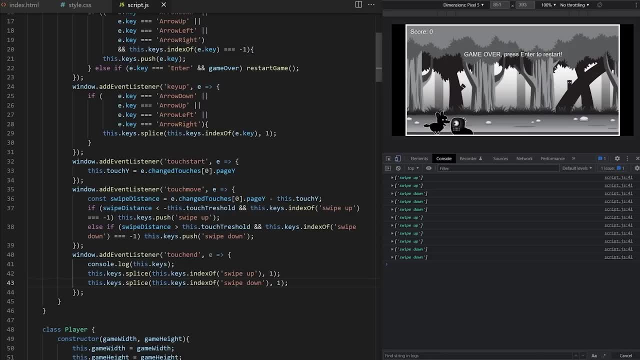 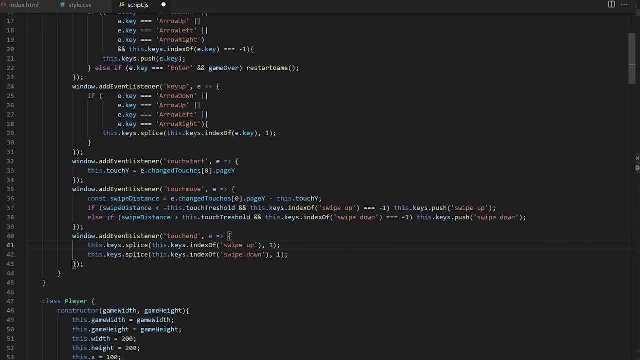 And in touch end I clean up and remove all touch events from our custom keys array. Let's remove this console log. I want to restart game when we swipe down. I might as well put it in here, Why not? So if we swipe down, callkeysarray. 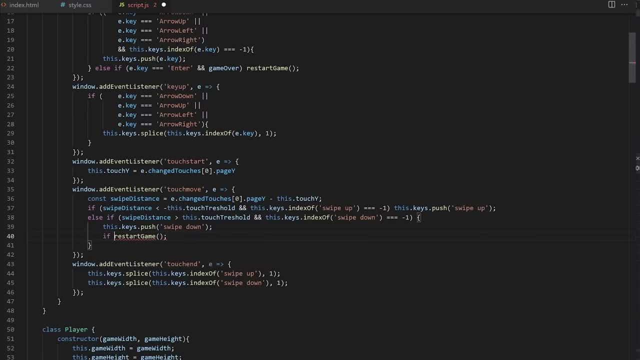 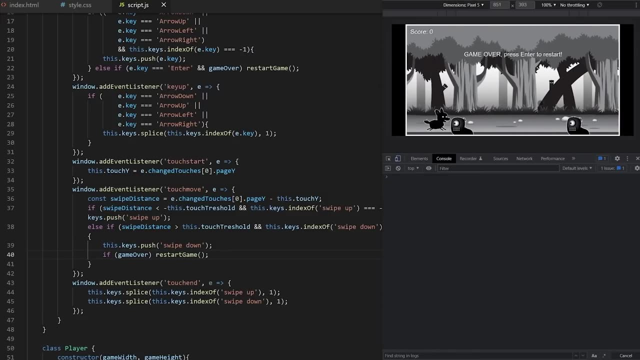 And now we have our custom restart game function. we wrote earlier, But only do it if game over is true, like this. So I get game over, I'm swiping up, Nothing happens, I swipe down and game restarts- Great. 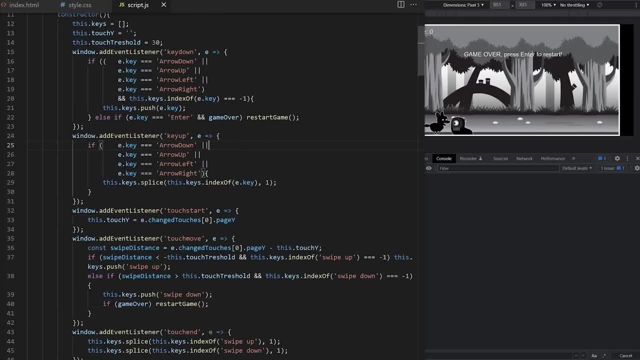 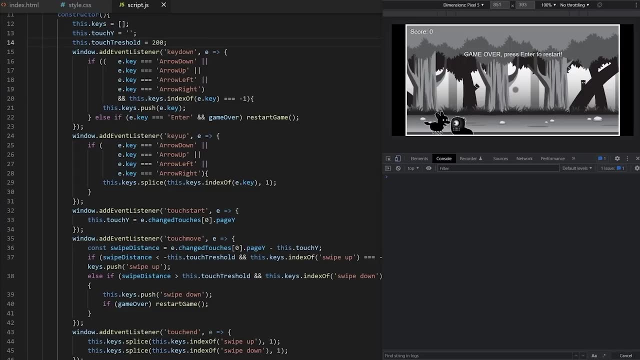 I can increase touch threshold if I want some functionality to work, only with very long swipes. I set it to 200.. I swipe down, but only short. Nothing happens. Longer swipe, still nothing. I have to swipe up Almost the entire screen from top to bottom. 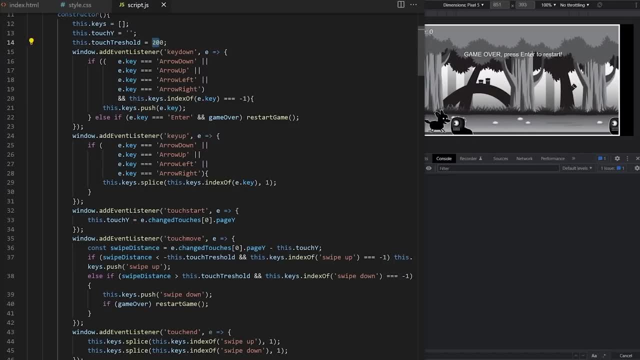 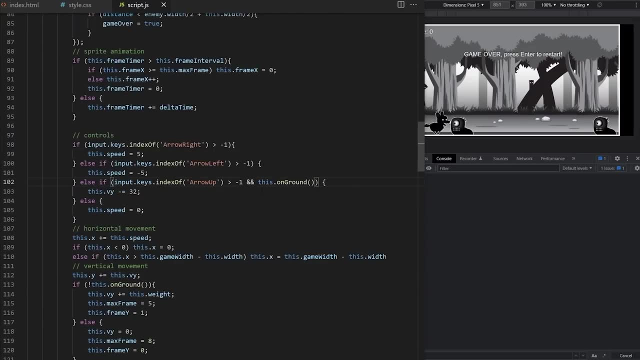 to restart game now. So let's put the threshold back to 30.. I want player to jump when we swipe up. So here inside update method on player class. I put this part in brackets because I wanted to evaluate first If keys array contains arrow up or if it contains swipe up. 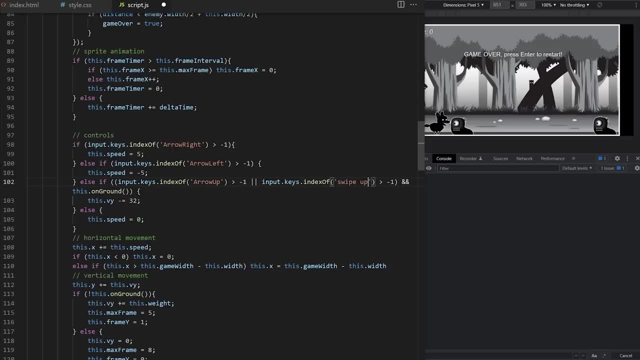 and at the same time, if player is on ground, make player jump. Be careful about brackets. It's easy to create a bug here. If you forget one, Let's see Reload game. I run, Swipe up and player jumps. 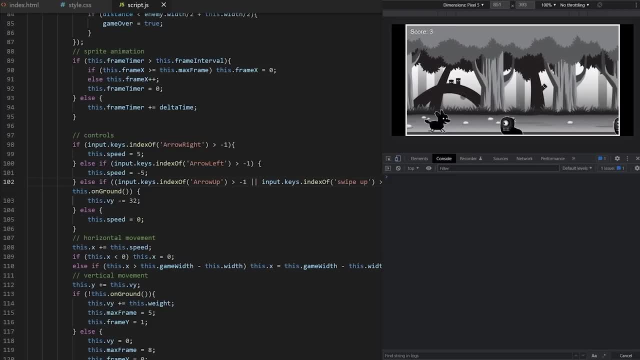 I swipe again and again. This works. Touch events work really well with simple games like this. In the next episode I will create a game with more complex moves and special abilities. Game like that is a bit more complicated when it comes to touch events. 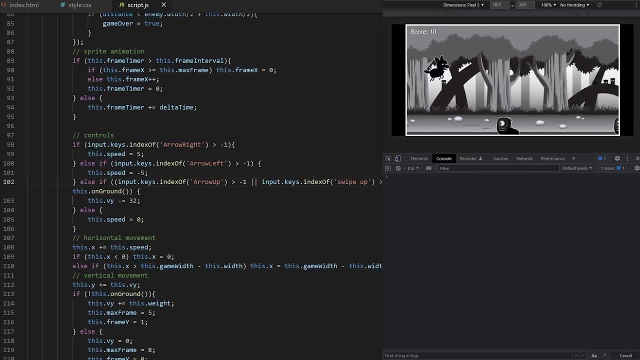 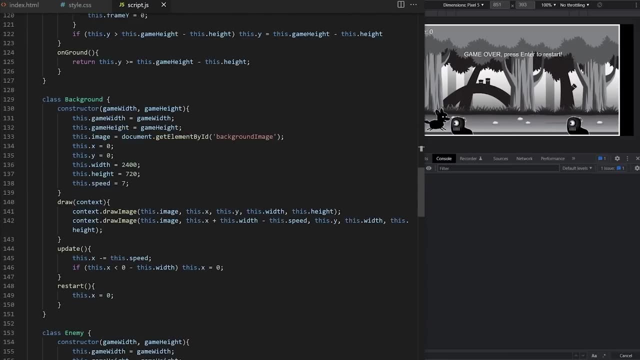 Also in most cases, to make a mobile game like this work, you should resize your art assets. My player's sprite sheet has frames 200 times 200 pixels. That's massive for a mobile game. And if I had many animated objects on screen? 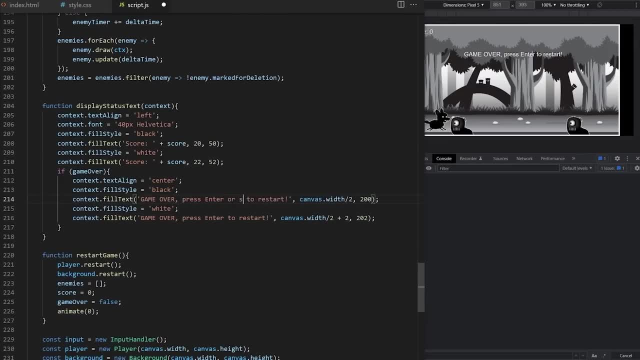 at the same time it would start lagging very fast. For a bigger game I would have to create two or more sets of art assets for different screen sizes. Let's change game over message so that user knows we can now swipe down to restart. 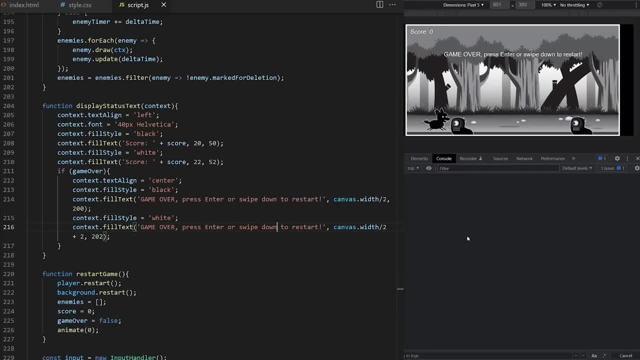 JavaScript also offers built-in native full-screen API that's easy to use. It's now well-supported in all modern browsers. As far as I know, only Internet Explorer and more mobile version of Safari don't fully support it. We are web developers here, so I'm 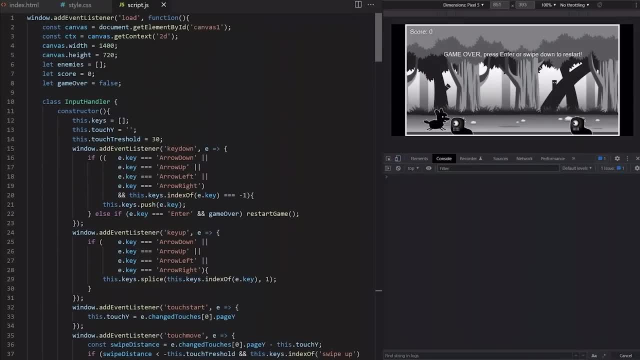 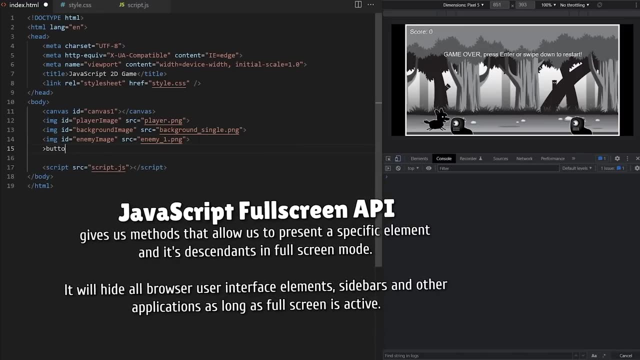 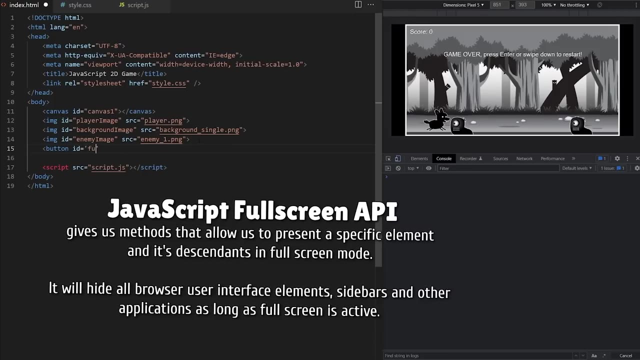 sure all of you use updated version of a modern, secure browser on your machine. Full-screen API gives us methods that allow us to present a specific element and its descendants in a full-screen mode. It will hide all browser user interface elements, sidebars. 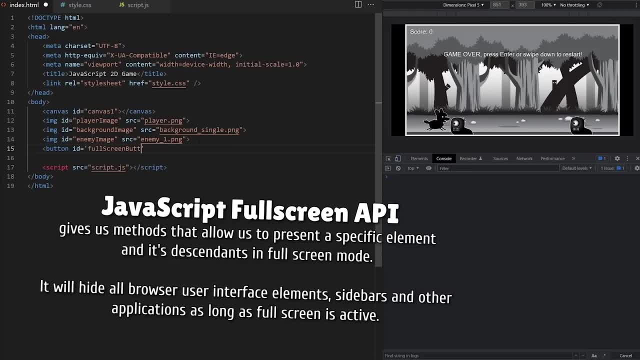 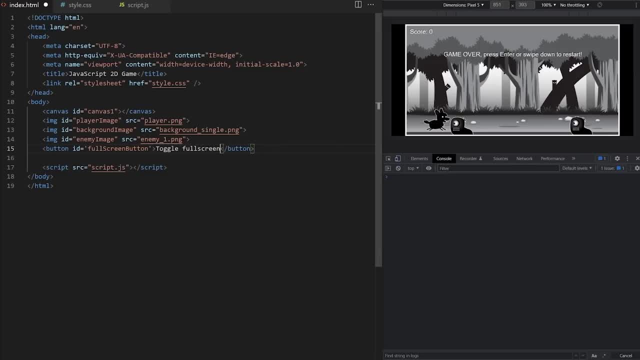 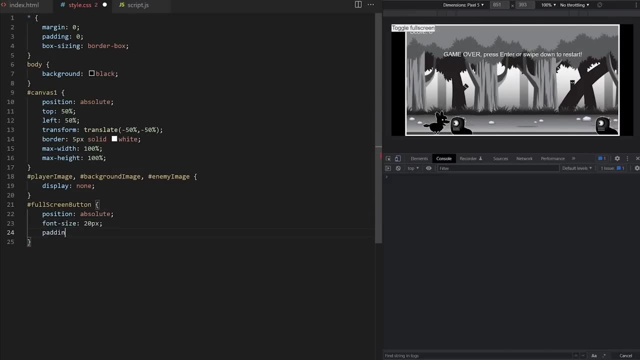 and other applications as long as full screen is active. Let's create a button to toggle full screen. I give it ID- full screen button, For example, and it will say toggle full screen. In CSS I give it position: absolute font size: 20 pixels. 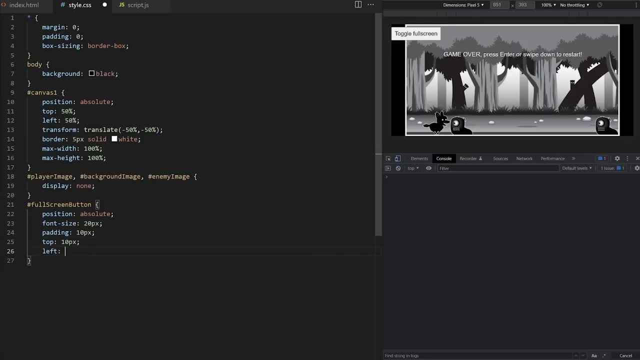 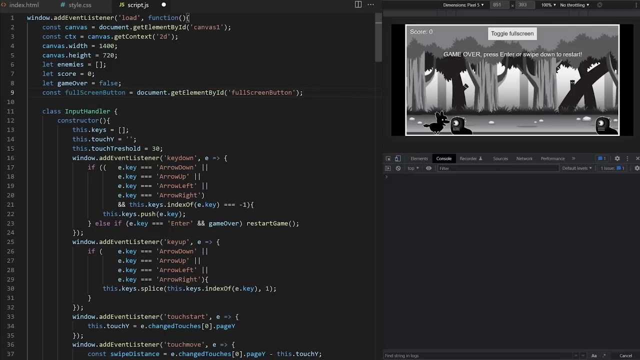 padding 10 pixels, top 10 pixels and transform, translate X minus 50% to center it horizontally. I bring it to my JavaScript project. using get element by ID, I create a new function. I call, for example, toggle full screen. 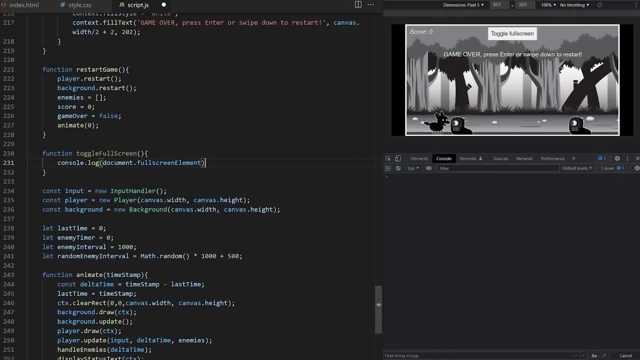 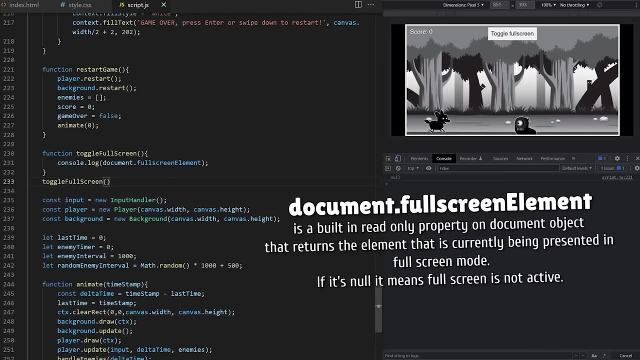 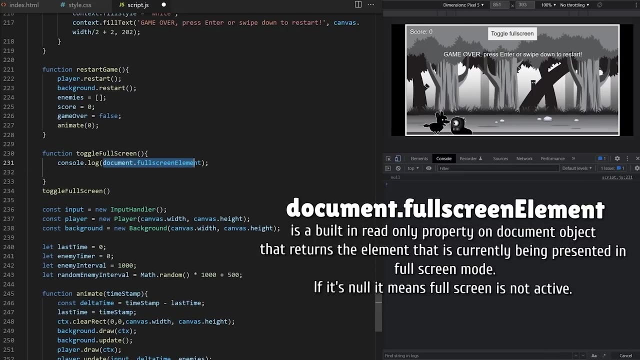 Let's consolelog documentfullscreenElement like this and call toggle full screen function we just wrote. Full screen element is a built-in read-only property on document object that returns the element that is currently being presented in full screen mode. If it's null, it means the full screen is not active. 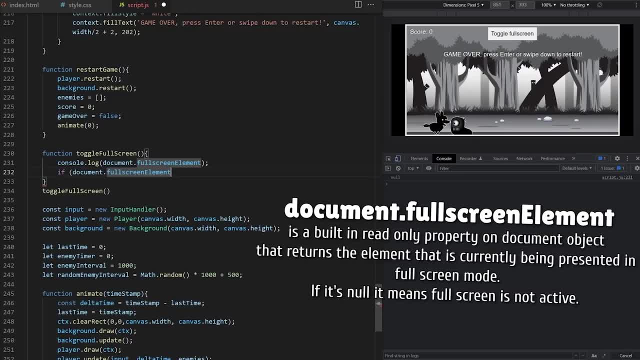 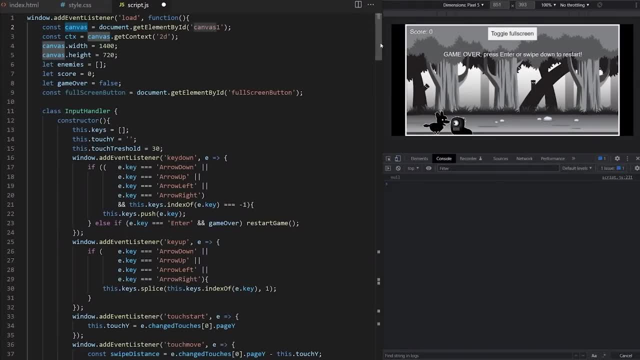 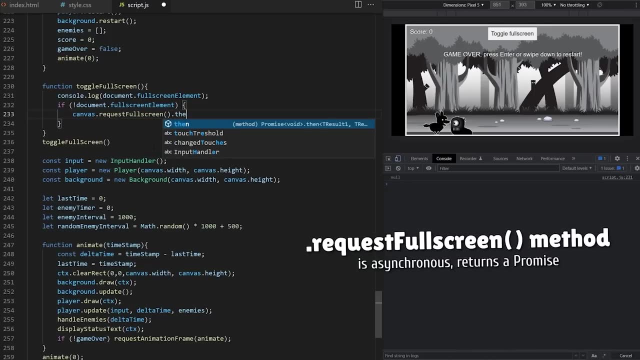 We can use this property to check if we are currently in full screen mode. I say, if full screen mode is not active, take canvas variable from line two and call built-in request full screen method. This method is asynchronous. It returns a promise, which means I can chain. then. 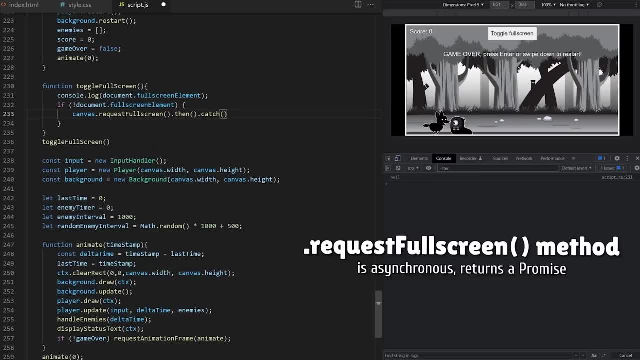 and catch methods to run some follow-up code when the promise is fulfilled or rejected. I will just use catch today to display potential error. Notice that the request full screen is called on the element I want to make full screen, but full screen element property. 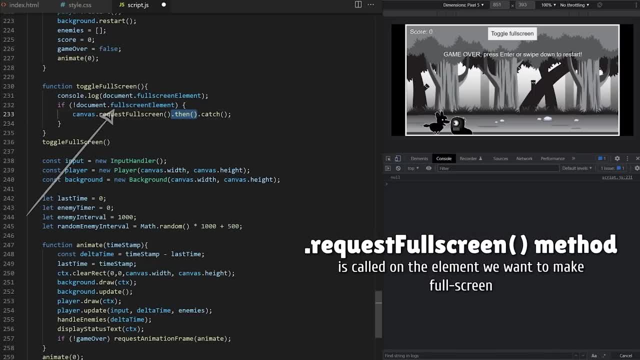 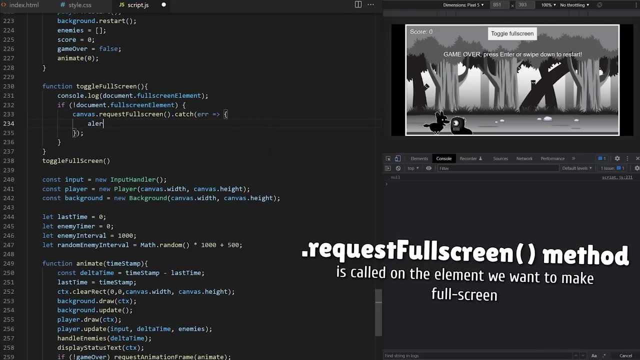 sits on the document object. Today I won't put any follow-up code in then method so I can delete it In catch. I will take the auto-generated error object. If error happens, we will create alert and it will say some error message. 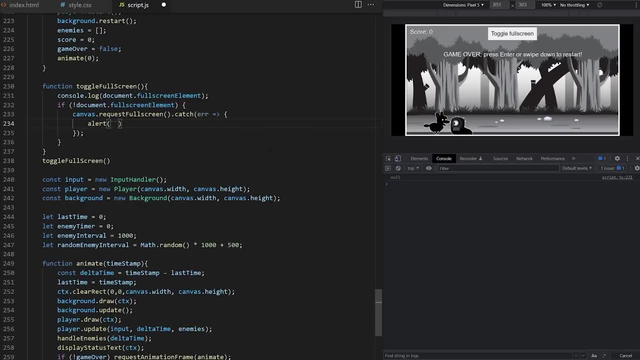 To concatenate message, I can use backticks instead of quotes. This is so-called template literal syntax. It's just a simple way to combine strings of text and expressions that need to be evaluated into a single final line of text. I say, for example, error. 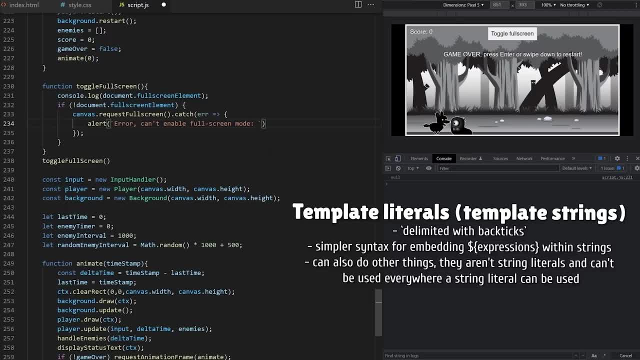 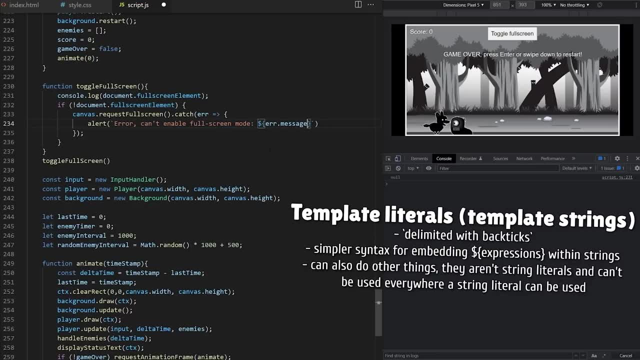 Can't enable full screen mode And to insert variable or expression inside template string, we use dollar sign and brackets like this Here. I just put this auto-generated error object and its message property so we can read what went wrong. So if full screen is currently not active, 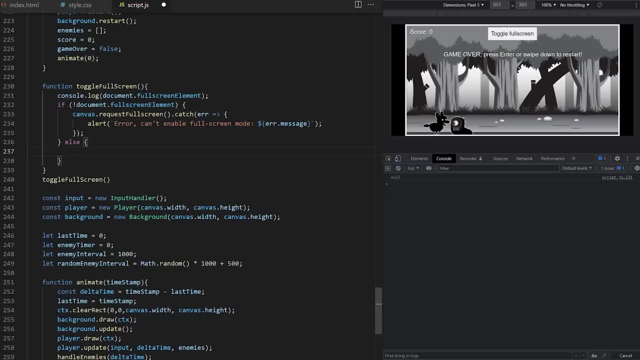 present canvas in full screen mode. Else meaning full screen is active. call built-in exit full screen method to switch back to windowed mode. Notice that exit full screen is again called from document object If I save my project and refresh browser window. 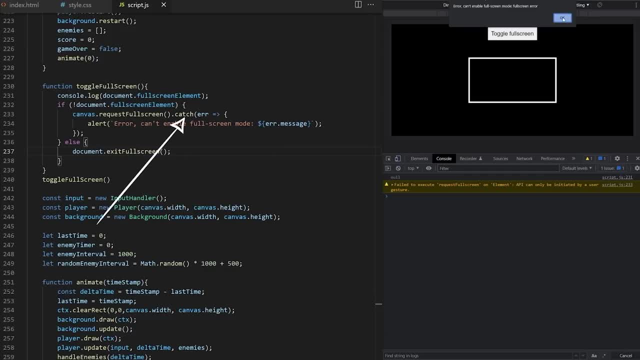 I get an error. You can see catch method worked and created alert pop-up window with our message. In console I can see more information. It says full screen can only be initiated by user gesture. Here I declared my toggle full screen function. 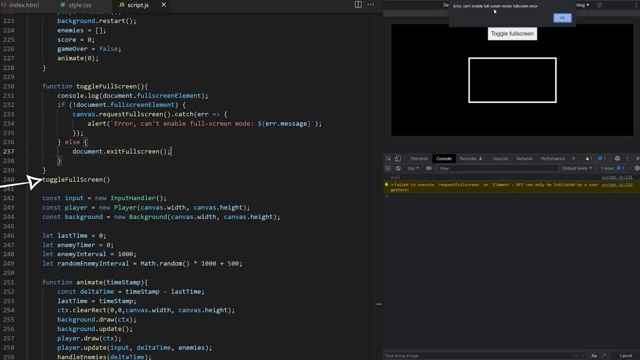 And here I'm calling it on the first page load. We can't do that. Full screen can only be triggered by user-generated events such as click or touch. That's what this error message is telling us. We can't just make JavaScript to automatically show. 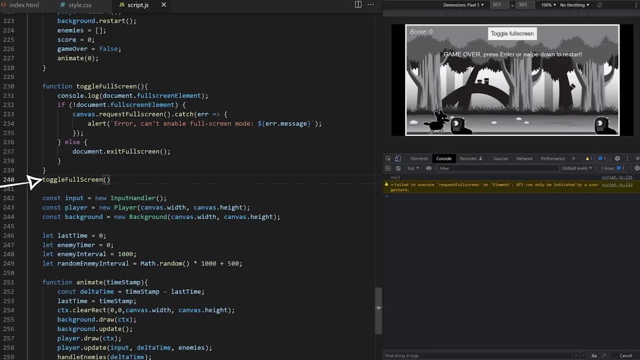 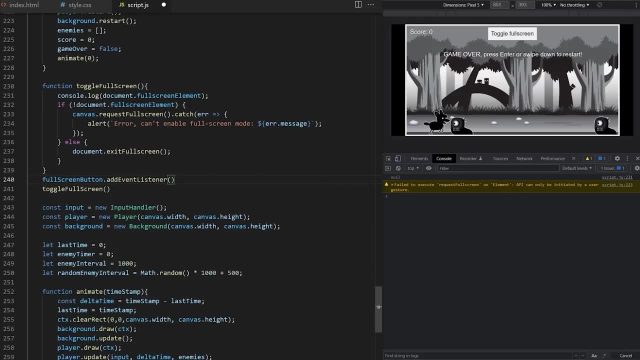 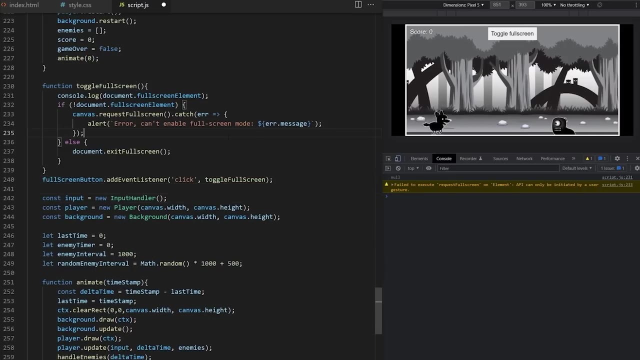 right trigger full screen. It needs to be triggered by user generated event So instead of running it on the first page load, I create an event listener for a click event on full screen button element we created earlier. When user clicks button, then run toggle full screen To exit full screen on a. 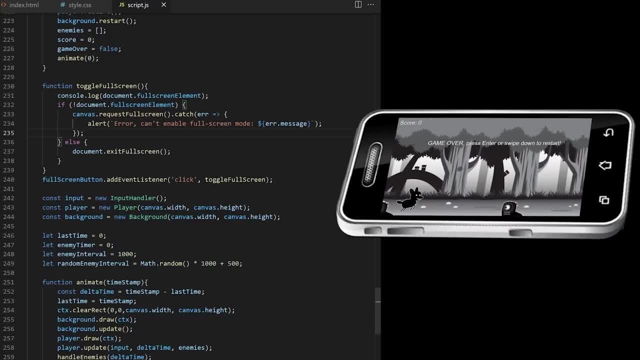 computer you can also just press escape key. On mobile, you can exit full screen by swiping to reveal main controls and press back or home key, depending on which phone you are using. Sometimes we get unexpected collisions and game over when player and enemy images are not actually touching, like 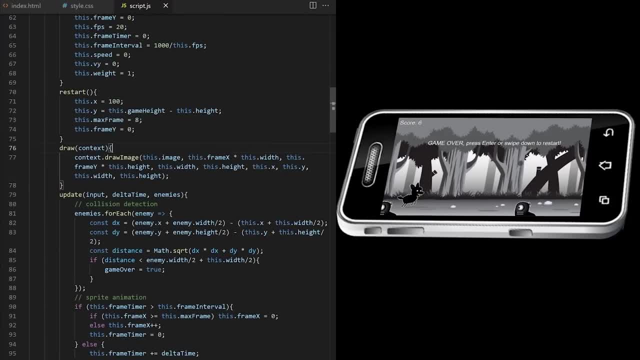 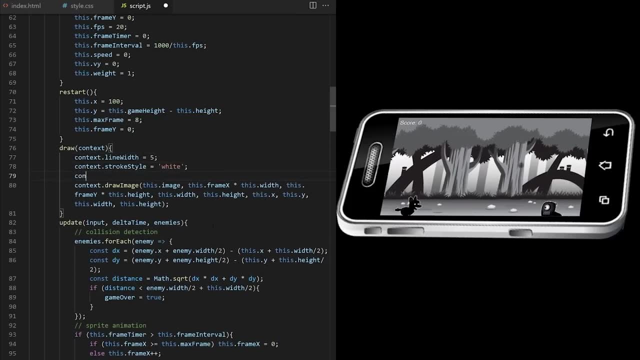 this? It's because we are checking for collision detection on the circular hitboxes around player and enemy and these circles don't exactly match the sprite sheet image. Collisions between complex shape take a lot of performance, and especially for mobile games. performance is something we need to be. 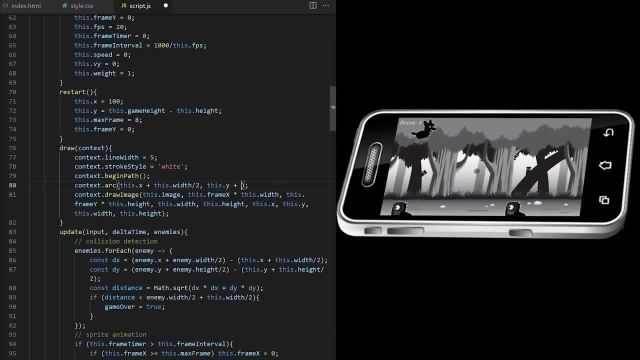 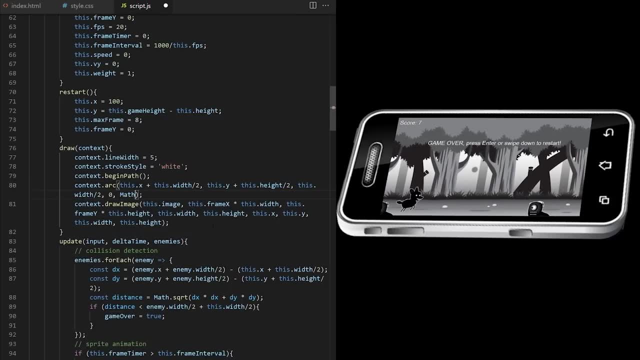 more careful about. Phones don't have as much computing power as our desktop computer. It's usually not a problem when hitbox doesn't exactly match sprite sheet shape, but it should be positioned in a way that it's predictable when collision can and cannot happen. I drew a simple circle. 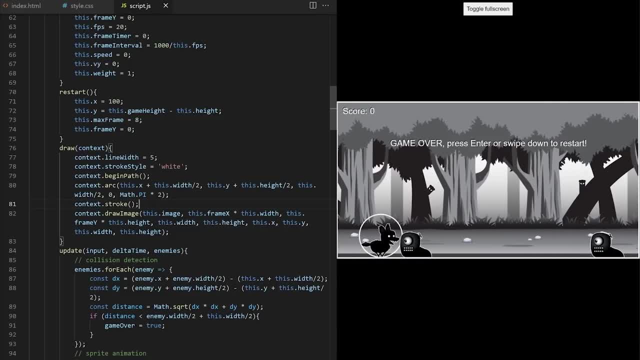 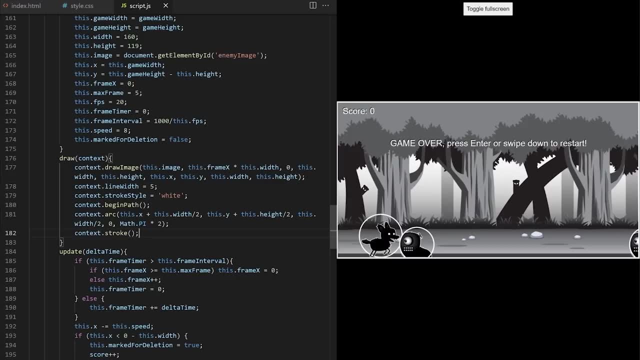 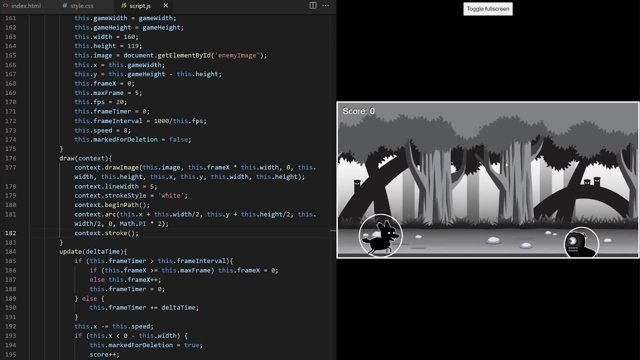 around player and now we can see its collision area. Let's copy this code to display collision area of enemies as well. You can see when these two white circles touch, we get collision. and since the circles are larger than player and enemy image, sometimes we get collision when player and enemy images are. 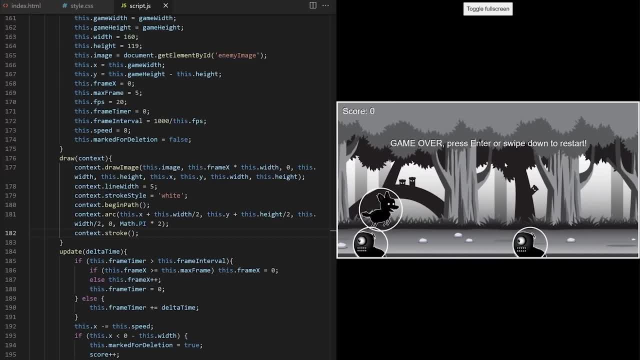 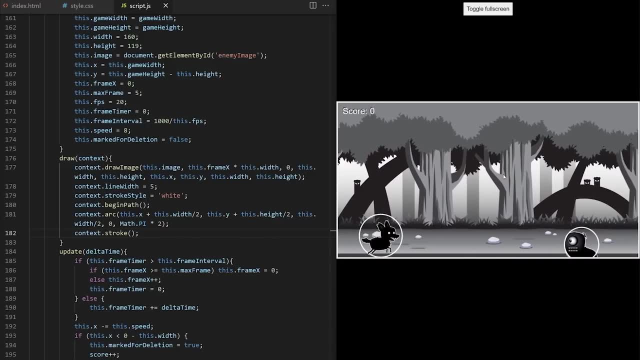 colliding. We can see that the hitboxes are clearly not touching especially this one, when we are about to land from what seems to be a successful jump. How do we fix this? Since player and enemy images are not scalable in this game, they are drawn at. 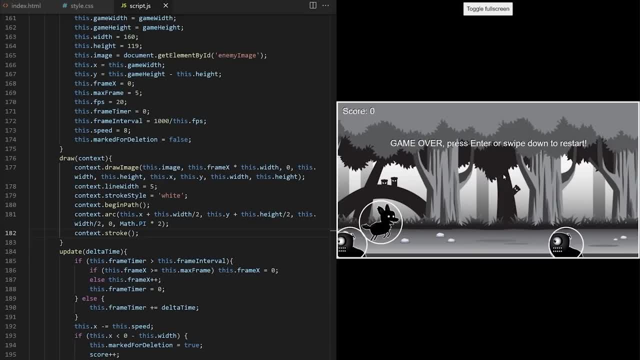 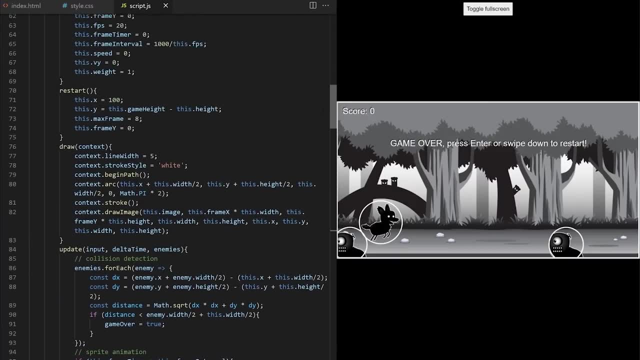 fixed width and height. we can shrink and scale hitboxes by a value relative to image size and we can also move the hitbox left and right by specific pixel amounts to try and match images more closely and make collisions more predictable. We don't want surprise game over like this. 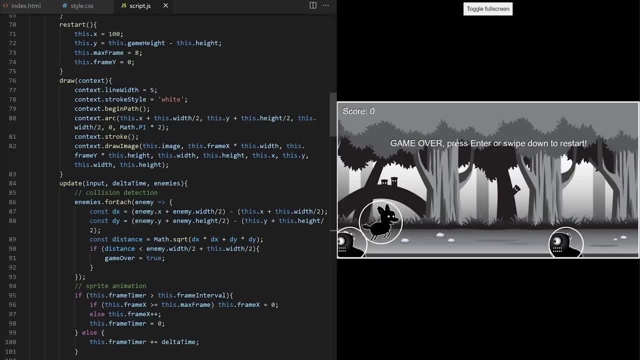 I think it's a bit unconventional technique here because sprites are in a sense rectangular. They have starting X&Y position and width and height, But I chose collision detection between the circles to remove rectangular edges from sticking out outside player and enemy shapes. what I'm about to do well work. 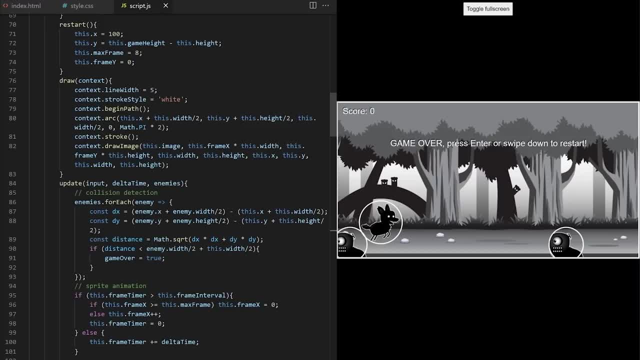 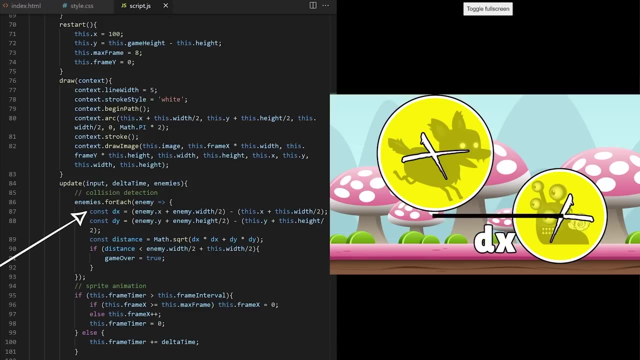 with rectangular collisions as well, if you prefer that. we are calculating collision detection between player and all active enemies here. I explained it in the previous episode. We are basically checking distance between the center point of player circle and center point of player circle, center point of enemy circle, first horizontally and then vertically. 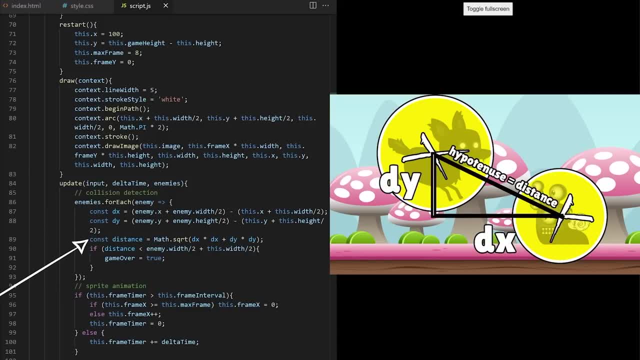 We are drawing imaginary right triangle and using Pythagoras theorem to calculate the length of hypotenuse, which is basically the distance between center point of player circle and center point of enemy circle. Then we are comparing radius of player circle plus radius of enemy circle to that distance. 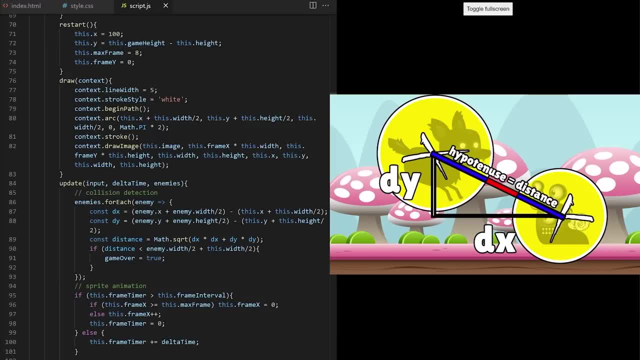 If distance is more than sum of these, two radii circles are far apart. If it's, the same, circles are touching, And if the distance is less than sum of radii circles are overlapping. Here I'm just drawing white collision area circle. 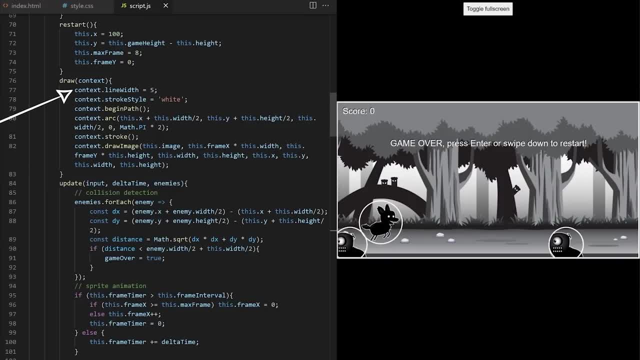 It's just a visual. it doesn't actually detect collision. Collision is being detected here. We are inside player class and this is the horizontal center point position of player circle. This is being used for collision detection here. This is vertical coordinate. This is the net of that center point which is being used in collision detection formula. 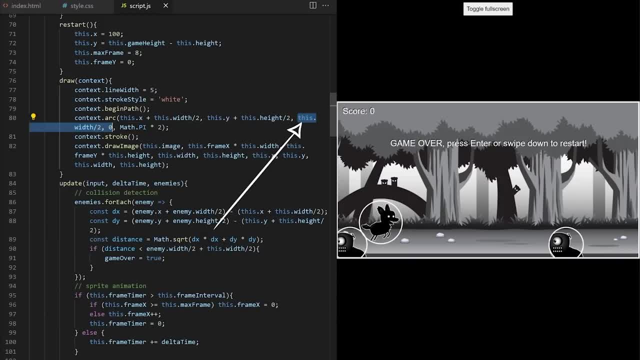 here And this is the radius of collision area circle we are drawing and that same value is being used in collision detection formula. here I can simply offset and resize that collision circle visual in this area and then replicate those changes inside the actual collision detection calculation area here. 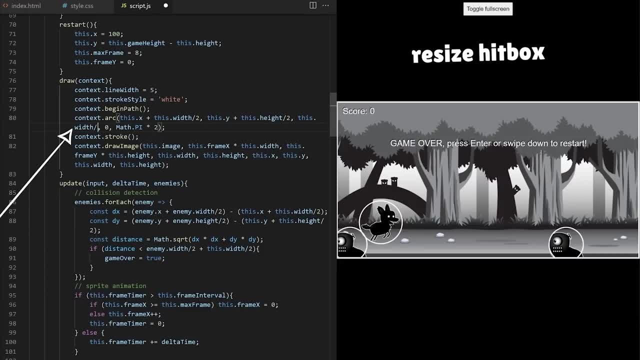 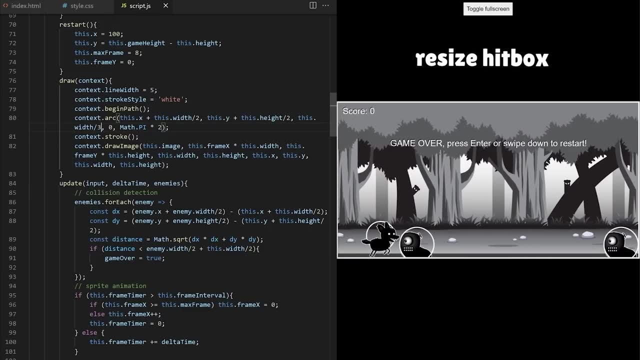 Let me show you what I mean. What if I want player circle to be smaller? Maybe I don't mind that. ears and tail, Let's say they are soft and they don't count when it comes to collision. Also, maybe I want to make my game a bit easier and forgiving. 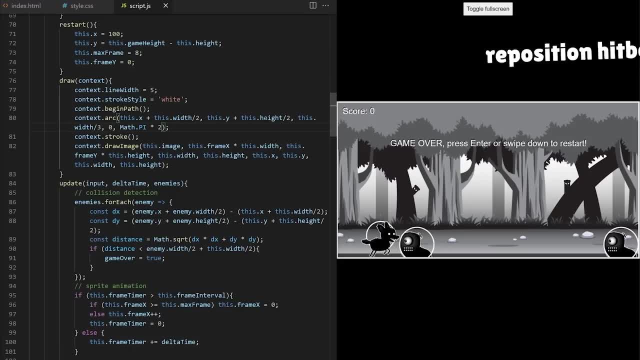 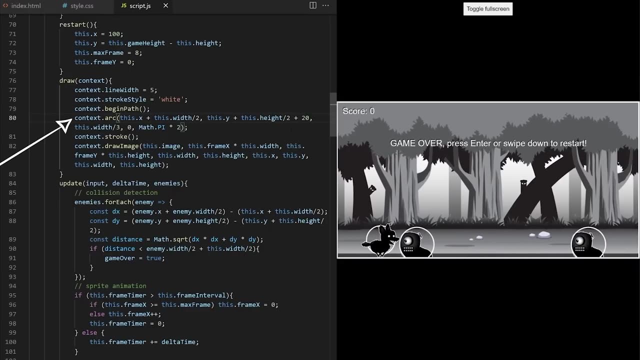 This will allow a small overlap between player and enemy image. What if I want to move the collision hitbox downwards relative to player image? I change it's vertical center point position here plus 20 pixels seems fine. Now I compare changes I made to the visualization and I make sure I update the actual collision. 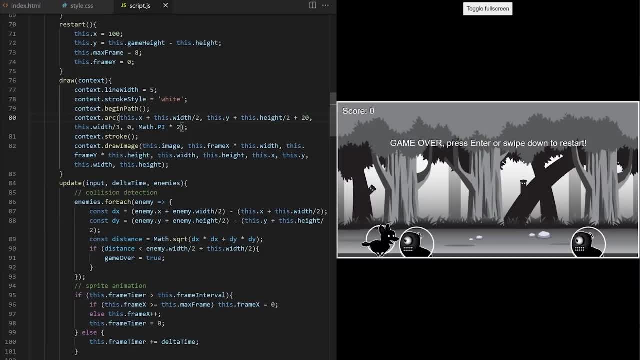 detection formula to match these new values. Here I can see the collision in the middle position and I can change it to the center. I didn't make any changes to horizontal center point so that value stays the same. I added plus 20 pixels to vertical center point so I update it in collision calculation here. 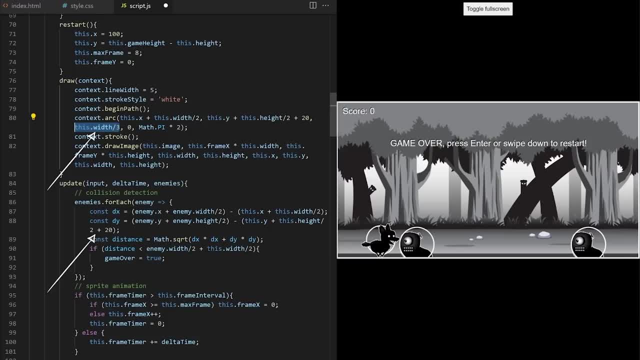 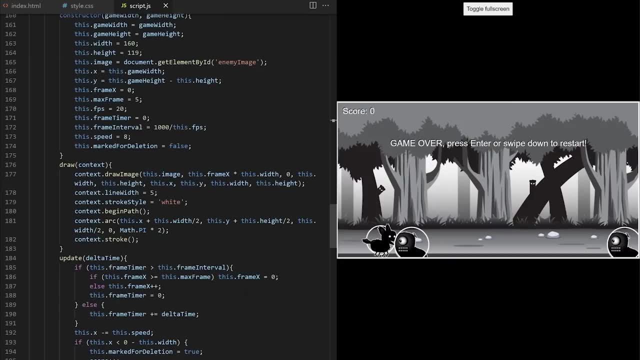 I also made the circle smaller, so I update player radius value. in this area. We successfully adjusted player hitbox. Let's also do something about enemies. I can, for example, reduce the radius of enemy circle. I also want to move it to the left. 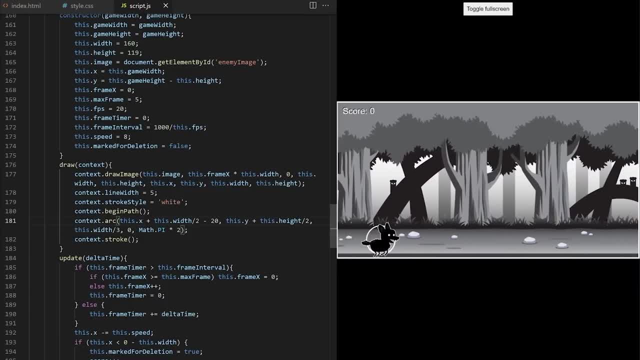 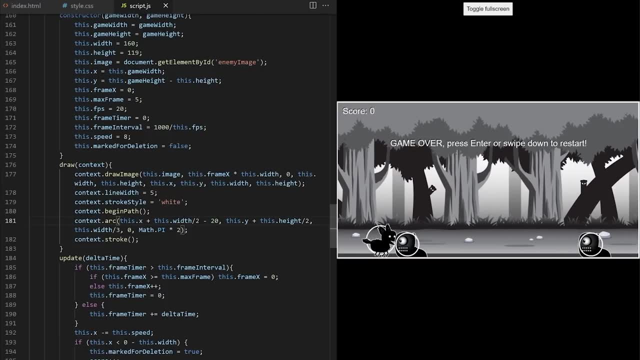 To cover head of the worm better. Maybe minus 20 pixels for horizontal center point. I'm actually happy with this. I want collision to only happen when these two adjusted smaller circles collide. Let's take the changed values we used to adjust enemy hitbox visual. 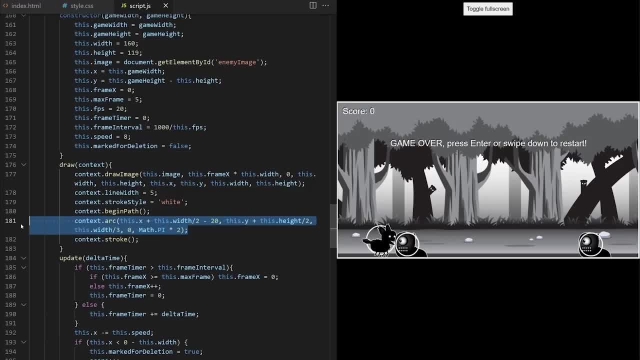 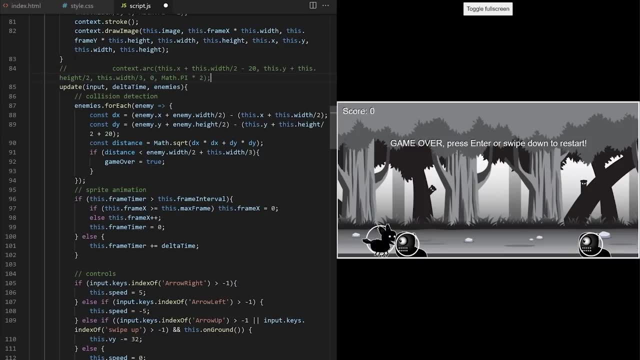 And transfer them into collision detection formula, like we did with player. I copy this line just so I can look at it for reference. I put it here just temporarily: Collision detection is inside player class, So this key word here points to player object. 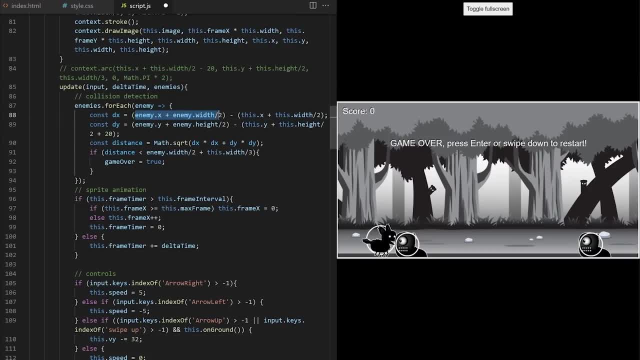 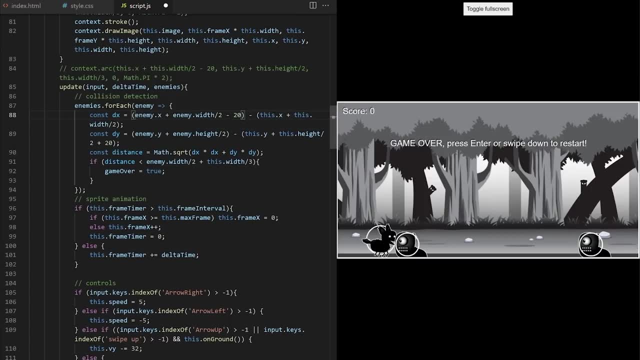 If I want to point towards enemy object, I can't use this key word in this area. We adjusted horizontal coordinate of enemy circle center point, so I need to adjust it here, minus 20.. Vertical center point of enemies stayed the same, so I will not be making any changes here. 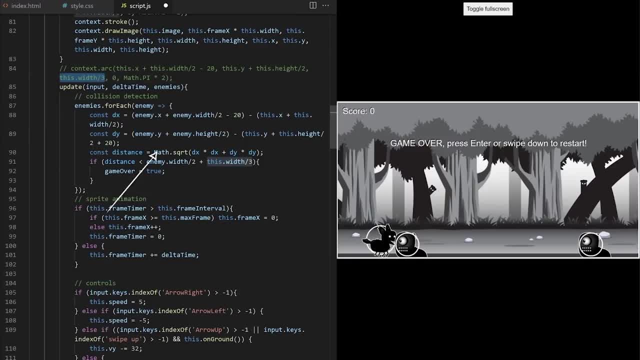 We did change enemy radius, so I will change enemy radius here. And this is how you resize, scale and reposition hitboxes in your game to make sure they match your art assets more closely. So this is how you resize, scale and reposition hitboxes in your game to make sure they match your art assets more closely. 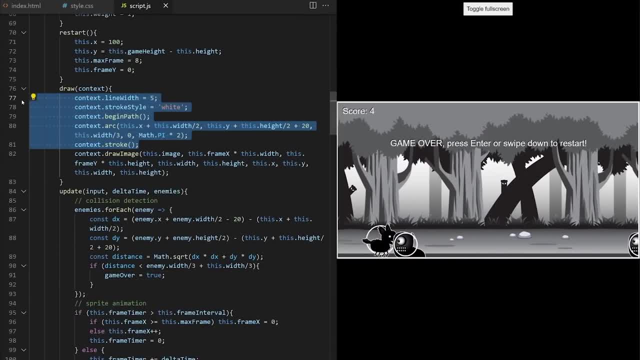 So this is how you resize, scale and reposition hitboxes in your game to make sure they match your art assets more closely. I didn't plan to make this episode, but so many of you asked how to add mobile support to our games, so here we go. 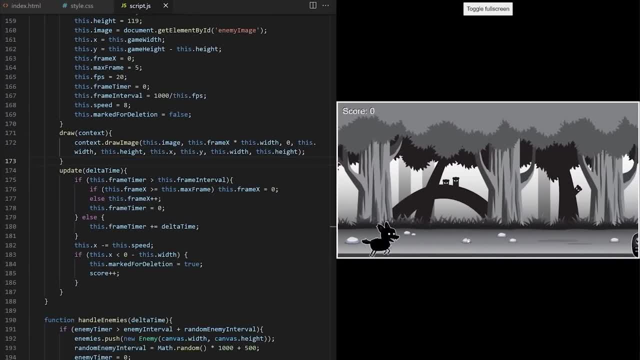 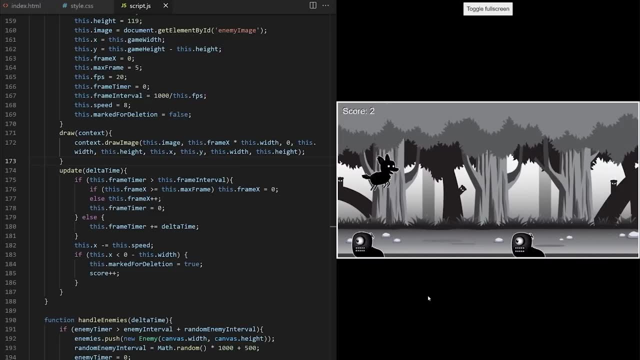 We can take it much further, but I think this was a good beginner friendly introduction. Check out full series in the video description if you want. I'll see you there When your games and applications start getting bigger, more exciting and full of extra features. 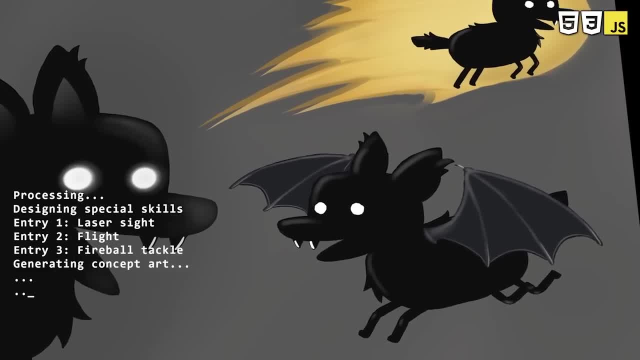 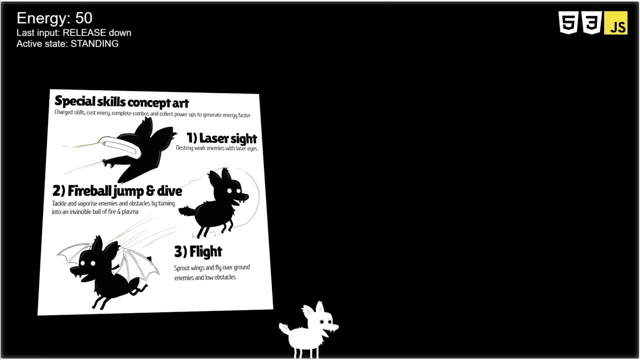 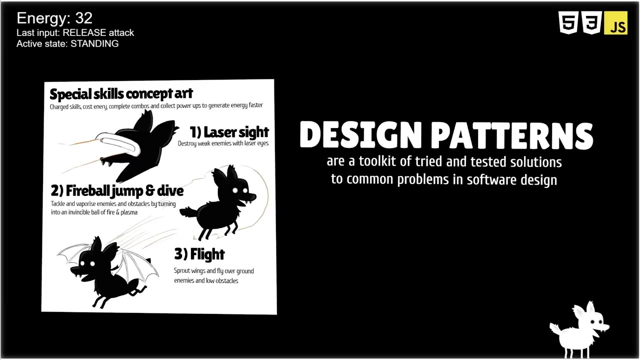 it will be more and more challenging to keep your code clean and organized Over time. Over time, we've come up with general, reusable solutions to commonly occurring problems. These well-tested and widely used code structures are called design patterns. Design patterns are a toolkit of tried and tested solutions to common problems in software design. 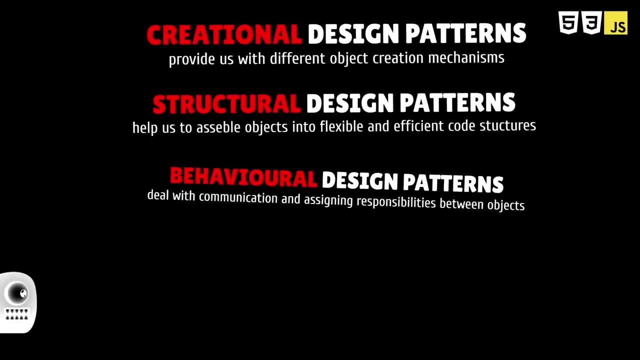 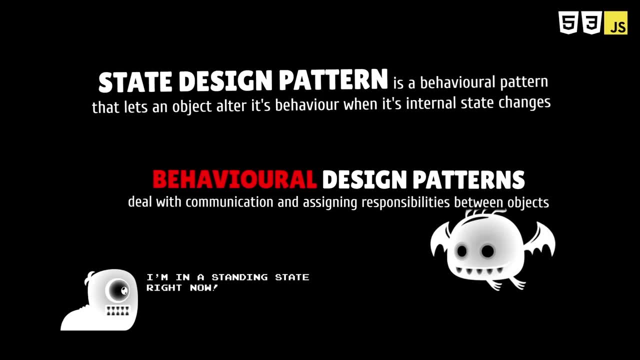 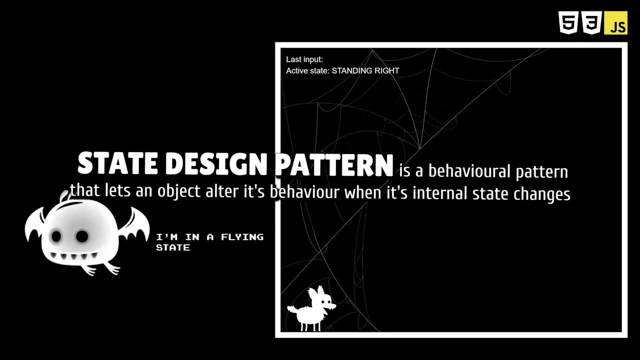 You could split design patterns into three main categories. In this class we will use State Design Pattern to control player character in a game. It's a behavioral pattern that lets an object alter its behavior when its internal state changes changes. Why do we need to manage player state? Let's say we have a simple side-scroller game. 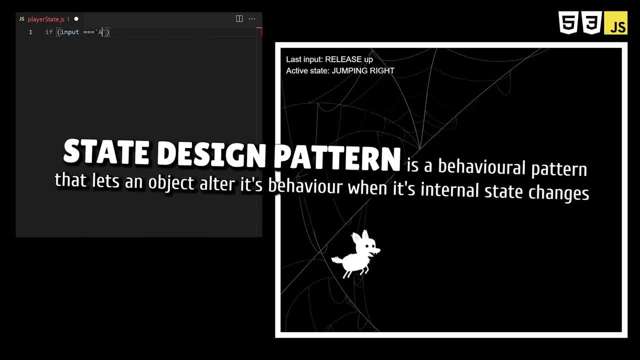 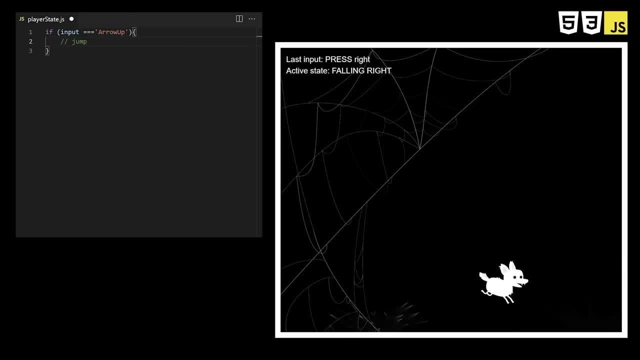 Our character is standing and when I press up arrow key I want it to jump. This code has a bug. If I keep pressing up arrow while jumping, player character will fly off screen. So I have to do a check here. Only run this code and jump if character is standing on solid ground. Great, 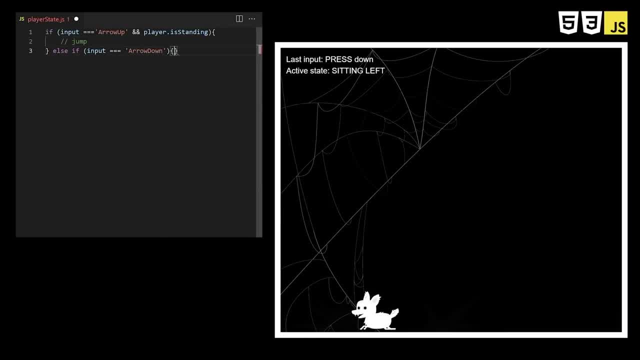 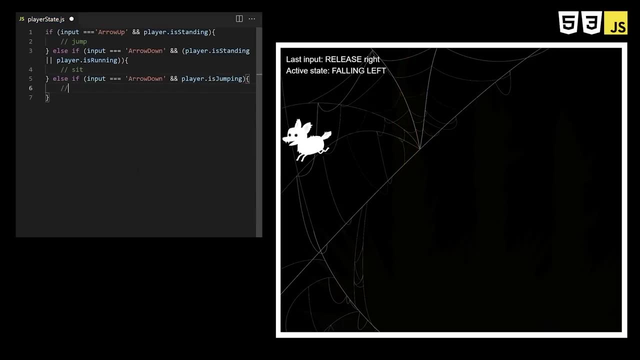 that fixed it. I also want to add sit-in animation, but player can't enter sit-in state while it's in middle of jump. Player can sit down only when it's standing or running on solid ground. Maybe I also want a dive attack when player tackles enemies from the air. Again, this move can only be entered. 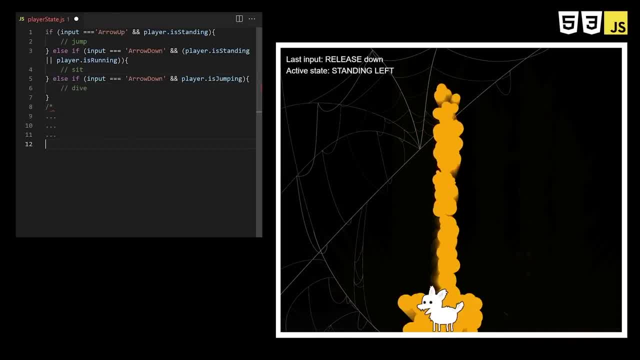 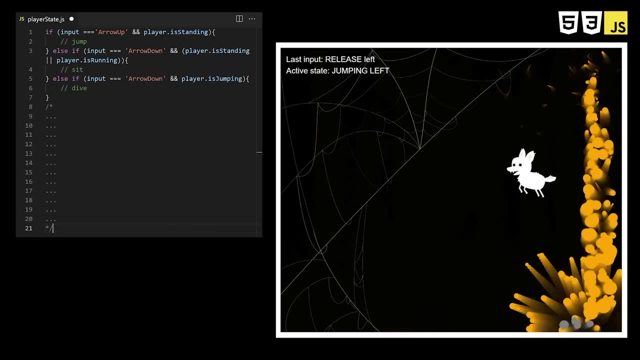 by pressing down arrow key while jumping, because when we are standing down, arrow key will make player sit down. I'm sure you can imagine how adding more moves will create a very complicated if-else statement and since all of that is contained in a single piece of logic, adding one. 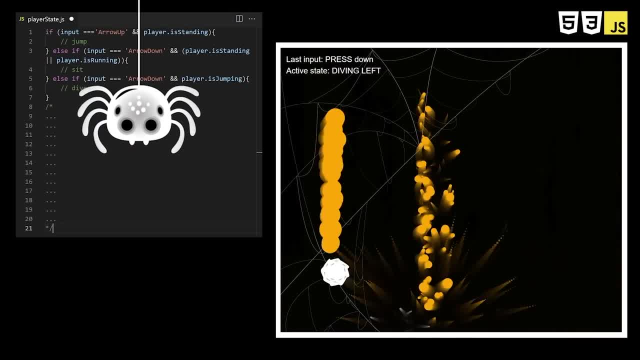 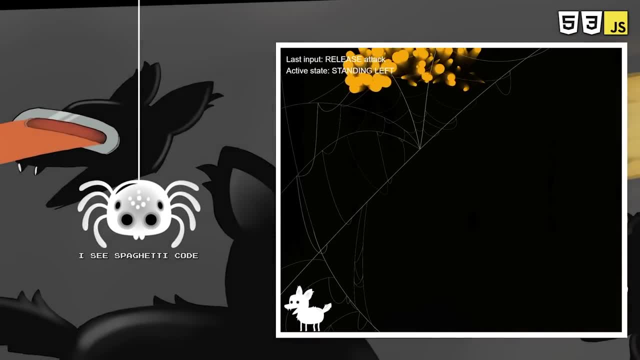 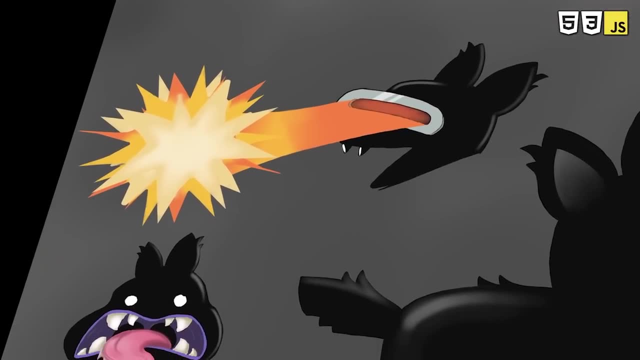 new move later on can break all your other existing conditions and you will have to review that single massive logic tree every time you need to fix a bug or add a new feature. Since this is a very common challenge game designers had to deal with for a long time, there is a tried and tested way to do this right. 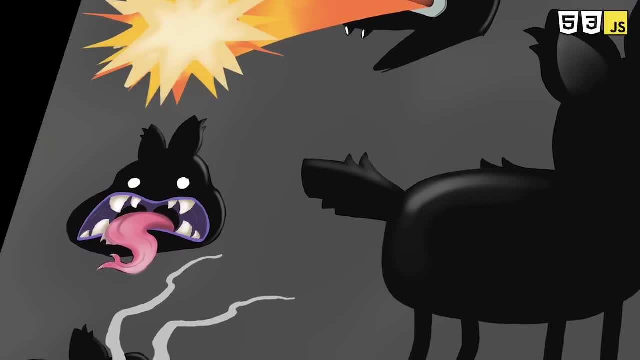 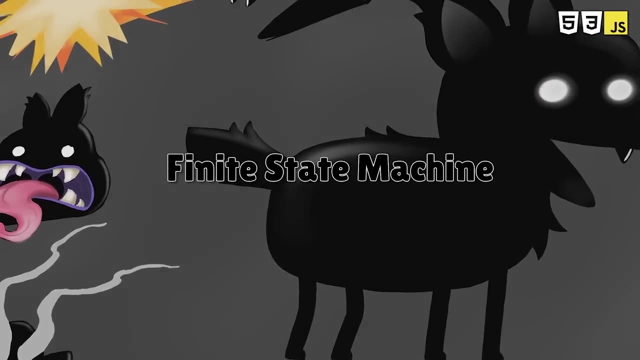 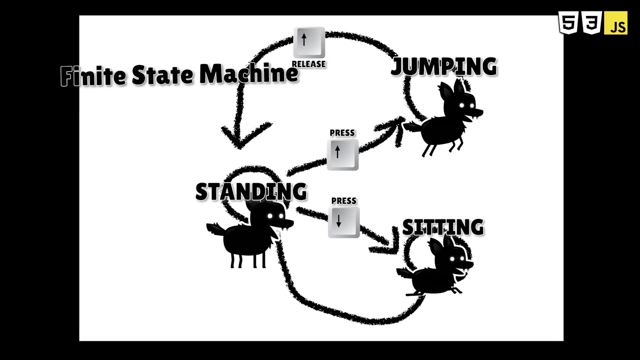 What if, instead of this complicated spaghetti code if-else statement, we model our code structure based on finite state machine? We want to have a limited set of states player object can be in, such as standing, jumping or sit-in. The object can only be in one of those states at a time and for each state it will only. 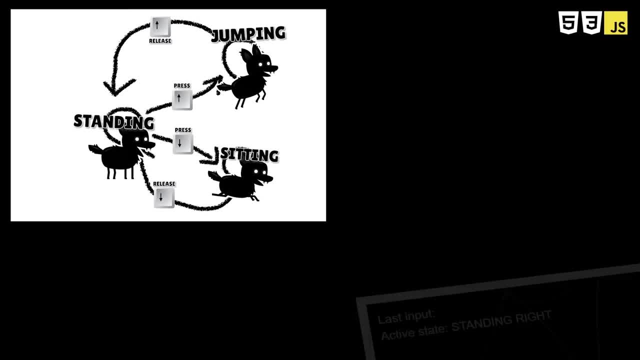 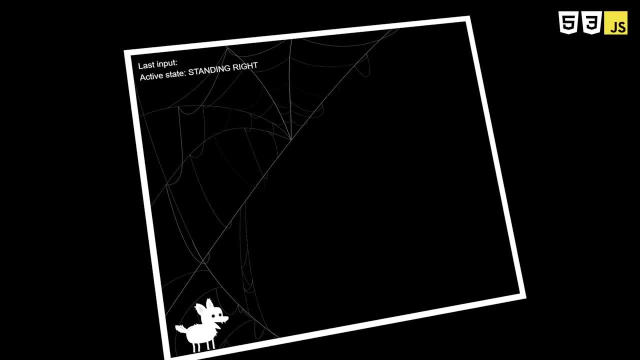 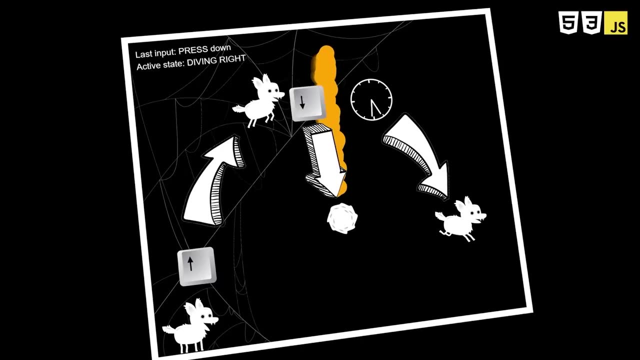 react to a limited set of inputs. we define That way. we have a class for each state and in rules of that class I can say that, while player is jumping, wait for a certain time before switching it to falling state or, if you detect down arrow key input transition. 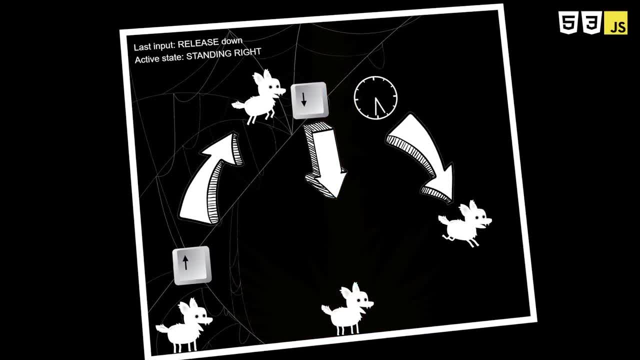 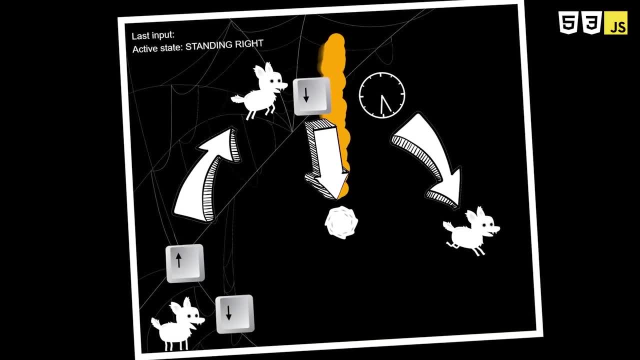 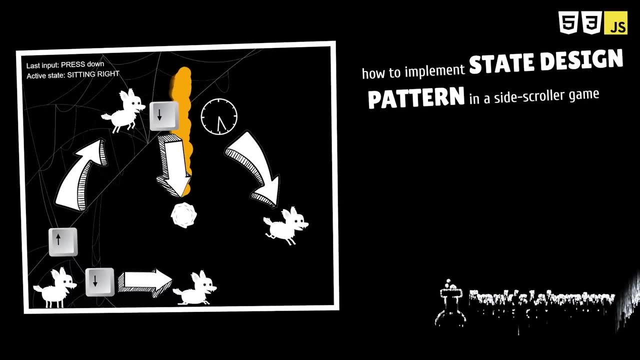 player into diving state Other than that, while in jumping state, ignore all other inputs. Pressing down arrow key while jump in will switch player into diving state. Pressing down arrow key while stand in will transition player into sitting state. In this class we will learn how to implement state design pattern in a side scroll game. 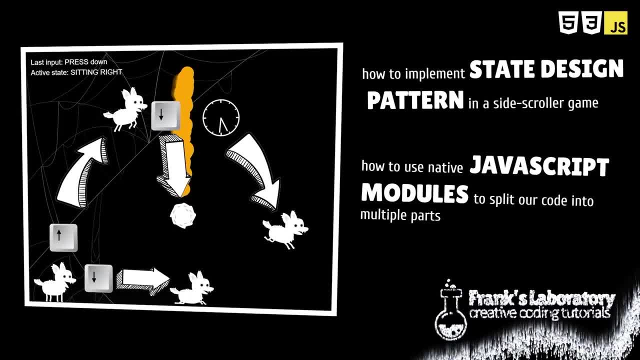 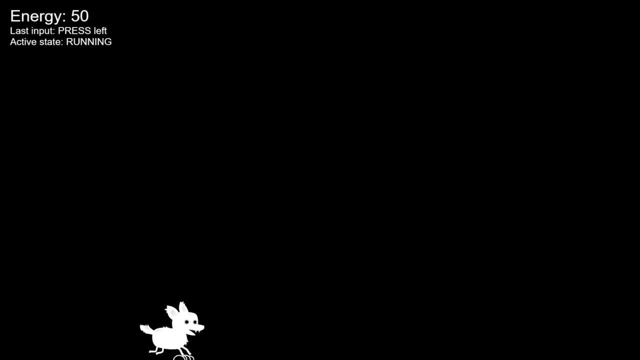 We will learn how to use native javascript modules to split our code into multiple parts and many other important game development tricks. and techniques. as usual, Pick the like if you are ready to start building bigger games and learn how to make our code bases scalable, easy to navigate in, easy to manage in and easy to use. 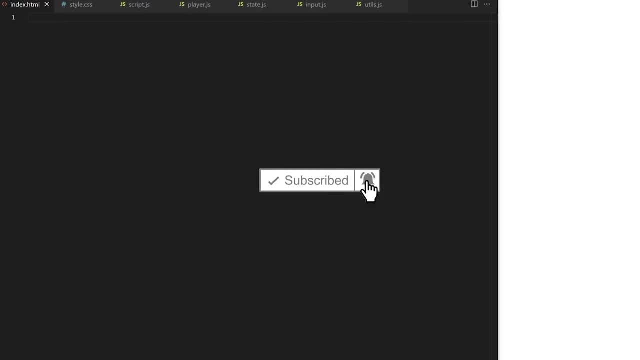 Thanks for watching. We are diving into more advanced territory today. The challenge for beginners will mostly be to keep track of what each class and function is doing and how they interact with each other. Check out some beginner friendly game development tutorials in the video description, if you. 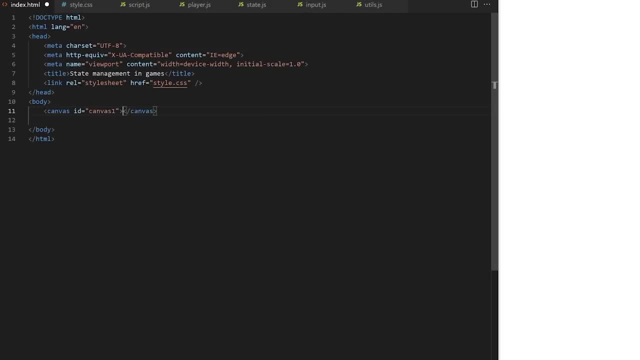 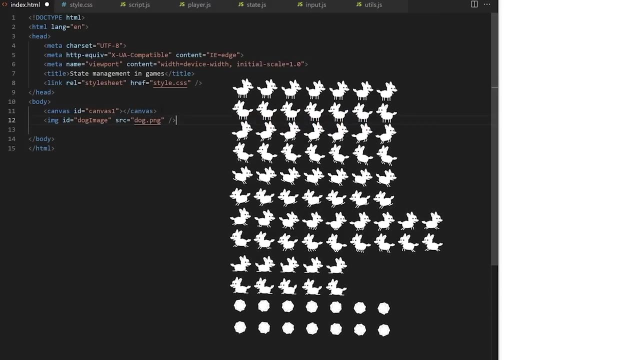 just recently started with HTML, CSS and JavaScript. I created a simple web page. This doc image will be our sprite sheet. You can download it in the video description. It was made by this amazing artist. Check out his site for more game development art assets. 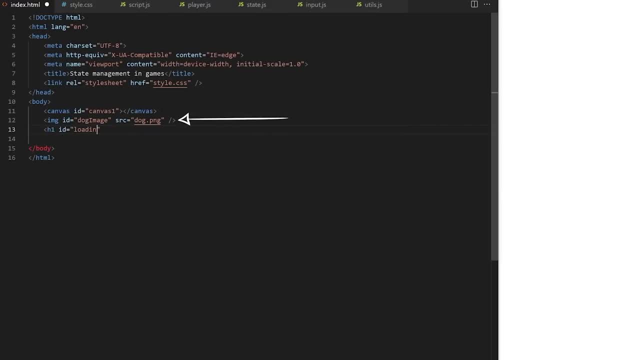 I include my image as img tag this time. That way I can wait for the image to get fully loaded before I run any javascript. I include my javascript by using a script tag, but this time I will set its type attribute to module. This will cause the browser to process any 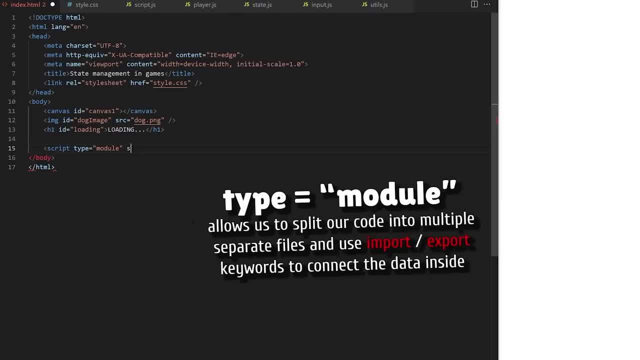 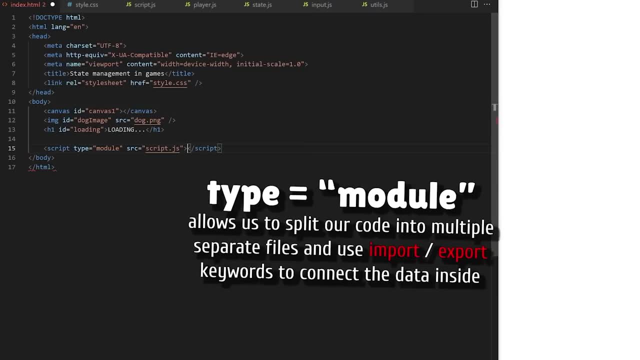 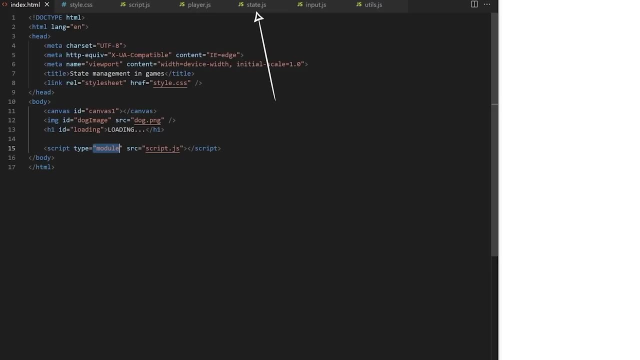 contents of this particular script as a javascript module which will allow us to split our code into multiple separate files and use import-export keywords to connect the data inside. You can see I'm importing only the main scriptjs file, but we will also have playerjs, statejs, inputjs and 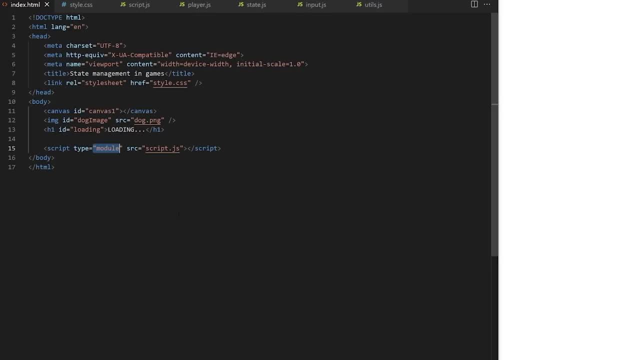 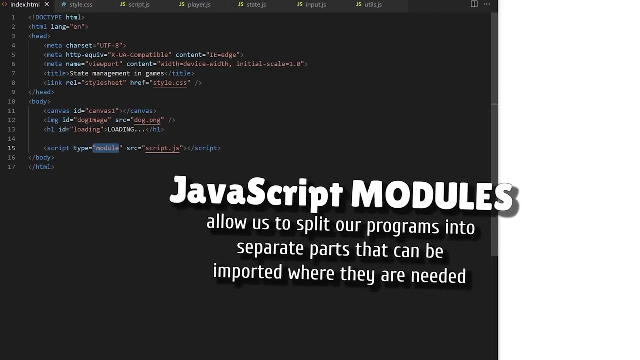 utilitiesjs. Splitting files like this makes our project a bit cleaner and easier to navigate in. JavaScript modules allow us to split our programs into separate parts that can be imported where they are needed. Nodejs had this ability for a long time, but now modern browsers support module. 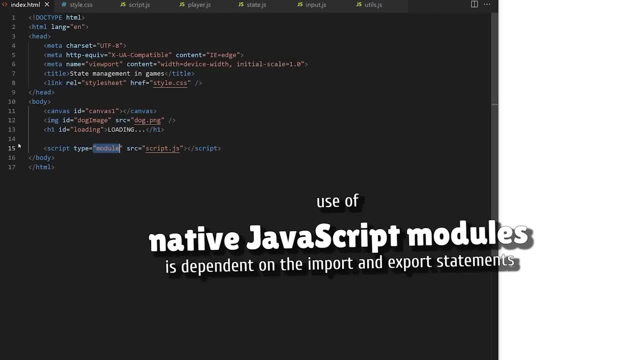 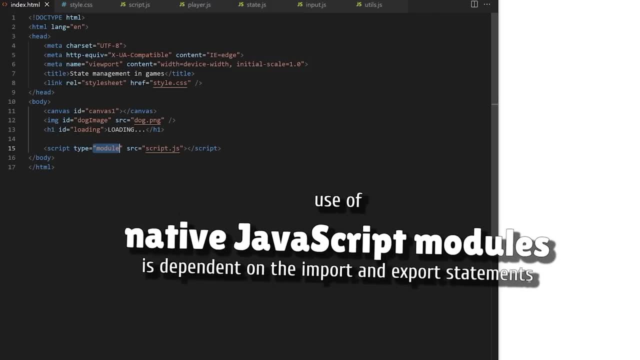 functionality natively. Use of native javascript modules is dependent on the import- export statements, and we will cover how to use them today. It's easy, don't worry. There is only one catch when using modules: You need to run the code in some kind of dev environment. You need to have a 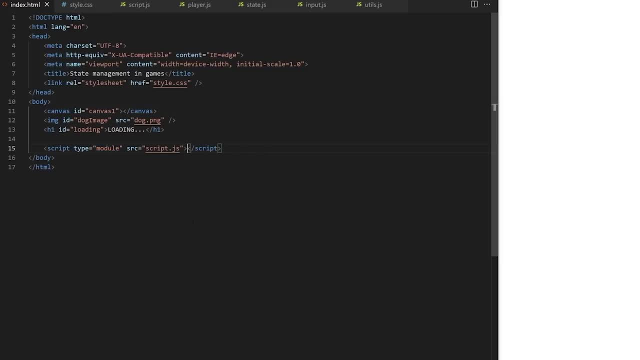 server. If you just write indexhtml file and click to open it in browser locally, as you can do with all my other course projects, import- export keywords will not work. You need to run this code through a server. There are many ways to set up local. 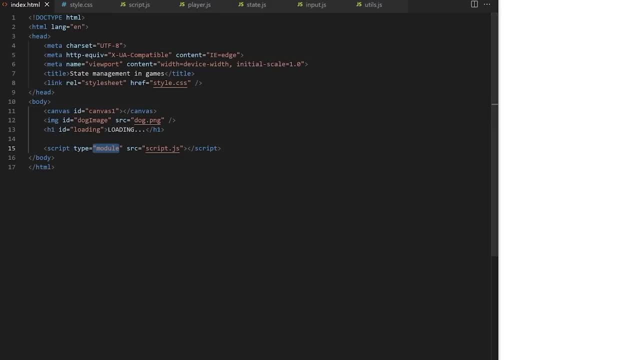 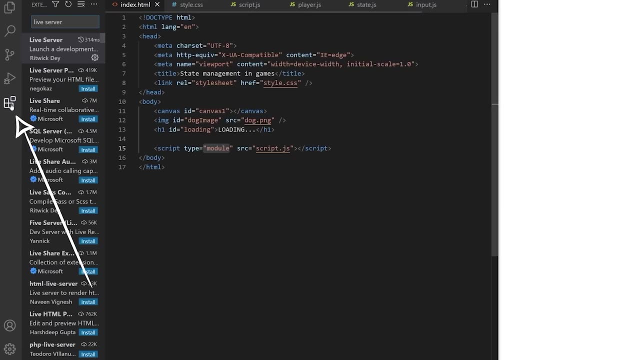 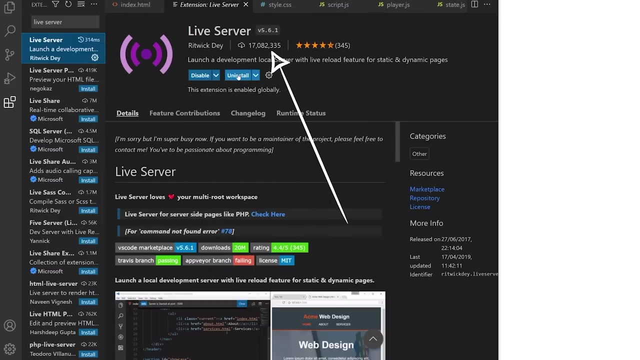 server. The easiest one is to install a small plugin to your code editor. I'm using visual studio code and when I click here on the left side on the extensions icon and I search extensions for live server, I find this plugin. It's been downloaded over 17 million times, so it's very 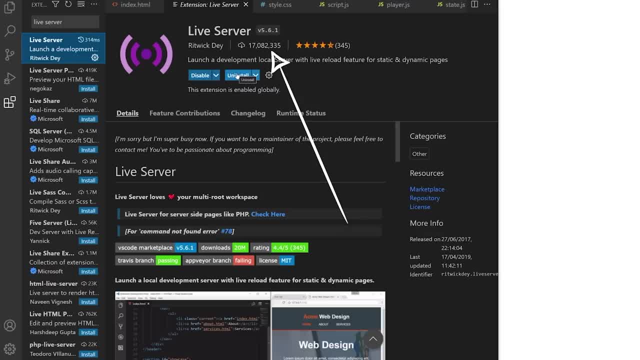 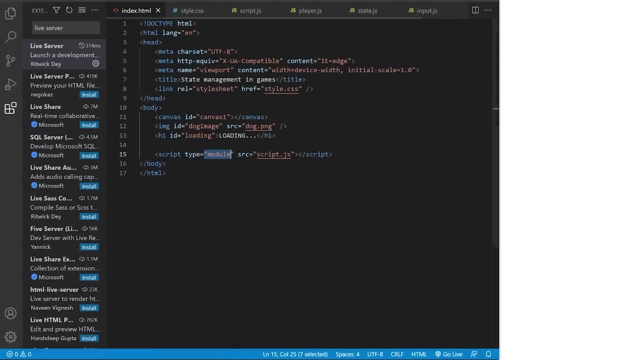 popular. Mine is already installed, but if you don't have it, it will say install here. After installation you might have to close or reopen your vs code. When it's successfully installed, you will see this go live icon right here. If you never used it, it can act a bit unexpectedly When you click go live it. 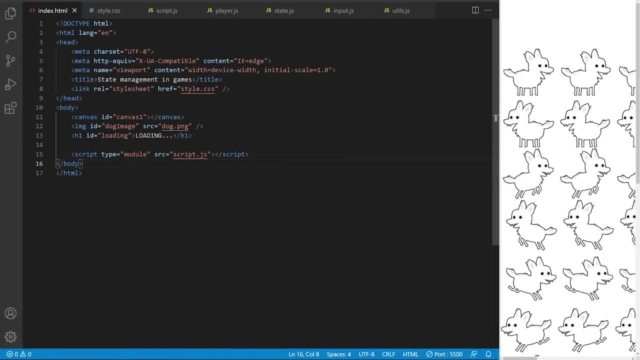 doesn't open the file you are looking at at the moment, It will run code from the entire project folder. your vs code is currently pointed at. To make sure your live server goes live with the correct set of files, you click file in the top left corner and then click open folder and you. 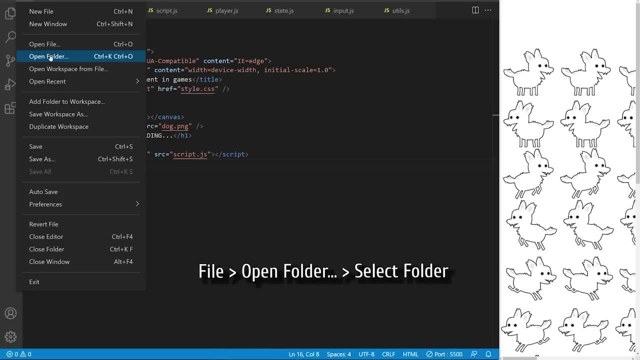 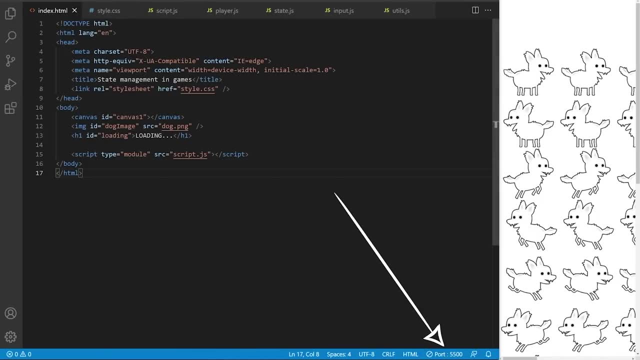 navigate to your project folder on your local computer. When you find it, click select folder and then, when you go live, the correct project will open. If you can't see this new live server notification area, close your vs code completely and reopen it and it will get loaded. The best thing about live server. 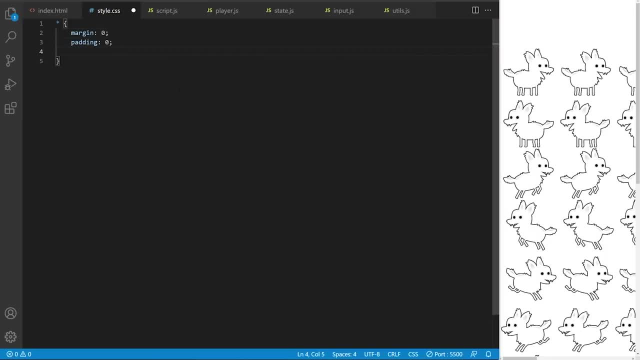 extension is that when you save any of the project files, it will reload browser window automatically. You can always see the latest preview of your code without constantly manually reloading browser. On my windows computer I use ctrl plus s keyboard shortcut to save changes to my file. 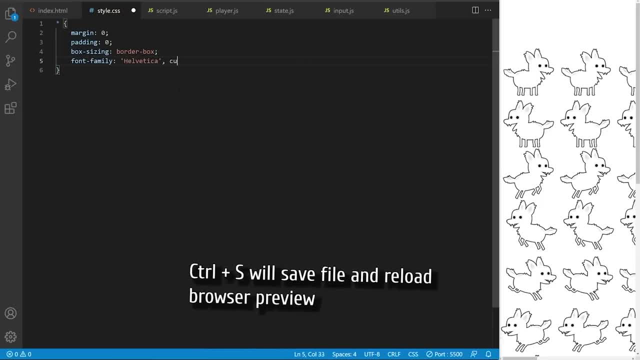 I use it a lot while working in this environment. So now we should have a project folder running through live server extension. We have index html file, style: css: main script js file. We will have player js where we write all the logic to control and animate our player character. State js will be where we write state. 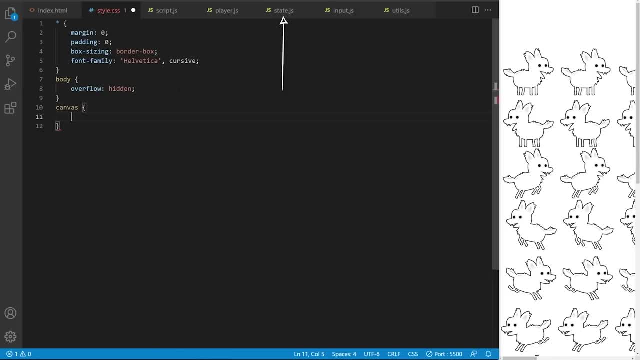 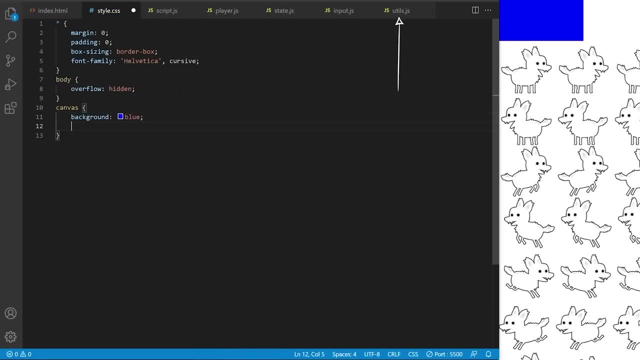 design pattern to swap between different player states. Input: js will handle keyboard input and utilities js will have small useful functions that, for example, display status text or some other tasks. I will speed up css setup because that's very basic. Global reset to make sure the page. 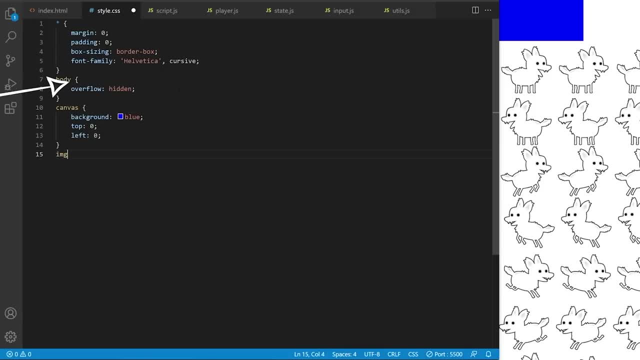 looks the same across different browsers. I will give canvas some background so we can see it, and I will hide the spreadsheet image, since we will be drawing and animating it with javascript. I will also show you how to create a very simple loading screen. I wrote this h1 tag with an id of loading. 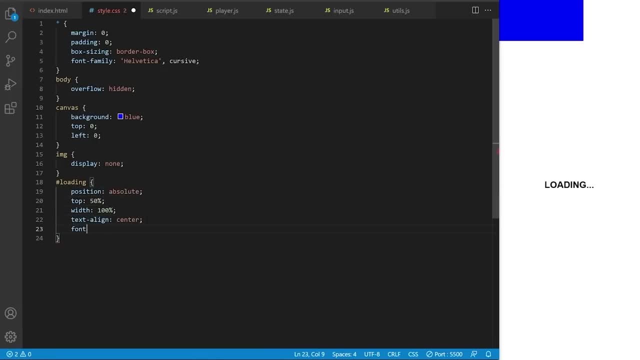 so I grab it here, I center it in the middle of the page and I adjust its font size. Script js is my main module, which will connect all other parts into a final piece of logic. The spreadsheet we are using today is a big image file, so it might take a second to fully load. To make sure, 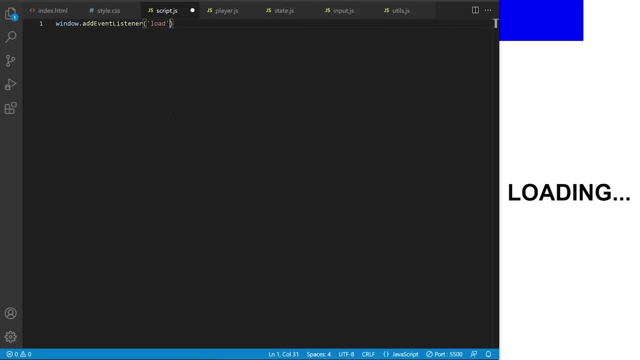 javascript waits for all the assets to be fully loaded before it runs. I will create a simple event listener for load event. Load event will wait for the entire page to be fully loaded and available, including page content such as style sheets, images and so on. In the meantime, this text that says: 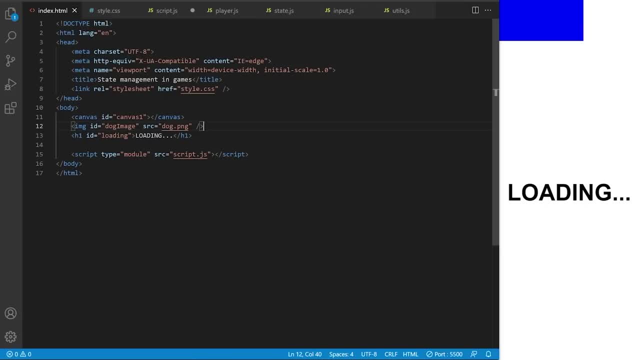 text is visible. so if you add more art assets, user will see this loading screen for however long it takes to load all assets. When everything is fully loaded, this event listener will run its code and inside I will target this loading text and I will hide it, because the page is fully loaded at the 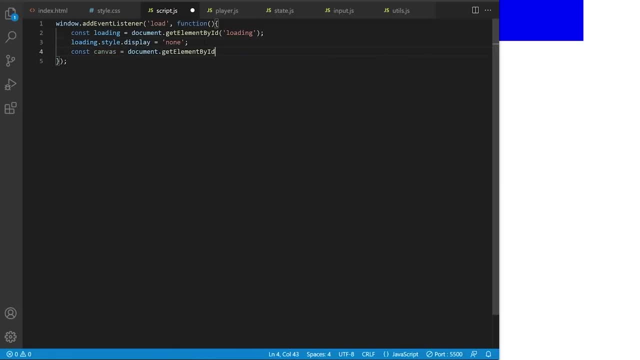 point. when this code runs, I will also set up my canvas. so document dot get element by id: canvas 1.. I instantiate context object which contains all the drawing properties and methods we will need today. I set canvas-width to window-inner-width and canvas-height to window-inner-height. 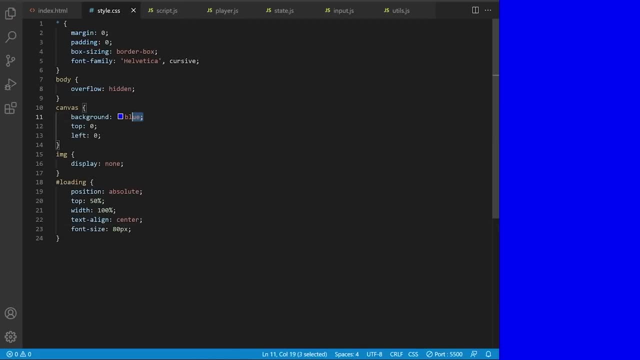 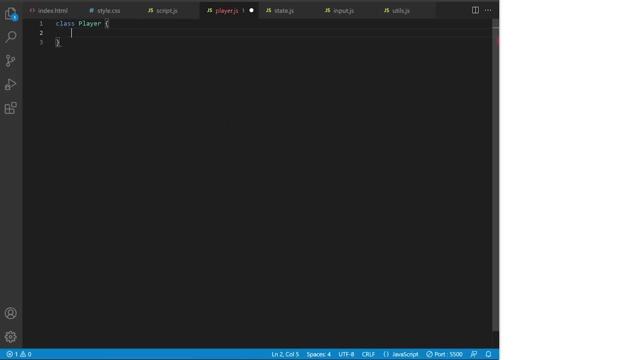 I can see canvas is now full screen so I make it transparent. It's time to draw the player. In playerjs I create a class I call player. Player always needs to be aware of boundaries of game area, since we will be running and jumping around and we need to know when we reach the edges of screen. so I will pass it. 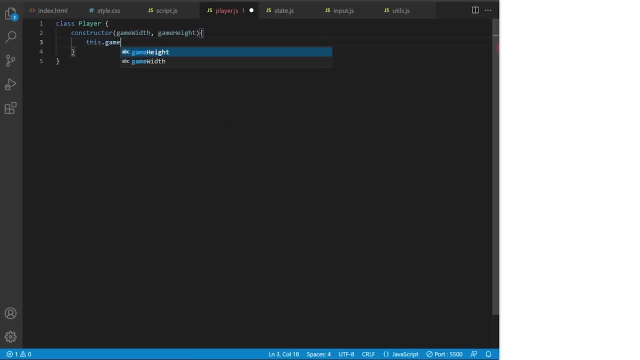 game-width and game-height from the outside as arguments, And I will convert these arguments to class properties like this: Today we are learning about state management. We will be swapping player between different states. This dot states will be an array and each position in that array will be one possible. 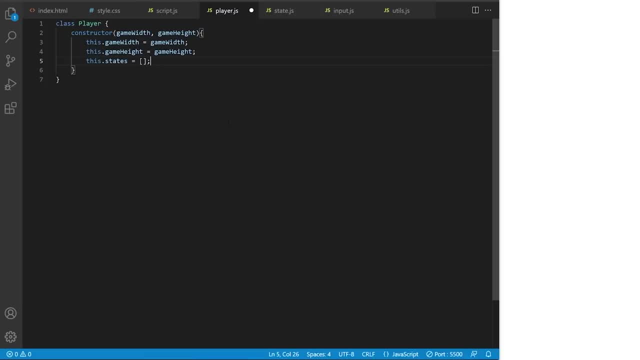 player state, such as running, jumping, sitting and so on- Then we will have this dot current state property. because player can only ever be in one state at one time, Current state will be one of the options from this dot states array. so, for example, 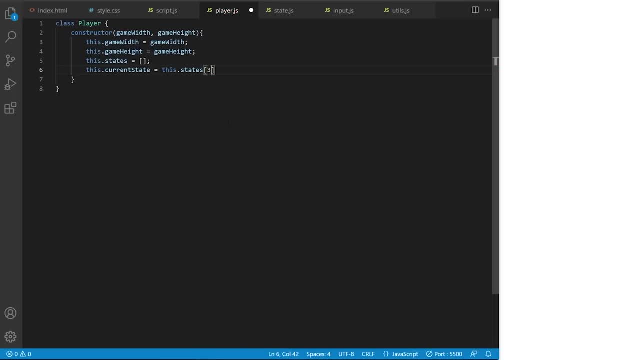 this dot states. index 0 will be standing state, index 1 will be jumping state, and so on. This dot states is an empty array now, but we will fill it with states very soon. This dot image will be the dog spreadsheet. I already loaded it into our project on line 12 in indexhtml, so here I just point this. 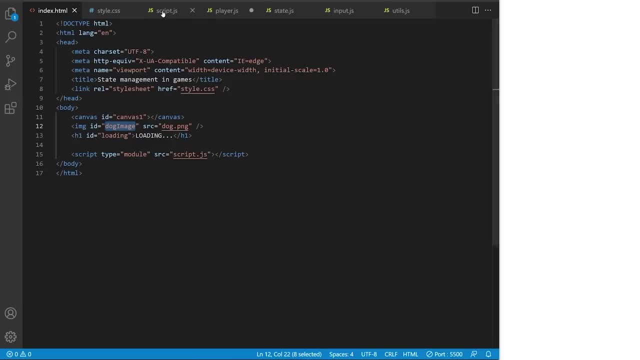 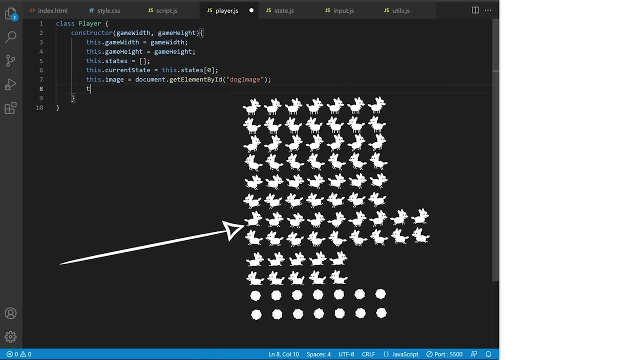 variable towards it using its dog image id I gave it. The dog image is a spreadsheet. It is a multiple frame. When you divide width by number of frames in the longest row- or you can think of these as columns- you will get width of 1 frame. 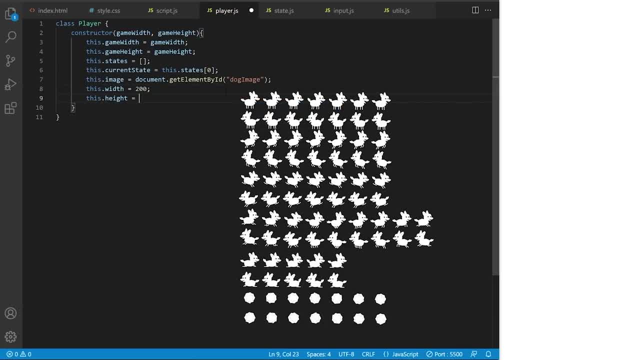 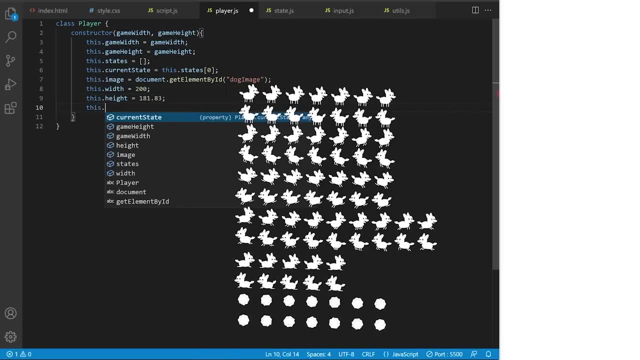 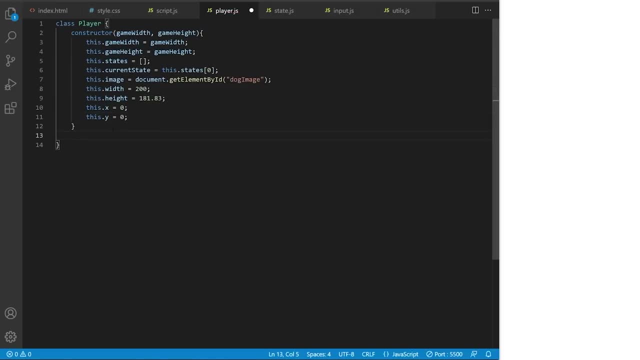 In this case it is 200px. Height divided by the number of rows will give us the height of a single frame, In this case 181.83px. Lets first draw it at x and y coordinates. So from the top left corner of canvas area: 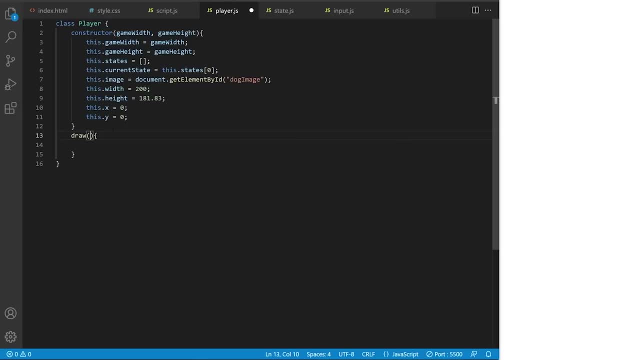 I create a public draw method that takes context as a reference. I will call it x and y coordinates and I will also give it a name. I will have a name argument to specify which canvas element we want to draw on. I call built-in. 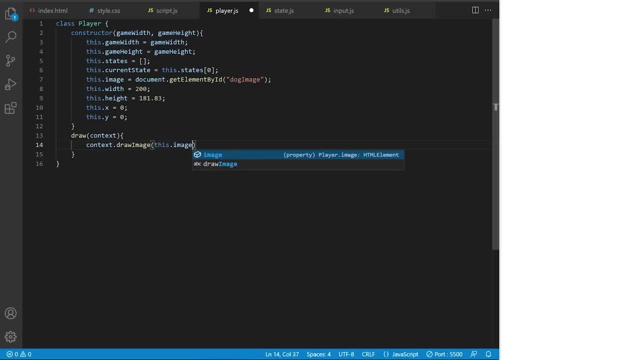 canvas drawImage method. I pass it, my doc image from line 7 and I draw it at coordinates X and Y. So this is our player class. Creating a self-contained class that handles all player functionality is a good example of the first principle of object-oriented programming, called encapsulation. 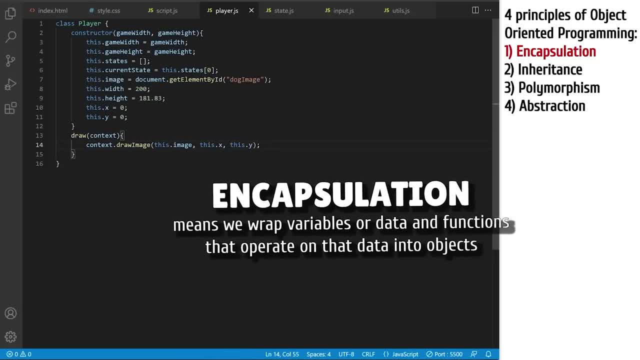 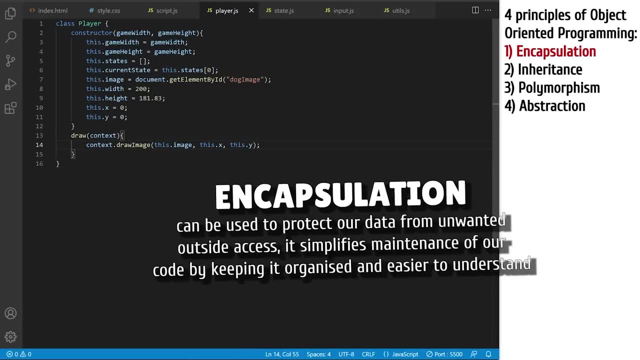 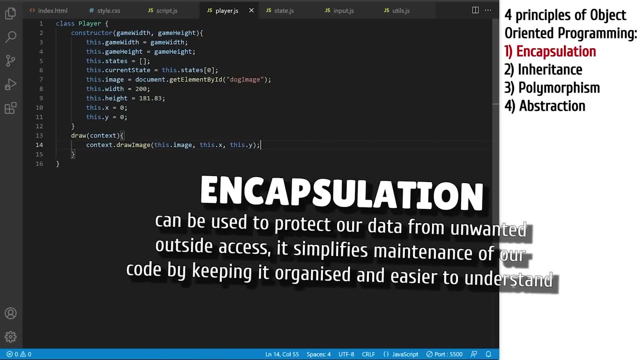 Encapsulation means we wrap variables or data and functions that operate on that data into objects. Encapsulation can be used to protect our data from unwanted outside access. It simplifies maintenance of our code by keeping it organized and easier to understand, Since we are including our main scriptjs. 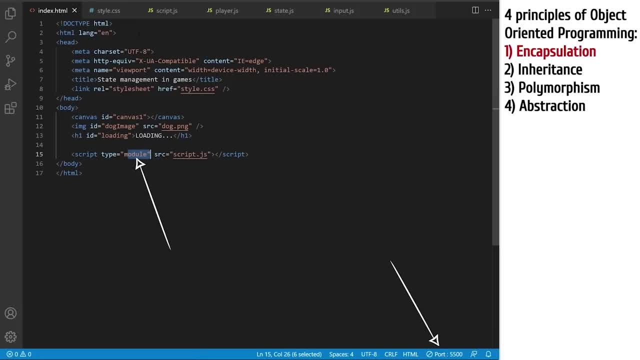 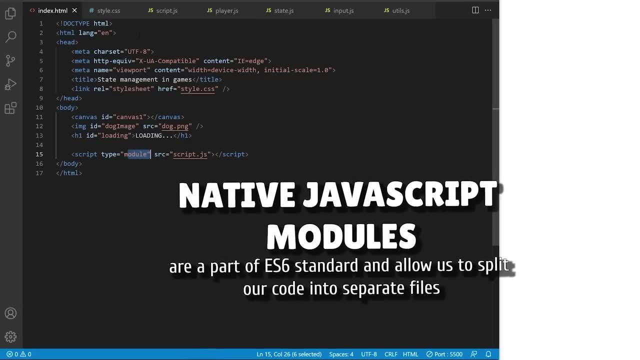 file as a module and we are running our code through a local server. we can use export-import statements. Native JavaScript modules are part of ES6 standard and allow us to split our code into separate files, so-called modules. Members of a single file are called modules. Members of a single file are: 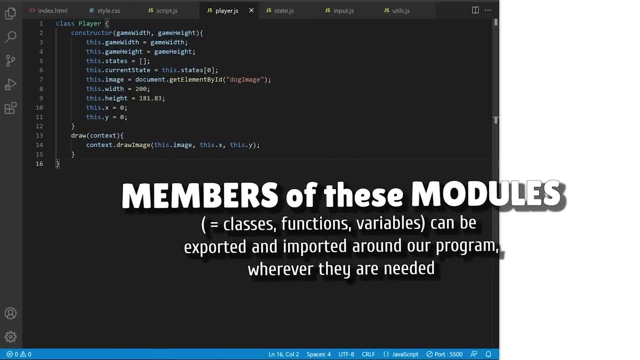 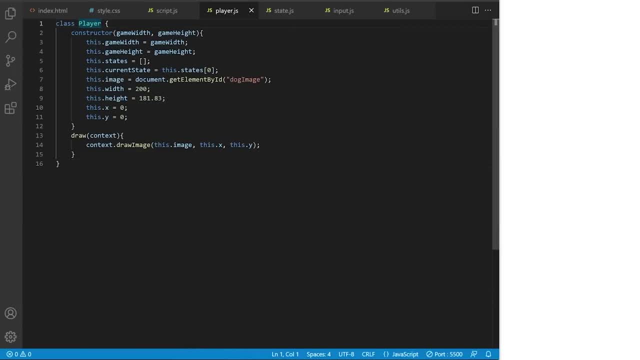 called modules, Members of these modules. so classes, functions and variables can be exported and imported around our program wherever they are needed. I want to export my player class. There are two types of exports: Named exports and default exports. Each module, each file can have only one default export. but 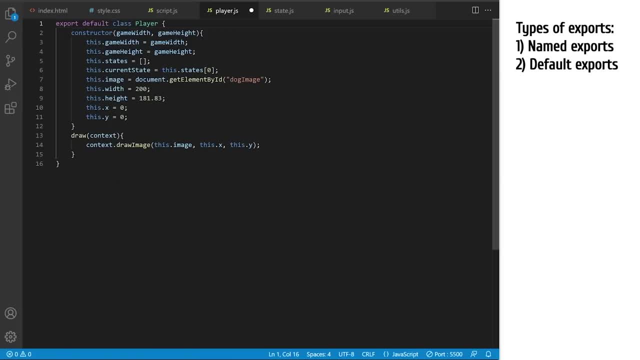 there is no limit on the number of named exports. Named export looks the same, just without this default keyword. To make my player class available in main scriptjs file, I go up top and I say import player from playerjs. This dot slash means that 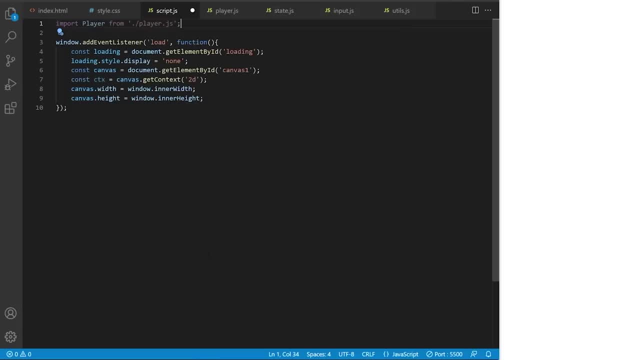 playerjs file is in the same folder as scriptjs. Since player is a default export, I don't need brackets For named exports- exports that don't have default keyword in front of them. I would have to wrap them in brackets like this, but 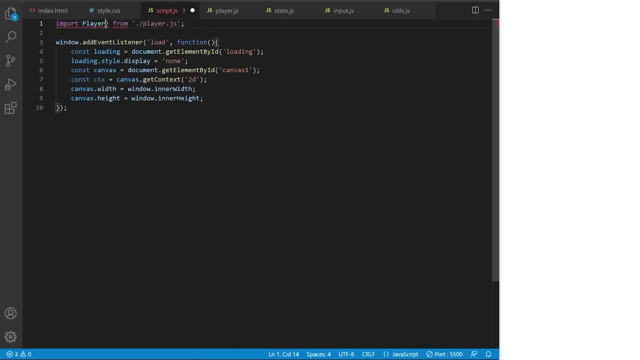 since player class is a default export, we don't need brackets here And I can also refer to player using default here. But there is no need to go into that much detail about modules today. I just want you to understand the main idea and get comfortable exporting and importing. 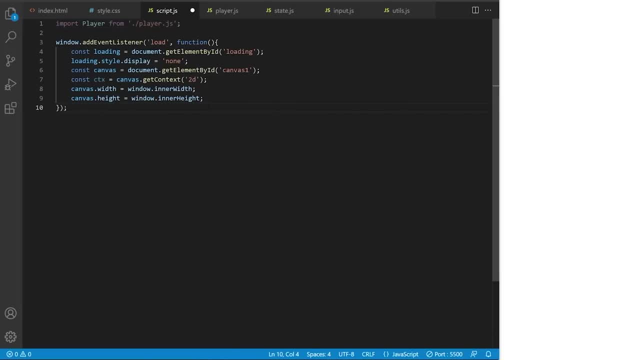 your variables, classes and functions between modules. So now player class is available here. Let's test if it works and instantiate it. I create a constant variable, called, for example, player, and I set it to new player. Here on line 2 in playerjs I can see our player class expects game width and game height. 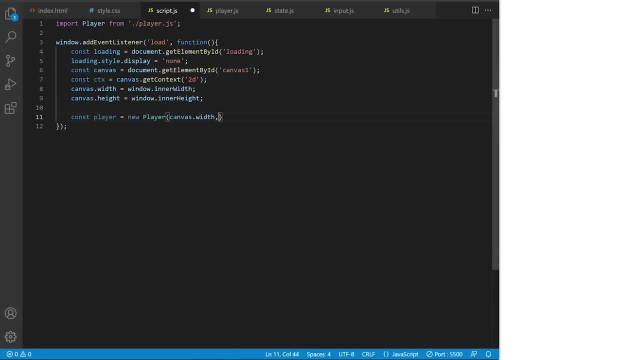 arguments, so I pass it: canvas-width from line 8 and canvas-height from line 9.. If I consolelog player, I can see my object here and I can inspect it to see all its properties and values. Congratulations, now you understand how to use native javascript modules. 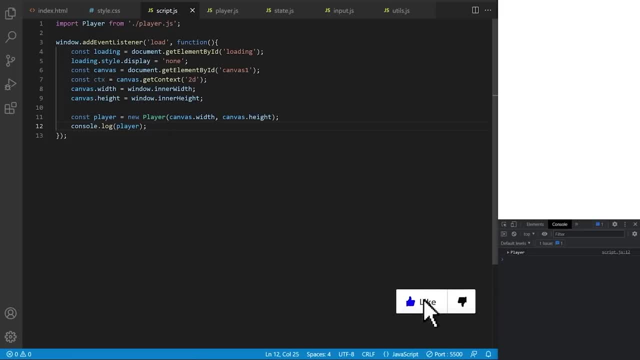 What else should we learn today? Click the like if you are getting any value. We created a public draw method on our player class, so let's call it here. I have an error, because draw method needs an argument for context, otherwise it doesn't know what canvas to draw on. 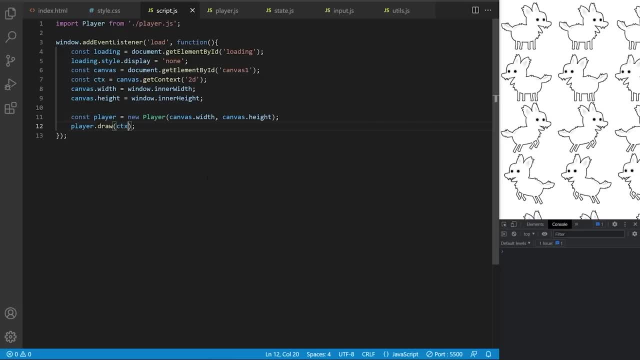 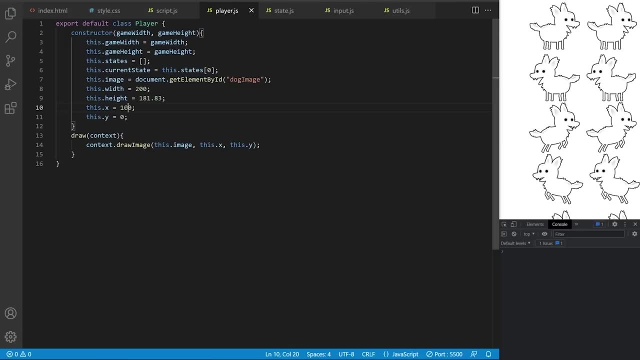 I pass it ctx from line 7 because in this project we only have one canvas element. Nice, we are drawing player image on canvas. What you see on canvas right now is the entire sprite sheet On line 14. here we are telling draw method, what image to draw and what coordinates to. 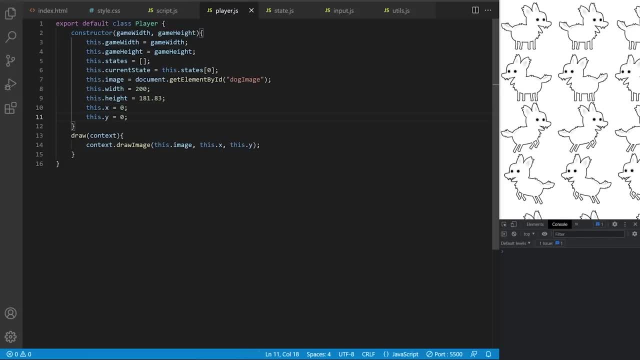 draw it at. Draw method will just take the entire image at its original size And it places it at these coordinates. I can change the coordinates here. Built in canvas. draw image method can take 3,, 5 or 9 arguments, depending on how much. 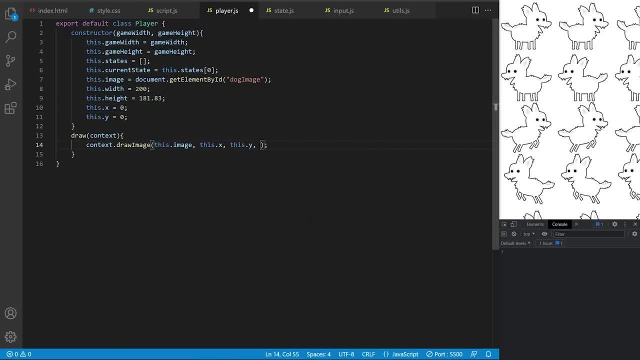 control we want to have over the image we are drawing. If I give it optional 4th and 5th arguments, these stand for width and height and the entire image will be stretched to fill the rectangle defined by these starting coordinates and these ending coordinates. 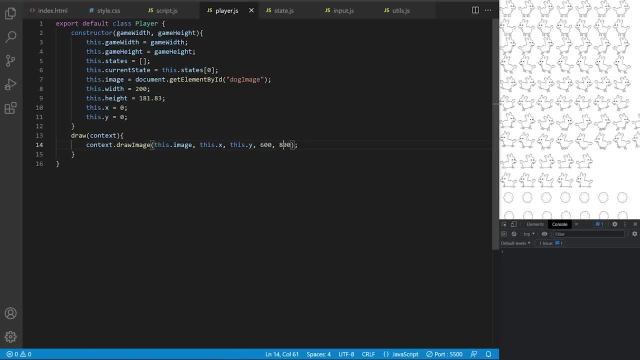 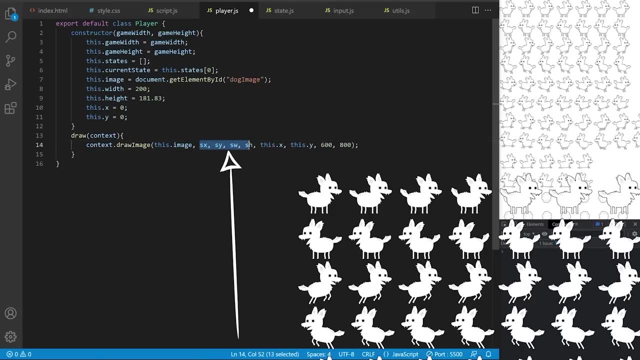 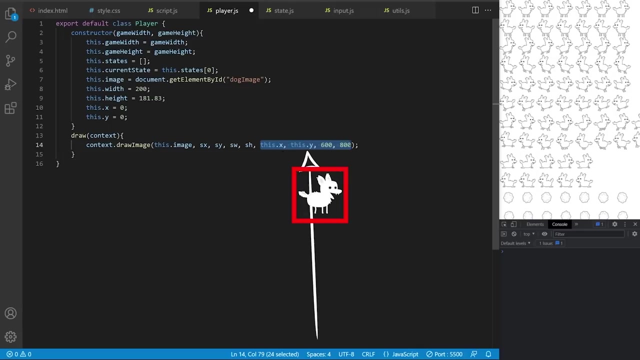 The last longest version of draw image method. The draw image method expects 9 arguments and it gives us full control over the image. We pass it image. we want to draw x- y, width and height of rectangle. we want to crop out from the source image and x- y, width and height of rectangular area where we want to place. 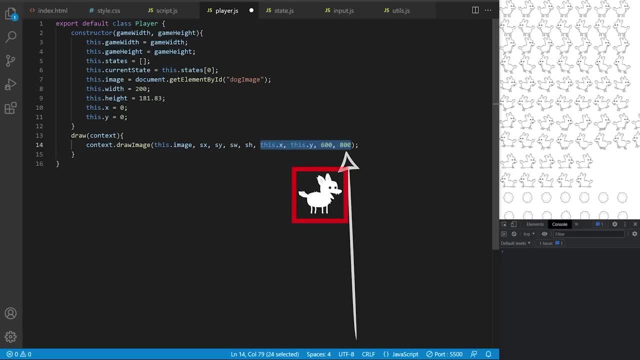 that cropped out piece of image on destination canvas. So right now I want to draw just a single frame from player sprite sheet. So destination values will be this dot x, this dot y, this dot width and this dot height. So destination values will be this dot x, this dot y, this dot width and this dot height. 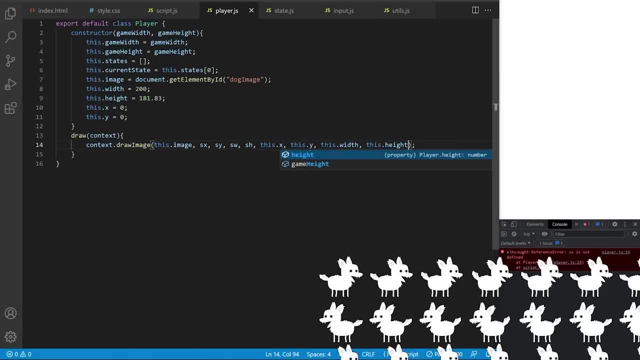 So destination values will be this dot x, this dot y, this dot height, And source values will be: hmm, let's start by cropping out this frame in the top left corner. so from coordinates 0, 0 to coordinates this dot width, this dot height. 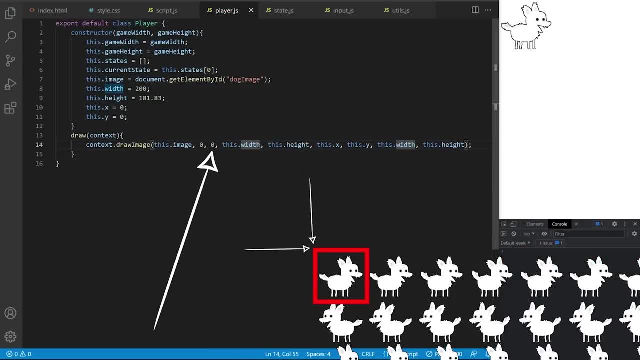 These two values determine start of cropping rectangle. so I can navigate around the sprite sheet horizontally and vertically just by changing these two values. Now I'm traveling along the sprite sheet horizontally. It's not very obvious. on this simple standing animation You'll see we are swapping between frames. 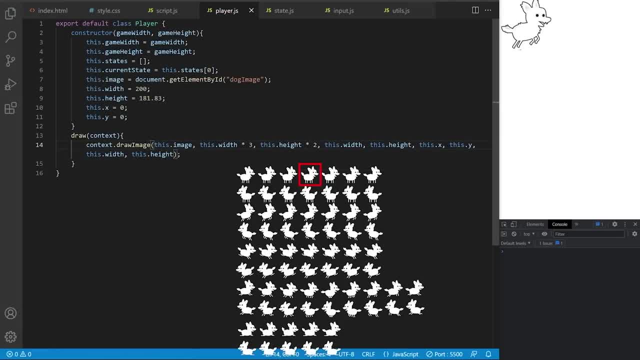 Source y argument here is for vertical navigation. Now I jumped to this frame. I can swap between frames just by changing these values. I might as well put them into separate variables. I create framex variable for horizontal navigation and I replace it here. 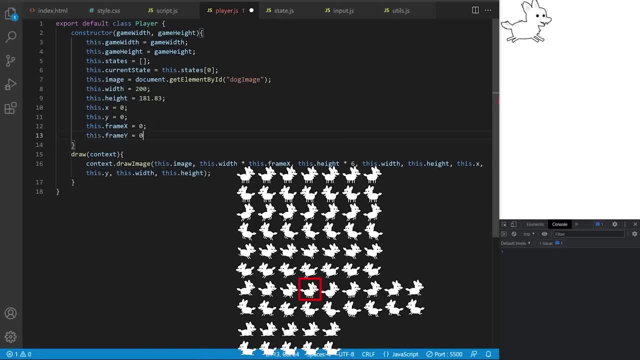 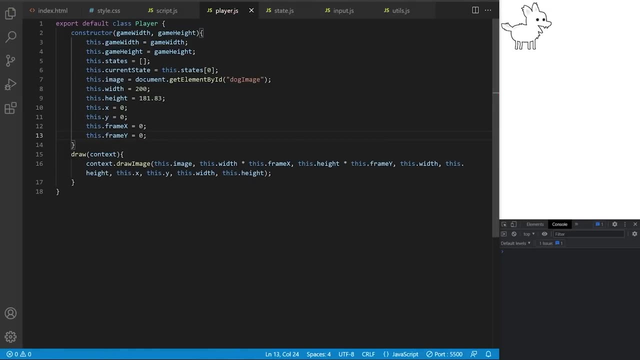 I also create frame y for vertical navigation and I replace it here. Now I can jump between frames in our sprite sheet by changing framex and framey variables. Wow, we covered the main principles of javascript sprite animation so fast today. I have a special class about it. if you want to go deeper, To finalize sprite animation, we just 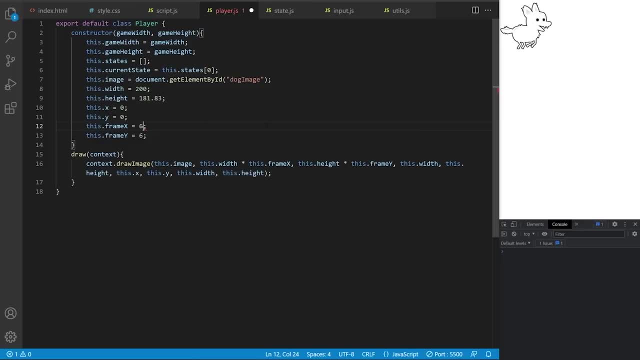 rotate between sprites on each row endlessly using framex property and as we swap between different player states, such as running and jumping, we will be swapping between rows of sprite sheet vertically using frame y variable. Before we do that, let's place player in the middle, bottom of. 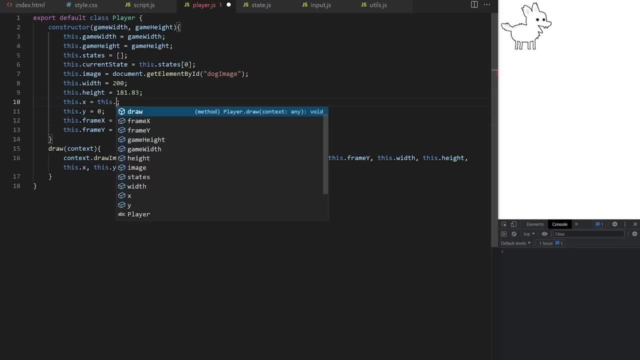 canvas to make it seem like it's standing on the ground. This dot x is a game width divided by 2 minus players width divided by 2, and middle bottom placement is game height minus height of the player. like this, There are many ways to handle keyboard inputs. I want to keep our code clean. 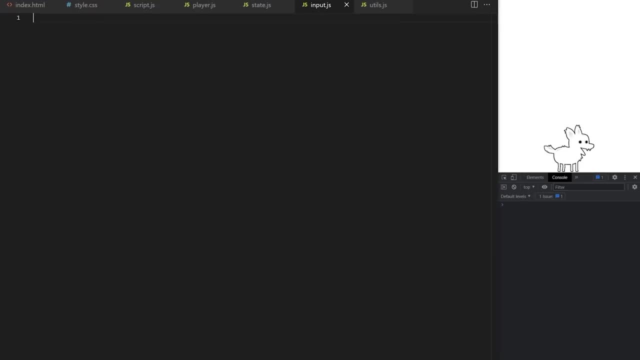 and modular. so I have this inputjs file Inside. I create a default export again and this time it will be a class called InputHandler. This class will be called InputHandler because this class will have the inputjs file. We will use this class to make our inputjs file Inside. I create a 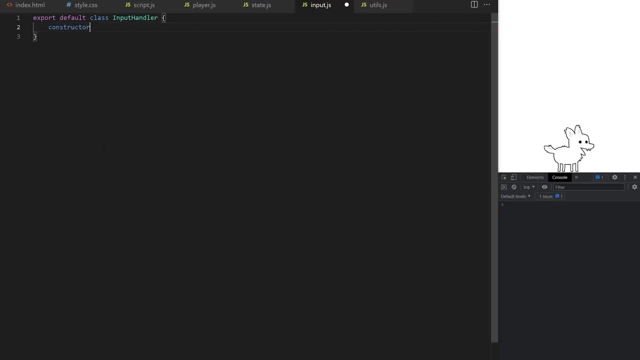 This class's job will be to set up listeners for specific keys and to keep track of the last key that was pressed or released, And it will have only one class property called, for example, thislastKey. This value will be updated every time one of our selected keys is pressed or released. 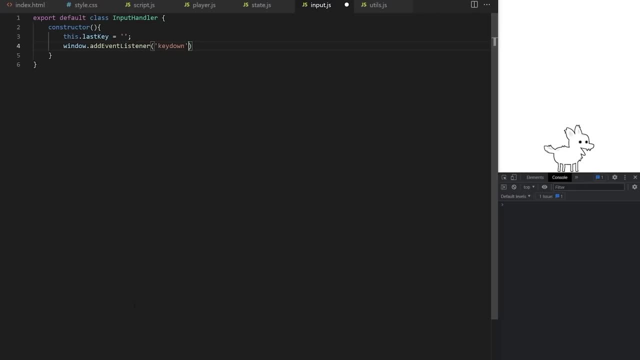 Inside constructor I create an event listener for keydown event Callback function on event listener in JavaScript has this auto-generated event object that is automatically passed as an argument. here I will refer to it as e, for example. This e event object has all kinds of different information about keydown event that just 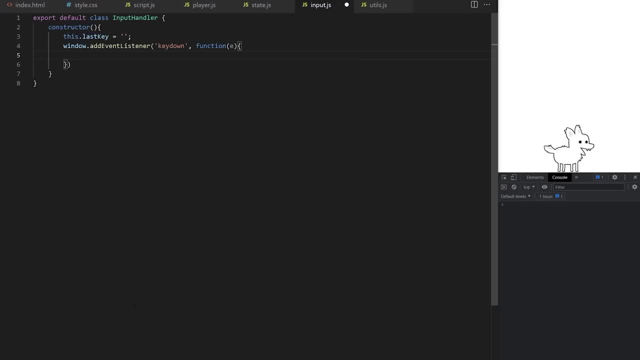 occurred. You can consolelog e to see it. I used it many times before so I know this event object has a property called key that gives us the name of keyboard button that was pressed. I could use, if else, statements here, or I can use a JavaScript switch statement which is: 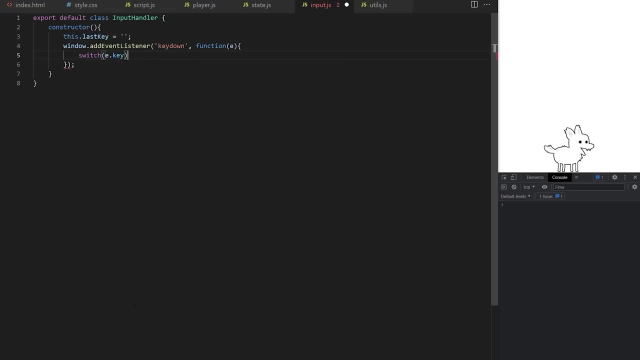 used to perform different actions based on different conditions. We use it to select one of many blocks of code to be executed based on which key was pressed. The syntax goes like this: I open switch statement and I pass it expression to validate. In this case, I wanted to check for value of eventkey which contains name of the key that 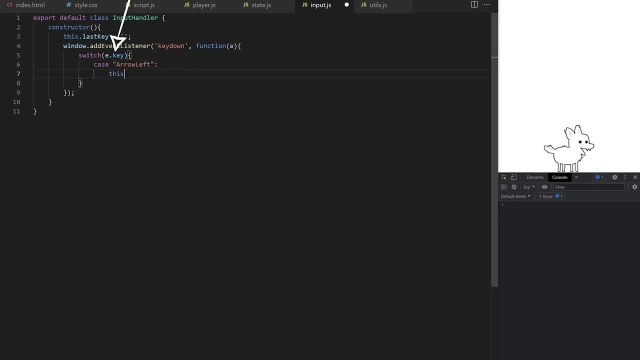 was just pressed. in this keydown event I say case arrow left. and here some code to be executed: if ekey is arrow left In this case, I will take thislastKey from line 3 and I give it value: press left. Make sure you spell it the same as me: it's case sensitive. 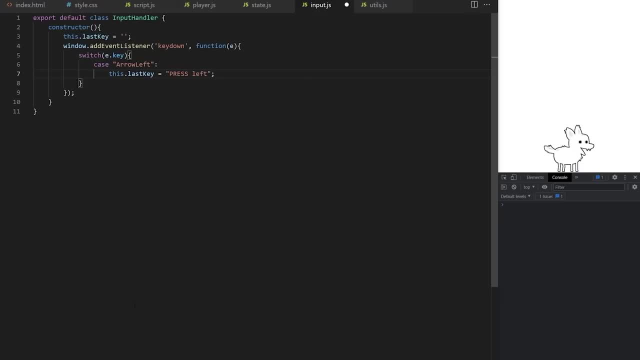 We can have multiple cases here. So far I just have one, but I will add more arrow keys in a minute. Switch expression on line 5 is evaluated once and it is compared with each case. In this case it will check if ekey is equal to arrow left. 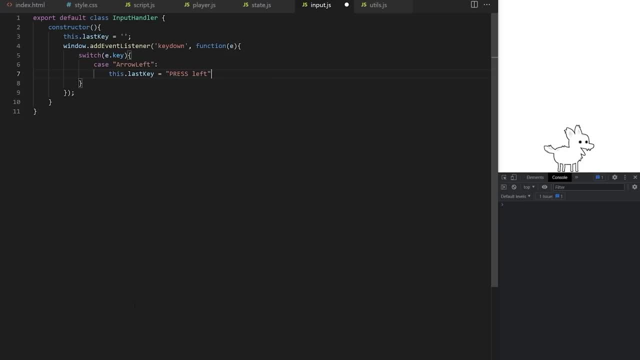 If it is, code on line 7 will be executed. We can also give it default case with code to run if there is no match, But I will not be doing that today. Let's copy this event listener and I change it to keyup event. 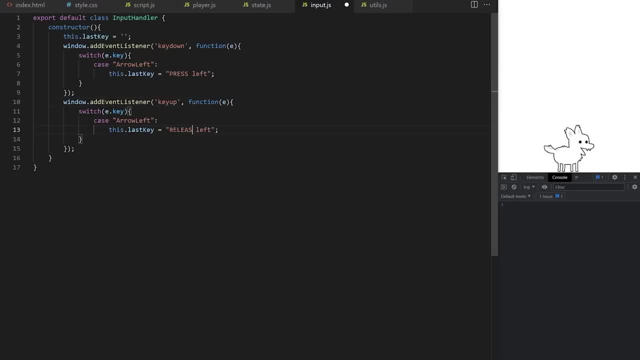 When arrow left is released, I will set thislastKey from line 3 to release left. This way I can keep track of specific keys being pressed and released. I consolelock ekey inside keydown event just to check if everything works so far. 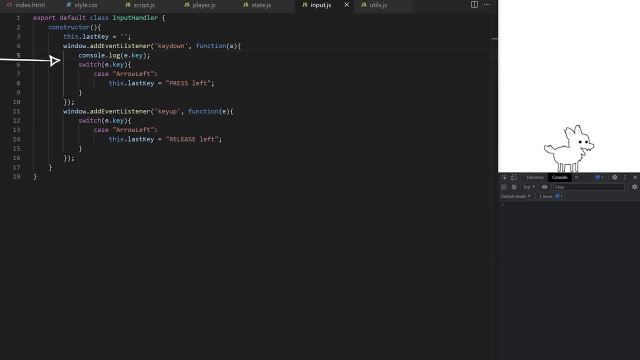 So I have this custom input handler class and all this code is inside its class constructor, Which means all this code will get auto executed. when I create an instance of this class using the new keyword, Instantiating input handler class will automatically attach these two event listeners to our browser. 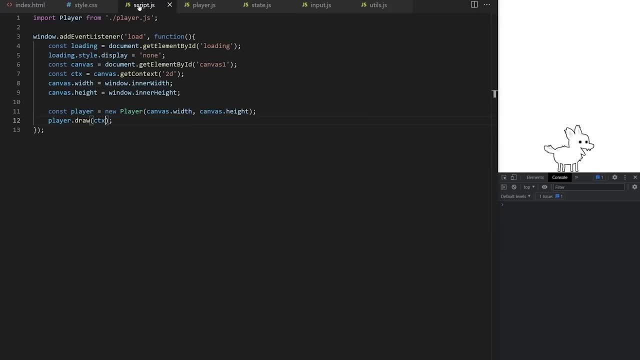 window object. I'm exporting this class here and I will instantiate it from a main scriptjs file by saying import input handler from inputjs. With input handler class available, I create a constant variable called for example input, And I set it to new input handler. 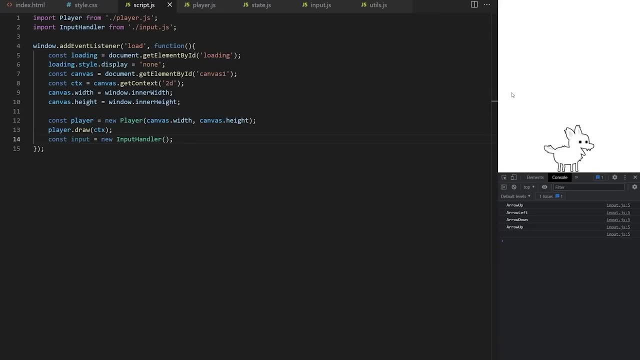 That's it. Now, when I click my canvas and I start pressing keyboard, It will consolelock names of those keys. Those names are values of key property on auto generated event object coming from ekey here. So creating an instance of input handler class automatically executed all the code inside. 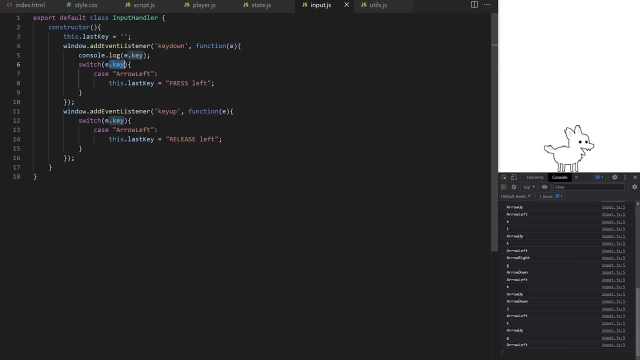 its constructor, which added event listeners to our project. We care only about certain keys, we will ignore others. Right now, Pressing and releasing left arrow key will update this dot. last key property. Last key stores the last keyboard input that was pressed or released. 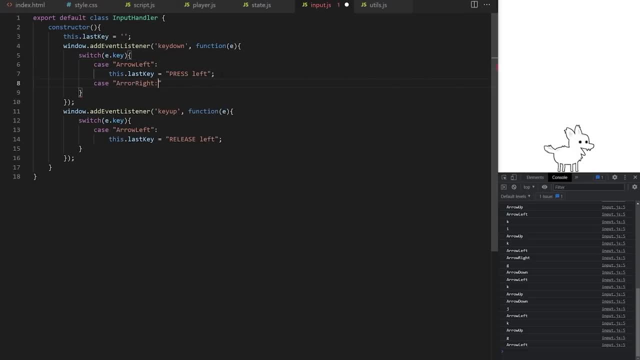 I will add more keys. In key down, I add case for arrow right and I set last key to press right. And in key up- event listener- we set it to release right. I will add break keyword after each case. if we find a match, we don't have to check the. 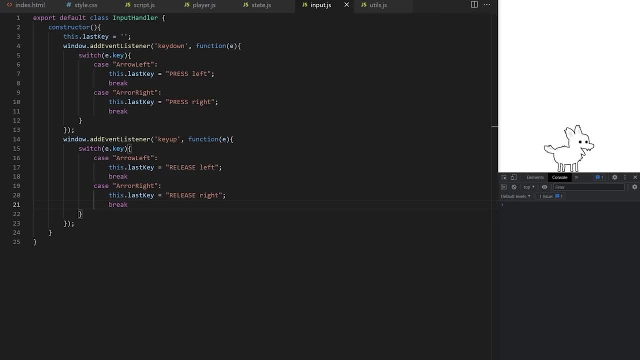 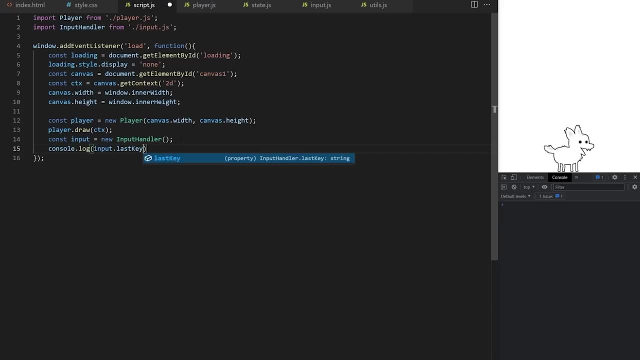 others. We are listening for presses and releases of left and right keys. Let's see if everything works. I consolelock input from line 14.. Dot, last key, which is coming from line 3 in inputjs file. It's not working because we have a problem with this keyword. 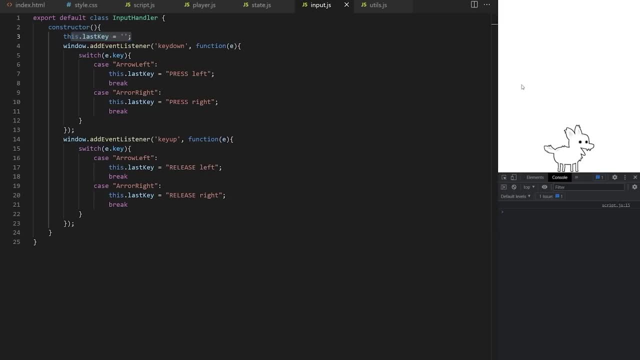 Since I'm attaching event listener to window object from inside a class, I need to bind that reference to this keyword so that when event listener runs this line later, it still remembers that this keyword is still there. So that's it. Thanks for watching. I hope you enjoyed this video. 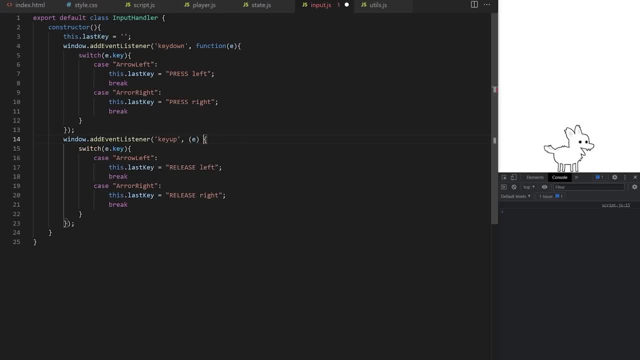 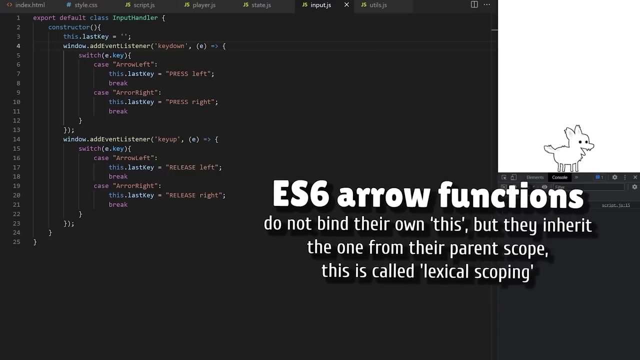 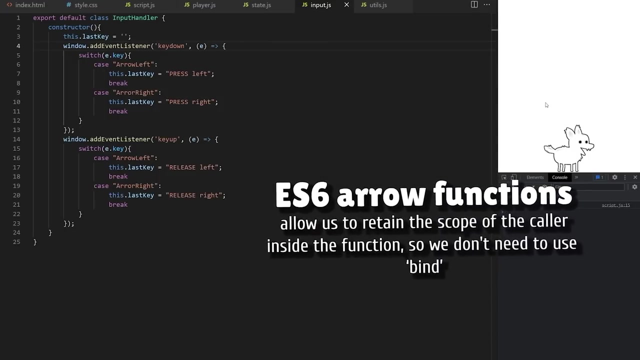 If you liked it, please subscribe to my channel and hit that like button. I will see you in the next video. Bye, bye. Use an arrow function here will make sure these lines of code will correctly remember we are pointing them to this class property. 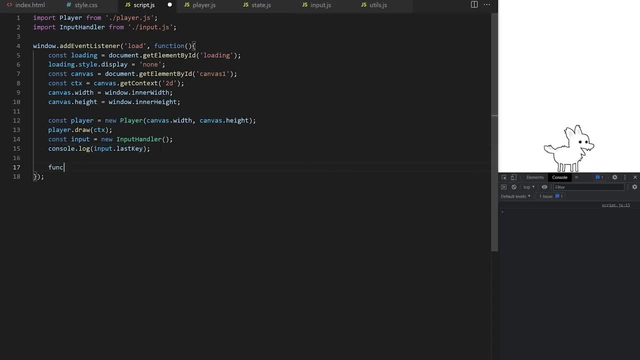 I will also need animation loop, so custom function. I call, for example, animate Inside, I will consolelock input dot last key Request animation frame and I pass it animate, which will create an endless animation loop. I start the loop by calling animate like this: 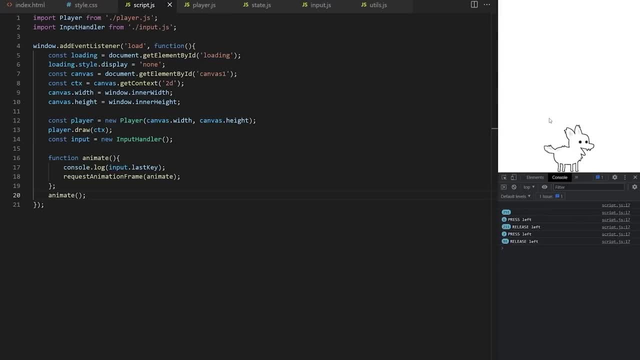 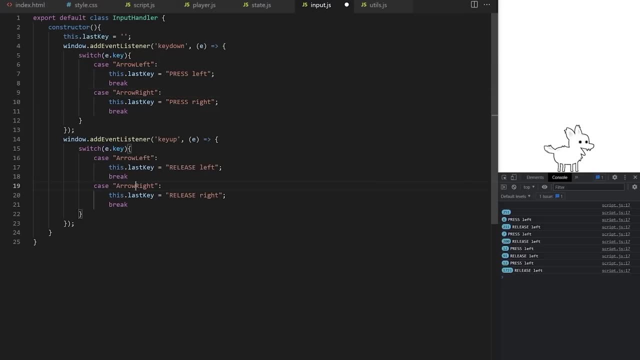 Now, when I click on canvas and I press left or right arrow keys, We get the correct consolelock for left. Hmm, I misspelled arrow right on lines 9 and 19.. Now everything works Great. Utilsjs is just a place where I can have my small utility functions. 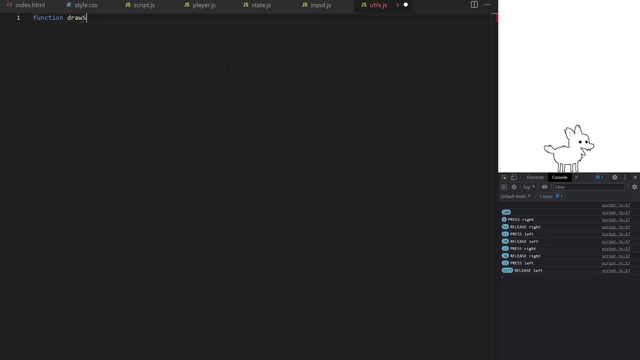 I want the function that will display the last key that was pressed. I want to draw that text on canvas so that I don't have to change the text. That's it, so that I don't have to check console. It will be very simple. 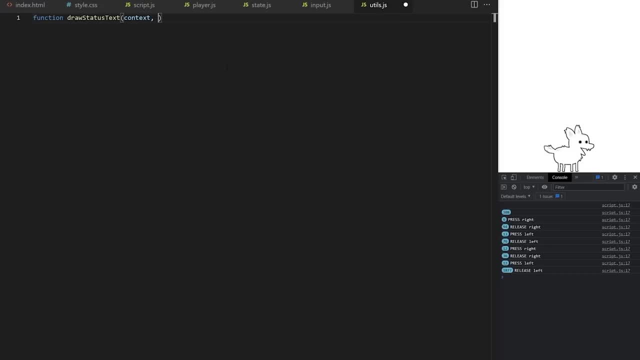 I call it DrawStatusText. It will take arguments for context, the specify what canvas we want to draw on and input so that we have access to the last key value. I set canvas font property to 10 pixels- Helvetica, for example. 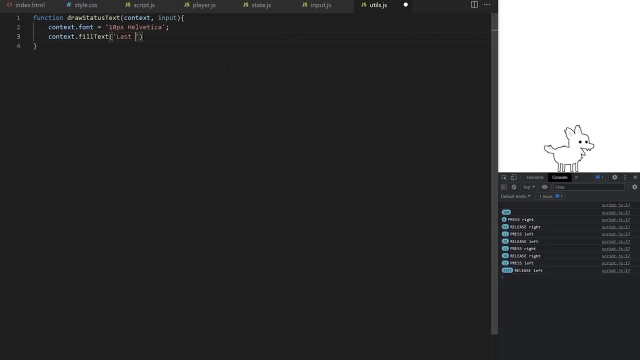 FillText method takes text we want to draw and x and y where on canvas we want to draw it. So I pass it last input colon space plus input dot, last key, and I want to draw it at coordinates 10,, 20, I guess. 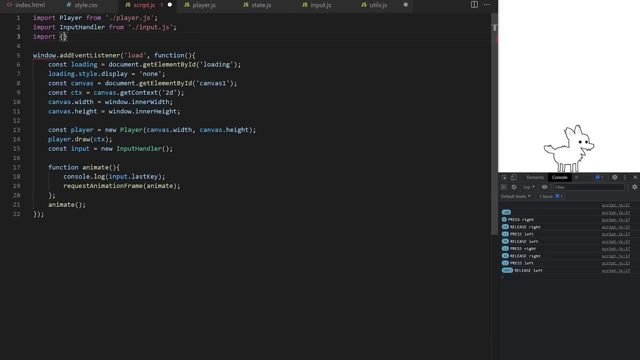 Let's export it and import it in scriptjs This time. I'm not exporting it as a default, so I have to wrap it in curly brackets like this: I import DrawStatusText in brackets from utilsjs and I call it inside animation loop here on line 19.. 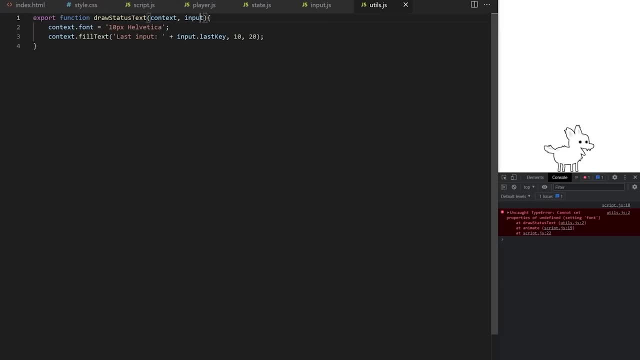 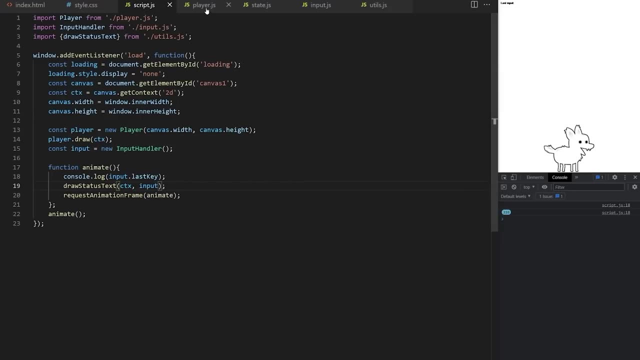 It expects context and input as arguments, so I pass it: CTX from line nine and input from line 15.. Hmm, let's make it larger, maybe 30 pixels, And coordinates 20, 50.. Nice, it works. 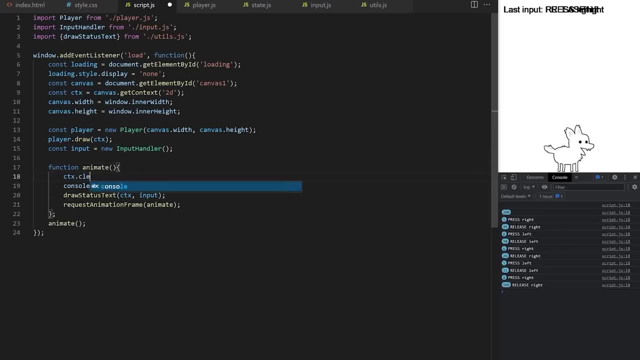 I need to make sure I clear my canvas between frames to delete old paint Built in clear rectangle method and I want to clear the entire canvas from coordinates 0, 0 to coordinates canvas width, canvas height. This will delete my player. 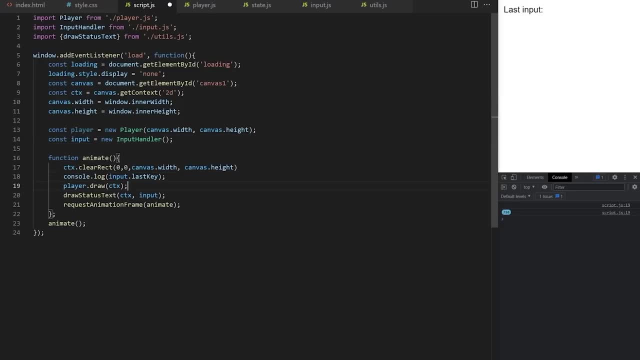 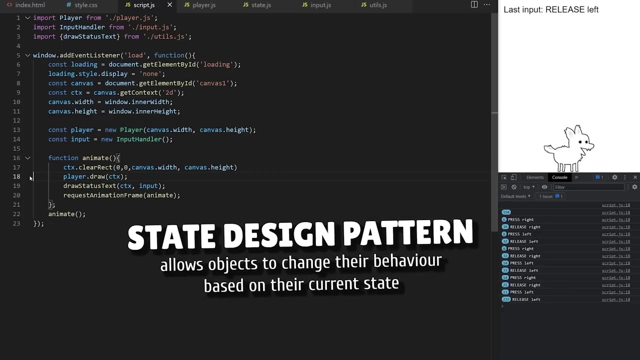 so I have to redraw it for every frame by placing playerdraw inside animation loop. Nice, So far, we only care about left and right arrow keys. When we press them, canvas gets updated. Let's delete this console log. State design pattern allows objects. 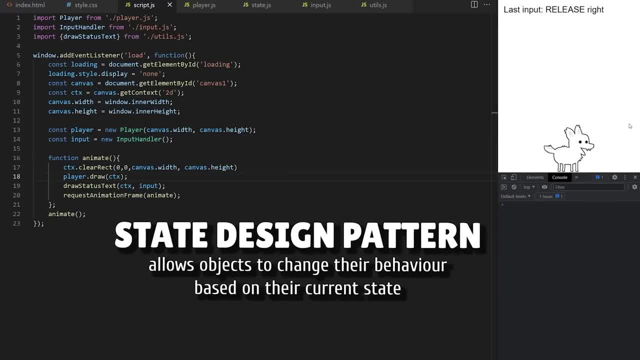 to change their behavior based on their current state. In this case we will start very simple. to demonstrate the main idea, We will swap player between standing left and standing right state Entering each state will draw a different row, a different row in sprite sheet. 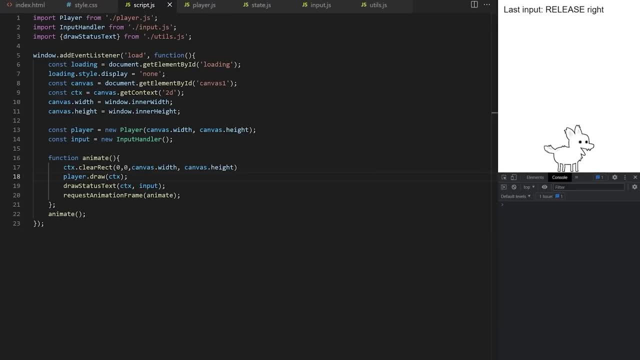 and in each of these states, player will only respond to a limited set of keyboard inputs. When we are standing left, we will ignore additional presses of left key and we will only react when user presses the right key, which will swap us to standing right state. 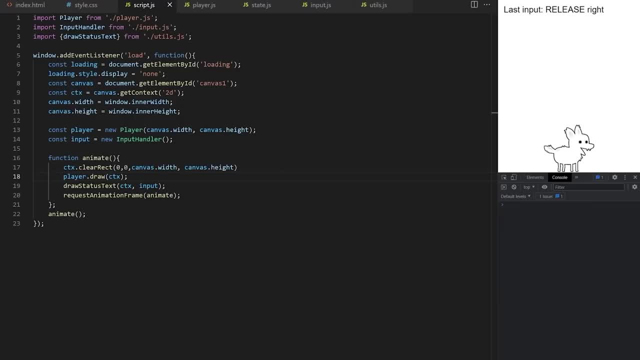 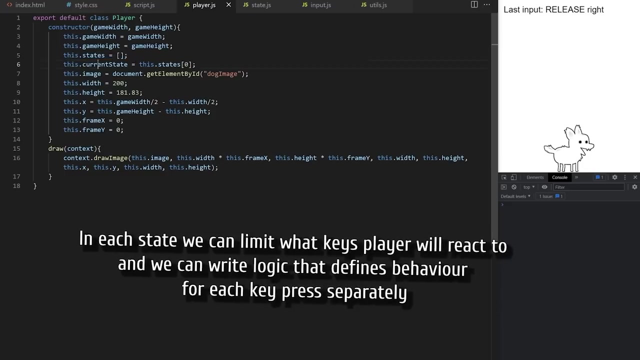 In standing right, we will ignore any additional presses of right key and only pressing left arrow key will swap us to standing left state. In each state we can limit what keys player will react to And we can write logic that defines behavior for each key press separately. 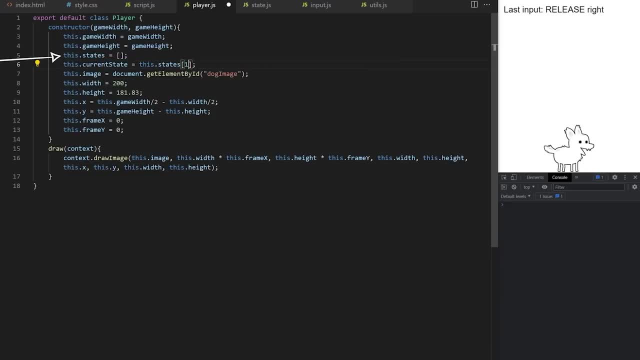 I will keep all potential player states in thisstates array here and I will keep track of the current one in thiscurrent state here. The way this is done is that each state in thisstates array will be its own object, generated by a separate class. 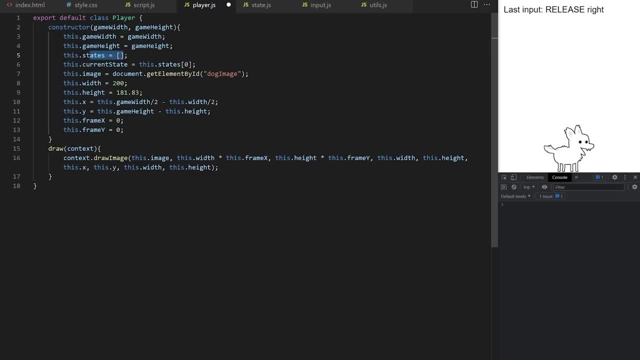 Don't worry, let's go through it now and make sure we explain it properly so that it's easy to understand. In statejs, I will define class for each state. I will define class for each state. I will have an object that will contain a list of all possible states. 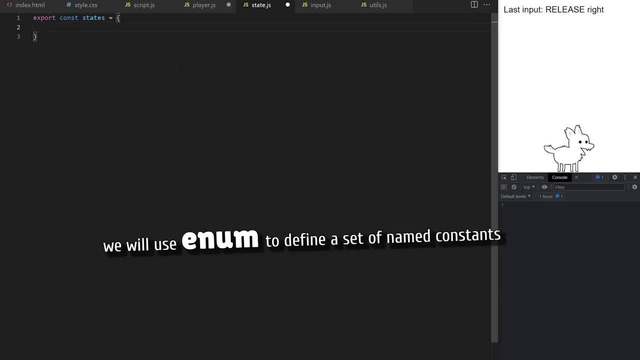 Usually, it's a good idea to use enum for this. In this case, we will use enum to define a set of named constants. We define a name for each state and assign it a number. The order of these states must match the order. 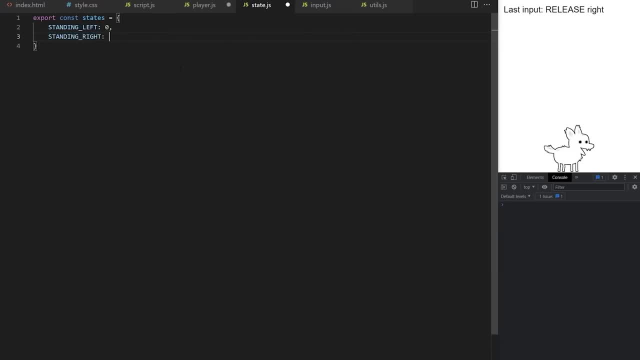 in which we add them to playerstates array, And that way swapping between states will be more readable, because instead of swapping to state zero, I will be able to swap to state standing left, for example. I will be able to swap to state standing left, for example. 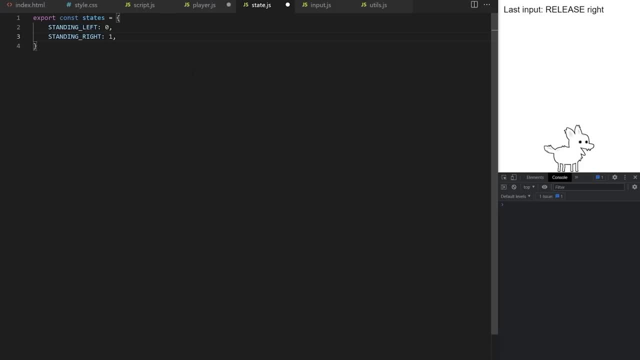 It will make our code easier to read. That's why we're writing this enum statement. I will have just two states at first, to demonstrate the entire logic on a simple example, Standing left will be state zero and standing right will be state one. 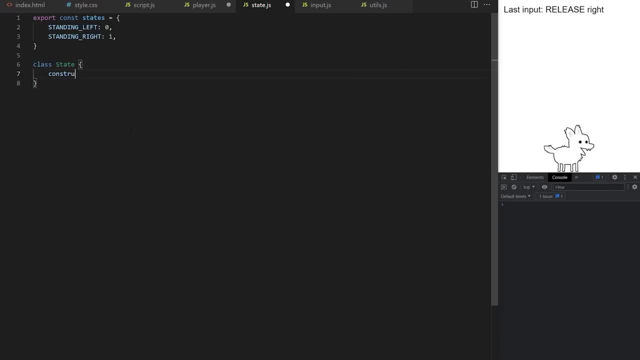 I create a custom class called state. Its job will be just to hold thisstate property, which will be passed to constructor as an argument. It will take this argument and it will turn it into class property. This is just to keep track of name. 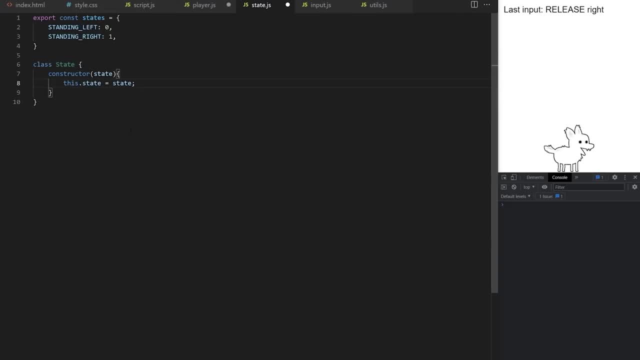 of the active state so that we can write that state name on canvas. In state design pattern, each state is usually defined by a separate class, So let's create a class called standing left and that class extends state class. from line six- Extends- keyword is used to create a child class. 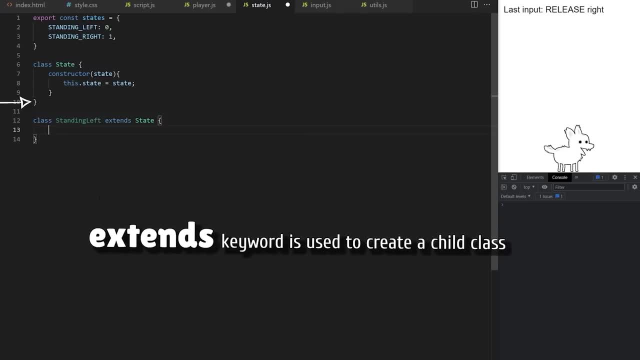 By extending a class, I'm setting up a relationship between these two classes: This is parent and this is child. Extending classes is a good example of one of four pillars of object-oriented programming, called inheritance. Inheritance is a process where one class inherits attributes. 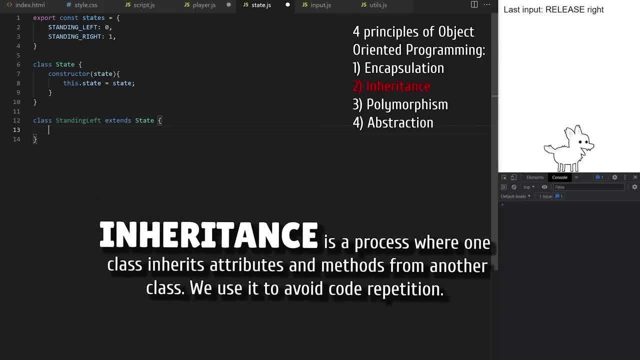 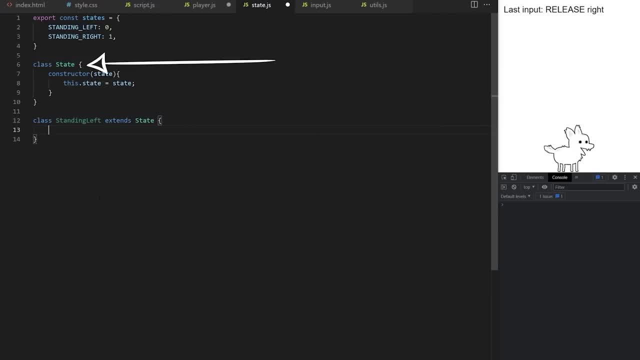 and methods from another class. We use it to avoid code repetition. I will create multiple child classes that all extend this state class. If I want, I can define a method on parent state class and it will be inherited by all child classes automatically so that I don't have to define them on each class separately. 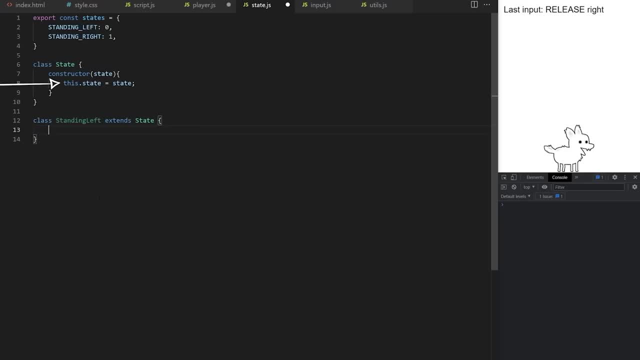 All child classes will also have access to thisstate class. If I reference a method or a property from inside a child class, if JavaScript can't find it on this class, it will go look for it automatically on the parent. So this is our parent class, also called superclass. 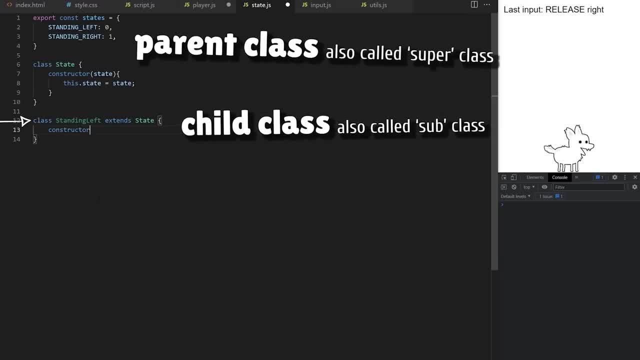 and this is so-called child class or subclass. It will have its own constructor and that constructor will expect player object as an argument, because I need access to player properties on here, since I want to be changing things like playerSpriteSheetRow or playerSpeed as we swap between different states. 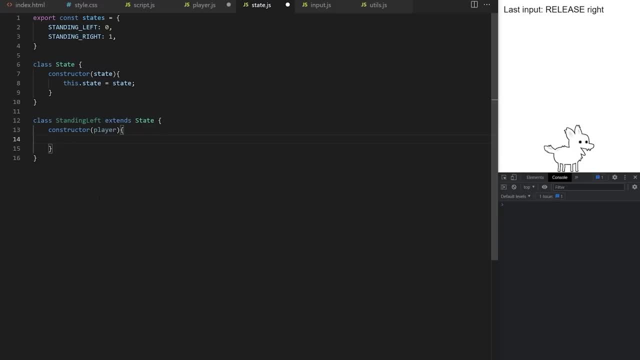 Constructor is automatically executed when we create an instance of a class. So the first thing I will do is use super keyword. We can use super keyword in child classes to access and call methods on objects parent When super is used in a constructor, like we are doing here. 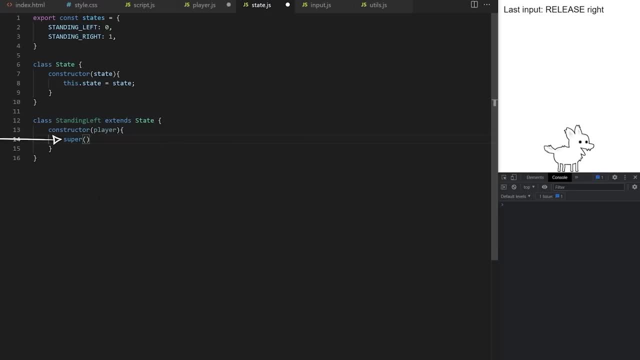 it must be used before this keyword. Calling super here will execute all the code inside the parent constructor on line seven. In this case we need to pass it: name of current state stand in left and constructor will set it as a value for thisstate class property on this particular subclass. 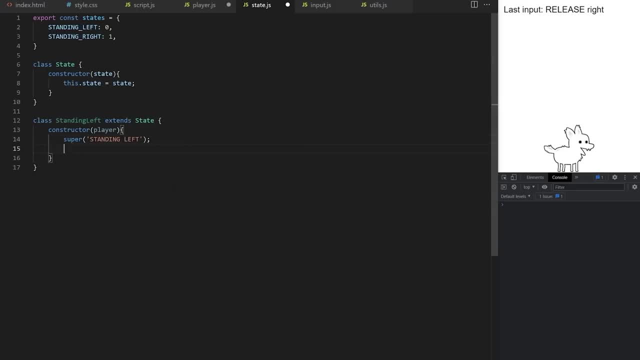 We will just use that to write currently active state on canvas a bit later. Now I take player object passed as an argument and I convert it to class property. here My stand in left child class will have enter method. that will do everything that needs to be done. 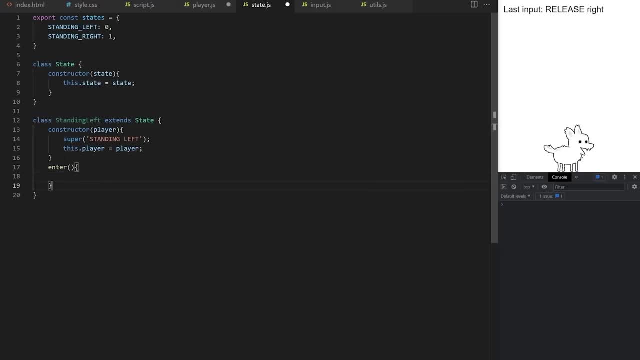 when player enters this particular state, For example, it will change its speed or spreadsheet. Also have handle input method which will listen for a predefined set of inputs and swap to a different state when the correct key is pressed. Enter method will just run once. 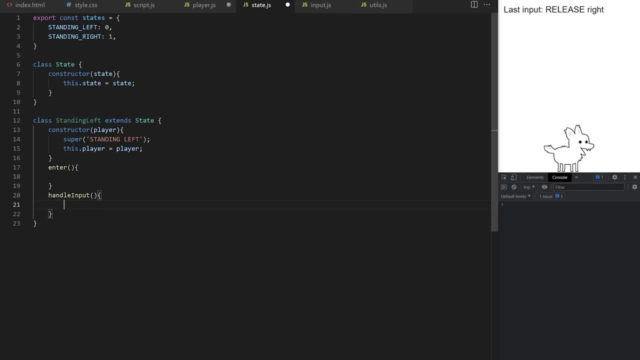 when stand in left state is entered, Handle input method will run over and over for each animation frame. Let's copy all this and make another child class called stand in right. I pass stand in right string to its super class constructor. Notice that we have two subclasses extending one super class. 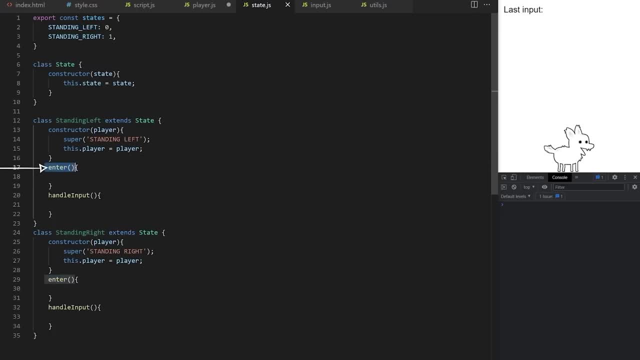 both of these child classes have methods that are named exactly the same. This is very important. Placing methods with the same names on different objects is an example of one of the core concepts of object-oriented programming, called polymorphism. Out of these four concepts, 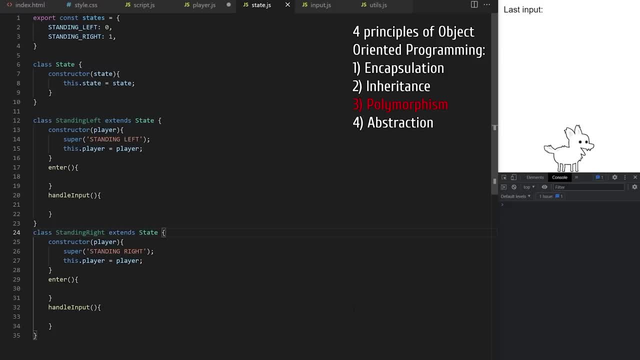 it's the most complex one to fully understand, since it has multiple types. In this case, polymorphism allows methods to display different behavior depending on which class calls it. We will be calling enter and handle input methods from player class using the same line of code every time. 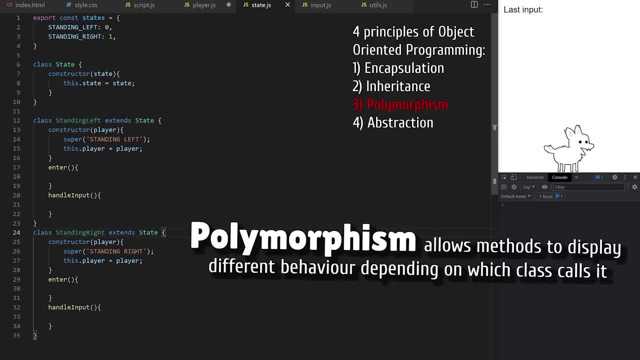 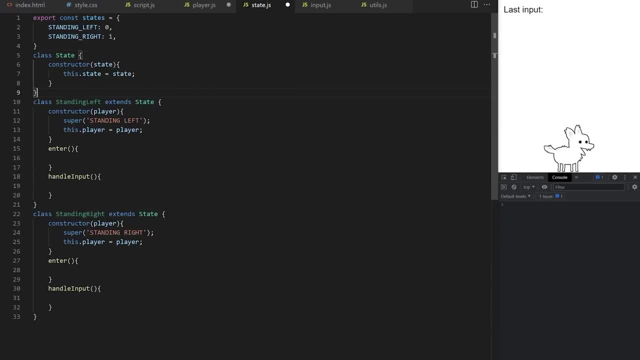 But as player swaps between different states, different code will be executed because enter method and handle input methods will contain different behavior for each player state, for each class. Those differences will be defined here. So for this code to work, every player state class we define. 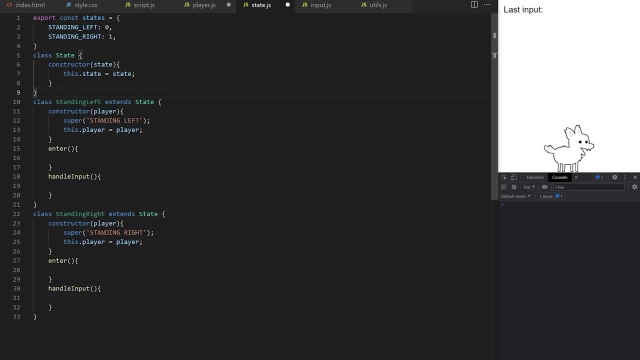 needs to have enter method that runs once every time we enter that state to set things up, and it needs to have handle input class method that runs continuously waiting for specific inputs to be pressed to switch player object to a different state. Handle input method will take input as an argument. 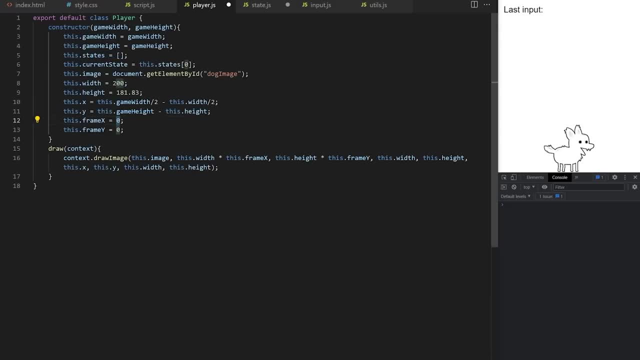 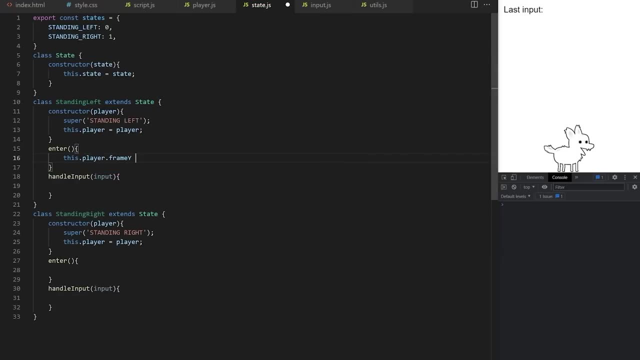 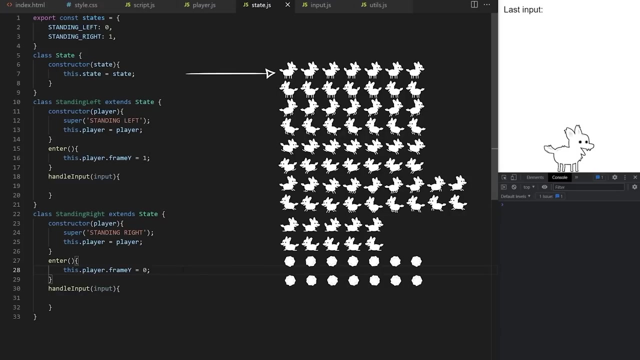 Player object has thisframeY property which determines which row of player sprite sheet we are animating When we enter standing left state. I want to animate row one Standing right. animation frames are on row with index zero, The main principle of state management pattern. 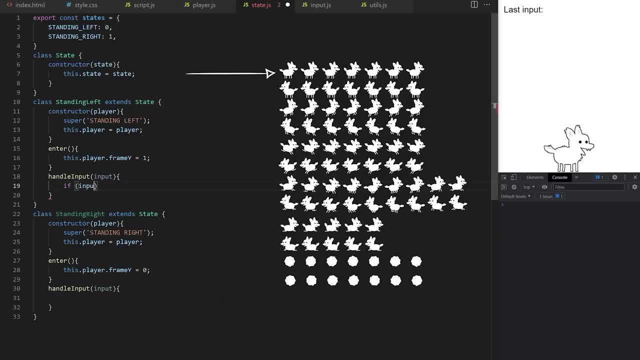 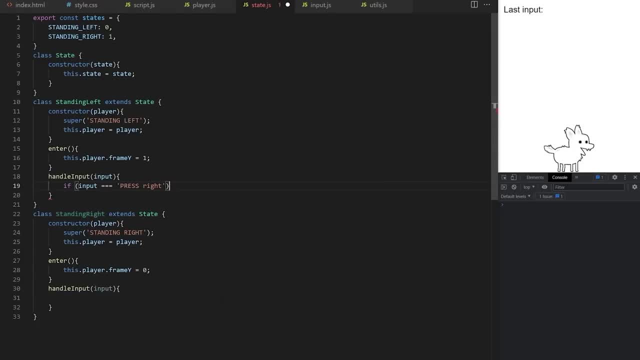 is that when in specific state, object will only react to a limited set of inputs, Other inputs, for which we don't define behavior here, will be ignored. So inside standing left class, if input is press right, we will set state to standing right. 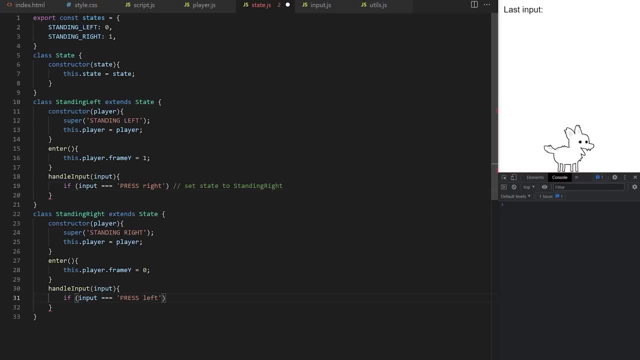 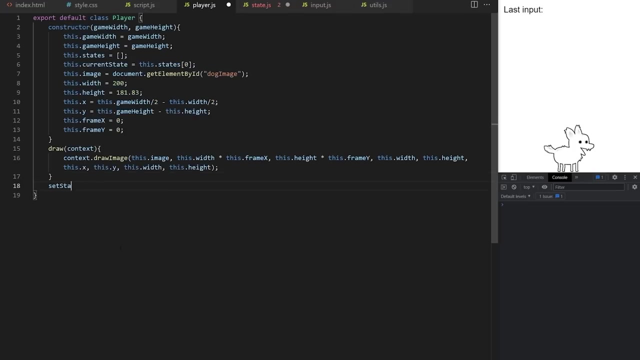 When player object is in standing right state and input is press left, we will switch player to standing left state And the final piece is the mechanism that will actually allow us to swap player to a different state. That code will come here. I create a custom public method on player class. 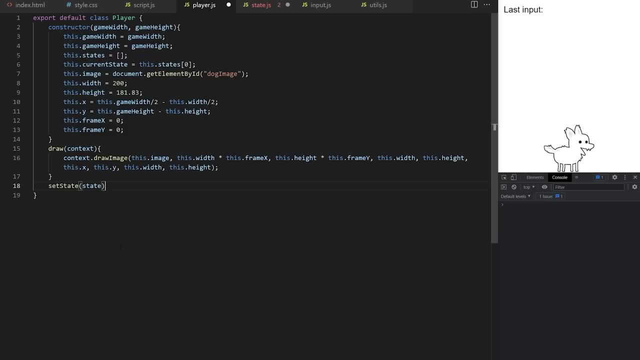 called for example, setState, and it will take the new state as an argument. Inside I set thiscurrentState from line six to thisstates from line five and index will be this state number we passed as argument. Of course, this will only work. 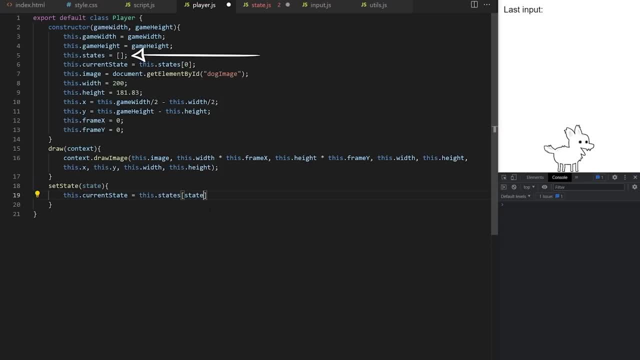 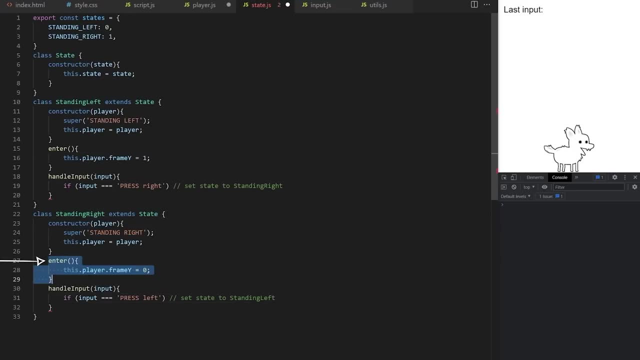 if thisstates actually contains some states. Right now it's empty. We will fill it in a minute. We know that each of our states has enter method which will run once when player enters that particular state to set up our sprite sheet to make sure we are animating the correct row. 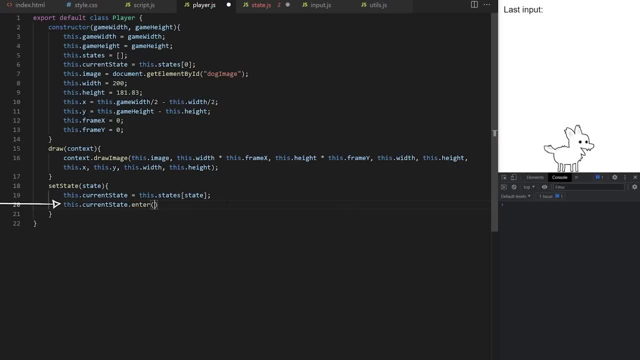 Back in setState. we switch player to a new state and we call that enter method. If we pass it one here, enter method will be called on standing left state. If we pass it zero here, method will be called from standing right state. 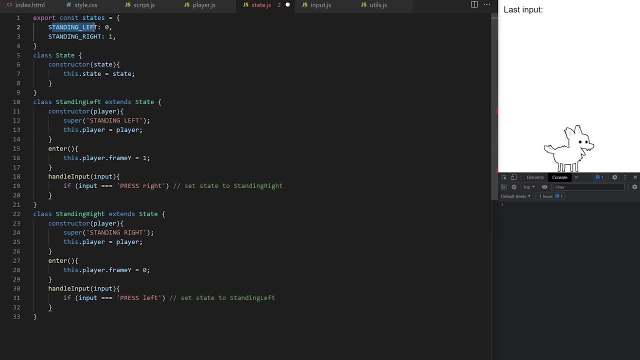 Because in our enum we gave standing left state, because in our enum we gave standing left state a value of zero and standing right state is value one. So now we have a public method that can swap player between different states. 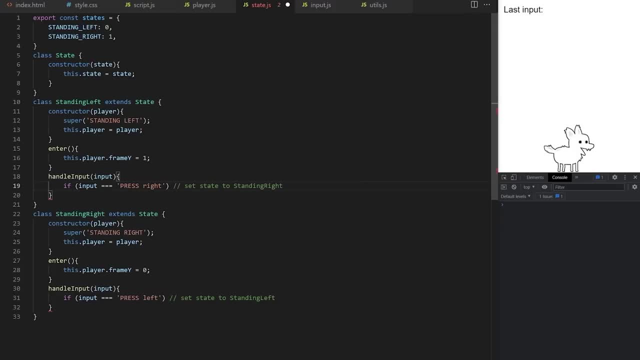 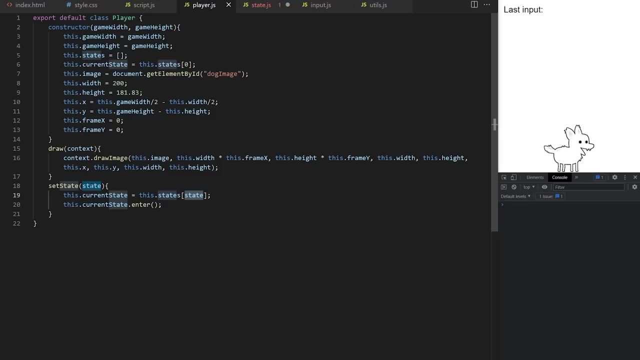 If player is currently in standing left state and handle input method detects that we pressed right arrow key, we call it thisplayersetState and on line 18 here I see it expects state as an argument. That argument will be a number. Right now we only have two states. 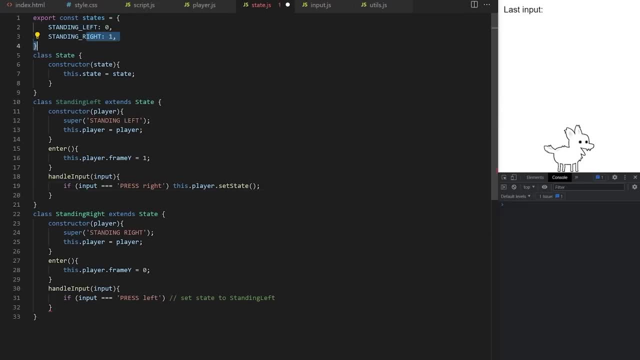 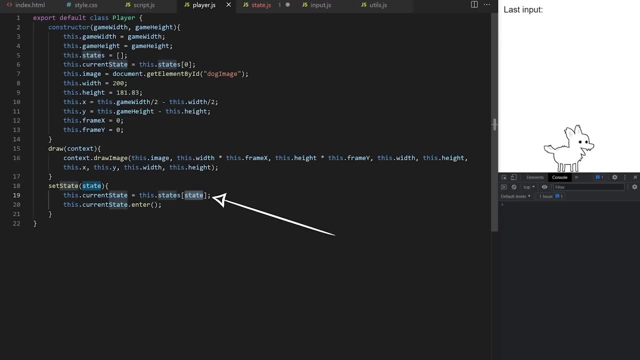 So either zero for standing left or one for standing right will come here. You can see we say thisstates and index in square brackets. So we are referring to thisstates from line five. Again, we will fill this array. 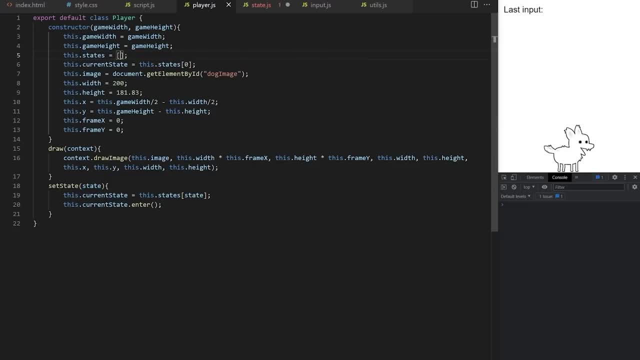 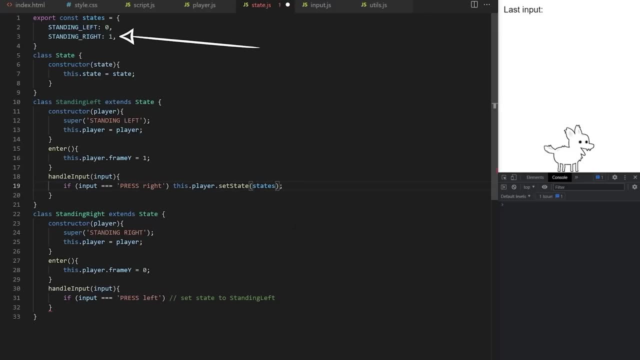 with state objects in a minute So I want to swap player to standing right state here. I can see standing right is one here, So to pass it number one. I pass it. states from line one, dot standing right from line three. This entire enum object is here. 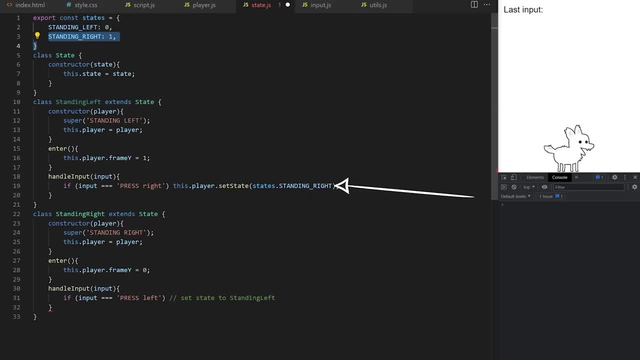 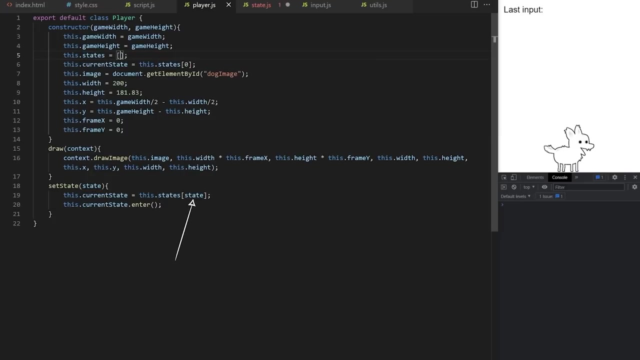 here just to give me more readable values to these numbers that represent states. It would also work if I just passed it number 1 directly here, But number 1 passed. the setState method will be passed here on line 18 as an argument and thiscurrentState will be assigned. thisstates from line 5, index 1.. 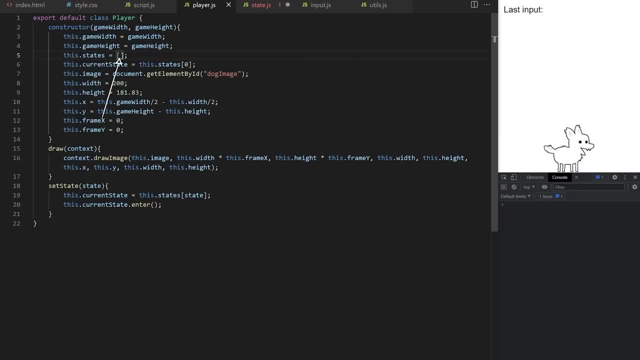 This array will need to have two elements, as we have two states: element with an index of 0 and element with an index of 1.. These will not be just simple numbers like this. These will be entire instances of standingLeft and standingRight class. but before I can use 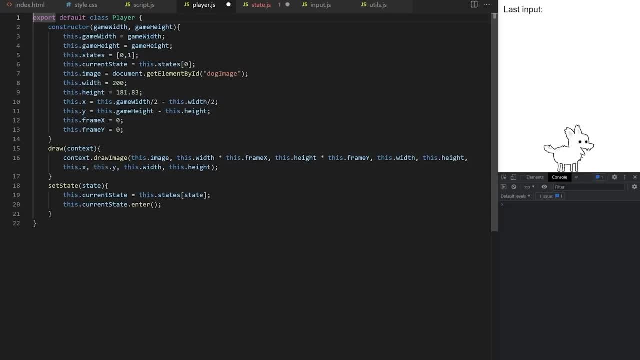 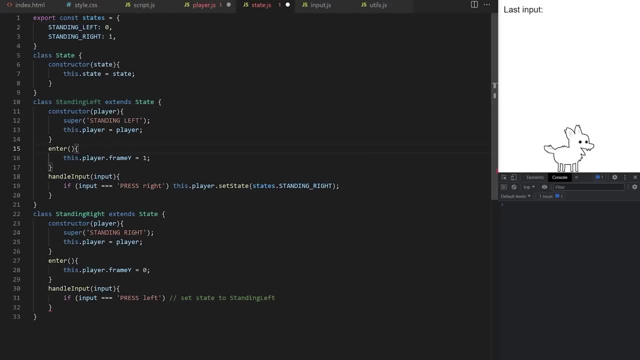 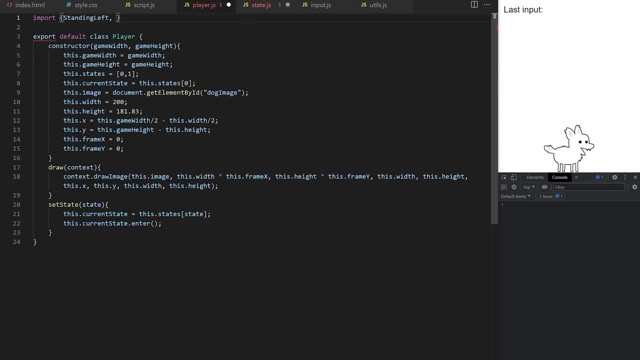 those classes here in Playerjs I need to import them. To import multiple classes from the same file, we need to wrap them in brackets. In Statejs I export standingLeft class from line 10 and standingRight class from line 22.. In Playerjs I import both of them from Statejs like this: 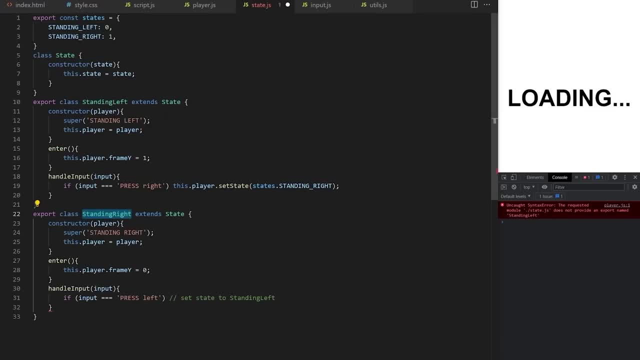 I need to make sure I save changes to all files. I have an error because I didn't finish this other if statement. If player is in standingRight state and handleInput method detects, we pressed left arrow key, call setState on player class and pass it number 0.. 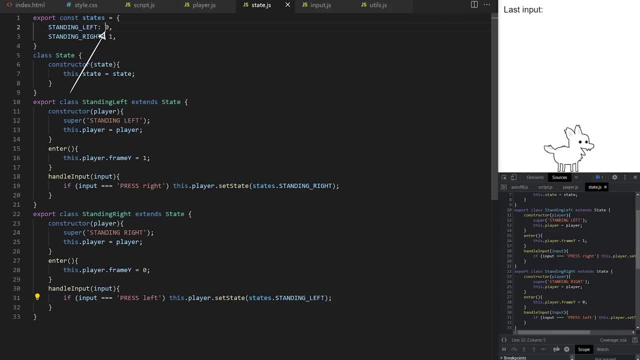 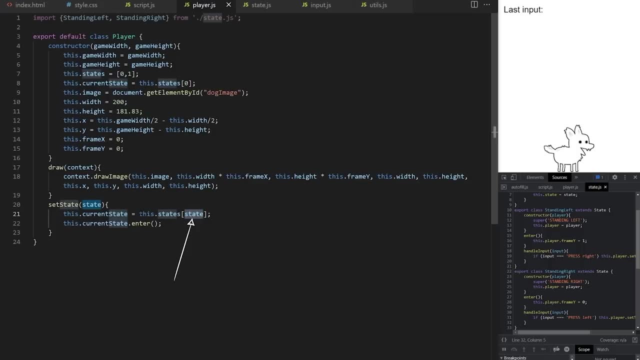 statesstandingLeft. This stands for 0, so 0 is being passed here to setState and thiscurrentState is set to thisstates from line 7, index 0, which is this: Now we need to change this. Now we can finally define our states here properly. so index 0 in playerStates array. 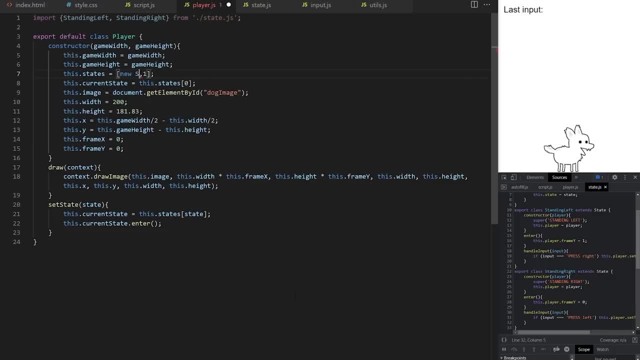 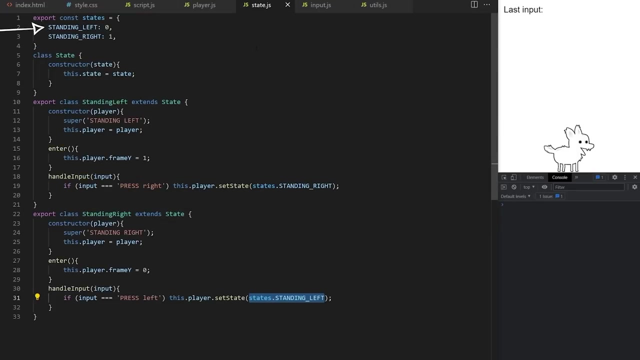 will be an instance of standingLeft class. so new standingLeft and index 1 will be new standingRight. We need to make sure that state objects in this array have the same indexes as numbers we defined for each of these states inside enum. here, Now that we can swap between states, I also need to be calling handleInput method over. 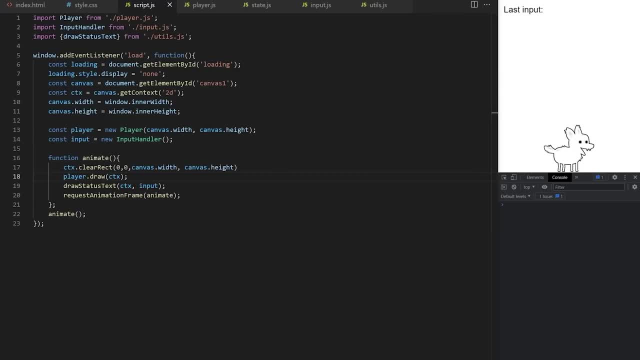 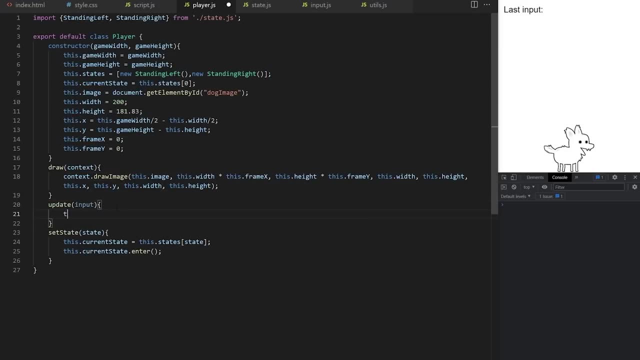 and over so that we can listen for new inputs. I create an update method on player class and it will take input as an argument. Inside this method, I will be periodically calling handleInput from thiscurrentState property from line 8.. This property represents currently active state. 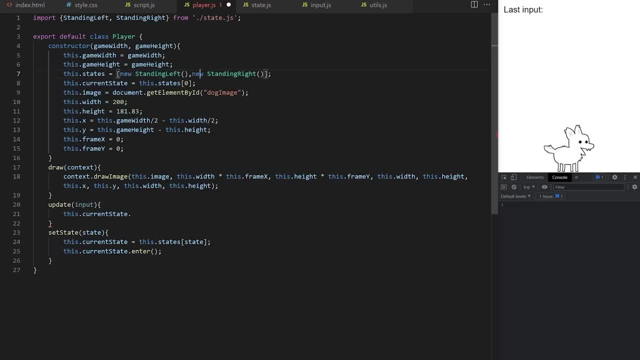 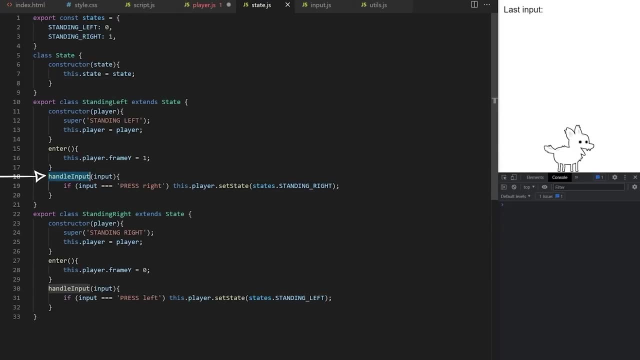 Because of logic we defined on line 24, so player will be either in standingLeft or in standingRight state. It will call either handleInput method from line 19- that reacts only to pressRight, or handleInput method from line 19.. I call it like this and I pass it input that we passed here as an argument. 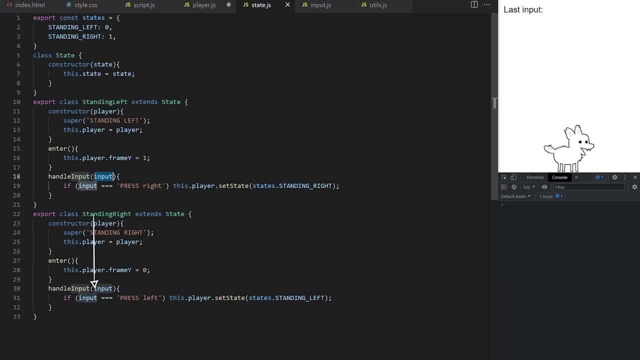 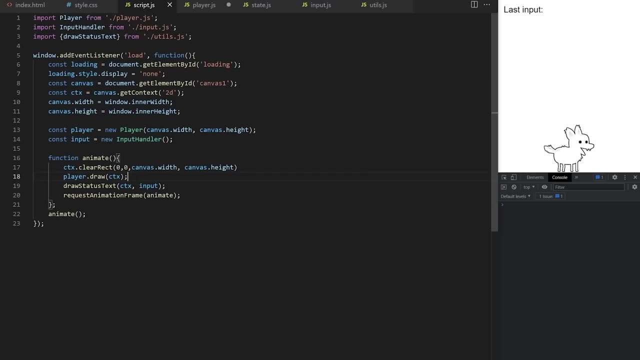 That input then comes through here so that handleInput method can check what was pressed and if the right key is pressed it will swap player states. We call playerUpdate. we just wrote from animation loop and I pass it. input from line 17, dot. last key from line 3 in inputjs. 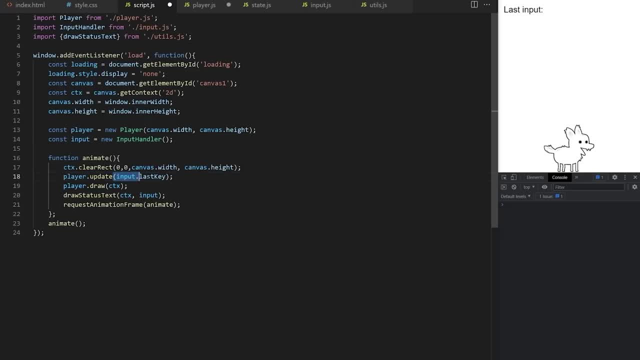 We are done. We just wrote the entire logic. This is for state management of player object. Let's quickly follow the logic one more time to make sure it's clear. We are calling update method for every animation frame and passing it. input dot last key. 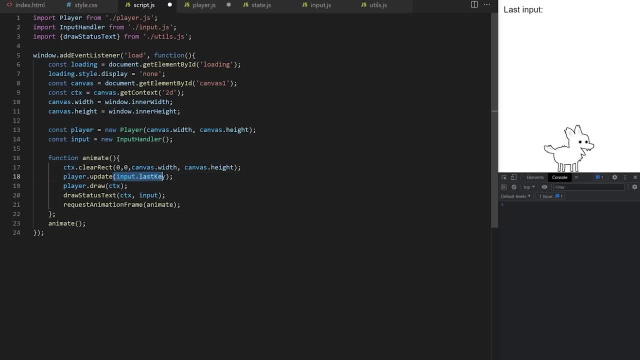 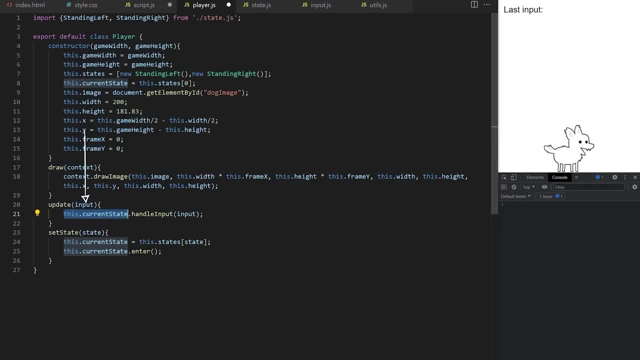 The last key from selected inputs that user interacted with. That input last key is passed here. This time I call it just input and I pass it to thiscurrentState from line 8.. Dot- handleInput And I pass that same input value along. 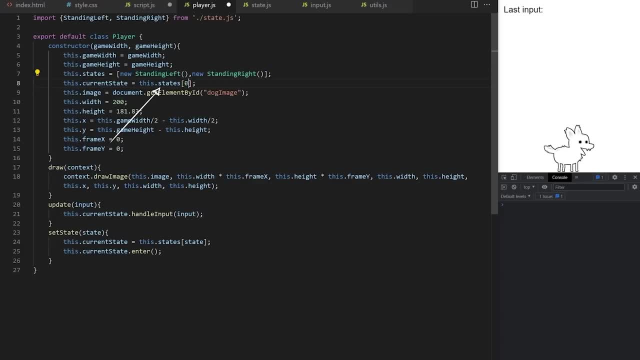 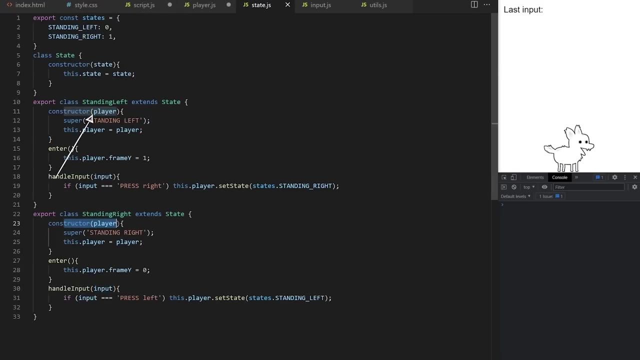 This dot currentState represents the entire state object. First I am setting it to thisstates index 0, which is this standingLeft object. So for this animation frame, handleInput will be called from standingLeft class. So from here I can see constructor for standingLeft and standingRight expects player as an argument. 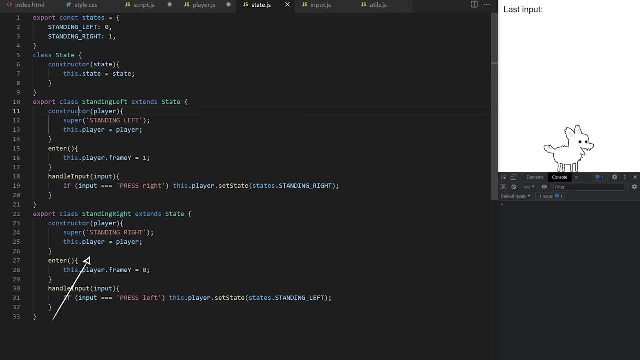 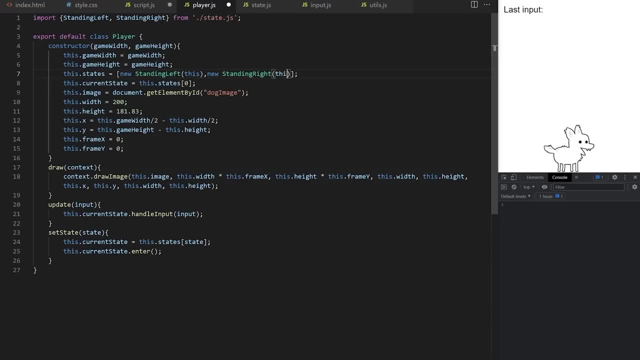 so that we can then correctly set up our sprite sheets here and here Inside playerjs. I need to pass it, that player argument. Since we are inside player class right now. I pass it this keyword: This scope of this class represents the entire player object. 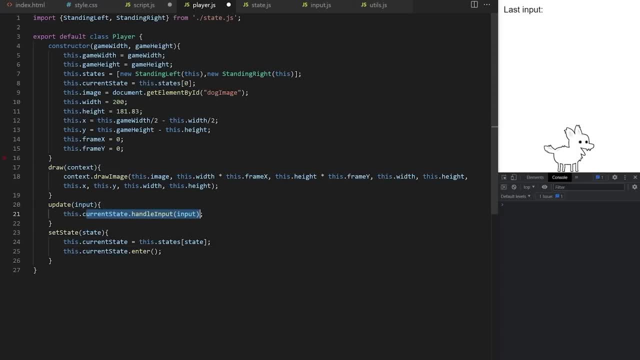 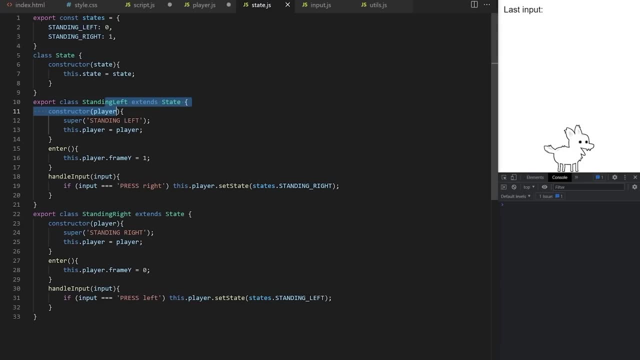 Ok, so thiscurrentState is thisstates index 0, which means our standingLeft class, and we are calling handleInput on it. so handleInput from line 18 will be called. If the initial currentState is index 1, that would be standingRightState. So this handleInput method will be called from line 30 instead. 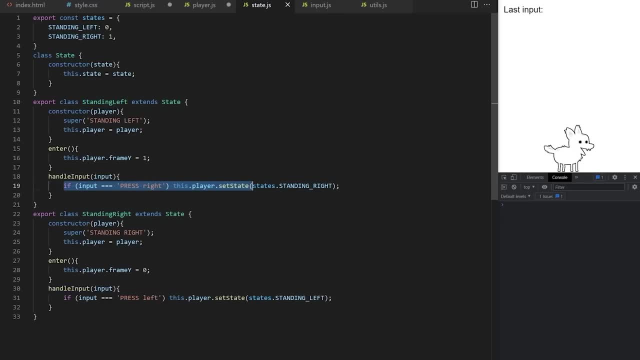 If handleInput is called from standingLeft class, it will only react if right arrow key is pressed And it will swap player to standingRightState. If player is currently in standingRightState, handleInput will only react to left arrow key being pressed and it will swap player to standingLeftState. 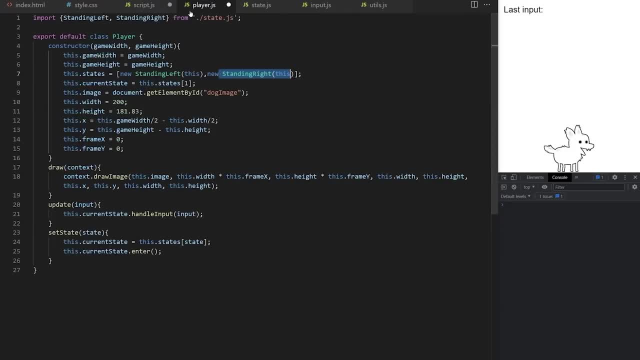 Whenever we set a new state, it will update which of these two states thiscurrentState is pointing towards, and then, from that new state, it will call this enter method. Enter method was defined on lines 15 and 27 and, depending on the current state, it will. 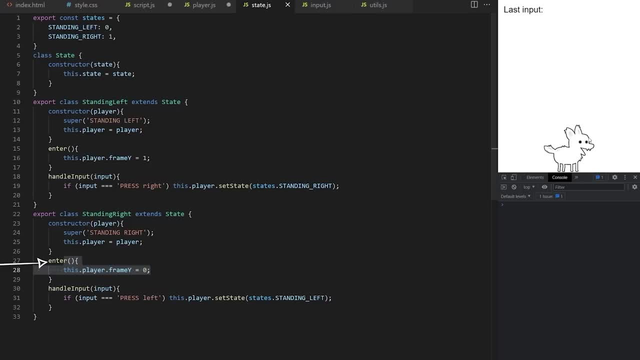 set sprite sheet to animate. I save changes to all my files and when I click my canvas and press left and right arrow keys, we are correctly swapping between standingLeft and standingRightState. Let's display what state player is currently in on canvas as well. 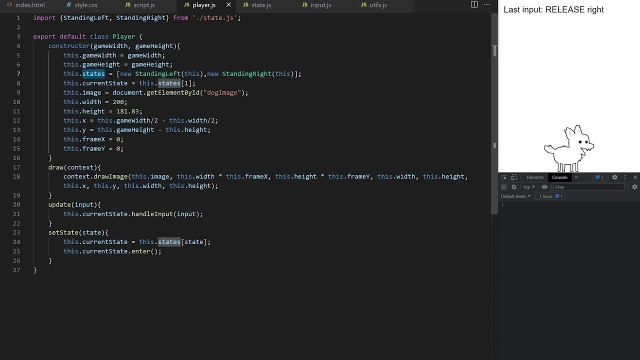 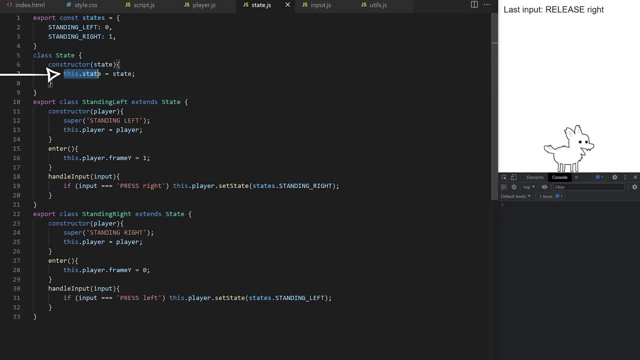 Here on line 24, every time setState is called we set thiscurrentState from line 8 to one of our available states. So far we have standingLeft at index 0 and standingRight at index 1.. Parent class of all our states has thisstate property in its constructor. 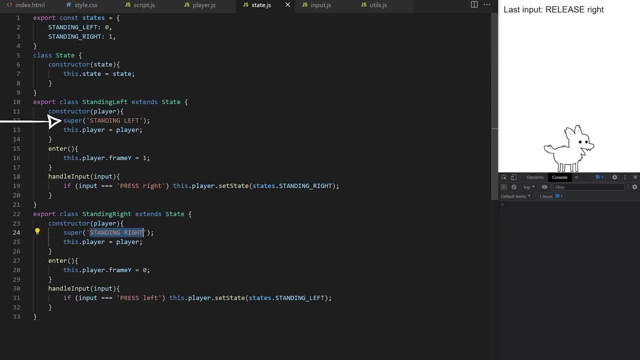 We are giving that property a different value from each child state by calling superclass constructor from each subclass. Basically, all that this is. we are declaring thisstate property on parent class. That property is being inherited by all child classes and it's set to standingLeft on this. 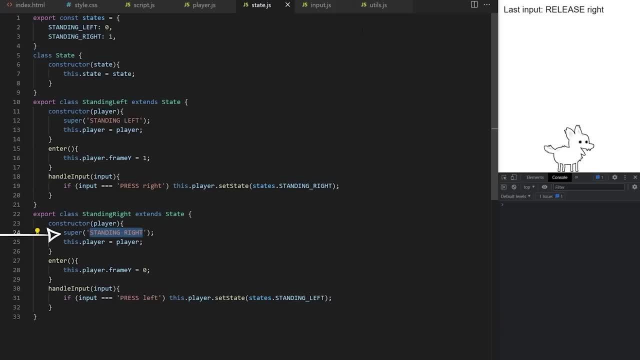 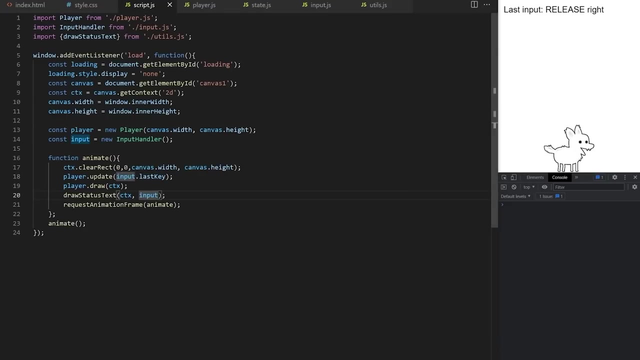 class on line 12 and to standingRight on this class on line 24.. I just want to draw this value on canvas so that we know currently active state. I will use our existing drawStatusText function for that. We are calling it from inside animation loop here and I need to pass it player object. so 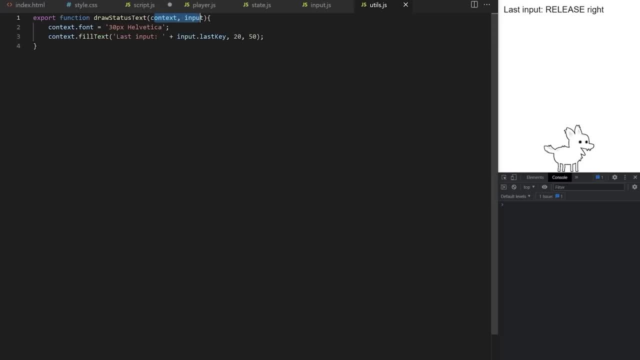 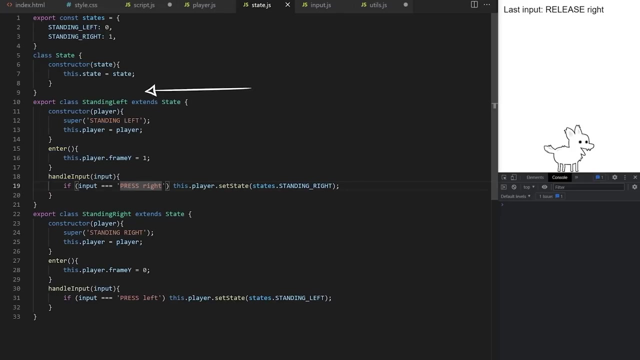 that we can access current player state Here. I make sure my function expects that argument, the same as we did with input last key. I will call fillText and I say active state, colon space plus player. we passed as argument dot currentState dot state. When currentState is set to standingLeft, this dot state here will be set to standingLeft. 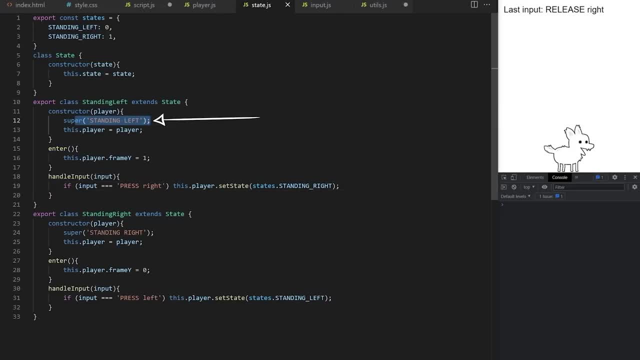 and that's what will get displayed For standingRight. it will display this line, As I said before, using super keyword inside child class, constructor will call constructor of its super class its parent class and it will execute all its code. In this case, this code will assign value of standingRight to this inherited state. 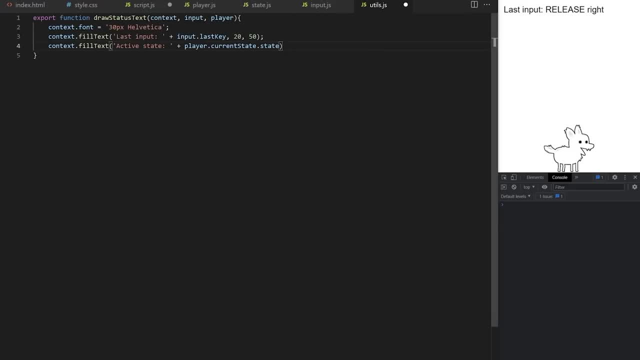 When using live server in VS code, watch for these dots here. It means you have unsaved changes in your file. so just make sure you save all your code in each file. if you are not getting the same result as me, I save my changes. 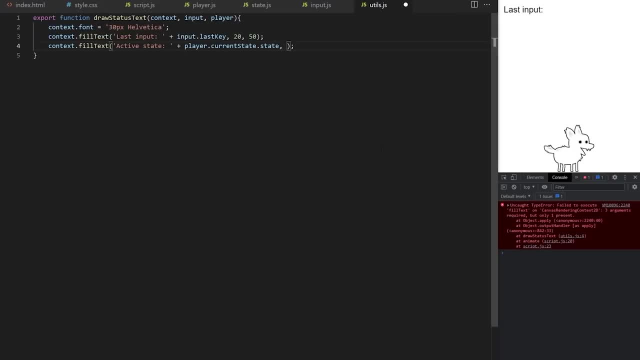 I also have to give fillText some x and y coordinates. How about 2100, maybe 90? and I reduce font size to 28 pixels When I save my changes and interact with canvas. Now, When I press left and right keys, we see status text that tells user the last input that was. 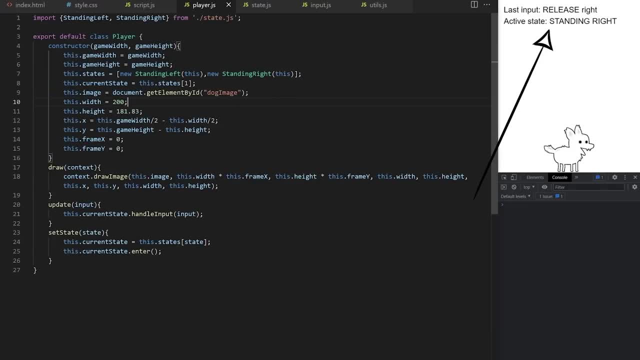 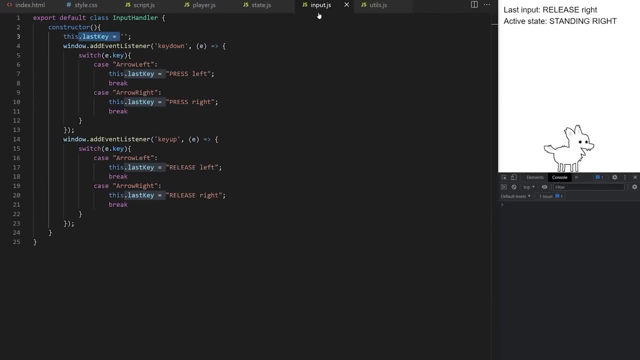 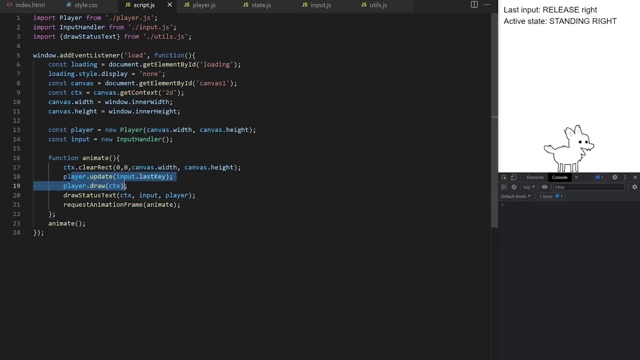 pressed or released and currently active player status. That's it. state pattern is complete. now we just add more states by extending it. Before we add sitting and running state, let's recap the logic, because I realize this must be lot for beginners to follow. If you are following so far, well done. you are doing great. 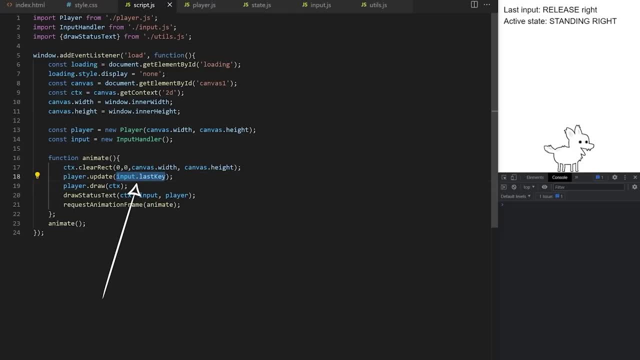 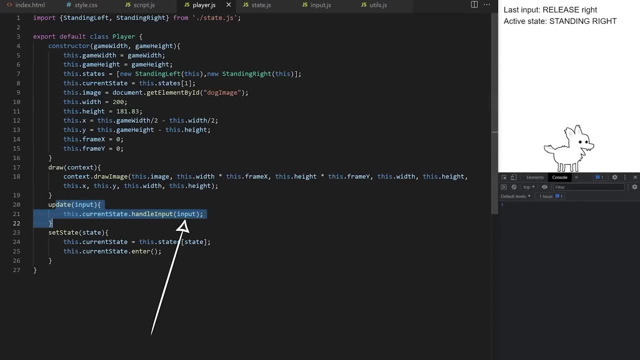 It all starts by calling player update and passing it the last key that was pressed or released Inside update method. we take that input and we pass it along to handle input method. The whole trick here is that we are calling handle input from thiscurrentState property. 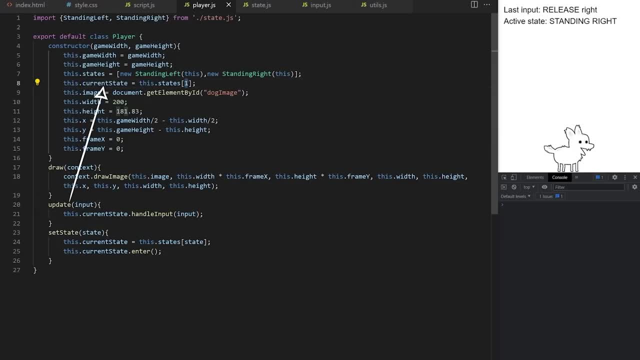 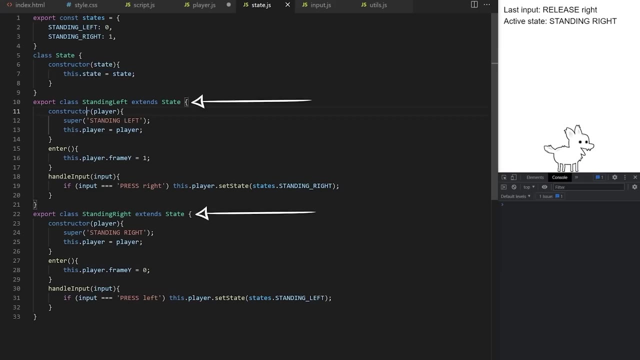 which swaps between different states. When we pass it 1, it points to state with index 1 inside thisstates array. so in this case, standing right object. If it's 0, it points towards standing left state object. Both of these objects have their own version of handle input method. 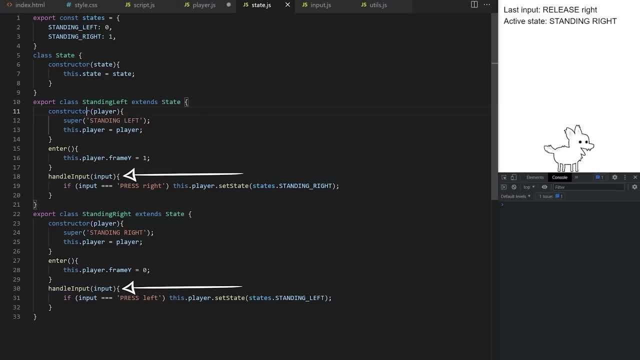 So that as we point current state towards different state objects, behavior of player will change, even though we are always calling the same handle input method. It's important that all our state objects have their own definition of enter method and handle input method. I could also create it a back up: enter and handle input method on their parent class. 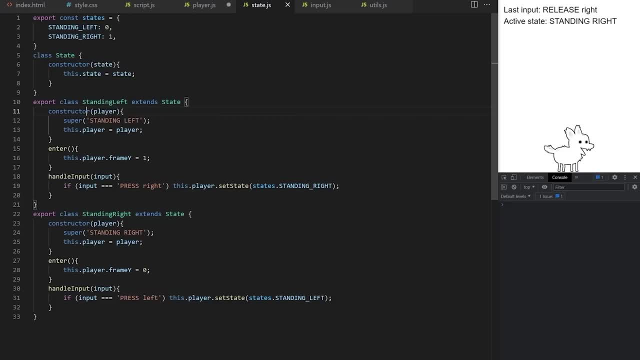 here In case child class doesn't have methods with these names. but lets not overcomplicate things. I like to think of this type of state management, as We are Lock-In Player in player in different states. While player is in a specific state, it will. 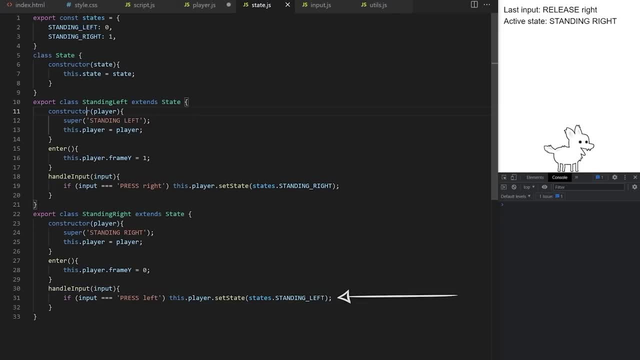 ignore some inputs and it will only react to inputs we define in its handle input method. Here we can see that, while in standing left state, player will only react to pressing right arrow key and it will make it switch to standing right state. While in standing right state, player will ignore all inputs except for. 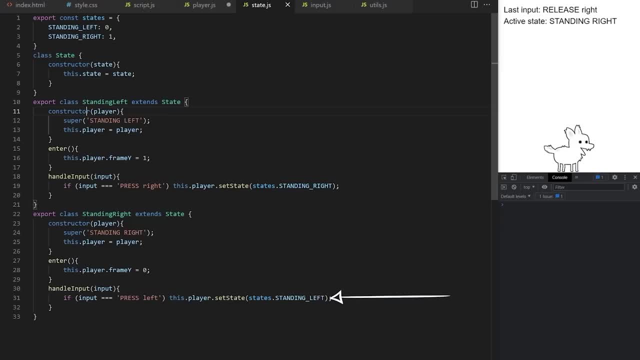 pressing of left arrow key, which will make it swap to standing left state. You might notice that state design pattern has some code repetition, but the code is easy to navigate in and if we get a bug it will be limited to a specific state, making larger projects much easier to manage and debug If we 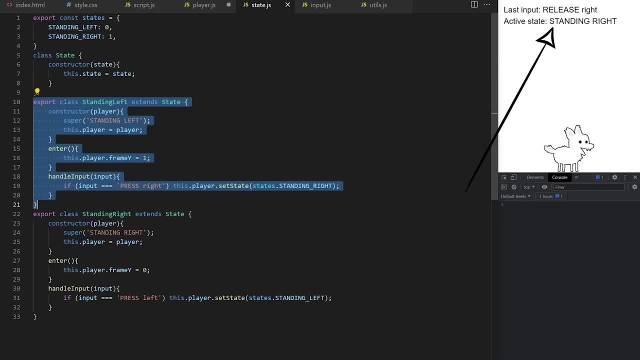 get some unexpected behavior. we can see what state was our player object in when that unexpected thing happened and what was the last input key that was pressed or released, and we check our code inside handle input method on that particular state to see what went wrong. Structuring your code like this comes very useful when you want to give your 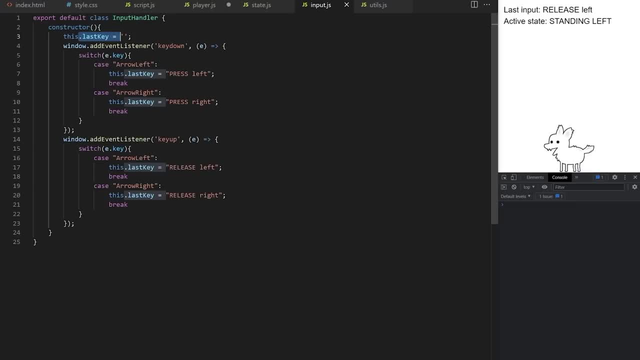 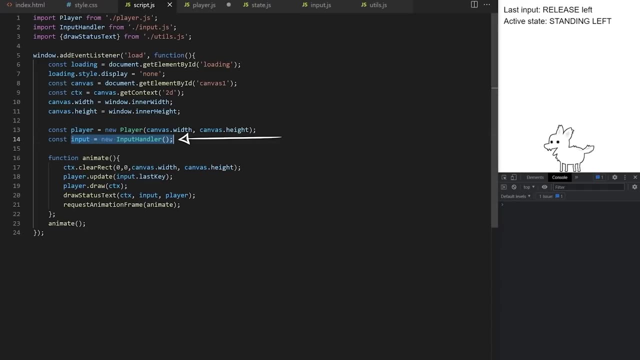 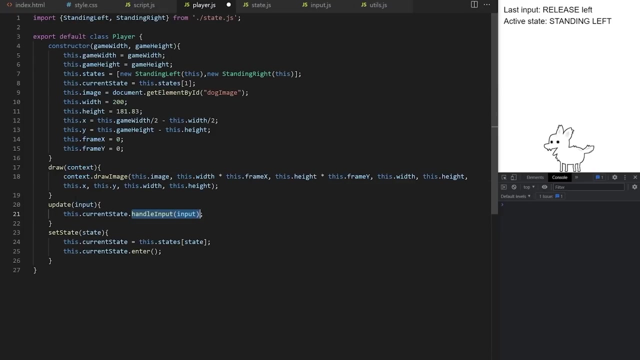 player multiple abilities, weapons and special moves. We are capturing the last key that was pressed here inside our input handler class. I'm importing and instantiating that class here in the scriptjs and passing it to player update method. We pass that input value along to handle input method and value of that. 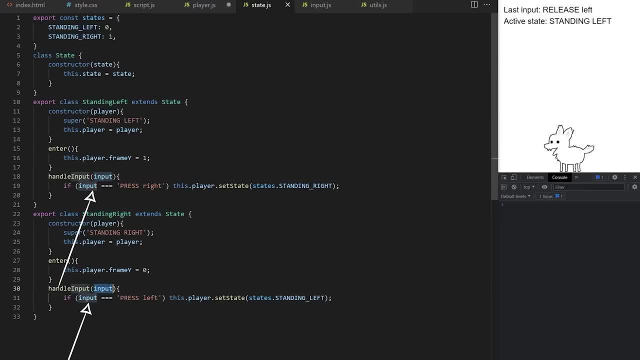 input gets checked against the set of specific values we define for each state and based on that we can check whether the input value that is going to be used or not. Based on that, we swap player to a different state using our custom setState method. 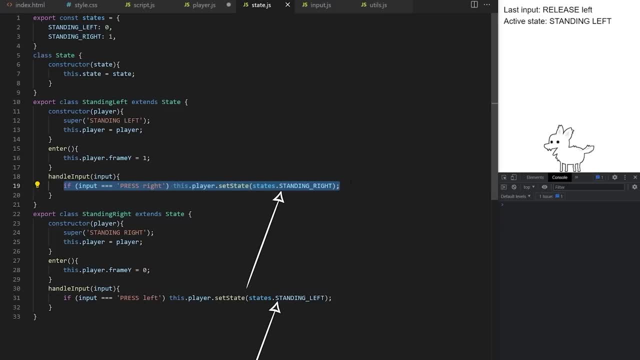 setState method takes a single number as an argument. as we defined them inside enum, statestandInRight is 1, statestandInLeft is 0, so right now I'm basically passing it number 1 here. That number travels as an argument passed to setState here. 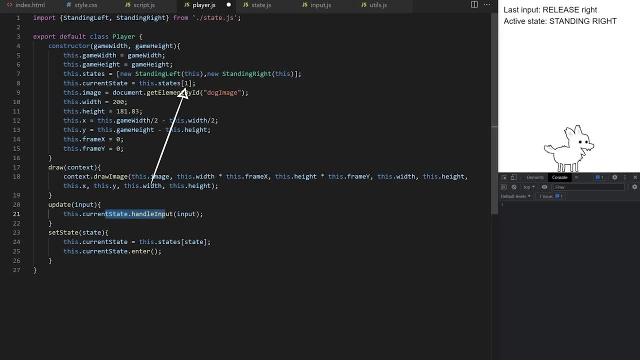 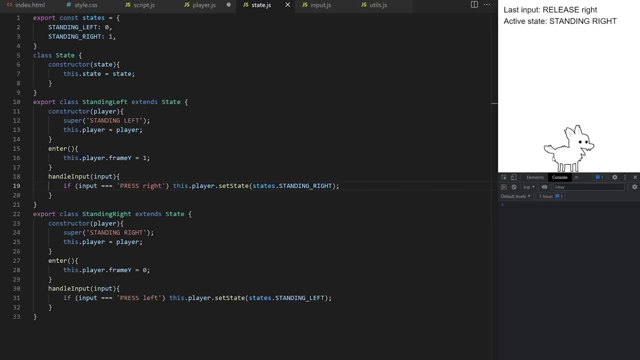 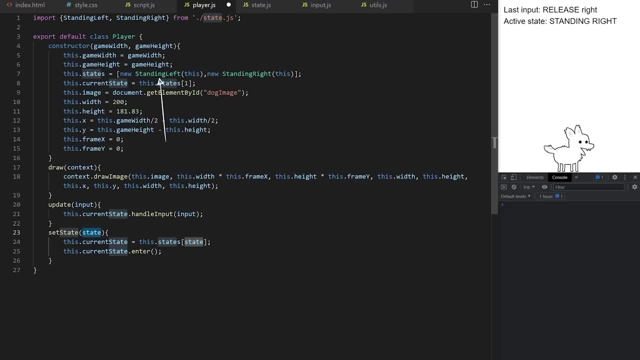 It's passed along here and it represents index of that state inside thisstatesArrayOnPlayerClass. so number assigned to each state inside enum object in statejs have to correspond to index of each of these particular states inside thisstatesArrayOnPlayerClass. 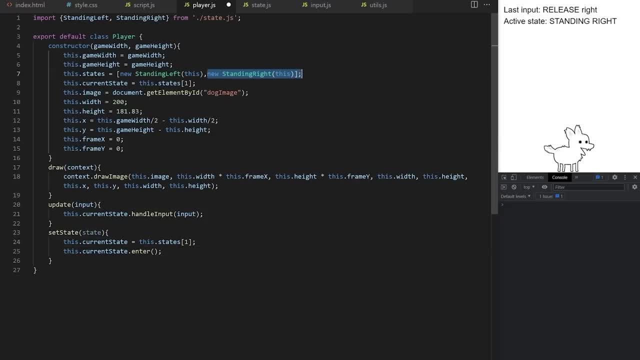 That way, when it receives number 1 here it swaps to standInRight state. if it receives number 0, it will set state to standInLeft. After swapping to a specific state, enter method will run once to set up player object for entering that state. 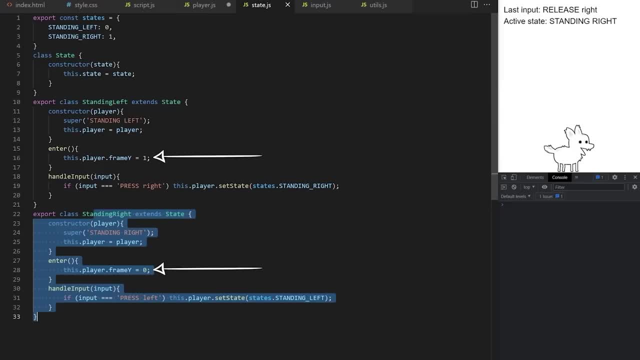 In our case, we just adjust SpriteSheetRow for now, and then it continuously calls handleInput method from that state class which listens to specific set of keyboard inputs. That's why we have enter and handleInput methods with the same names on each state. 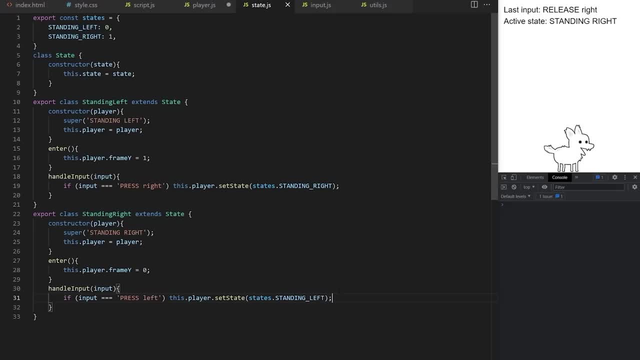 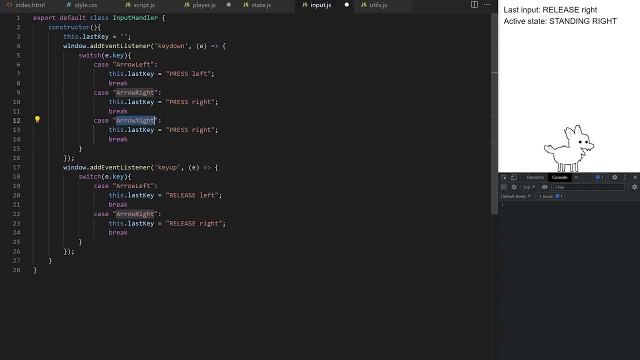 so that we call them from the same place but we get different behaviors depending on which state object is playercurrentState pointing towards at that state? Let's add sitting state. I copy this code block and case will be arrow down. If you want to know what are the values of ekey so that you can check for correct spelling. 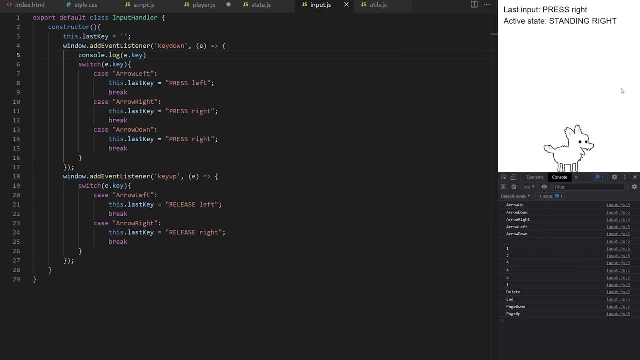 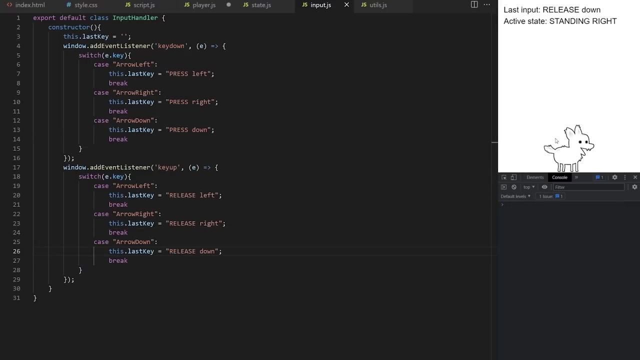 of key names. you can just console log it here. I'm going to say: if ekey value is arrow down, set thislastKey from line 3 to press down In key up event. we set it to release down In statejs. I copy this code: block: 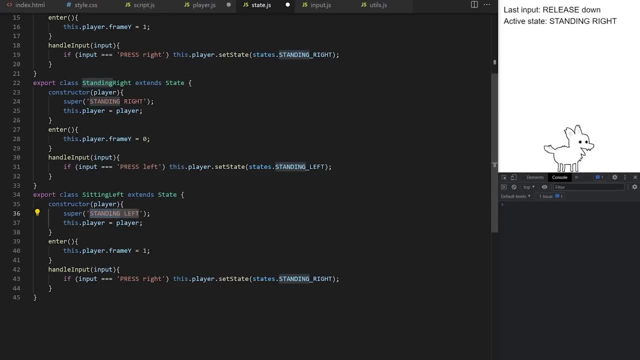 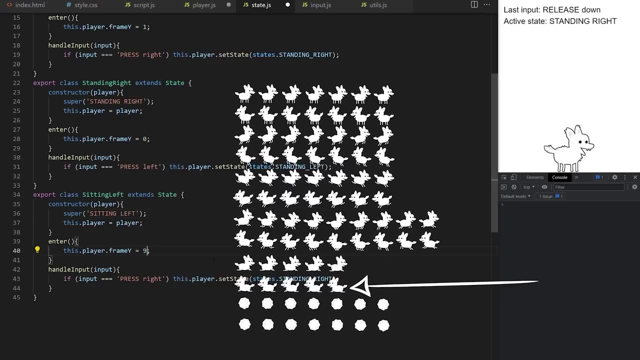 I use it to create a new class called sittingLeft. I pass it sittingLeft here. I check my SpriteSheet and I see that sittingLeft animation is on row 9.. We are counting from 0.. While in sittingLeft state, if we detect that user pressed right key, we will swap player. 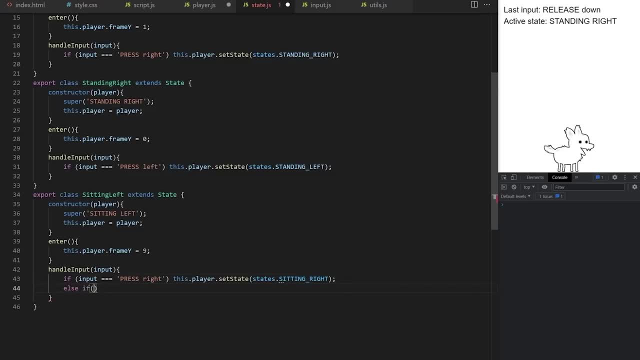 to sittingRight state, which we will create in a minute. Else, if we detect that user pressed up arrow key, We will make a change. We will make it stand up again. I need to create these new key value pairs in my enum object up here. 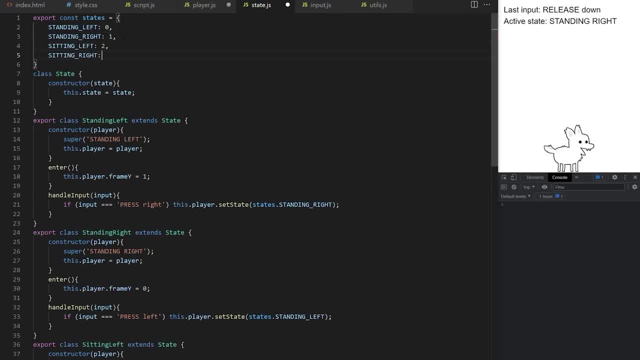 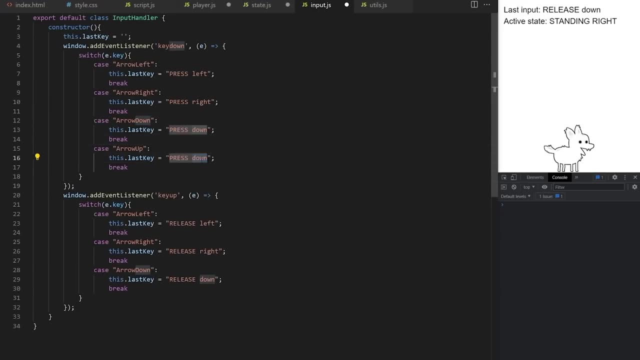 So sittingLeft will be 2 and sittingRight will be 3.. In inputjs I will check if pressedKey is arrow up and I set lastKey to press up. In key up event I set it to release up, So now we are tracking presses and releases of all 4 arrow keys. 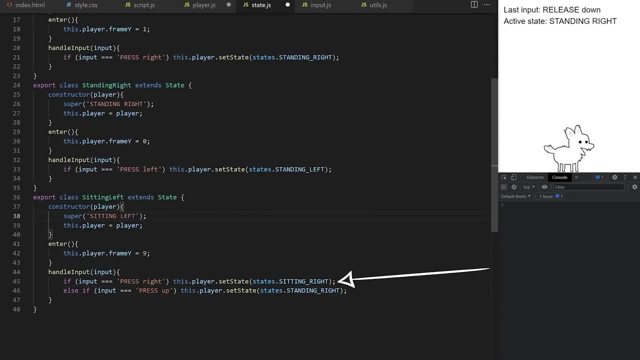 Perfect In my new sittingLeft class. when we press right, we set state to sittingRight and when we press up, our dog will simply stand back up. So here I need to do standingLeft because we are going from sittingLeft state. 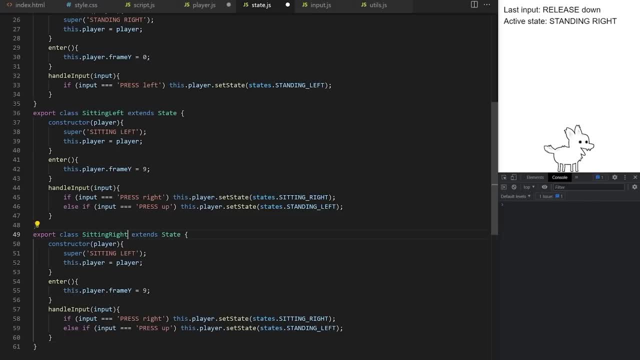 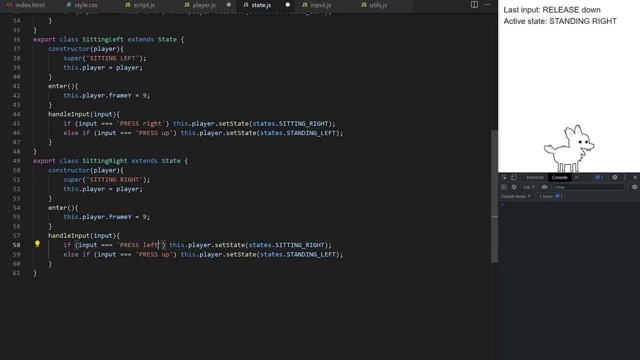 I copy this code block and I turn it into sittingRight class. We set name of state to sittingRight so that it displays correctly here, While in sittingRight state, if we press left, we set state to sittingLeft. If we press up, we set state to standingRight. 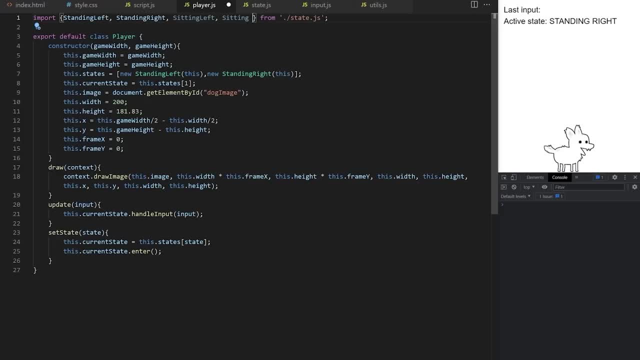 In playerjs. I import these two new state classes, I instantiate them inside thisstates array, while making sure I am adding them in the right order. Nice, so we have two new state classes. I hope you can see now how state pattern limits the number of inputs player reacts in each. 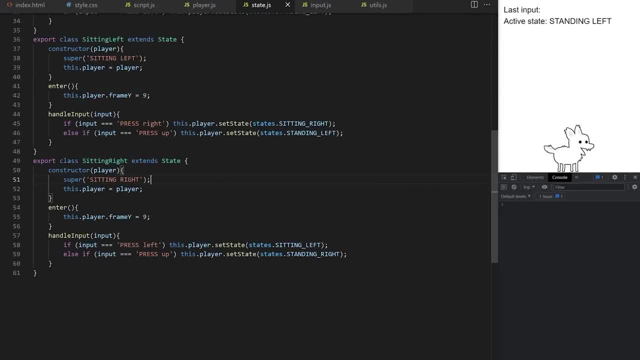 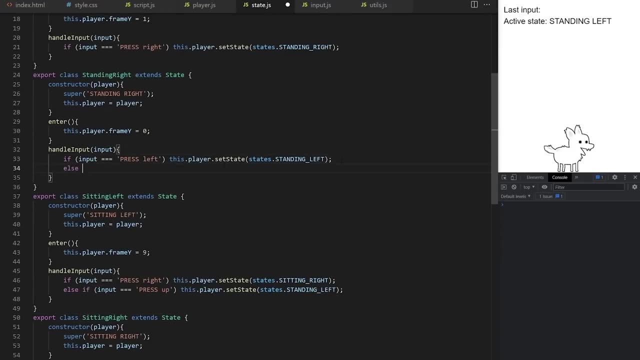 state. We have logic that defines how player behaves while in these two new sitting states, but we have no way to actually enter these sitting states. I go inside standingRight class and I say if input is pressed down, we set state to sittingRight. 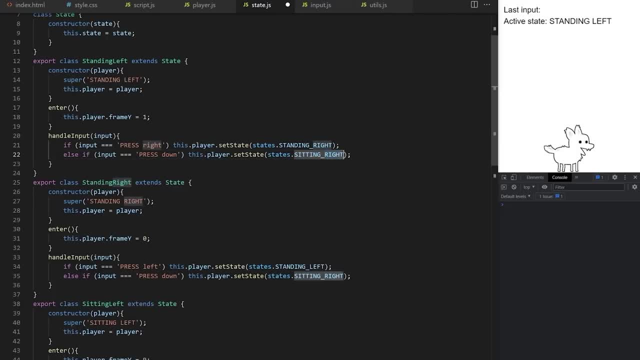 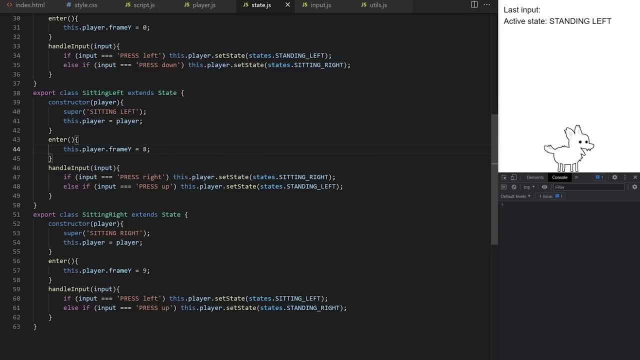 If we press down while in standingLeft class we set state to sittingLeft. I also need to make sure enter method on sittingLeft class sets player sprite sheet to the correct row. SittingLeft is row with index 8.. Actually sorry, sittingLeft is row index 9.. 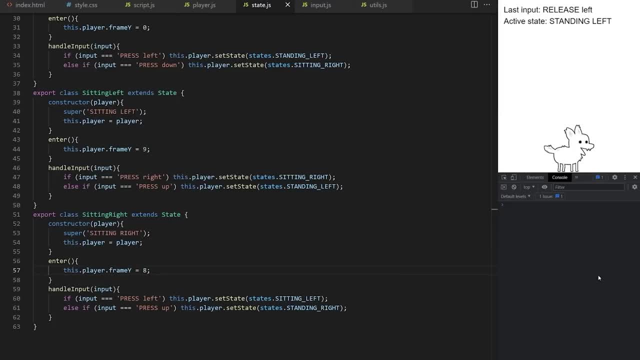 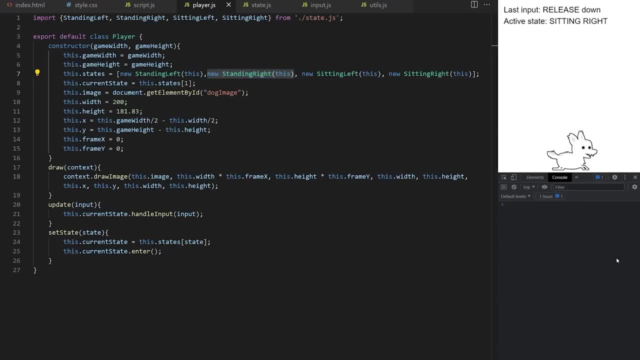 SittingLeft is row index 8.. Now it's correct. I will also set the initial state to standingRight, so thisstates index 1, just for the first page load before we start pressing keys and swapping player states. Now, when we press down arrow, key player will sit. 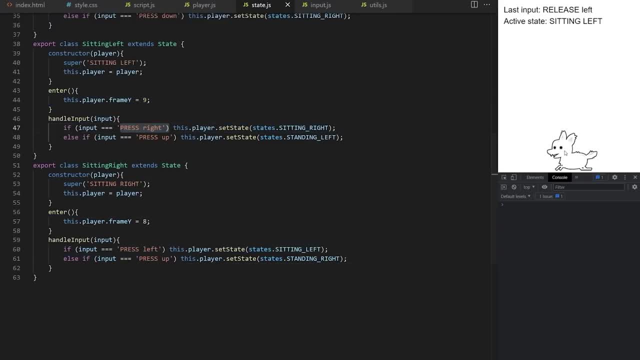 We can press left and right keys to make player turn left and right while sitting, and pressing up arrow will make it stand up and face the correct direction. This is going really well. We can also change how the entire sitting state works By only making the player sit while arrow down key is being pressed and when it's released. 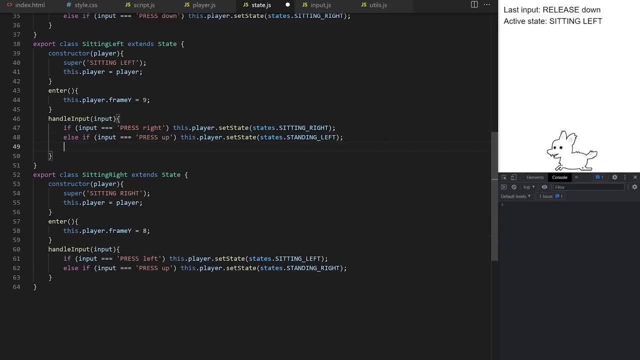 player will stand back up automatically. So inside sittingLeft state, if input is released down, we set player to standingLeft And inside sittingRight we set player to standingRight. It really depends on what kind of game you are building and what player behavior you. 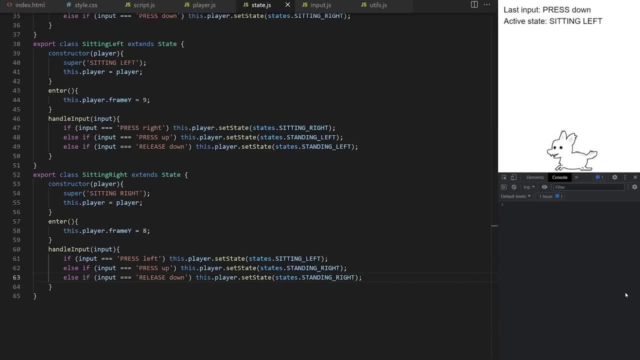 want. I hope you can see that you get a lot of freedom and flexibility with this code structure. You can easily control every detail of player behavior when you structure code like this. The way I wrote this code, we only react to the last key pressed. 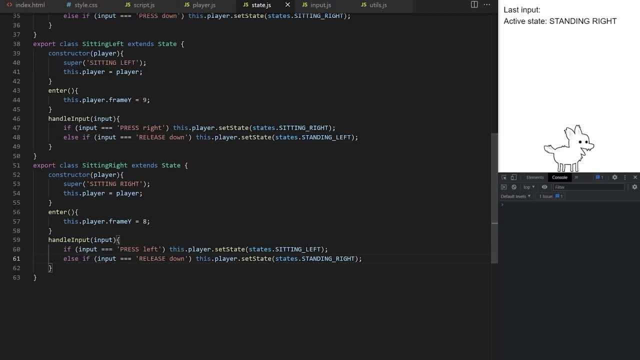 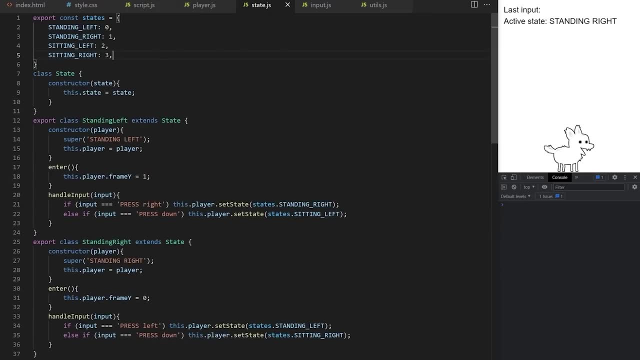 I'm not keeping track of multiple key presses in memory, since I want to keep this simple, but I will cover how to handle pressing multiple keys at the same time in a special episode as well. probably, Adding running states will be similar, but we will have to handle horizontal speed, so 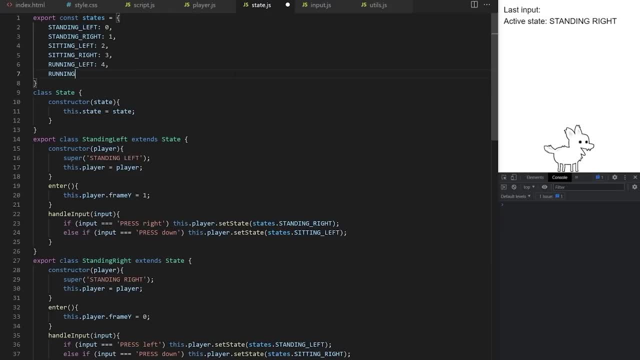 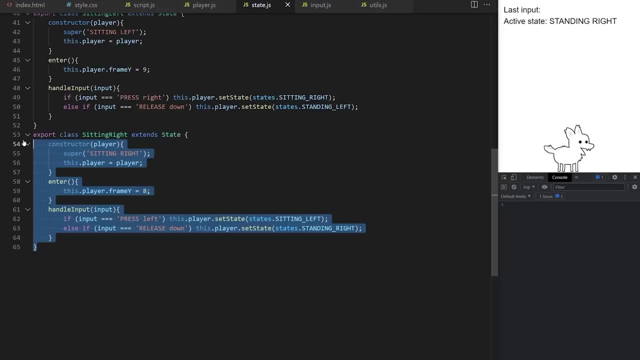 let me show you how to do that Again. I start by adding new states inside my enum. Running left will be state number 4, running right will be number 5.. I make a copy, I copy of this block and name it runningLeft. 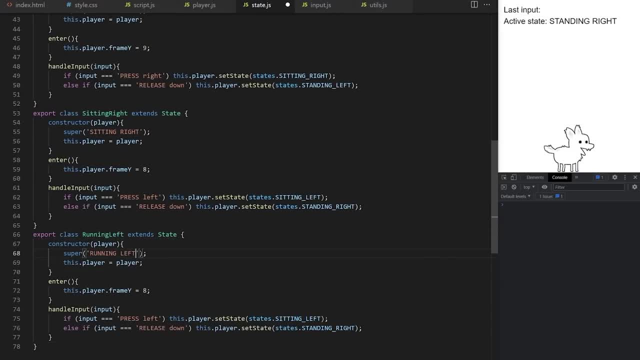 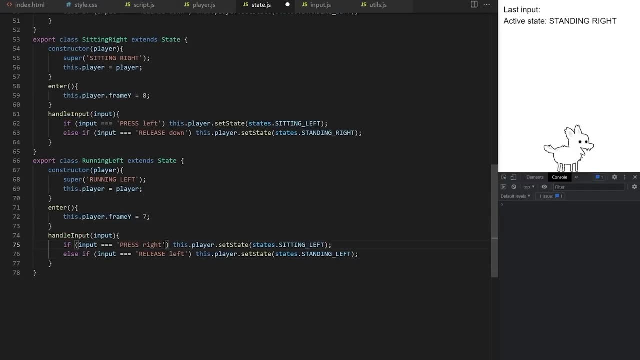 I put runningLeft here. I check my sprite sheet and the row for this animation is 7.. When we release left while in this state, we will switch player into standingLeft state and when we press right, we will switch into runningRight. 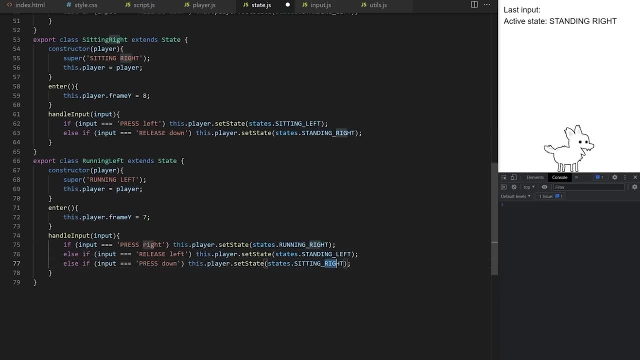 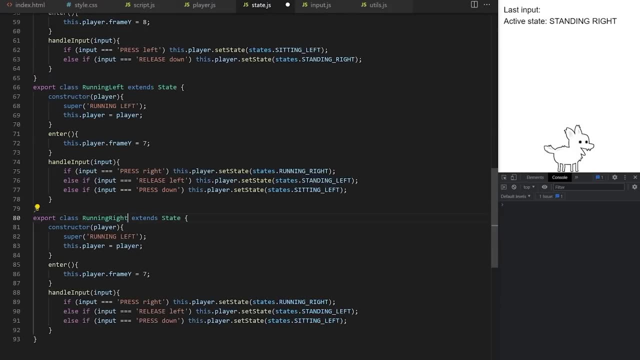 I also copy this line of code from here: and when we press down from runningLeft state, we will go into sittingLeft state. Duplicate this and turn it into runningRight state. If we press left arrow key while in runningRight state, we will get runningRight. 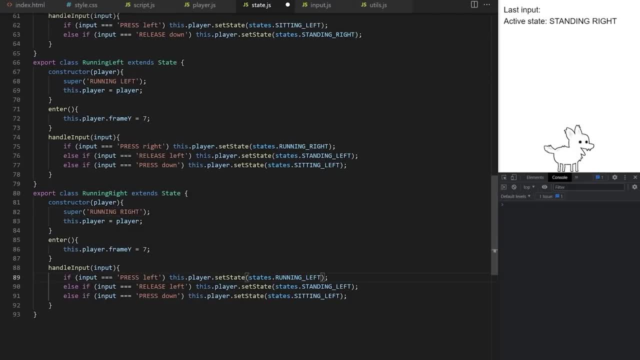 I copy this block and name it runningLeft. If we release right key while in runningRight state, we will switch into runningLeft. If we release right key, we will go into standingRight and pressing down arrow key will make player sit to the right. 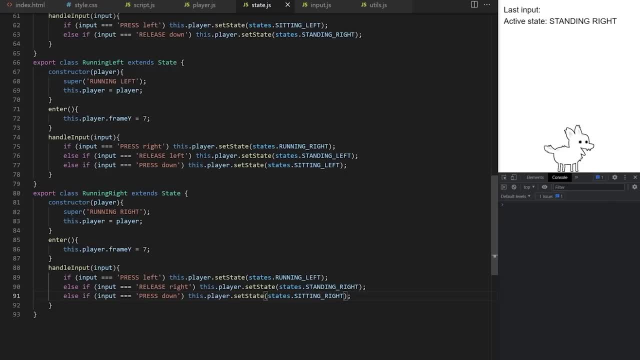 Not every game needs to have left and right version of each state. Also, there are other ways to write code when you have a set of states that each has left and right version, or maybe each state has a version with weapon ready and weapon hidden, for example. 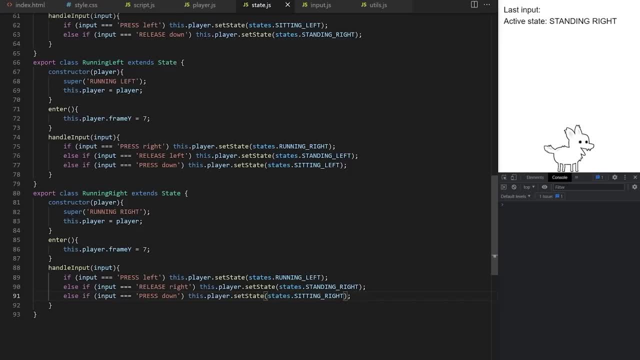 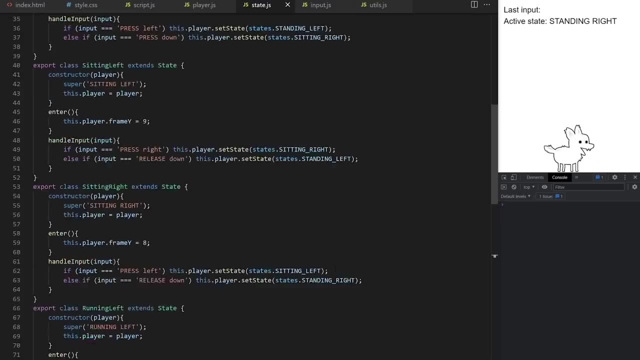 Again, I am doing it like this for simplicity and to demonstrate the main idea of my version of state management pattern. So we defined behavior for player while in running states. Now we need a way to actually enter these states. We can enter running from standing state, for example. 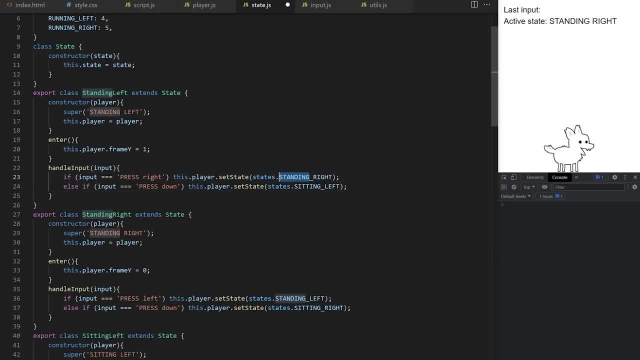 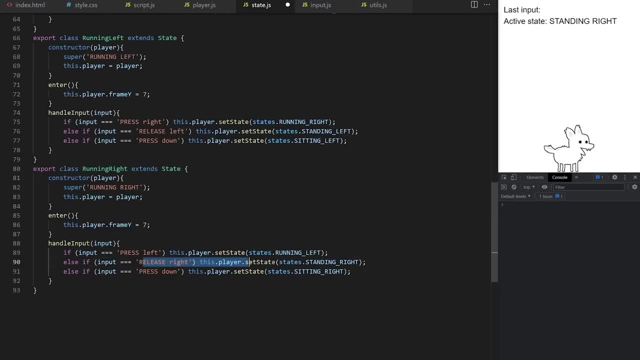 While standing left. if we press right, we set state to runningRight. Here inside runningRight state we see that when we release right key it will switch back to standingRight state. So we are only running as long as the key is being pressed down. 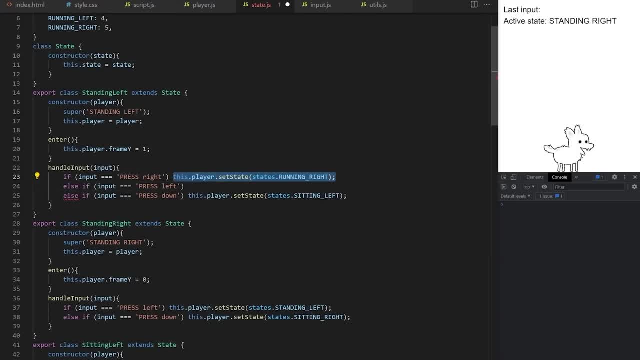 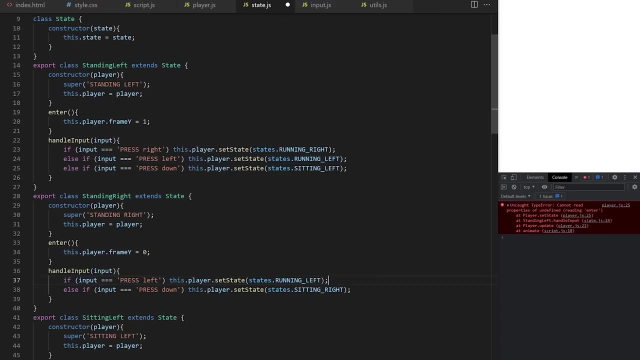 If we press left while in standing state, We will start running to the left. I get this error because I refreshed my project before I finished adding new state on player class. Don't worry about that. While in standing right state, if we press left, we will start running left. 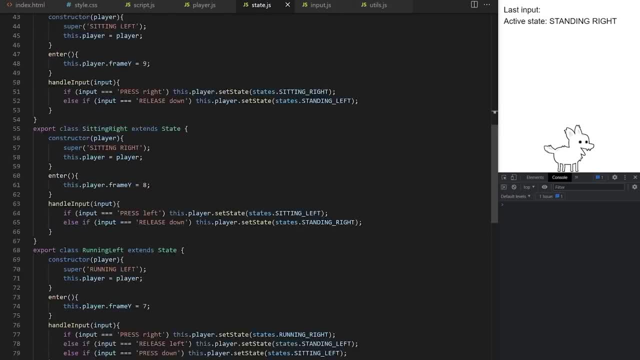 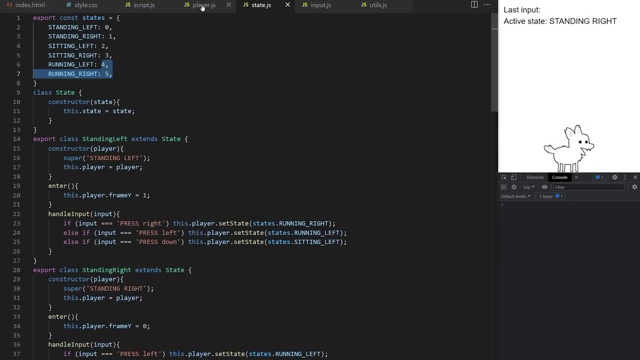 If we press right we will start running right. So here we are exporting two new state classes we just wrote Here we are assigning them values 4 and 5. These numbers need to correspond to indexes, to order in which we add these states inside. 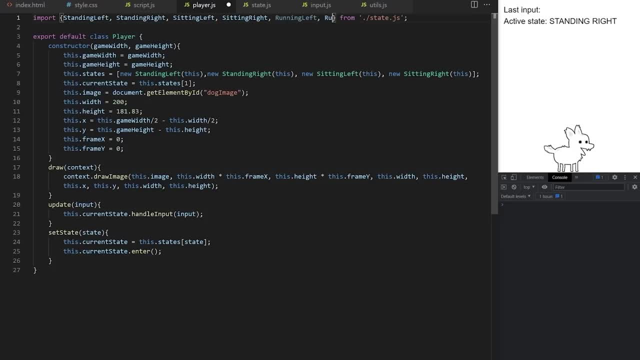 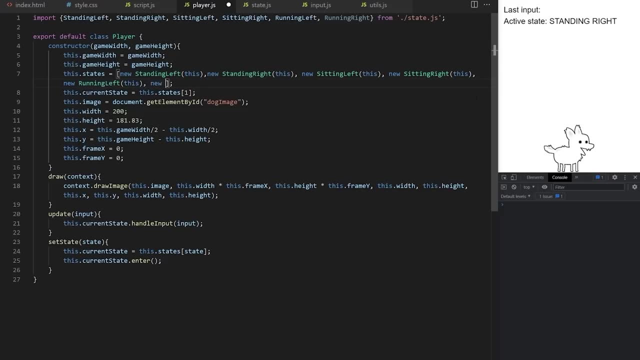 this states array here. First I import them on line 1 as usual, And then I add instance of runningLeft class as index 4 in this array, And runningRight will be the fifth item in this array, counting from 0.. 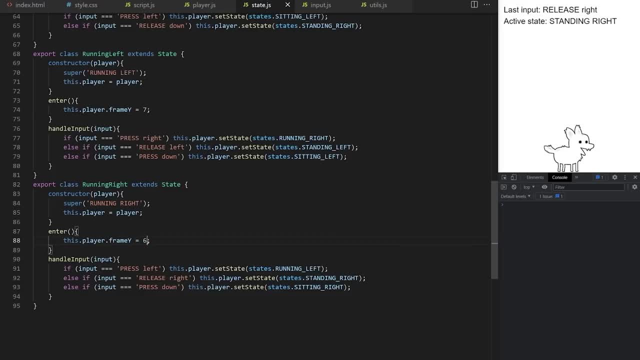 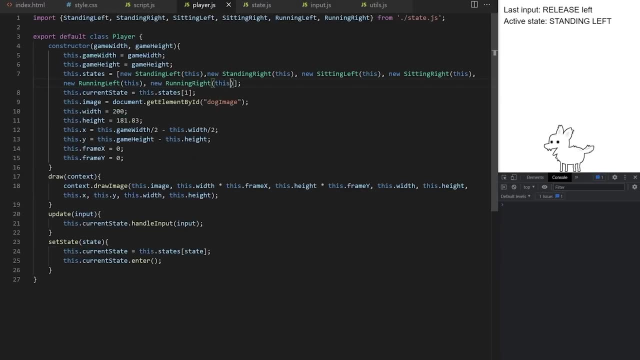 I save changes to all my files. RunningRight animation is row 6 in our sprite sheet. Perfect, It works. We also want player to actually move when in running state, So let's give it thisspeed property and set it to 0.. 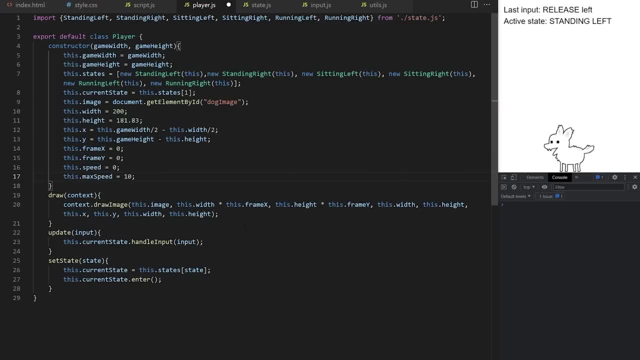 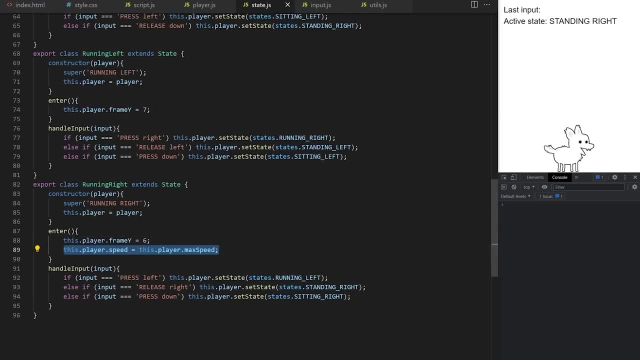 Then I create maxSpeed property and I set it to 10px per frame. for example, When we enter running state we set playerSpeed to playerMaxSpeed And in runningLeft we set player to minus playerMaxSpeed because movingLeft is in the 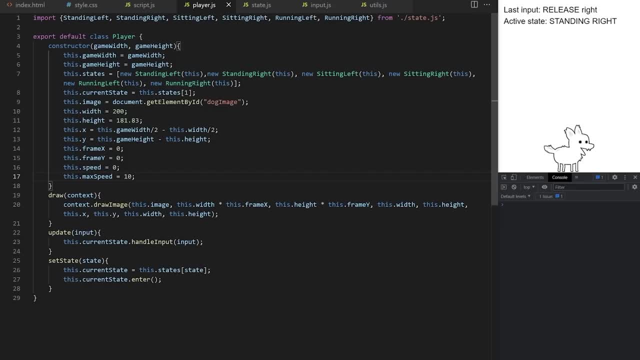 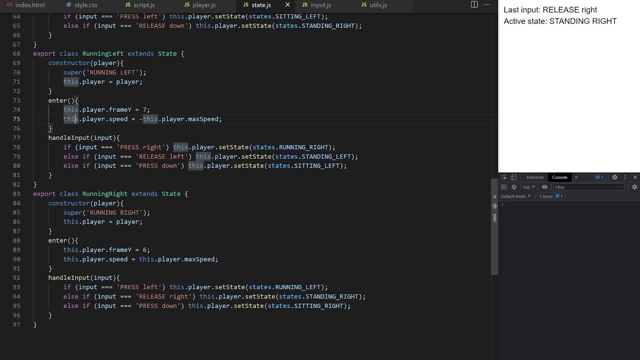 negative direction. on horizontal x-axis Inside update method on player class, I will be adding playerSpeed from line 16 to horizontal position from line 12.. Problem now is that player will just move off screen because even when we switch away from running state, nothing is set in playerSpeed back to 0.. 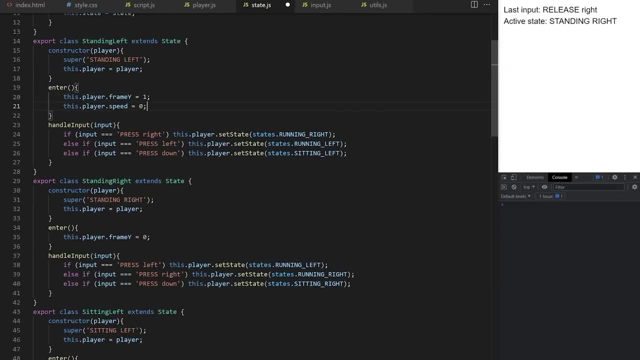 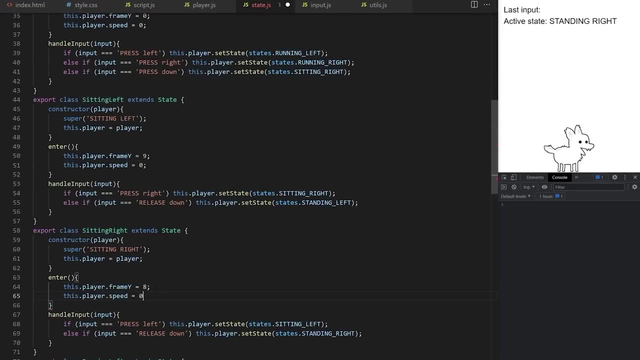 So when we enter standingLeft state, we set playerSpeed back to 0.. We do the same thing inside enter method on standingRight, sittingLeft and sittingRight state. Perfect Player now stops moving when we enter standing or sitting state. I will also increase the speed of the player. 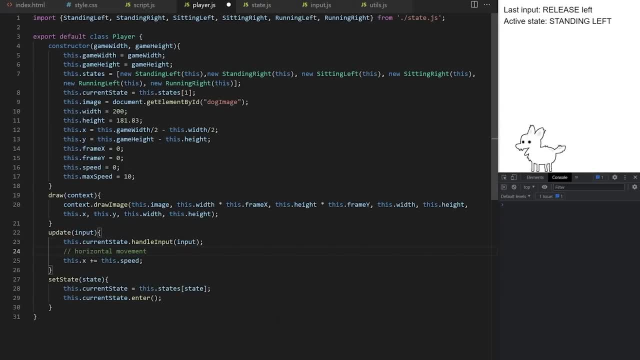 I will also increase the speed of the player. I will also increase the speed of the player. I will also introduce horizontal boundaries so users can't move player outside the canvas. If horizontal position of player is less or equal to 0, I set the position to 0. 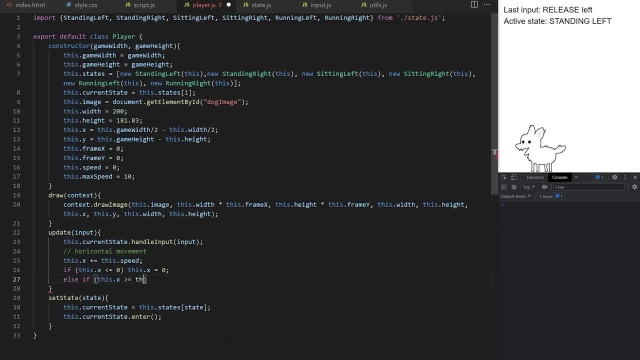 Else, if the position is more or equal to game width minus player width, meaning player's right edge is touching right edge of canvas. I will also not allow it to move past that point. This is going so well. We applied state management to our player and we have granule control over its behaviour. 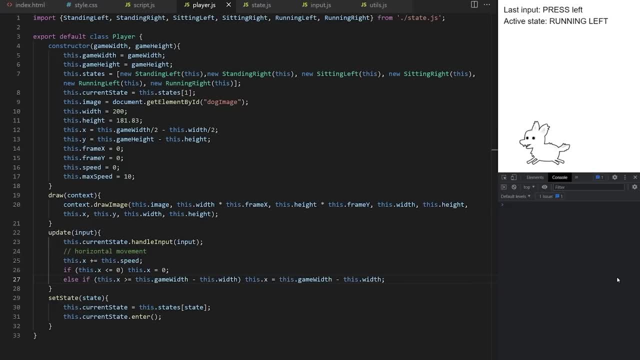 separated for each state. We can do so many things with this. Common thing you will see in games is jumping. Again, there is a new small trick we have to use here. If you never coded jumping in a 2D side-scroller game, we will learn how to do it properly. 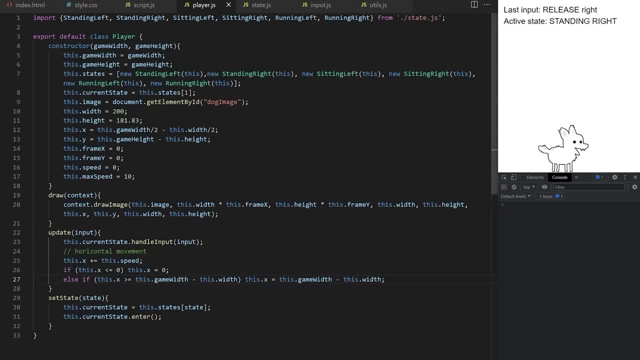 right now, and we will make it look really good by switching player to a separate falling animation after it reached peak height of its jump. Let me show you that swapping between states doesn't always have to happen on user input. We can also tie state swapping to other game events. 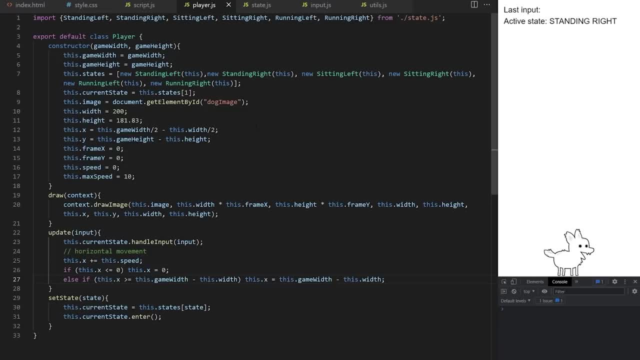 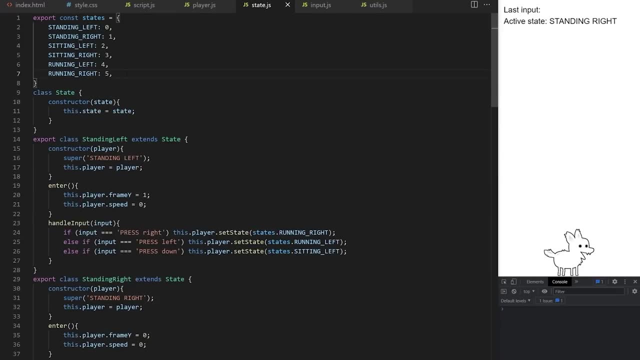 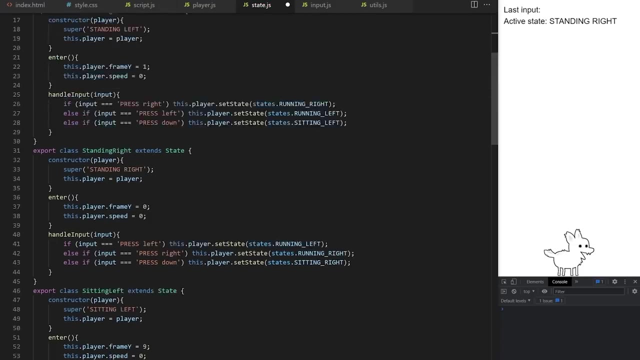 In this case we will swap a player from jumping to jumping. We are creating new states. As usual, I will first add them up here to our states object, which we are using to pair readable state names with numbers that represent each state. I copy already existing state class and I turn it into jumping left class. 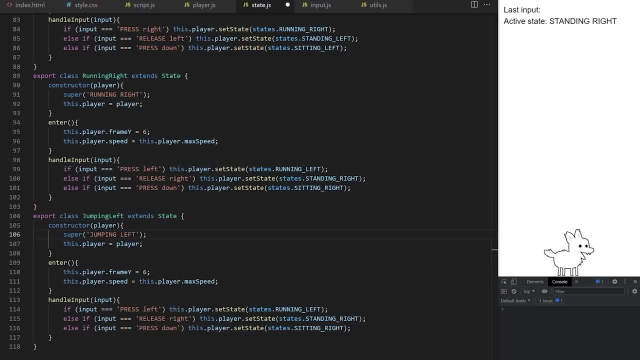 I check my sprite sheet to see which row has jumping left animation frames. I delete player speed, I think, because I want the speed to be inherited whether we enter jump from standing on running state. Hmm, we will see about that. I delete all these inputs for now. 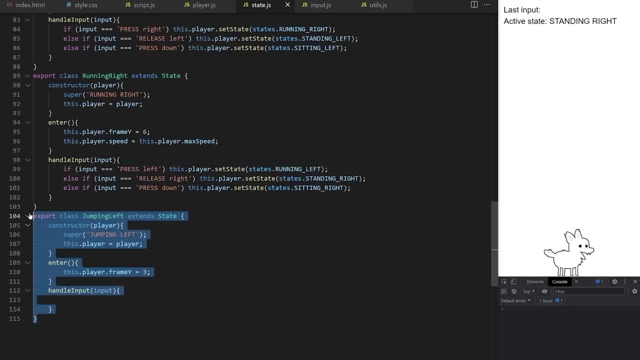 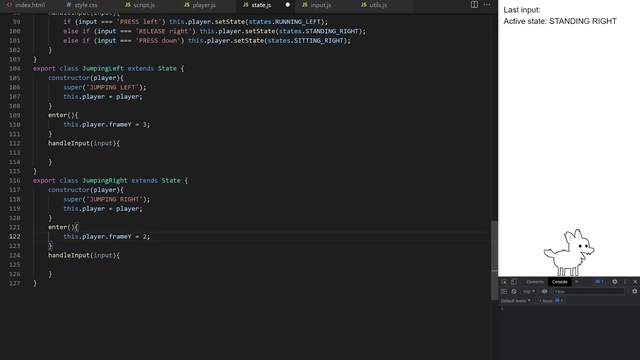 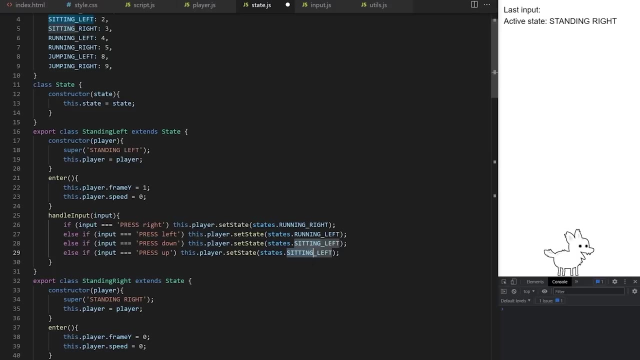 I copy this block and turn it into jumping right. class Frame Y for jumping right is row with index of 2.. I go up to standing left state and when input is pressed, we switch player to jumping left. Inside standing right state. when we press up arrow key, we switch player to jumping. 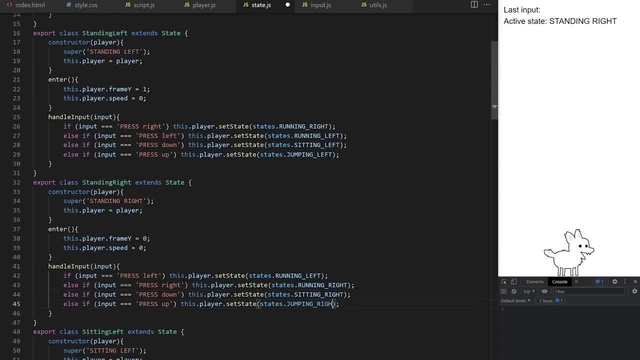 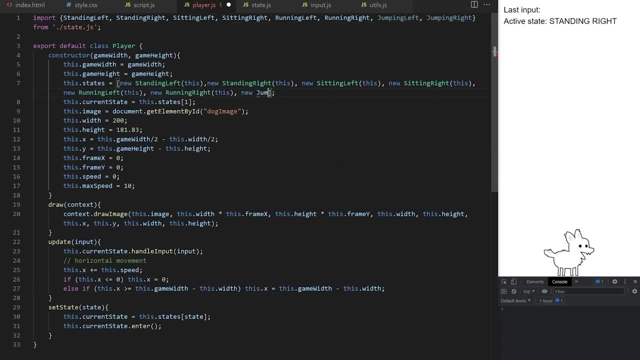 left. Inside standing right state. when we press up arrow key we switch player to jumping left. I set state to jumping right. I am exporting these new state classes so in playerjs I can import them and I instantiate them inside player states array. 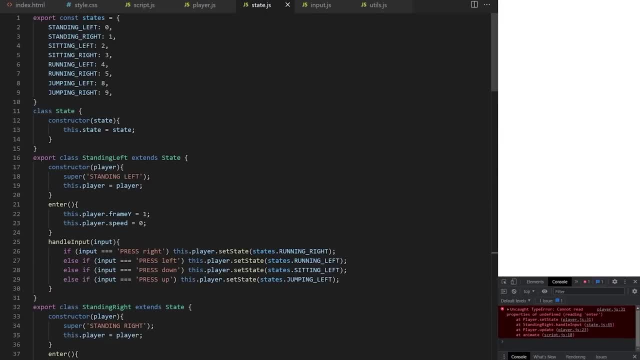 I am getting an error, It's because up here in my enum I skipped some values. Let's assign my new states to the correct values. Now we correctly enter jumping state. When I am in that state, it doesn't matter what I press, we are locked in that state. 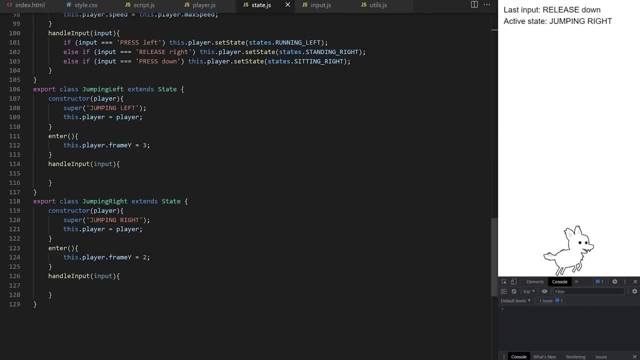 inside handle input method. I didn't give it any way to switch off to a different state. First, when we enter jumping state, let's push player upwards on minus direction on vertical Y axis. When we enter I say thisvelocityY minus equals 20.. I do the same for jump in right state In playerjs inside update. 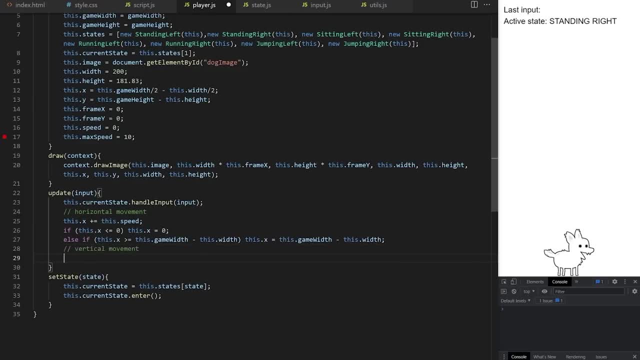 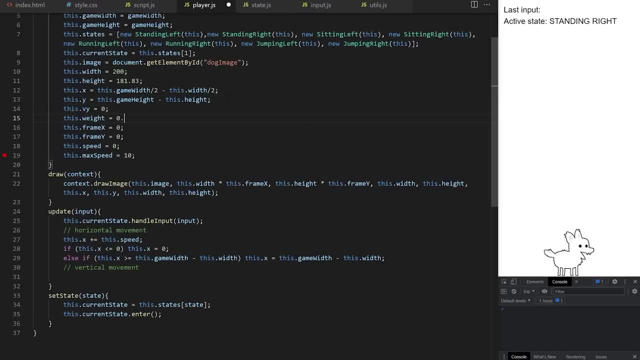 method. we will deal with vertical movement here. I give player VY velocity Y property and I give it property. I call, for example, weight. I could have also called it gravity or something. I will use velocity Y to pull player upwards and weight to pull player down, As the ratio between these two values changes. 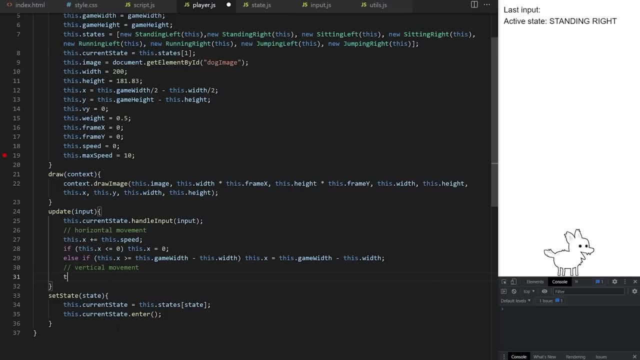 during the jump. it will create a nice jump in curve For every frame. we will add thisvelocityY from line 14 to players. vertical Y position from line 13.. Right now velocity Y is 0, so even when we have a vertical movement, we can add thisvelocityY from line 14 to players. vertical Y position from line 13.. Right now velocity Y is 0, so even when we have a 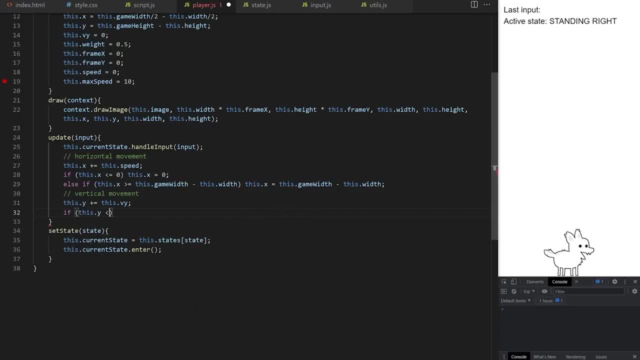 adding it, there will be no vertical movement If player is not standing on the ground. so if player Y is less than thisgameHeight minus playerHeight, gradually add value of player weight to velocityY, Else meaning player is standing on the ground. set velocityY back to 0.. Give me a second to figure. 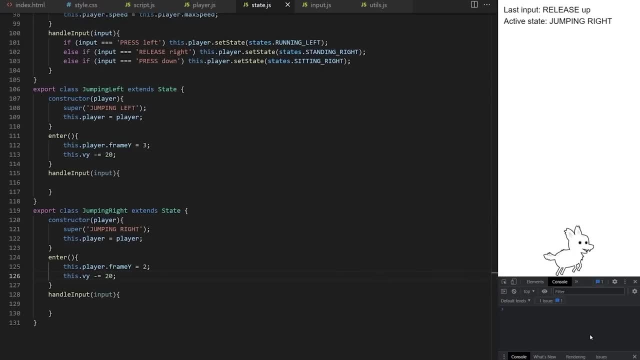 this out to make sure I'm doing it correctly In statejs here. I actually want to access a velocityY property on player object. so thisplayerVY minus equals 20.. I get a small jump and it stops moving again. hmmm, Oh yeah, this is a typo. this needs to be gameHeight. 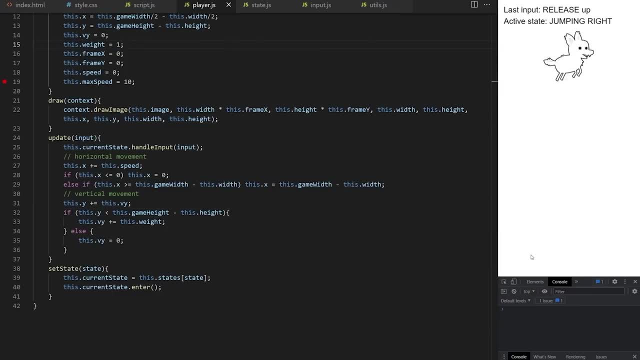 Now it's working. We have multiple places in our code where we need to check if player is standing on the ground or if it's currently in the air. This is a good time to create a small utility method on our player. I will call it onGround and its job is to check if player is standing on the ground. 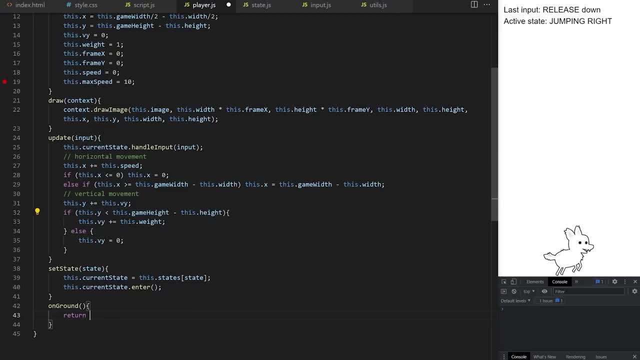 I will just make it return true or false directly, like this: based on how this expression evaluates: If player's Y coordinate, which is the top edge of player image rectangle, if it's more or equal than gameHeight. so this point minus playerHeight. so if this point is more or equal than this point. 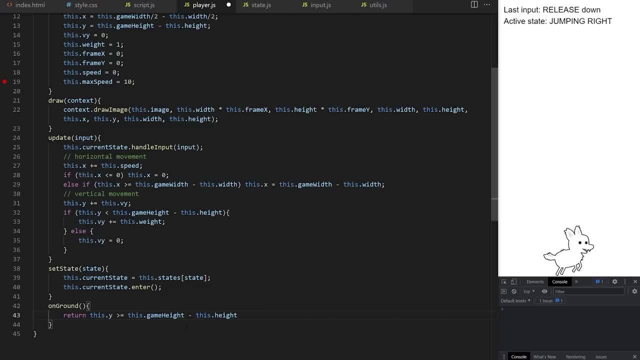 we know player is standing on the ground, so this method will return true, Else it will return false. Now I can just call this method whenever I need to do this check and it will also make the checks more readable. Here on line 32, I'm checking if player is not on ground, so I say if onGround is false. 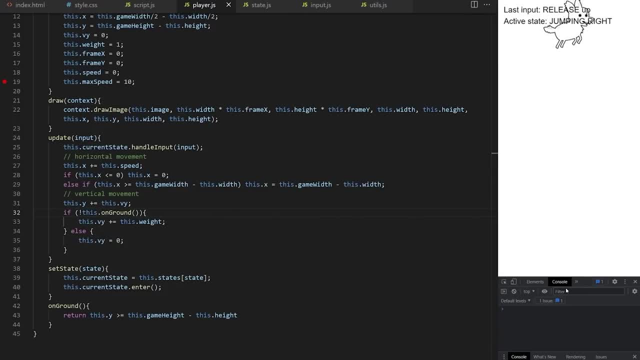 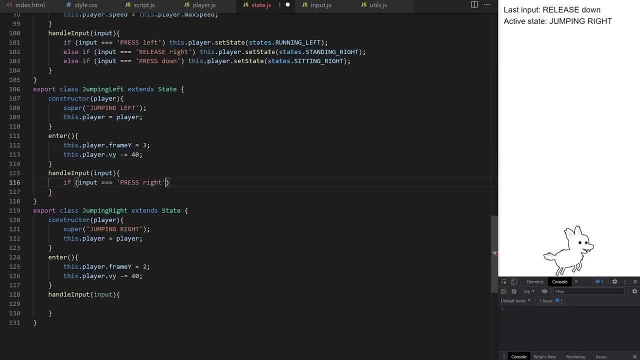 actually, if this dot onGround is false, now it's working. I want player to be able to switch sides while jumping. so in jumping left state, if we press right arrow key, we set state the jumping right. In jumping right state, if we press left arrow. 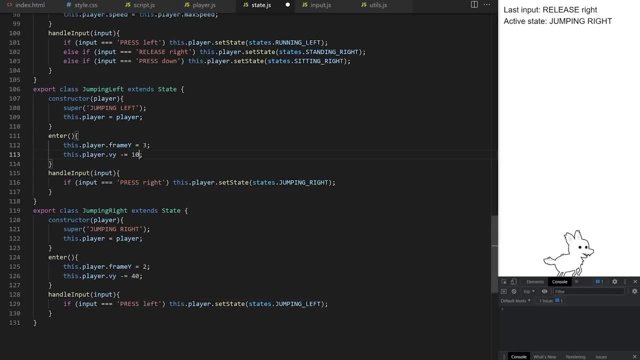 key we set state the jumping left Player is flying off screen really far. Let's change this to minus equals 10. That's a very small jump, but you will notice a bug here If I swap between jumping left and jumping right quickly each time we enter these states, we are 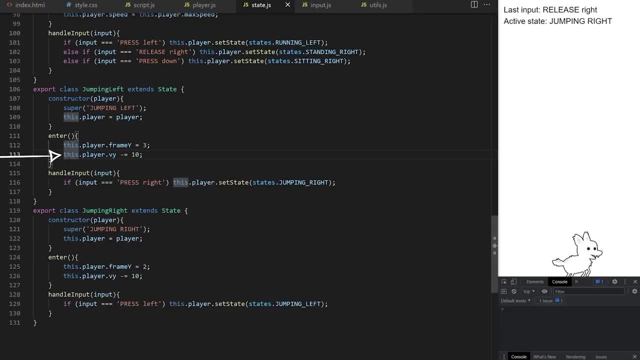 running their enter method. so each time we push player further and further up, I want the player to only be able to propel itself further up if it's standing on the ground. so in enter method on both jumping states I will first check if playeronGround is true before we. 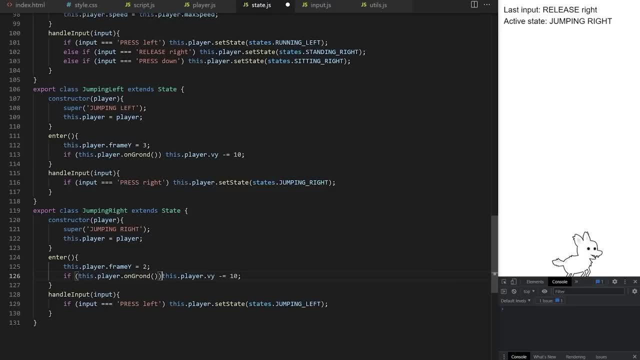 push it upwards If it's already in the air. this will be false and player will receive no vertical push. I change these values to minus equals 40.. I just make sure I spell onGround correctly. Perfect, we are able to turn to sides while. 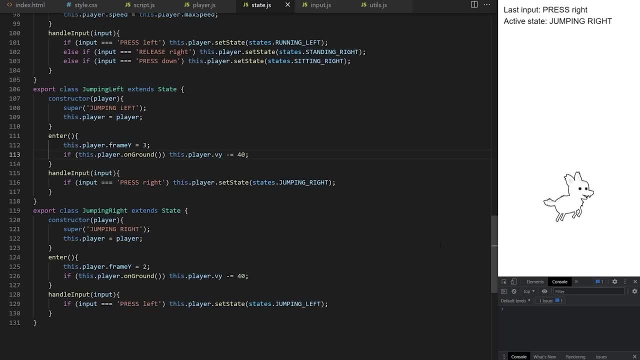 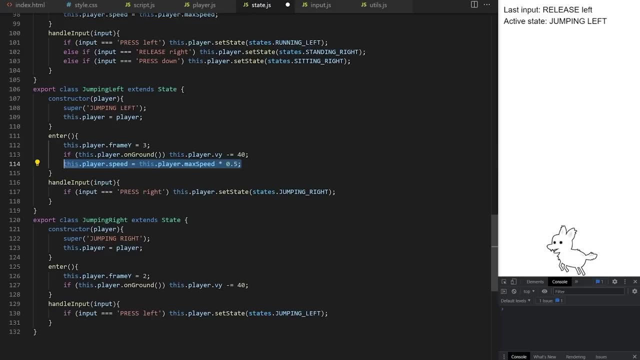 jumping. I will actually give it some horizontal speed as well. When we enter jumping left, set player's horizontal speed to half of player's max speed and the same for jumping right. In jumping left it actually has to be negative number, since we want to move in. 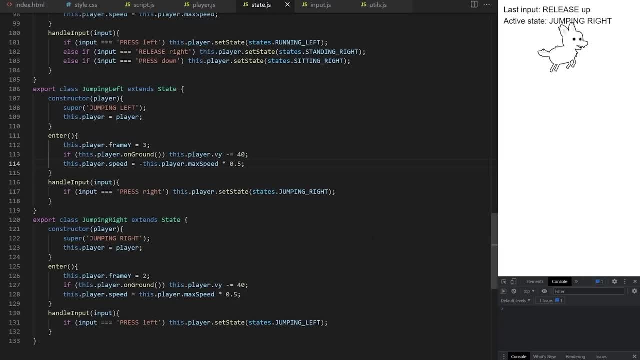 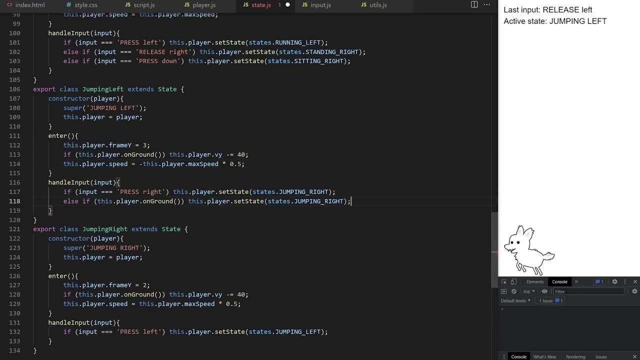 minus direction on horizontal x-axis. That works awesome. I can switch between jumping left and jumping right states, but otherwise I'm locked in jumping. I didn't give it any way to get back to running or standing state. Inside jumping left, I check if playeronGround is true and when player gets back on. 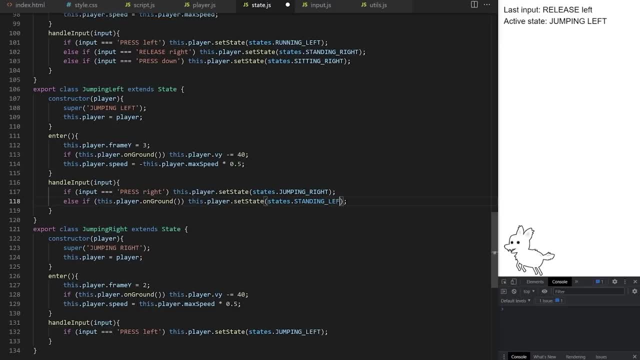 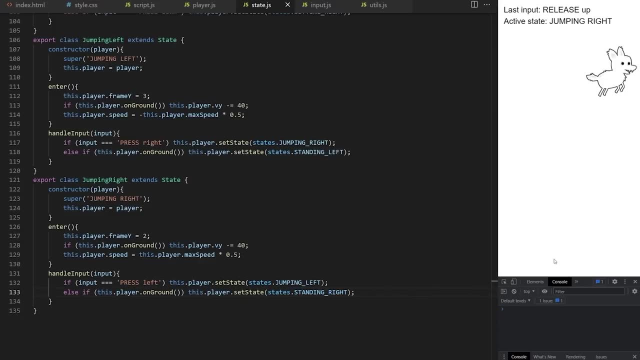 the ground, we set its state to standing left. In jumping right again, we check if playeronGround is back on ground and we set it to standing right. We are running, standing, sitting and jumping. Well done if you followed it this far, Let's. 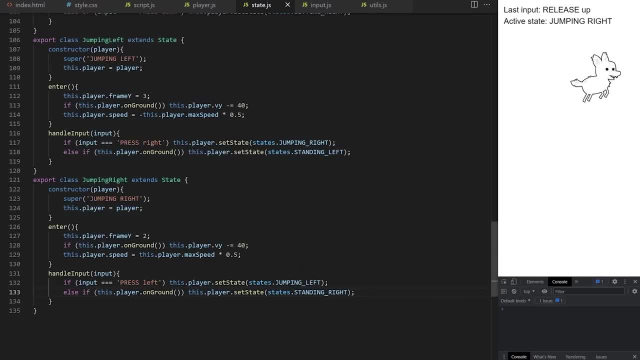 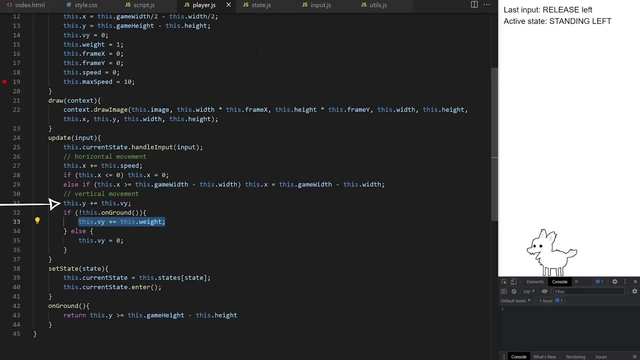 polish this and make it look even better. Jumping works this way. We are always adding velocity y to player's vertical position, here on line 31.. Most of the time that velocity y is zero, so there is no vertical movement. When we enter jumping state, we set velocity. 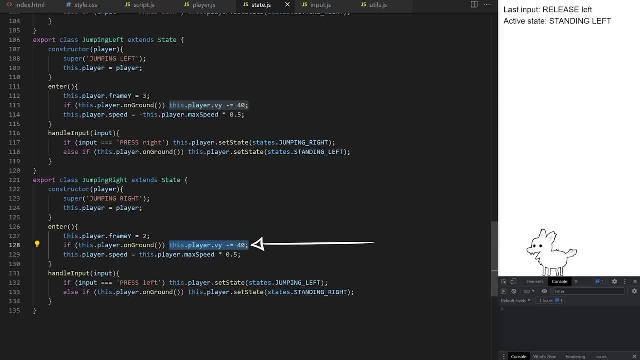 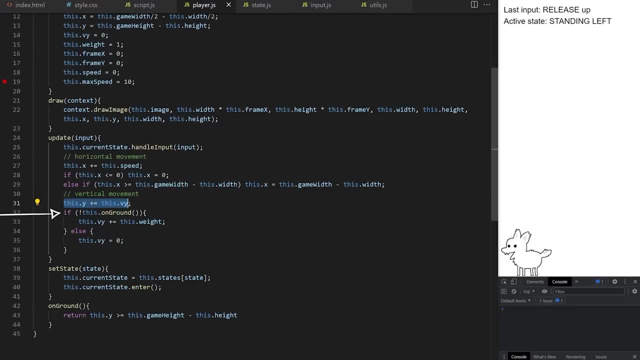 y to minus 40, which will push player upwards In minus direction on vertical y-axis. When we enter jumping state we set velocity y to minus 40, which will push player upwards. So this, if statement triggers and we start increasing velocity from line 14 by 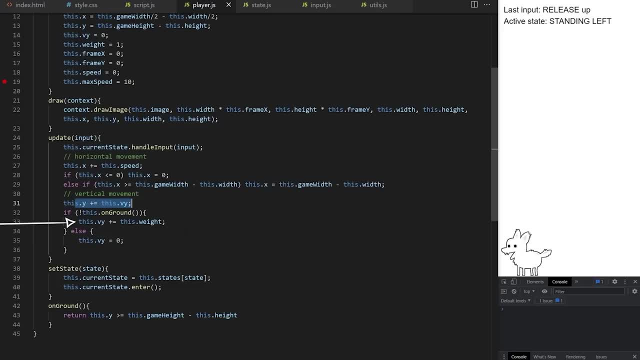 player weight from line 15.. This happens for every frame, step by step. So actually velocity y goes from minus 40 to zero, making player move up slower and slower. When it's zero, player will stop moving. At that point we are still not on the 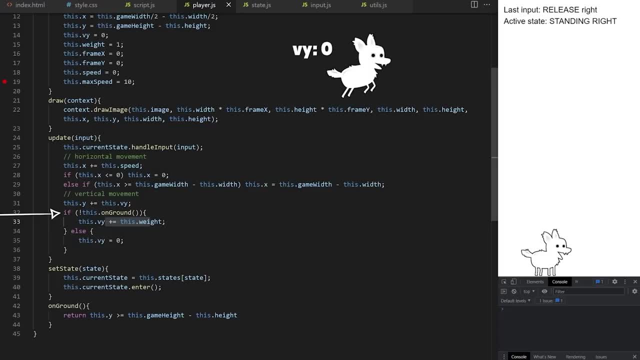 ground. so this line of code keeps increasing and it moves velocity y from negative to positive numbers, which will make player reach peak of its jump and it will start falling back down When we touch the ground. this L statement triggers, Velocity y is set back to zero and vertical movement will stop. 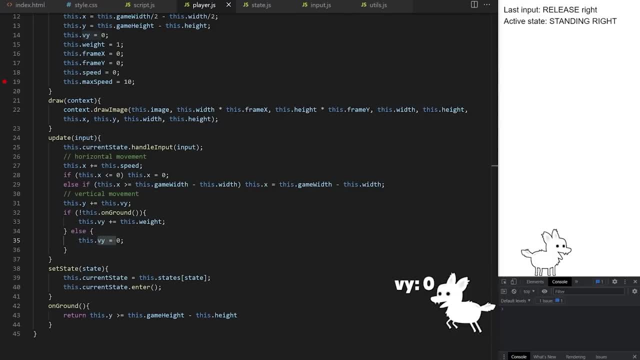 Understanding how velocity y goes from minus 40 to zero and then into positive numbers gives us ability to tie player state change to it. I can tell that player is at its peak of its jump because its velocity y switched from negative to positive values. I will just 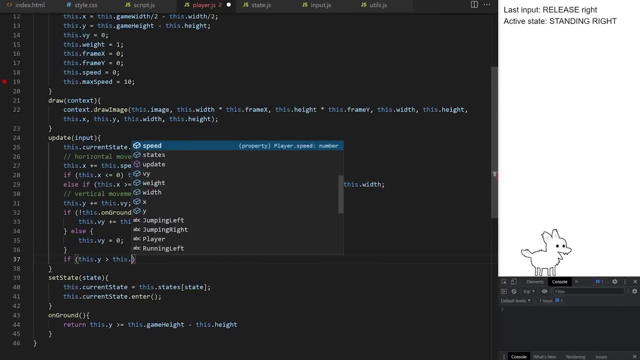 add a quick check here to make sure player doesn't fall through the floor. It shouldn't happen, but this is kind of my insurance. If player y is more than game height minus player height, set player y to game height minus player height. This line will make it impossible for a player to move below ground level. 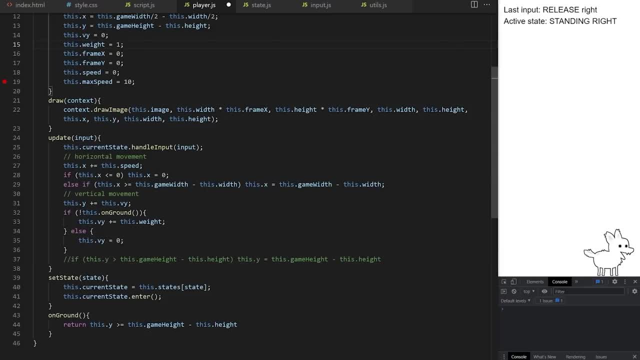 under any circumstances. I don't think this check is needed. even when I increase player weight to 10, we still don't fall through the floor. Maybe you can just comment it out. it's up to you. It's just a check to be secure. 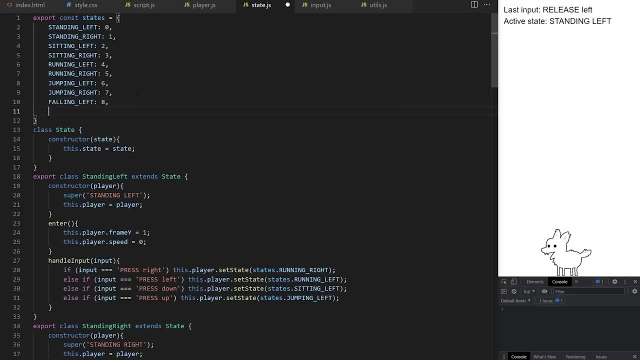 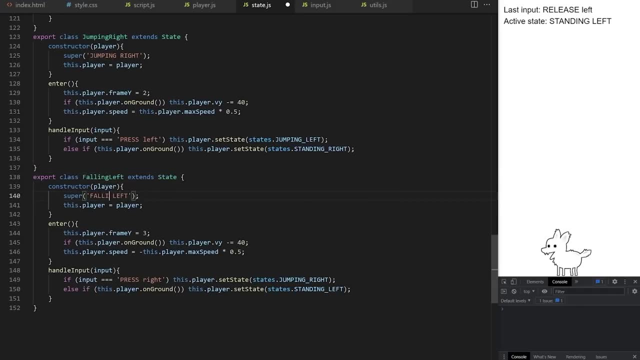 I created falling states. Fall in left is 8 and falling right is 9.. I copy one of my state classes and I turn it into falling left. Enter method will just set frame y to 5. Inside handle input method, while in falling left 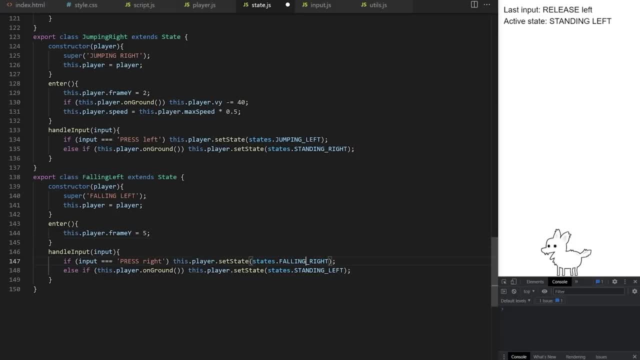 if we press right arrow key we want to turn, so we will switch to falling right. I also want to keep this check: When we fall all the way to the ground, we will switch player to standing left state. I copy this and turn it into falling right class. 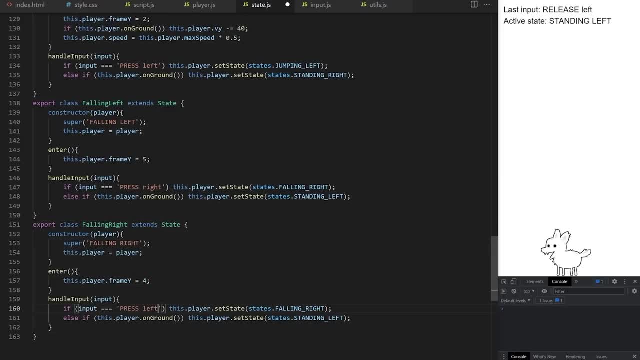 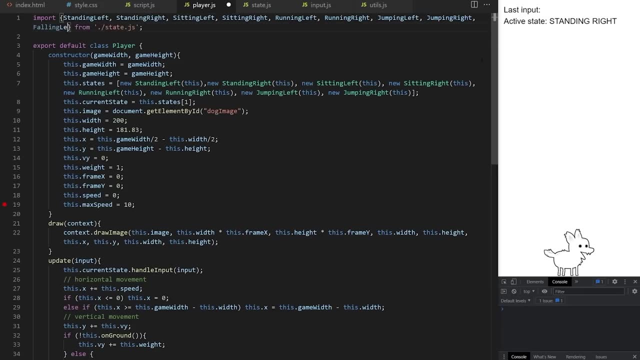 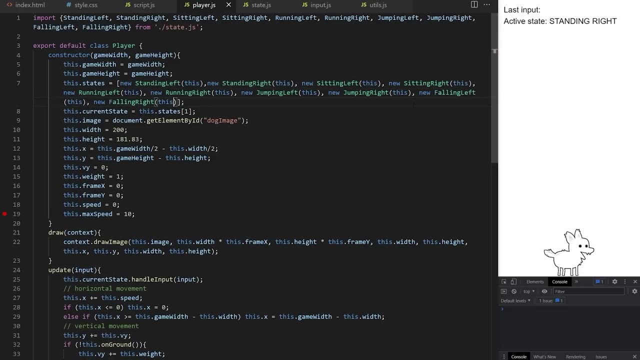 Frame y here will be 4 and when we press left we set state to falling left. I import these classes in playerjs and I instantiate them inside player states array. So how do we enter falling state? As we said when we enter jump velocity y? 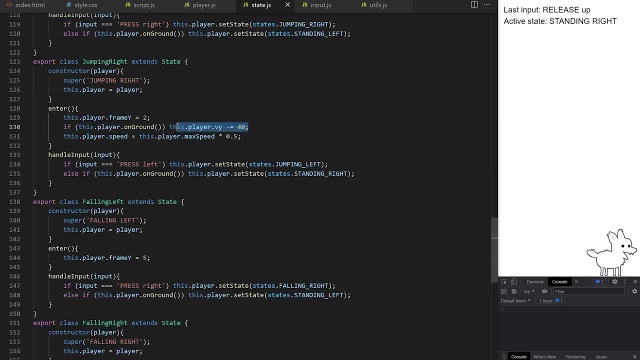 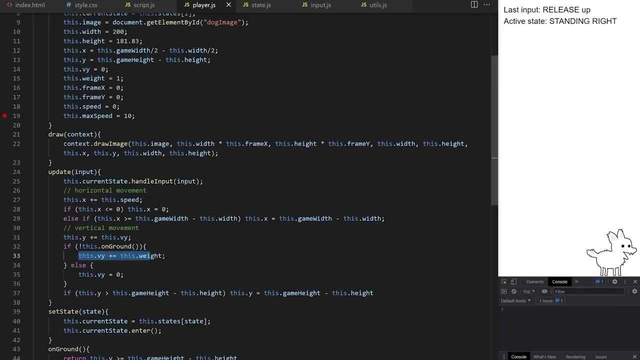 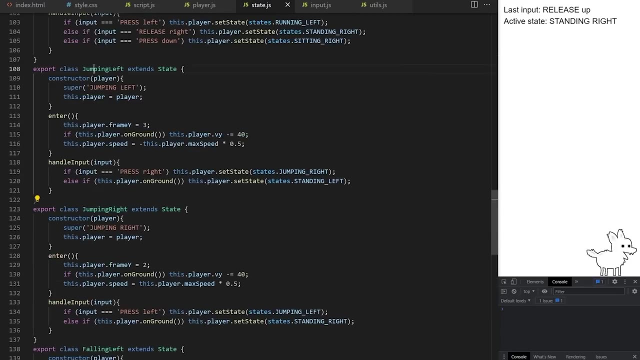 is set to minus 40 and we start adding player weight to it. So it goes all the way to 0 and into positive numbers. I know at the point velocity y reach 0, we are at the peak of jump and as it goes into positive numbers, player is falling back down. 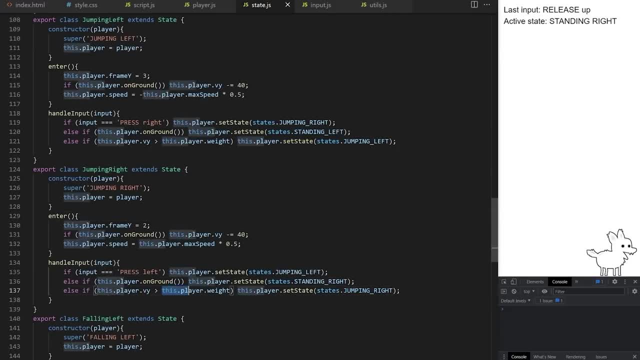 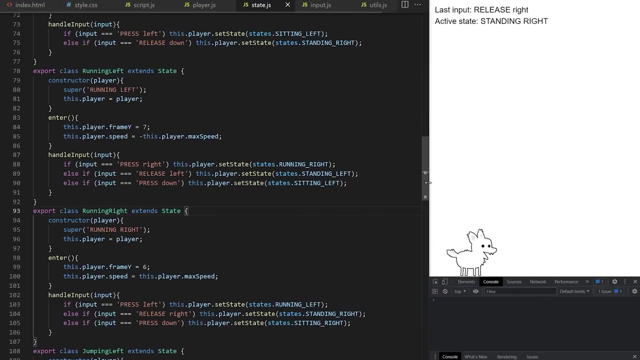 Bear with me a second here, please. So inside jumping left state: if velocity y on player object is more than 0, we set player to falling left. Inside jumping right state: if velocity y is more than 0, we set state to jumping right. So this is one example of how you can switch states based on other conditions. 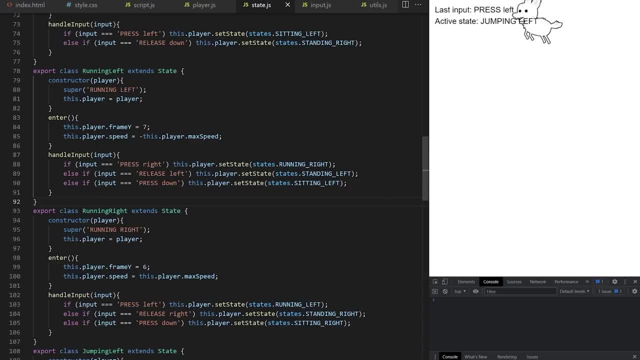 State changes don't always have to be triggered by user pressing keys on keyboard. This works really well. We created standing, sitting, running, jumping and falling states. We are just drawing the first frame in each spreadsheet row. Let's actually animate the frames horizontally. 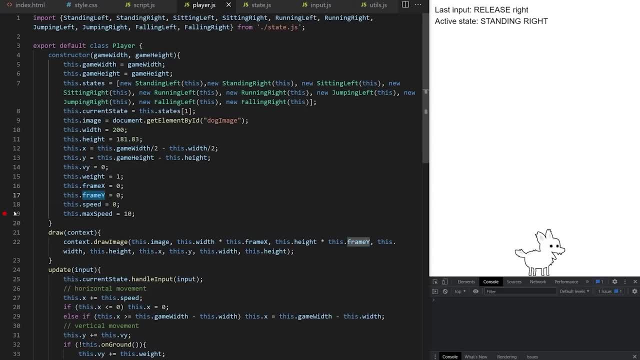 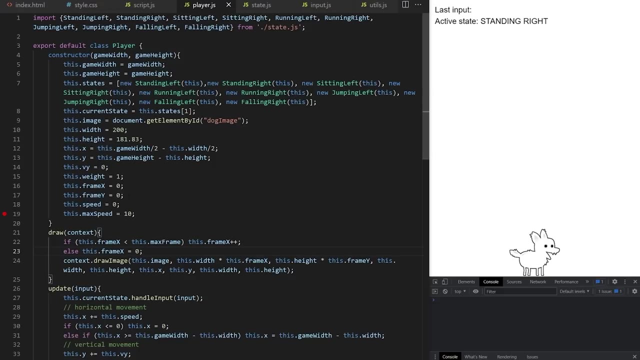 We have frame x property for horizontal navigation within our spreadsheet. For every animation frame I check if frame x is less than max frame and I increase frame x by 1.. I set frame x back to 0.. Some rows have different maximum number of frames but that's easy to deal with. Initially I set 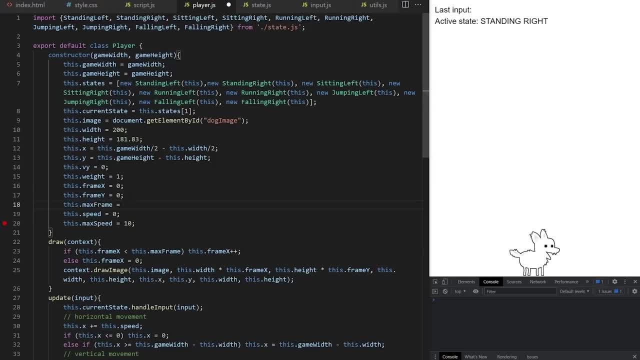 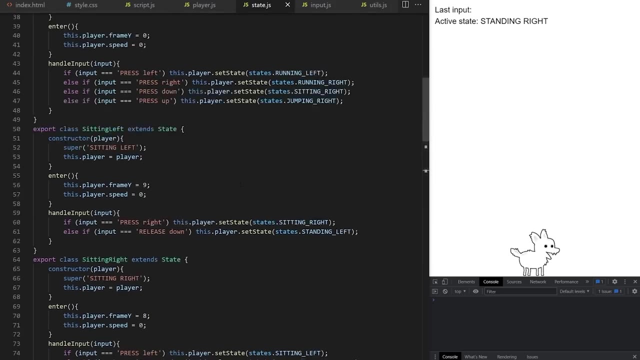 max frame to 5.. We are counting from 0.. You can see that sitting animation has less frames, so it's blinking. since we are animating empty frames, We will start with. standing animation frame is 6.. Every time we enter a new state, we set max frame to a different value When. 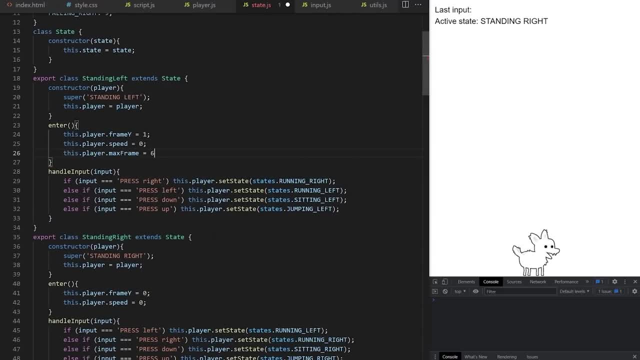 we enter standing left, we set max frame to 6.. Probably I should be setting max frame before I set frame y, because in some cases if I switch row at first we can get blinking before the right max frame is applied. Or maybe I could also set frame x to 0 every. 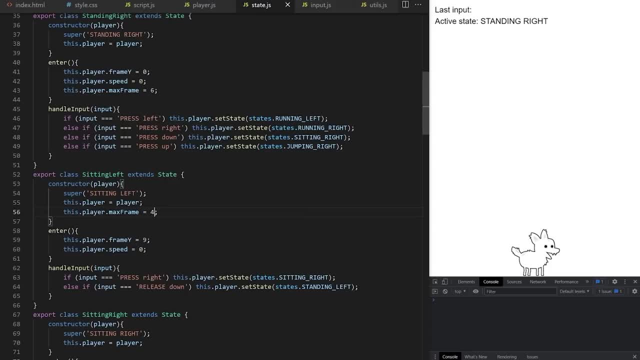 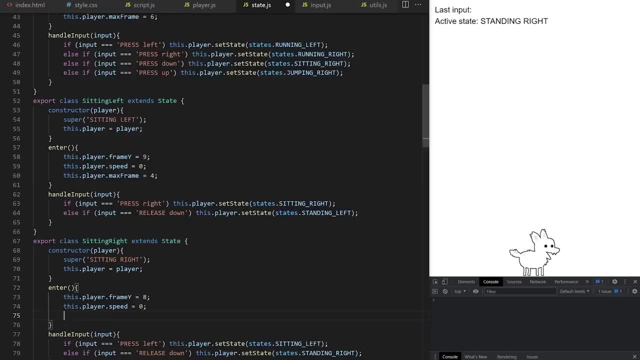 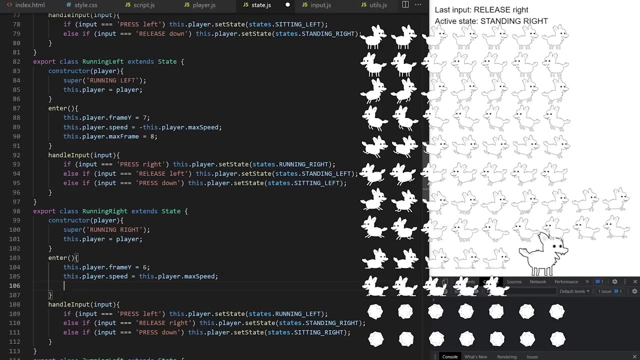 time we enter a new state. I'm not gonna go deep into this today. I made other episodes about sprite animation. This is just a quick solution. Running left and running right will set max frame to 8. Jumping and falling have max. 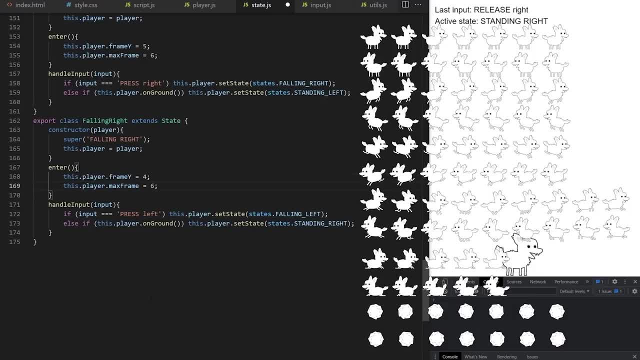 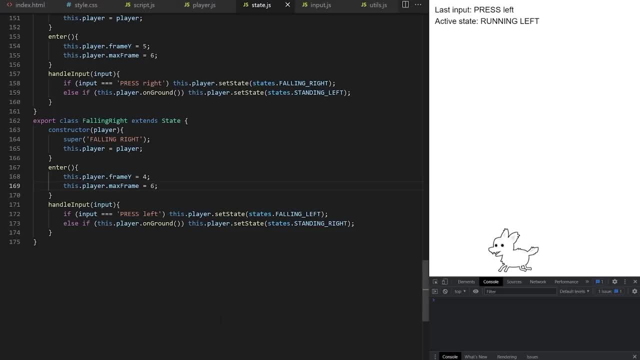 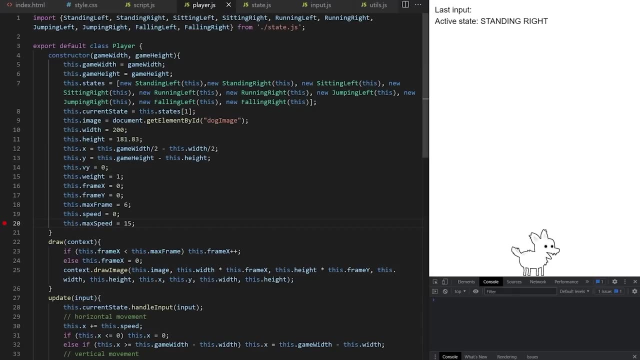 frame 6.. Awesome, We are correctly animating all our rows. If you want to make player move faster, you can change max speed property here on line 20.. This value affects horizontal movement. The sprites are animating very fast. Maybe I want to slow them down a bit Without. 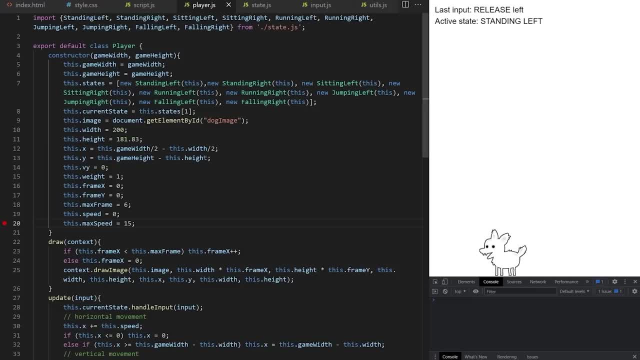 changing fps of the entire game. How do I set fps for how often we switch between horizontal frames in sprite sheet while still keeping everything else running at max 60fps? As always, we can use timestamps and delta time. Last time will be the value of timestamp from the. 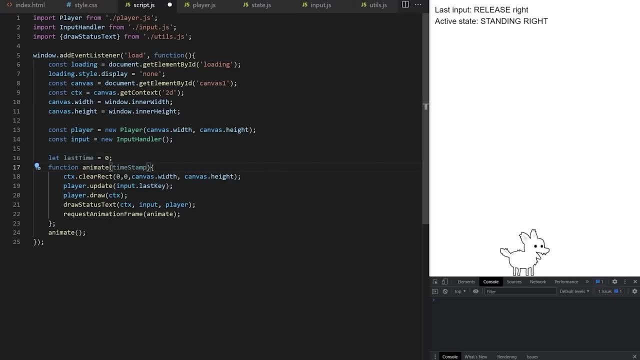 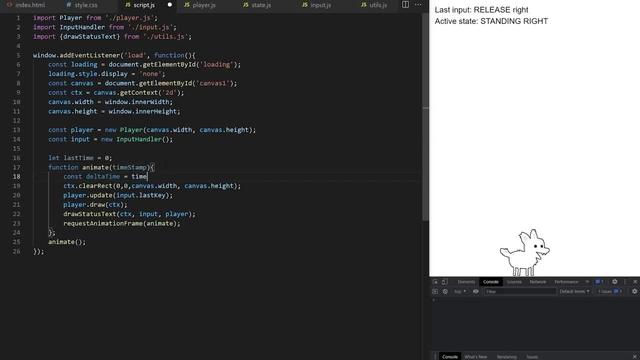 value from line 23.. Delta time is a number of milliseconds that passed between the last animation loop and this animation loop. It's the difference between timestamps from each loop. So delta time equals to timestamp from this loop minus timestamp from the previous loop. When we have that calculation, I set last time to the current timestamp so that 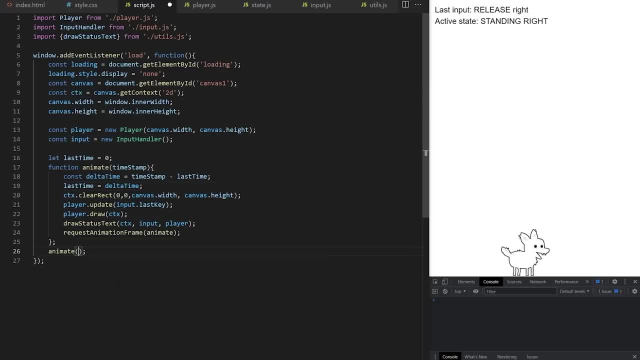 it can be used for the next loop. I also have to pass animate the initial timestamp just for the first loop, because request animation frame auto generates it from the second loop onwards. So now we have delta time. We know how many milliseconds it takes for our computer. 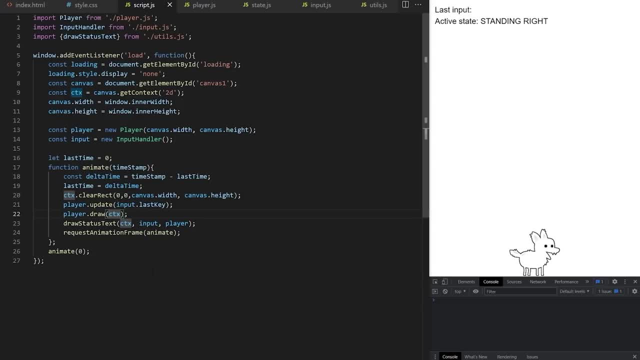 to serve the next animation frame. It depends on power of our machine, how much animation and calculations our game is doing per each frame, as well as on refresh rate of screen we are using. This number can be different for every computer, but we can use it to unify. 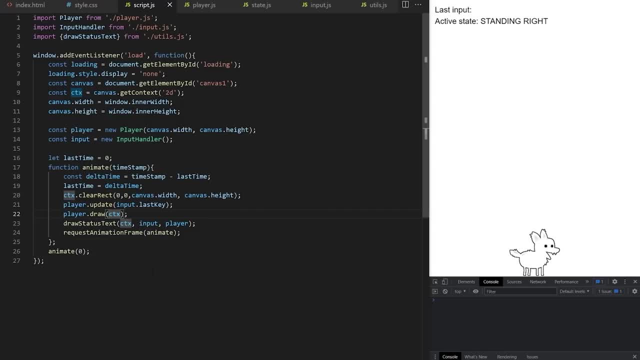 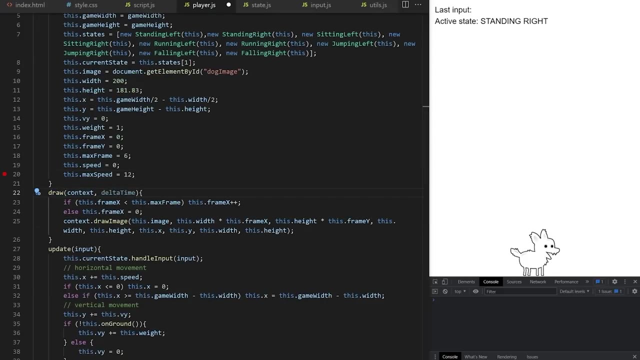 how our game runs across different machines. Today I will use it to control how often we serve the next horizontal frame in Docs sprite sheet. I pass delta time to player draw method here and in playerjs. I make sure draw method expects that argument. Timing things with delta time needs three helper variables. One variable 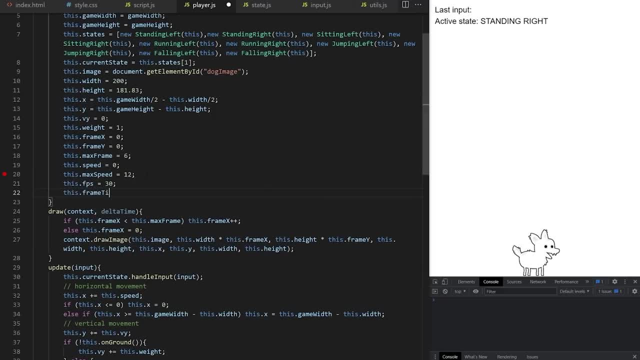 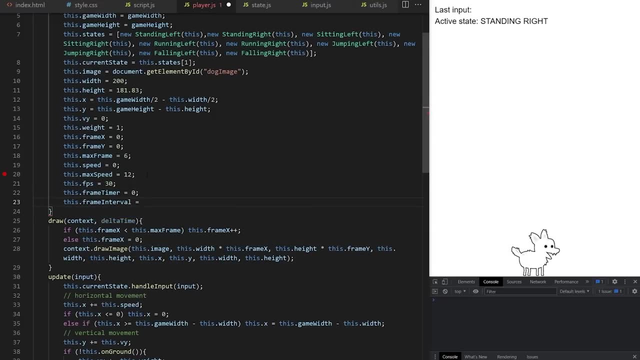 to set FPS frames per second, One timer variable that will accumulate delta time until it reaches a certain value And one variable that defines that value we want to reach. I call that value frame interval and it will be 1000 milliseconds divided by frames per second, which will give 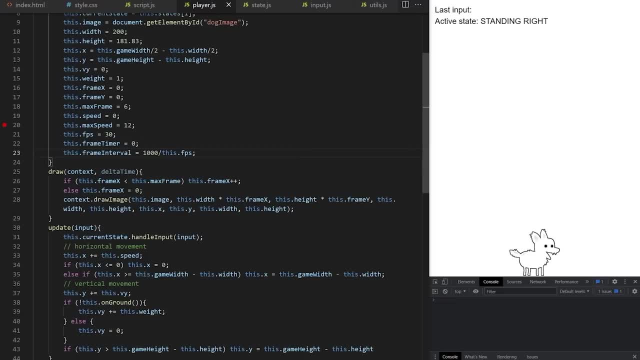 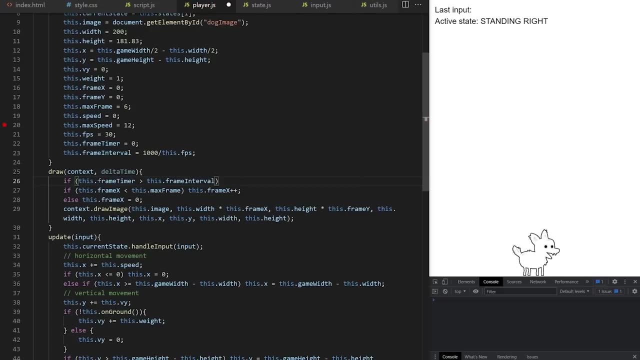 us the number of milliseconds. I want each frame to be displayed on the screen before we switch to the next one. So if frame timer from line 22 is more than frame interval from line 23, only then switch frame x variable. At the same time set frame timer back to zero. 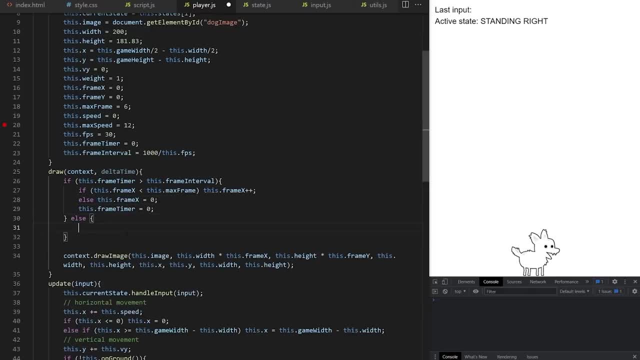 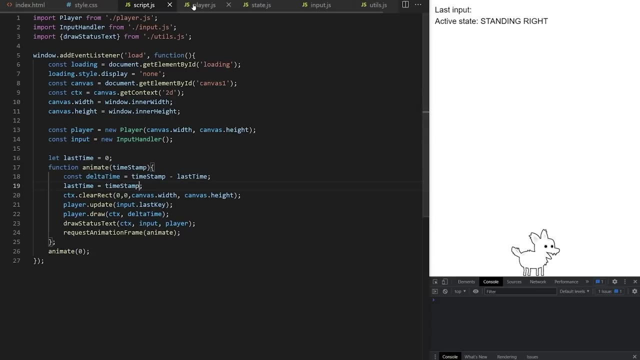 so that it can count again. Else, just increase frame timer by delta time and wait until it accumulates enough milliseconds. Hmm, it's not working. I see here an animation loop. I need to correctly assign last time to the new timestamp value after we used it to calculate delta time, so that it can be used to calculate delta time in. 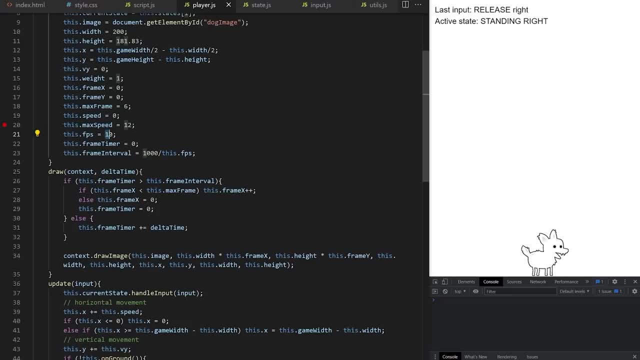 the next loop. If I change FPS, it affects how fast we serve horizontal sprites while still allowing player to move around at maximum 60 frames per second or whatever your request animation frame can handle on your computer. If I give it FPS that's higher than my screen's. 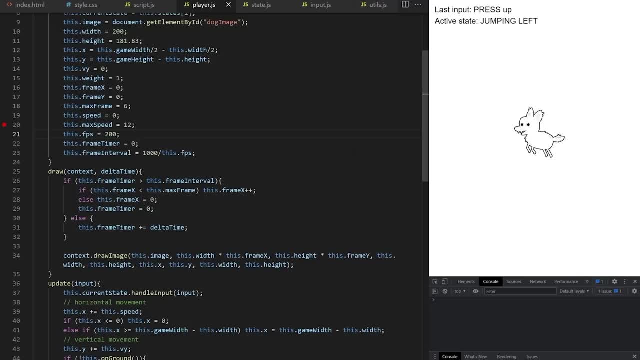 refresh rate. Request animation frame will automatically cap it, so it won't animate a faster past a certain value. That maximum value of frames per second is limited by your screen's refresh rate. Making games with JavaScript is one of my favorite ways to practice coding. 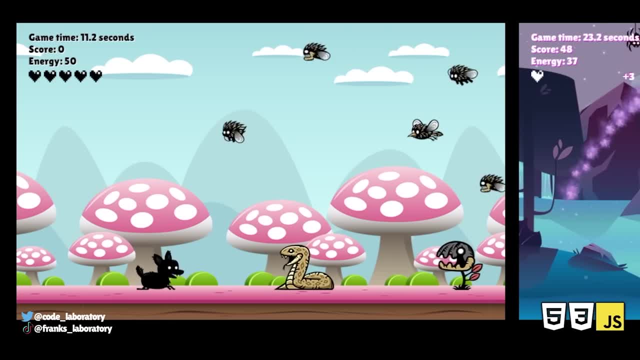 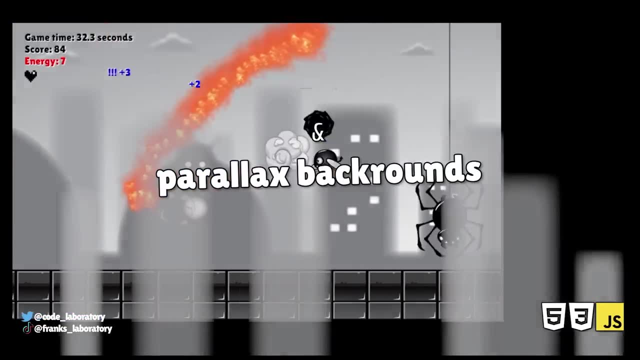 Today we will build a 2D game and we will animate everything to bring it to life. I want to show you how to make keyboard controls feel quick and responsive. We will apply animated sprite sheets and parallax backgrounds. We will learn how to give our game different. 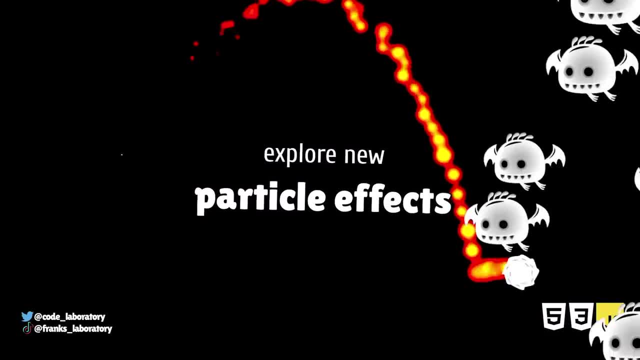 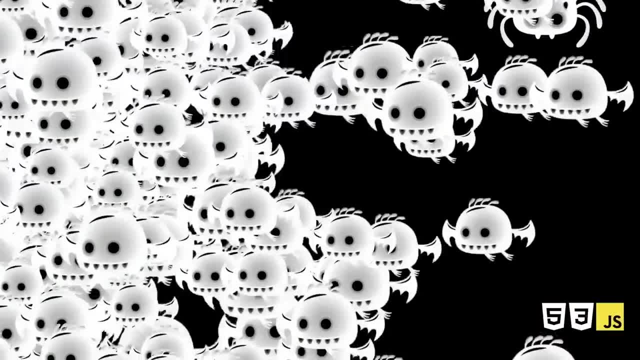 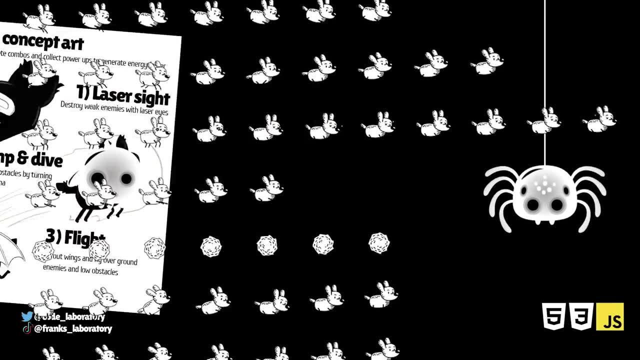 how to make a new animation, And we will learn how to make a new animation And we will challenge our players by giving different enemy types different behaviors. On my community page, I asked you to choose between three superpowers and you chose the fireball tackle. So let 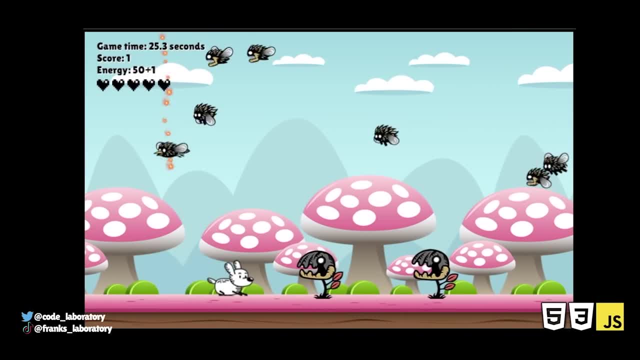 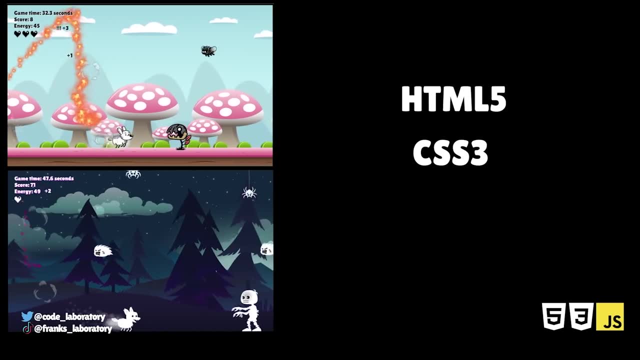 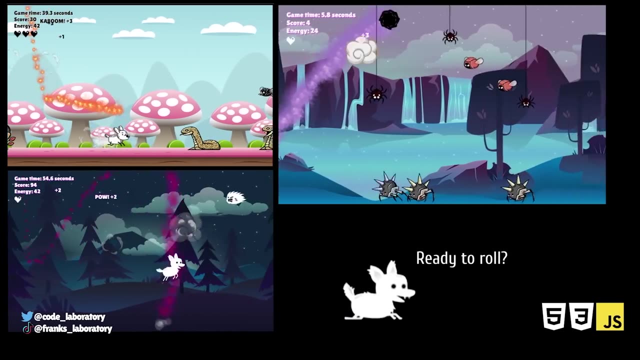 me show you how to turn into a flaming ball of plasma and vaporize enemies to earn points. Come join me and learn how to create your own 2D adventures with HTML, CSS and plain vanilla JavaScript, No frameworks and no libraries. Click the like if you want more games. 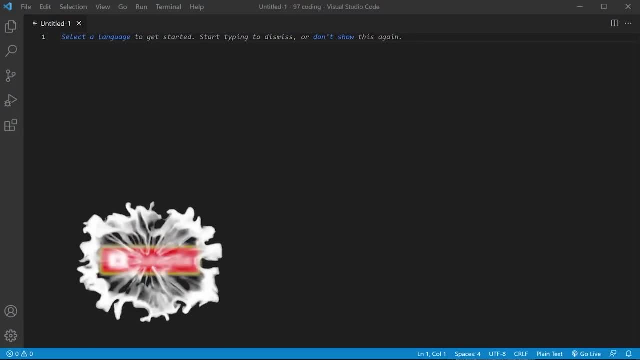 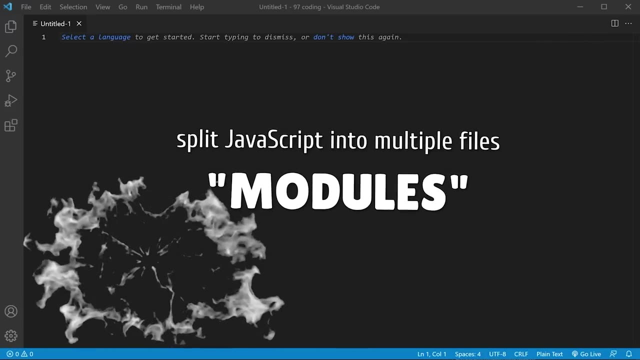 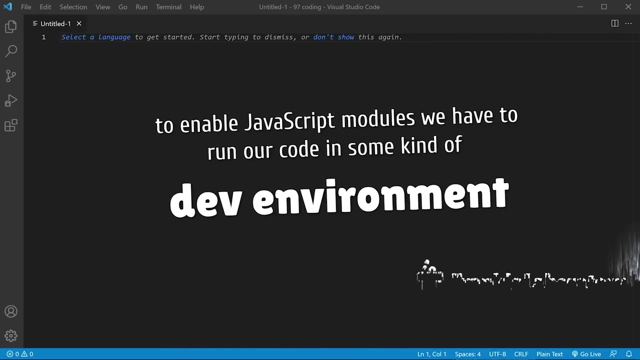 To keep the code organized and easy to navigate in, I will split JavaScript into multiple files, so-called modules, And I will export and import them around the code base as needed. To enable this functionality, we have to run our code in some kind of dev environment. 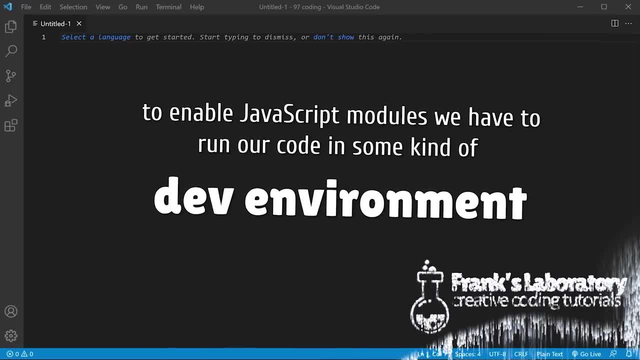 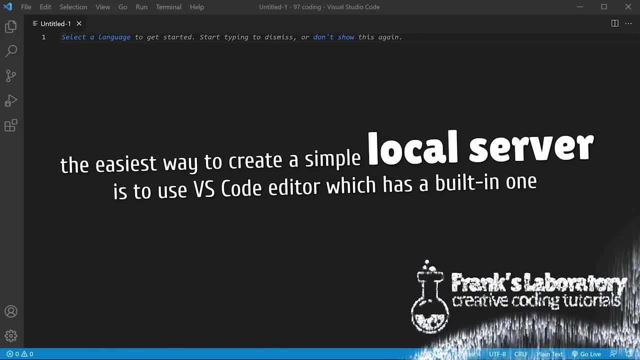 They need to be run through some kind of server. You might already have a preferred way to run a local server. You can go ahead and do that. For the rest of us, the easiest way to create a simple local server is to use the code that. 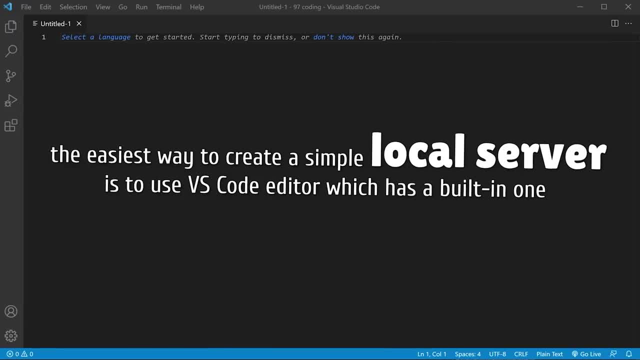 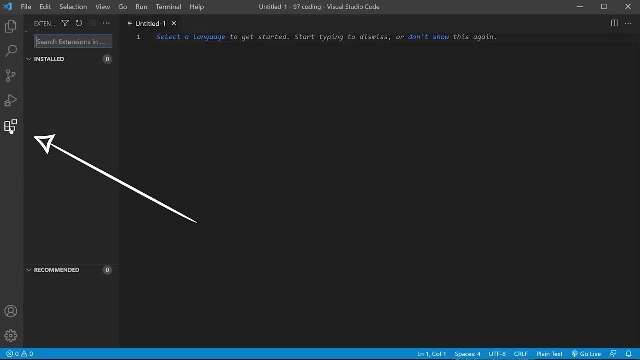 is already in the server. When you open your VS Code, check if you have this notification area down here that says go live. If you can't see it, you can just come here to extensions and search for live server. It's this one. Mine is already installed, You can just click. 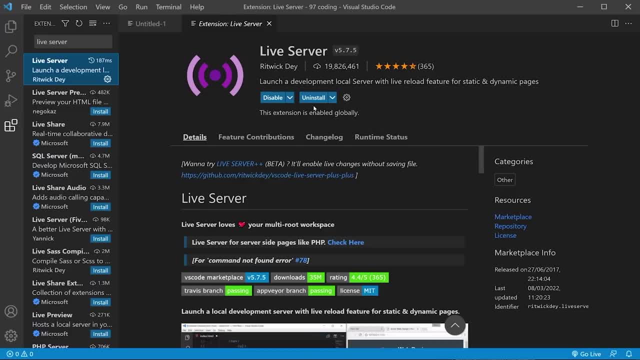 install here. When you install it, close your VS Code and reopen it and you will see, go live down here. One last thing to do: We have to point VS Code to the correct folder with the files we want to run through this live server. We do it. 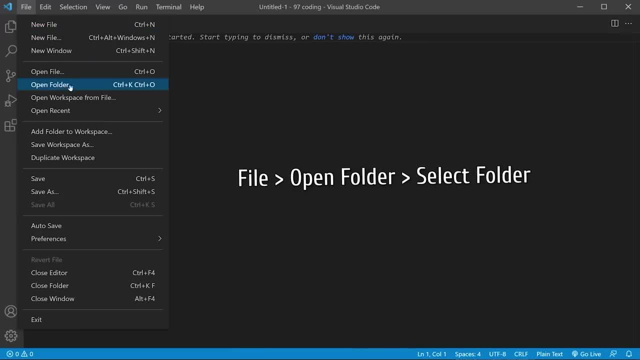 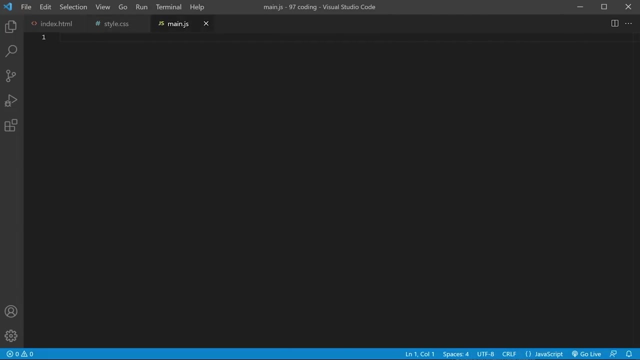 by going to file open folder and in there you navigate to the folder you will work with today on your local computer and click open. Now, when I create new files, they will be automatically created in that folder. So I create indexhtml stylecss and mainjs. 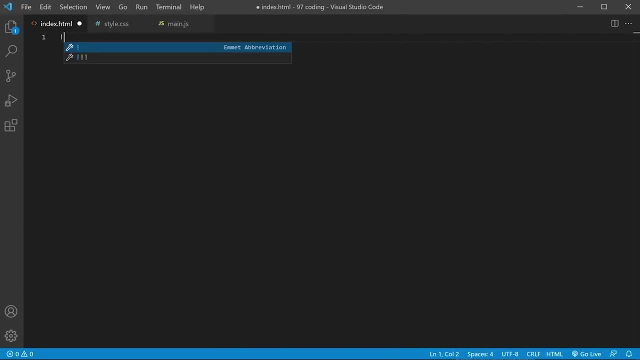 In indexhtml. I create a basic blank web page markup In VS Code. you can just press exclamation mark and tab key and it will create it for you. Let's give it some title and link stylecss file. I create a canvas element with an id of canvas1.. Down here I link my javascript using a script. 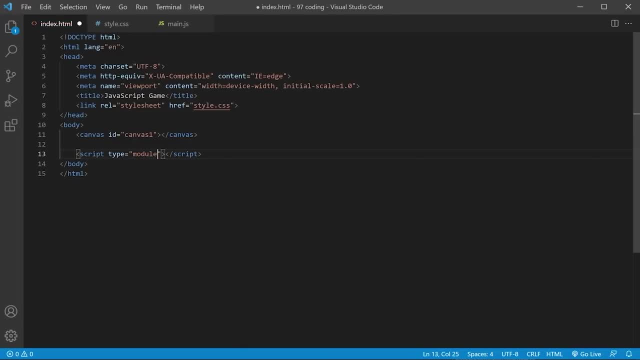 doc. I give it type attribute and set it to module. This specify that this file will be a javascript module. It will be my top level module and we will be importing other javascript modules inside. I click this go live button and a live server plugin will automatically. 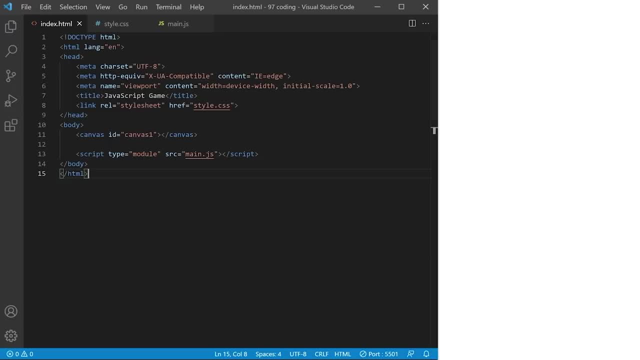 open my default browser and it will run our project in it. It will also automatically reload the browser window whenever we save any of the project files. You don't have to use VS Code and live server plugin If you know how to create your own local server in. 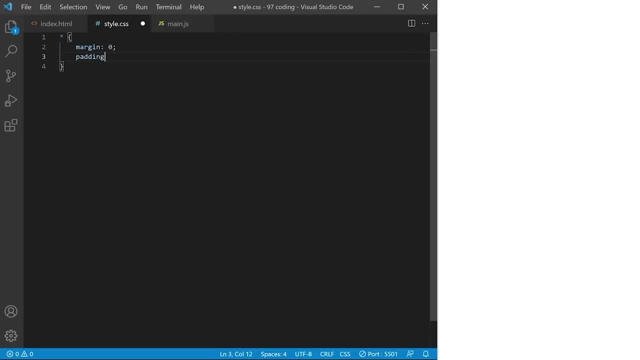 a different way. feel free to do that. So now I can see my live server is running on port 5501. It will reload browser window. whenever I save any project file, I usually use ctrl plus s keyboard shortcut to save. Sometimes you have to manually reload the browser page for the first time and then it. 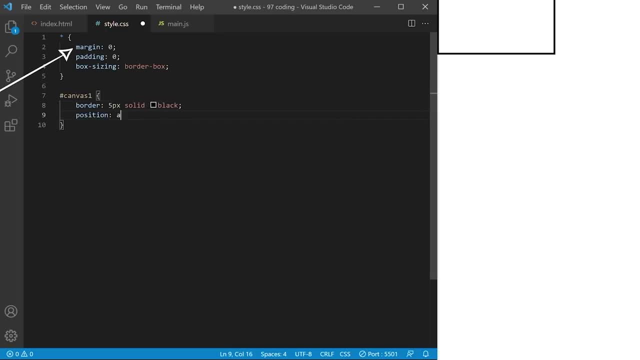 will start doing it automatically. In stylecss I reset margin and tab key, I click save In indexhtml, I create indexhtml and padding to 0 on all elements and I set box size into border box. This is so called global reset and we do it to make sure our page looks the same across different browsers. 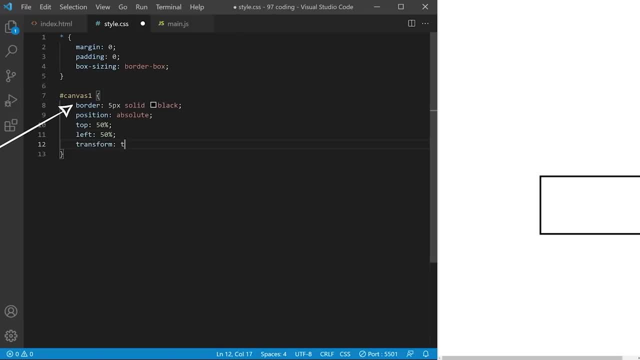 Canvas 1 will have border: 5px solid black and I center it in the middle of the page. so the usual 4 lines of css position: absolute top 50%, left, 50%. transform translate: minus 50%. minus 50%. 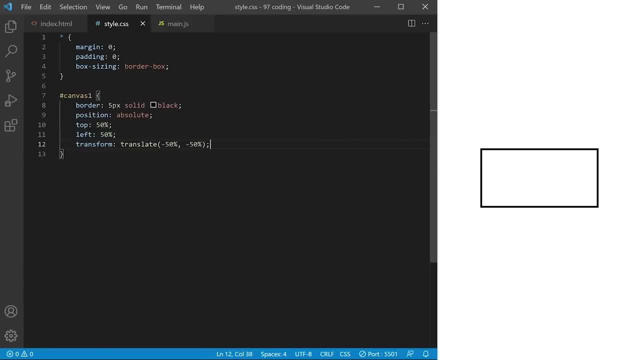 I will provide you with game art assets you can use to code along with me, and at the end, in the experiments sections, I will show you how to apply different skins to your game so that you can make it unique based on your own creative preferences. 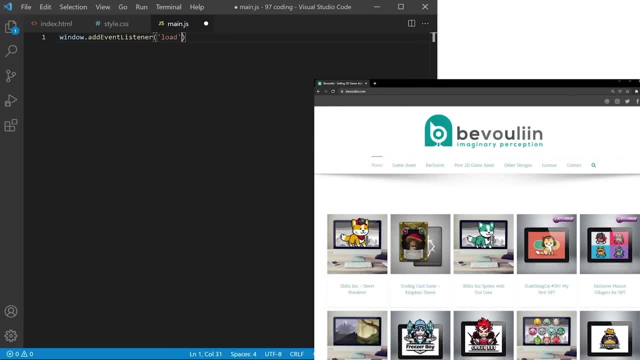 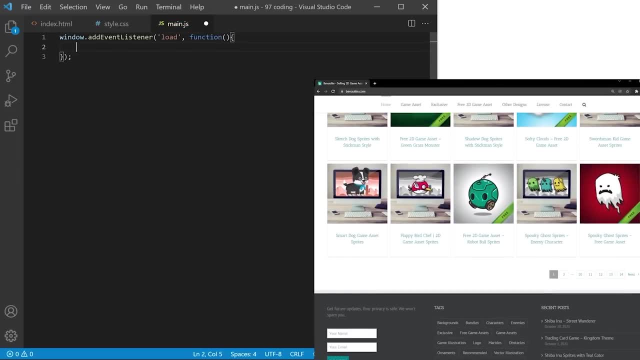 Check out this website for more beautiful art assets that are already compatible with today's project. Today, we will be using images for player backgrounds, enemies and other things. The easiest way to make sure our code runs only after all art assets are loaded is by: 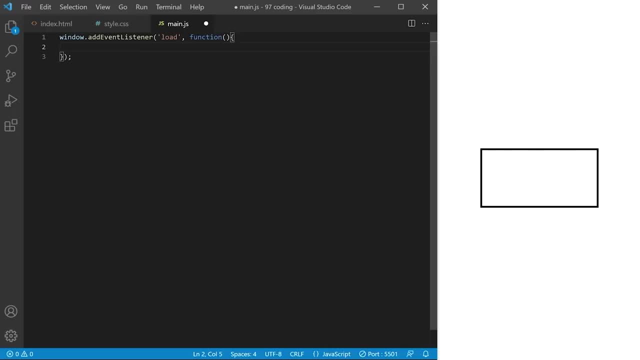 placing the images inside indexhtml, which we will do in a minute, and we will put all javascript inside a callback function on event listener For window load event. That way, javascript waits for all dependent resources, such as stylesheets and images, to be fully loaded and available before it runs. 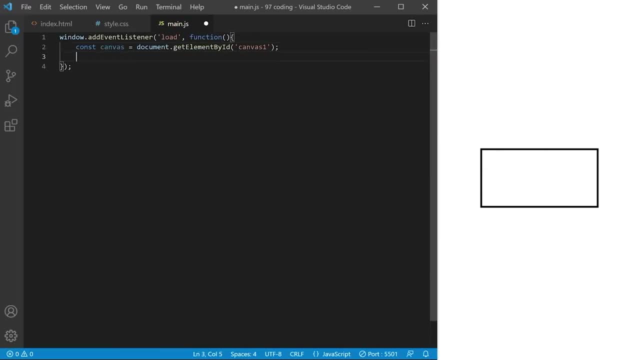 When the page is fully loaded, we will point javascript towards our canvas element using its id. I create an instance of built in 2d drawing api using get context method and I save it as ctx shortcut for context. Canvas width will be, for example, 500px and height 500px as well. 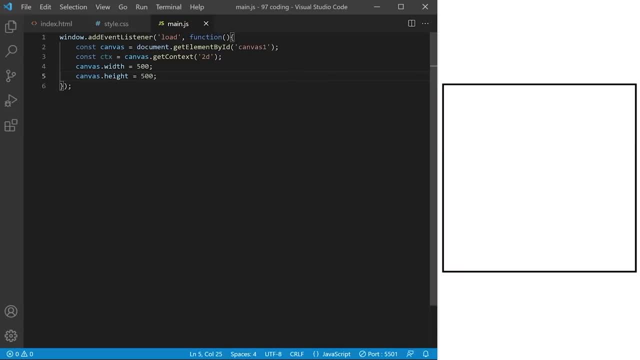 You can make your project wider, But keep the height at 500px for now because I optimized the background images for that size. We can make canvas, scale up and down to make sure it's always fully visible. If I set width to 1500px, we can only see the middle. 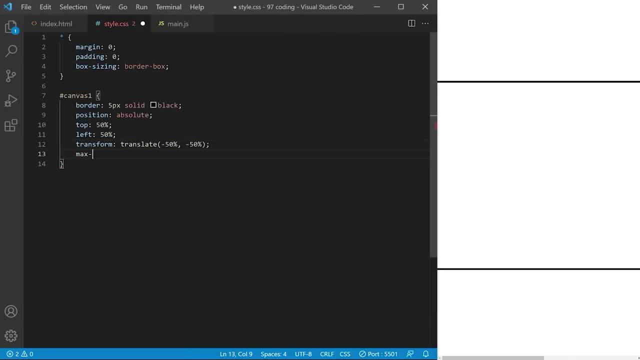 It's cut off on left and right. I can give it max width 100%, and it will make it scale down until it's fully visible. Whenever the width of the page is less than the width of the canvas element, I can also give it max height 100%, in case that the restricting factor is page height. 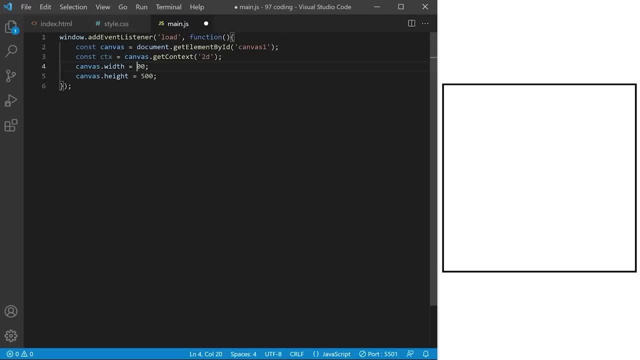 Now we can always see the entire canvas regardless of its width and height. I set it back to 500-500 for now. The main brain of our project will be this game class. All logic in our project will somehow go through it. It will expect width and height as arguments and inside we convert these to class properties. 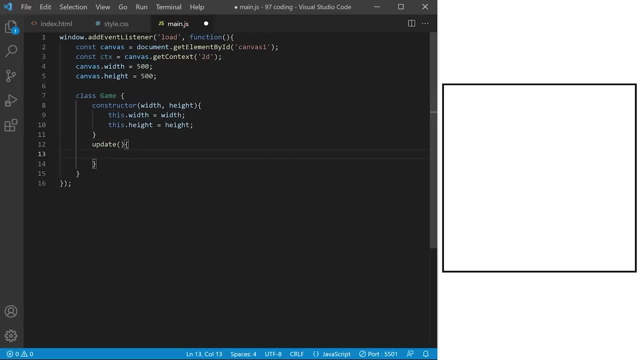 like this: It will have update method that will run for every animation frame and trigger all calculations that need to happen, and draw method will draw our images score and so on. Right now we don't have anything to update. I create a new javascript file called playerjs. 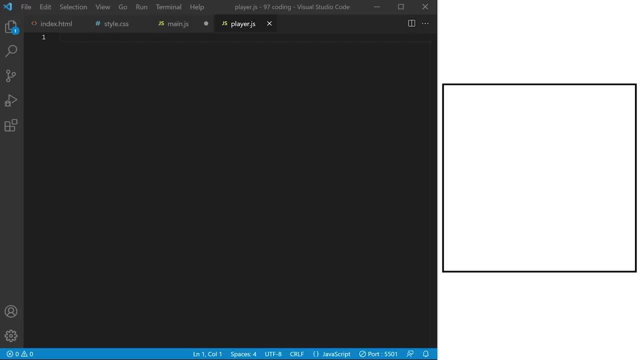 If you are a beginner, it will be easier for you if you follow my code exactly and use the sprites and images I provide you, and only once you have a working project, then you can modify it and add your own art assets and game features, if that's what you want to do. 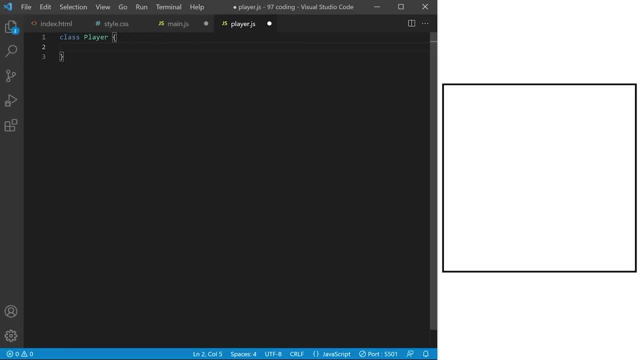 Inside playerjs, I create a class called player. Its job will be to draw and update our super dog. character Constructor will take the entire game object as an argument. Through it, we will have access to some things we will need, such as width and height of. 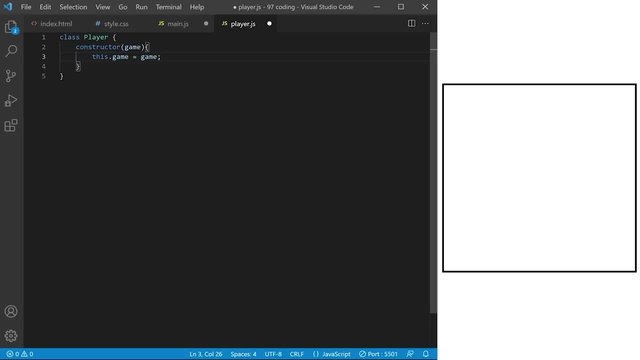 the game area and so on. Javascript objects are so called reference data types, which means when I pass the entire game object to other classes like this, I'm not creating a copy of the game object, I'm just pointing to it. So now it's time to bring player image to the project. 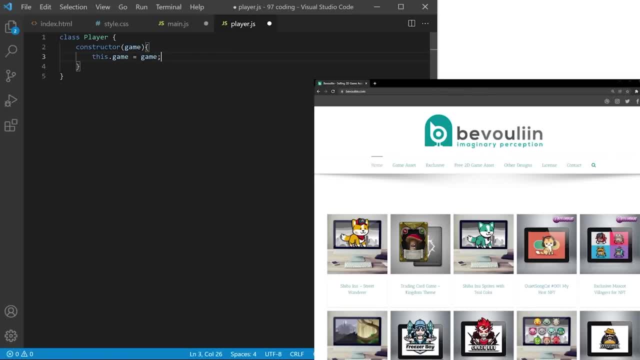 It was provided by this talented artist and you can download it for free in the video description and use it for learning purposes to follow along with this class. Check out their website for more game art assets if you want to make your project. Thanks for watching. 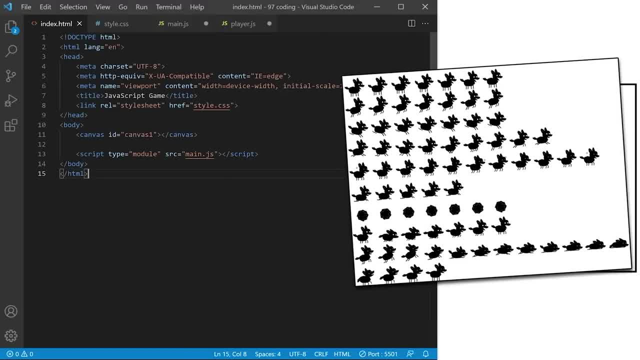 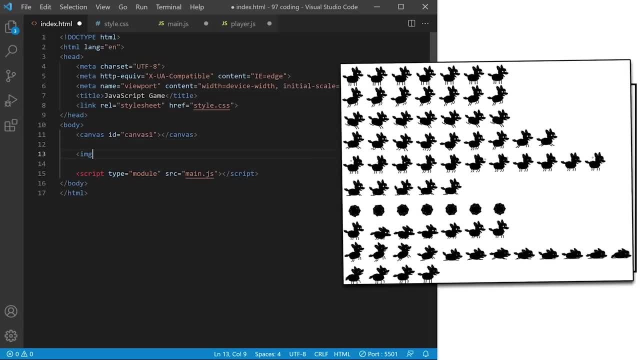 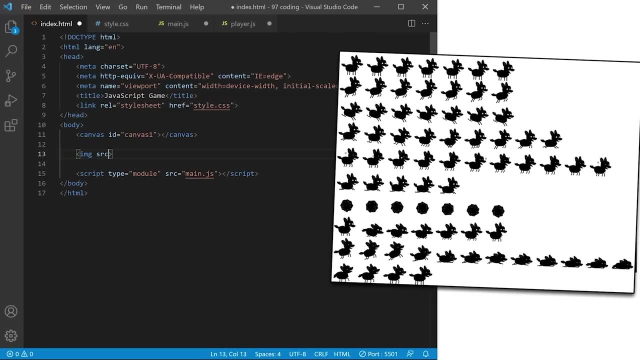 So we have some images, and sometimes it can take a while, maybe even a couple of seconds, for the images and audio files to load In javascript. if you try to use an image that hasn't yet been fully loaded, you will get an error. We need to make sure our images are loaded and available before we draw them. 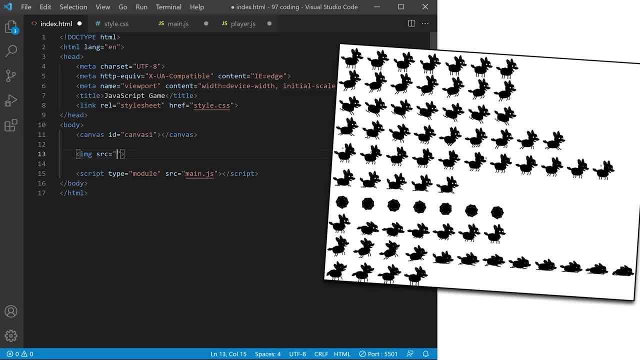 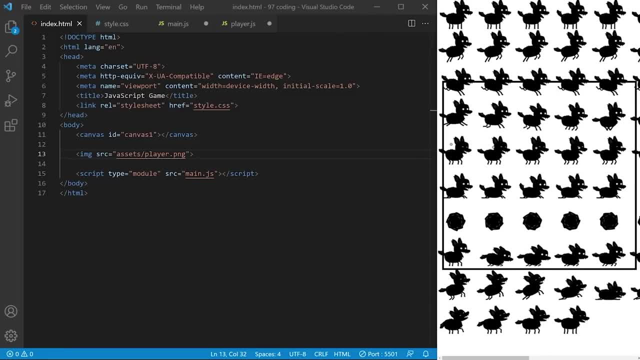 One way to do that, and the simplest way to do that, is to actually include those images on our web page. I simply create an image element and as a source I point it towards the image file. I have a folder called assets in the same place where my indexhtml file is, and in there. 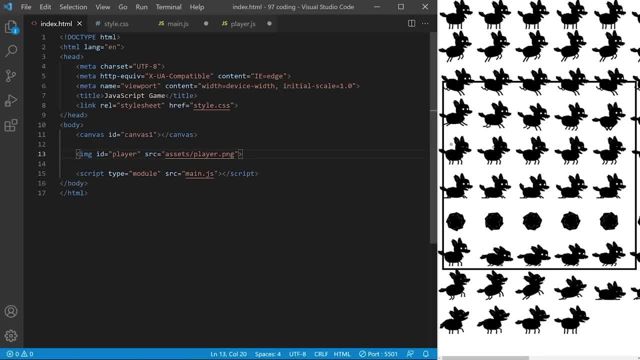 the image I want is called playerpng. I give it id: player, like this. I will draw that image on canvas with javascript, so I don't really want to display it on the web page like this: Install css. I target it using its id and I set its display to none. 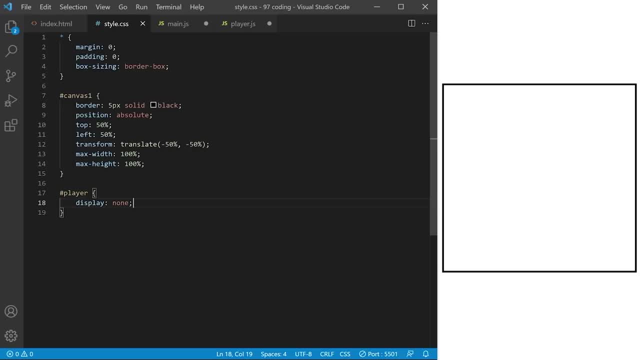 It's a good practice to make your images the exact size you will use in your projects. We can scale it down with javascript, but for maximum performance it's better to size your images in photoshop or some other graphics editor. I already did that with the images I gave you today and I sized each frame to the same. 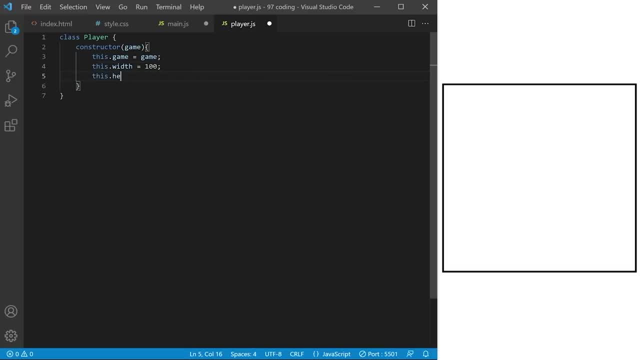 size we will display in game. The width of each single frame in the sprite sheet will be 100 pixels and height will be 91.3 pixels. If you are using your own sprite sheets, you can get the width of a single frame by taking 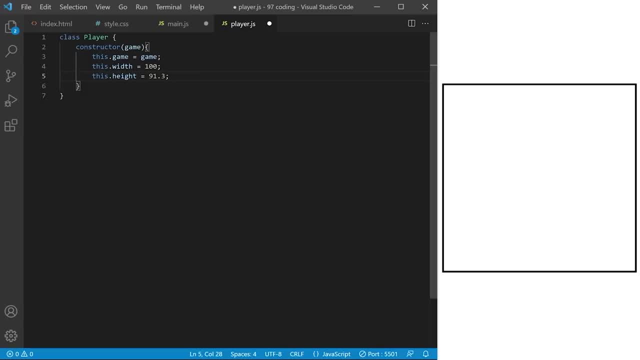 the width of the entire sprite sheet and dividing it by the number of horizontal frames And height is the height of the entire sprite sheet divided by the number of vertical frames, not the number of rows. Player will also need to be positioned somewhere on canvas, so it will need x and y position. 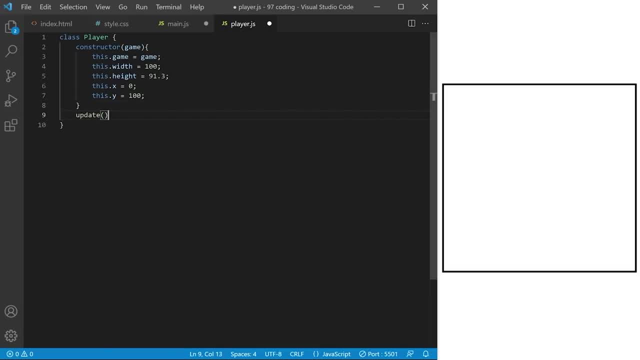 It will have update method that will move it around based on user input and it will cycle through the sprite frames and draw method will take those values and it will draw currently active frame at the current coordinates. It will need context as an argument to specify which canvas element we want to draw on. 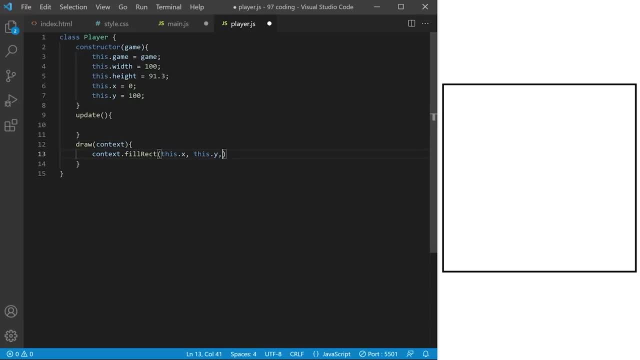 Let's start by calling fill rectangle first and we draw it at coordinates thisx, thisy and we also specify its width and height. If I want to use this javascript class in a different module, in a different file, I need to export it. I can just say export, like this. 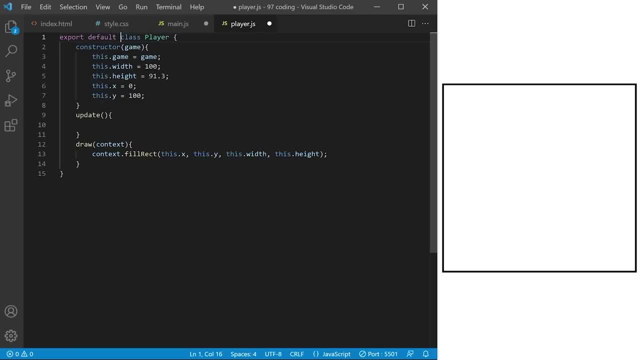 Each file can have unlimited amount of exports Or I can say export default. Each file, each module can have only one default export. In mainjs I import player class by going up top and saying import player in brackets like this: from dot forward slash playerjs in quotes. 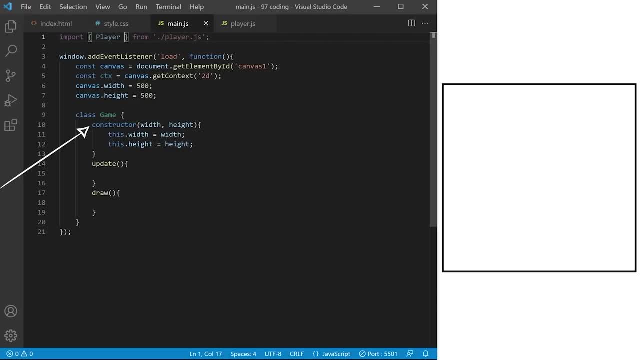 Class constructor on javascript class is a special thing. It gets automatically executed when we call this class using the new keyword. It will create one new instance of this class and, as a side effect, all the code inside the constructor will run. We can take advantage of that by putting in any code we want to run at that point. 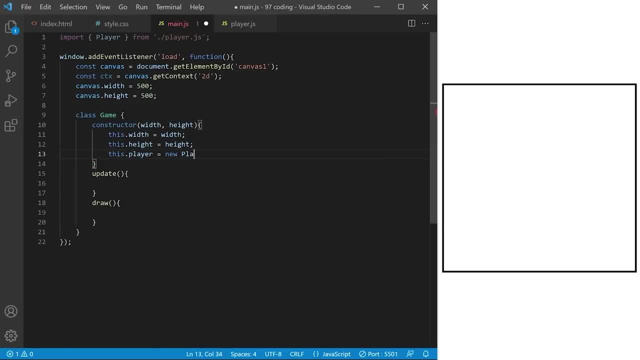 When I create an instance of game class, I also want to automatically create an instance of player class. Since I'm importing player class on line 1, I can instantiate it here. This dot player property on game class will be new player like this: 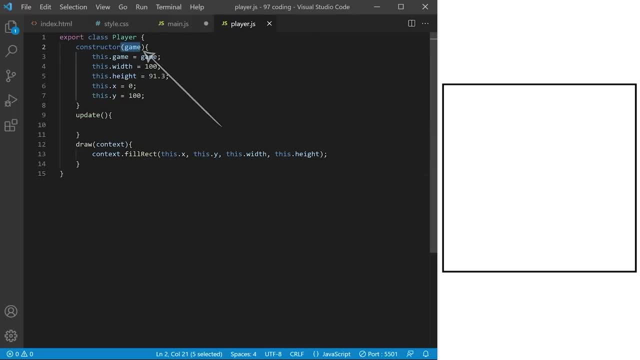 Inside playerjs. on line 2 I can see that player class expects game as an argument. So here, since we are inside that game class, I will pass it this Inside game class. this keyword means this game object, Now that we have access to the player object from within game class, here inside draw method. 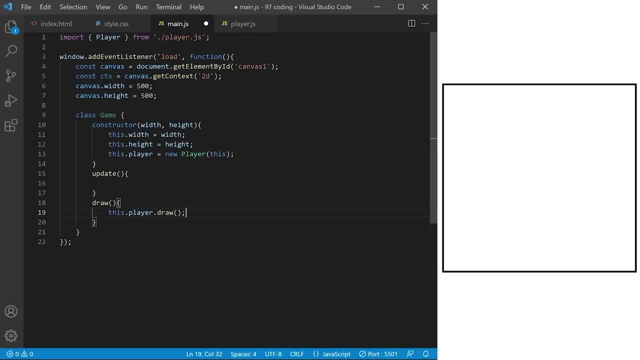 I can take this dot player from line 13 and I call its draw method. We declare that draw method here on line 12 inside playerjs, And I can see it expects context as an argument. My main public method will be this: draw on game class. 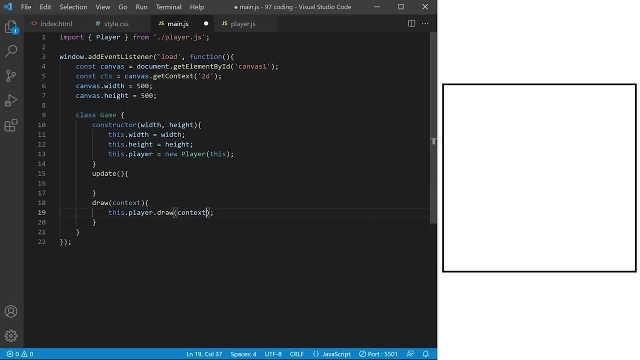 It will get context pass from the outside in a minute and we will just pass that reference along to player draw like this: Our game class is complete. Let's create an instance of it. I need to pass it width and height. so I pass it: canvas width from line 6 and canvas height. 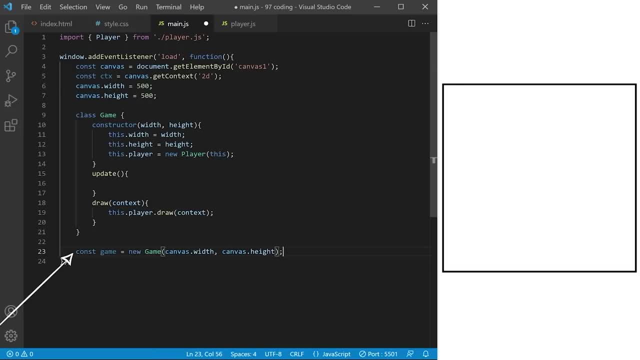 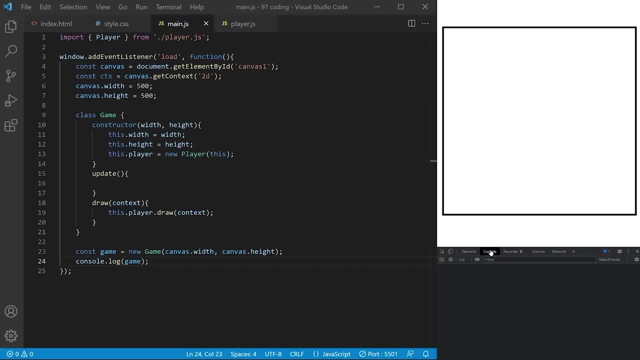 from line 7.. So now we created an instance of game class which triggered class constructor and that automatically triggers class constructor. Now I can see that constructor on imported player class and also creates our player. Make sure you save changes to both playerjs and mainjs file every time you make any change. 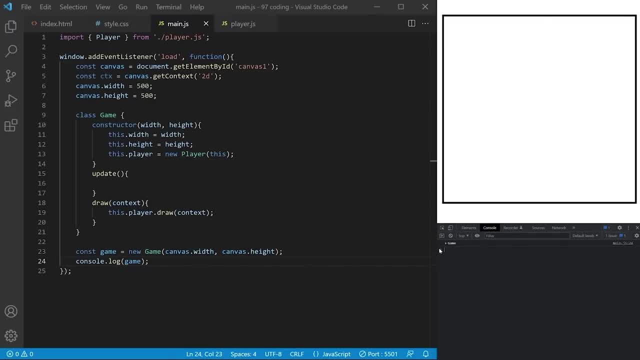 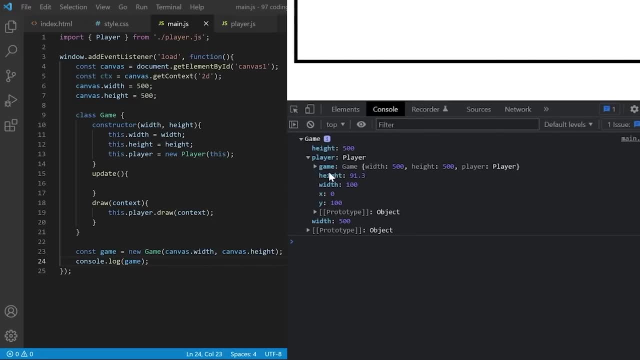 If you have any unsaved changes in playerjs at this point, you will not get the same result as me. I console log a game and I can see it has height, width and it contains player object as we defined in the constructor- Perfect. 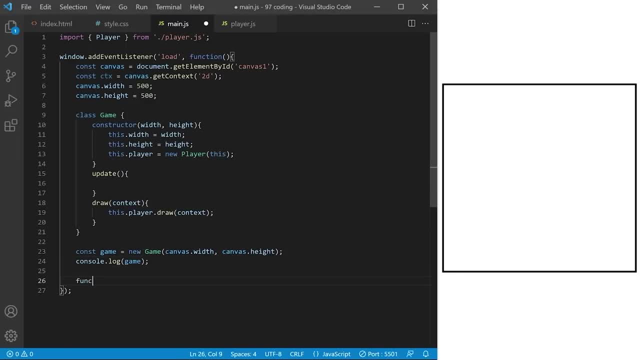 We will also need animation loop. because I want the game to update and draw over and over 60 times per second. I create a custom function. I call, for example, animate Inside. I call gamedraw from line 18 and as context I pass it ctx from line 5.. 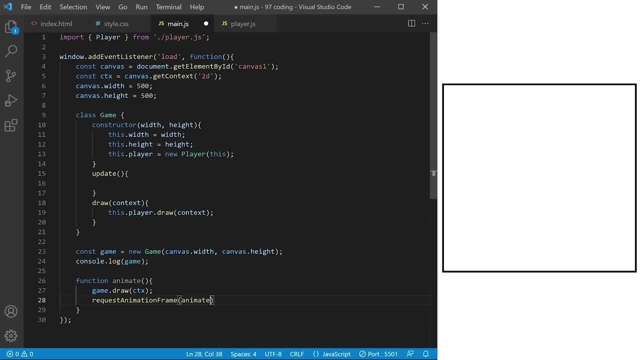 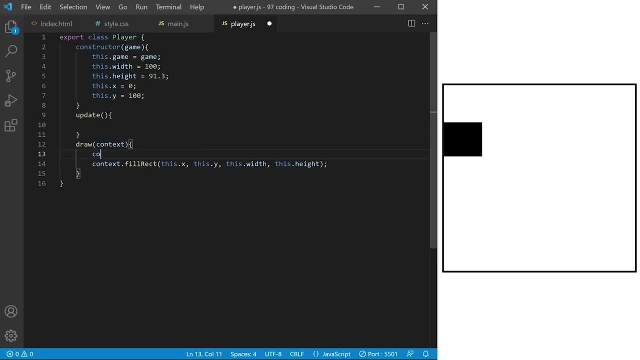 Then I call requestAnimationFrame and I pass it animate to create animation loop. When I call it, we are drawing this black rectangle representing player object Nice. This code inside draw method on player class will determine what the player looks like. I can make it red, for example. 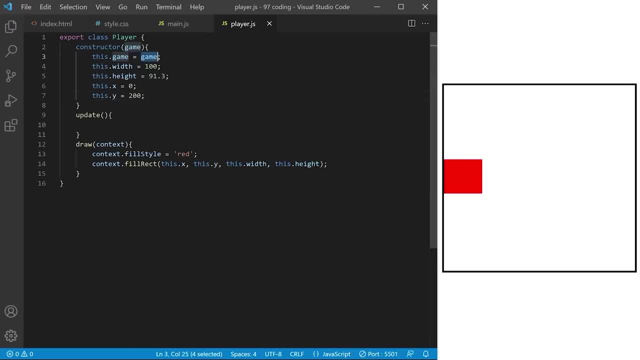 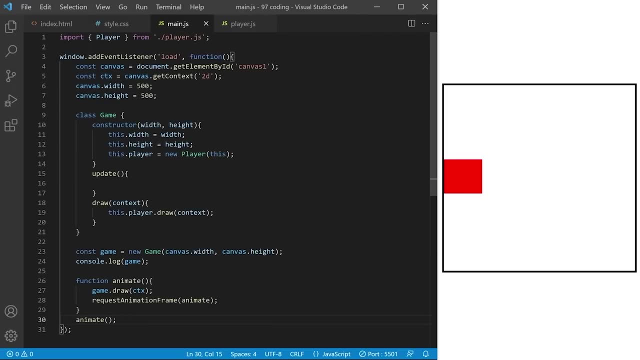 I can move it around by changing its coordinates. If I want to align the player on the board, Let's do that. of the game area. player object needs to be aware of game height. I have width and height of the game area here as properties on game object and I'm 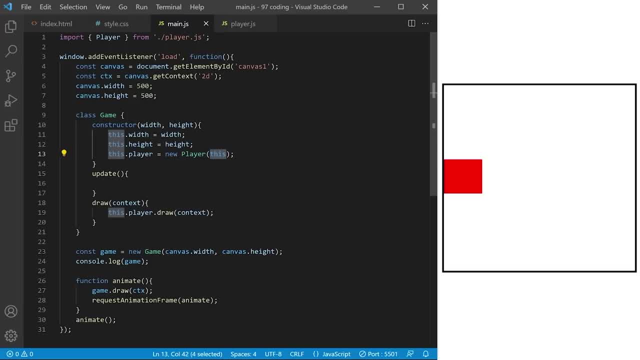 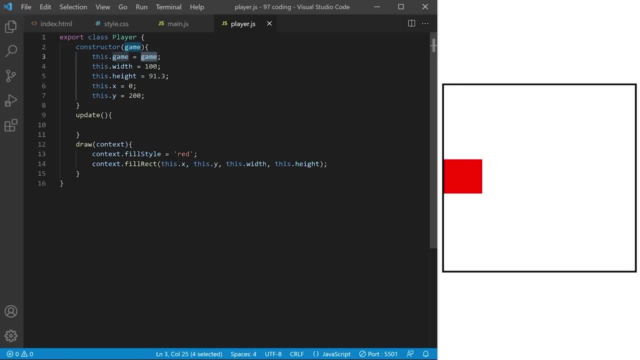 passing a reference to the entire game object to the player. here Inside playerjs I convert that reference to a class property called thisgame and I can extract width and height of the game from that. So to position the player on the bottom of game area, I set its vertical Y coordinate to thisgameheight. 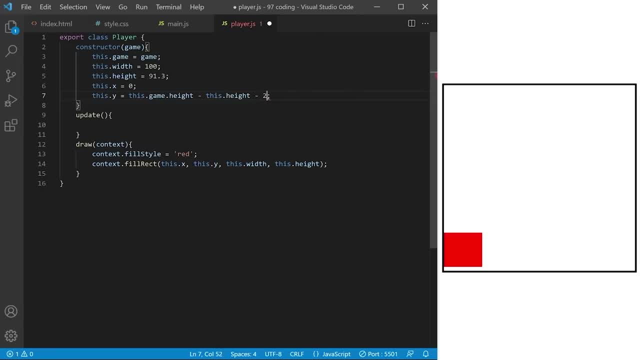 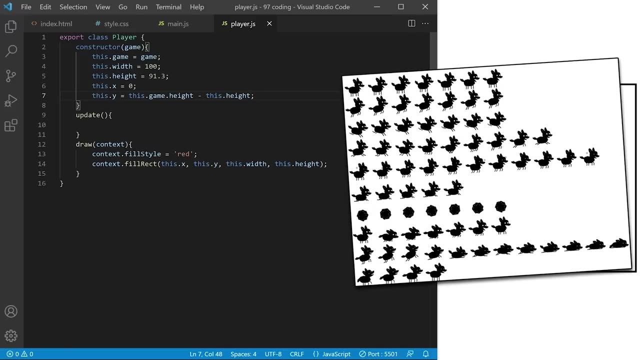 minus thisheight height of the player. I don't really want the player to look as a red rectangle. We have a special sprite sheet with our super dog to use here. We are about to learn how to use built-in draw image method to 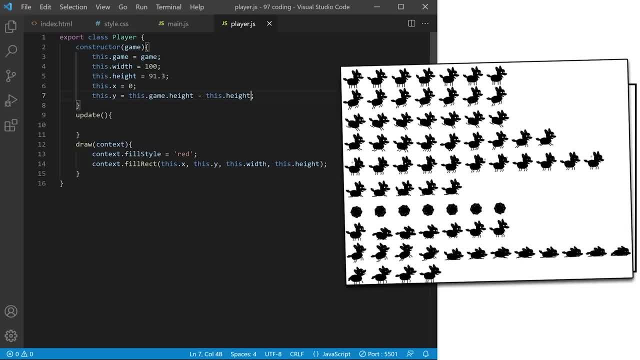 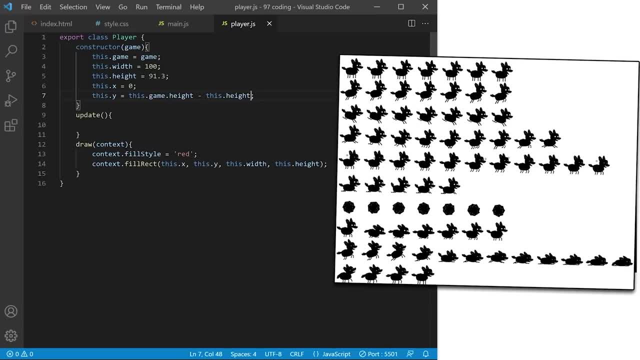 animate a game character from a sprite sheet. If you want to go deeper on sprite animation, the very first episode in the series linked below will explain it in a beginner friendly way. This is an advanced video. If you feel it's too challenging for you at some point, don't worry, it will make more sense if you. 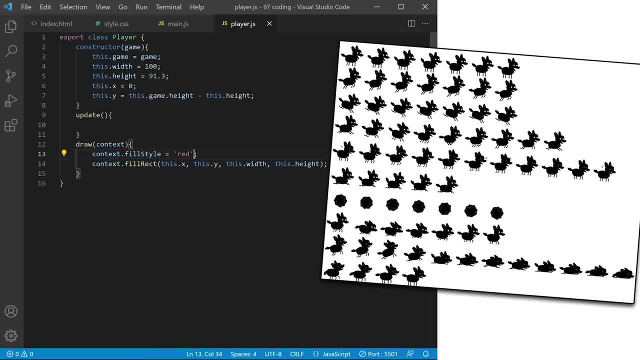 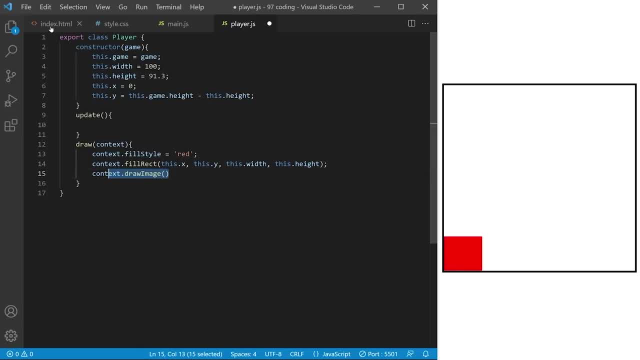 keep going and you can always watch a special episode later Describing each technique on a simpler project. So draw image is a special HTML canvas method we can use to draw and even to animate an image. It's simple. I have my player sprite sheet here in indexhtml and I gave it an ID of player. 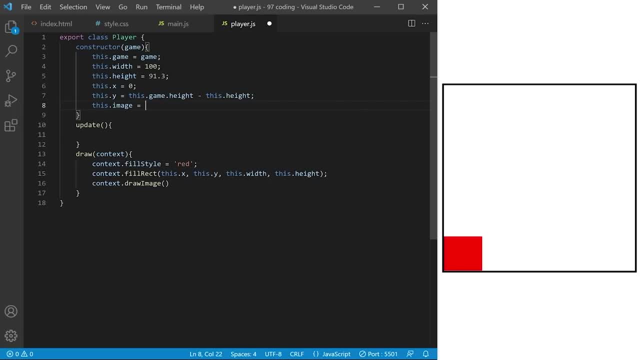 I create a property on player class called thisimage and I point it towards that image element using get element by ID. Now I can draw that image. Draw image method needs at least three arguments: Image we want to draw and X and Y where to draw it. 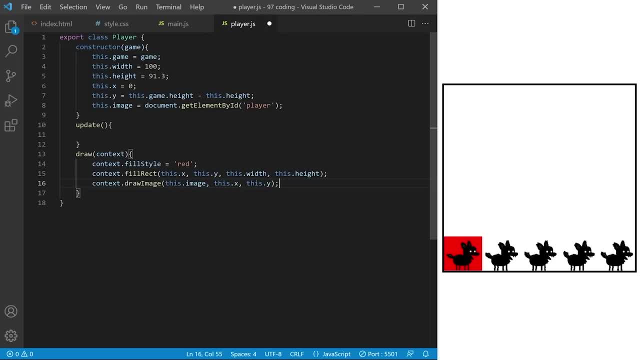 By the way, I'm not sure if you know, but I don't really have to use get element by ID. here I give my image ID of player here and JavaScript automatically creates references to all elements with IDs into the global namespace using its ID as a. 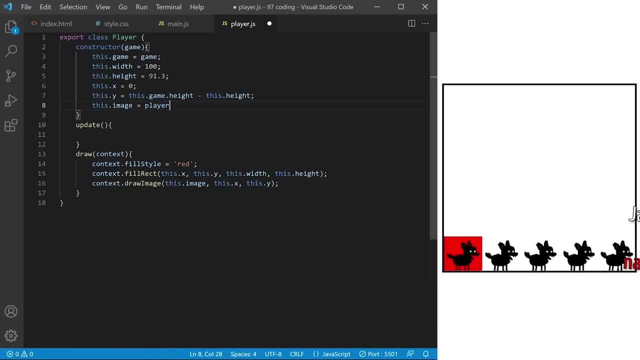 variable name, So I can simply just use that ID as a variable name here, and it will still work. It's a bit strange and for some reason nobody uses this feature, but it will work. I will go back to get element by ID here, even though it's kind. 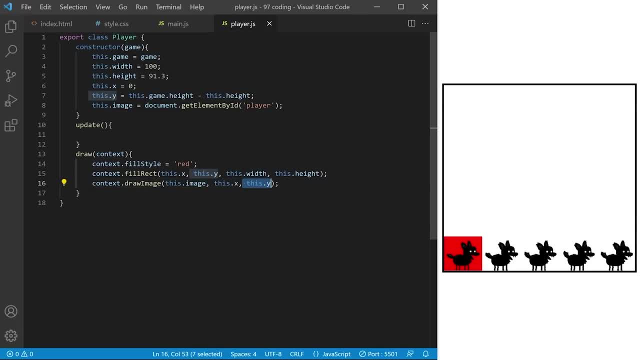 of redundant, I'm going to go back to get element by ID here, even though it's kind of redundant. Draw image method can also accept optional fourth and fifth argument for width and height and it will shrink or stretch the image to occupy these dimensions. Now it's just squeezing the entire. 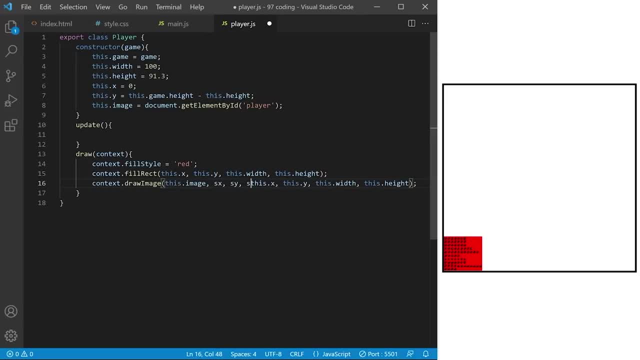 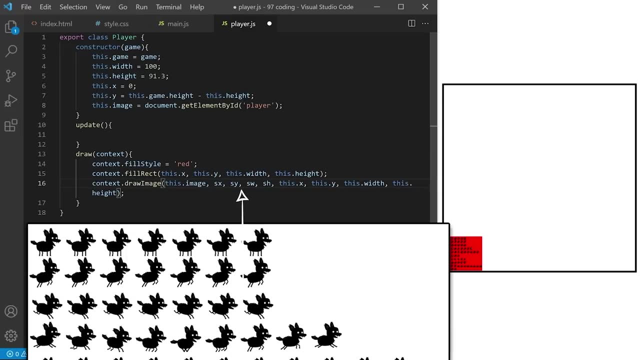 sprite sheet into the small space. The longest version of draw image method takes nine arguments and that's the version we need. We pass it image. we want to draw source X, source Y, source width and source height of the rectangle we want to crop out from the source image. 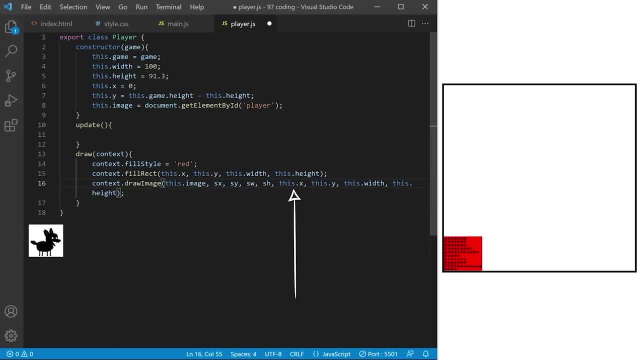 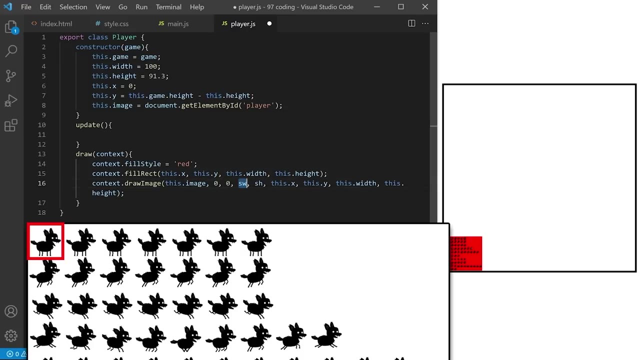 in our case a single frame of the sprite sheet and destination X, destination Y, Destination width and destination height will define where on destination canvas we want to draw that cropped out rectangle onto. At first I just want to crop out the top left frame in my sprite sheet, so I crop from coordinates 0, 0 and the area will have a width of 100 pixels. 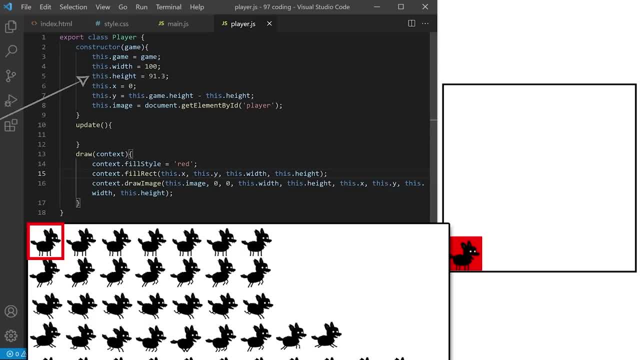 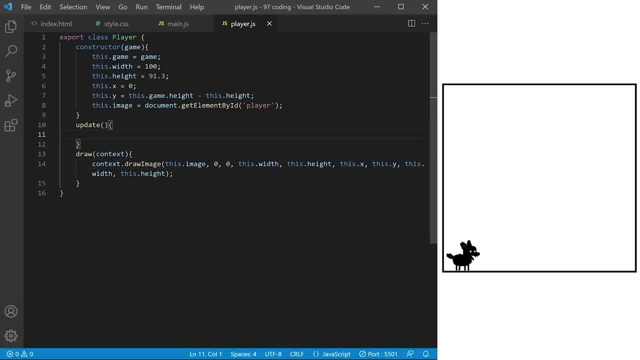 and height of 91.3 pixels. I'm cropping out exactly one frame. I don't need the red rectangle anymore. We are redrawing the same image over and over 60 times per second, but it looks static. Let's check if we are actually animating by putting some code inside player. update method For every. 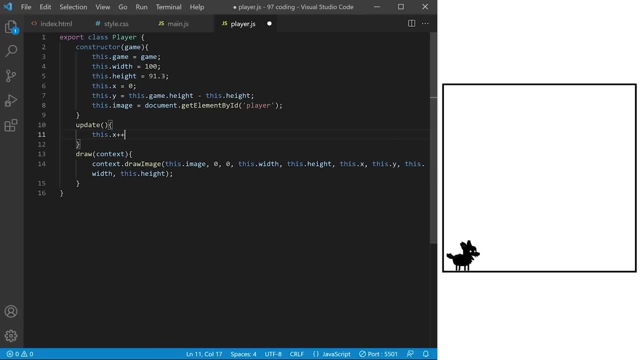 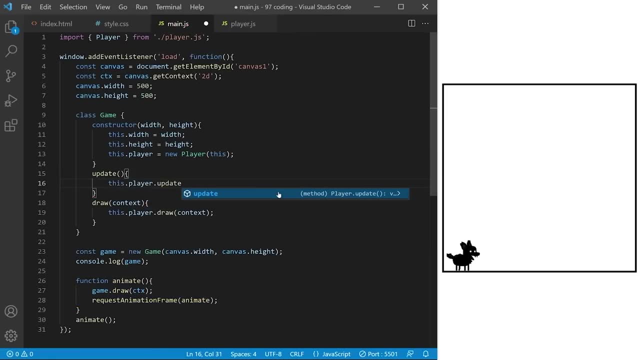 animation frame. I want to increase player's horizontal x coordinate by 1 pixel. To actually run the code, I need to go to update method on game class and I take thisplayer from line 13 and I call update on it like this. Finally, I call gameupdate from inside animation loop and we have 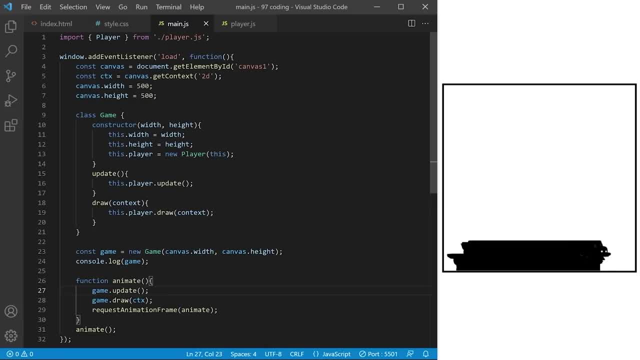 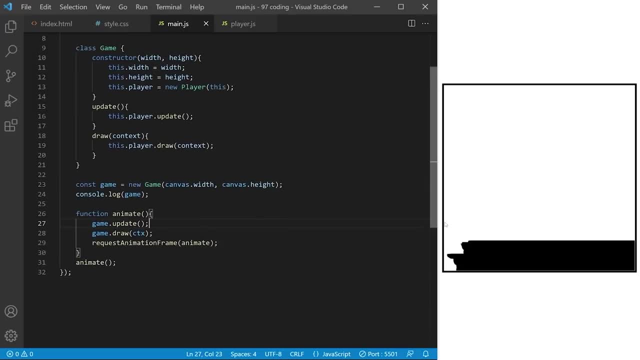 some motion. Congratulations: you are a javascript animation master. Okay, we can do a bit more with this if you want. The dog is leaving a block of the map black trail behind. That's old paint. we can just see all the previous frames. 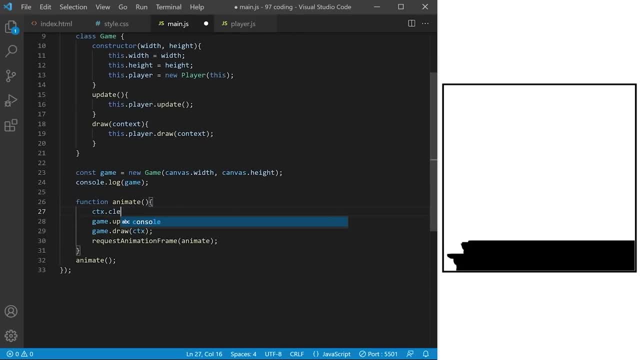 If you want to see only the current animation frame. we need to clear canvas each time we update and draw. I call built in clear rectangle method and I want to clear the entire canvas from coordinate 0, 0 to canvas width, canvas height. Now we can just see the current animation. 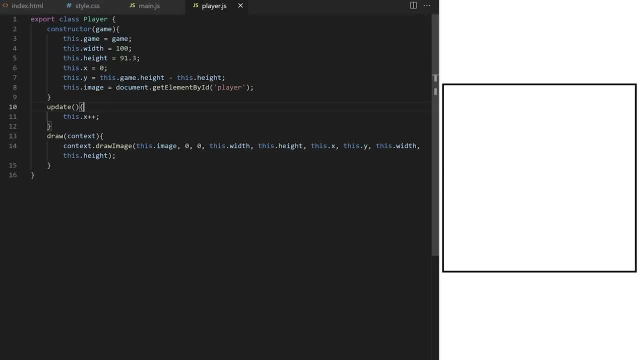 frame. I don't really want the player to move like this. Let's comment this out. I want the player to move left and right, jump and to use superpowers based on keyboard inputs. I create a new javascript file, a new module. I call it inputjs. Its job will be to capture. 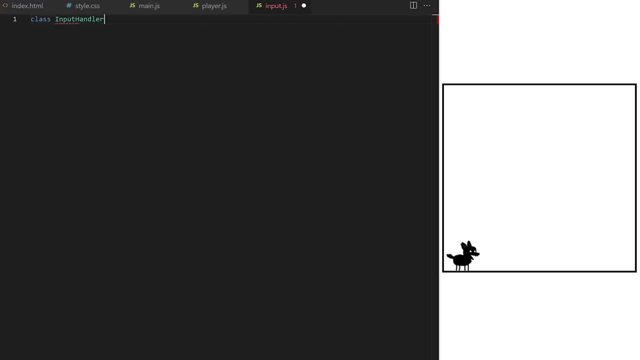 and keep track of user input. Again, I will create a javascript class here. I will call it, for example, input handler. Inside its constructor, I create a property called thiskeys and I set it to an empty array. at first, I will be adding keys that are pressed down into. 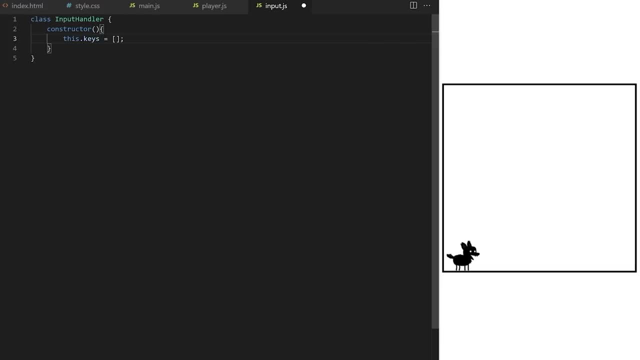 this array and removing the keys. That way, we can always check if a specific key is pressed by checking if it's included in this array. As we said before, the code inside a class constructor is executed automatically whenever we create an instance of this class. so I will take advantage of that and I will 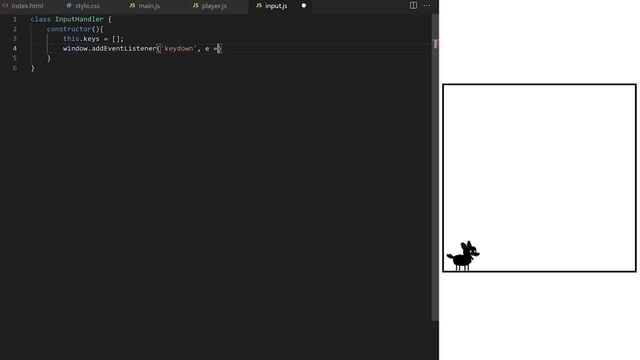 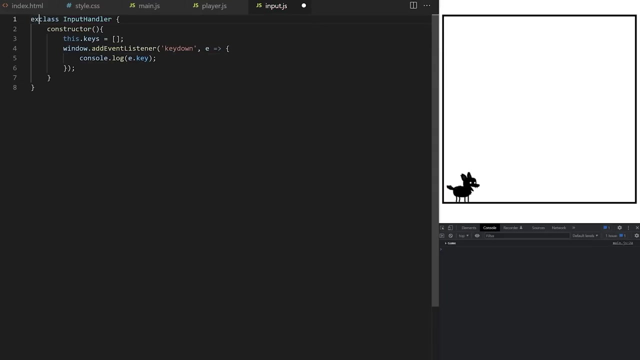 apply key down event listener. from here, Event listeners return an auto-generated event object which contains all kinds of information about the event that just occurred. The property that holds the name of the key that was pressed is called key, So let's consolelog ekey. 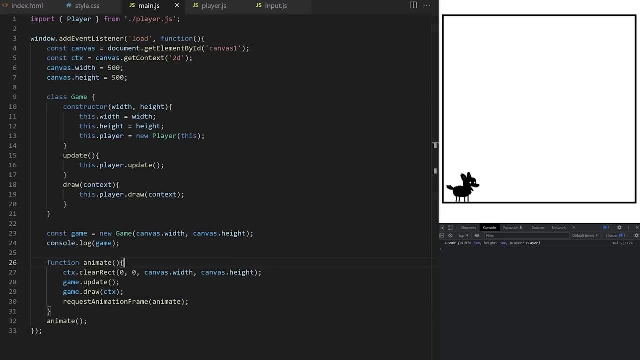 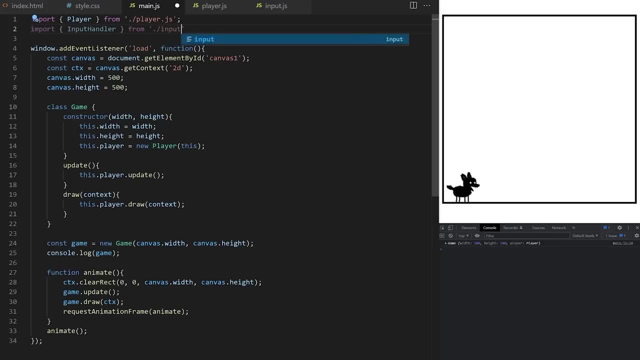 I export input handler up here Inside mainjs. I import my new input handler class same as I did with player. I will create an instance of input handler class inside game class constructor. I will call this property thisinput. This way, input handler class gets automatically. 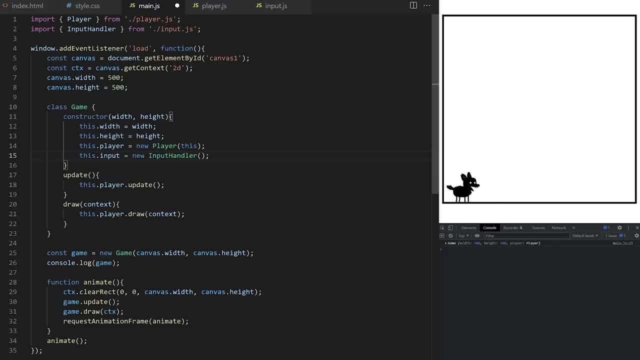 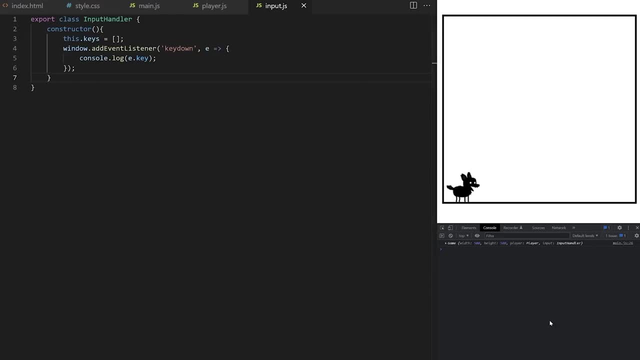 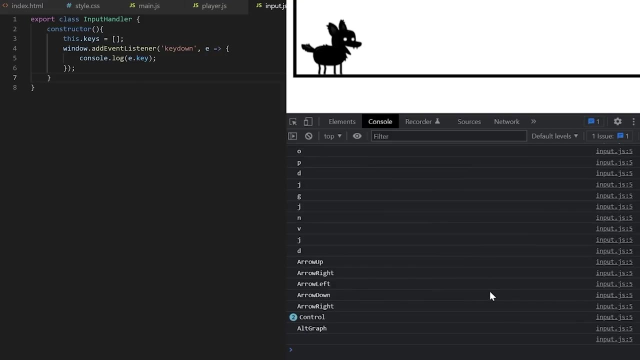 instantiated. when I create an instance of game class, I will create thiskeys array from line 3 and it will also automatically apply this key down event listener. Now, when I press keys on my keyboard, I can see their values. I don't want to react to every key. We will ignore some and we will only respond to specific. 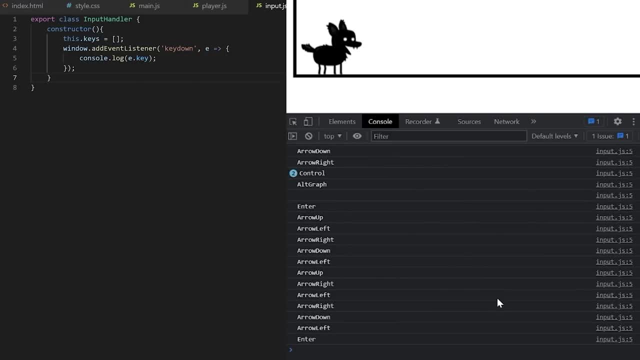 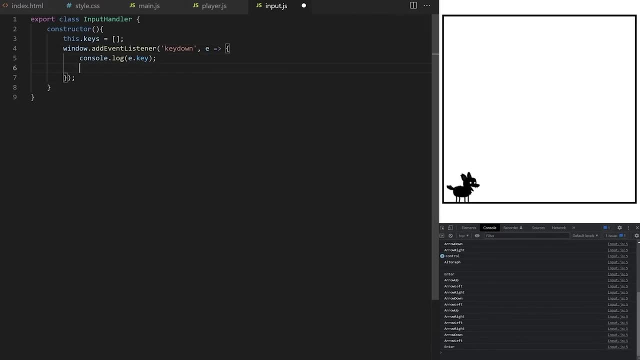 controls defined here. We will also make sure each key can be added to thiskeys array only once. so when the user holds down a specific key, it will not be added 20 times, it will just be added once. Let me show you. I say if ekey. 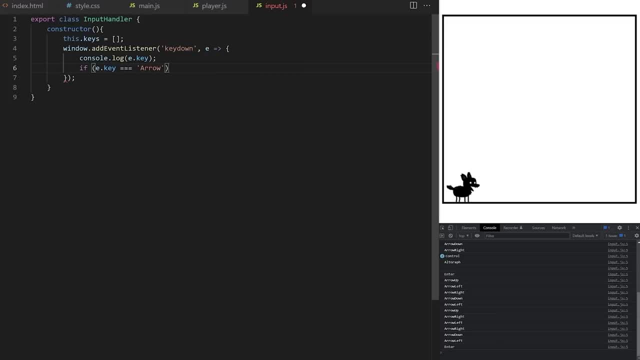 Meaning. the key that was just pressed has key value of arrow down and at the same time, this key that was pressed is not yet included in thiskeys array. so thiskeys index of ekey is equal to minus 1.. You can also say: is more than minus 1.. 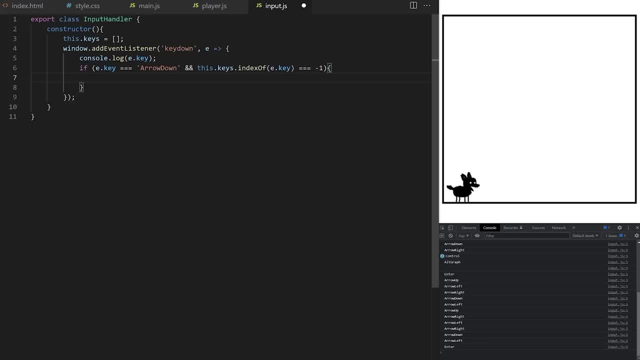 In javascript, when element has index minus 1, it means it's not present in the array. Then I just do thiskeys push ekey. so if the key that was pressed is arrow down and if arrow down is not yet inside thiskeys array, push arrow down into thiskeys array. 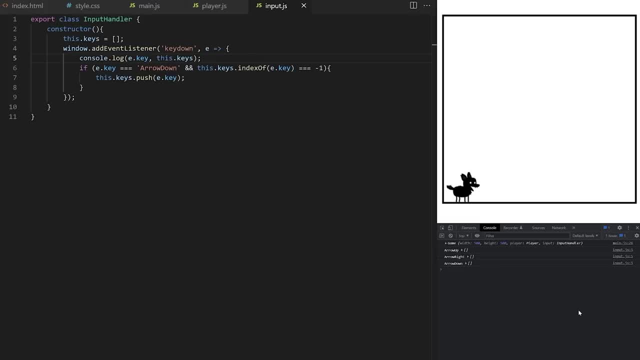 I can console lock key that was pressed and thiskeys array. You can see it will stay empty until I press arrow down. If I press it, it will be added to thiskeys array once. I will also create an event listener for key up event. 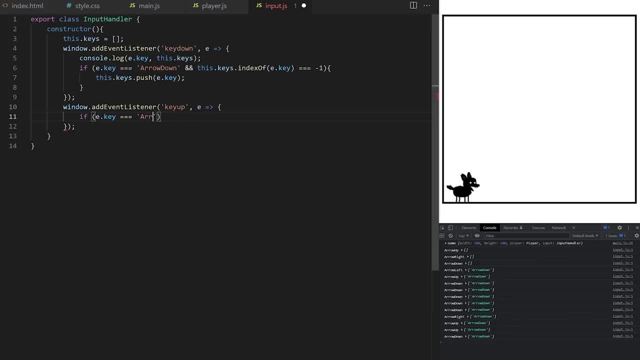 If ekey is arrow down, meaning if the key that was released is arrow down, I will use splice method to remove it from thiskeys array. Splice method takes at least two arguments: The index of the element we want to remove and how many elements to remove at that index. 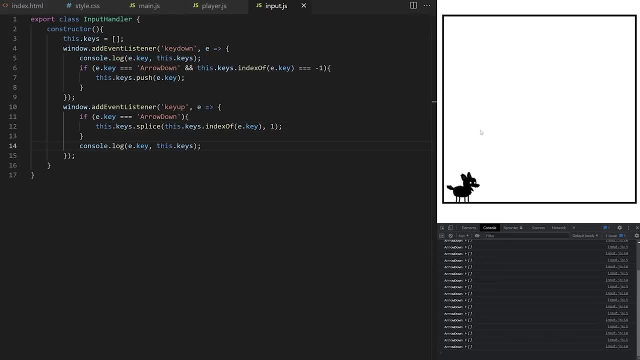 Let's test it. Actually, to test it properly, I want the console lock after the if statement. Now, when I press arrow down, it gets added to thiskeys array through the code inside key down event. When I release it, key up event removes it from the array. 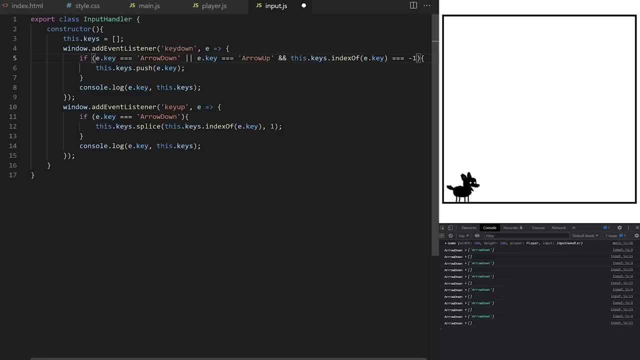 Perfect. I also want to listen for arrow up key, So I use OR operator: Be careful about brackets here. I have to wrap this block in brackets like this: If key that was pressed is arrow down or arrow up in brackets and at the same time, the key. 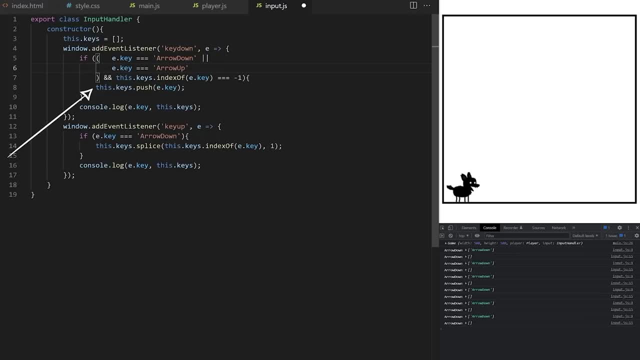 is not yet present in thiskeys array, only then push it inside. I also need to make sure I remove that arrow up key on key up event. Again, pay attention to how I use brackets here. It's easy to make a mistake here and break your code. 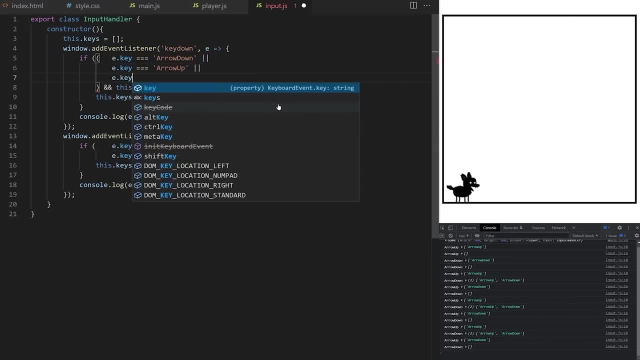 We will also listen for arrow left, So OR operator, Ekey is arrow left And another OR operator and I check for arrow right. I will check for one more key. for now I will use it for a special move and attack And you can use alt control, but be careful. 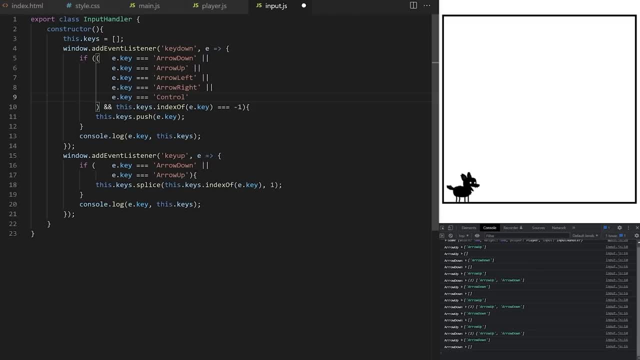 Mac and Windows call, alt and control keys differently. They might have a different value. Console, lock, Ekey and press them on your machine to check for that value. In this case, I will use enter key, which should be more universal and compatible with both Mac and Windows systems. 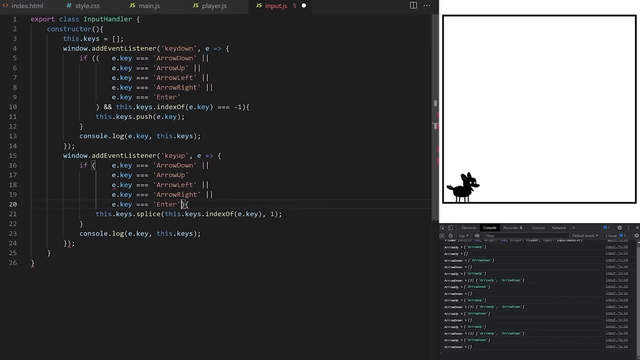 Let's add all these keys to key up event as well, And I have to make sure my syntax is correct. Now it should work. I click my canvas to select it and when I start pressing arrows and enter, I can see they are correctly being added and removed from the array. 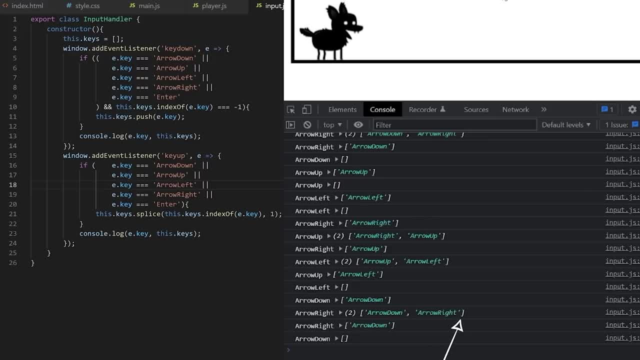 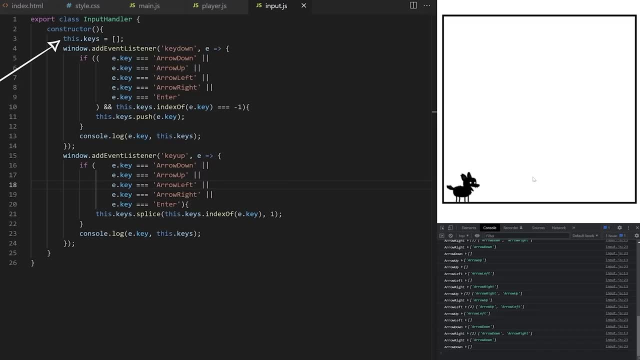 You can see we are also keeping track of multiple key presses at the same time. Great. So now thiskeys property on input handler class always contains all currently active keys. I have an instance of that class here Saved as a key As thisinput. 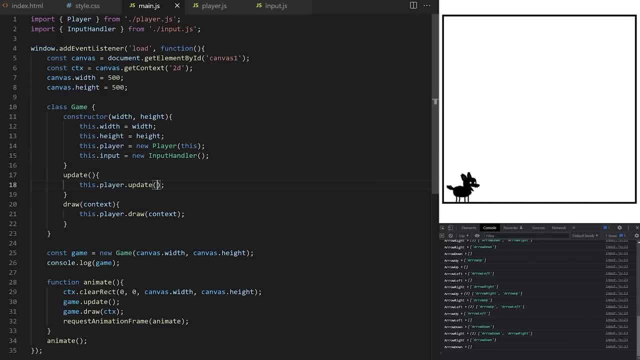 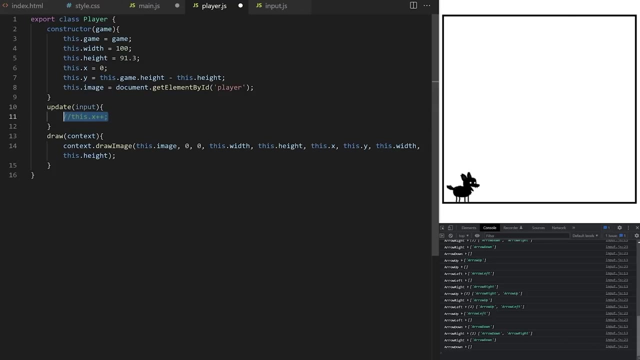 For every animation frame. I want to pass the current list of active inputs to player update method as an argument so that it can react to it. I will pass it thisinputkeys Inside playerjs. I make sure the player expects that input value. I will call it, for example, input. 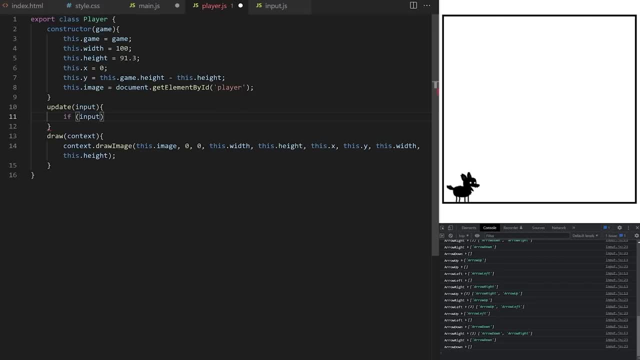 It still refers to thiskeys array. we have on our input handler class. Inside update method on player class. I want to check if it includes specific values. I use built in array includes method. I could also use index of method here. it would work the same. 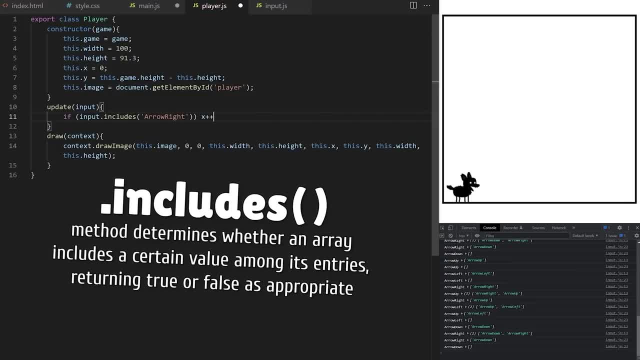 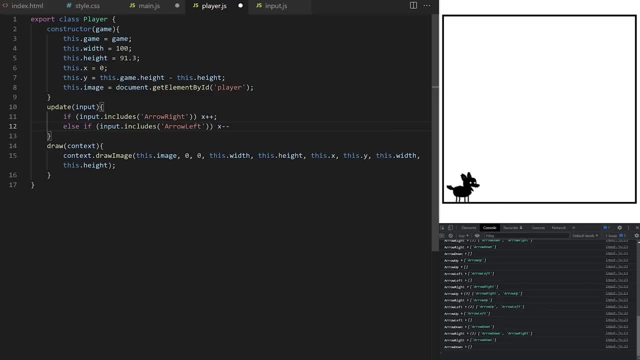 If input includes arrow right, increase horizontal x coordinate of the player by 1.. Else, if it includes arrow left, decrease x by 1., Making the player move left on the negative direction on horizontal x axis. I actually need to say thisx to correctly refer to the property from line 6.. 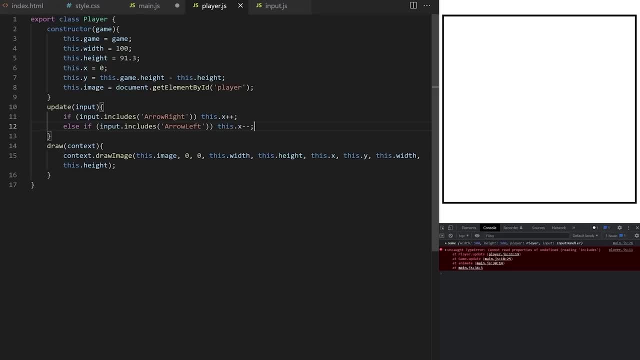 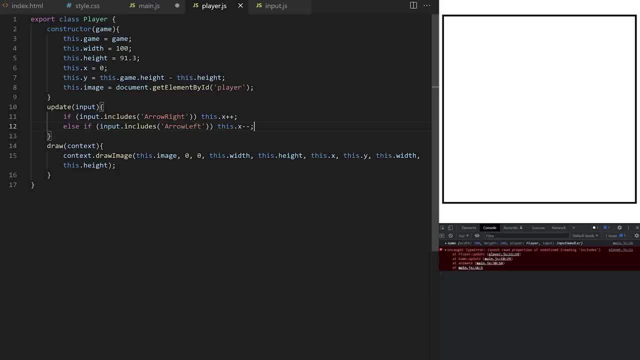 I can't save my changes to inputjs or mainjs files. I can't save my changes to inputjs or mainjs files With file structure like this. when we're using modules, we always have to make sure we save every file whenever we make any changes to it. 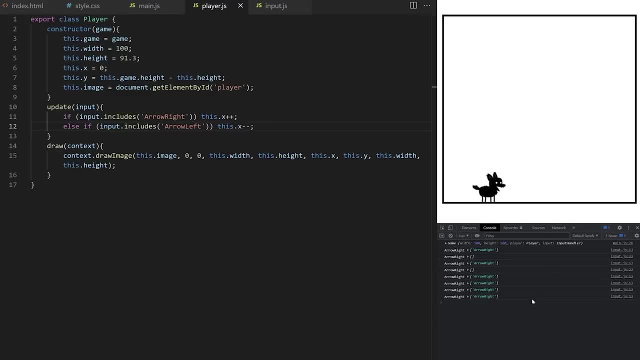 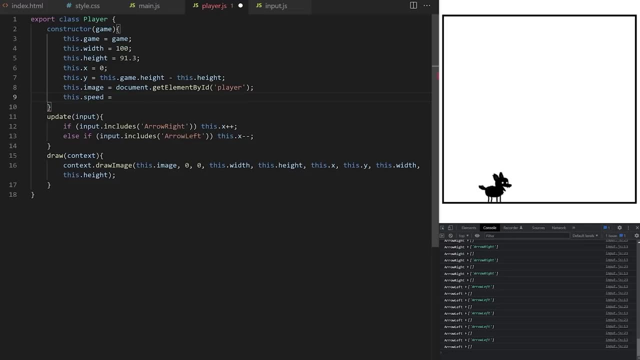 Now, when I press right arrow, player moves right. When I press the left arrow key, the player moves left. Let's refactor this. I give player a speed property and initially I set it to zero. I also give it max speed property, which will be its speed in pixels per frame when it's 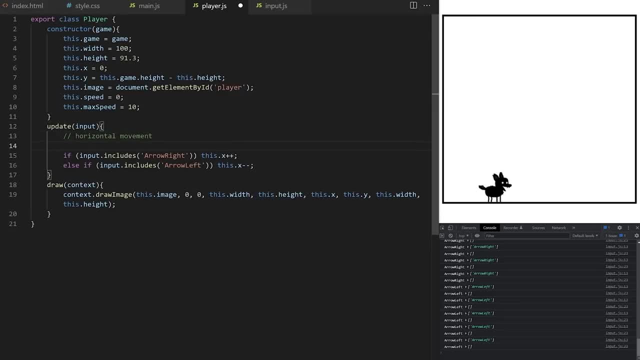 moving. So this section of code will handle horizontal movement for every frame. I will also give it max speed property, which will be its speed in pixels per frame when it's moving. I will also give it max speed property, which will be its speed in pixels per frame when. 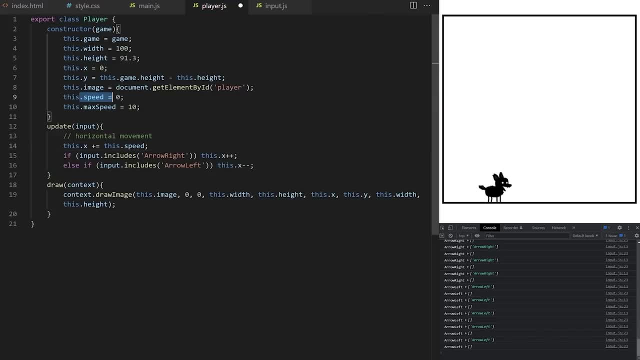 it's moving. I will also give it max speed property which will be its speed in pixels per frame when it's moving. I will increase players horizontal x position by its current speed. So right now the speed is zero, so the player is not moving. 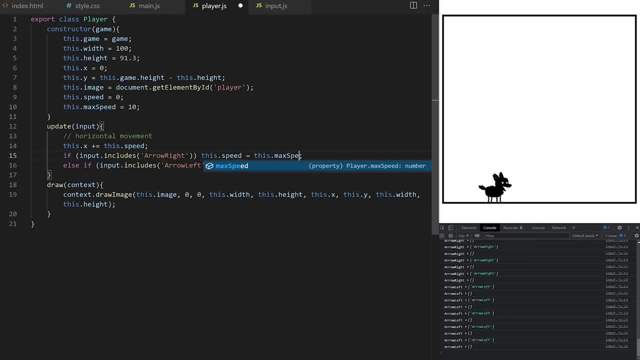 Down here. I say: if input includes arrow right, set thisspeed to max speed. If it's arrow left, set speed to minus max speed. Now I can move left and right again, but I can't really stop. There is no condition when the speed returns back to zero. 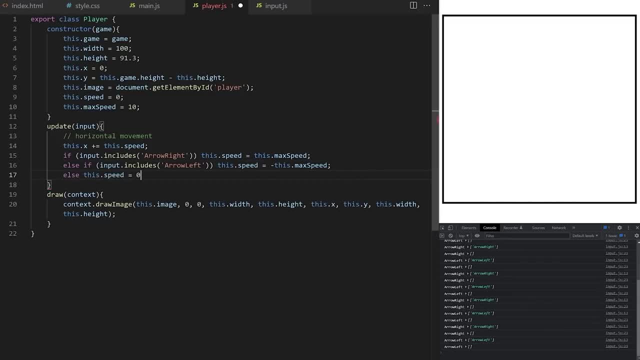 I can fix it by saying: else, thisspeed is zero Meaning. if input array doesn't include arrow right Or arrow left, stop the horizontal movement. I also don't want the player to be able to move outside of the game area, so I need to. 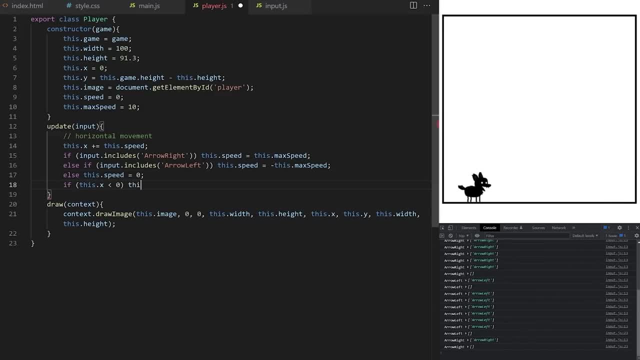 introduce some boundaries. I say: if thisx is less than zero, set thisx to zero. Now I can't move past the left edge. I also say: if thisx is more than thisgame width minus the width of the player, set x to game width minus player width. 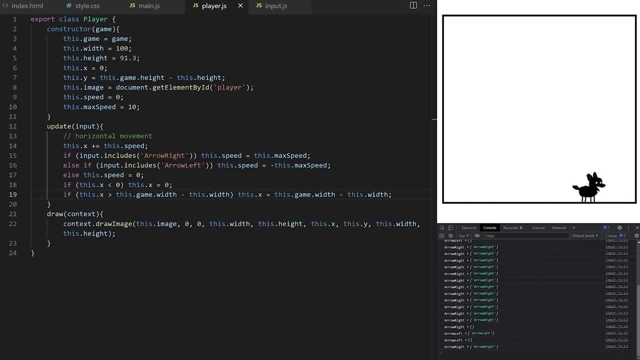 Now I can't move past the right edge of game area as well. Perfect. It's time to handle vertical movement, which will include jump in and also a special dive move where we crush enemies from above. I create a new class property called thisvy velocityY, basically a vertical speed. 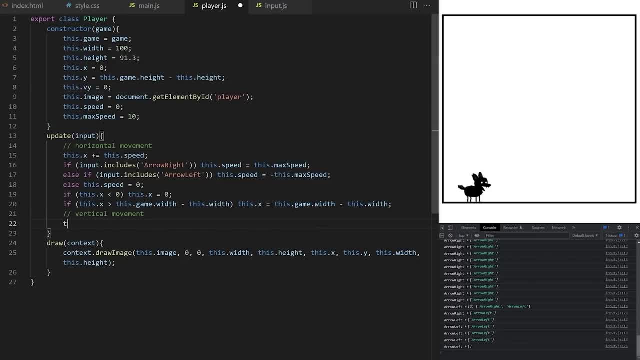 Initially I set it to zero. For every animation frame we will add the current vertical velocity vy to player's vertical y position. Currently vy is set to zero, so there will be no vertical movement at first. I will have to check in multiple places in my code. 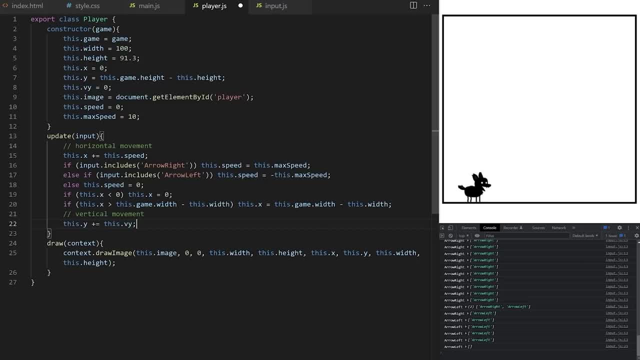 Whether the player is standing on solid ground or if it's currently in the air. To make our code more readable and to avoid code repetition, I will put that check into small utility method. I will call it, for example, onGround, and I just want it to return true if the player 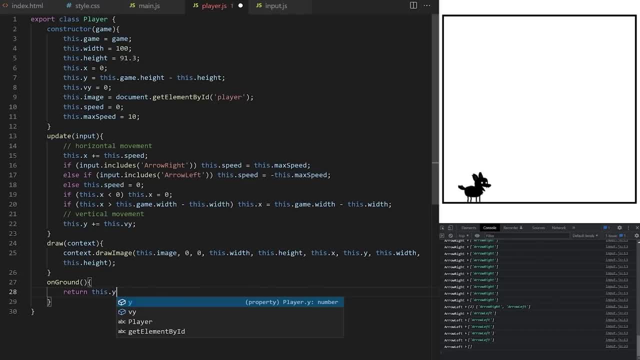 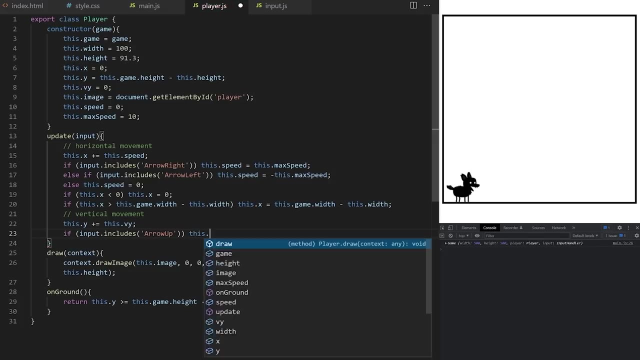 is on ground, or false if the player is in the air. I do that simply by saying: return thisy is more or equal to height of the game minus the height of the player. Let's start by saying: if input includes arrow up, Set thisvelocityY from line 8 to minus 20.. 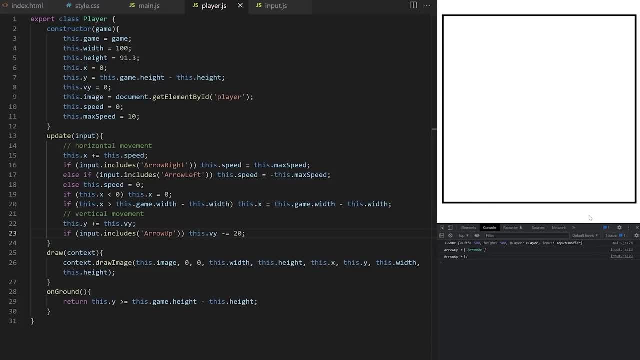 I press up arrow key and the player just flies up off screen. Ok, that worked. I only want the player to be able to jump while it's standing on ground. I don't want it to jump higher and higher in the air when we are pressing up arrow repeatedly. 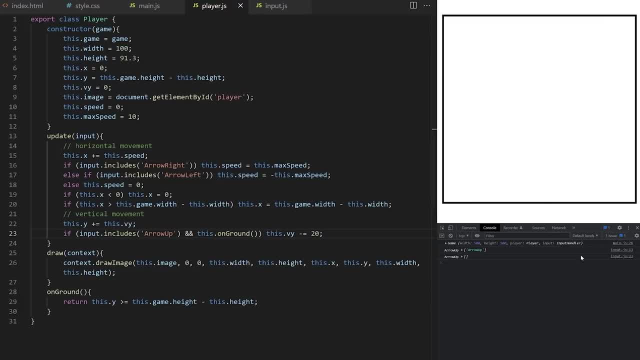 I add one more check here to see if onGround from line 28 is true. I set velocityY to minus 2.. Nice, If you want a nice jumping curve in a 2D game, then you can do that by pressing up arrow. 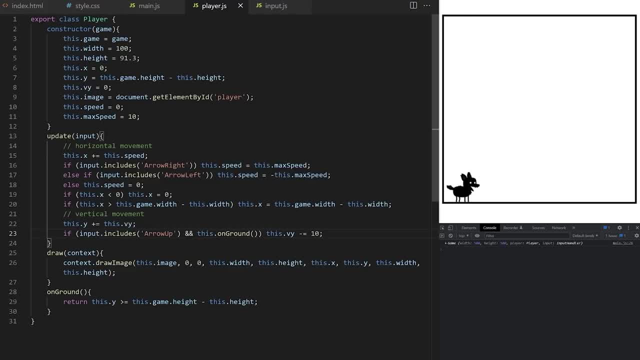 key In a 2D game. we usually do it by making the power of the jump- in our case vy, property work against the gravity or weight of the object, And while that object is in the air we keep increasing its weight until it eventually. 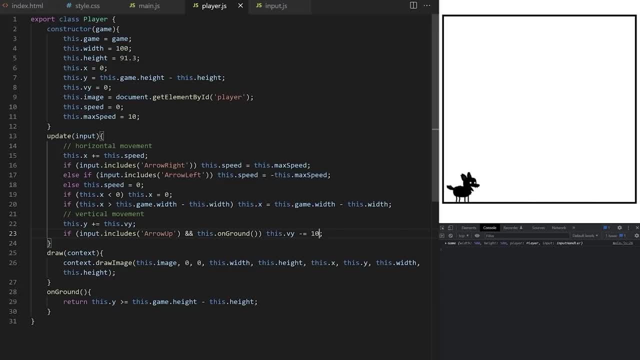 is higher than its jump power, and it will make it slow down and start falling down. Let me show you exactly what I mean. This used to be a bit confusing for me, but it becomes easy when you use it a few times. I create a new property called thisweight, for example, and I set it to 1.. 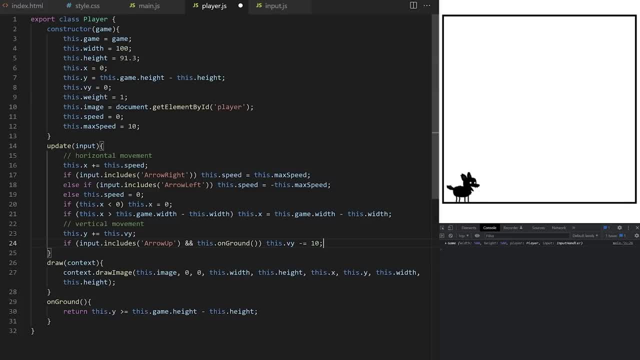 So we have velocityY property And when we press up arrow key, we set it to minus 10.. This will be the power pulling the player upwards. At the same time, I want the weight of the player from line 9 to be pulling it down, and 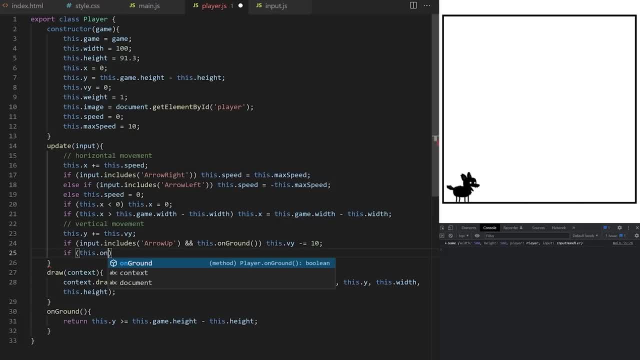 I want that pull to be stronger the longer the player is in the air, to get that smooth curve when we jump. I do that by saying: whenever thisonground is false, whenever the player is not standing on the ground, increase its velocityY by thisweight. 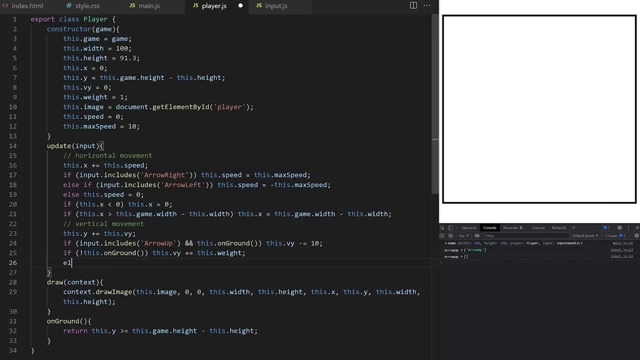 Nice, We kinda jumped, Haha. I also need to make sure that when the player lands back on the ground, velocityY is reset back to 0 to stop all vertical movement. I say else: thisvelocityY is 0.. For this to actually work as intended, I need to first run this line of code and then this: 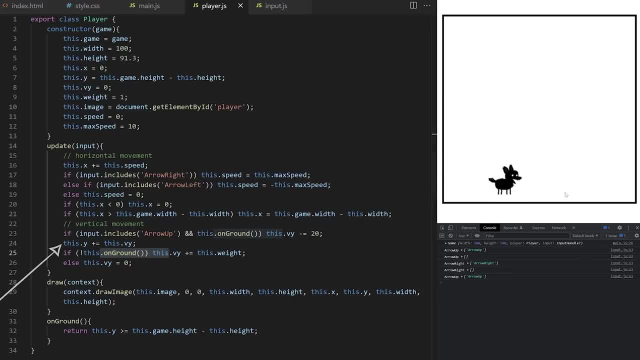 one And we are jumping. VelocityY is constantly being added to player's verticalY position. At first it's 0, so nothing is happening. When I press up arrow key, I give it a push in the negative direction on the verticalY axis, so upwards. 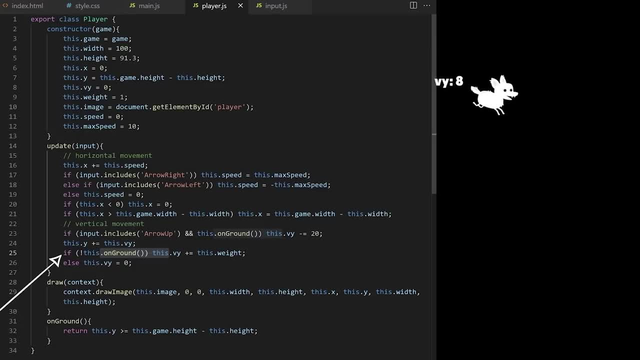 At that point the player is currently not on the ground, so this line of code will start running and velocityY, which is currently set to minus 20 and which is moving the player 20 pixels up per animation frame, will start decreasing by thisweight from line 9, so minus. 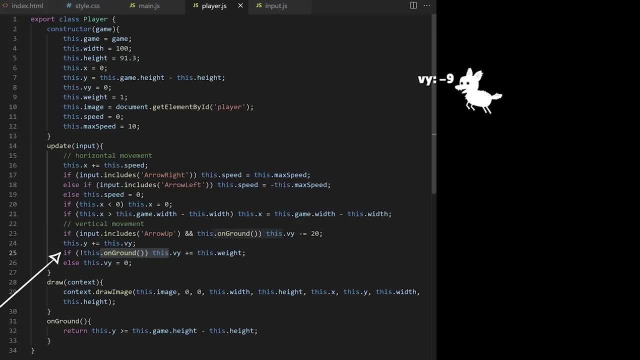 20 plus 1 is minus 19,, minus 18, minus 17, all the way to 0.. When we reach velocityY of 0, player is at the peak of it's jump, But it's still not on the ground. so this line is still adding weight to velocityY making. 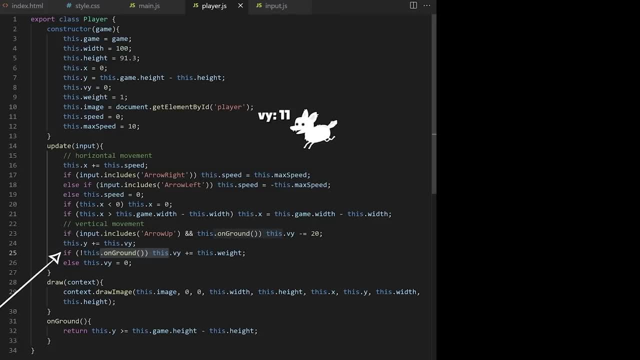 the player fall down faster and faster When the player hits the ground. this else statement will set velocityY back to 0 and the jump is finished. The ratio between weight and this minus value will determine the curve height and speed of the jump. 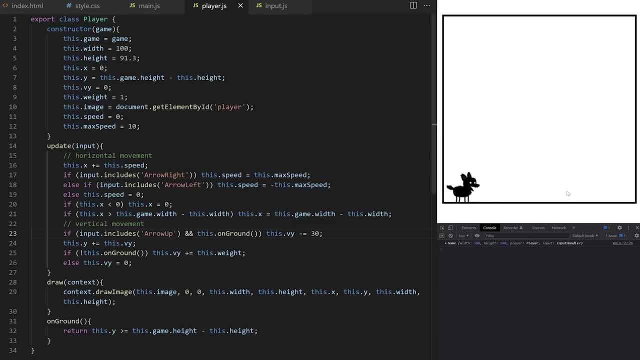 I will keep weight at 1. And I will adjust velocityY to make the player jump. I will set the velocityY to 0.. jump all the way to the top of the game area. We have running and jumping. I would like to add more player states and properly animate them. We need a fireball. 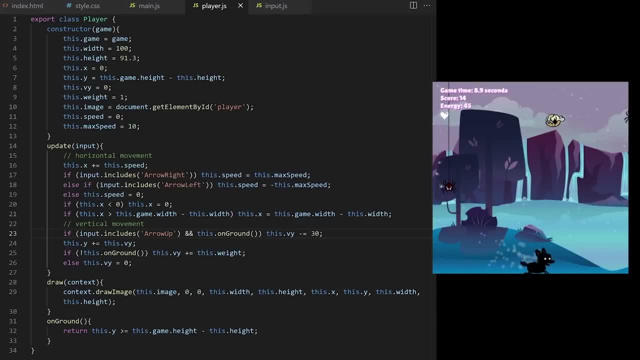 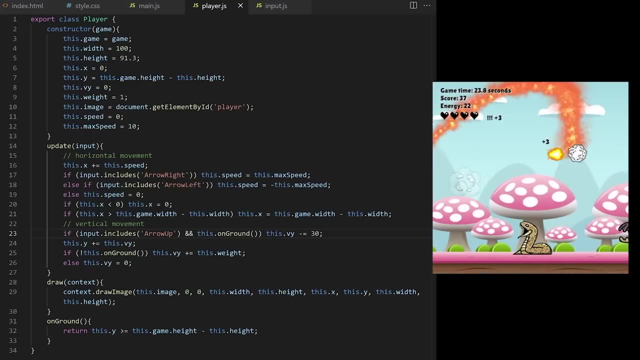 attack, and when the player sits down, I want the game to stop scrolling. How do we organize and manage this functionality? By structuring our JavaScript code in so-called state design pattern. I will show you exactly how to do that in the next part. We are building a fast-paced animated side. 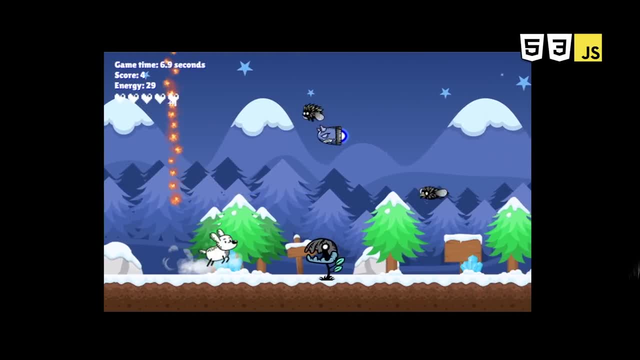 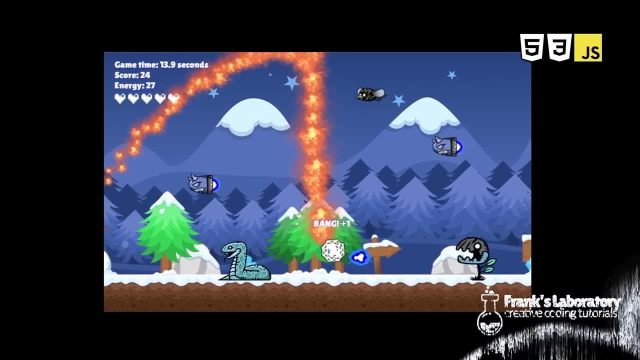 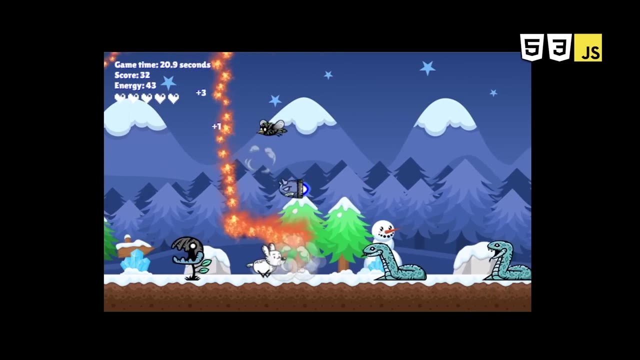 scroll game with vanilla, JavaScript and HTML canvas. In the first episode we created the main game, logic, animation loop and the player. Let's continue building our game. In this class we will apply state design pattern to our player to make it switch between the states properly. We will learn how to control. 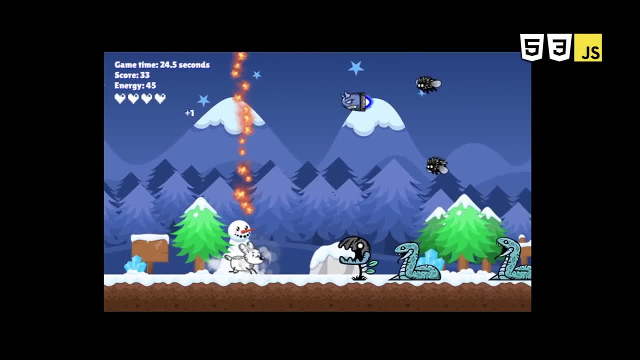 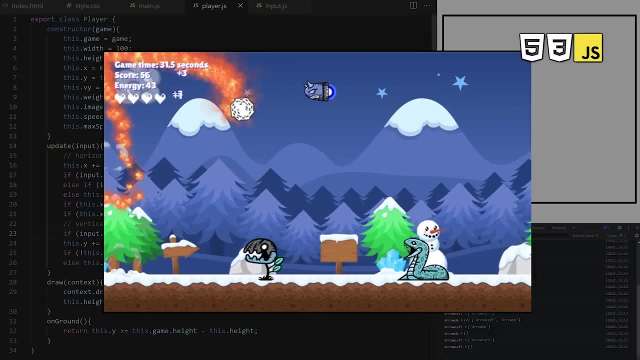 FPS, how to animate sprite sheets and how to implement multi-layered seamless backgrounds with scrolling speed that reacts to player movement. Part one is linked in the video description. Let's go. I like writing my code like this for small, simple games. As you can see, there are quite a lot of, if else. 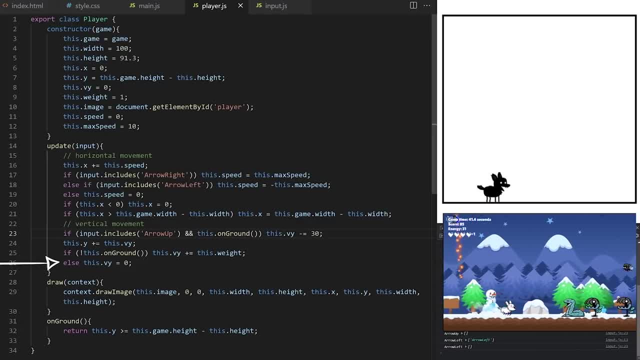 statements in here already. I want to add some special moves. This single code block already does so many things and we have just run in and jump in. If we keep adding more and more in here, we can get to the stage where changing one line of code can break something else unexpectedly. 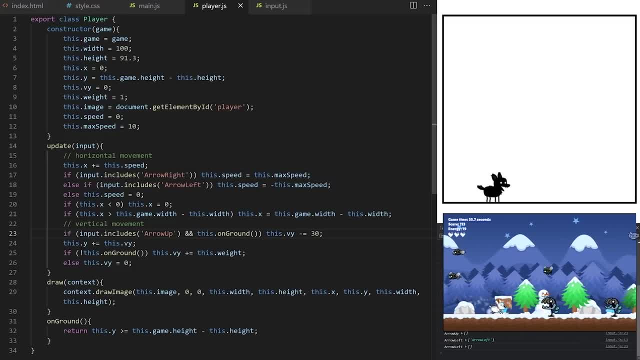 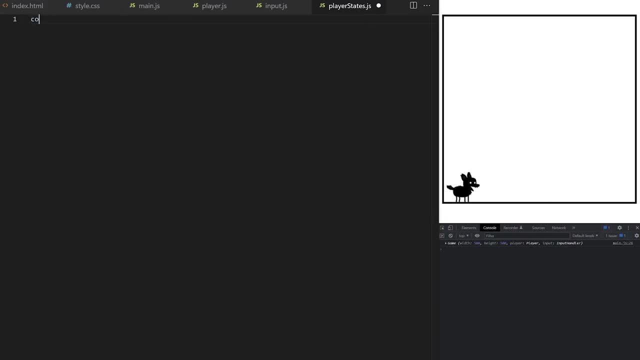 For small games it's fine to have all logic in one place like this. but for this game we will go ahead and structure our code a little bit better. I will manage player states separately in its own file. I call it player statesjs. At first I will create a simple enum object that will pair values. 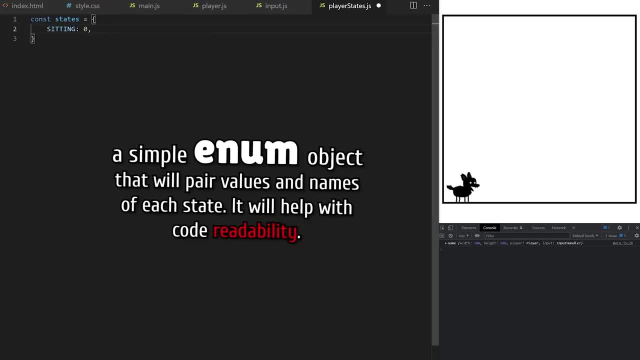 and names of each state. It will help with code readability. Rather than swapping to state 2, I will swap to statejumping, which has a value of 2 behind it. It will be easier to see what our code is doing. This episode might be a bit challenging for beginners. We will be passing. 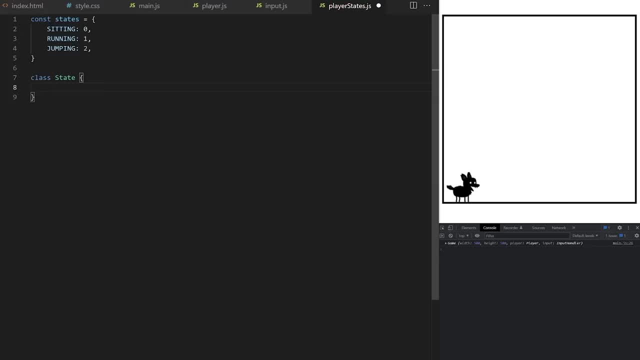 values around between javascript modules and classes, and I can imagine if you are a beginner, it might take some effort to do this. If you are a beginner, you might want to do this as well. I will guide you through all the steps and we will make our code easy to navigate in. 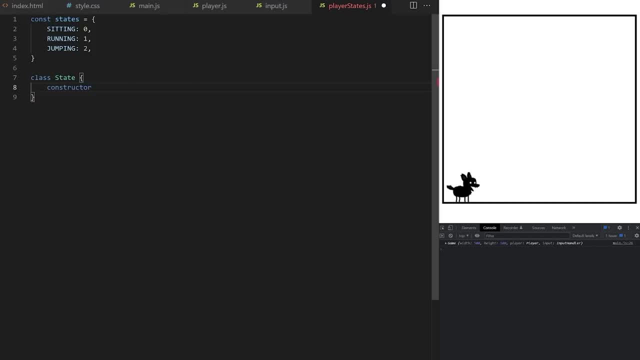 but this is the finale of my vanilla javascript 2d game development series, so I expect you either already watched my beginner friendly episode on state management linked in the description, or that you have already done some javascript coding before I will explain everything today. No previous knowledge is needed, but it will be easier if you watch the beginner class first. 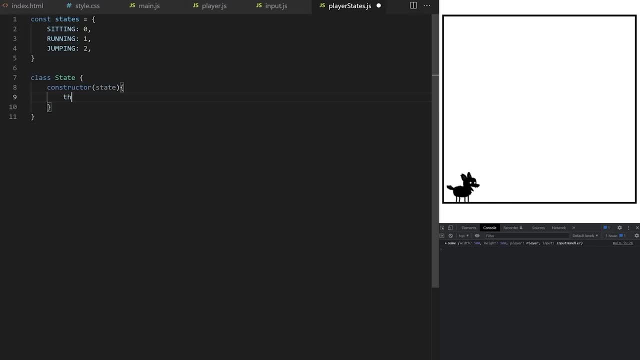 It's up to you. Today's tutorial is mainly to show you how I put everything together to make a polished animated game that feels good to play. Check the video description for the full series. I create a class. I call for example state. Each state will have its own class so that I can. 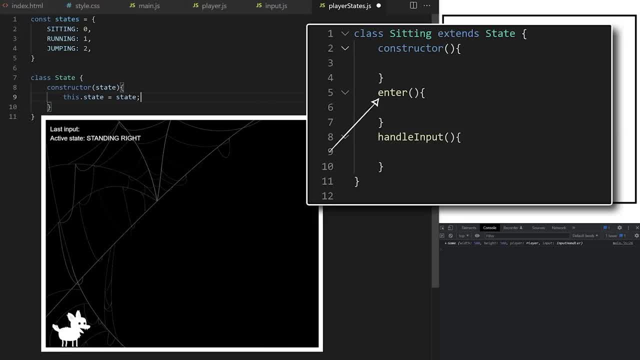 give each state a different enter method to set the player up when it enters that particular state and handle method that will react to different user inputs depending on which state the player is in at that moment in time. For example, when the player is in the running state and I press arrow. 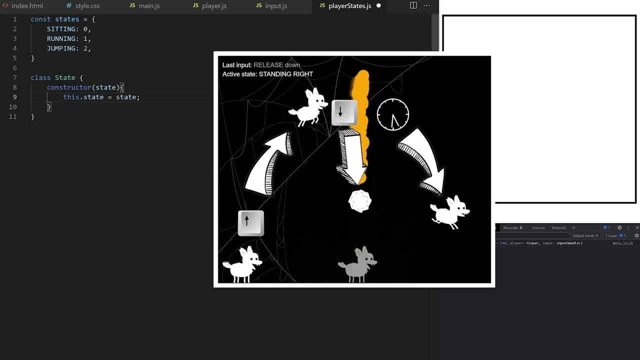 down. I don't want the player to sit in the air, I want it to do a crushing dive attack from above. State design pattern is perfect for changing how the object behaves depending on its current state. I will show you exactly what I mean as we write the code. Constructor will take a single argument. 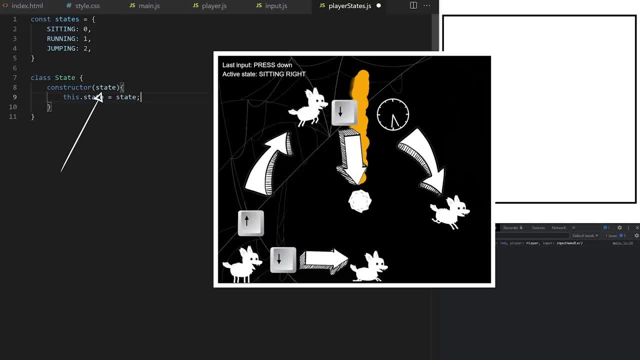 called for example state. It will be a simple line of text with the name of the state, such as sitting, running, jumping and so on. Inside, I convert the state to a sitting state. I will change the name of the state to a sitting state. I will also change the name of the state to a sitting. 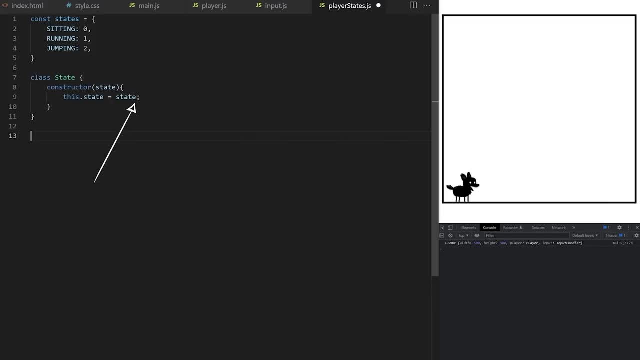 state. I will convert that argument to a class property. I will use this value only so that I can consolelog the name of the currently active state for debugging purposes. It's not important for the logic of state swapping. We will have one class for each state. The first state will. 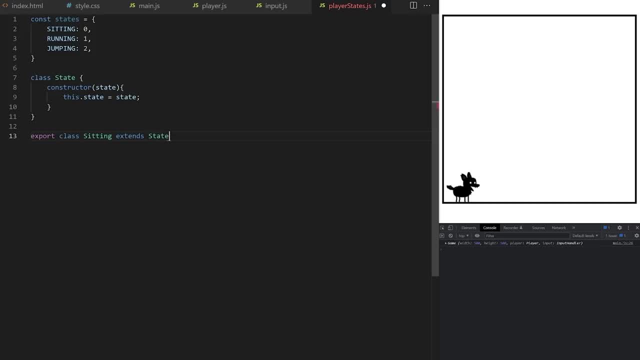 be sitting, which will also be special because it will stop the game from scrolling as the player sits down. We will export it. so export class sitting Constructor will take a reference to the player object as an argument so that it can access properties on the player class. 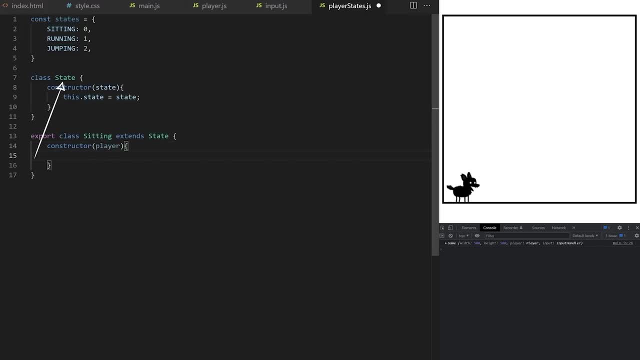 I am extending a class and I want the code from this constructor on the parent to run as well. so I have to call super keyword here to trigger constructor of its parent class, also known as a super class. We can see that the parent class constructor expects a value for state. This is: 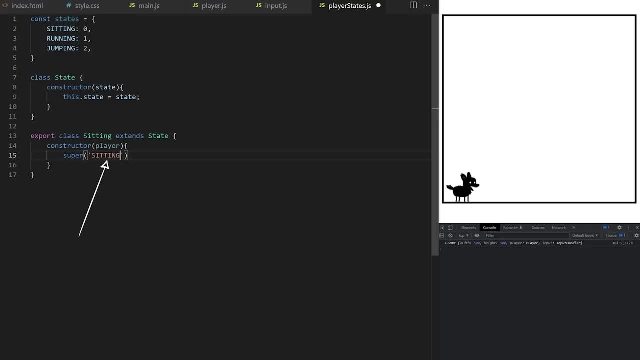 simply for monitoring purposes, I will pass it word sitting and it will get converted to thisstate property here Only after we called super. we can use this keyword here In a child class if we use this keyword before the parent class. we can use this keyword here In a child class if we use this. 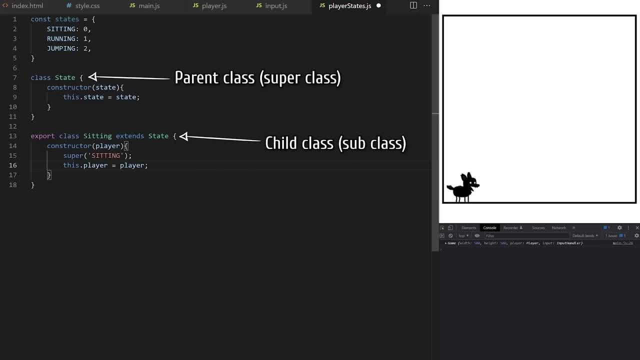 keyword before using super, we will get an error. Super on child class always needs to be called before this keyword is used. Each class will have enter method that will run once when this state is entered and handle input method. that will take input as an argument and it will keep checking if. 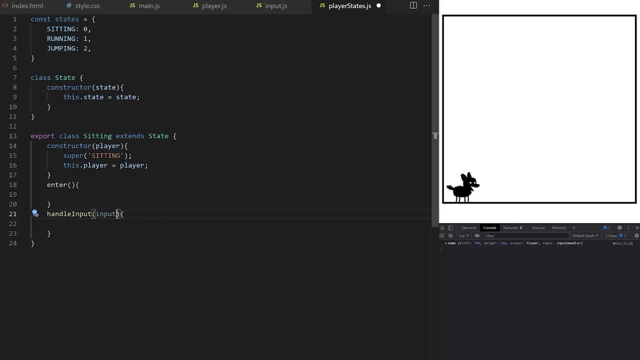 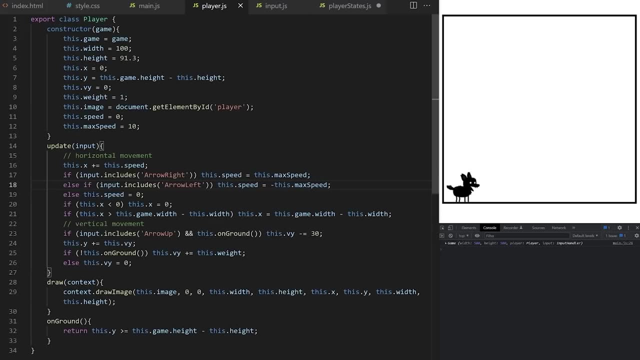 the correct key is pressed and it will switch player to a different state. when that happens, For example, it will switch to jump in state when we press up arrow key In player js. we will need properties to apply state design pattern. Let's just write them and I will explain in a minute. 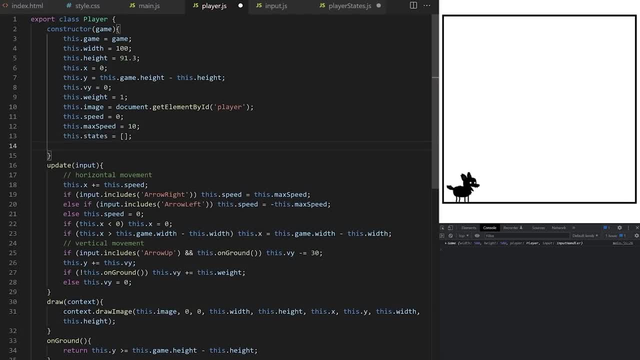 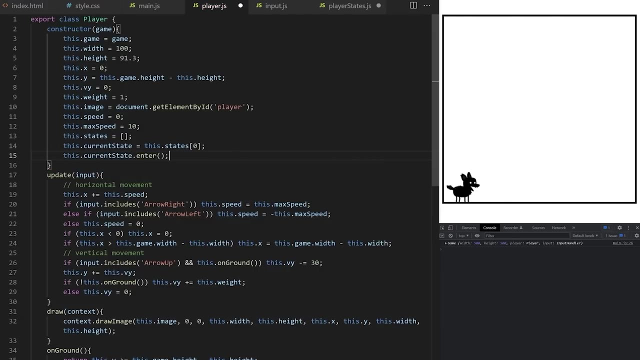 We will need a property called thisstates, which is an array of values. We will also need thiscurrent state, which will point to indexes in this array. When the player object is initialized for the first time, we will call its enter method to activate its initial default state. 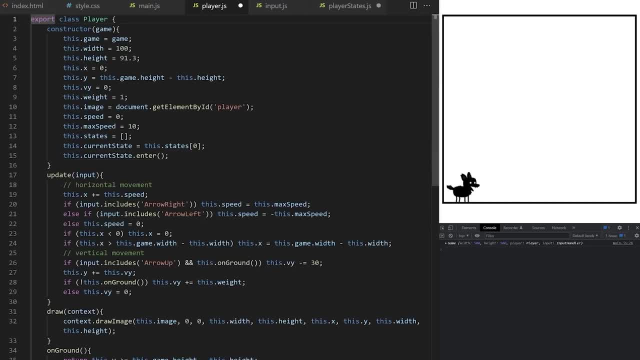 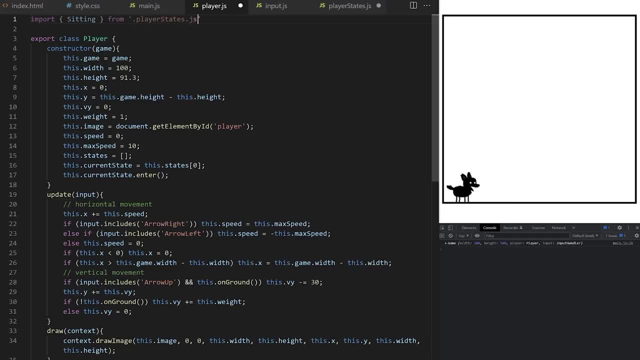 I'm exporting my sitting class here. Let's import it up here in player js. I import the entire sitting class from player states js. Quick overview of how we will apply state design pattern into our code base today. Player object will have thisstates property, which will be an array containing 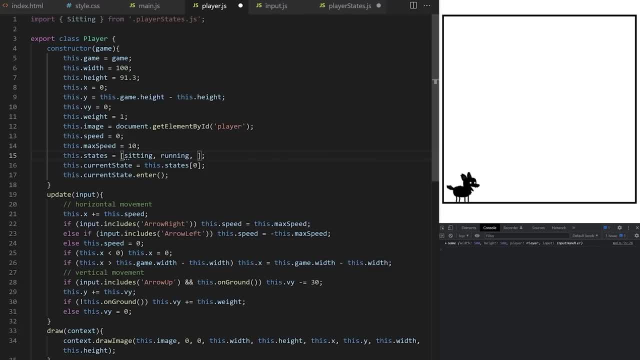 individual states, such as sitting, running and so on. The player can only be in one state at the time, so we will have another property here called thiscurrent state. When thiscurrent state is equal to thisstates index, zero player is sitting. When it's thisstates index one, the player is in the running state, and so on. 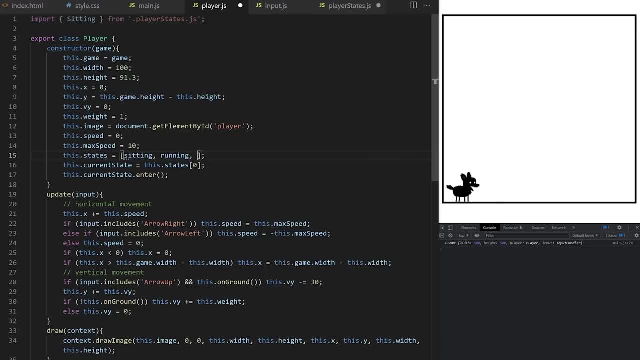 The final piece of logic will be that each player state is actually its own class. We will have a class for sitting, another class for running. there will be a separate class for every state. The reason for that is that each state needs to have its own separate enter method. 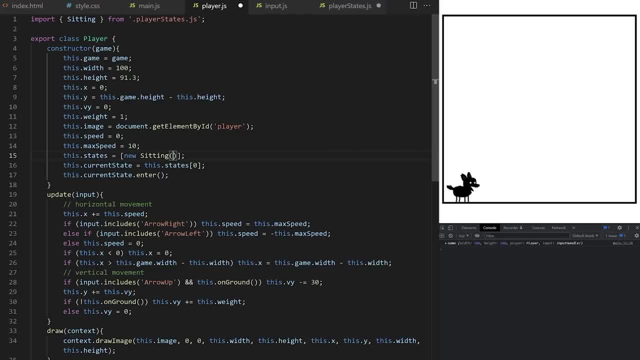 that will set speed, animation row and everything else that needs to be done whenever the player enters a new state. Each state class will also have a handle update method which will listen for keyboard inputs, and also have a handle update method which will listen for keyboard inputs. 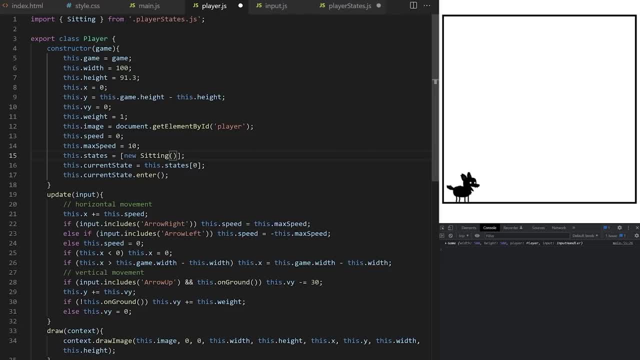 And it will be ready to switch the player to a different state whenever the correct key is pressed, Because all state classes have their own enter and handle input method and because thiscurrent state points to different states as the player switches from one state to another. 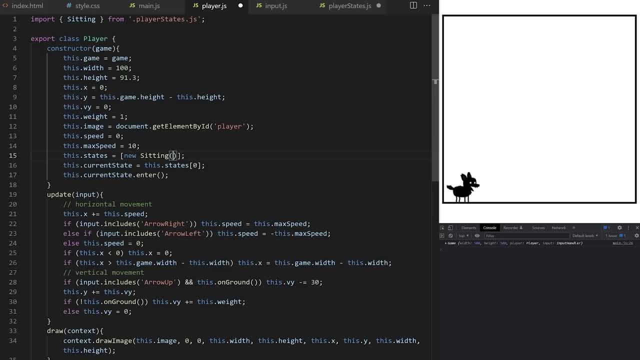 we can just keep calling thiscurrent statehandle input and we will get different behaviors depending on the current state the player is in at that point in time, And this is the entire logic behind state design pattern. If it's still not clear, don't worry, I will go over it today, step by step, as we write the code. It will make more sense if 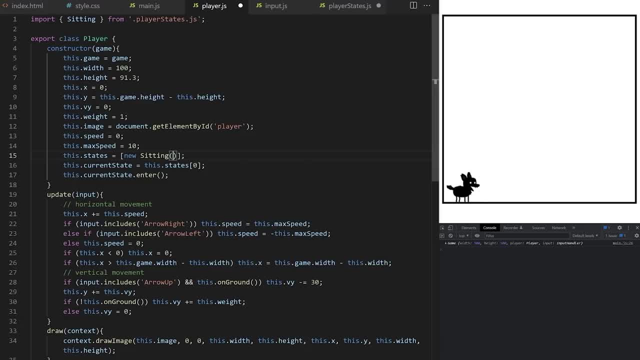 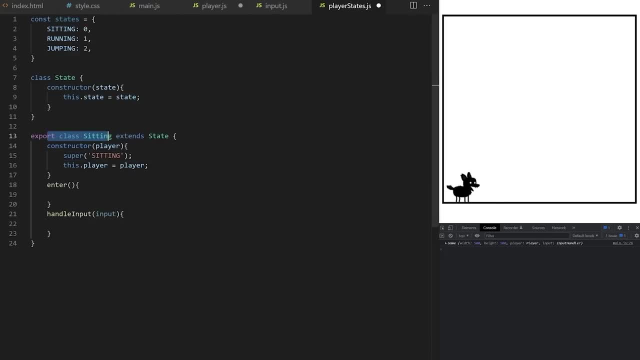 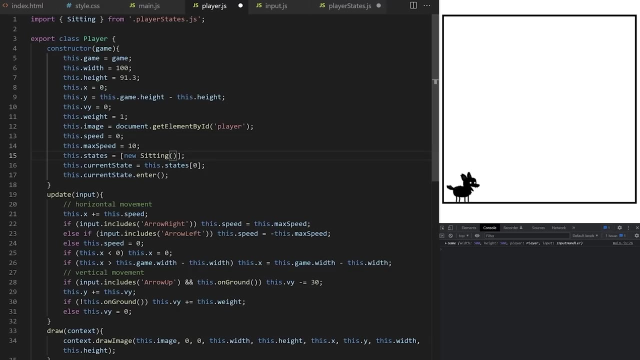 you practice and code with me Inside thisstates array, I will instantiate each state class. Right now I'm creating an instance of sitting class Here, on line 14, in player statesjs, I can see that it expects a reference to the entire player object as an argument. Because here we are. 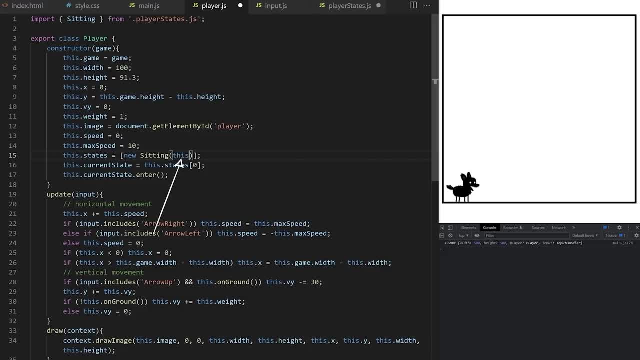 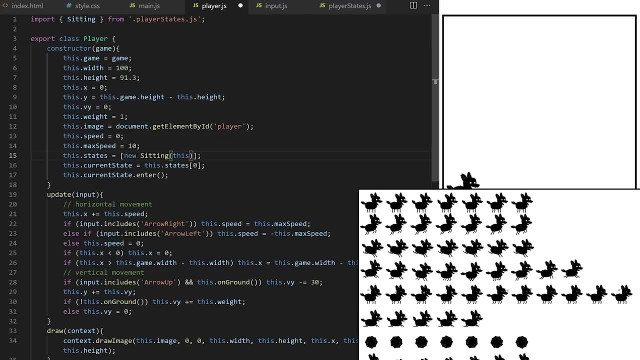 inside player class. I pass it this keyword, which references this entire player class. When we enter a sitting state, I want to draw a different animation row in player's spreadsheet. Let's set up sprite animation. We will have frame x horizontal frame that will cycle from left to. 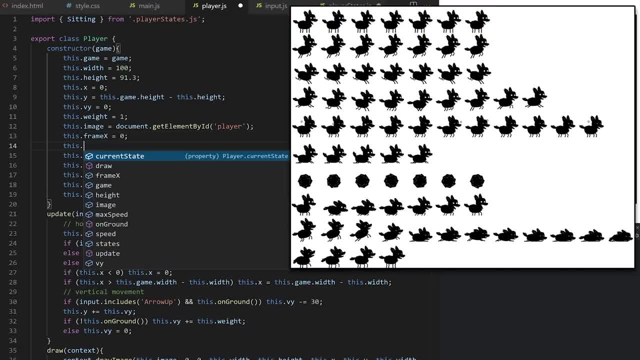 right, animating the player, and we will have frame y which will travel in the spreadsheet vertically whenever we switch to a different state. You can see that frame y zero is standing, frame y one is jumping, and so on, Changing the values of frame x and frame y will jump. 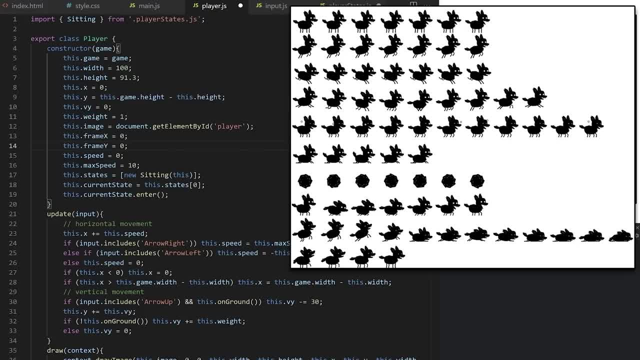 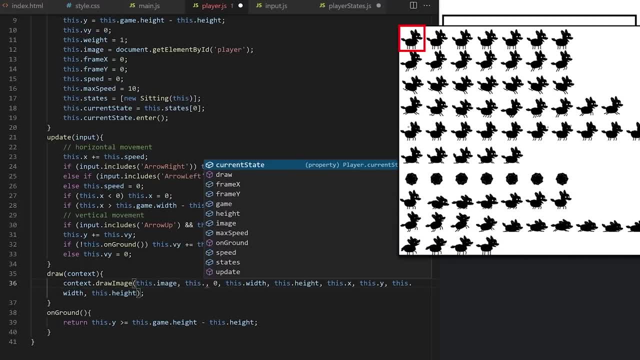 by the width and height of a single frame so that we can animate the sprite sheet. In draw method, I replace hardcoded coordinates 0,0, which are currently displaying this top left frame, to dynamic values. Source x value will be thisframe x times the width of. 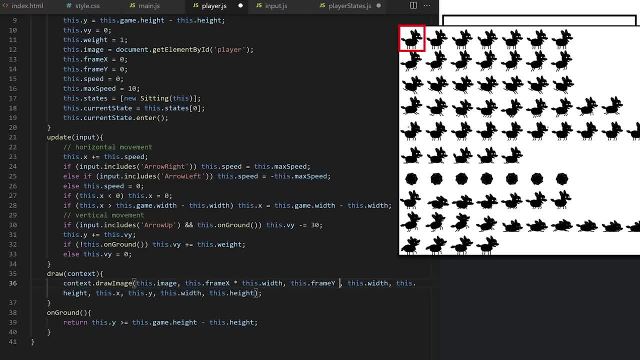 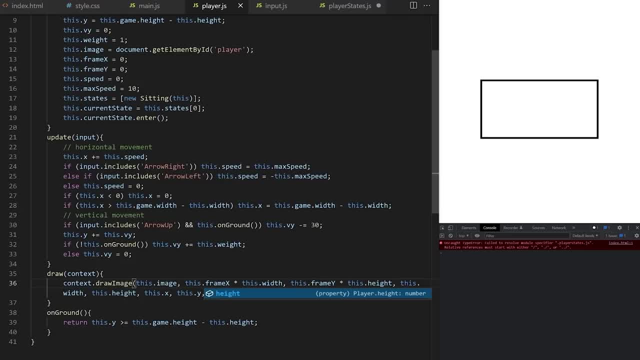 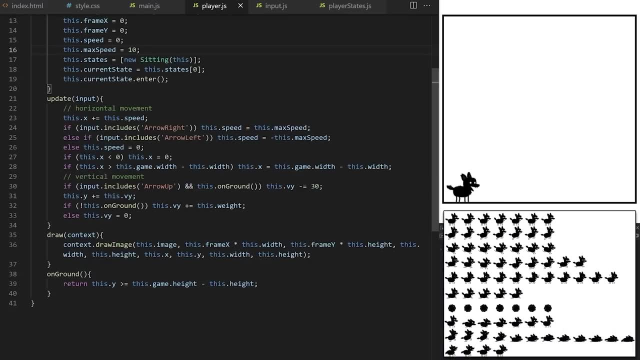 the player frame. Source y will be thisframe. y times the height of the player frame. I'm getting a console error. It's because I forgot a forward slash here on line 1 in playerjs. Now it's fixed. So now frame x cycles back to the original statejsonjsonjsonjsonjsonjsonjsonjsonjsonjsonjsonjson. 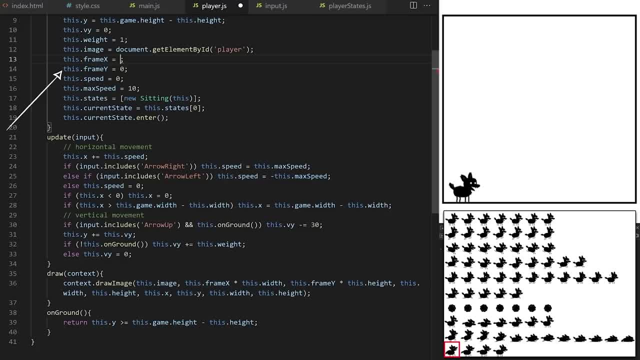 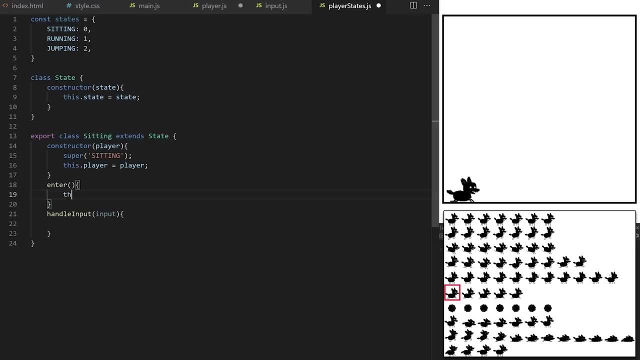 horizontally. Frame y travels around the sprite sheet vertically. I can see that the sitting animation is frame y 5. When we enter sitting state, I take thisplayer from line 16, which points towards the player object, and I set its frame y property to 5.. I could have defined getters. 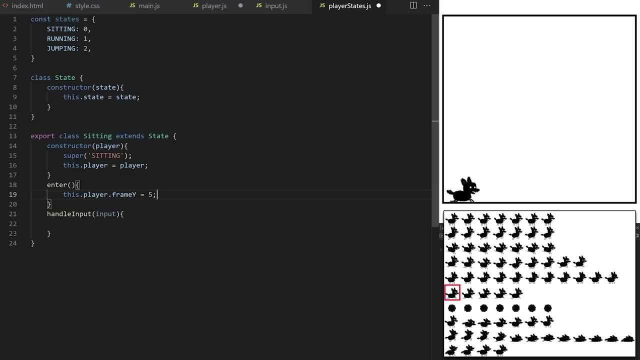 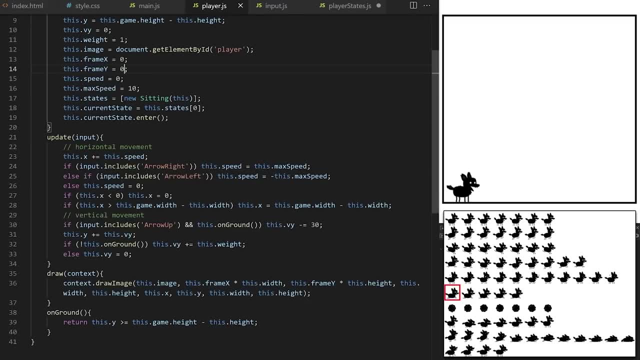 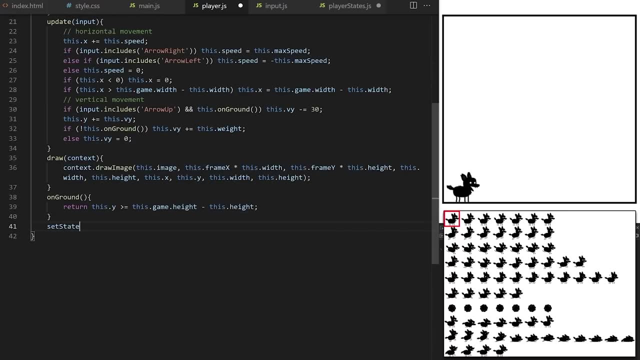 and setters on the player object to do this by the book, but I don't think it's necessary for our purposes today. This code will work well Back in playerjs. I set the initial frame y to 0, which is 1.. Now I need a method that will allow us to switch player between states. I define it down. 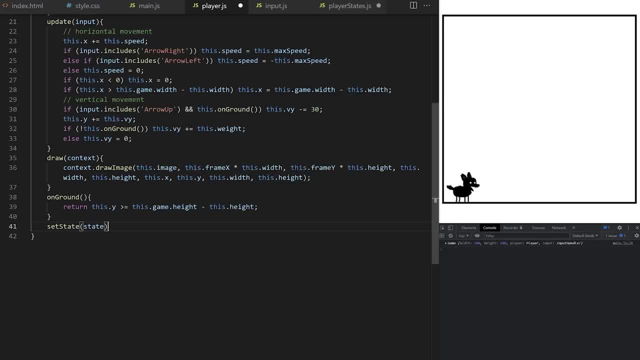 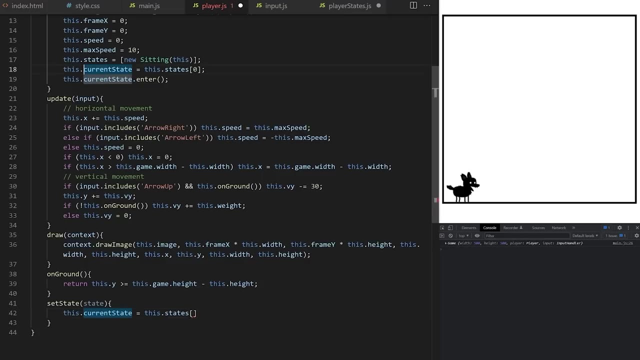 here on the player class. I will call it, for example, setState. It will take this new state we are about to switch to as an argument. It will be a number corresponding to indexes in thisstates array from line 17.. Inside, I set thiscurrentState from line 19 to one of the states from line 17,. 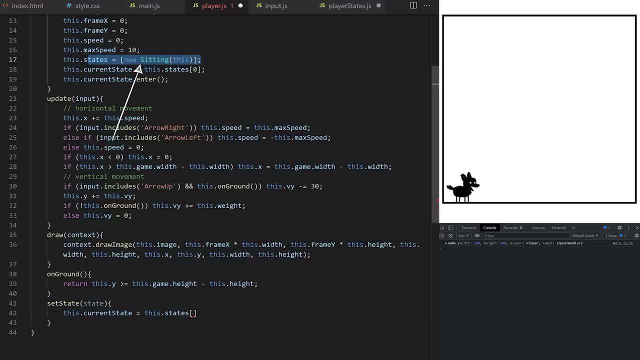 depending on which index I pass to it. Right now we only have one element in the array, the sitting state, That's index 0.. If we have more state classes in the array on line 17 I will be able to swap to index 1, 2 and so on to switch player to those states. Keep in mind setState will take. 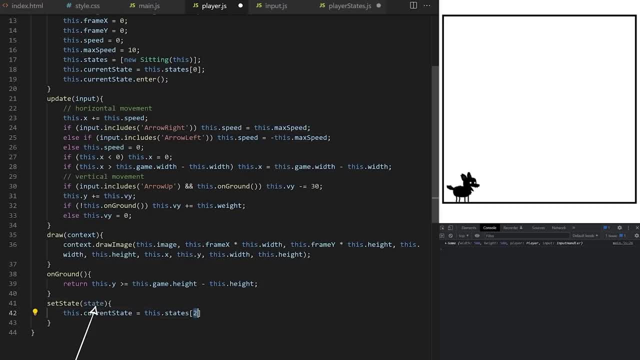 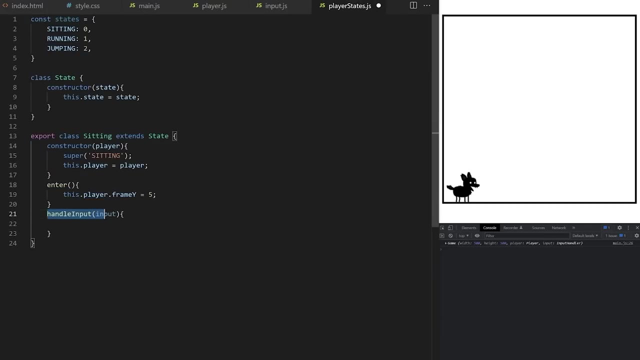 one argument called state, which will be a number corresponding to the index in thisstates array. Then we call enter method on the currently active state to set up things like speed, sprite, animation and so on. There's also handleInput method we defined here. Enter method will run once. every time we enter that state, HandleInput method will be. 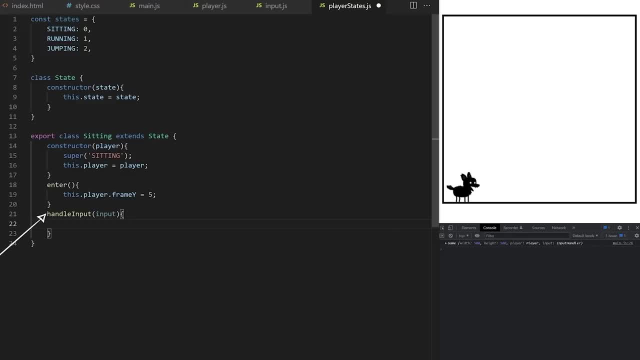 running 60 times per second waiting for keys to be pressed so it can switch the player into a different state when the user requests it by pressing the right set of keys, In our case mostly arrows. so far, I will be calling it from inside: update method on player class here. So 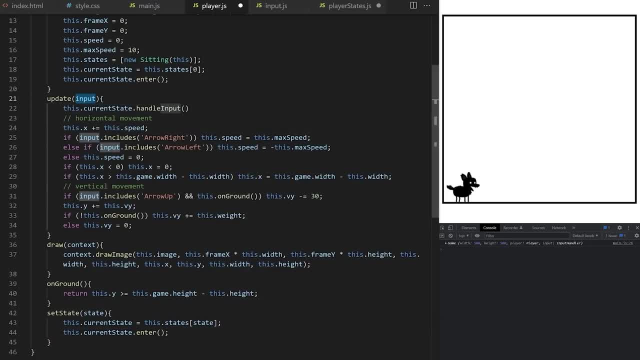 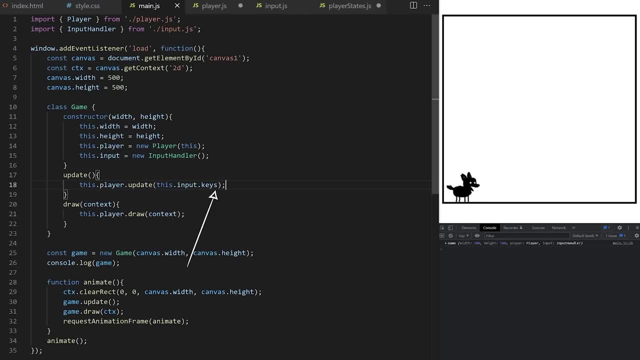 thiscurrentStatehandleInput. I'm passing input value as an argument to the update method here. The value of input is coming from update method on game class, pointing to keys array on an instance of inputHandle class from line 15.. This way, player update method can always see what keys are being pressed in our game. 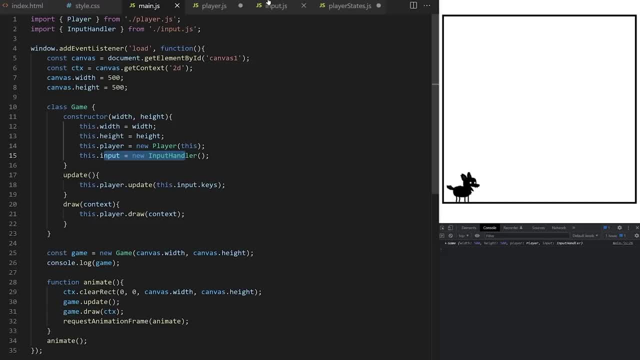 by checking if they are present in this input keys array. We defined it before here on line 3 in inputjs, if you remember. We pass it through game class to update method on player class and I will just pass that argument along to handleInput method like this: 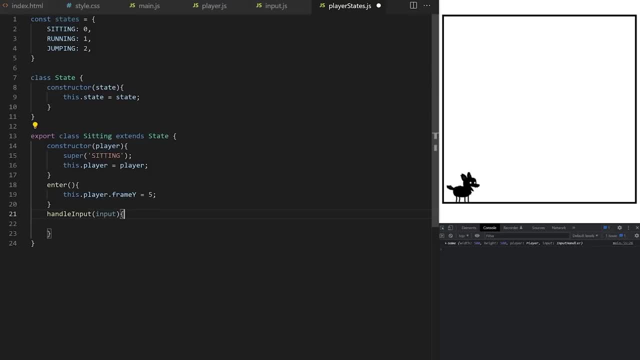 This code will be running 60 times per second, constantly checking what keys are present in input: keys array. HandleInput expects keys array. here, as an argument, I called it input and we will be checking and waiting for specific keys to be pressed. The main function of state design pattern is that we are basically locking player object. 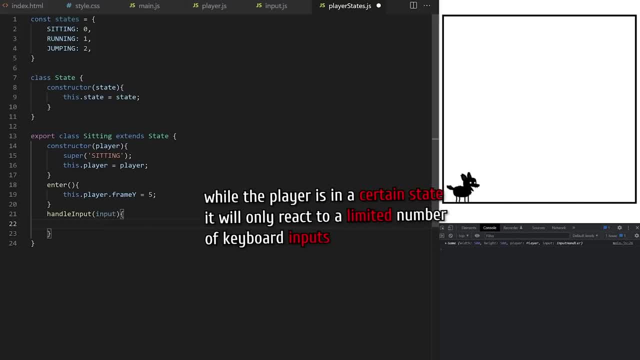 in one state at a time, and while the player is in a certain state, it will only react to a limited number of keyboard inputs. While the player is in the sitting state, we will react to arrow left and arrow right keys and when they are pressed, we will switch into running state. 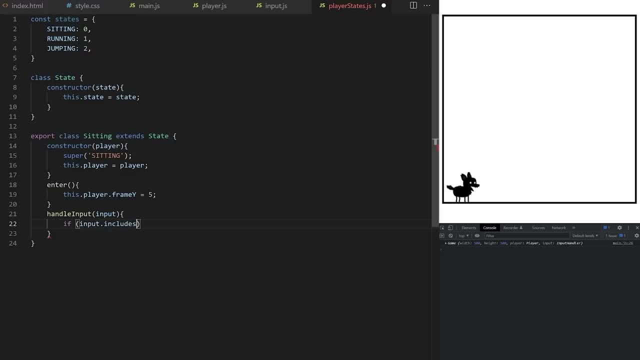 So I say, if this input value that was passed as an argument which points to thiskeys array on inputHandle class, if that array includes arrow left key or if it includes arrow right key, call setState method on player object. Here we can see that setState method expects state as an argument and it will set the current state. 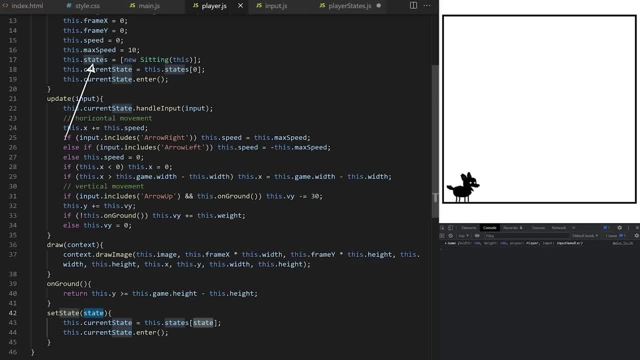 of the player to that index in thisstates array from line 17.. Right now that array has only one element, so it will only work when I pass it index 0 as a value of this state argument here. It will then call enter method on that new state we just switched to. 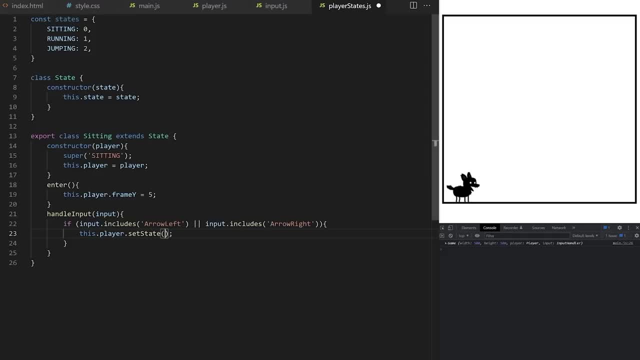 Back to playerStatesjs. So now we know that we have to pass this setState method- a number that will be used as an index in playerStates array, to correctly switch it into that state. I can pass it number 0 here, but we have this enum object here to convert numbers to words like sitting. 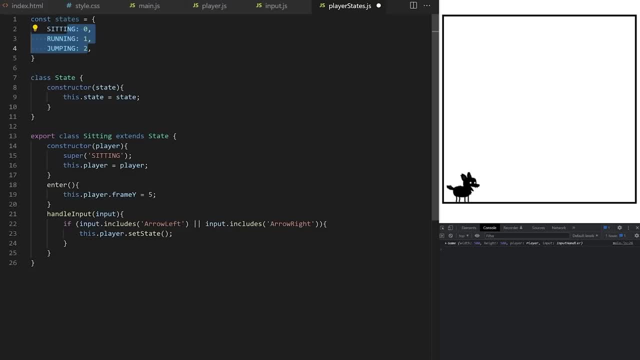 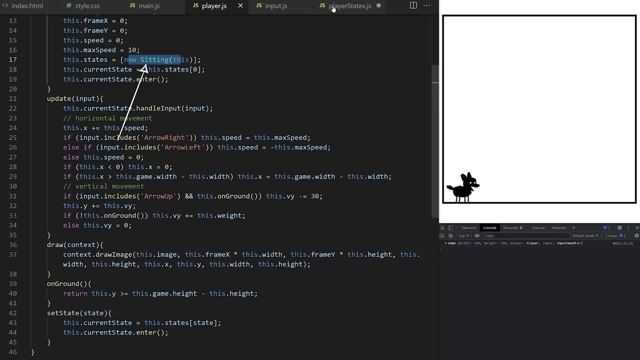 and running. to make our code more readable, The order of states in this enum must be exactly the same as the order of states in thisstates array. on line 17 inside the player class Index, 0 is sitting state, because it's the first element in the array. This enum also needs: 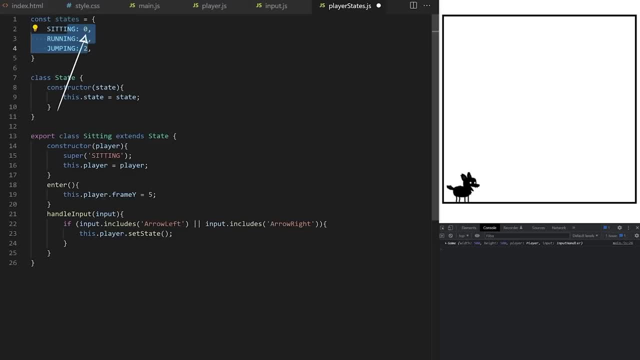 to have the value of 0 paired with sitting, which it does Now. I can call setState and instead of 1, which would also work, but it would be less readable, I pass it. states from line 1, dot running, which has a value of 1 behind it as well. I hope it's a bit more clear. This is the 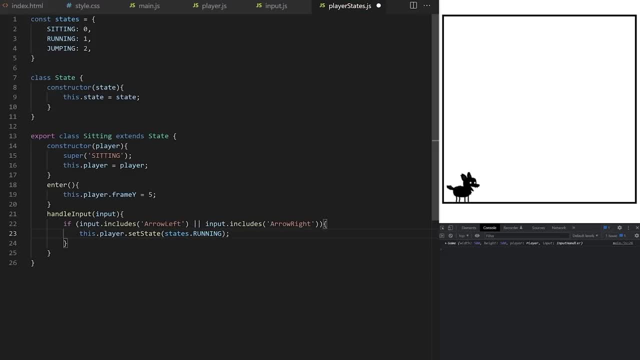 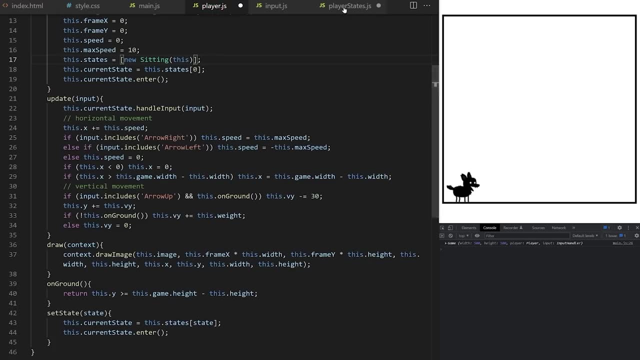 most complicated part and we just covered it. Just keep coding with me and it will start making more sense. Right now there is no index 1 in this array yet. We need to create running class to add it. I copy this code block and I rename it to running and I also put running here. 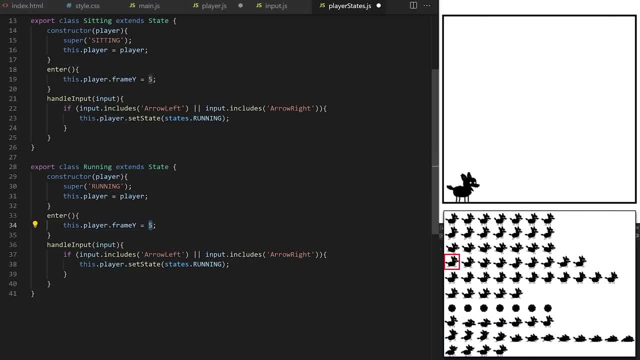 I check the sprite sheet and I can see the fourth row in the sprite sheet is running. So I set frameY to 3 because we count from 0.. In handle input on running class, we will listen for arrow down and when it's pressed we switch player to the sitting state. 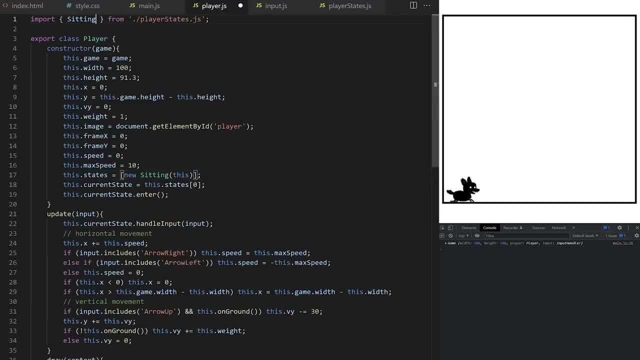 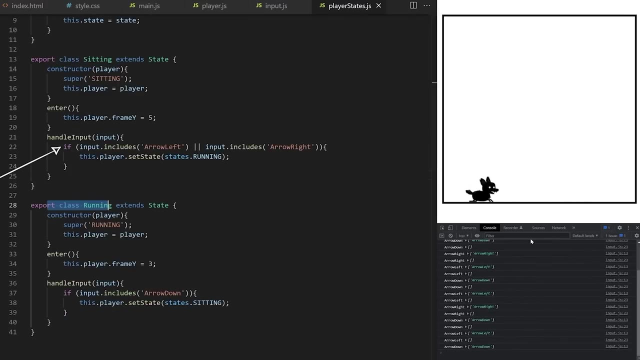 We are exporting running class here. I import it up here in playerjs and I instantiate it as an element with an index of 1 inside thisstates array, Nice. So now, when we are in the sitting state and we press left or right key, we switch into the running state. When 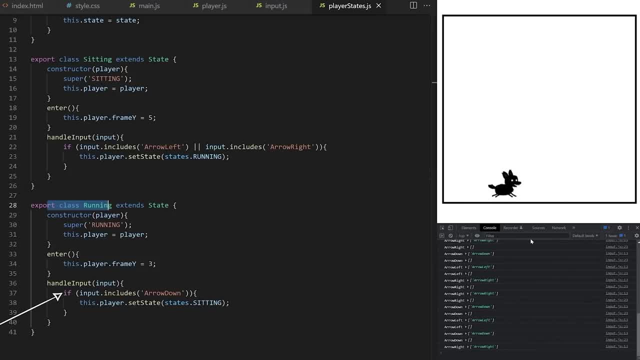 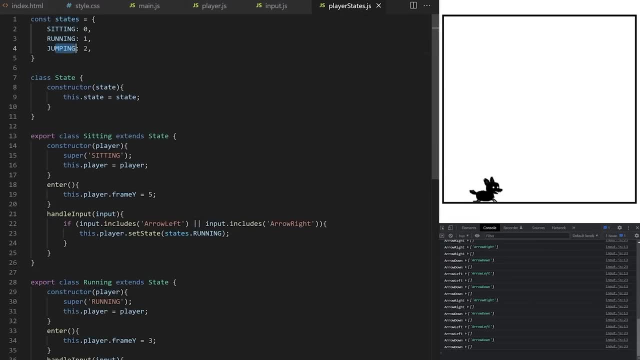 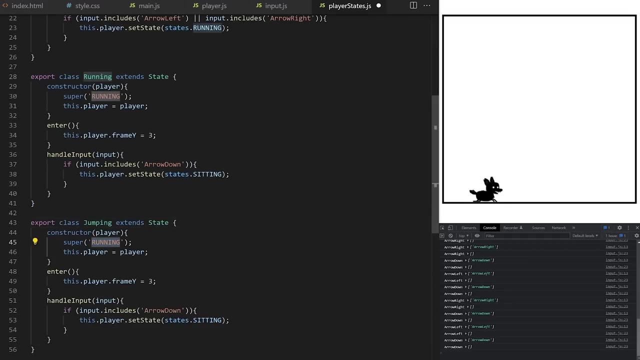 we are in running state, we listen for arrow down key and when it's pressed we switch back to the sitting state. Perfect, We have all the logic for swapping states in place. Let's add a jumping state Again. I copy this code block, I rename it to jumping and I put the jump in here. 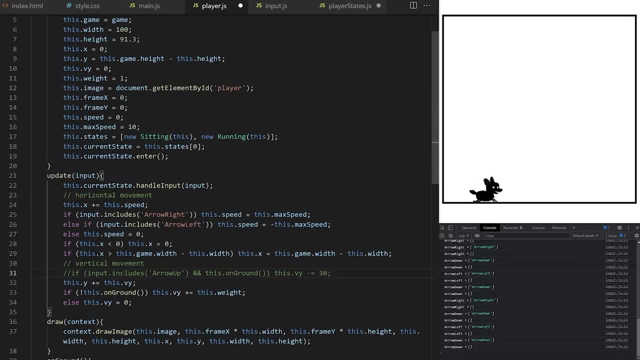 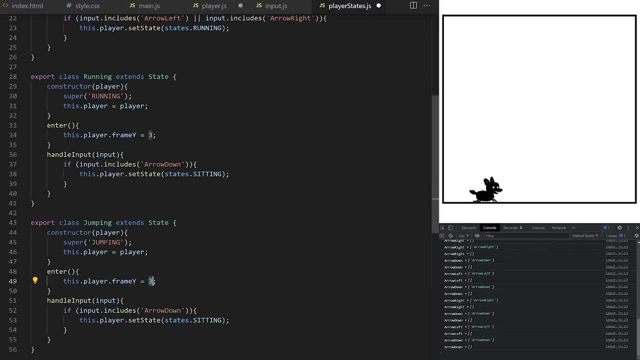 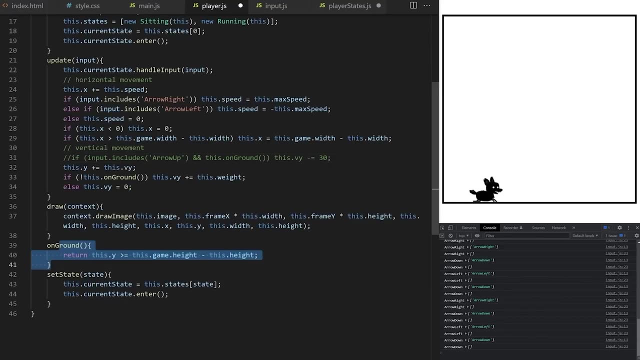 I comment out line 31 inside playerjs and I add a jump in here. This is the same method we used for jumping before. Let's refactor it. When we enter jumping state, we set frameY to 1.. If the player is on ground, that method comes from. 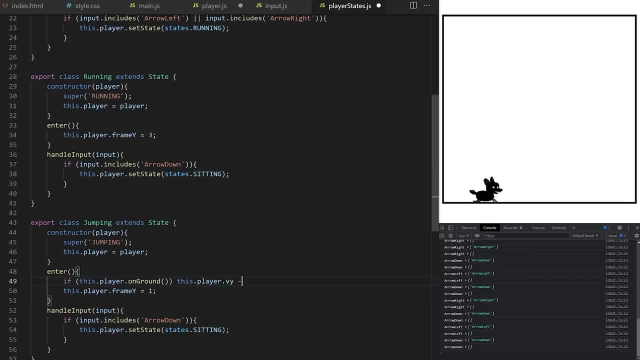 line 39 in playerjs we set velocityY on the player to minus 30, pushing it upwards As we discussed in part 1. during a jump, velocityY goes from minus 30 to 0. moving the player upwards into positive numbers, the player will start falling down. We have a nice falling animation. 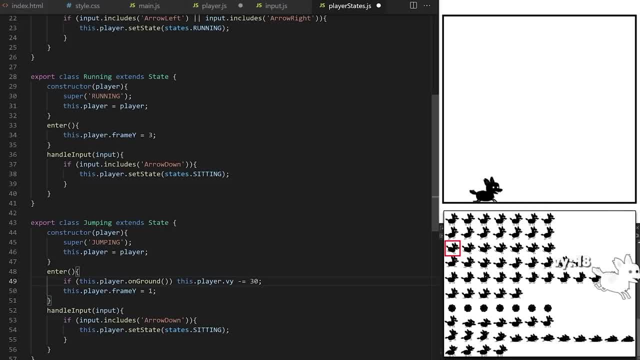 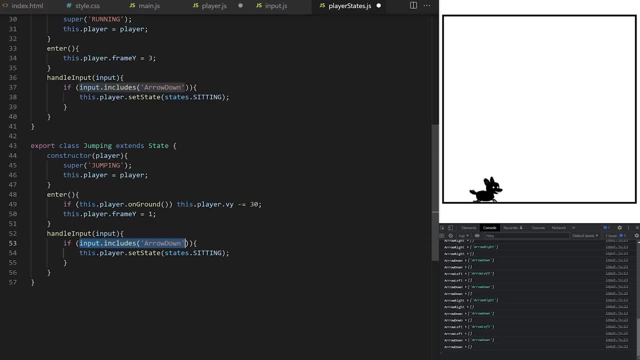 row in our sprite sheet, so let's switch the player into falling state when it reaches the peak of its jump. Instead of listening for key presses, we can also check for values of properties on the player When velocityY switches to the positive values and is more than player weight. 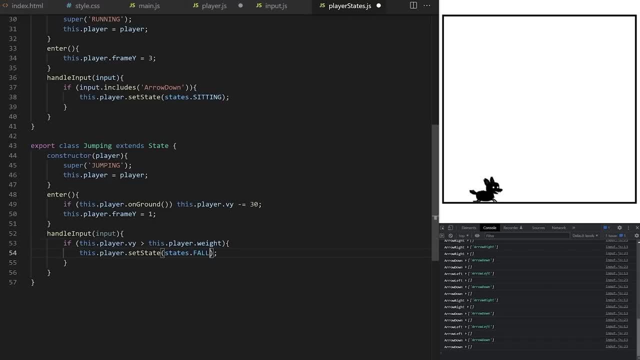 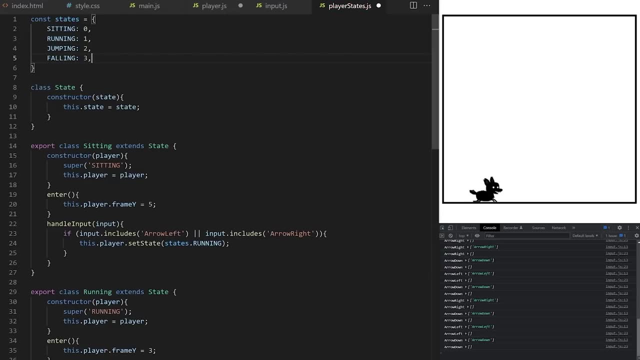 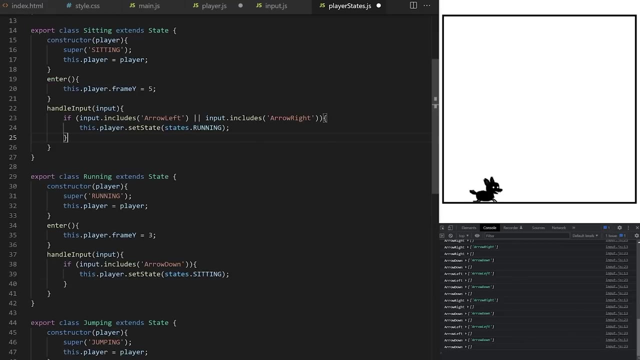 more than 1. we know the player is falling down at that point, so we set state the states dot falling. That will point up here. so I add falling in our enum and I give it a value of 3.. We have our new jumping state but there is currently no way to enter jumping in our game. 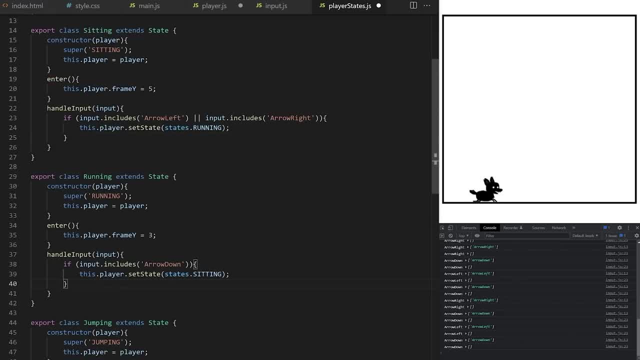 We can enter it from running state, for example, When the player is in the running state. we already listened for down arrow key. We will also be checking for up arrow like this If input includes arrow up while the player is running, set state to jumping. so value 2.. 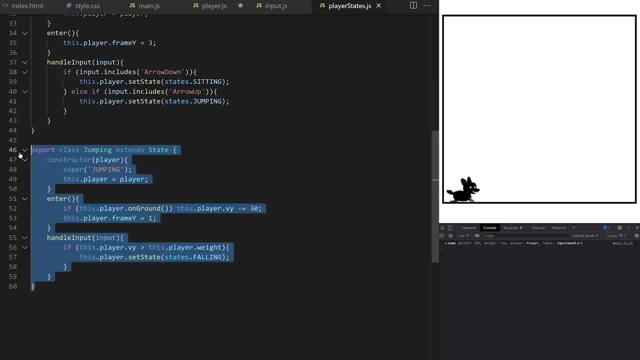 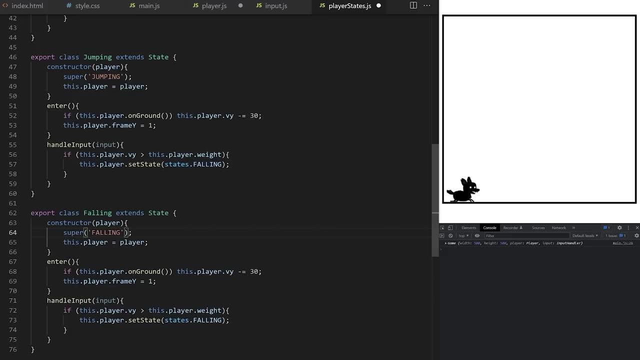 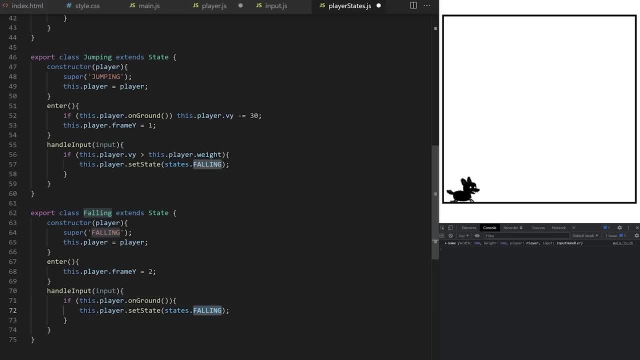 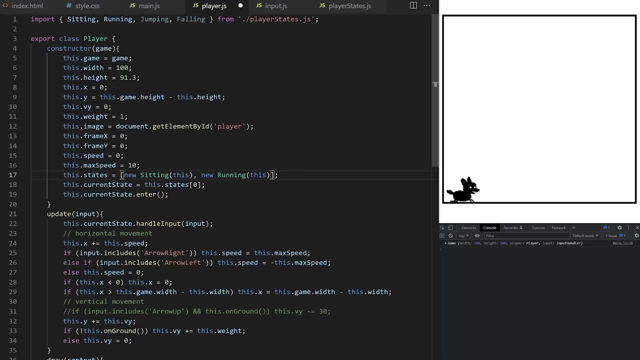 for the player to be back on the ground and then we set state to running. We are exporting jumping class on line 46 and falling class on line 62. I import them up here inside playerjs, Then I instantiate both of these classes inside thisstates array. The order in which you do that is important and it. 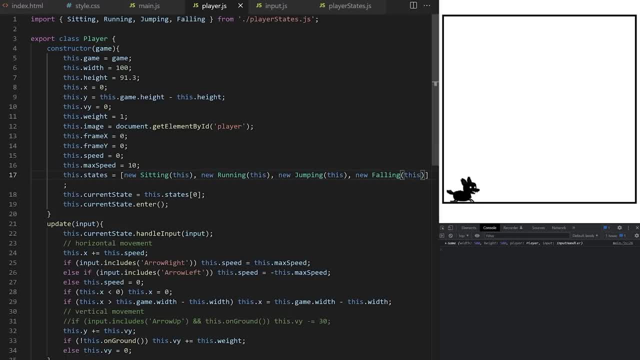 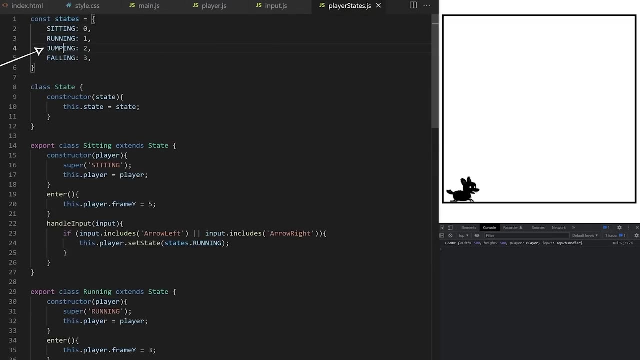 needs to be the same as states enum. we have on line 1 inside playerstatesjs. Those indexes have to match. You can see I'm importing jumping as index 2 in thisstates array Falling is index 3 and here inside enum object jumping has also the value. 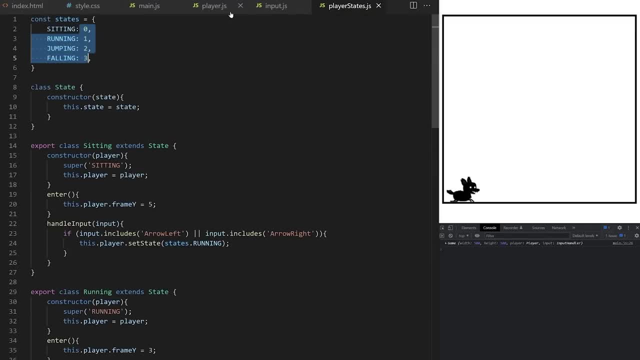 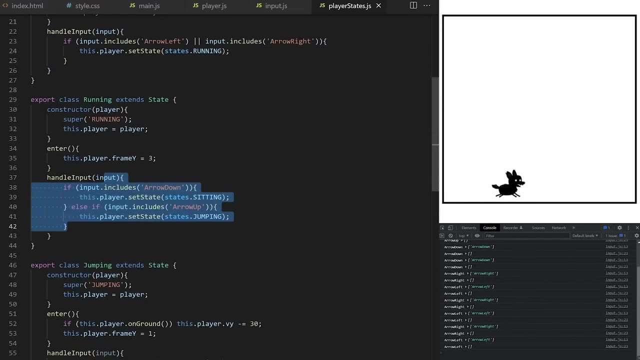 of 2 and falling has value of 3.. It needs to match. While we are inside the sitting state, we can press arrow left and arrow right and it will switch player into running state. While we are inside running state, we can press arrow down to sit or arrow up to jump. To keep things simple, I can also: 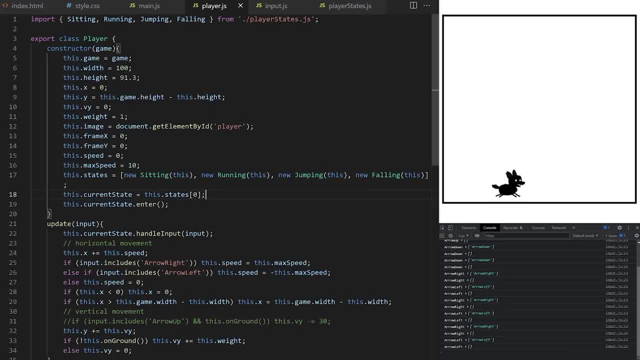 check for arrow left and arrow right here inside update method, because I want the player to be able to move left and right in basically all states when the arrows are pressed. The controls feel better that way. That means we can move left and right in the air even. 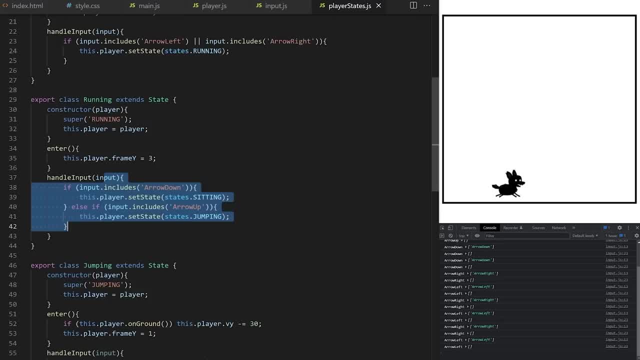 while we are jumping or falling or rolling. When I'm in the running state, if I press up arrow key, we jump and when we reach the peak of the jump we get automatically swapped into a falling state. When we hit the ground, we automatically switch into running state. Great, 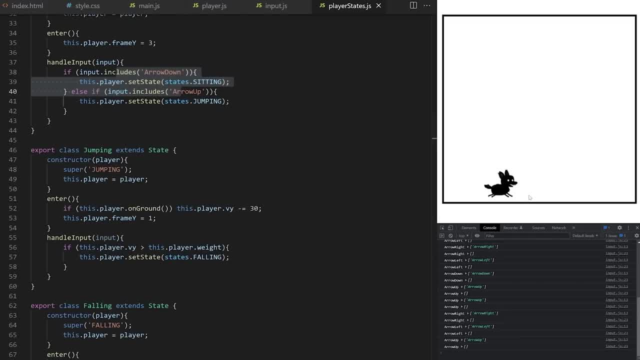 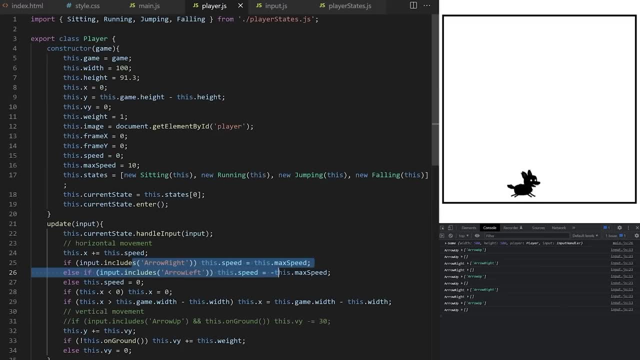 I adjust this minus velocity y value to change the height of the jump. Well done, if you follow the code all the way here, You can also change the height of the jump value. Now you can. Now you know how to apply state design pattern, which is quite an advanced technique especially. 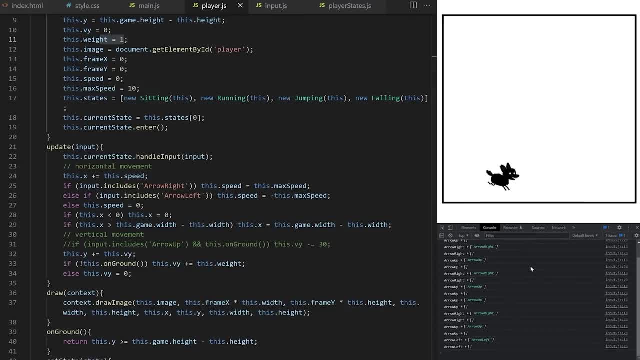 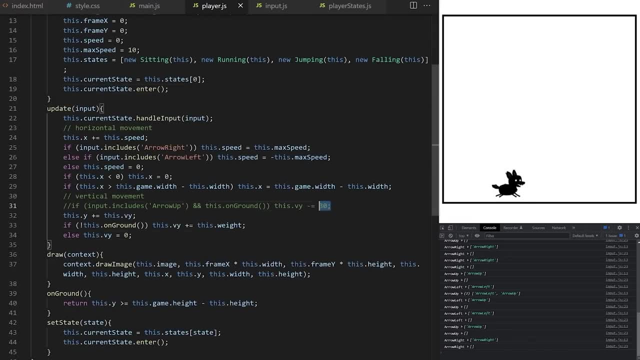 if you are a beginner, We will add more states to it soon. but before we do that, let's properly animate the sprite sheet of our dog. I want it to animate and move. I delete this line of code. We will handle sprite animation in this area. 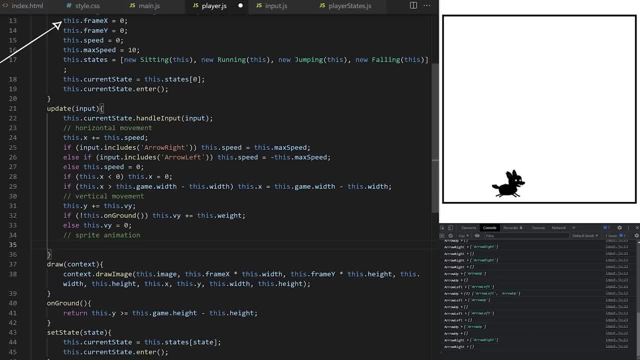 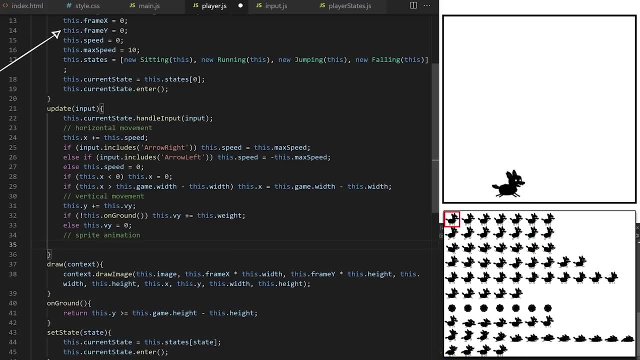 Inside update method on player class. We have frameX property which holds the index of horizontal frame. We have frameY, which refers to the vertical position. in the sprite sheet You can see that different rows have different number of frames. I want to rotate between frame 0 and max frame on that row, depending on which row we currently 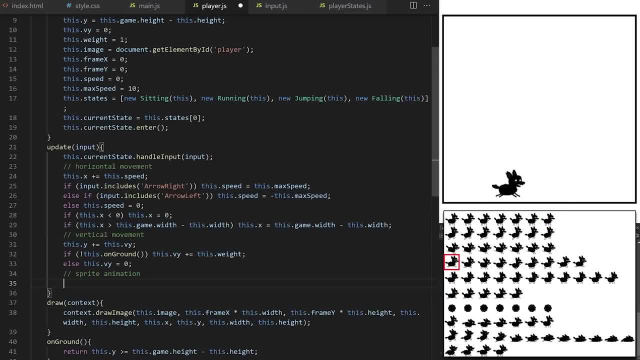 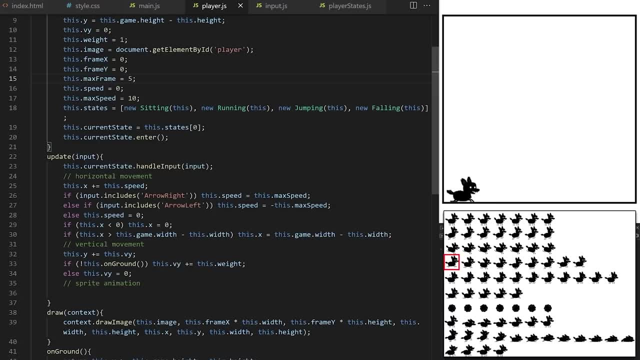 are on Sitting state and running state have different number of frames. We will hold that value in this dot max frame property and we will adjust its value every time we swap states. Since we have our code nicely organized in state design pattern, it's easy to do that. 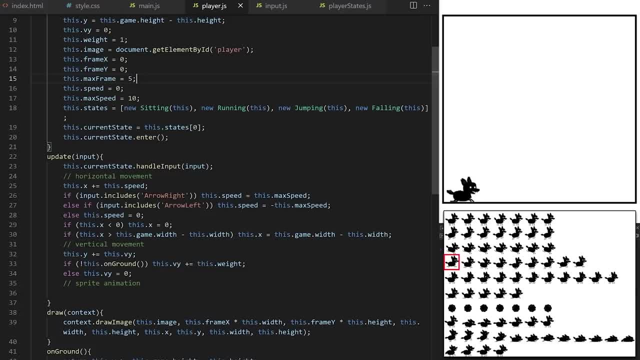 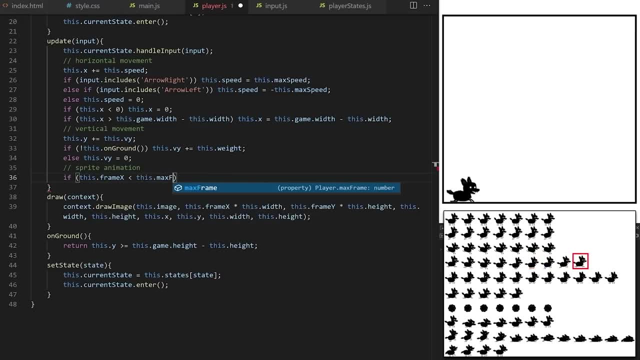 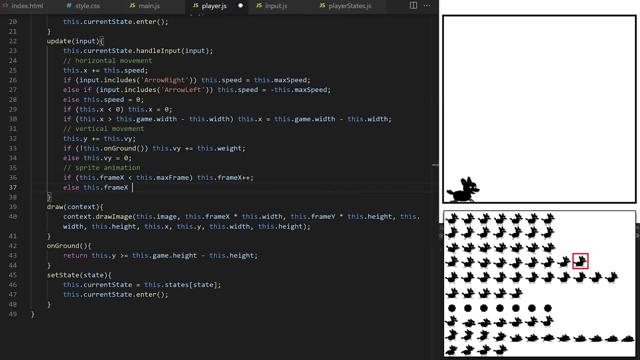 and to keep track of each state. Let me show you So: to animate each row, we will always cycle between frame 0 and max frame on that row. If frameX is less than max frame, increase frameX by 1, else reset frameX back to 0.. 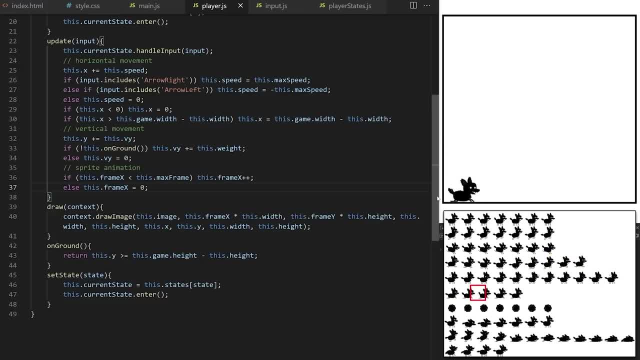 It's going too fast and it's blinking for sitting state because we are including empty frames. It's animating so fast because this particular sprite sheet was designed for lower frame rates. It doesn't matter on which art assets you are using, but it's also easy to control FPS. 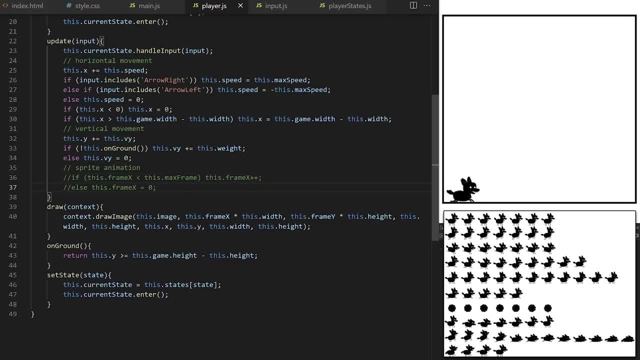 of sprite animation independently of the FPS of the entire game. I can, for example, have the dog sprite sheet animate at 10 frames per second while the entire game is still updating at 60 FPS. You can do it by checking animation timestamps and calculating delta time. 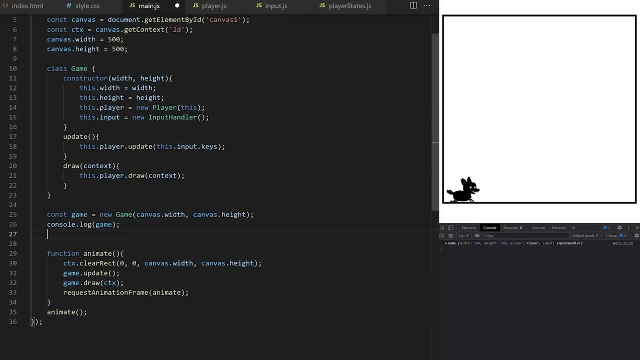 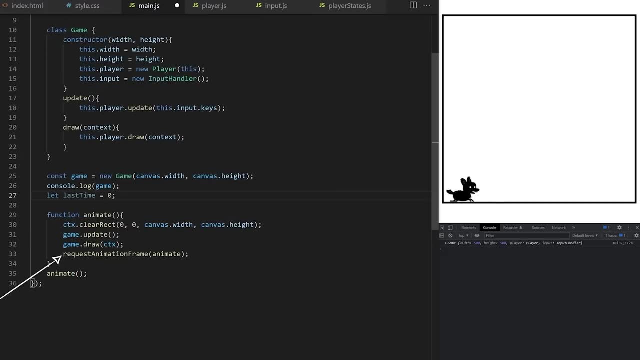 It's easy. let me show you. I will explain it right now. We will need a helper variable here. Last time will hold the value of the timestamp from the previous animation loop. RequestAnimationFrame method has two special features. First, it automatically adjusts the screen refresh rate. 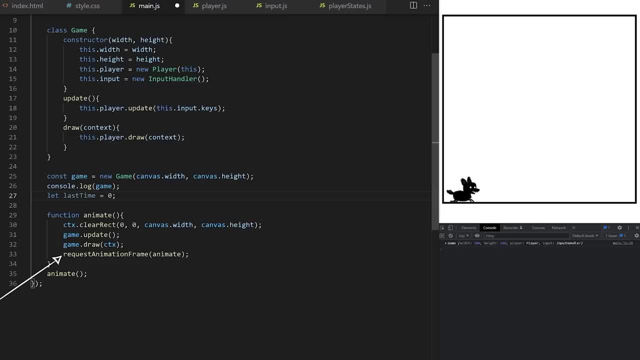 So most of us will get 60 animation frames per second, unless you have some gaming high refresh screen. RequestAnimationFrame also auto generates a timestamp value and it automatically passes it as an argument to the function it calls, in our case animate. I can assign it a variable name here I will call it timestamp, for example. 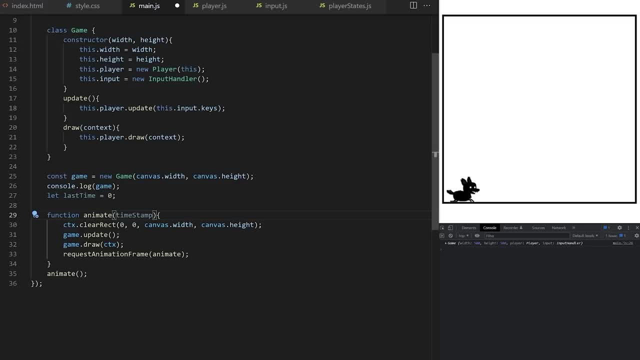 So this timestamp is auto generated by RequestAnimationFrame. As you can see, the frame will be automated every time it serves. a new animation frame, Every time it loops. I will use it to calculate so called delta time. Delta time is the difference in milliseconds between the timestamp from this animation. 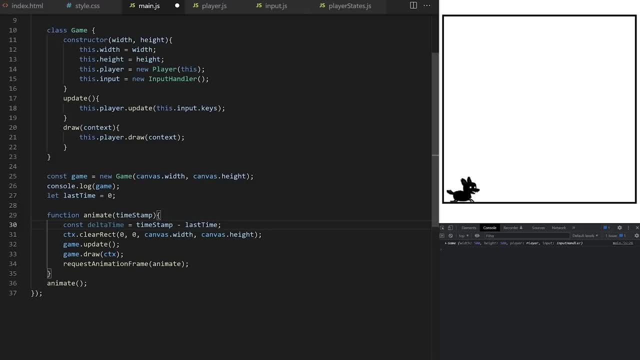 loop that was passed here and the timestamp from the previous loop. It will give us the value of milliseconds for how long each frame stays on the screen before it gets redrawn. Last time will always hold the value of the timestamp from the previous loop. so when 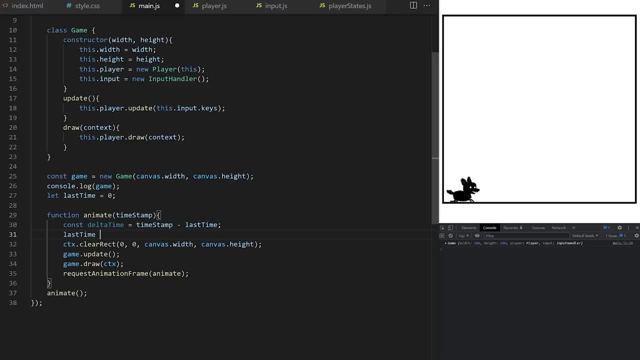 we used it to calculate delta time. we override last time with the value of timestamp from this loop so that it can be used to calculate delta time in the next loop. This might be a bit complicated to understand at first, but don't worry, it will make. 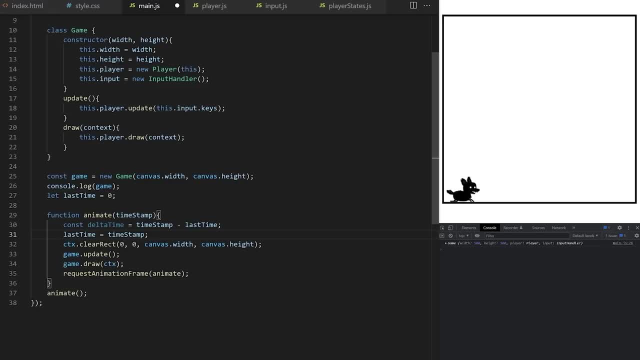 more sense as you use it more often. For this to work, timestamp gets auto-generated only when it's called by requestAnimationFrame. so for the very first initial call of animate I have to pass it some value. for timestamp I will pass it 0.. 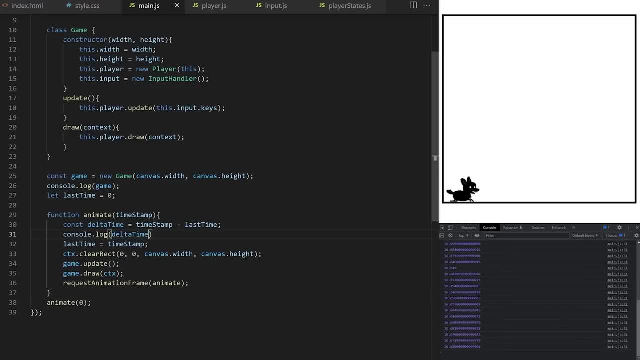 I consolelog delta time and I can see that it's around 16.6 milliseconds, which is around 1000 milliseconds divided by 60. My framerate is 60 frames per second. Perfect, Yours should be similar. The value of delta time calculated this way depends on the power of your computer and 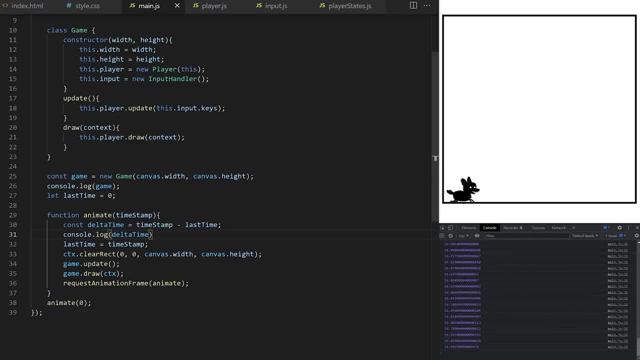 on the refresh rate of your screen So as the animation loop runs, we are recalculating delta time over and over. Every time we calculate it we pass it the GameUpdate method Up here on line 17,. I make sure UpdateMethod expects that argument. 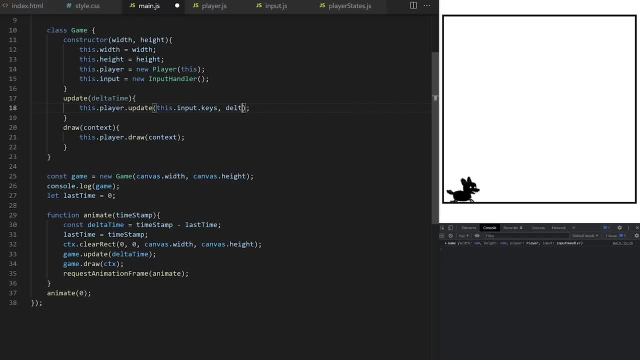 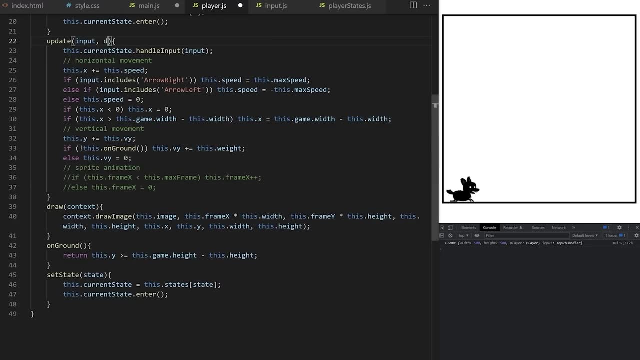 I want that delta time value to be used inside PlayerClass, so I pass it along to PlayerUpdate method as the second argument here. Inside PlayerJS we make sure that it's expected. So now the PlayerClass has access to delta time value. 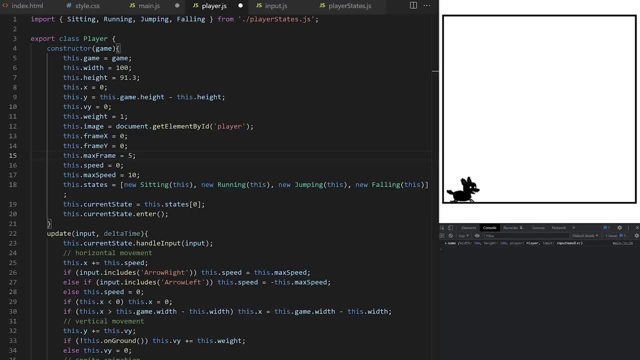 We know how many milliseconds it takes to serve the next frame. We can use that value to adjust sprite animation speed. for example, Only serve the next horizontal frame in the sprite sheet every 50 milliseconds or something like that. We can get complete control over that framerate. 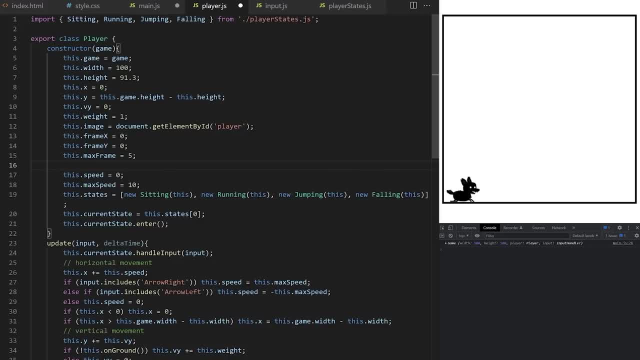 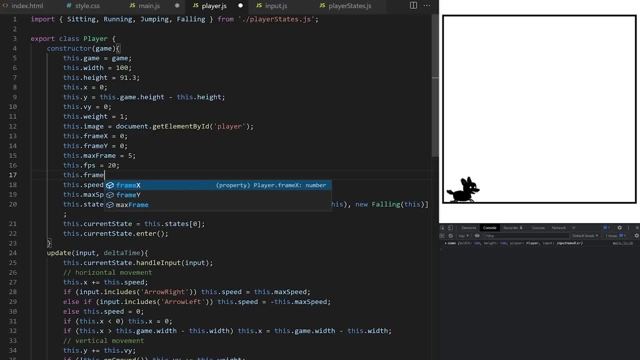 It's simple. Let me show you how This particular doc sprite sheet works the best when it's been animated at 20 frames per second. I will need a number of milliseconds for how long each frame should stay on the screen. If the framerate is 20 frames per second, one frame should stay for 1000 milliseconds. 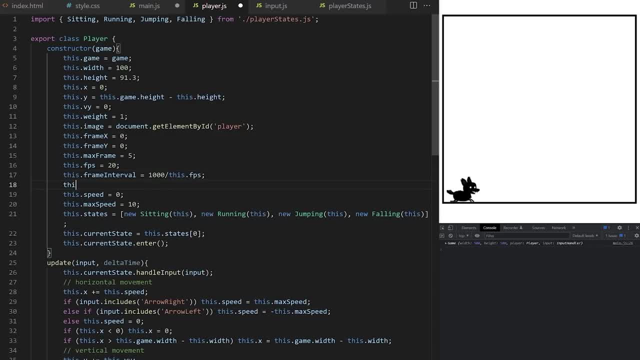 divided by thisfps divided by 20.. We can also circle between 0 and frame interval, increasing by delta time for each frame. Every time it reaches the interval, it will trigger the next frame and it will reset. We will handle that logic here. 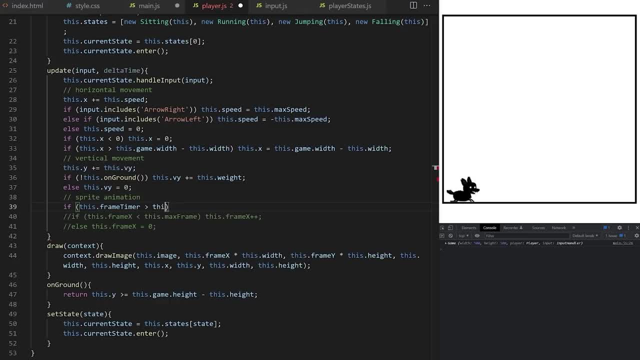 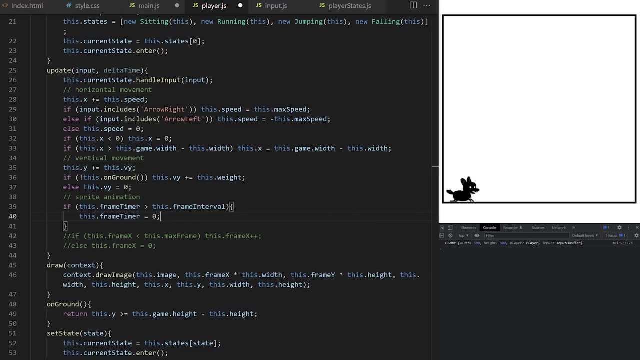 If this frame timer, which starts at 0, is more than frame interval, set frame timer back to 0 so it can count again When that happens. also serve the next frame x horizontal frame in the sprite sheet. Keep increasing frame timer by delta time until we reach that frame interval value. 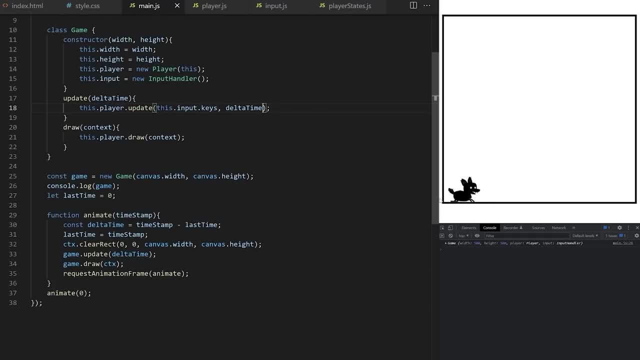 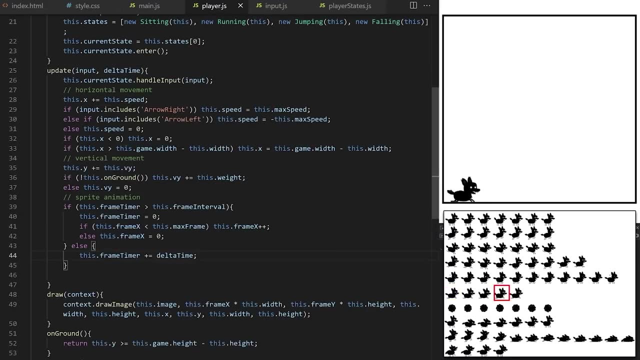 Perfect, Now you know how to control fps in the game. The sprite sheet of our doc is animating at 20 frames per second. You can see it's blinking. It's because we are animating this empty frame here For sitting animation max frame isn't 5, so I remove this value. 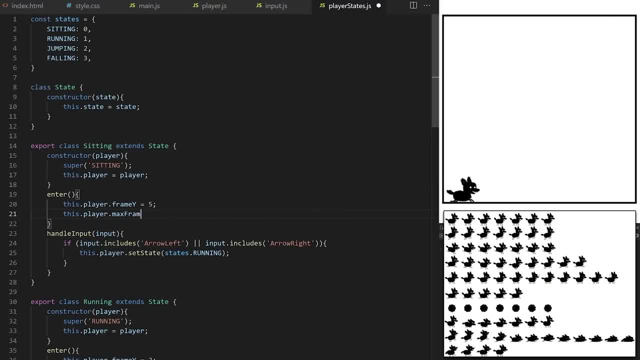 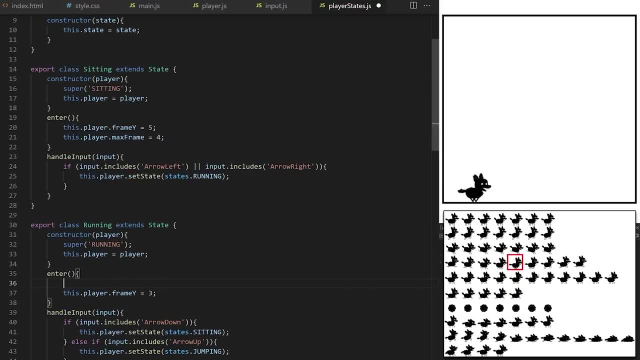 When we enter sitting state, we set max frame on player class to 4.. We count from 0.. When max frame is 4, we are not seeing the whole running animation. so I set max frame inside running state to 6.. 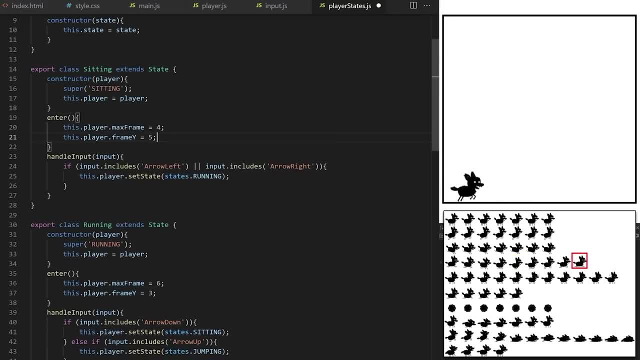 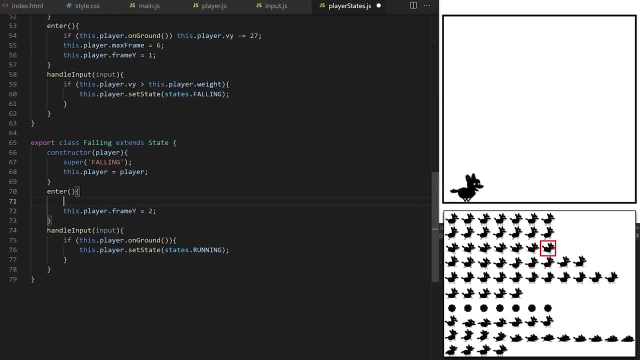 I will also swap max frame and frame y to prevent occasional blinking if we swap states too fast. In jumping, max frame is 6, and falling is also 6.. Now we are correctly animating each state. Do you see how it's easier to keep the code organized when we separated each state into? 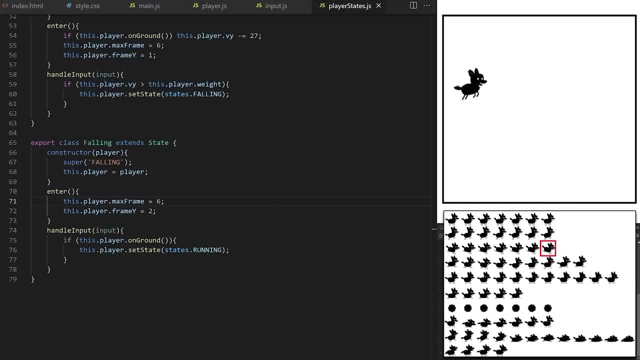 its own class. Occasionally, we can get a situation where we swap state and frame x is currently 6, and frame x is currently 1.. Frame x is currently too high and that row doesn't have that many frames, so we get. 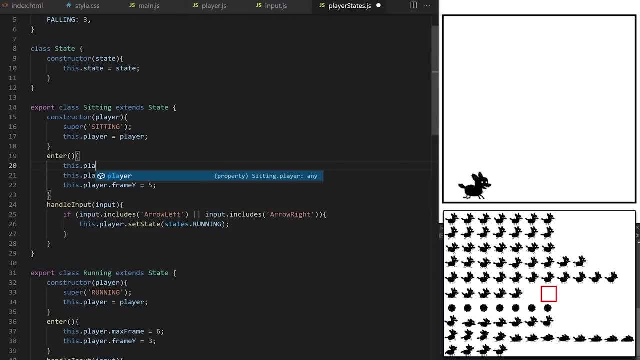 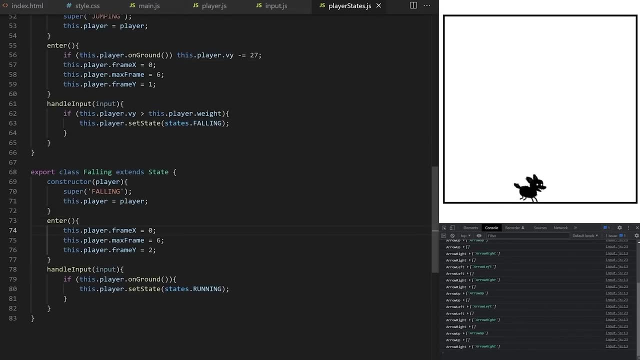 a quick blink To prevent that from happening. every time we enter a new state, we set frame x back to 0, before we swap to a different vertical sprite row with frame y. It's just a small thing. We have complete control of FPS- how fast we serve frames in player sprite sheet. 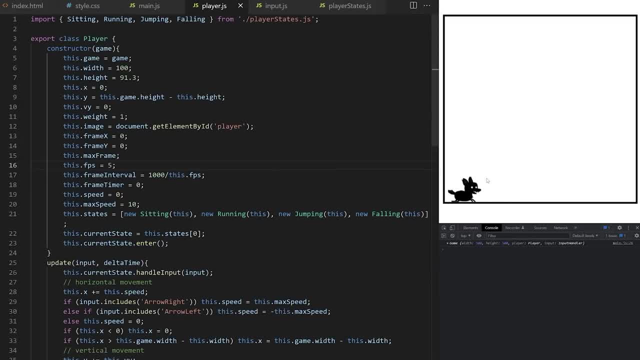 I can come here and set it to 5.. The great thing is that the player still moves At 60 frames per second, But the sprites are animating at 5 frames per second. We can control these two things separately. It would be very bad if controls reacted so slowly. but maybe you have a sprite sheet. 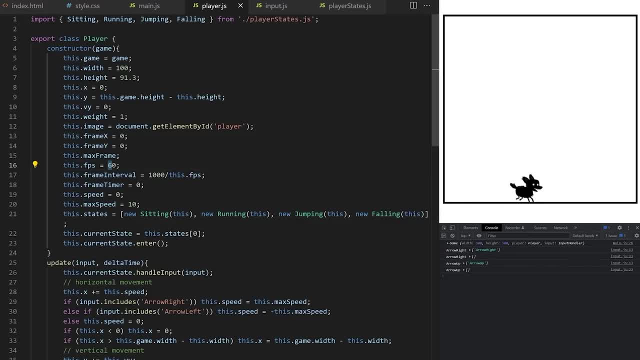 in your game. that was designed for lower FPS. Our sprite sheets were designed for speed around 20 FPS, Depending on what art assets you are using for your game level. you might not want the player to be standing all the way at the bottom of the game area. 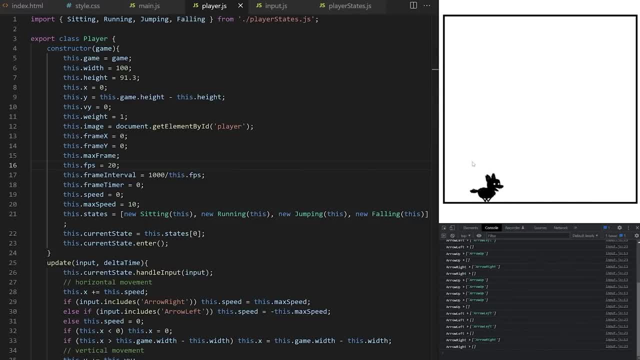 Sometimes you need to adjust this value. Today I will give you all art assets that you can use in your game- All art assets to use. so I know we will need to create some margin on the bottom. That margin will have to be considered in more than one place around the code base. 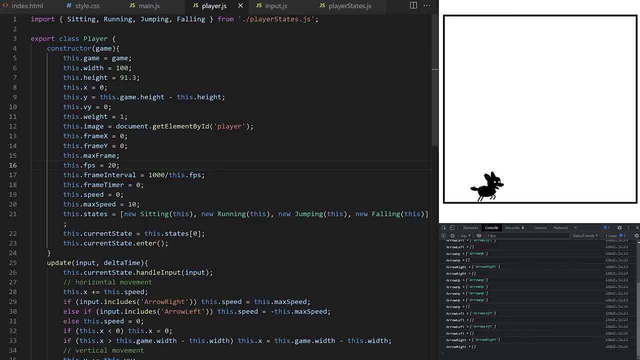 so let's put it in the main game class so it's easy to access. I want the ground level to be 50 pixels from the bottom edge of canvas. This dot ground margin is 50.. Inside playerjs we have access to it through this dot game reference. so the initial vertical. 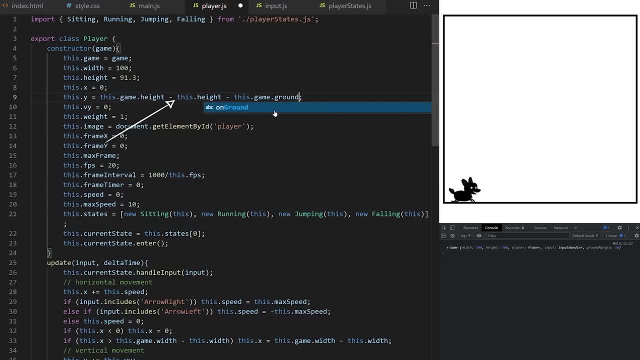 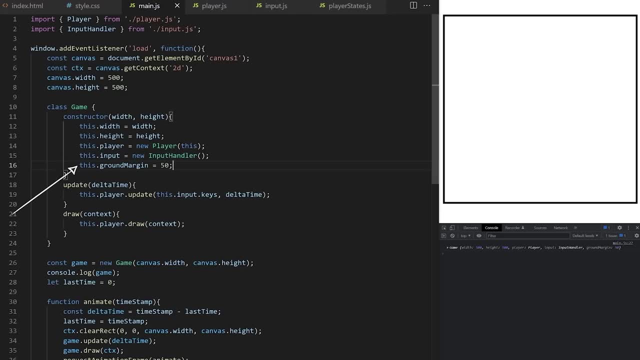 coordinate will be height of the game minus the height of the player, minus ground margin. like this, This will not work, because here I am creating player. before I declare that class property, I need to put it up here so it's available at the point when the player is created. 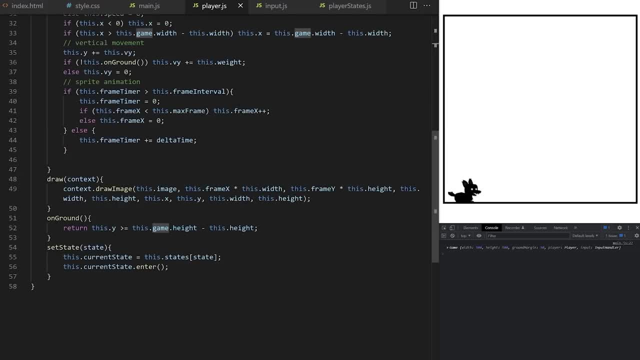 That worked. I also need to adjust this on ground check, because being on ground now also involves this ground margin. Perfect, You can adjust ground margin value to match the environment in which your character is currently moving in. Our environment will be an abandoned, monochrome city. 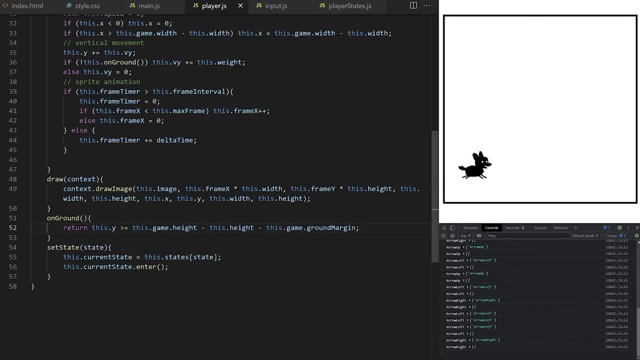 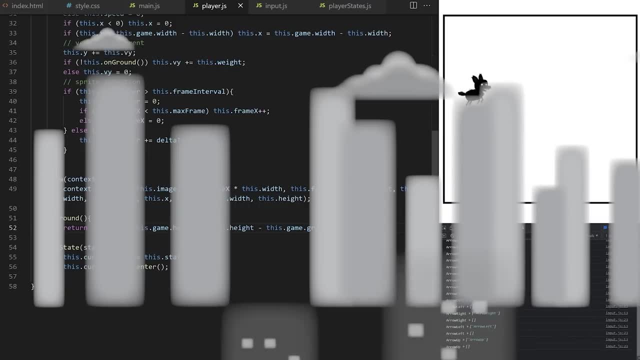 You can download it. Download all art assets in the video description. If you are a beginner, I suggest you use my art assets first and get the game to work before you start adjusting it to your own version. It will save you a lot of headache if you encounter some unexpected challenges, because 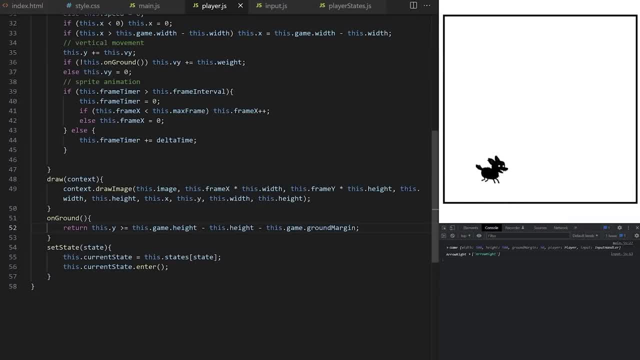 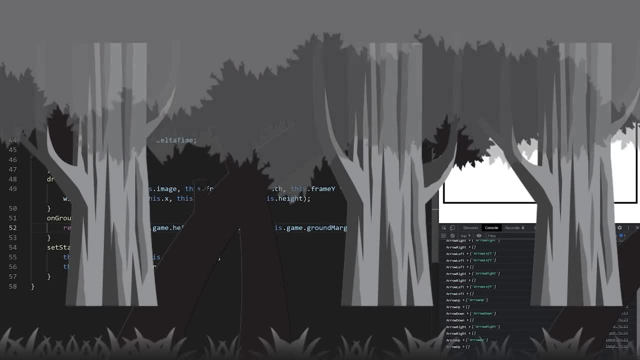 you can just look at my code to fix it. We will be animating a parallax multilayered background. I made a special episode about this. if you want to go more in depth at a beginner friendly pace, We built a small standalone project in there showing all the concepts and alternatives. 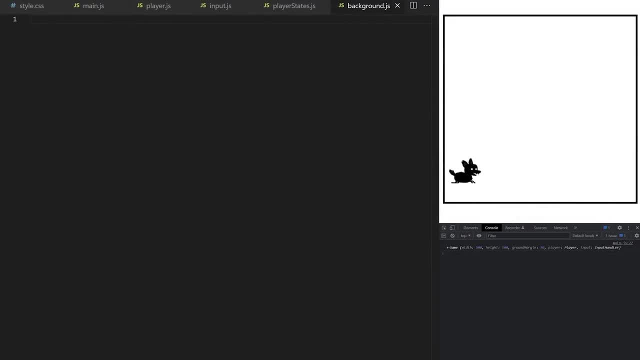 Let's use the quickest version here. So we have a new file I called backgroundjs. I will need two classes here: Helper layer class that will handle logic for each state separately, and main wrapper class. I will call, for example, background that will be exported and animated from the main game. 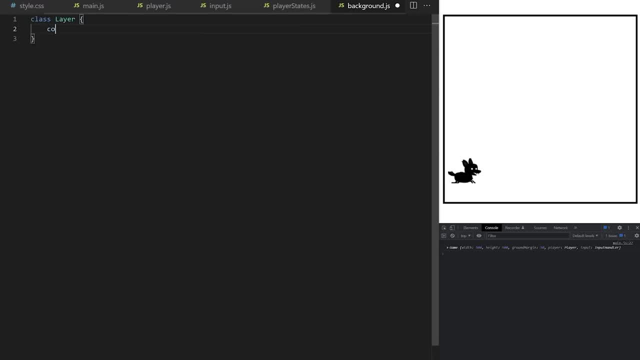 class. It's actually quite simple. Let me show you. Layer class will need access to the game object because we need to be constantly aware of width and height of the available game. We will also need the width and height of the actual background image. 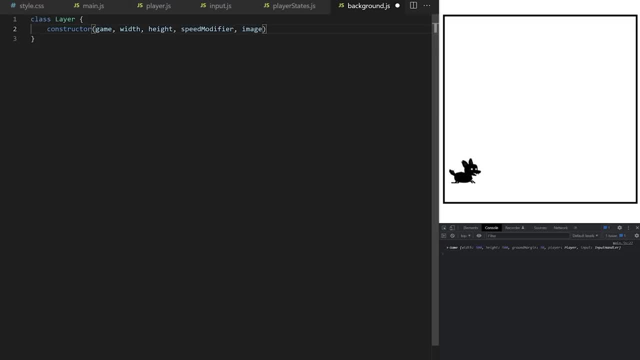 We will need speed modifier argument because each layer will move at a different speed, but relative to the current game speed. The last argument will be an image. Each layer will have a different image. All five images are available to download in the video description. 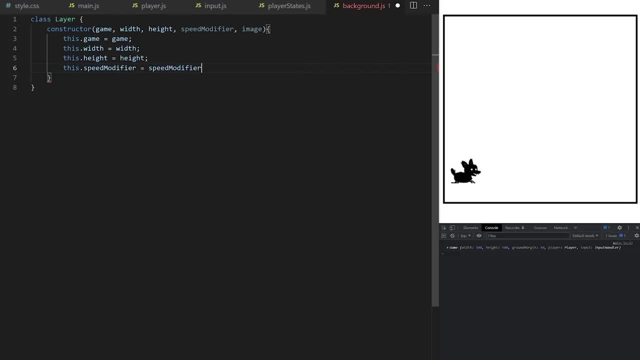 I might also include some alternative art assets in there for experiments later. As usual, we convert the arguments that are passed to layer class constructor into class properties. Each layer will also need x and y position update method to move it and draw method to draw it on canvas. 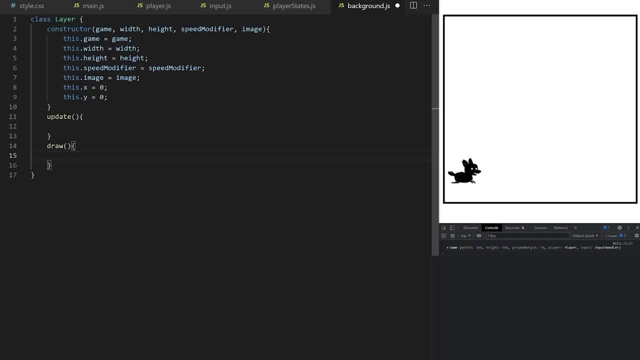 You know how it goes now. I try to keep similar code structure across all classes. for clarity, I could also name these methods something else if I wanted to. The background images we use today are seamless, which means that when they are scrolling from left to right continuously, we can't see where they end and where they begin. 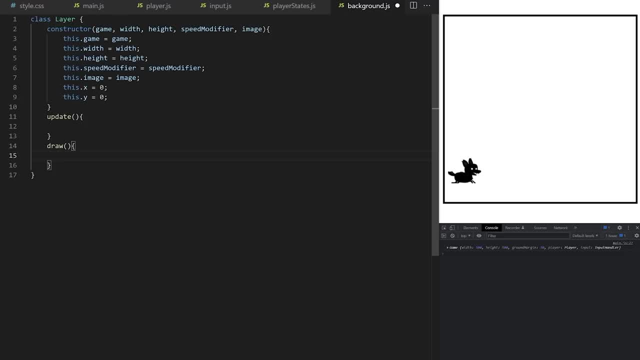 There is a small, simple trick to create an illusion of endless background in a side scroll game and we are about to learn it right now. Click the like if you are getting any value today, We will be updating horizontal x coordinate. Vertical y coordinate will always be zero. 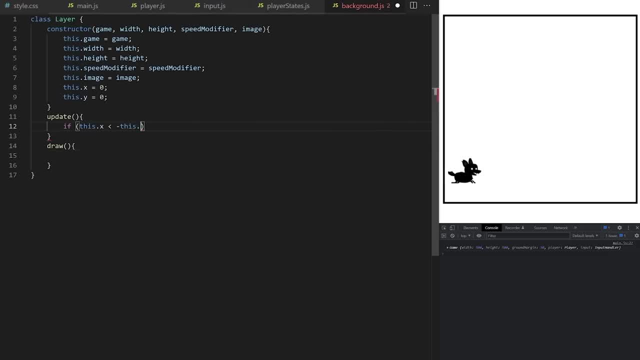 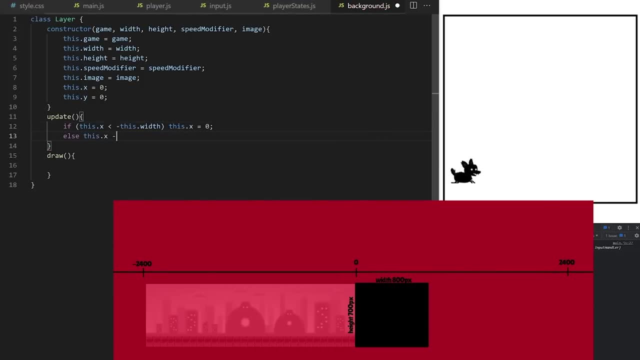 If this dot x is less than minus its entire width, which means it has scrolled all the way behind the left edge of the game area and now is hidden, reset it back to zero so it can scroll again. Else, keep decreasing x by the current game speed times speed modifier, because I want. 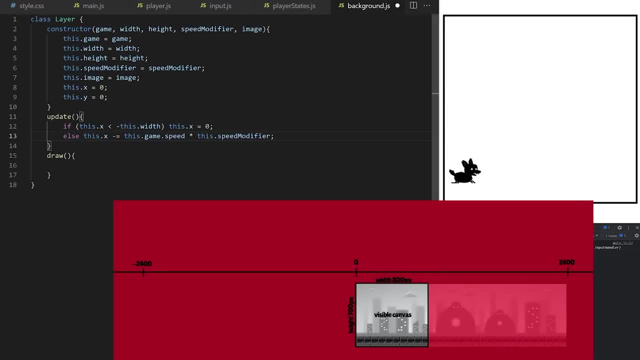 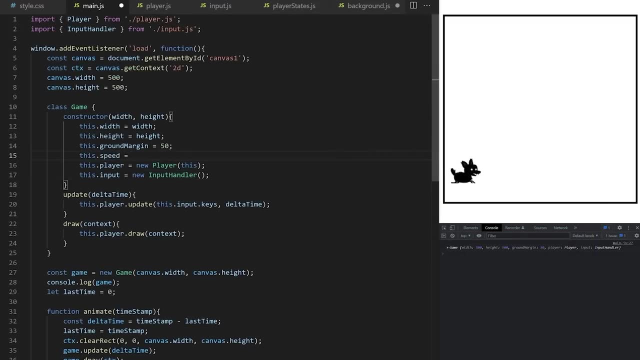 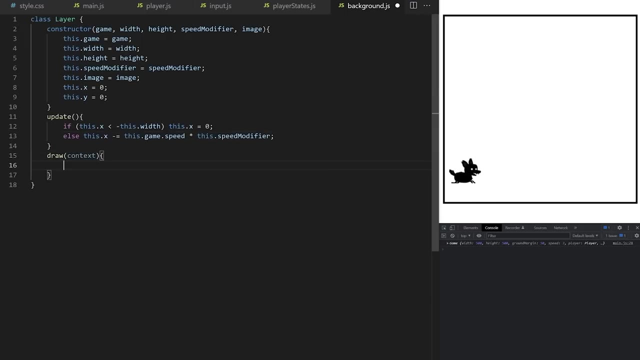 each layer to move at a different speed. Game speed doesn't actually exist yet, so I declare it here on line 15 inside mainjs: Let's set it to 3 pixels per frame. for example, Draw method will need context as an argument to specify which canvas element we want to. 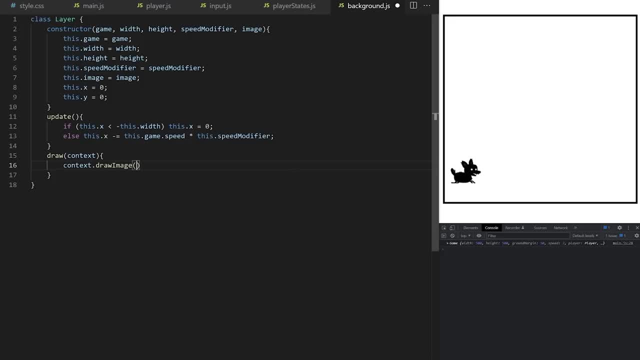 draw on. We call built in canvas draw image method again. This time we don't need the longest version with 9 arguments For backgrounds, we just need the passed 5 arguments Image: we want to draw X and Y. where to draw it? 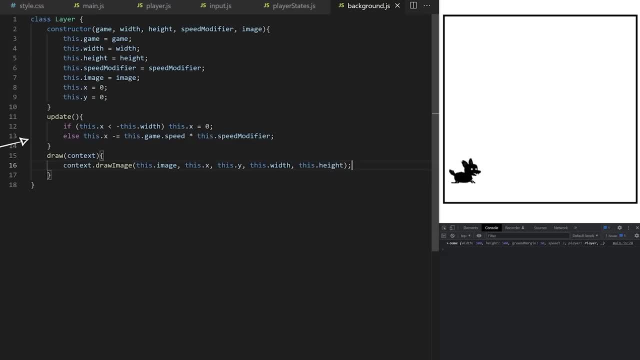 And width and height of that image. So this is a helper class that will handle logic for each individual layer. Our parallax background will have 5 layers. We create and combine them together in another class. I call, for example, background and I will be exporting that class. 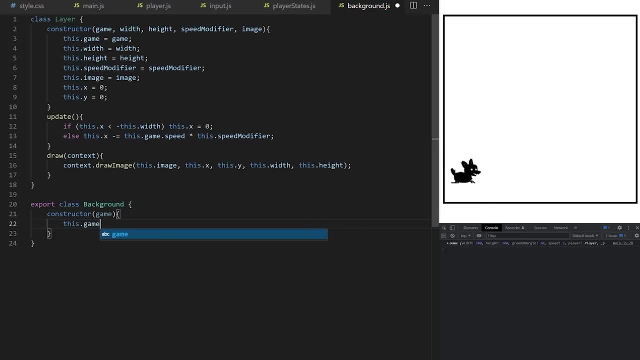 It will need access to the main game class because we need its width and height and game speed properties. I'm providing you images of a specific size for this project. The width of each layer image is 1667 pixels and height is set to 500 pixels. 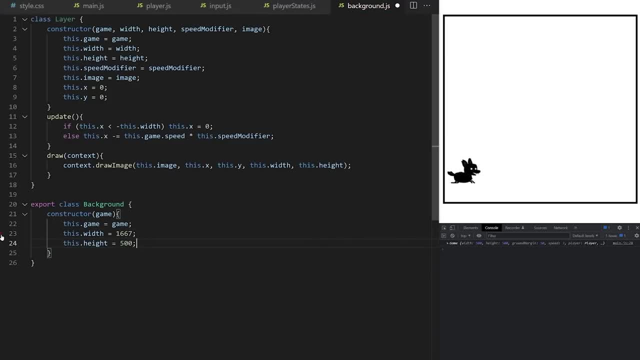 I made those images the exact size we will draw on canvas for performance optimization reasons. You can also use larger images and you can scale them down with code, but that will take more computing power and it can affect the FPS of your game. Let's bring all 5 images for our layers into the project. 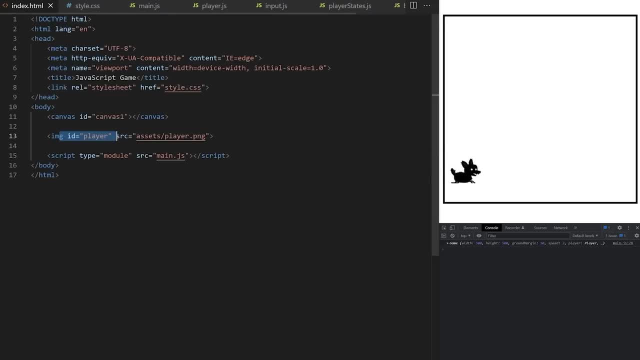 This layer5 image is equal to layer 5.. If you downloaded the project images And placed them inside your assets folder, You can go ahead and, inside indexhtml, bring them into the project Image element with an id of layer 5 and source assets. slash layer dash 5 dot png. 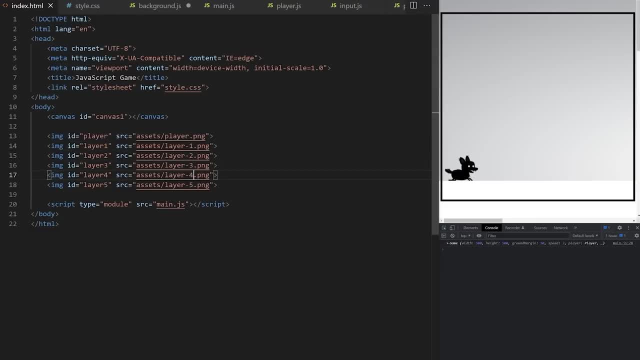 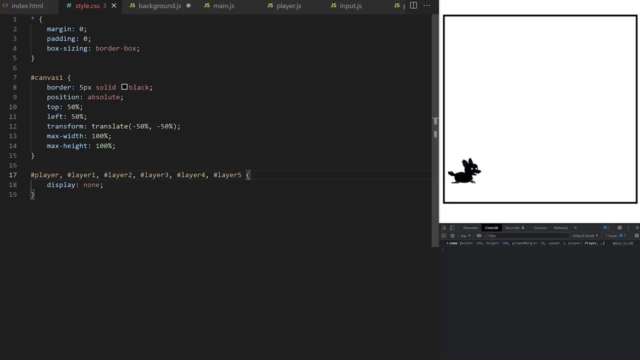 I also bring layer 1,, 2,, 3,, 4, 5 like this In style css. I give all of them display none. We don't want to draw the actual image elements on the website, We want to draw them on canvas. 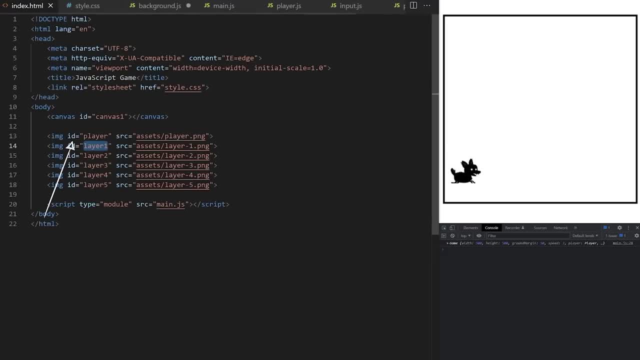 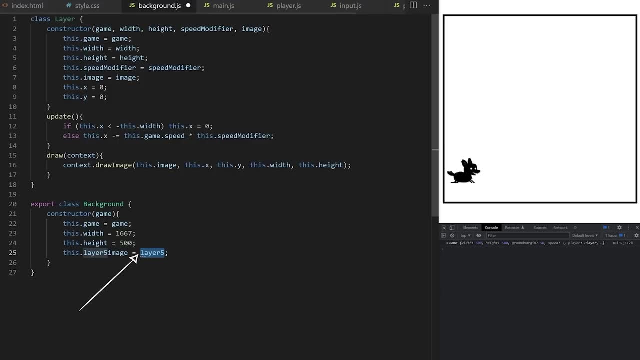 As I said before, Javascript automatically creates references to all elements with an id in the global namespace, So I can just pull the images in using its auto generated variable name like this. It would work like this, but I noticed more people are comfortable using get element by. 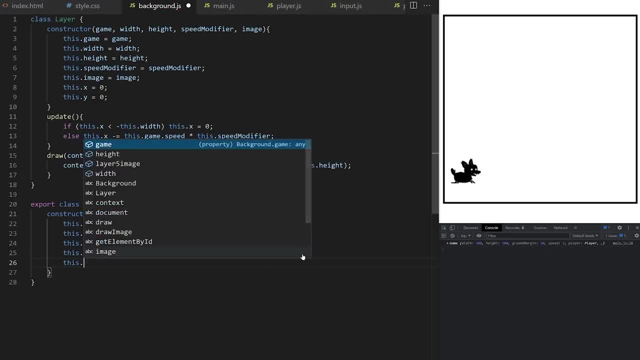 id in here, so I will do that. We will also need an array that will hold all background layers, so I create it here And here inside background class constructor. I will create an instance of layer class from line 1.. I call it, for example, thislayer1.. 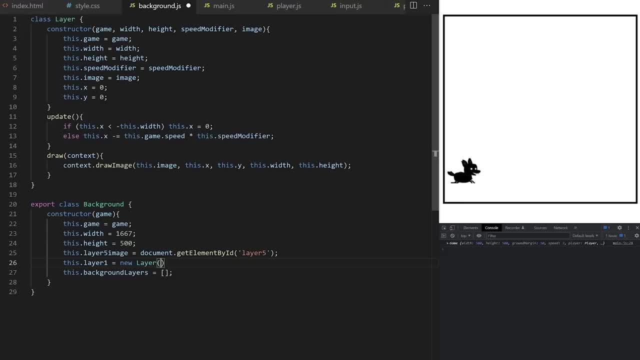 And it will be equal to new layer. You can see it expects 5 arguments, so I pass it. thisgame. thiswidth, thisheight speed modifier will be 1 for now and the image will be thislayer5 image from line 25.. 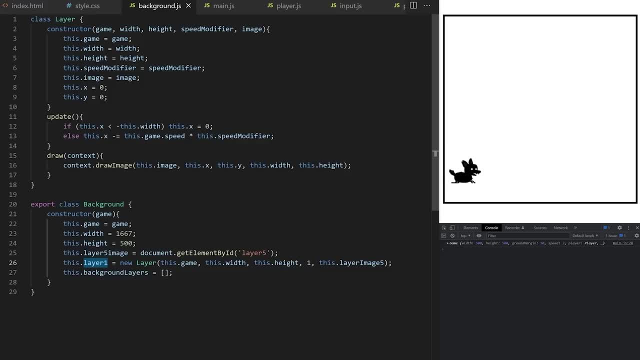 Now we have one instance of our layer class. Let's put it inside background layers array. I give it update method and inside I take that background layers array and I call for each array method on it. For each layer object in the array, I call its associated update method. 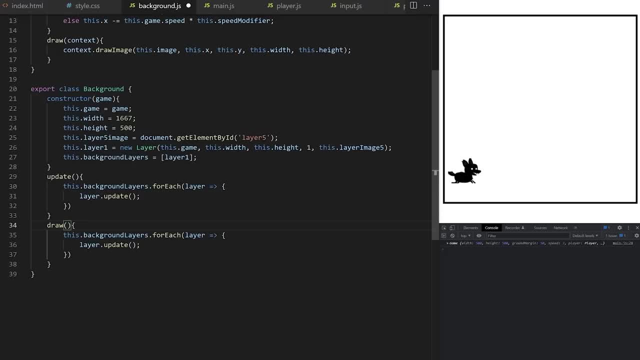 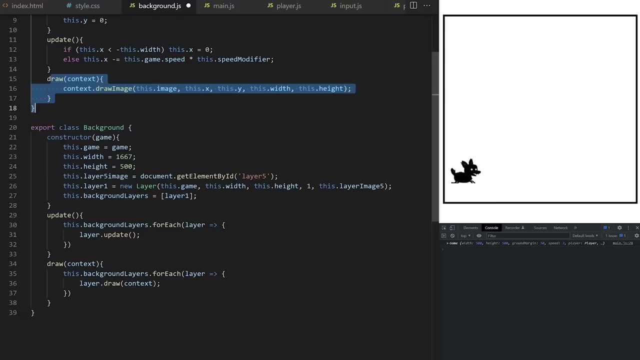 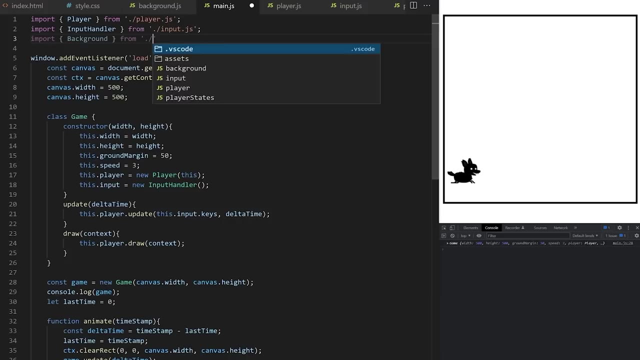 I also do the same for draw method And I pass it context because we know it expects it up here on line 15.. Let's see if it works. I import the new background class up here in mainjs. I instantiate it inside game class constructor. 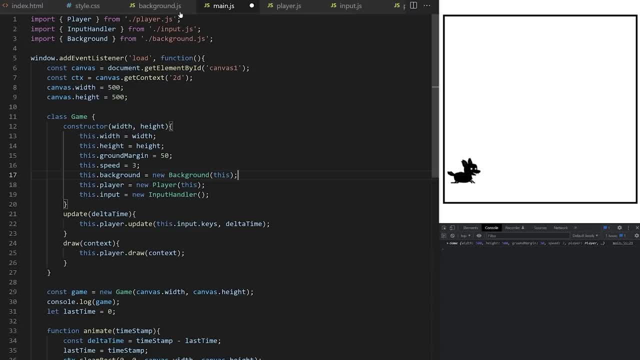 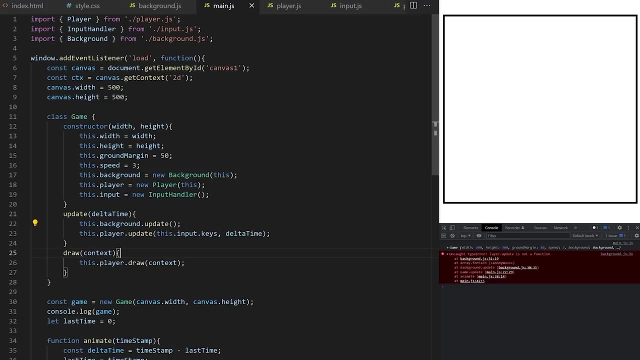 And I pass it this key As a reference to the entire game object because I know it expects it here. I have my background now so I can call its update method. I get an error? We will fix that in a second. I will also call draw method on the background. 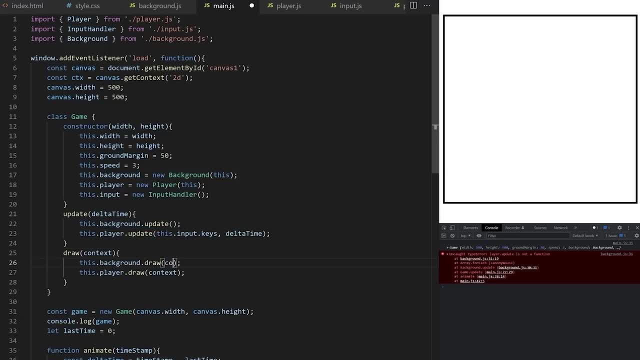 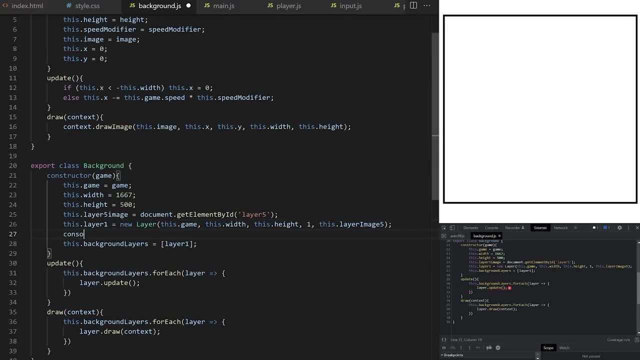 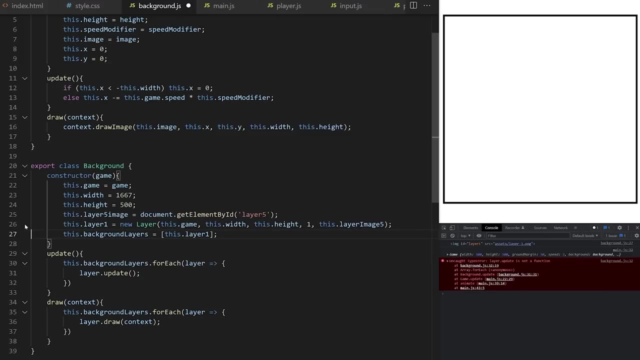 And I call it before I draw the player, because I want the background to be behind the player And I pass it context. So we have an error somewhere inside our background class. The first typo I made here. I already noticed. I need to use this dot here to correctly point to the instance of layer class. 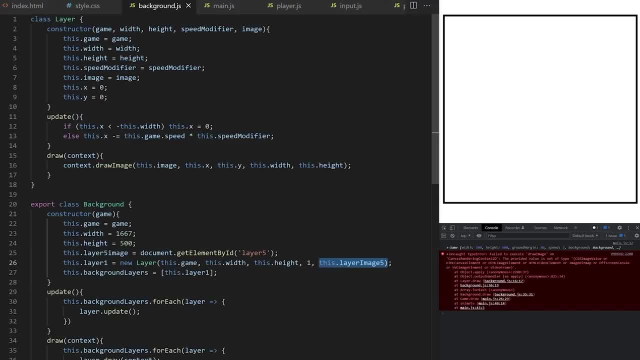 Now we get draw image error. so I know something is wrong with the way I'm linking my image. If I check here I can see I misspelled the name. It's supposed to say this: dot layer 5 image. Nice, We are animating our background layer. 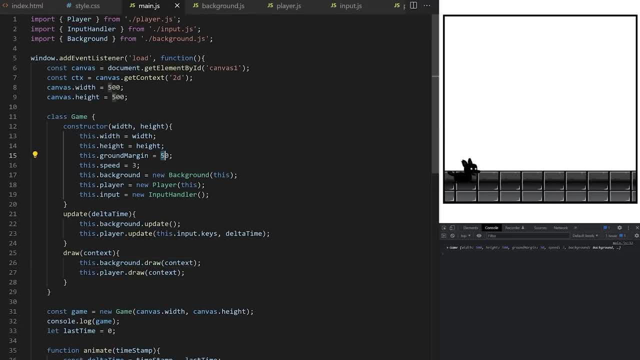 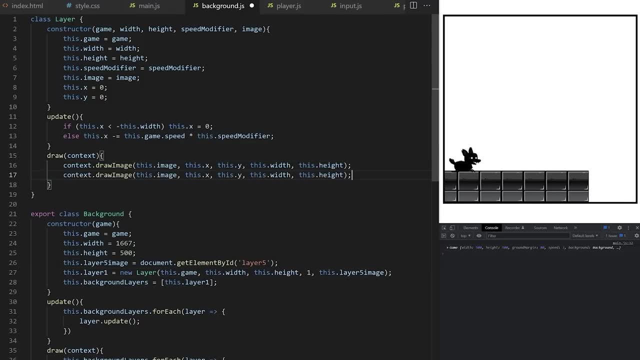 I can adjust ground margin to move the player a bit up to match the background artwork. The trick to create seamlessly scrolling backgrounds is to draw the same background layer on the same image twice next to each other, So one at the position x and the other at the position x, plus this dot width like this: 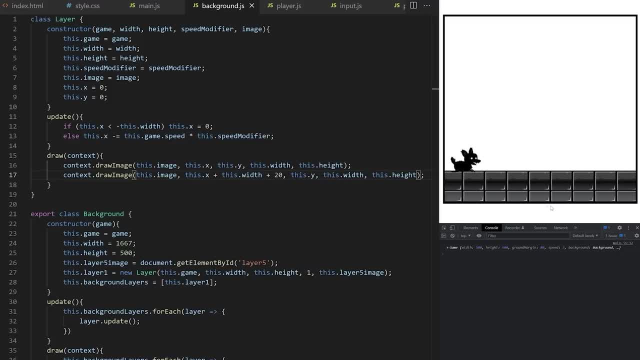 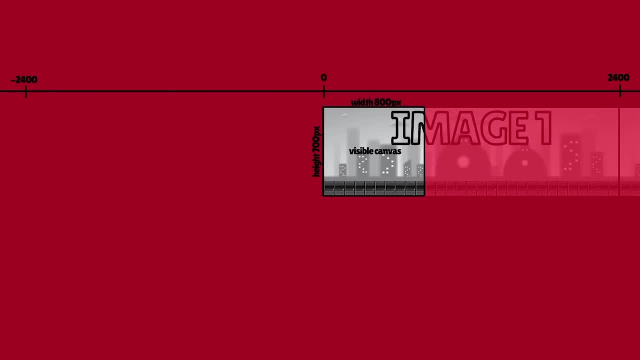 I give it additional plus 20 so that we can see where the second one starts Here. So what is happening here? We have two identical images scrolling side by side. When the main image 1 scrolls all the way off screen, we quickly reset it so that it. 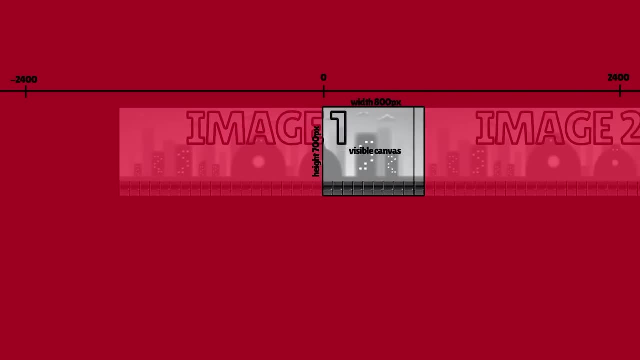 can scroll again. Image 2 is never fully visible. It's just there to fill the left half of the screen. It's just there to fill the left half of the screen. I'm just going to go ahead and select Gap before the first image has a chance to reset. 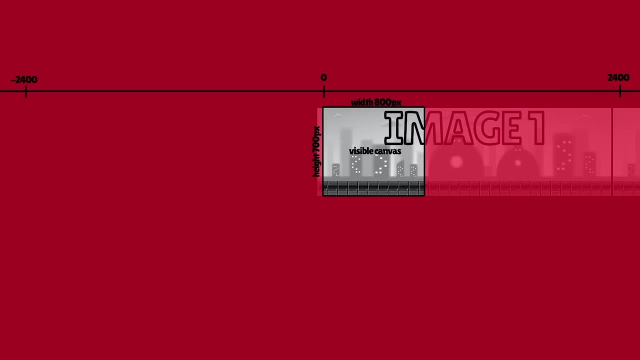 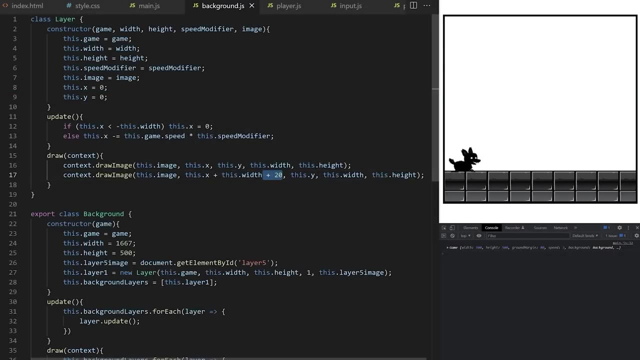 I hope this visual makes it clear what's happening And now you know the secret of endlessly scrolling seamless backgrounds. It's easy: Let's make them parallax, which means it has multiple layers that move in slightly different speeds to create an illusion of depth. 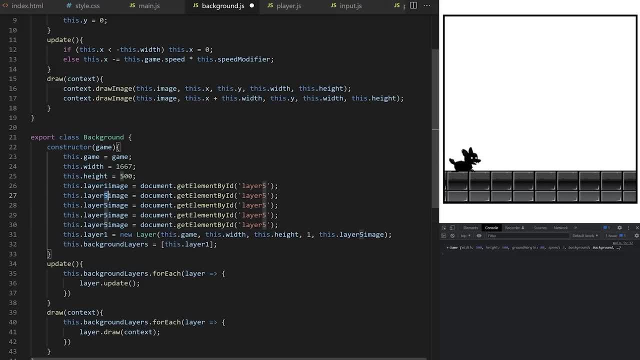 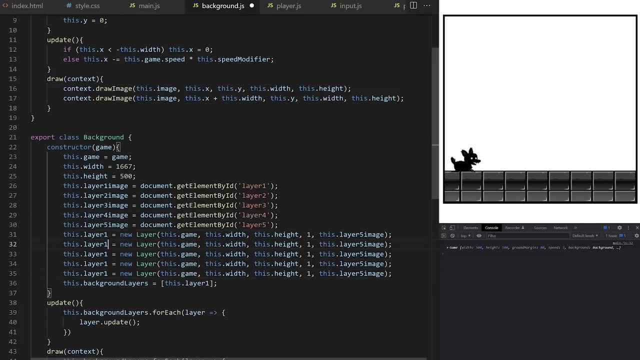 Of distance. I already brought those images into our project in indexhtml, so I just turn them into class properties here. I instantiate each layer class with its associated image. This will work as well. image. I put all those layer objects inside this dot background layers array so we can cycle. 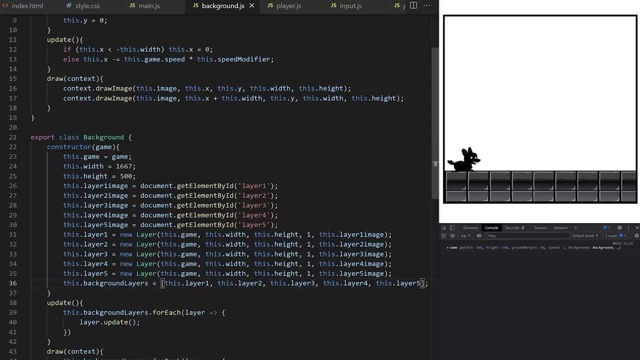 through all of them at once, using for each method Inside update and draw. Now we are animating all layers at the same speed. I can give them different modifiers. Layer 1 is just gray sky. no need to move it at all, so its speed will be 0.. The speed of layer 2 will be game speed times 0.2,. layer 3: 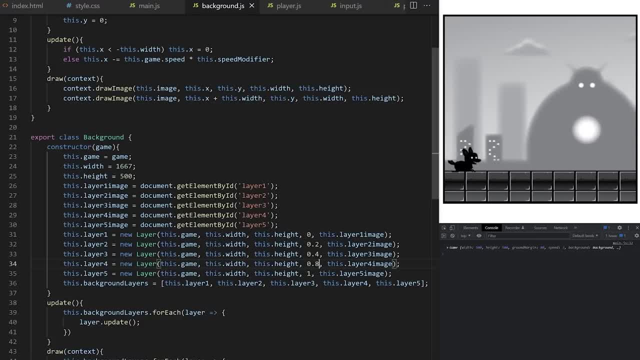 is game speed times: 0.4, layer 4 will move at 80% of the current game speed and layer 1 will move at the same speed as the actual current game speed. Perfect, You can see that if I change the modifier. 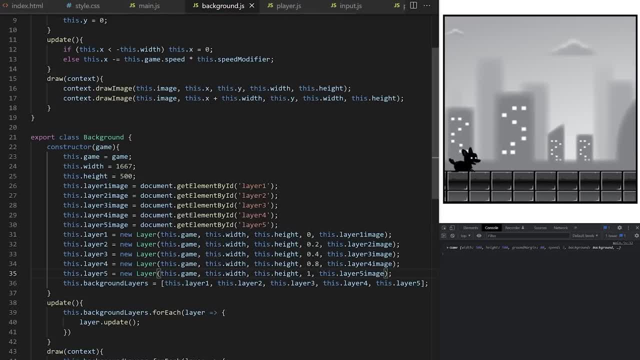 even higher. it gives us faster scrolling. Since we connected everything to the current game speed, I can change the scrolling speed of the game When the player switches to a different state. Maybe. I want the game to stop scrolling when the player sits down and I want double scrolling speed when the player does a special attack or a roll. 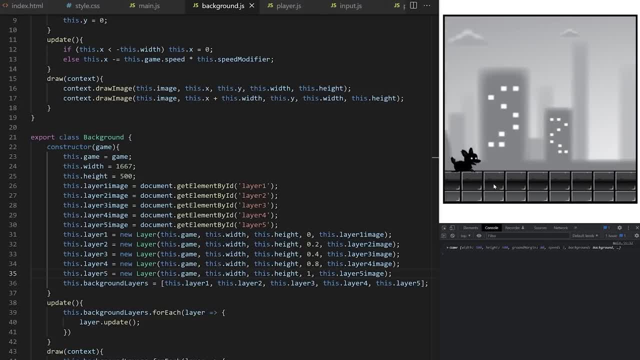 There are many ways how we can structure the code. at this point. I can either bring a reference to the main game object into player states so that we can manipulate game speed property from there, or I can, for example, do it from within set state method on player class, because from there. 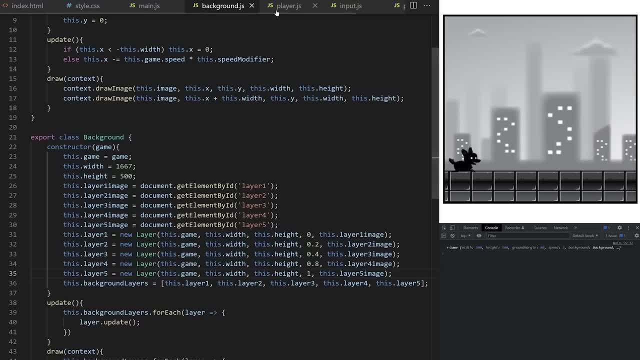 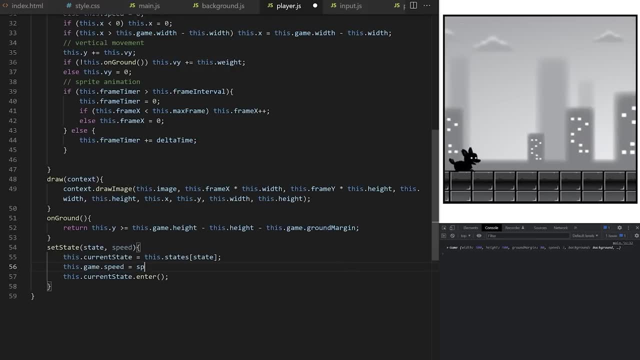 we already have access to game speed. I will give set state to the game object and I will give set state to the game object. I will create a second argument called speed. Inside I set speed property on game object to the speed value passed as an argument. 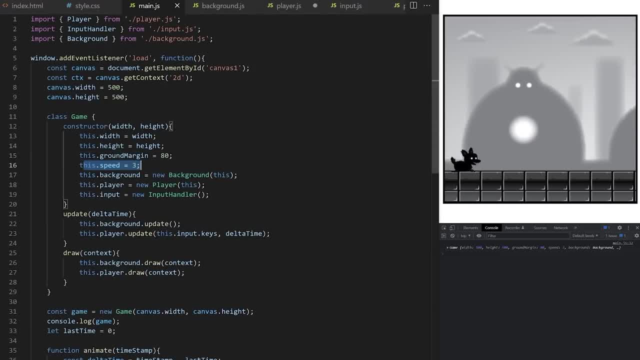 At first the speed of the game is 3 pixels per frame. Since we start in the sitting state, the initial game speed should be 0. In player set state. whenever I set state, I will also set game speed. I might refactor this later. maybe it's not the best solution, but it should work. Let's see. 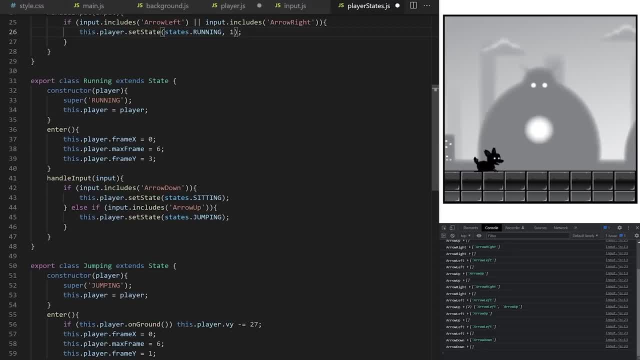 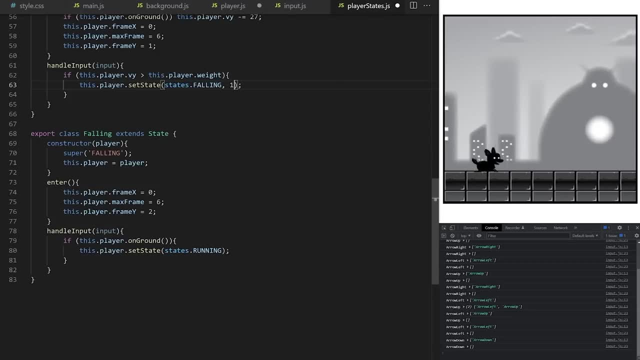 When we are running, game speed will be 1.. Sitting game speed: 0. Jumping game speed is 1.. Falling also: 1. Running: 1.. I save all unsaved changes in all my files. Now. the game stops scrolling when we sit and it starts scrolling again when we start moving. 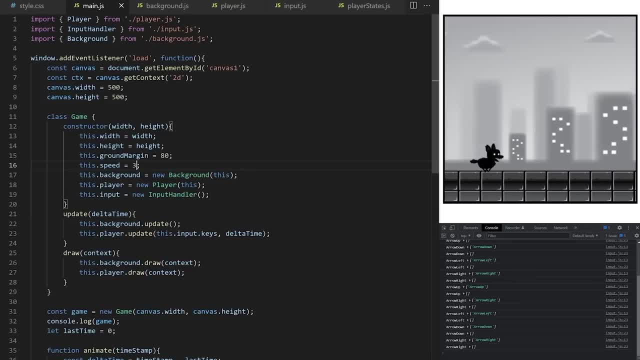 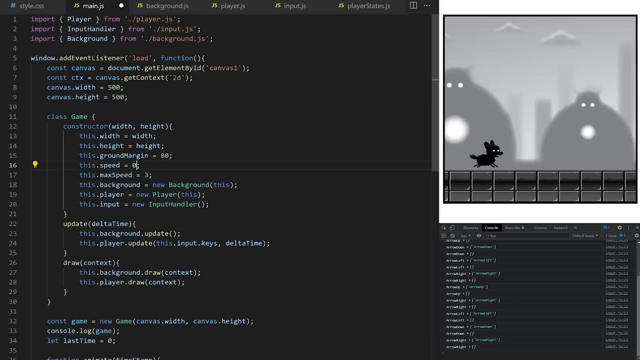 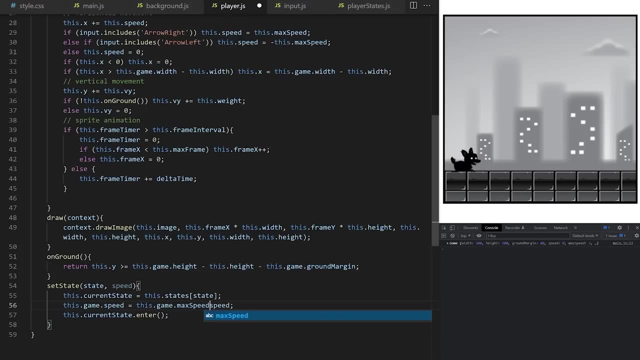 We can refactor this to make this code a bit better. On the game class, I create a new property called thismaxSpeed and I set it to 3.. I set thisspeed to 0 at first. Inside set state we set the current speed to max speed times- the speed that was passed to set state. 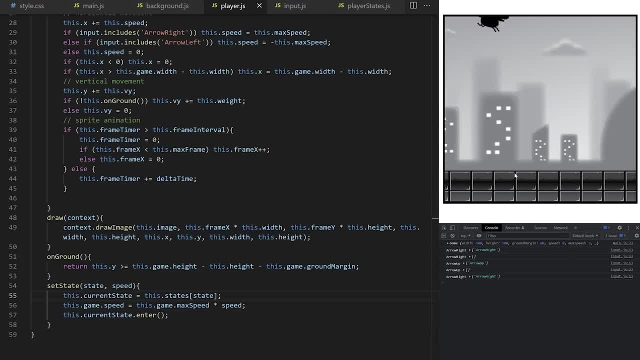 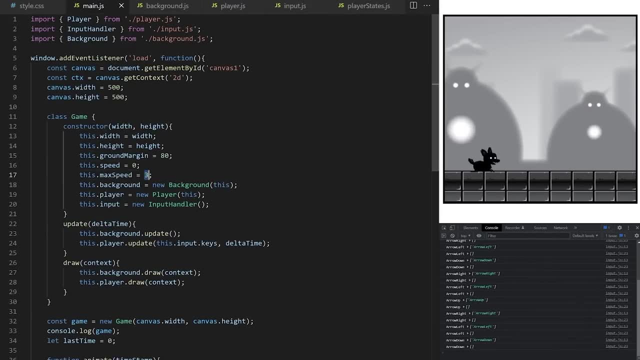 That way I can adjust the actual game speed by adjusting just the max speed property on the main game class, Rather than adjusting the values we passed to set state in all those places in player statesjs. Now we have quite a lot of logic going on. If you are a beginner, well done. You should be really proud of yourself if you manage to follow along. 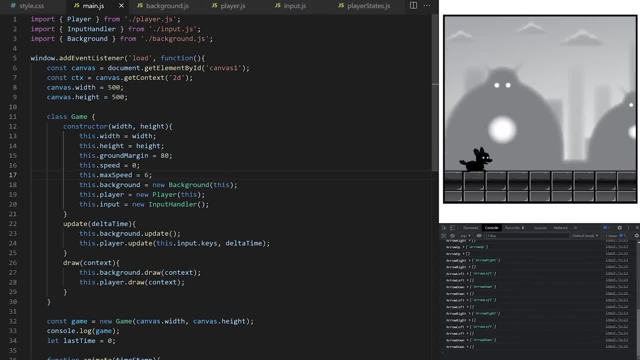 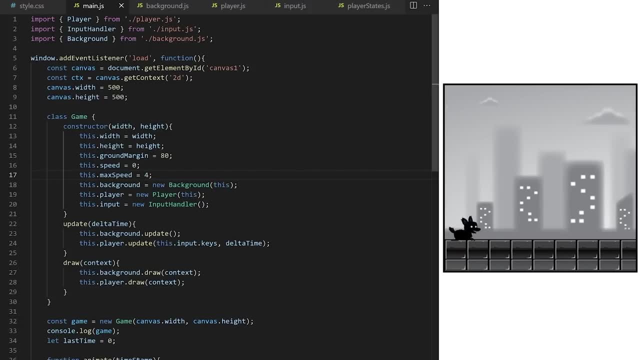 This was the most complicated episode in this episode. The rest will be relatively easy when you understand the tips and tricks I'm about to reveal. It's important that player feels like they have control over the character. Quick, responsive controls add a lot towards positive user experience. 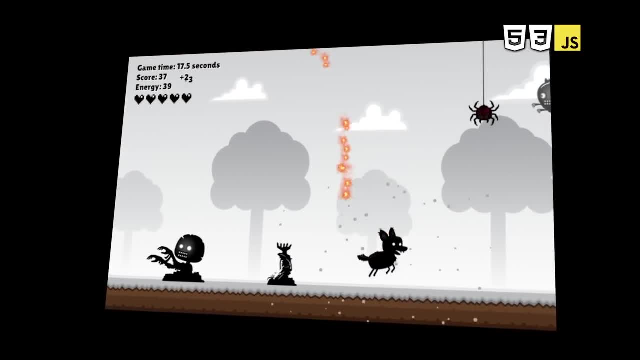 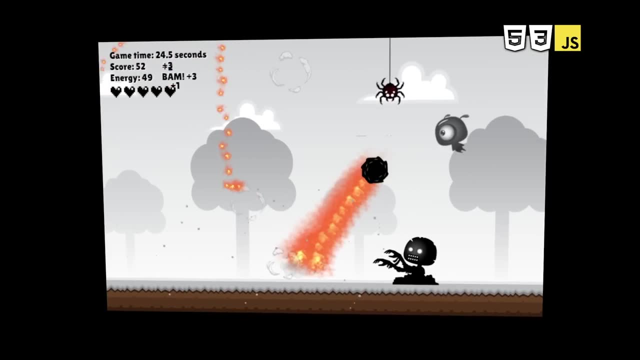 We are building a fast paced animated 2D game with plain vanilla javascript and HTML canvas element. We applied state design pattern to animate our player. We have endlessly scrolling parallax backgrounds where scrolling speed reacts to player movement. Today we will learn how to do this. 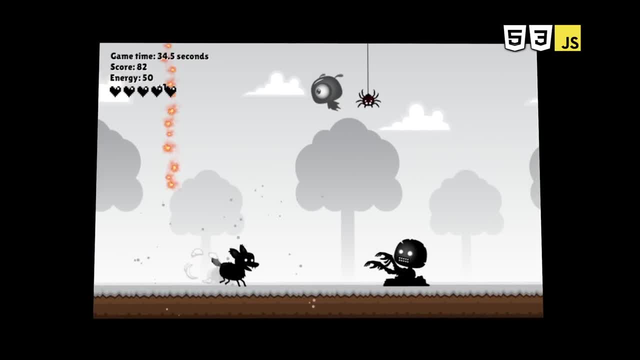 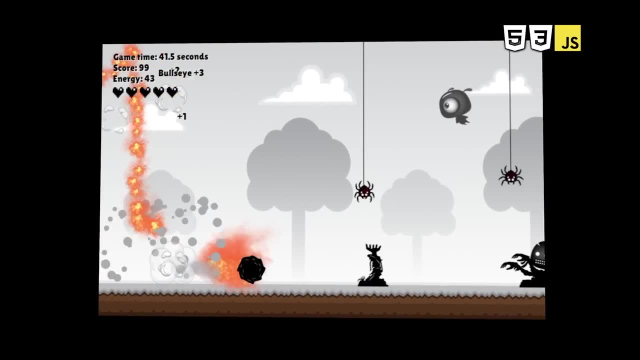 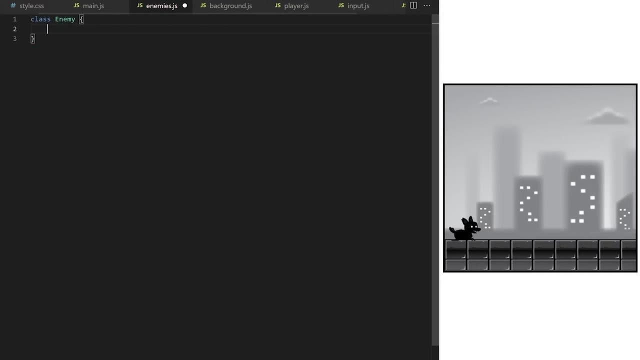 We are going to make our game more fun by adding three very different enemy types. Are you ready to take our dog for an adventure and help it find its way home while avoiding enemies and creatures of the dark? Let's go. I create a new file called enemiesjs and inside we declare a custom javascript class. I call, for example, enemy. 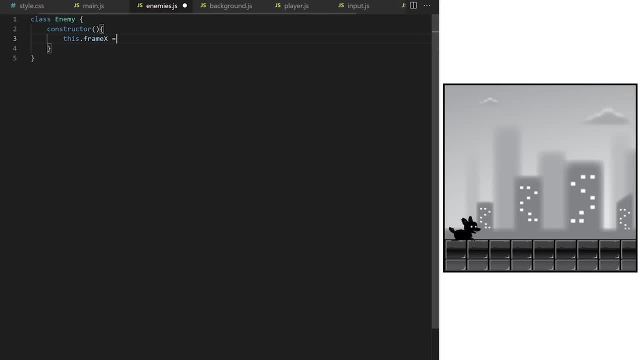 I will have a constructor and inside I declare thisframeX, which will handle horizontal sprite sheet navigation, And frameY will navigate in sprite sheet vertically. The sprite sheets we will be using are optimized for 20 frames per second, so we will control them with timestamps and delta. time again. 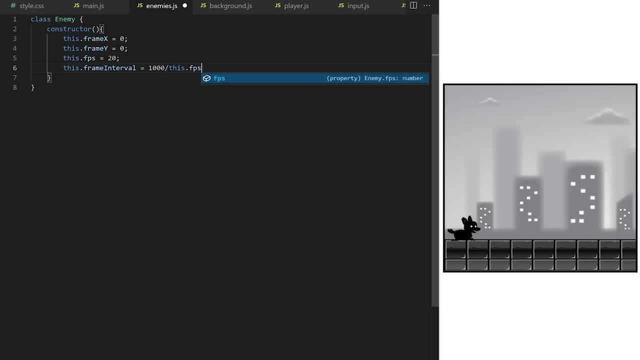 So three helper variables: FPS, frame interval and frame timer. It will work exactly the same as it did in player class. We will also need update method to move enemies around and draw method to actually draw their sprite sheets. I want to create multiple different enemy types. 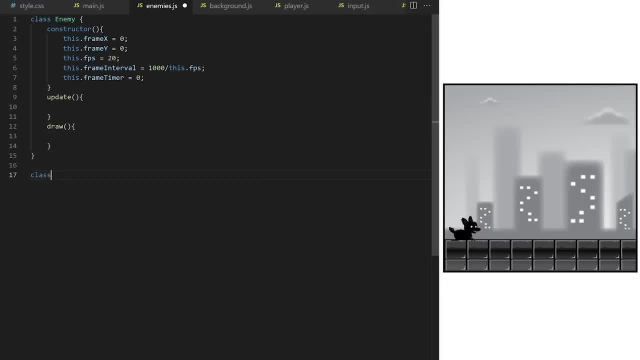 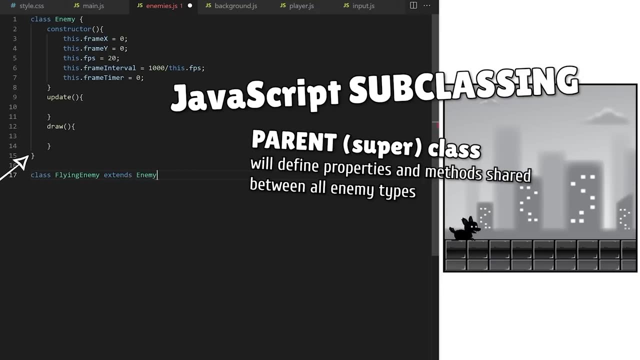 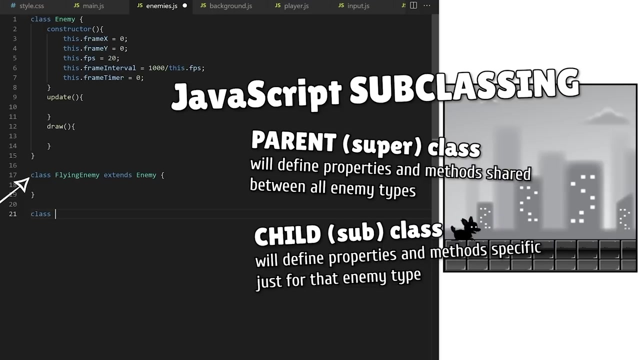 To keep our code organized and easy to navigate in, we will use javascript subclass, in which means we will have a parent enemy class that will define properties and methods shared between all enemy types and we will extend that parent class into multiple different subclasses. Each subclass will have properties and methods, behaviors that are specific just for that enemy type. 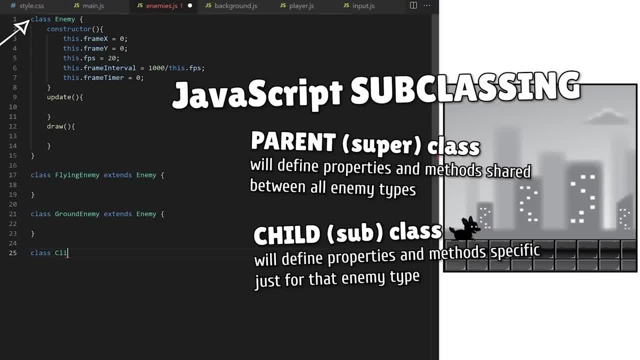 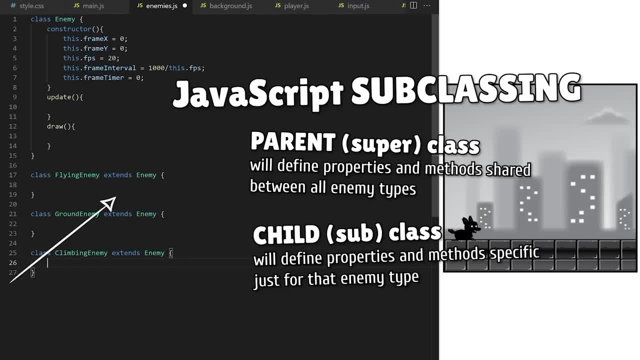 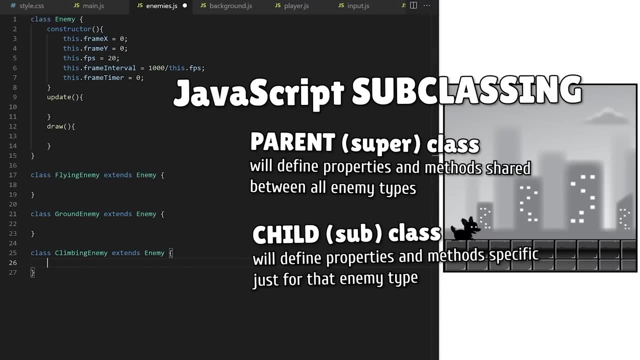 So enemy is so called parent class, also called a superclass, and we are using this special extends keyword to create three child classes, Also called subclasses. Javascript actually doesn't have classes. this is just syntactical sugar. Modern, cleaned and simplified javascript syntax. 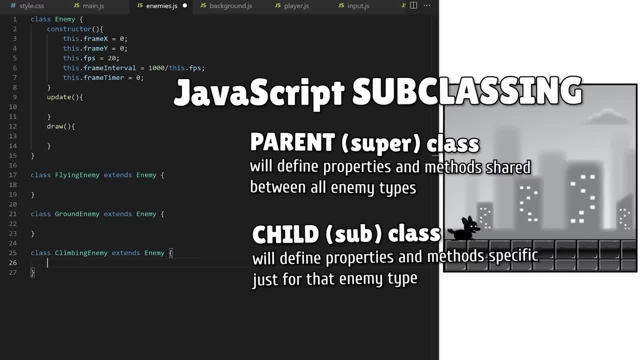 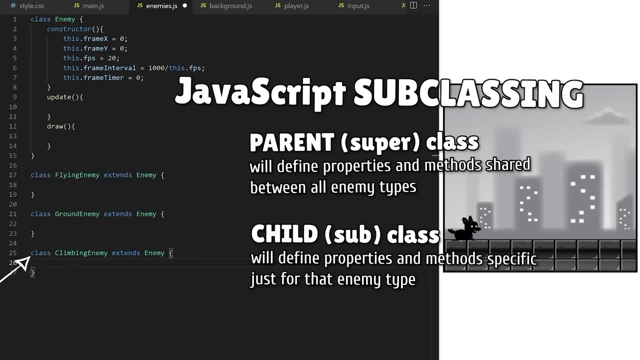 Behind the scenes. this code is just setting up prototype chains using javascript inheritance. It just looks cleaner and easier to navigate in if you write your code this way. So we have a parent enemy class and three child classes called flying enemy, ground enemy and climbing enemy. 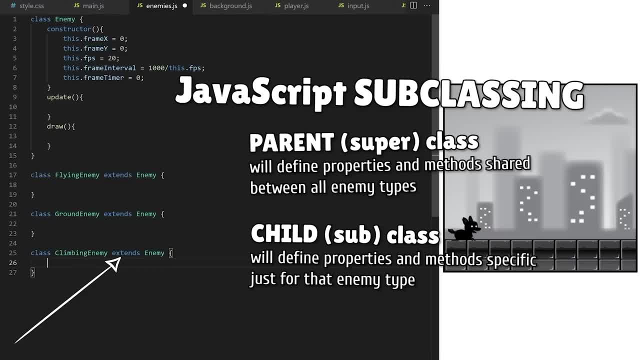 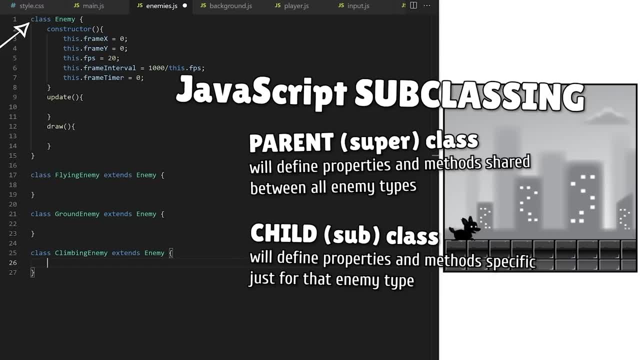 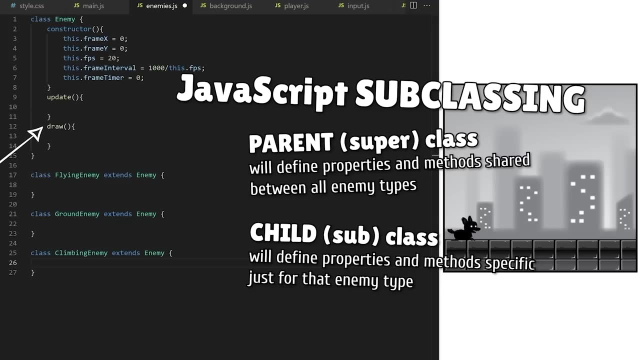 All three child classes are using extends keyword pointing towards their parent enemy class. This will automatically set up prototype chain behind the scenes and all these classes will have access to properties on their parent class and also to this update and draw method. That way, we can avoid code repetition. 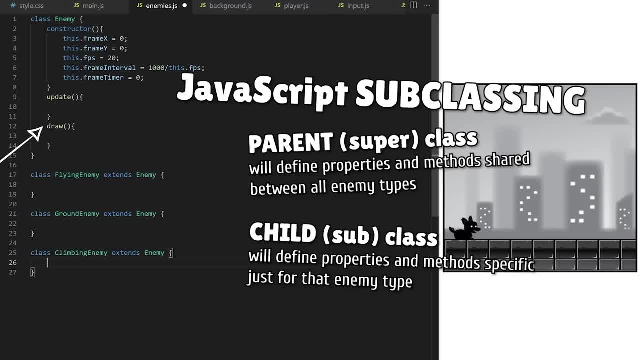 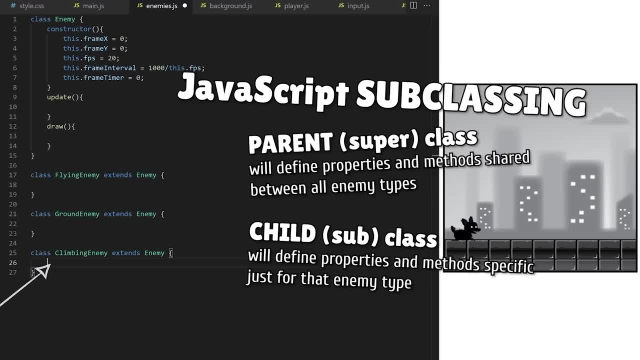 and we don't have to redeclare methods and properties that are shared across all enemy types. Inside each subclass, we will only define what's unique about them. I will show you exactly how this works, as we create three unique enemy types with very different behaviors and movement. 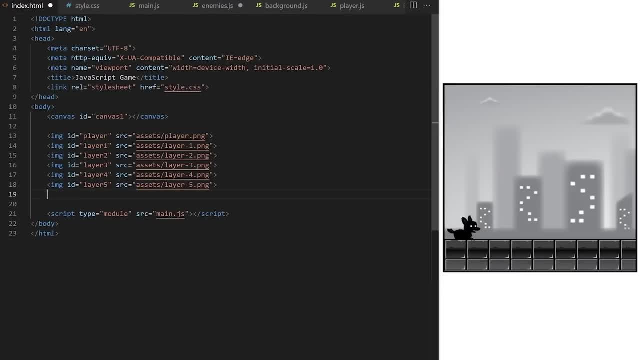 Click the like if you are getting any value. Let's start by bringing images into our project. In the video description I will give you sprite sheets for many different enemy types. For now, we will use just three of them. If you are a beginner, you should maybe use the same ones I'm using. 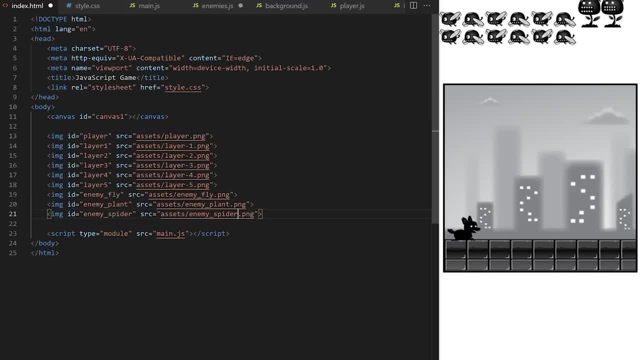 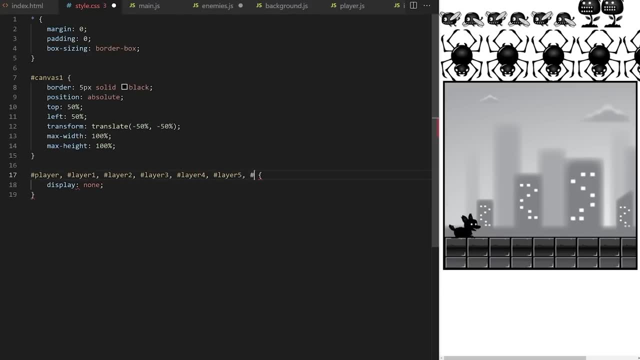 and when you have a fully working code base, you can play with it and use your own custom sprite sheets. We will use enemy fly, enemy plant and this big spider. I will hide images with CSS because we want to draw them with JavaScript on canvas. 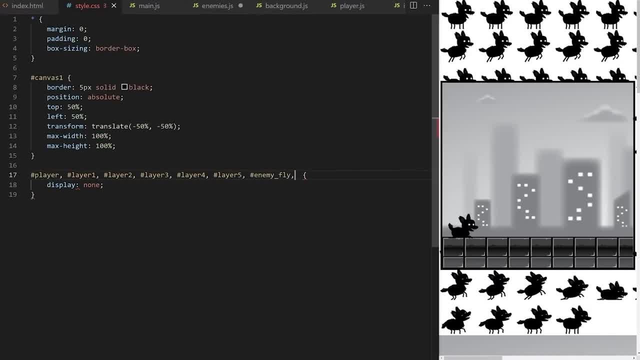 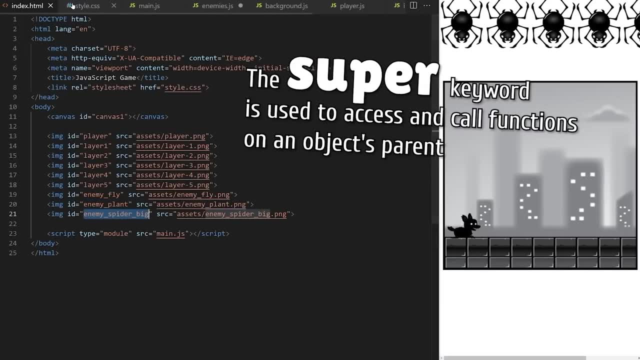 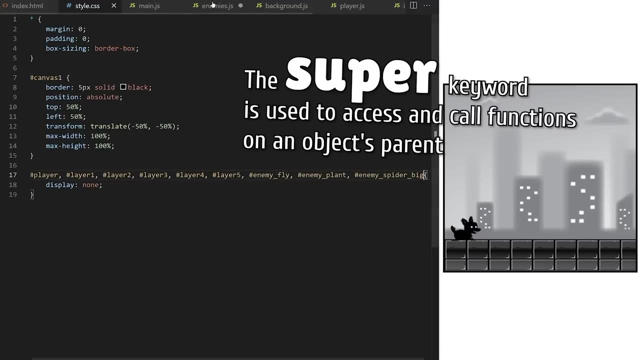 There is one more thing we have to understand when extending JavaScript classes. There is a special keyword called super. It's used in two different ways, because we can extend code from parent class constructor or we can extend a method from the parent class. I will show you how to do both, as we create different enemy types with different behaviors. 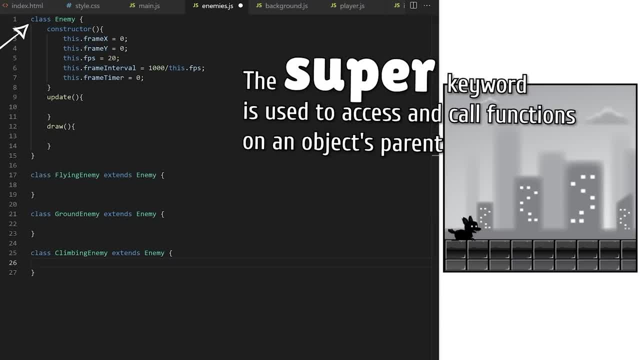 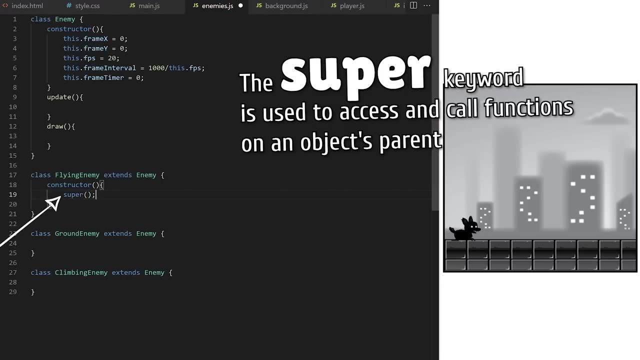 I have flying enemy subclass that extends this enemy super class. When I create a new flying enemy I want to run all this code from parent class And then I want to add some additional properties that are specific only to the flying enemy. I do that by first calling super, like this: 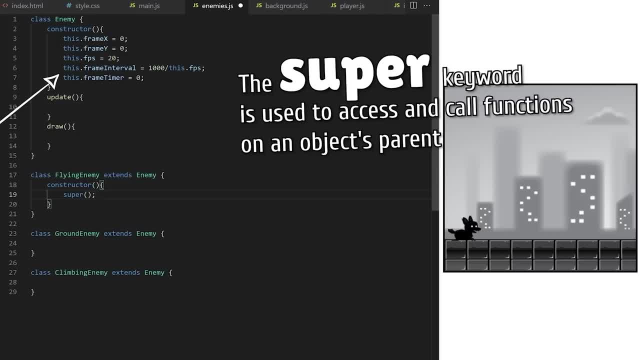 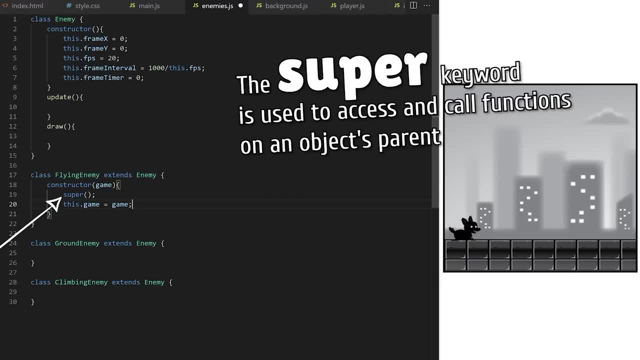 This will automatically run all the code from here While extending classes. I can only use this keyword after I used super. If I use this keyword before super, I will get an error. Flying enemies will need access to the entire game object because they need to be aware of game area, width and height. 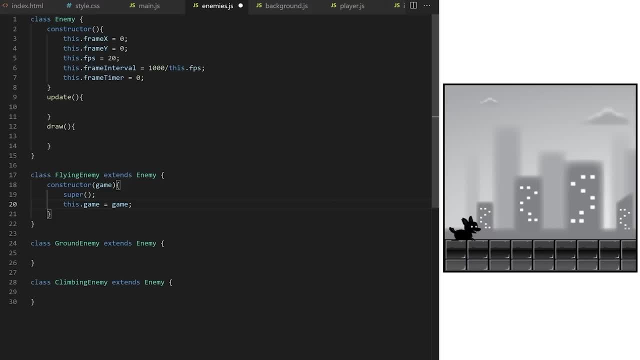 so that they know when they are off screen. I will pass game as an argument to the constructor here and I will convert it into a class property. as usual, Each enemy type will also need width and height, But because each enemy type has a different size, 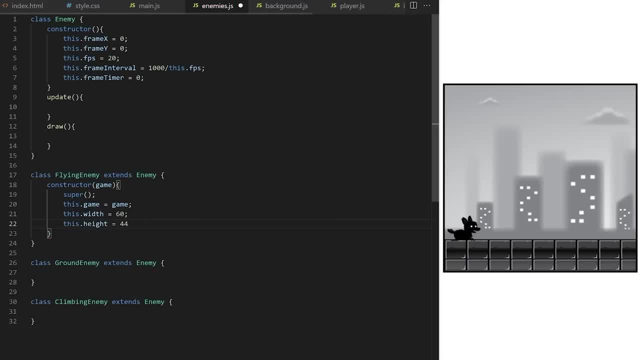 I couldn't put these values on the parent class. Width and height will be declared here. I look at my fly sprite sheet and I can see that the width of a single frame is 60 pixels and the height is 44 pixels. Each enemy will also need starting x and y coordinates. 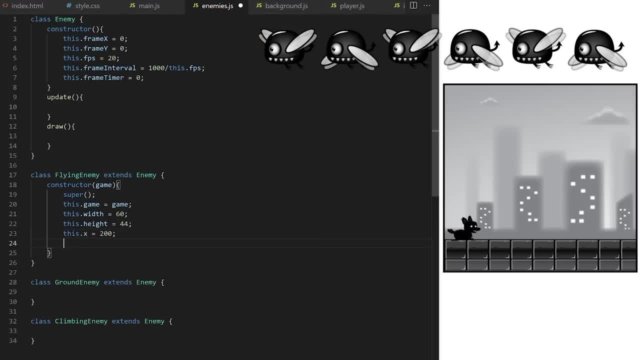 Flying enemy will start at a different position than a ground enemy, so x and y properties will also have to be on the child class, not on the parent class. Speed x will be horizontal speed and max frame on our fly sprite sheet is 5.. By the way, all my flying enemies will be flies for now. 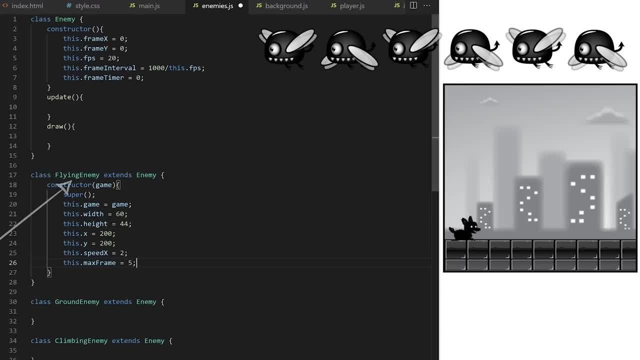 But I could also have multiple flying enemy types. I can have flying enemy class that extends parent enemy class and I can have bird fly and ghost classes that extend flying enemy class. We can go down multiple levels if we want to. In that scenario, flying enemy class would only have properties and methods. 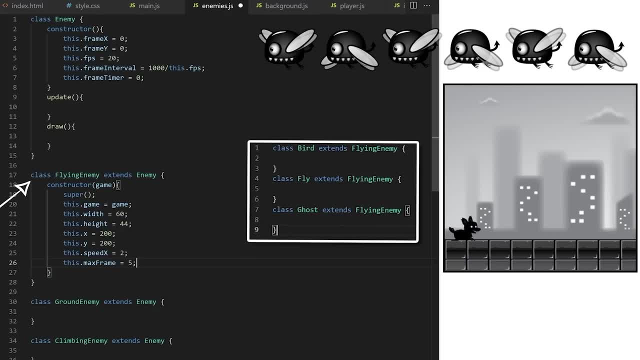 shared between all enemy flyers and things like width and height, speed, x or max frame would be declared separately on each subclass because each enemy will have different sprite sheet. We are keeping our code modular and well organized so that it's easy to make these changes later if we want to. 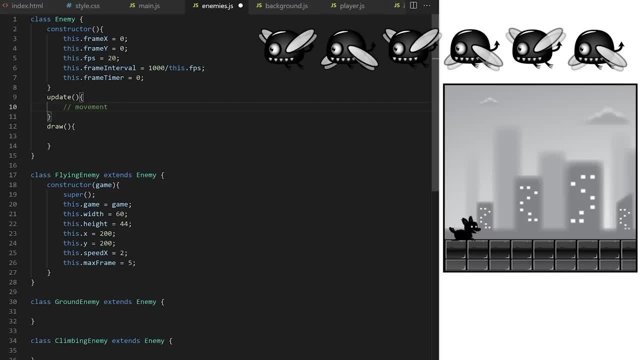 Inside update method on the parent class. we will handle movement For every animation frame. I want the horizontal x coordinate of the enemy to be increased by its speed x property. I will do the same for vertical y coordinate and speed y property. We will also handle cycling through sprite frames here. 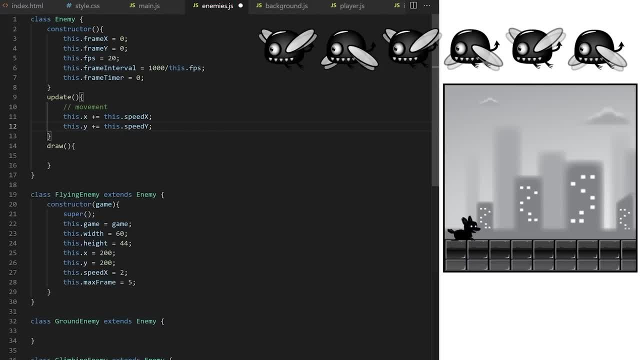 It will work exactly the same as it does for our player. sprite sheet Update method will have access to delta time difference in milliseconds between the previous and the current animation frame If frame timer from line 7 is more than frame interval from line 6. 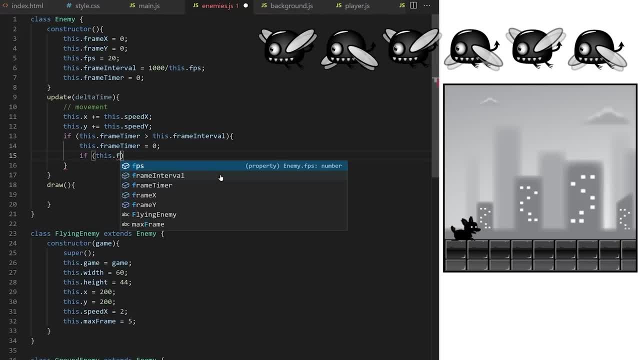 we reset frame timer back to 0 so it can count again for the next frame and we serve the next horizontal frame in the sprite sheet. Or if we are at the last horizontal frame, we reset back to frame x 0. Else meaning, frame timer is not yet higher than frame interval. 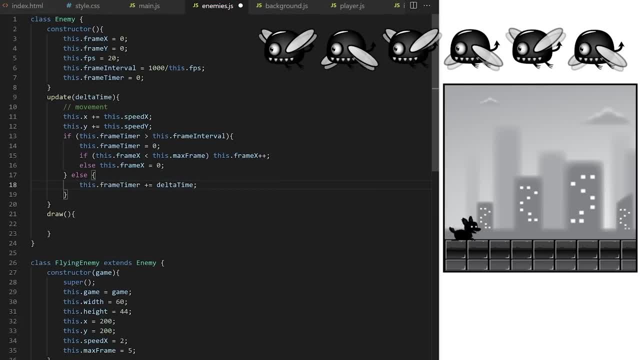 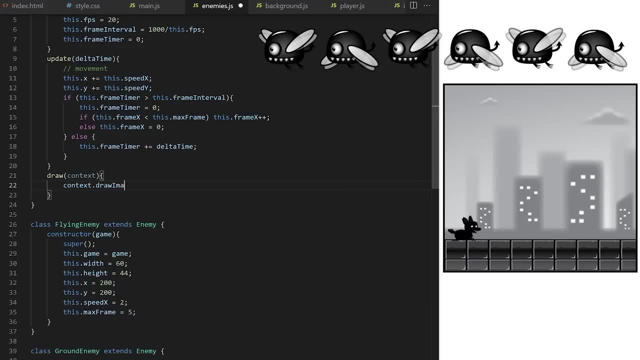 we keep increasing frame timer by delta time until it gets there. Draw method will expect context as an argument. Inside we will draw enemy sprite sheet using canvas. draw image method. It will need 9 arguments. The first argument is the image we want to draw. 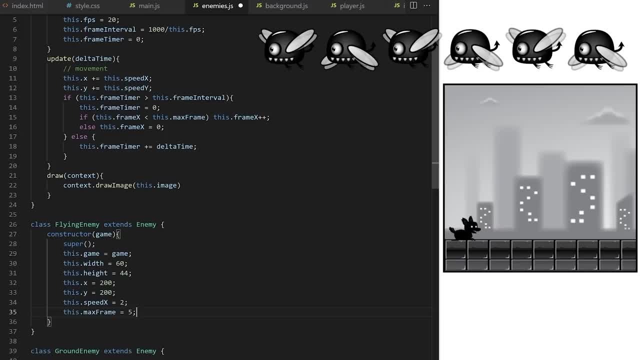 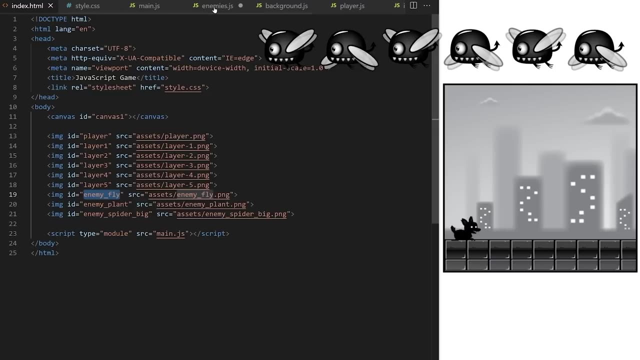 I will hold a reference to that image in thisimage property. Since each enemy type will have a different sprite sheet, it needs to be placed here. on fly in enemy class, I use get element by id and I will point it towards this img element with an id of enemy underscore fly from line 19 in indexhtml. 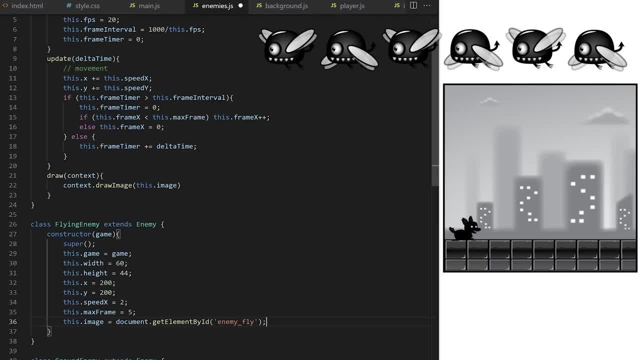 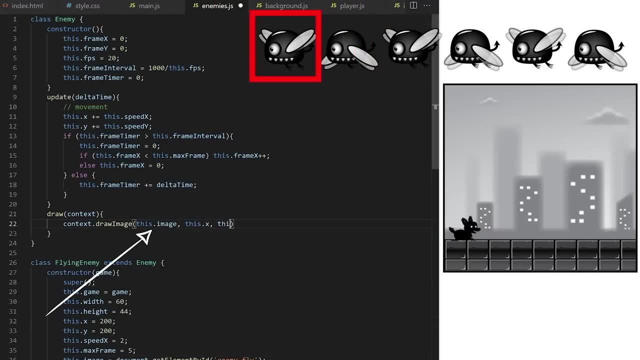 So draw image expects 9 arguments. in this case, The image we want to draw, Source x, source y, source width and source height of the rectangle we want to crop out from the source sprite sheet and destination x, destination y, destination width and destination height. 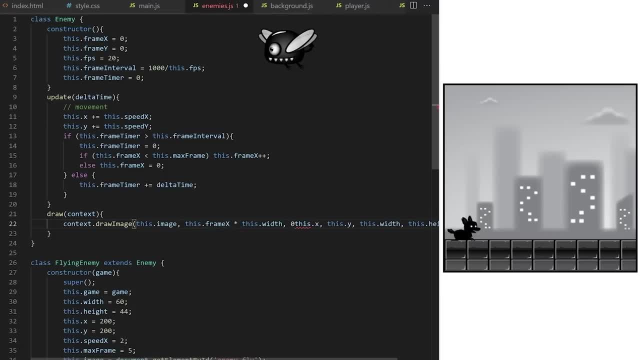 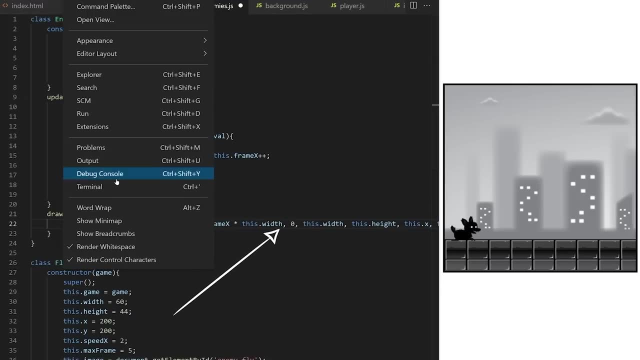 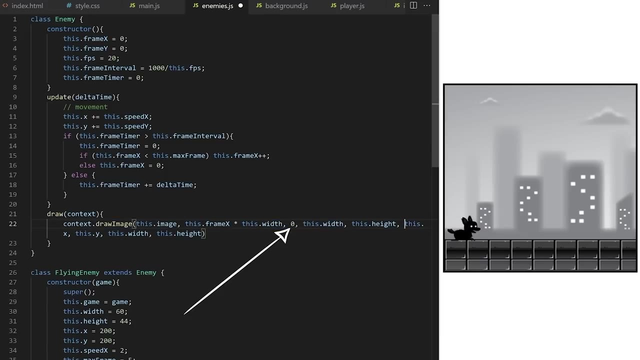 to specify where to place that image on destination canvas. It will work exactly the same as it does with player. We already explained before how frame x multiplied by the width of a single frame travels sprite sheet horizontally. Source y argument will always be 0 because enemy sprites will only have one row. 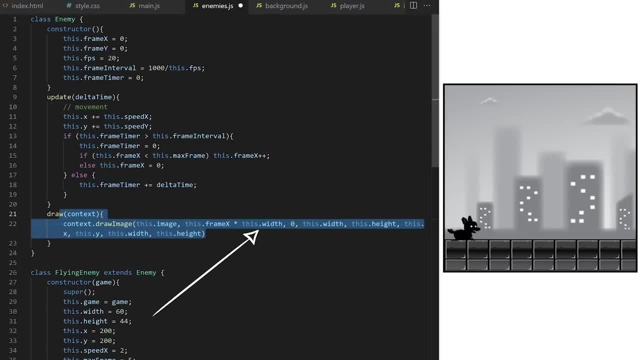 So we have image to draw. These four values define what to crop out. These four values define where to place that cropped out image on canvas. As I said before, we can extend parent class constructor using super keyword. We can also extend a method from a parent class. 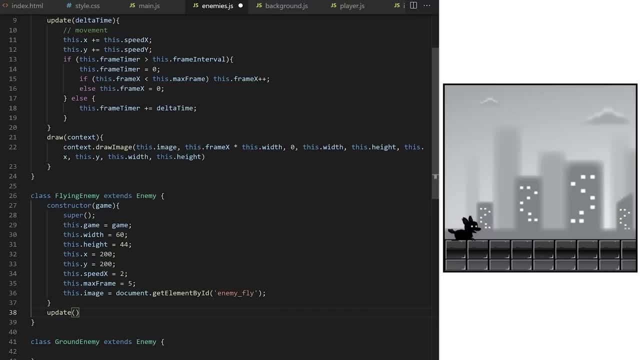 In this case I want to have update method on fly in enemy type. I want it to first run all the code from update method on the parent class and then I want to add a little bit of code that will be specific only for fly in enemies. 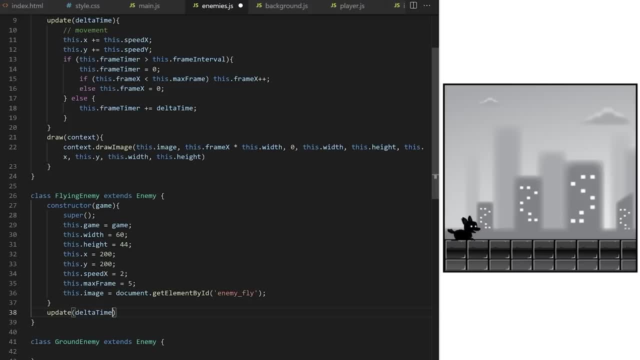 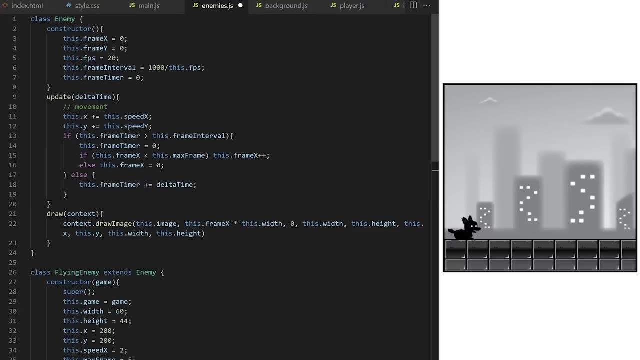 Update method will expect delta time. as an argument, I will call update method on the parent class from line 9 by saying super, referring to its super class, dot update and I pass this delta time long because it's expected here on line 9.. Doing that will first run all the code between lines 9 and 19.. 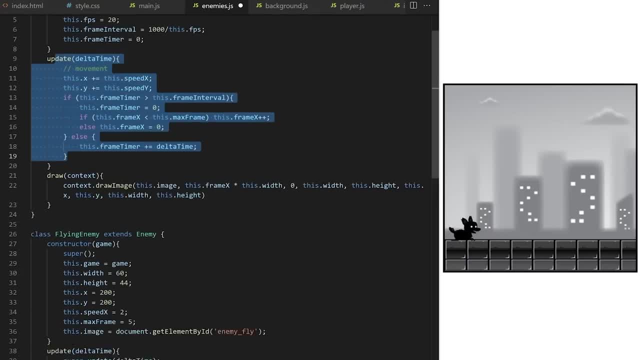 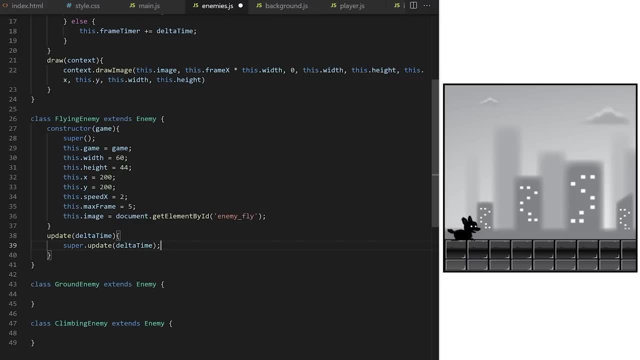 That code will be shared for all enemy types. After I run that code I will add a little bit of code that will be specific only for flyers. I can make them do so many different things here. I made a special episode focusing only on enemy movement patterns before. 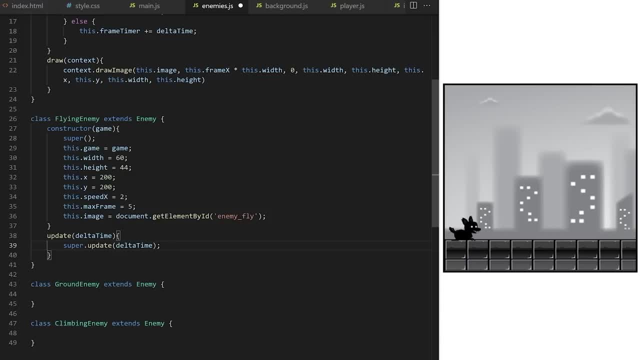 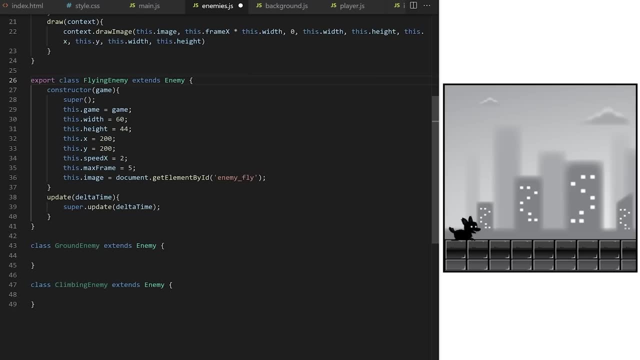 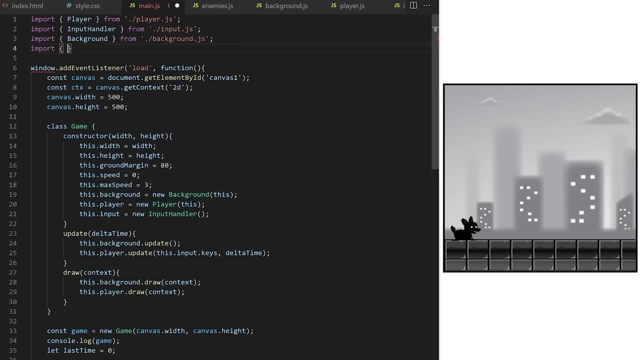 Let's just pick one. Maybe. I want vertical wavy movement. Before we do that, let's actually add some enemies into the game to see how the movement changes. Let's make sure we are exporting all our child classes. I imported them up here inside mainjs. 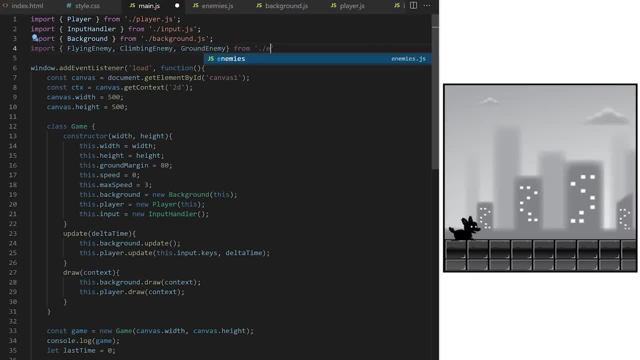 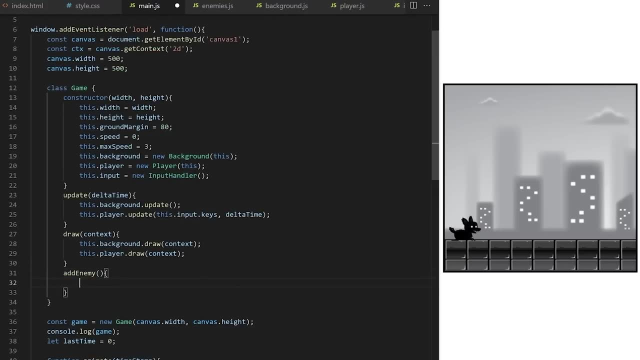 I want to periodically run some code that will add enemies in a specific interval. I will declare that code in mainjs In a special method on game class. I call it, for example, addEnemy. We will need some helper properties to build this functionality. 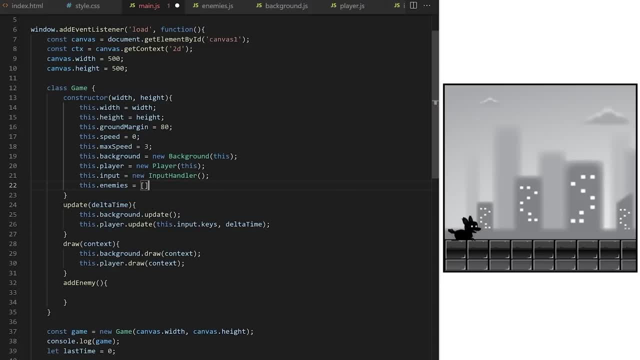 Thisenemies will be an array. It will hold all currently active enemy objects. Every time addEnemy method runs, it will take this array and it will use built-in JavaScript push method to push one new enemy in there. Push method adds one or more elements to the end of an array and returns the new length of the array. 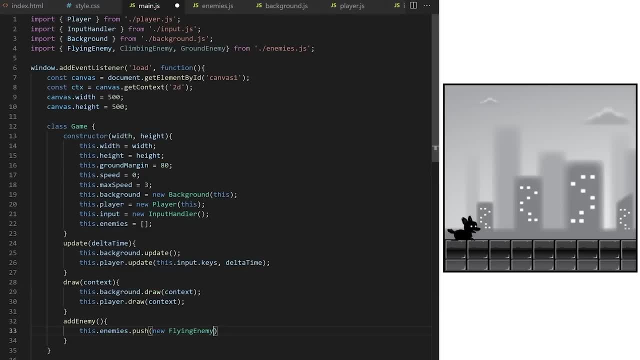 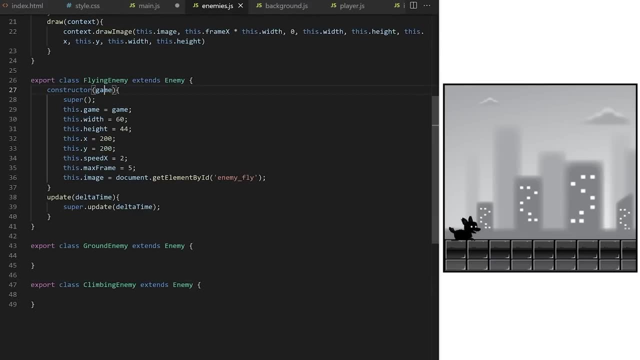 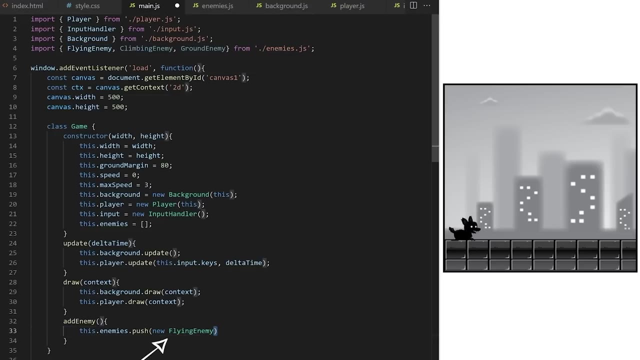 We want to push one new flying enemy. We are importing flying enemy class here from enemiesjs and here I can see flying enemy class constructor expects game as an argument. So down here in mainjs I'm creating an instance of flying enemy class and I pass it this keyword as an argument referring to this main game. object: 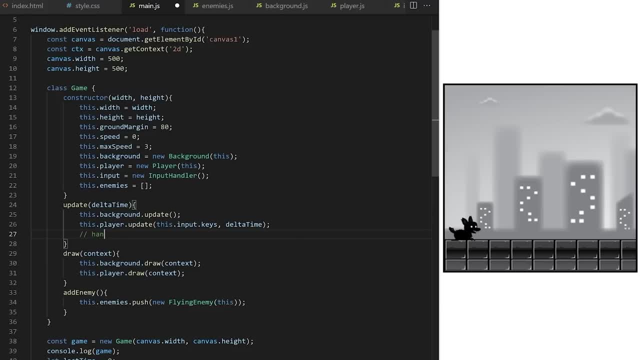 We will handle enemies here inside update method on game class, Similar to how we use delta time to periodically serve the next class In our sprite sheet. we will have timer and interval helper variables to periodically add enemies into the game. Enemy timer will start at zero. 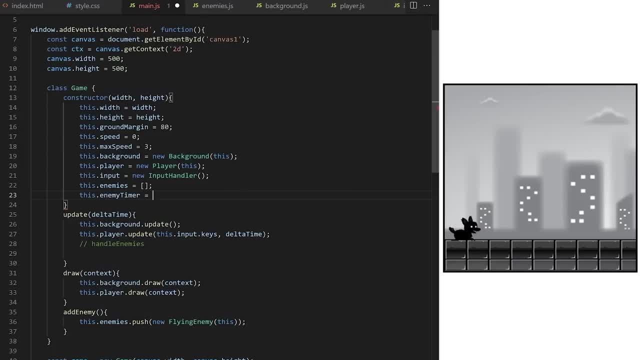 It will be increasing by delta time. Every time it reaches a value in enemy interval we will add one new enemy into the game and we will reset enemy timer back to zero. Let's say, I want to add new enemy every second, So thousand milliseconds. 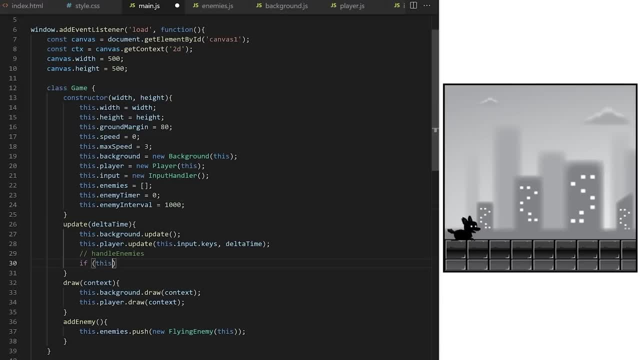 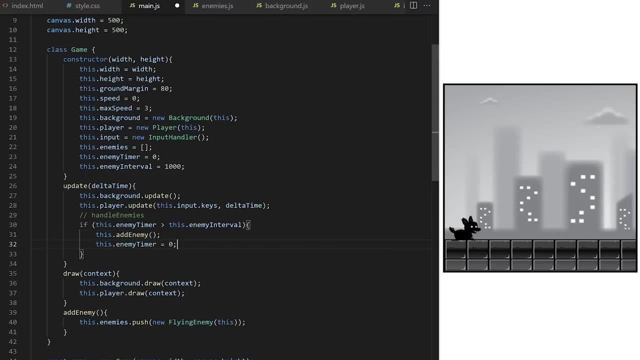 Let's write that logic in code: If enemy timer falls From line 23 is more than enemy interval from line 24.. Call thisaddEnemy custom method from line 38.. And also reset enemy timer back to zero so it can count again towards the next enemy time. 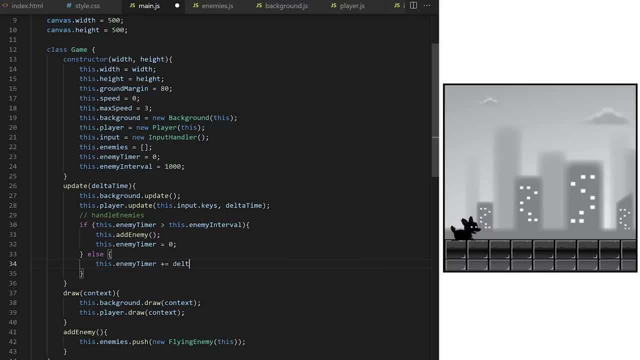 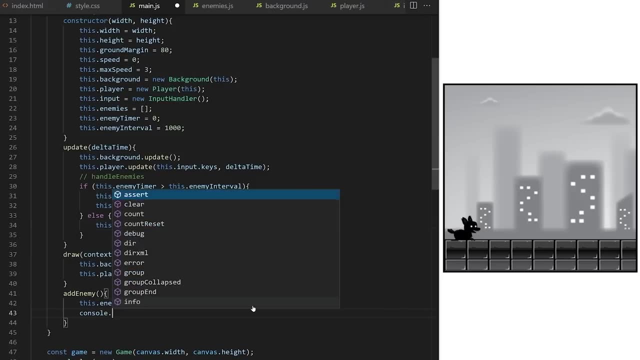 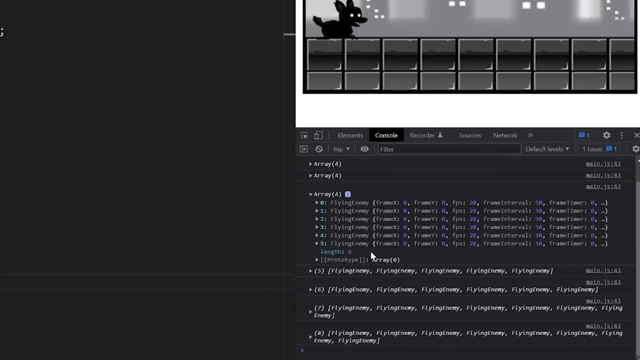 Else keep increasing enemy timer by delta time until we reach enemy interval again. Let's put a console log inside addEnemy to see if it's working. I will console log thisenemies array from line 22.. Nice, You can see as the game runs: every second one new flying enemy object is added into enemies array. 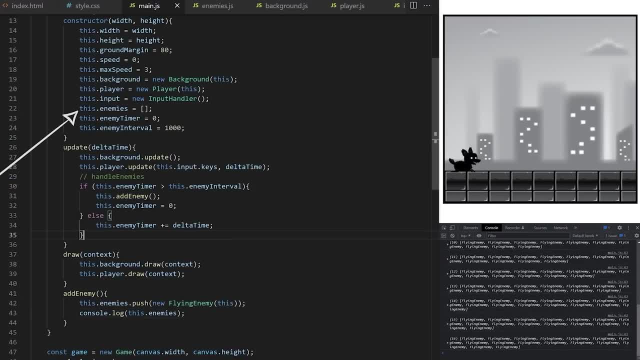 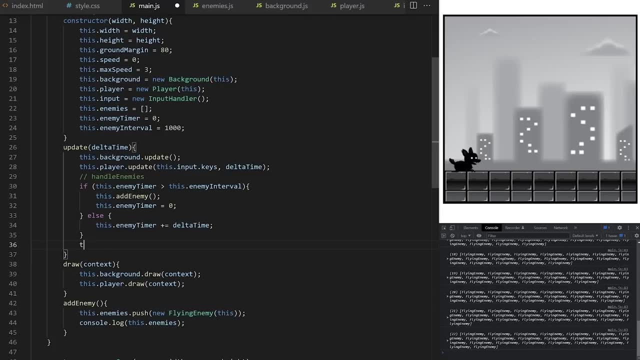 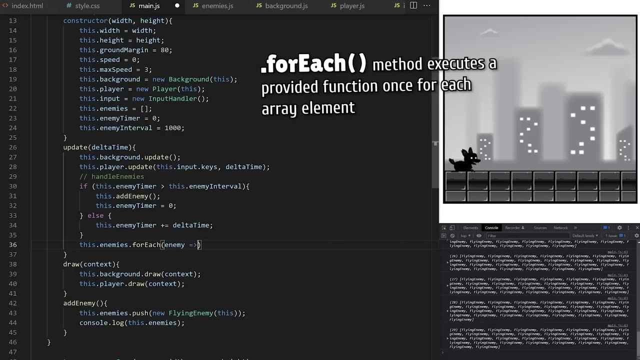 Perfect, So all our enemies are held inside thisenemies array. I will run through the array and I will trigger their update method to make sure they move around, For each method executes a provided function once for each array element. I will use fat arrow ES6 syntax here. 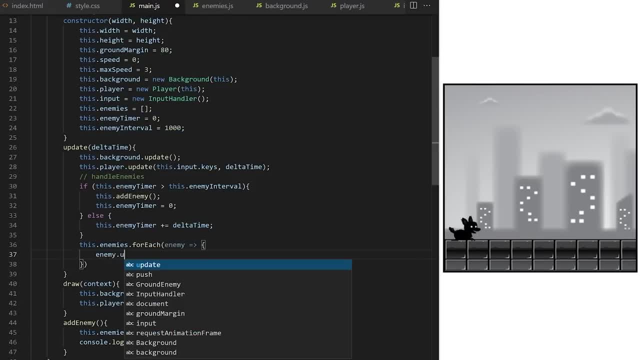 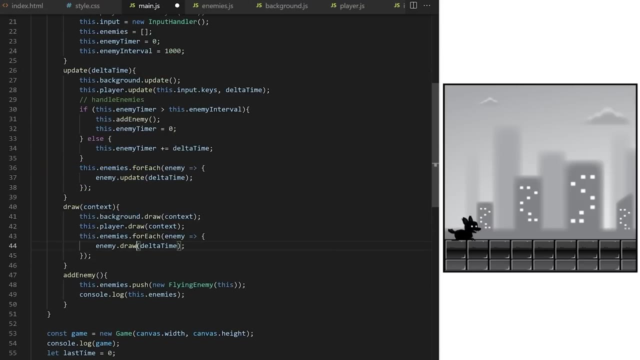 In the callback function. I just trigger update method on each enemy element And I pass it the delta time from here, Because I know it's expected there. I will do the same thing inside the draw method. I will cycle through all enemy objects and I will trigger their draw method. 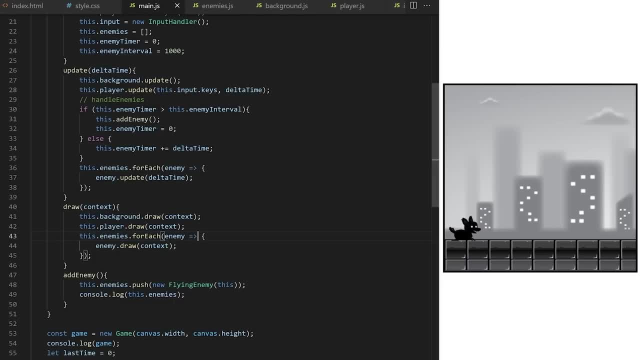 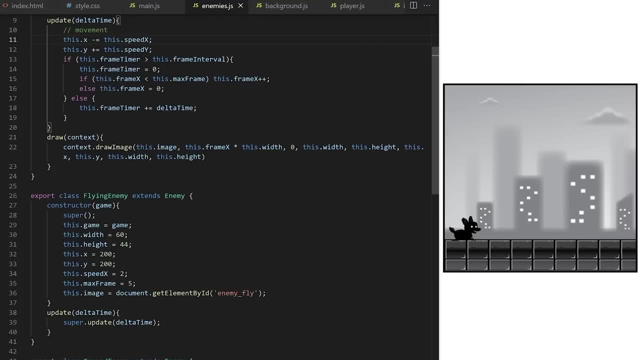 I pass it context as an argument. I don't see any enemies coming. Let's try to use minus equals here to make them move to the left. Still nothing. I'm console logging enemies array. so let's check the console. I open up the array. 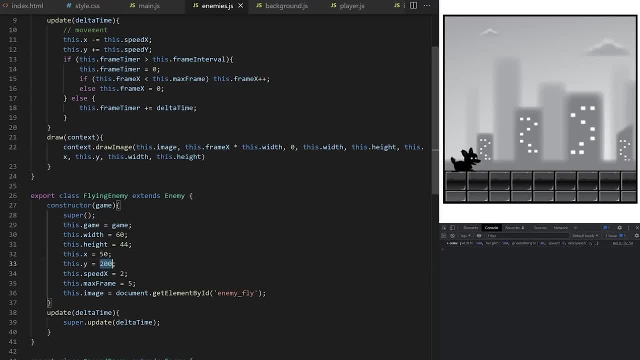 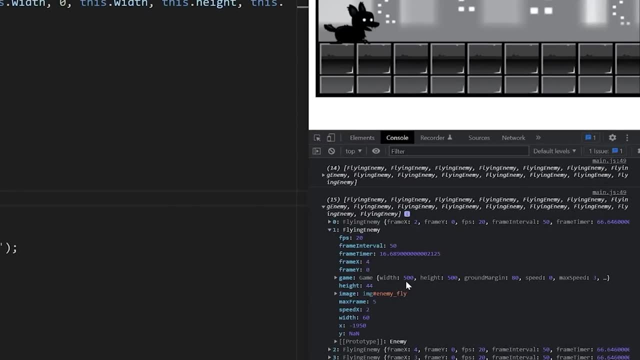 Let's change the initial x and y coordinates to 50- 50. now If I open the array again and I check one of my flying enemies, I can see their vertical y coordinate is none, Not a number. JavaScript doesn't know where to draw them vertically. 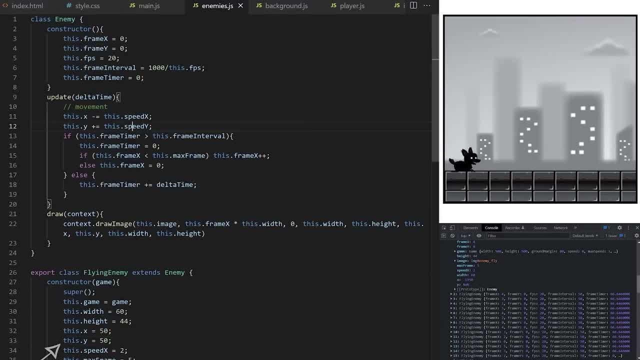 Let's track the problem. I define vertical y coordinate correctly on line 33. But as the game runs, I'm increasing it by speed y property here on line 12.. Speed y doesn't exist, So as a result, we are breaking our code. 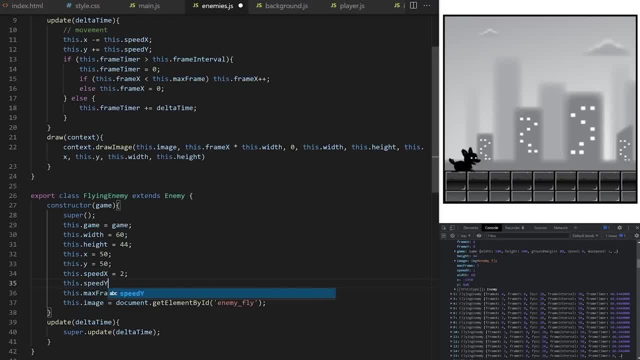 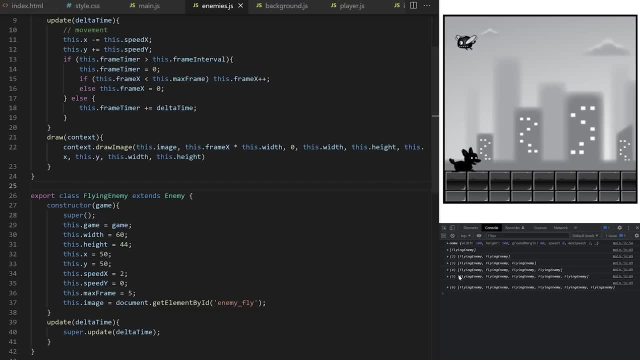 I will define vertical speed y property on my flying enemy class. Let's set it to zero. Nice, We have enemy flies moving from right to left from the initial starting coordinates- 50, 50, as defined here. I actually want them to start from the point just behind the right edge of available game area. 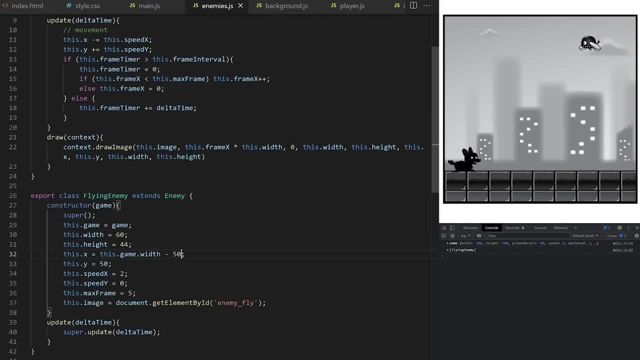 So the initial x coordinate will be this dot game from line 29, dot width Nice. I randomize vertical y coordinate to spread them around. I want them to only move in the upper half of the game area. So math dot random times, this dot game, dot height times 0.5.. 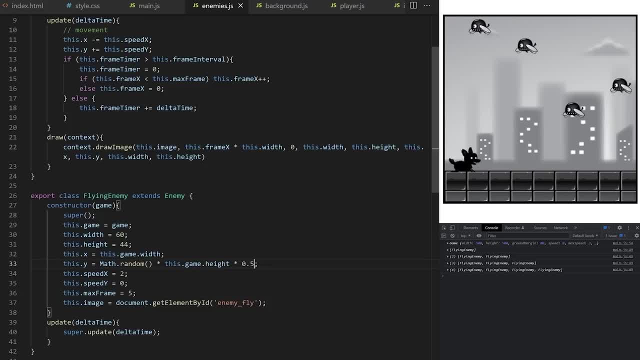 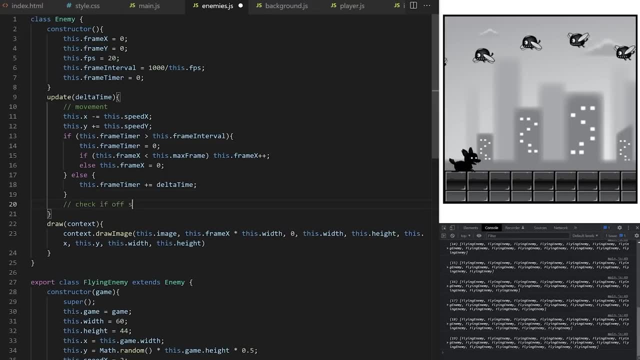 In console you can see we have an endlessly increasing array as more and more enemies are being added. I actually want them to be removed when they fly past the left edge of screen. I will check if enemies are off screen in this area If horizontal coordinate of the enemy plus its width is 0.. 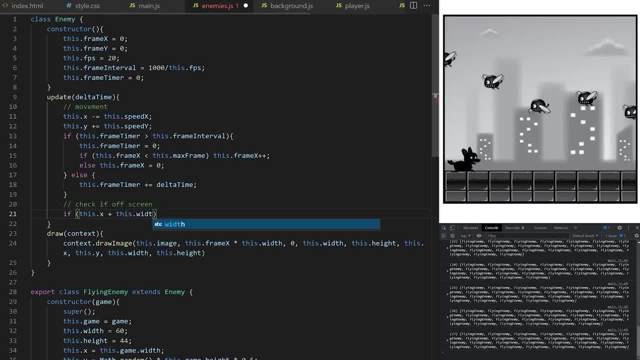 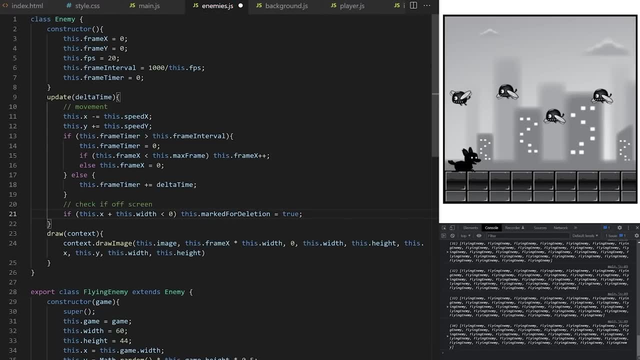 Meaning it's completely hidden behind the left edge. Set its marked for deletion property to true. This property will be shared for all child classes, So I can define it only once up here on the parent class. Initially I set it to false, So we are adding new enemies. 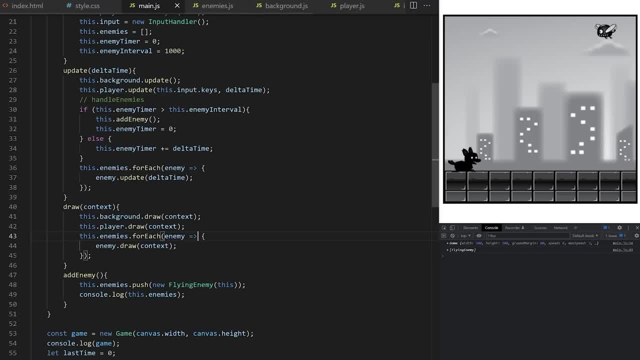 They fly from right to left. When they are hidden behind the left edge, we are setting their marked for deletion property to true Here. inside update method on game class. initialize update method on game class In the area where we handle enemies. we are cycling through every object in enemies array, triggering their update method. 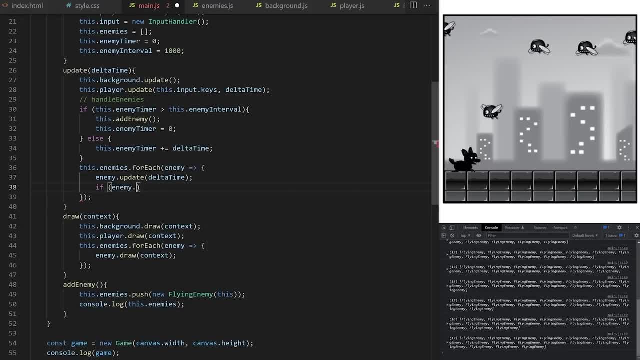 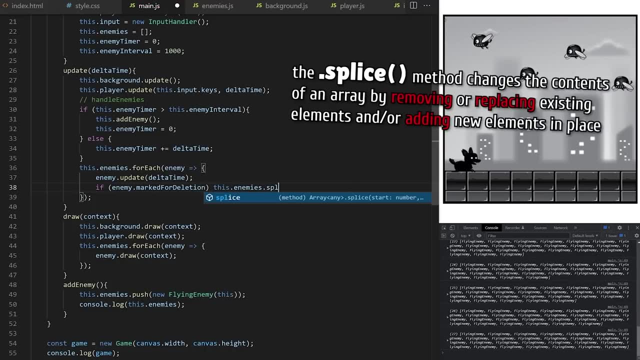 At the same time, I will also check if their marked for deletion is true And if it is, we splice it out of the array, removing it. Splice method needs two arguments, In this case, index of the element we want to remove from the array. 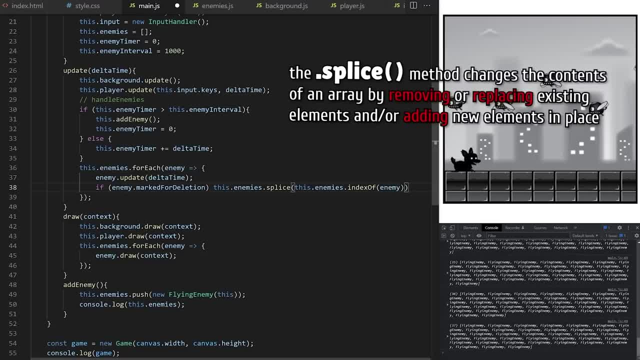 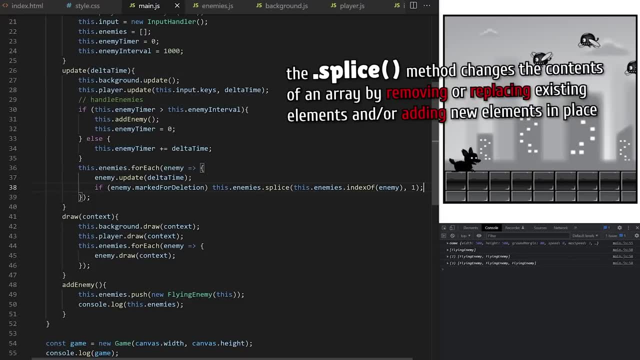 So index of this enemy with marked for deletion set to true And how many elements to remove at that index? We want to remove only one element. Now I check in the console and I see that new enemies are being added and old enemies are being correctly removed. 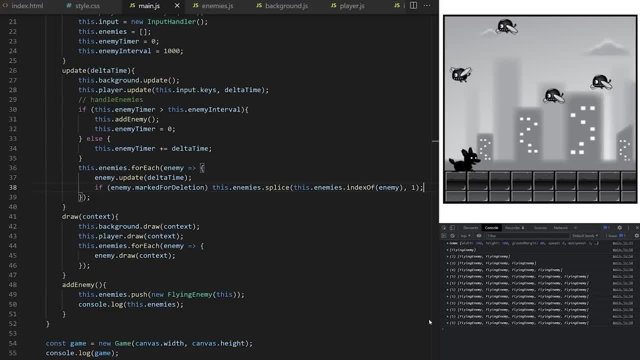 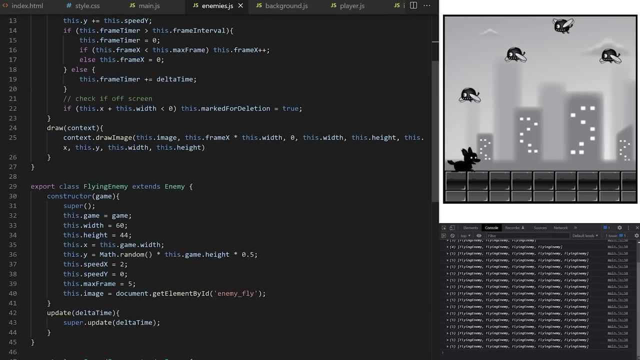 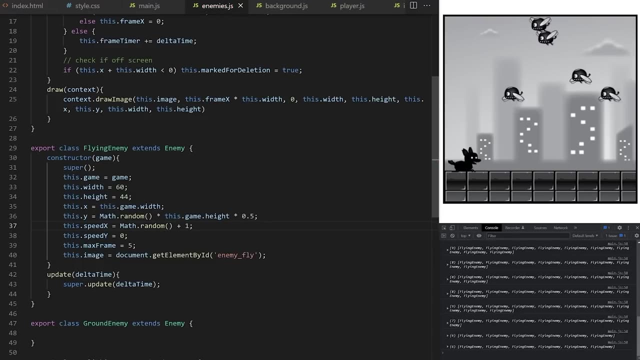 Perfect. Let's play with the movement a little bit. I can do so many things here, and there is a special episode about it. I can, for example, randomize their horizontal speed x value so that each enemy flies at a slightly different speed. Let's try a random value between 1 and 2 pixels per frame. 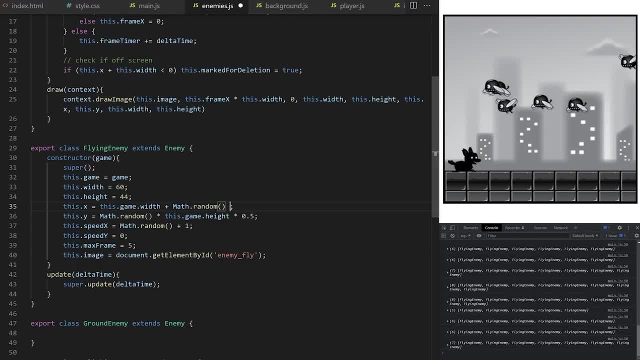 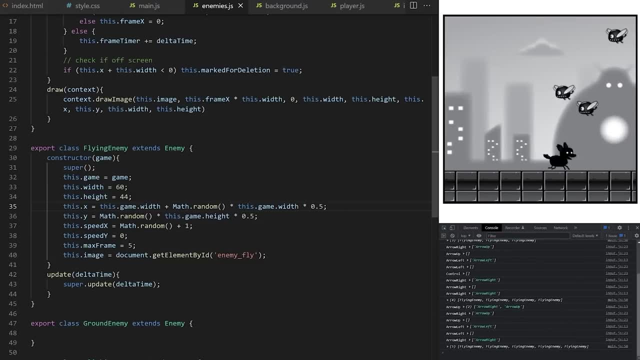 I can also randomize their initial value. I can also randomize their initial x coordinate so that we get even more randomness in their spacing. When the player starts running, it becomes obvious we need to account for the current game speed when making enemies move. 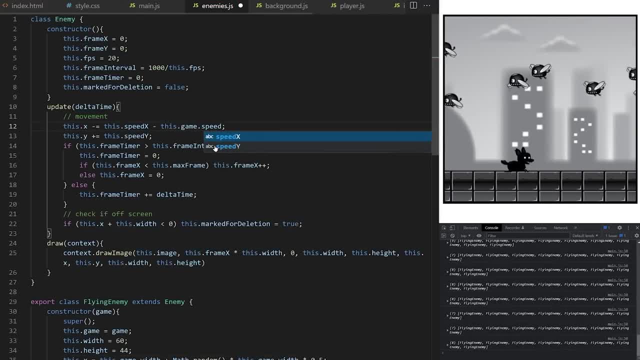 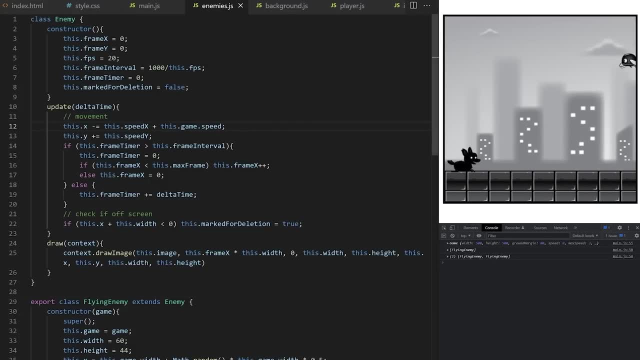 Up here on line 12, I just include game speed in horizontal position calculation. I actually need to use plus here Now, when the player moves and when it stops moving. I need to make sure it is positioned correctly in relation to our dynamically scrolling game world. 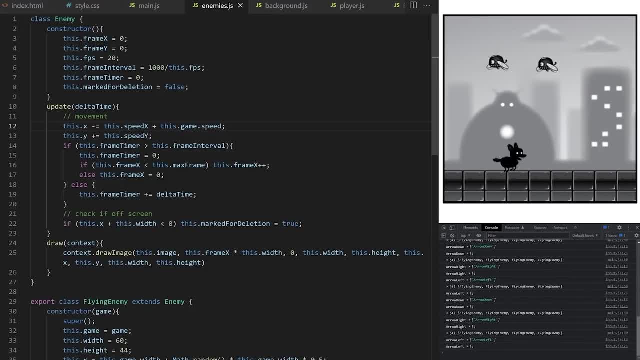 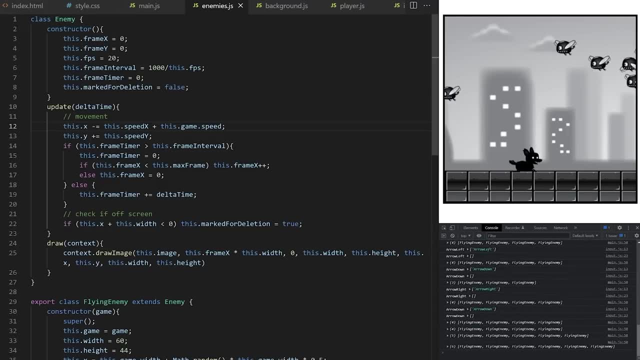 We made a lot of progress today. If you are still following, well done. These are all fundamentals of 2D game development. I hope you are getting some value out of this. So the flies are moving in a straight line from right to left. 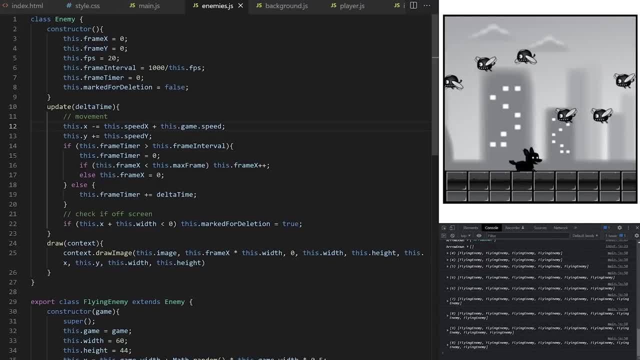 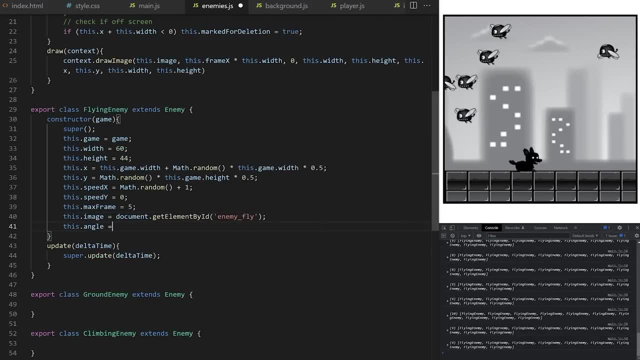 What if I want to give them a wavy up and down wobble as they move? It's easy: I will need two helper variables, and these will be specific only for flying enemies. so I declare them down here. Angle will start at 0.. 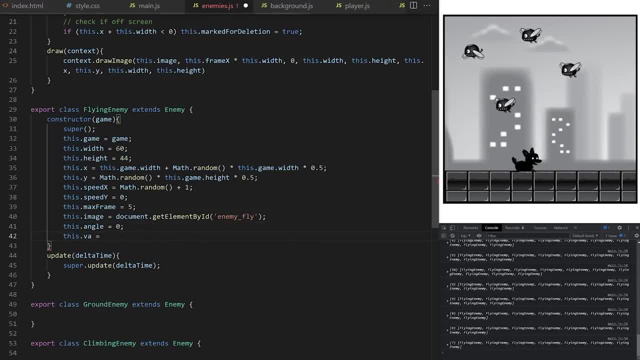 And we will be increasing it slowly and feeding it to mathsign method, which will map it along a sine wave. It will be increasing by this custom VA value- Velocity of angle- and it will be a random value between 0.1 and 0.2. 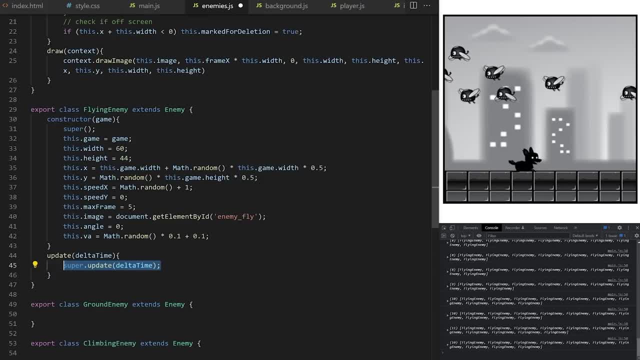 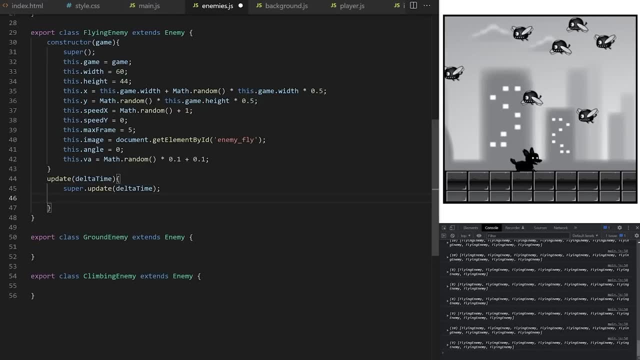 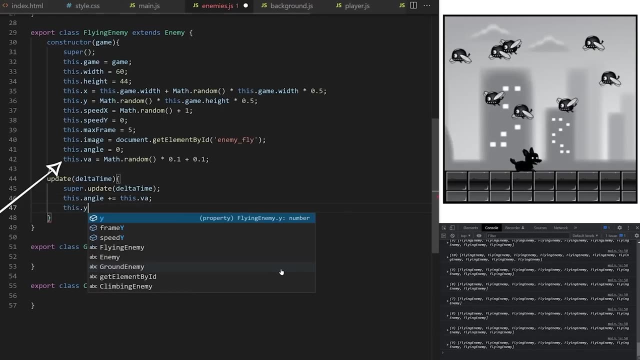 Inside update method on flying enemy class. I first trigger all the code from the parent enemy class And I will add some extra custom code that will be specific only for flying enemies. For every animation frame I will increase angle By VA value And then I update vertical Y coordinate by mathsign of this ever increasing angle value. 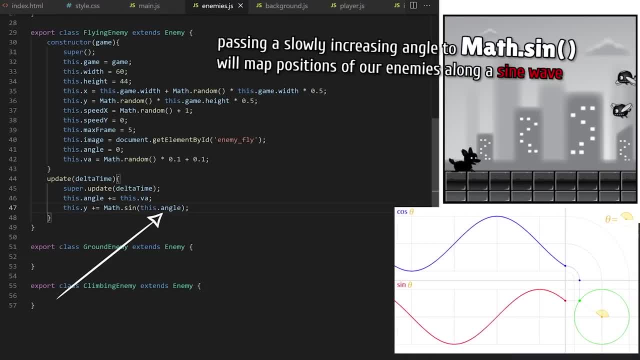 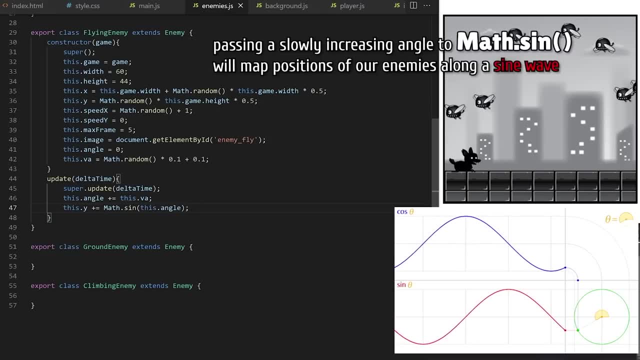 Passing a slowly increasing angle to mathsign will map positions of our enemies along sine wave. We can also create a circular movement by using mathcosign on horizontal X coordinate. For now, let's leave it like this. We have our flying enemy type. 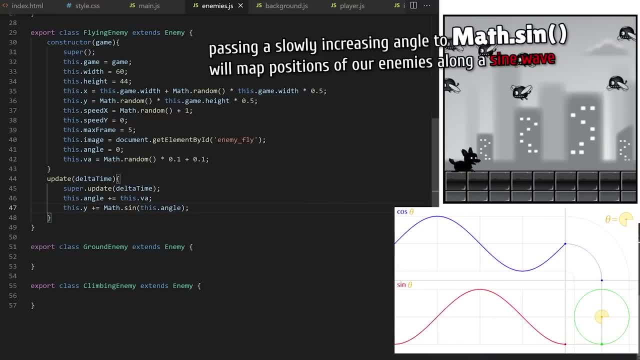 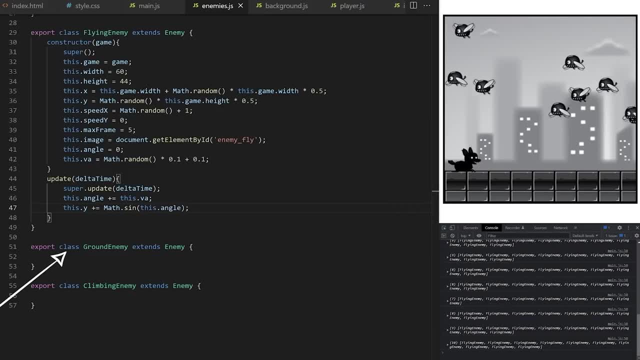 Perfect. Let's create a ground enemy. It will be a plant, so it will have different behavior. It will be much simpler to implement. Let me show you Class. ground enemy extends enemy. So again, this class will automatically inherit everything from the parent enemy class we declared up top. 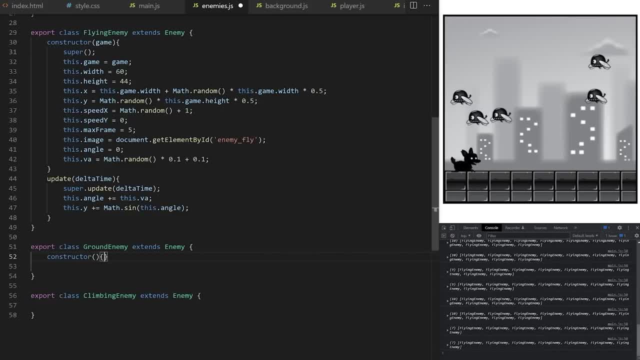 The only properties we will declare here are the ones that are specific to ground enemies. Shared properties will be inherited automatically because of this extends. keyword Constructor will expect game as an argument and we convert it to thisgame property. The width of a single frame is 60.. 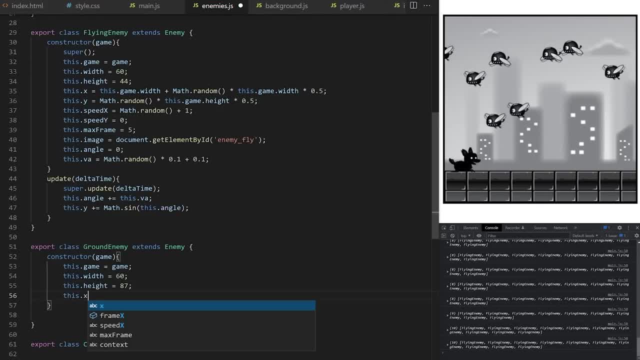 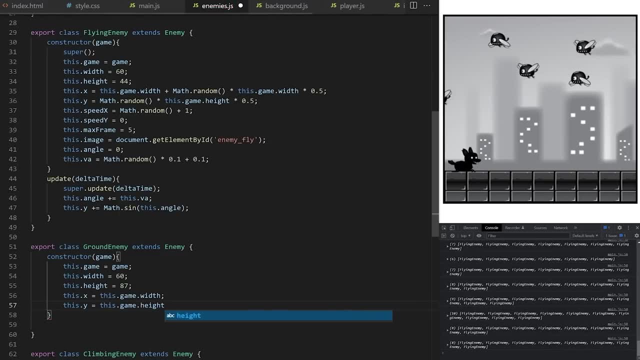 Height is 87 pixels. Initial X is just behind the right edge of canvas, So thisgamewidth. We want the enemy to be sitting on the ground level of our game world, So vertical Y coordinate will be game height minus height of this enemy, minus ground margin. 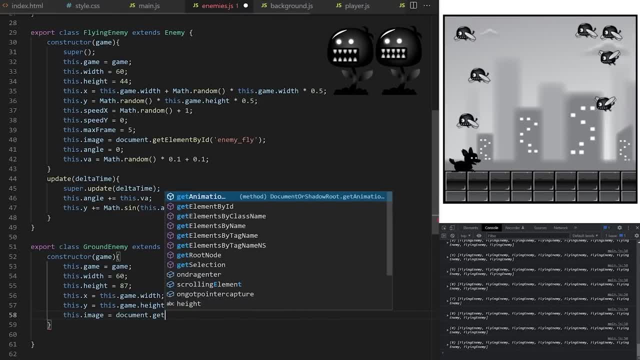 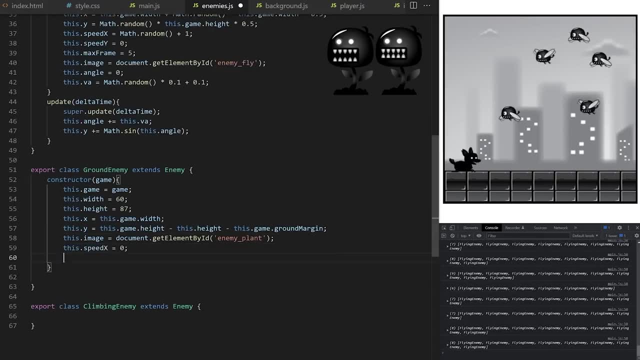 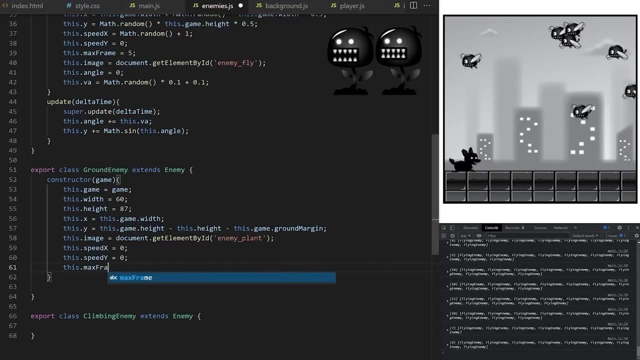 Image will point towards enemy plant image from indexhtml. Horizontal speed will be 0.. And vertical speed will be also 0.. This is a plant. It won't move around. Sprite sheet is very simple. It has only two frames. Max frame is 1 because we count from 0. 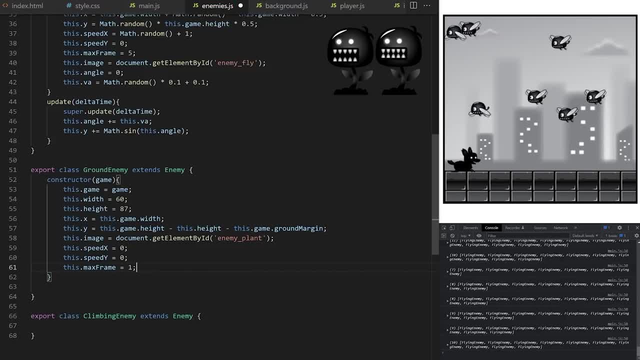 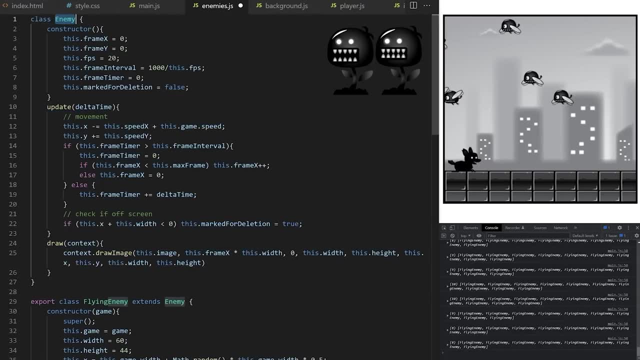 If I don't declare update and draw methods at all on ground enemy class, JavaScript will automatically travel up the prototype chain and it will find update and draw method on the parent enemy class In mainjs inside addEnemy function. we only want to be adding ground enemies when we are moving. 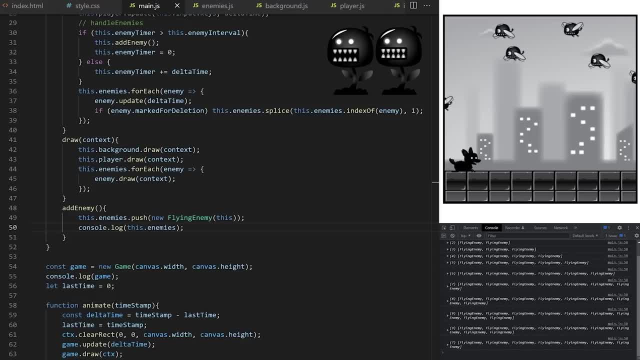 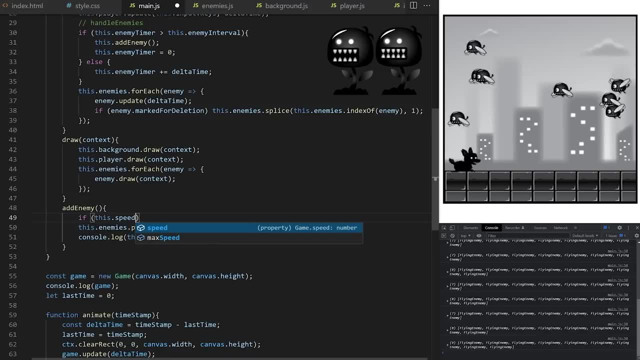 If we are sitting down. we don't want the game to keep adding new ground enemies because they would just be accumulating off screen. We only want to add a new enemy if game speed is more than 0. When the game is scrolling, And also I don't really want to add it every 1000 milliseconds. 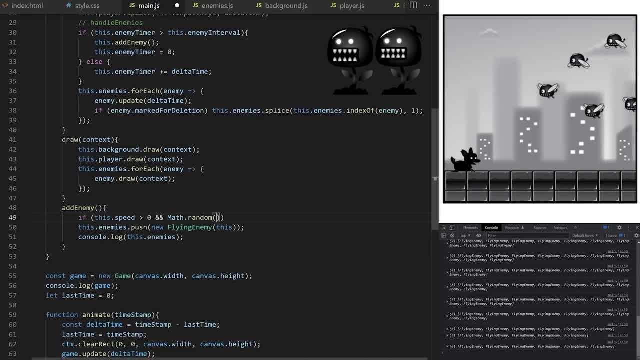 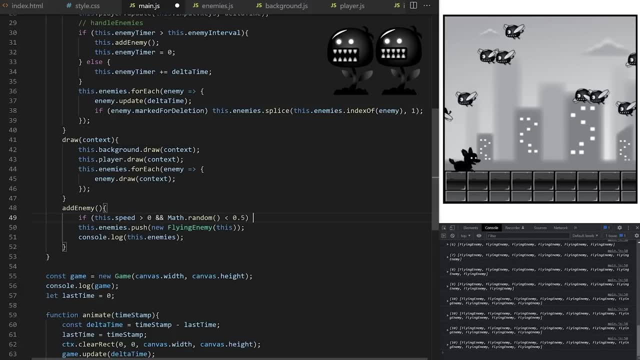 Every time addEnemy method runs, I only want there to be a 50% chance that we add one. So Mathrandom is less than 0.5.. Mathrandom code like this returns a random value between 0 and 1.. So a value lower than 0.5 should occur on average 50% of the time. 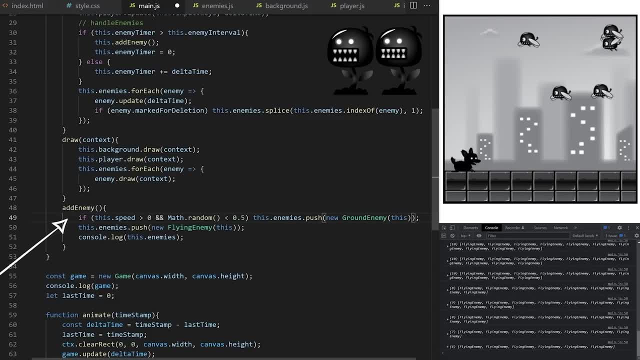 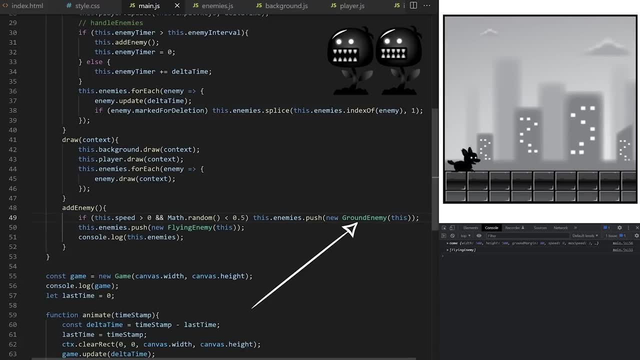 So every time addEnemy method runs, we always add one flying enemy, And if the game is scrolling and this 50% check is true, we also add one new ground enemy. I get an error which tells me I forgot to call superclass constructor on my subclass. 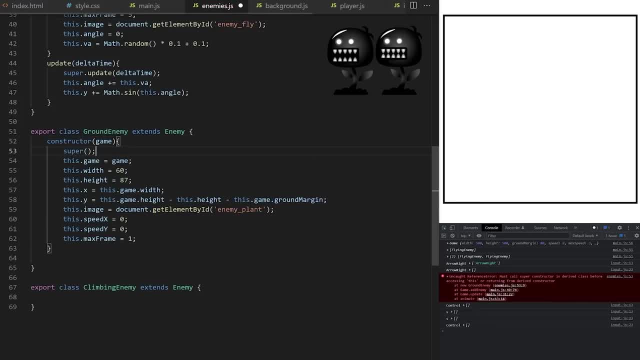 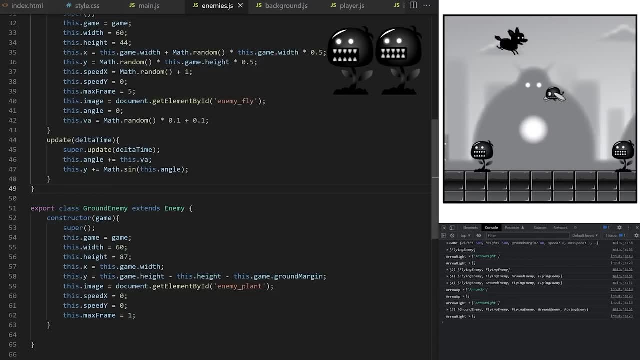 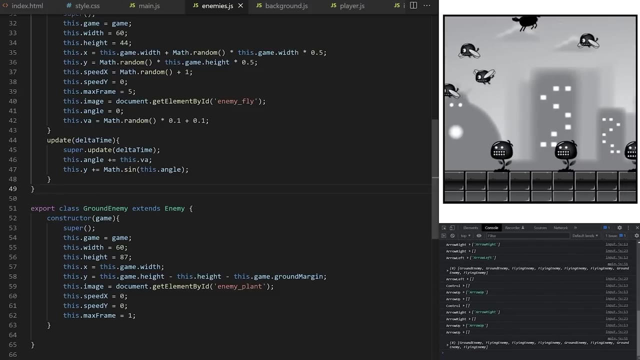 Easy to fix Like this. Nice, we have a ground enemy in our game. You can see there is a small wobble between enemy plants and the ground texture. I'm not really sure what's causing it. now. If you know, let me know in the comments. 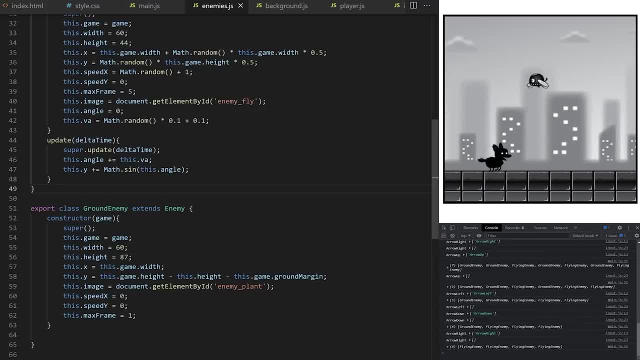 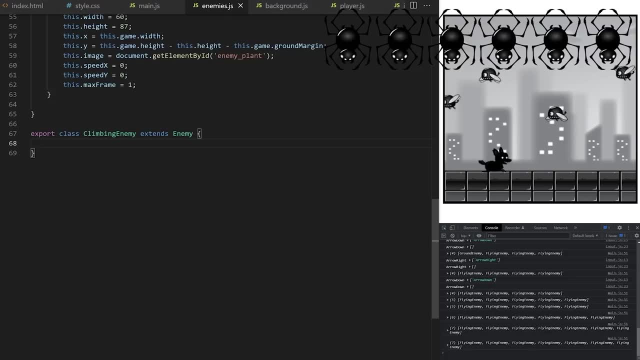 We will fix this later. Let's add a climbing enemy. Climbing enemy will be a big spider suspended from a web. I showed you how to extend update method to make our flies move in a different pattern. I also showed you how it works when you don't need to declare any additional update and draw methods with the plant. 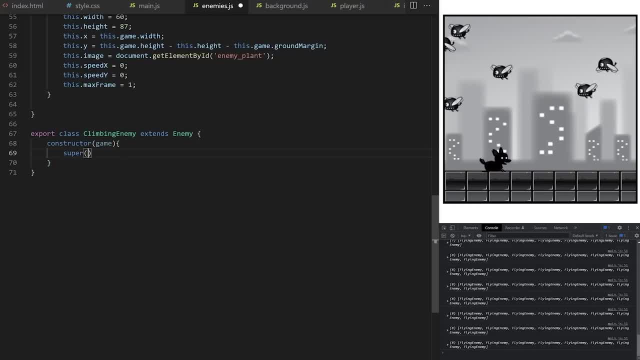 Now I will show you how to extend draw method and how to add some additional graphics. In this case, spider webs Constructor will expect game as an argument. We call super to trigger class constructor from the parent enemy class. Thisgame is game as usual. 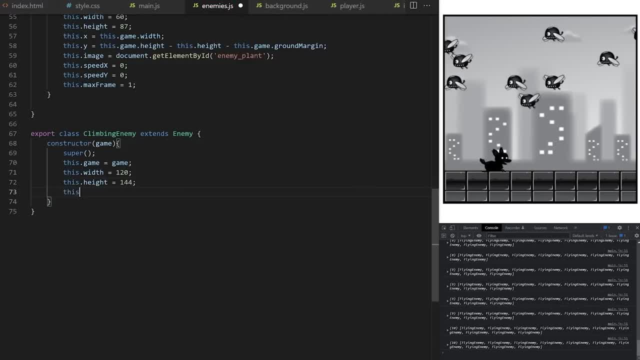 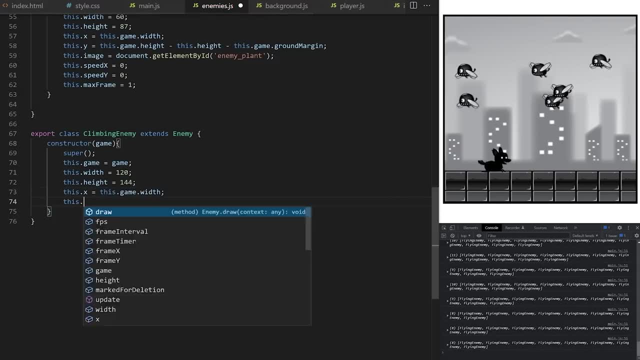 Width of a single frame is 120.. Height is 144 pixels. The initial starting coordinate is behind the right edge of canvas, so thisgamewidth Vertical Y coordinate will be a random position in the top half of the available game area. Image will point to the big spider image we linked earlier in indexHTML. 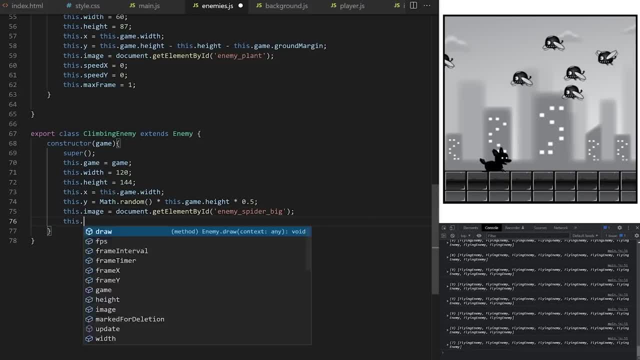 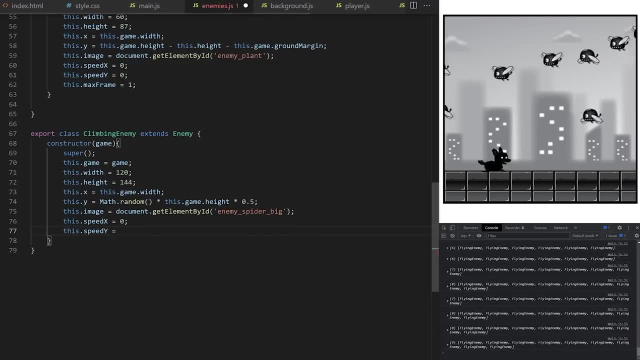 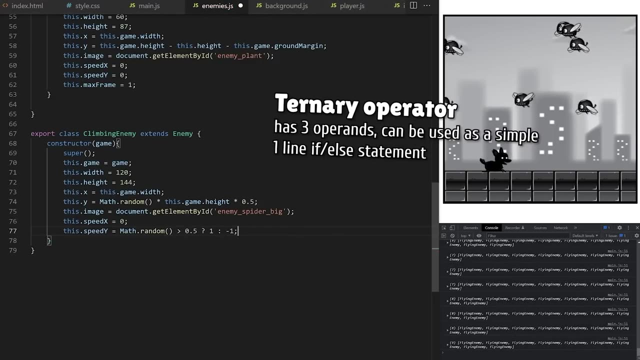 Horizontal speed X will be 0.. Our spiders will be moving up and down vertically. Vertical speed Y will be either plus 1 or minus 1, depending on this mathrandom check. This is so called ternary operator. We are using it as a simple one line, if else statement. 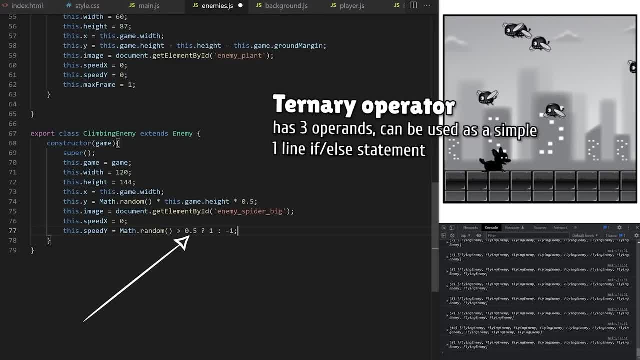 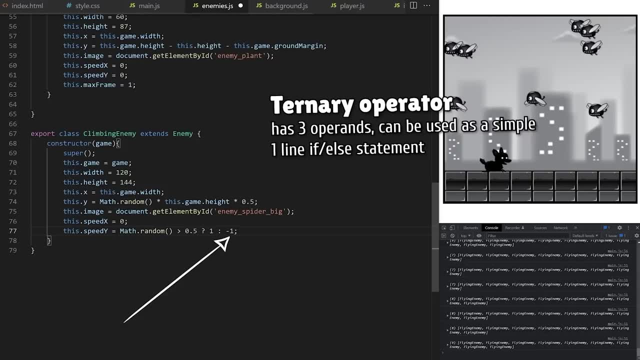 If mathrandom is less than 0.5, which should be roughly in 50% of cases, Set speed Y to 1.. Else, set it to minus 1.. So if condition is true, question mark: return this. else, colon: return this. This will make sure some spiders are moving up, some are moving down, when they initially spawn in our game. 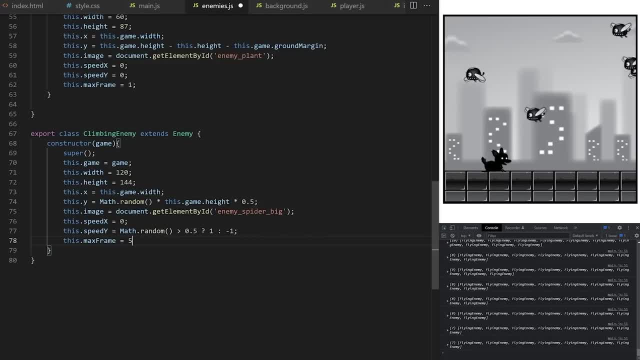 Max frame of spider sprite sheet is 5.. Update method will take delta time as an argument. It will first call update method on its parent enemy class to run all the code from there. We will also do the same thing for draw method like this: 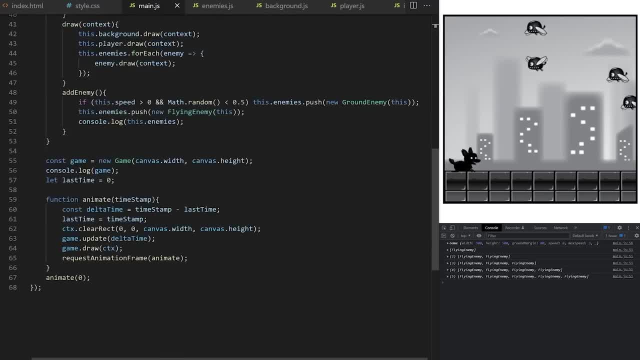 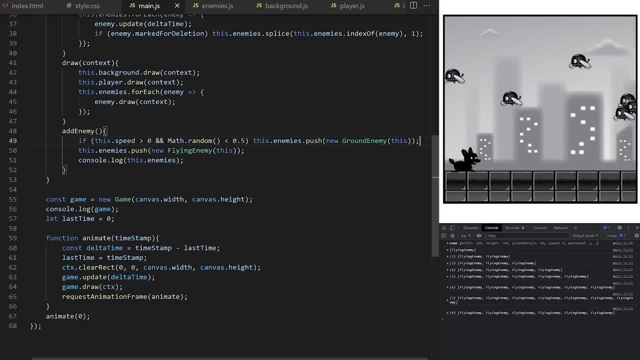 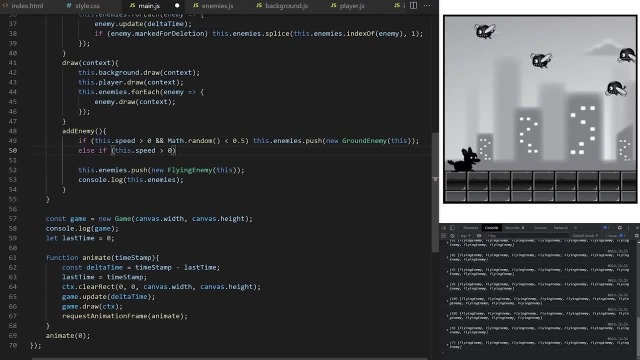 Here I am checking if game speed is more than 0 and if random check is less than 0.5 and I am adding new ground enemy I am going to add. else, if here and if this random check is false, and at the same time if game speed is more than 0, we will add one new climbing enemy into our game. 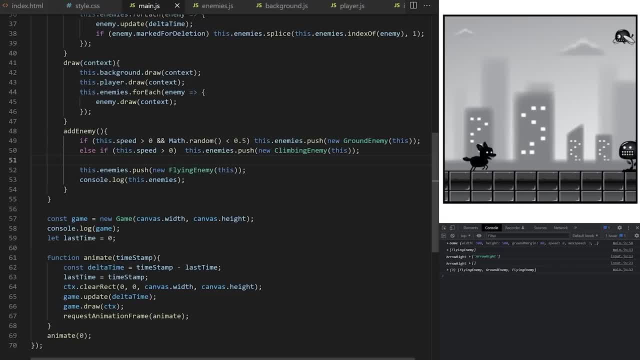 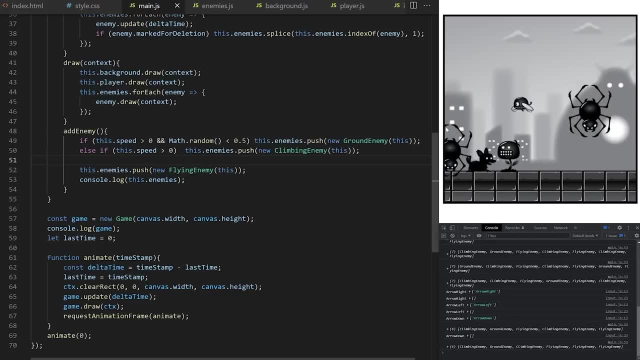 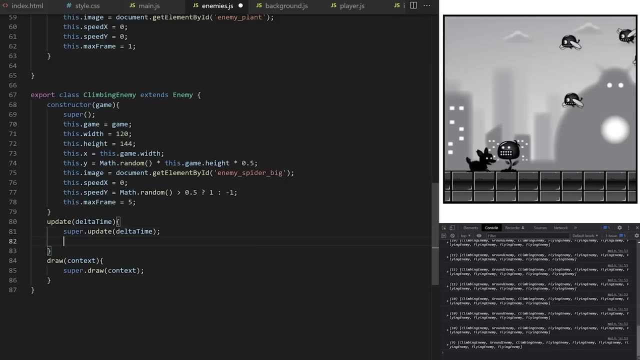 Now, every second, we always get one fly and we get either one spider or two spiders Or one plant. Nice, I am extending update method on climbing enemy because I want to climb up and down. When it is moving down and it reaches a bottom boundary we defined here, I want it to kinda bounce and start moving in the opposite direction, upwards. 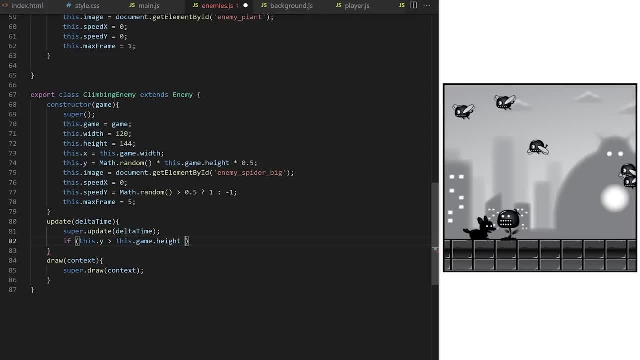 Let's make it move upwards whenever it climbs all the way down and touches the ground level. So if vertical Y coordinate is more than gameheight minus height of this spider enemy, minus ground margin, Set its vertical speed to its minus value. So thisspeed times minus 1.. 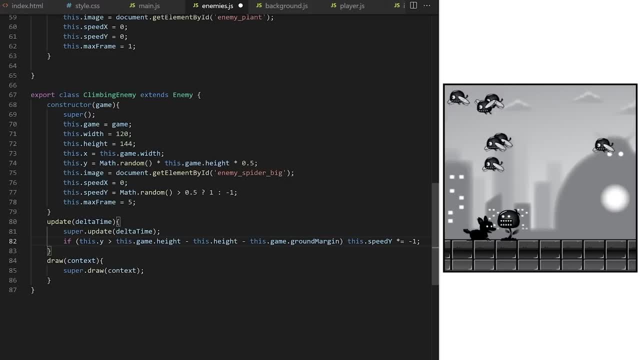 Also, I want to set its marked for deletion to true if it climbs off screen vertically. So if thisy is less than minus height of the spider sprite sheet, set its marked for deletion to true. This spider spawned moving up. This one is moving down. 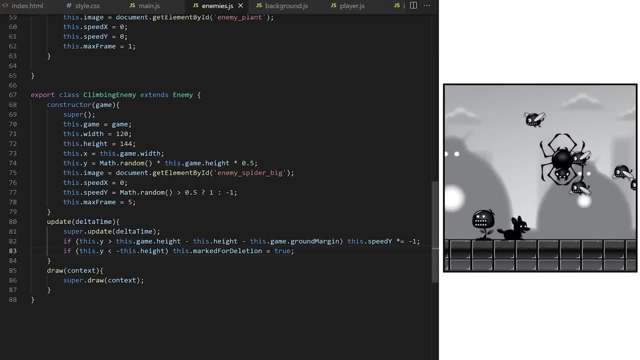 When it reaches ground it bounces and it starts moving back Up. Perfect. We are also extending a draw method. so let's draw a spider web. Spiders don't fly, They should be hanging from a spider web. We are calling draw method on the parent enemy class. that will handle drawing of the actual spider sprite sheet and we will add some extra code here just to draw the spider web. 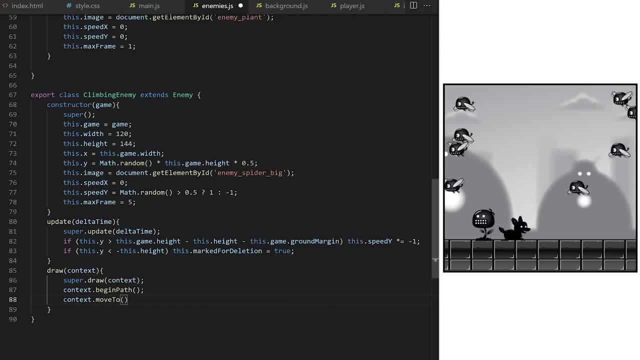 I want to create a line, so I start by calling beginPath. Move method will set the initial X and Y coordinates of the line. I give it coordinates 0,0 for now. The top left corner of canvas. Line 2 will define the ending X and Y coordinates. so I pass it spider's current X position as X and 0 as vertical Y. 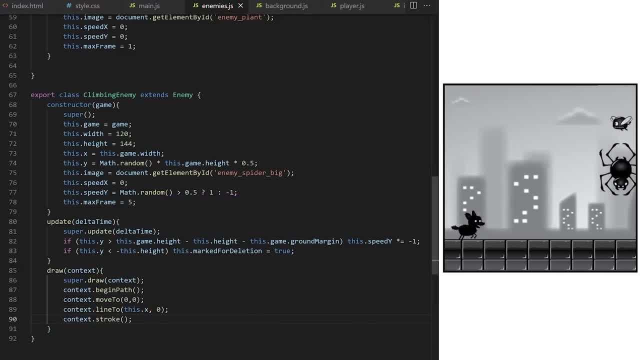 Now I can stroke my line. I don't see any line Right. I need to use thisy here to move it on screen. And here's our spider web. It works, Let's make it look better. I want it to start from thisx and 0, so just above the spider. 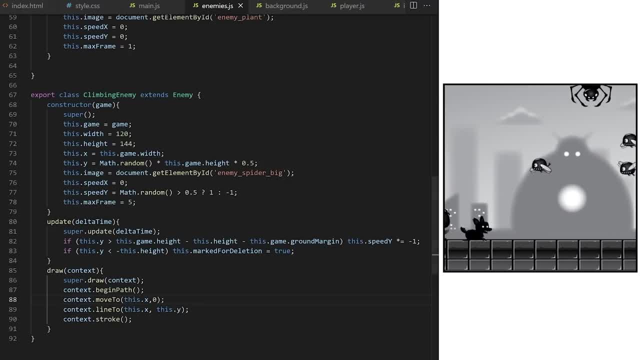 Nice. So it goes from the top left corner of spider sprite sheet upwards. I need to center it horizontally. so plus the width of the spider divided by 2. And I increase Y by 50 to actually touch the spider image Almost there. 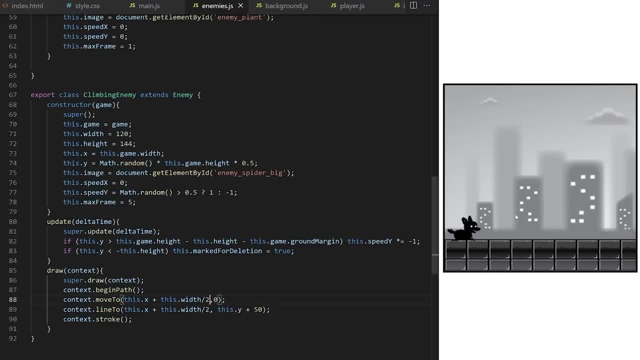 I just need to also offset the initial starting point of the line like this. I'm happy with this. If you are designing a game with multiple levels, you can, for example, have a different flyer, different ground enemy and different climbing enemy for each level. 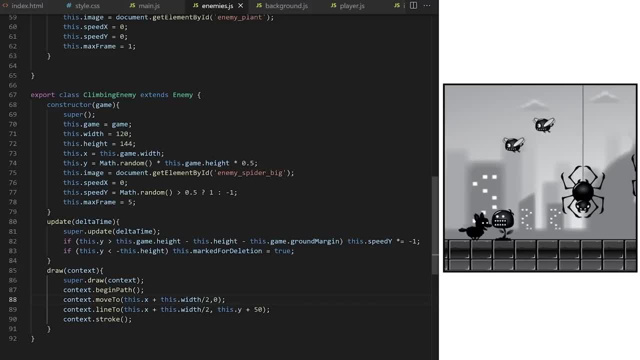 So three enemy types like this could be enough, depending on your game structure. Also, it's possible to put many more enemy types into the game and mix them together. It's up to you. I gave you all the tools you need. If you have any questions, let me know. 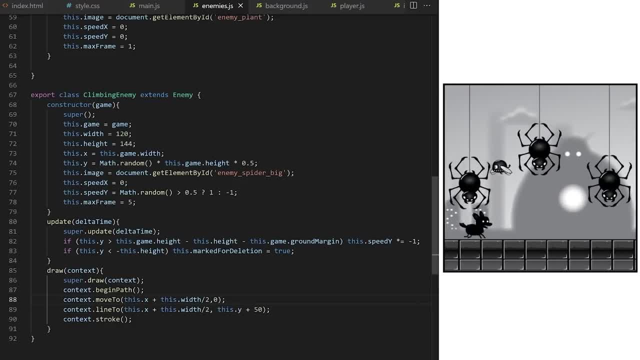 We will learn how to handle collision detection. next time We will also apply particle effects to give the player a fire trail, and we will add two more states with unique animations for when the player is attacking and when it gets hit. Well done on completing the lesson. 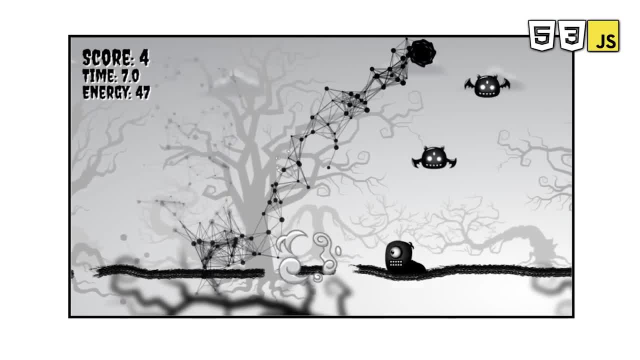 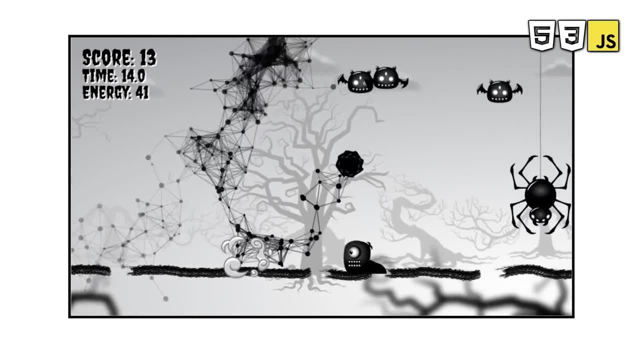 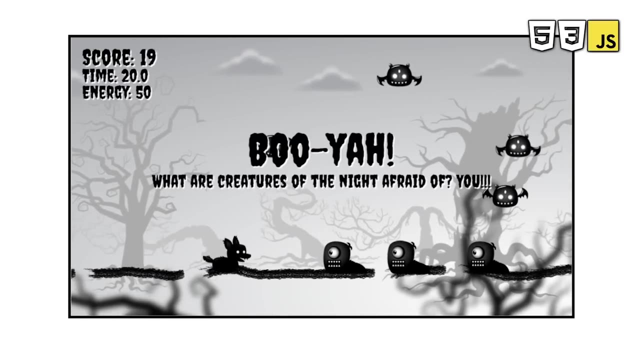 See you in the next one. We created a player, we have our game world and we added dangerous creatures of the night. It's time to add some interactions and special moves. Today we will learn an easy way how to handle collision detection and we will resolve collision between player and enemies in two different ways, depending on the current player state. 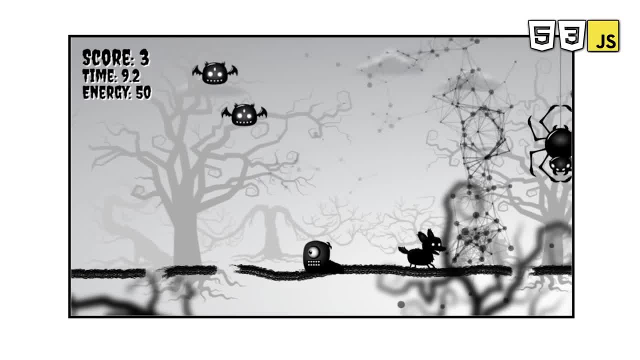 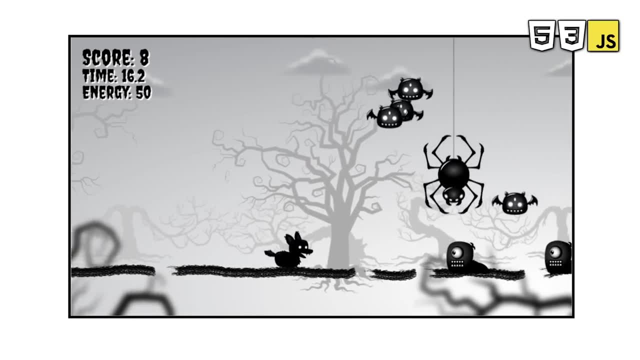 If the player is rolling, enemies are destroyed and we get score points. In any other state, it's the player who receives a hit. We will also add dust particles and fire trail. If you want any of my other creative courses, you can also use those animated trails and use them here, like you see in this demo. 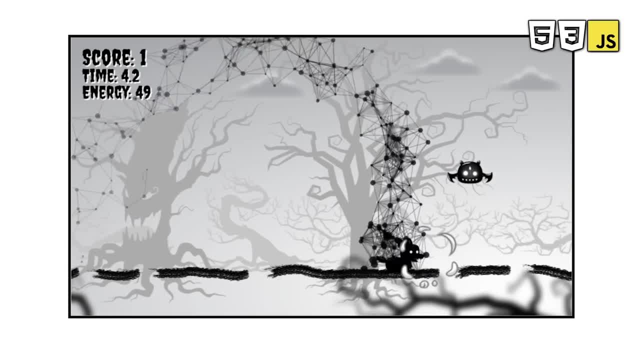 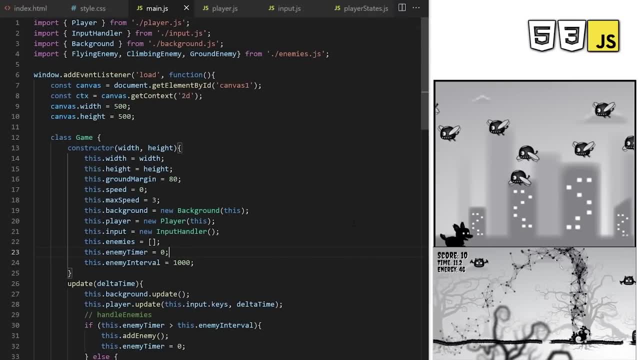 I like to combine game dev and creative coding With JavaScript and HTML canvas. it's all the same set of techniques. Let's go. We have player and enemies in our game. We want them to be able to interact in different ways with each other. 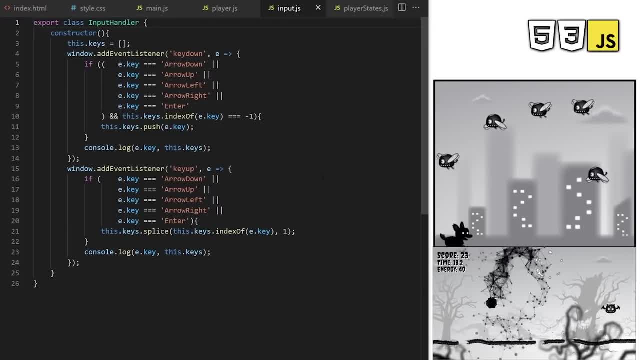 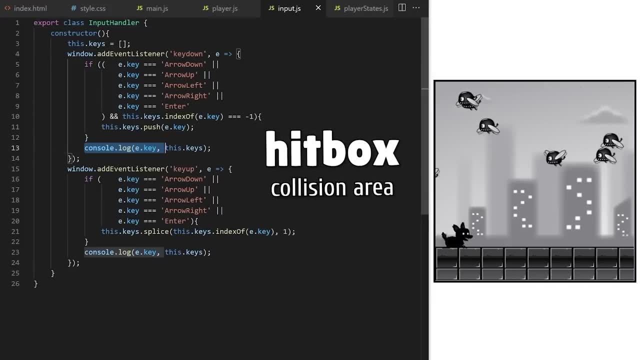 Let's apply collision detection First. I want to draw a rectangle around the player and around each enemy to see their collision areas, so called hitboxes. I go to input checkbox, I go to inputjs file and I delete these console logs. I want our game to have a debug mode. 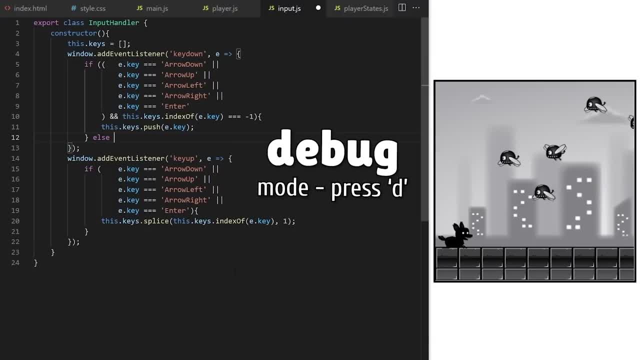 When I press letter D on my keyboard, we enable debug mode and collision hitboxes will be drawn. When we press D again, we exit debug mode and hitboxes will be hidden. It's very simple to implement. In keydown event I create an else if statement. 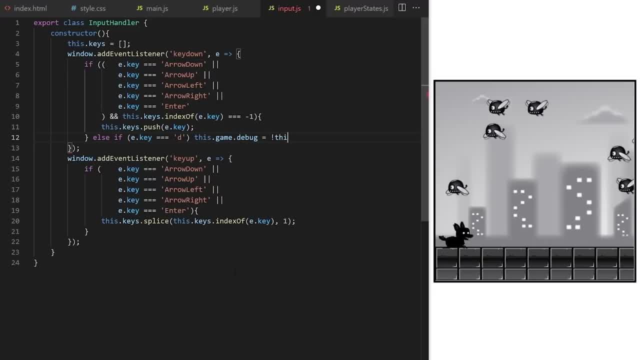 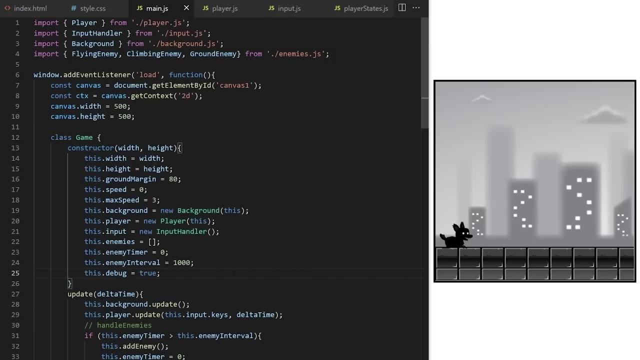 If ekey is D, set debug property on the main game object to its opposite value. If it's currently true, set it to false. If it's false, set it to true. In mainjs I create thisdebug property on game class and initially I set it to true. 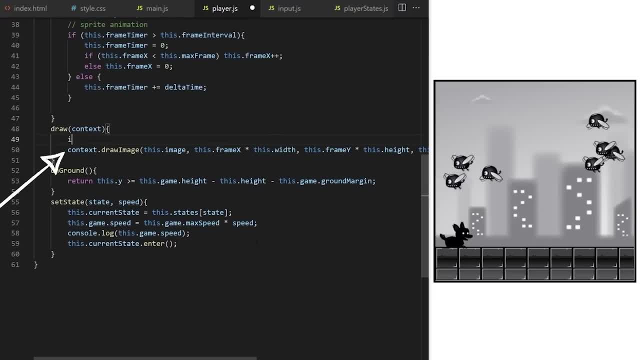 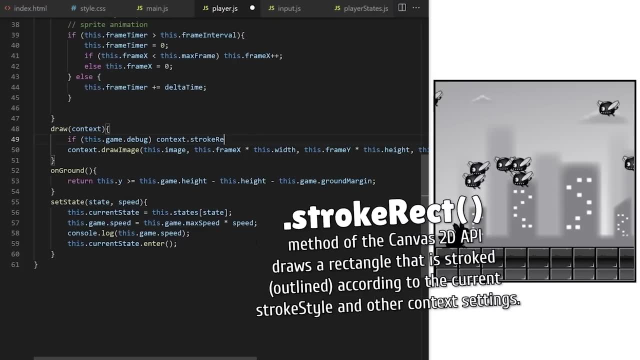 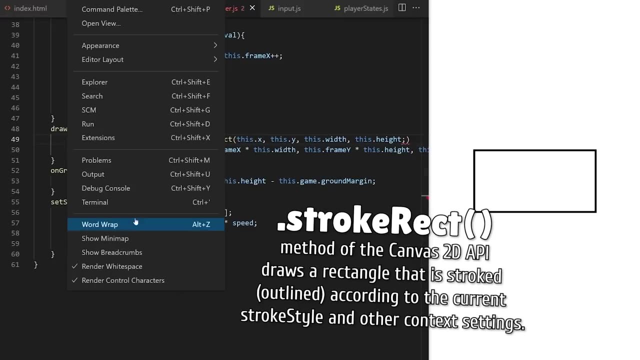 In draw method on player class. before I draw the player sprite sheet, I say: if thisgamedebug is true, draw a rectangle around the player. This rectangle will be exactly the size of player's hitbox. so from thisx, thisy player's coordinates, to player's width and height, like this: 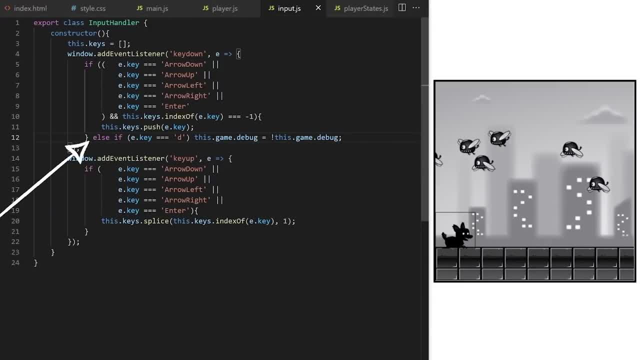 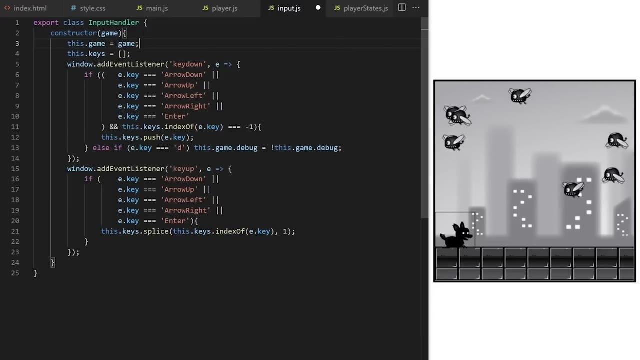 Now I can go back to input checkbox In inputjs. here we are toggling debug mode on and off by pressing letter D. For this to work I need to bring a reference to the main game object. here. I pass game object as an argument to the class constructor and I convert it to a class property. 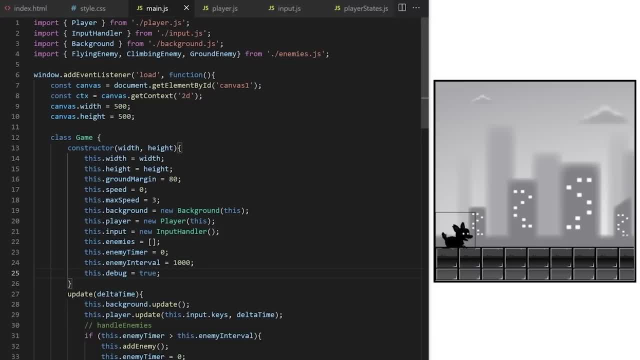 From here we can point to the game object and toggle debug mode on and off. Finally, we know that input handler class expects game as an argument. So here on the main game class, I pass it. this as an argument. When I press letter D on my keyboard we are toggling debug mode on and off. 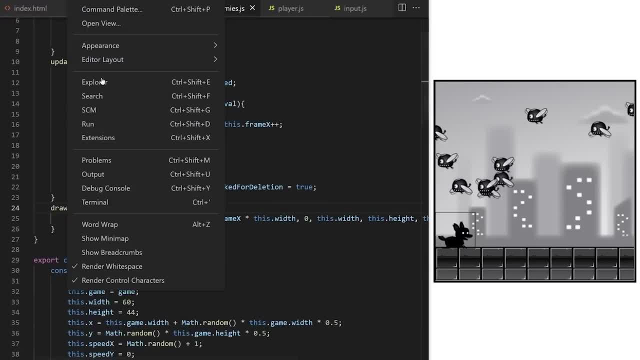 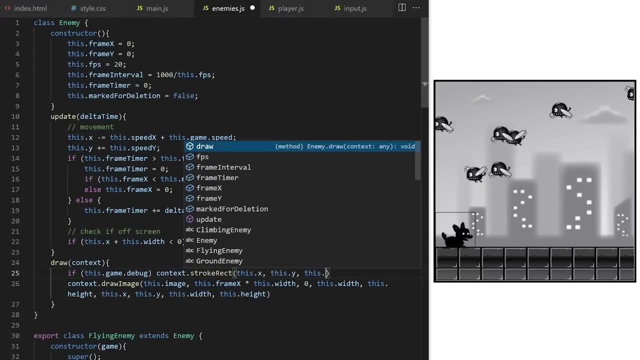 Perfect. I can also create hitboxes around enemies Inside the draw method on enemy class. I say, if thisgamedebug is true, stroke rectangle around the enemy Like this, This will work. Reference to the game object is not on the main parent enemy class, but we have it down here on each enemy type separately. 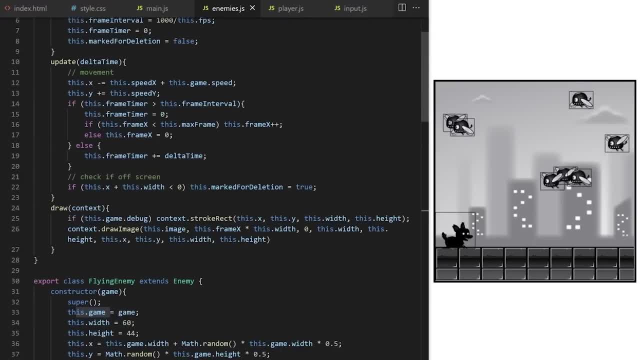 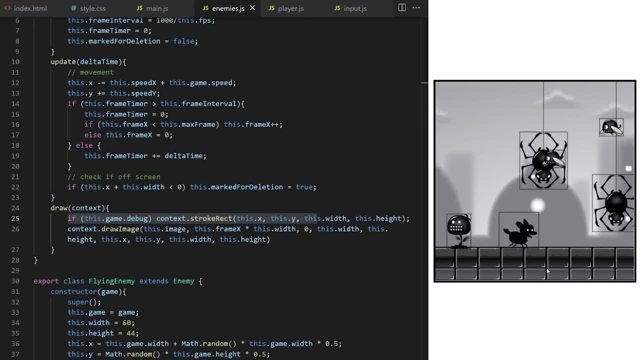 Our game now has a debug mode. You can toggle it on and off by pressing D. These hitboxes represent collision areas. When the player hitbox touches any of the enemy hitboxes, I want them to interact in some way. We can have multiple different interactions. 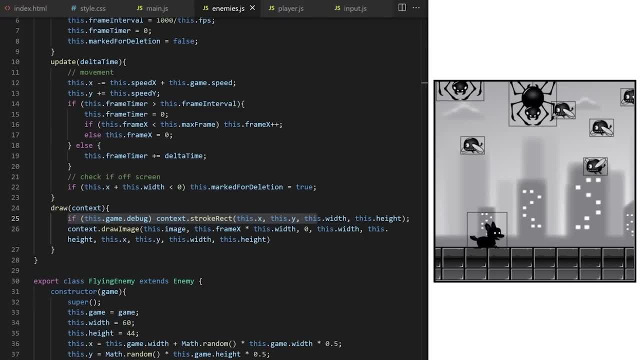 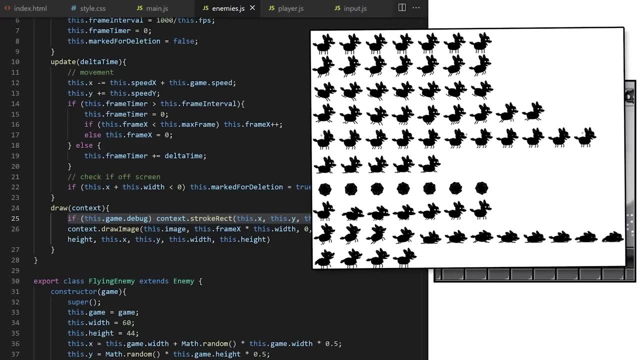 Today I will show you how to have two different interactions. When the player collides with an enemy while in rolling state, it will destroy that enemy and we get some score points. If the player is not rolling, it will get hit and it will stop its movement for a moment and play dizzy animation from our sprite sheet. 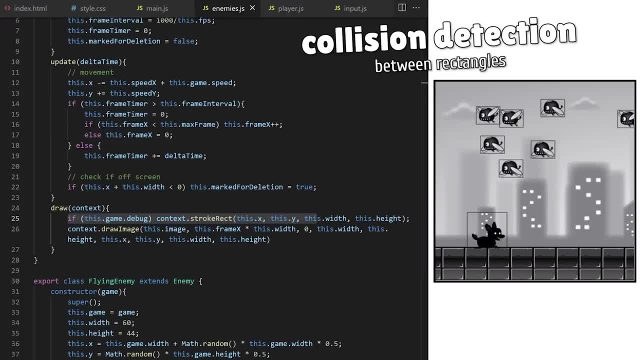 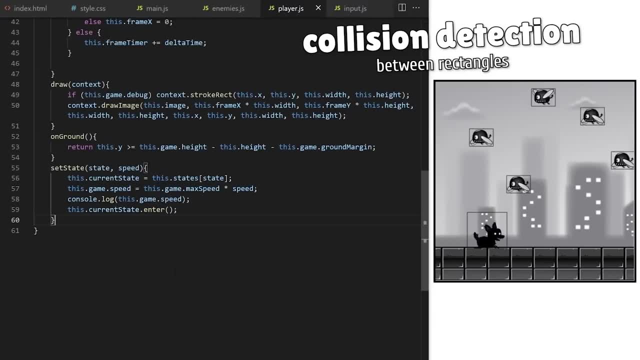 We will use a simple collision detection formula between two rectangles To check if player and enemies interact Here inside the player class. I create a new helper method. I call, for example, check collisions Inside. we will cycle through enemies array that holds all currently active enemy objects. 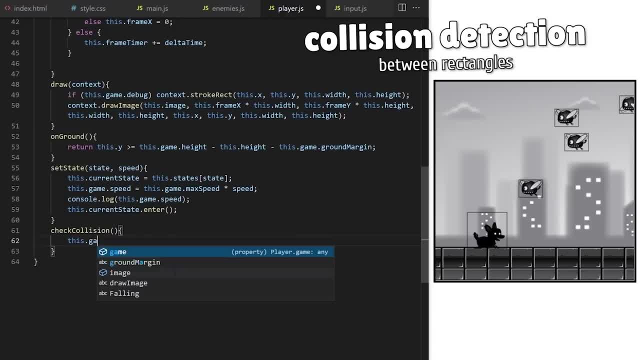 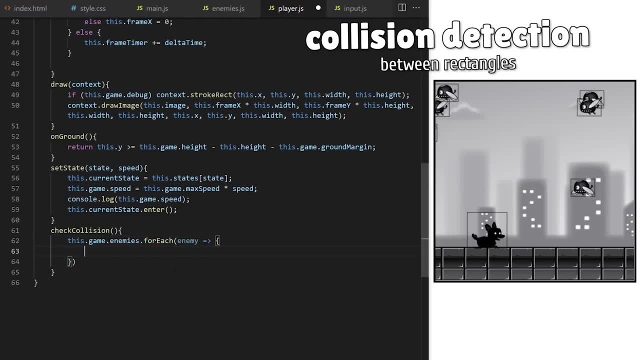 And as we cycle through them one by one, we will compare their xy width and height to the current xy width and height of the player object. So thisgameenemiesforeach, and for each enemy object I will run the following callback function. We will have a simple, if else, statement. 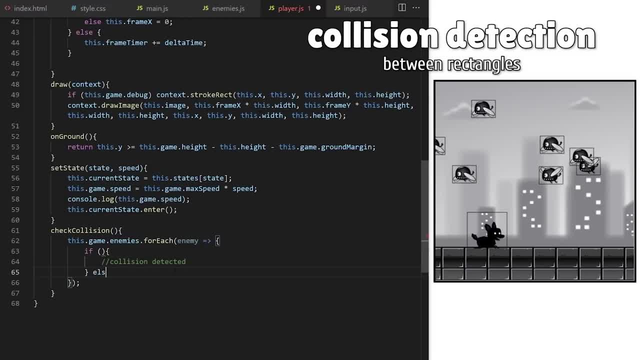 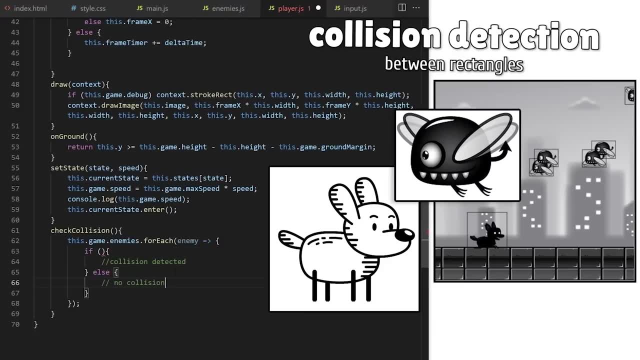 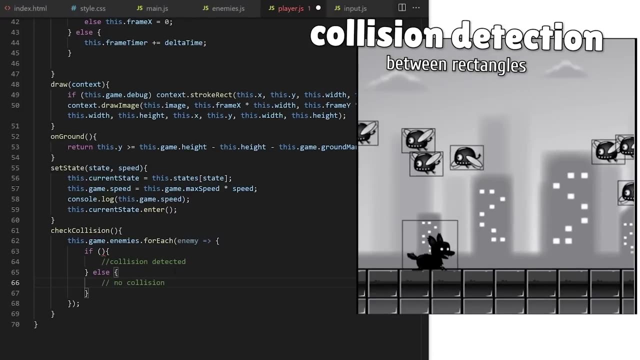 If some conditions are met, collision is detected. else there is no collision. To check if two rectangles collide, which means they touch or they overlap, we have to compare their xy, width and height. Keep in mind that the way images or sprite sheets are drawn on canvas, we go from their x and y coordinates from the top left corner of the image to their width and height, like this: 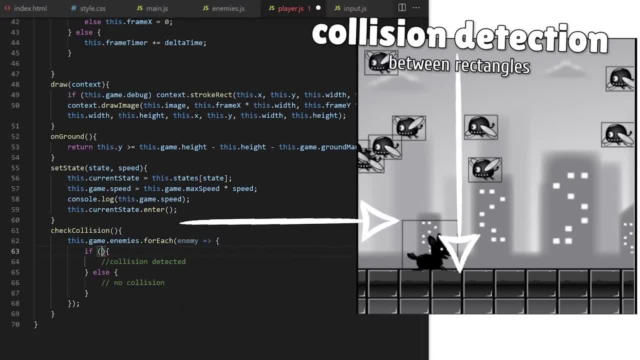 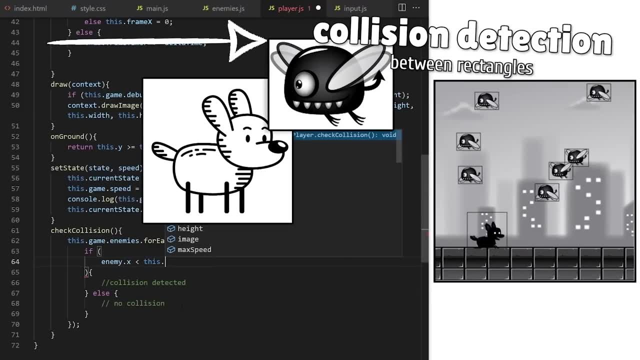 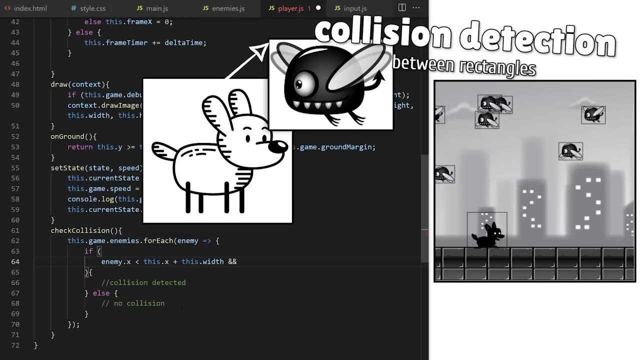 So now player's current horizontal x position is here And vertical y position is here. For example, We need to check if x coordinate of this enemy is less than x coordinate of the player plus player width. If this point is less, or to the left on the horizontal x axis from this point. 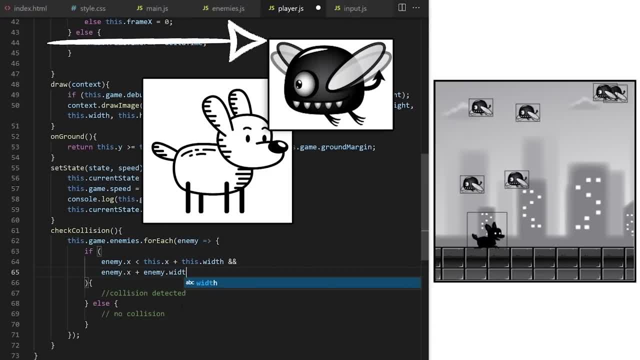 At the same time, we check if x coordinate of the enemy plus the width of the enemy is more than the current x coordinate of the player. If this point is to the right of this point, If these two conditions are true, we know that the player and enemy are colliding. 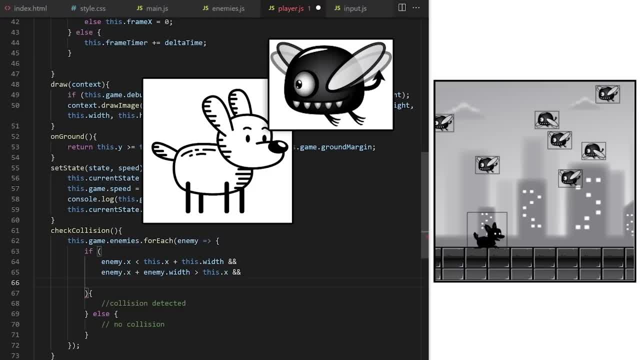 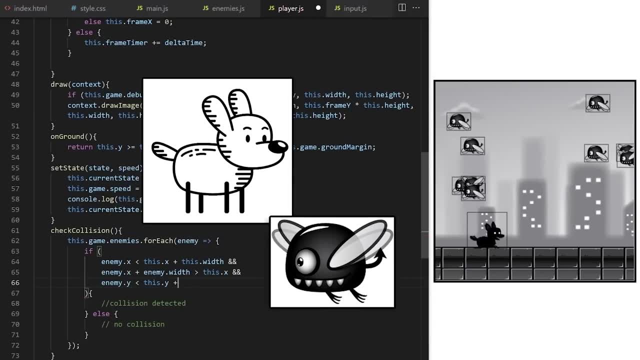 We still don't know if they collide because they could be far away from each other vertically. We will need two more checks here. We check if the enemy's current vertical y position is less than vertical position of the player plus player's height. We check if this point is above this point. 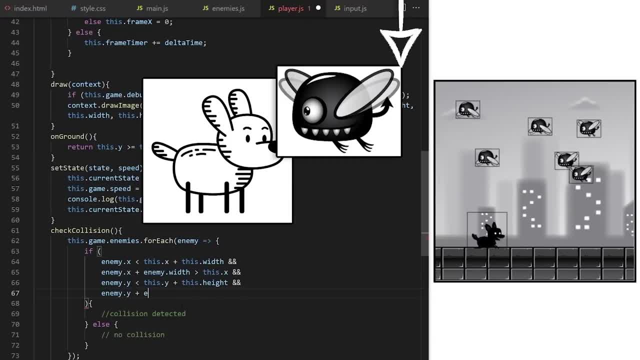 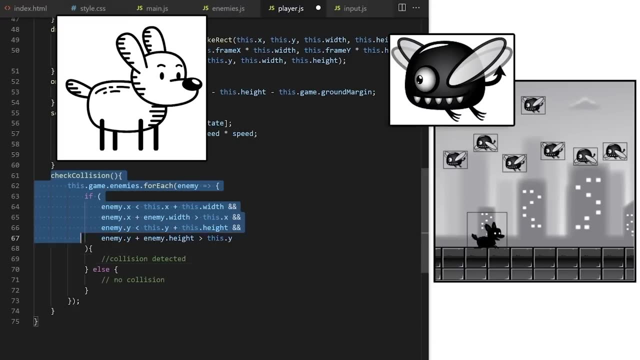 And finally, we check if enemy's y position plus its height is more than y position of the player. If this point is below this point, Only if all four of these conditions are true, Player and enemy are colliding. Even if one of these is false, this entire if statement will evaluate to false and we know there is no collision. 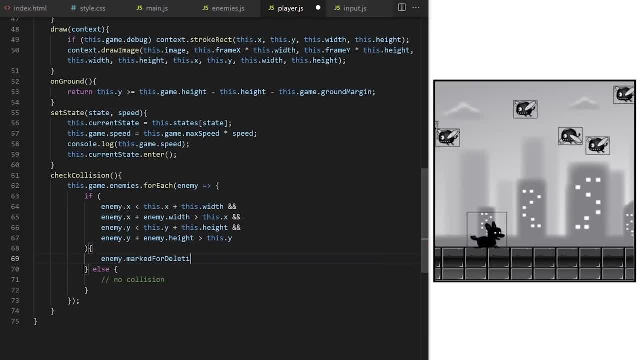 If we collide we will set marked for deletion property on that enemy object- the true. I will also add one more score point. so thisgamescore++, I save changes and in mainjs I need to create thisscore property and initially I set it to zero. 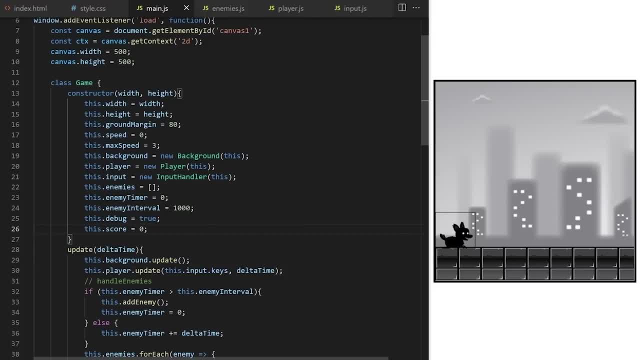 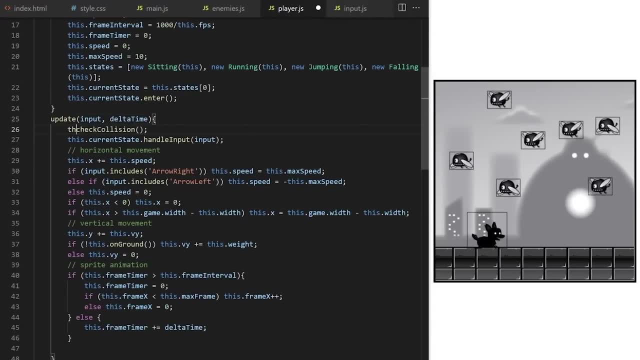 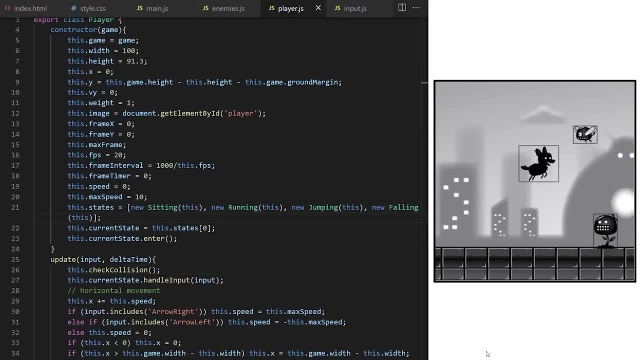 Now I go back to playerjs. I take our new check collisions method and I will be constantly calling it over and over from up here inside the update method Like this: And we have interactions in our game: Whenever the player hitbox touches a hitbox of any enemy, that enemy gets deleted. 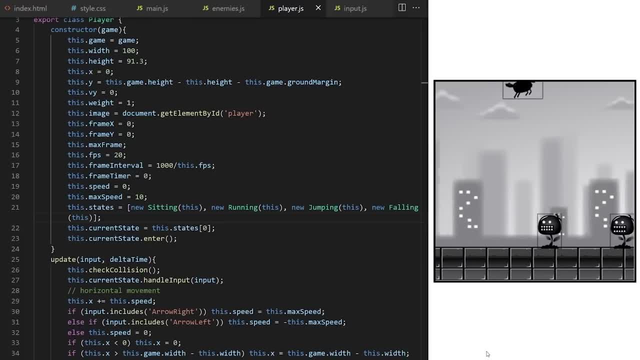 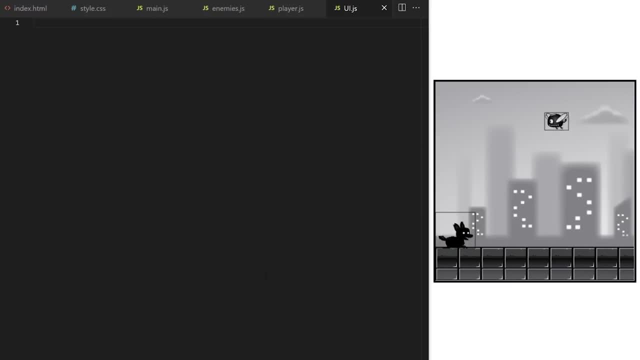 Perfect. Whenever we destroy an enemy, we are also increasing our score. But we can't see it yet. Let's create some UI elements. I create a new file called uijs. Inside I create a custom class. I call, for example, ui and I will be exporting it. 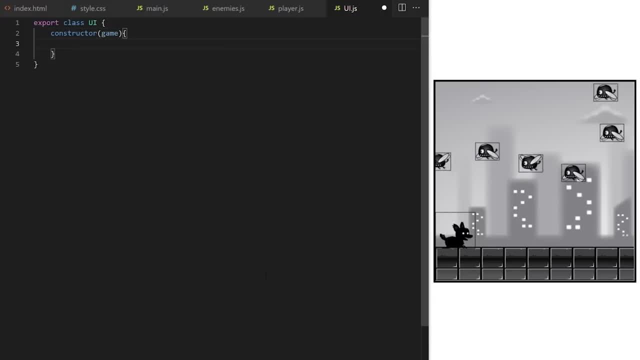 Be careful about lowercase and uppercase letters with the word UI. Make sure you spell it the same across our codebase. Constructor will need a reference to the main game object because that's where the current score value is stored. I create a property called font-size and I set it to 30 pixels, for example. 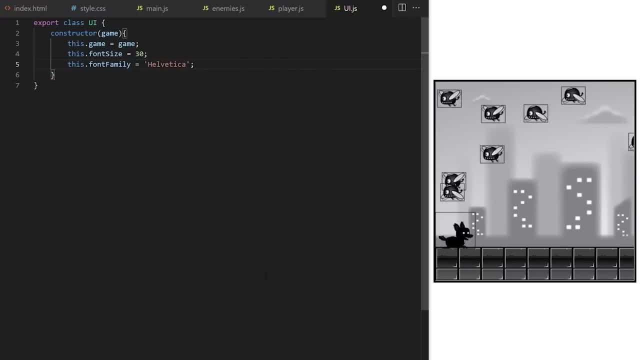 Font family will be Helvetica. You can also use any Google fonts here. Just link them in indexhtml And use their font family name here. if you want to, It will work. This UI class will have just one method. I call, for example, draw: 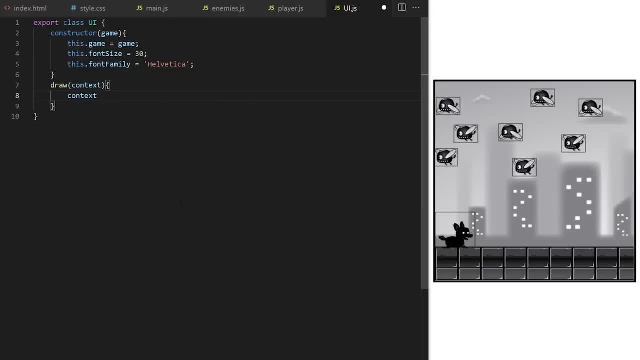 It's job will be to draw all UI elements and game statuses that we need. First I declare some basic settings. Contextfont will be thisfont-size plus pixels, space plus thisfont-family. In this part we will declare code that's specific to draw in score. 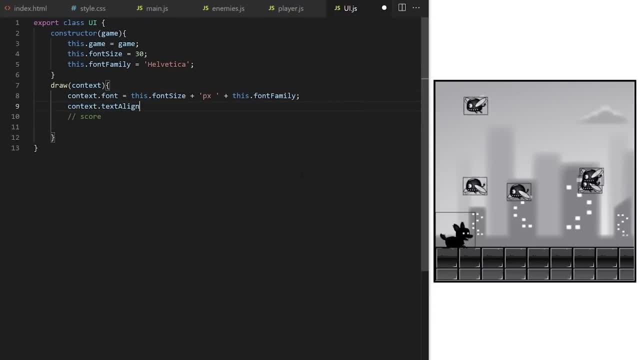 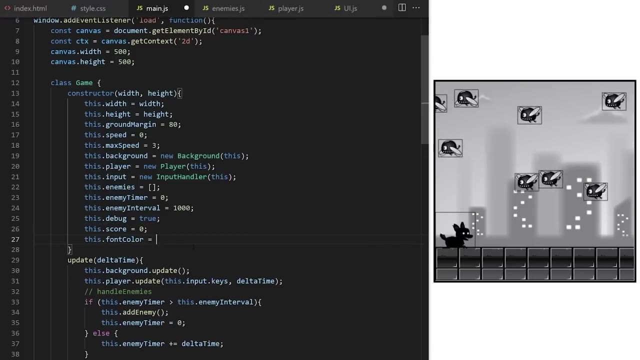 Up here some more global settings. Text align will be left And fill style for all fonts will be kept on the main game object, in case we need to draw fonts from some other modules as well. Thisgamefont-color- It doesn't exist yet, so I declare it here on line 27 in mainjs file. 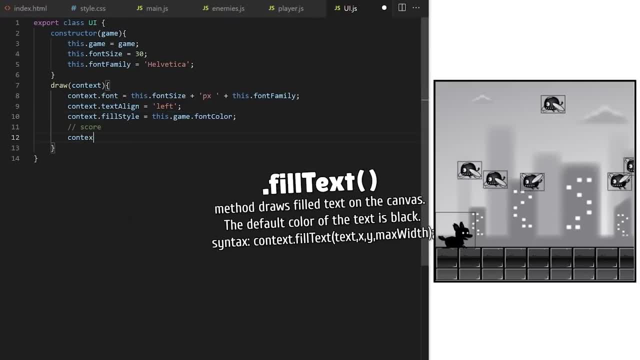 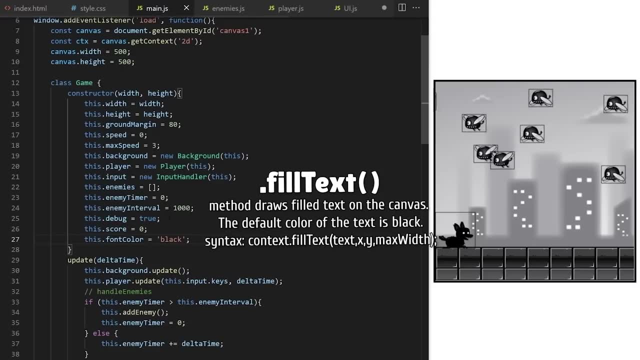 To draw score. I call built-in fill text method and I pass it some text. we want to draw. So score: colon space plus thisgamescore. That's a variable from line 26 in mainjs And I want it to be drawn. I want it to be drawn at coordinates 20, 50.. 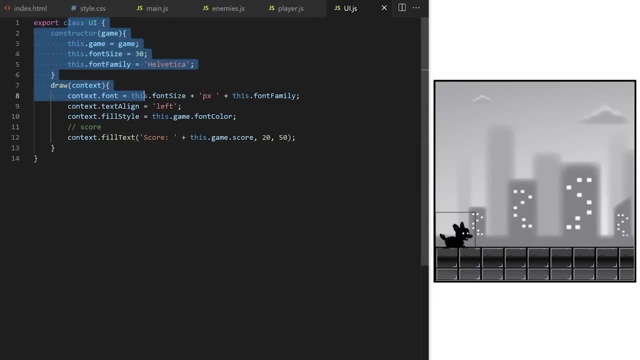 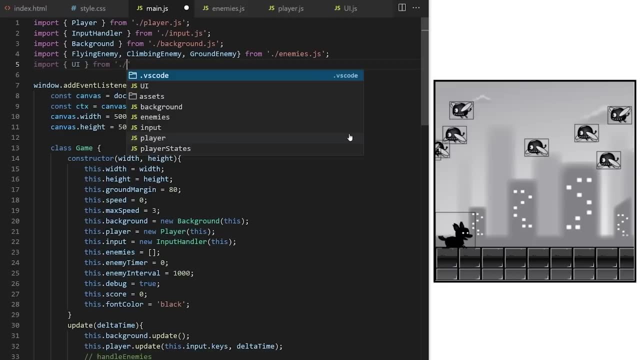 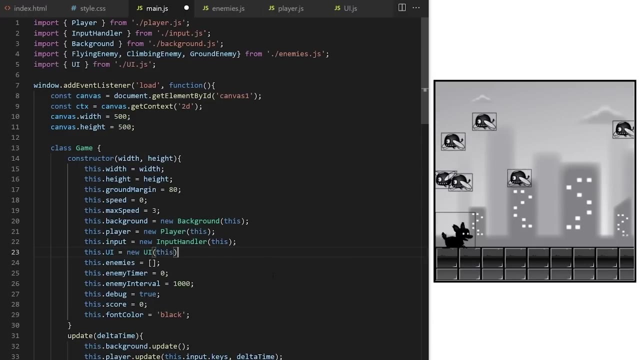 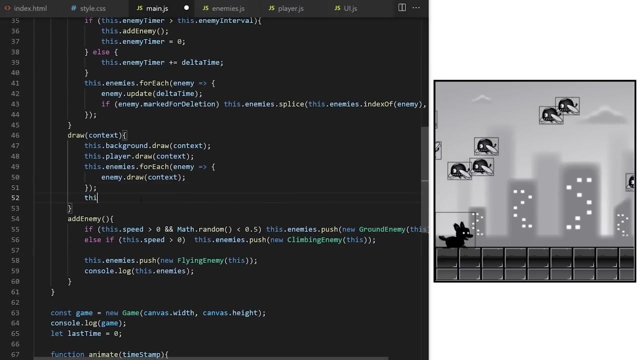 We are exporting our new UI class up here so we can import it to mainjs like this: I will instantiate UI class inside game class constructor, as usual, and I pass it the reference to the main game object. so this keyword Inside draw method on game class, I take thisui property that holds an instance of our new UI class. 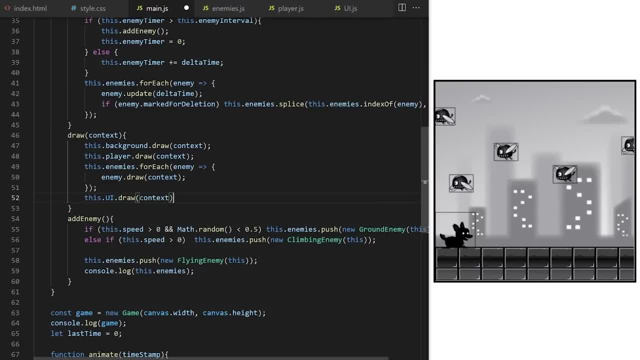 Be careful about capital letters here. And I call its draw method and I pass it context Perfect. We are drawing score and it's increasing as we collide with enemies, So this is how I like to handle drawing game text and statuses. If we want to display more information to the user, we can just add more code inside the draw method. on our new UI class. 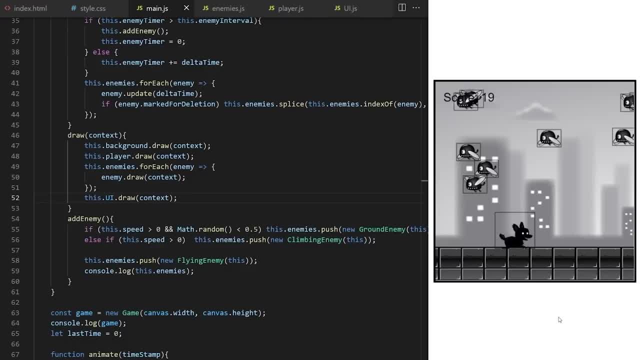 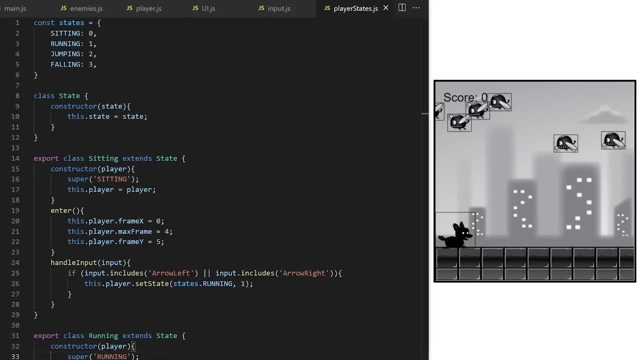 We are keeping our code modular and organized today. It's easy to expand it later. I want to add more player states. We will have two different attacks and a separate state that will play dizzy animation when the player gets hit by an enemy. Let's go ahead and add them up here inside player statesjs into our enum object. that holds key value pairs and it assigns each state number a more human readable value. 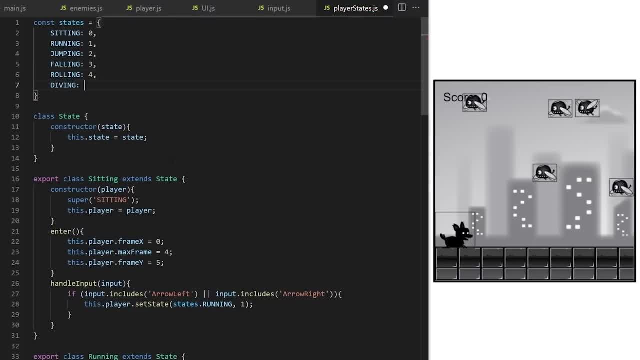 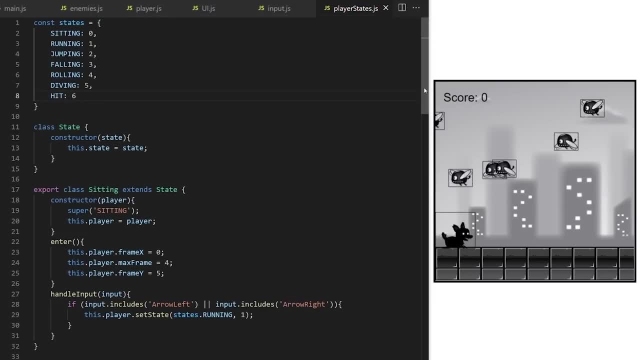 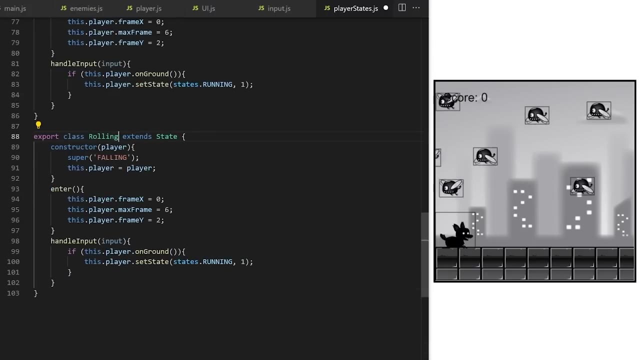 We will have rolling state with index 4, diving state with index 5 and hit state with index 6 for when the player gets hit. I copy this in progress. I change the entire code block and I rename it to rolling. I will also put rolling in all caps here. 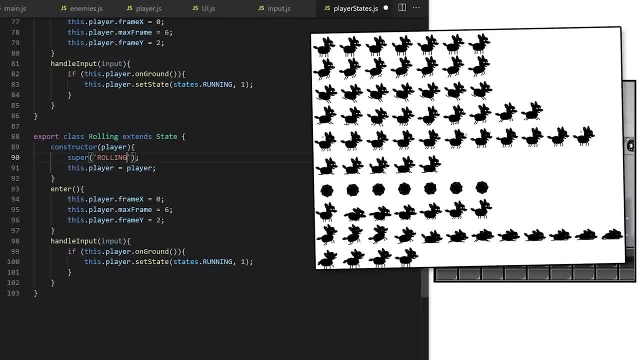 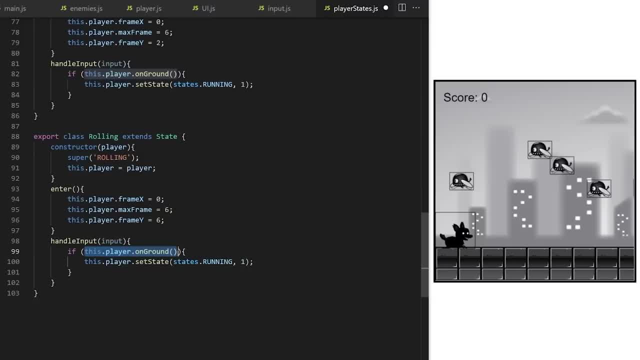 I check my sprite sheet and I can see that rolling animation is on the row 6, counting from 0.. So frame Y is 6.. I want player to start rolling when we press enter And I want it to keep rolling as long as enter key is pressed down. 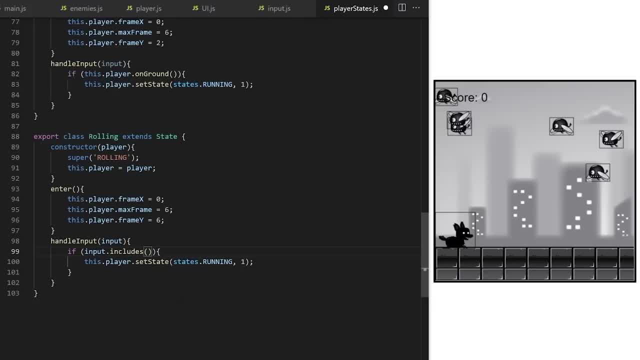 Inside handle input we deal with switching states. We only want to switch player to a different state when enter is not pressed anymore. So If input doesn't include enter and at the same time if player is currently on ground, we can exit rolling state and switch the player into running state. 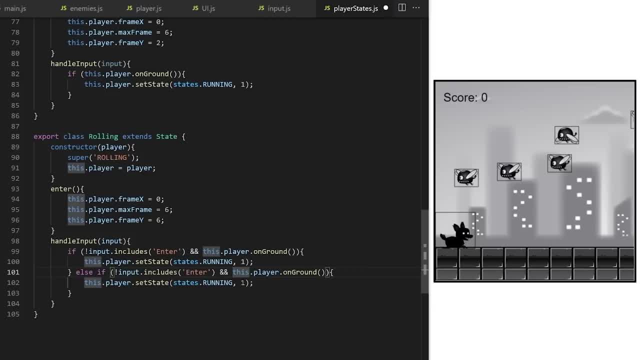 Else if input doesn't include enter and player is not on ground. if we stopped rolling in the air, switch into the falling state. like this, We have our rolling state. Now we can decide from which states we will allow the player to enter rolling. In this case, I will allow it from all states. 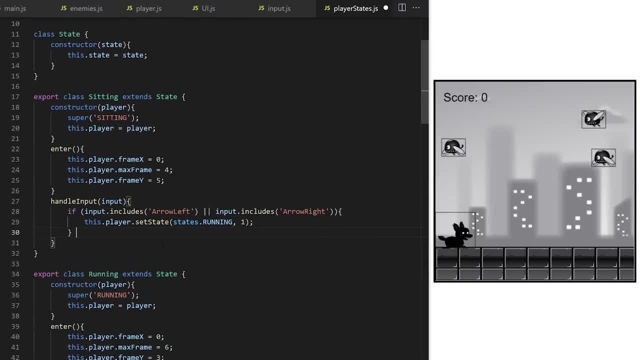 Because player can start rolling anytime Inside handle input method. on sitting class I say Else: if input includes enter, set state to rolling and pass it speed of 2. Rolling will increase the scrolling speed of our game compared to the regular running speed. I take this else statement and I paste it down here inside running class. 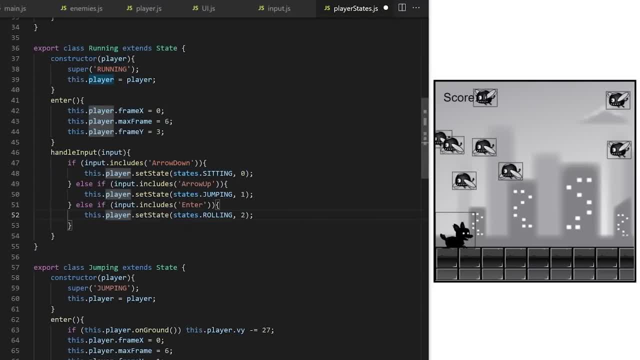 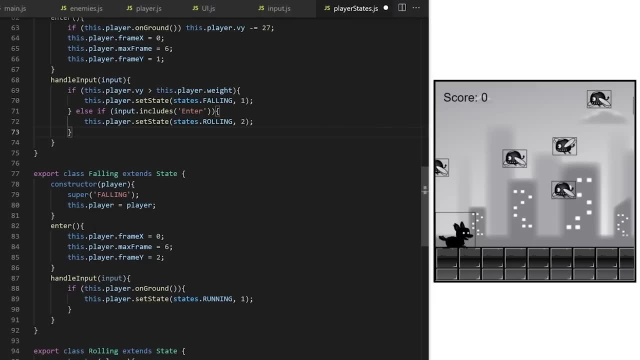 We can also start rolling when we are running. I do the same in jumping class. We can also start rolling while we are in the middle of a jump. For now, I will not allow player to start rolling while it's falling. Let's see how that feels. 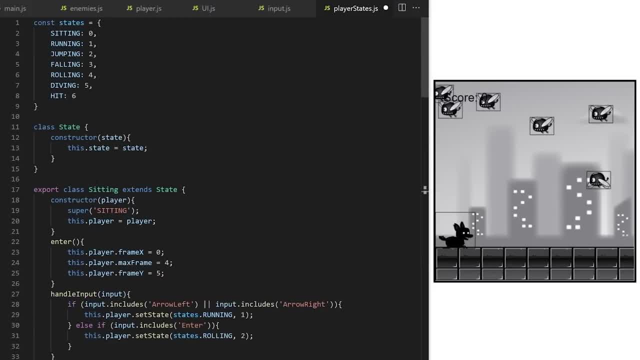 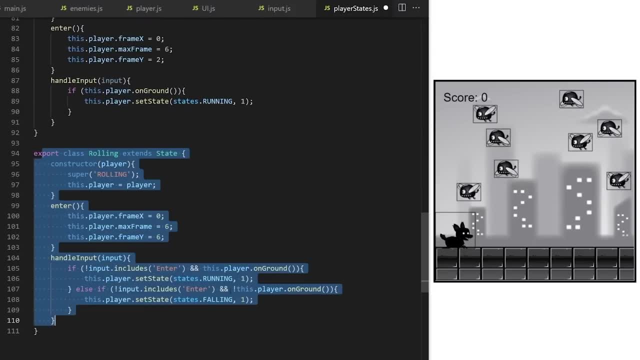 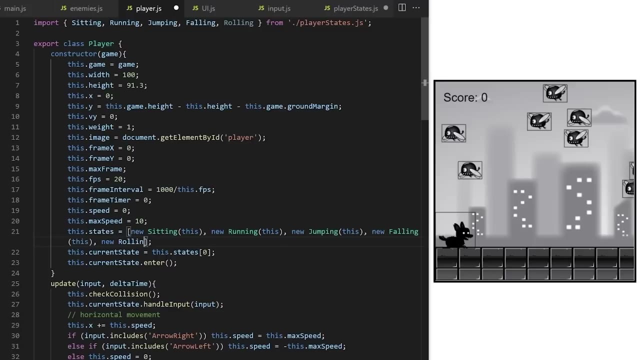 We can always add it later. So now we have rolling with a value of 4 up here inside our enum and we are exporting rolling class on line 94.. On line 1 in playerjs I import rolling and I create an instance of it inside thisstates array on line 21.. 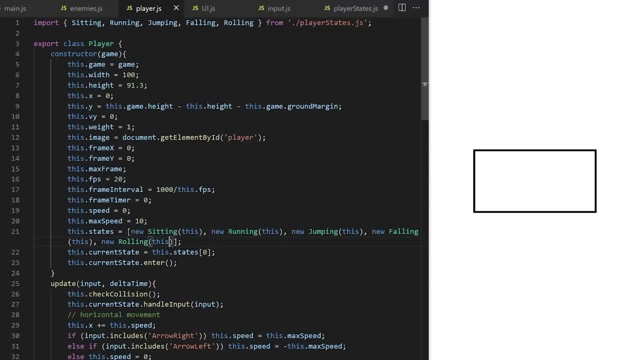 I get an error, It's because I didn't save changes. I made two player statesjs VS. code editor indicates that you have unsaved changes in a file. with this little icon, here I go in, I save it And now I can press enter and I can roll around. 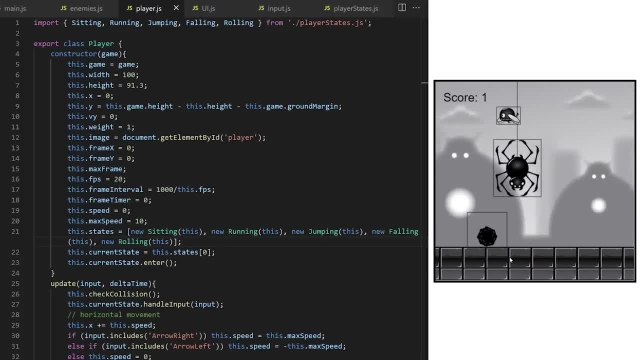 Nice work. I can start rolling from running state, from sitting state and from jumping state. I'm testing my gameplay and I feel like I would like to start a jump in while I'm rolling on the ground like this, But the game won't allow me to do that. 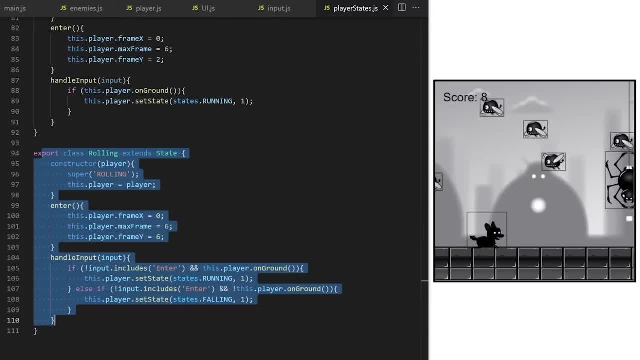 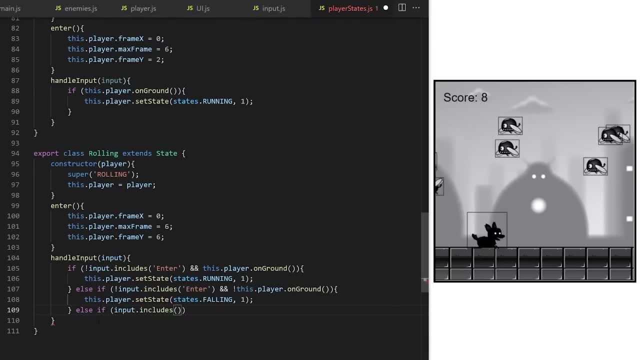 I can't enter jump while rolling on the ground because we didn't write that behavior. Let's do it In handle input method. on rolling class, I say if input includes enter, which means we are rolling, And if input also includes arrow up at the same time. 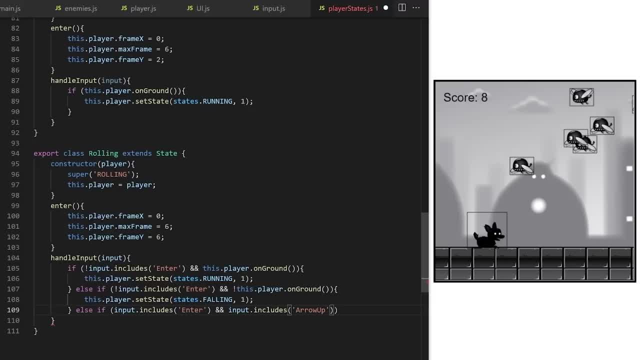 Remember that our input keys array can hold multiple keys at the same time. If enter and arrow up are pressed at the same time And if we are rolling on the ground at that moment- So thisplayer on ground is true- We will push player up in the negative direction on the vertical y axis. 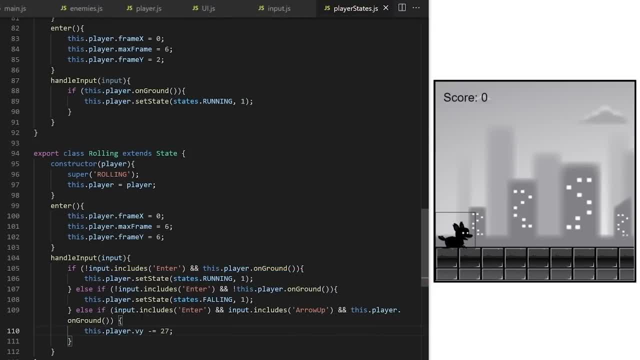 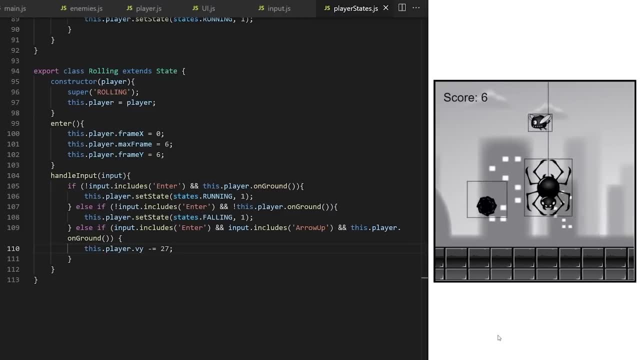 Thisplayer, velocity y minus equals 27.. Now I can roll around and I can jump up and down like this. This feels much better to play. This is a superhero dog. I want the controls and movement to feel good and quick. This dog can roll and jump around freely and the controls are very precise. 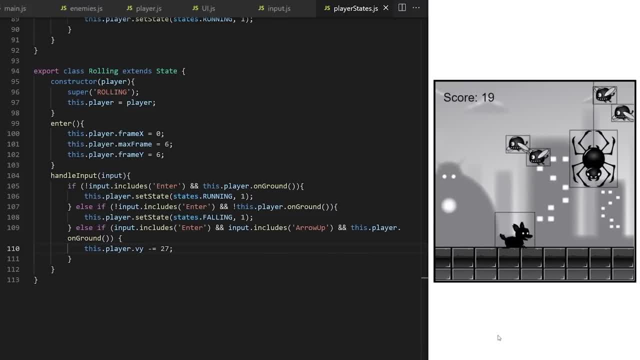 Time to add some particle effects. We will have three different particle types in this game: Dust that comes from the ground at player's feet when it runs on solid ground. Blazing fire trail when the player runs on solid ground. When the player is rolling and diving. 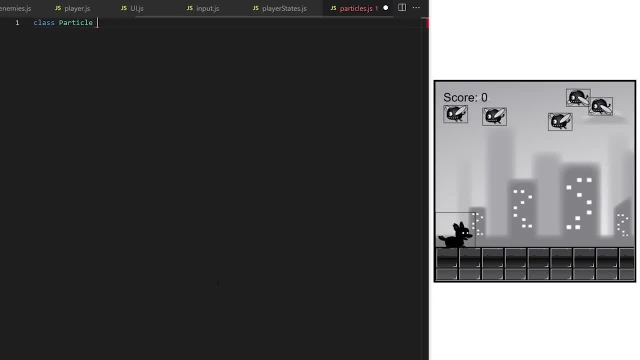 And a big splash of particles when we dive and stomp into the ground. I create a new file I call, for example, particlesjs. Inside we will have the main parent class called particle. I will not be exporting it, It will just contain properties and methods shared between all three particle types. 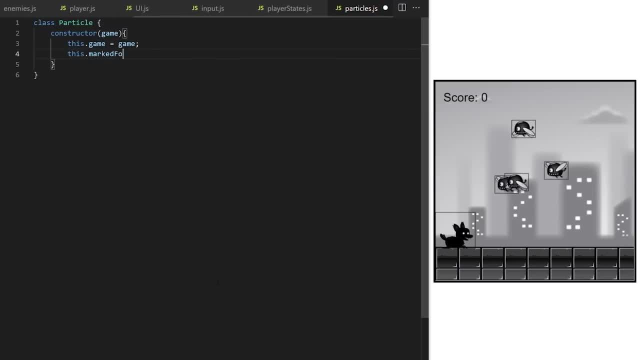 Constructor will need a reference to the main game. object Marked for deletion will be false at first. Update method will also have some code shared between all particle types. Horizontal x coordinate will decrease Despite the amount of speed x and game speed like this: 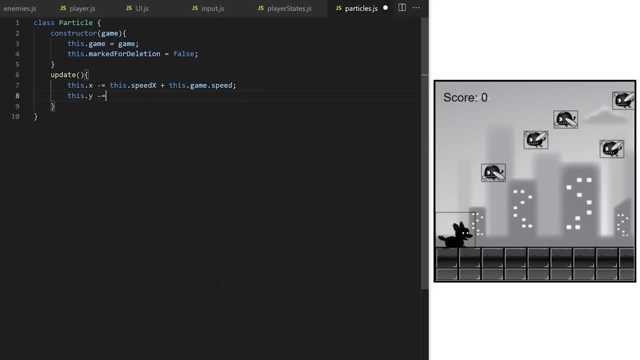 Vertical y coordinate will be affected by speed y property. For every frame, the size of each particle will decrease by 5%. When size is less than 0.5 pixels, the particle is small enough and we will set its marked for deletion property to true. 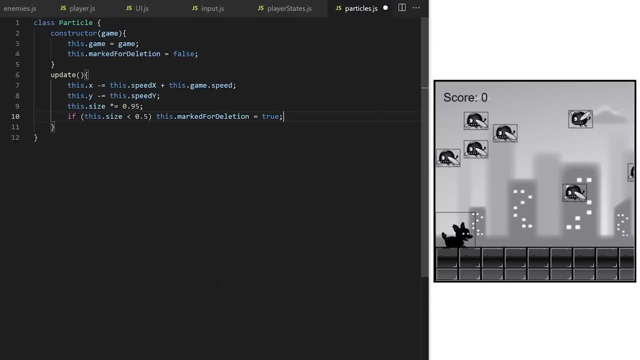 Values like speed, x and size don't exist, yet I didn't declare them on the main particle class because they will have different values for each particle type. We need to make sure we define them on the child classes because if javascript can't find these properties when update method runs, we will get an error. 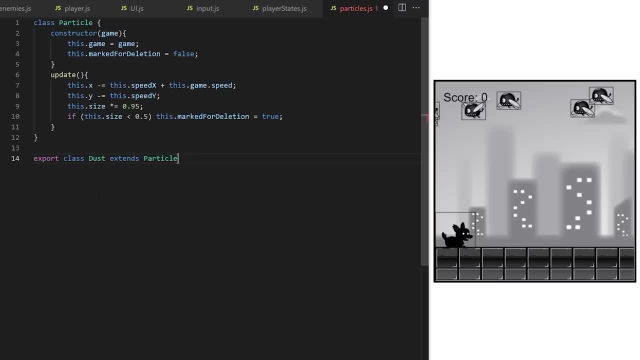 So child class I call dust extends parent particle class. We will be exporting it. We will also have splash particles for when we hit the ground at high speed and fire particles for the attack animations. I start with the dust class Constructor will need a reference to the main game object and x and y coordinates because the location of the particle will depend on the player's script. 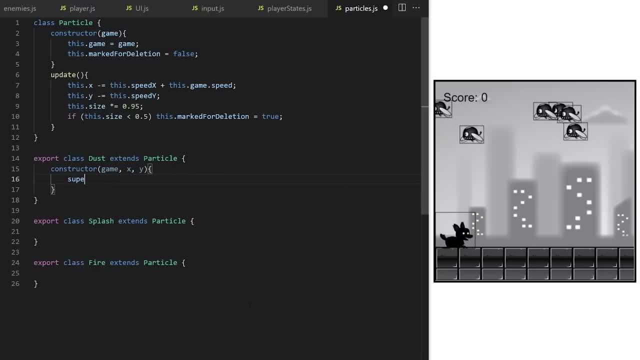 We want them to appear under the player as it moves around. I call super and pass this game along because it's expected up here. This will trigger class constructor on the parent particle class, activating all shared properties. Size of dust particles will be a random number between 10 and 20.. 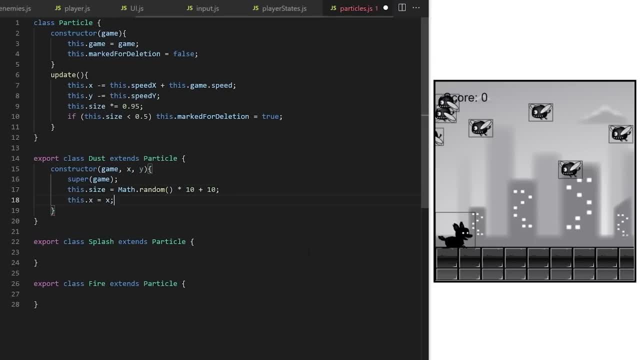 X coordinate will be x. that is passed as an argument. Same goes for the y coordinate. Horizontal speed x will be a random number between 0 and 20.. Vertical speed y is also a random number between 0 and 1.. Color will be black. 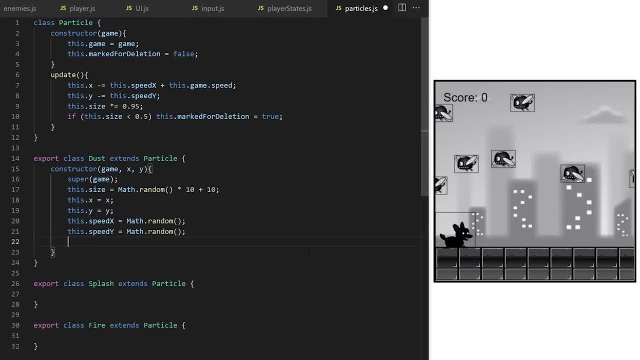 Draw method will take context as an argument. as usual, I want to draw dust particles as circles. so we start with begin path. We create an arc, Add coordinates: thisx, thisy. With a radius, of thissize, Start angle will be 0.. 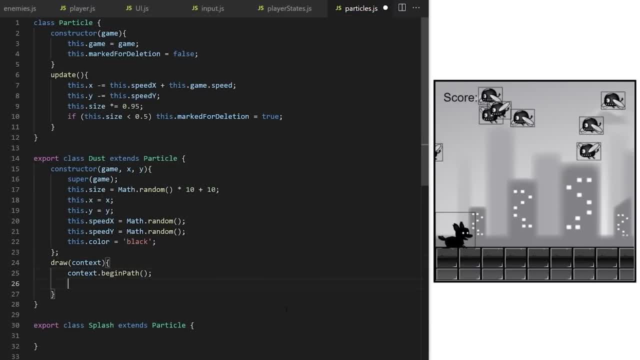 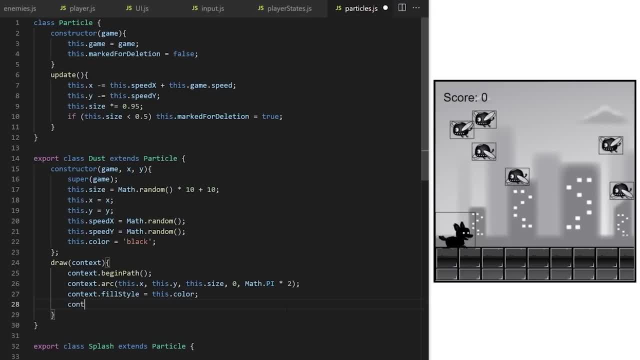 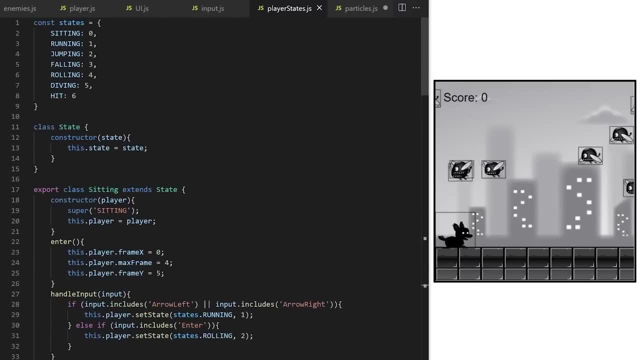 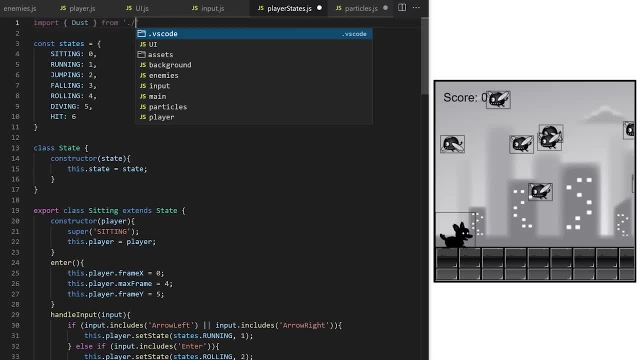 End angle is mathproperties. Start angle will be 0.. End angle is mathproperties. Start angle will be 0.. End angle is mathproperties. Start angle will be 0.. code: I thought I would only need access to the player class, but we need to go one level up and 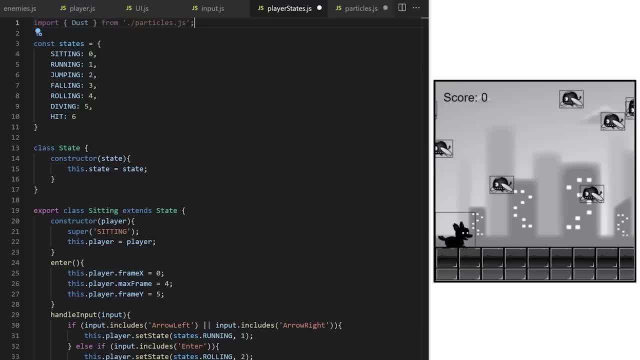 access the game object. This is why it's good to plan your code bases well before you start writing the code. I will have to do a little bit of refactoring here to make sure we have access to the main game class from within each individual player state class. Here on line 14, I pass the 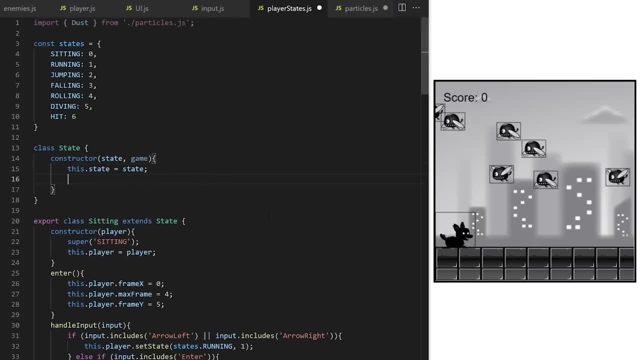 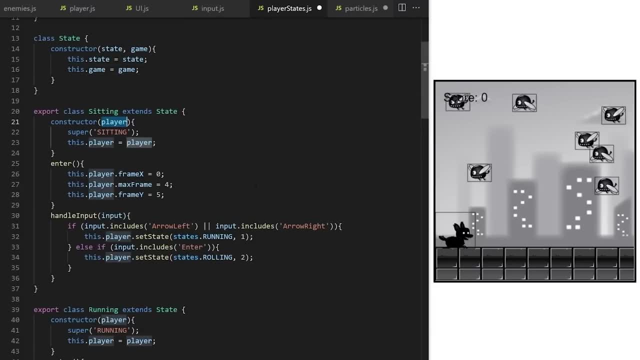 main state parent class. a second argument called game and inside I convert it to class property. thisgame equals game. I want to replace all references to the player object with references to the game object. Game object contains the player, so I will still have access to the player object. 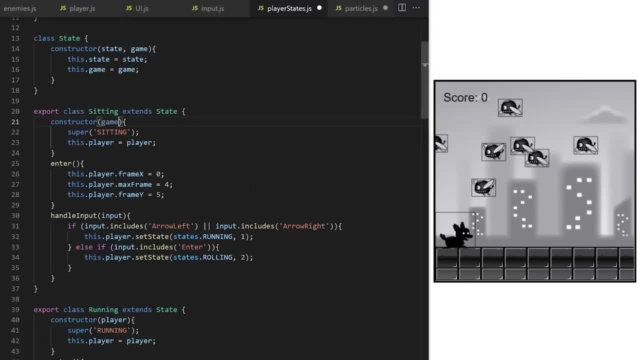 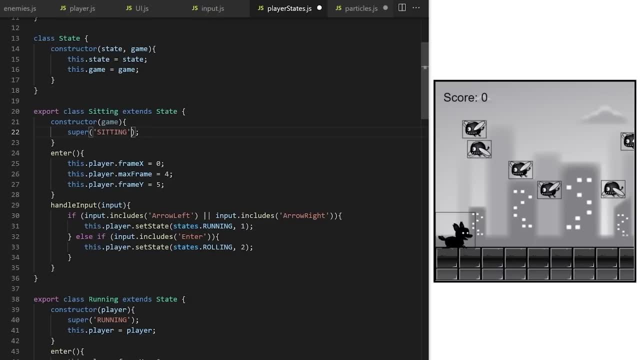 from there. Constructor on the sitting class will expect game as an argument. We delete this line with player. I pass that game object reference along to the parent class constructor as a second argument because I know it's expected here on line 14.. It will get converted to thisgame class. 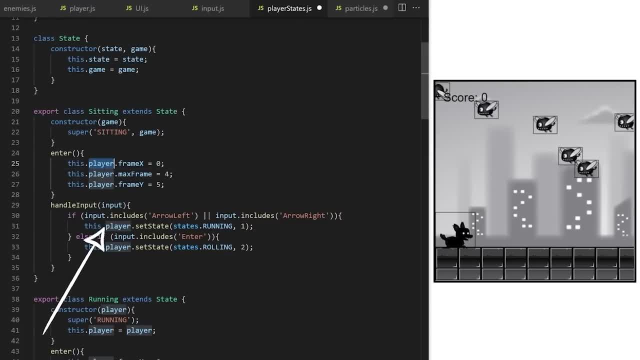 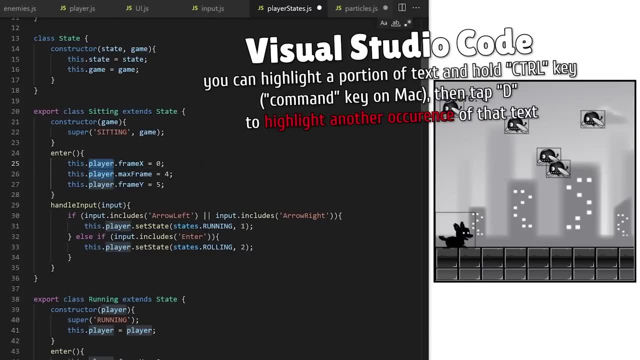 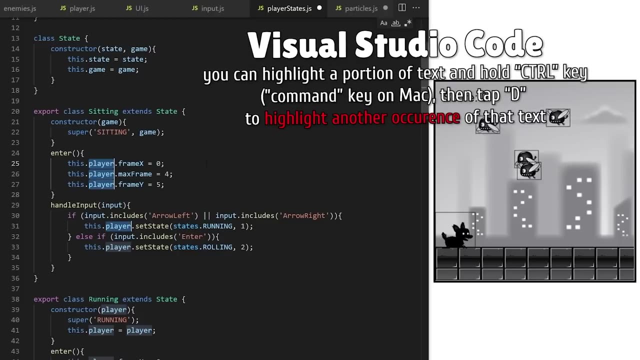 property. Now, if I want to access player in these five places, I need to say thisgameplayer. In VS code, you can highlight a portion of text and hold ctrl key down. then, whenever you tap letter d, it will highlight another occurrence of that text. Using this, you can select multiple lines at the same. 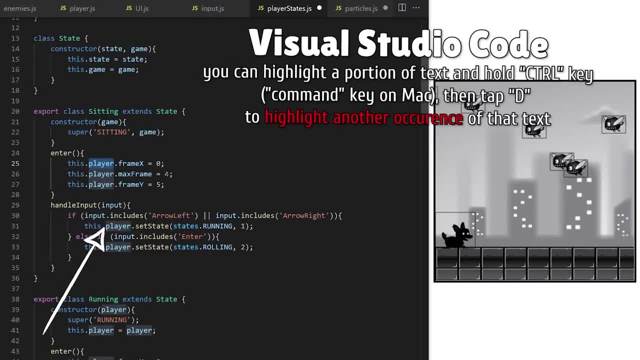 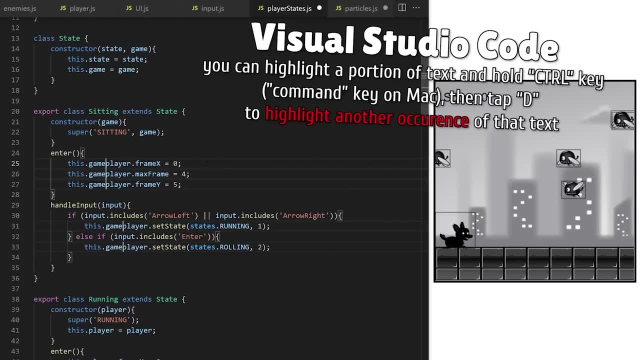 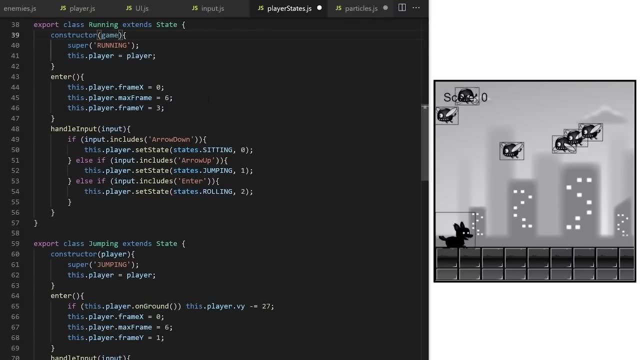 time. I tap d four times to select all five occurrences of this text and that gives me multi-cursor selection. I can use left and right arrows to move around and I just type game. I do the same in the running class, I pass it game, I remove this player line and I pass game as the 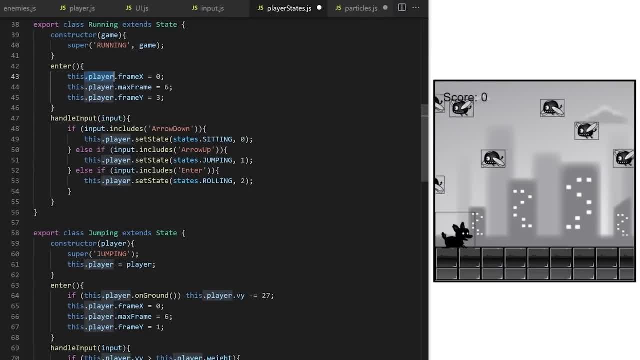 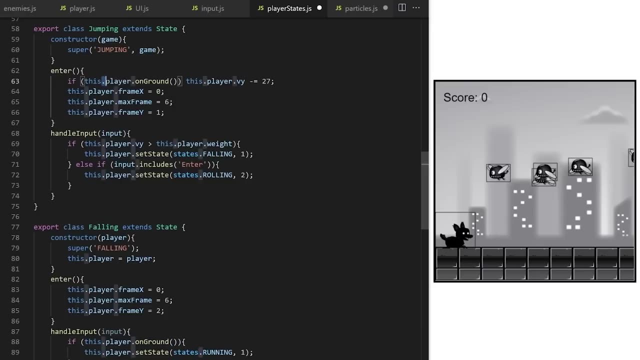 second argument to the super class constructor. Then I select one, two, three, four, five, six, and I need thisgameplayer here in all these places. I do the same in jumping class Refactoring. Sorry, I should have planned this part better. We are almost done. I replace all nine occurrences of thisplayer. 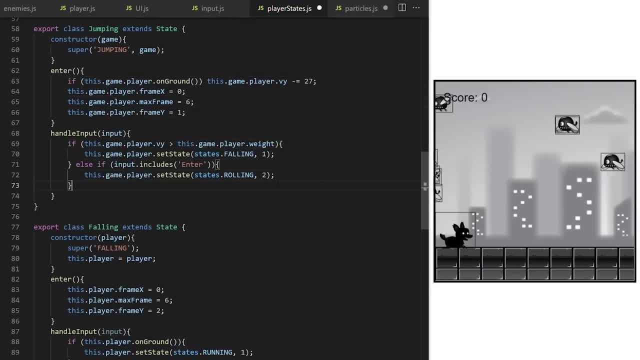 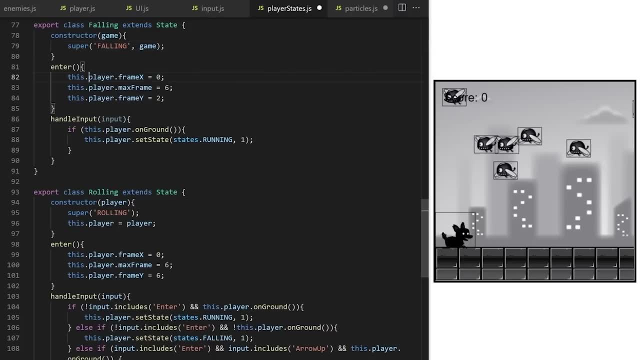 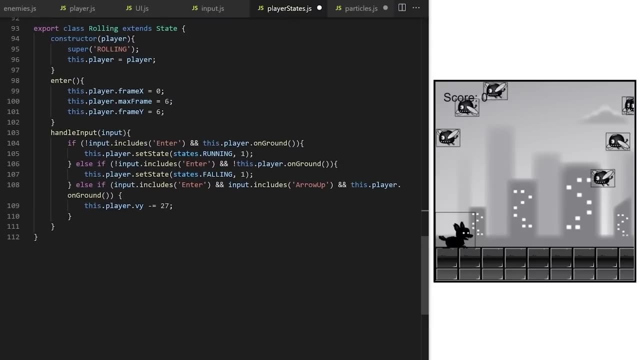 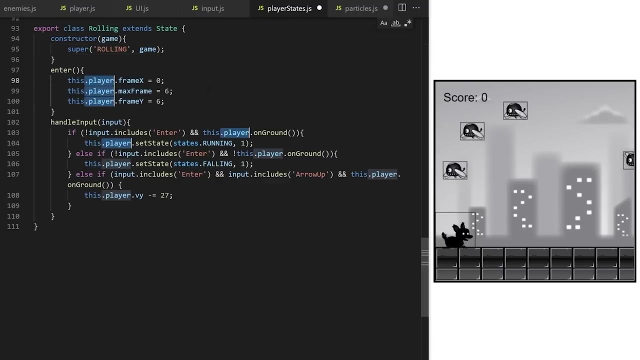 here with thisgameplayer. Falling class doesn't have much code, so this one is easy And rolling class is the last one. we need to refactor 1, 2,, 3,, 4,, 5,, 6,, 7,, 8,, 9 and thisgameplayer. 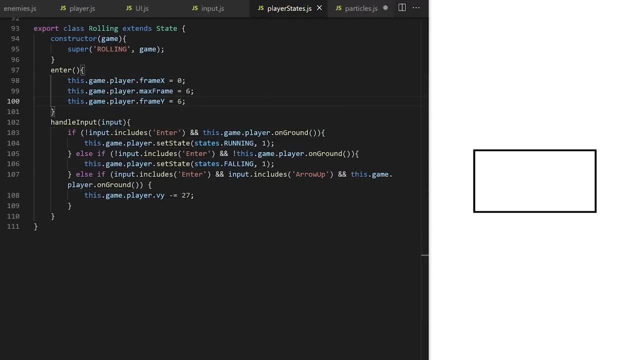 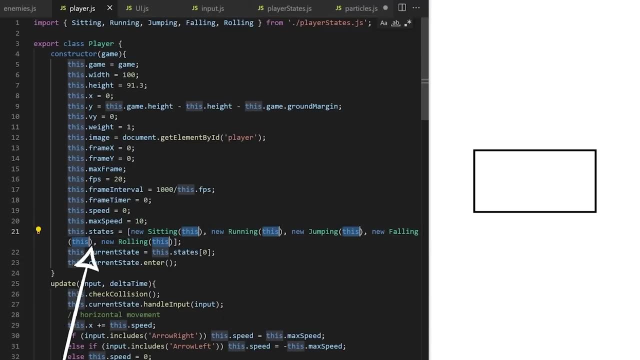 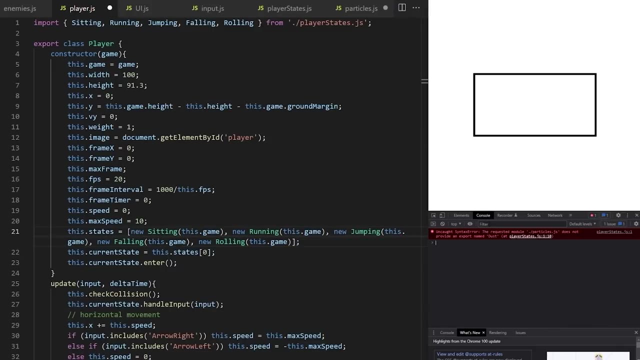 If I save this, it will break our code because our state classes are expecting game as an argument now. So on line 21 in playerjs, we are currently passing this keyword, which means player object. I need to pass thisgame from line 5 instead to all of them. 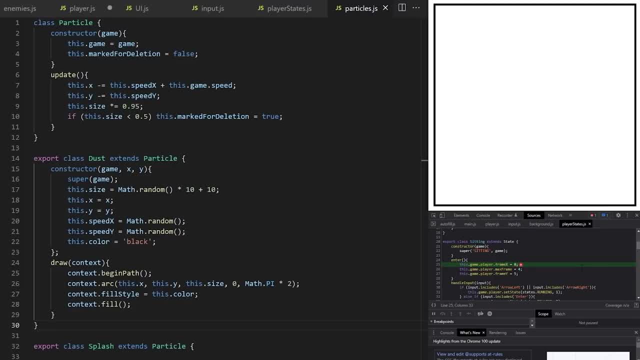 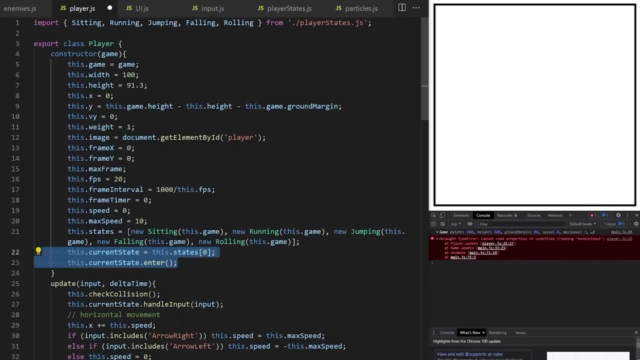 Now we are getting some new errors, and that's because I'm passing game object as an argument and immediately I'm triggering that state class And it's enter method, but at this point the game object is not yet completely loaded, so the initial state is failing. 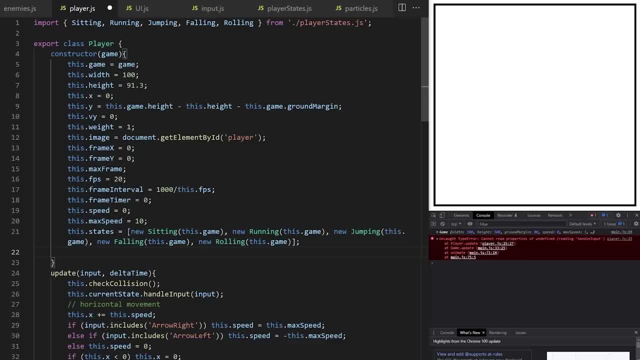 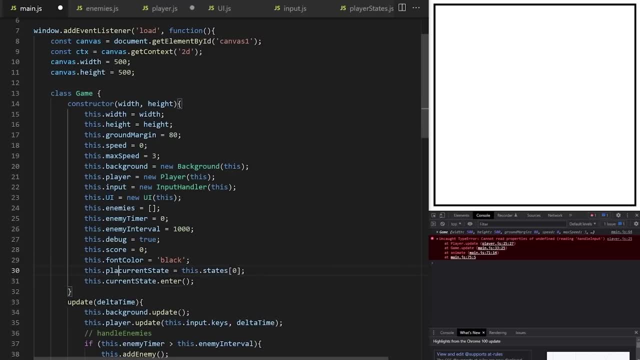 I need to cut these two lines of code and I only want to run them when the rest of the game object is ready. So at the end here, When everything is ready, including game class, player class and all state classes, we take current state property on player class and we set it to states 0, sitting state. 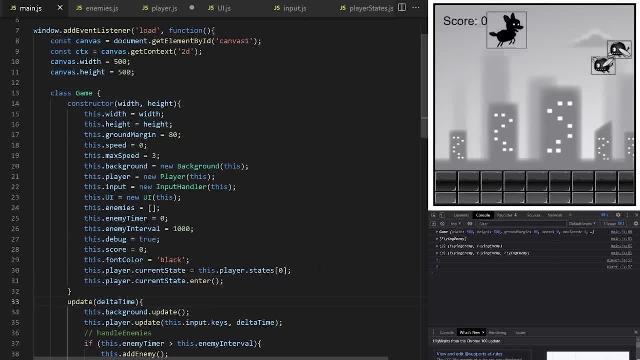 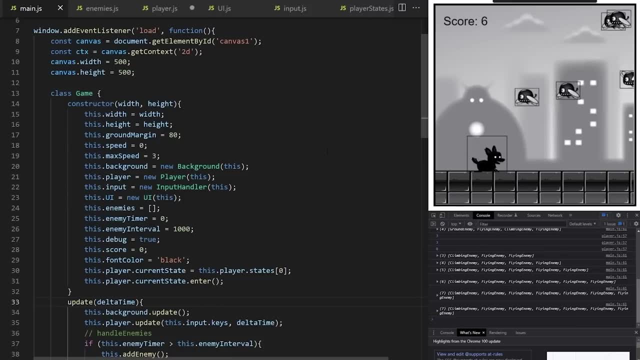 And we trigger enter method on the sitting state. We refactored our code and now everything is working again. We are well positioned to start adding particles through our state classes. We have a lot of console logs here. I press control F and I search for console. 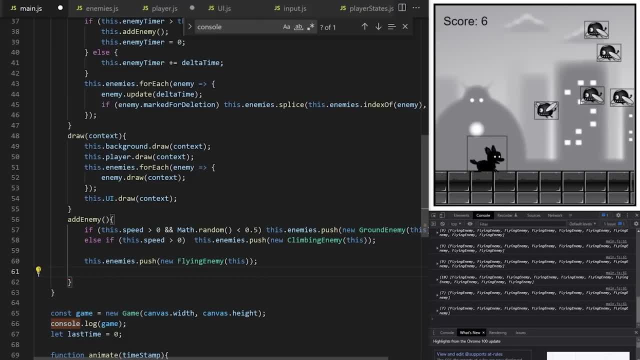 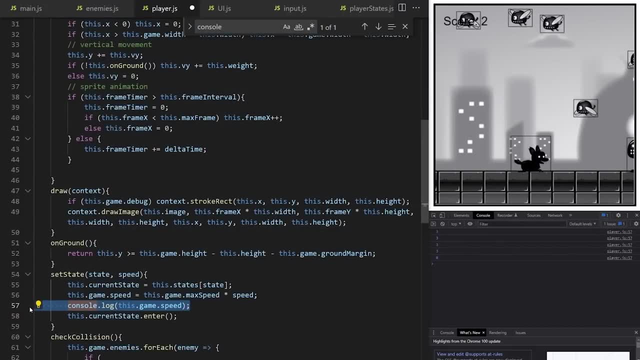 I delete this one on line 61 in mainjs and this one on line 65.. We also have a console log on line 57 in playerjs. I delete it. Debugging is better with a clean console. So we are exporting dust class here. 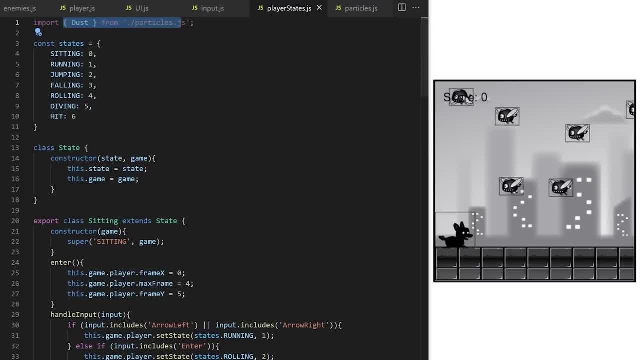 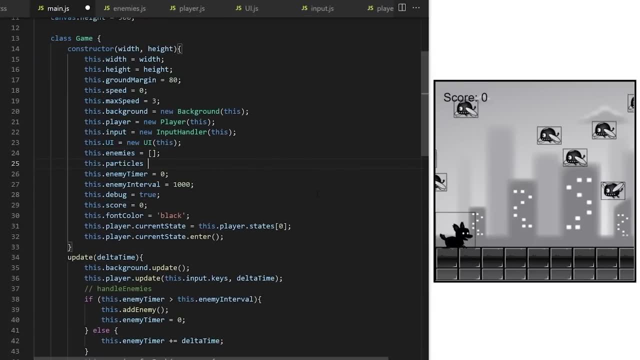 And we are importing it up here in player statesjs. I will hold all currently active particles in an array on the main game object, So I create it here. Thisparticles will be an empty array at first. Back to player statesjs. 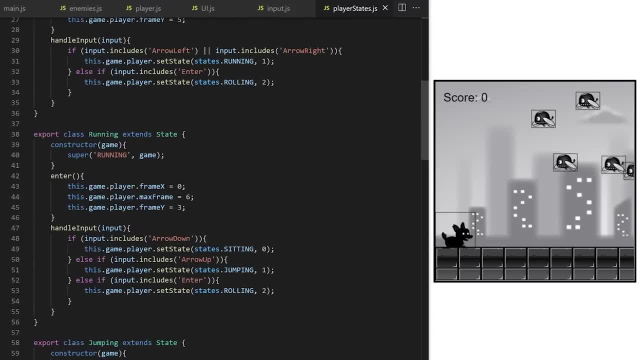 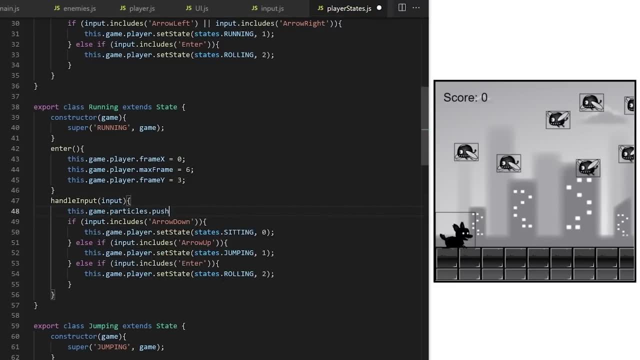 I only want to add dust when the player is running. so inside handle input method on running state that runs 60 times per second. I will be pushing one new particle in every time it runs Thisgameparticlespush and I pass it new dust. 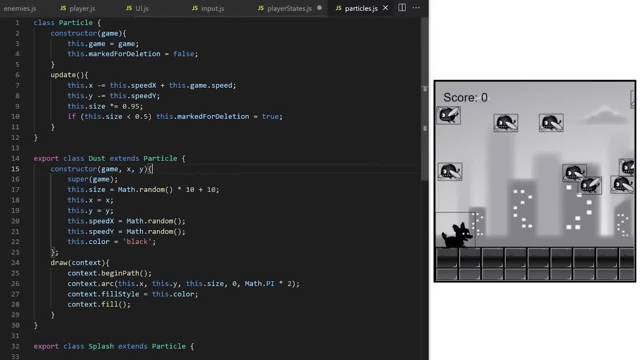 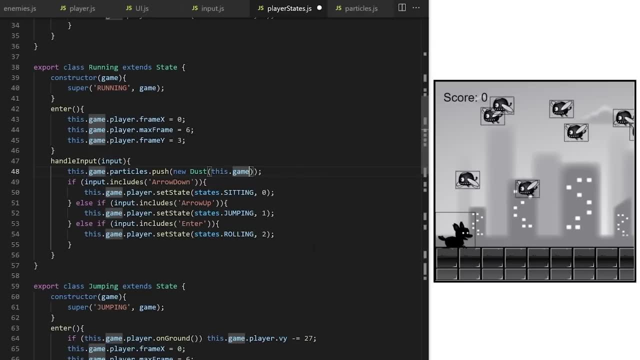 On line 14 in particlesjs I can see that dust class constructor expects game x and y as arguments, so I pass it thisgame from line 16.. I will also be passing the current x and y coordinates of the player because I want the. 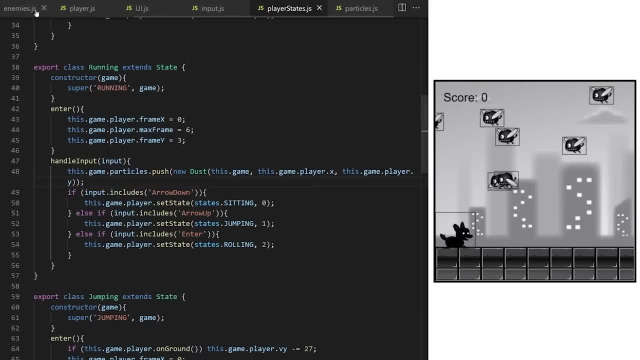 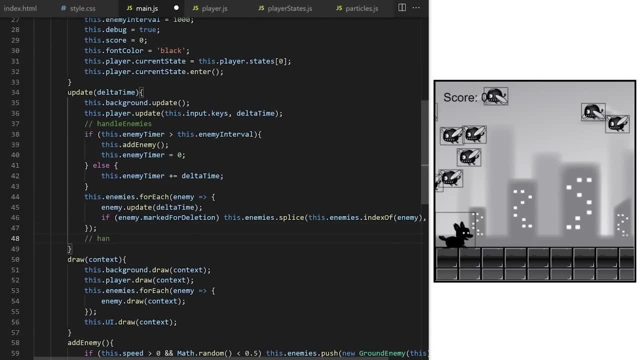 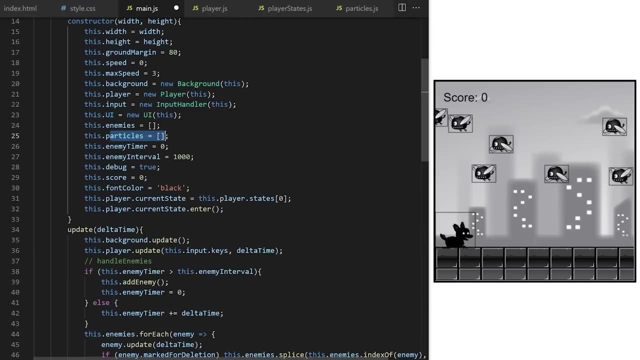 new particles to appear at player's current position. I close some of these javascript files for now to keep our workplace clean. Inside update method on the game class. after this block that handles enemies, we write our code to handle particles. On line 25 we have thisparticles array that holds all currently active particle objects. 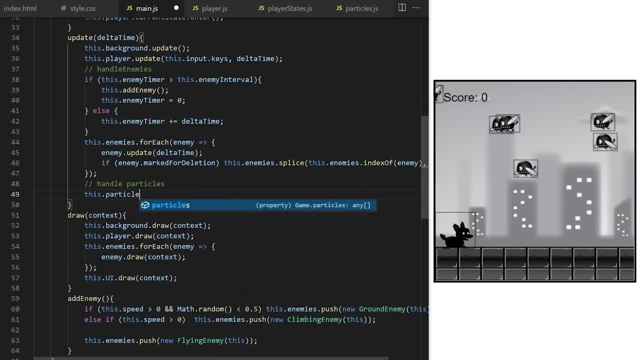 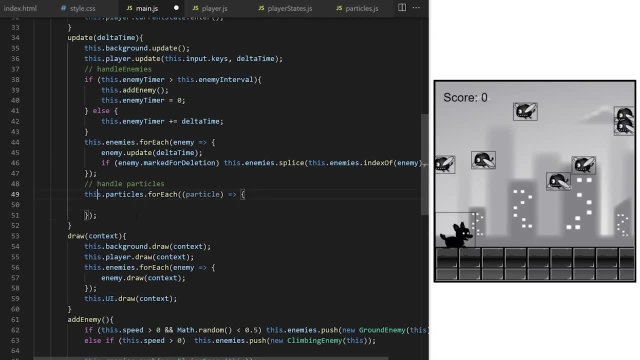 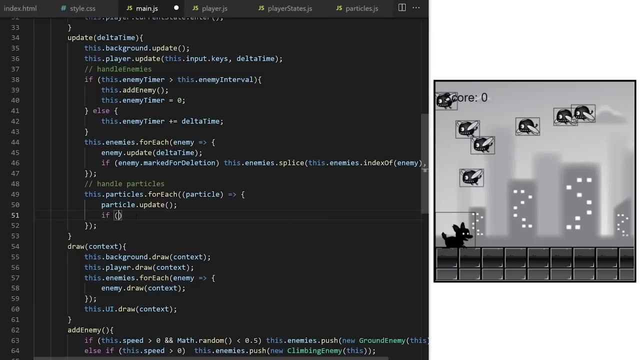 We are pushing new dust particles in here from inside running state class. I take that array and I call for each. For each particle in the array, I will call their update method If particle is small enough and its marked for deletion property has been set to true. 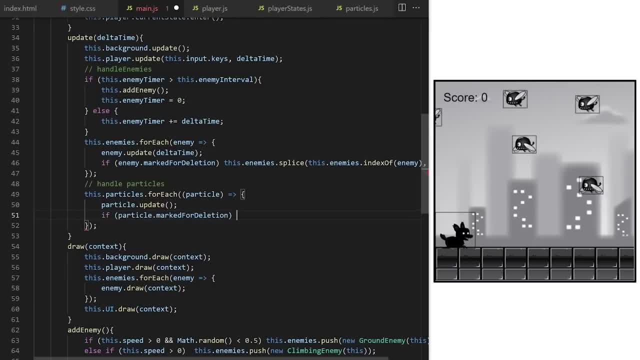 we call splice method. to remove it, Splice method will need index of the particle we want to remove and how many elements to remove, starting from that index. For each method passes autogenerated index argument, so I can just assign it to a variable name here. 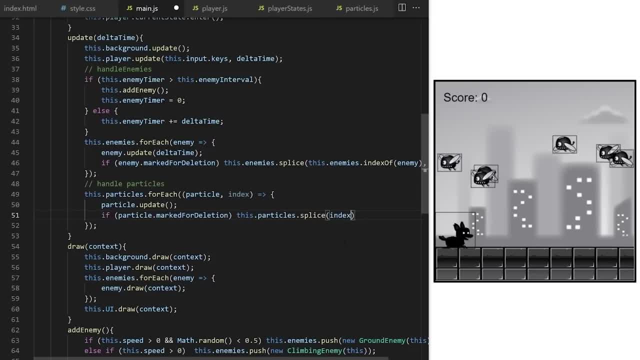 I call it, for example, index and I pass it to splice to identify the particle to remove. and I want to remove one element at this index. So here we call update on all active particles and we delete old ones. Inside draw method. I will cycle through all the particles again and I will call draw method. 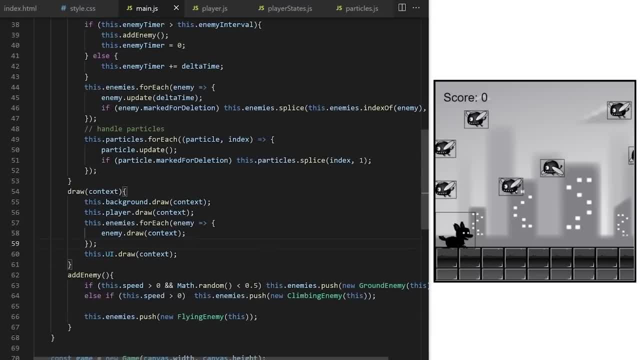 One optimization tip here would be not to cycle through the same array once in update. I will call it draw method and I will call the same array once in update And once in draw method. I can, for example, have utility handle particles function that does all of that. 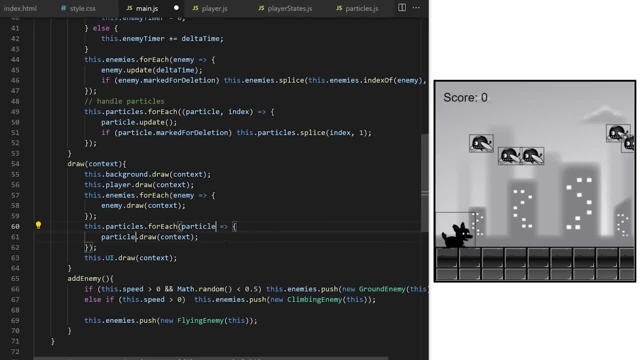 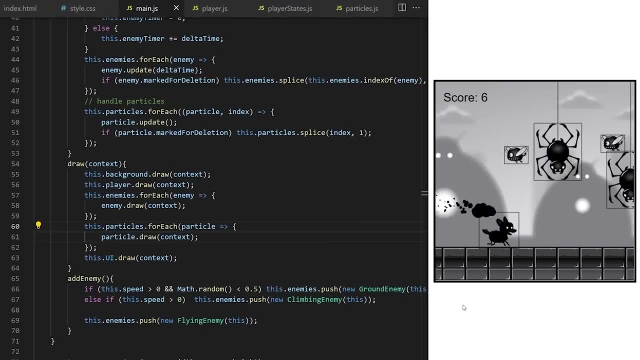 There are many ways to refactor this code. We might do it later. For now, this code will work well. You can see, we are drawing our dust particles from the top left corner of the player hitbox only when we are in a running state. 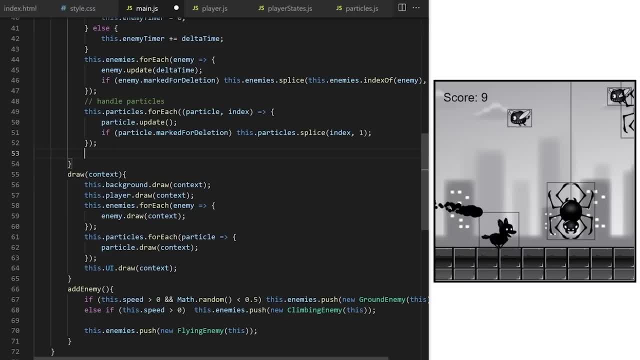 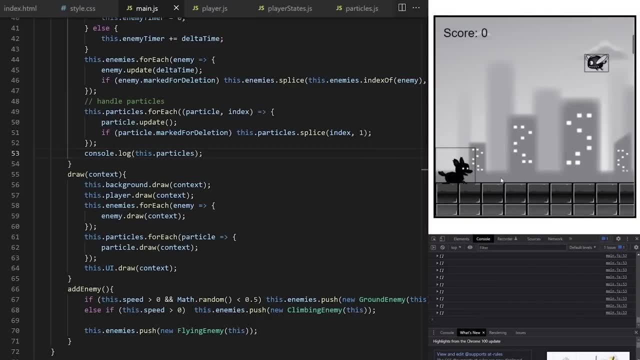 Nice. I will const log thisparticles array to check if old particles are being correctly removed. We don't want to have an endlessly growing array in our project. That would become a performance problem soon. In console I can see that particles go up to 50 or 60 and when we stop running the array, 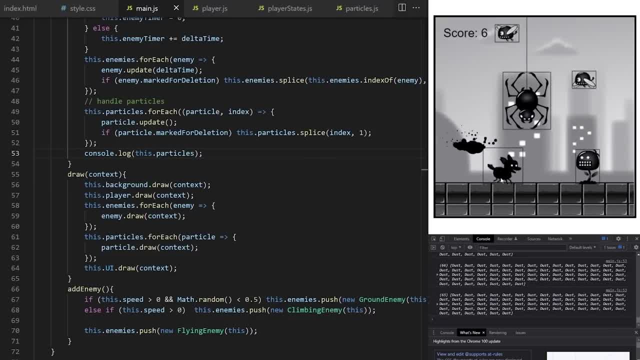 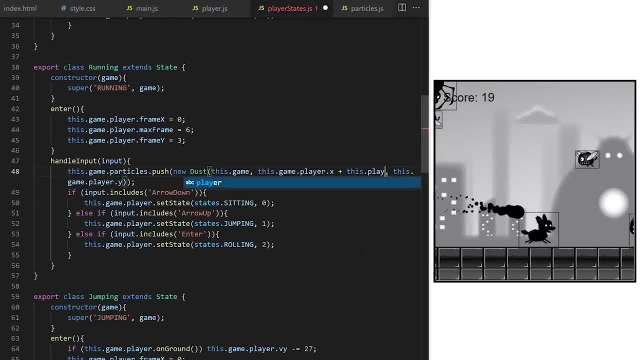 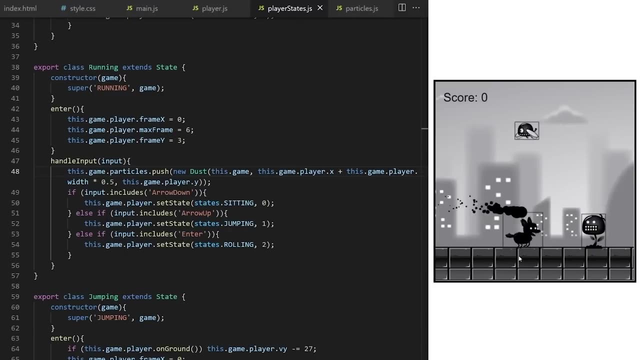 is getting smaller and smaller until it's empty again. Perfect. I want the dust particles to come from a different point relative to the player. I adjust horizontal x coordinate by the half of player's width. like this, I will also adjust vertical y coordinate by player's height, pushing the particles initial. 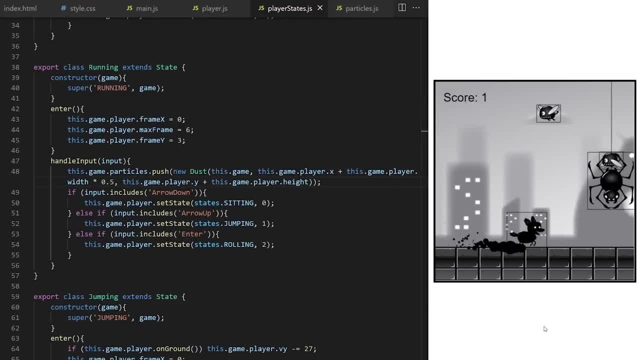 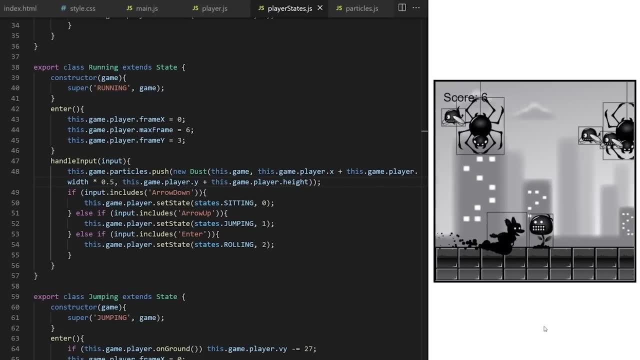 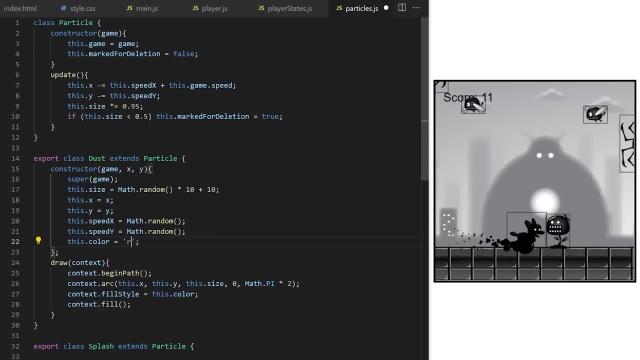 coordinates down closer to the game level ground. You can see how well this works in combination with state design pattern. We are only adding new particles when in running state, When player's feet are moving and touching the ground, I can go to my dust class and play with properties of the dust. 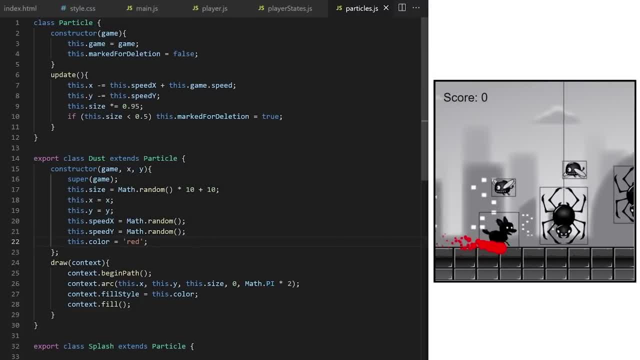 I can make the particles different shape or size here if I want to. I can also give them a different color- Red, Blue. It will all work. I can also do a semi-transparent color using rgba color declaration like this: I am happy with this, but feel free to play with the code and adjust these effects. 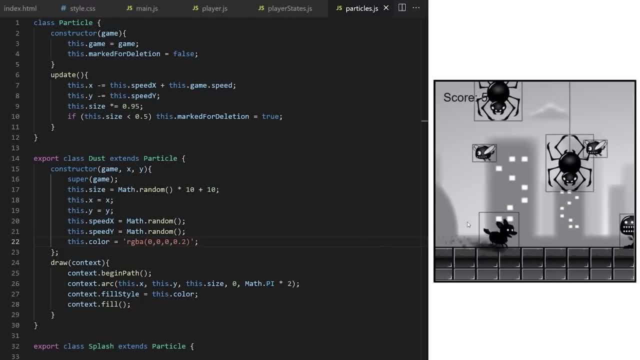 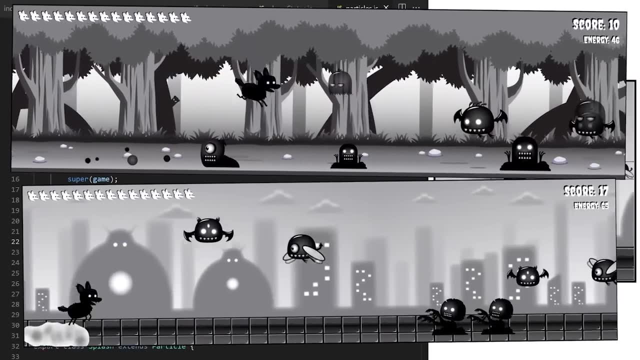 I came up with two different versions to animate fire for this game. I showed you both versions. This is the version with SVG filters, where we are blurring and sharpening particles to create this liquid smoke effect. I use this a lot in my generative art videos. 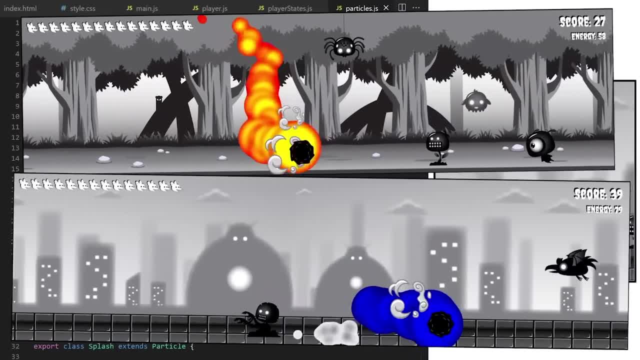 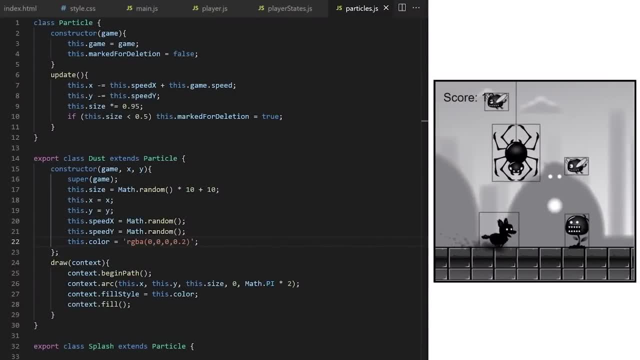 You could actually look at any of my creative coding videos where we build trails and use that code to give your player a unique trail effect. It will be compatible with everything. Today I will do something else. I will create a trail, Something I haven't showed you how to do before. 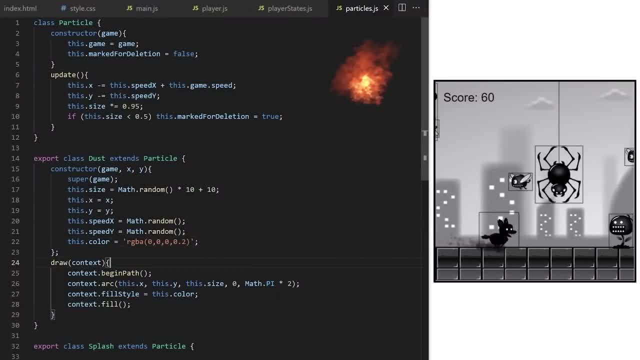 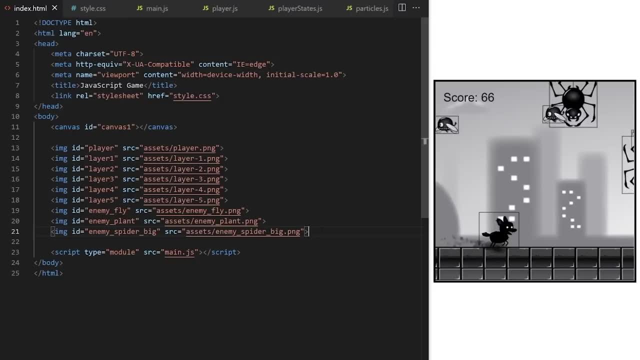 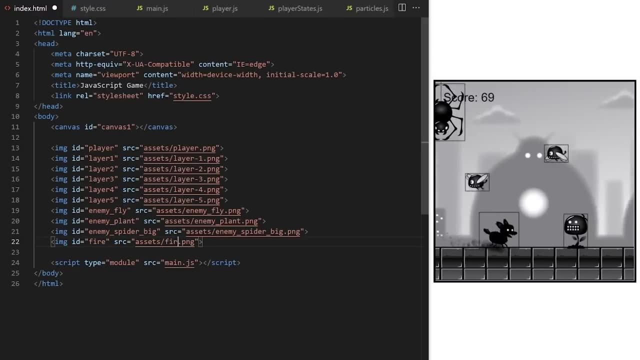 I will use a particle image. It will be this simple flame texture. Canvas is very good and efficient at drawing images. Drawing a rectangle or an image are often two most performance efficient options for an effect like this. You can download the fire texture in the video description. 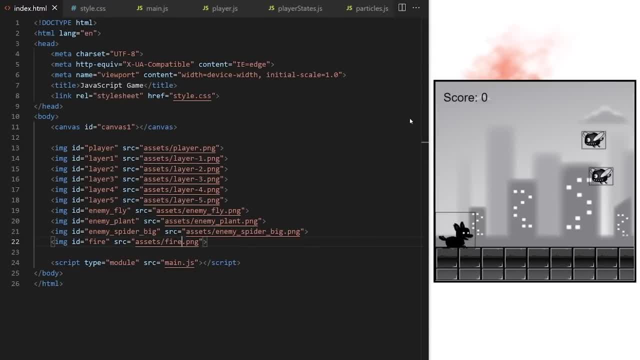 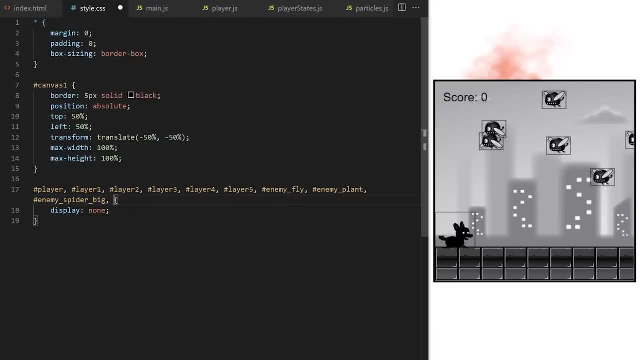 The texture is big. I will probably make the image smaller before I give it to you for download. You can also color shift the image in Photoshop to create blue or red fire trail, If it fits your level art assets. I set its display to none with CSS. 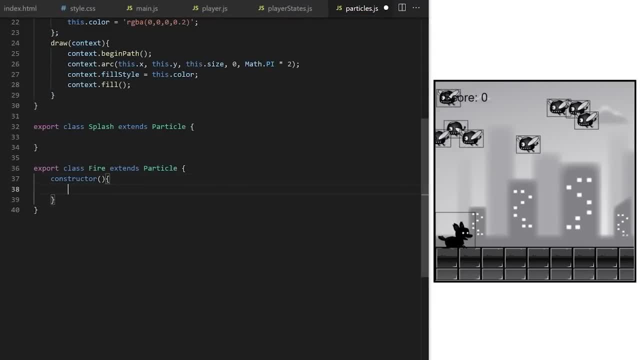 We will use this image here for our fire class Constructor will expect game x and y as arguments. This dot image will be this fire texture image. I gave it an id of fire. Size will be a random value between 50 and 150 pixels. 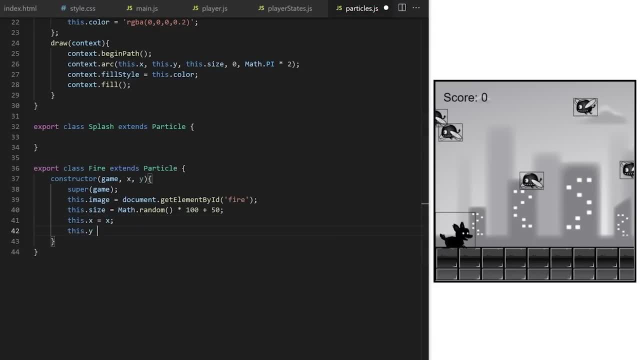 X will be passed as an argument, and same goes for y. Horizontal speed will be 1 pixel per frame and vertical speed will also be 1 pixel. We have update method on the parent particle class. I will first call the code from here. 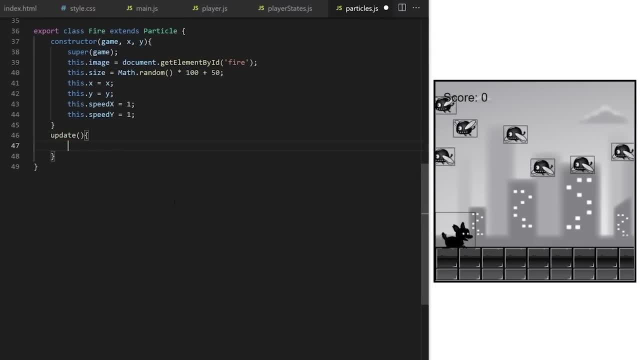 So update, super update, like this Draw method will take context as an argument and it will call draw image. I pass it this dot image from line 39.. This dot x, This dot y, This dot size as width And this dot size as height. 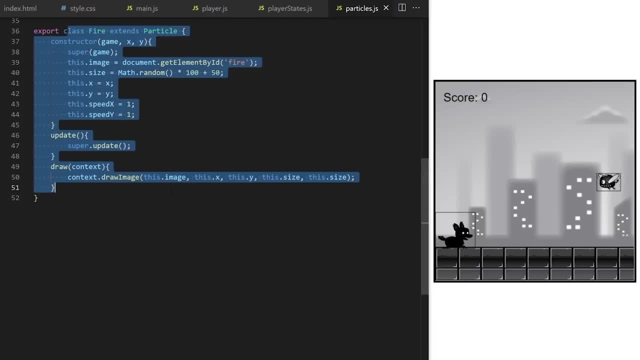 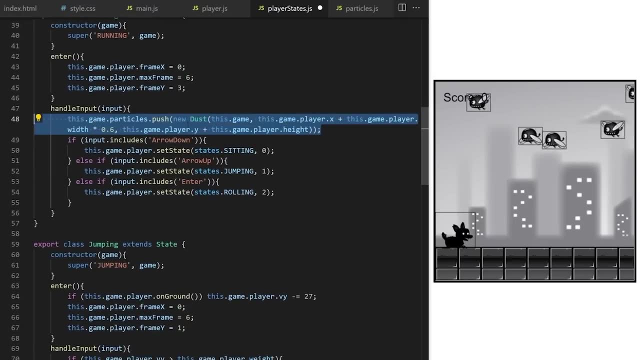 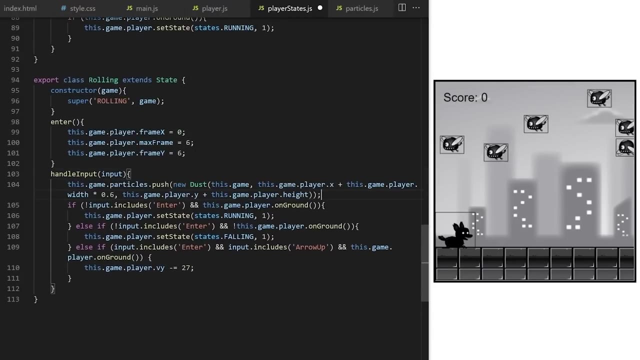 Nice. So this is our fire class. We are exporting it, so I can import it on line 1 in player states JS. I can copy this line of code from running class that is adding new dust particles. I paste it inside handle input method on rolling class and instead of dust I instantiate the 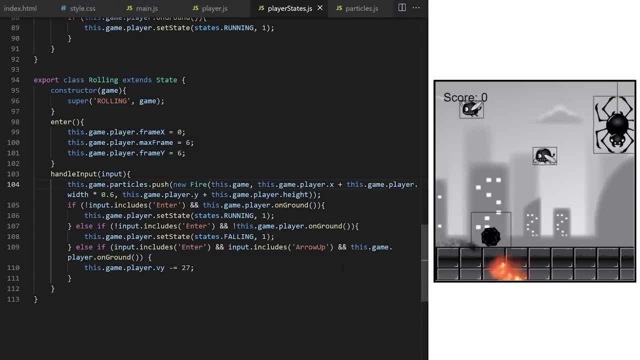 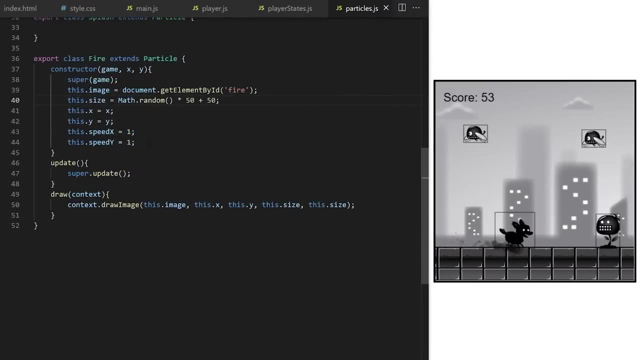 new fire class we just wrote. Now when I roll I am getting a trail of fire. I adjust these properties a bit. Before we fix the position of our fire trail, let's make the individual fire texture images rotate. I will need two helper variables called this dot angle, which will start at zero, and this: 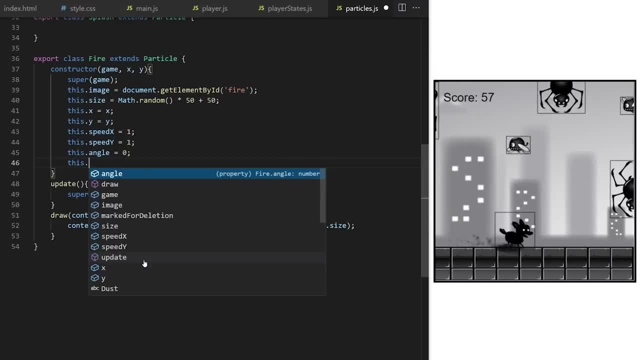 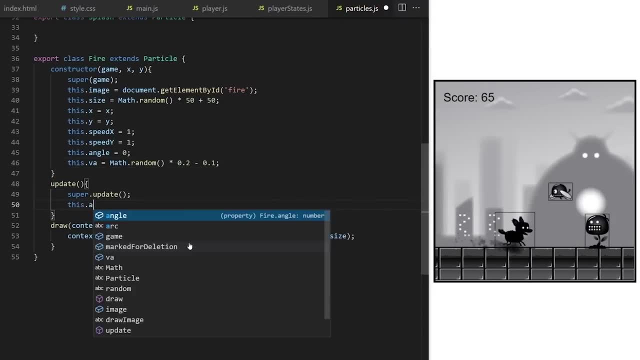 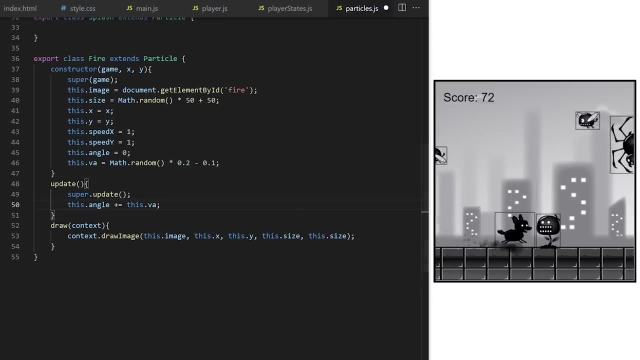 dot va. velocity of angle. It will be a random value between minus 0.1 and plus 0.1.. Inside update method I will increase angle by va for every animation frame We will be rotating. So to make sure The rotations don't overflow to other elements and only affect this fire particle, I will 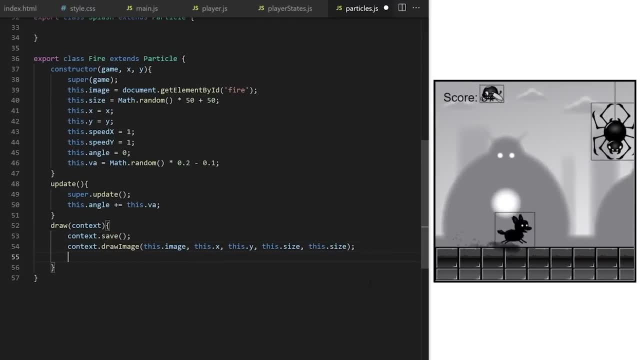 wrap this code between save and restore. This will make sure all canvas settings I declare in between will only affect this one particle. To rotate anything on canvas first we have to translate rotation center point from its default position at coordinate 0,0 in the top left corner of canvas over the center. 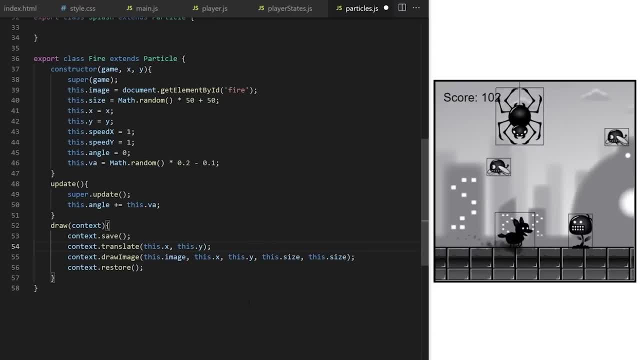 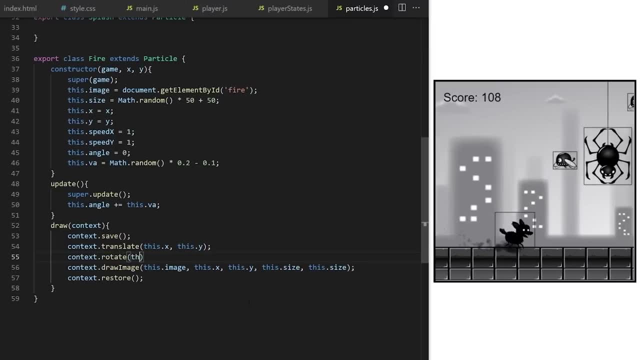 of the item we want to rotate. So I will translate to this dot x and this dot y of this fire particle. That particle Is a rectangular image, so I am translating to its top left corner. Then I call: built in rotate method that takes angle value in radiance and it will rotate. 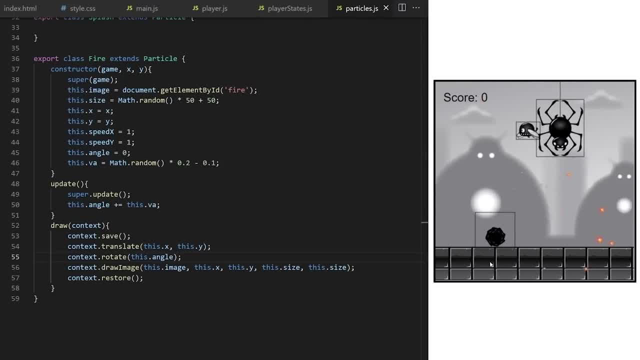 everything that's drawn after this call, unless we restore canvas again to its original default state. If I roll now we are getting a spiral of small fire particles in a big circle around the player. It's because we are translating to this dot x, this dot y, and from that point we are drawing. 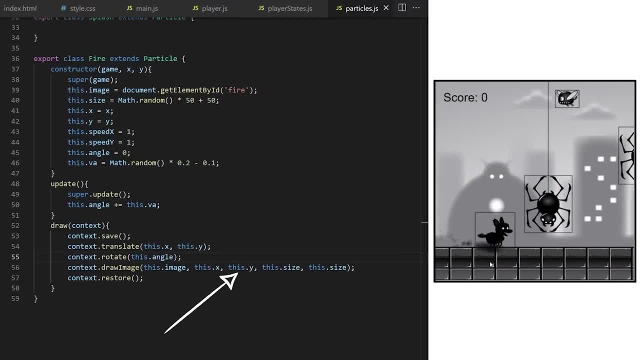 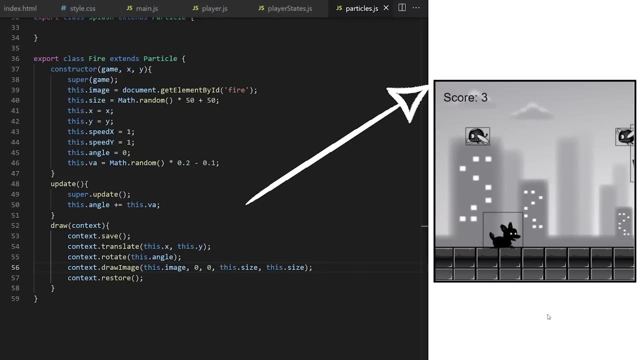 again to the distance of this dot x, this dot y. here I fix that I am translating this to 0,0 because position of particle on canvas is already defined in translate method. here Translate method moves rotation, center point and what is considered coordinate 0,0 on canvas. 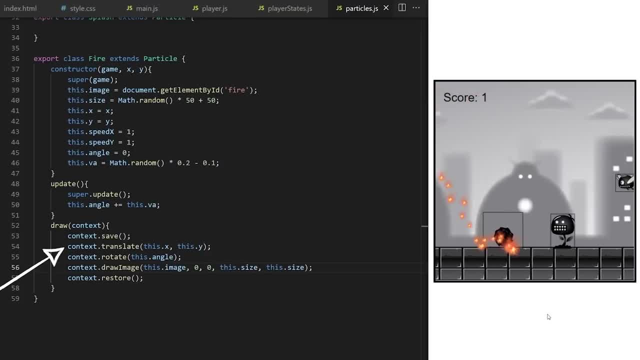 to the coordinates we pass to it. So, because of this translate call for these particles, coordinates 0,0 on canvas are here in this area. I am translating to the top left corner of each fire image of each particle rectangle. I want to center it, so I adjust this value by half of its width. 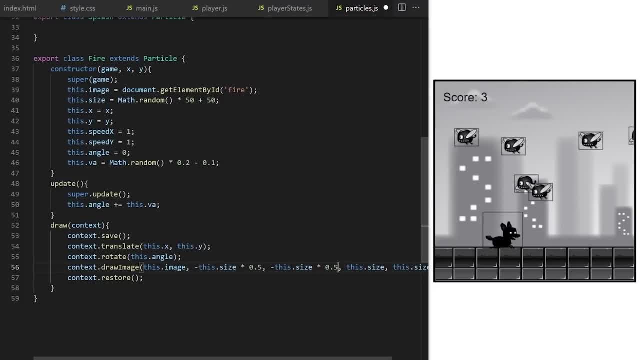 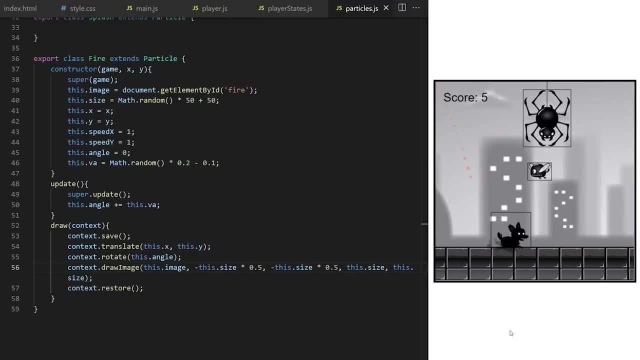 Then I move it to the center, And this one by the half of its height. Canvas rotation can be difficult for beginners, but we just covered all of it. I have more detailed lessons on this topic, but for now let's just move on. I can increase the size of fire particles here, on line 40.. 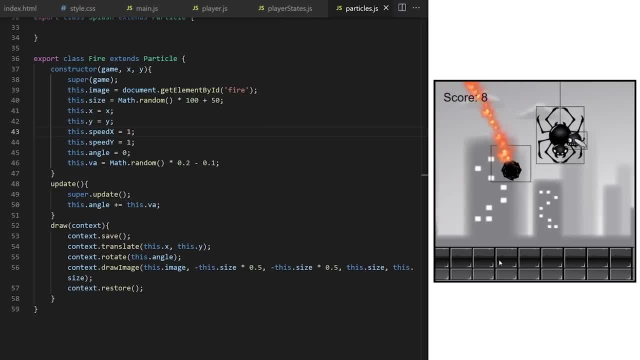 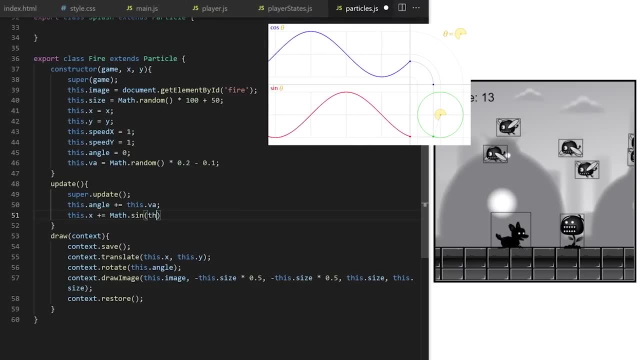 I can also give them some horizontal wobble, using the same technique we used for flying enemies. For each frame I increase x by assigned value of ever increasing angle and it will map horizontal x positions along an endless circle. I can also give them some horizontal wobble, using the same technique we used for flying. 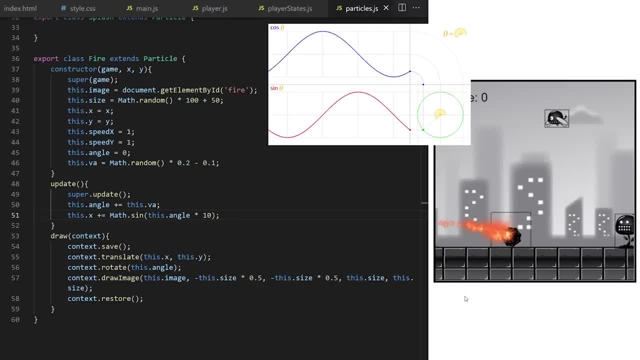 enemies. I can also give them some horizontal wobble, using the same technique we used for flying enemies. I can also give them some horizontal wobble, using the same technique we used for flying enemies. I can also give them some horizontal wobble, using the same technique we used for flying. 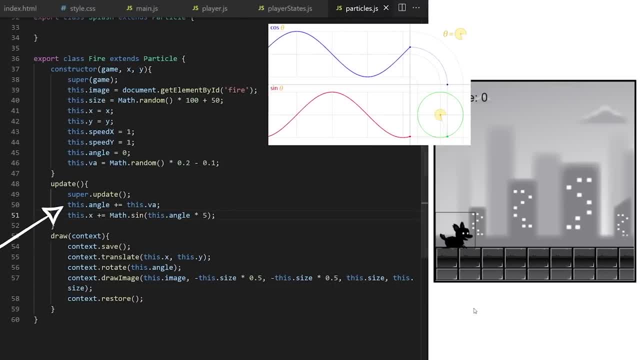 enemies. So just to give you a bit more information: how to gap this particle. If you are a beginner, all you have to understand about this is that if you pass mathsign and ever increase in angle value, our angle is increasing here on line 50, it will map. 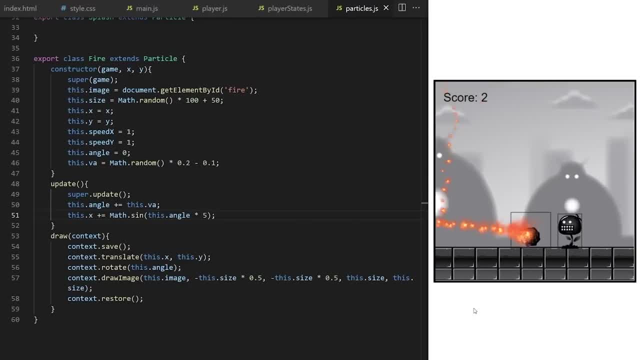 positions along a wavy path. Now you can see that there is some left to right wavy movement. If you look at the particles now there is left to right wavy movement. I can also make the particles shrink slower by adjusting this value. 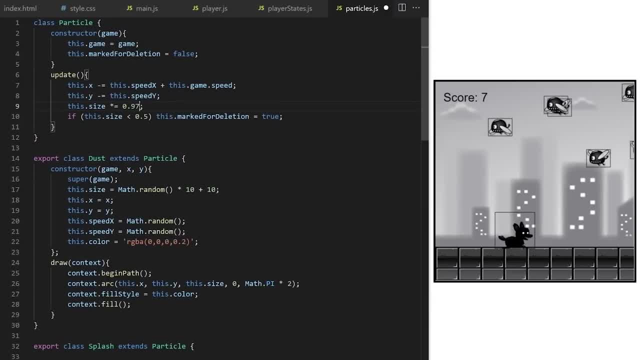 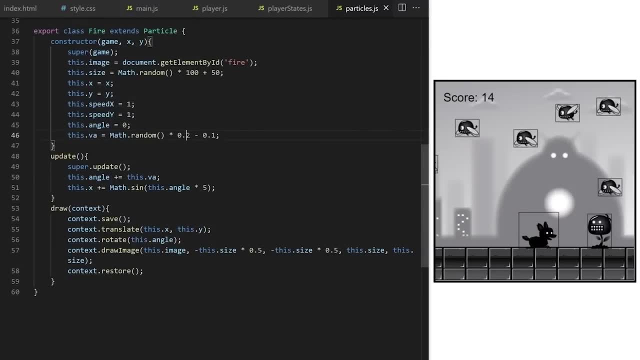 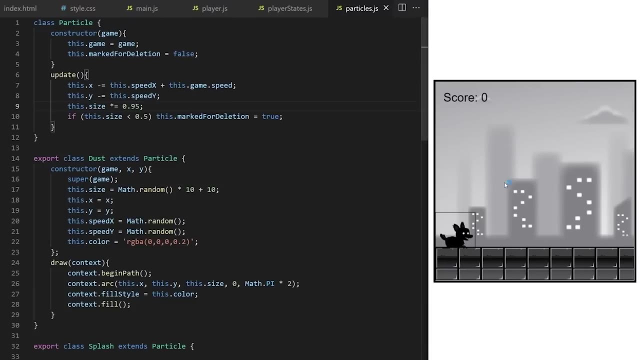 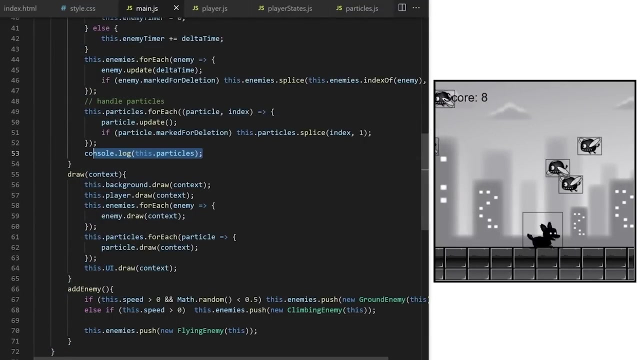 This will result in a longer fire trail as particles take longer to be small enough to be removed. by adjusting this range of values i can increase particle size. i can make them shrink faster in mainjs. i remove this consolelog on line 53.. i want to make sure we don't get too many. 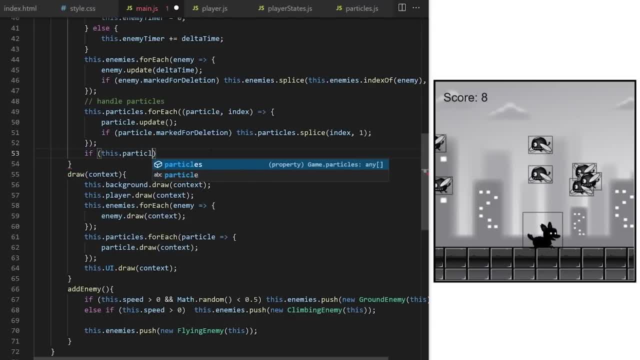 particles. i want to have a property that will limit the maximum amount of particles we allow in our game so we can easily adjust that value if we need to. so inside update method on the main game class in this section where we handle particles, i say if the length of particles array 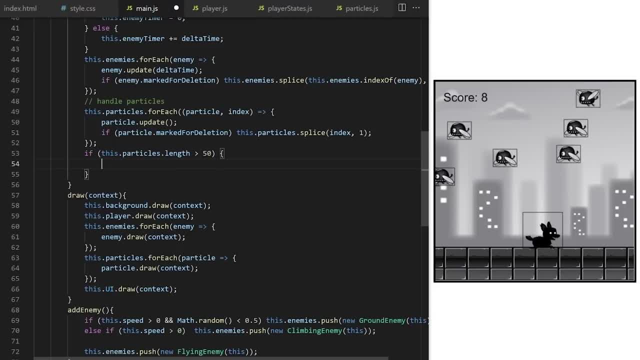 is more than 50. i want to slice the array and remove everything from 50 upwards. i do that by taking thisparticles and assigning it to the same array, but sliced from index 0 to index 50. it will only allow the first 50 particles to be in this array. anything over and it will get sliced away. 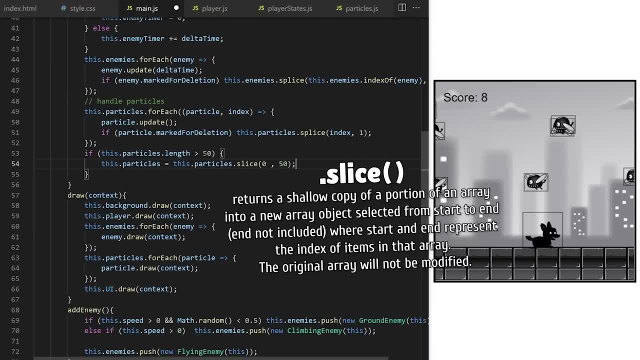 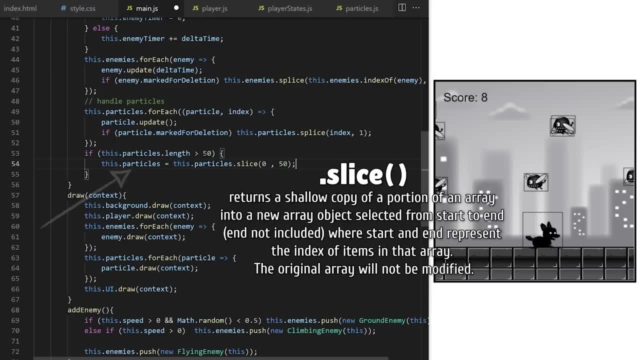 slice method returns a copy of an array with only a portion of elements from start index to end index and then a copy of an array with only a portion of elements from start index to end index we defined. the original array will not be modified, so that's why i'm overriding it like this, because 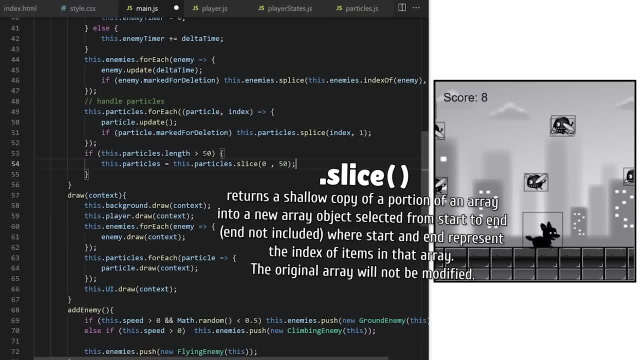 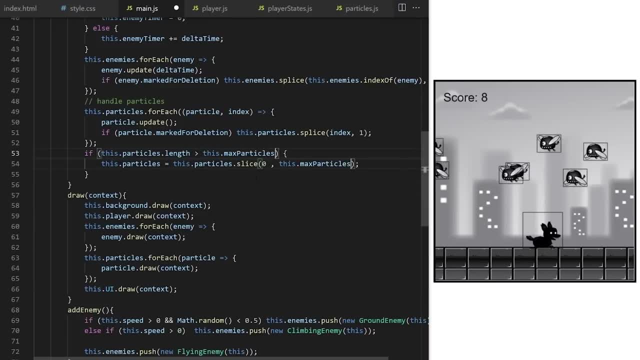 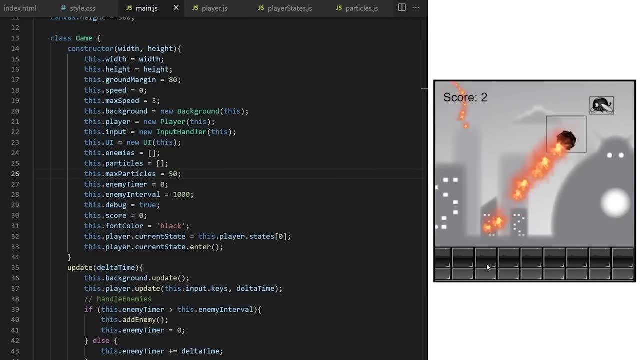 in this case i want to modify the original array. so we have some hard-coded values repeated here and here. let's replace them with a variable. i call it, for example, this: dot max particles. i declare it up here and i set it to 50.. i can see it works because it slices particles from. 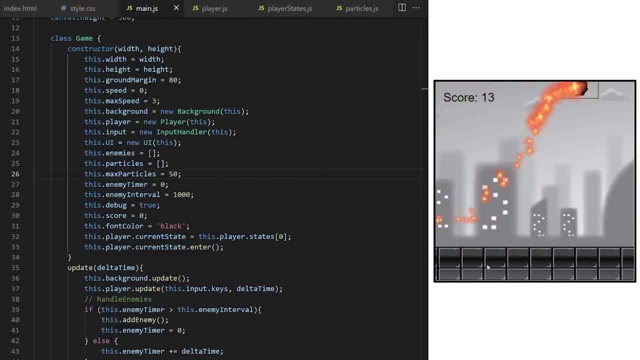 the array. you see how they disappear and we are getting gaps in our particle trail. i actually want to slice particles from the other side of the array. i want to remove the old ones, not the new ones. i can change the arguments. i pass the slice method or i can change how we push our 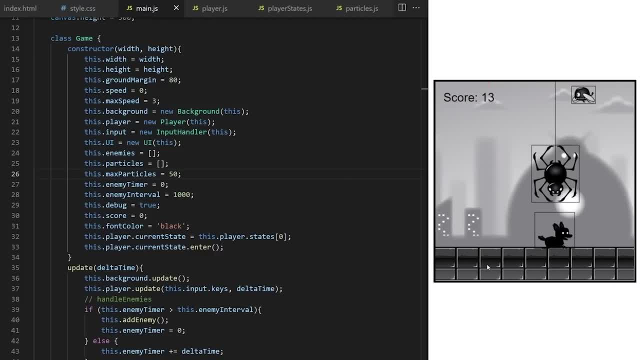 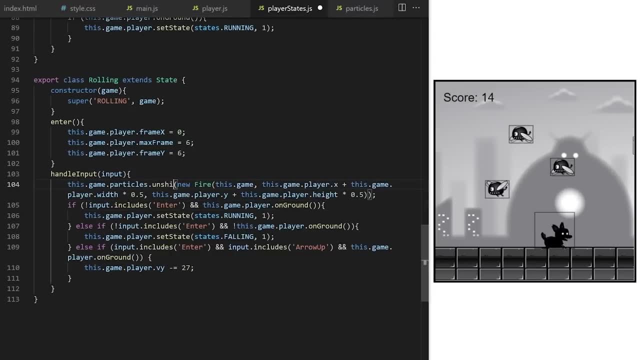 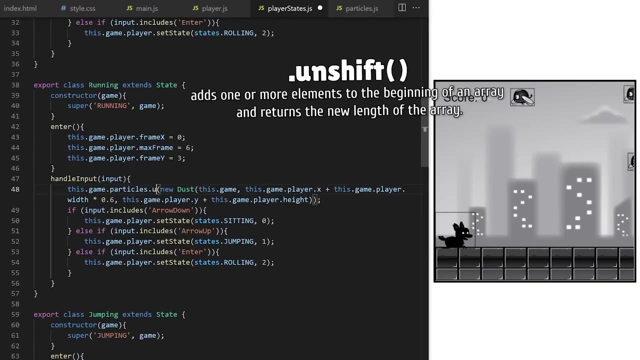 dust and fire particles into particles array in player states js on line 104. instead of using push method, which adds one more element to the end of the array, i will use unshift built-in array method instead. unshift method adds one element to the beginning of an array. so now when i'm slicing from: 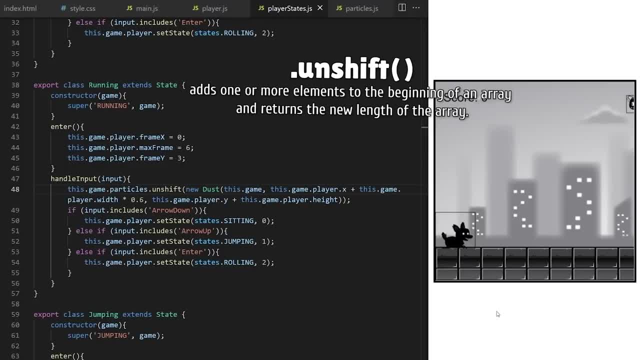 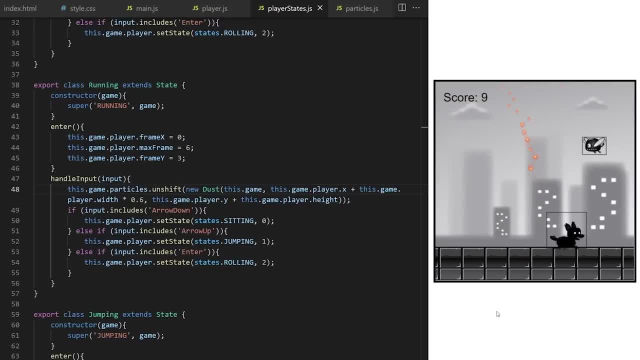 index 0 to index 50. i'm going to slice particles from the other side of the array. i want to remove those new particles and i'm removing old ones if their index exceeds the value stored in max particles variable. i do the same thing on line 48. i will be unshifting dust particles, adding them to. 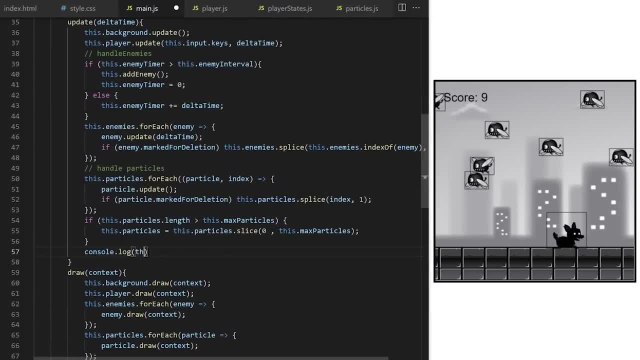 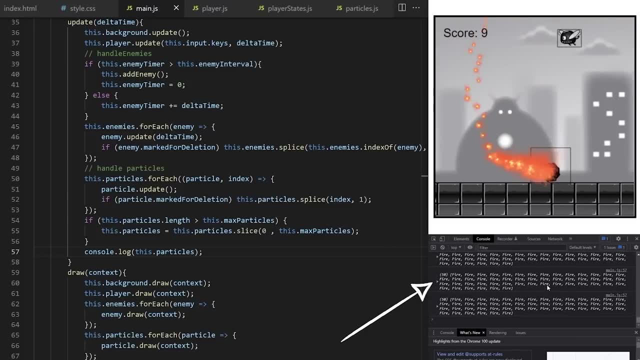 the beginning of our particles array to check if everything works. i will consolelog thisparticles from here. it starts empty. if we start rolling it fills with fire particles. if we run it fills with dust particles. it never exceeds 50 particle objects, so our slice method is correctly limiting. 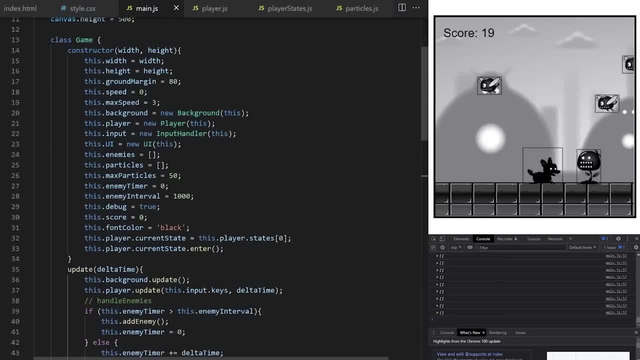 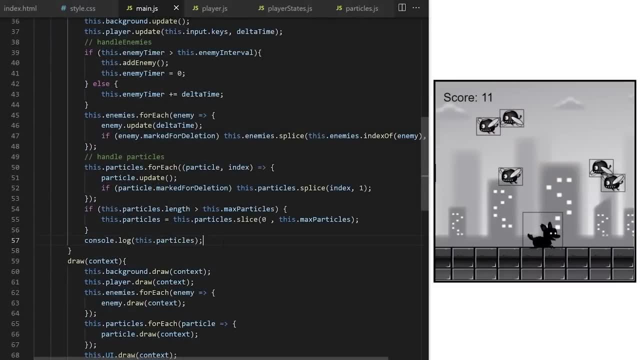 the length of the array. nice, i'm on a strong computer so i will set my maximum particle limit to 200, but you can keep it on a lower number if you want to. it's up to you. i will also delete this console log on line 57 to clean up. 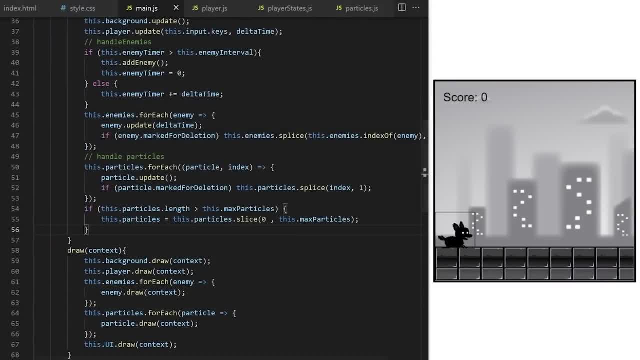 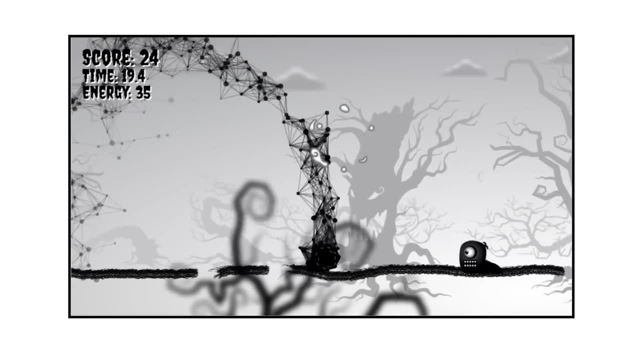 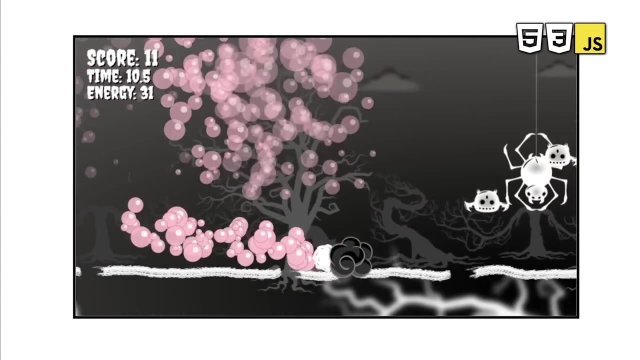 congratulations on completing this lesson. in the next part, we will make our game look and feel better by adding more animation. it will help the player to get more visual feedback to the events happening in the game. i'll see you there, hey. creative coders, in this episode we will finalize player abilities and particle effects. 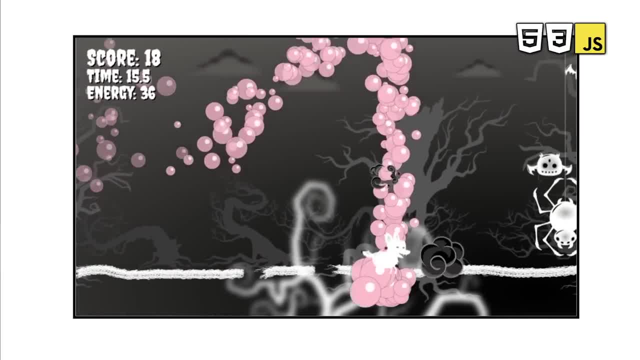 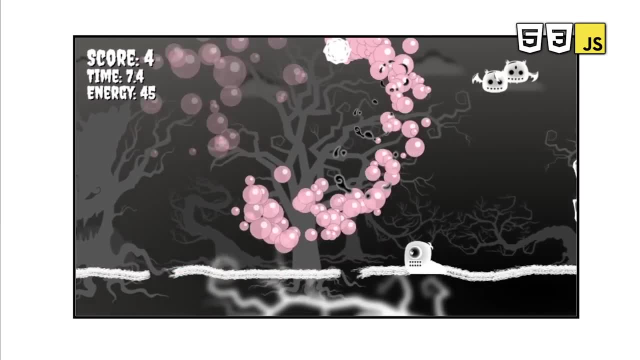 with a special sprite sheet and we will add win and lose condition based on game timer. we will also clean up some loose ends in our code. let's finish the base game and then we can talk about some optional bonus features. have fun. i want to create a second attack. this time it will 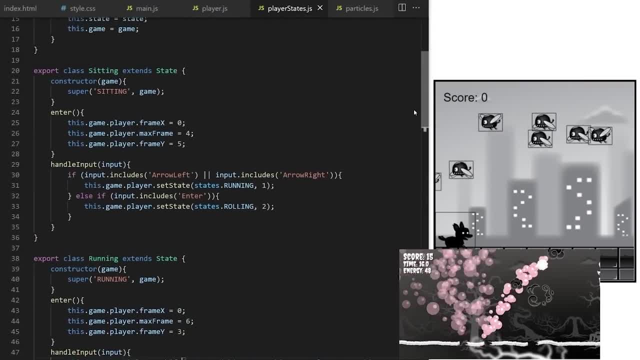 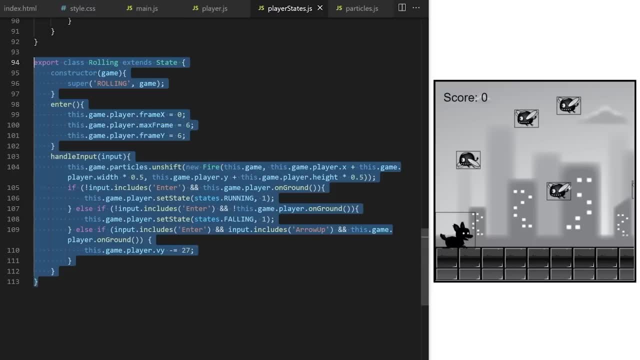 be a crushing meteor attack from above. player can only enter this state when it's in the air. it's a perfect use case for state design pattern we have here in our code base. when the player is running on the ground and we press down arrow key, it sits down when the player 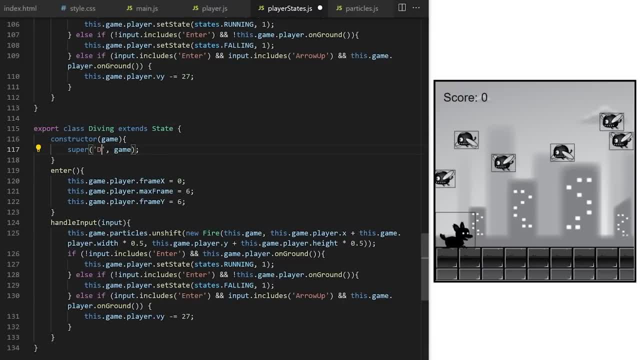 is in the air, we press down arrow key, it will do a crushing dive attack from above. i copied the entire code block with the roll in state class and i call it dive in. i also pass a string that says dive in in all caps to super class constructor. 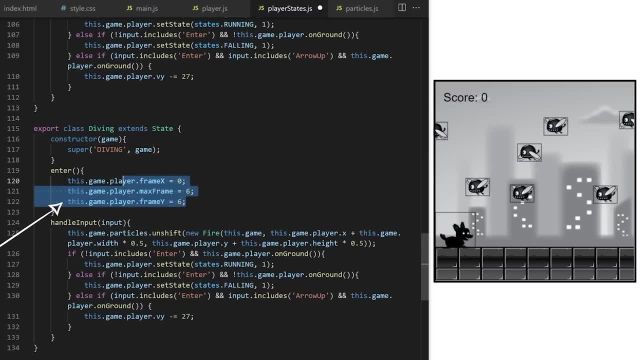 all the values inside enter method will stay the same, because dive in uses the same sprite animation row as rolling. we will also leave the same fire particles code because dive in also leaves a fire trail while the player is in diving state. it is just moving fast towards the. 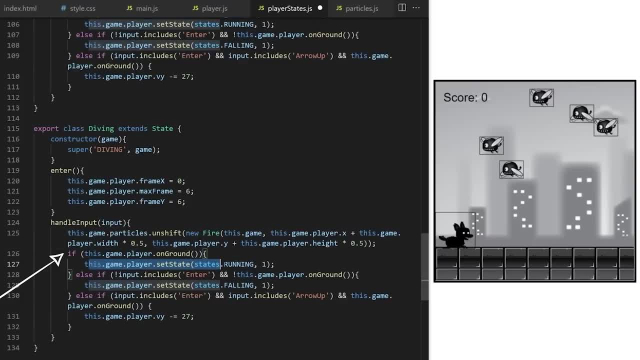 ground. When it hits the ground and this statement is true, we switch player to the running state to keep the momentum going. I can delete this entire else if statement. and here I say else: if input includes enter and player is on ground transition directly into rolling state, It should make the transition animation. 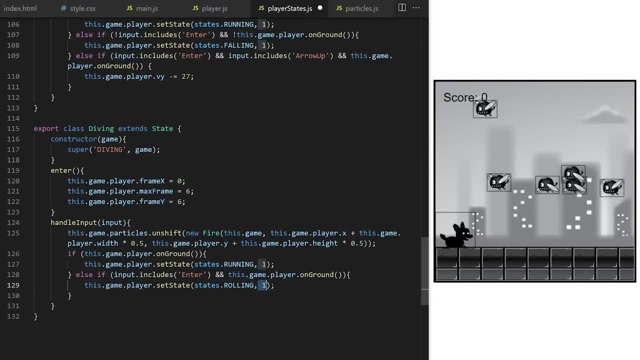 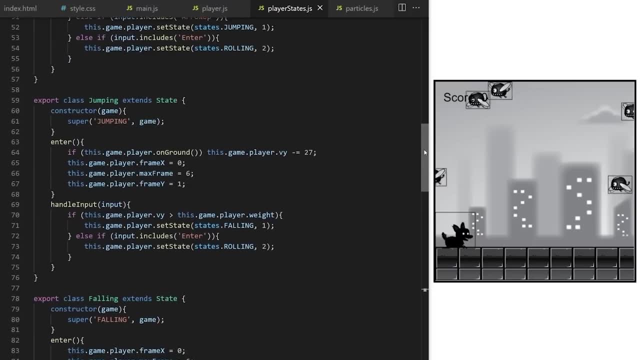 connect better. We have our dive in state, but there is currently no way to enter that state. Let's define rules for when it can happen. We can enter dive in state while we are in a jump in state, When we are jump in and we press arrow. 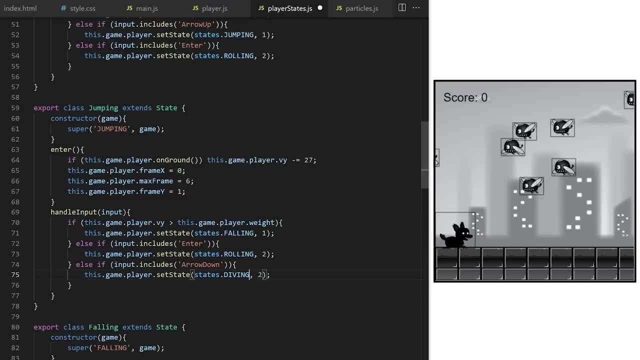 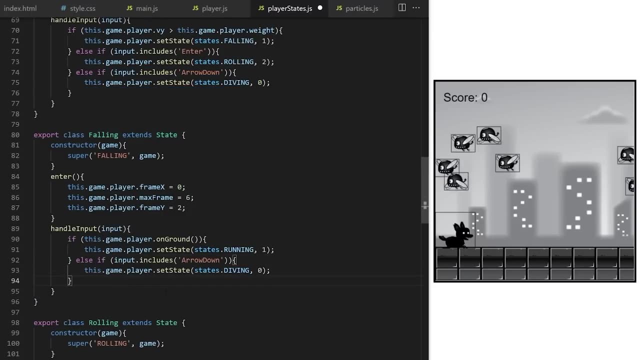 down. we set state to dive in and game speed will be zero because we are moving directly down. Let's take full advantage of the fact that the scrolling speed of our game world is connected to player states. We can also enter dive in state while falling, so I just copied the same else if statement here, And we can also. 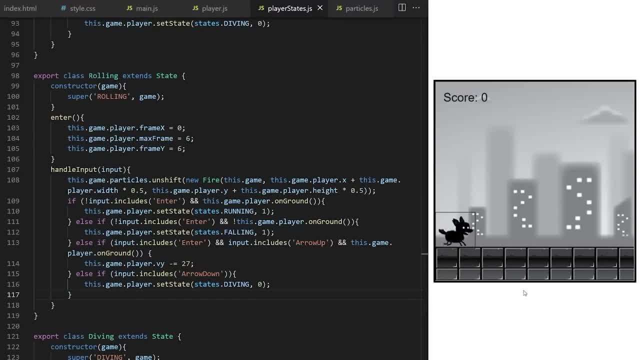 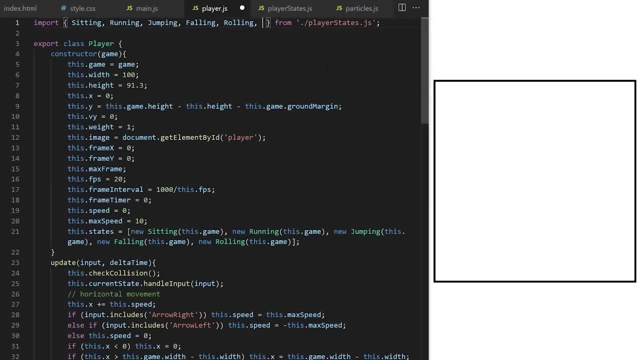 dive while rolling. Let's test it and see. I save my changes and the code breaks because we need to save the changes To import and instantiate the new dive in class. I import it on line 1 and I create an instance in thisstates array on line 21.. It works. I want to feel like. 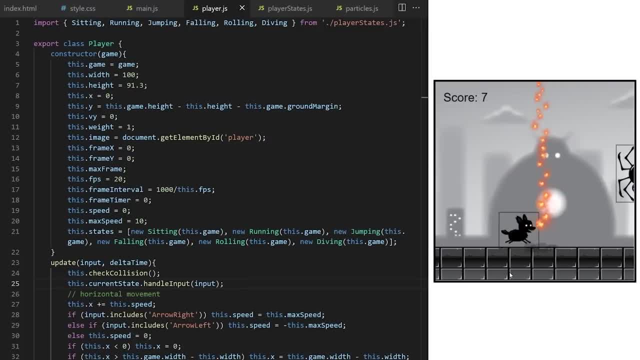 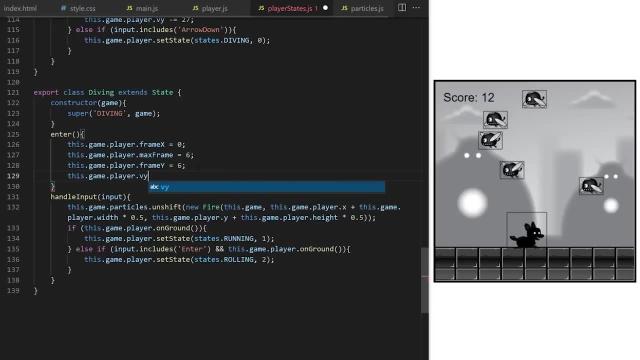 we are slamming into the ground with a great power, but right now the player hovers in the air for too long. In enter method on diving state class, I set velocity y to plus 15, instantly giving the player a massive push towards the ground. Nice, now it feels like there is some. 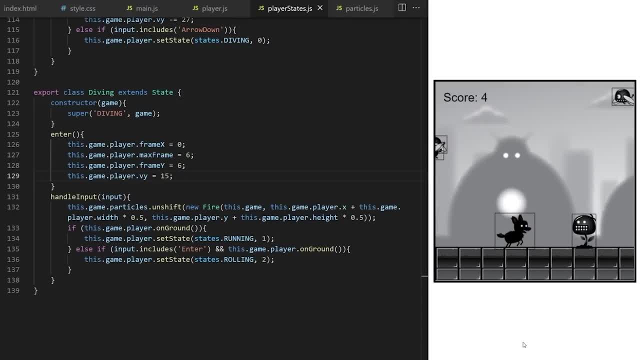 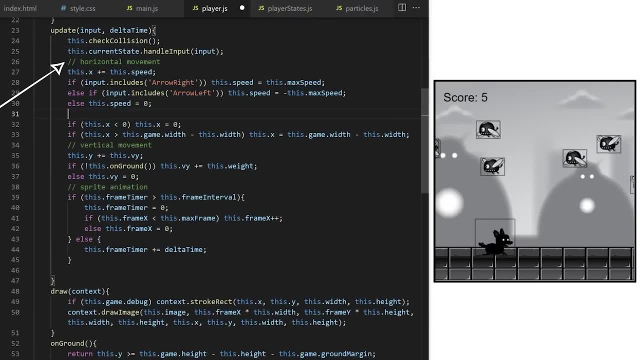 power behind that special move. As I'm diving and hitting the ground, player kinda gets stuck below the ground level. Let's fix that. So here, inside update method on player class, we handle horizontal movement and horizontal boundaries. Here we handle vertical movement and vertical boundaries will be defined here. Let's keep ourselves. 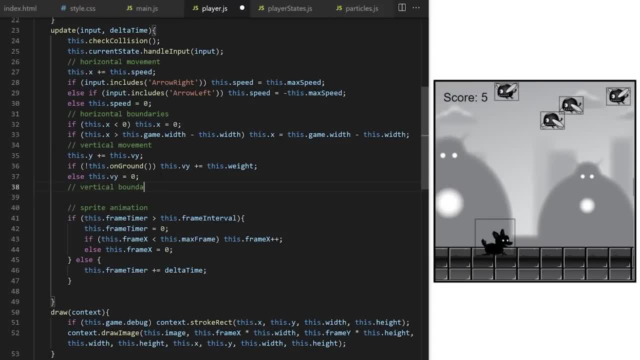 organized. I want to make sure that the player cannot get stuck below ground level like this, so I will limit its vertical position If thisy is more than the height of the game area minus three. the height of the player minus ground margin set player's vertical Y position to game height. 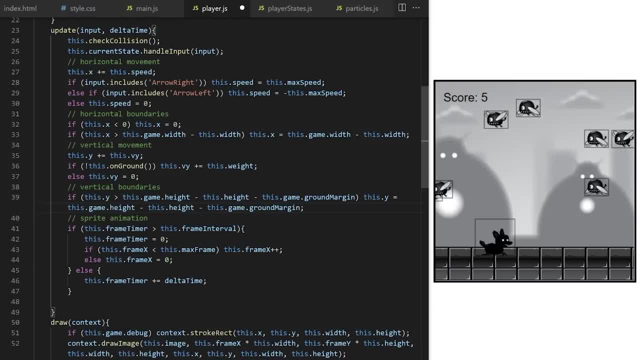 minus player height, minus ground margin, Like this. Now the player can never move to the space below this point, Below the level of ground texture. in our game world We have one more particle class I called splash. When the player does a meteor dive, attack from. 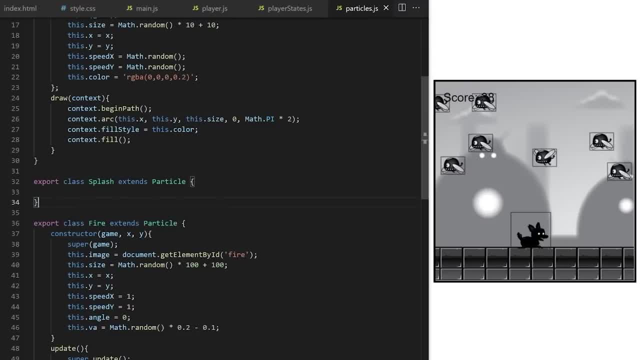 above and it hits the ground. I want it to do a flame explosion and I want the flames to splash in all directions to make that move look and feel very powerful. Constructor will need three arguments, as usual, Game and X and Y positions. I trigger. constructor on the parent superclass. 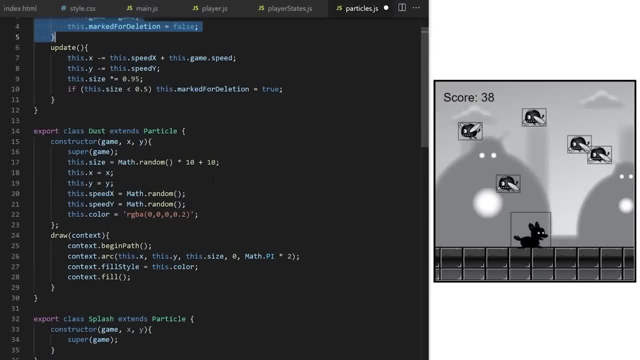 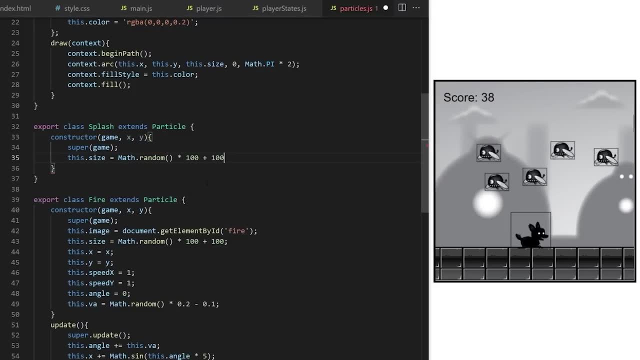 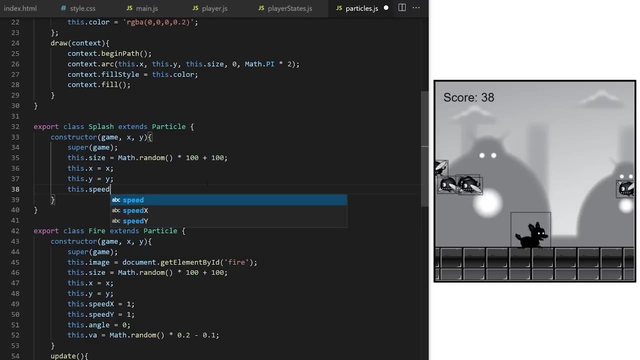 and I pass the game along, So this code will run. Size of the splash particle will be a random number, between 10 and 200 pixels. This dot X is X. this dot Y is Y. Speed X will be a random number. 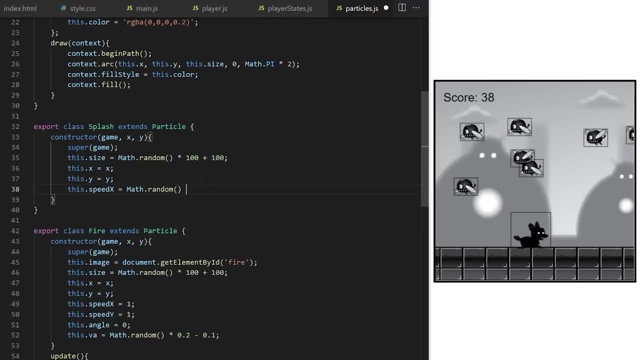 between minus and minus, Speed X will be a random number. between minus and minus, Speed X will be a 3 and plus 3, because I want them to splash in both directions. horizontally, Speed y will be between 2 and 4, for example. 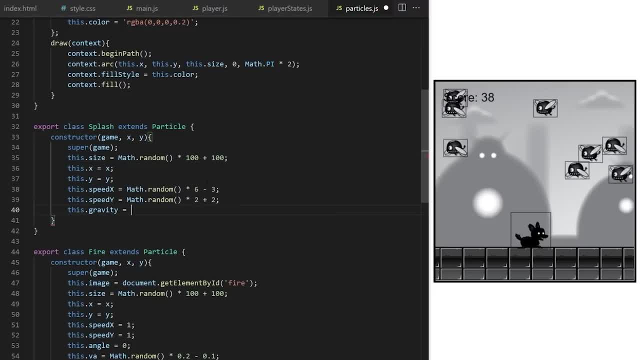 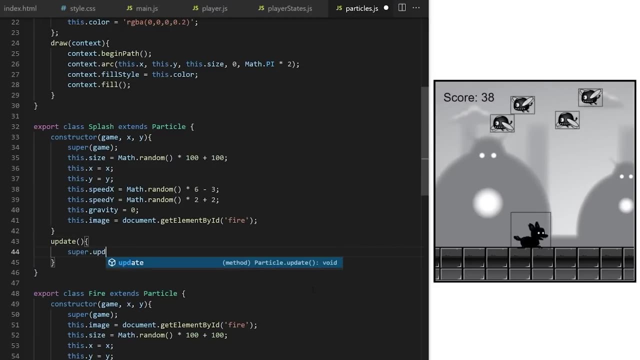 I want the particles to start moving up, but as the gravity slowly grows stronger, I want them to curve and start moving down. similar principle we used for player jumping logic Image will be the same one we are using for fire. particle class Speed method will at first call update on the parent particle class, as usual. 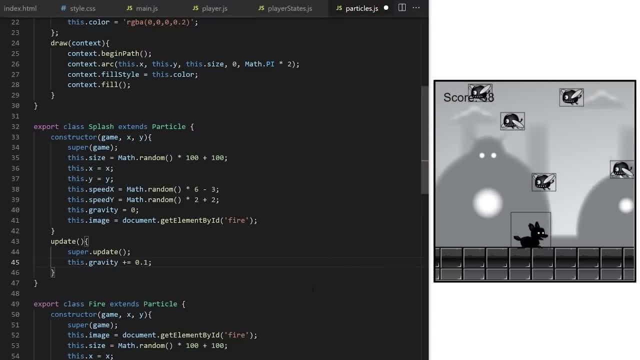 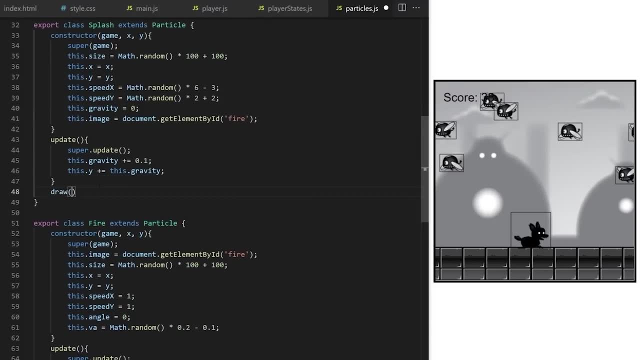 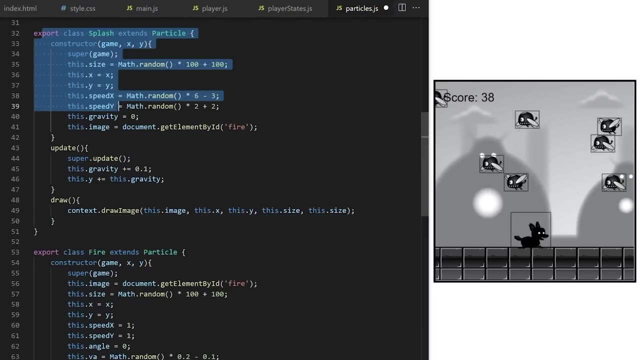 Gravity from line 40 will be slowly increasing by 0.1, and this dot y will be increasing by the ever increasing gravity value. to get that curved path Draw method will just draw the fire image from line 41.. We are exporting splash class, so I import it on line 1 in player statesjs. 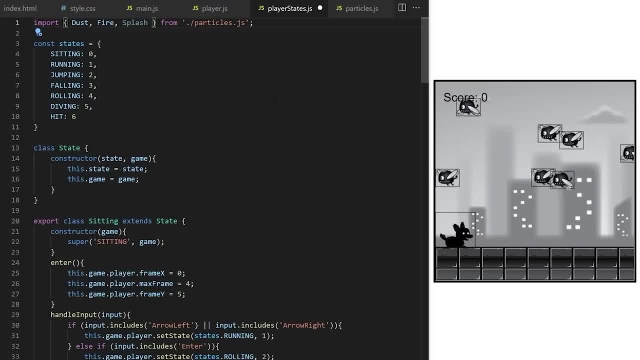 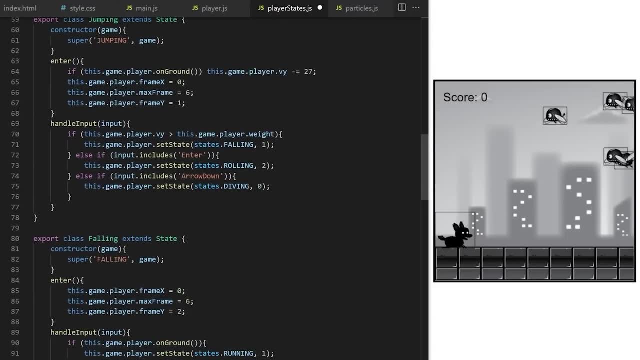 I can't really create this particle explosion when we enter diving, Because at that point the player is still in the air. I want to create it as we hit the ground, so I could add exit state to all my states, which would be an ideal location for this to happen, given our code structure. 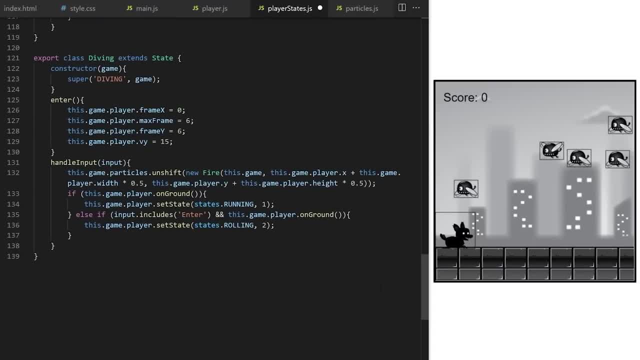 I can also create some small transitional state just for this, Or I can just do the simplest option and create the explosion in this. else, if statement on line 133. When player is in diving state and handle input method- detects we touch the ground, we set player state to run in. 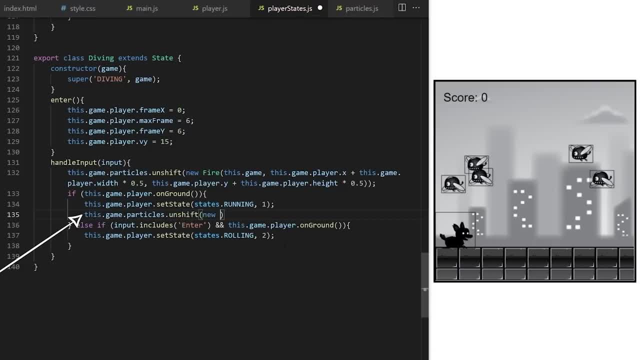 And we create our state, Our splash particle. I use unshift again to add one particle to the beginning of the array and I pass it. game x and y: position of the player. One particle wouldn't be very impressive, so I create a for loop here and I will run. 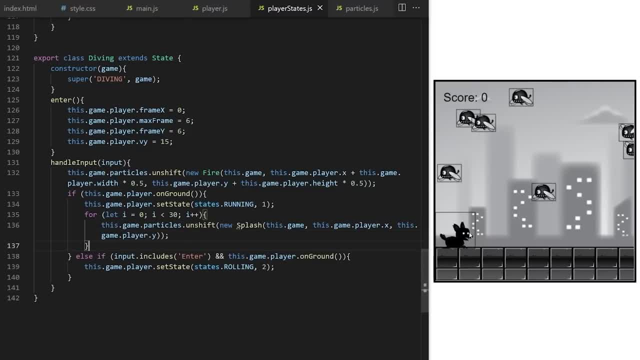 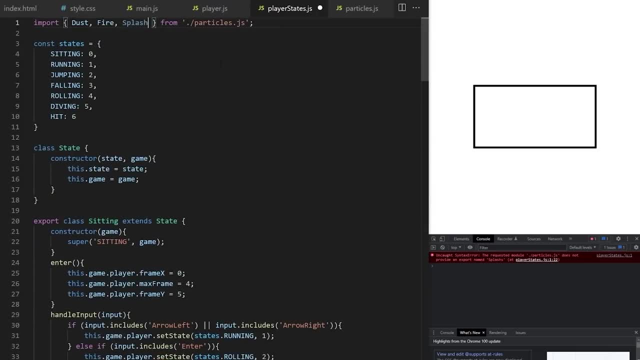 it 30 times, We will create a splash of 30 particles. I'm getting some errors. It's here on line 1 in player statesjs. I misspelled my class name. When I dive I get another error. It just says that I forgot to pass context to draw method on source. 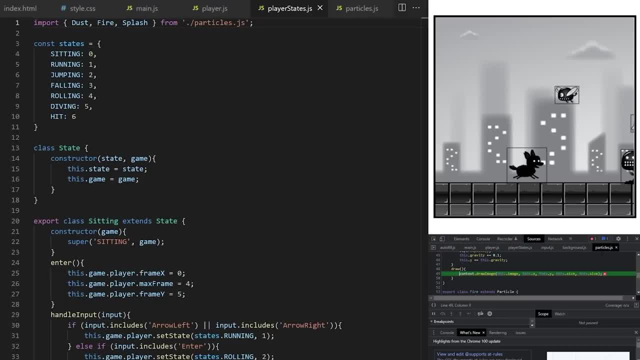 I'm not sure if it's a good thing or not, but it's a good method. on splash, class Console errors are usually good at pointing us to the file and line of code where the problem is. These two errors were easy to find and fixed thanks to my browser console. 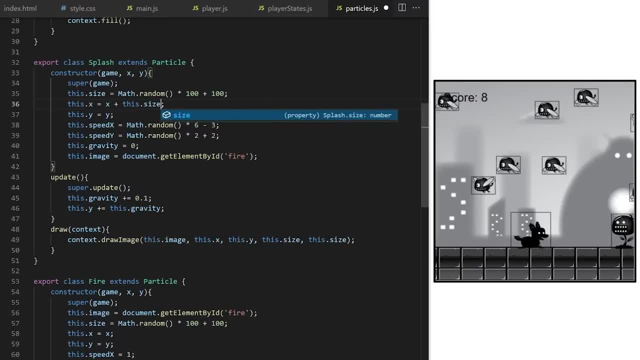 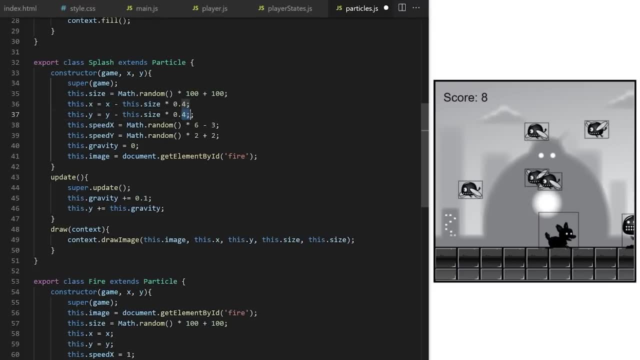 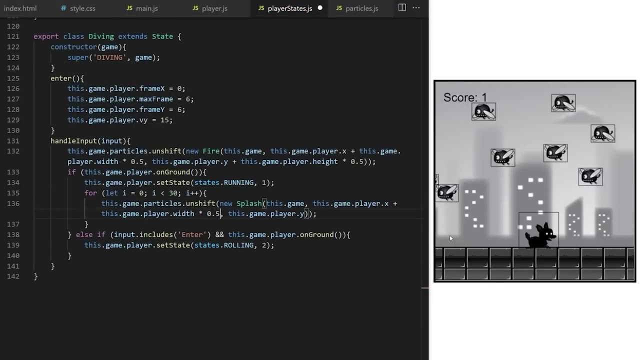 Now when we hit the ground we get a splash of particles, I offset initial x coordinate, maybe like this: I also offset the y coordinate. I adjust the initial position values. I pass to splash particle class constructor. I'm kinda just playing with the values and offsetting them. 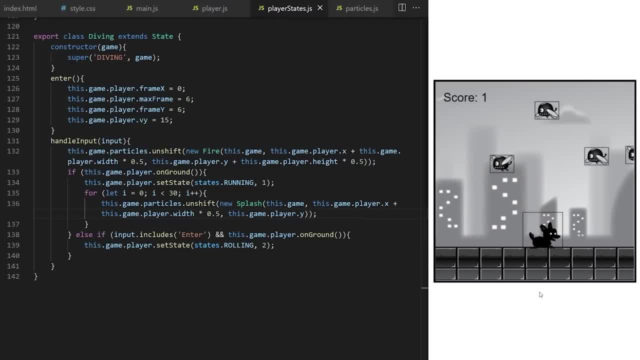 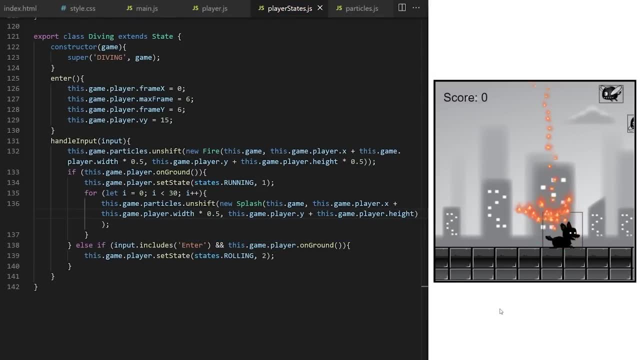 Because I want the particles to shrink in size, which makes them move towards their top left corner, I adjust this value. There is a better way to deal with this, but I think for the purposes of this class, we can just do this quick hack. 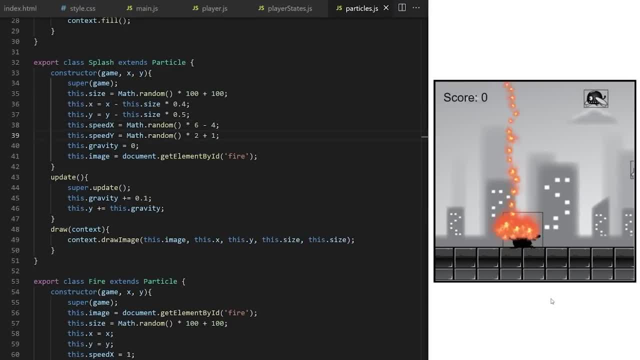 It will look good enough And I adjust speed x like this. This looks alright for now. I think We get a nice impact animation when we hit the ground- Perfect. I also want to have a player state that will play dizzy animation when we get hit by an. 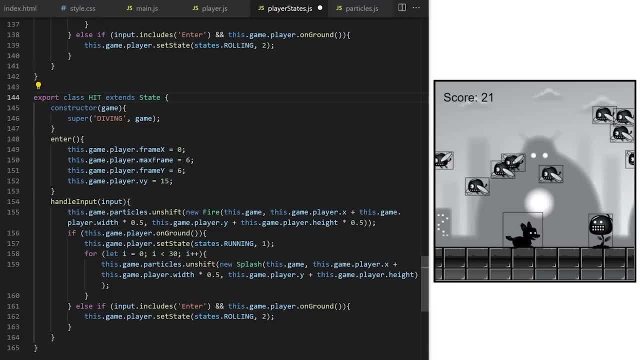 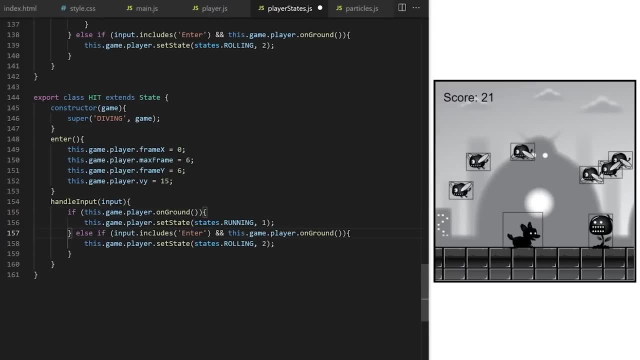 enemy while we are not in a fireball state. I call it hit. I delete this line that adds fire particles. I also delete this. I check my spreadsheet and I can see that max frame for this animation is 10.. Frame y is 4 and I delete this. 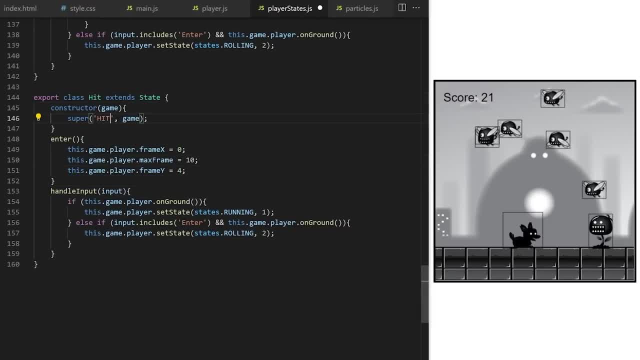 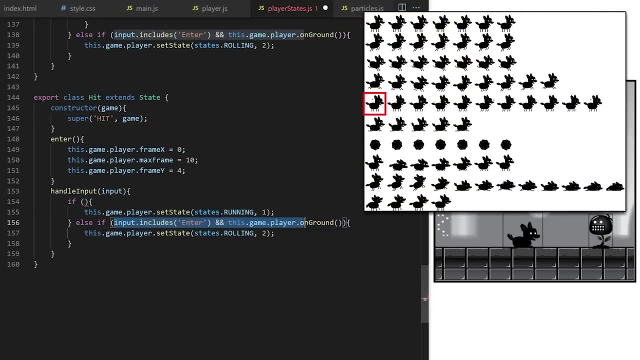 I will spell class name like this and I pass it: hit here With this state class. I will do something I haven't showed you before. Then enter a state, have it play its animation row once, and when that animation has been played, we automatically transfer to another state. 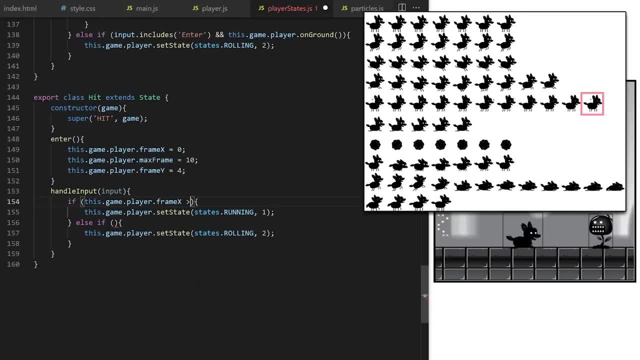 So the trigger for switching state will be animation frame this time. So while we are in this hit state, this animation row is playing. I will wait until frame x is at position 10 and I check if player is on ground and I switch player back to running. 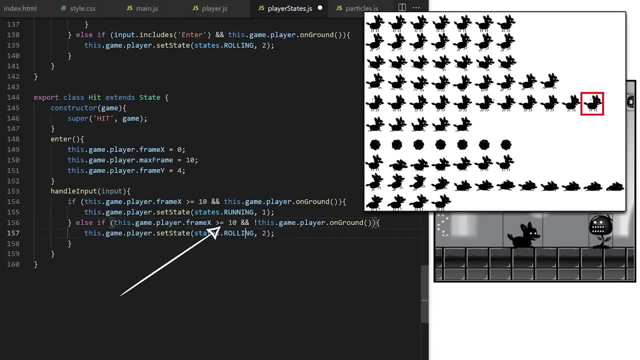 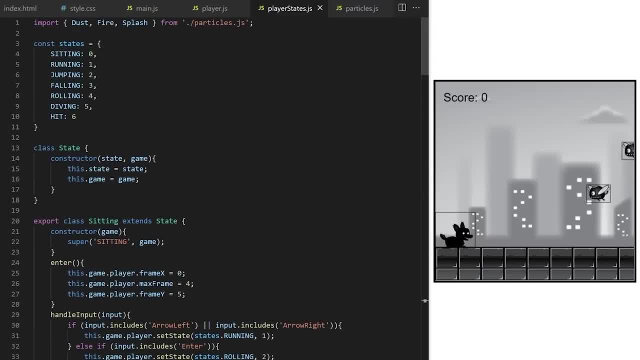 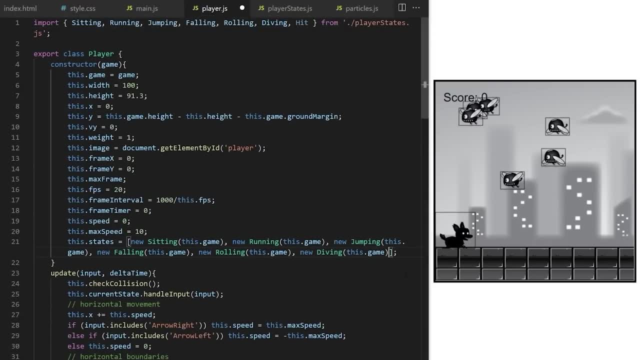 Else, if we are on the last frame on this animation row And if player is not on the ground, we set state to fallen. Nice Up here I can see that hit state has an index of 6.. I import it into playerjs module and I instantiate it as the item with an index of 6 inside thisstates. 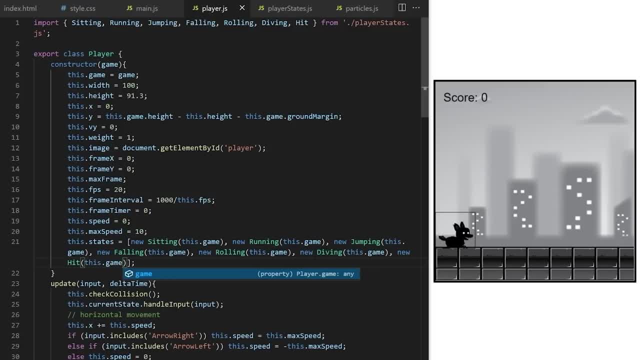 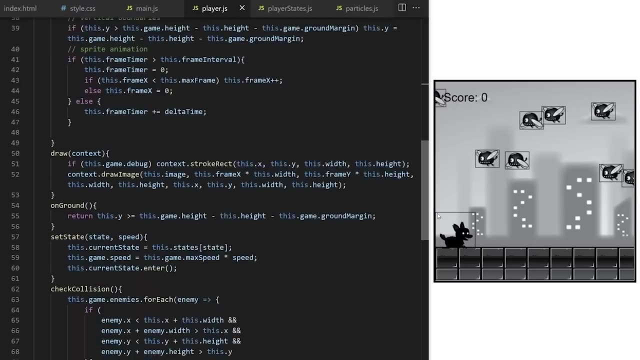 array. Ideally, I want to do all my state swapping from within playerstatesjs. I could do it through a set of flags and flipping values around, but since this class is beginner friendly, I will do a simple thing and switch my state. I want to enter this new state when player collides with an enemy, and it's currently. 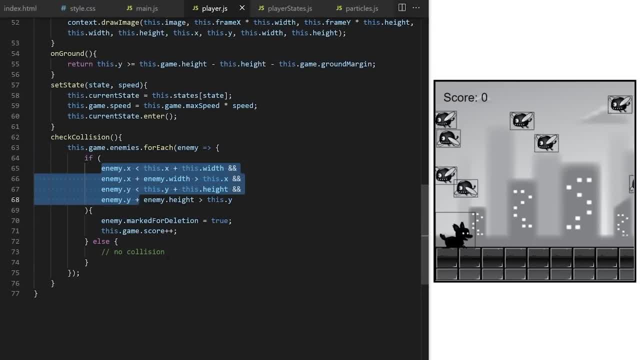 not in rolling or diving state. So if collision is detected, we will always mark enemy for deletion, regardless of what type of collision it is. I delete this else block. we won't be needing it. We are going to run if else. statement: if collision is detected. 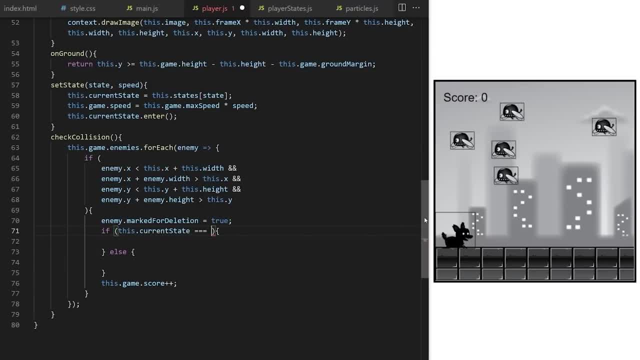 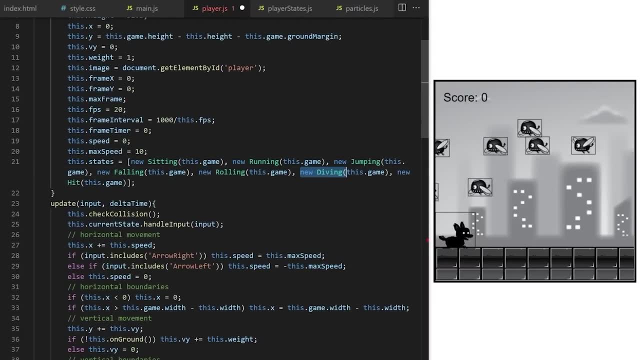 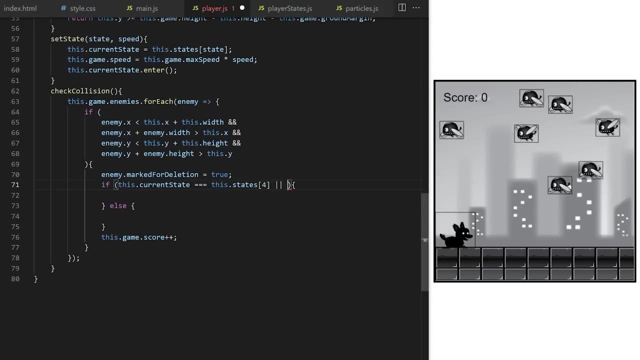 If we detect collision and player is currently in rolling or diving state, so index 01234, and 5, player is invulnerable in these states, so it will destroy enemy and give us plus one score. ThiscurrentState is thisstates for rolling or if thiscurrentState is thisstates 5 dive. 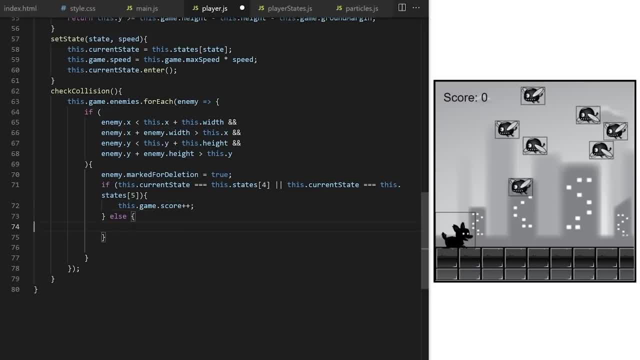 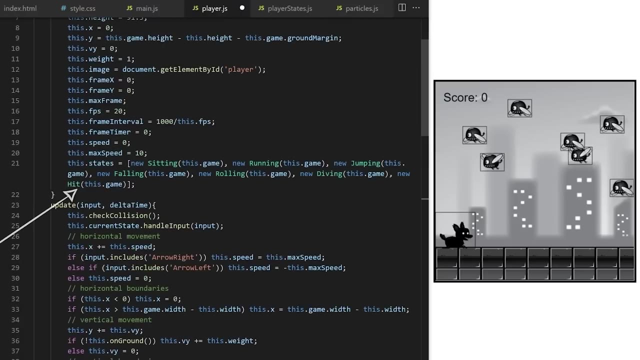 in increase the score Else, meaning the player collided with an enemy while it wasn't in one of those two states. it means player will get hit by enemy and it will play the hit animation. We will, of course, get no score points for that. I call thissetState and I pass it 6, the index of hit state and I pass it speed 0 because 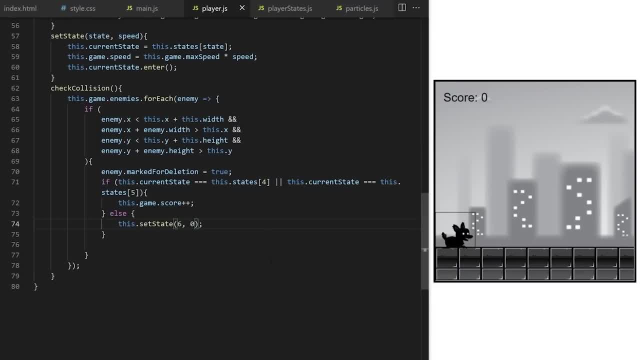 I want the game to stop moving for the duration of this state To properly emphasize that we collided with something. If I test it, I can see the score is correctly increasing as we hit enemies in rolling or diving state and if we collide with an enemy while not in one of these states, we enter. 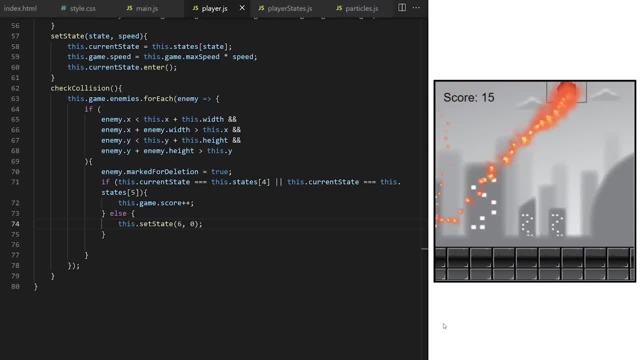 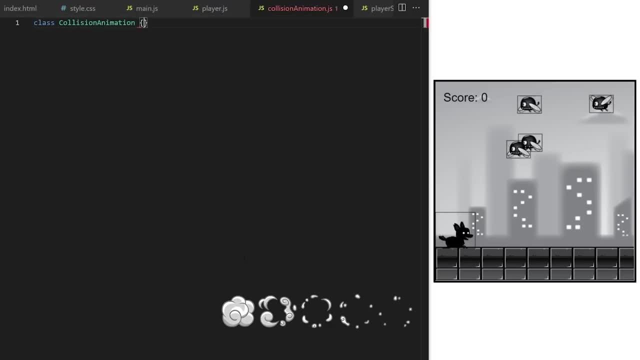 hit state Perfect. Great job. if you are coding alone, hope you are getting a lot of value. When the player collides with an enemy, I want to run this speed. Let's handle that logic in a separate module. I will call it, for example, collisionAnimationjs. 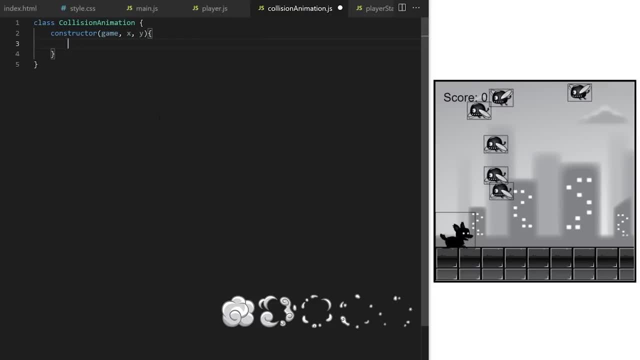 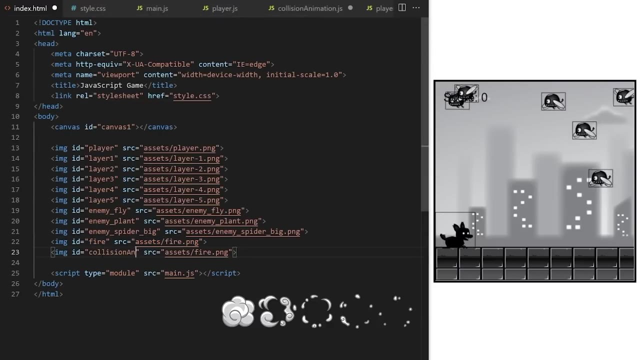 You know how we do this by now. There will be a class called collisionAnimation. Constructor will expect game object reference and x and y positions. We convert game into class property as usual. You can download the image in the video description. I place it in my assets folder and I link it here in indexhtml. 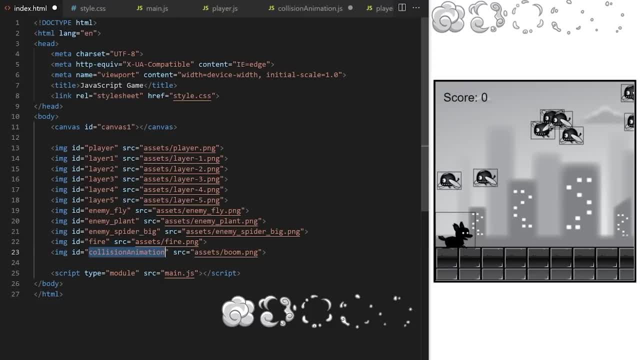 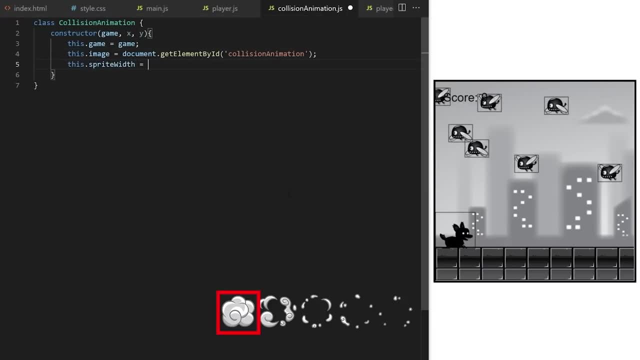 I give it an id of collisionAnimation. I hide the image with css. Sprite width: The width of a single frame is 100 pixels. Sprite height is 90 pixels. We will have size modifier to randomize the sizes a bit. It will be a random value between 0.5 and 1.5.. 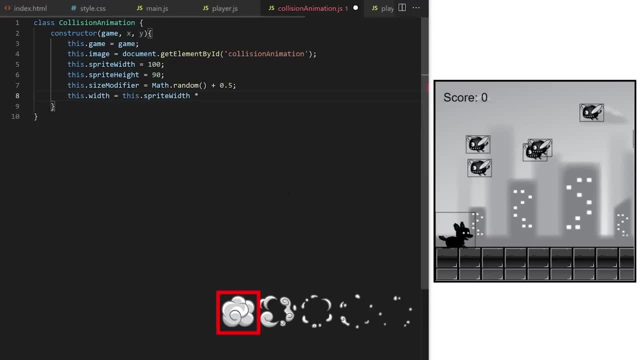 The width will be multiplied by this dot modifier value. like this: Sprite width times size modifier. Height will be sprite height times size modifier. It's a rectangular image And I want x position to be in the middle of the image. That's why I waited until now to convert x and y into class properties. 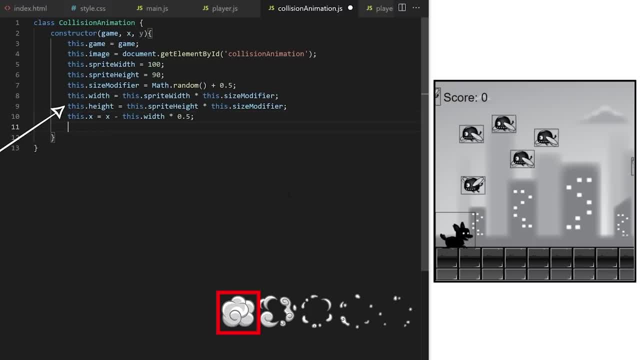 We can only do it after we calculate the width and height of the animation. I want to push x and y over the center of the animation, So x will be x coordinate, passed as an argument, minus half of the width, Y will be y coordinate minus half of height. 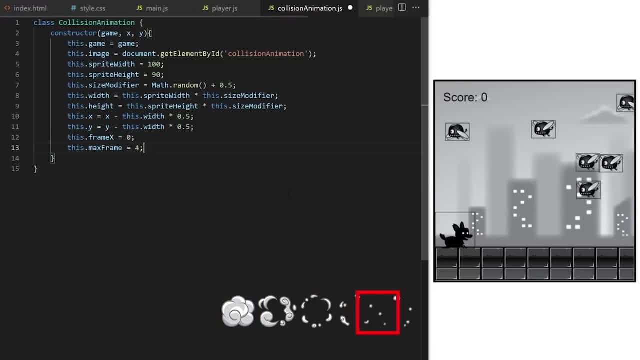 Frame x will start at 0.. Max frame is 4.. Marked for deletion will be false at first. We are out of time. We are animating a sprite sheet, so, as usual, we use a draw image built in method and pass it. 9 arguments. 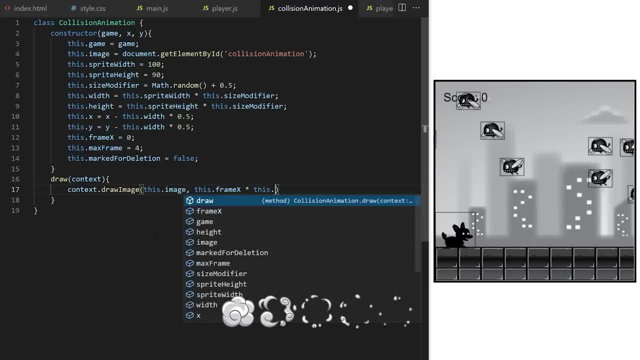 Image we want to draw, so this dot image from line 4.. Source x will be frame x Times. sprite width for horizontal navigation around the sprite sheet. Source y will be 0, because this sprite sheet has only one row. Source width is sprite width. 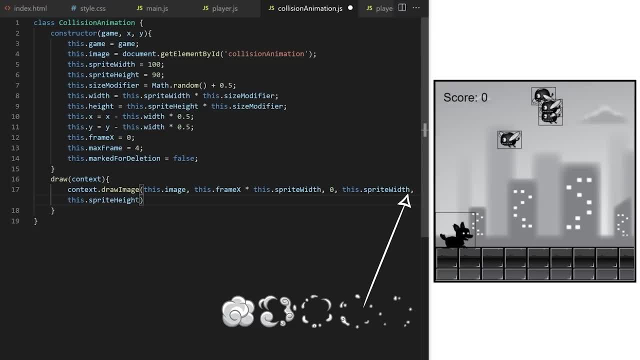 Source height is sprite height. So these 4 values specify which area we want to crop out from the source sprite sheet. Now I pass it 4 more values. Destination x will be this dot x from line 10.. Destination y is this dot y. 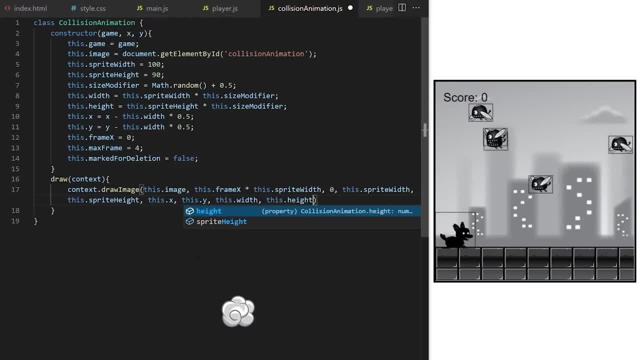 Destination width and height will be the width and height we calculated on lines 8 and 9.. These last 4 values determine where to draw that cropped out frame on destination canvas. Update method will make sure that collision animations move with the game world, so this: 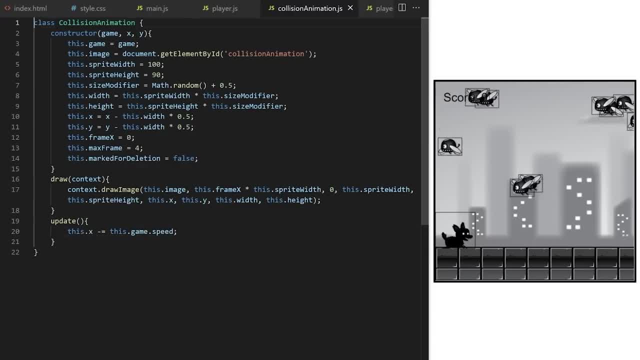 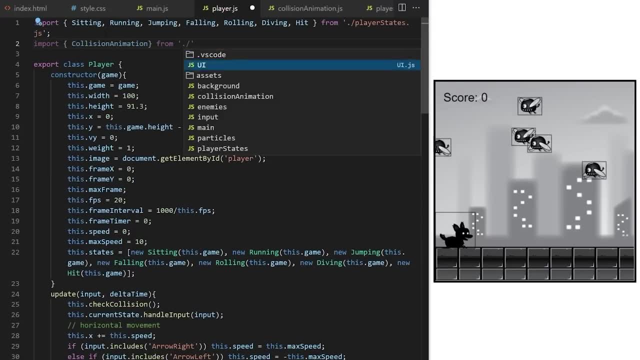 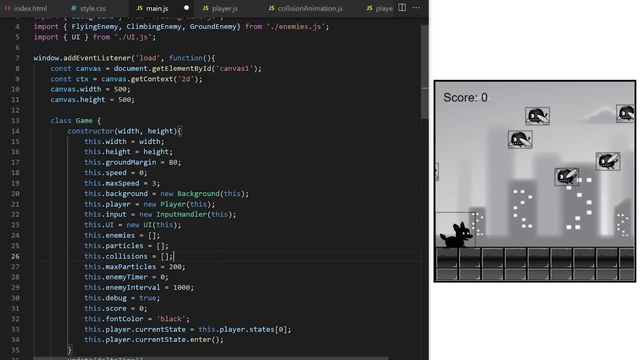 dot y minus equals this dot game, dot speed. We export the class up here on line 1.. I import it up on line 2 in playerjs because this is the module where we handle collision. I create an array that will hold all currently active collision animation objects. 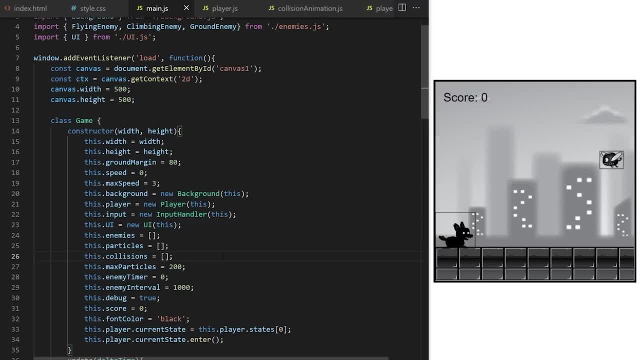 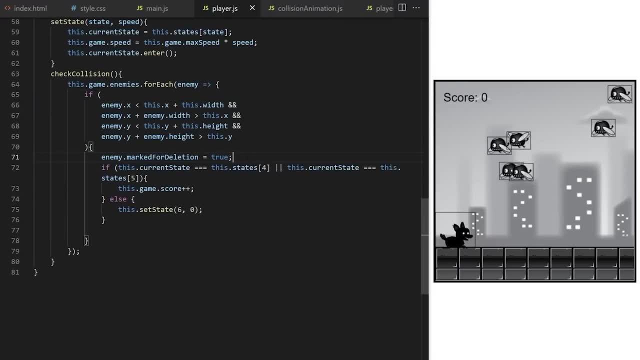 I call it this, dot collisions, and it will be an empty array at first. We have collision animation class available, so I go down to check collision method and every time player collides with an enemy we set marked for deletion on that enemy to true. and I will also push one new collision animation object into this dot collisions array. 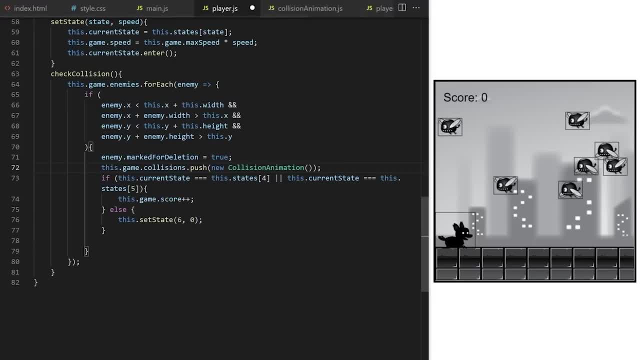 I can see it expects game x and y. so I pass it this dot game and I pass it x and y coordinates of that enemy. Since enemy is a rectangle, I pass it the middle of that rectangle horizontally and vertically. like this: I want the collision animation to be centered exactly over the enemy that just collided. 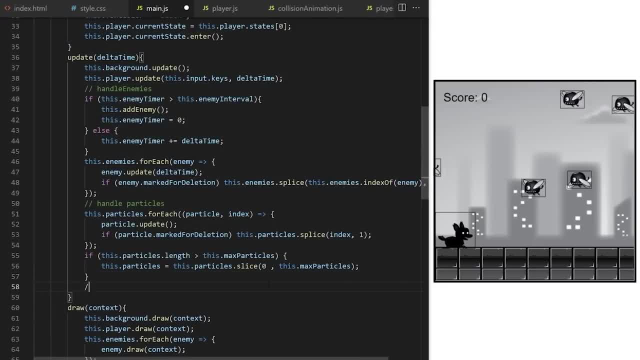 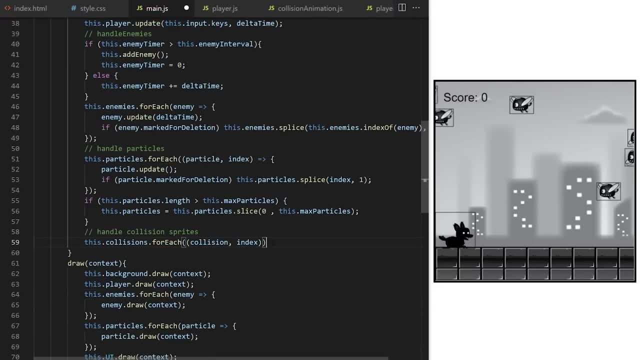 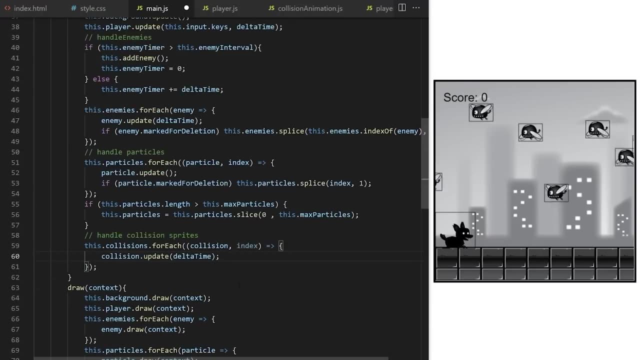 with the player Inside update method on game class. down here we will handle collision sprites. For each object inside collision array we will call its update method. Then I will pass it delta time because we want to slow the animation down. If that collision object is marked for deletion, I splice it out of the array. 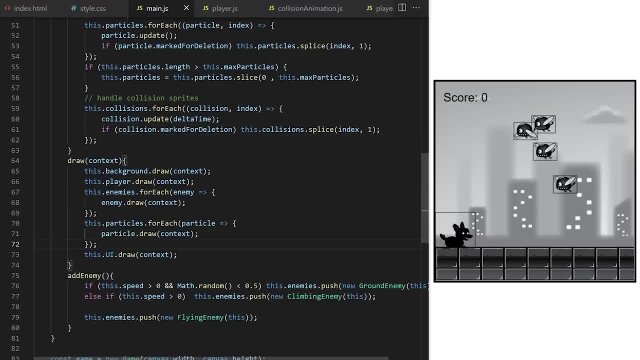 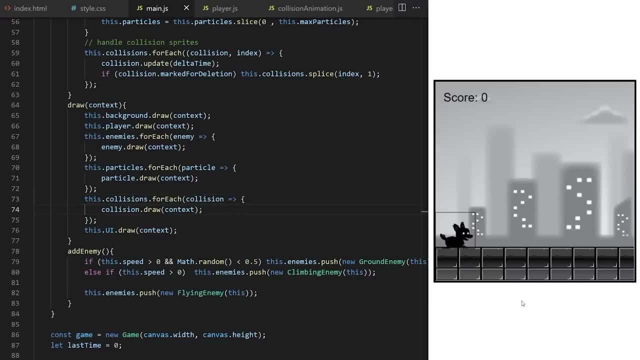 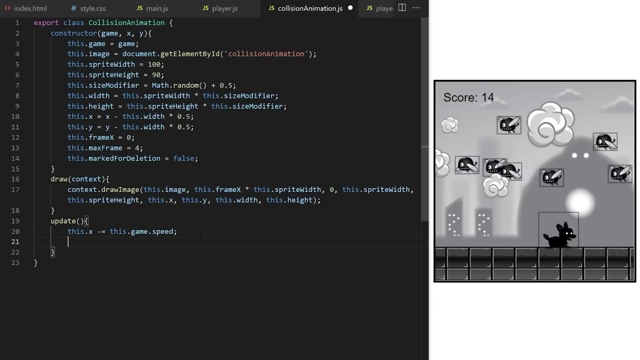 Same as we did with particles: Inside draw method. I will cycle through all the collision objects again and I will trigger draw method on each one. Nice, we are drawing collisions. We are just drawing the first animation frame in the sprite sheet. Let's go here inside draw method on collision animation class and animate frame x. 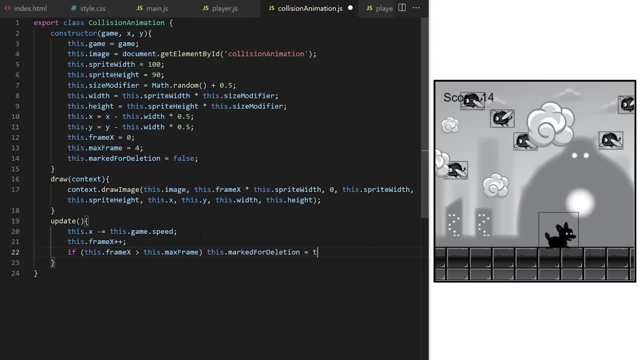 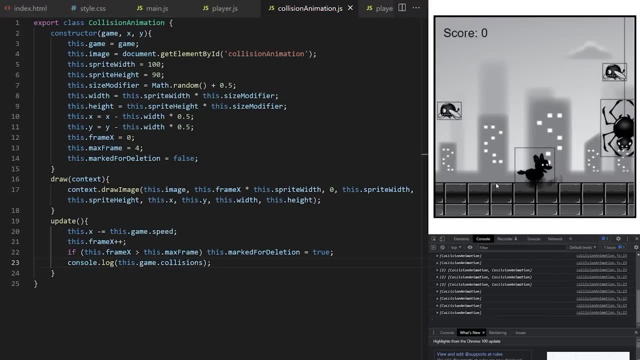 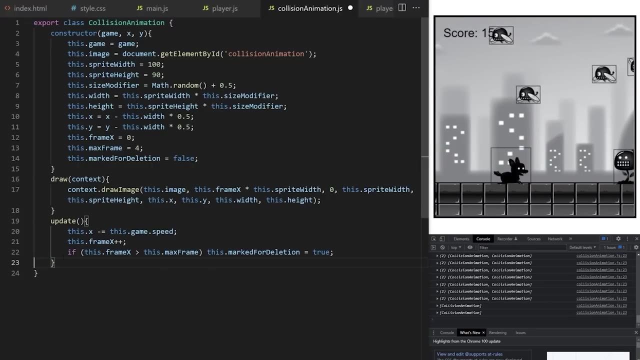 If frame x is more than max frame set marked for deletion to true. I console log collisions array and I can see that collisions are correctly being added and removed. I can delete this console log. Collision animations are running very fast. We can control their FPS. 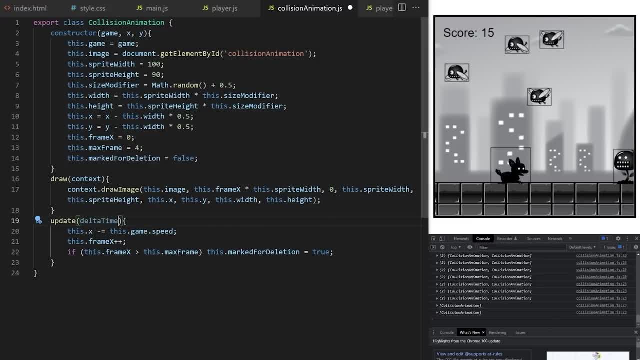 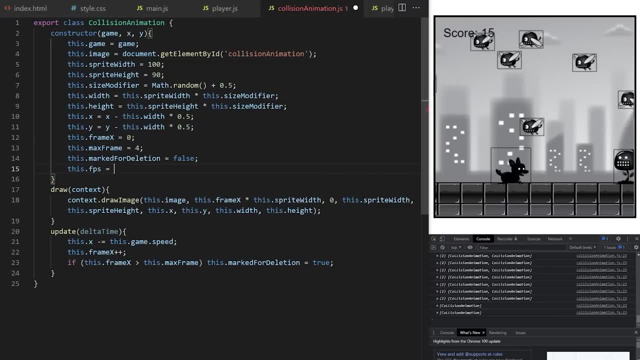 Frames per second using delta time. Delta time is the difference in milliseconds between the timestamp from this animation frame and the timestamp from the previous frame. It will be passed as an argument up here. We will need three helper properties. FPS will define frames per second. 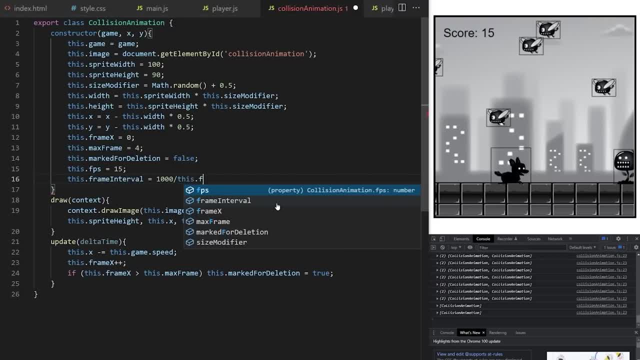 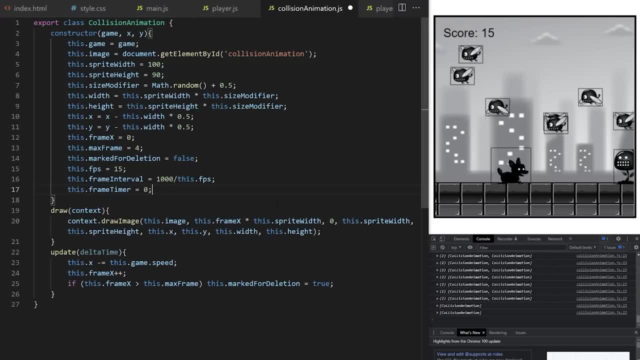 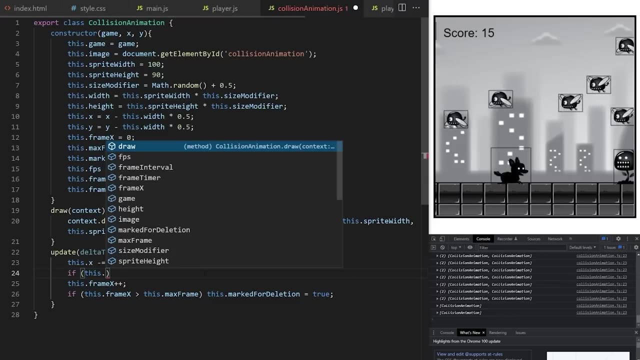 Frame interval will be the amount of milliseconds that need to pass before we serve the next animation frame. It will be 1 second, 1000 milliseconds divided by FPS. Frame timer will be counting from 0.. To frame interval over and over: Every time it reaches the value in our frame interval, it will reset back to zero and it. 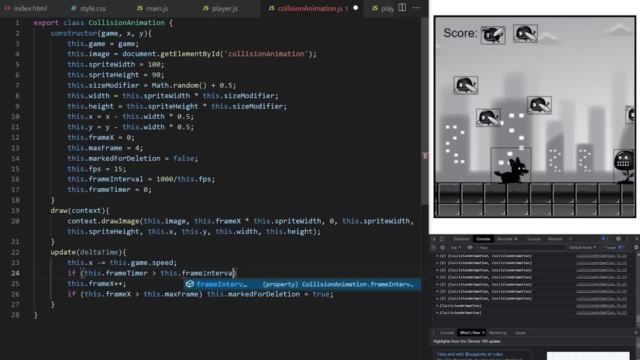 will serve the next animation frame in our collision animation sprite sheet. So here I say: if frame timer is more than frame interval, only then serve the next horizontal frame and reset frame timer back to 0 so that it can count again for the next loop. 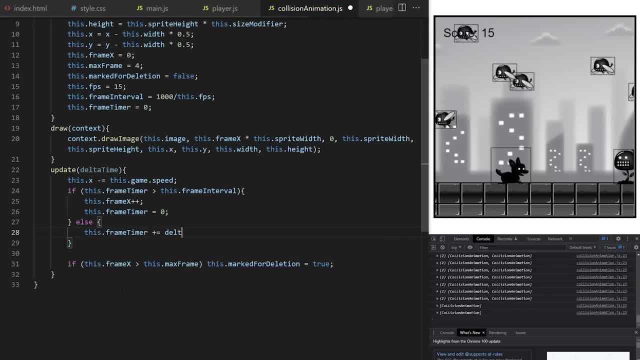 Else, keep increasing frame timer by delta time And in the end we will have a frame timer. If frame timer is more than frame interval, only then serve the next horizontal frame. and Now collision animations are animating at 15 frames per second. I can also 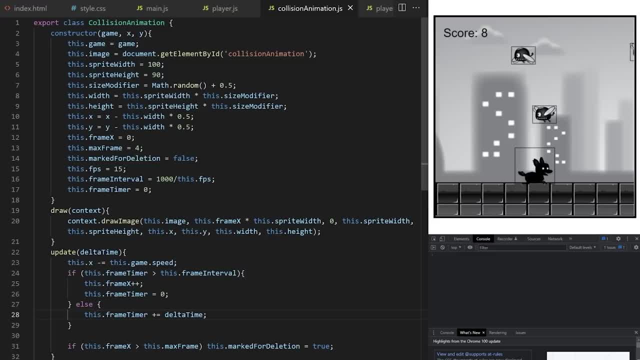 randomize that FPS. Not sure what that will look like. Let's try a random number between 15 and 25 frames per second. I can make that a larger number. It will be capped at 60 FPS. anyway, I think smaller numbers will look better since this. 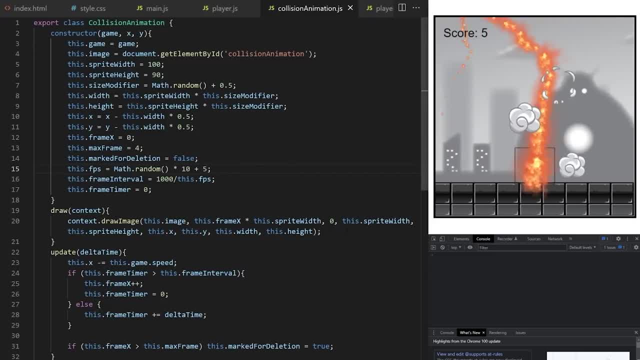 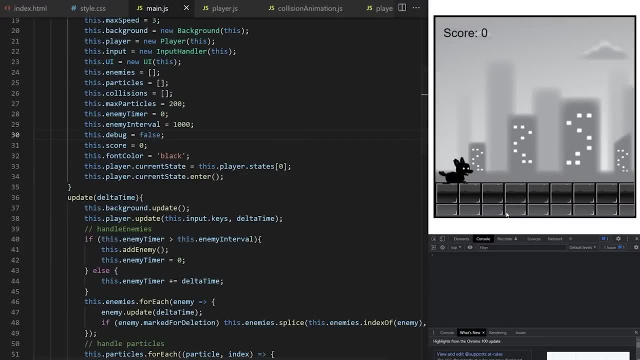 spreadsheet only has 5 frames. This will make sure they don't disappear too fast. I will set the initial value for debug to false so we don't see collision rectangles on the first page load. You can still view them by entering our debug mode by pressing the letter D. Win condition for this game will be a time. 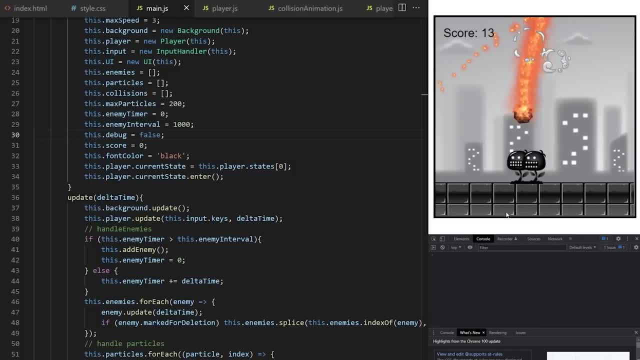 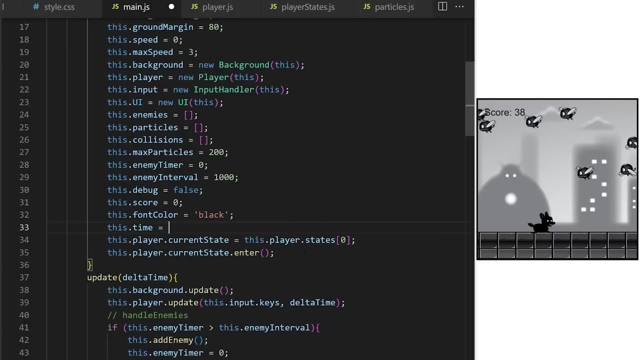 limit. We need to get as many score points as possible within a specific game time window. I want a fast-paced fun game. We will store game time in this dot time variable here on the main game object. When time reaches max time value, the game level is controlled. 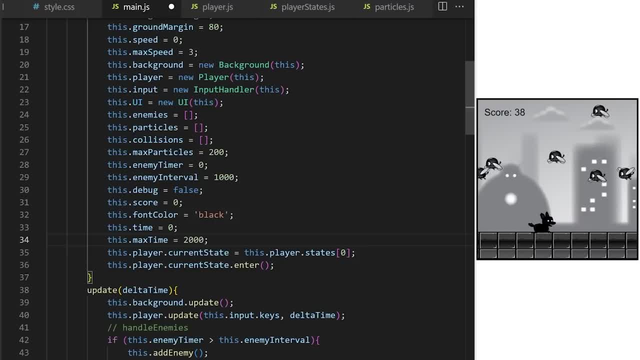 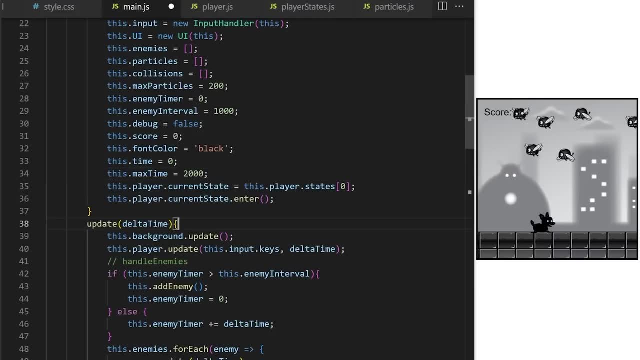 Complete. For testing purposes, let's set that time to 2,000 milliseconds- Two seconds just for now. Inside update method: we will be increasing game time by a delta time that's passed as an argument up here. Milliseconds between animation frames will be accumulating in this dot time variable, giving us the 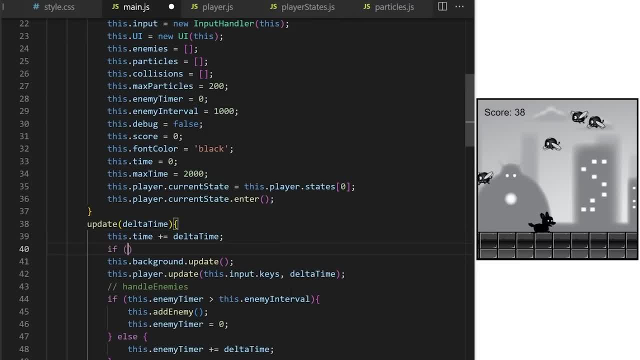 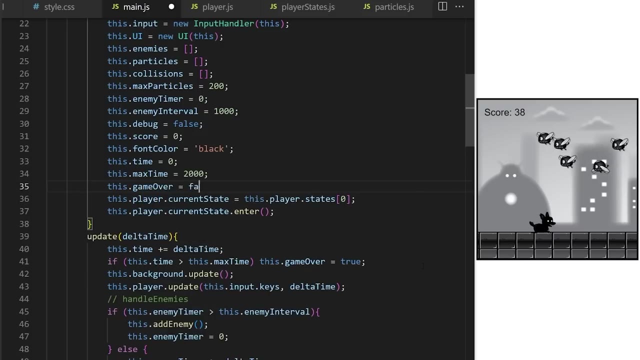 total amount of time that has passed since the game started. If time from line 33 is more than max time from line 34, we set game over to true. We need to declare this game over property up here. When the game over is true, I want to display a scoreboard, a custom message, and I want the game to. 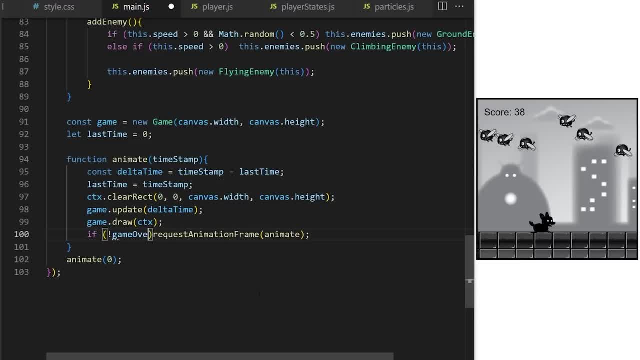 stop animating. Down here in animation loop I say only request the next animation frame if game over is false. This will make the game freeze and stop animating when the game over happens. I could also have just disabled controls and have the player running endlessly in the background. You can customize your. 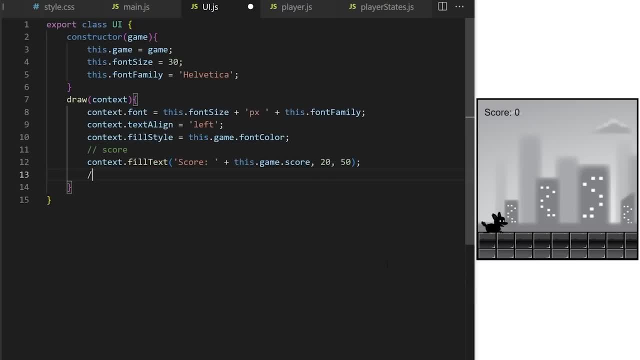 game over screen. later, based on your preferences, I open UIJS and here I want to display game time and game over messages. Let's start with the timer. I want the font to be smaller, let's say 80% of the font size we used to draw score. 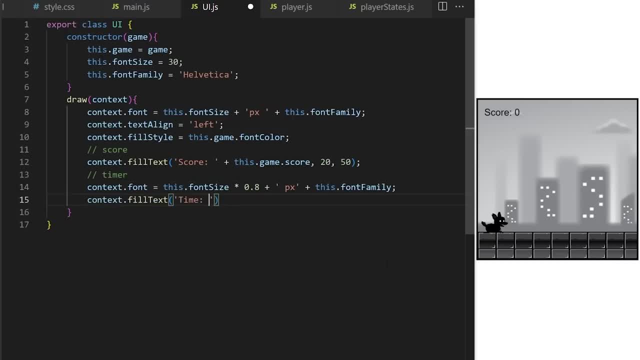 I call fill text and I say time, colon, space plus this dot game time at coordinates 20,, 80.. Nice, we are drawing game time. We will fix this, but first let's also draw game over message. If game over is true, set text align to left. 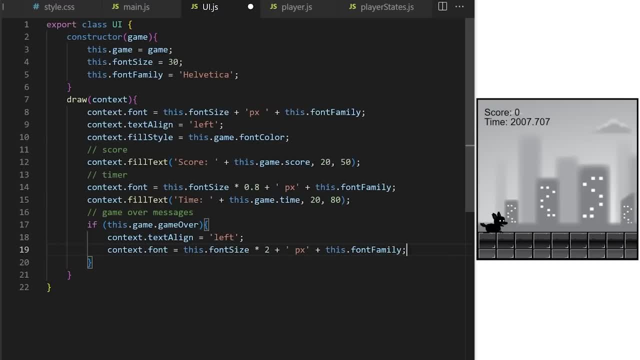 I want font size to be double of the base value. I will have two messages: One where the level is successfully completed and one for when the player fails to get enough score points in time. This will be the winning message. I will say booyah in large letters. 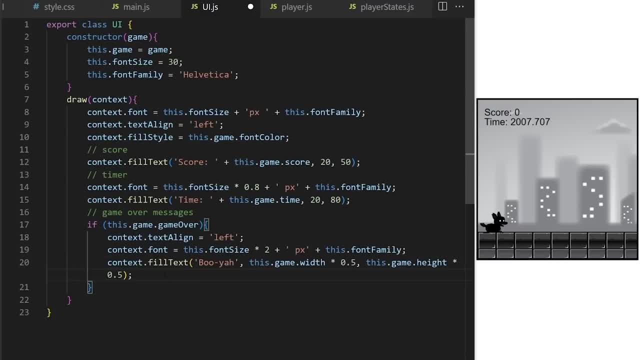 Coordinates will be the middle of canvas. So game width times: 0.5 and game height: Okay, I set text align to center. I need to fix this to actually set font size correctly. I need to move this space from here to here And the same on line 14.. 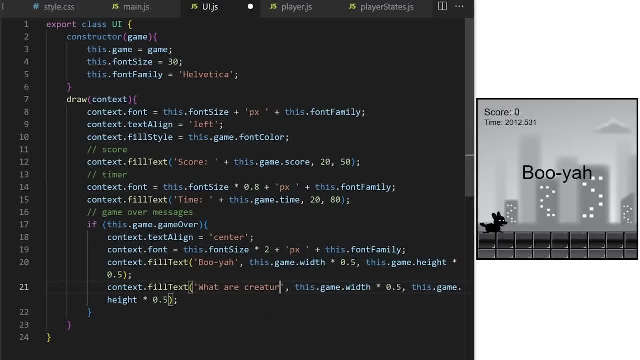 Nice Winning message will have a second line of text with smaller font size that says: what are creatures of the night afraid of You? exclamation mark. exclamation mark. This message will show up when we win. I change font size to 70%. 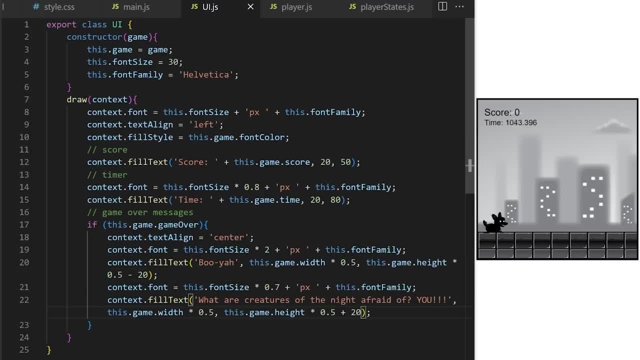 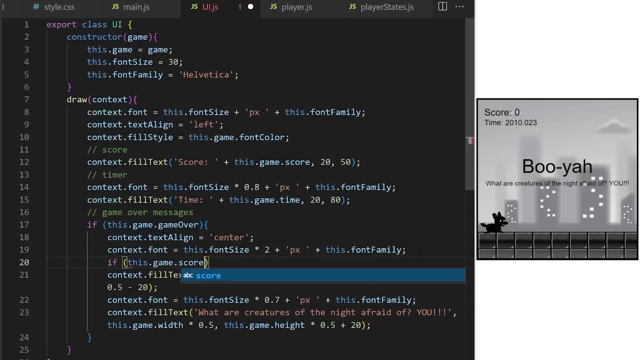 I move the first line up 20 pixels and the second line down 20 pixels. Nice, so this is our winning message. I want this message to display if score is more than 5, for example. This is just for testing purposes. When we have the whole game working, you can tune it and you can set game time and the score. 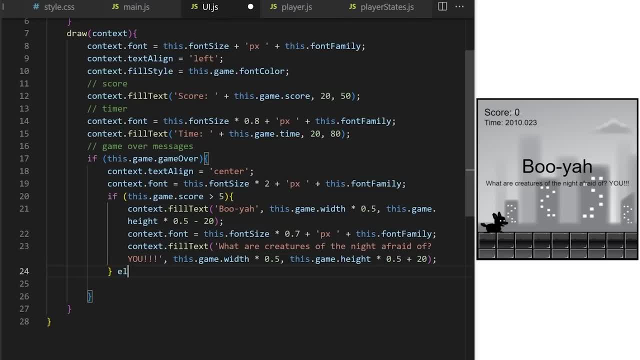 required to win the game, to different value depending on how difficult you want your game to be. If game score is more than 5, we display this message. Else meaning game over is true and game score is less than 5, we display a different message. 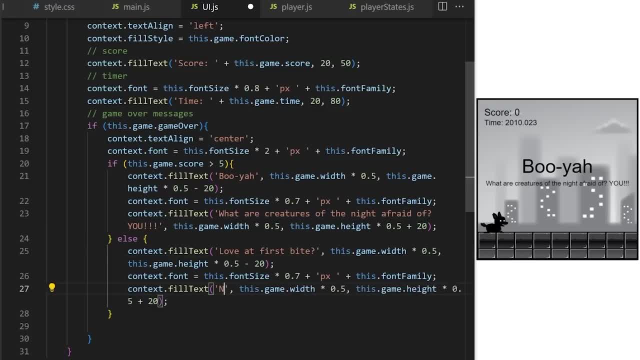 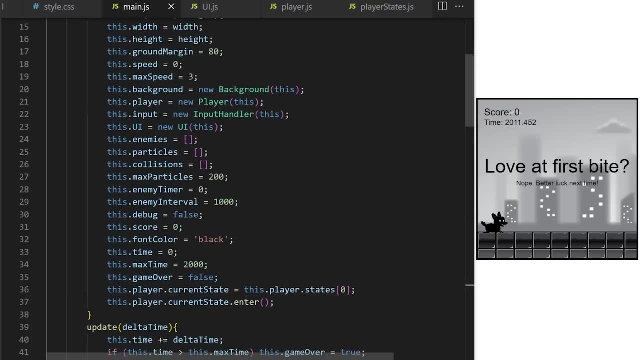 I will say love at first bite. I like to keep the halloween theme. The second line will say: nope, better luck next time. So this is when we fail the level. To test it, I give us more game time so we can get enough score points. 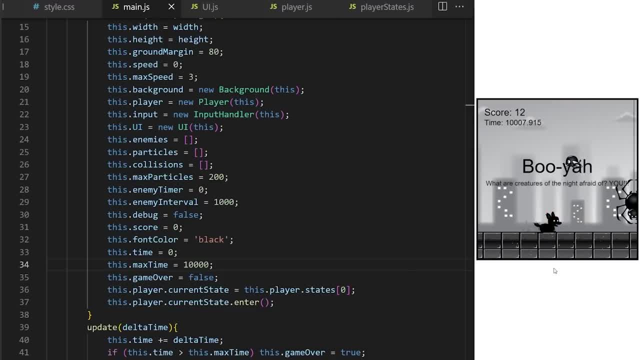 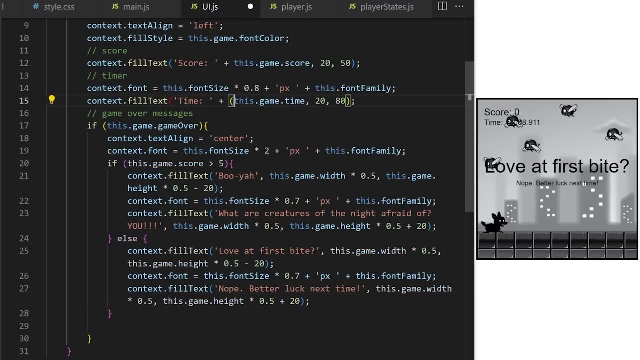 10 seconds, Nice. win condition works well. And now lose condition, Let's wait. Perfect. we can also lose if we don't get enough score points in time. We need to fix game timer. It's showing milliseconds. I want it to show seconds, so I multiply it by 0.001 to move the decimal point from milliseconds to. 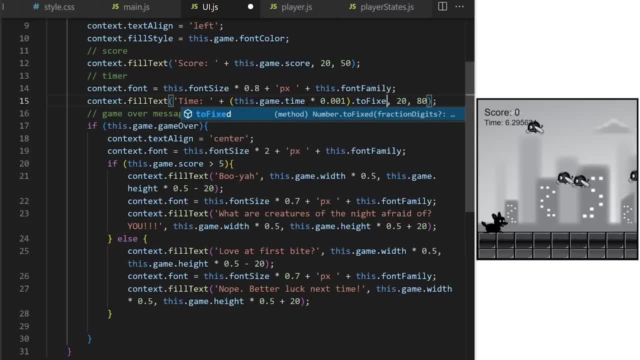 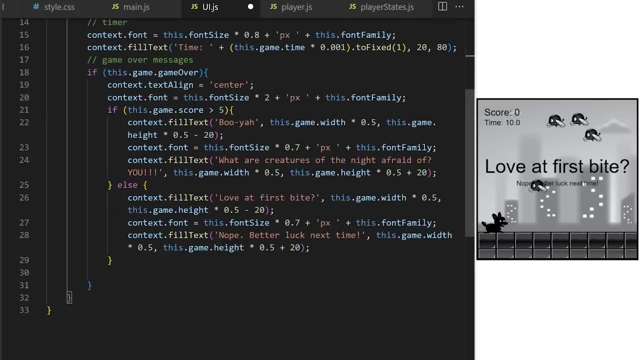 seconds And I only want to see one decimal space. So build in javascript to fixed method and I pass it. 1. We can also highlight the text to make sure it doesn't blend in with the background. I wrap all the code inside draw method on UI class between save and restore. 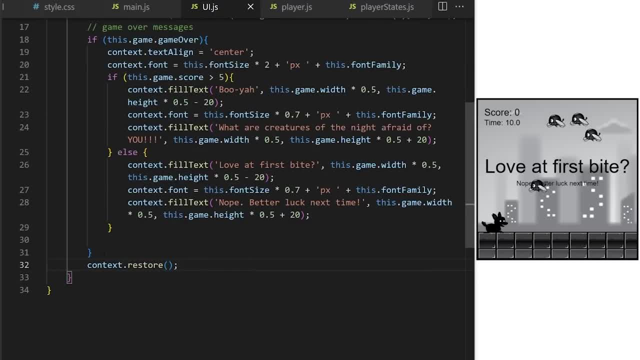 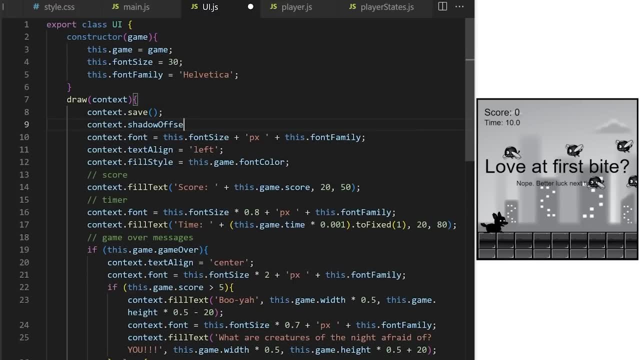 That means all the settings here will only affect this text. I want to apply canvas shadows and I don't want them to be applied to player and enemies. Canvas shadows are still not well optimized in firefox, so if you notice lower frame rate, I suggest you don't use them. 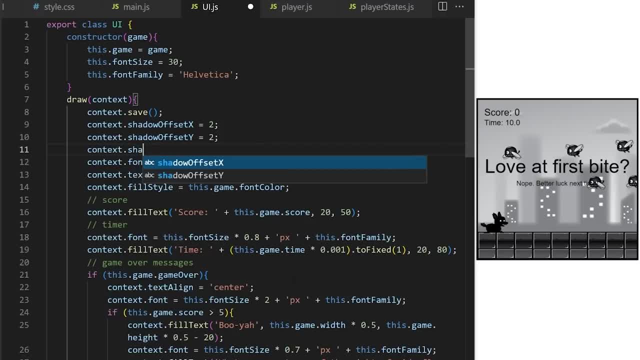 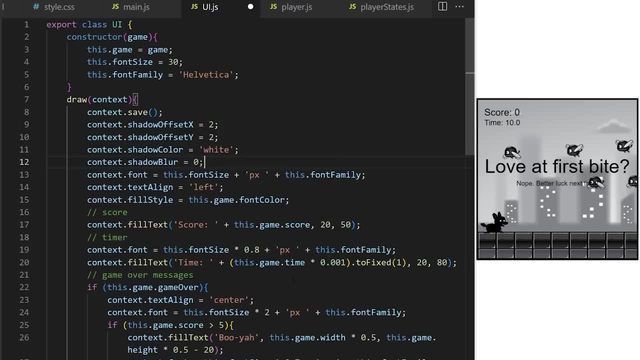 But if you want to know how to use them, it's simple. Shadow offset x- 2 pixels. Shadow offset y- 2 pixels. Shadow color white And shadow blur 0.. Now our text gets a nice white highlight. We could also achieve the same effect by drawing the same text twice, and the second one would: 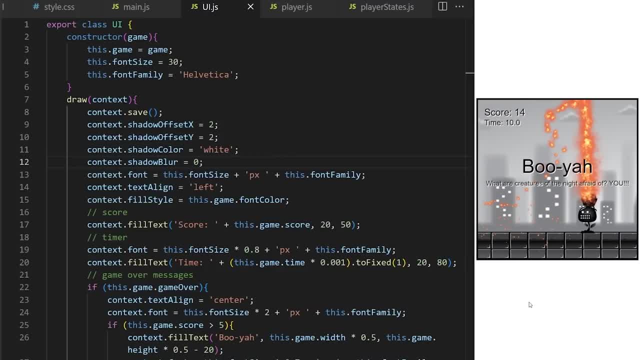 have 2 pixel Horizontal and 2 pixel vertical offset. That would be more code, but it's more performance efficient than using built in canvas shadows. Let's clean up the code and fix some small bugs we have here. When the player gets hit, I don't want it to be able to move left and right. 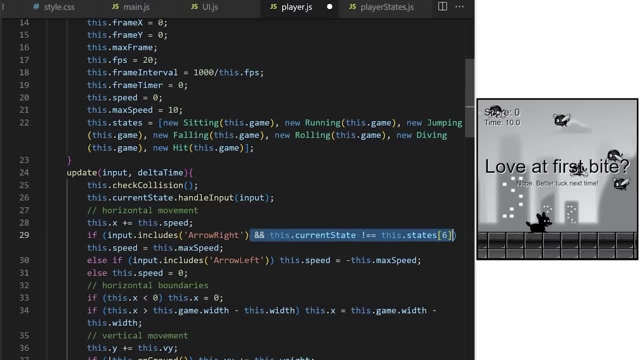 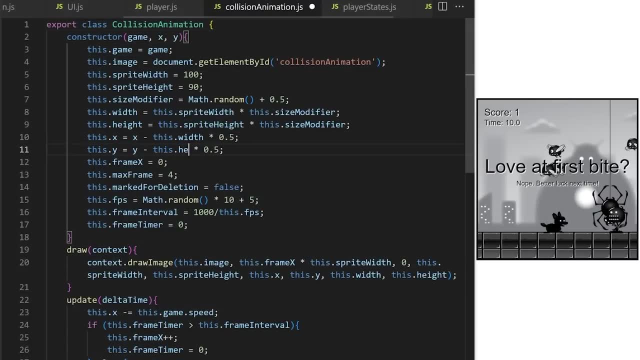 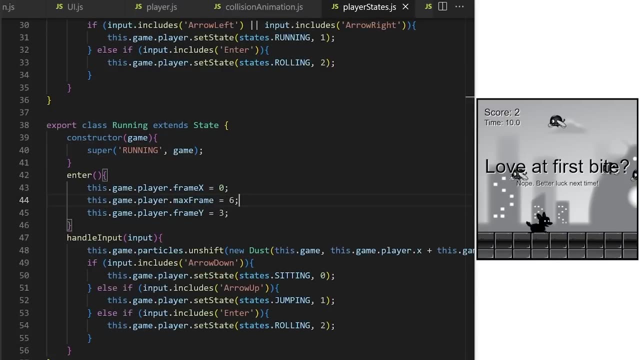 When the player is in state 6, left and right arrow inputs will be disabled. On line 11 in collision animation js we are calculating vertical y coordinate, so this value should be height. In running state we are setting max frame to 6. We are missing 2 frames. 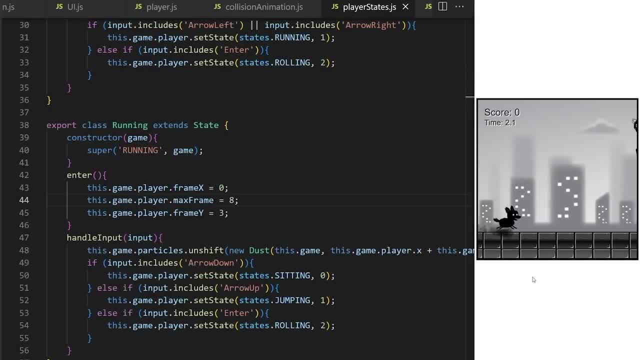 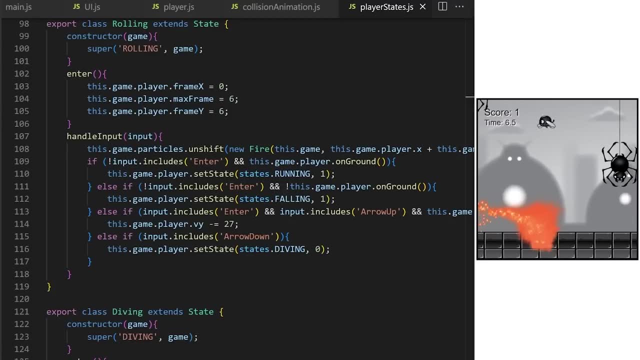 Max frame should actually be 8.. When I'm rolling on the ground and I press down arrow, key player starts diving and it's causing this weird movement pattern. We are not supposed to be able to do a dive attack when we are on the ground. 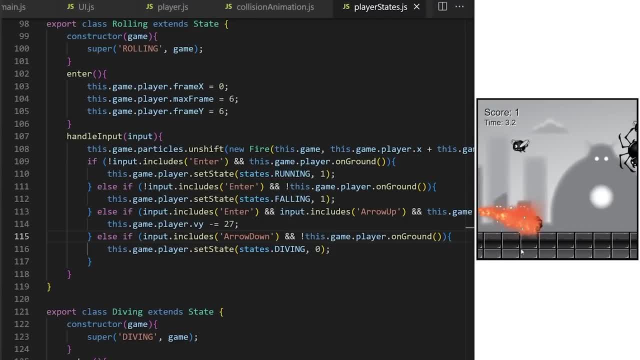 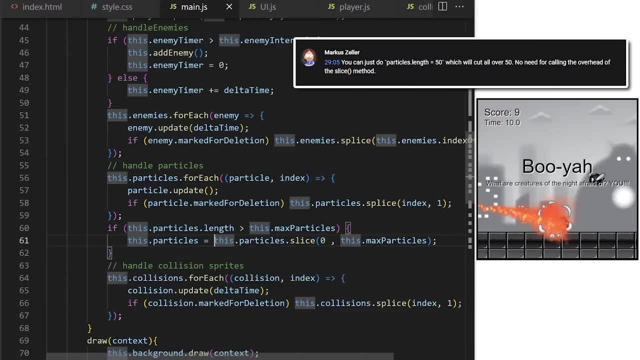 We can only switch to diving state when the player is not on the ground, Like this. That fixed it. One last small thing is here on line 61 in main js. We don't really need to call slice method. We can just set length of particles array to max particles value, like this: 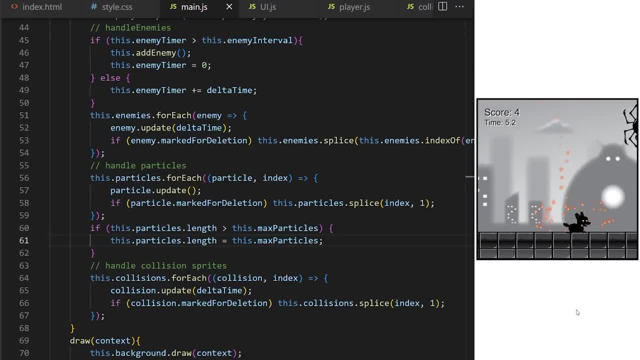 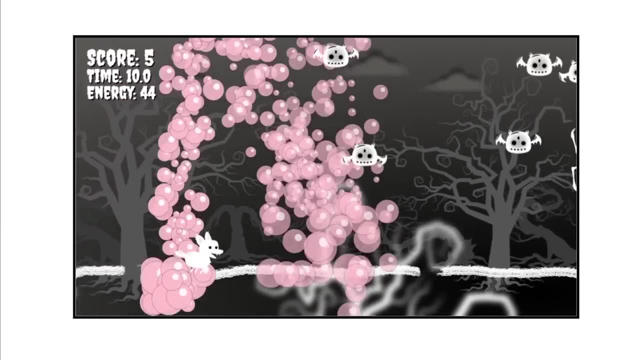 In the next episode we will add more bonus features, but from this point you can consider the game complete. Feel free to add your own features and run your own creative coding experiments. I'll see you in the next one. This is a final episode where we quickly implement some of the bonus features I showed in the 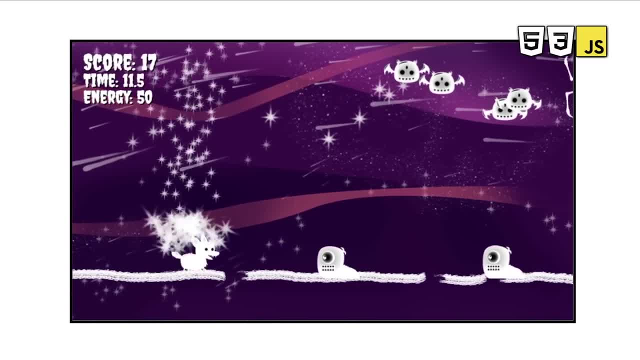 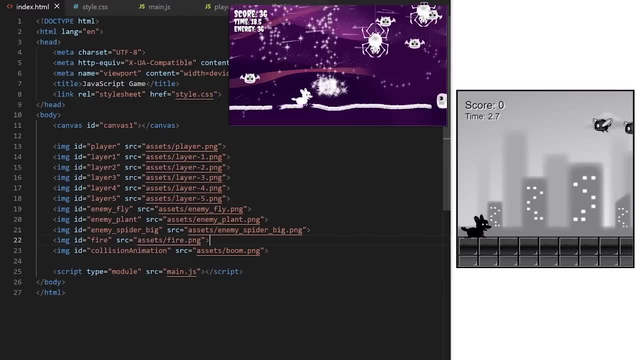 previews. We will improve visuals and clean up our code. I will start by quickly changing background images. just to keep things interesting, You can download the forest background layers in the video description and I just replace them in the assets folder overriding the city images. 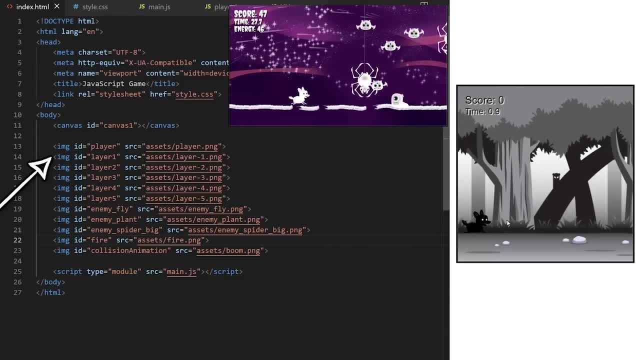 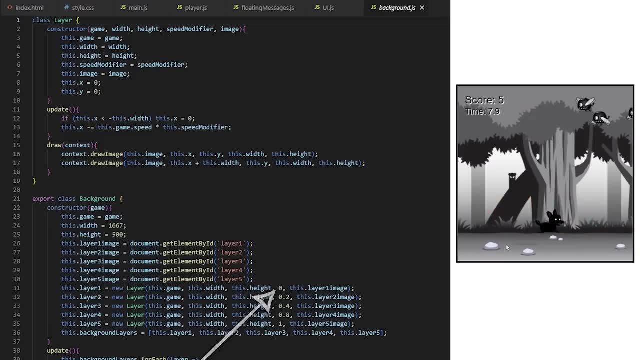 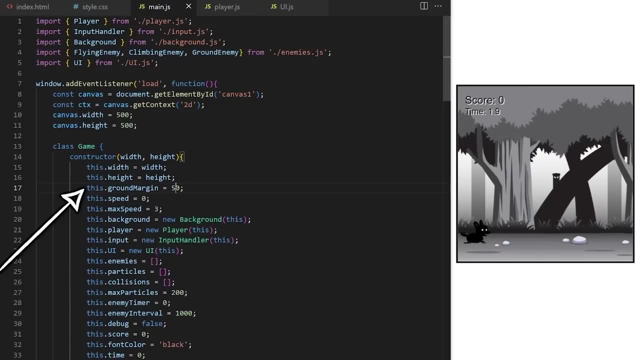 I backed the old images up somewhere else on my computer. You can also go to background js and adjust speeds of individual layers. Sometimes different background art looks better when speed modifiers on the background layers are adjusted. I also change ground margin on line 17 in main js to better fit this new forest environment. 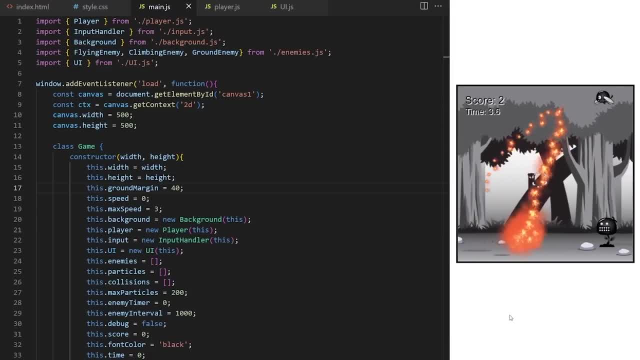 Since we are changing visuals, let's also change the font to something nicer. You can go to google fonts and choose any font from there. It will all work and it's very easy to implement. Let me show you with creepster, because this is a halloween themed game. 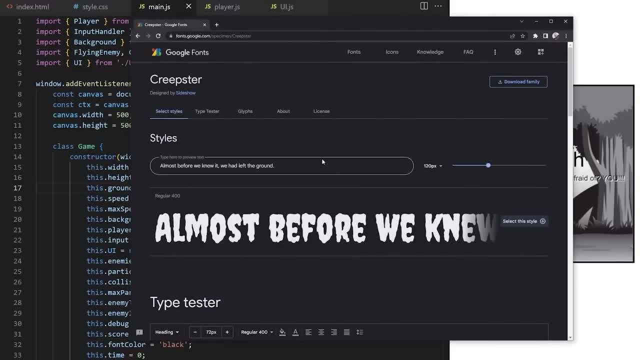 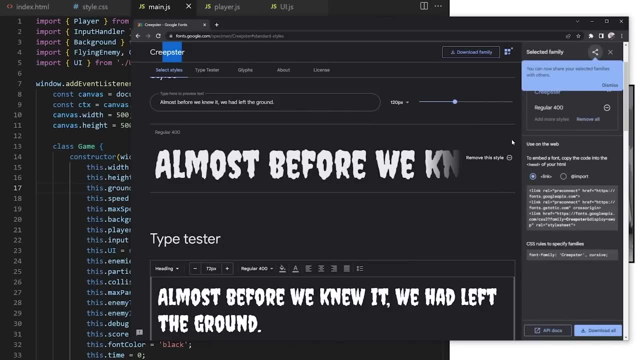 We are in a scary dark forest escaping from creatures of the dark. When you choose your font, click. select this style. Now I click up here and it will give us everything we need to use this font on the web. in our web browser game. I copy this link tag. you can also select multiple fonts and 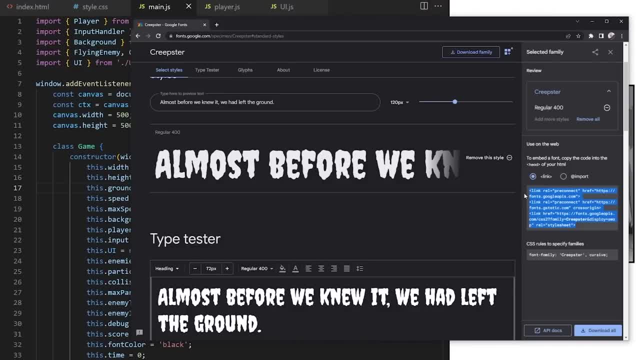 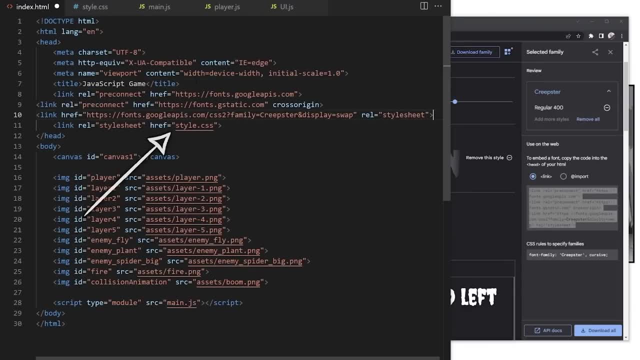 they will be automatically added to the same tag. I will use just one font for now. I copy the link tag and I paste it up here in index html. Notice I put it before my custom style css file because I want the font to be available. 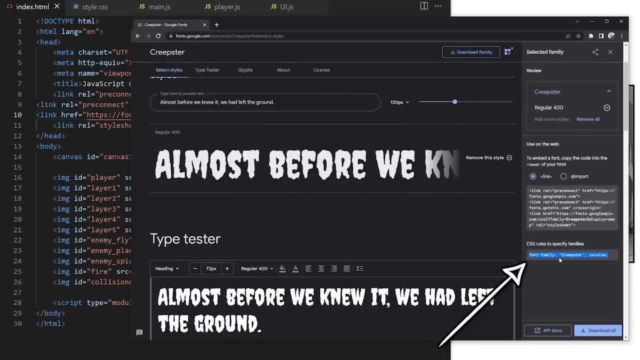 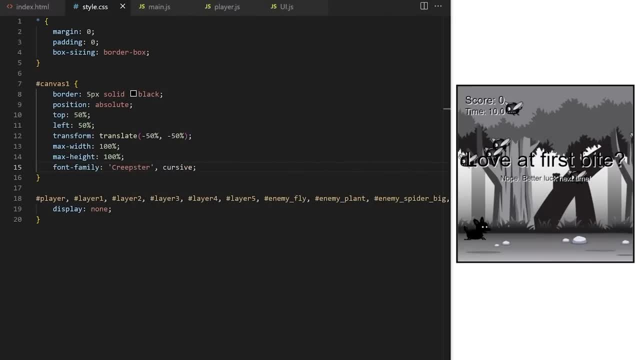 when that file loads. Then I just take this css rule and I apply it to canvas element. Now I can use this font all over my project and canvas will draw it. I will use it in UIJS for score timer and game over messages by replacing helvetica with 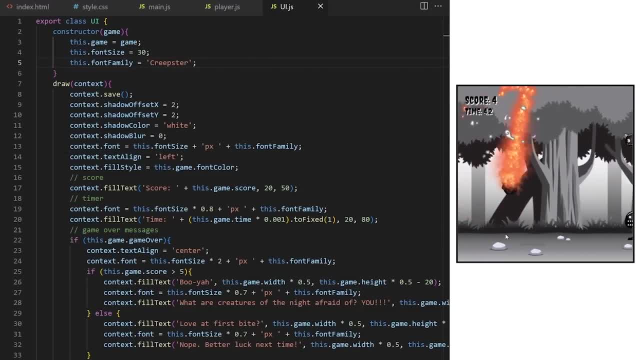 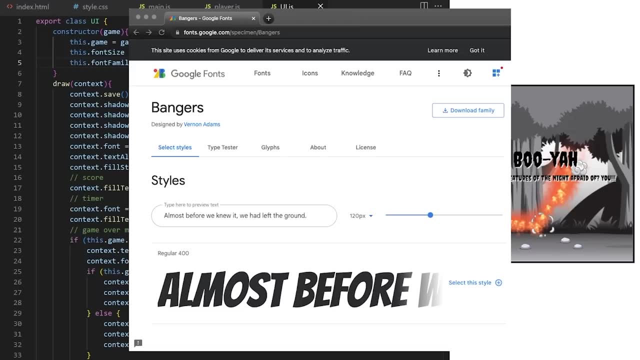 creepster here. I think this looks much better and you can choose from so many different google fonts to fit the art style of your game. I have other favorites on here, for example, a font called bangers for a really cool comic book art style. 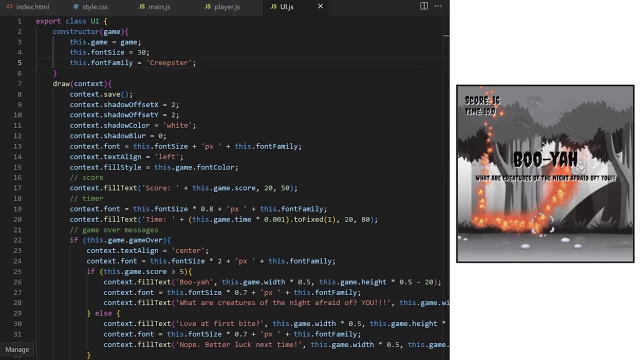 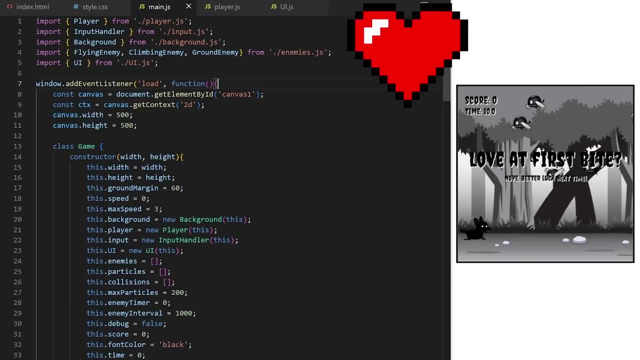 I want the player to have a limited number of lives and I want those lives to be displayed on screen. Each life will be represented by a small image of dog head. You can also use heart image or something completely different. it's up to you. 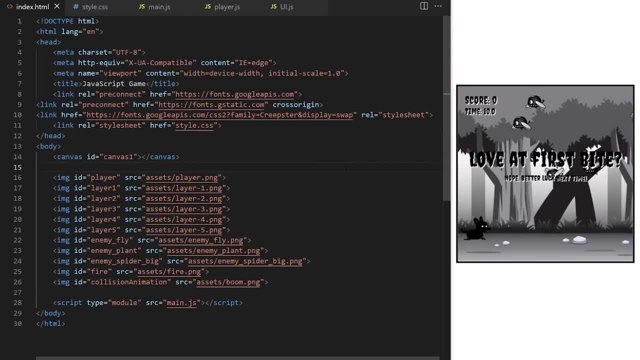 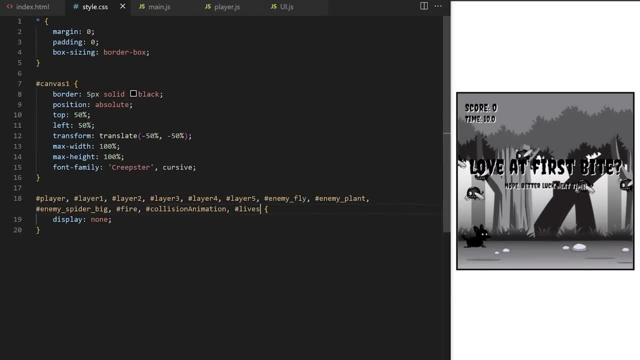 If you want to use the same image as me, you can download it down below. As usual, I bring it into the project Here in index html first, Then I hide it with css. I will be drawing the lives here in UIJS, so in the constructor I bring the image into. 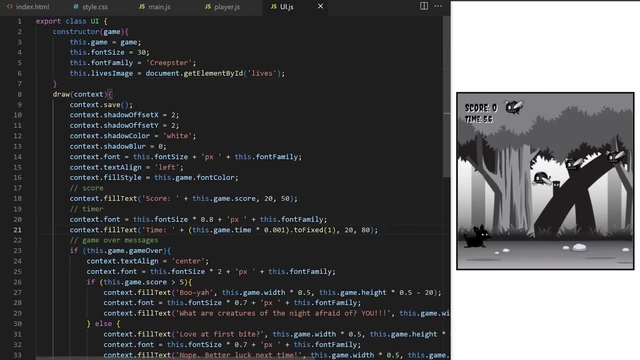 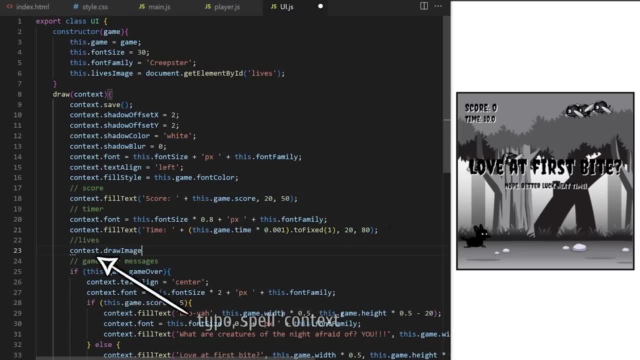 the project like this. I will call it, for example, thislives image. Down here under timer, we will draw player lives. I will call draw image and I pass it the image I want to draw. I want to draw it at coordinates 20, 95 and width and height will be 25 pixels. 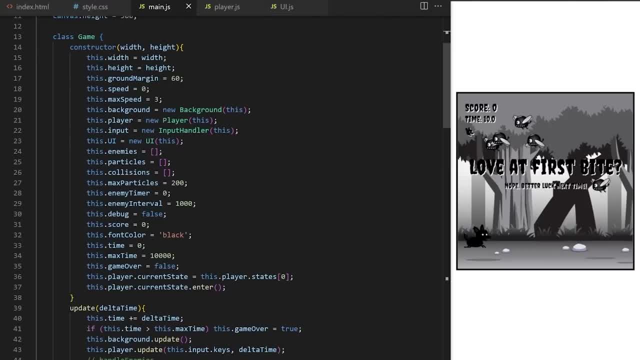 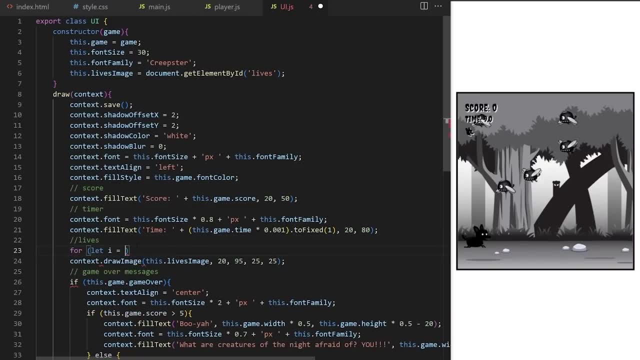 Nice. We are drawing it here. I create thislives property on the main game object. Let's start with 5 lives. Back in UIJS, I create a for loop that will run once for each life and it will draw an image that represents it. 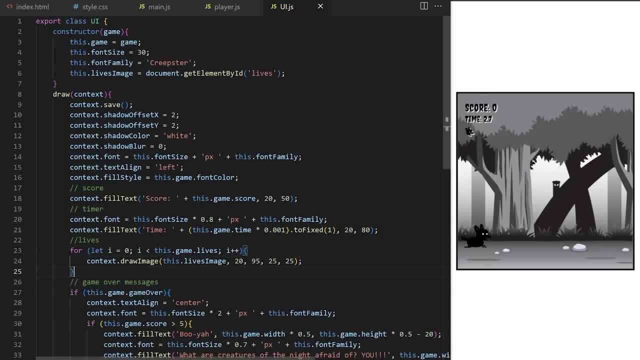 Now I'm just drawing 5 images on top of each other. I need to multiply horizontal x position times index from the for loop. Actually it will be the width of the image, so 25 pixels times index plus left margin of 20 pixels. 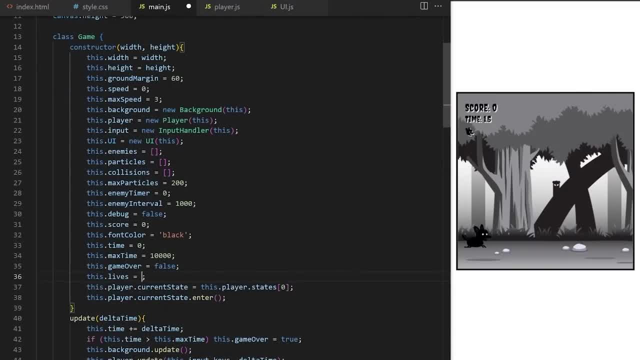 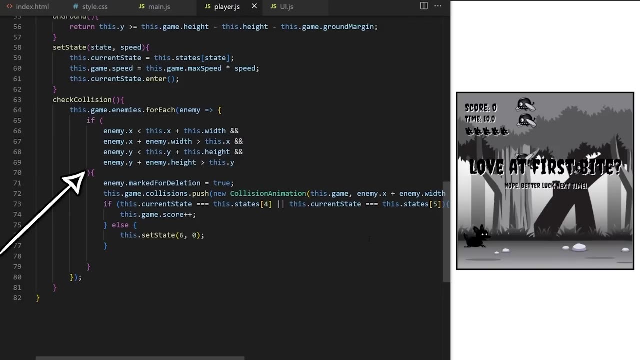 Perfect. Now when I change the value here, it changes how many lives are drawn on screen. Maybe you want your game to be easy. you can give the player 15 lives to start with. I will go back to 5 lives In playerJS, in the area where we handle collisions, when the player collides with an enemy while 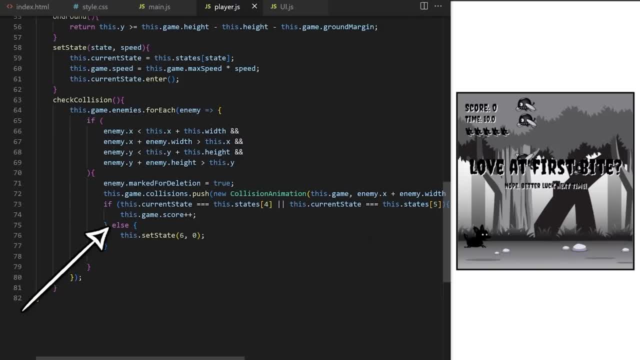 not rolling or diving. this animation is played by setting state to state 6. We call that state hit and at the same time I want to remove one life. so thisgamelives is minus. After we removed one life, we check if total lives are less or equal to 0 and if they are, 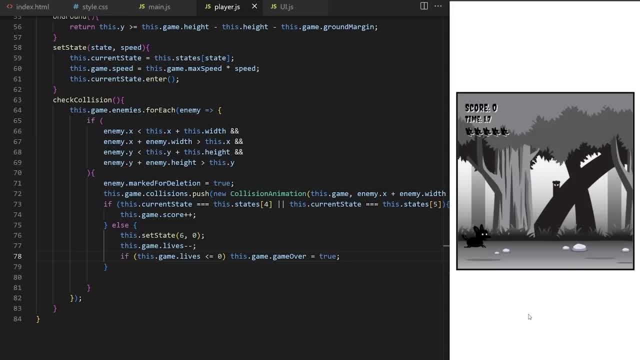 we set gameover to true. I test it by colliding with enemies on purpose. You can see that each time we collide we lose one life per enemy and when we lose the last life we get game over screen Perfect. I want score numbers to fly from enemies as we defeat them. 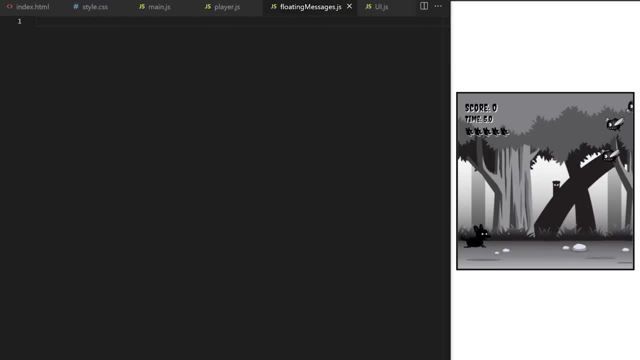 This can also be used for other floating messages in our game. I create a new file called FloatingMessagesjs. I create a custom class, I call, for example, FloatingMessage and I export it. Constructor will expect value of the floating text. start in x and y, position and target. 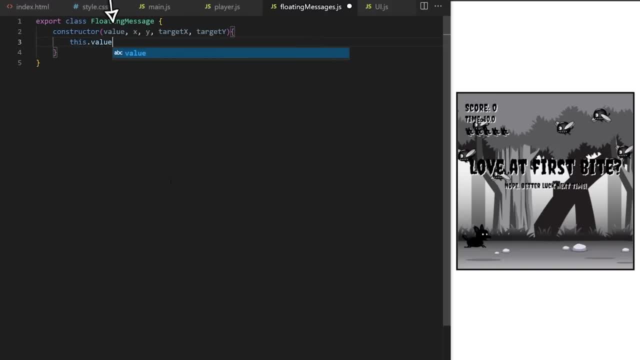 x and y position. Text with this value will float from this position to this position and then it will disappear. I convert these values to class properties, as usual. I also create a property I call timer, just to set some simple time limit after which the message is displayed. 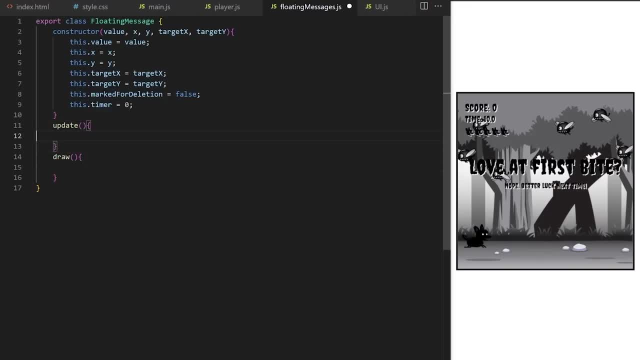 We will need update and draw methods as usual. Update method will push horizontal x position by the difference between target position and the current position, making it slowly move towards the target. Same for the vertical y position: Difference between vertical target and current vertical position. 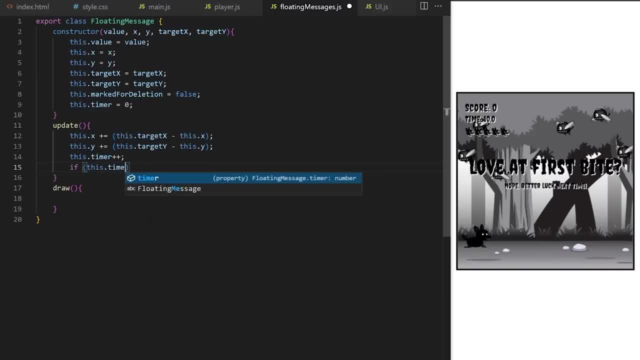 For each loop timer will increase by 1.. When timer is more than 100, we set marked for deletion to true. Draw method will take context as an argument. We set font to 20px. creepster, Fill style will be white And fill text will draw value from line 3 at its current x and y coordinates. 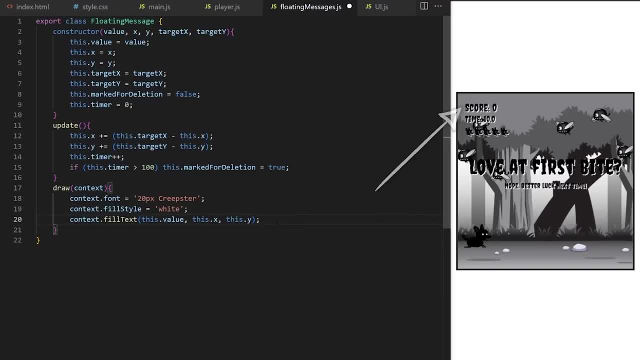 Now I show you an alternative to using canvas shadows For score and timer. we are using canvas shadow properties Here. we will achieve the same effect by drawing the same text twice White first, Then black on top of it, And we give it 2 pixels horizontal and 2 pixels vertical offset. 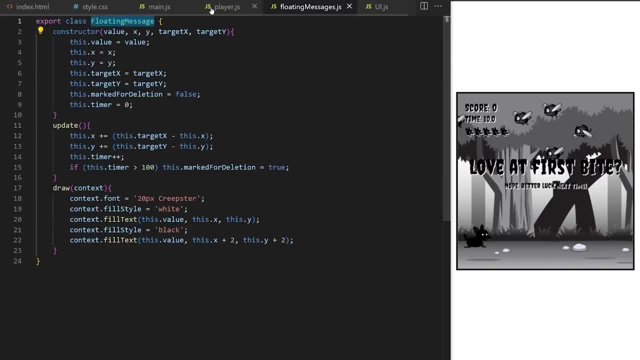 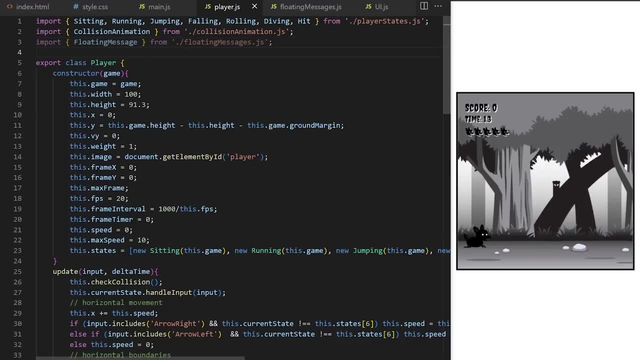 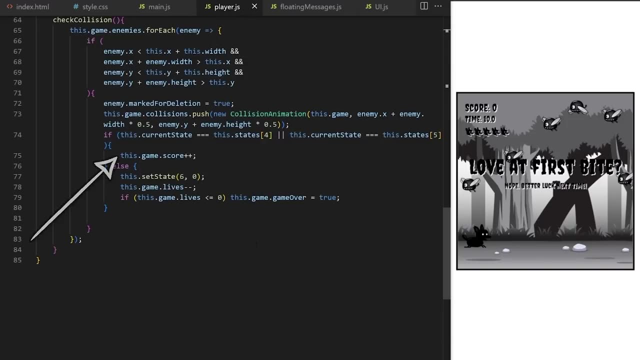 We are exporting our new floating message class. I import it up here on line 3 in playerjs Inside check collision method. when we successfully hit an enemy and score increases, I want those score points to fly from that enemy towards our scoreboard. I say thisgamefloatingmessages push and I want to use floating message class to create 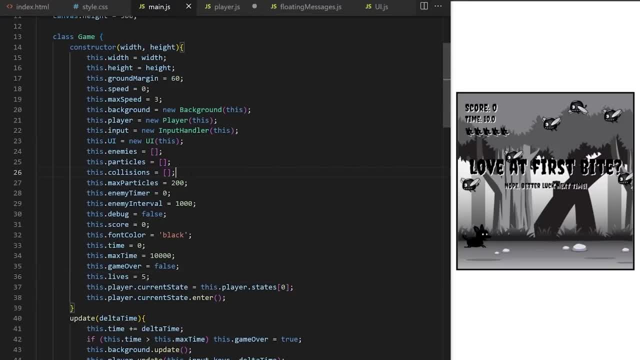 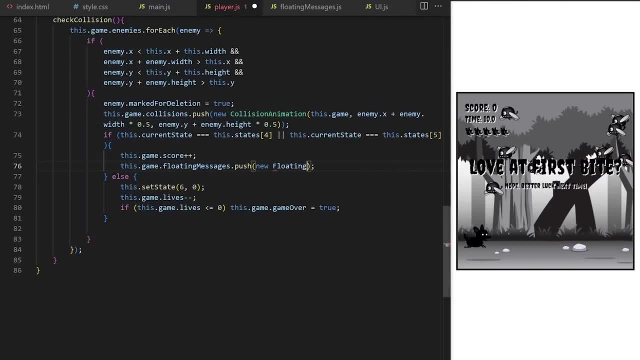 one new floating message object. But I'm too busy to do that, So I cut out the one that I have already created and create a new floating message object. With that friend of mine, I can create a new floating message effect on the mainjs class. 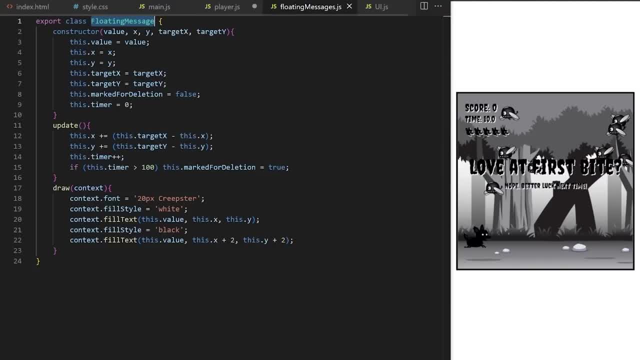 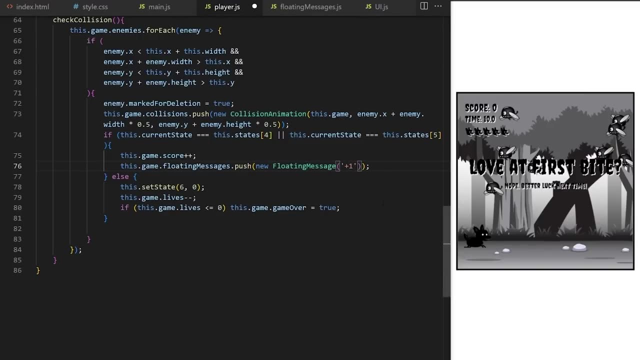 It will be an empty array at first. Now I'm pushing a new floating message into it like this: I check here and I can see that class constructor expects text value starting x and y coordinates and target x and y coordinates. Value will be plus 1 because we get 1 score point. 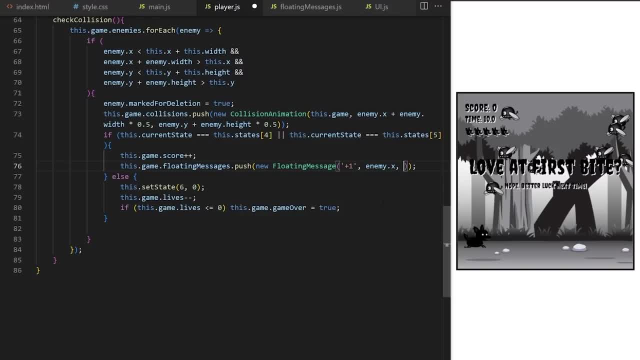 We could also make this value dynamic. if every enemy type gives different amount of scorepoints, coordinates will be x and y of the enemy we just collided with, and target x and y will be, for example, the top left corner of canvas. so coordinates 0, 0. 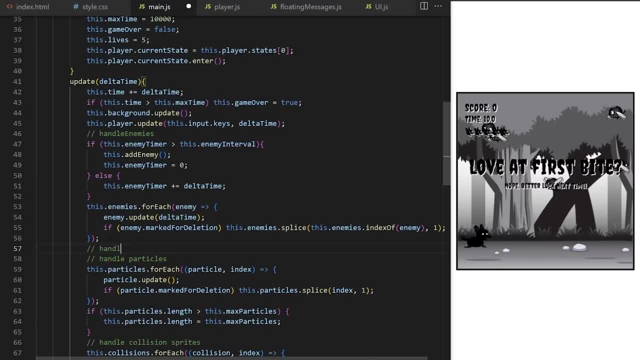 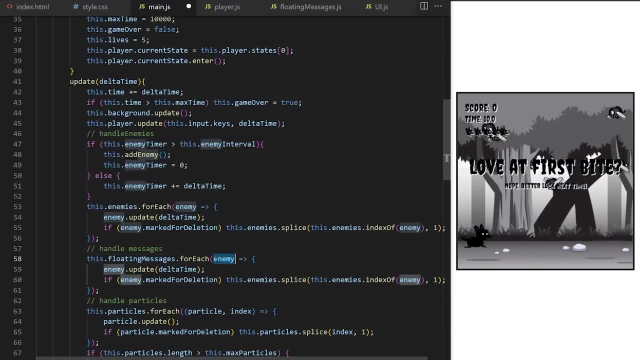 Inside update method on game class. The same way we cycle through all enemy object inside enemies array, we will also cycle through all floating message objects inside floating messages array. For each message, we will trigger its update method. I delete this splice to remove old messages because we will do it in a better way. I'll. 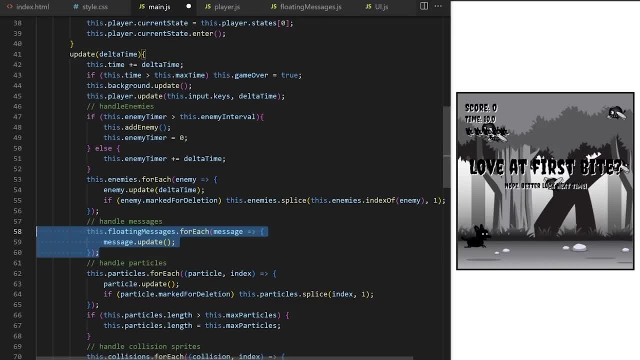 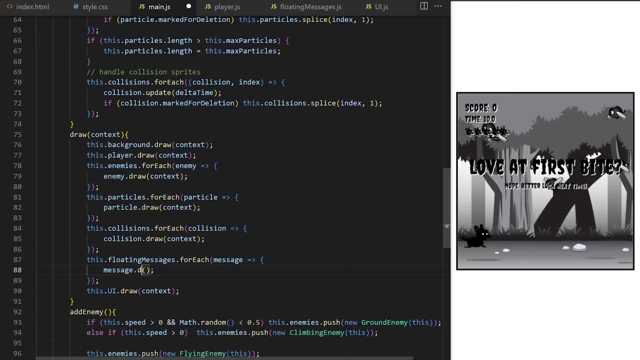 get to it in a minute. So for every floating message object I call their associated update method. I copy this code block and inside draw I also call draw method on every message and I pass it. context. If I play the game, messages will be moving too fast, so there is no animation, I just 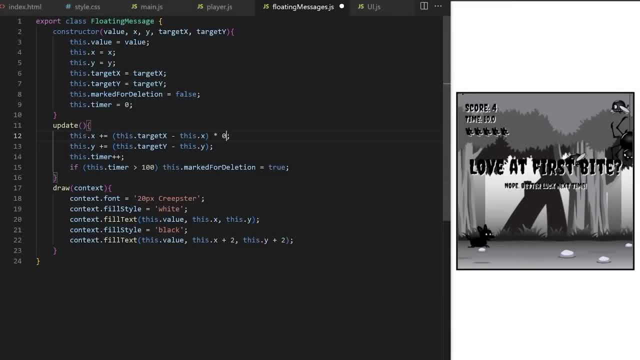 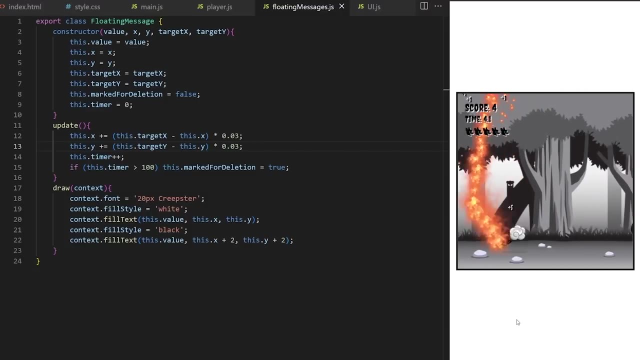 see the bottom of the letters. here I need to go to update method and I need to multiply both of these by 0.03.. So I'm saying here: for each animation frame, increase the current vertical and horizontal position By 3% of the difference between the target position and the current position. 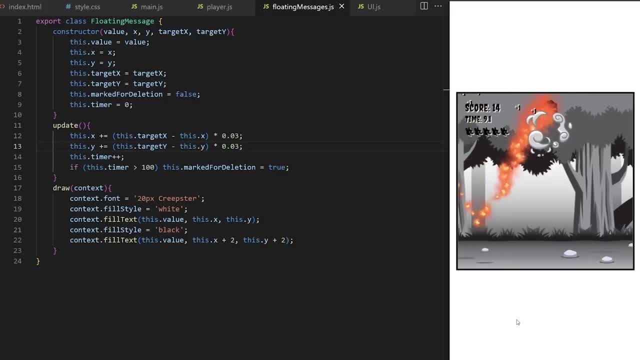 This will make the text move towards its target position by 3% of the distance per animation frame, Meaning it will start moving fast and as the distance between current and target position gets shorter, so it's a smaller number. 3% of that value is less pixels, so it will travel. 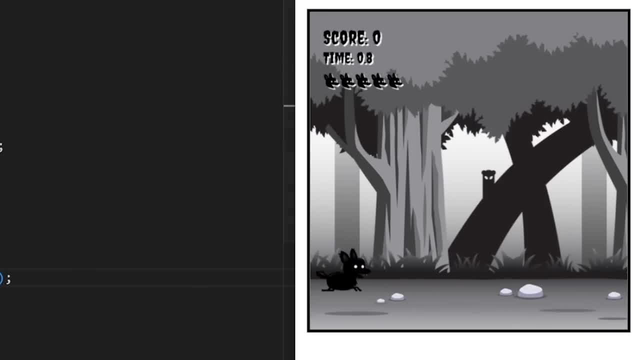 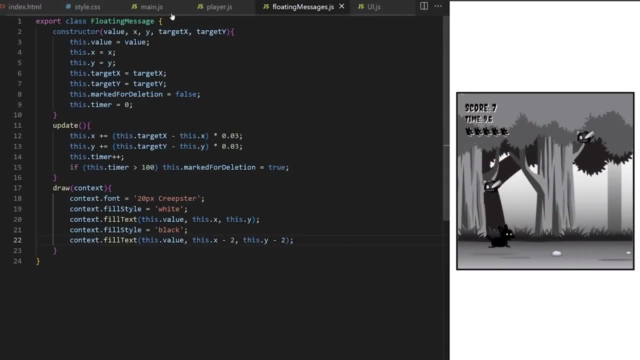 slower and slower, giving us a nice ease out effect. You can see that the movement is faster at first And it slows down As the letters float closer to target. 0,0 coordinates on canvas. I adjust the target coordinates. I want them to flow somewhere to the end of score line. 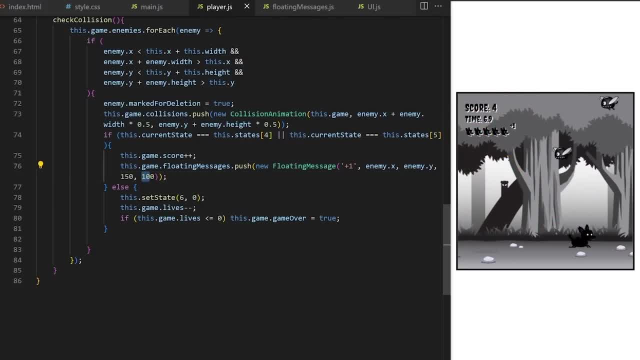 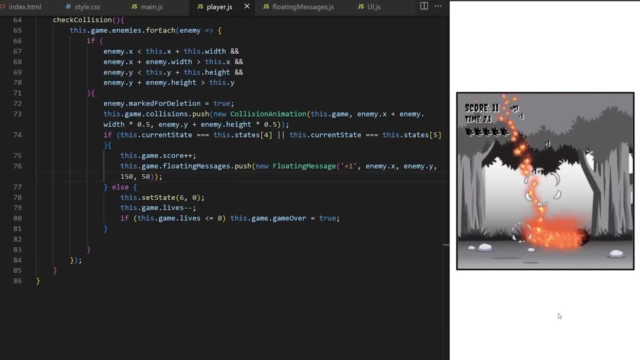 Maybe these coordinates: Yeah, let's do 150 and 50.. Right now we are creating an ever increasing floating messages array because we are not removing the old ones. I will use filter array method to do that. It's better than using splice for a reason I will explain in a minute. Built in array. filter method runs a provided callback function. I will use filter array method to do that. It's better than using splice for a reason I will explain in a minute. It's better than using splice for a reason I will explain in a minute. 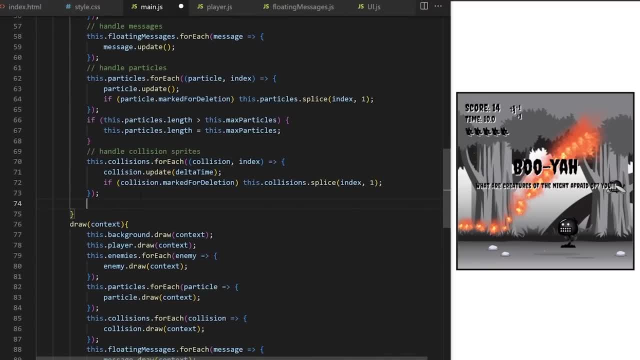 It's better than using splice for a reason I will explain in a minute Once per each element in the array Array elements which do not pass the callback function test are skipped and are not included in the new array. So when I say thisfloatingmessagesfilter and as a callback I say markedForDeletion. 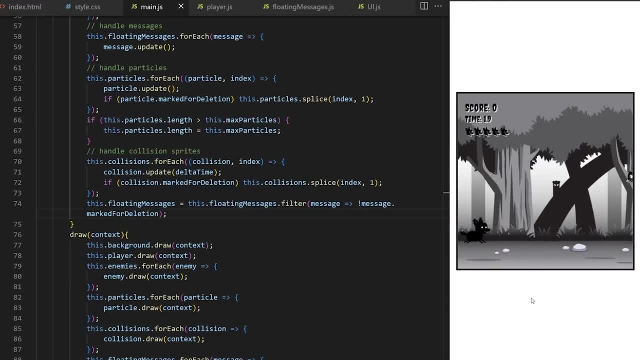 property on each object needs to be false. The new array will contain only elements that have markedForDeletion set to false. Elements that are set to true will be excluded. At the same time, I am assigning this new filtered array to the original floating messages. 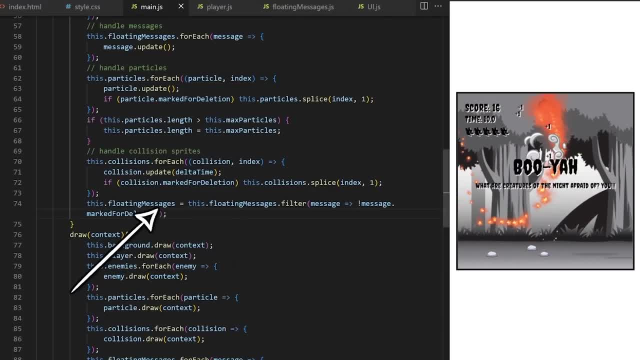 I will use filter array method and then I will say this: MarkedForDeletion property on each object needs to be false. MarkedForDeletion property on each object needs to be false messages array overriding it. So this simple line of code filters out all. 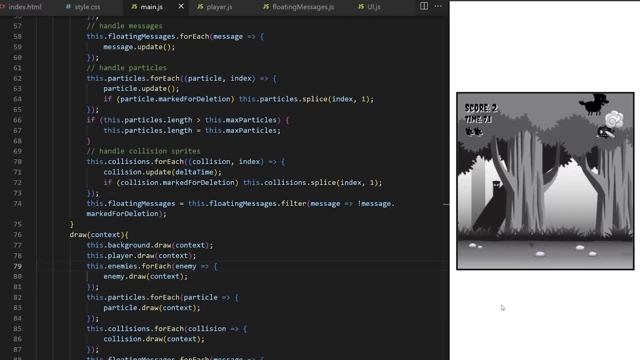 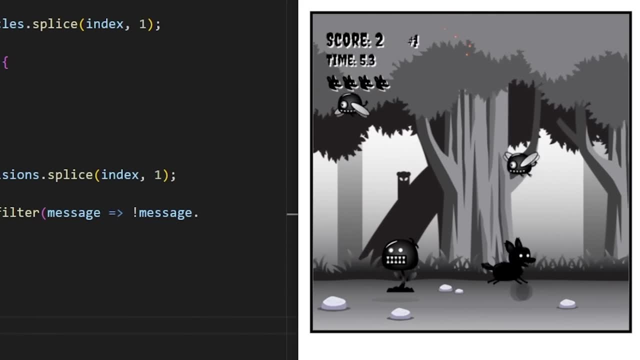 elements that have marked for deletion set to true. In the previous episode I mentioned a bug where I noticed that ground enemies jump and wiggle horizontally even when they are supposed to be static. It's especially visible when comparing ground enemies against the ground texture, but it is actually. 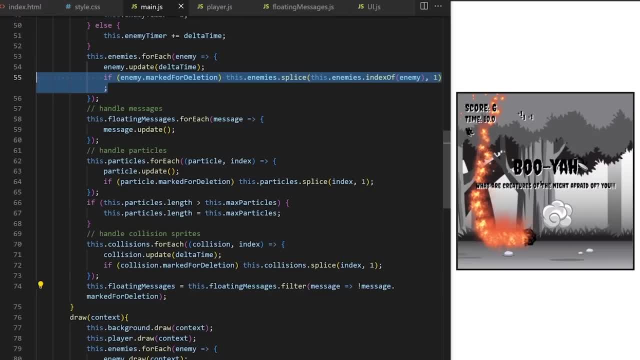 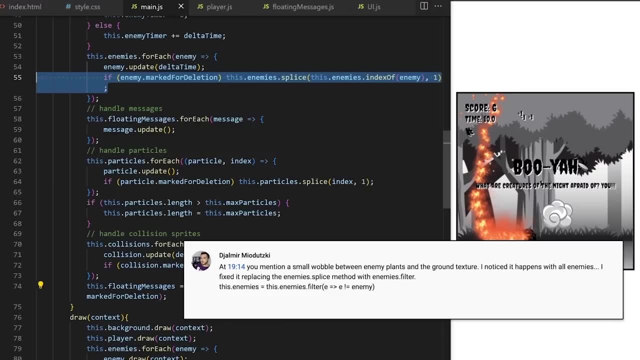 happening with all enemies. It is because as I cycle through the array, I am removing enemies that collided with player or moved off screen using splice. Problem is that when I splice out and remove enemy from the array while I'm in the middle of cycling through that array, it changes. index of all the following: 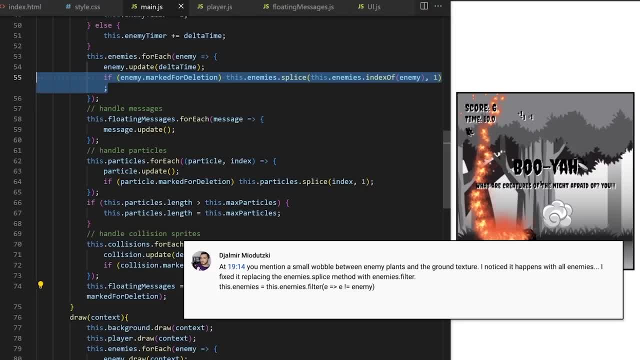 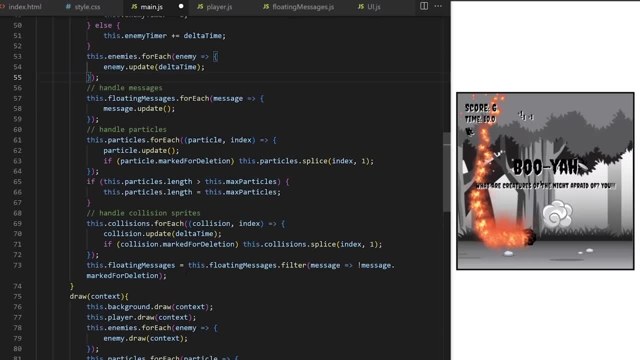 elements, in our case, enemy objects. Because of that, their position is not calculated correctly for that loop and they jump around. Instead of splice, I will use filter method and I will only remove enemies that have marked for deletion properties set to true after we finished cycling through the entire. 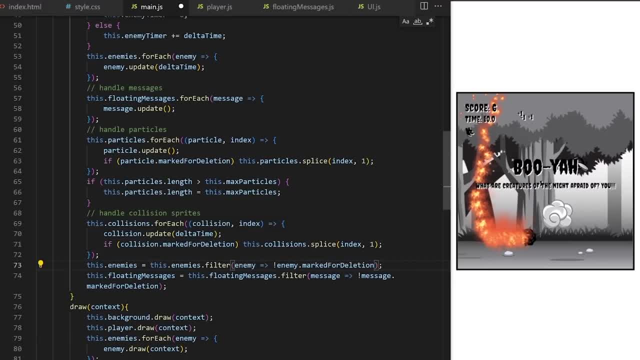 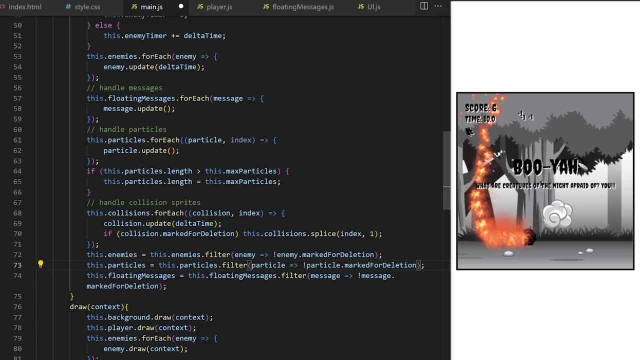 array, so there are no problems with indexes and skipping positions. Basically, I will do the same thing for enemies, I just did for floating messages. I will also do the same thing for particles like this and finally, I also do it for collision animation objects. Now that's better. We fixed the bug and I think this syntax is a bit cleaner, as 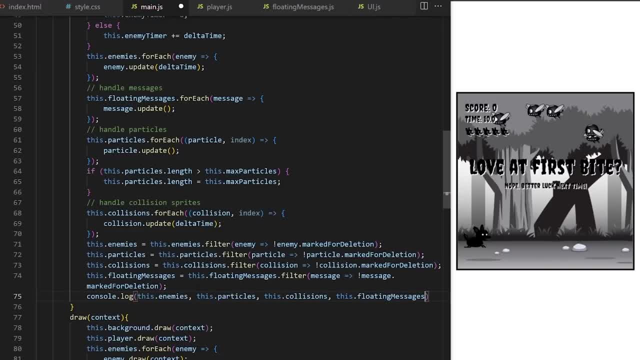 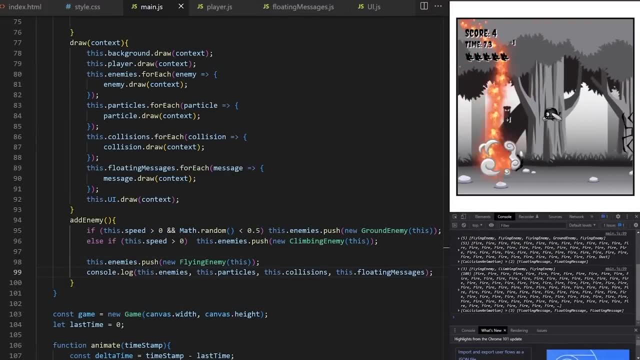 well, I just quickly console log all my object arrays. I put it inside add enemy so it logs it only periodically, Not for every animation frame. I play the game and I can see that all the arrays are being correctly filled with objects and those objects are also being removed. 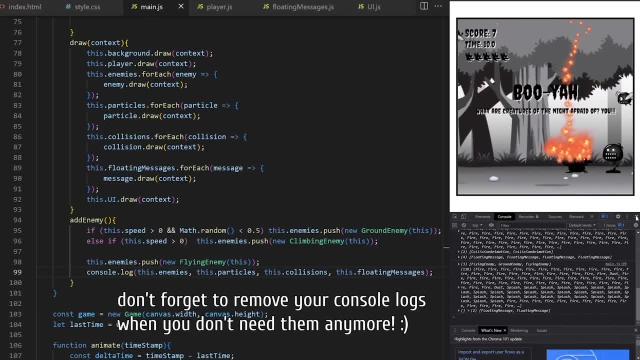 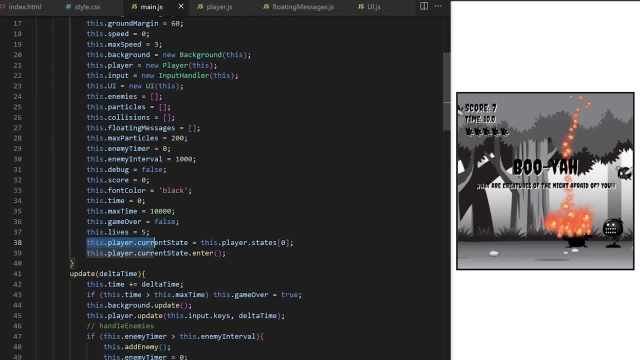 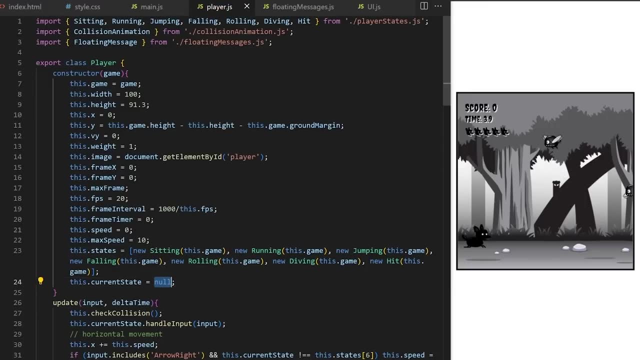 Perfect Player class doesn't have this dot rights policy because I had to define it from inside game object here. That property belongs on player class, so I can define it here and initially I set it to null. This is just to clean up. the code will still work the same. 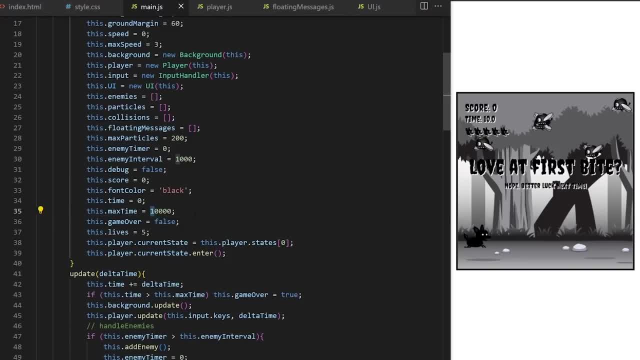 Lets tune the game difficulty to make it a bit more challenging. Max time will be set to NULL. No need to createή Not staying to. otherities will be 30,000 milliseconds or 30 seconds In this time the player needs to. 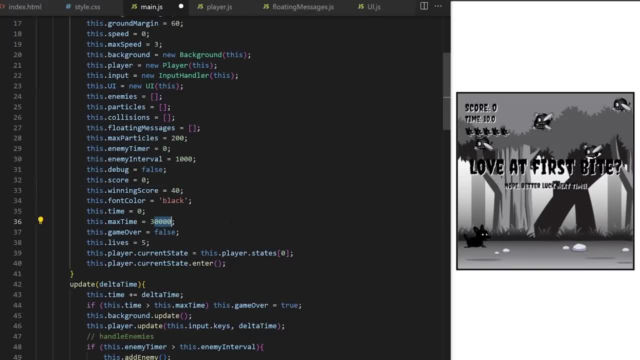 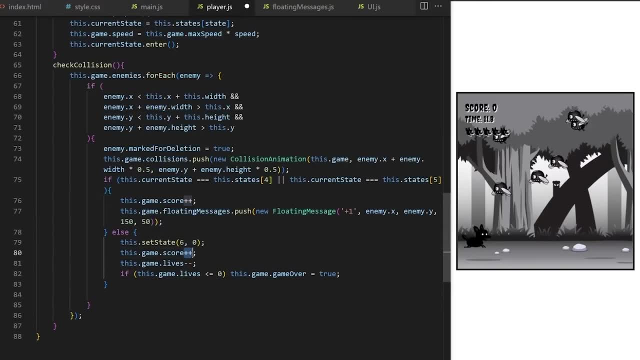 reach at least the minimum winning score of 40 to see the winning message. We can do other things. for example, every time player gets hit by an enemy and this animation is played, we can remove five points from the score as a penalty. You can tune your game however you want. You can make it easier or more difficult by 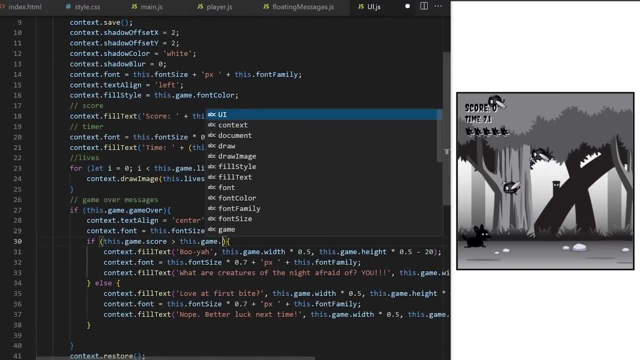 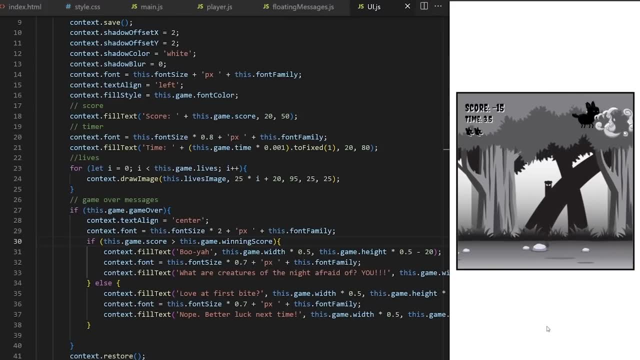 adjusting these values. When the game is over. after 30 seconds, I check if score is more than winning score and if it is, we display winning message. else we display the losing message. Let's test it. I play it and I get hit over and over My. 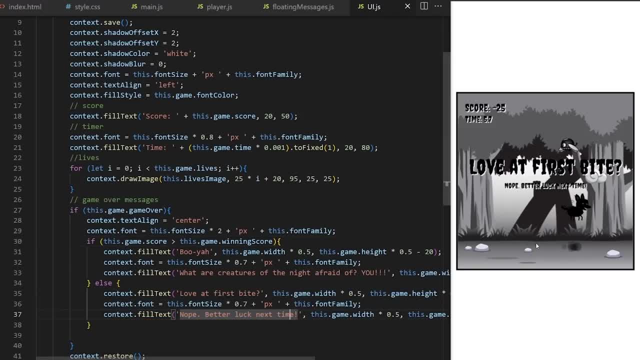 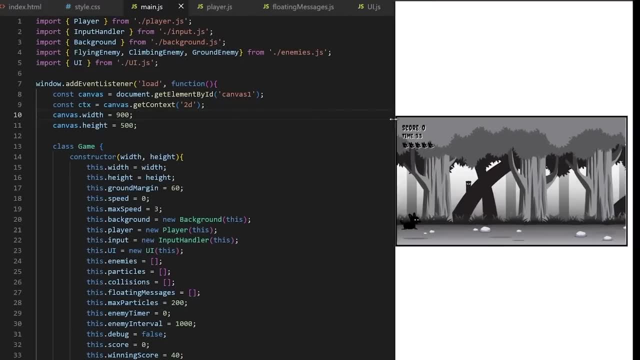 score is in minus values, I get game over and losing message from line 35 is displayed. Nice, I increase game width to 900 pixels. I will keep game height at 500 pixels because our background images are optimized for that size. We're not gonna.